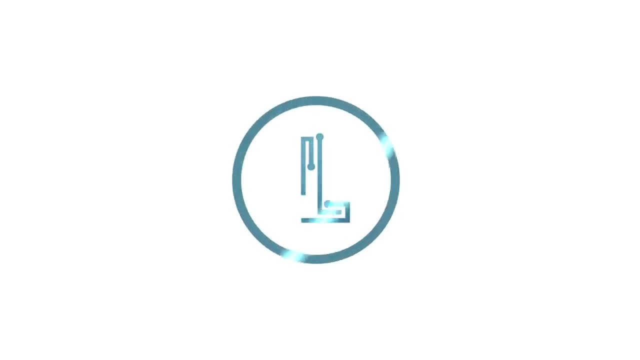 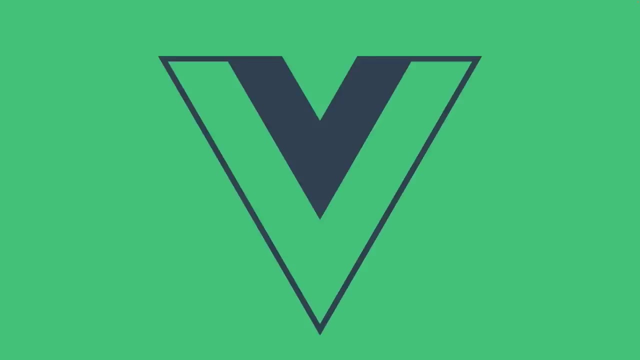 Hello YouTube, welcome back to the channel and welcome to this five hour view crash course. I'm super excited about this crash course because this is actually five hours of an 18 hour long course that I hosted on Udemy. So if you really want to take your view skills to the next level 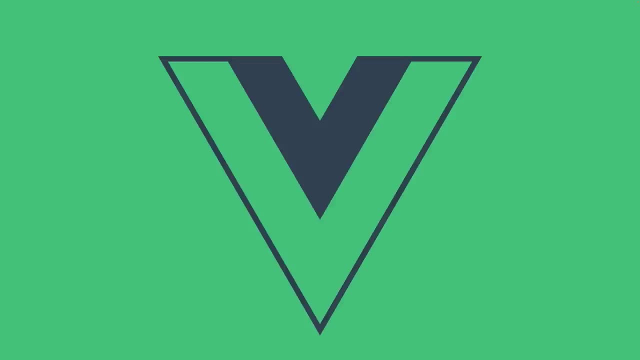 and really really be job ready, go to Udemy because we're going to learn a bunch of other things like authentication, Vue with TypeScript, as well as Global Store. So I'm going to go ahead and host a discount code in my description box below. Go ahead, it should not be more than $9.99. 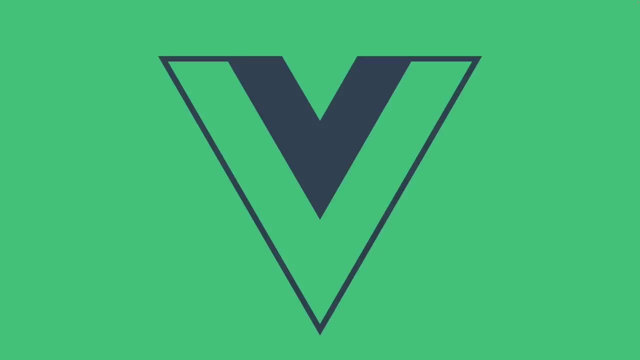 Well, enjoy the rest of the video. Welcome everybody to the most comprehensive Vue 3 Composition API course on the market. This course is going to be down packed with a bunch of different knowledge and it's going to take you from an absolute beginner with no knowledge of Vue to learning some of the more advanced Vue features 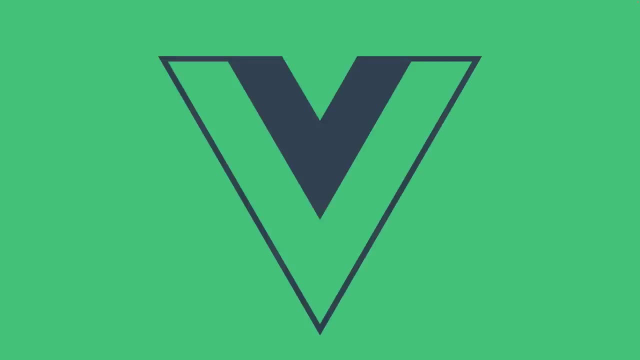 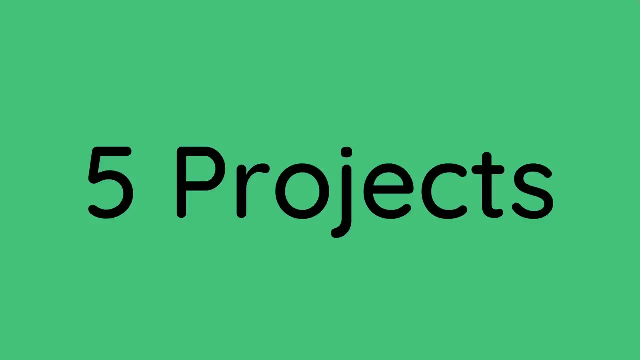 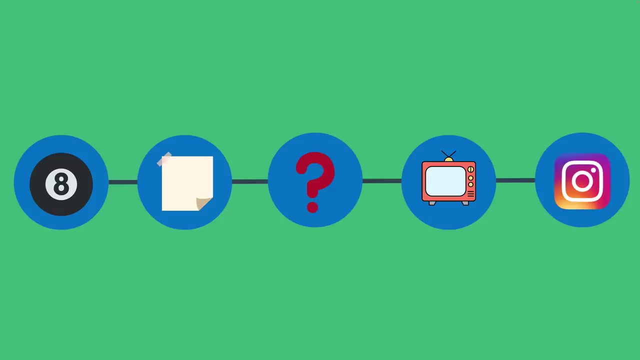 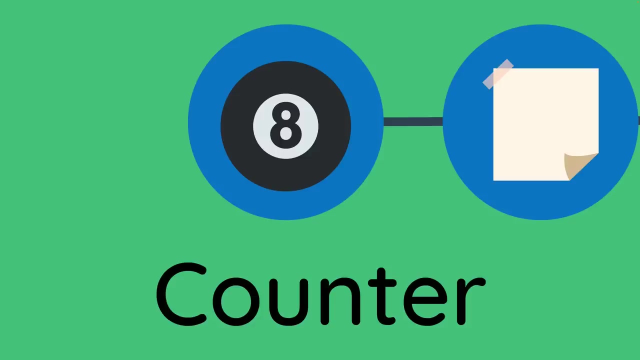 and pretty much ready for a Vue development job. In this project, we are going to be building five different projects and all of these projects are going to help us grow as Vue developers and each project is going to build on top of the previous one. So let's go ahead and quickly introduce these projects. The very first project is just going to be a very simple counter and it's going to serve to introduce Vue to us. It's going to teach us about some of the important 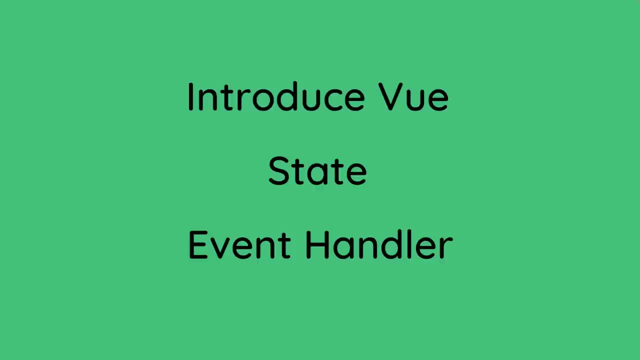 Vue concepts like state as well as event handling. Once we're done with this very simple project, 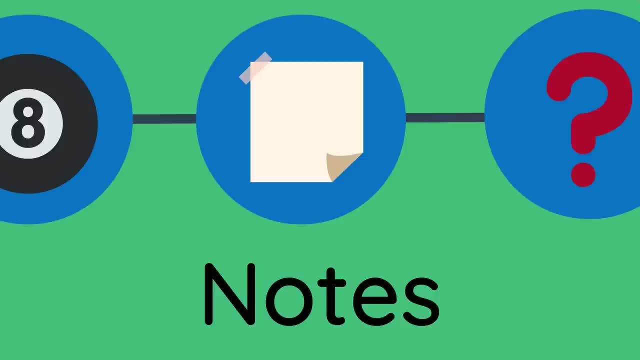 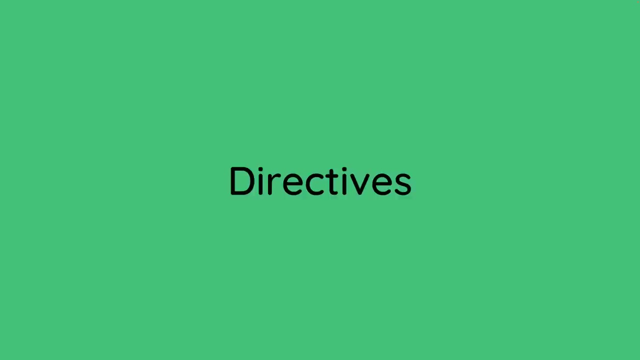 then we're going to move on to a little bit more complicated project and this is going to be a notes application where we can save and take notes. Now this main project is mainly directed so we can learn all about directives. Directives is an extremely important concept in Vue and we're going to be utilizing it throughout our application 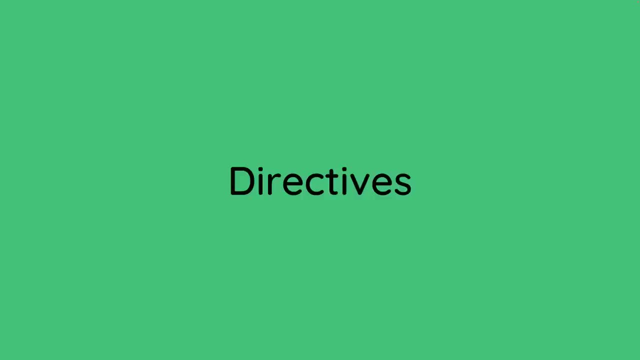 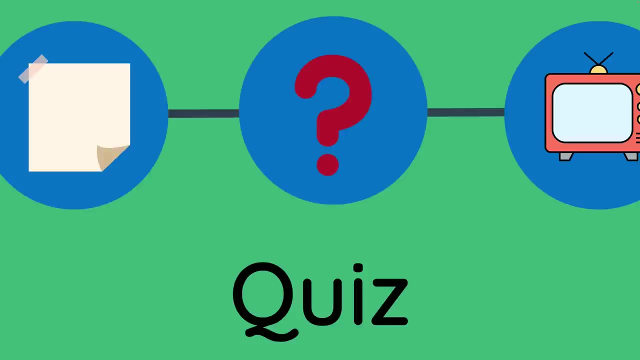 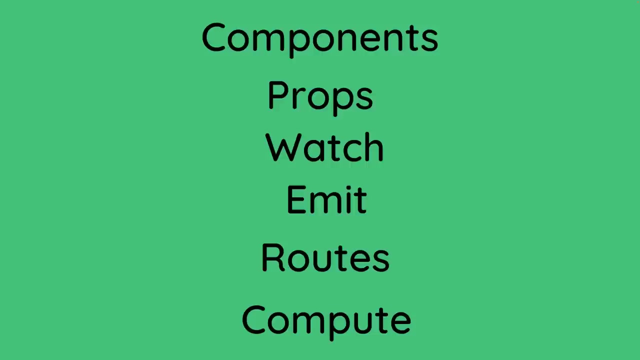 and we're going to learn a bunch of directives in this project. Then we're going to introduce a massive application which is going to be a quiz application and this is going to teach us a bunch of new concepts such as components, props, watching events, emitting events, routing for having multiple pages, as well as computing values. Now once we're comfortable with that, let's move on to the next project. So we're going to be using a lot of directives 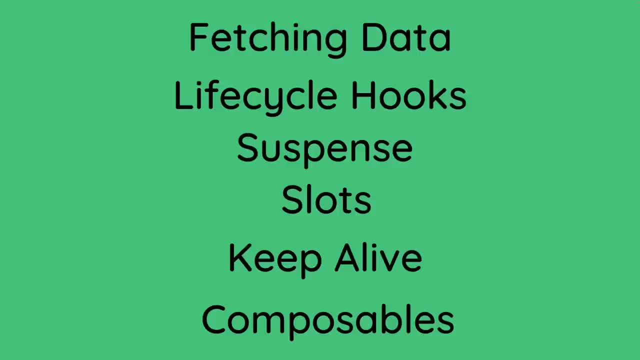 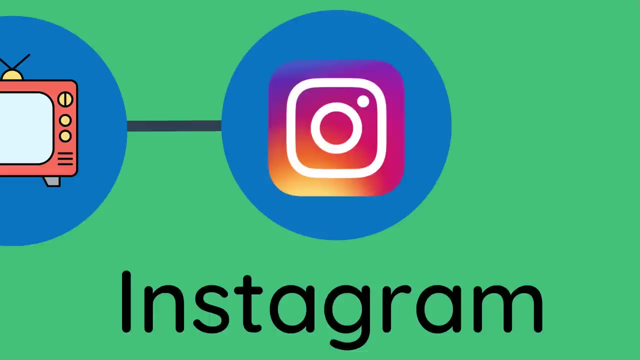 and we're going to move on to the TV shows application where we're going to learn about how we can fetch data from an external API, learn about some of the lifecycle hooks, suspense, slots, keep alive, as well as composables. And once we're done that, then we are going to move on to a humongous, huge application and it is going to be an Instagram clone. So it's going to be very similar to what we actually see when we go to Instagram.com. And over here, 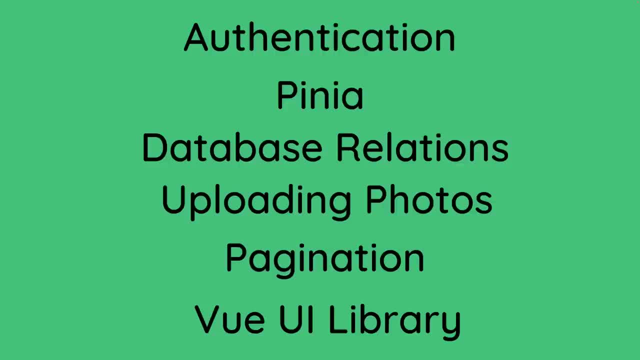 we're going to be learning some of the cutting edge features. We're going to be learning about authentication, so how we can log in, sign up. And then we're also going to learn about PINIA, meaning how we can store our state globally. We're going to learn about database relationships. We're going to spin up a Postgres database. We're also going to learn about how we can upload photos and actually upload it to the cloud and retrieve it within our app. We're also going to learn about some of these scalability features like pagination, and we're going to learn how we can implement something like role-based pagination as Instagram does. And then all of that, we're going to be building our UI with an external Vue library. So we're going to learn how we can incorporate these libraries within Vue. So I hope you guys are definitely excited for this course. I definitely am. And it was a pleasure making it. Now let's go ahead and proceed to the next video. 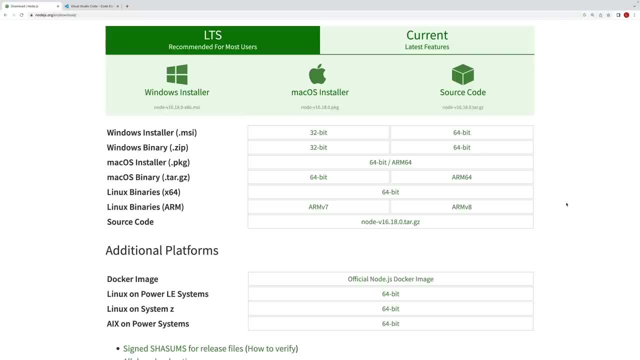 Before we get started with the course, there's just a bit of setup that we need to do. And luckily for Vue, we're going to be able to do a lot of things. So we're going to be able to do a lot of things. So we're going to be able to do a lot of things. So we're going to be able to 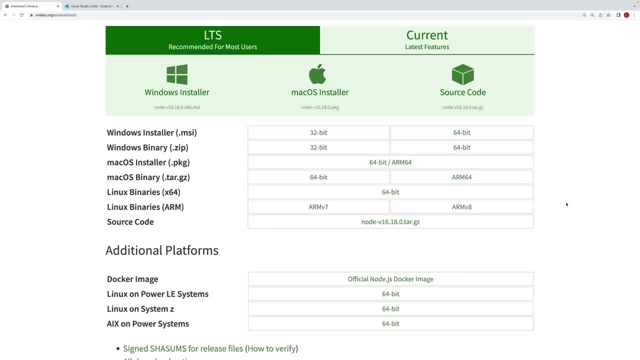 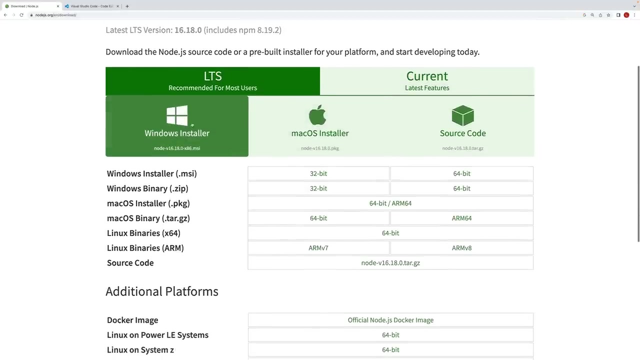 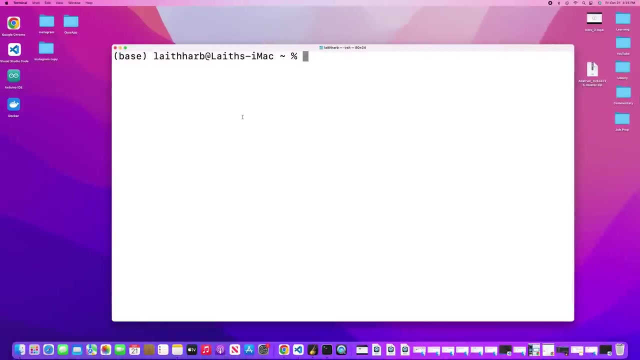 There's actually not a lot of setup and the setup is pretty easy regardless of your operating system. So the first thing that we need to do is ensure that we have Node.js installed on our machine. So if you have Node.js already installed, this is not a problem. However, if you don't have Node.js, we'll just go to nodejs.org slash download and download it for your operating system. So if you have a Windows machine, click on this. If you have a Mac, click on this. Or if you have a Linux machine, click on this right over here. Now this is a very, very simple install and I actually already have it installed on my machine. All it does is very simply just trigger a wizard, just continue, just click next, next, next, and then you should have it installed on your machine at the end of the process. Now to check that you have it installed or not, what you can do is open up your terminal or your command prompt and just do very simply node-v. This is going to get the version of Node that you have installed on your machine. So if you have Node.js installed on your machine, as you can see, for me, I have 16.17.0. If you get any version, it doesn't have to be my 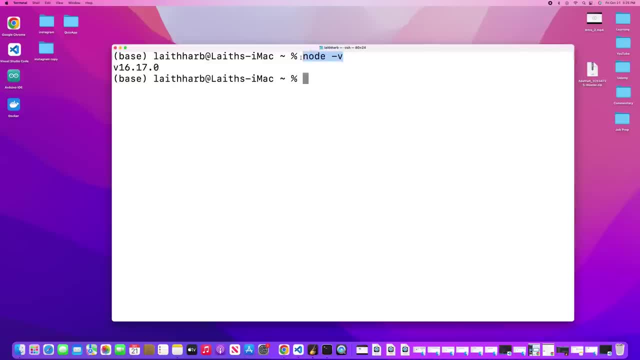 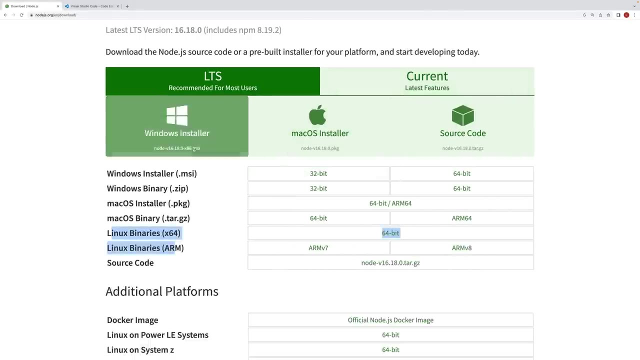 version, just any version, that means you do have it successfully installed. However, if you're getting an error saying this node command is unknown, doesn't know what this node command is, then you haven't installed it and you're going to have to go ahead and troubleshoot it yourself. And it's really, really easy. You can watch a few videos on it or you can just try to redownload it. Maybe you downloaded the wrong installer. 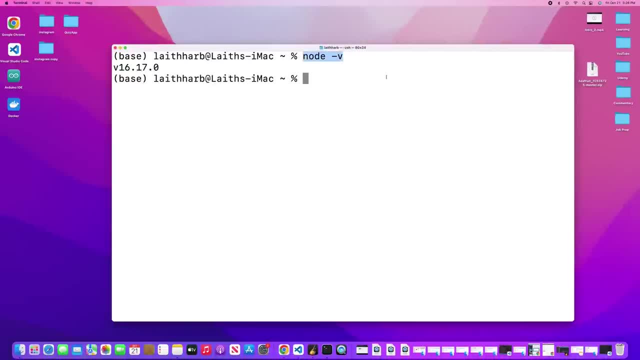 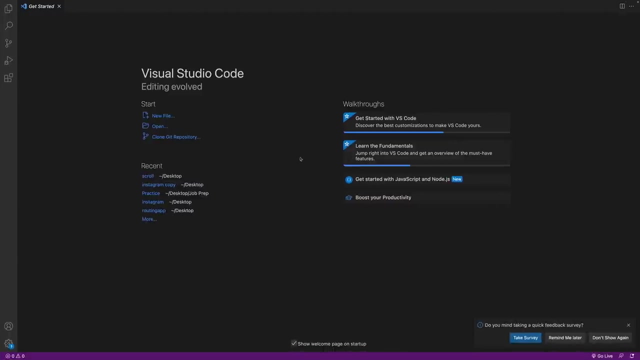 Now, once you go ahead and do node version or install node itself, it actually installs another thing called npm. And this is a node package manager. And we'll talk about this a little bit later. But to check that we also have that we can just do npm dash v. And we should also get a version. So that is the well very, this is probably the biggest step that we need to take the other steps or the other step because there's one more step is actually really, really easy. So the next 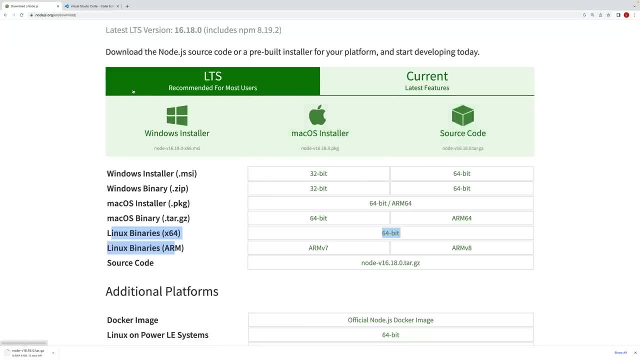 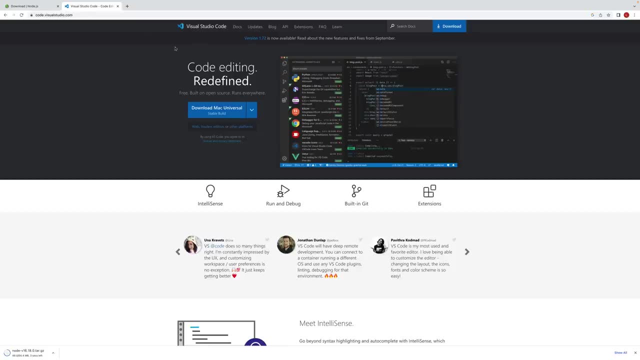 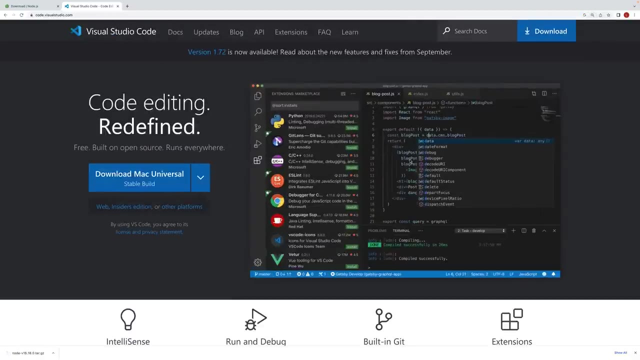 step is to download a text editor in order to go ahead and start well utilizing that text editor when coding out our view application. So throughout this course, I'm going to be utilizing VS code because it comes with a lot of amazing extensions, as you can see over here, and it's just overall the best text editor. However, if you want to use another one, if you already have one installed, like sublime, or whatever it is that you want to use utilize, go ahead and use that if you want. But just to warn you, 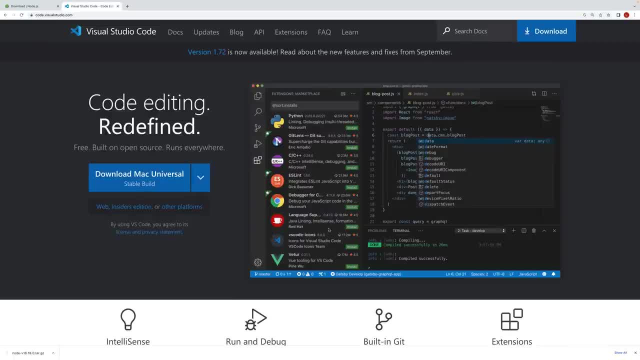 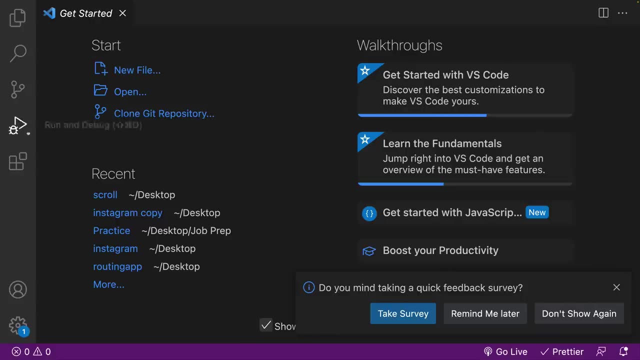 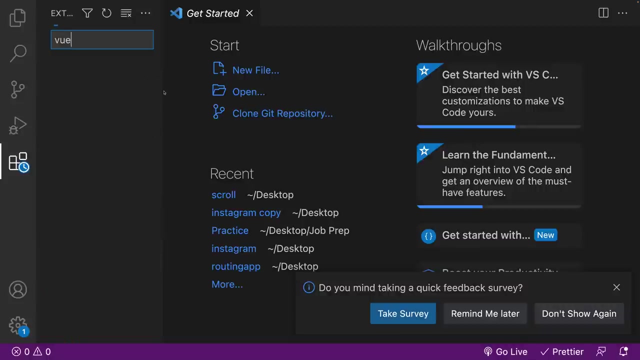 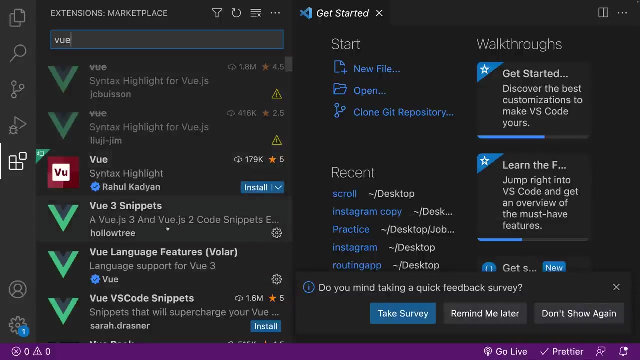 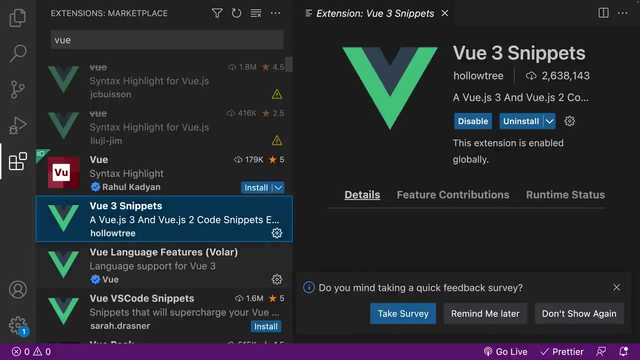 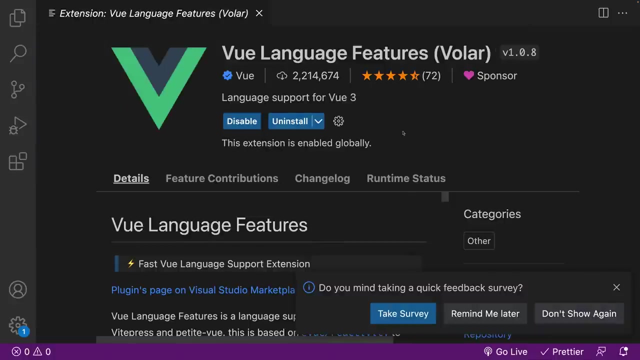 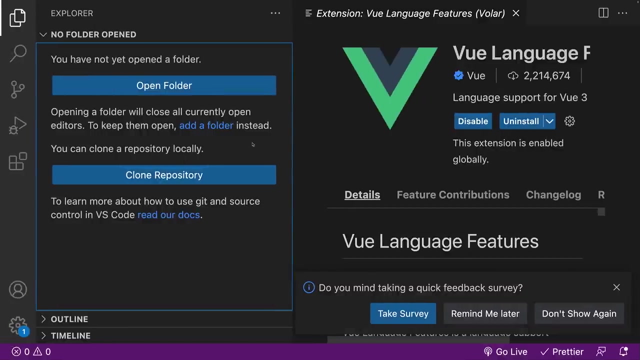 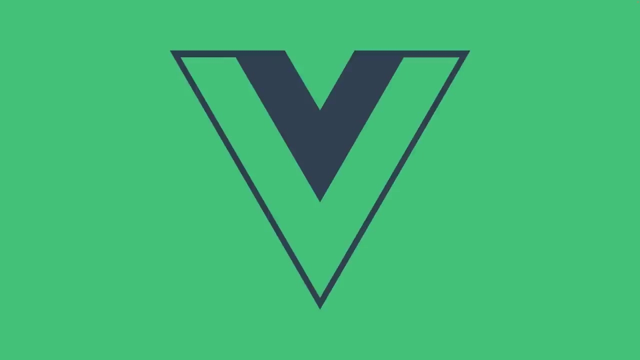 I am going to be using VS code. And we are going to be using some VS code extensions. So I highly recommend just go to code visual studio code.com, download it for your operating system. And you should get something like this. Now once you get something like this, go ahead and open it up. And I want you to go to this extensions tab over here. And then I want you to search for view. And then I want you to go over here to the view snippets. So view three snippets, as well as this view language features. And I want you to go ahead and actually install both of these extensions. So view language features is actually by view itself. And also the view three snippet by hollow tree, go ahead and install it. And what this does is it gives us a lot of nice syntax highlighting that we'll see a little bit later. But again, for now, just go ahead and install them. And that's actually pretty much all it is that we need to do to get started with view three. Now the rest of the course, we're just going to go ahead and start coding. All right, everybody, enough of the introduction, let us go ahead and move on to view three. Now typically, this is the point in the tutorial where an instructor defines exactly what view three is, and defines exactly why we would want to use it. However, I always find that these 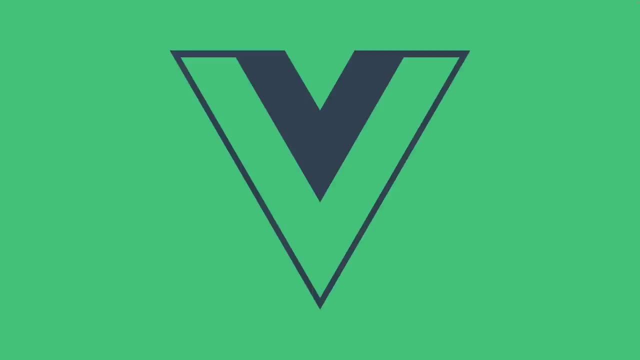 definitions, especially if I am brand new to the technology, really are not 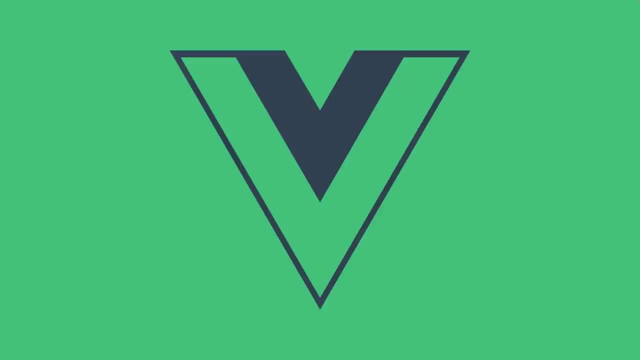 that useful and actually make things a little bit more confusing. For example, 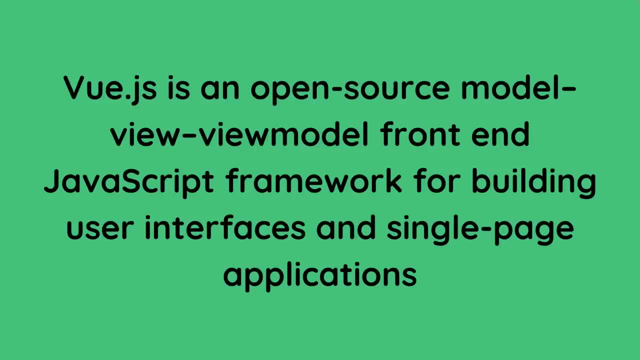 this is the definition of view that I found on Wikipedia. View is an open source model view view model front end JavaScript framework for building user interfaces and single page applications. Now, does that make any sense to you if you are a complete beginner, which I assume you guys are to view JS? Well, absolutely not. This makes no sense. What is 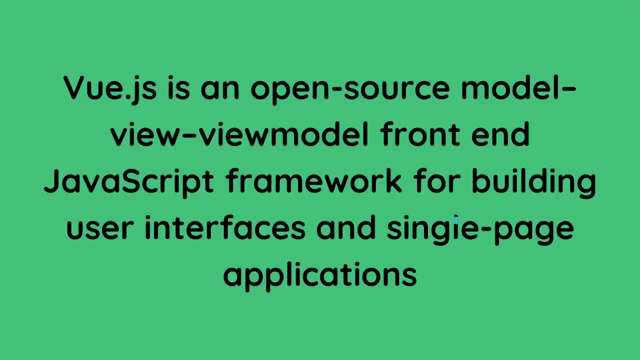 a model of if you model? What is a front end framework? What is a user interface? What is a single page application? This makes no sense. So that is not what I'm going to do, I'm not going to define what view is. Instead, I am going 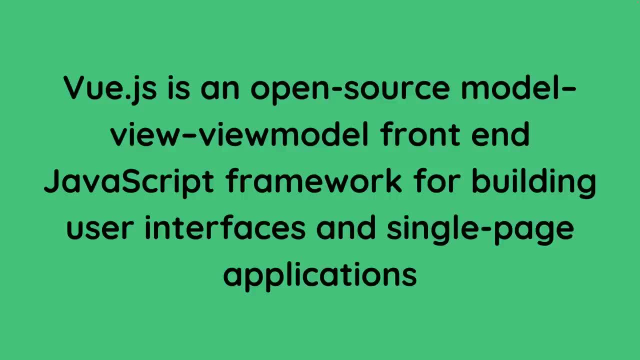 exactly why you would want to use it and the powers of Vue.js. 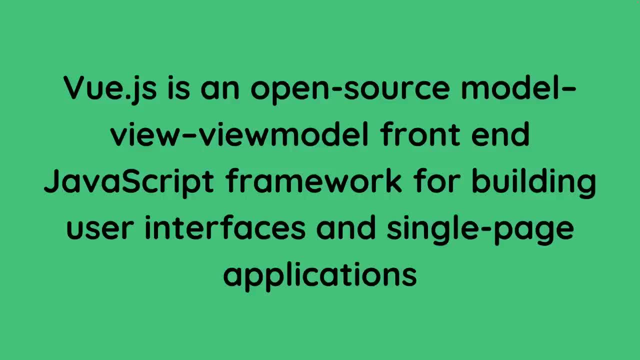 Now, how am I going to show you what Vue is? Well, I'm going to show you what Vue is by building a very simple web application. Super, super simple. You cannot get a simpler application than this. 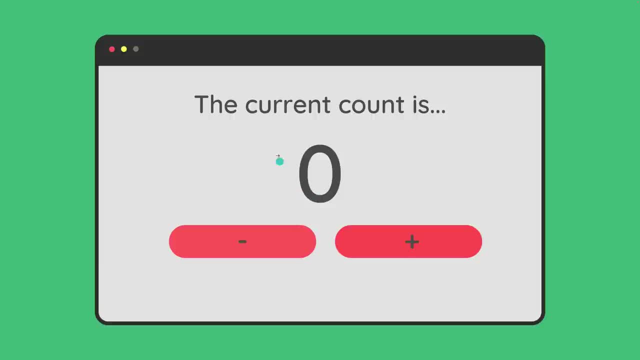 And it is, as you can see from the screen, a counter application. So we have this title here saying the current count is, and then over here, initially, it starts off as zero. 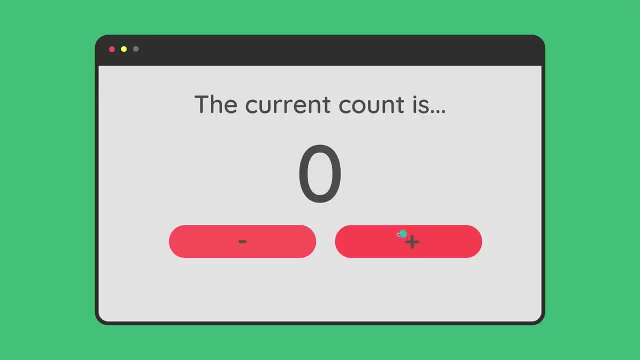 And of course, the user can change the count by either clicking on the plus button or the minus button. 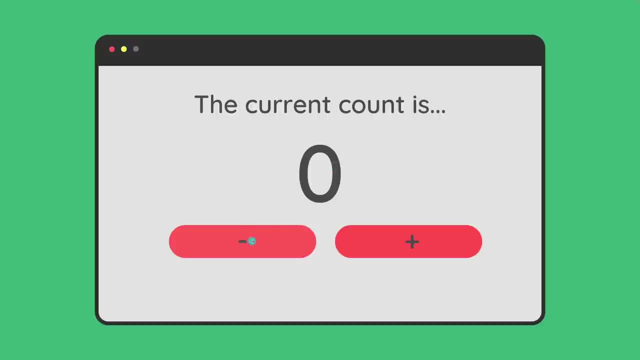 If they click on the plus button, we add one to the count. If they click on the minus button, we subtract one from the count. 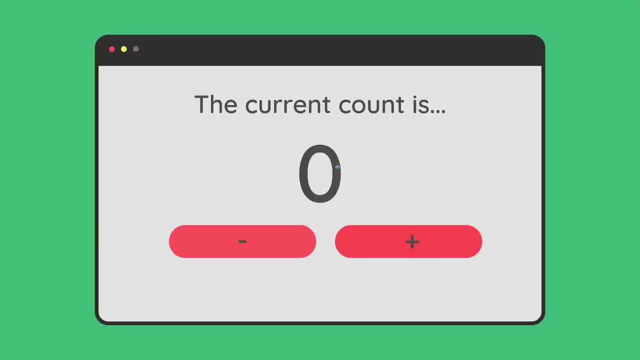 Now, how is this going to show us what Vue.js is? Well, here's the thing. 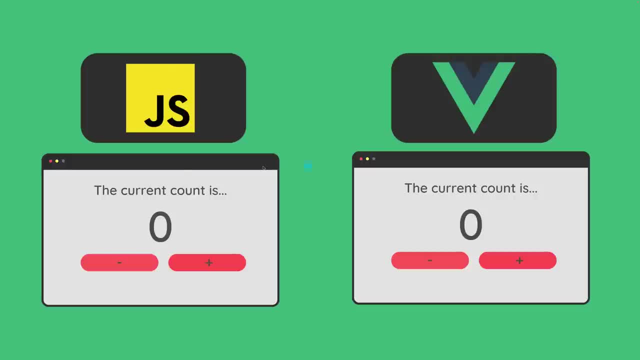 We're going to build this application twice. We're going to build it first with vanilla JavaScript. So this is just pure JavaScript. And then we are going to build it with, and we're going to see the differences between the two. 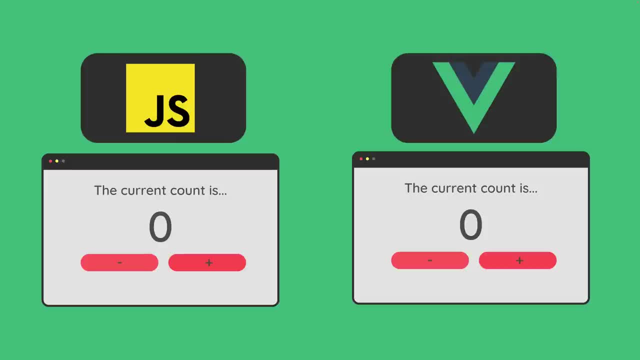 And trust me, you're going to understand after we build it, what the difference is with Vue and why we would prefer to use Vue with larger scale applications than pure vanilla JS. So you know what? Enough of that. Let us just get into it. 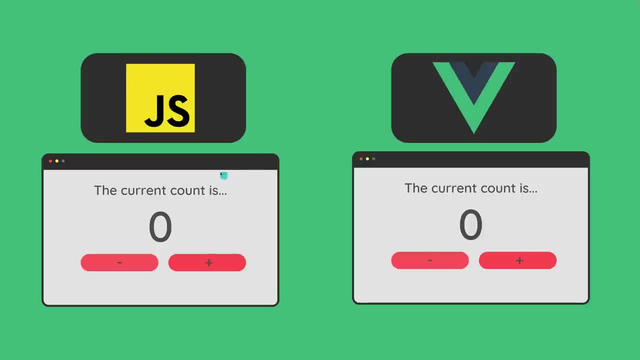 All right, my good friends in this video, what we're going to do is build the counter application, but in a pure vanilla JS. So what we're going to do is we're going to go to our desktop 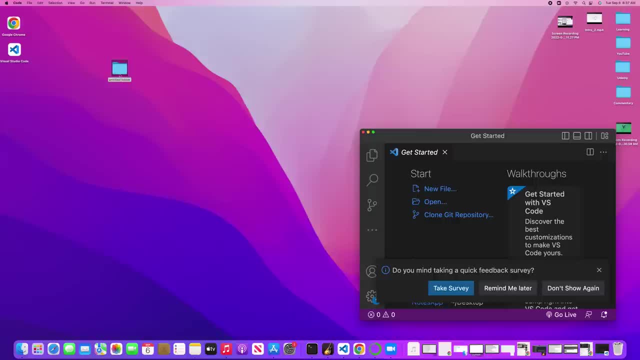 and then I'm going to right click and create a brand new folder. 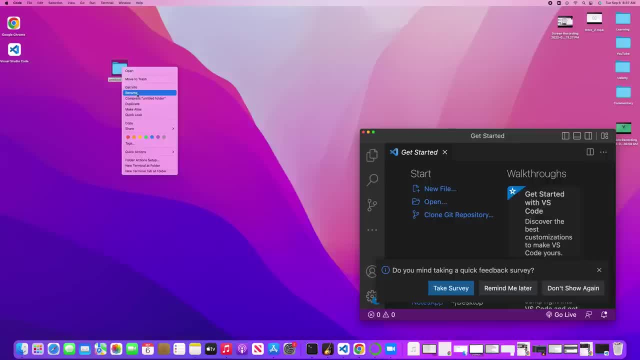 Of course, this folder doesn't have to live in your desktop. I'm just creating it in my desktop. You can create it wherever it is that you want to create it. 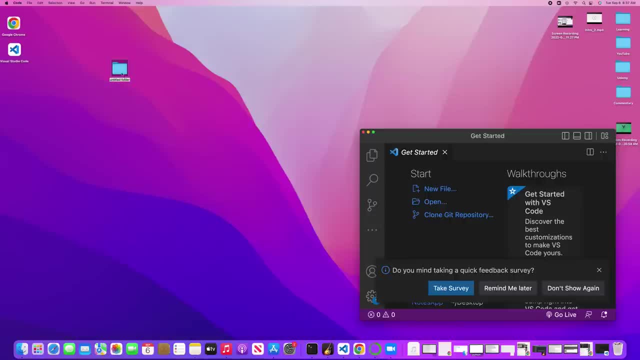 And I'm going to rename it JS counter app. So let's go over here. I'm going to say JS. 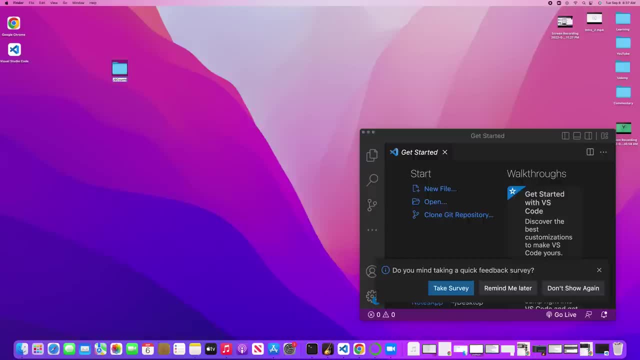 Let's go counter app like so. 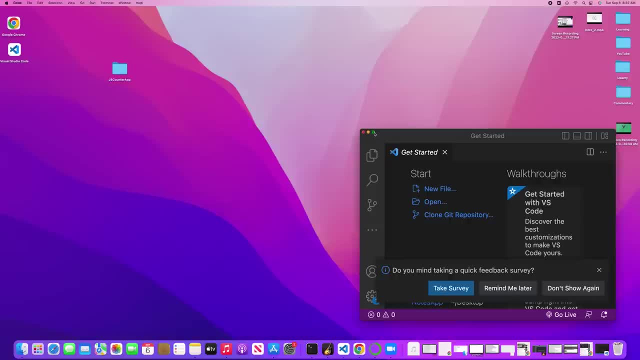 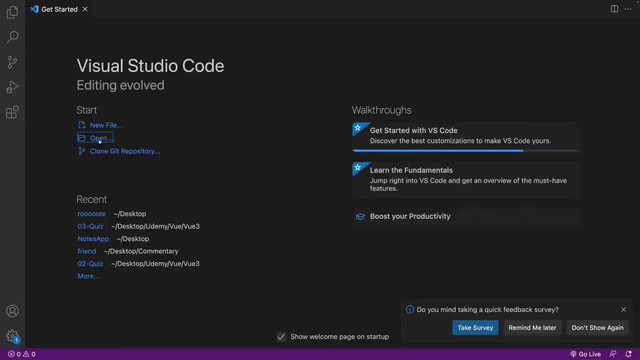 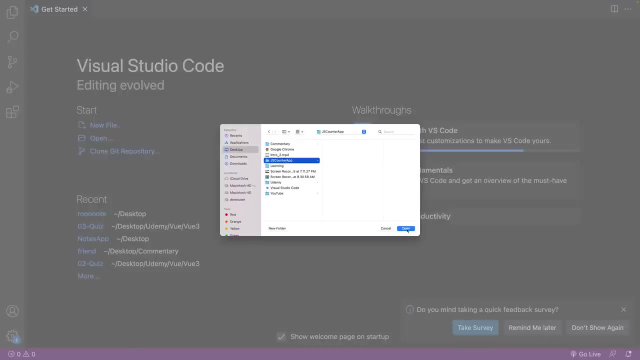 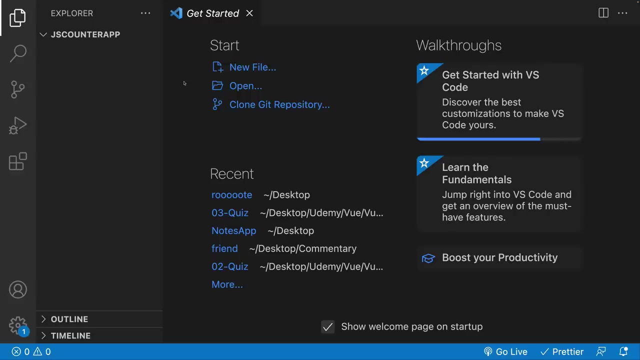 And now what I am going to do is open up VS code. So if you open up a fresh instance of VS code, it should look something like this. I'm going to click on open over here, and then I'm going to find that brand new folder that I created in my desktop directory. So I'm going to go ahead and open that and I should see VS code like this. I'm going to zoom in just so you guys can see a little bit. Let's zoom in. I think zoom out a little bit. That is good. 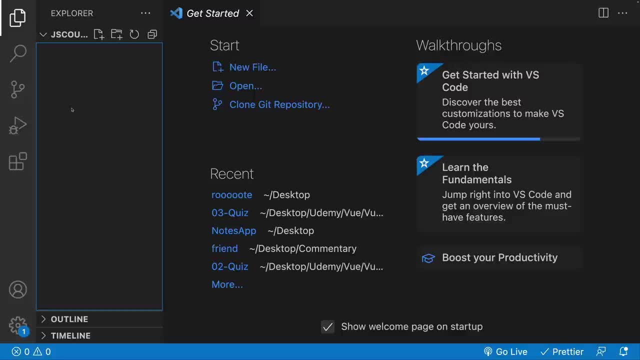 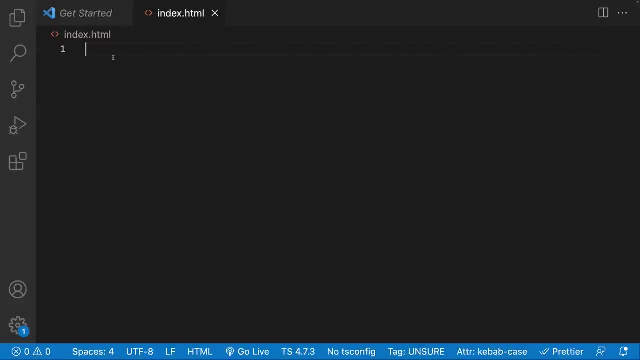 So let's go ahead and open that. So this is where we are going to create our application. So, of course, our web application is going to need some HTML. So let's first go ahead and create an index dot HTML file. Now, if you are using a VS code, you can actually use a little trick called Emmet. And this is going to create a bunch of boilerplate for us. So instead of us having to create the HTML boilerplate, what we can do is say Shift 1. 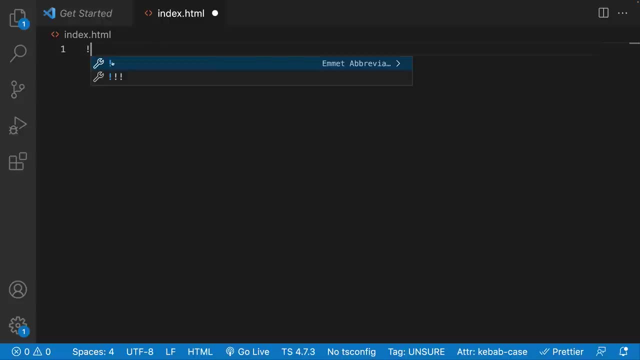 Shift 1 to get the exclamation point, and then we say Tab, and there we go. Now we have some boilerplate HTML, and it's just a little bit faster instead of us having to write everything out. 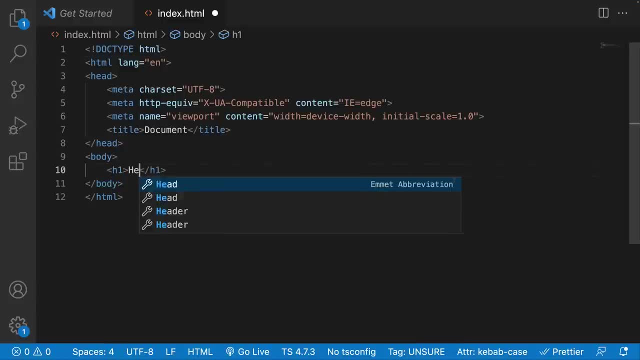 Inside of the body, I'm just going to create a quick H1, just saying hello world, just so I can see this up and running. So now what I want to do is, of course, I want to, well, serve this application onto my browser. So how are we going to do that? 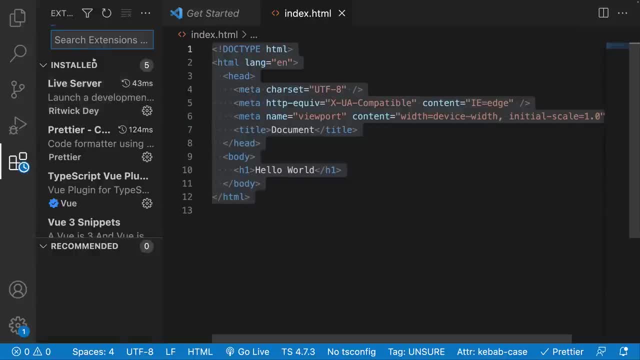 Well, we're going to do that with an extension called Live Server. So go to your extensions right over here. Let me just zoom in once more. 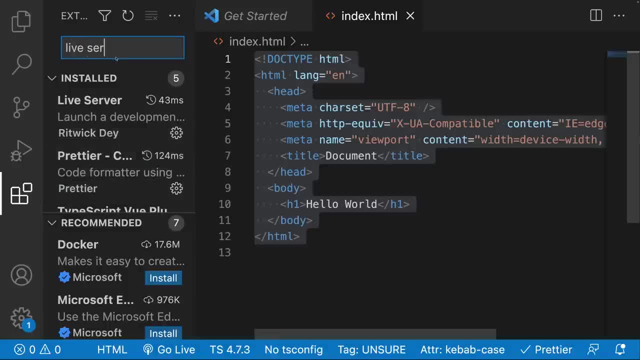 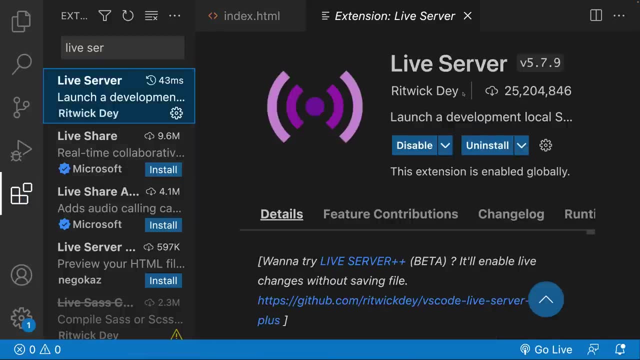 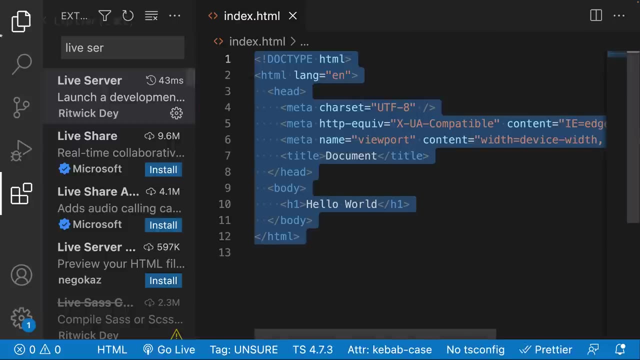 Go to your extensions right over here and then go to Live Server and then install this extension. As you can see, I already have it installed. It's by this person over here. And it has, well, at the moment of recording, 25 million downloads. Now, what you can do is once you install this, you can actually go to your HTML. 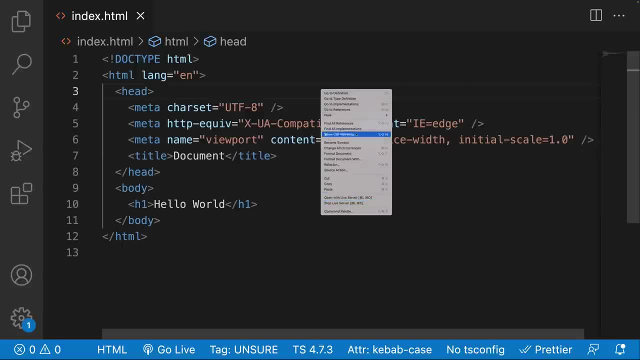 You can right click on it, and then you can see an option where you can open with Live Server. 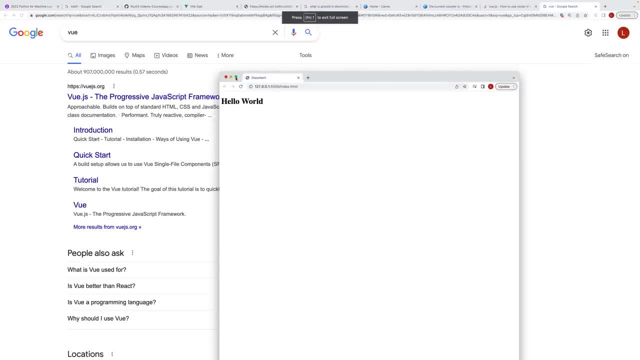 Now I'm going to go ahead and do that, and I'm going to go over here like so. 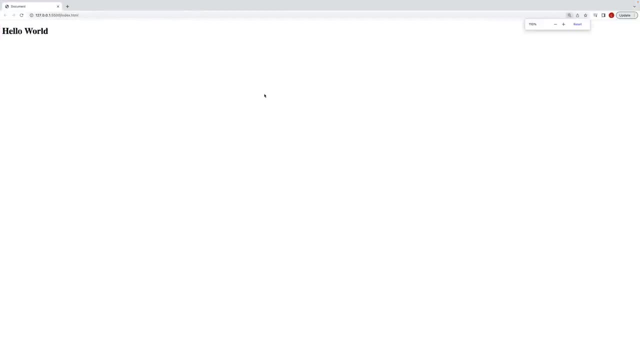 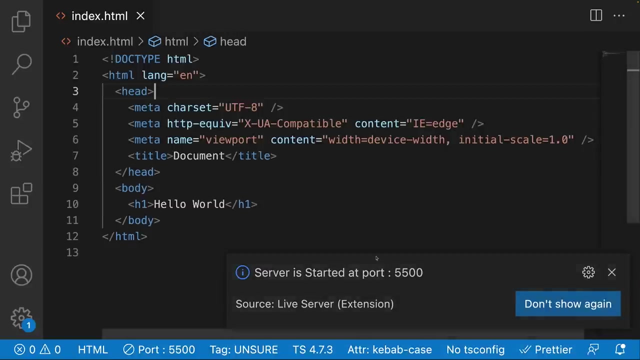 And as you can see, my application is now up and running on localhost 5500. For you, it could be different, but I think most of the time it is going to be 5500. So this is how we are going to, well, view our counter application. 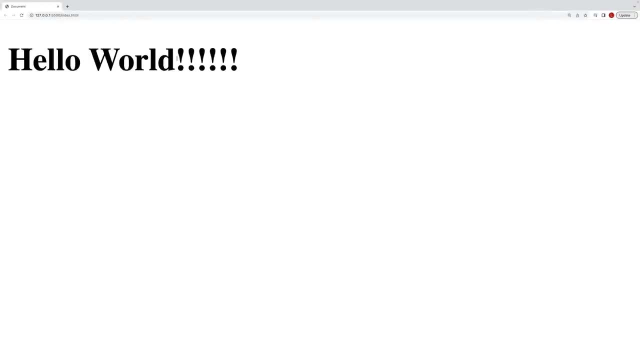 Now, if I were to add some exclamation points, Live Server is actually smart enough to detect them. 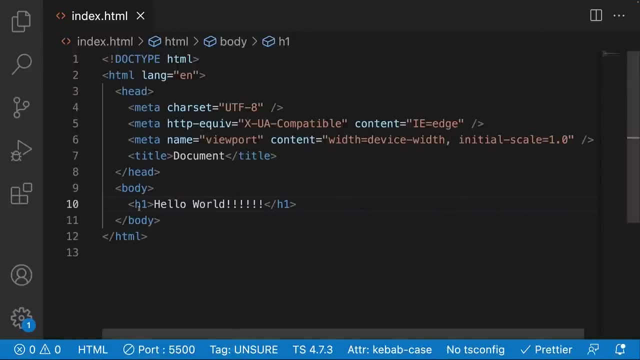 Let's actually go ahead and build out the HTML template for our counter application, which, of course, is going to be really simple. So inside of the body, let's add a div. And then inside of this div, what I'm going to do is add an h4. And then this is going to be the current. 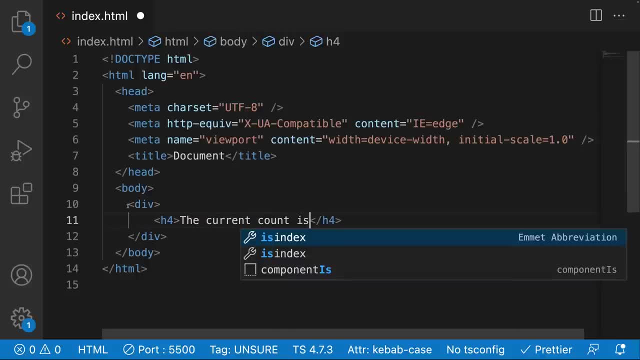 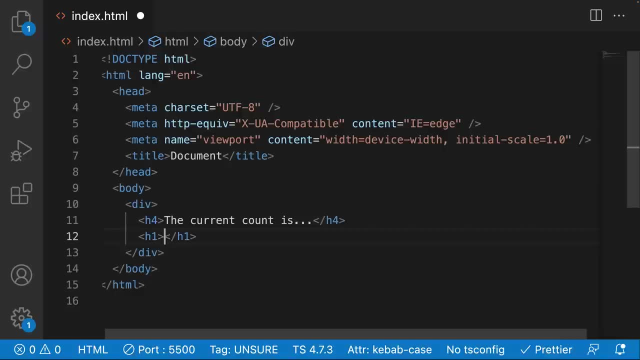 Count is, and then dot, dot, dot. That's how it's going to show, like so. And then over here, we're going to add an h1. And then inside of the h1, we're going to have the current count. Initially, we'll start it off at zero, of course. And then over here, we're going to have two buttons. So we're going to have a button. One is going to be the minus button. And then we're going to have another button, which is going to be the plus button. 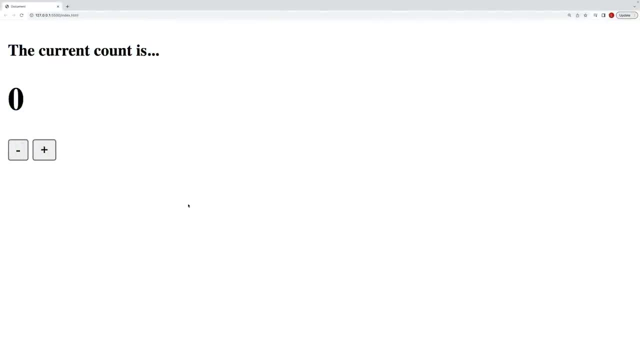 And there we go. We have our wonderful application. How beautiful is that? Well, actually, it is not very beautiful. So let's actually work on just styling it a little bit in the next video. 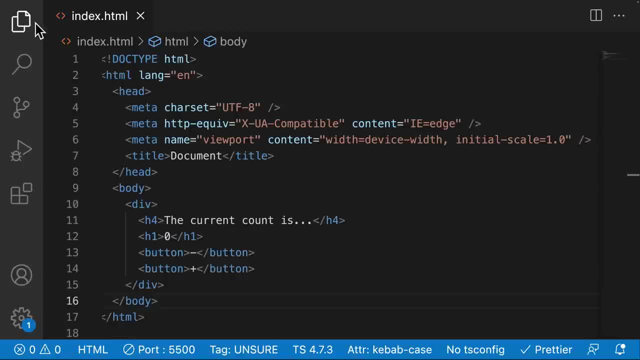 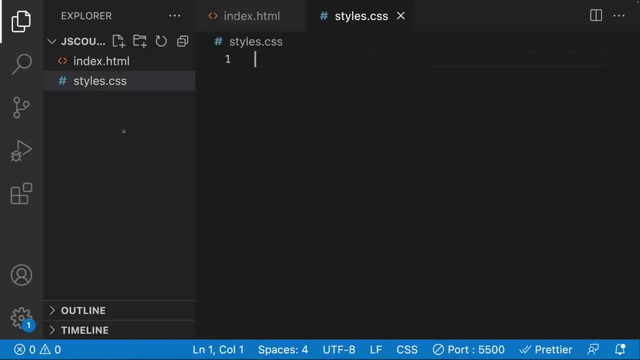 Let us now go ahead and style our application. So to do this, we're going to create a new file. I'm going to call this styles.css. Now, we're not going to do much styling. 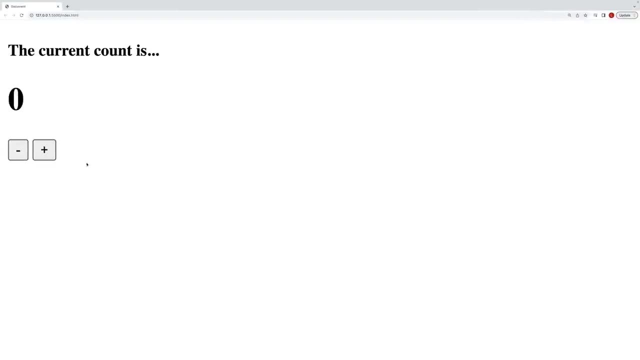 We're not going to make this the prettiest application just because I don't want to focus all too much time on it. 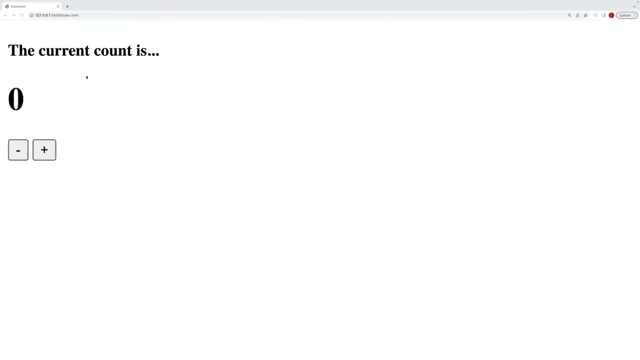 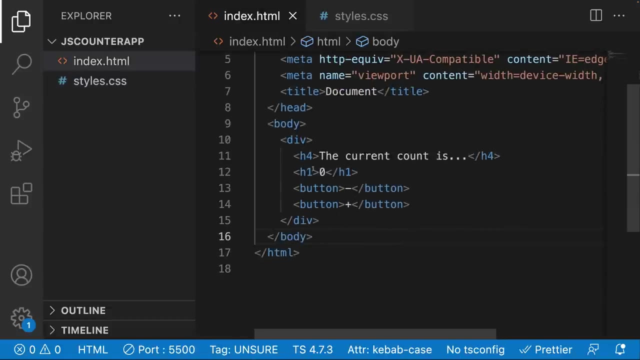 So we're just going to go ahead and just make it look better than this over here. So let's go to our style sheet. And we're really only going to style two elements. We're going to style the div. And then we're actually going to style another element. We'll call this just the main element that is going to encapsulate the div. So we're going to have a main element. We're going to have a div. And we're just going to style these two. The rest of these, we're not going to style. Who cares? Whatever. 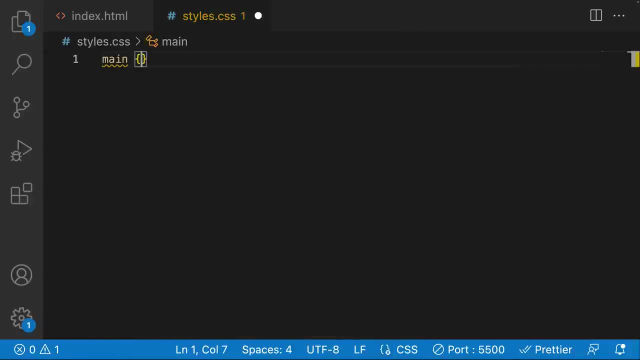 So let's go over here. We're going to style the main HTML element. 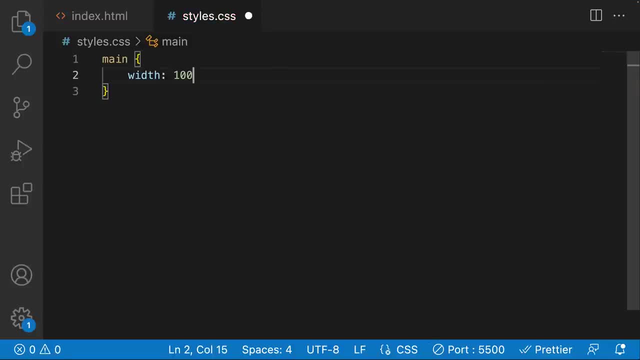 We're going to give this a width of 100vw, which is going to be 100% of the width of your machine. So whatever machine that you're on, it's going to be 100% of that. 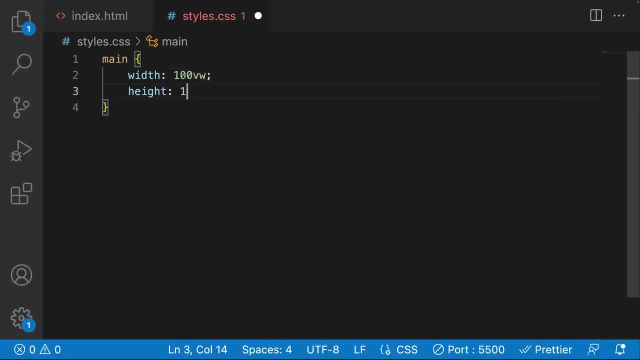 And then, of course, we're going to do the same thing for the height. This time is going to be 100vh, 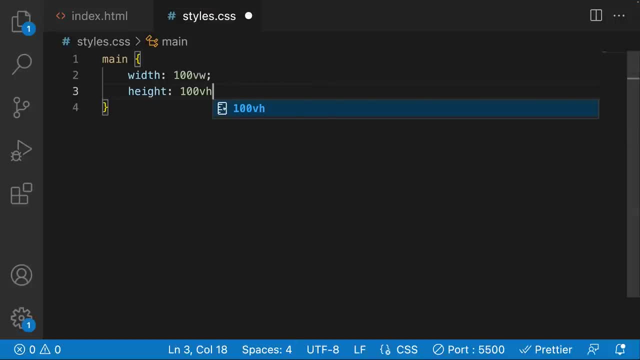 which is going to be the 100% of the height of your machine. All right. 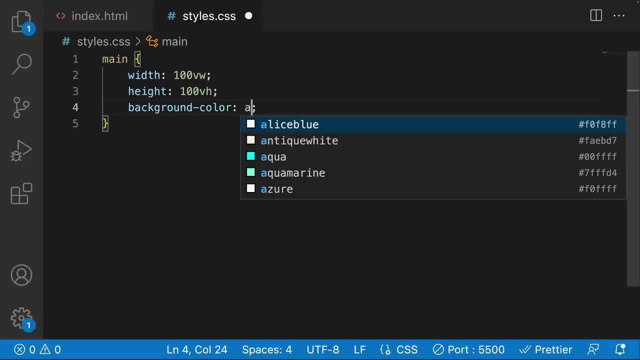 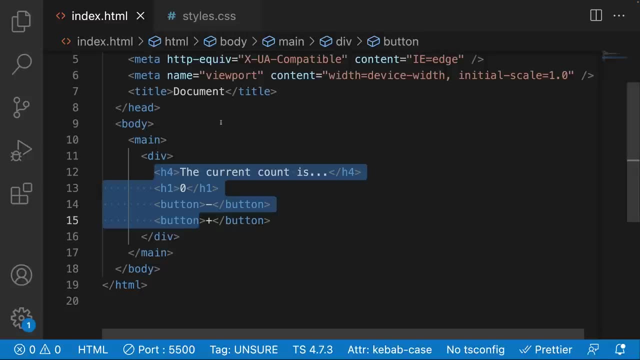 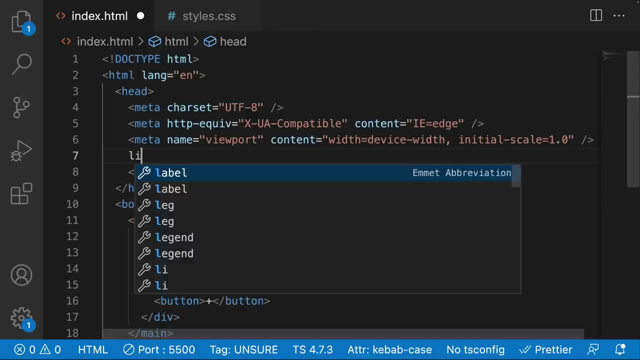 And now we're also going to give this a nice background color of Alice blue. So now if I were to refresh this, of course, this doesn't work because what we now need to do is go to our HTML and actually link it with the styles. So over here inside of the head, what we're going to do is we're going to add a link tag. 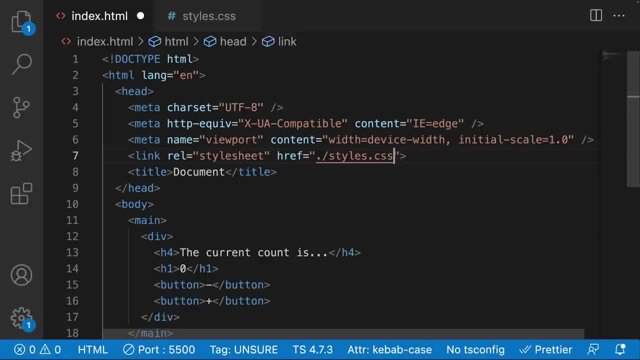 And then we're going to, well, define exactly where the styles are. And now if I were to go here, 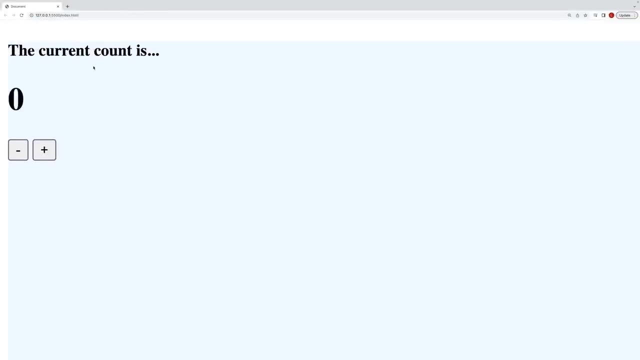 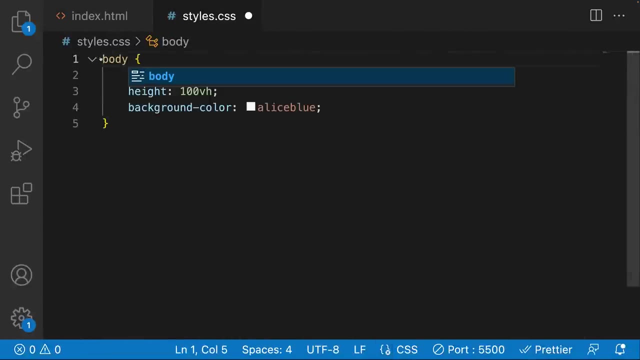 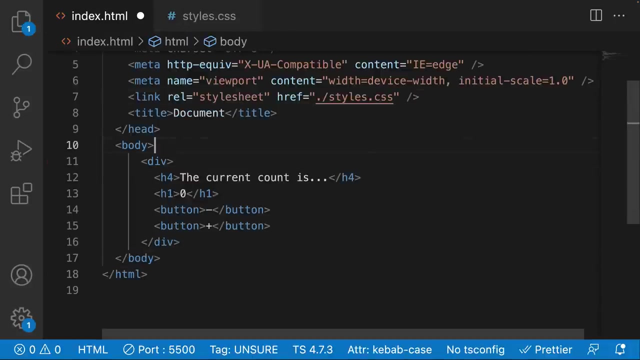 you can see right away we have our wonderful styles. And actually, instead of adding these styles to the main tag, let's just add them to the body itself because the main tag has some default styles that I do not want to override at this point. Let's just add them to the body. So get rid of the main tag. Just add them to the body themselves. Okay, there we go. 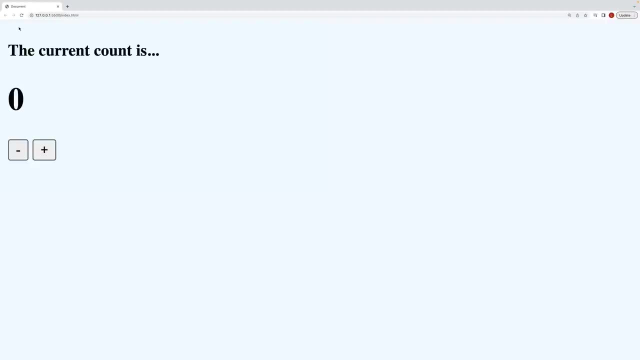 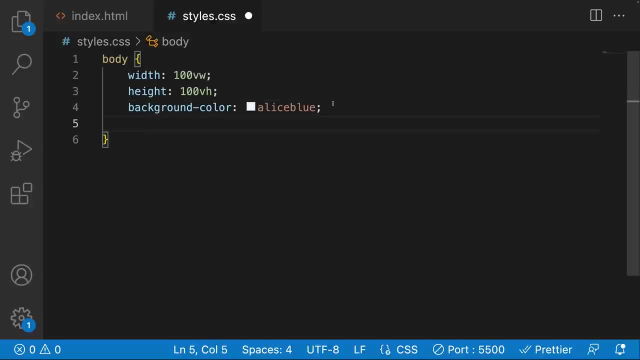 So you can see that we have some nice styles. I think it would be nice to center this div right in the middle. Now to do this, what we can do is we can do a display flex. And then we can do an align items center and then justify content center. Now if you're not familiar with flex, maybe you can go ahead and research it. 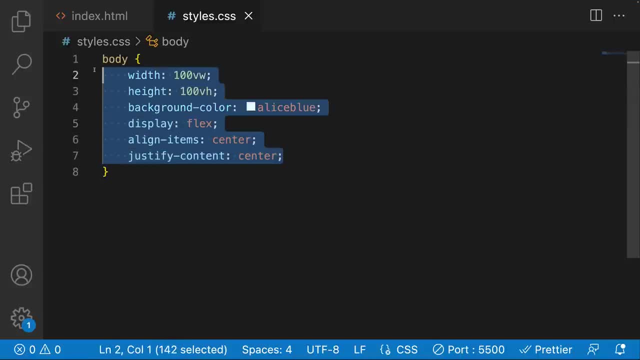 I kind of do expect you to know the basics of these styles if you're taking this view course. 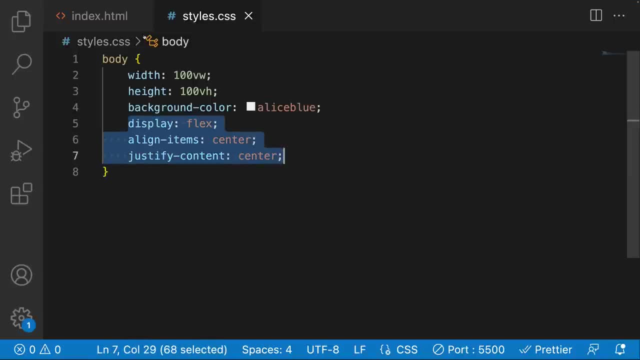 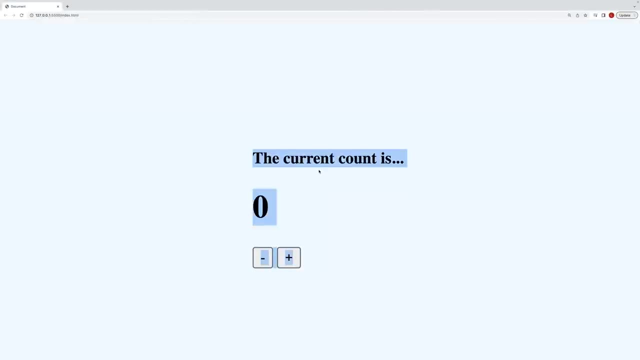 But essentially what these three lines do is just center any of the children elements right in the middle. So as you can see here, it's centered right in the middle. Now even though the div itself is centered in the middle, the text within the div isn't centered. 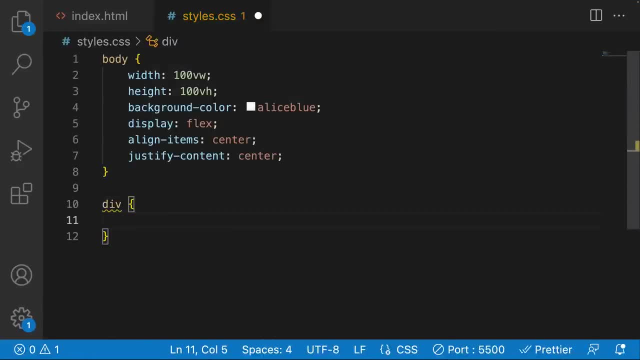 So what we can do to fix this is very simply just go ahead and do a text align center on the div. 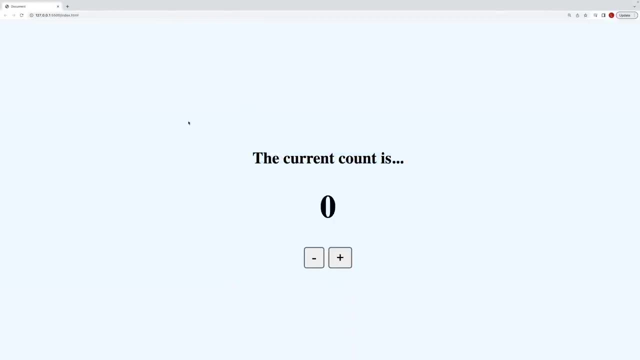 And there we go. That is our complete application. I know it doesn't look all too great, but it looks better than what it used to. So you know what? Give me some props here. 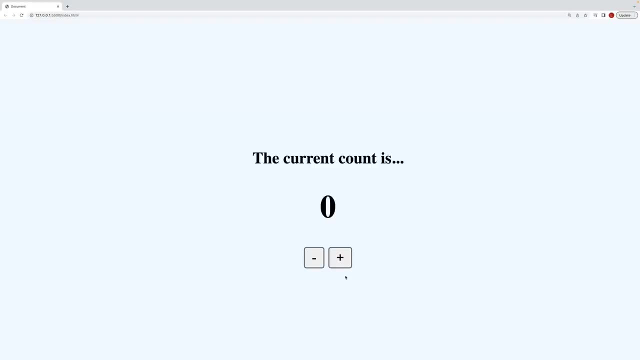 So now that we are done with the styling, let us make our application functional. So when I click on this button, this should change, add one. 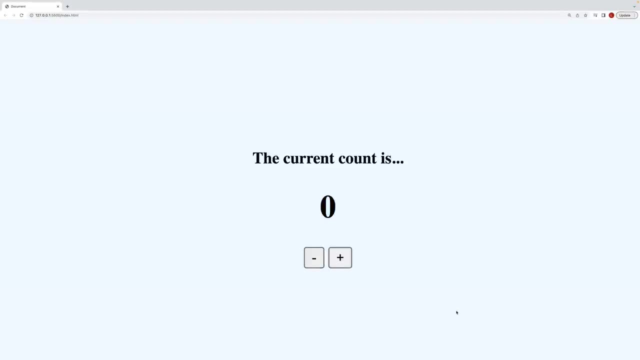 When I click on this button, this should, well, subtract one. So let's do that in the next video. 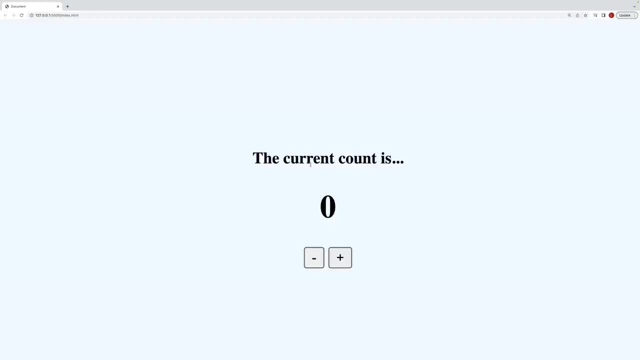 Now go ahead and implement the logic that is needed to make this application functional. Now what is functional? 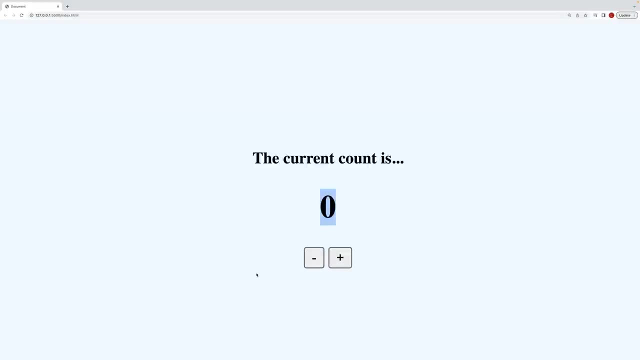 Of course, when I click this button, it is going to add one. When I click this button, it is going to minus one and it is going to count. 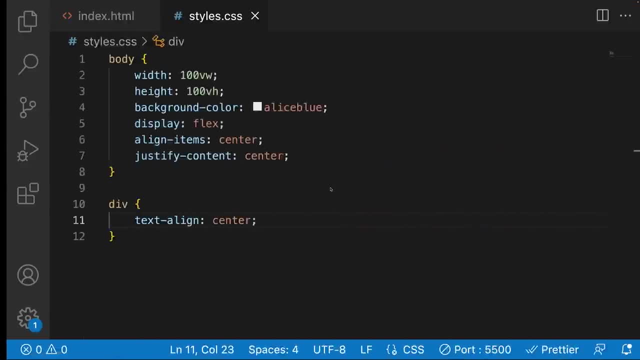 So in order to do this, there are going to be three different steps that we need to take. 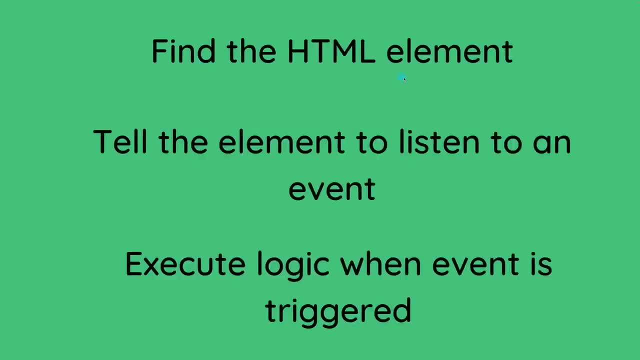 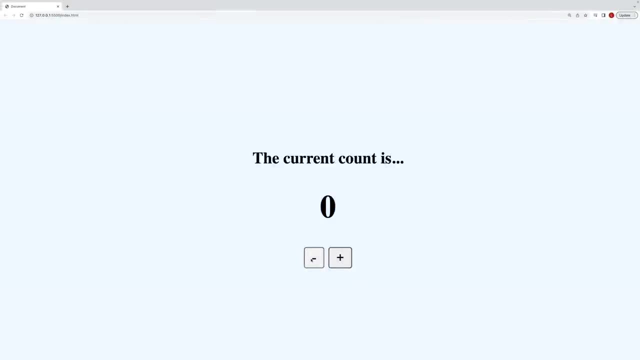 Step number one, we need to find the HTML element. So what are the HTML elements that we need to find in order to trigger our logic? 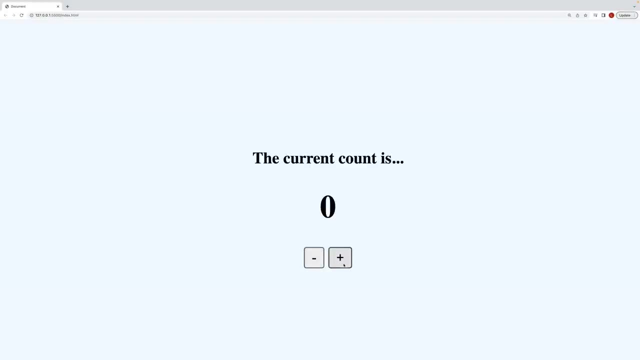 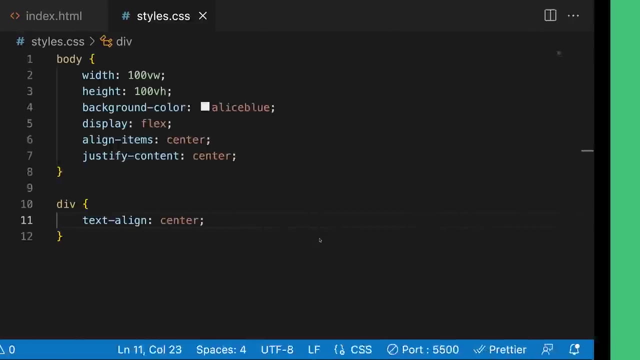 Well, it is going to be these two buttons right over here. When I, well, click this button, I want this to change, of course. So it is going to be these two elements that I want to find. 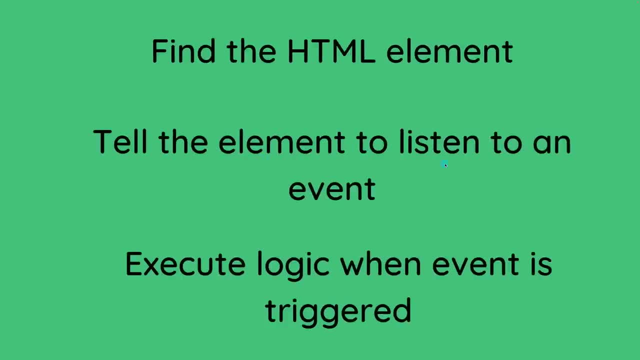 And the next step is to tell those elements to listen to a particular event. What is the event going to be in this case? Well, it is going to be a click event. 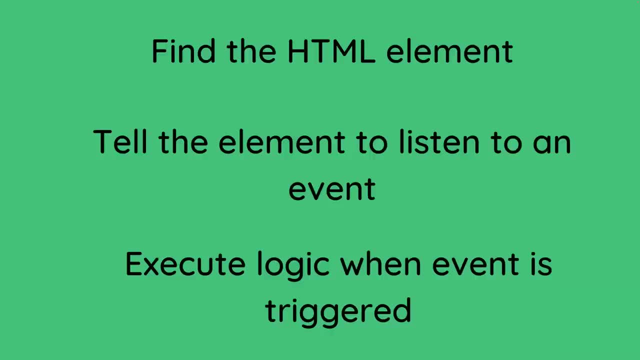 So I'm going to have to find the elements, tell them, hey, I want you to listen to a click event. And then if a click event occurs, so if that event was triggered, I want you to execute some logic. 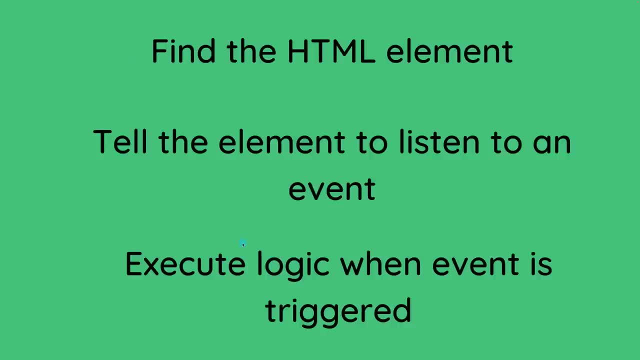 So let's go ahead and actually follow these three steps in order to make our application functional. 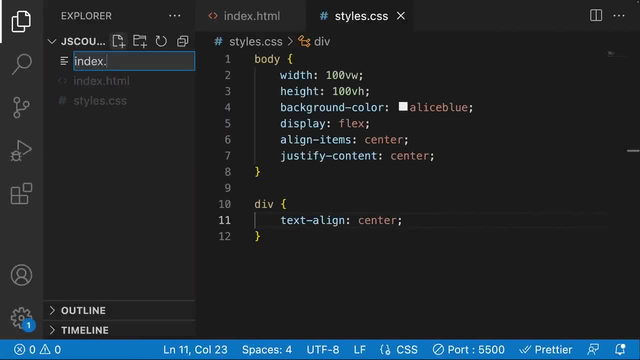 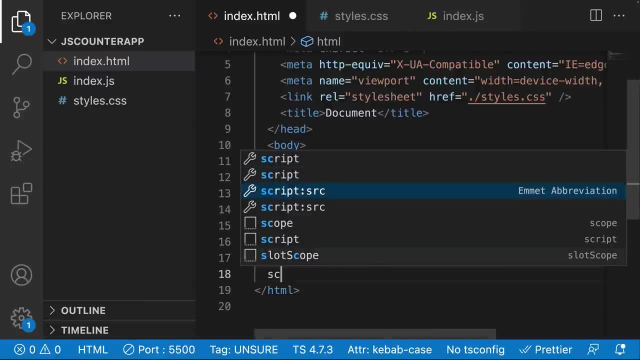 So we're going to go over here, and we're going to create an index.js file. And right away, we're just going to go ahead and link it to our HTML by creating a script tag with a source, and we're going to link it to our index.js. 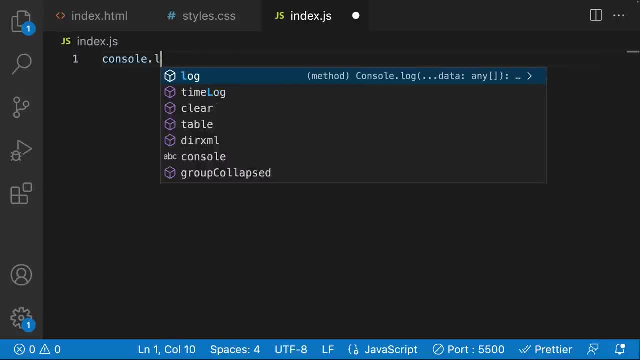 And to see that everything is linked correctly, let's actually use an alert. 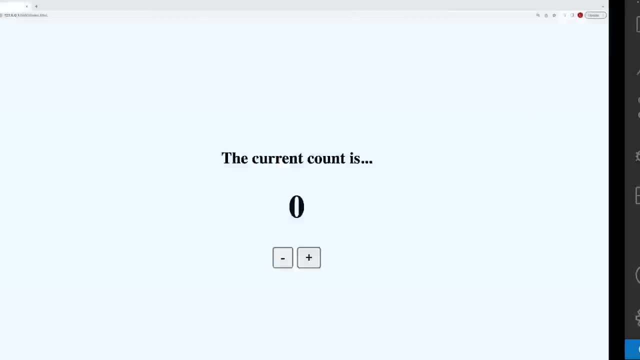 So we're going to say alert, and I'm going to say hello, like so. And if I were to refresh, of course, nothing happens. 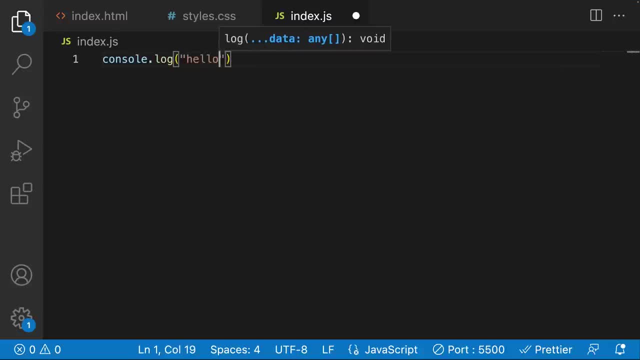 Let me go ahead and instead console.log, and I'm going to say hello. 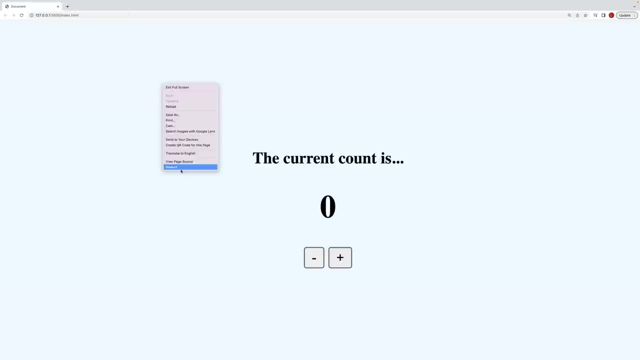 And let's go over here and inspect. Let's go to our console. 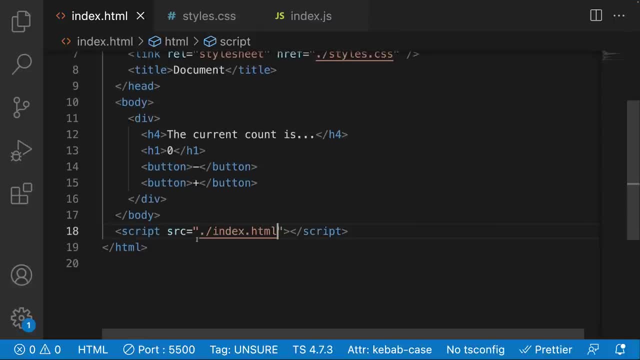 We have invalid syntax. I wonder why that is. 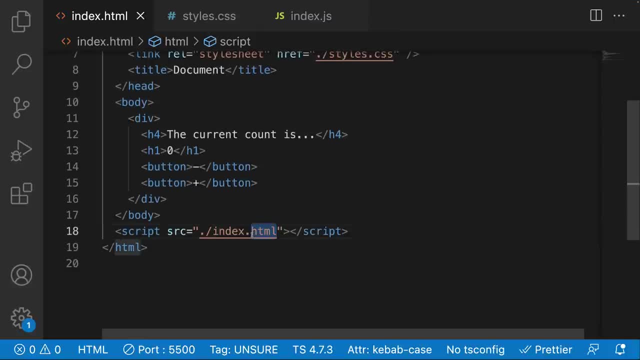 So we got the script tag. We got the source. Oops, I have the JS here. This should be JS, not HTML. And there you go. 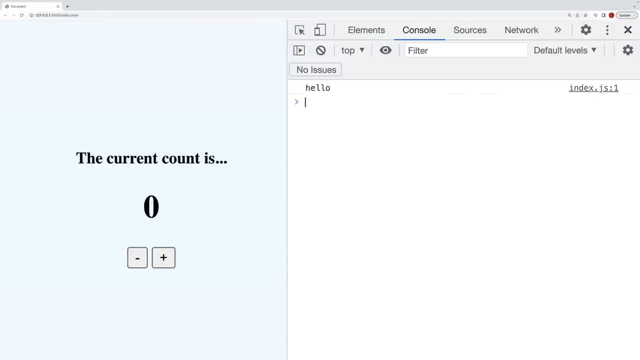 You can see the hello very faintly right over here on my dev tools. So you can see that this works a-okay. Okay. 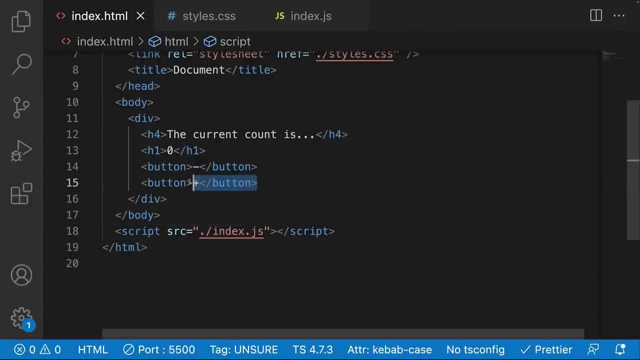 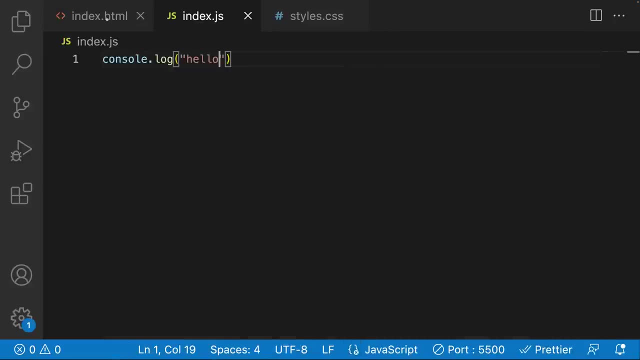 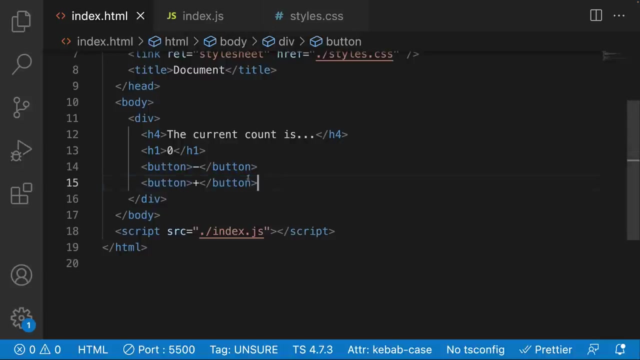 So now what I want to do is I want to find, let's just begin with the plus button. I want to find this plus button. So how in the world am I going to find that particular plus button inside of my JavaScript file? Because right now there are two buttons. Well, typically the way that it's done is that you go to your button and you give your button a particular ID. 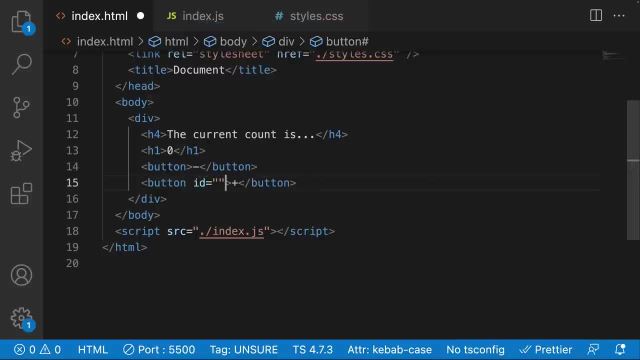 So I'm going to go ahead and give this the ID of let's say add. 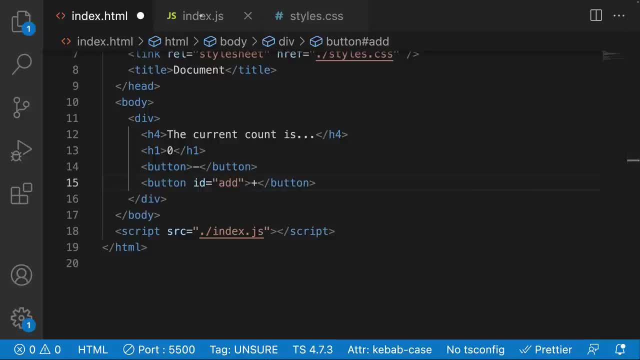 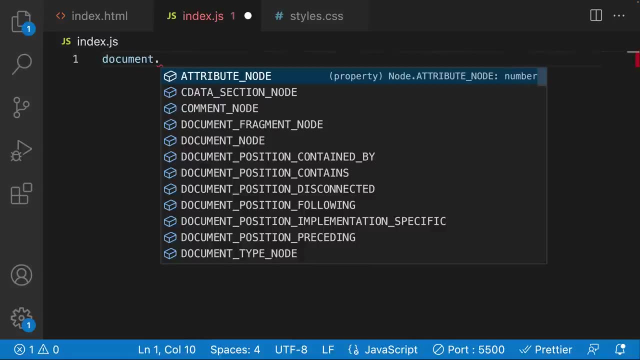 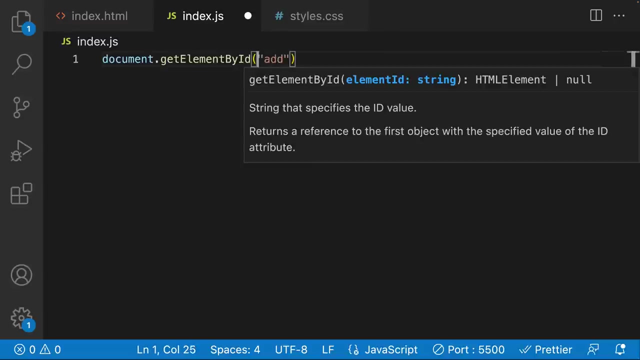 And then inside of my JS, I'm going to go and save this. I'm going to go inside of my JS. And then I'm going to do a document.getElementById. And then I'm going to supply it with the ID, which in this case is string. And then, of course, I'm going to store this as a variable. So I'm going to say const. 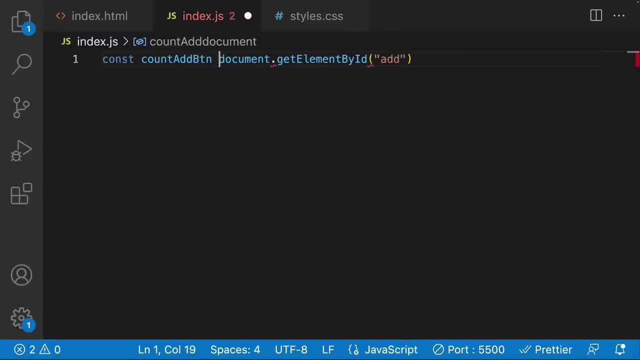 I'm going to say countAddBTN. And then I'm going to say that that is going to be equal to document.getElementById and then add. 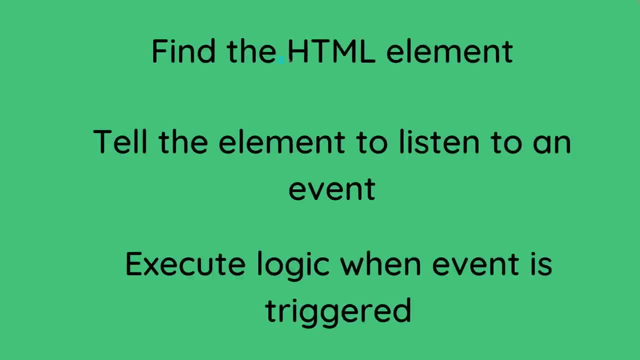 All right. So that is the very first step. We have accomplished this step. Then what we need to do is tell that element to listen to a click event. So let's go over here. 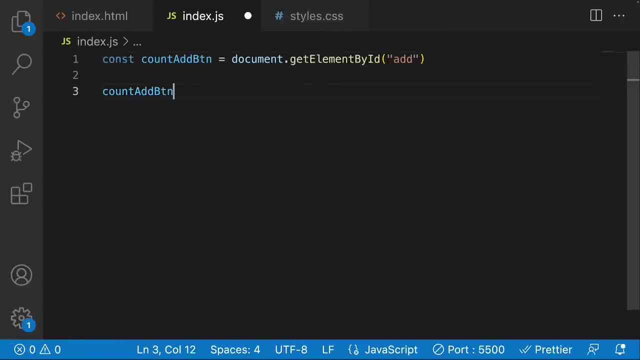 And I'm going to say a countAddBTN. 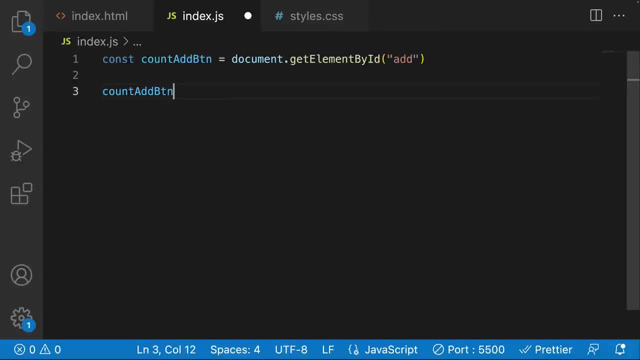 And I'm going to go a little bit faster here because I kind of expect that you know this already. 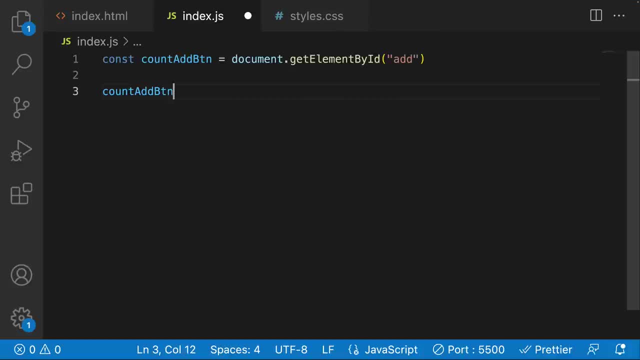 This kind of was a prerequisite. To take in this course, you should know the basics of elements 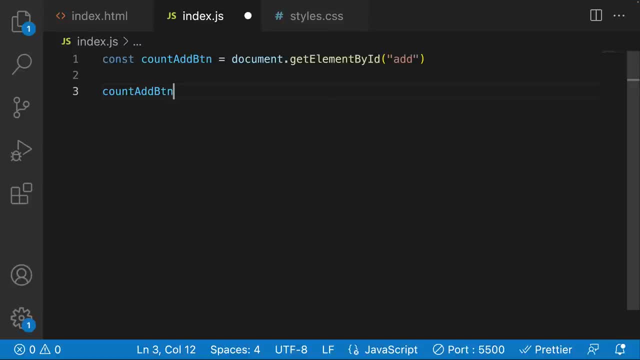 and all the DOM elements and the JS to manipulate it. So I'm going to say here countAddBTN. And in order to add a listener, we very simply just say addEventListener. And this is going to be a method that we are going to call. 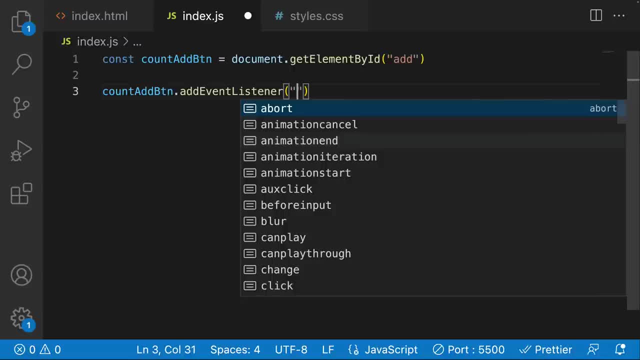 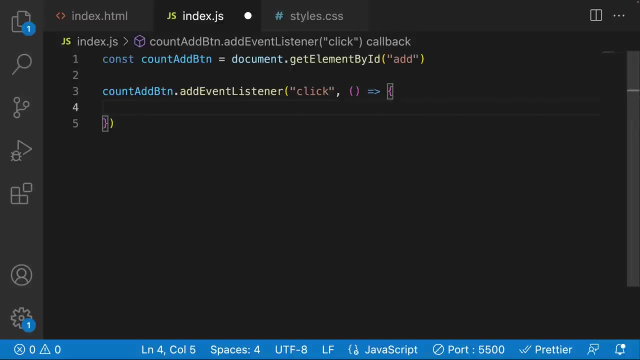 And it is going to take two parameters. The first parameter is the event that we want to listen to. And as you can see, we have many different events. I specifically want to listen to a click event. And then the second parameter is going to be a callback function. I'm going to make it an arrow function. And this is going to be a function that is going to be executed whenever a click event occurs on this button. And just to prove this to you, I'm going to go ahead and console.log hello from the add button. 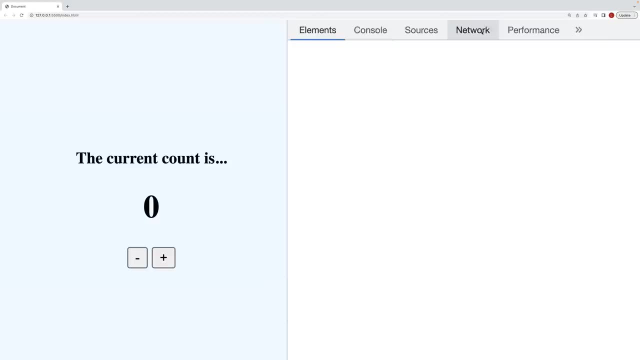 So let's go here. Let's go ahead and inspect. 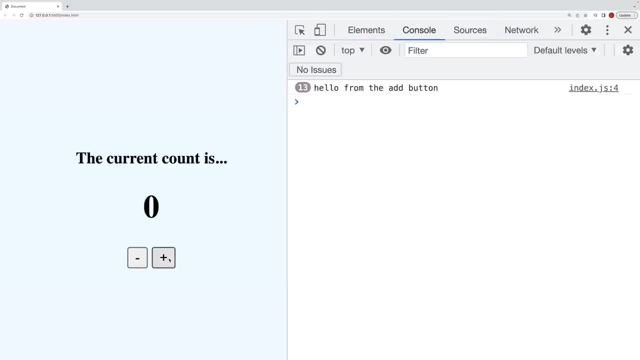 And whenever I click on this button, as you can see, I get a hello from the add button. If I click on the minus button, of course, I don't get this. 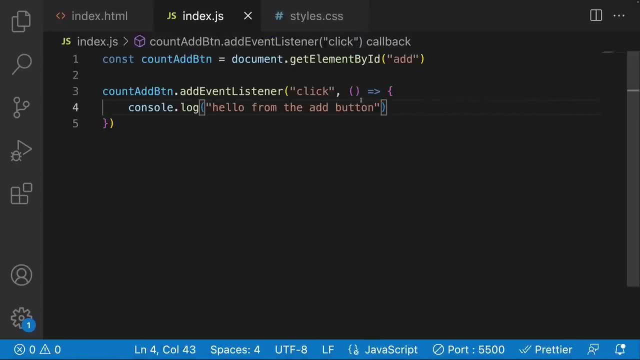 So now what I want to do is, of course, I want to update the current count. Now we're going to actually need to store this count variable 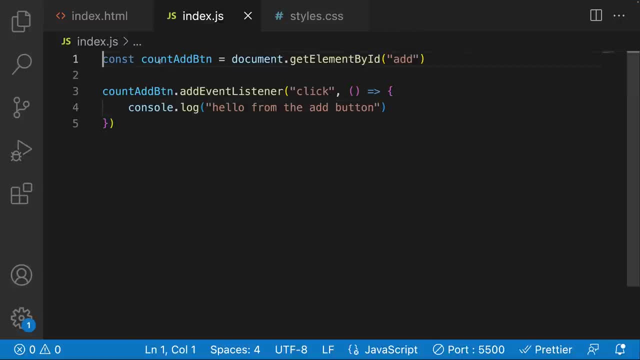 inside of the JavaScript because it is something that is going to be changed and manipulated. 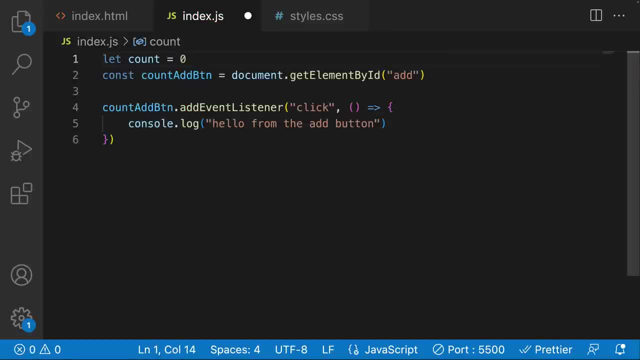 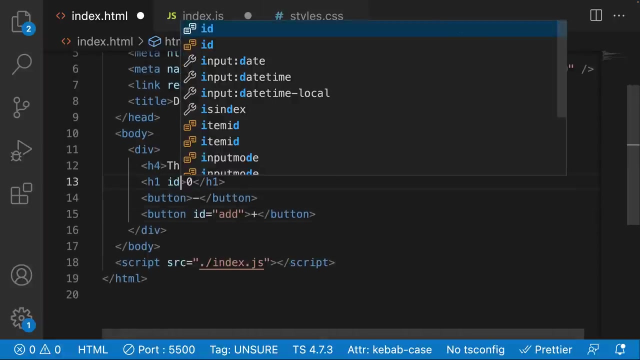 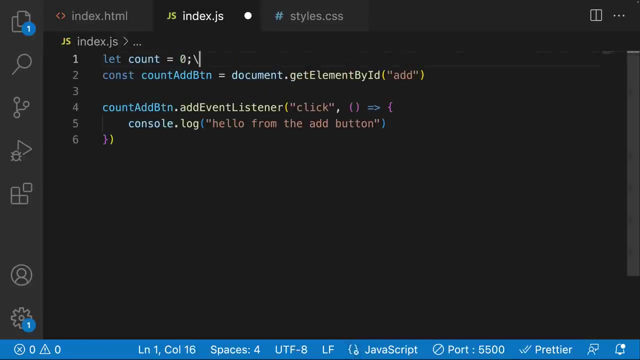 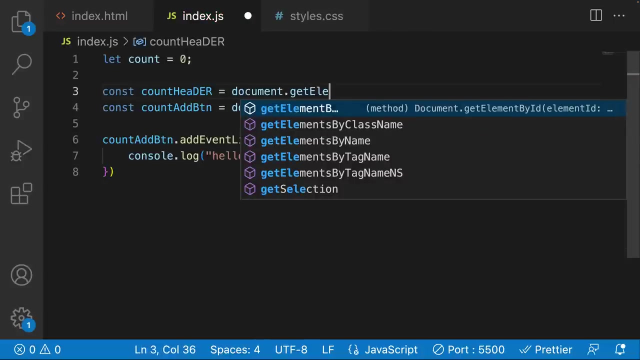 So over here, we can say something like let count is equal to 0. And I actually want this count right over here, whatever the value of this variable is, to be the value that is inside of this h1. So let's actually go ahead and give this h1 an ID of count. So let's give it an ID of count. And let's go ahead and do a const. And I'm going to say count header is going to be equal to documents. So document.getElementById. 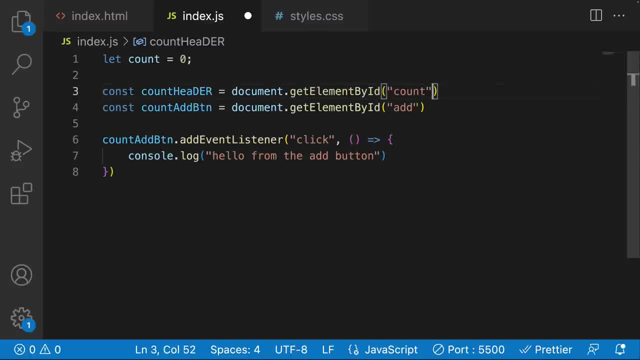 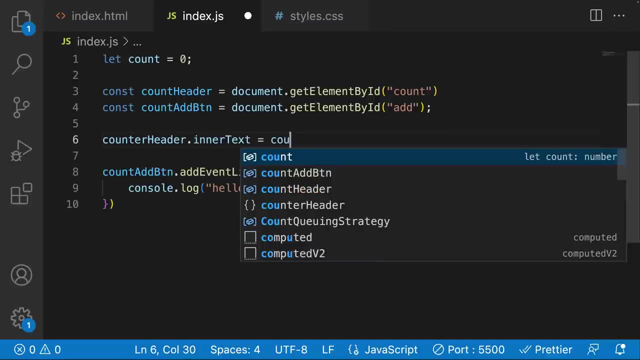 And I'm going to call this just very simply count. And then, and let me change the header. I don't know why I sold capital there. Let's do header. And then over here, we're going to go ahead and say count header.innerHTML. So inner, or maybe even inner text is better. So we're going to say count a header.innerText. And that's going to be equal to, to the count variable. 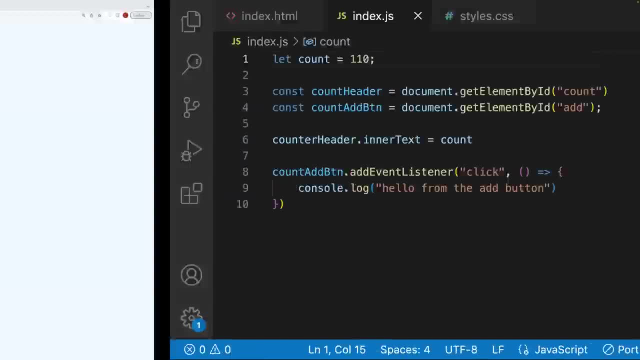 So right now, as you can see, it is still 0. But if I were to change this, for example, to 110, and do a little refresh, it does not work for some reason. 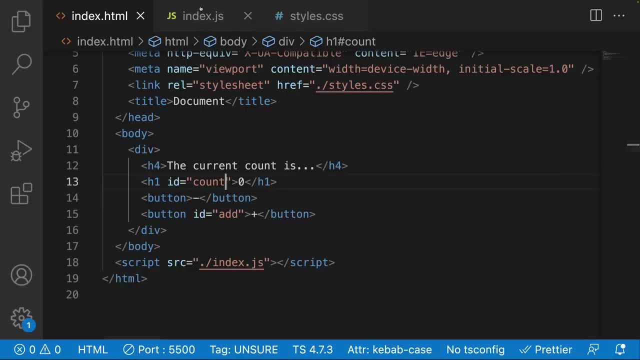 Is that because, it doesn't work for some reason, which is a little bit confusing. 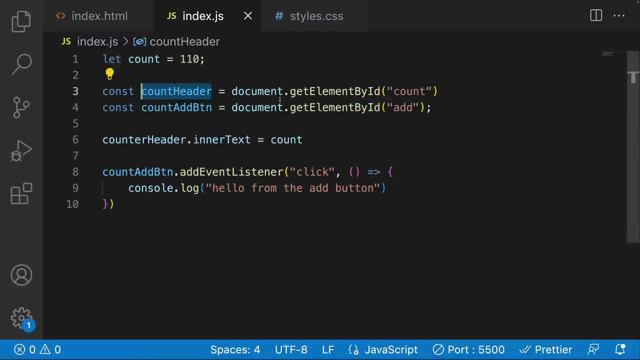 So we have over here the count header. And then we have a document, getElementById count, which is the count over here. 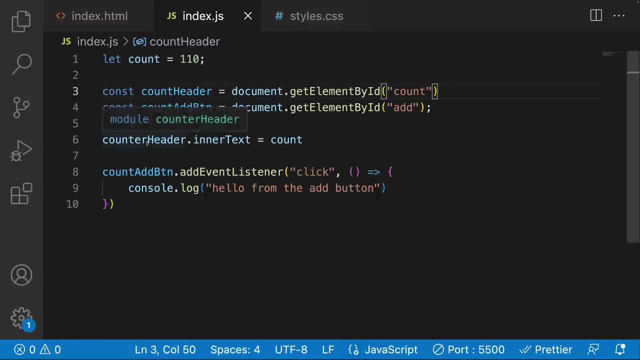 And then what we have here is the count, oh, that's what it is. There we go. 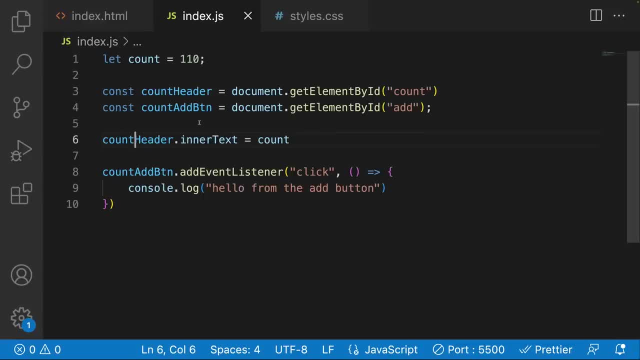 You guys should have told me why I had to do all this debugging. Why don't you tell me I just misspelled it. Okay, so now let's go over here, change this back to 0. 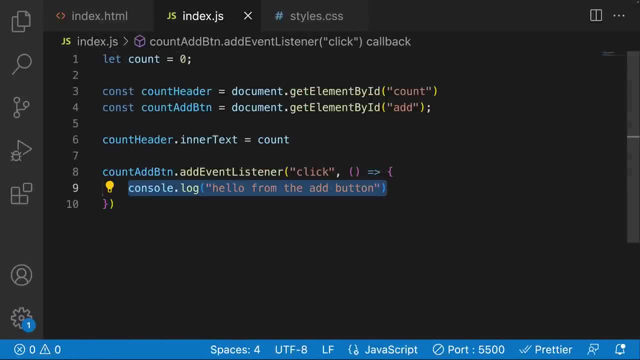 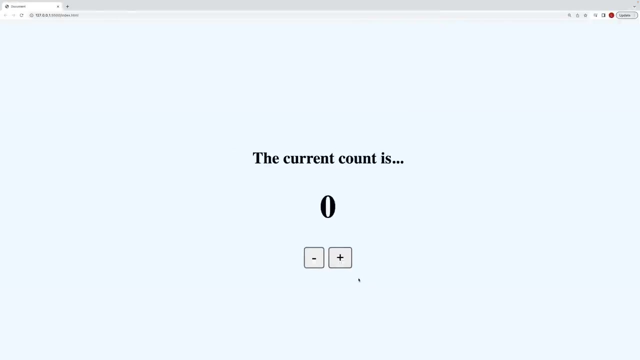 That is looking great. So what I want to do here is, well, when I click this button, I want to increase the count by 1. But just increasing the count by 1 isn't going to set the inner text of the count header to whatever the count is. For example, now, you can see here, I'm increasing the count, but the current header needs to be updated. So over here, we're going to just go ahead and do this. We're going to say, the currentHeader.innerText is going to be equal 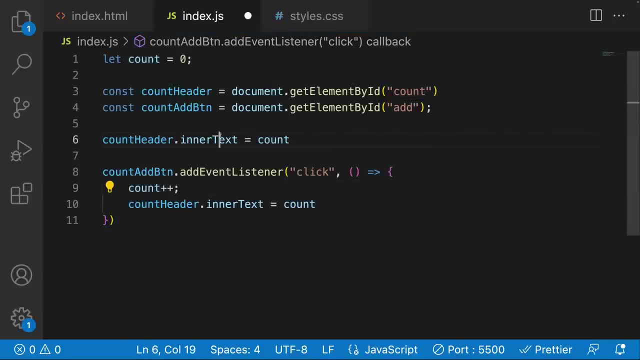 to what the count currently is after I updated it. 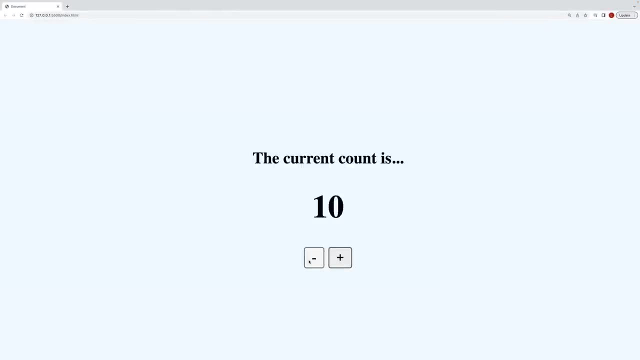 So now if I click on this, as you can see, it is updating. 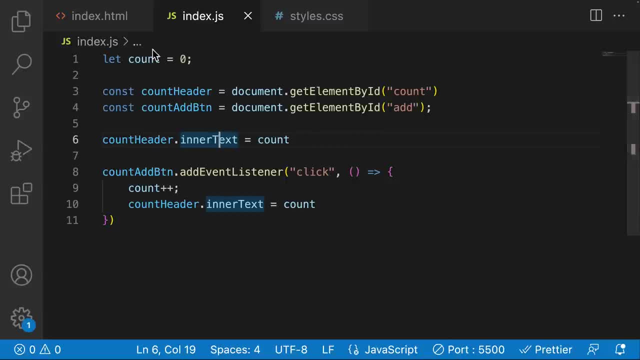 So now we need to do the exact same thing for the minus button. 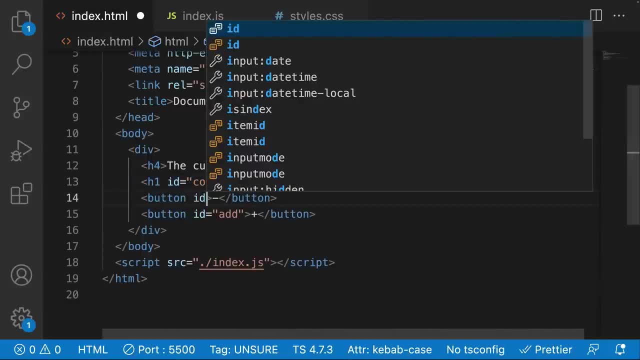 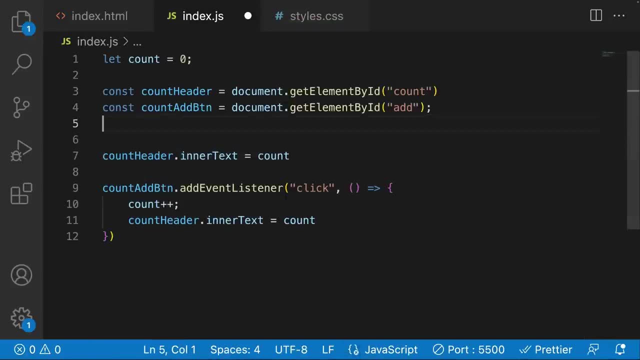 So let's go over here, and I'm going to create an ID, and I'm going to call this, well, subtract. Let's go ahead and save that. And I am going to say const. I'm going to say this one, countSubtractBtn. That's going to be equal to document.getElementById, and we're going to say subtract like so. 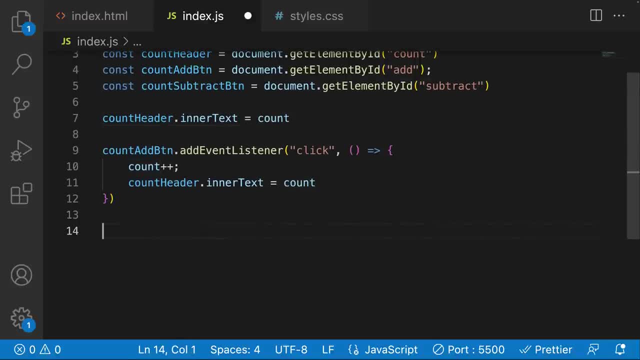 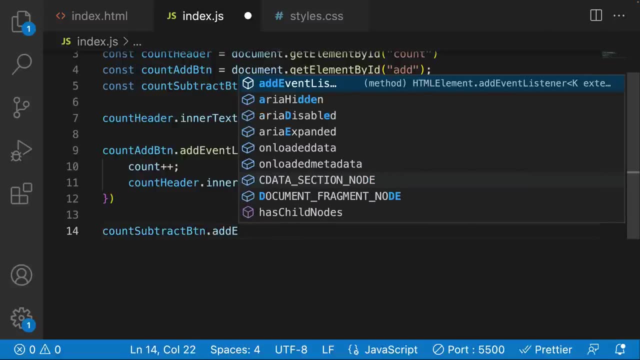 Now over here, we're going to have the exact same logic. We're going to have an event listener for this. We're going to say count, and then subtract btn.at, addEventListener, and we're going to listen to a click event. 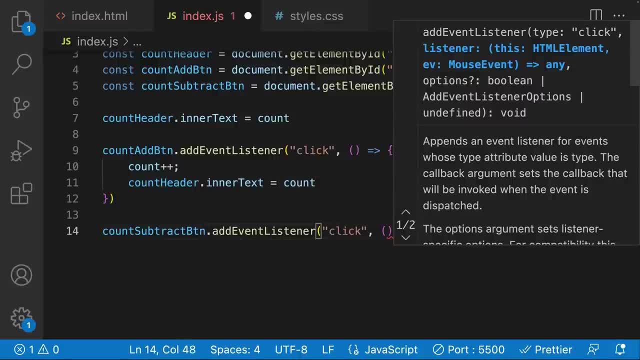 And then over here, we're going to execute a callback. So over here, we're going to say count minus minus, so we can minus it by one. 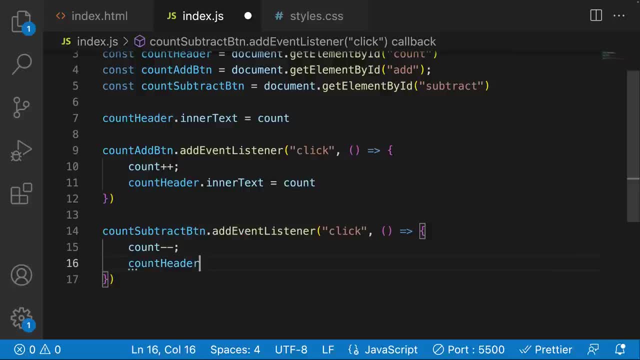 And then we're going to say countHeader.innerText is going to be equal to the count that we have just updated. So let's go ahead and save this. 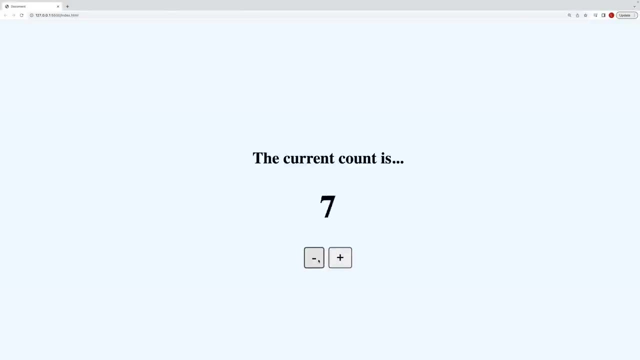 And let's go over here. And as you can see, everything is working as expected. 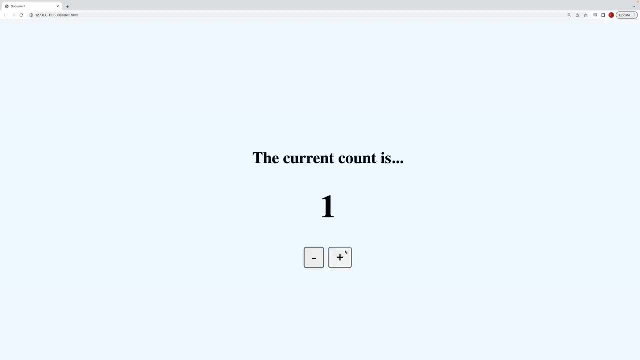 So we pretty much finished this application. That is great. And that is pretty much all it is that we're going to need to do 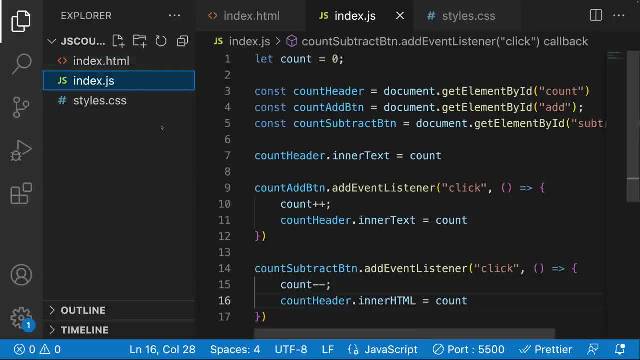 if you want to build an application like this with Vanilla.js. 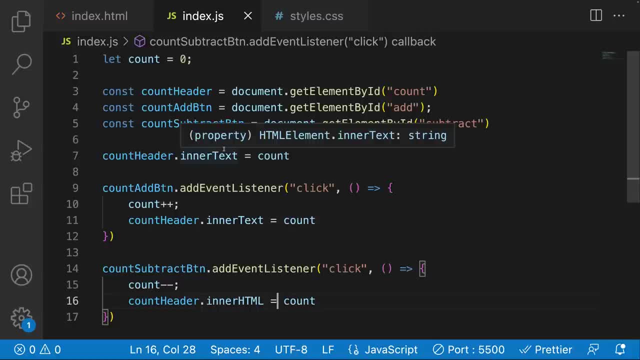 Now this is a really, really simple application, but it actually took quite a bit of code 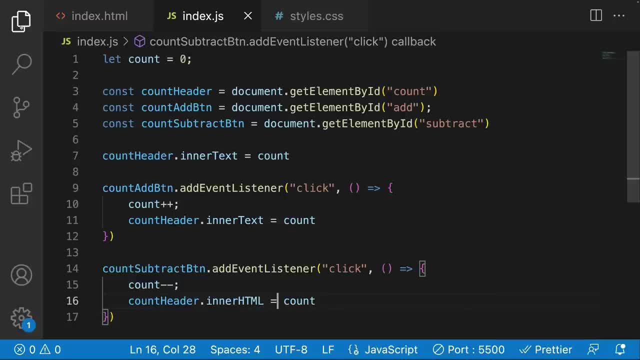 to execute with Vanilla.js. Now let's actually go ahead and 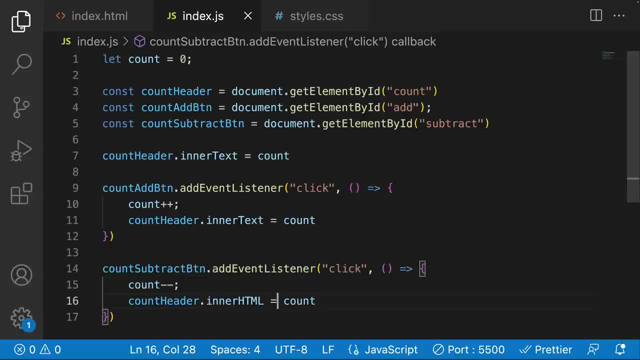 build this really simple application, but with Vue.js. 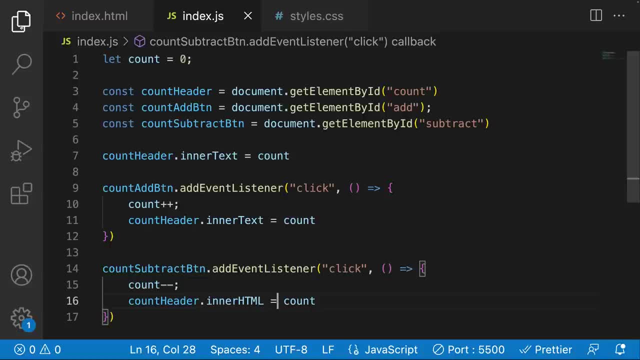 And trust me, you're going to see the difference. All right, everybody. 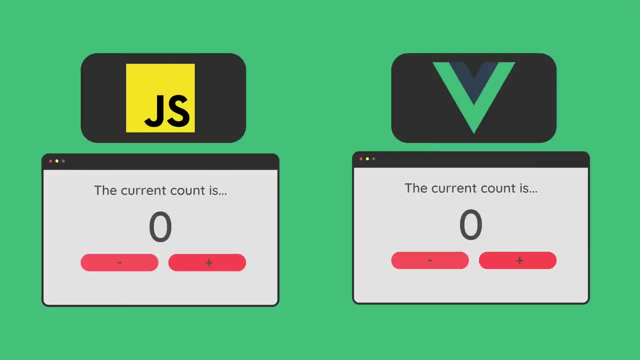 Let us now replicate the counter application, but this time with Vue.js. 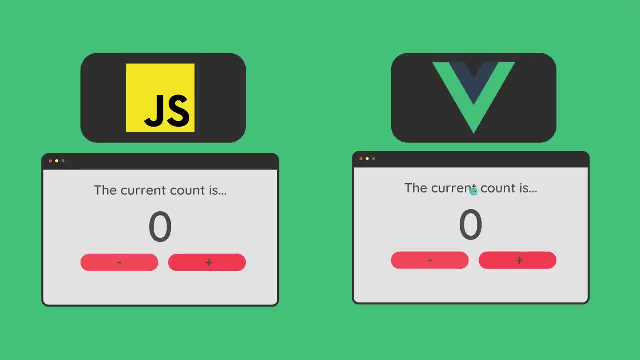 So in order to do this, we first actually need to create a Vue project. 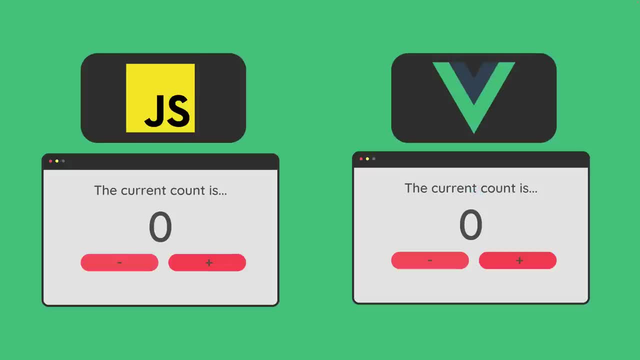 And there are two approaches that we can take to create this Vue project. 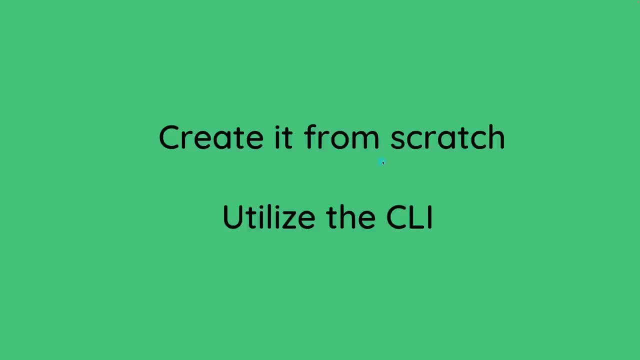 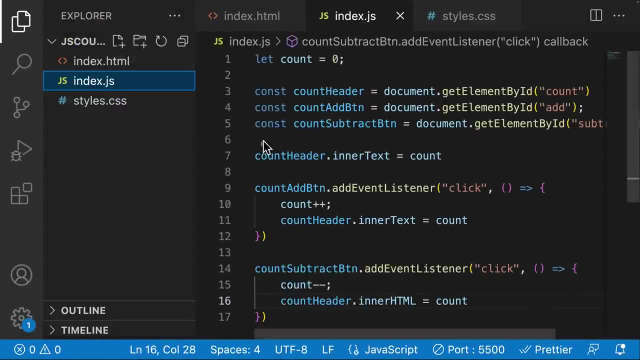 Approach number one is to create the Vue project from scratch. So very similarly to what we did with our application over here, we would create an empty directory, and then we would just start creating all of the different files that we need in order to create our Vue application. 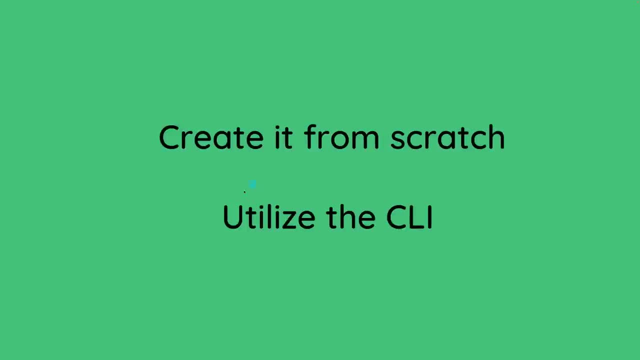 So that is the very first approach. The second approach is to use a command line interface to create a Vue project 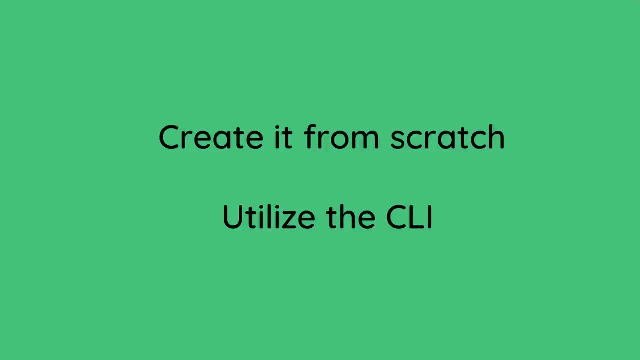 that has all of the boilerplate code that we already need. And this is actually the better approach 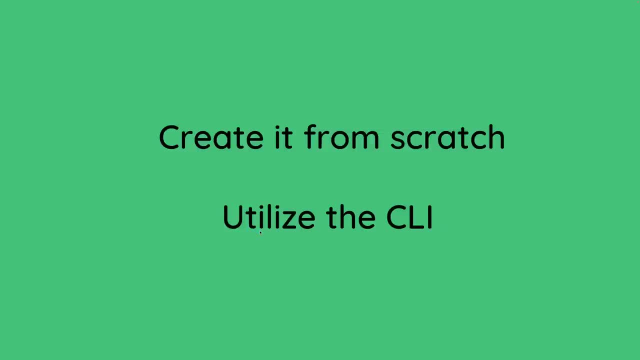 because every single time we create a Vue project, we always need kind of the same files and folders. 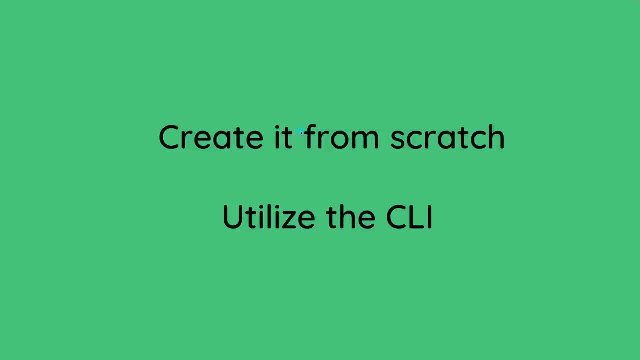 And it would be just a quick pain and it is going to be error prone to create it from scratch. 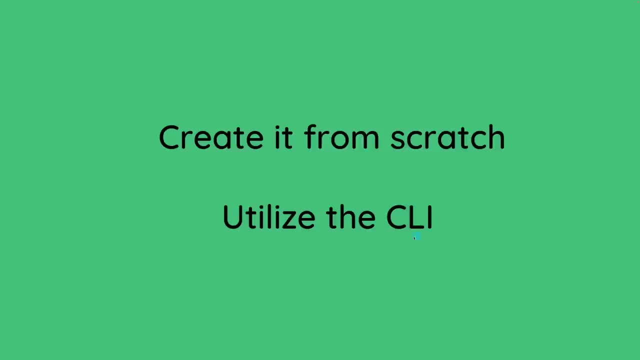 So instead, we are going to use a command line interface in order to create our Vue project. 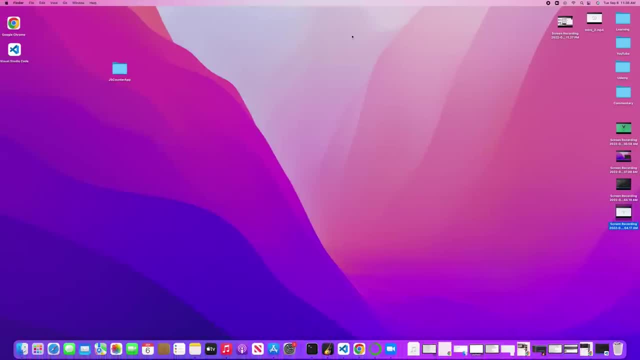 So to do this, go over to your terminal. So I'm going to go here. 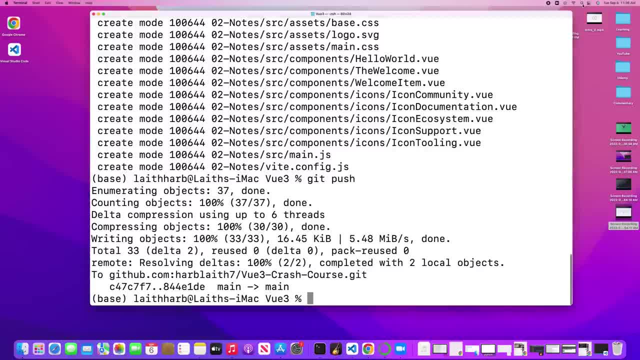 I'm going to open up my terminal. So you can open up a terminal or if you're on Windows, a command prompt. 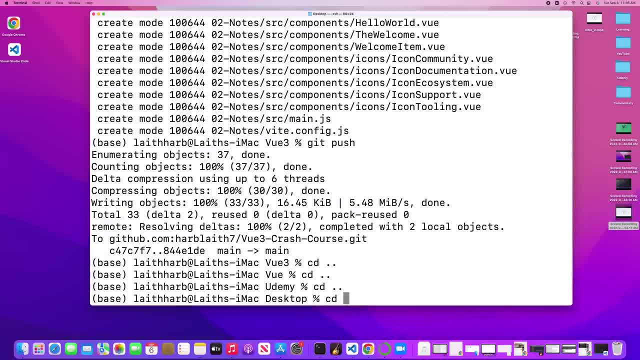 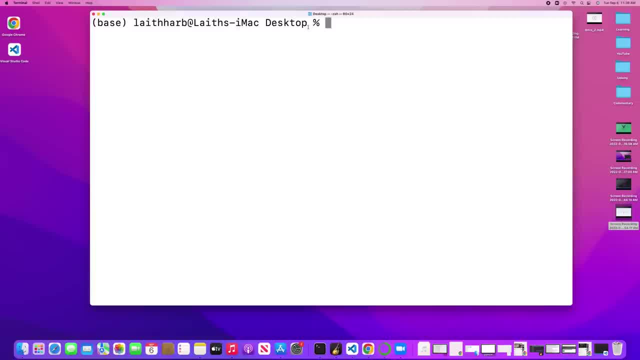 And what I'm going to do is I'm going to move into my desktop directory. So over here it should say desktop for me. And now you can go ahead and move into whatever directory you want to create this project into. Again, I want to create it in my desktop. 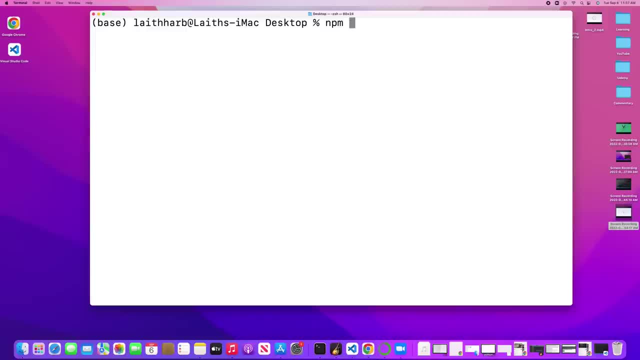 And then all we have to do is npm, which we already installed, init Vue at latest. 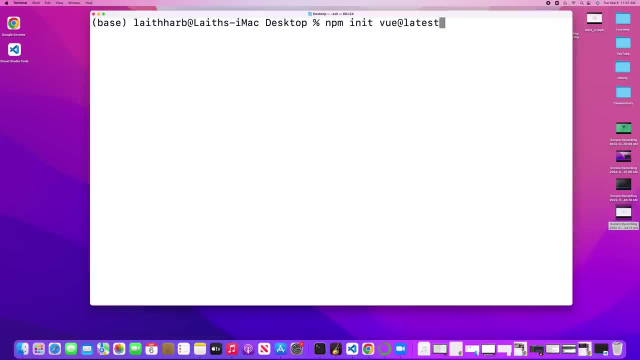 And what this is going to do is initialize a Vue application for us, a brand new Vue application at the latest directory or the latest version. 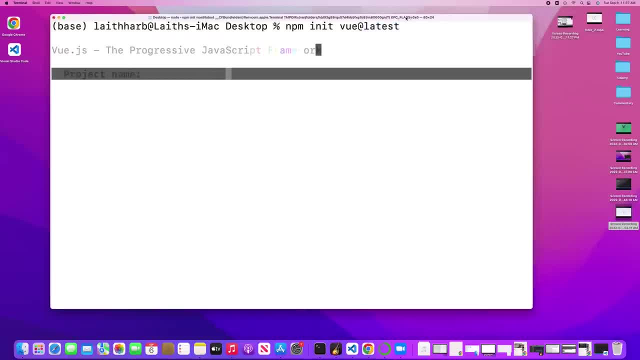 So now what we can do here is actually go ahead and create it. 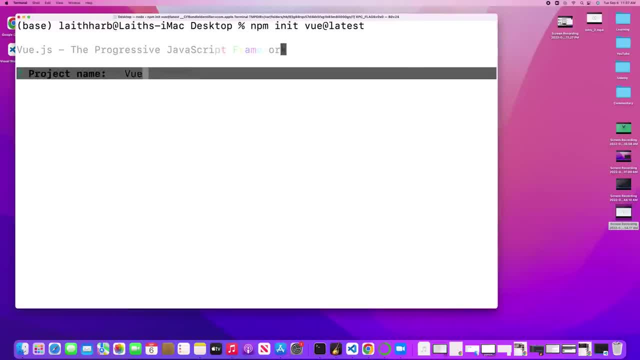 And it's going to ask us with some questions. So I'm going to call this VueCounterApp. That's going to be the project name. Package name we'll just leave as a default. TypeScript we'll say no. JSX we'll say no. Vue Router we'll say no. Everything we'll say no. And we'll talk about these things a little bit. 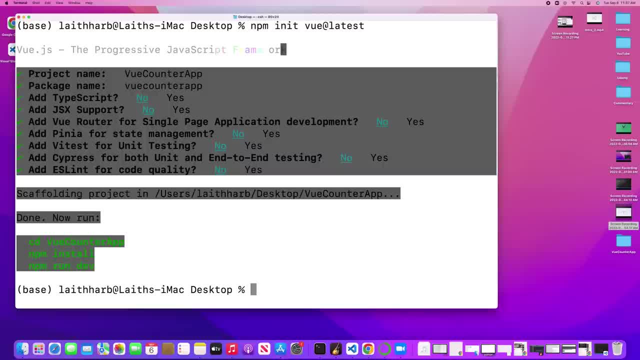 Later in the course. Do not worry. But for now we'll just say no for everything. 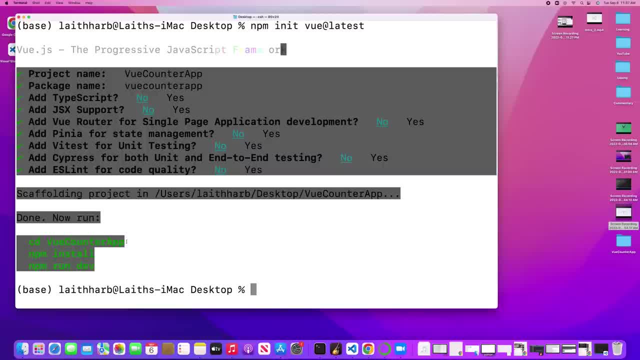 And then over here it says, well, everything is done. And we have created our VueCounterApp. And if you look at your desktop directory or whatever directory, you should see a new folder. 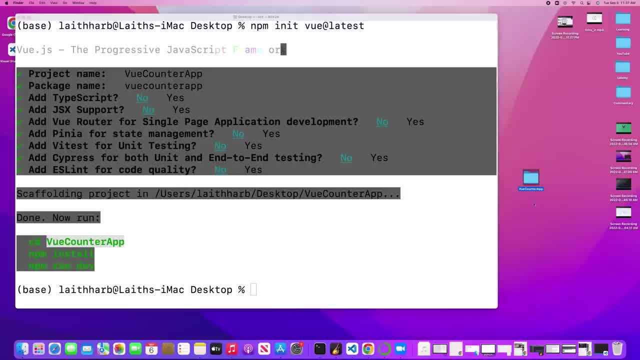 And then what it's saying, in order to actually start this application over here, what you have to do is an npm install as well as an npm run dev. So let's actually go ahead and run these commands. I know a lot of these commands might not make a lot of sense. Don't worry. Again, we're just going to go ahead and code this out really quick. And then we'll talk about it in great detail a little bit later. 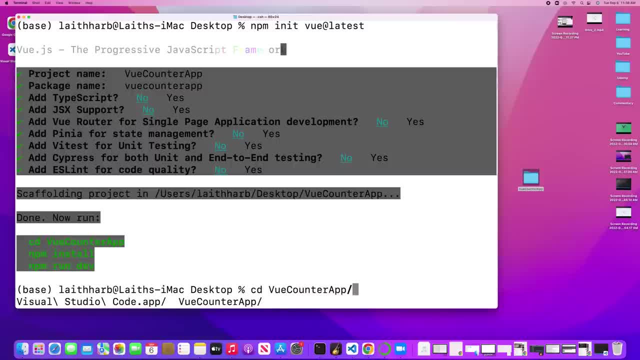 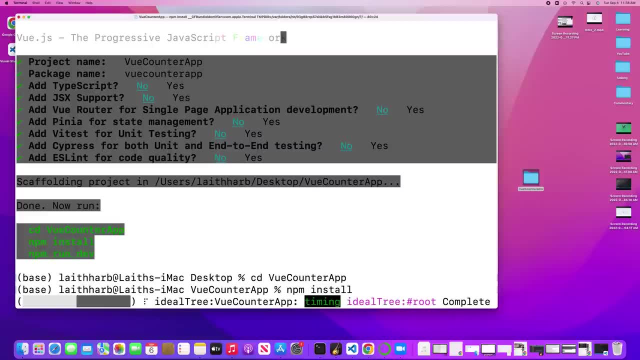 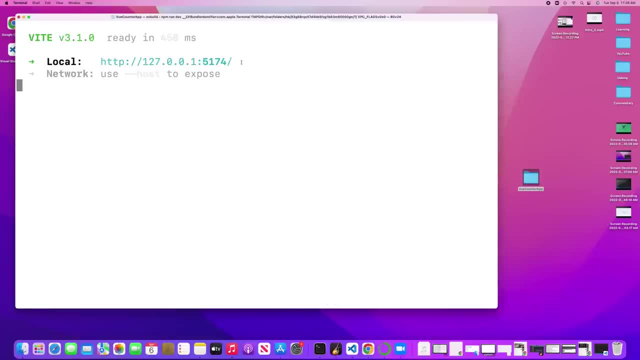 So let's move here. And we're just going to move into our counter app. We're going to do an npm install. And then let us do an npm run dev. And that should run our application on this port right over here. So it should be localhost 5174. 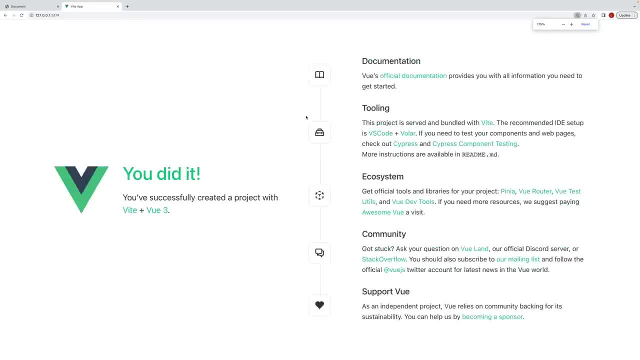 So now if I went there, you can see I actually have a Vue application up and running on that port. 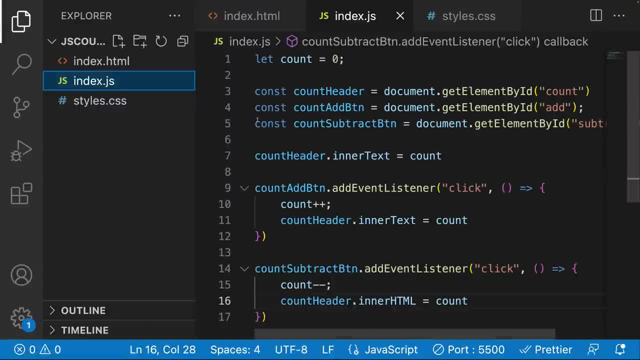 So we have successfully created our Vue app. Now the one thing I want to do is actually want to have this Vue app opened up in VSCode. 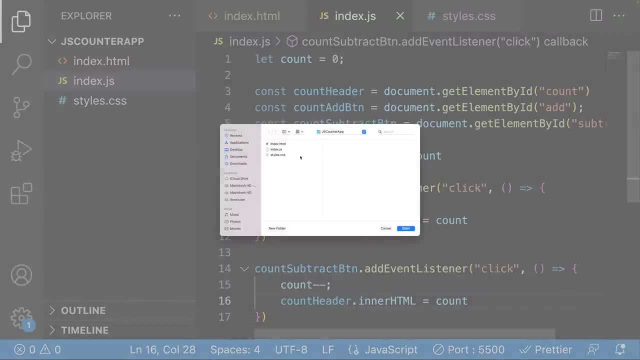 So over here, I'm just going to open up the application, which is in my desktop, the VueCounterApp. 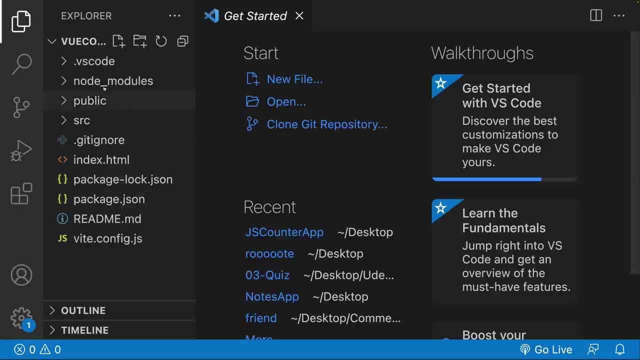 And there we go. So now I opened it up in VSCode 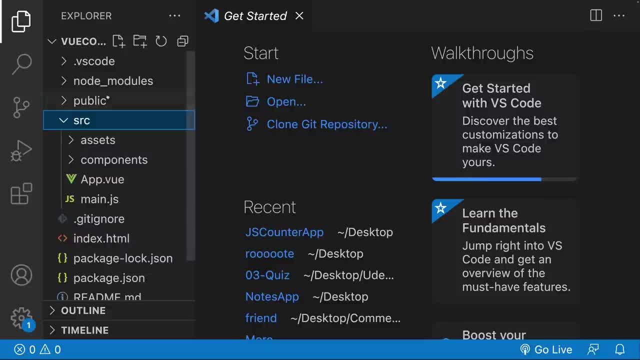 and actually see all of the different files and folders. Now there's a bunch of different files and folders. Don't worry, 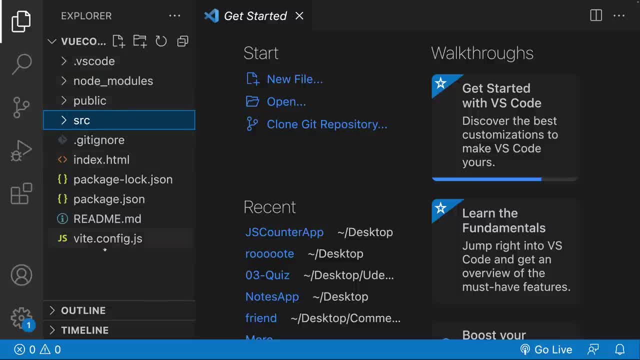 we're going to cover everything in tremendous detail. So do not get too overwhelmed. Okay. 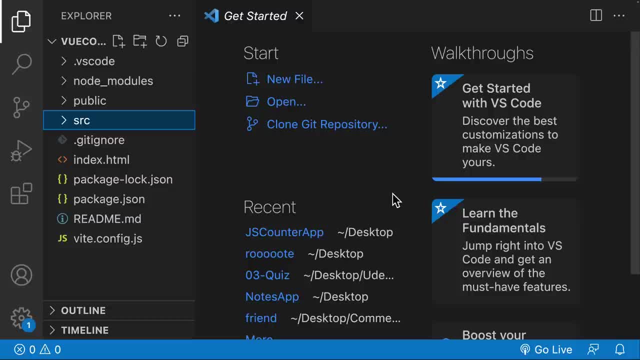 So now that we got our application app on running, let's go ahead and actually convert it into this counter application that we have right over here. 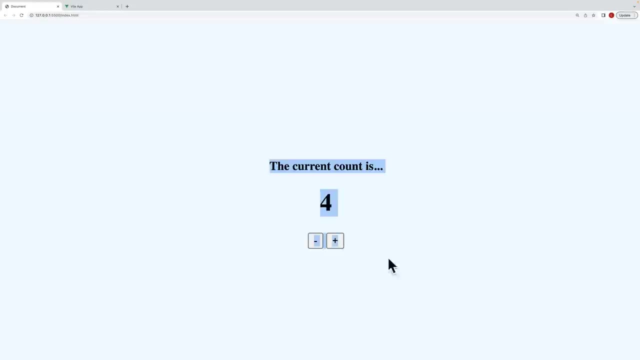 So what we want to do is we want to just have the, basically the same application, the same logic, but this time using Vue. 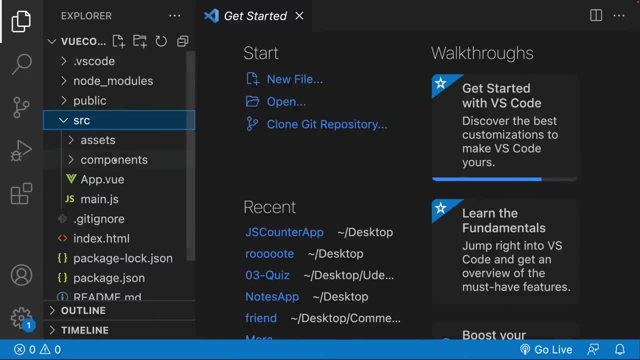 Now inside of Vue, in order to actually accomplish this, all we have to do is work with the app.vue file. So this might not make a lot of sense to you. 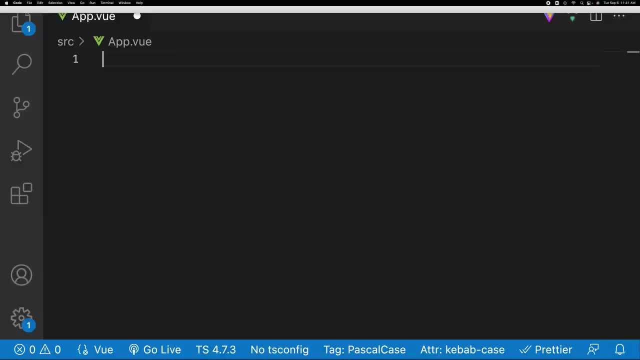 That is okay. But what I'm going to do is I'm just going to go ahead and code out the application from scratch. 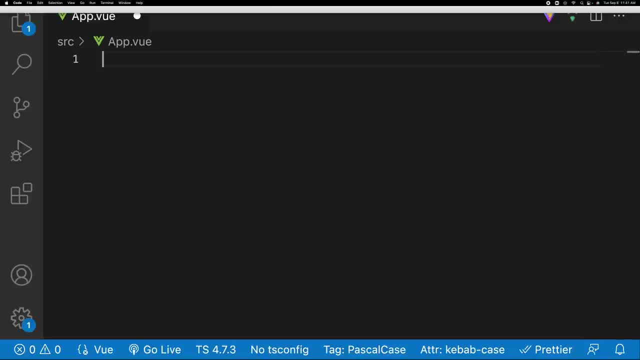 And I'm going to do very little explanation. And as soon as I'm done, we're just going to quickly compare it to the vanilla JavaScript version. 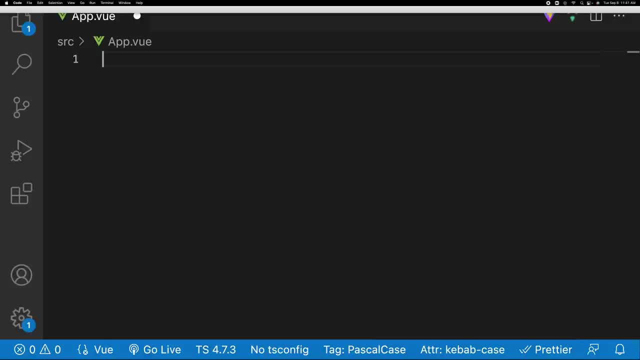 And then in the next section, we're going to rebuild this application, but go through everything in tremendous detail, more detail than you can ever imagine. 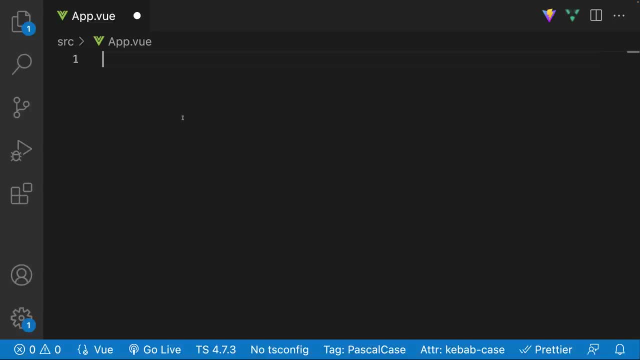 So if you feel like I'm going really fast here and I'm not explaining things, don't worry, we're just going to code it out really quick. And then we're going to explain everything a little bit later. Okay. So inside of the source directory, we have our app.vue file. Over here, I just went ahead and I removed everything. I'm going to go ahead and save it. 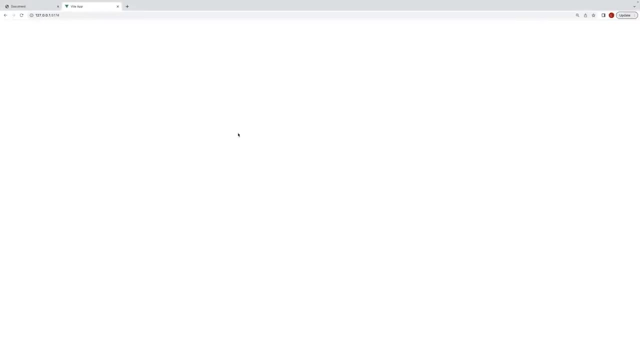 And as soon as I save it, you can see now I have a blank screen. 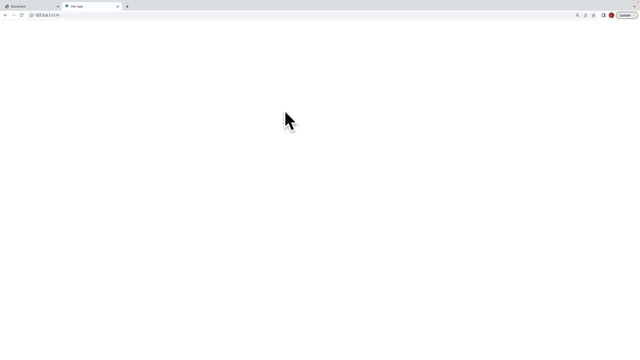 So it seems as though that this file is responsible for what is rendered over here. 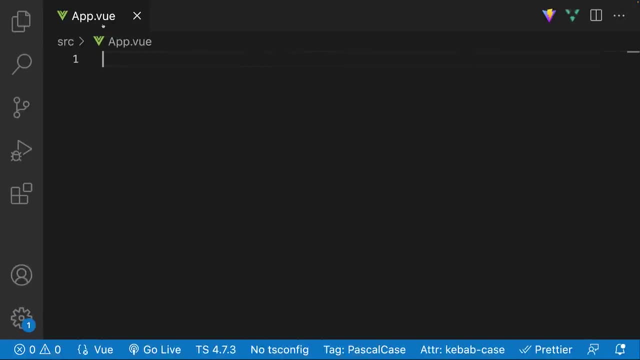 So the first thing that I'm going to do inside of this app.vue is I am going to create the HTML template. 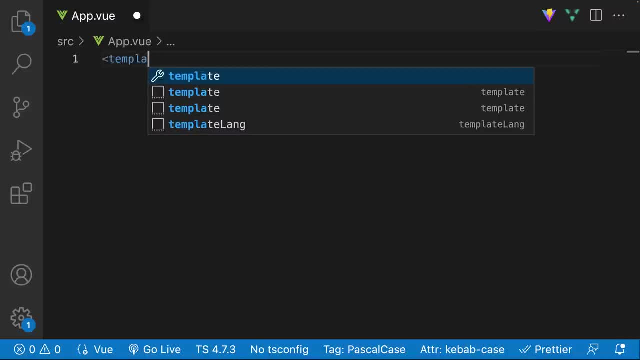 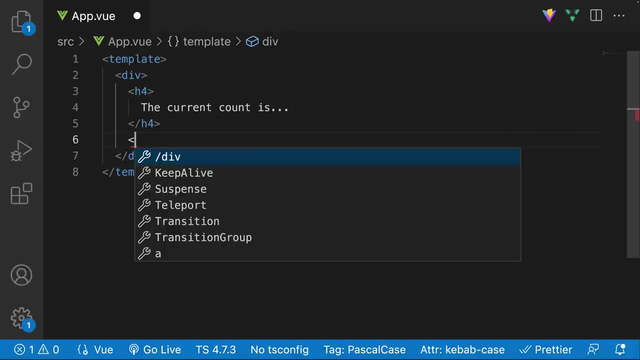 So let's go over here. I'm going to say template as my first HTML tag. And then I am going to say, well, div. And then over here, let's have an H4 like we did before. And then I'm going to say, let's say the current count is and then dot, dot, dot. And let's have an H1. 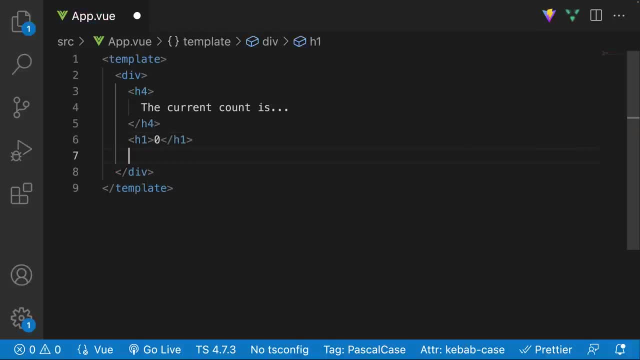 And then over here, we're going to say, initially we'll have it as zero. We'll just hard code it as zero. 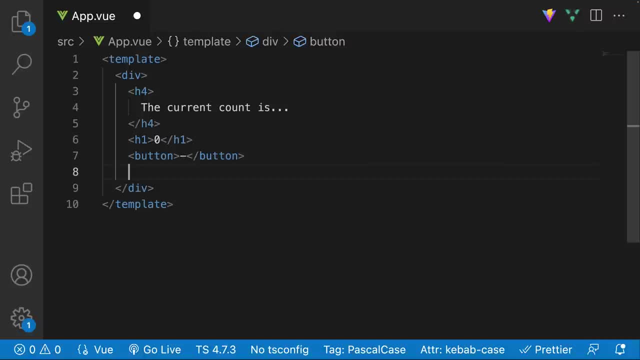 And then we'll have a minus button as well as a plus button. 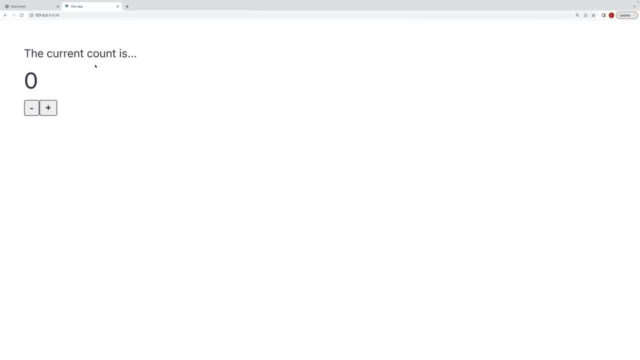 So now we're going to go ahead and well, as you can see, we have our wonderful app 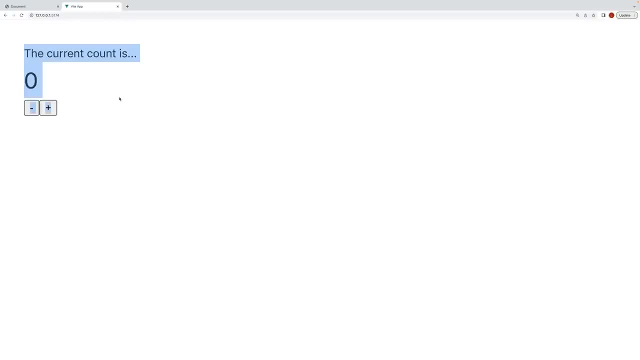 and it is, well, nice and the font's a little bit different, but that's okay. But you can see it is, well, the template is there. 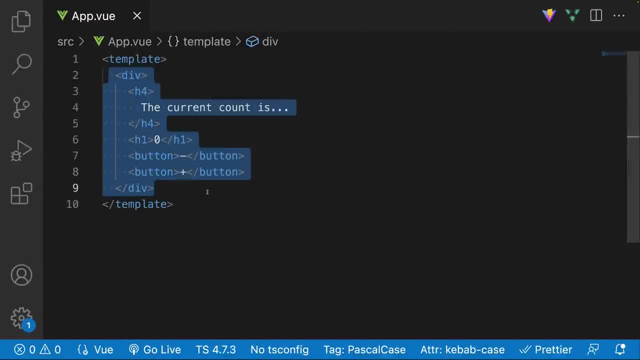 So now what we're going to do is we're going to need to style our application. 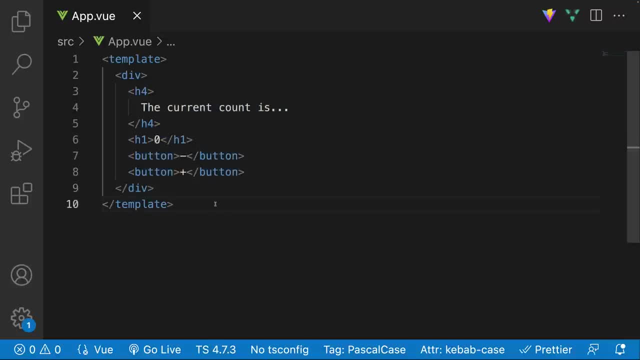 So still inside of the app.vue, what we can do is we can actually add style tags. But this time inside of this style tag, inside of this very first tag, I'm going to add a keyword called scoped. Don't worry about what this does. We'll talk about this later. Do not worry. But we're just going to add that for now. 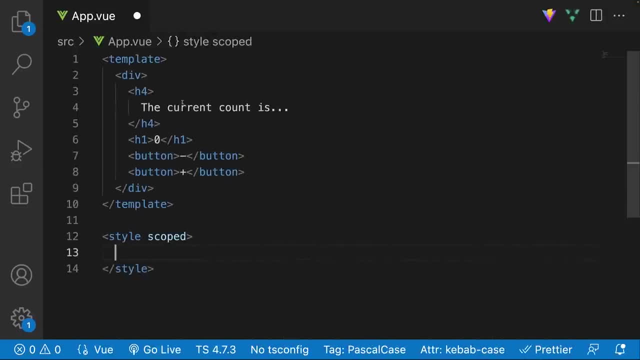 And what I want to do very simply is just kind of center this right in the middle. 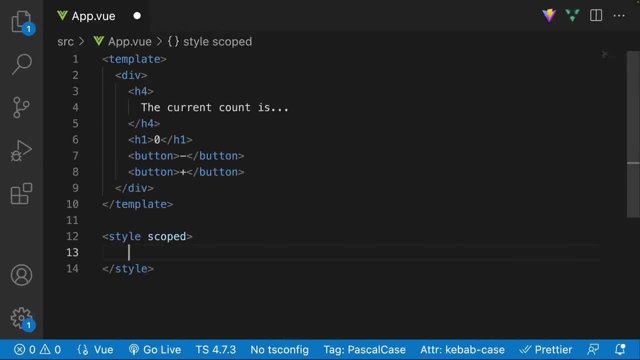 So let's go ahead and style this div. So really there's only one div here. So let's just say div. 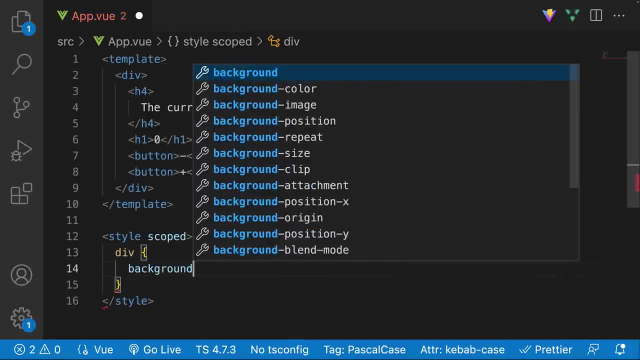 We can say, let's give it just a background color of Alice blue. 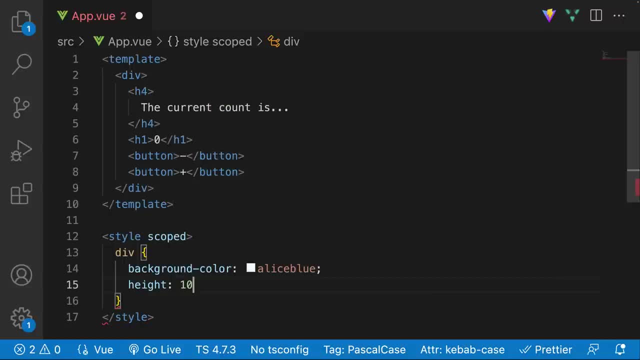 And then let's give it a height of 100 VH. 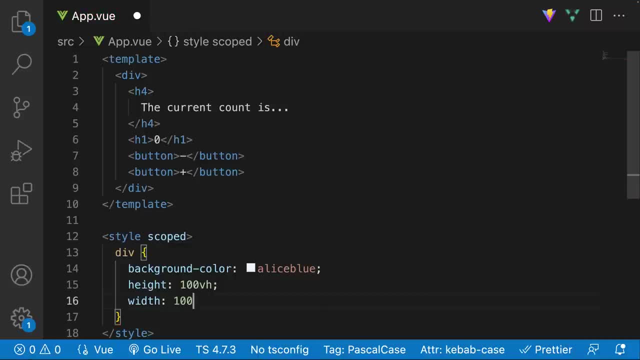 And let's give it a width of 100 VW. 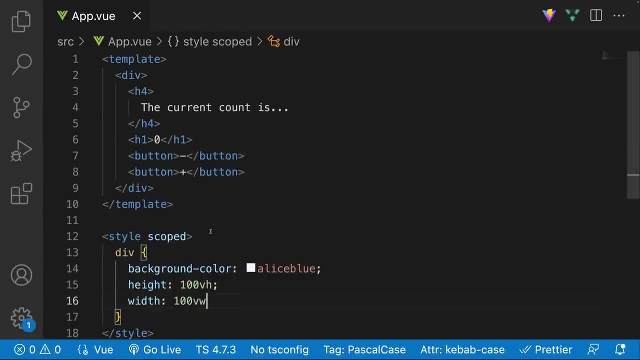 And there we go. You can see it's kind of centered in the middle. That's fine. There's some styling here that's just kind of awkward. 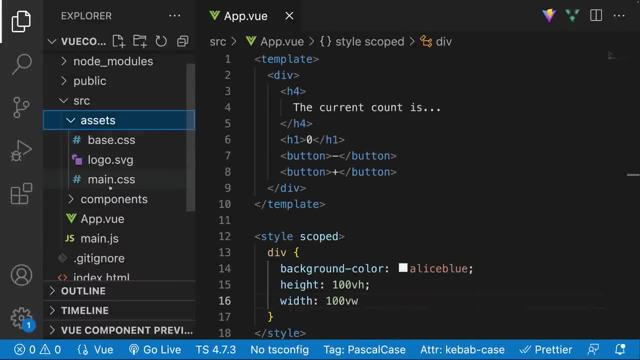 So what we can do actually to remove that is we can go to the main.css file and just remove kind of all the styling over here. Let's just remove that. And there we go. So now the styling is gone. 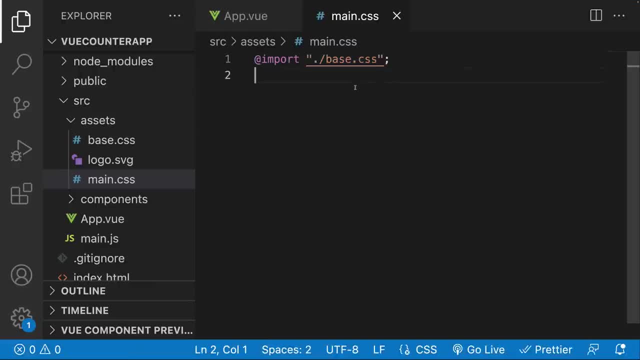 We can just leave this if you want. We'll talk about this a little bit later, but we can leave that because I like these styles right over here. Okay. So we have that. 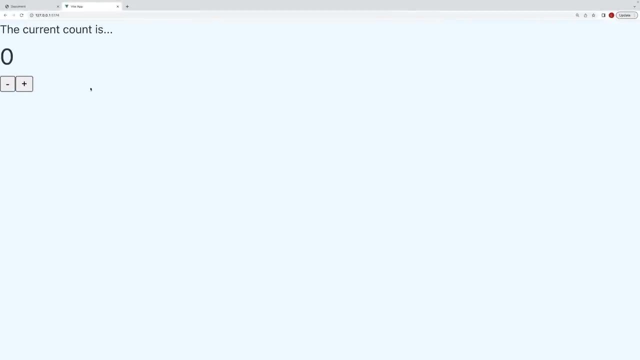 So now we have the styling done. And now all is left is to kind of center this right in the middle. 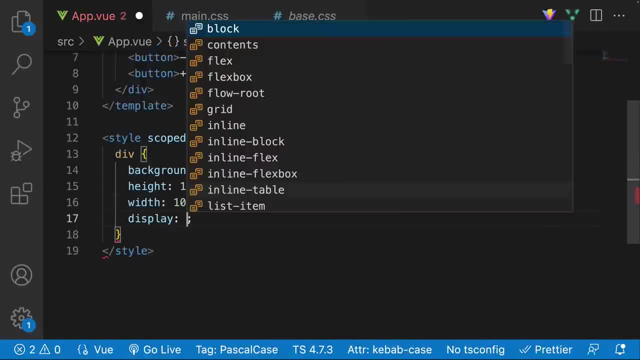 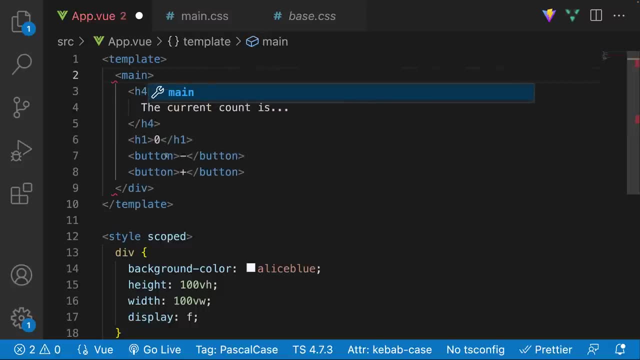 So let's just give it a display of flex. And actually we're going to need to kind of, let's actually wrap this inside of a main tag like so. So main. 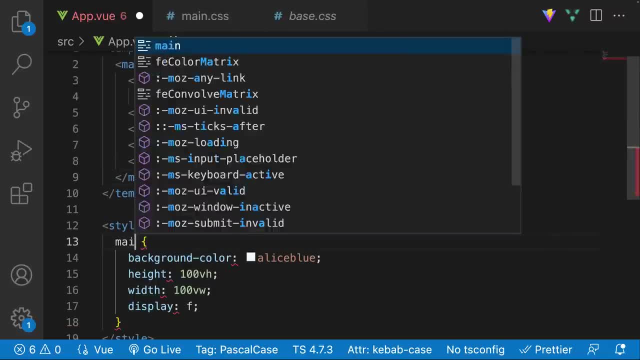 And over here, let's wrap this with a main as well. Okay. 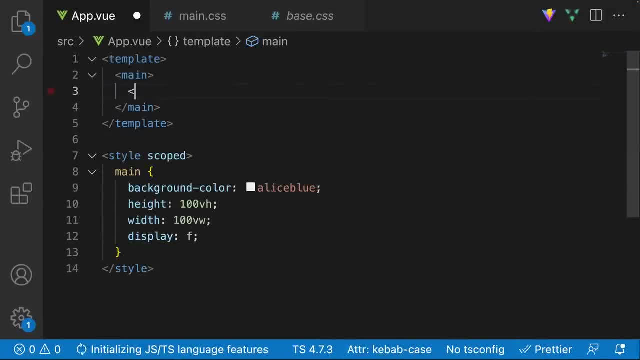 And then over here, we can wrap everything inside of the main with a div like so. There we go. Okay. 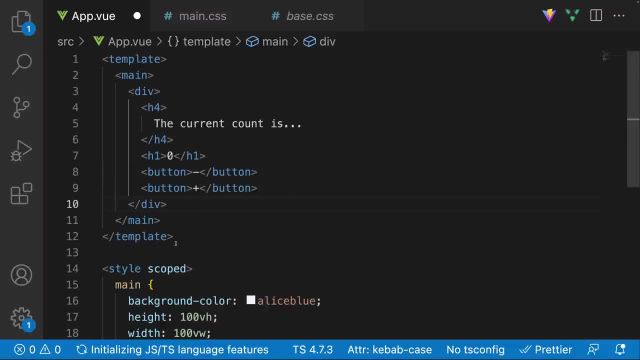 So now that we got that out of the way, and by the way, if you don't have any syntax highlighting, just like I told you to do in the beginning of the, or the introduction, 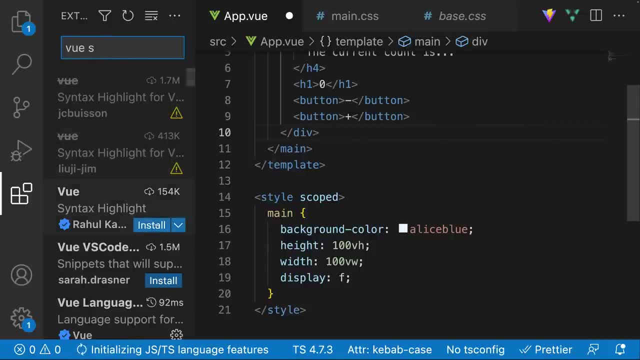 just go to view syntax and install this right over here, which is going to go ahead 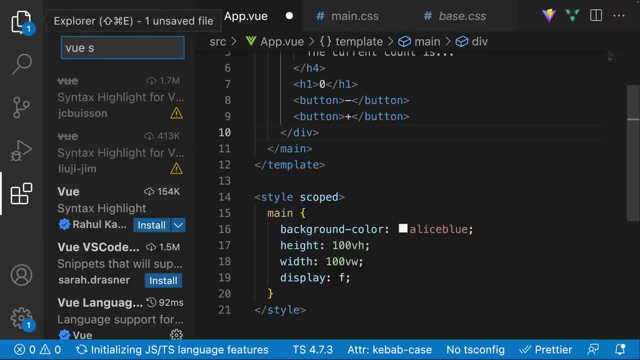 and we'll give you some syntax highlighting for your view file. Okay. So let's go ahead and save that. 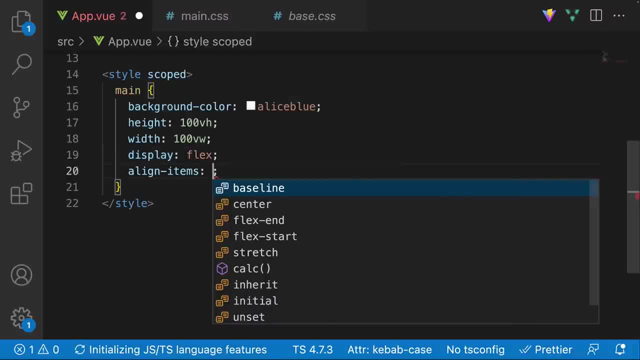 And then over here, we're going to do a display flex, align items center, justify content center. So we can get things right and centered. Looking good. 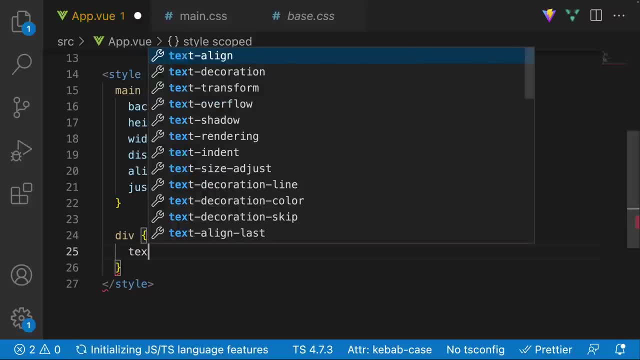 All is left to do now is to style the div and just give it a text align of center. And there we go. 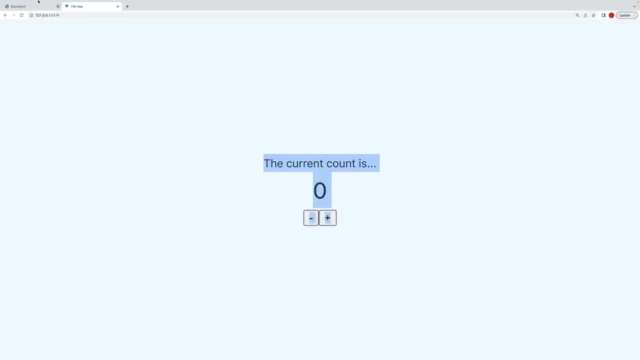 So now, it is, you know, the font's a little bit different, but that's okay. 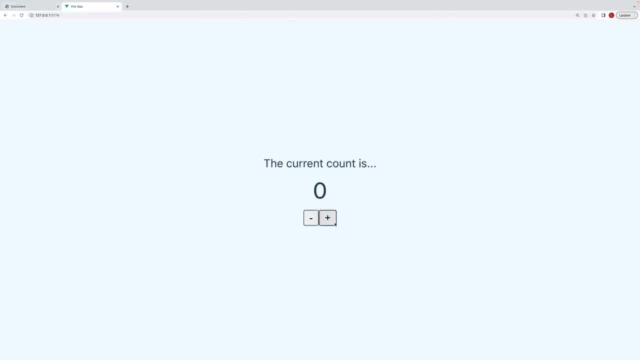 But you can see here that it is, at least stylistically, extremely similar. 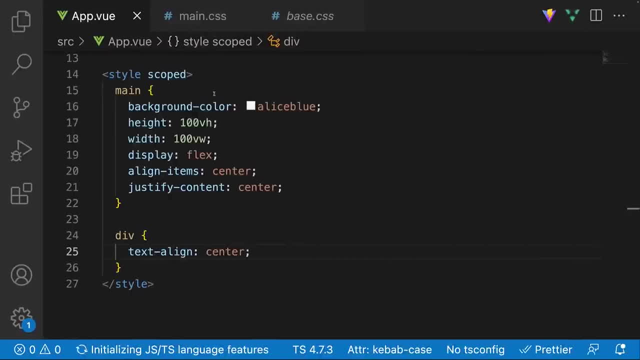 Now, what we want to do is we want to make it functional. And remember, this was the part that, well, took the longest with the JavaScript. 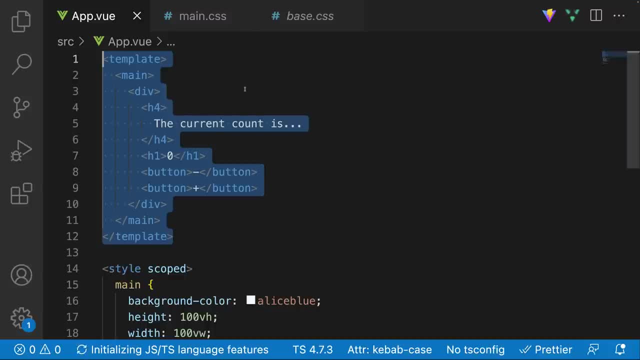 So let's actually see how long this takes with pure view JS. 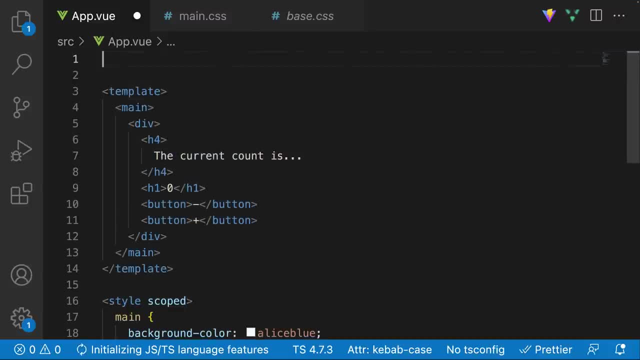 So what we're going to do is we're going to add right above this, we're going to add script tags. And this is where our JavaScript is going to live. 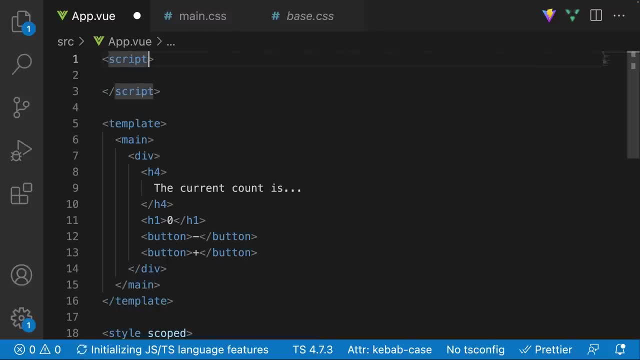 So still inside of the app.view. And then just like we did with the styled, we're going to have another keyword called setup. Now, again, I'm going extremely fast here. I'm not really explaining what's going on. Do not worry. 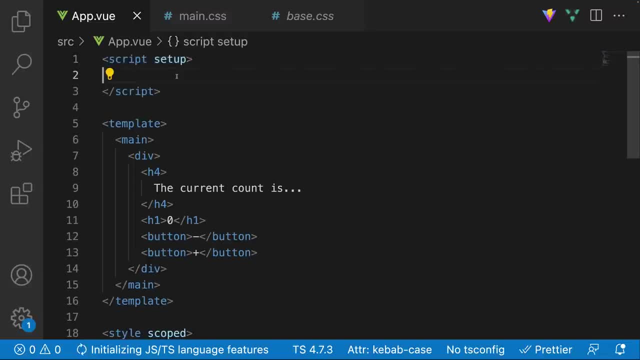 We're just coding this out just for the comparison. We'll talk about exactly what everything is a little bit later. So we have our script tag. 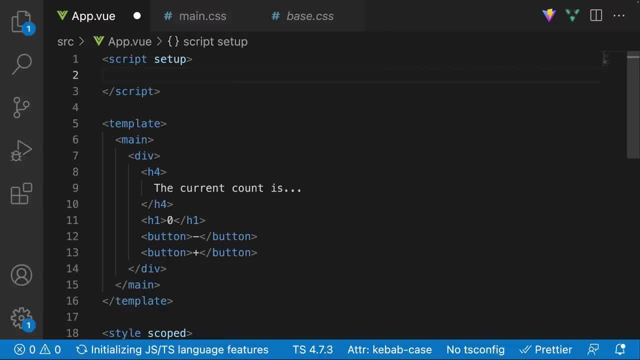 We have set up right over here. The first thing that I'm going to do is I am going to declare my, uh, state or my variable, which is this right over here. So the count. So I'm going to say const count is equal to zero, but I'm not going to declare it just like this. 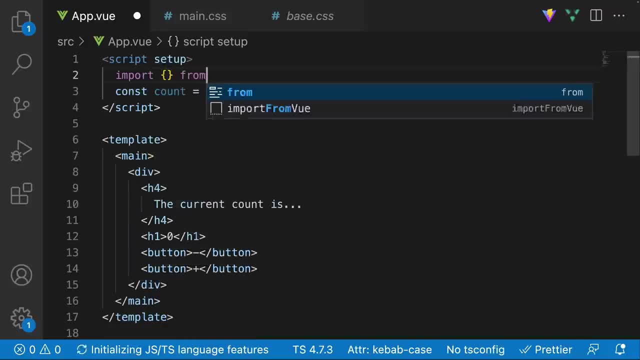 Instead, what I'm going to do is I'm going to import something from view. Again, I, each time I go through these things, I, I feel the need to explain this doesn't make sense. A okay. 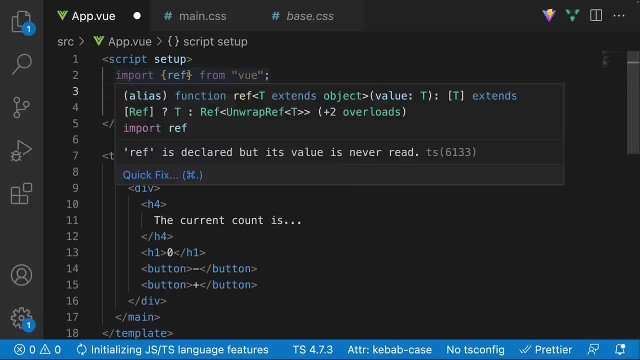 We're going through this really fast for a reason. So over here we have, 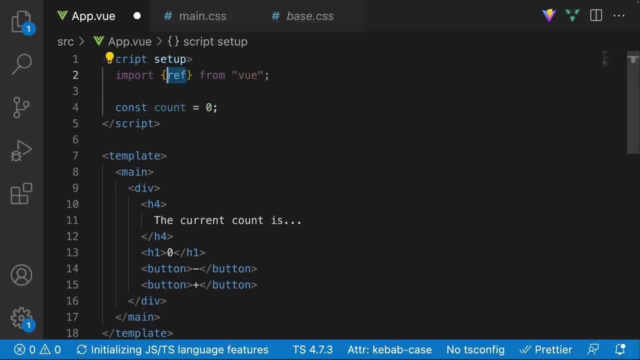 we're importing this thing called ref from view. And we're going to say, what we're doing is instead of having it like zero, like, so I'm going to say ref, 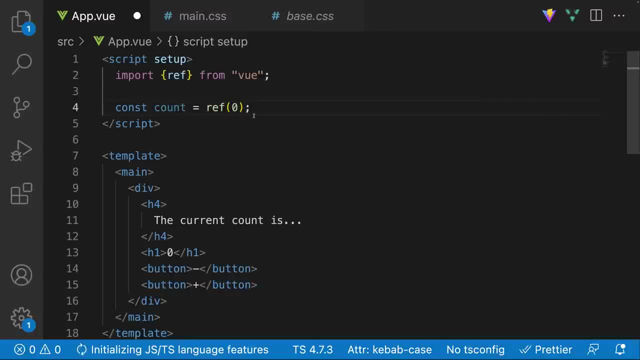 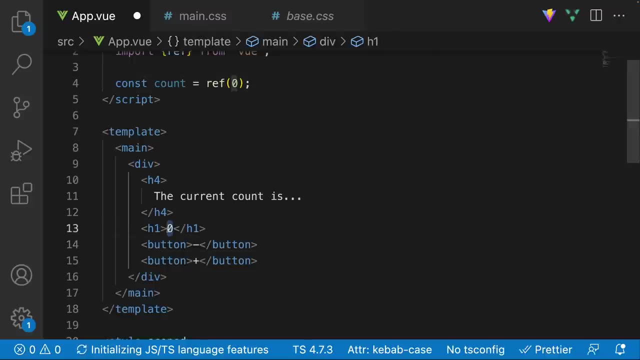 invoke it and then have zero in there. And then in order to actually use it inside of my H one, what I'm going to do is I am going to get rid of this zero. 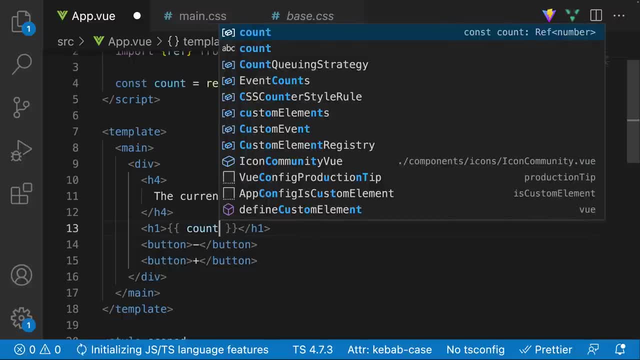 And then I'm going to do two curly braces. And then in here, I'm going to say count. I'm going to go ahead and save that. 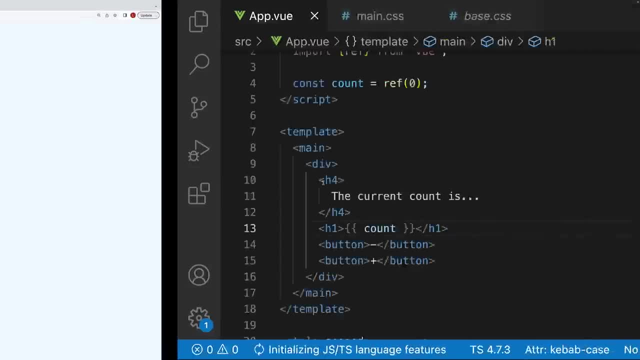 And you can see that the count is working a okay. Now, 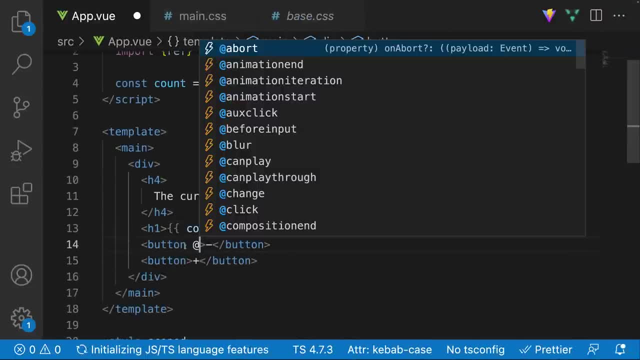 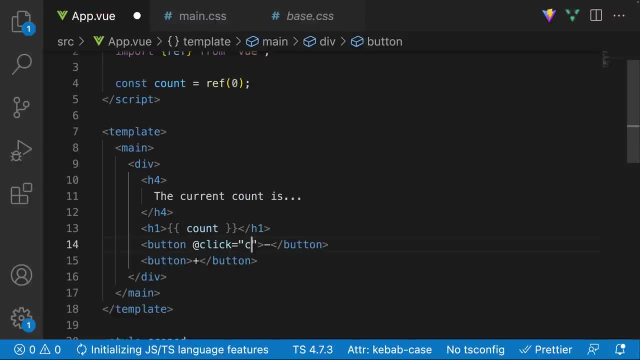 what I'm going to do is I'm going to go over here to the buttons and then very simply, I'm going to add an act, click, and I'm going to say that this is going to be equal to, and then count minus minus. 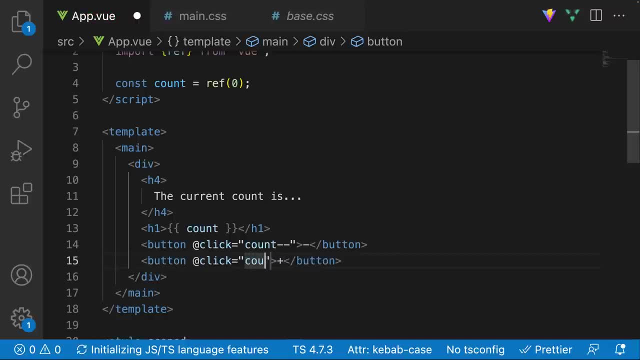 And similarly over here, I'm going to say, click, and I'm going to say count plus plus. 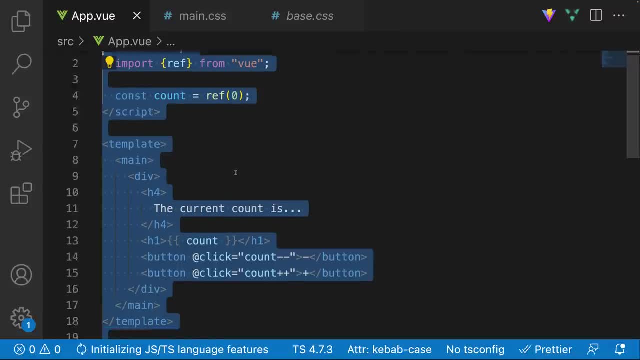 And there we go. We are completely done. Believe it or not. 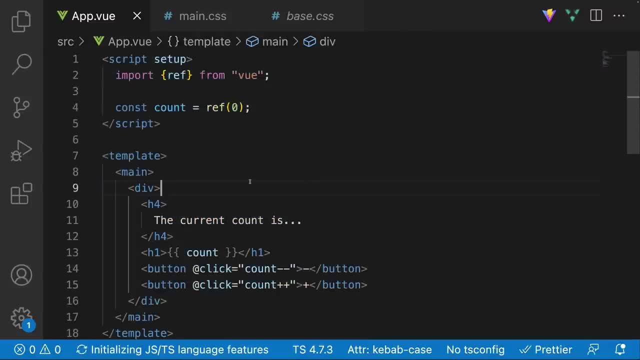 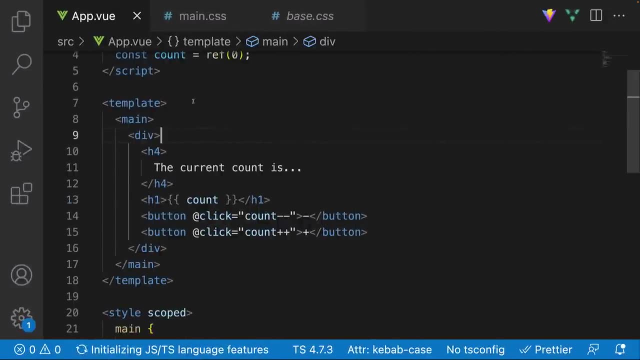 This is all it is that we need to do to get the exact same application working inside of view. Js just, just for a quick second, look at the JavaScript that we wrote. 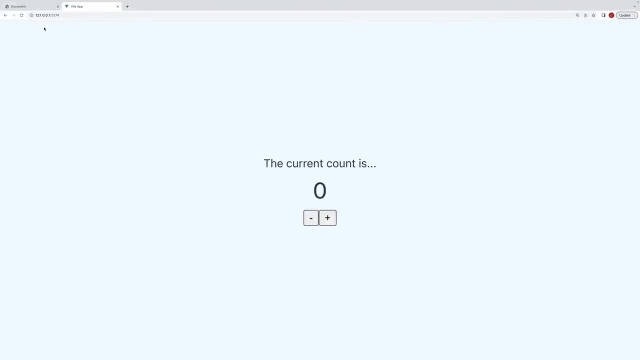 This is all the JavaScript that we wrote compared to what we had before, which again, we'll do a little bit later, but to prove to you that it works, look at that. There we go. 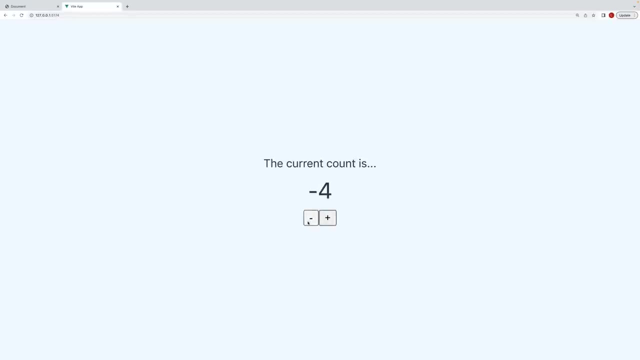 It is working a okay. How terrific is that? All right. 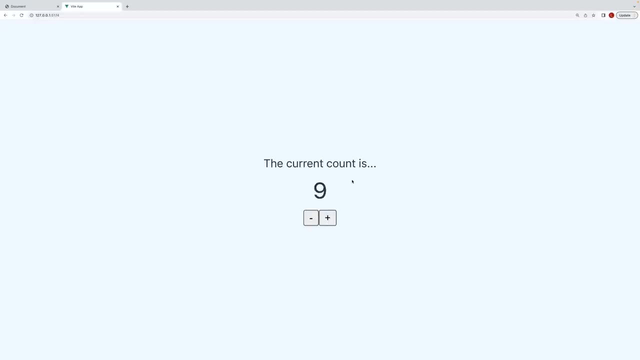 So now that we got that done with view Js in the next video, let's just compare what we did with vanilla Js versus what we did with view Js. 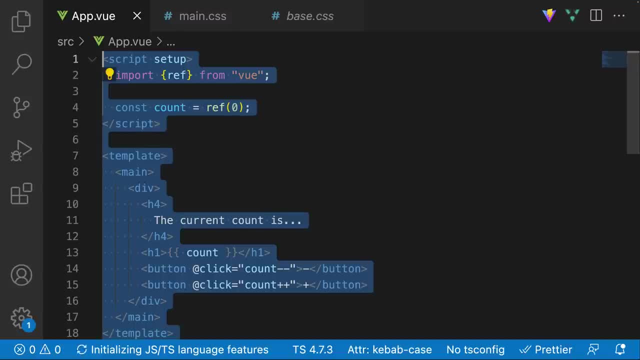 And hopefully you can actually see the benefits of using an application like view. Okay. 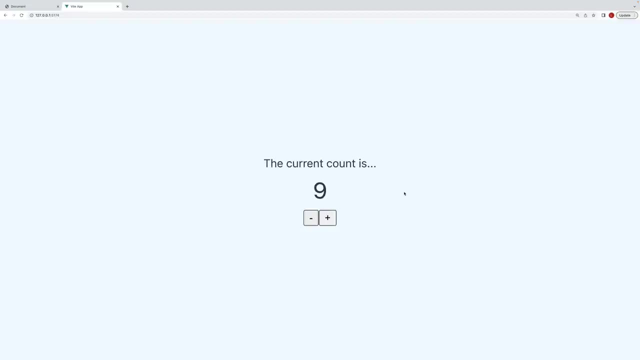 So now that we finally built our view application, let's now compare and contrast what we did when we built it with vanilla Js versus what we did when we built it with view Js. 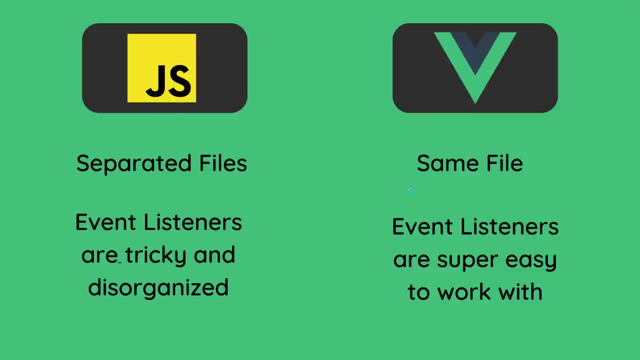 So there are actually two main things that I can quickly point to that just makes development in view significantly easier. So when we built it with vanilla Js, 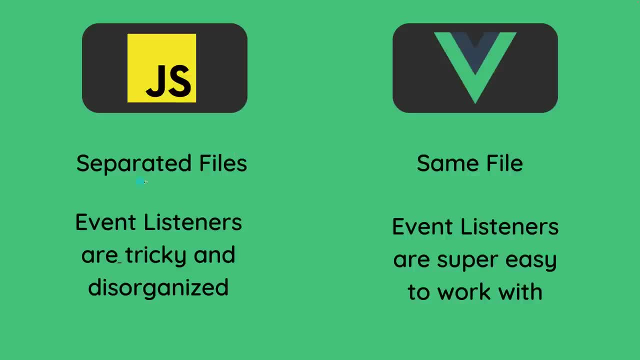 we didn't have to, but it is ideal and it is also a best practice to separate your files. 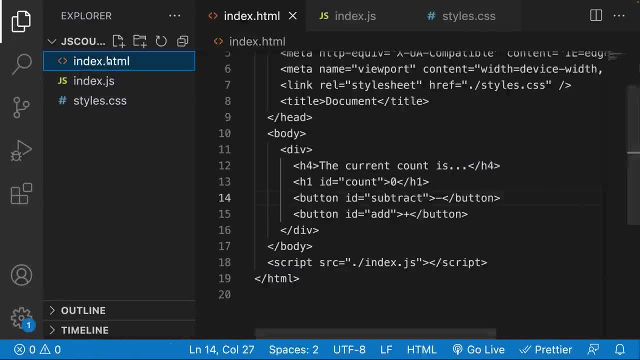 So we had to have separate files for the HTML, the Js and the CSS, and then we had to link them together to have them work together. 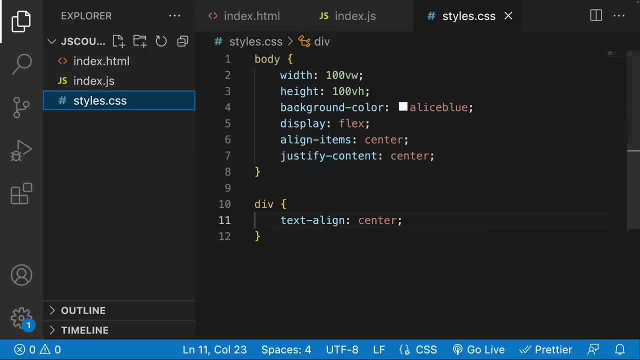 So this is something that we had to do. However, 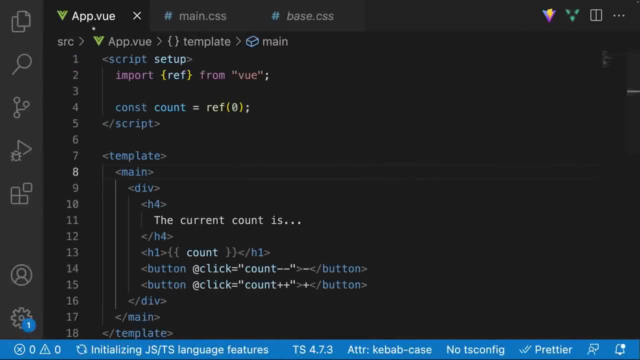 this is something that we actually did not have to do when dealing with view Js, because with view Js, we only had this one app dot view file. 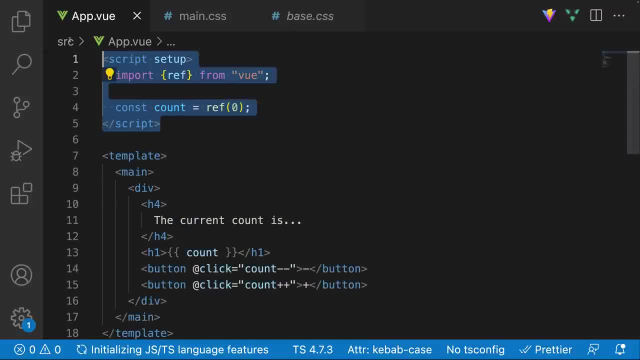 And as you can see, very simply, we had our script, which is our JavaScript. 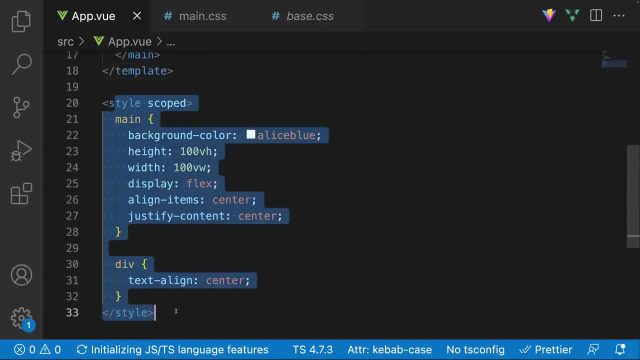 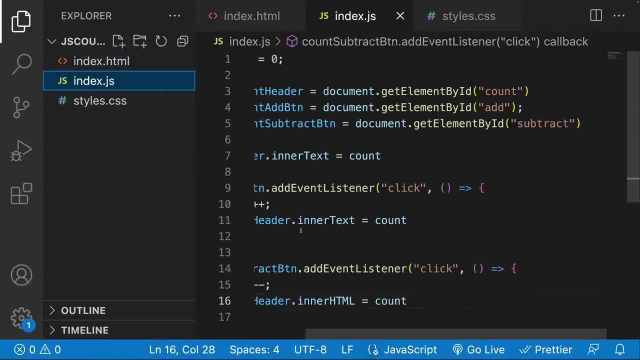 We had our HTML and we had our CSS so we can quickly modify anything that is needed. Whereas we over here, we had to go find the file, find the link that is attached to, et cetera, et cetera. So you can see that this is not the best approach. 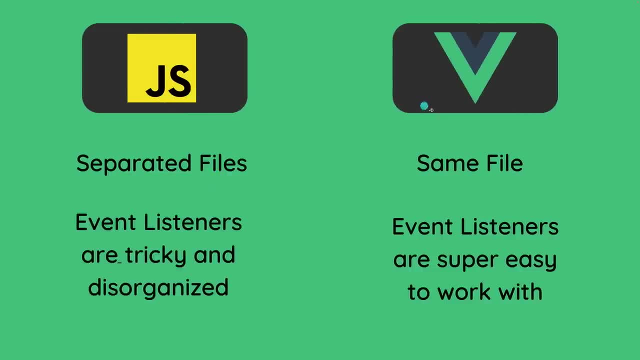 The second thing that I found that was way more confusing, convenient with view Js are event listeners. 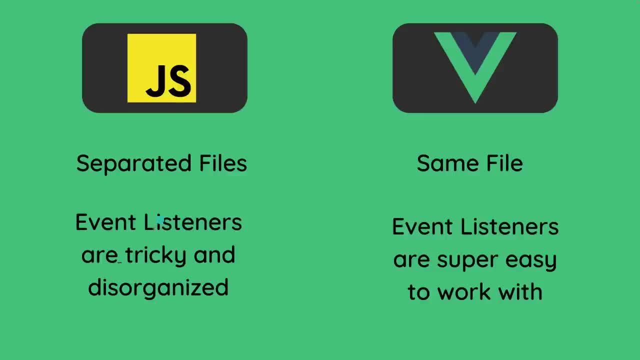 So with JavaScript, event listeners are actually pretty tricky and they can get pretty disorganized because over here, 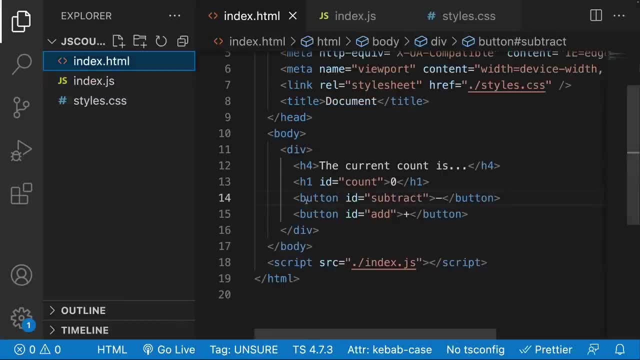 if you go back to our JavaScript application, let's say we wanted to add a listener over here. 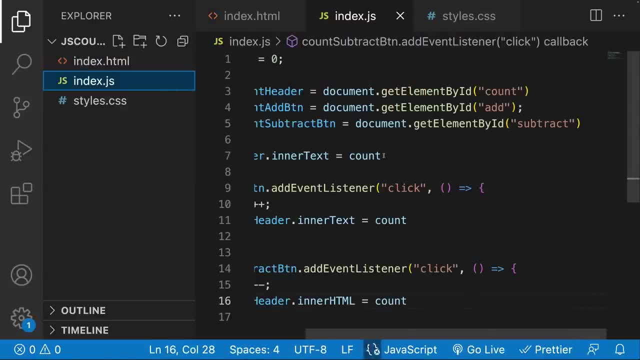 What we had to do was add an ID. Then over here, we had to find the variable and then add event listener to it. 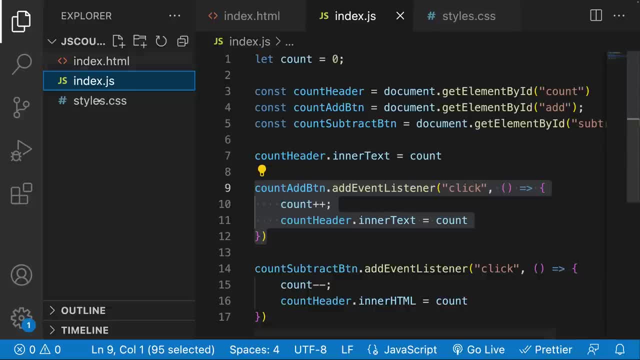 And now let's say that later on in our application, somebody was like, Hey, for the ad button, add, you know, further logic. 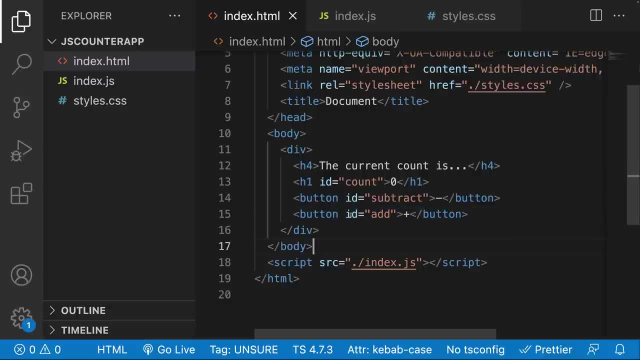 Well, in order to do that, I would have to go over here to the HTML. I would have to see, okay, this has an ID of ad. I then have to find the JavaScript file. 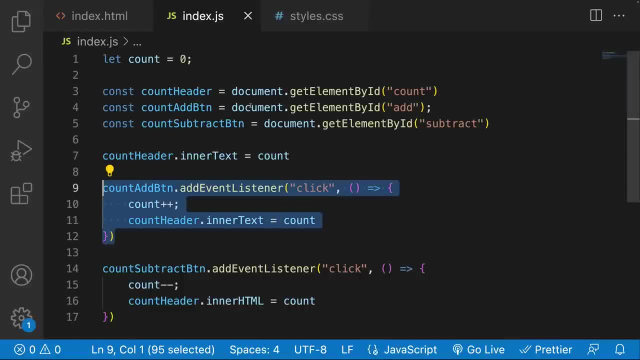 And then what I would have to do is, well, go over here, try to find the variable. Oh look, it's this one. 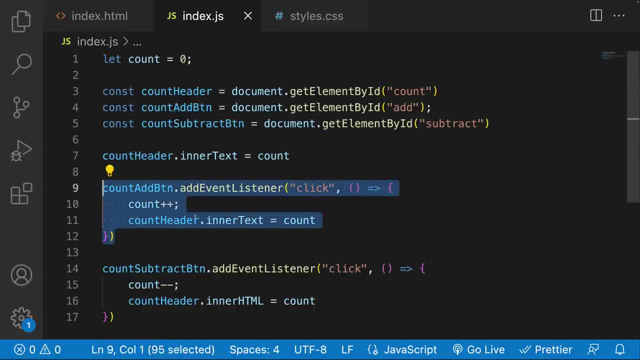 And then I would have to find the event listener and then I can change the callback. So this is kind of tedious and is pretty disorganized to be honest. Whereas with view, it is far, far simpler. 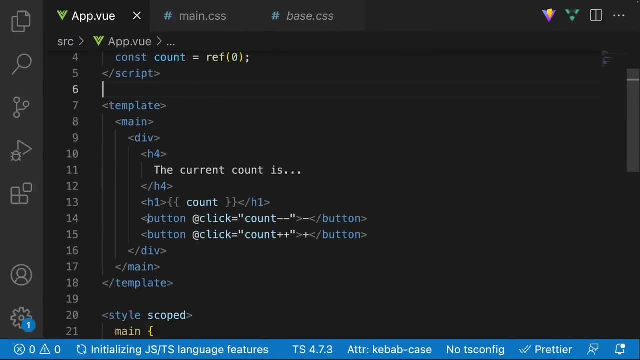 The event listeners are actually attached to the HTML elements themselves. So you can see here, right over here, this is the ad button. 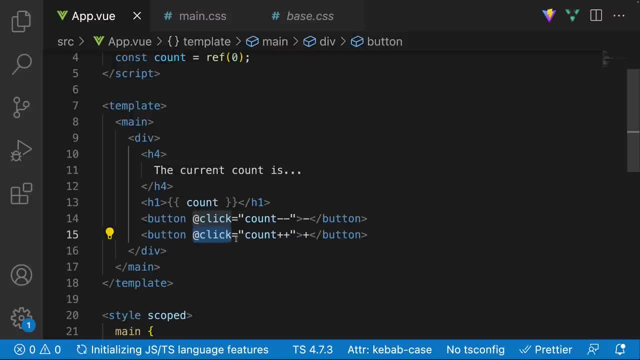 Oh, I just found it. Oh, here's the event listener. 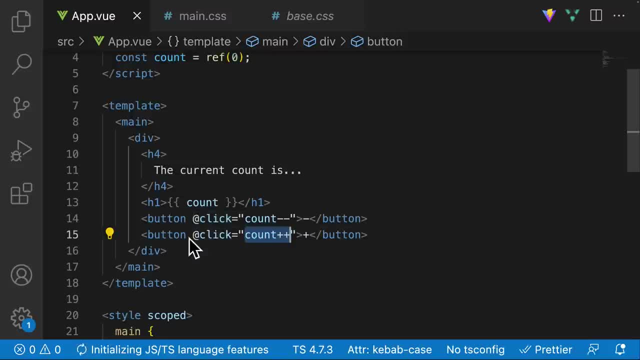 And Oh, here's the function that is being called, or here's the logic that is being called when this button is being pressed. So I can go ahead and update it. 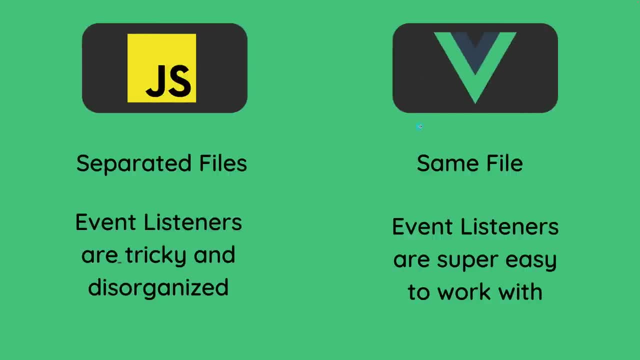 So at the end of the day, view JS just makes developing web applications, far, far, far simpler. That's pretty much all it is. 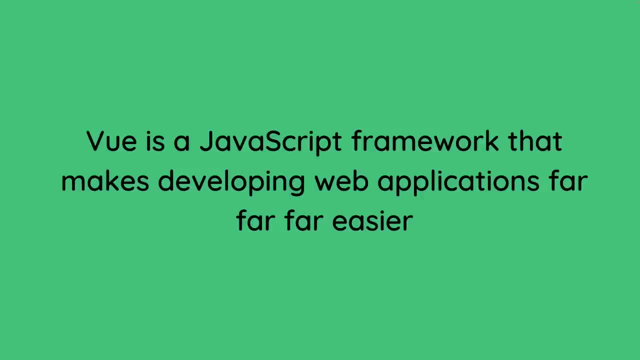 View is a JavaScript framework. So it is built off of JavaScript. It is a tool that we can utilize that just makes developing web applications just significantly easier than building with vanilla JS. Now, at the end of the day, we can always accomplish the same thing with vanilla JS and view. View doesn't have some sort of magic power that we can actually do something that we can't do. Something that we cannot accomplish with vanilla JS. 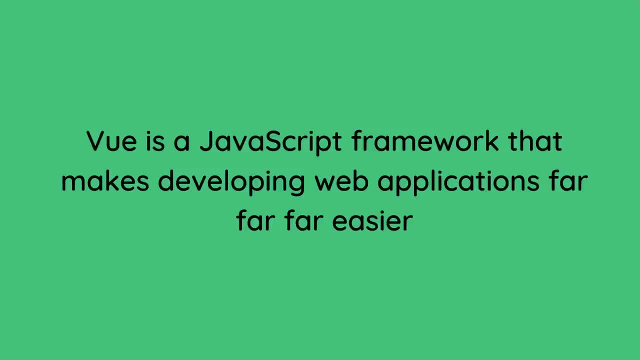 But trust me, especially with more complicated applications, an application that might take, I don't know, 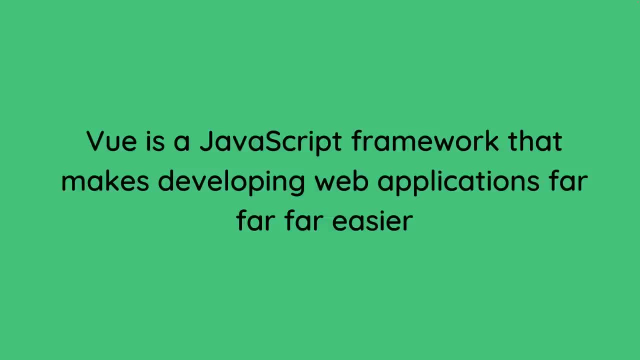 view five hours to build will probably take vanilla JS, maybe something like 50 hours to build. 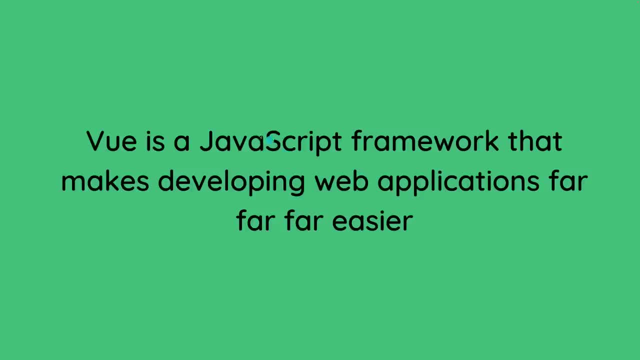 I promise you, this is why view is significantly better. 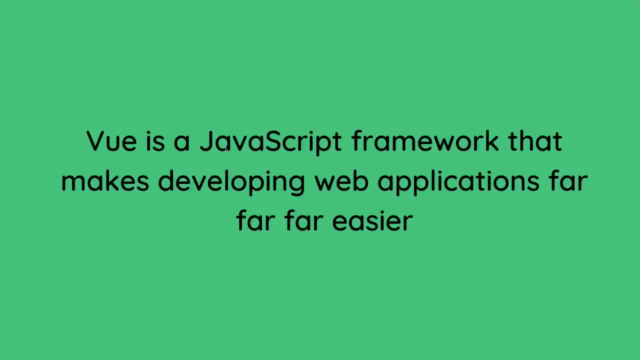 But again, at the end of the day, we can accomplish the exact same thing with view as well as vanilla JS. 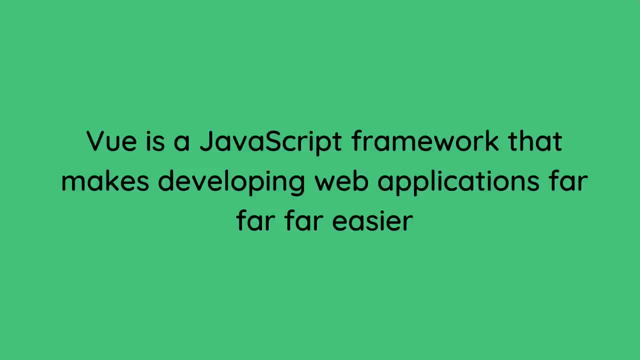 So hopefully, now you have an idea of what view is. 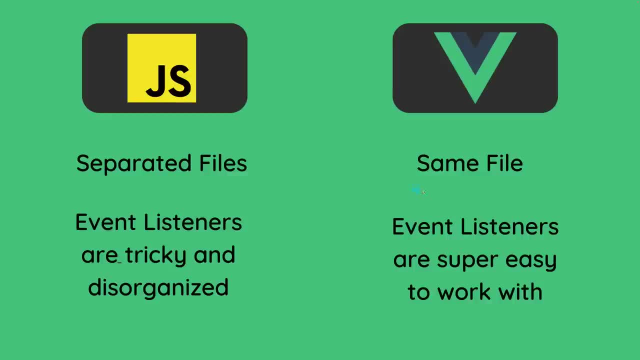 And these comparisons right over here, they're just scratching the surface. 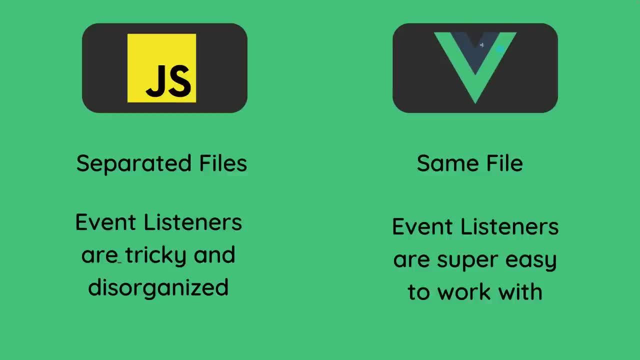 There's so many more things that view JS does as a convenience. Whereas with JS, it's just going to be such a pain to do. 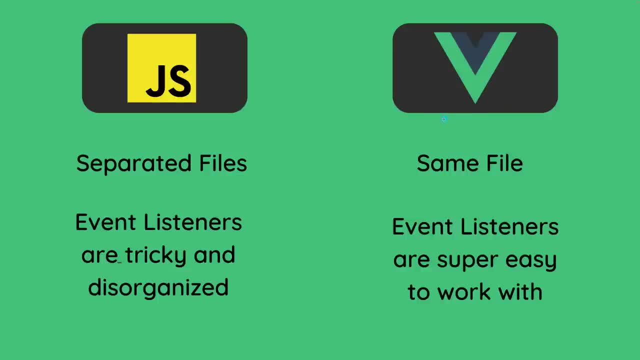 Now, for example, routing is something that view makes super, super easy. 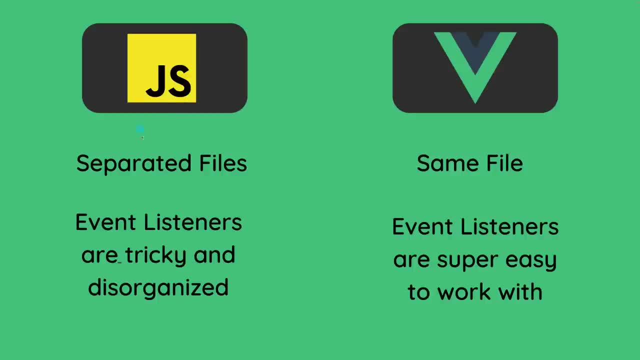 But with JavaScript, with pure vanilla JavaScript, it is a huge pain to configure. 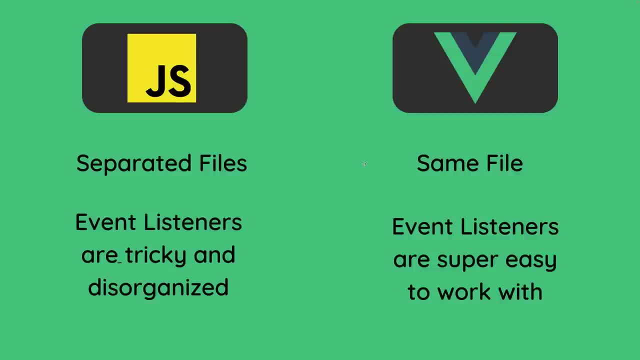 But we'll see all of the different benefits and I'll mention them as we go. Throughout this course. 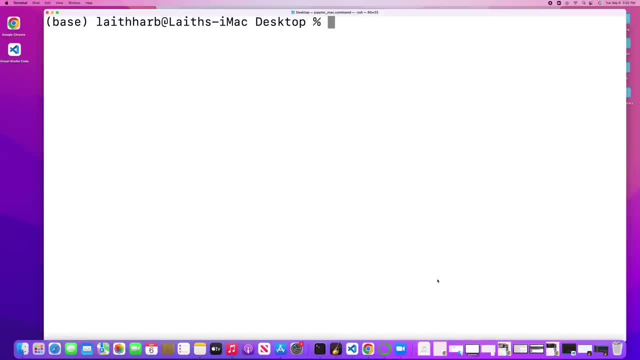 All right, everybody in the last section, we created our very first view application. 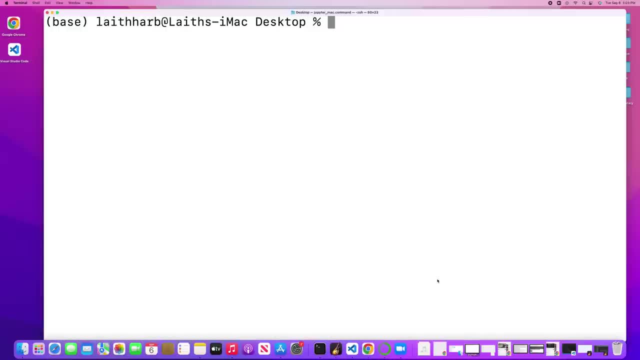 However, we didn't really go through what we wrote or why we did things or how things work. 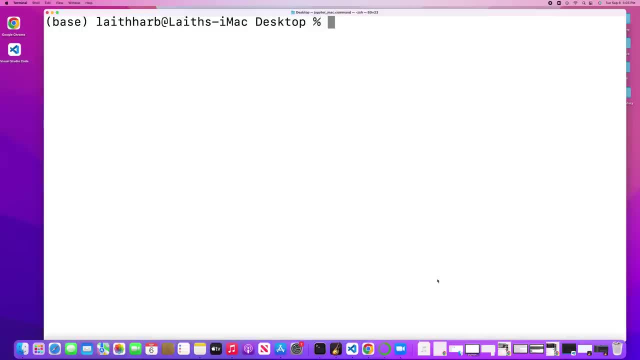 So in this section, what we're going to do is replicate that counter application, but we're going to go through every little step that we do in tremendous detail. 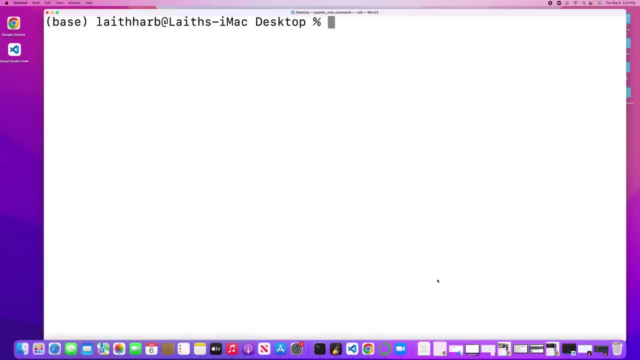 So by the end of this section, you should have a vast understanding of the application, that we just built. All right. 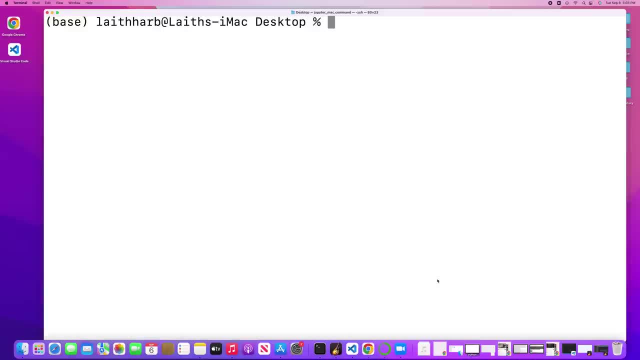 So the first thing that we need to do is to close the terminal that is currently running our legacy, our old counter application. 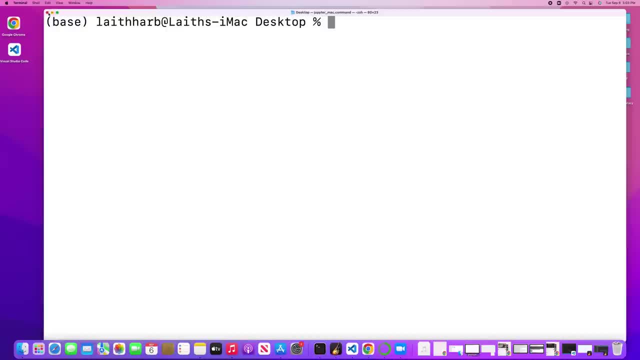 So just go to that terminal window and then just go and click close. I actually already did this. 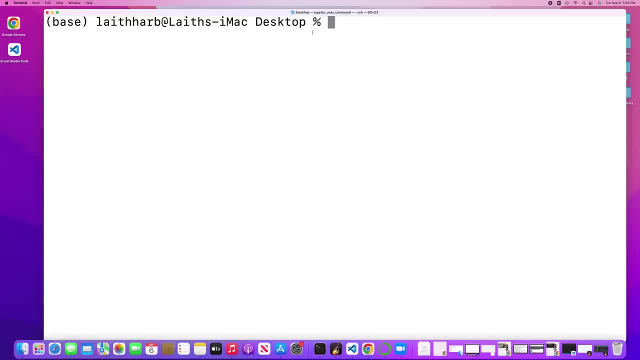 And what I also did is I opened up a new terminal window and I moved to the desktop directory. And this is where I want to create or recreate the new to do counter application. So let's go ahead and do that. So we're going to do an NPM in it. And then we're going to say view at latest. And of course, it's going to ask us a few questions. 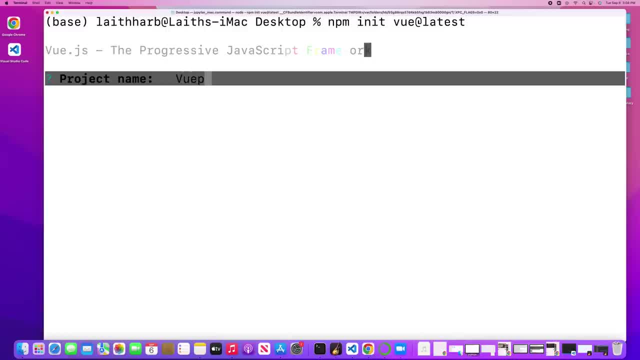 First question is the project name. I'll call this view counter. 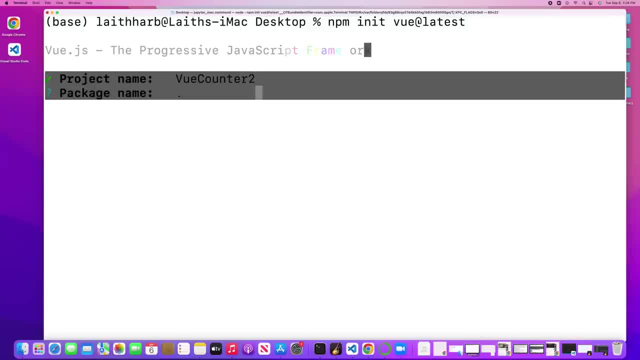 I'm going to call this view counter two and the package name. I'll just leave as is and everything else. I'll just say no. All right. 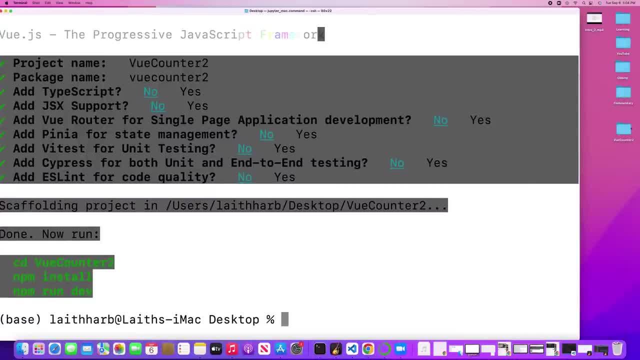 So this is going to create this new application inside. Of my desktop directory. Of course, we can go ahead and actually go to V.S. Code. So let's go open this up in V.S. 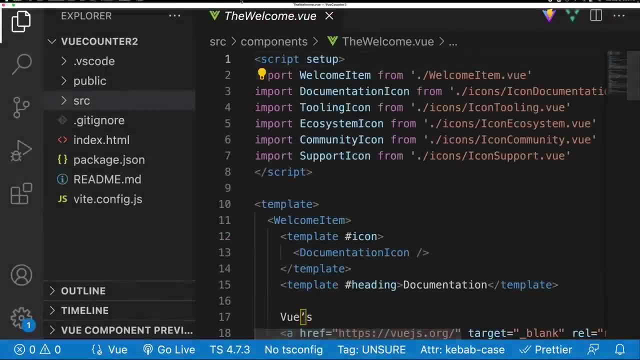 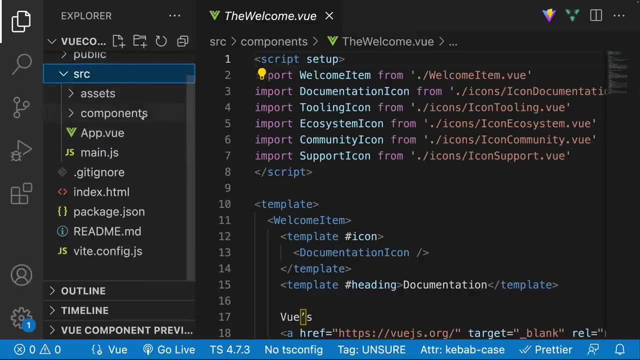 Code so we can actually see the code itself. So I click open. And as you can see here, we have all of the code. And this should be relatively familiar. Over here, we have our app dot view with all of the different boilerplates. 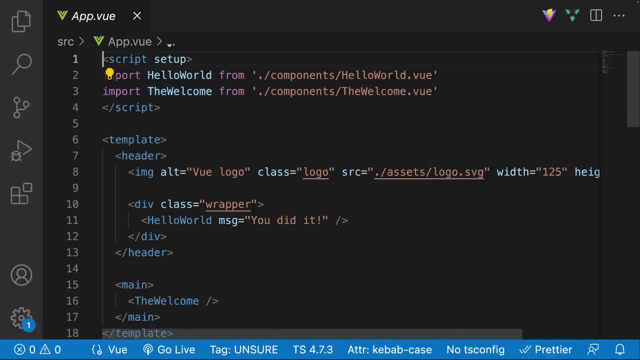 Okay. So what do we need to do in order to actually get this application? 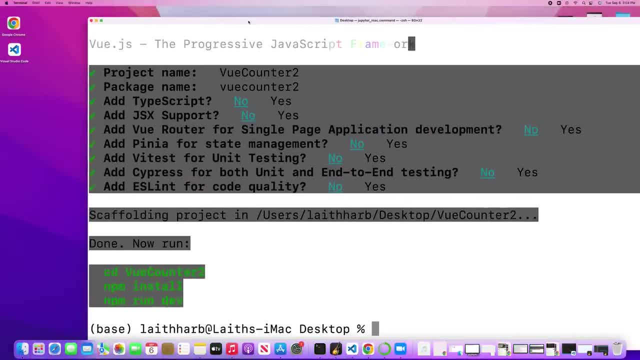 Up and running on our machines? Well, over here, the steps are, well, move into the view counter to directory. So move into that directory and then do an NPM install and then an NPM run dev. 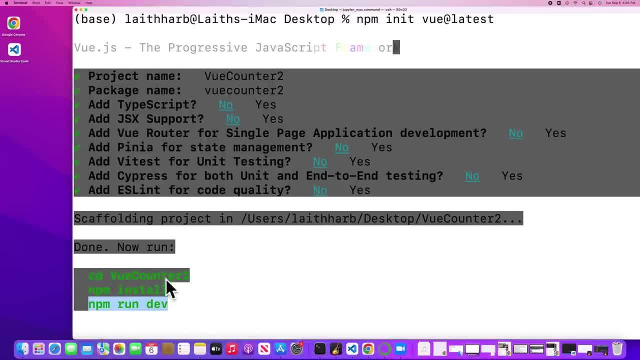 So in the last section, we just quickly did these without really understanding exactly what they do. Well, not in this section. In this section, we're going to understand again every little thing that we do. 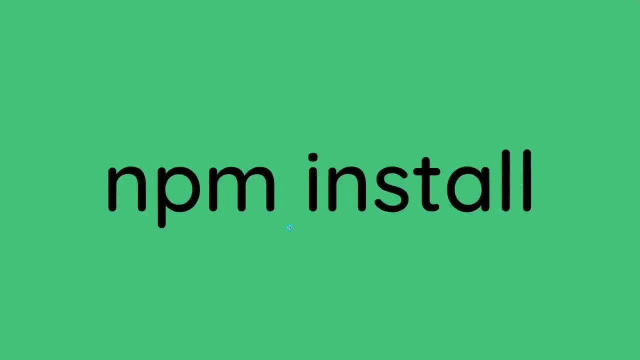 And we're going to begin with NPM. NPM install. So what is NPM install? 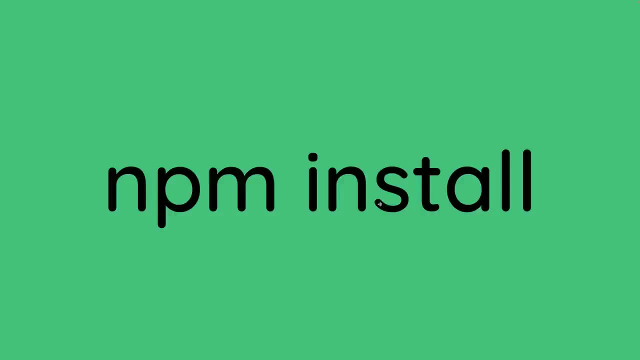 Well, when we created our view application, we have a situation that looks something like this. 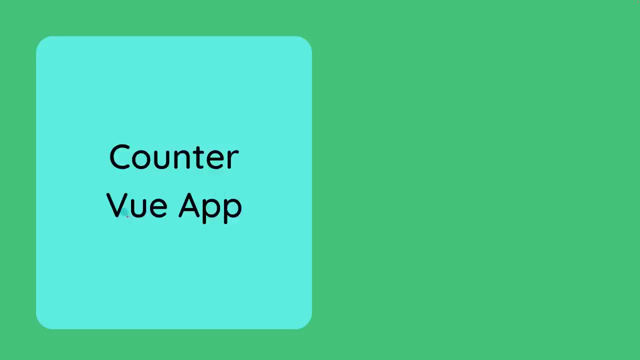 So we have our view counter application. And this is basically the boilerplate application. And it has a bunch of different code within this application itself. However, 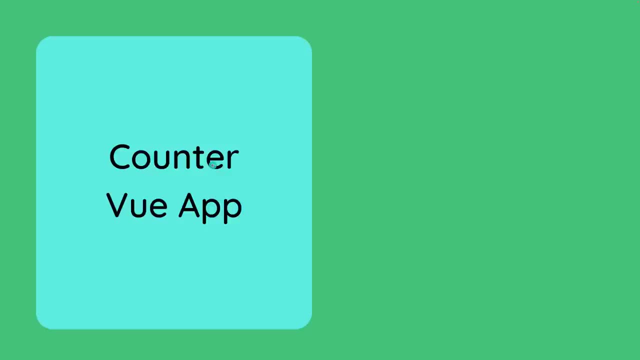 this code is not the only code that we need. In order to run our application. So for example, 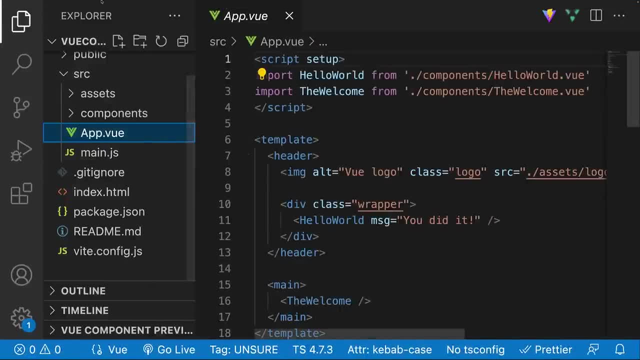 I'm going to go over here to my VS code and I'm going to open up the integrated terminal. So this is just going to open up a terminal similar to this. 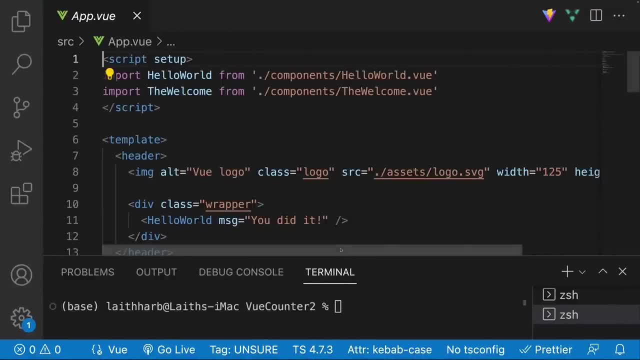 But this time is going to be in that exact directory. And what I'm going to do is I'm going to skip the NPM install step. 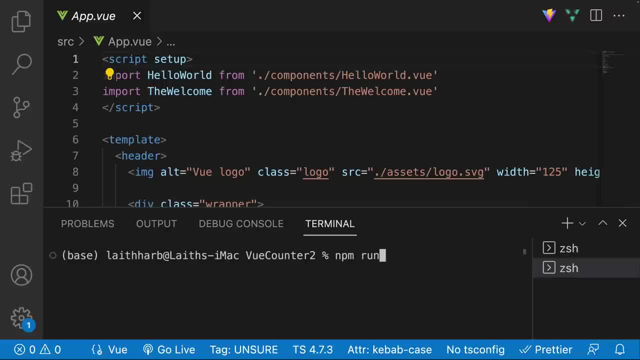 And I'm going to run NPM run dev. 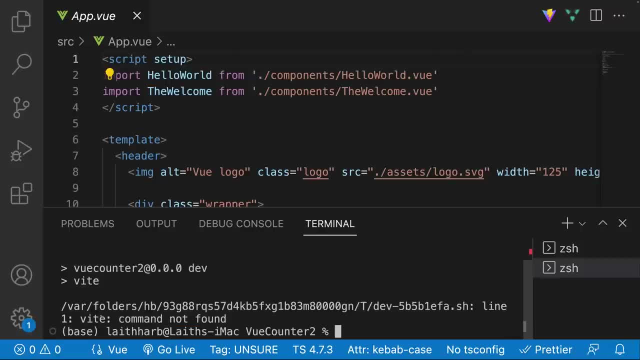 Now, as soon as I run that, it actually gives me this error right over here, saying, Veet is not found. So what is going on here? Well, Veet is actually a package that lives in the node package manager. 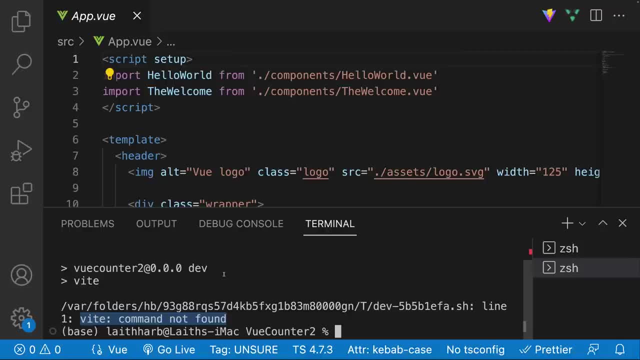 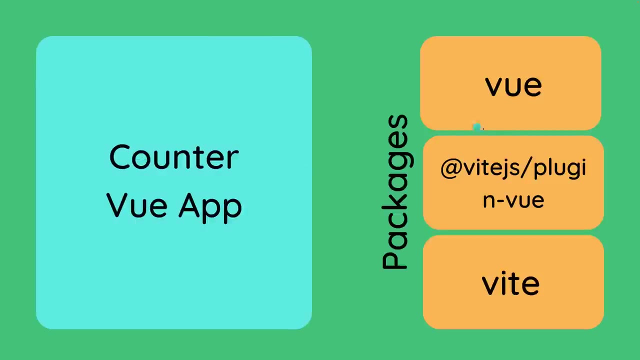 And it is some third party code somewhere all the way in the cloud that we need access to. And we need to bring into this application over here. And in fact, we actually don't need just Veet. We need three other packages. We need a package called view. We also need a package called at VJS slash plugin view. And of course, we also need Veet itself. 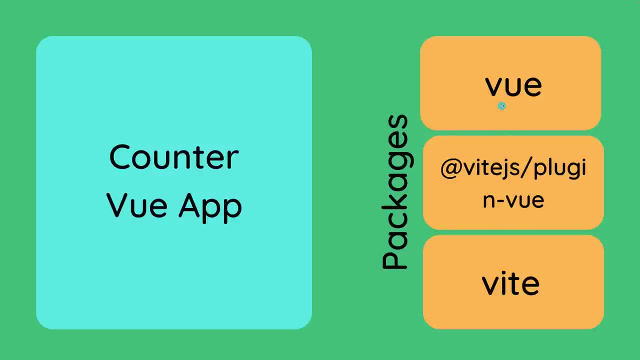 So all of these are third party packages, code pieces of code that somebody wrote and hosted into the cloud. And we need to bring those pieces of code into this application, into our counter application in order to run our application correctly. And that right there, 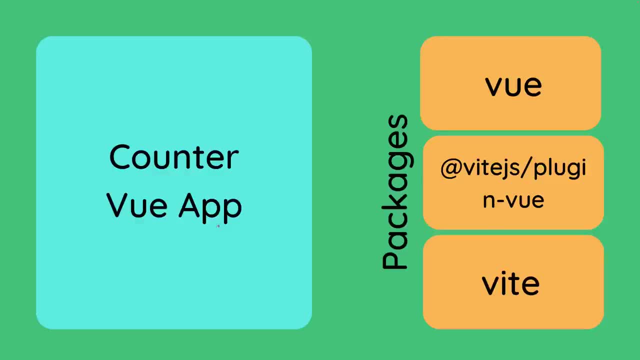 is exactly what NPM install is for. 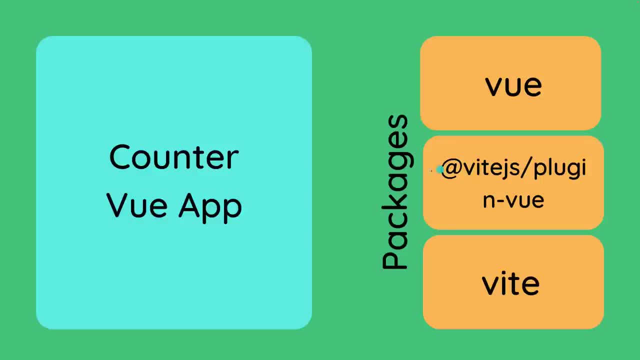 So we do NPM install to install all of these packages, all of the code associated to these packages into our local project. Now you might be thinking, 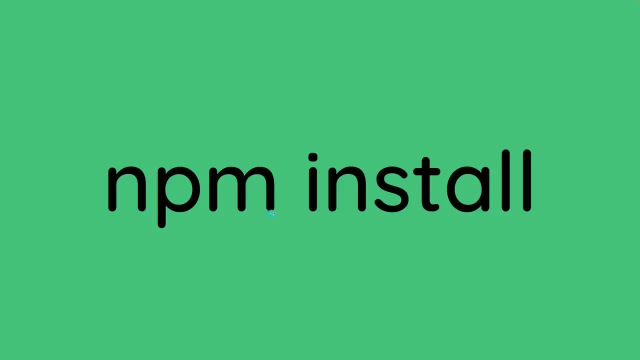 well, if I run NPM install, how is it going to know that, Hey, I need view. I need this. I need this. 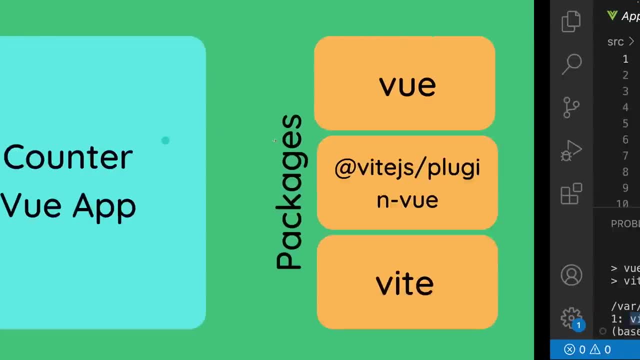 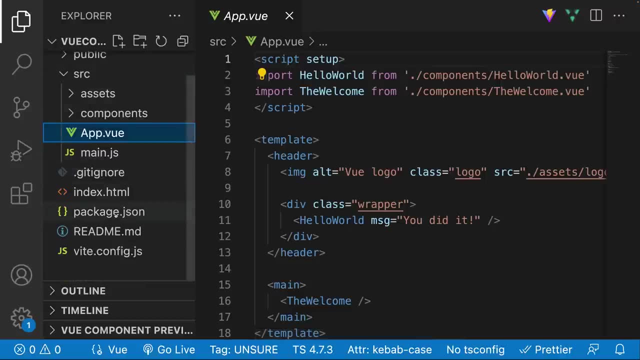 How does it know exactly what packages my application needs? Well, I'm going to go back to here. And what I'm going to do is I'm going to open this up. And then I'm going to go to the package dot JSON. And this here contains really all of the instructions for our application. Now there's a bunch of things going on here. 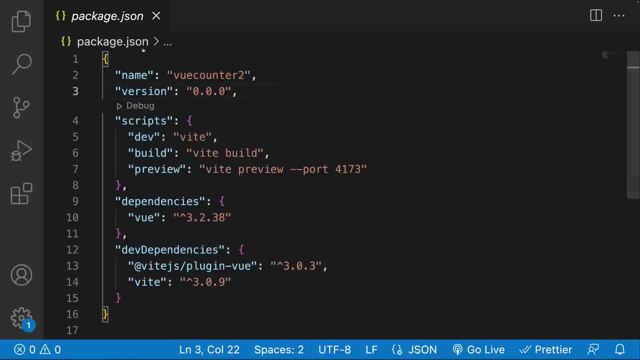 And of course this is in JSON format. So it's very similar to JavaScript objects, but everything is just wrapped in quotes. 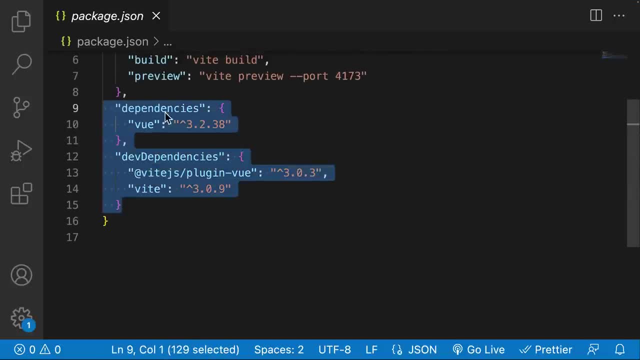 But right over here, you can see right here, we have dependencies. 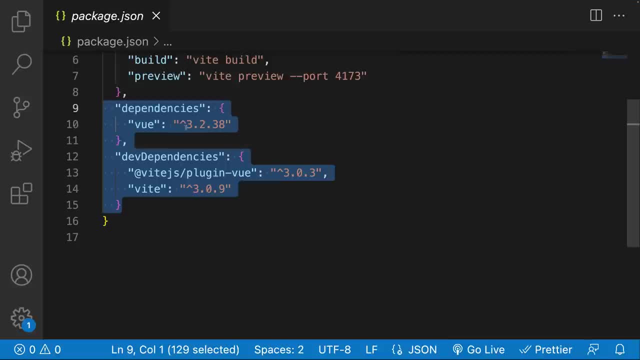 And then we also have dev dependencies. So dependencies, if you do not understand are in essence, things that our application or packages that our application are dependent on. 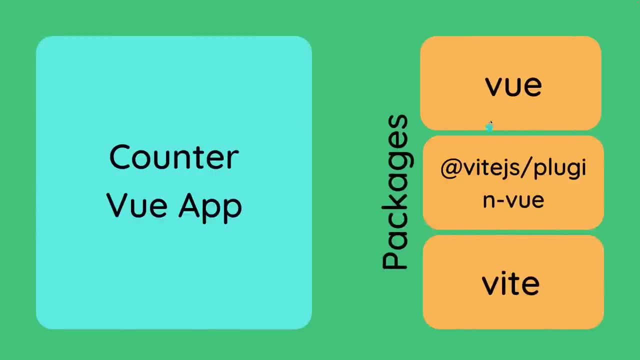 So these packages right over here are actually dependencies for our app. And we need to go ahead and install them in order to get our application up and running. 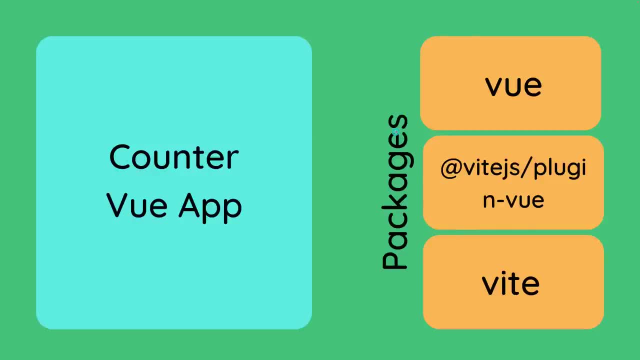 Our application is dependent on these packages. 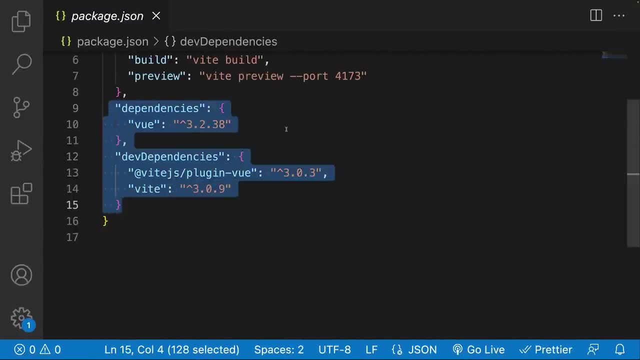 So right over here, we've actually listed all of the different dependencies that we need. 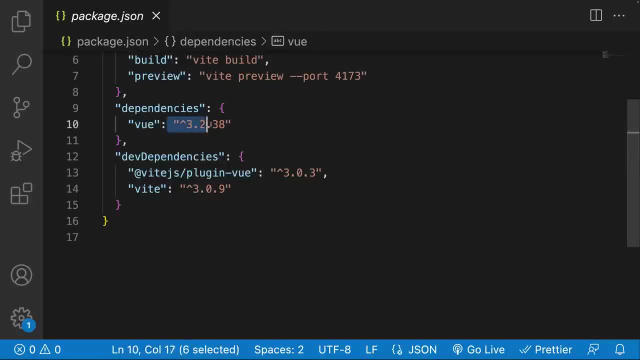 We need this right over here, this package at this version. 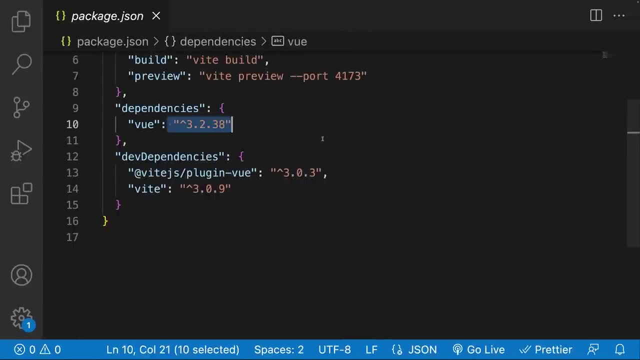 Over here, as you can see here, view, and then of course it's at this version right over here. 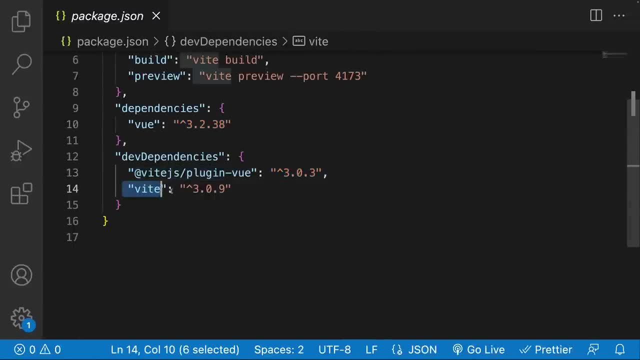 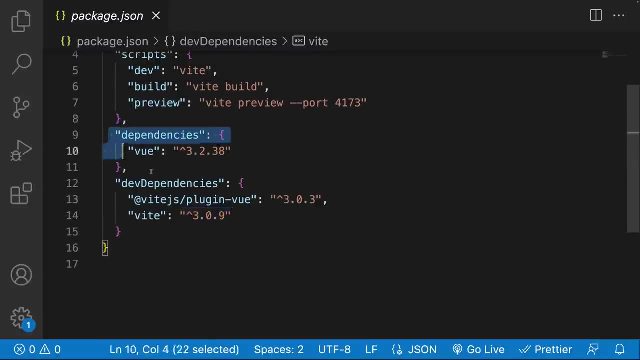 Now also we need this package at this version as well as this package at this version. So what npm install does is it looks at this package dot JSON file. It looks at all of the different dependencies, and it just goes ahead and installs them from, from the cloud onto our machine. So that is exactly what it does. Now you might be wondering what in the world is a dependency versus a dev dependency. They're both dependencies, but one is a dependency that is going to be needed in both development and production. 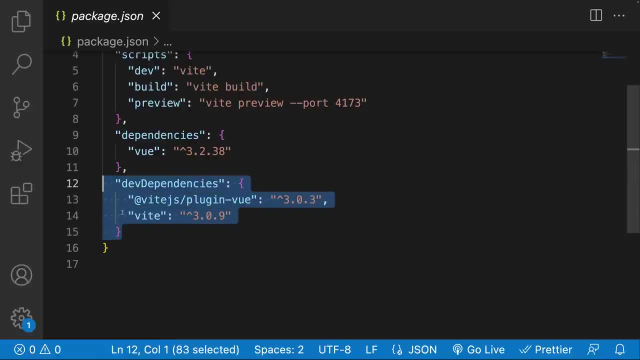 Whereas this one is just really a development dependency that we actually do not need in the prod environment. But that's not really something that we need to worry about at this moment. 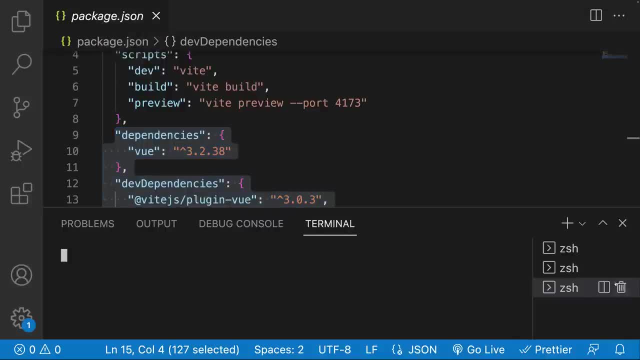 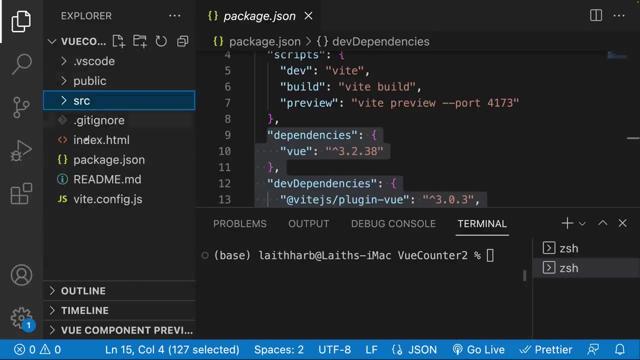 So let's actually go over here to the terminal, and I'm going to run npm install, and I want you to kind of notice something that occurs to all of the different directories inside of our app. So I'm going to do an npm install, and as I do this npm install, please keep a close eye right over here. So let's do this npm install, and okay. 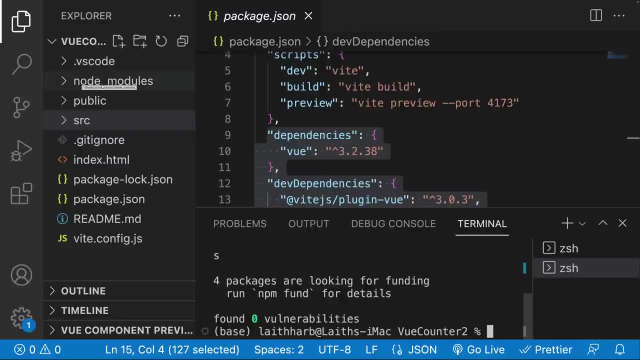 So if you noticed, right over here we have this new directory called node modules. So node modules, and you can see this, it has a bunch of different folders within it. But most notably, it has, well, this view folder. 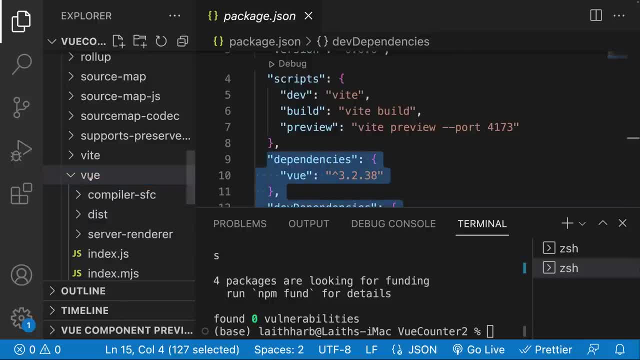 So right there, now we have the view code that we need in order to run our app. 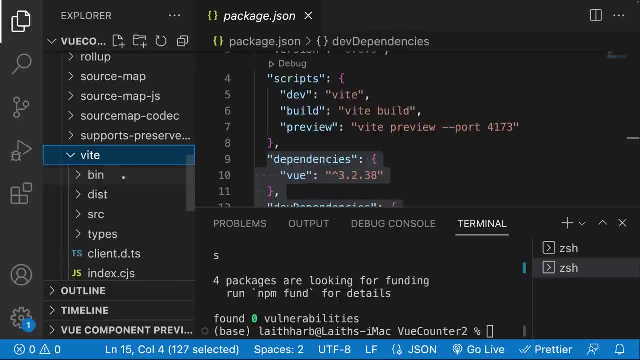 We also have Vite. So now we have all of the Vite code that we need to run our app. 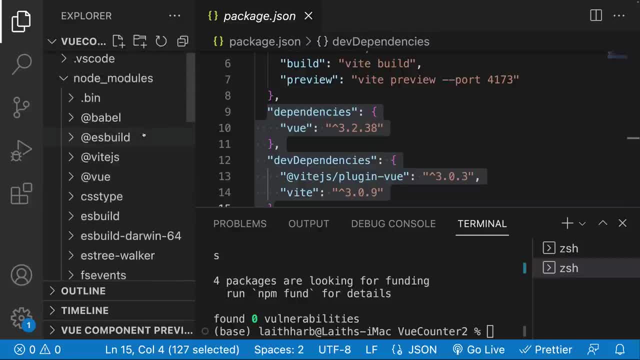 And if I were to scroll all the way up, we also should have at ViteJS plugin view. 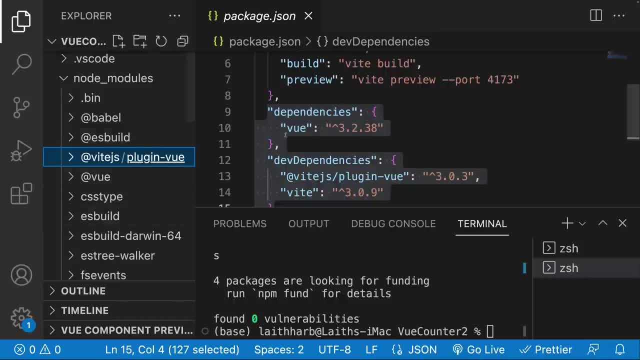 So now we have all of that to run our application correctly. 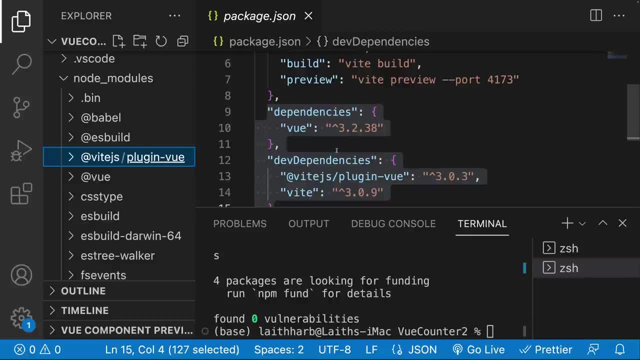 So now we managed to get all of that third party dependencies into our application. 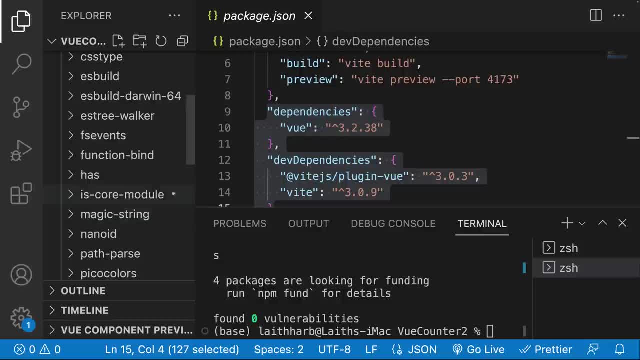 And you might be wondering, why in the world are there all these other things? 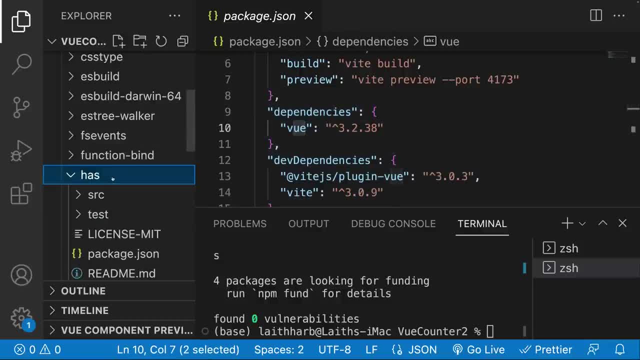 I only downloaded these three. Why do I have this package right over here or this package right over here? Well, 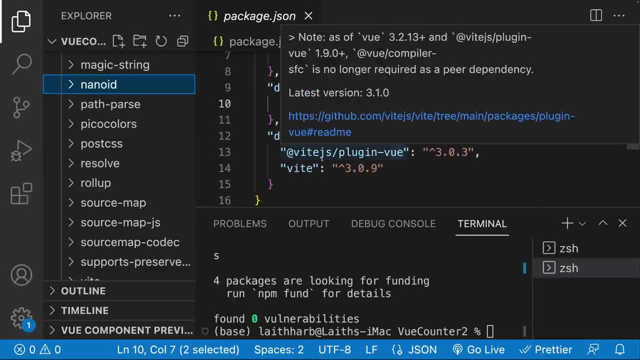 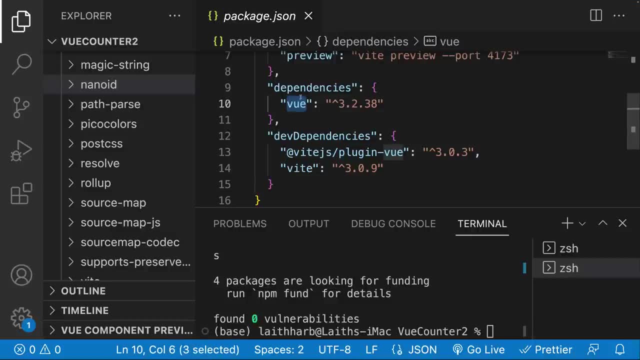 it just so happens that it is extremely common that dependencies also have dependencies of their own. So in order to run view, well, view might have some other packages that it is utilizing, 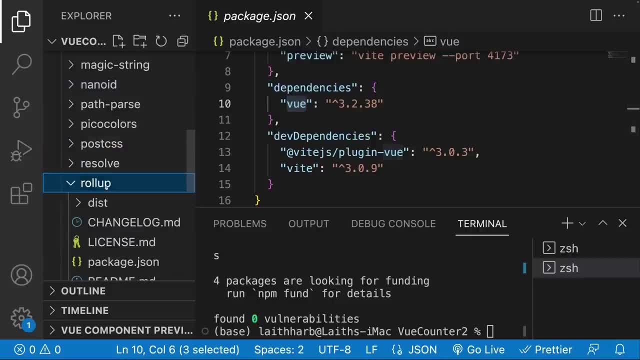 such as like, let's say post CSS or revolve or rollup. 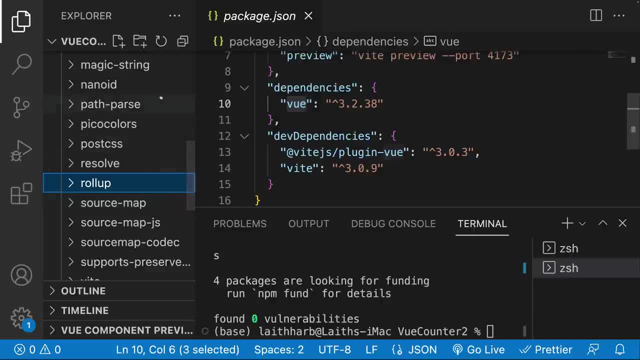 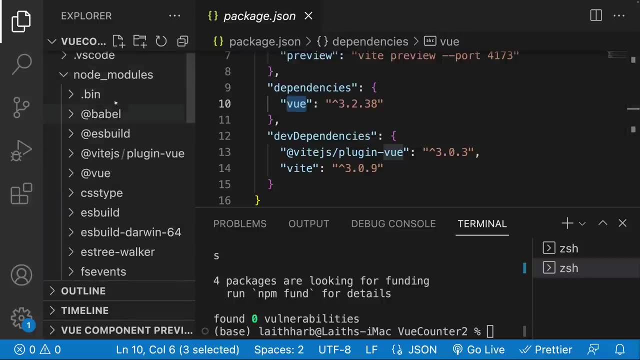 And so we actually have to install those dependencies into our machine in order to get the initial dependency that we want to work to work. And well, maybe those dependencies also have dependencies. So we need to also install those dependencies. So you can see it kind of has this really big loop. And it causes us to download a lot of different packages onto our machine. 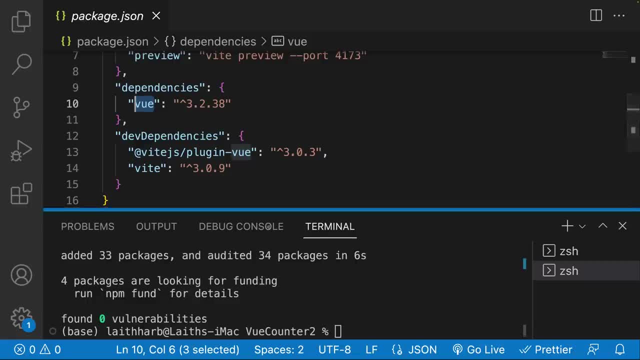 All right. So that's pretty much it. And that was the NPM install step. 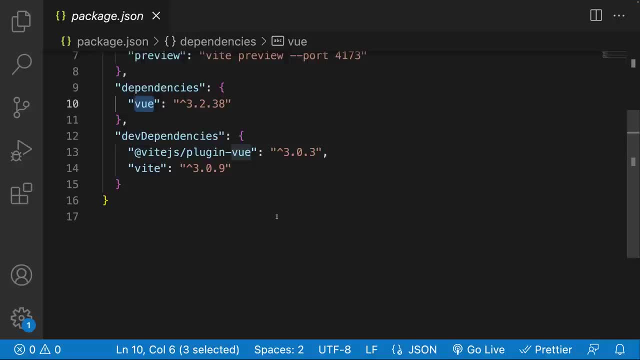 It allows us to install all three different dependencies onto our project. 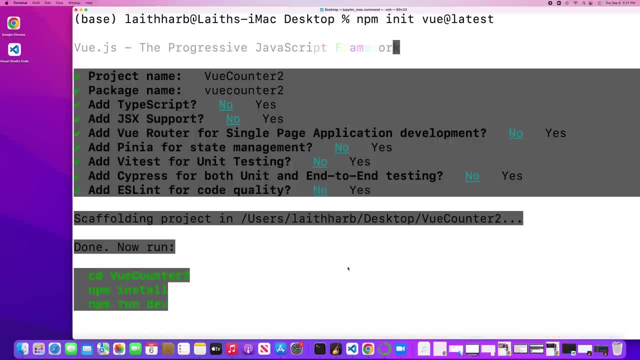 Now that we have a vast understanding of the NPM install step, let us move on to the NPM run dev step. What exactly? What does this mean? And what does this do? 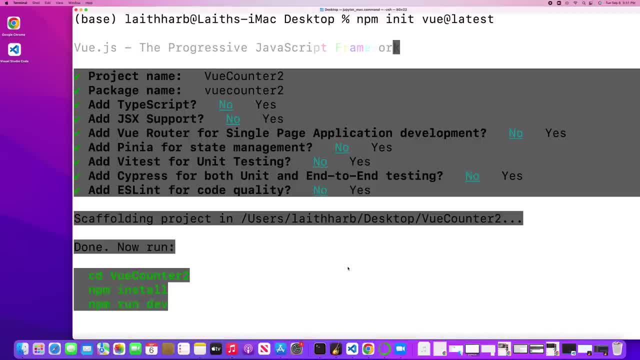 Now, in order to understand this, we first need to understand how web browsers get content when you go to a particular URL. 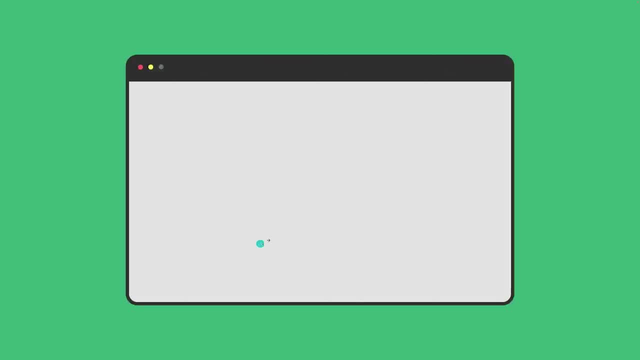 So let's go ahead and quickly try to understand this. So let's say you're on Chrome or Safari or whatever, and you write airbnb.com and then you click enter. As soon as you do that, you're greeted with a bunch of different content. So you have, you have pictures, you have styles, you have a bunch of different text. 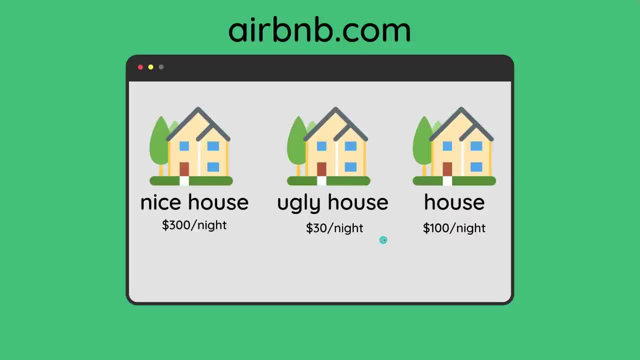 But how in the world does this content get to your browser? Well, 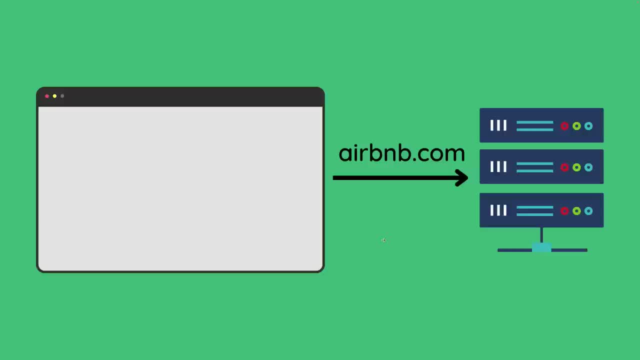 this is actually the step that it takes. The first step that it does is as soon as you go to airbnb.com, your particular browser on your machine makes a request to Airbnb's servers. 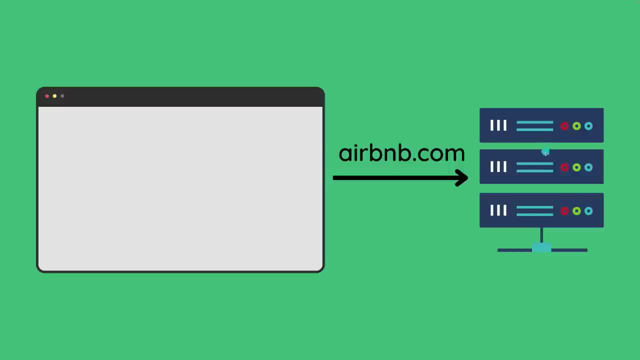 So it makes this request right over here. The server then processes the request and then it returns some data. So it goes ahead and returns some data. 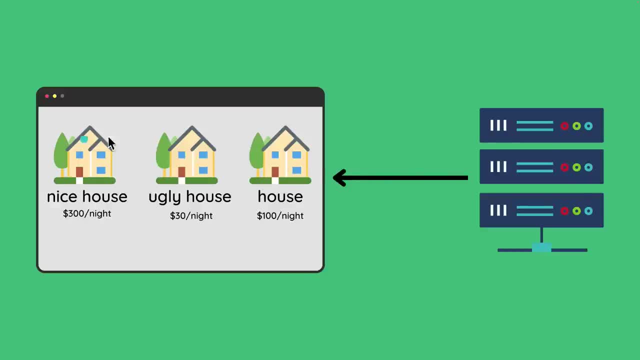 And in this case, this data, the browser takes it and starts rendering it onto the screen. 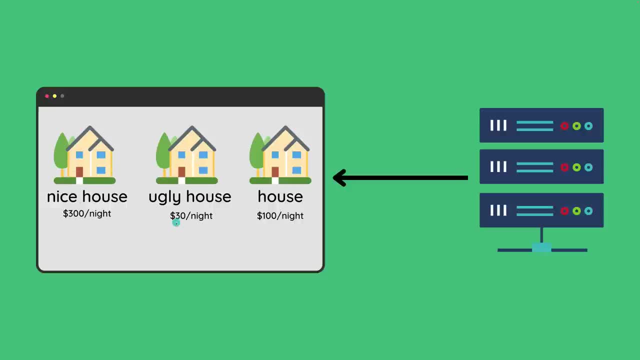 So it renders the images as well as the titles, as well as all of these styles. So everything that was returned by the server. 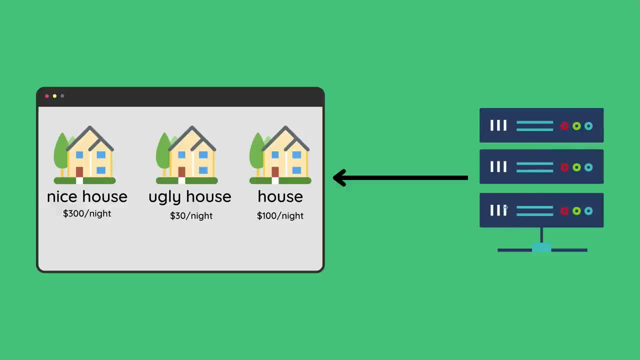 And this is how content is rendered to our browser. And if you actually go to a browser, window here, and let's actually go to Airbnb itself. 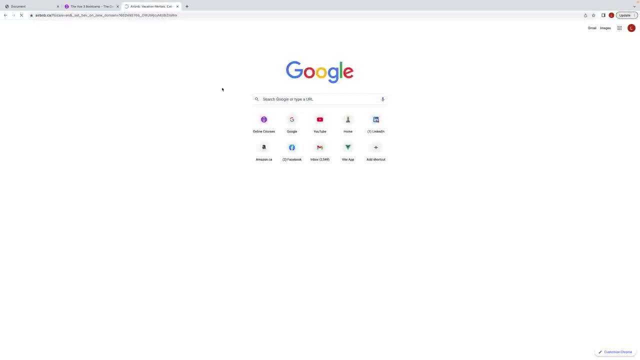 Let's go to airbnb.com. You can see, of course, right away we have a bunch of different content. 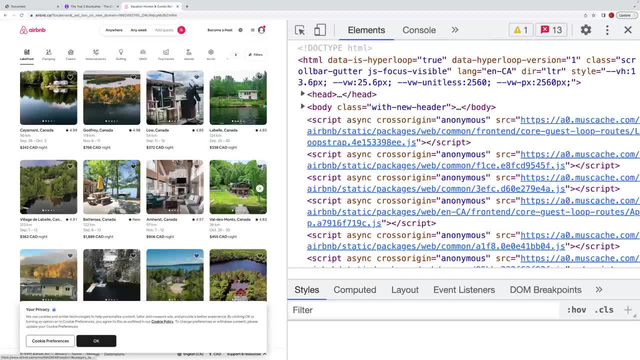 And if I were to right click inspect and I'm on Chrome for this. So if I were to right click inspect, 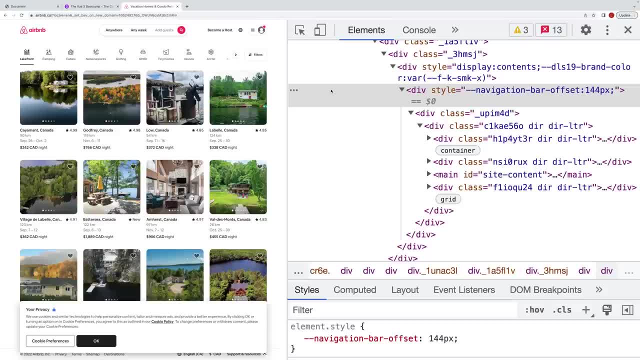 let me just zoom in here a little bit. Zoom in control zoom. Okay. It's not really working. Hopefully this is good enough for you. And if I go over here to the, the network tabs. 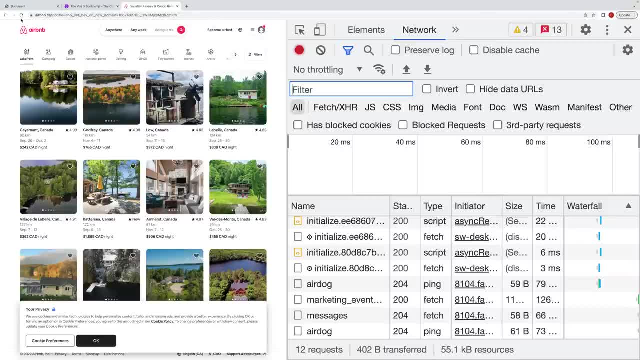 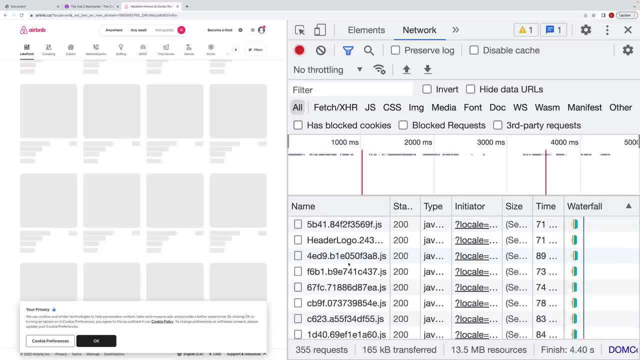 So let's go over here. I'm going to do a quick little refresh. You can see these are all actually network requests that we are making to our server. 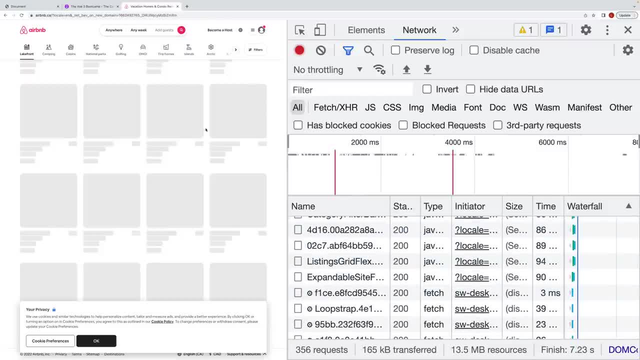 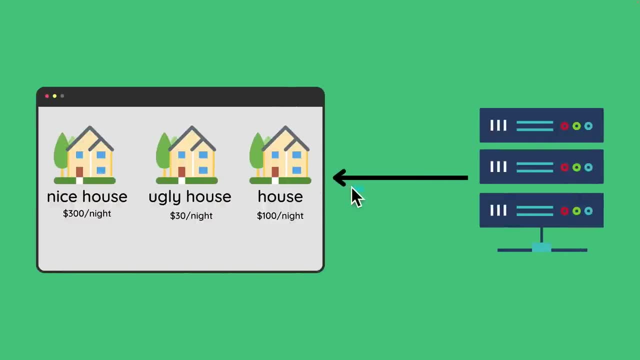 So these are all of these different network requests that we're making in order to get this content right over here. So this is typically what is, or this is what is happening when we go to a website. 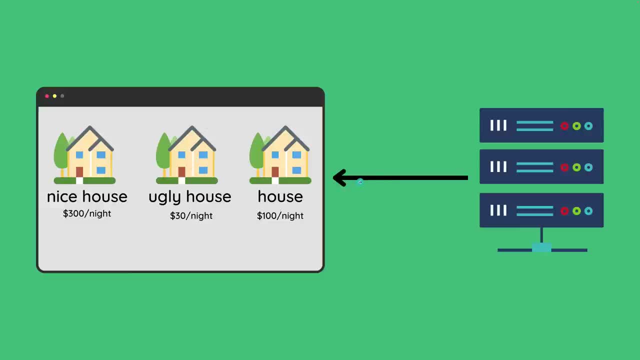 Now, this is, well, this is a process that we actually need to execute when running our application. 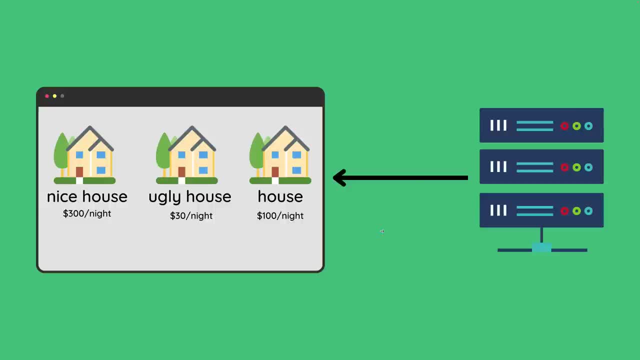 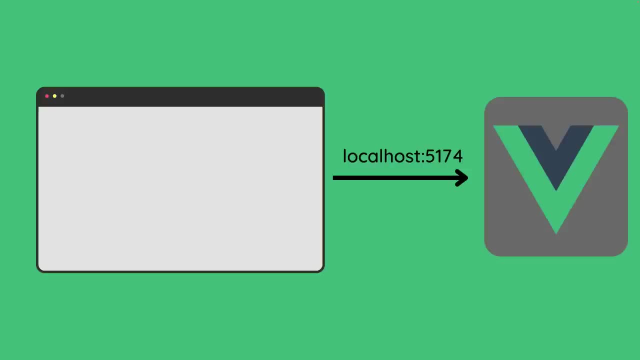 So what we do is we actually run NPM run dev. And what that does is it spins up a view development server on our local machine. 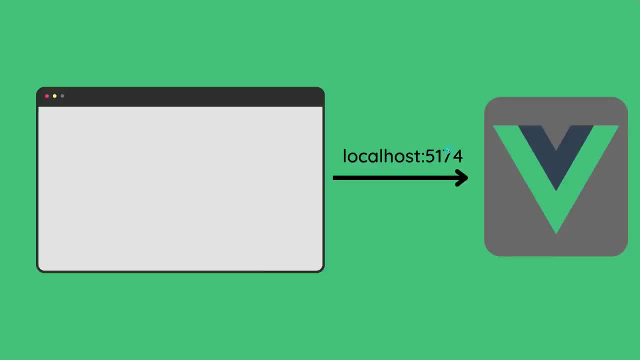 So when we go to localhost colon 5174, we're actually going to this view development server. 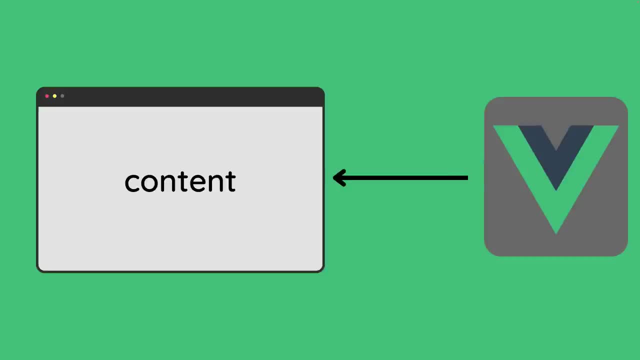 The view development server is going to go ahead and process this request. And then return the content. So the HTML elements, the styles, the JavaScript, et cetera. 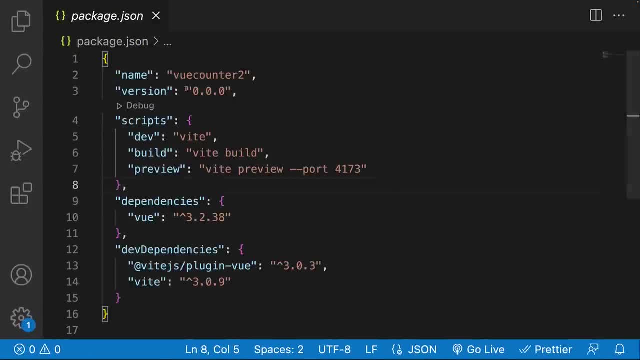 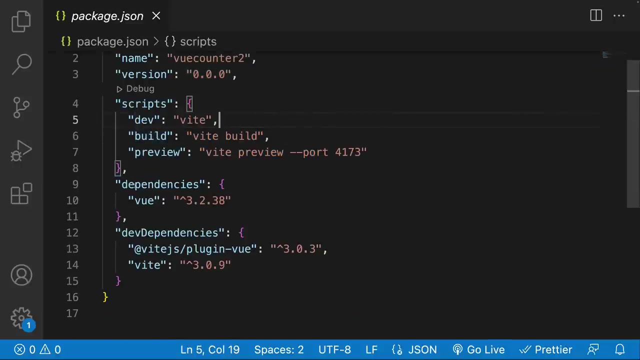 So let's actually go over here to our package dot JSON again. And we've looked at the dependencies, but this time I want to look at these scripts. When we run NPM run and then anything else, what's going to happen is it's going to run whatever is in the scripts. So for example, if you ran NPM run build, then what it's going to do is it's going to run Vite build. If we ran NPM run build, run preview is going to run Vite preview dash dash port 4173. 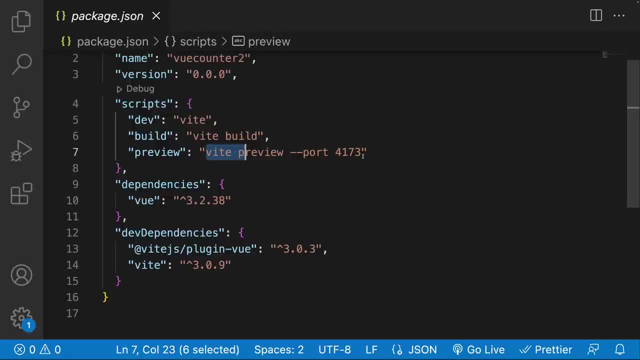 But in this case, what we did is run NPM run dev, which is just going to run Vite, which remember is actually a development dependency that we installed in the last video. And that's why you said development dependency. It is a dependency that is only needed in the development environment because it is going to spin up a development server. So this Vite thing is exactly the same. It's exactly what spins up that server, which is going to allow us to make network requests to that server and get content. 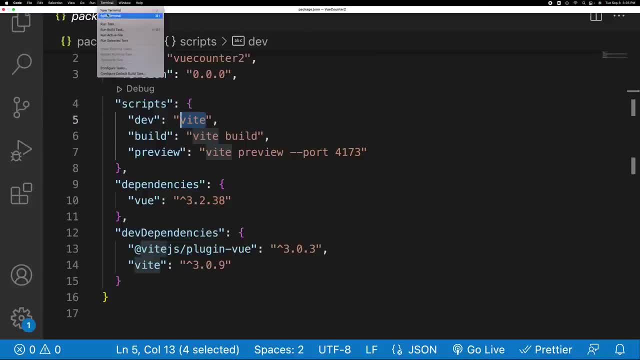 So what I'm going to do here is I'm going to go to my terminal. And now that we installed everything, I am going to do an NPM run dev. 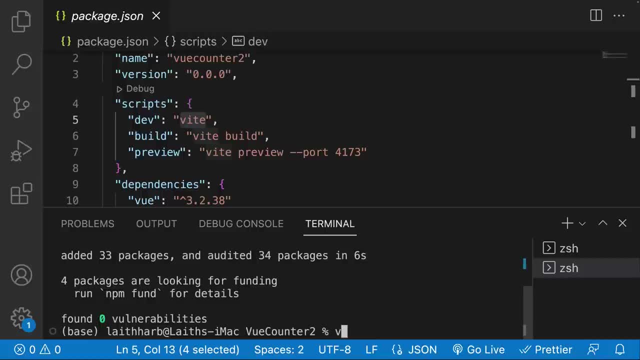 Now I could just as easily run Vite, but I'm going to do NPM run dev instead because that is the common convention. 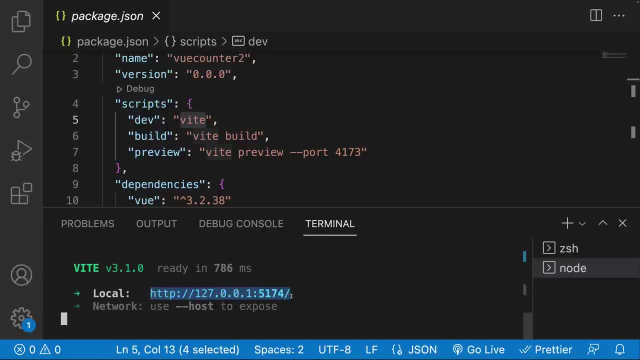 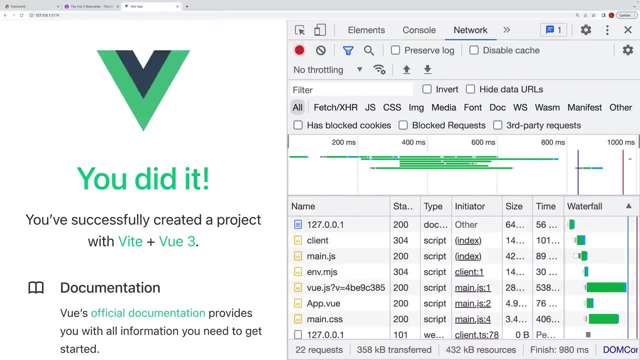 So now you can see our application is running on a local host, 5137. And now if I were to go here, you can see, 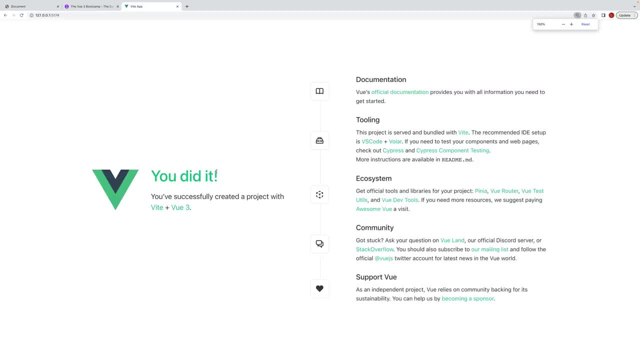 well, the content is being served to me. How terrific is that? 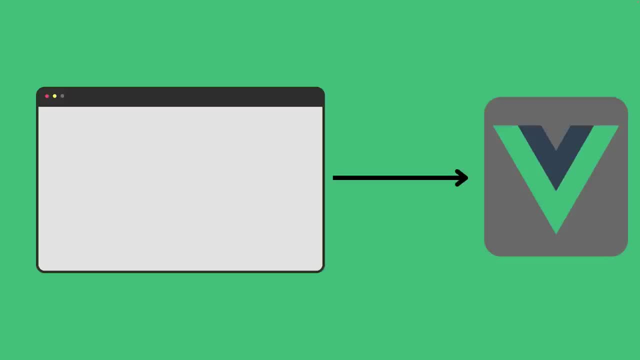 In the last video, we learned that the NPM run dev command spins up a development server that is going to serve content to our browser whenever we go to local host 5174. In this video, 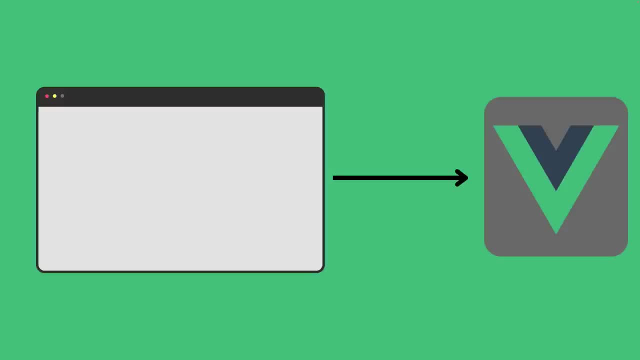 we're actually going to go into this in quite a bit more detail. So we truly understand exactly what's going on. 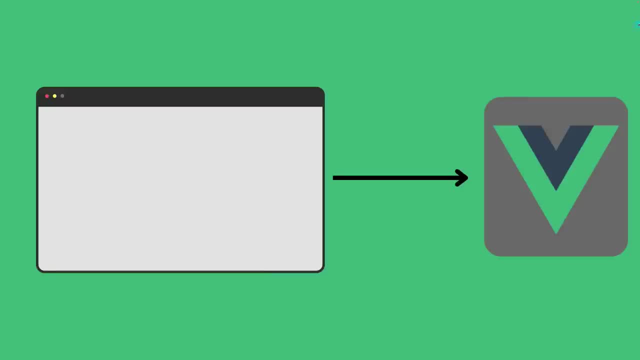 So let's say we went ahead, we ran NPM run dev, we have our view server up and running, and then we go to local host 5174. 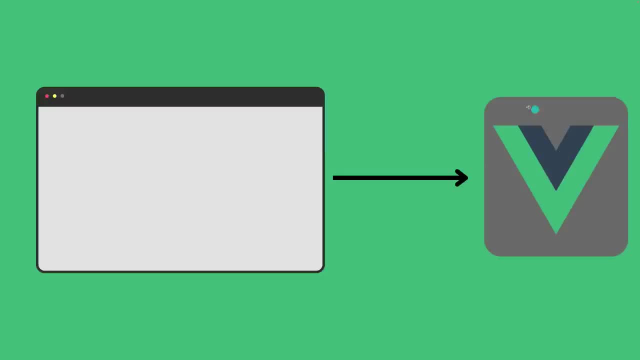 So we're going to go ahead and make a request to the view server. And then initially, as soon as we make this request, the view server is going to process that request and send us back an HTML file. That's the only thing that it is going to send us back, just this HTML file. And this is kind of a special HTML file because it is pretty much completely empty. 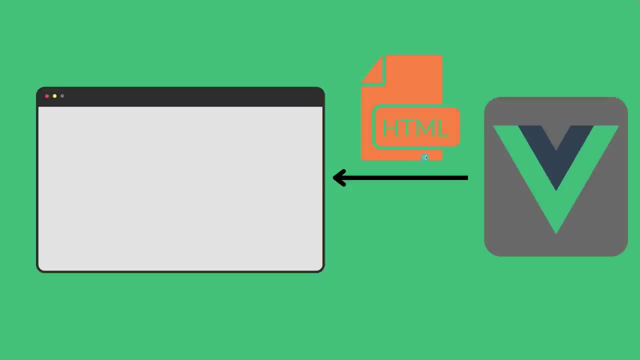 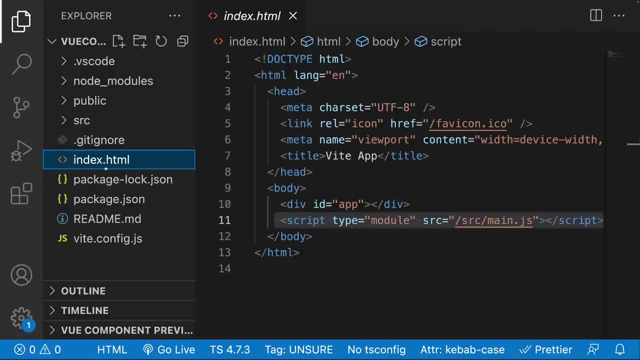 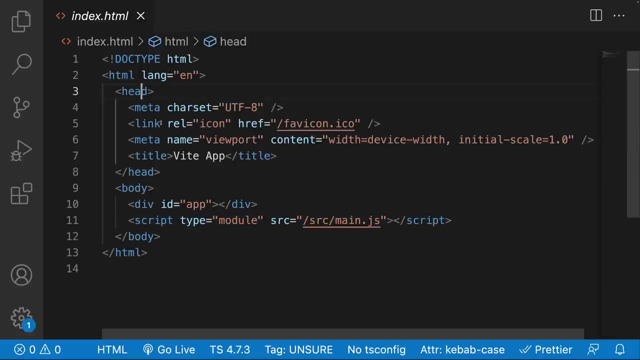 All it has is the basic boilerplate. We can actually check this out. If we go to our application, right in the root directory, we have an index.html, and you can see here that it is again completely empty. All that there is, is the boilerplate. So we have the HTML tag, we have the head, but most importantly, if you go look at the body, all we have is an empty div with an ID of app, and then we have a script tag that is going to get the JavaScript for main.js. 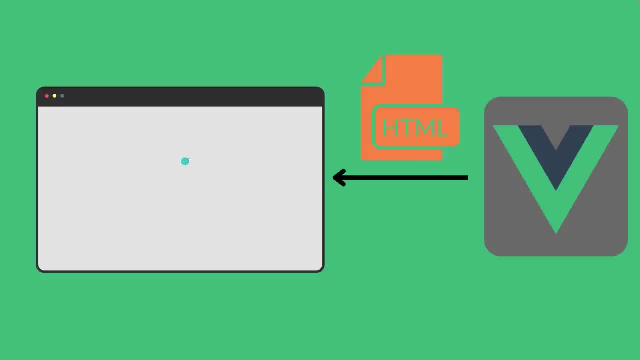 So again, completely empty. And actually, once the browser gets it, it's going to go ahead and render it, but because there's nothing really in the body, it's going to be just completely blank. 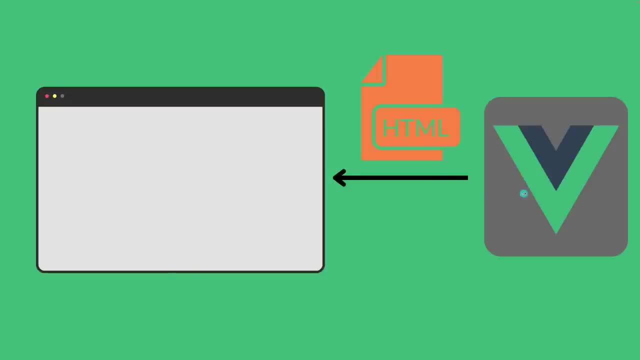 Now, well, that's actually not what we saw when we went to localhost 5174 We actually saw some content. 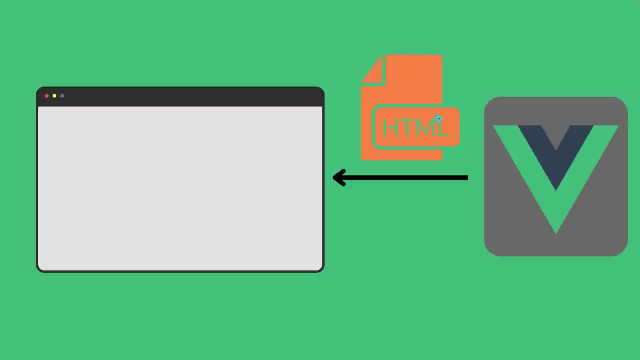 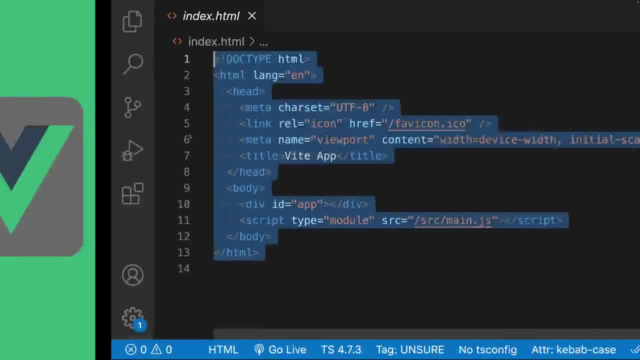 Well, that's because right after it sends the HTML, it actually bundles up all of our different logic into a singular JavaScript file, and it sends us that JavaScript file, or rather it sends the browser that JavaScript file. 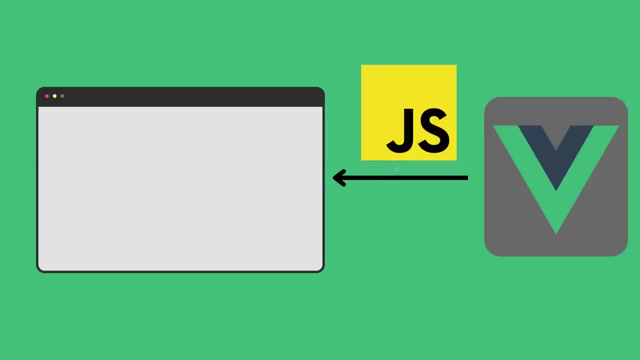 And that JavaScript file is going to contain all of the instructions about the elements that we need to render, as well as how those elements need to interact 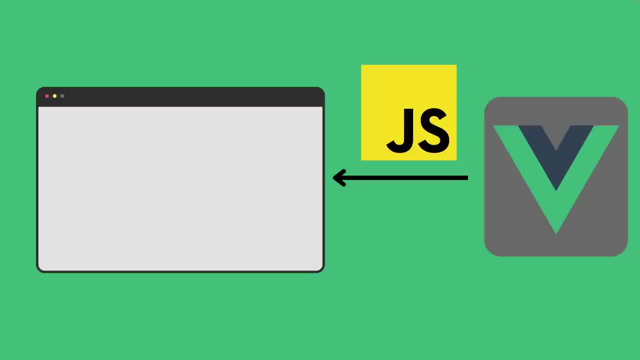 with one another to get our application to work. So what the browser is going to do is going to take this JavaScript file and start parsing it. So it's going to start creating documents, it's going to create the interaction, et cetera, et cetera. 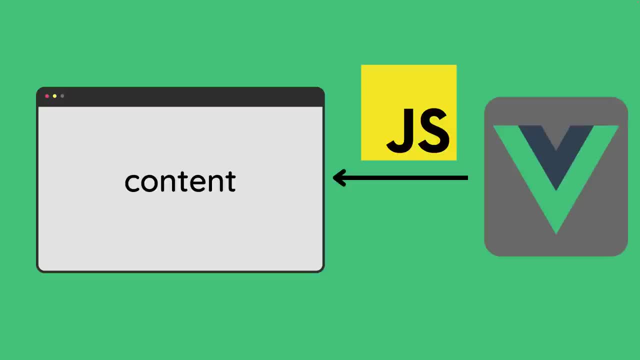 And only right after it does that do we actually have content within our application. 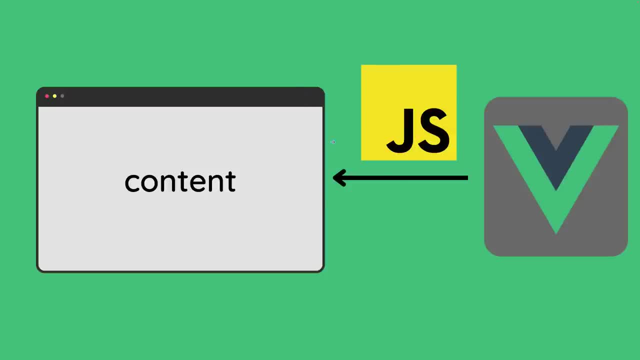 So this is how Vue application, Vue content, is actually serving content to our browser. This is how our Vue server serves content to our browser and is really, really important to understand. 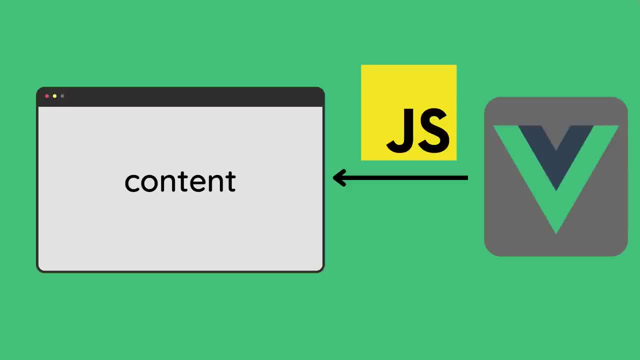 Now because this is how Vue servers serve content to our browsers, they are known as two different things. 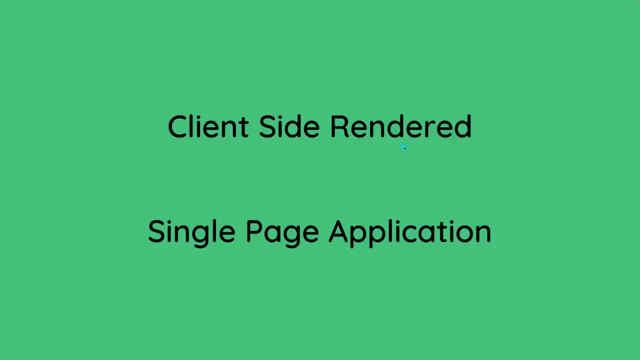 So Vue is actually known as a client-side rendered application, and it is also known as a single-page application. 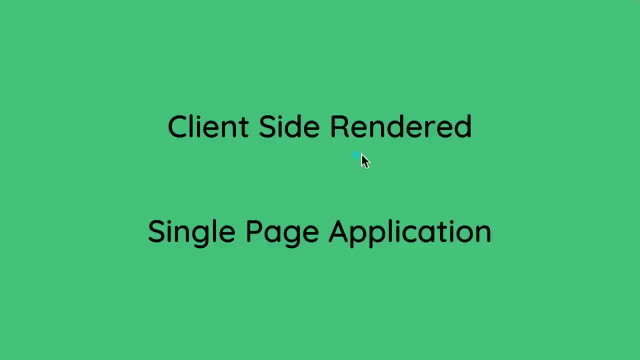 So let's actually begin with the very first one. So client-side rendered, or client-side rendering application. So what does this mean? Well, this means that the application is actually being rendered in the client. 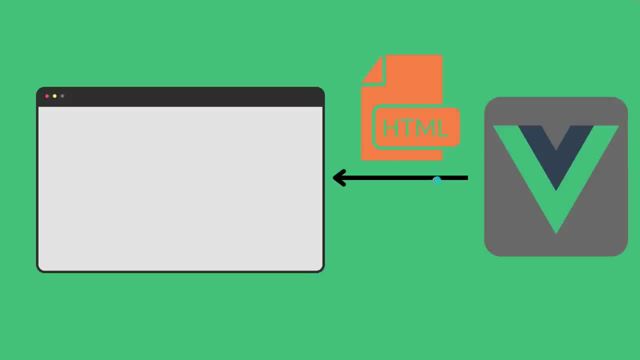 So let's remember over here, when we passed in the HTML, it was completely empty, and only once we gave it the JavaScript, the browser was able to parse the JavaScript, so the client, the browser, was able to parse the JavaScript and start rendering the HTML elements. 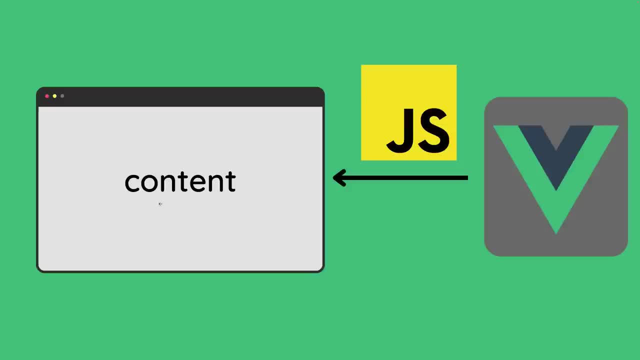 And that's why it's known as client-side rendering. 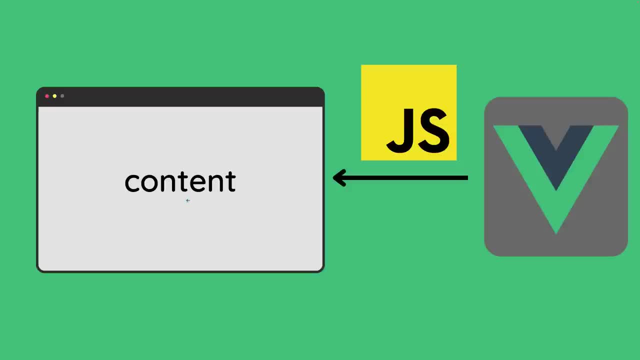 The Vue server didn't give us a completely full HTML file, it was actually pretty much empty, and then it gave us JavaScript, and it was up to the client, the browser, to parse that JavaScript and render the HTML elements. 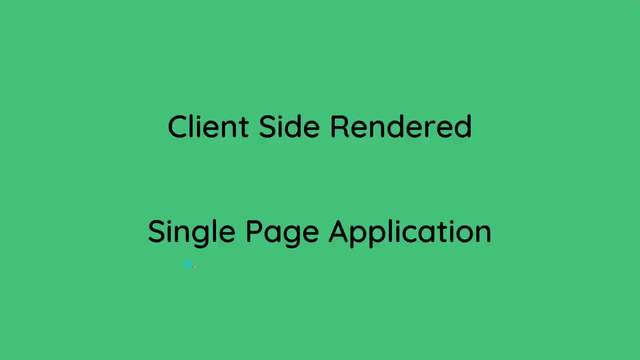 And that's why it's known as client-side rendered. Now it's also known as a single-page application. Why is that? Well, because it only sends us one index.html. So there's only one index.html that is ever sent to us. 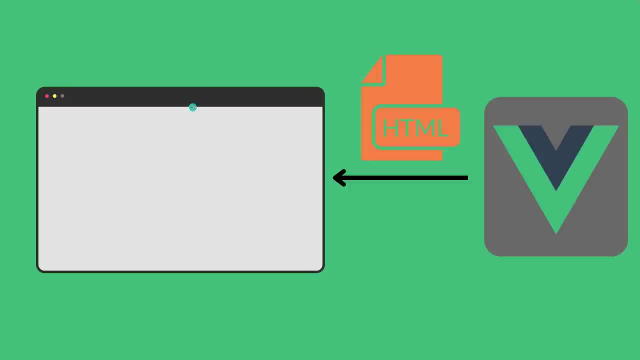 So if we went to our application, and let's say we went to, let's say our application is Airbnb, and it was built with Vue, and then we went to airbnb.ca, we got our application, we have it rendered, and then let's say we went to airbnb.ca slash houses, or slash condos in Toronto. 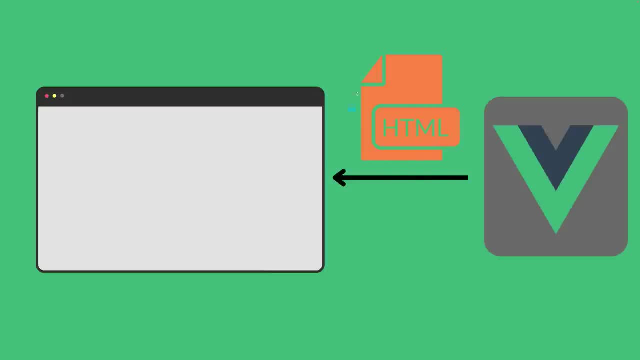 Well, our server is not going to send us another HTML file, it's going to be the exact same HTML file, but it's going to be up to the JavaScript to just change the HTML elements 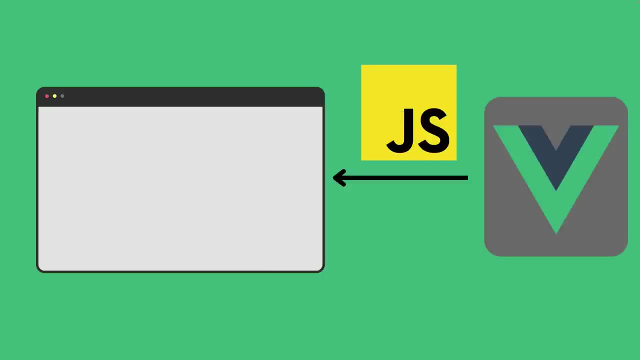 within that exact same index.html file. 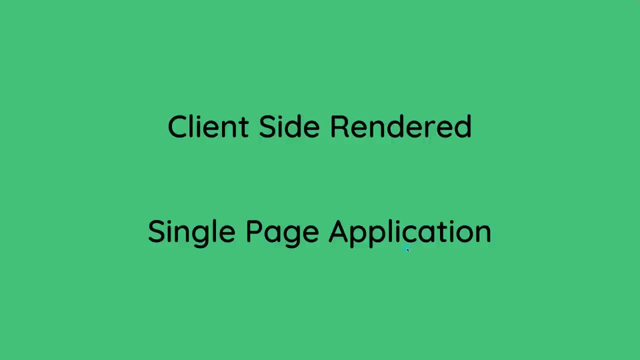 And that's why it is also known as a single-page application. So these are two terminologies that are going to be, you're going to see them all the time when it comes to Vue, and I think it is very, very important 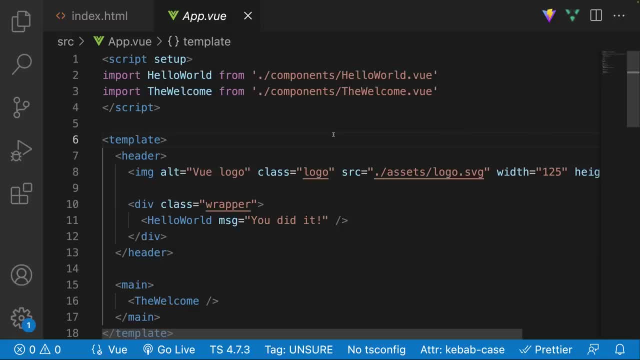 Enough of that, let's actually go ahead and start coding. 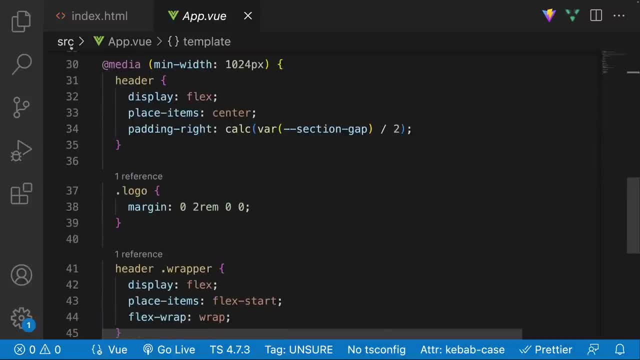 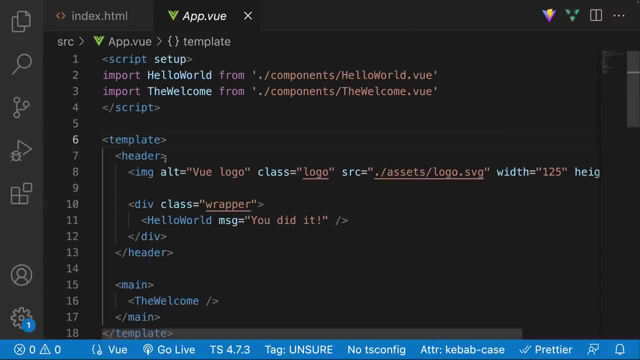 Now, in the last section, when we built out our app, we only did our logic inside of the app.vue. This is really where we wrote everything, the styles, the JavaScript, as well as the HTML. 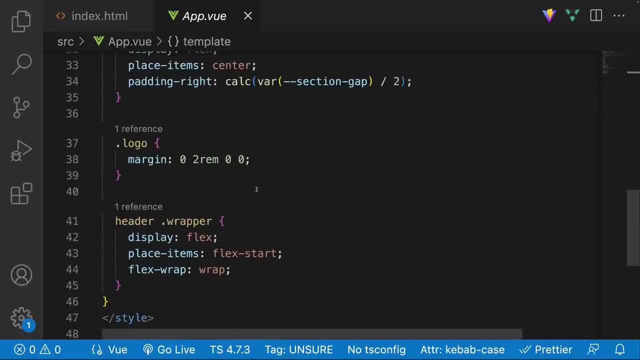 And there's a very, very good reason for this, and that's because, well, this right over here 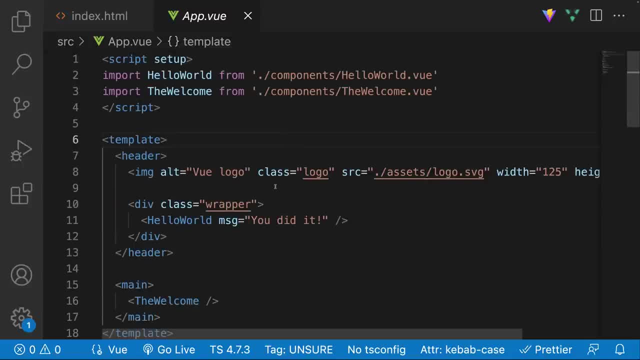 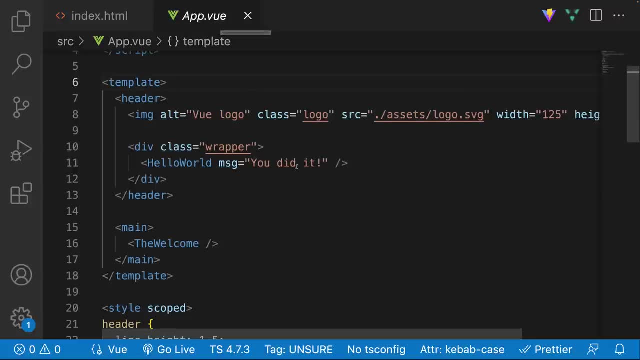 is our entire app. Every single piece of code that is existing to our application lives inside of the app.vue file. 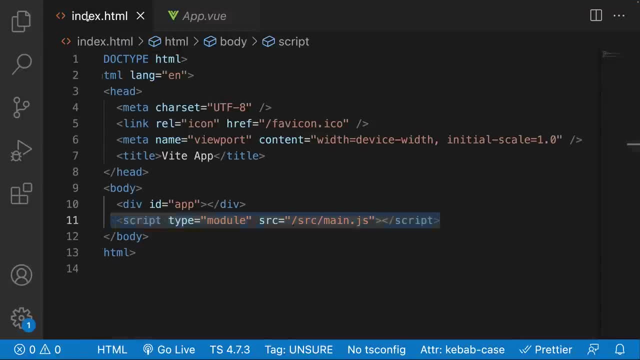 And let me actually tell you why that is. So let's go back to our index.html, and just as a quick reminder, let's look at the body tag right over here. 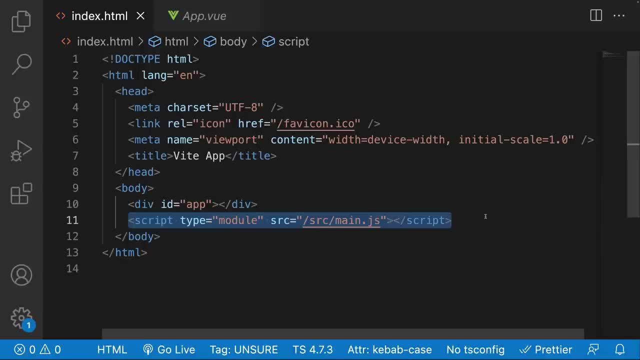 So we have this div with an ID of app, and we also have this script tag that is pointing to the main.js. And that, of course, is this file right over here. 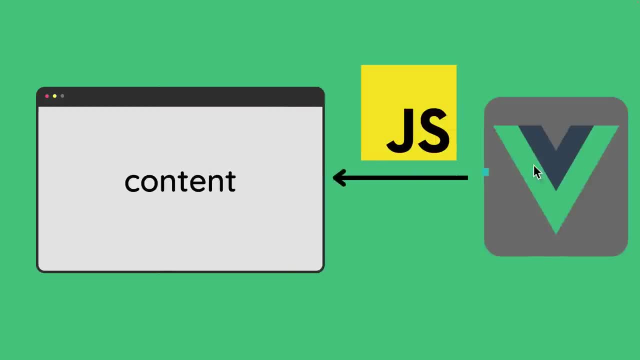 So this file right here is actually the JavaScript that our Vue server is sending to our browser. 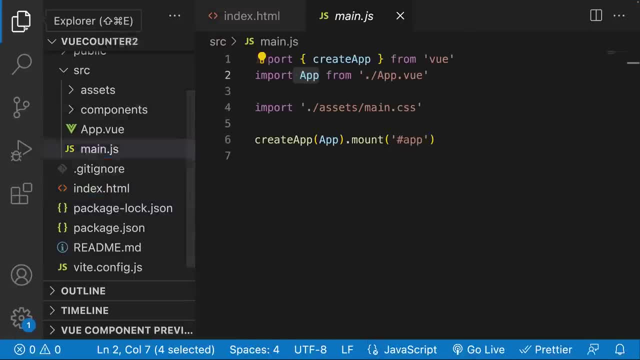 So let's go ahead and take a look at this file right over here. 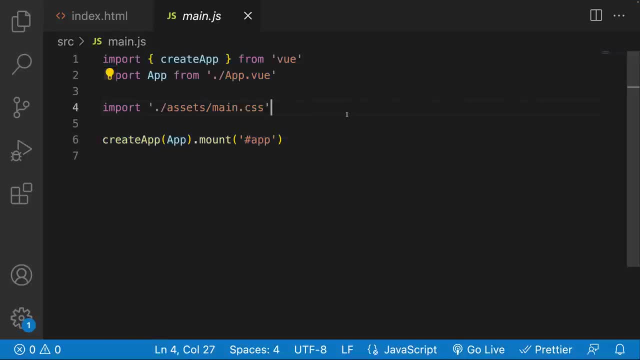 And this is a relatively simple file. There's only really four lines of code. 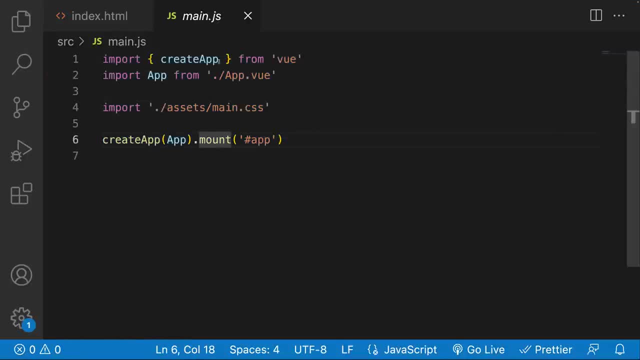 So the first two lines are import statements. So what we're doing is we're importing something called createApp from Vue. So this is the package that we just installed. And then what we're doing is we're also importing our app from, well, app.vue. And then let's just forget about this. 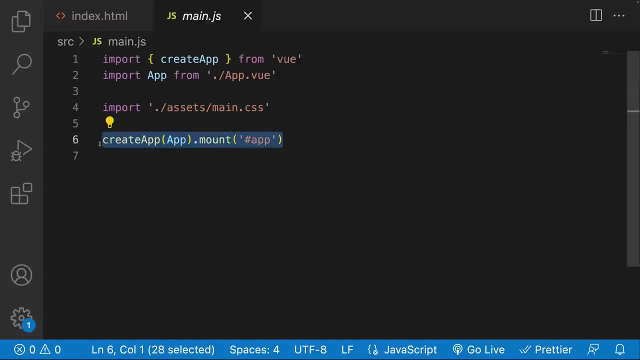 This is just importing some styles. This is where really the magic is happening. 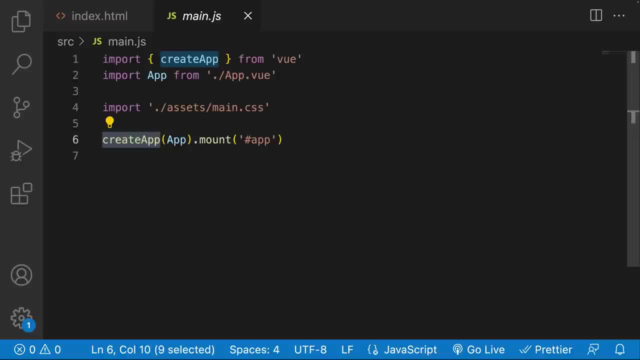 So what we're doing here is we are creating an app, and then we're passing in the app from the app.vue file. And then what we are doing is we are mounting all of the HTML elements inside of the existing HTML element that has an ID inside of app. 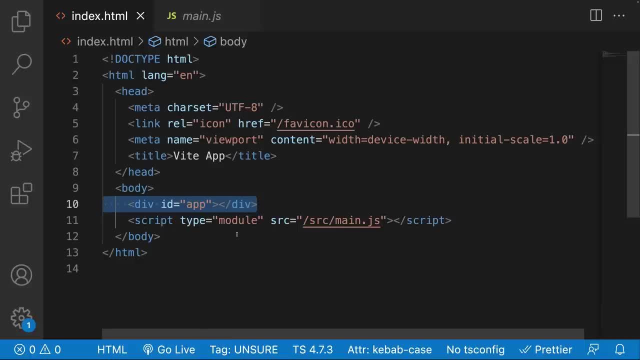 And, well, you guessed it, that is this div right over here. All right. 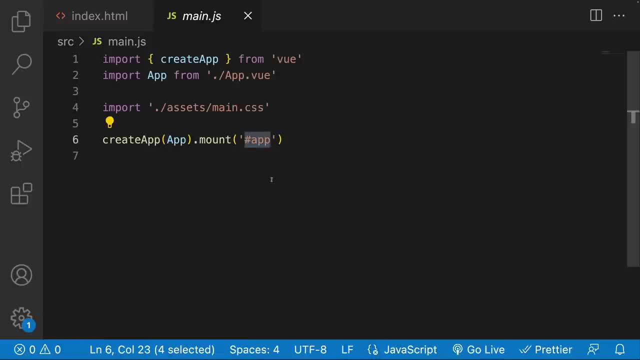 So this is pretty cool. So this right here is the JavaScript that is going to render everything inside of this div right here. 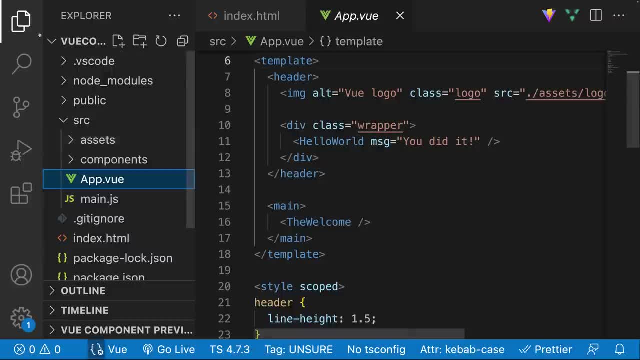 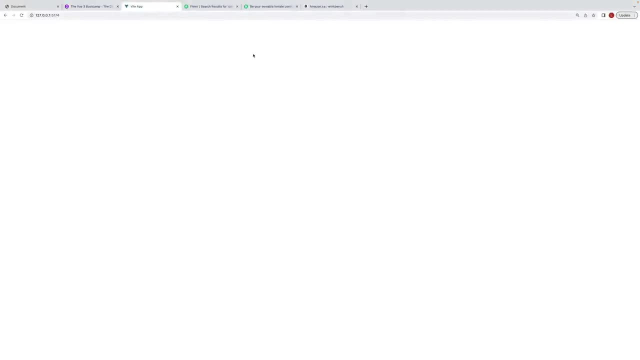 So what we can actually do now is we can go to our app.vue, and if we removed everything, well, you can see that our application now is, well, completely empty. 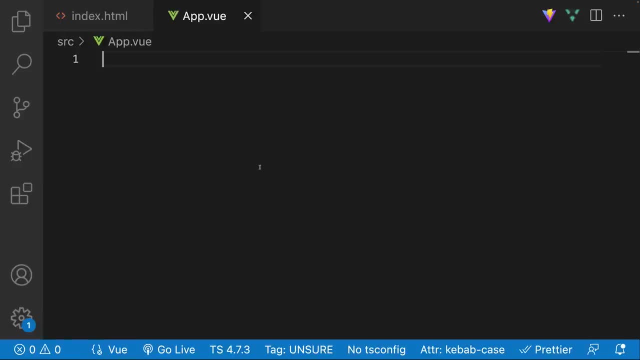 So now what I want to do is I actually want to start adding some HTML. So we can actually add HTML directly into the app.vue file. However, all HTML elements must begin with the template element. So it absolutely has to begin with this. Then we can add whatever it is that we want. We can add a div, and then over here we can say something like hello, or sorry, we can say h1, and then hello, first. 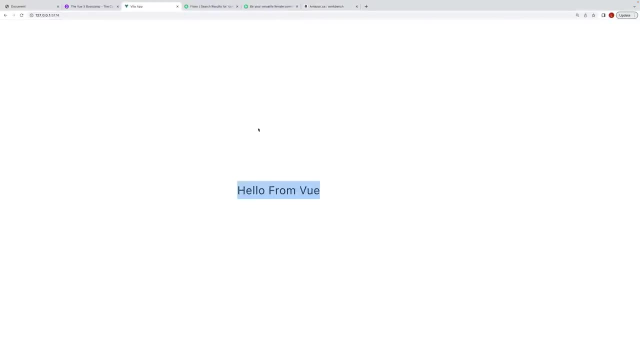 So we can add a div right over here. And this is going to make our app look like it's actually running. 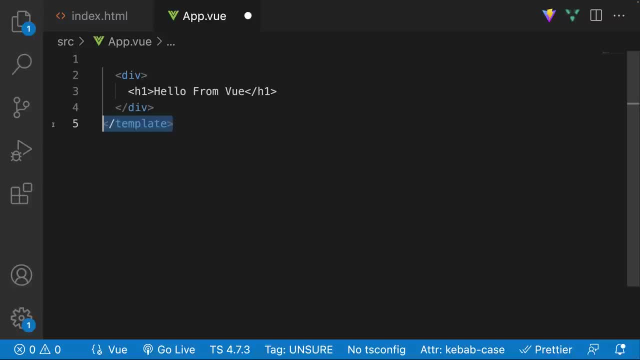 So, we can add a div right over here. And then we can add a div from view like so. 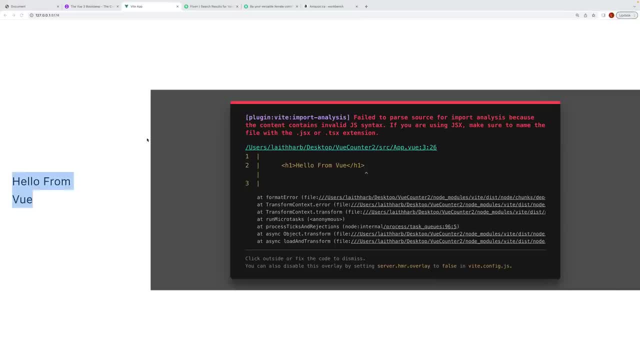 And now if I were to save this, you can see that this works A-OK. 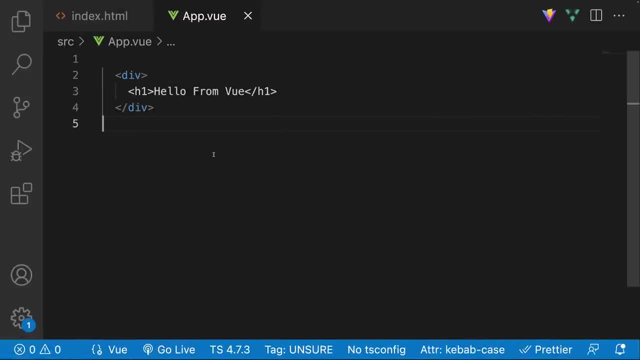 If I removed this template tag, now you can see that the syntax is a little bit different. 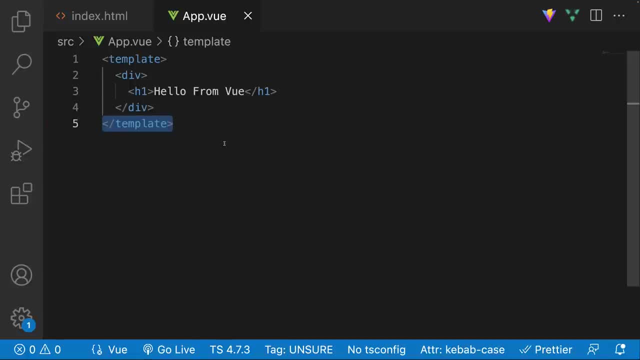 Like the syntax highlighting is different. And if I were to save this, right away you can see we get an error. 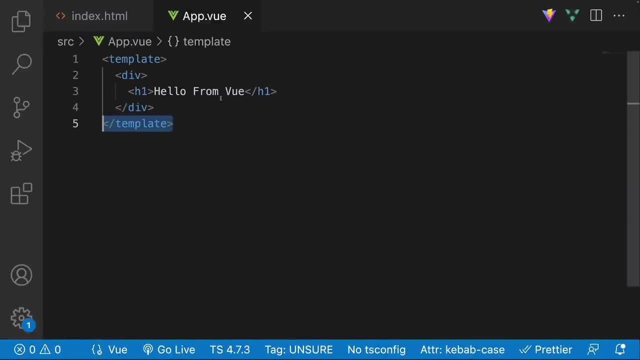 And you might be wondering why in the world do we actually need to add these template tags. This makes pretty much no sense. I don't want this to appear on my browser. 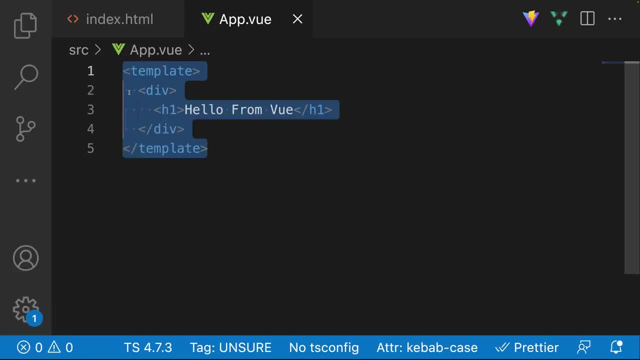 HTML, it looks like HTML, it behaves like HTML, but technically, it's not really HTML. Instead, it is a view template. And what it's going to do is we get this view template. And of course, then we're going to convert it into JavaScript, which is going to allow us to create, you know, elements within our client. So this right here is a view template. And the reason why it is a view template is you're going to see a little bit later, we're going to start doing some really weird and wacky things within our view templates that are not really valid HTML. And we kind of saw this in the last video, but we did something like at click is equal to count plus plus, this isn't really HTML, this isn't valid HTML. However, it is understood by view because this 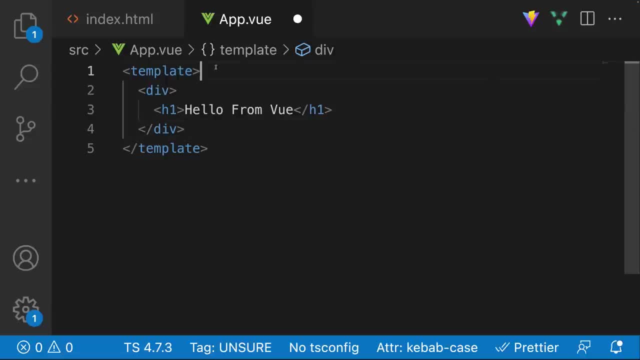 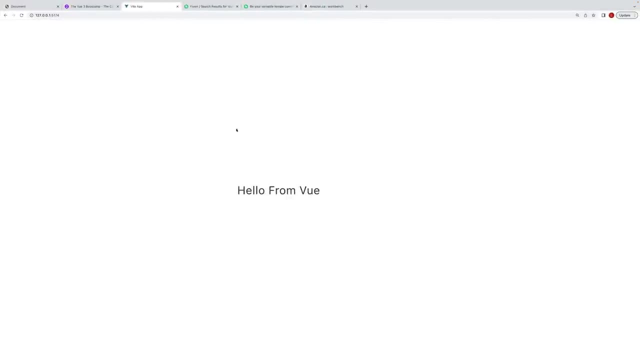 indeed is a view template. So that's why we need to add these templates. And actually, what's nice about them is that these tags, whenever they're actually rendered inside of the browser are completely removed. So these template tags are completely removed. 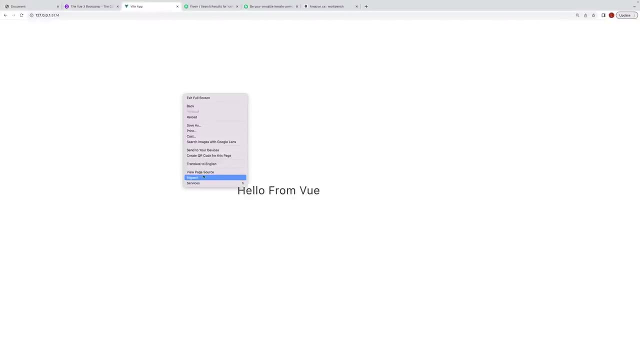 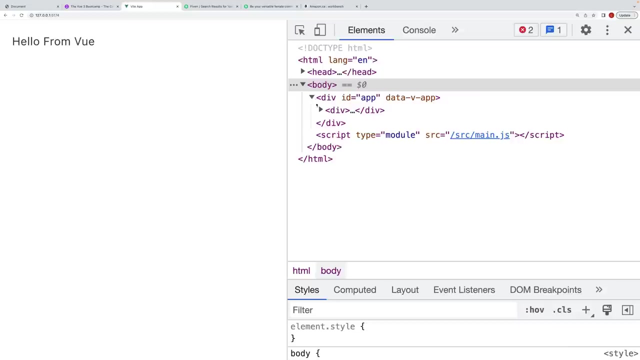 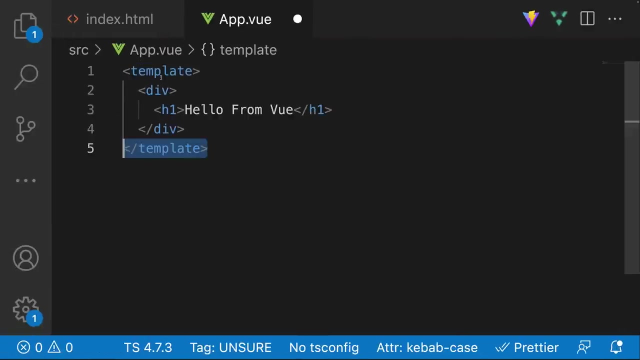 So if I were to go over here, and I were to inspect and look at all of the DOM elements, you can see we have our app right over here. And then I were to click here, you can see that we have no template, we just have a div. And then within that div, we have an H1. So it was actually completely removed. But we need to add them. And we're going to do that by clicking on the 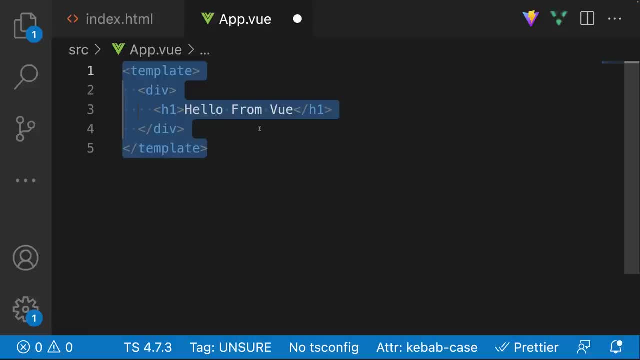 inside of the app dot view to specify that this is going to be our view template. So now let's go ahead and actually create our HTML or our view template for our counter application. So I am going to, first of all, I'm going to change this to a main, a main tag. And then within the main tag, let's add a div. And then within the div, we're going to have an H4, we're going to say current count is and then dot dot dot. And then we're going to say H1. For now, we'll initialize this as zero. And of course, now we want our buttons. So we're going to say button, and we're 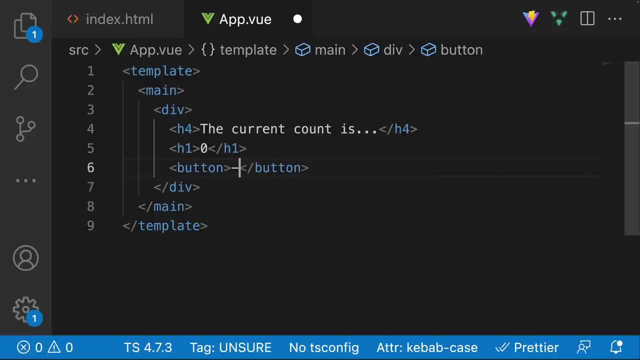 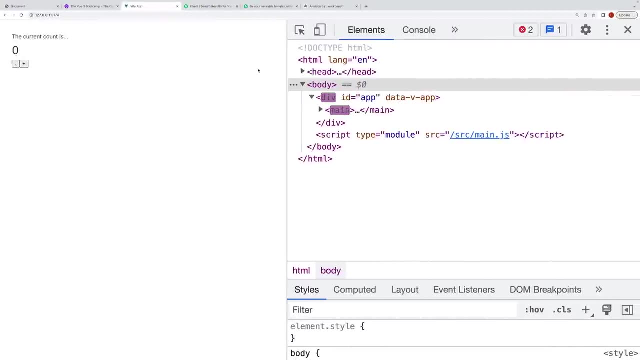 going to say button, we're going to say this one's going to be minus. And then over here, we're going to have another button that is going to be plus. So now if you were to save this, you can see we 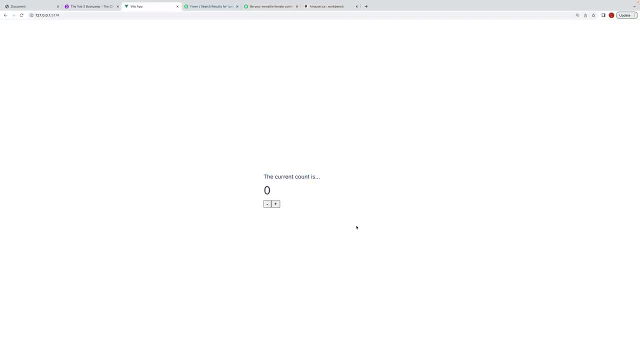 have our wonderful application right over here. And I'm not really going to increase the size of it, you can just zoom in or out to, you know, have 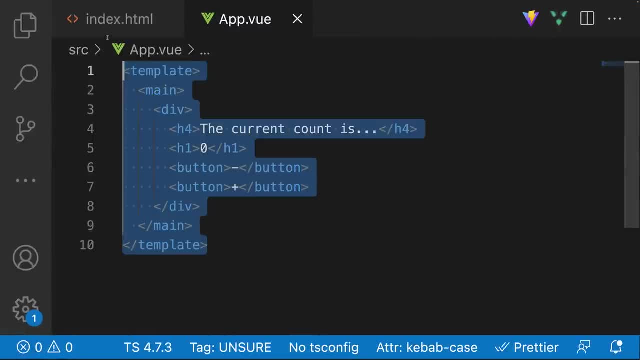 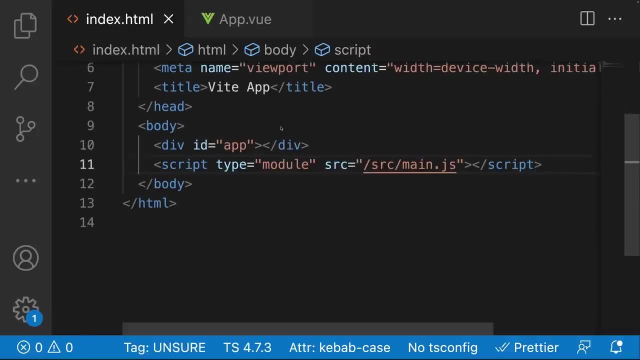 the size work a little bit better for you. So that right there is going to create the HTML within our browser. All right, everybody, let us now style our application just so that it looks a little bit 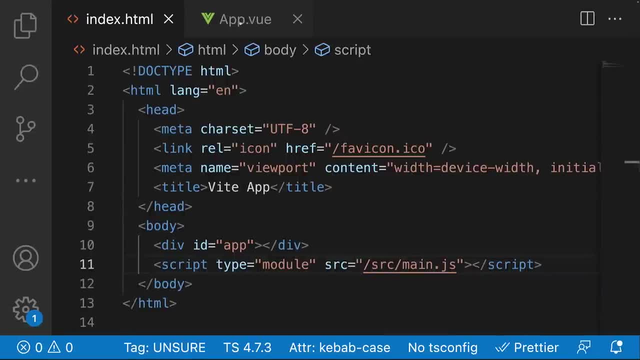 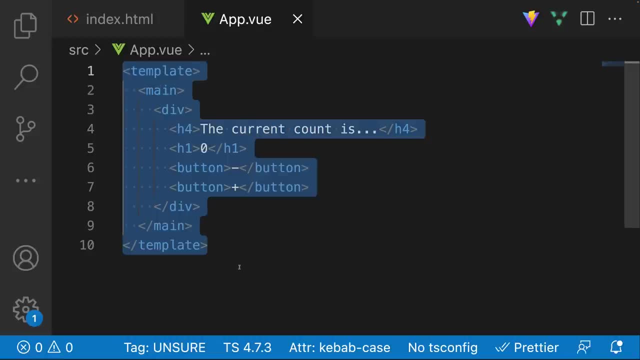 better than what it does right now. So let's go into our app dot view. And just like we can create our app dot view, we can also style that template as well. And to do that, right after the template tags, what we can do is add style tags. And in here, of course, we can start adding any styles that we 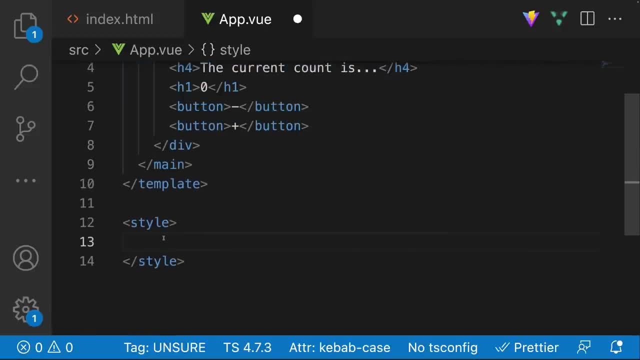 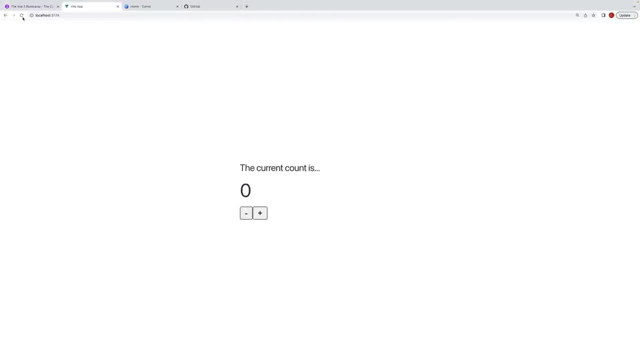 want to this template over here. So we can do something like mean, and let's say I want to change the background color to Alice blue. And if I were to do this and refresh the page, as you can see here, very faintly, you can see that there's an Alice blue. 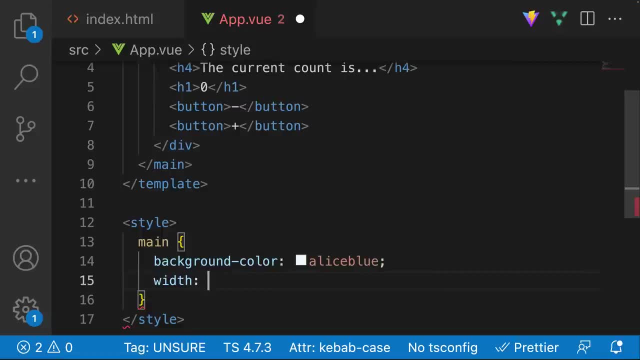 Blue background color. Of course, I can give this a width of 100 VW. So let's do a width of 100 VW, 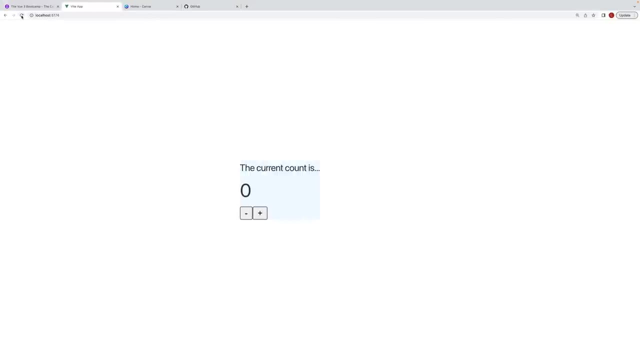 a height of 100 VH. And that way, if I were to refresh, that way it is as you can see here, it is taking up the complete page. Now there are some weird styling discrepancies. So to fix this, 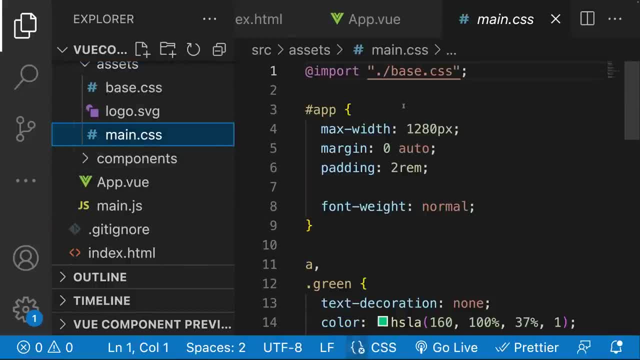 what we can very simply do here is just go to the main dot j s and just remove all of these styles. Let's go ahead and do that. 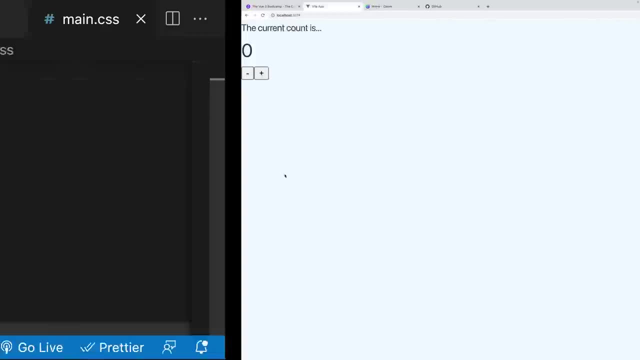 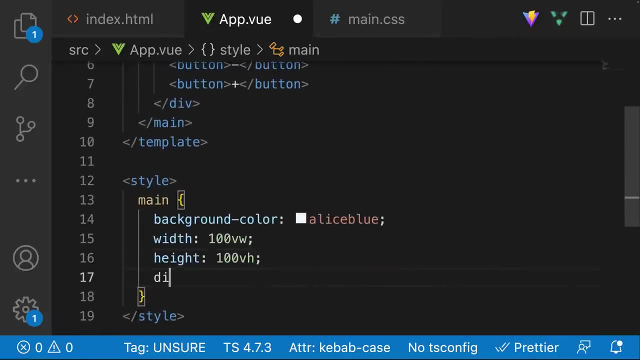 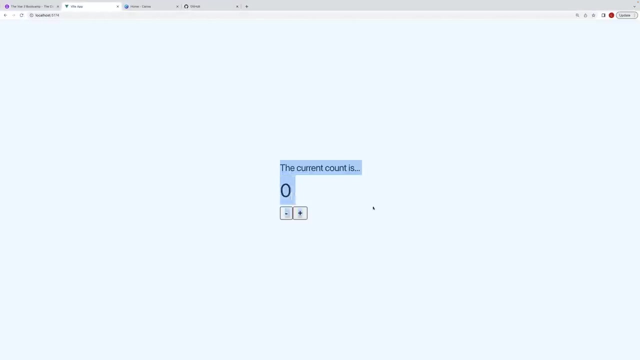 And there we go. So now we got these styles pretty much working the way that we want them to. So let's go back over here. And let us now do the display flex. So display flex. And then we're going to do an align items of center. And lastly, we're going to do a justify content of center as well, just so we can center this right in the middle. I'm having to refresh because I haven't worked on this project in a while. 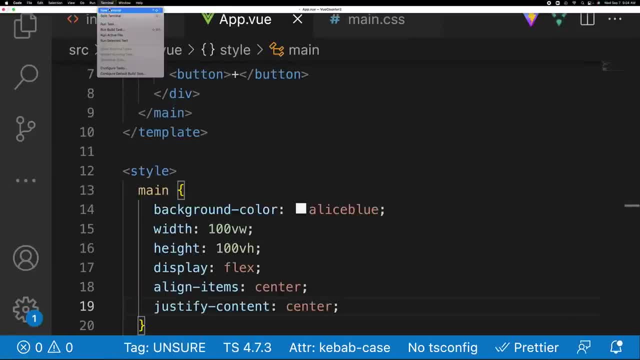 So that's why it's a not hot reloading for me actually what I can do if I wanted to is I can go open up my terminal 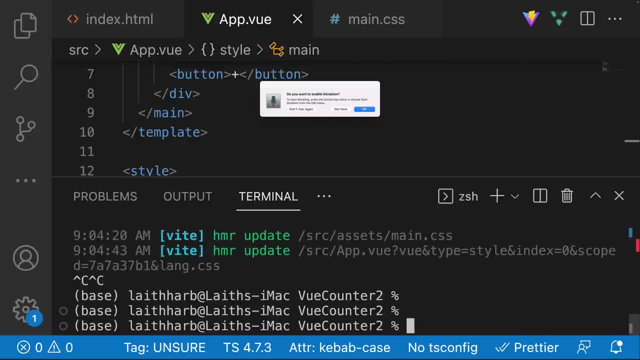 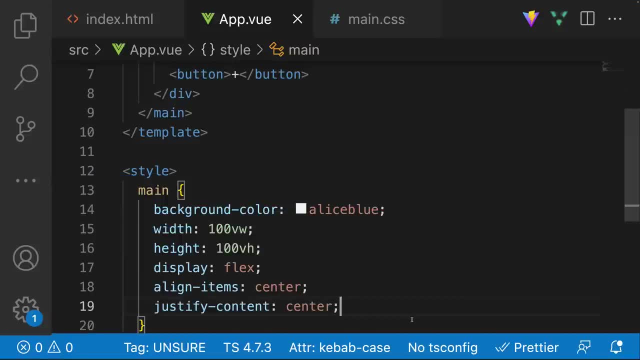 and just do a ctrl c if this ever happens to you and I can just say okay or cancel not now and then I can just do an npm run dev again okay so that is going to be the main and now let's just 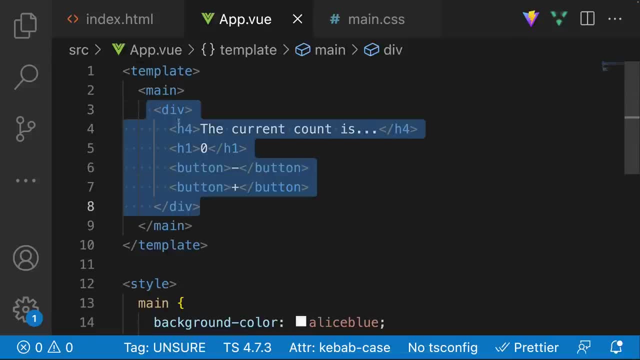 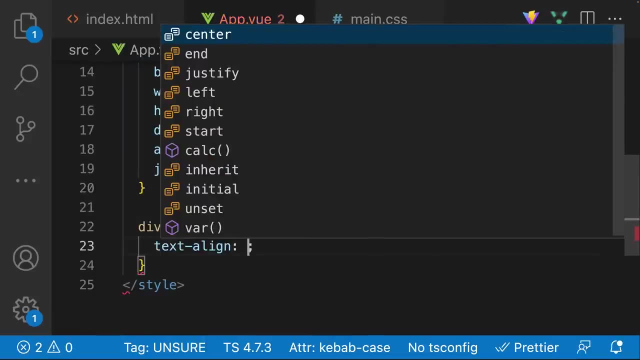 do a quick little uh styling so that everything within this div is nice and centered so over here I can add just add div and I can just say text align center and there we go so you can see that 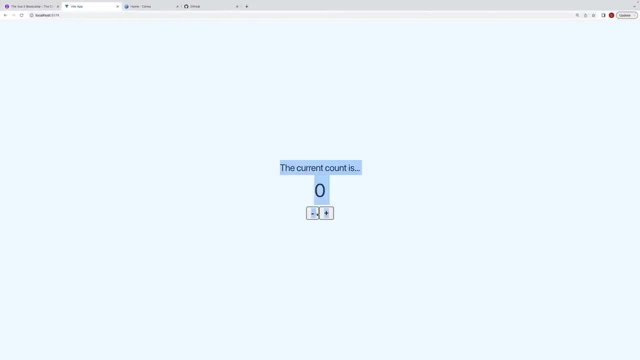 it is working a okay and of course it's not functional because so we haven't made it functional 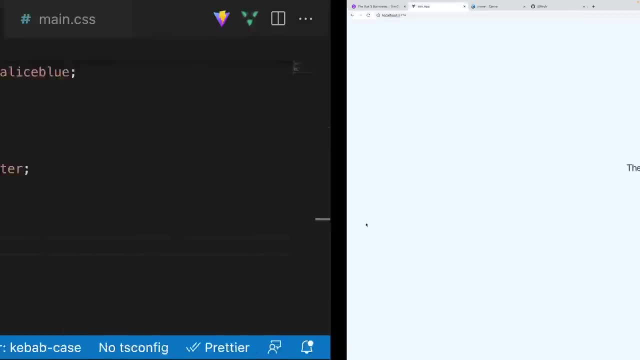 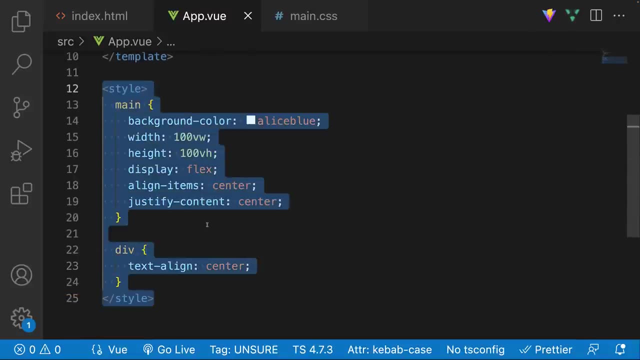 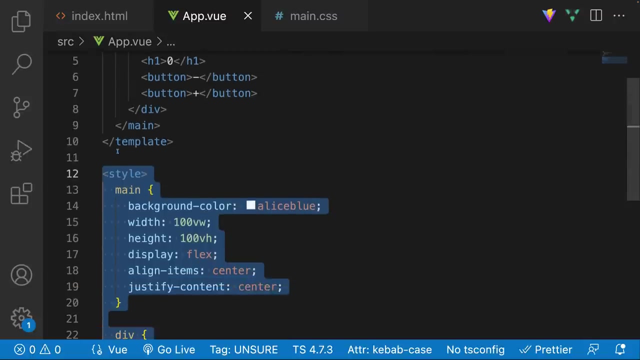 yet but the styling is working now there's one last thing that I want to add I think so far this should be relatively simple this isn't anything new this is just styling the only thing that might be new is that we can actually add these styles within the app.vue file themselves and this is 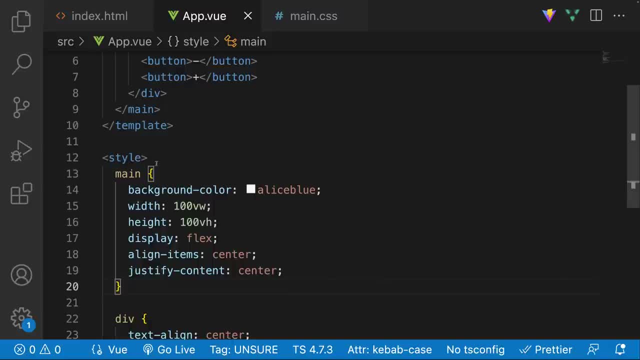 the format to do them however now what I want to do is something that you probably haven't seen before so right here 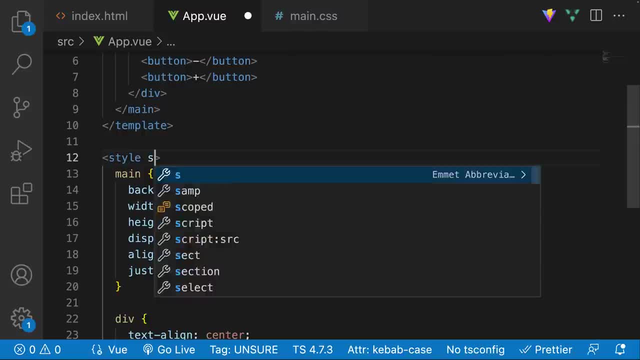 within this tag I'm going to do a space and then I'm going to add scoped and this is a best practice now what does this mean over here well let me explain so right now inside of our app.vue file 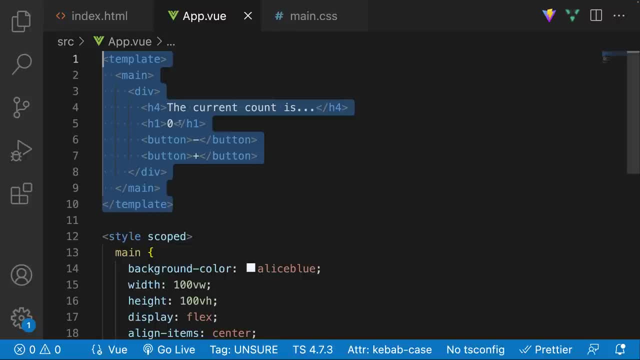 we have this a view template that is our HTML that we might eventually want to style however later on and we'll see this definitely later on you 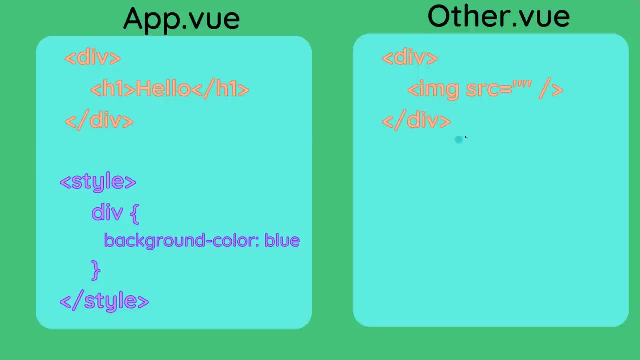 especially in bigger projects we're going to be working with multiple different view files so we could have our app.vue it could have our you know view template as well as these styles but with 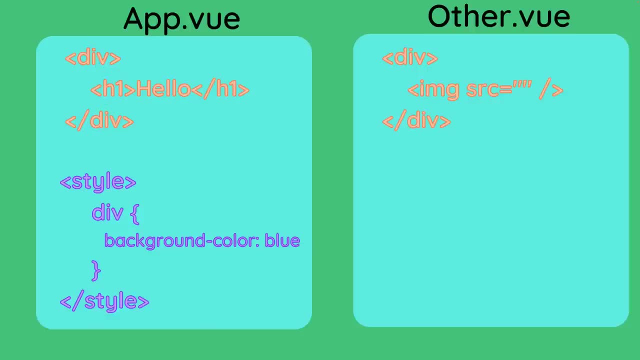 bigger projects we're not going to want to stick everything into one file even though right now that is exactly what we are doing later on we're going to want to have multiple different view files with multiple different templates so what actually ends up happening if let's say right here 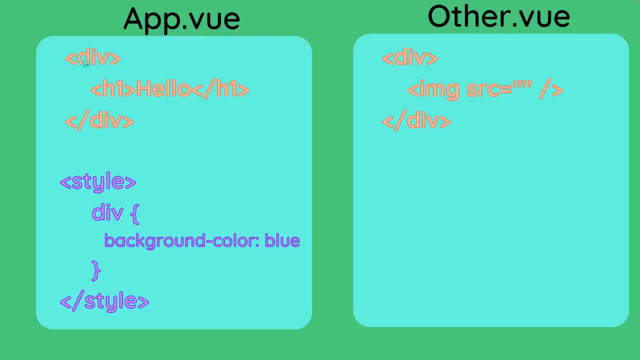 within my app.vue I want to style this div that is housing this h1 that says hello so I add these style tags and 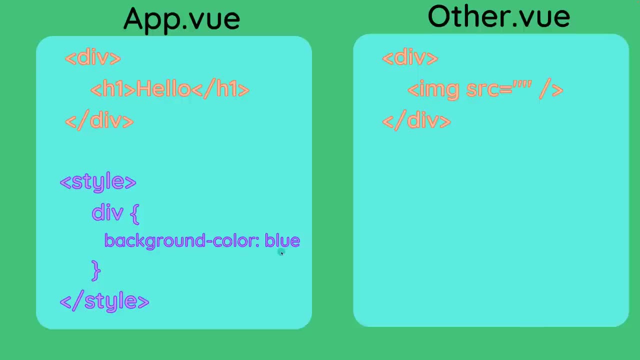 then I want to style the div and I give it a background color of let's say blue so what ends up happening is that this div right over here ends up having a background color of blue but actually so does this div right here even though it is in a completely separate file so this actually might 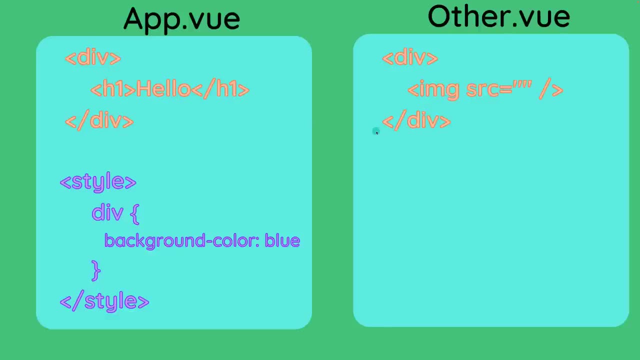 not be the! effect and most of the time it is not the intended effect right here we 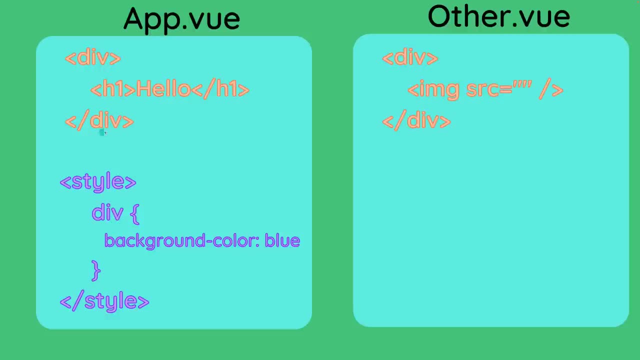 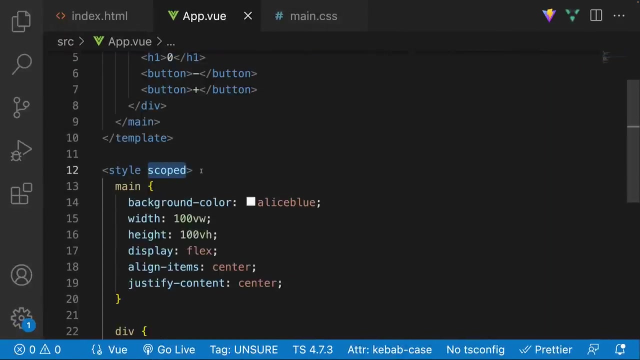 basically defined global styles that are going to apply to every div in our application regardless of where they live so what I actually want to do is I only want to give this div a background color of blue not this div so what do I do to kind of scope it to this file well very simply I add the scope keyword within the style tag so by adding the scope keyword what it does is it only applies these styles to the HTML elements within the file itself and that why it is very important to add this right over here so that we don't accidentally start adding global styles and affecting these styles of other HTML 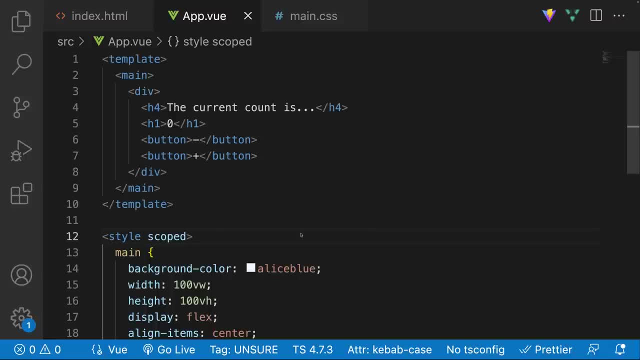 elements so we finished the HTML we also finished the styling the next thing that we need to do is we need to add the style tag to the HTML element so we need to do is of course make our application functional with well JavaScript so just like we can actually define the HTML as well as the CSS within the app dot view file we can also define the JavaScript and typically with view 3 this is actually going to be the very first thing that we have in our file so it's going to be typically the order doesn't really matter but it is 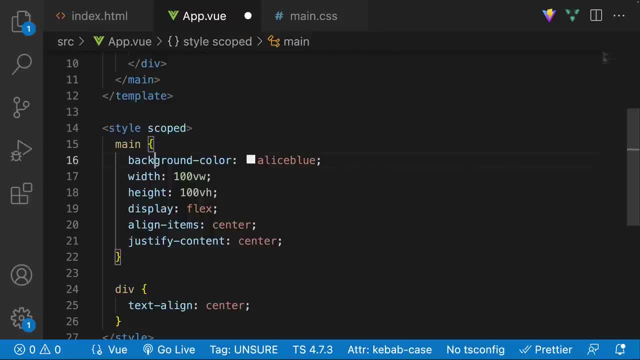 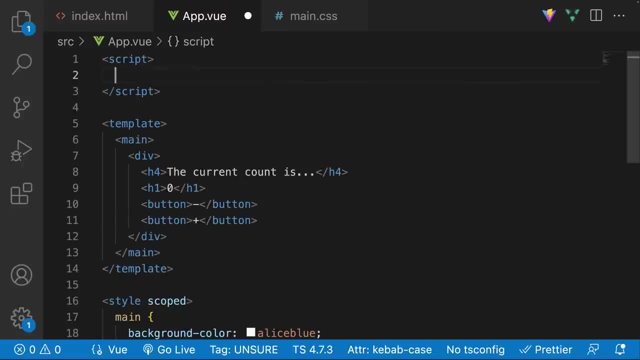 good convention to have JavaScript HTML and then CSS now how are we going to define our JavaScript well we are going to create script tags and just for now we'll talk about this later in great great detail but in order to get things to work just in this script tag this very first script tag we're going to do space setup so we're going to talk about exactly what this means a little bit later don't worry but we need it to get it to work so let's just go ahead and write this for now so the first thing that I actually want to do declare a new variable and actually utilize that variable within this HTML template right over here now specifically this is going to be the count variable so let's go ahead and create a count variable the way that we have always been creating variables so we're gonna say let's count and initially that is going to be equal to zero so now what we need to do is we need this h1 right over here to actually have the inner text of it be 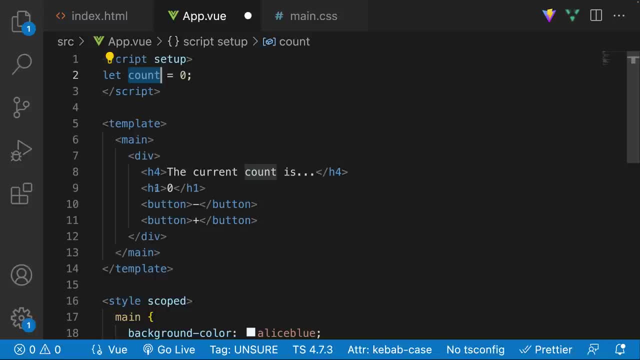 whatever the value is of this variable so how are we going to do that well before we did something like document dot get element by ID we gave this a particular ID like let's just say h1 whatever or just say one one and then over here we gave it an h1 one to get it and then we said we a a a a 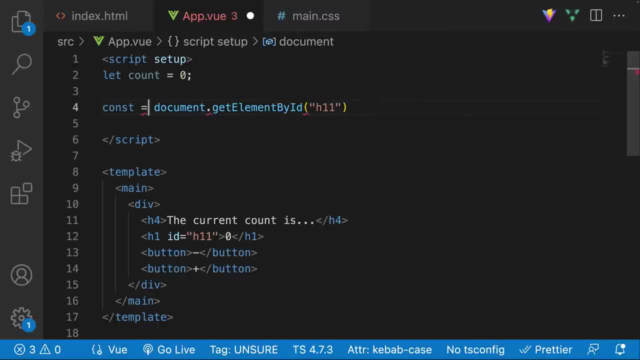 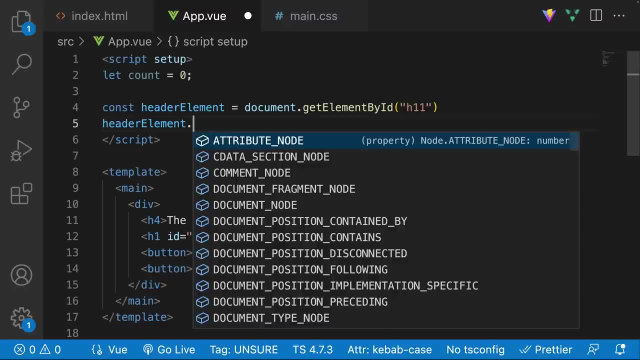 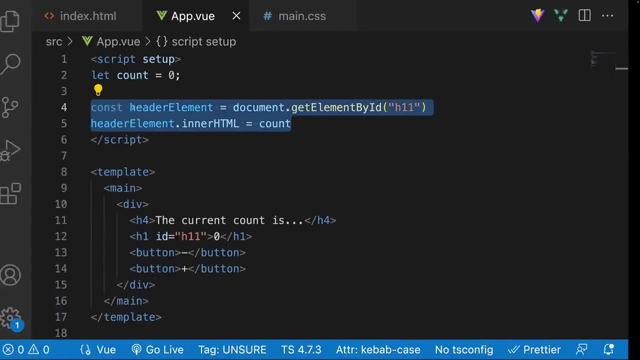 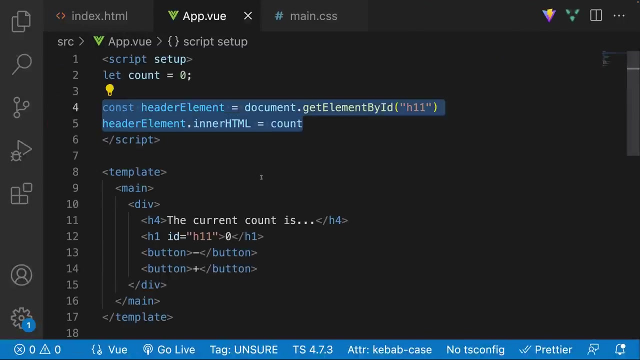 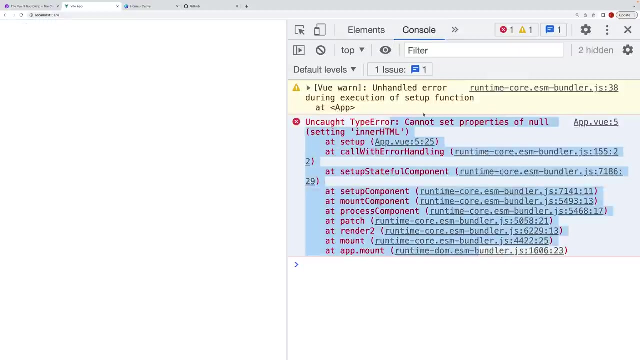 it to a particular we assigned it to a particular variable like something like header element and then over here we said header element dot inner html and we set that equal to the count that's what we did before so let's just go all the way over here and let's just see if this is working a okay it doesn't seem as though it is working so it seems like though it actually crashed something so if i were to inspect this and i go to the console you can see here we're just you know 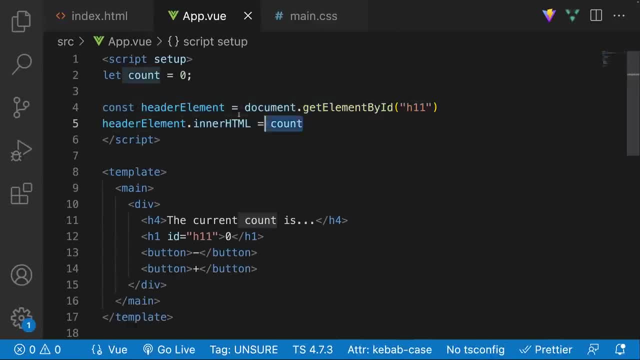 something is crashing so what we're going to do now is we're actually going to go ahead and completely remove this because this isn't the way that we are going to do things nowadays because 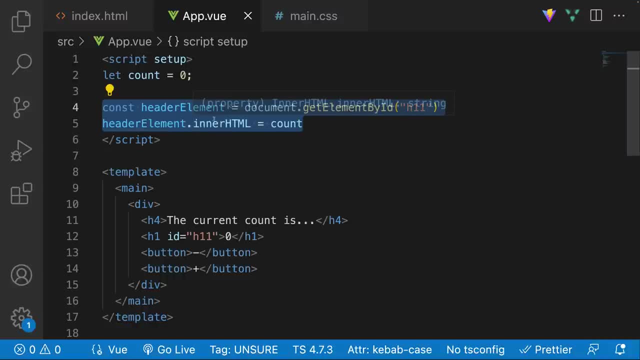 honestly this is the pain that we were trying to alleviate when utilizing view so what we're 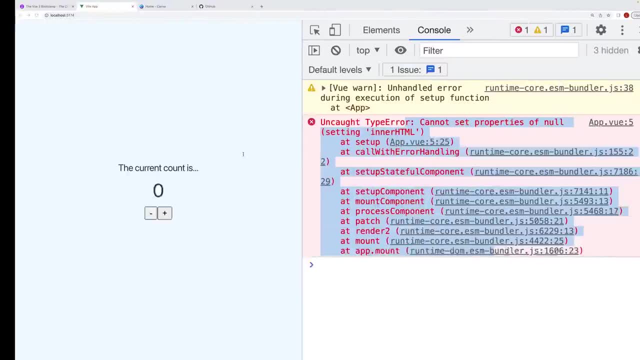 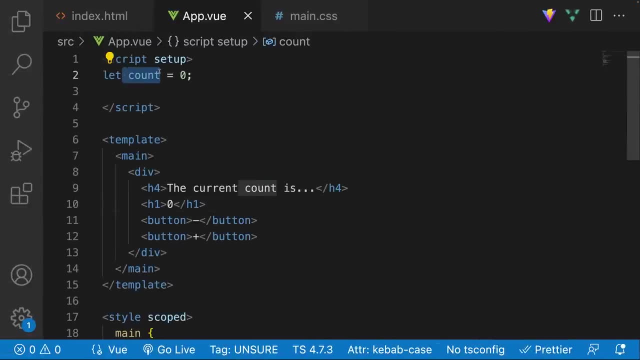 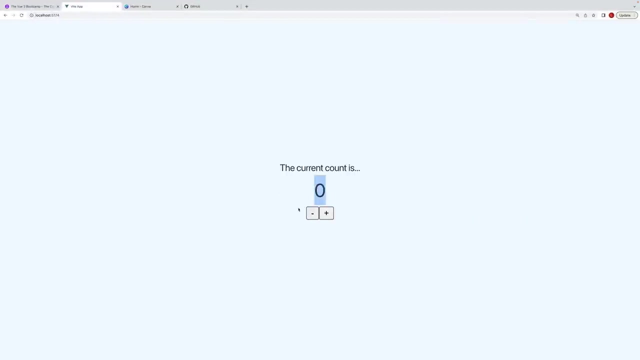 going to do is completely remove this let's also remove the id we don't need that as well you can see now everything is working a okay but still what i want to do is i want to get this variable the value of this variable within this h1 so how are we going to do that well we're going to do that really really easily so let me go ahead and get rid of this zero and i'm going to do an enter so within the h1 itself what we're going to do is curly braces so we have one open curly brace and then another closed curly brace and then we're going to do the same thing again so curly brace curly brace so we have two open curly braces and then we have a three open curly braces and then we have a three open curly braces and then we have a three uh another two closed curly braces and then within here we can actually add any of the javascript that we have declared within our script tag and this right here is going to actually act as javascript so for example if i say count it is going to take the count from here and parse it parse its value and set it as the inner html so if i were to save this you can see it is still zero and for example if i were to change this value to zero it would be zero so if i were to save this you can see it is 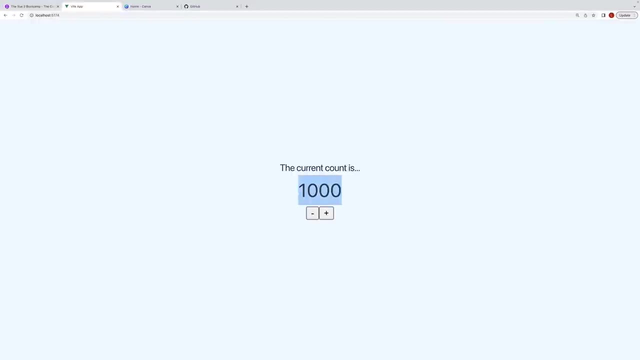 zero and for example if i were to change this to like a thousand you can see that it is well now a 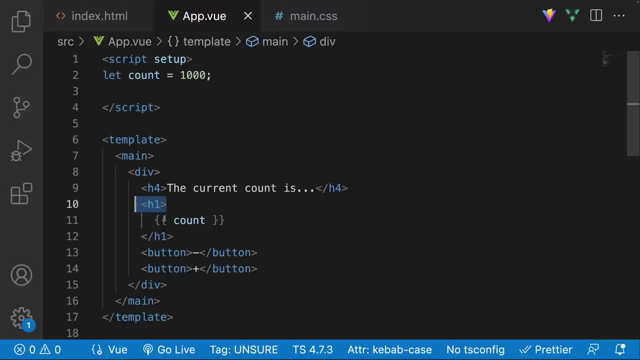 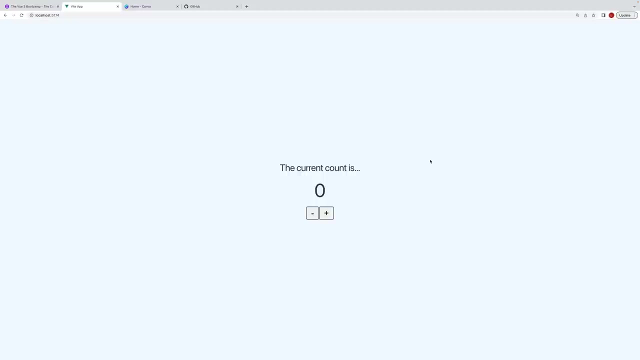 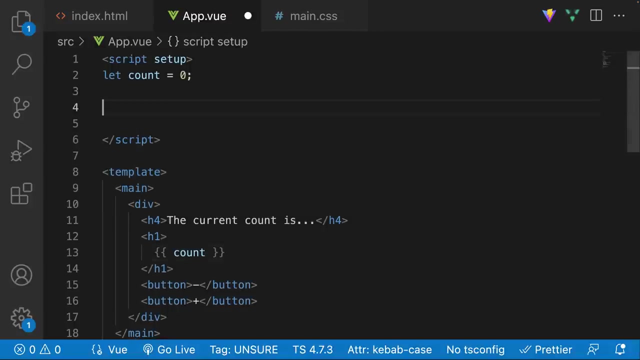 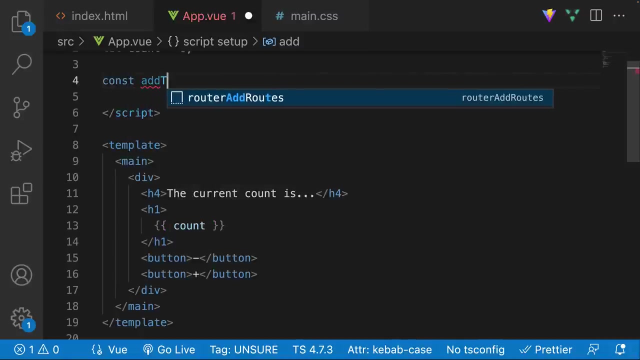 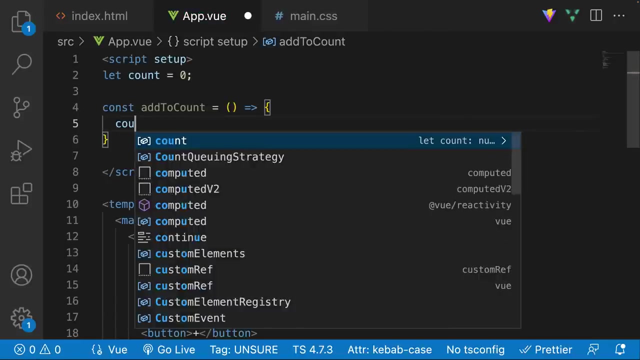 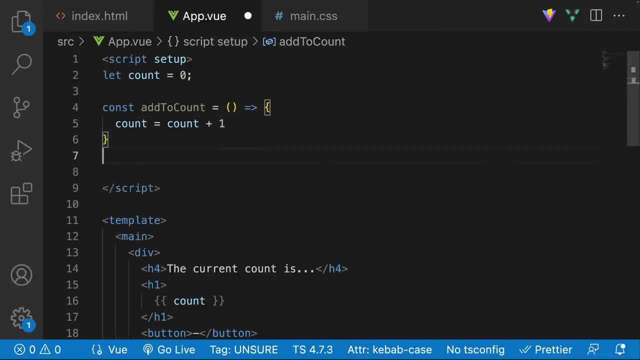 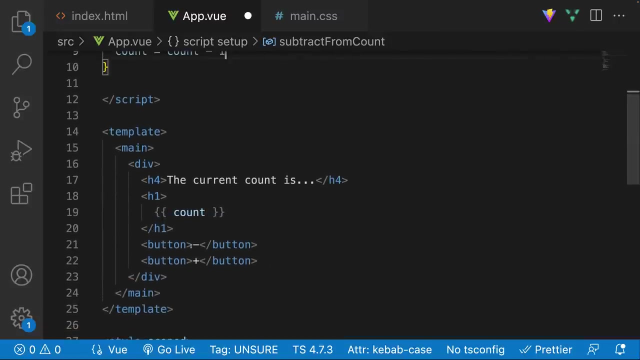 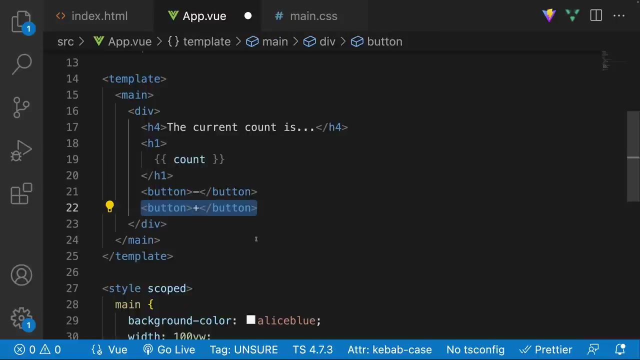 thousand how easy is that now i don't even have to find the html element set its inner text i can just do this right over here that right there is the powers of vue.js now let's go ahead and actually make our buttons functional so the first thing that i'm actually going to do is i'm going to go over here and i'm going to create two new functions and i'm going to call them view.js one to add to the count and then another to subtract from the count and whenever I press these buttons they should call the appropriate function so over here I'm going to say const I'm going to say add to count and let's just very simply make this an arrow function and I'm going to say count is equal to count plus one very very simple I could also do count plus plus but I think this is very explicit so that's how I'm going to say it and now let's also create another variable I'm going to say subtract or another function I'm going to call this subtract from count and let us say very simply that this is going to be count is equal to count minus one so these two functions are the functions that actually we want to call whenever we will press these buttons so typically what we had to do before is well find the buttons with a document dot find by id then we had to add an event listener to it and then we had to define the callback that we wanted to call 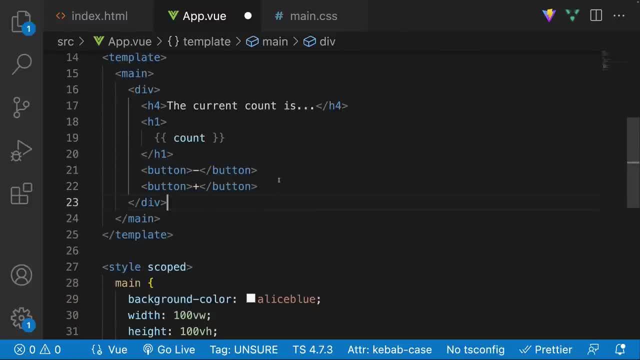 well with this as you can imagine going to be extremely simple not simpler I just fumbled my 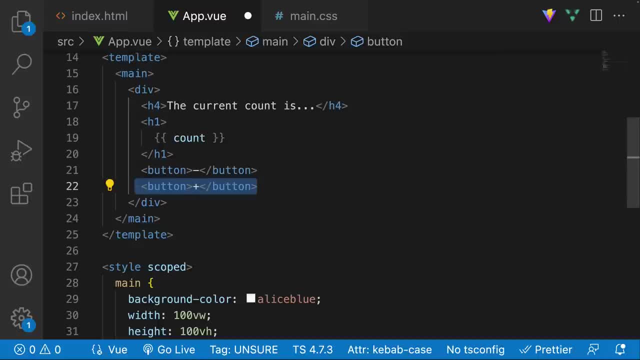 words there all right so over here what we want to do is we want to add some sort of listener 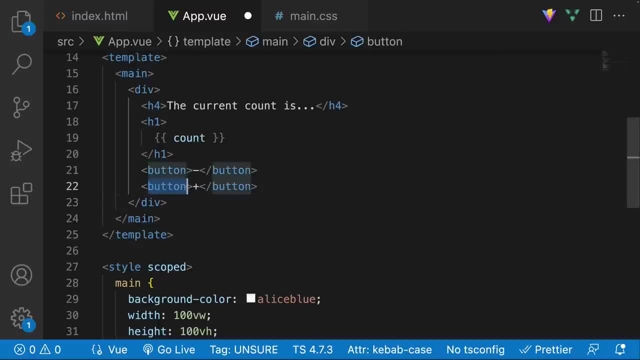 how do we do that well right on the button itself what we can do here is add a listener and we can add a listener by doing at and then over 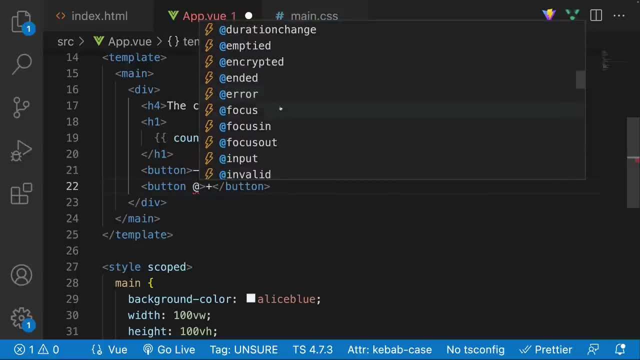 here we can see all of the listeners that we have saw before in the previous section where we built it with vanilla Js so they're all the same listeners now what I want to utilize is the 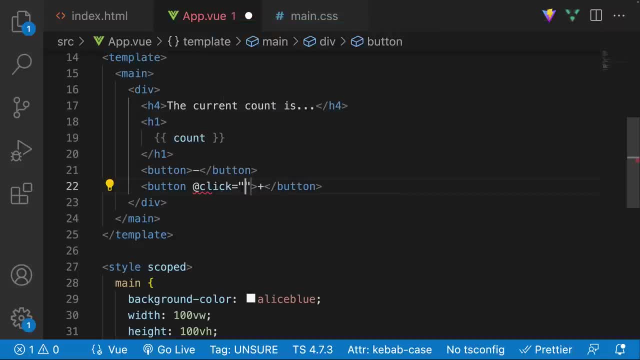 click listener and as soon as I do click it's going to say equals 2 and then over here some quotes now this is going to be an täggräns. 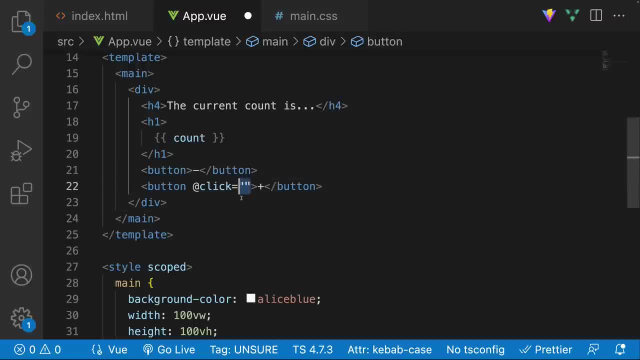 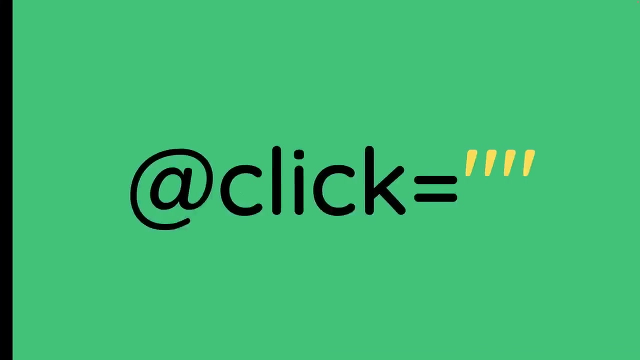 a little bit confusing because quotes we often symbolize with strings so over here i can add whatever string that i want well right here within these quotes we're actually not going to add any string because within these quotes it is actually javascript so over here we have this at click listener and it's equal to these strings and then within these strings we add valid javascript not any string and this is going to be pretty confusing because we're going to see other 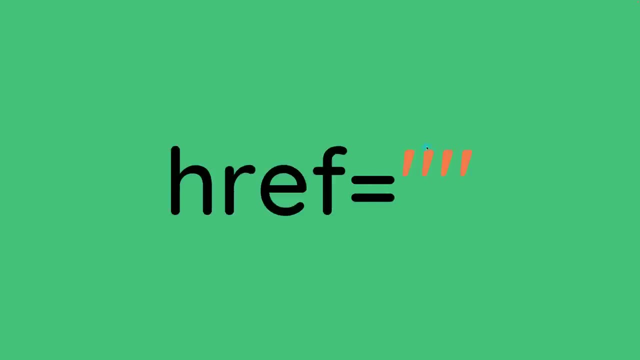 attributes out there like href that is going to be equal to and then these two double quotes and then within here we're going to add a string but within something like this it's going to be 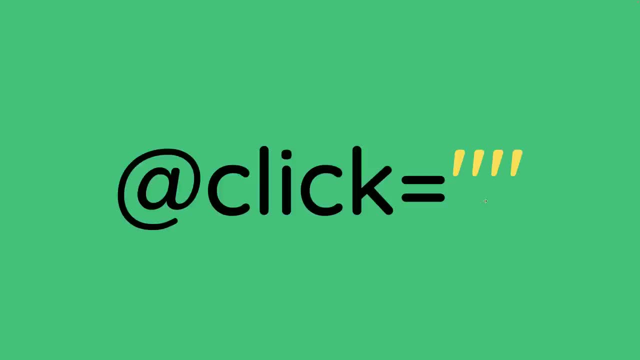 javascript so it's going to be a little bit confusing sometimes to distinguish exactly when we can add javascript within the strings and when to add a string within the strings but or within the quotes sorry uh but uh but don't worry later on we will figure out how to add a string to a quote and then we're going to add a string to a quote and 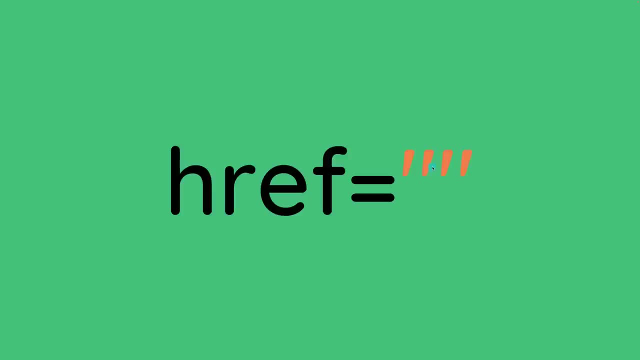 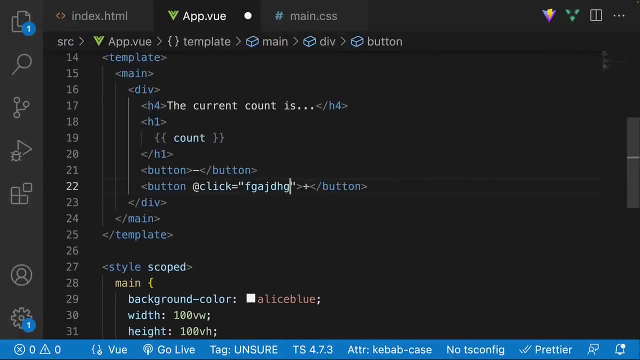 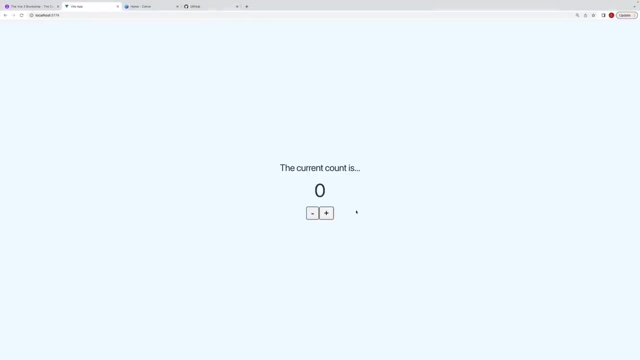 exactly when we add js in the quotes or when we add just the regular string within the quotes so right here again this is not going to be a string i cannot add like anything that i want because if i went ahead and actually saved this and i refresh unless i actually went ahead and clicked on this button uh it should give me an error in the console let's go over here and it's actually 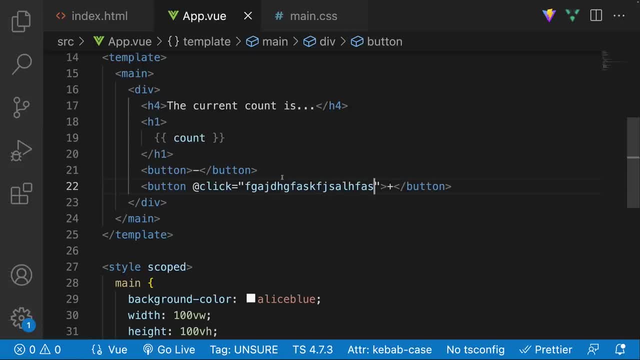 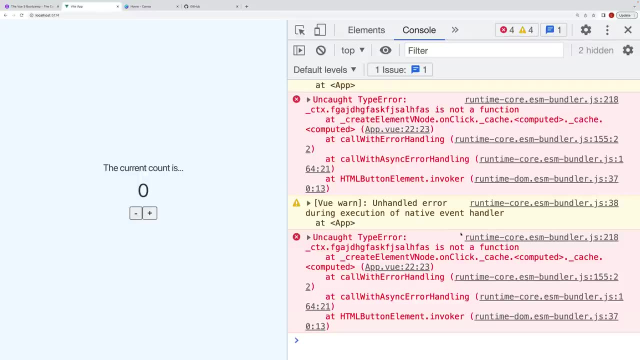 not giving me an error but i guess it's just not really doing anything let me just kind of like invoke it like so and let's go here you can see here right away it's giving me an error because 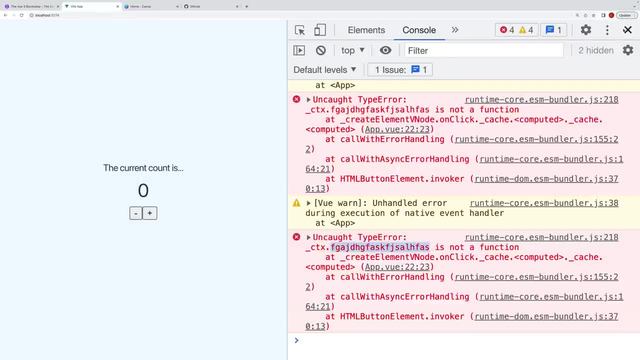 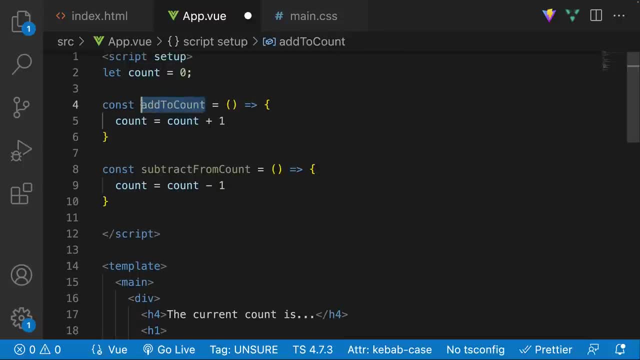 this is well javascript and not a string so we can't really add whatever it is that we want well what i want to do is i want to call this function right over here add to count whenever 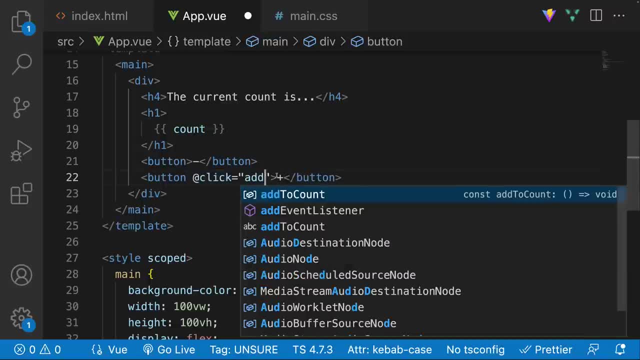 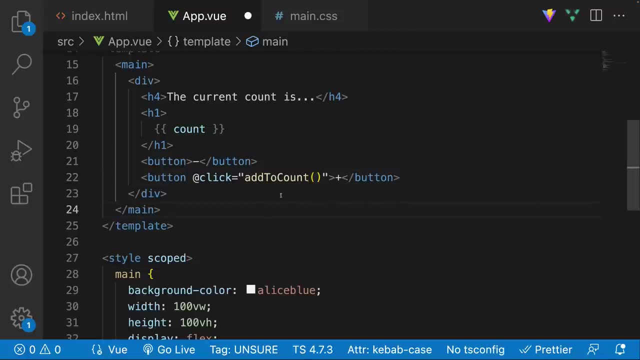 i click this button so what i can very simply do now is just add that function i can leave it like this or i can just go ahead and call it and invoke it view is smart enough to figure out that hey when you click this i want to call the add to 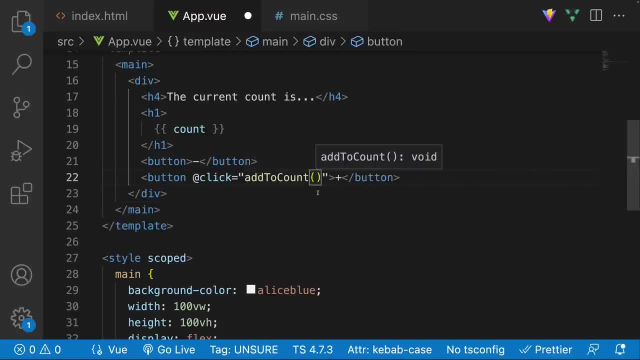 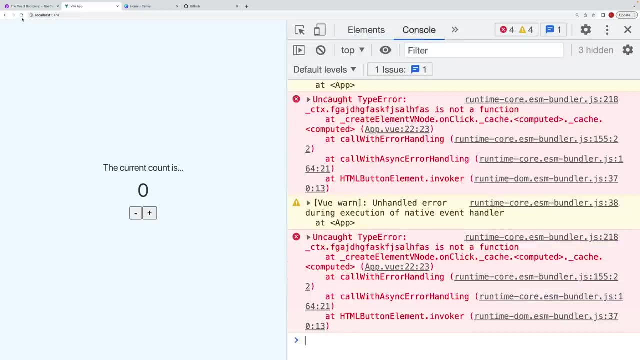 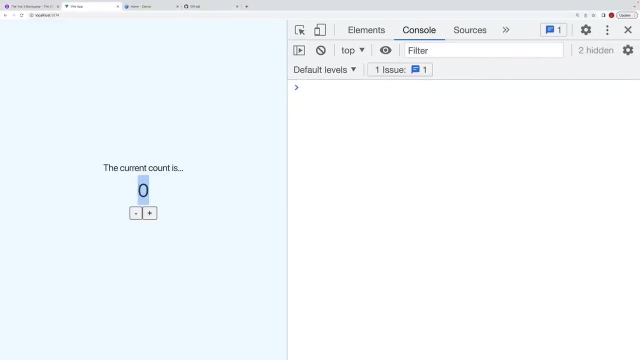 account function or you can do it just the same thing these two are just the same syntactically so now if i were to go over here and let's just do a quick little refresh or remove this now you can see i get no error however however uh well the count isn't updating so am i really calling this function well yes you are 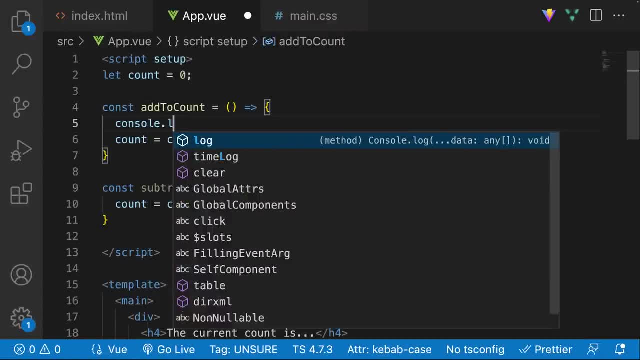 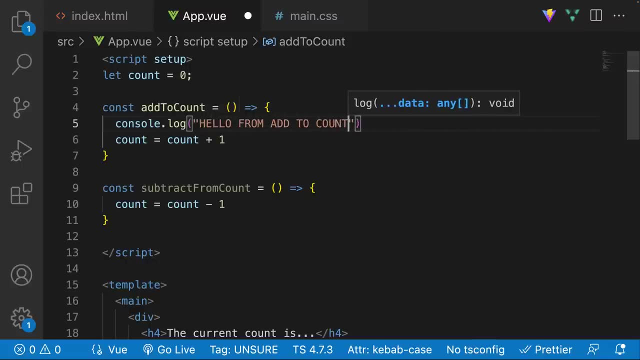 yes you are indeed calling this function and i can actually prove it to you by adding a console so i'm going to say well hey hello from add to count so now let's just do a quick 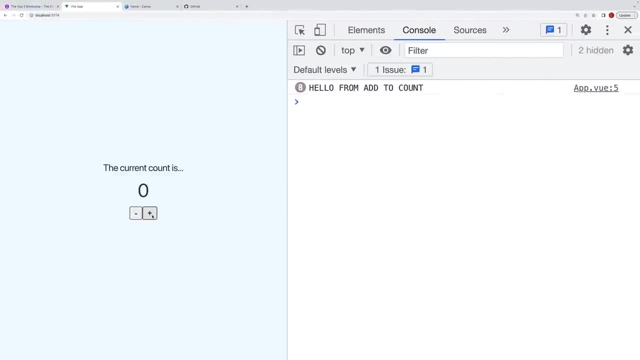 little refresh and when i click it you can see here it is indeed calling this function but again the count isn't updating and there's a very good reason for this and we'll get to this reason in 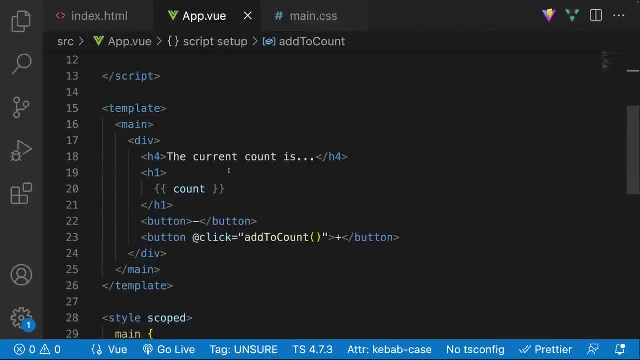 the next video but for now let's actually do the exact same thing 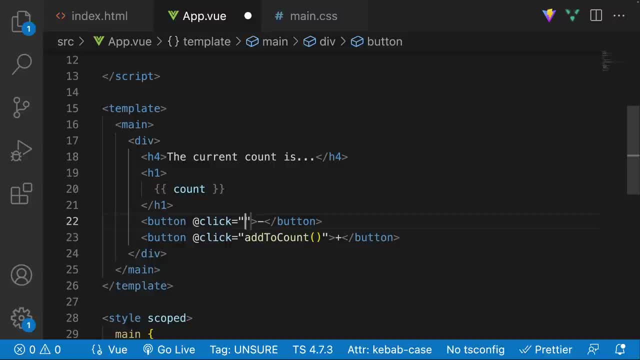 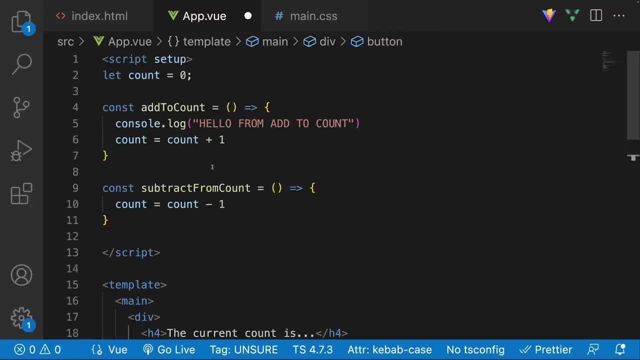 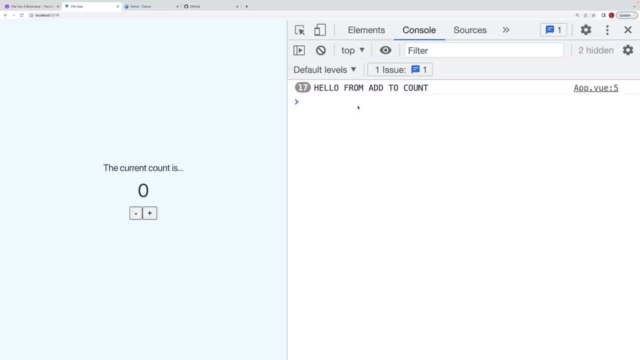 the subtract so over here let's add a click handler and this time i want subtract from count i'm going to just go ahead and invoke it so let's just go ahead and remove this actually let's keep the logs and let's go here and i'm going to say subtract from count just so we can see that this is actually uh calling the correct uh function so you can see here we're calling it and then when i click on this we're calling subtract 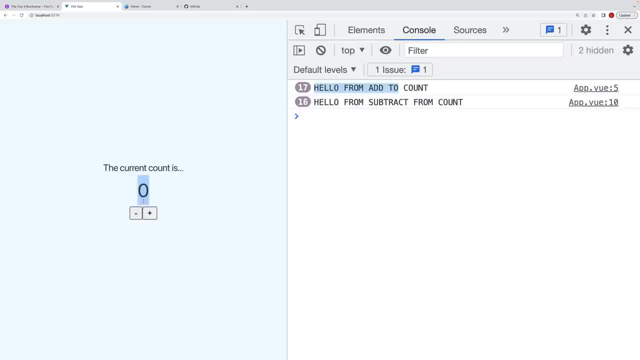 from count but again nothing here is updating why is that let's get to it in the next video 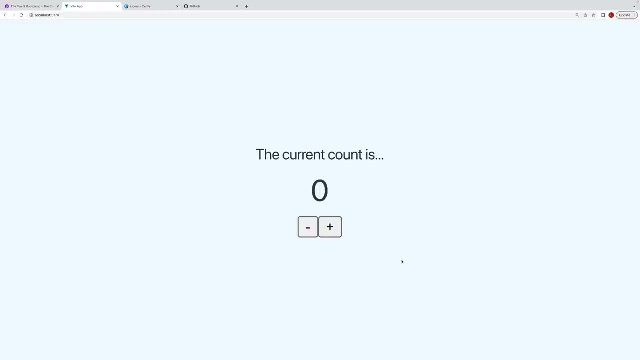 so we added these functions and they do indeed seem to be working however they're not really updating the counter within our application so when i click on plus it is indeed calling the function but it is not updating it onto the screen similarly over here when i click on minus it is also not updating it onto this screen so what is going on here well let's actually look at a diagram 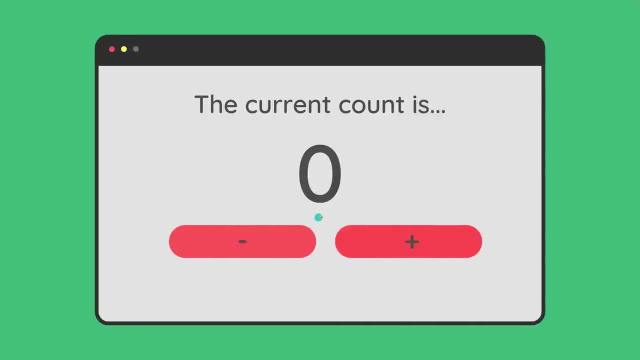 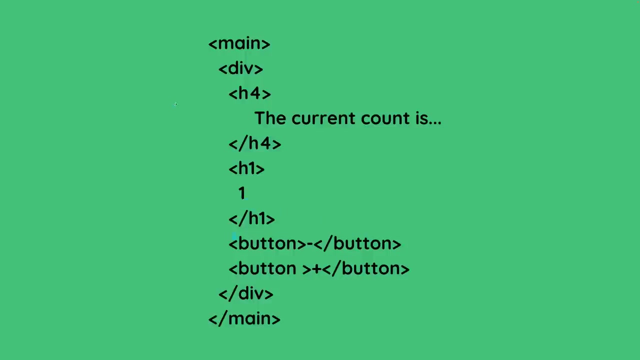 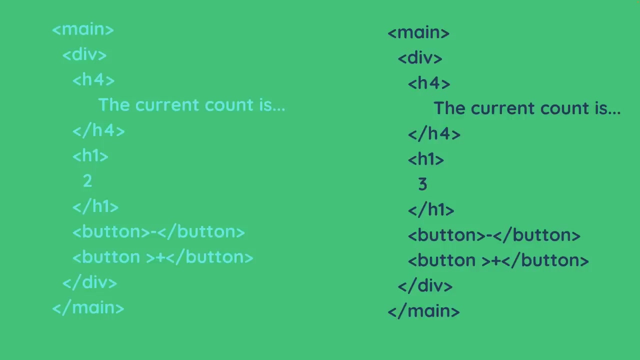 so right here this is the current state of the application and notice that i said something very important state so currently our application is in a state where the counter is zero now when i click this button over here i expect that the state of the application changes so that the current count is one and similarly if i click it again then i expect the state to change so that it is now two and of course this is going to also change inside of the html themselves so when i click on the plus button i expect this to be one when i click on it again then over here i expect this to be two so how does view actually update the state of our application so that it is reflective inside of the html well this is what it does so let's say this is our old state currently our count is two and then i click on the plus button and then right over here this is the new state so what does view end up doing in order to actually show this change in state within our browser well this is what it does 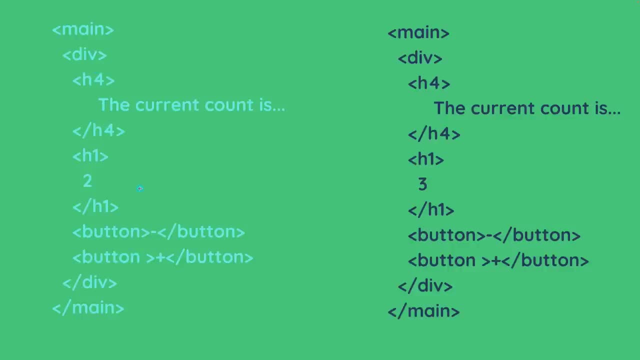 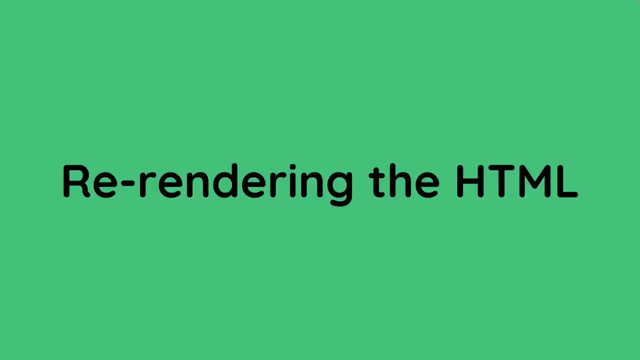 it takes the old state all of the html and it pretty much just throws it in the trash it completely deletes it and then what it does is it re-renders the new html with the new state so it re-renders another html exact same html tags but this time with the new state and that is how we will actually see this change from two to three through this re-rendering process so again then Vue is going to update the state of our application by re-rendering the HTML. 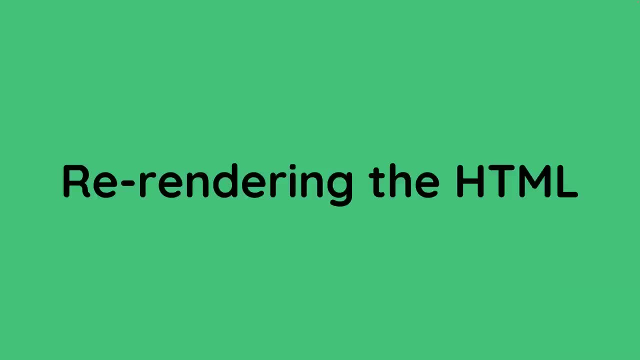 Now, this is something that we probably do not want to do often, not with every single operation, because continuously re-rendering our HTML can actually slow down our app, and it's just not great for performance. 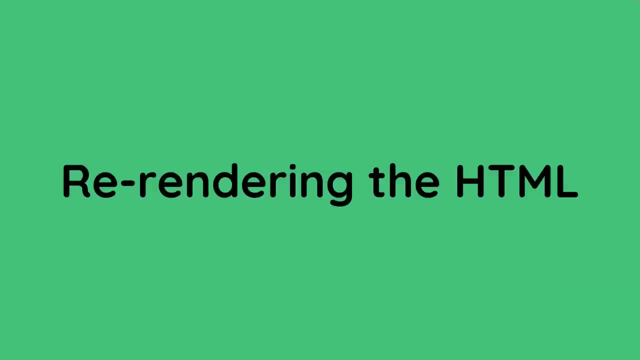 So Vue is smart. Vue is like, you know what? I'm only going to re-render the HTML whenever some sort of state within our application is updated. 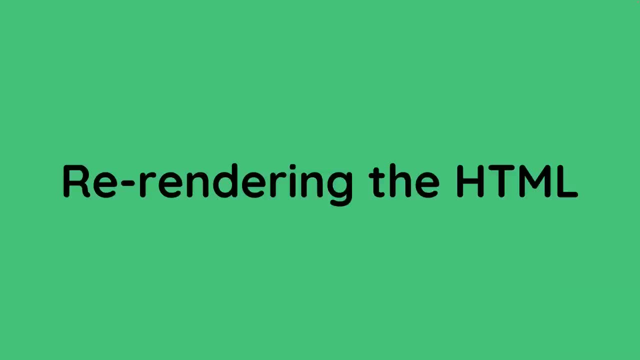 Anything else that occurs in the JavaScript, that's a-okay. We're not going to re-render. I'm only going to re-render when some state is updated. 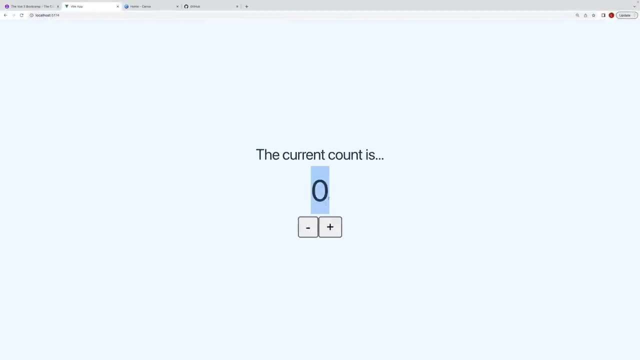 So that begs the question, well, this right over here is state, right? Why is this not updating? Well, Vue has no idea that this is... 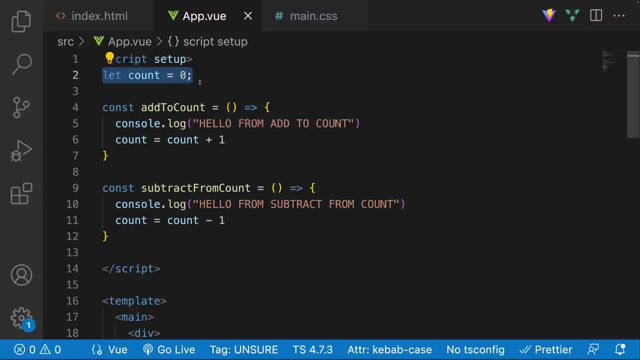 It sees this as just a regular JavaScript variable. It does not see it as a piece of state. 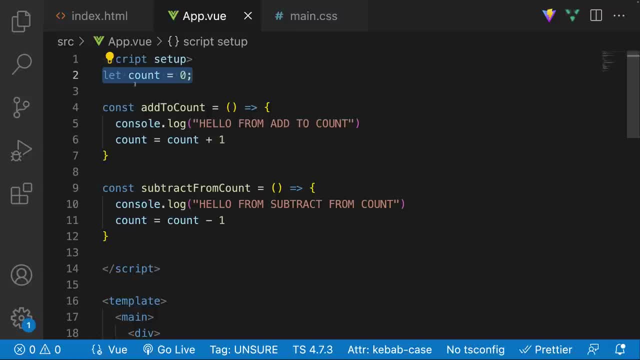 So what we actually need to do is define this as a piece of state. So to define this as a piece of state, what we're going to need to do is import something. 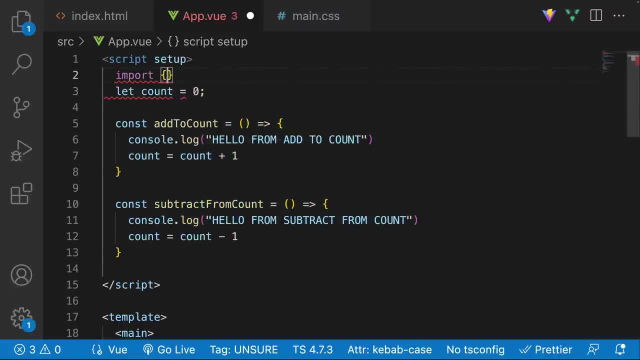 Let me actually tabulate this. It might look a little bit better. Is import something from the Vue library that we have just installed. And specifically, we're going to import something called... 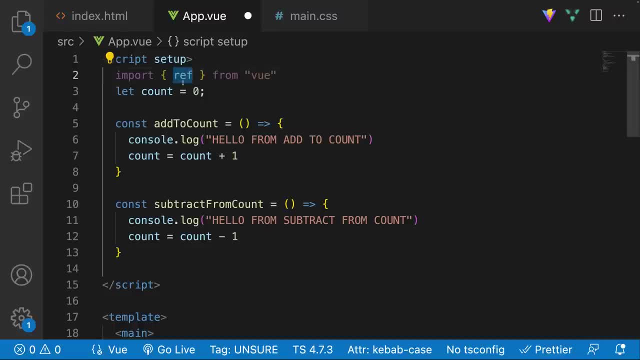 And we're actually going to utilize this over here in order to create or to transform this into a piece of state. So how are we going to do that? 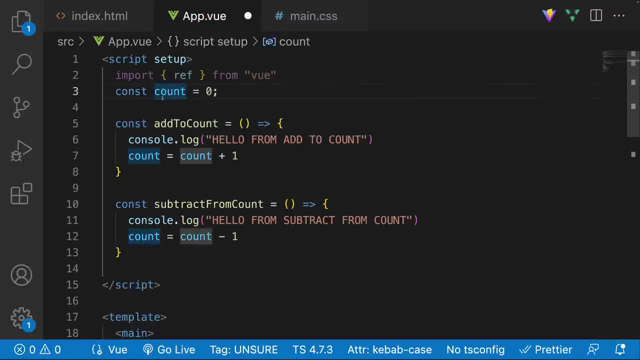 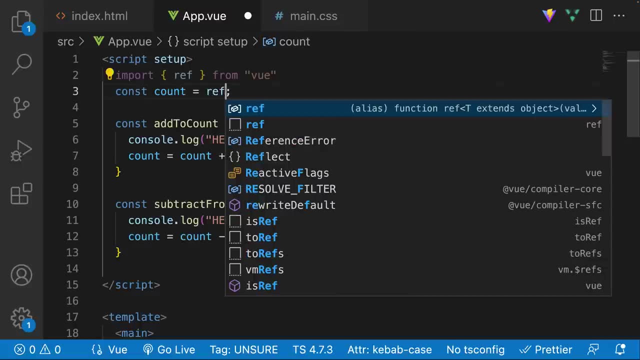 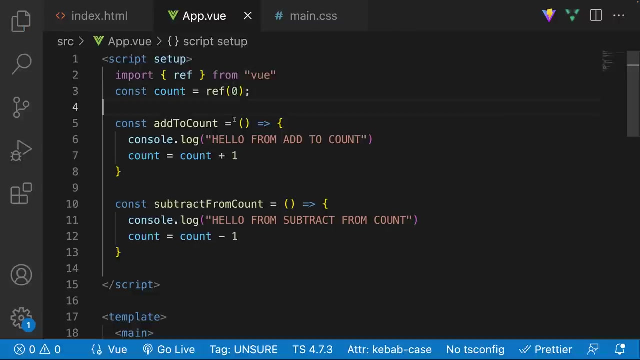 Well, the first thing I'm going to do is I'm actually going to change this to a constant. And I'll show you why in a bit. And then what I'm going to do is instead of having this be equal to zero, I'm going to say that this is equal to ref. I'm going to invoke ref. And then I'm going to say zero like so. So now if I were to save this, you can see that the application still works A-OK. 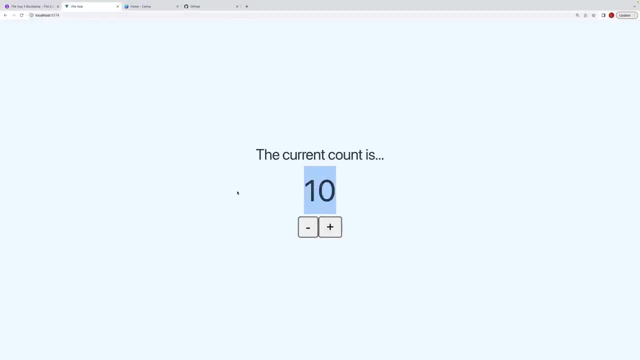 And if I went over here and let's say I change this to 10, you can see that this is updated A-OK. 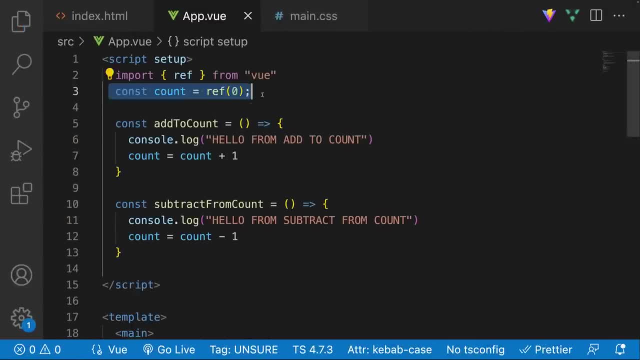 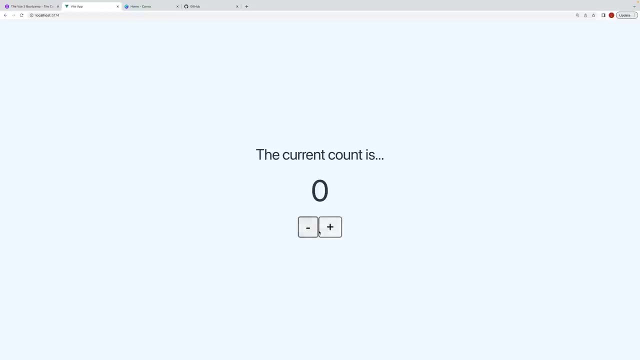 But this time, Vue actually recognizes this as a piece of state. However, now when I click on plus or minus, of course, it's still not getting updated. So what is going on here? 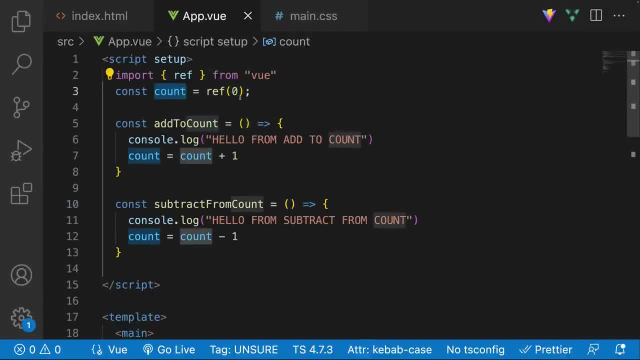 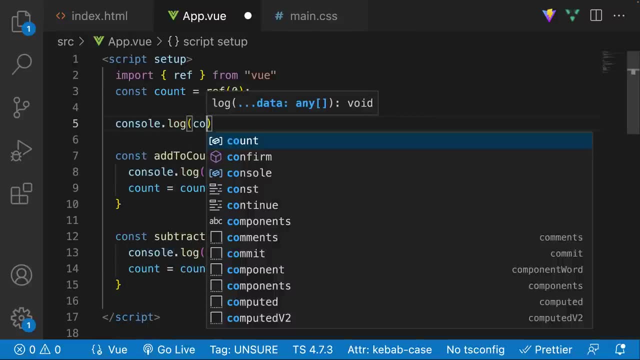 Well, this count over here actually isn't equal to zero. Indeed, it is actually equal to some sort of object. And let me just go ahead and console.log the count just to prove it to you. 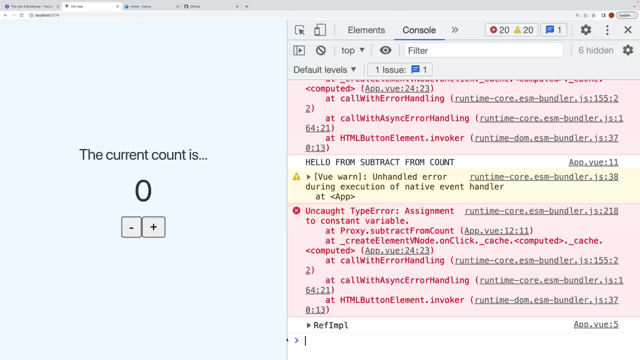 So whenever I actually declare some sort of variable as a state, 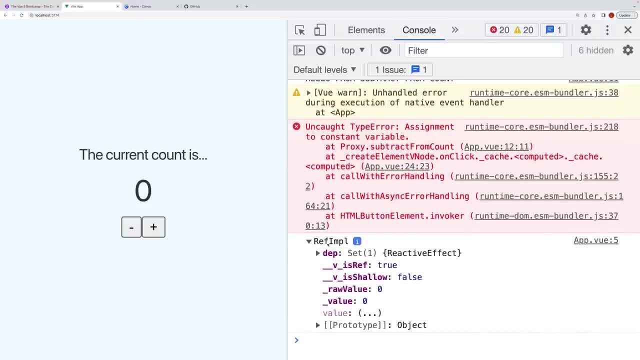 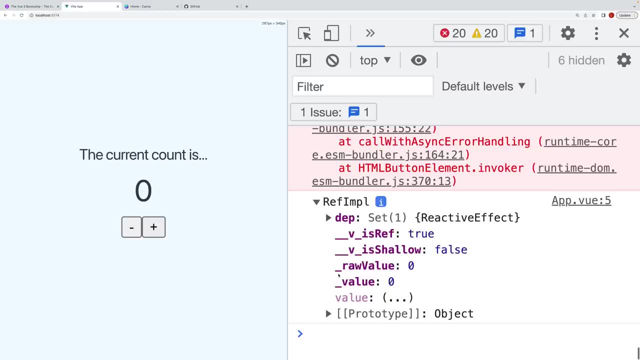 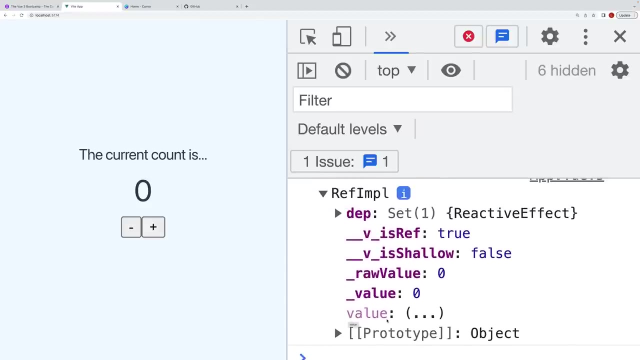 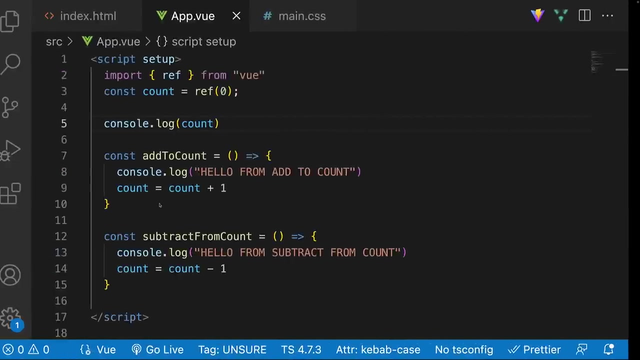 it actually has this object value. And this is going to be of type ref.imlp. Not really sure what that stands for. Now, specifically within this object, let me zoom in here. Within this object, there is going to be, well, a property on it called value. And that indeed is, well, the value over here. That we want to update. So instead, what we're going to do is we're going to say count.value. 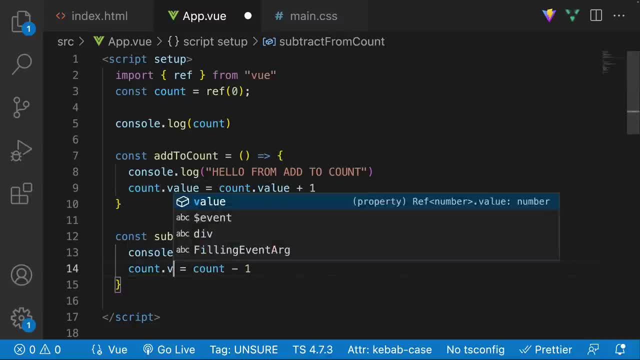 And then here, count.value. And then over here, count.value is going to be equal to count.value minus one. So that is what we want to update. 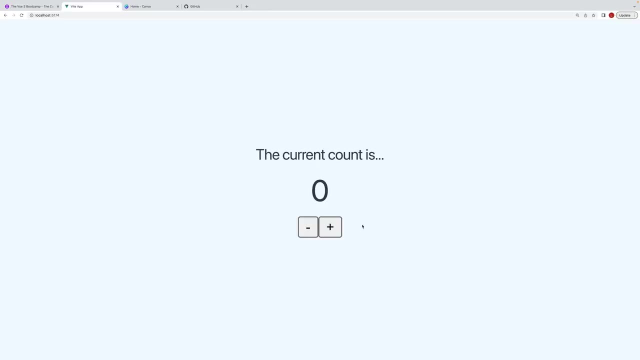 So now, if I were to refresh this, and I were to click here, you can see now it is actually updating that state. And it is triggering that re-render. 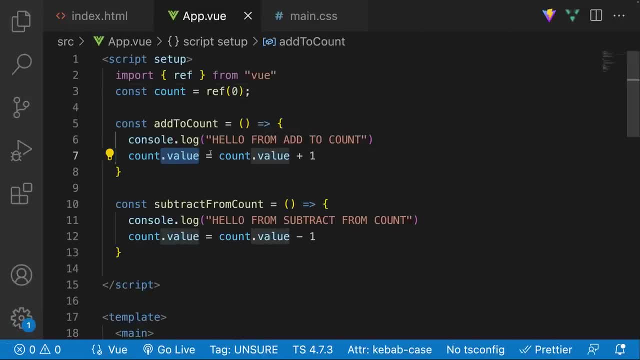 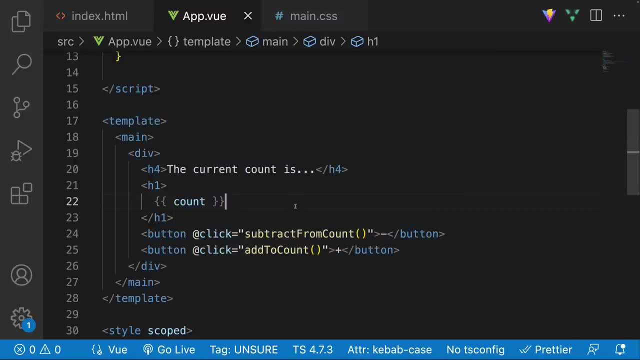 Now, you might say, well, what is this? You might be thinking, why in the world do I have to define value over here, but I don't have to define value within my HTML template? Well, within the HTML template, whenever I put any piece of state in there, it just extracts the value of it. 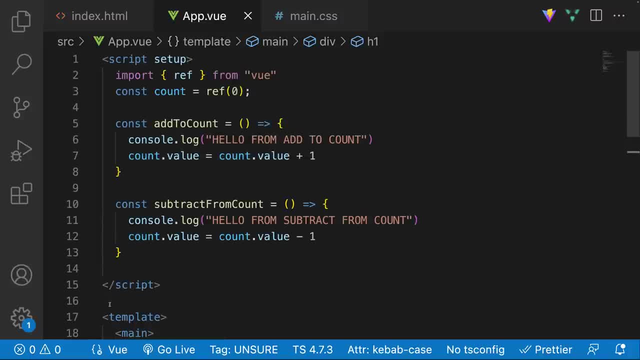 Because it just assumes that you do not want to use anything but the value. But within the JavaScript, we might want to use some other things. So we have to explicitly say that we want the value. 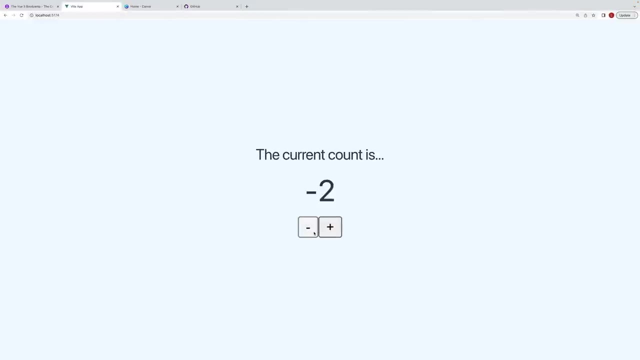 All right, so that's pretty much it. And we have pretty much, well, replicated, our entire application. How terrific is that? 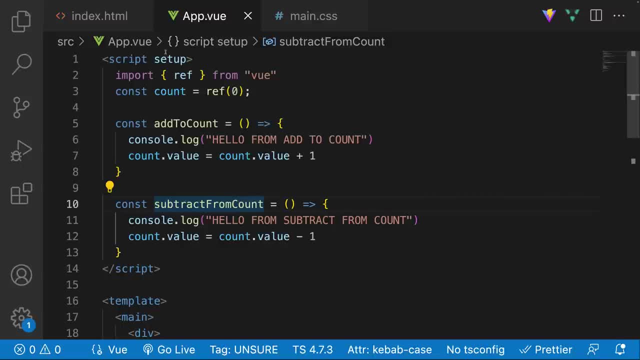 Now, the only thing that we are really missing in understanding is this setup. And tell me, and trust me, this is going to be quite a bit of a story. So let's talk about it in the next video. 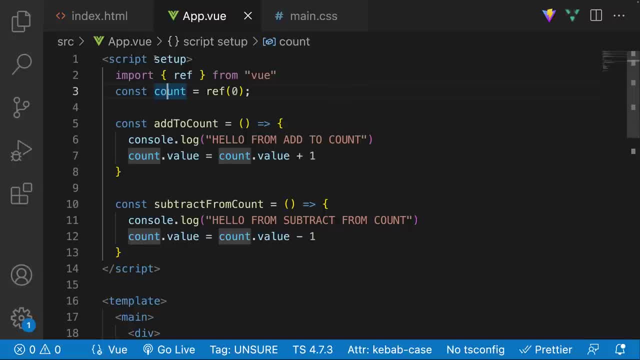 The last mystery that we need to discuss is this right over here. This setup keyword that we had to add to the first script tag. So let's first actually discuss exactly why we even need the script tags. Well, we need the script tags, at least in this case, to define our state as well as to define our handlers that are going to update our state. Then within the script tags, we also use these handlers as well as state in the HTML. 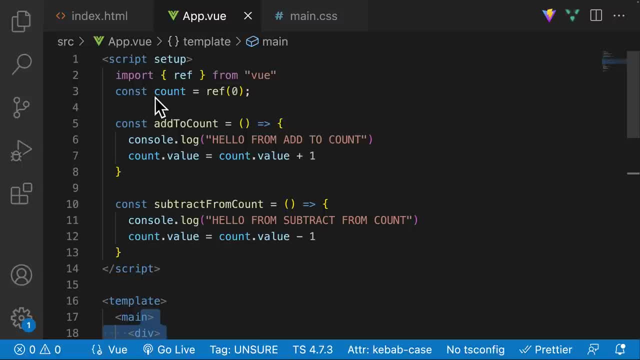 Now, there's actually two different ways that we can define our state as well as our handlers. 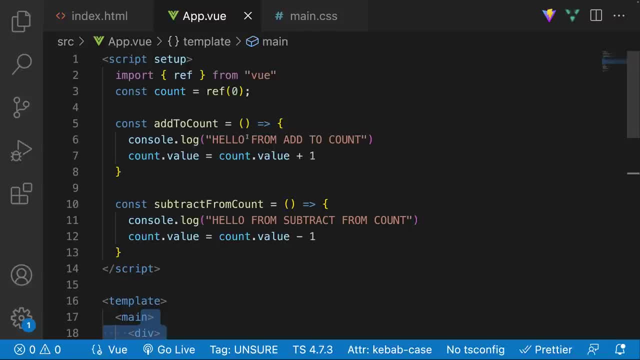 And it actually depends. On a certain option that you use. 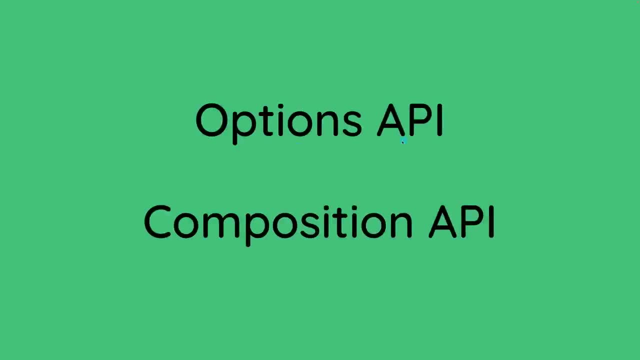 So there are two options. There's something called the Options API, and then there's something called the Composition API. 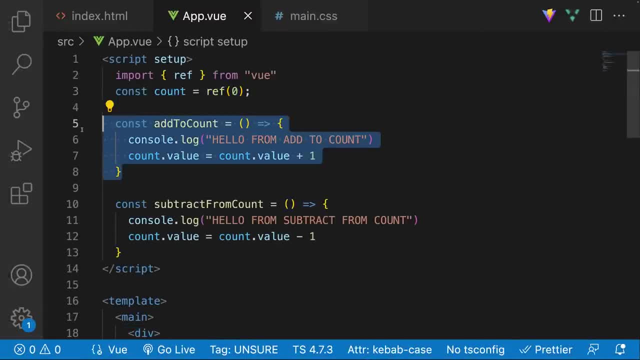 Now over here to define our state as well as our handlers, we used the Composition API. 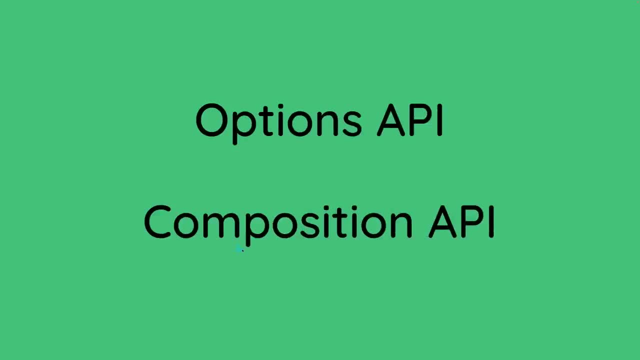 The Composition API is the new kid in town, and it is the way that Vue applications are going to be built in the future. The Options API is. kind of the old way of doing things you're still going to see it all over the place because it is 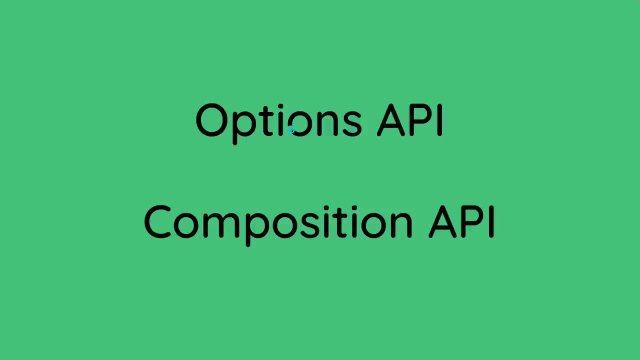 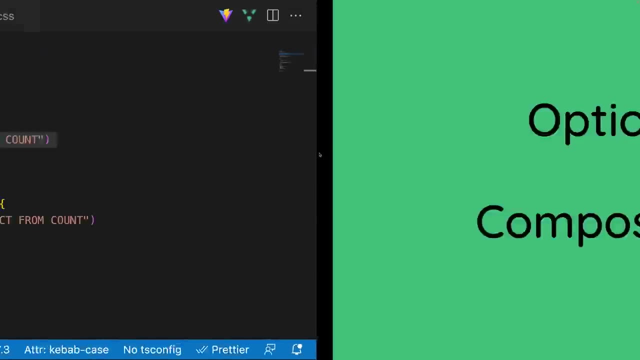 still pretty popular but i think it in in the future it is going to be replaced by the composition api and you know what i'll show you why so let's go ahead and actually quickly replicate what we 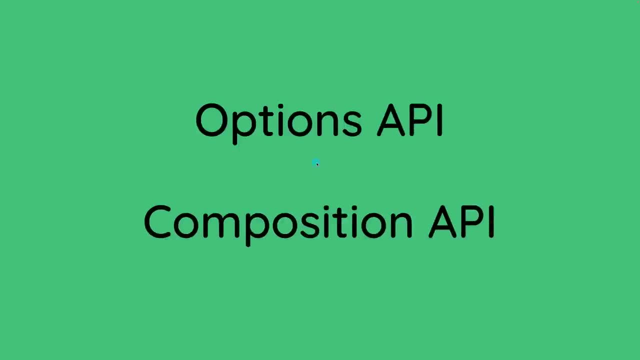 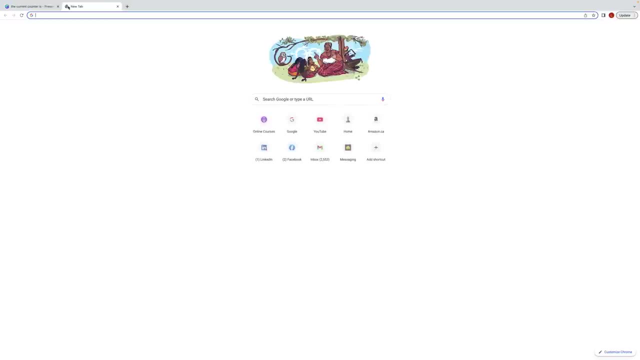 did over here in this script tag but with the options api so i'm just going to quickly comment this out and let's go over here to our application to localhost 5143 and of course nothing is working 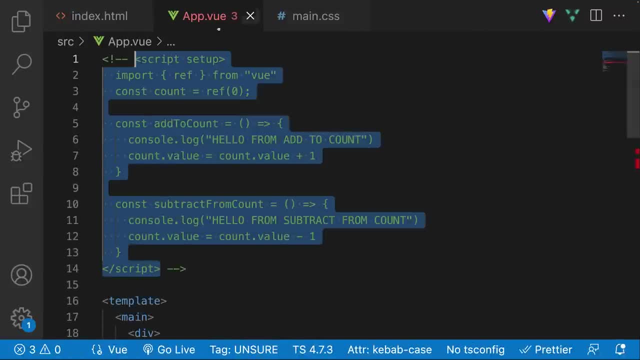 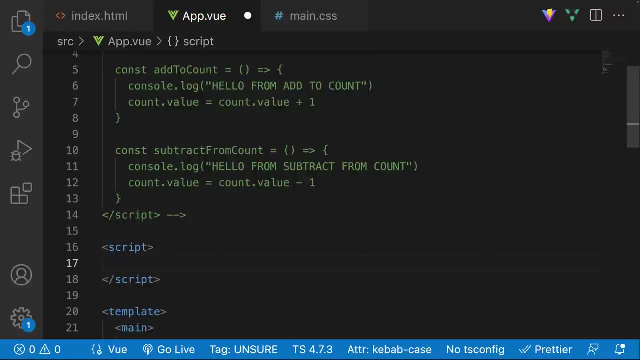 and actually our our count isn't there because well we removed that variable so now what we're going to do is we are going to create a script tag so let's create a script tag and then within 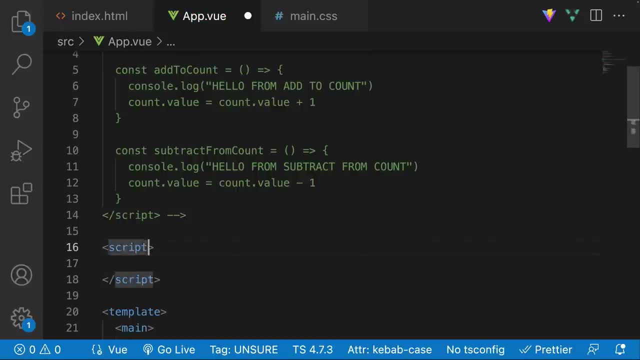 this script tag we are actually not going to add the setup instead what we're going to do is very simply export default and then we're going to invoke it and we're going to export a object now within this 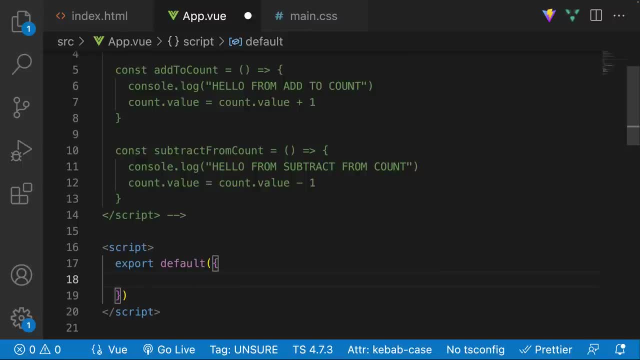 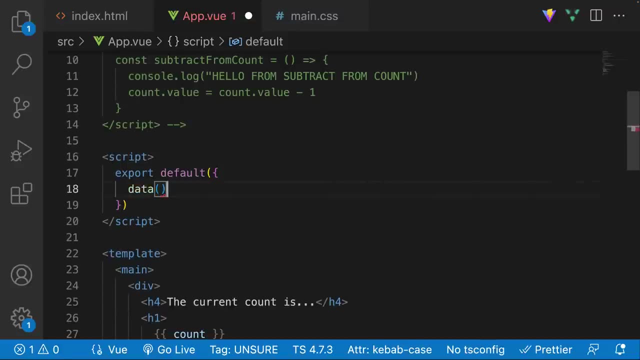 object we're going to have a bunch of different properties and methods now in order to store our state what we're going to do is create a method called data and this method is going to return 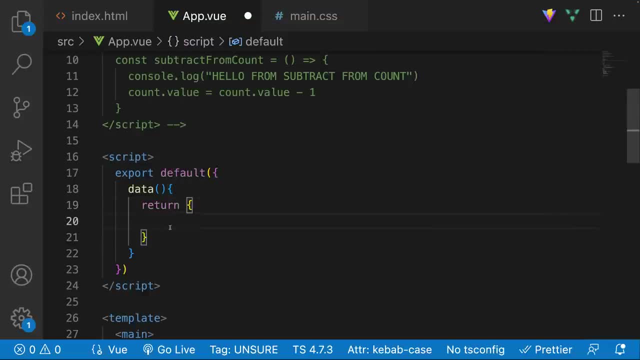 an object that is going to contain all of our states and their respective values in key value pairs so instead of defining it like this so 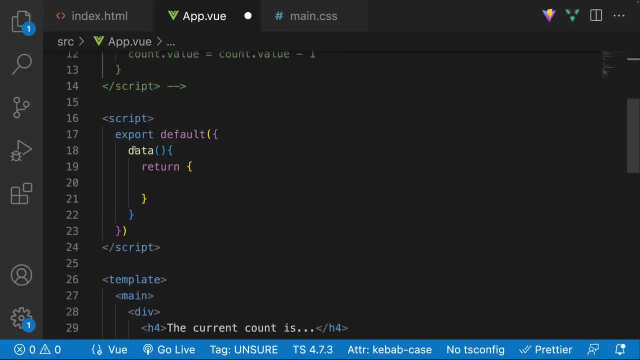 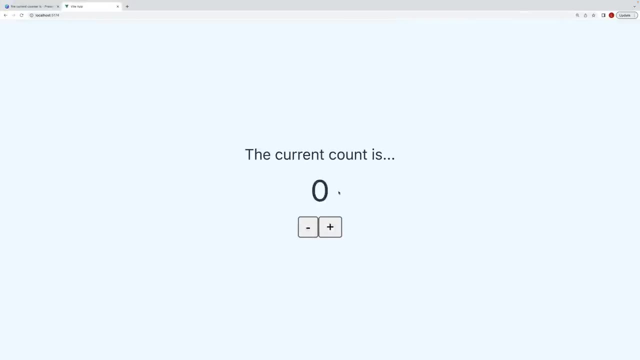 const count is equal to ref we're going to define our state within these objects so it looks something like count and then zero so if i were to save this you can see right away now we actually 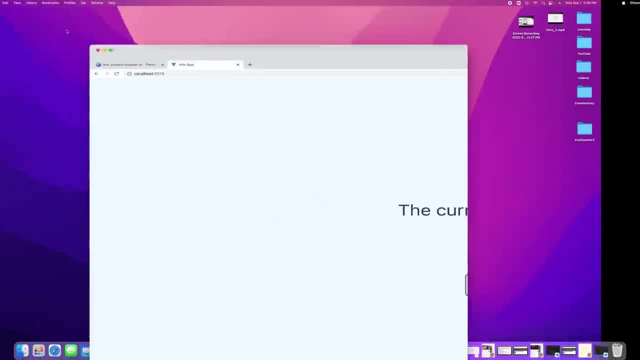 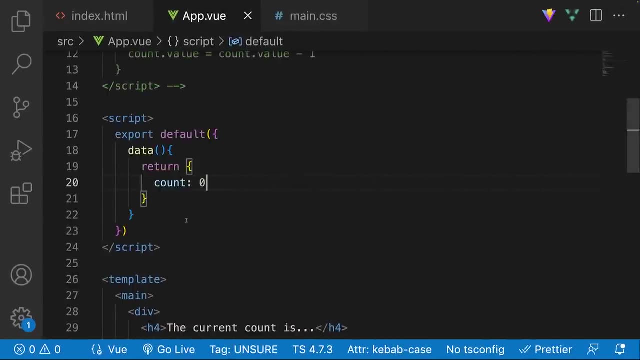 have the count all right let me actually just move this so i don't have to keep going back and forth and now i have to move this and there we go okay so that this is how we define our state in the 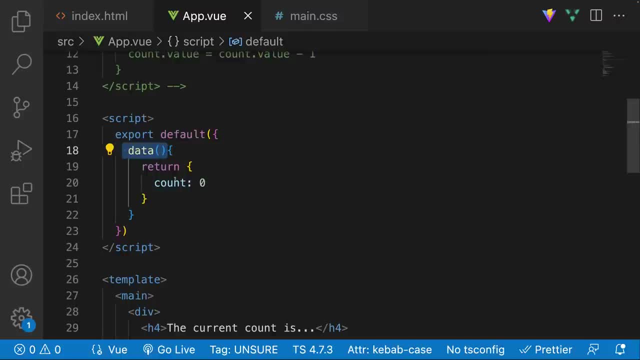 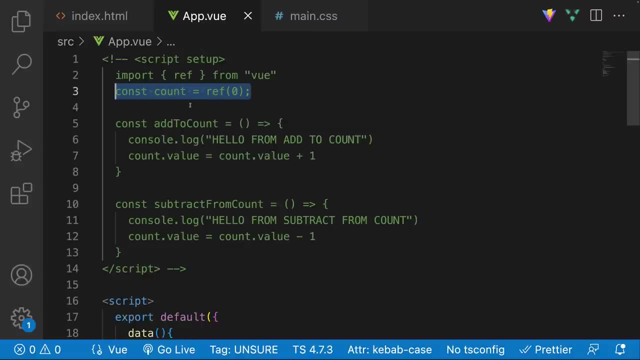 options api we define it in this data method now personally i honestly prefer this way over here it just looks cleaner and it just looks like normal javascript where this just looks like some sort of 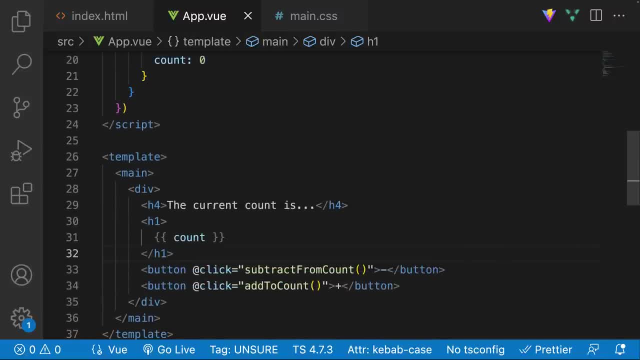 magic is happening in order for it to render onto the html template okay so that's the data but now 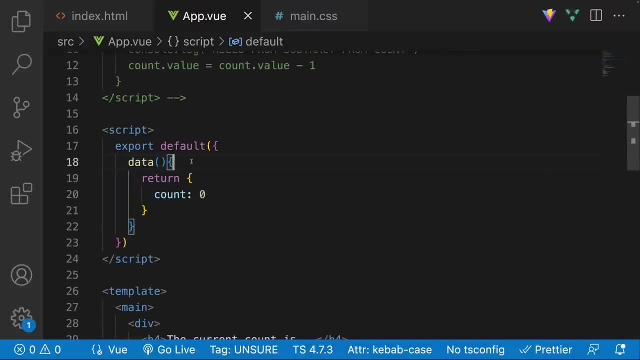 what we want to do is we want to define the methods so let's go over here so right after this data method we're going to create a methods property and this is going to be an object and 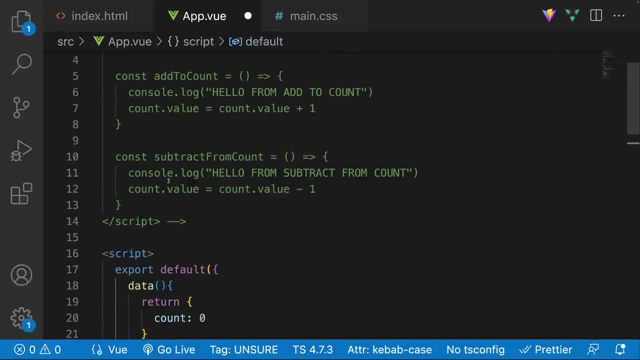 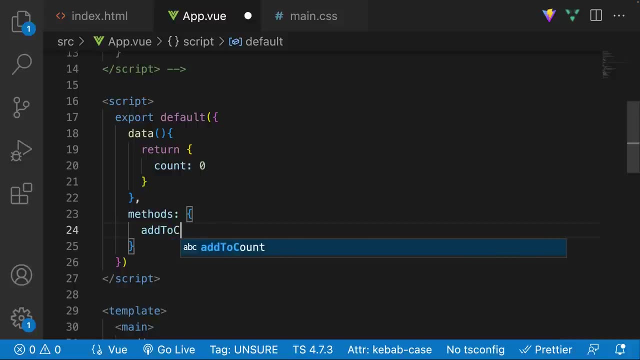 then within this object we're going to have all of our different methods so i'm going to say add to count so add to count and this is just going to be a method and what i'm going to do is just 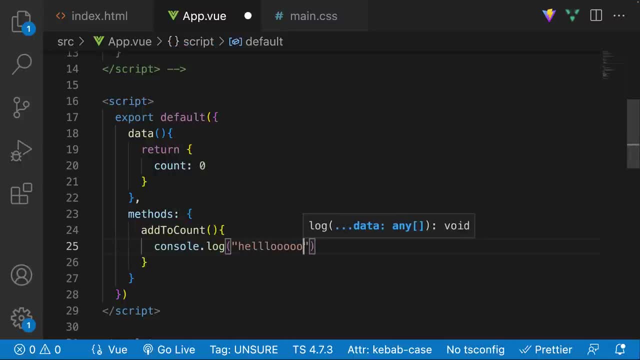 console.log hello hello so let's go over here and just to prove to you that it works and we're going to 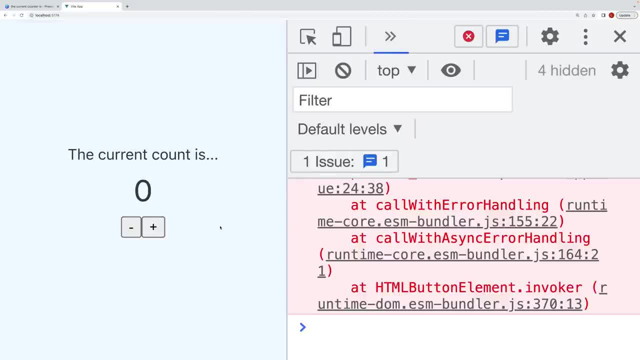 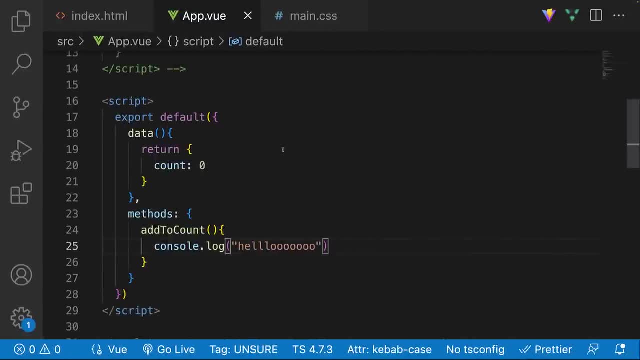 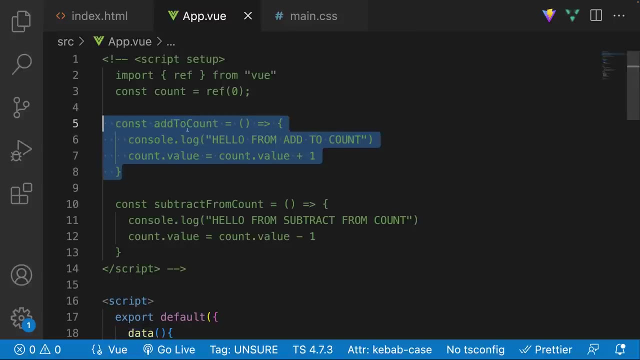 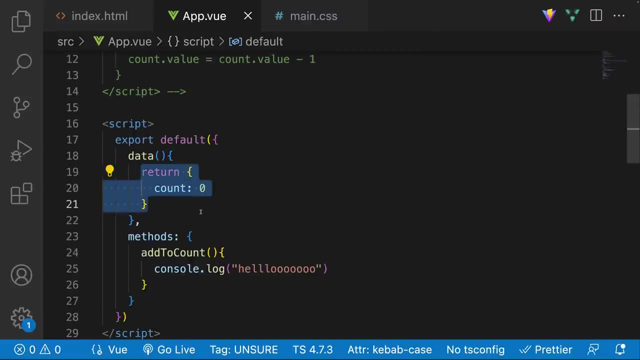 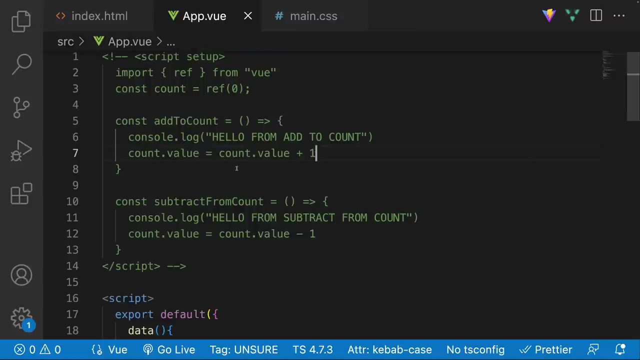 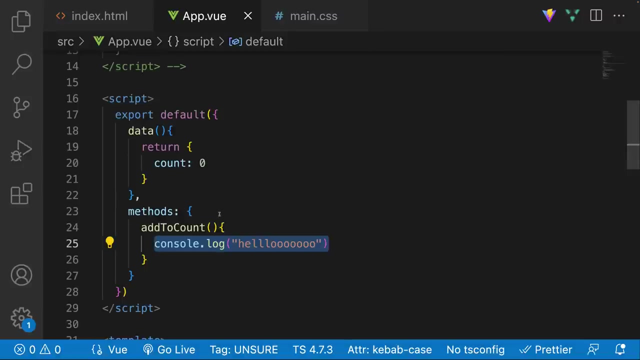 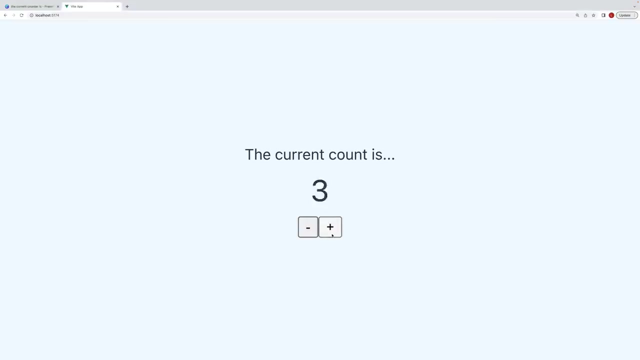 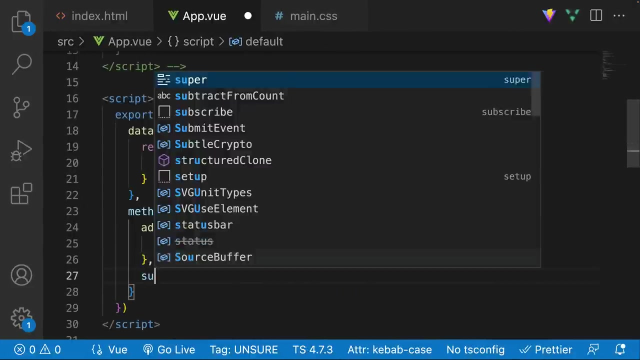 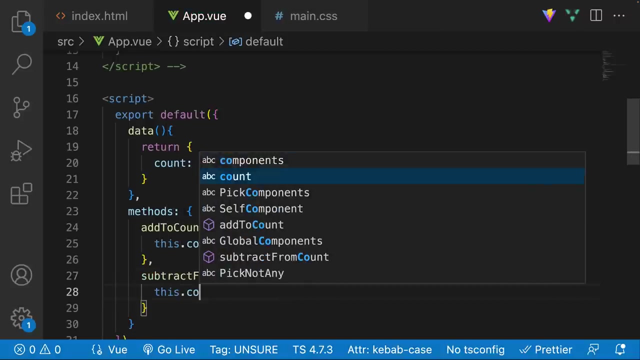 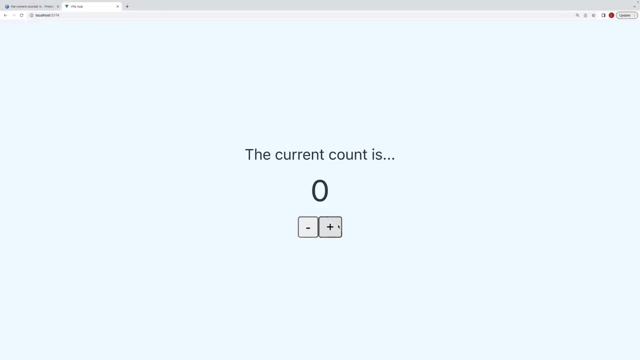 go to our console and let's just click on this method and as you can see it is indeed working so again this is how we're going to define functions that are eventually going to update our state again i kind of prefer this way i like having it this is more javascripty rather than having it in this object over here but now what we want to do of course is update the state so what do we do what did we do before we did count dot value is equal to the state of the object is equal to count dot value plus one well in this case we actually have to refer to the object that we currently live in to get the state so we have to use the dreaded this keyword that i know a lot of people don't really understand what is going on so they're gonna have to do something like this dot count is equal to this dot count plus one and honestly if you're a javascript developer which i am expecting you to be if you're taking this course you probably hate keyword but you have to use it with the options api so now let's go ahead and let's go over here and there you go you can see that it works now we have to define our other method so let's go over here and let's just say subtract from count invoke it we're gonna have to use the disgusting this keyword again so this dot count is equal to this dot count minus one and oh my goodness i keep going back to that one and then there we go 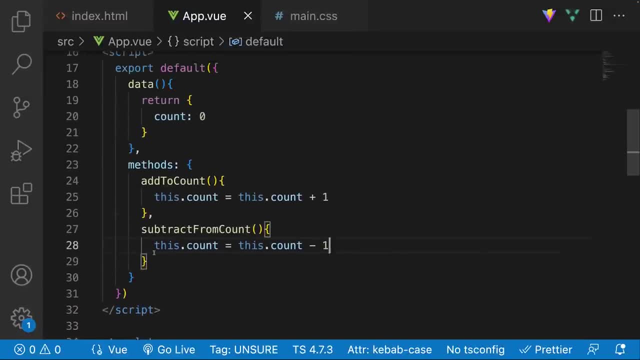 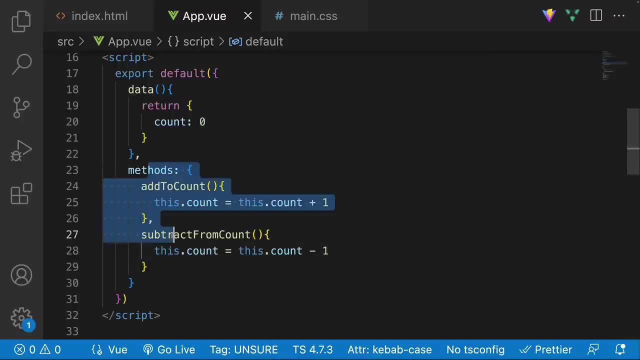 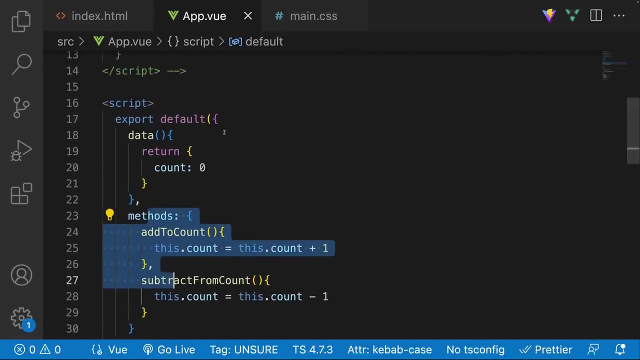 it should be working so this right here is the options api at the end of the day the functionality is exactly the same so we still have our state we still have our methods and we're still able to update our account the way that we should however syntactically they're different so this is how what we had to write in order to accomplish the same thing with the options api 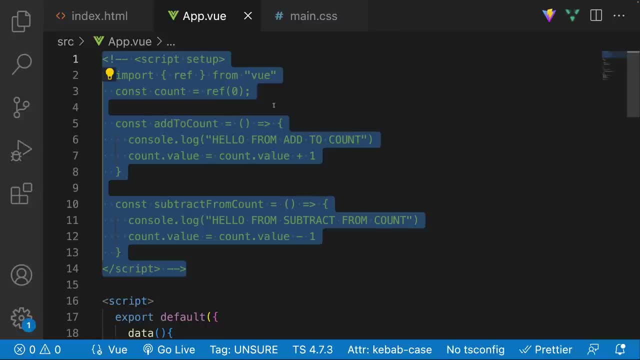 but we well this is what we had to write in order to accomplish the same thing with the 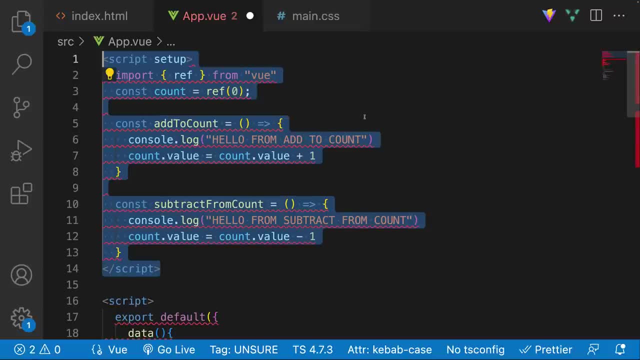 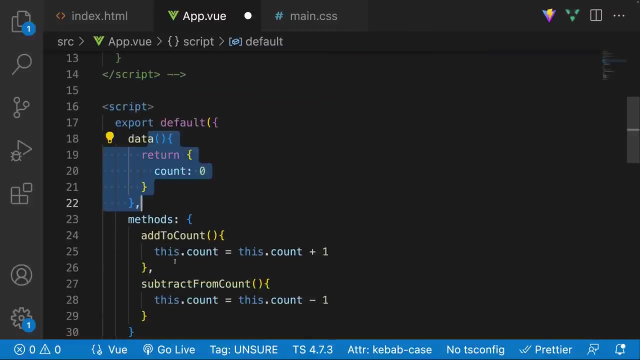 api now let's actually uncomment this oh well actually let's comment it again what do you prefer what do you prefer i honestly prefer this this looks cleaner this looks like pure just javascript whereas this kind of just looks like some magic that vue is doing in order 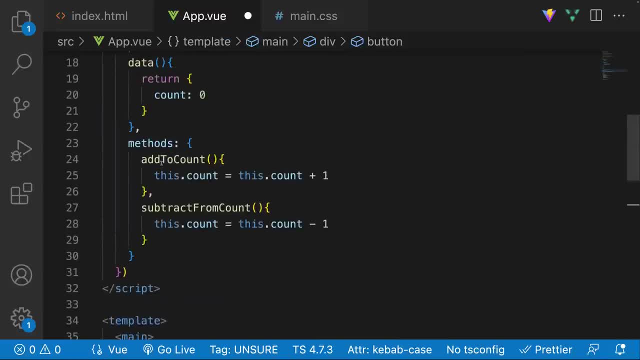 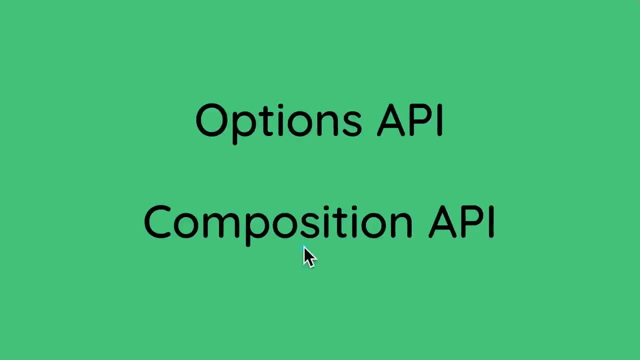 to relate it to what we have over here and that's why i actually prefer the composition api and that's why it is the new and well improved way 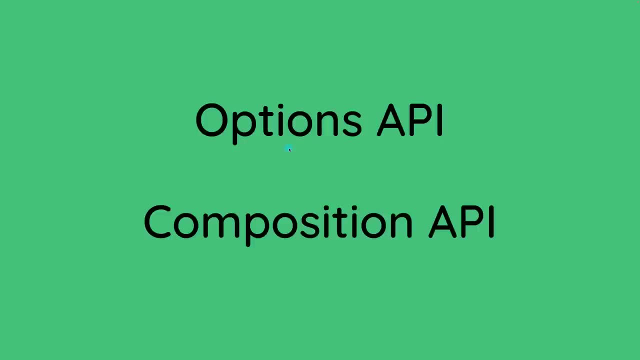 of writing view. So I wanted to introduce the options API because you will see it all the time because it was kind of the legacy way of doing things and I did want to introduce it to you but with new view applications the composition API is kind of the way to go and this is what we are going to be focusing on with the rest of this course. Now just because we're learning the 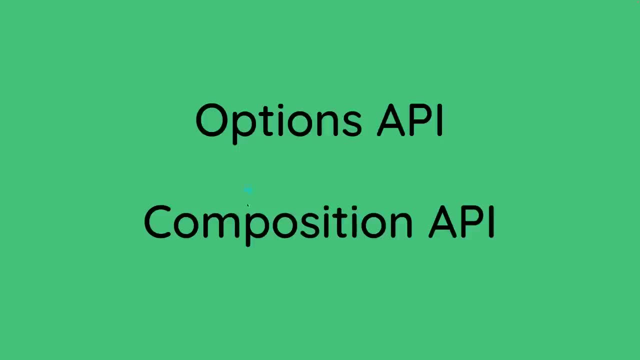 composition API it doesn't mean that well you're completely losing out on the options API. I think 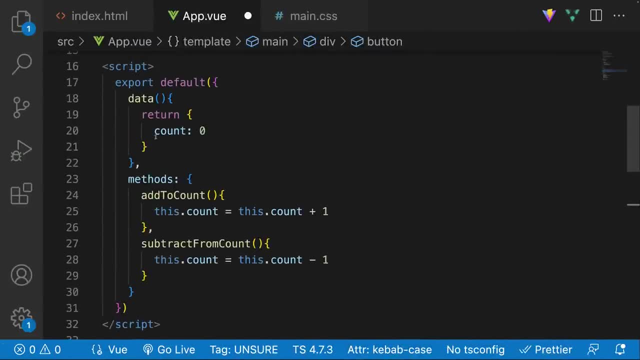 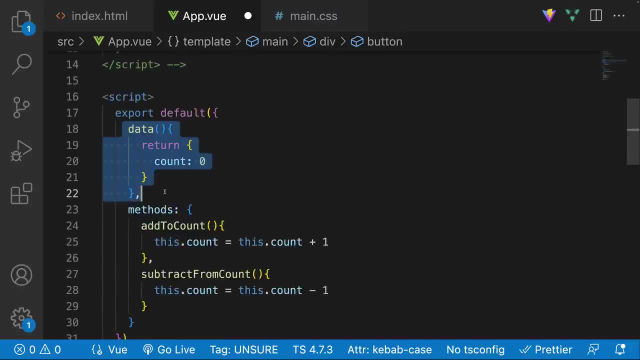 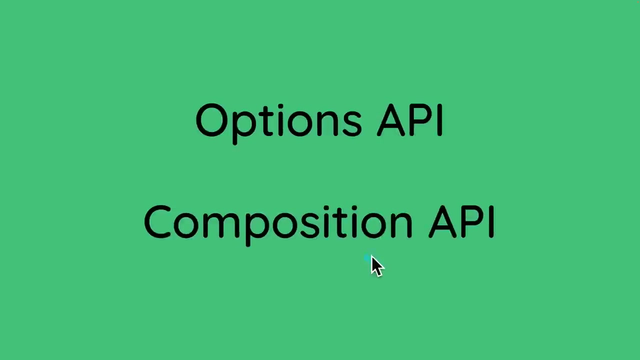 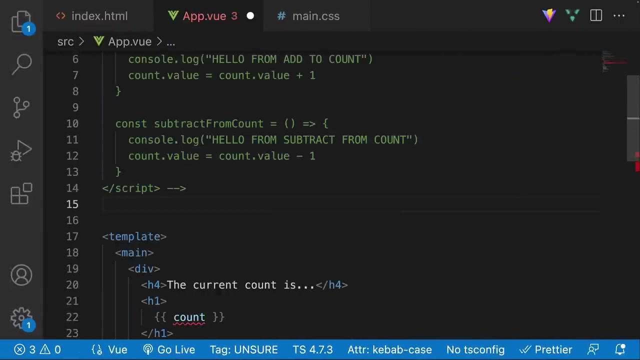 at this point you probably understood exactly what was going on here relatively quickly because you understood what was happening in the composition API. You understood okay this is my state these are my methods and I'm able to access them within my HTML template. So just because I'm going to be teaching the composition API and I'm going to be teaching a lot of other things within the composition API they easily also translate to the options API. So if you ever have to work with a project that has the options API believe me if you have a solid understanding of the composition API you will be a okay. You might be you know searching around for different you know syntax but you will have a great and a vast understanding of what to do. So don't worry you're not missing out. So let me go ahead and actually remove this options API. Don't want it anymore so let's go ahead and remove it. 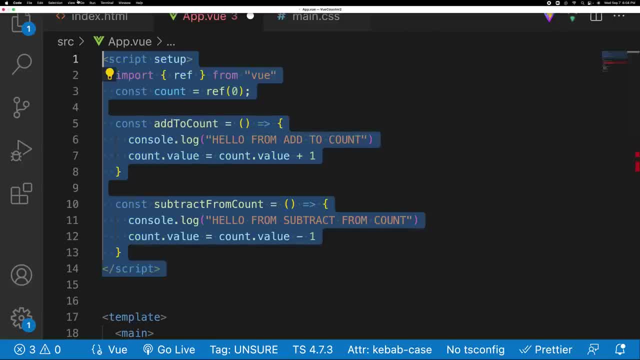 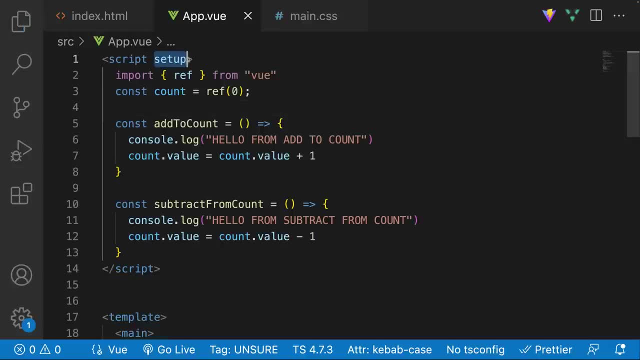 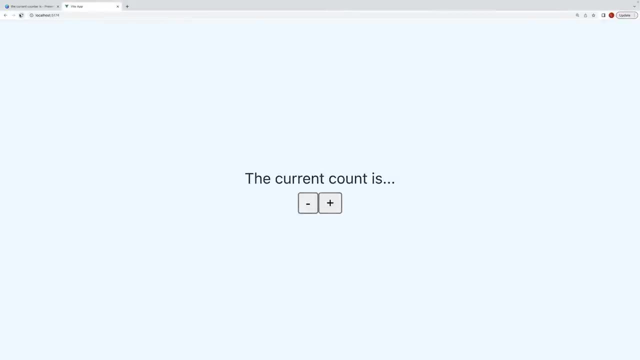 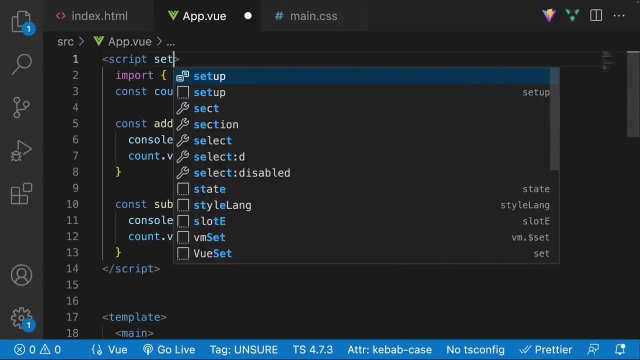 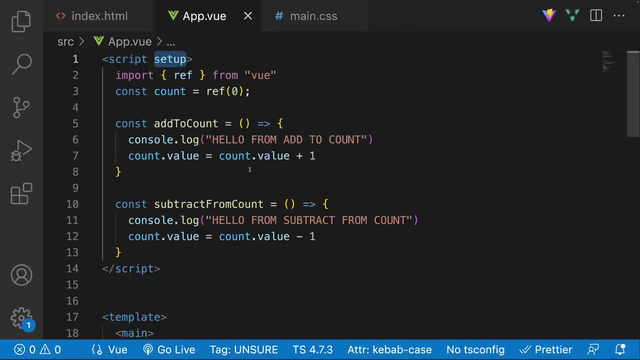 Let me just zoom in once more and what I want to utilize is well the composition API. Now in order to utilize the composition API I have to provide this right over here. So this setup keyword if I don't provide it and I save and I refresh you can see nothing is working a okay we don't have anything in there. So we have to tell it that we want to use the composition API by saying setup and it will know okay you want to use the composition API. So let's go ahead and remove this composition API. That's fine. Go ahead and define everything you need and we're going to set up everything correctly. 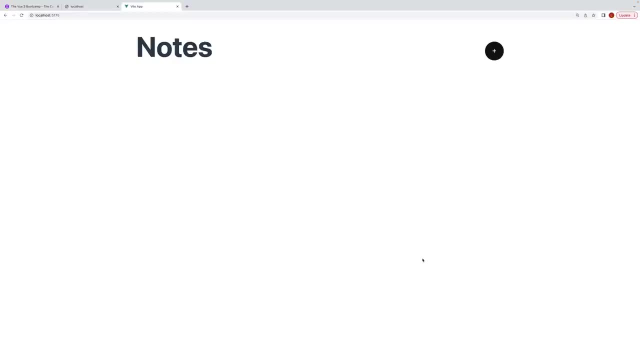 All right everybody welcome to a brand new section and a brand new project. This project is going to be a notes application. So very simply we're going to have a header here that says notes and we're going to have this button. And when we click on this button it is going to trigger this modal to appear. 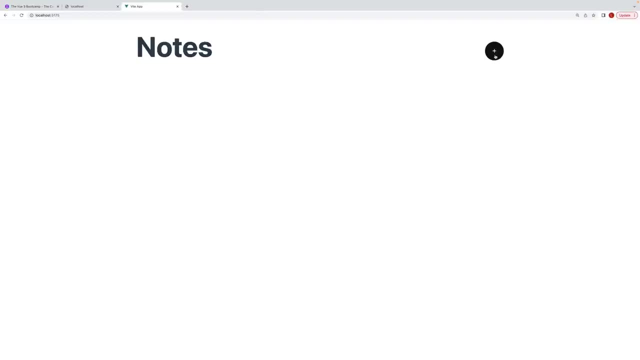 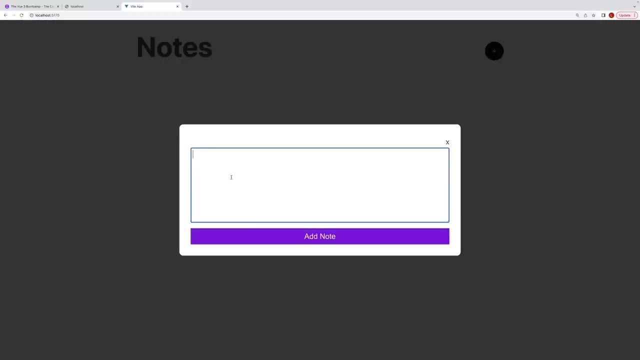 You can of course always close the modal as well. So it can trigger it to close it trigger it. Now right in here what we're going to do is add a new note. So I'm going to say this is my new note like so. Then what I'm 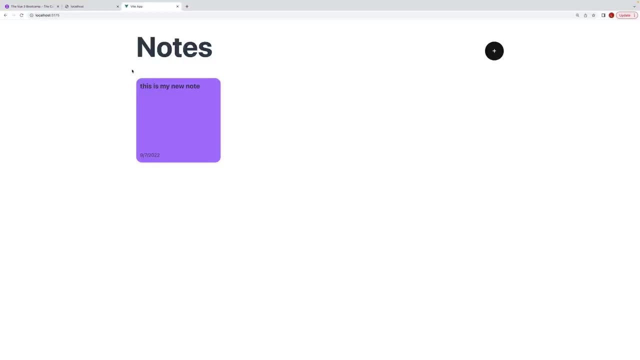 going to do is I'm going to click on add note. And as you can see here it's going to create this card with my note as well as the date when I created the note. So I'm going to go and zoom in here. That's a date when I created the date. So I'm going to go ahead and zoom in here. That's a date when I created the note. 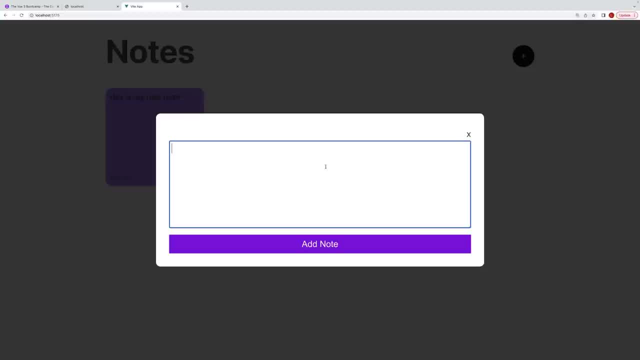 created this note now of course we can continue on we can add more notes this is another note my friends something like that and then I'm going to go ahead and add this and you can see it adds another note but this time in a different color and of course we can just keep going on and on 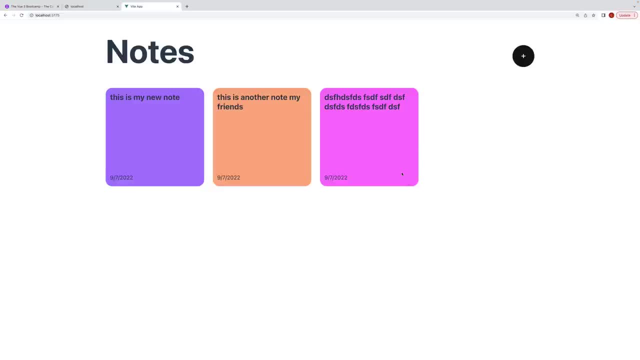 and on you guys get the point now this seems like a very simple application but it is going to introduce a lot of new view concepts that we are going to learn so I'm super super excited to teach this app and well let's get started now in order to get started we're going to actually need to build a lot of html as well as css so not really related to view so what I'm going to do in the 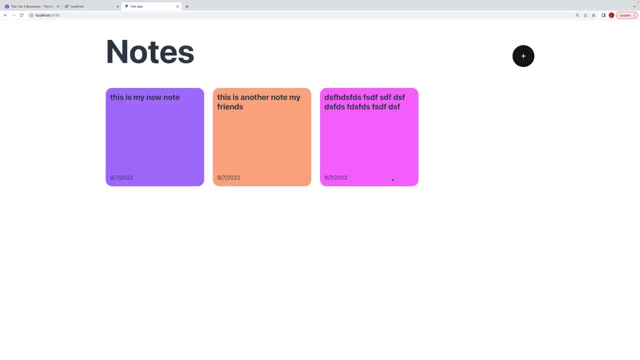 next video is dedicate that video specifically to building the html as well as the CSS for this application now if you do not want to build the CSS and HTML because this is something that you're already familiar with you can 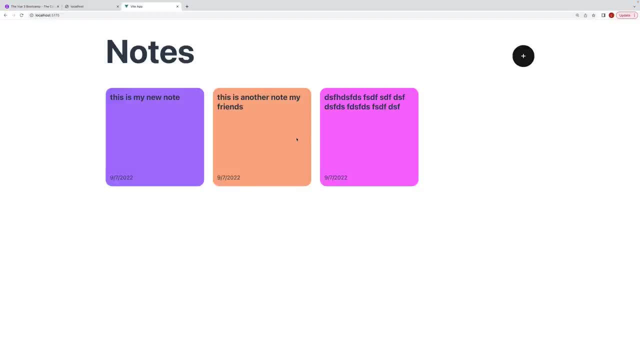 100% skip that video and just download the boilerplate code that is attached to this video right over here so you can download that and then skip the next video where we build the HTML as well as the CSS and just go directly and jump into the view if however you like to build things from scratch and you want 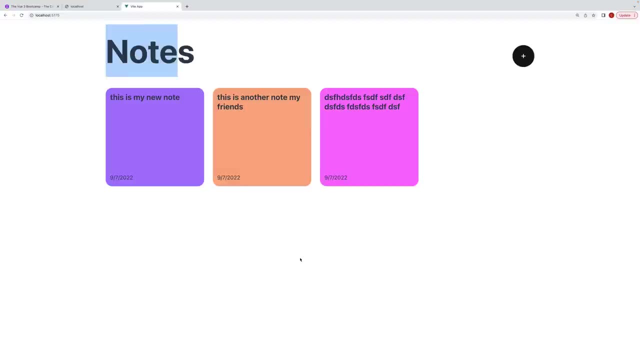 to build the HTML as well as the CSS with me well you can just proceed to the next video so let's go ahead and do that all right to create our application the 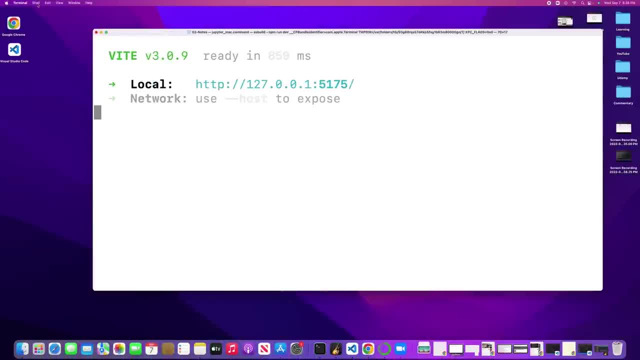 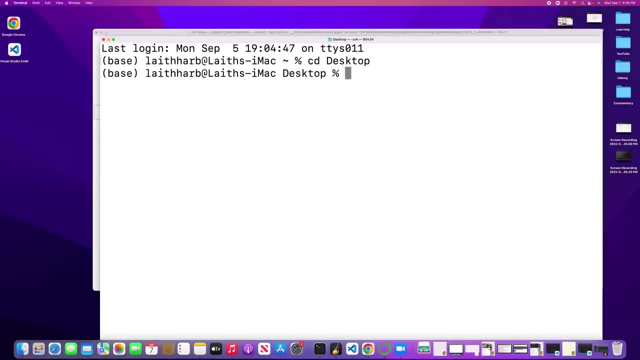 first thing that we need to do of course is to create a view app so I'm going to open up my terminal or if you're on Windows your command prompt let me go ahead and zoom in a little bit and then what we're going to do is I'm going to go ahead and zoom in a little bit and then what we're going to do is I'm going to go ahead and zoom in a little bit and then what we're going to do is I'm going to move into my desktop directory and then very simply I am 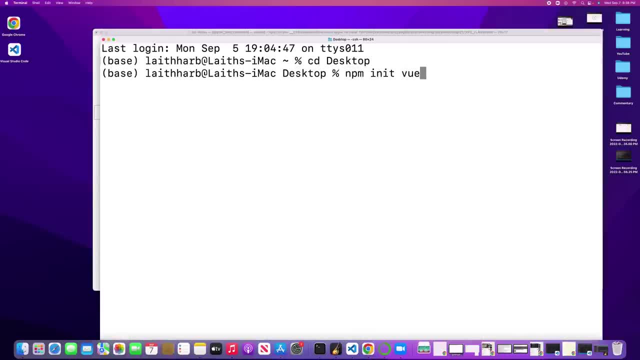 going to do an NPM in it and then view at latest like so so this is going to create a project I'm gonna call this project let's say notes app so let's 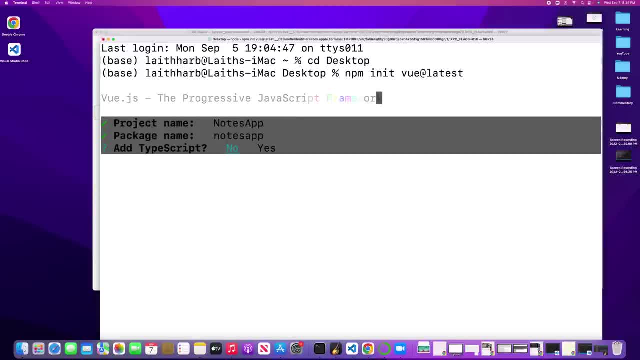 call this notes app will say the package name is nothing no no no no no no all 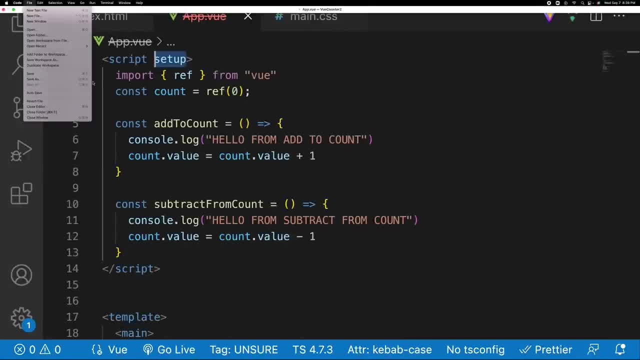 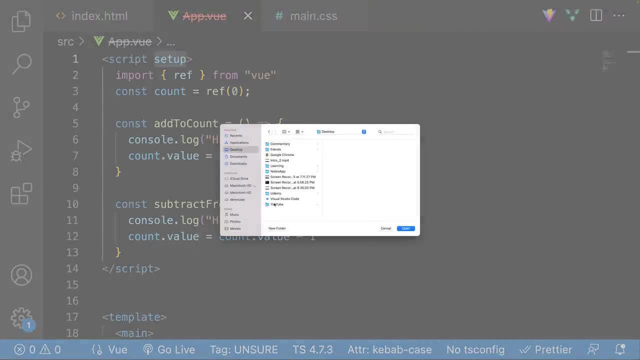 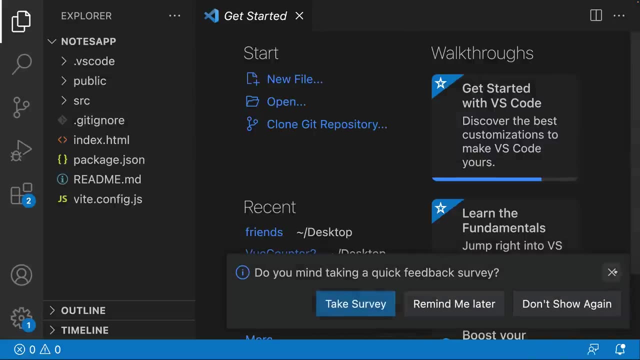 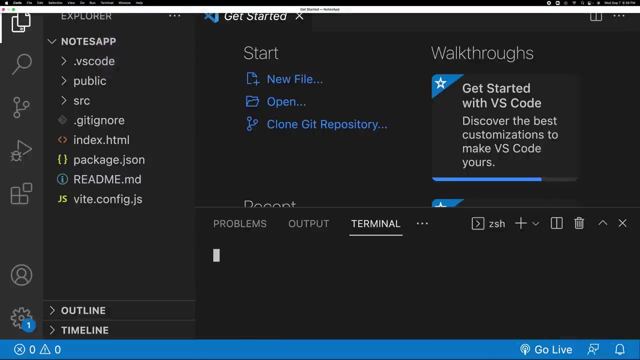 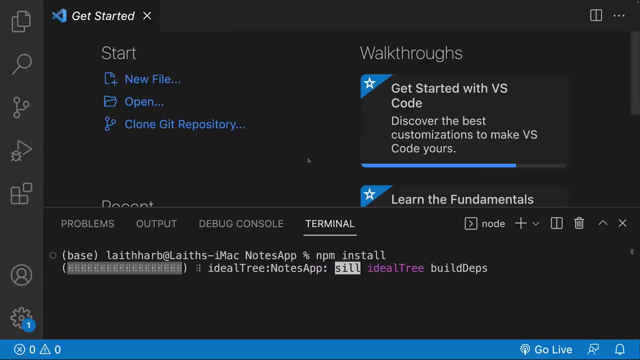 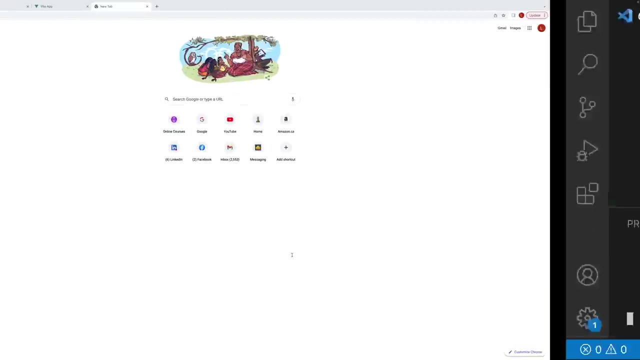 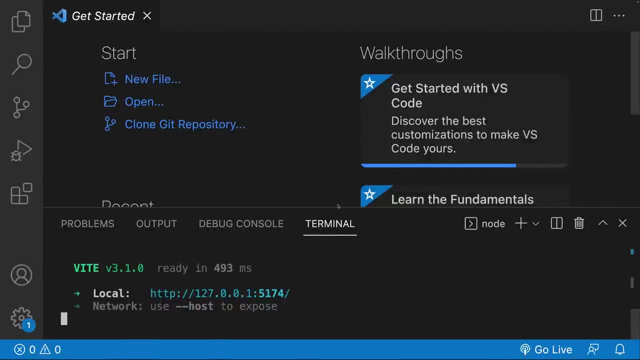 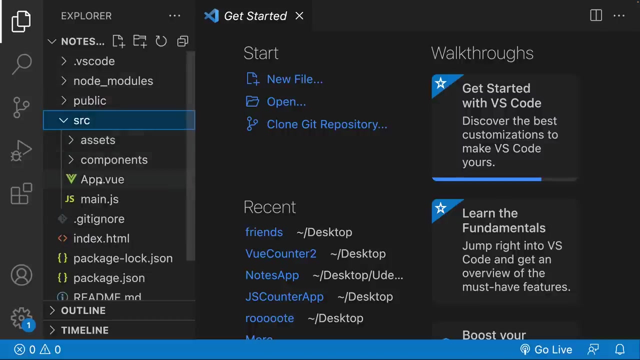 right so now we have created the notes app let's actually go ahead and open open this up in VS code. So I'm going to say open and I'm going to go to my desktop and I am going to go to the notes app. So let's go over here. This is my wonderful notes app. Okay. So now what we're going to do is build the HTML for this application as well as the CSS. But before we do that, of course, what we're going to need to do is an NPM install to install all of the dependencies. Let's remember that we need to do that. And then let's run our application with NPM run dev so we can spin up a view development server. So we're going to say NPM run dev. And it should run on port localhost 51 of 74. There we go. Very, very beautiful. Alright, so there we go, we have our application running. The first thing that I'm going to do is we're going to go to that app dot view file. 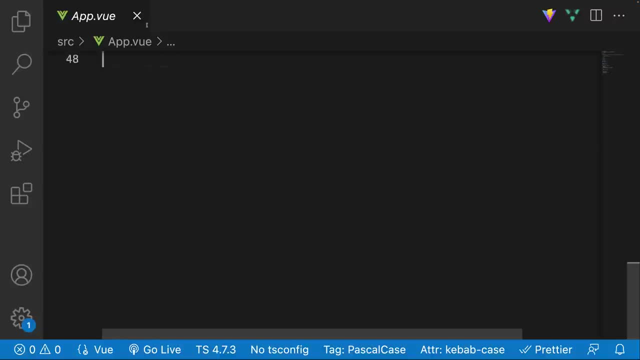 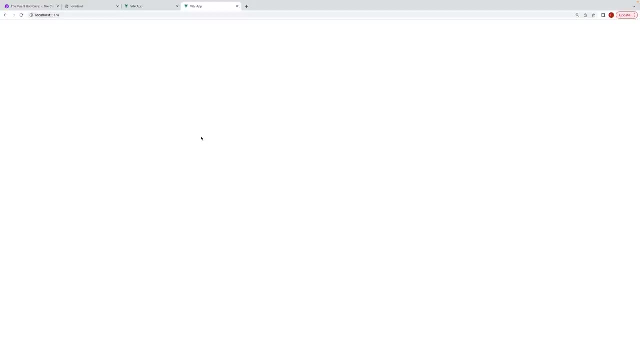 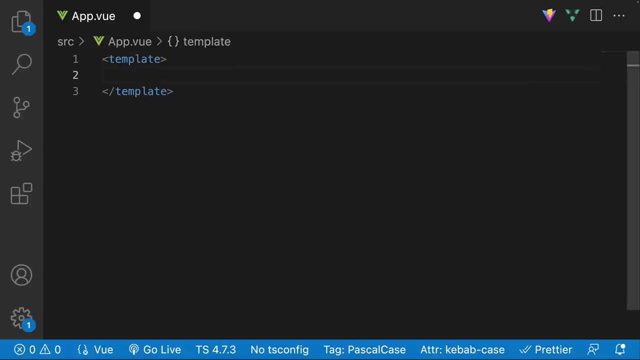 And then within this app dot view file, I'm just going to remove everything. And of course, once I remove everything, you can see here we have a completely blank application. So the first thing that I want to do is well, just let's build out the HTML template for this app. So let us go over here. And let's create a template. Let's create a main tag, a main tag. And then what we're going to do is we're going to go to the app dot view file. And then within this app dot view file, I'm just going to remove everything. And of course, once I remove everything, you can see here we have a complete blank application. So let's go over here. And let's create a main tag. And then within this app dot view file, I'm just going to remove everything. And then within this app dot view file, I'm just going to do is we're going to create a div and we're going to give this a class of container. I'm going to go relatively fast with this because again, I kind of expect you to know HTML and CSS. So I'm not going to bother kind of explaining what I'm doing. I hope this is kind of really basic for you if you're following along. So let's go over here, let's create a container. And within this container, we're going to have a header. And that is going to contain our notes header. 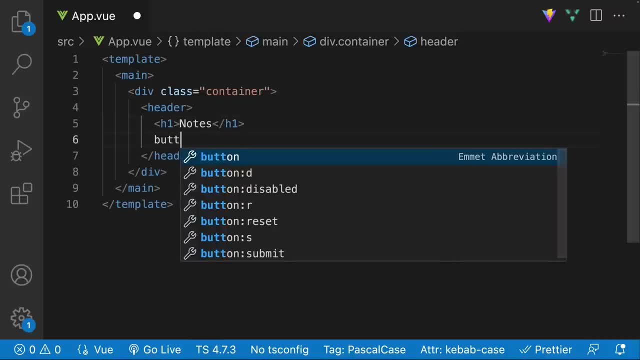 And it's also going to contain that button. So let's just create a button. And within it, we're just going to say plus. So there we go, we have our header. Now we're also going to create another 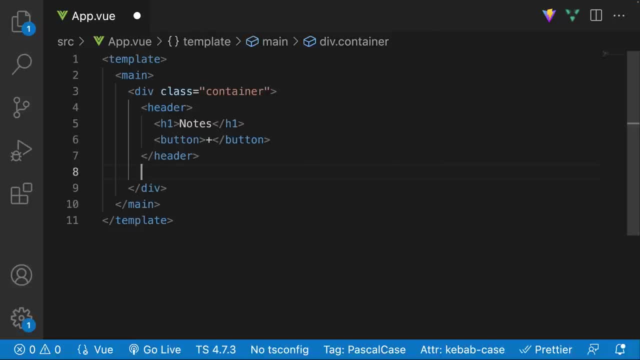 div. And we're going to give this a class of card styles. So let's create a div. And we're going to say, or sorry, card container, that's what we're going to call it or cards container. And notice 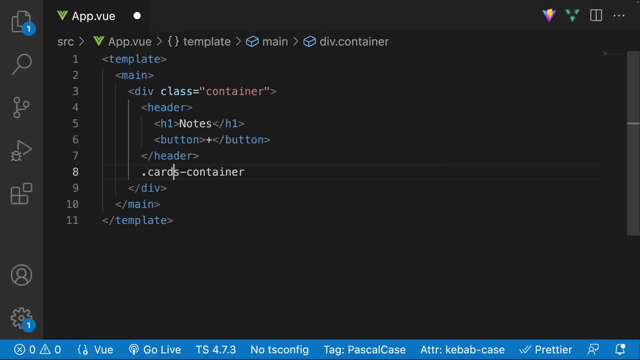 here what I'm actually doing, I'm, I'm doing a dot, and then I'm doing cards dash container, and so what this is actually going to do is create a div element with this class over here. So if I 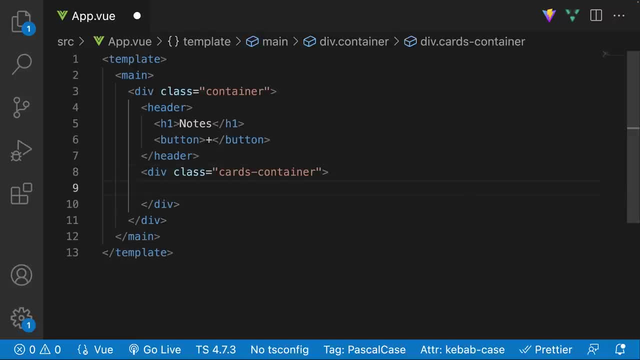 actually go ahead and do that, you can see it's just an Emmet abbreviation that you get right off the bat with VS code in case this wasn't something that you're familiar with. Alright, so there we go, we have created our cards container. Now within it, I'm just going to create the HTML structure 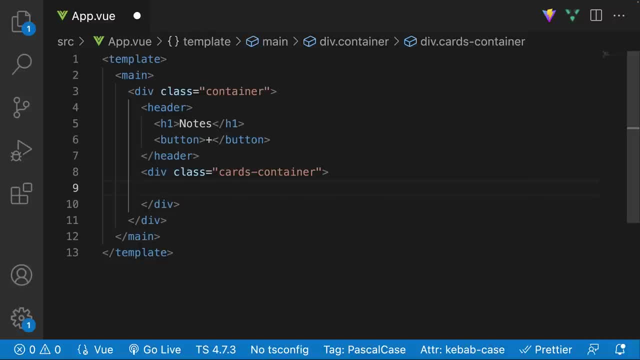 for one card. So let's go over here. And I am going to say, well, I want to create a div, with the class of card. And then within it, let's create a p tag that is going to contain the notes. 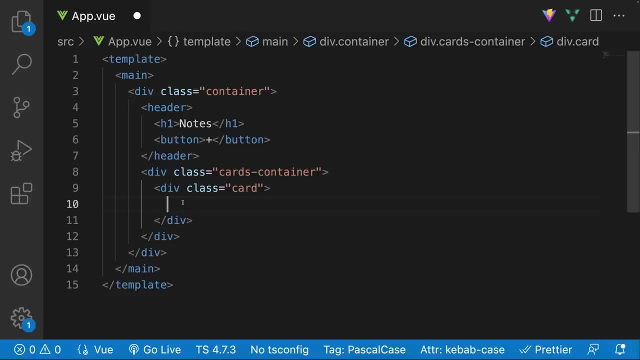 And let's give this a class of main text. So what I can actually do is say, hey, p tag, and then dot the class. And that's going to create a paragraph with this class. And then lastly, let's create 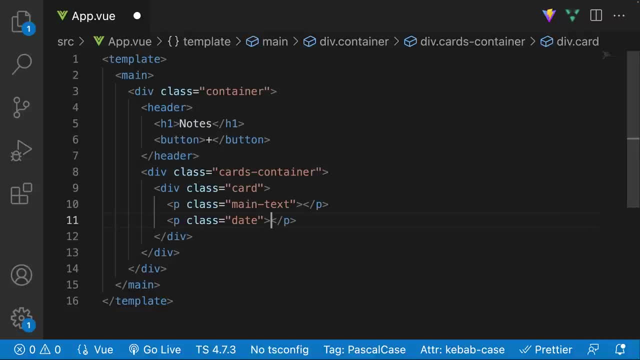 another p tag. But this time, this one's going to be the date. And there we go. That's really all the HTML structure that we need. Now we also need the HTML structure for the modal. 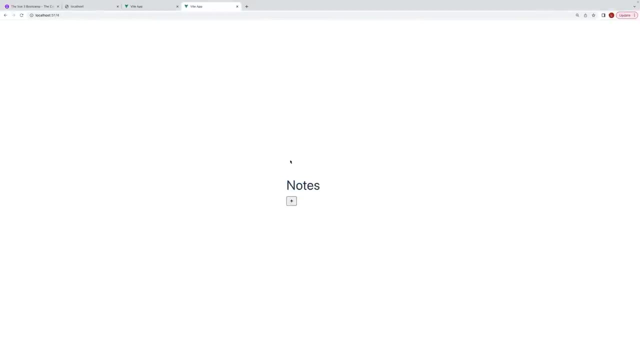 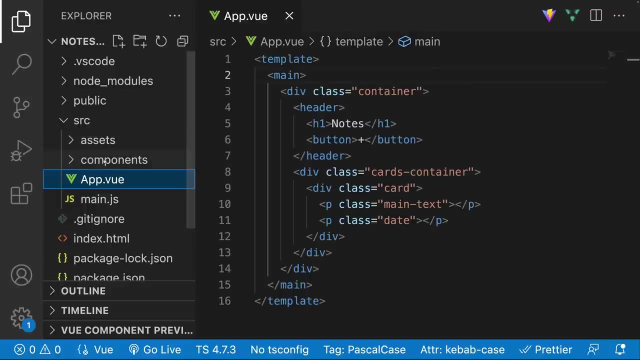 But we'll create that a little bit later. Okay, so this is looking a okay, one thing that we're going to need to absolutely do is to go to our, let's go over here to our assets to main dot CSS, 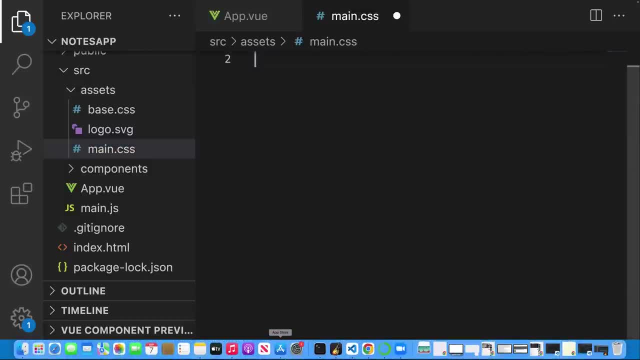 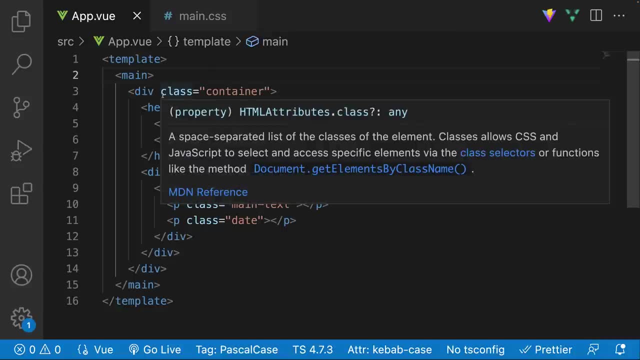 everything below this import, just remove it. And that way, it should look something like so. Okay, looking decent so far. Alright, so now, what is the next step? Well, of course, we're going to need to create a div, which is going to contain the notes. And then 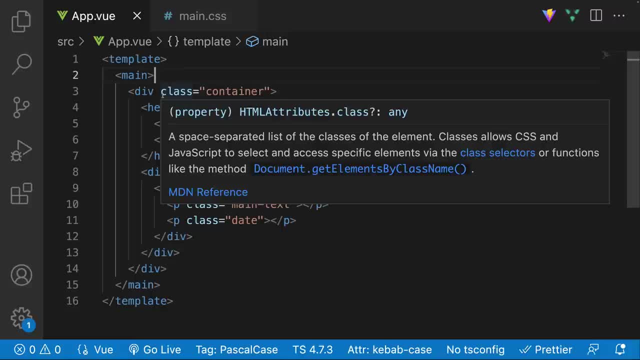 of course, the next step is styling. So let's actually go ahead and style this application. 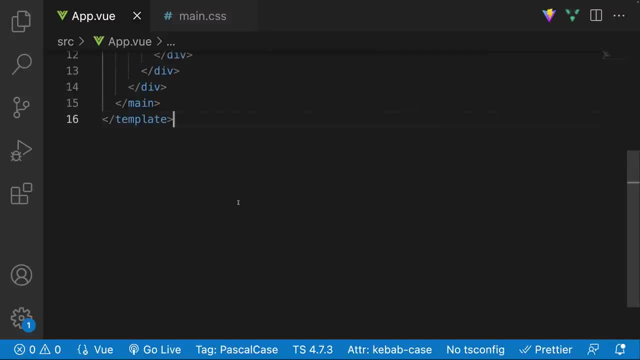 And let's begin with the main. So let's go over here, we're going to say the style tags, and we're going to add the scoped keyword to make sure that everything is scoped together. So all the styles are scoped to this HTML in this file. So I'm going to give I'm going to style the main first the main HTML tag, I'm going to give this a height of 100. 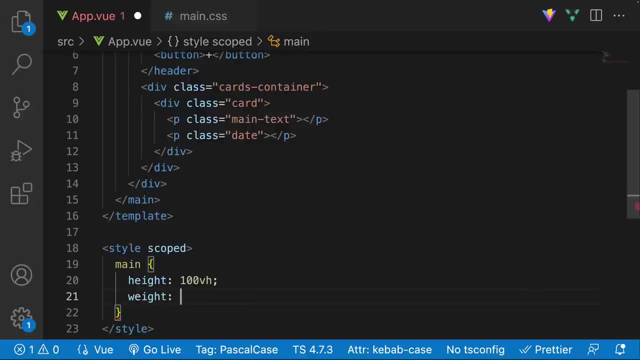 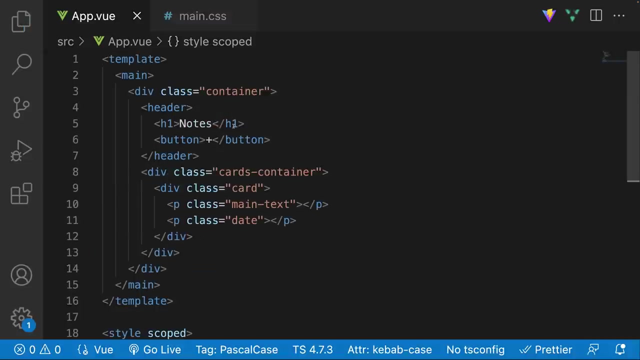 vh and a width of 100 vw. Alright, so this is looking pretty good. Not, not wait with misspelled that or I just wrote the wrong word, whatever. So there we go. So now we have that. So now let's 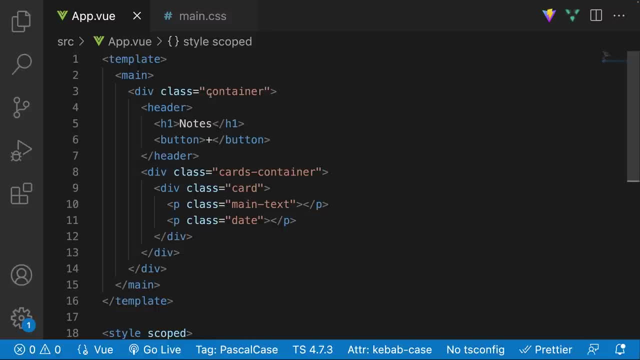 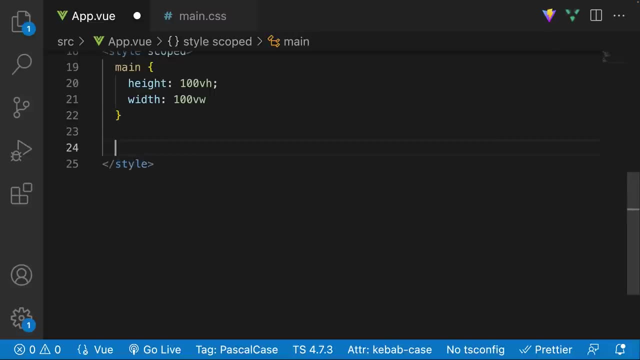 actually style the container. So how are we going to style this container? Well, let's go over here, let's grab that container class. And I'm going to say, oh, this is a container class. And I'm going to say, oh, this is a container class. And I'm going to say, oh, this is a container class. And I'm 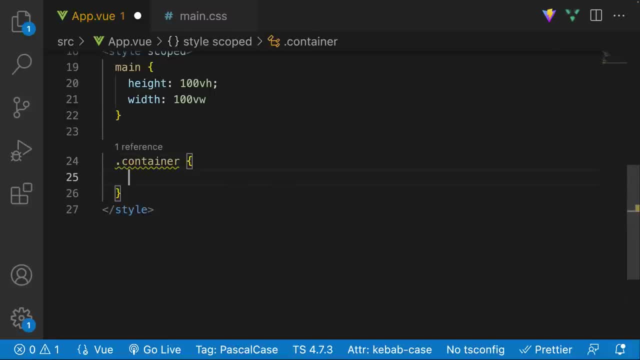 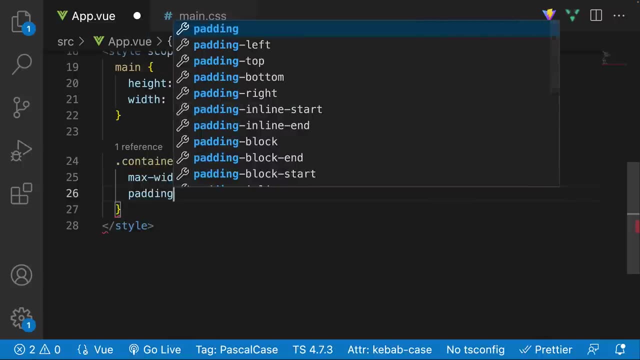 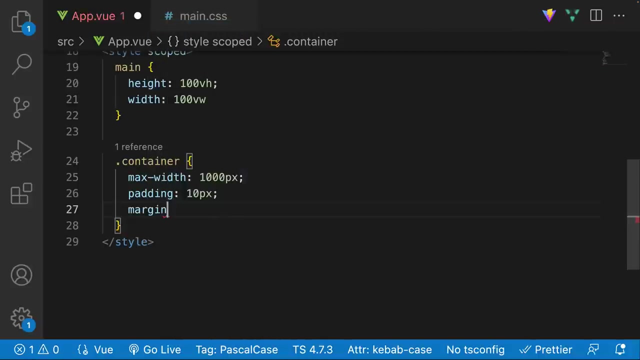 going to say container. And then I'm going to say the max width of the container is going to be 1000 pixels. And then I'm also going to give this container a padding of 10 pixels. And lastly, I'm going to give it a margin of zero auto. So it can actually center this right in the middle. And 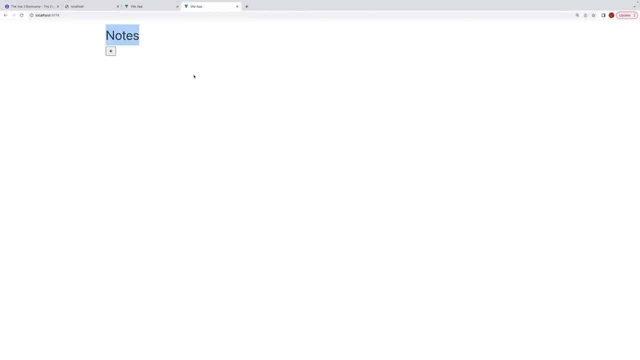 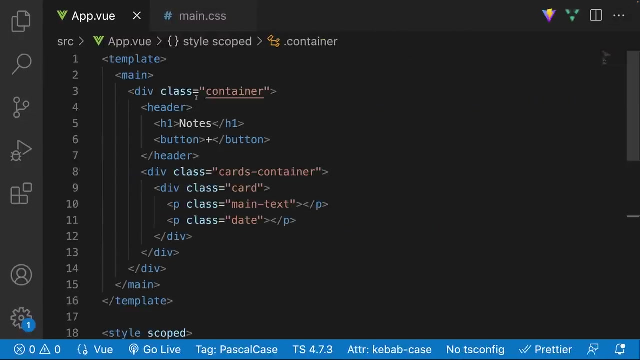 now you can see it's kind of old, it's kind of centered right in the middle. So we have our notes. Okay, so this is pretty good. But now, of course, we need to style our head. So let's go ahead and style this header. So let's give this a style. Now I want this to be positioned kind of 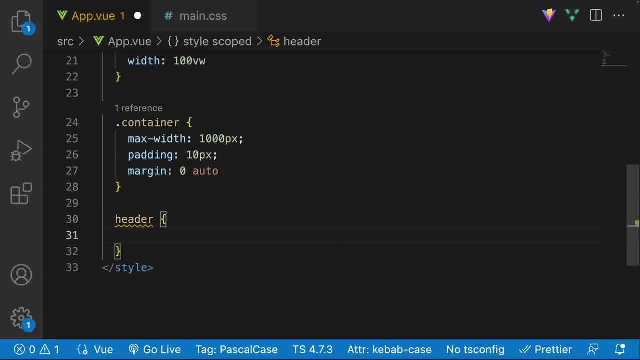 horizontally, not vertically. So the best way to do that is to very simply just give it a display of flex. And we also need to give it a justify content of space between so that, well, we can see here, 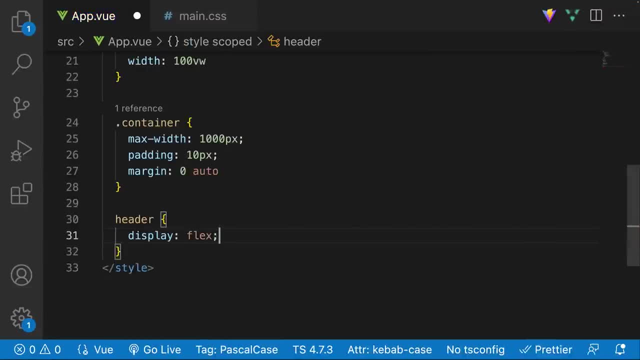 we they're kind of all separated apart. Now, lastly, we need to give it a justify content of space 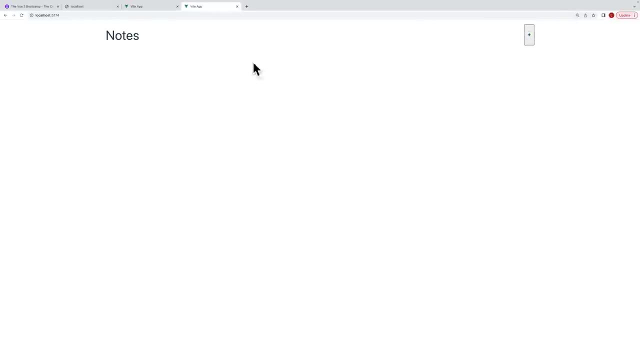 between so that, well, we can see here, we they're kind of all separated apart. Now, lastly, we need 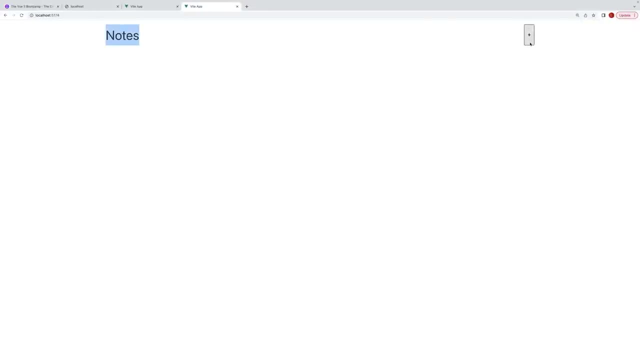 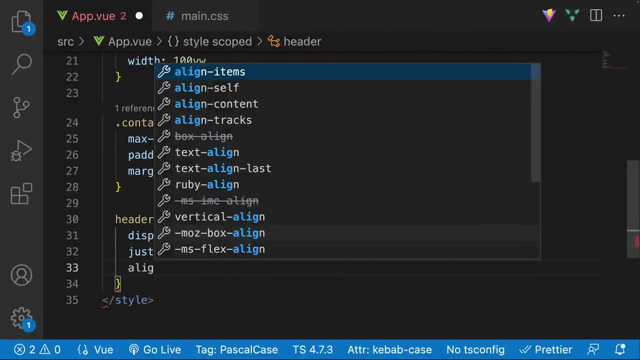 to give it a style of novalize. Okay, so we'll make this rel today. Now, lastly, so we don't have this kind of funky large button, let me zoom in here for you guys. So we will have this funky 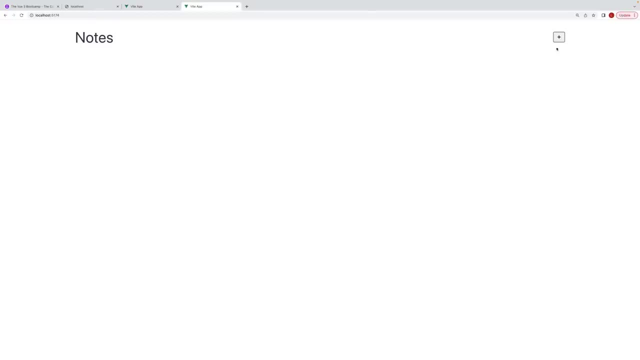 large button. Let's go ahead and give this an align items of center. And that's why we have 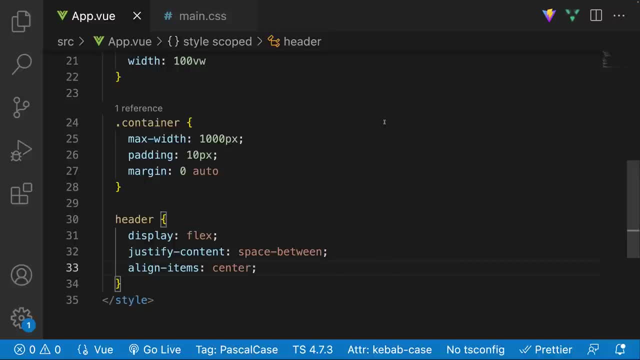 another nice looking button. Alright, so this is terrific. But now what we need to do, of course, 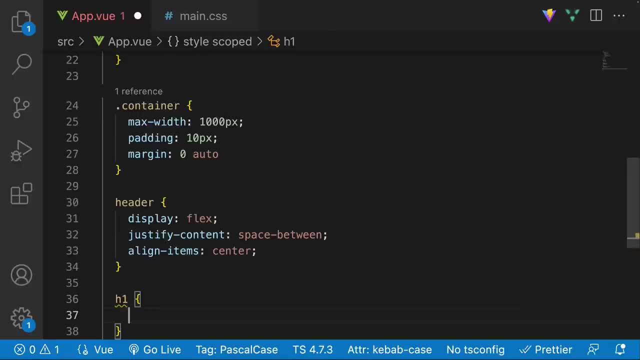 is here let's say h1 and we're going to give this a font weight of bold we're going to give this a 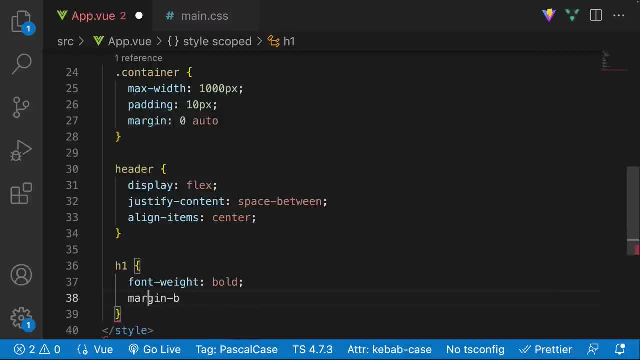 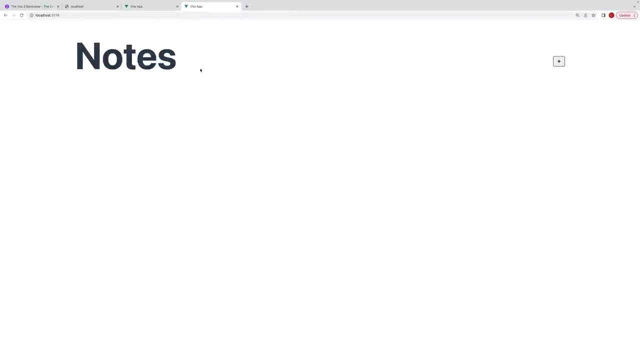 margin bottom margin bottom we're going to give this a margin bottom of let's say 25 pixels lastly let's also give it a font size of 75 pixels let's go ahead and save that and there we go we 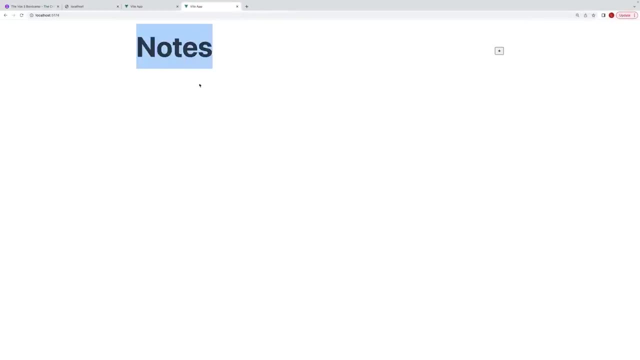 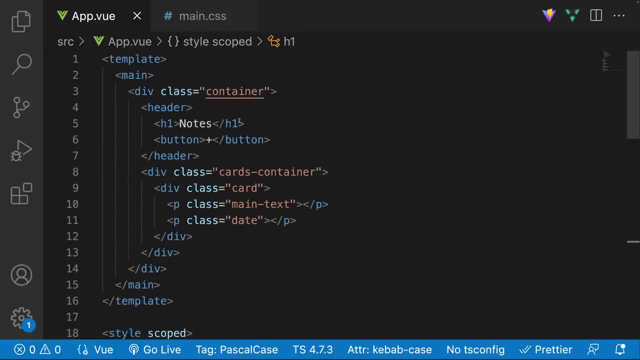 have our button that can actually zoom out a little bit now where we have the the header nice and big and well pretty beautiful so now what i want to do is style this button within this header 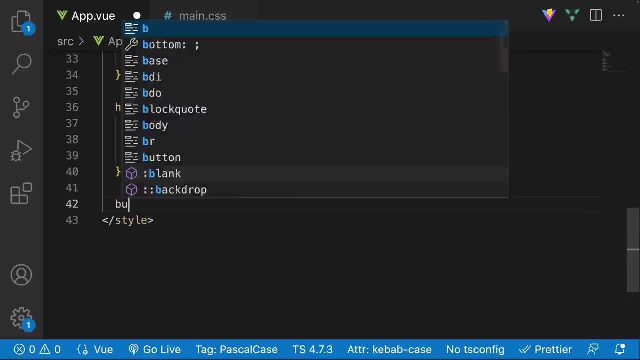 so let's go over here we only really have one button so let's just style the button itself 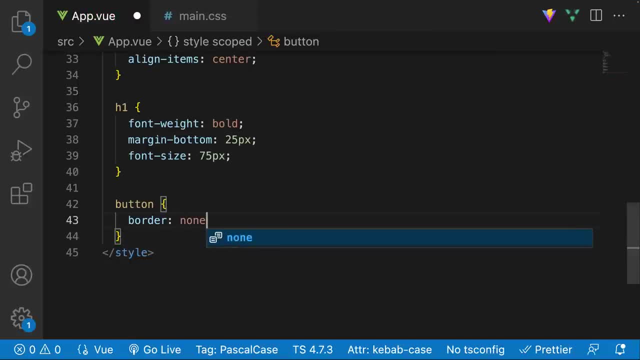 and we're going to give this a border of none and we're going to give it padding of 10 pixels we're also going to give it a width and we're going to give it a width of 10 pixels and we're going to give it a width of 10 pixels 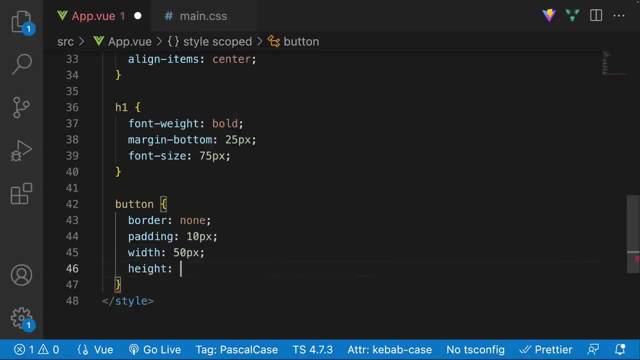 of 50 pixels a height of 50 pixels and then we'll give it a cursor pointer and let's also give it a background color of rgb i'll say 21 20 and then 20 and lastly let's do a 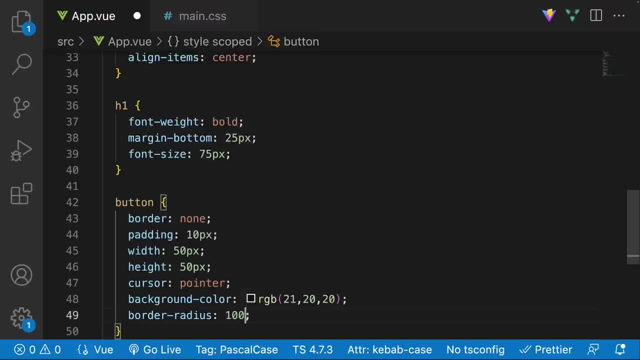 border radius of a hundred percent so it can be nice and round and let's do a color of white 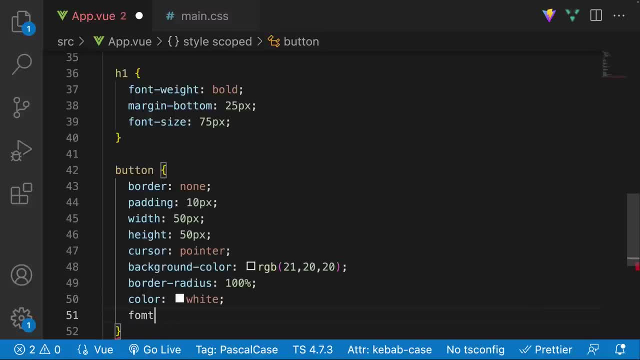 and the absolute last thing a font size of 20 pixels now if this is again too big for your screen 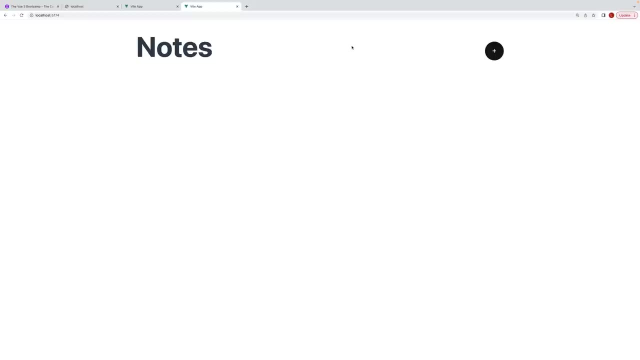 not a css course just adjust it so it looks a little bit better if that's something that you care about all right so that's pretty much all it is that we need to do for that now what we need 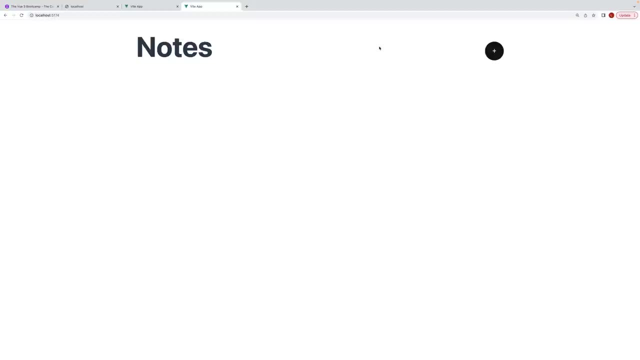 to start doing is to style our uh well our cards so let's go and just style the card itself 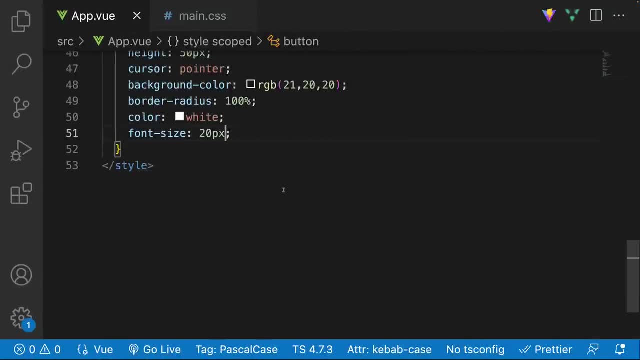 and so let's go over here and what i'm going to do is i'm going to say dot card and we're going to give this a width of 225 pixels a height of 225 pixels so the it can be a square we're going to 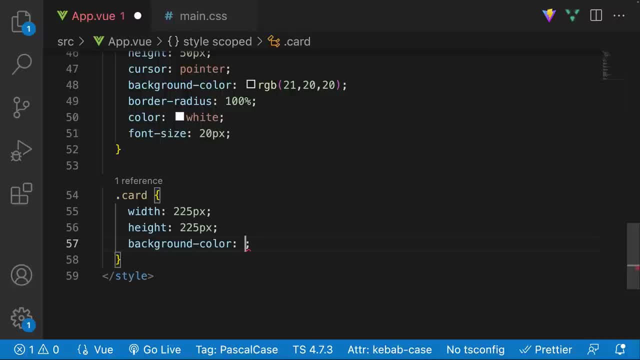 give it a background color now this is going to be dynamic this background color is going to be kind of just randomly generated but just so we can see it let's just give it a background color of rgb 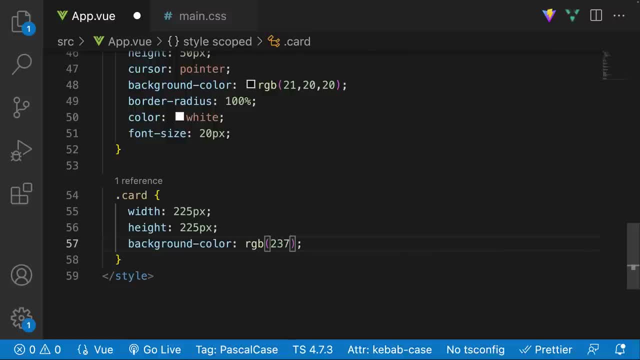 rgb and then i can say 237 and i can say 182 and i can say 44. all right so it can give us this nice yellow color let's also give it some padding let's give it a border radius so give it a border radius of around 15 pixels let's also give it a display flex because what we're eventually going to want to do is separate the um the uh the the notes from the actual data so we're going to give it a display flex and then we're going to give it a border radius 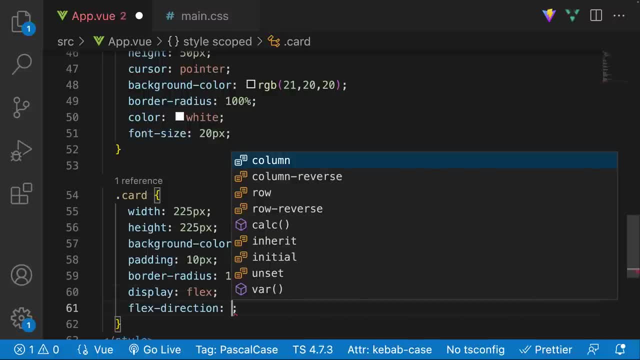 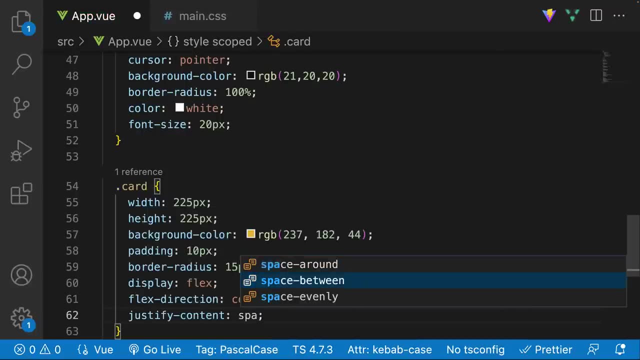 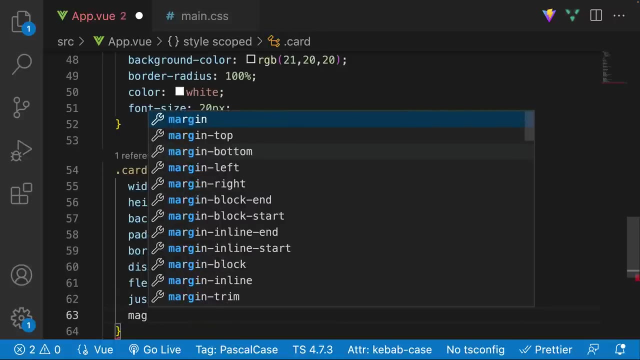 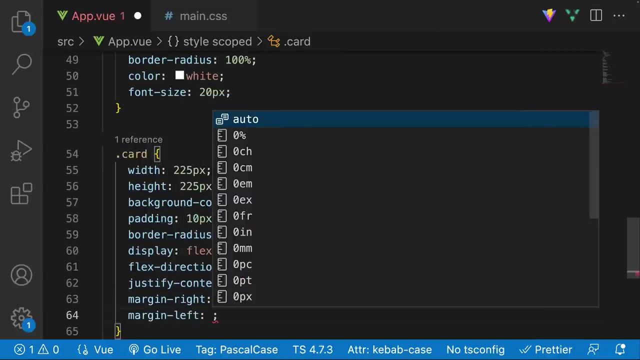 itself uh so to do that we're going to have to actually change the direction to column and then we're going to say justify content and we'll say space between and lastly we'll do just a little bit of margin from the uh from the right and the bottom so we'll say margin right we'll say 20 pixels and then lastly we'll say margin left which or sorry bottom rather which will also be 20 pixels 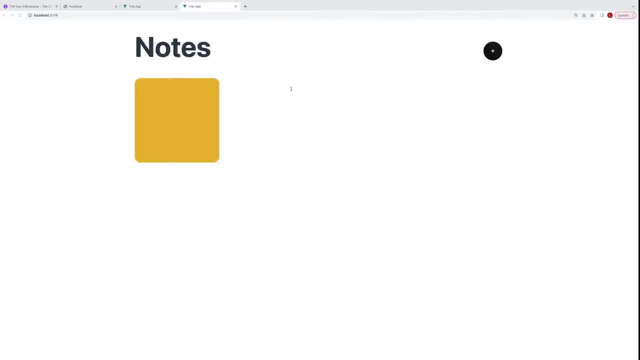 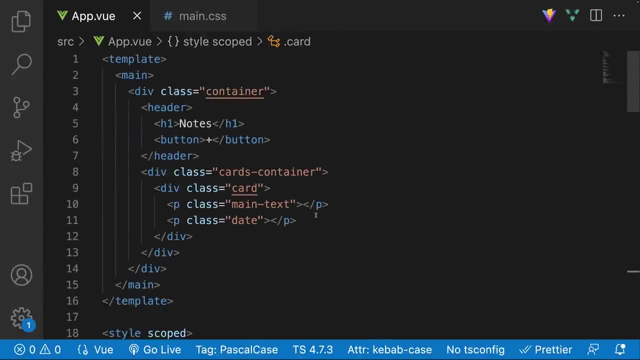 all right so this is looking pretty good so now if you went there you can see we have our wonderful uh card so let's actually now style the text within the card so let's first add some text so a nice little shortcut to adding text if you're using vs code is you can say lorem and then whatever number of words you want and it just generates just 15 words of gibberish that you 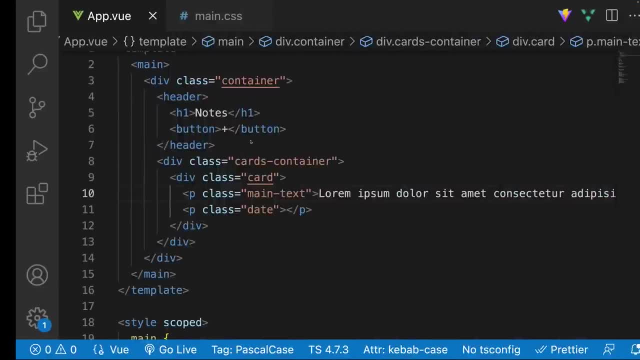 can actually utilize just kind of for like testing your styles so i think honestly this looks pretty good and i'm going to go ahead and add some text to this so i'm going to go ahead and add some text to this so i think honestly this looks pretty good i don't really have too much of a complaint with 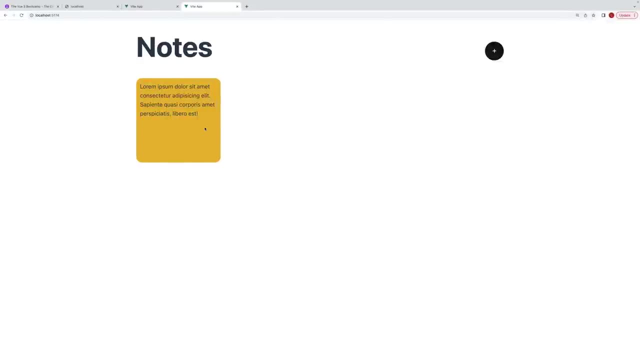 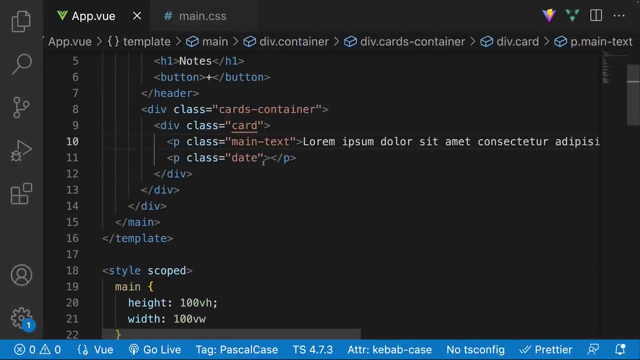 this i'm wondering if i should maybe change the size honestly i'm just going to leave it as is so usually i i had some styles for this but this honestly looks pretty good and let's go over here 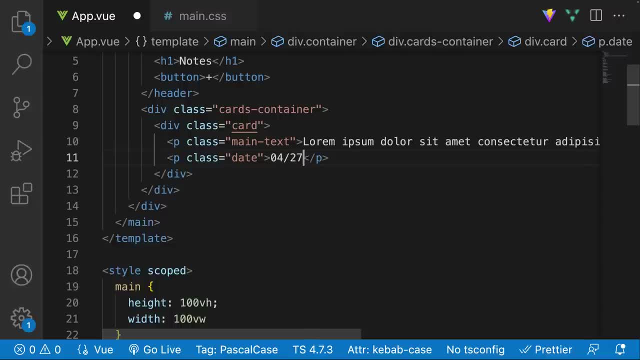 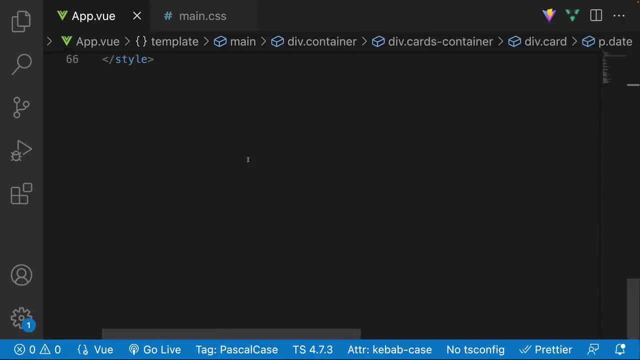 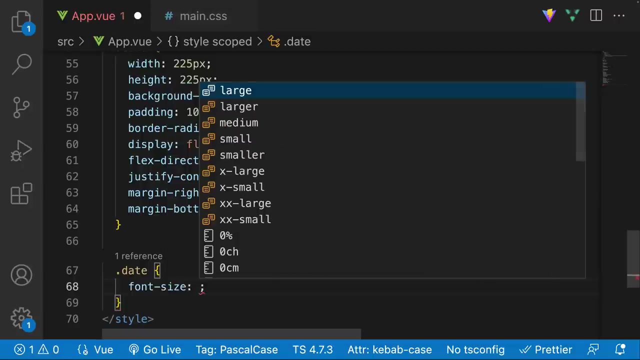 let's just give this a date of uh let's say yeah five years uh 6853 that's a pretty good year okay maybe this one's going to be a little bit smaller so let's go over here we can give this a date uh so you can say font size and we can give this a font size of let's say uh 12.5 pixels yeah a little bit smaller that looks good and maybe we 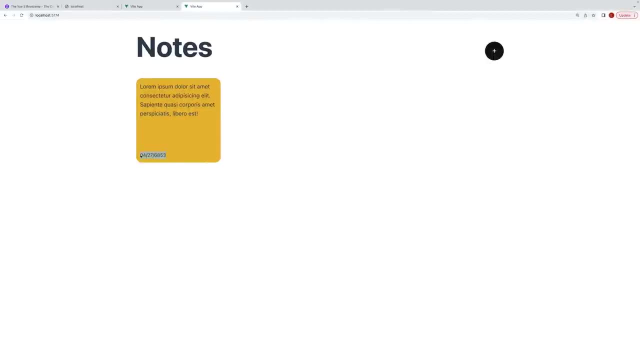 can also give it i think that's good we'll just leave it like that maybe we can also make this bold actually let's do font weight of bold 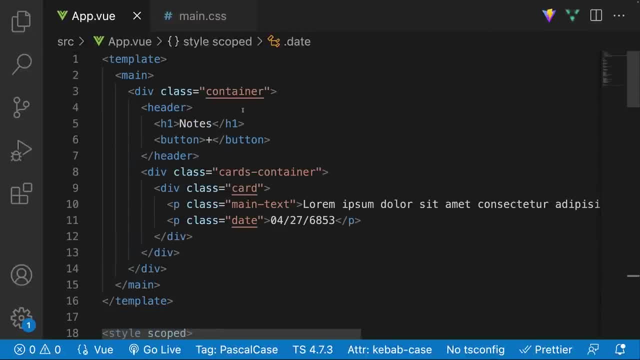 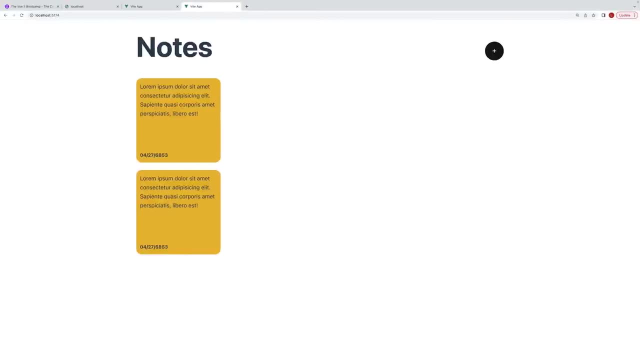 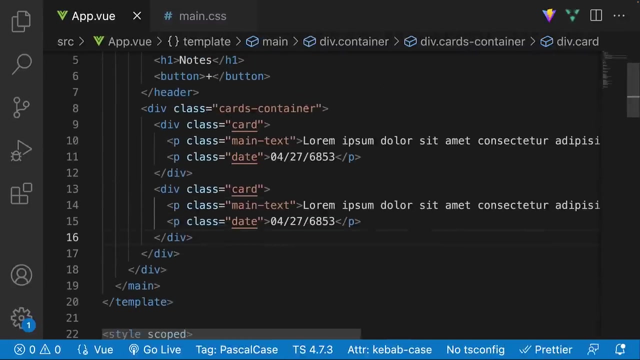 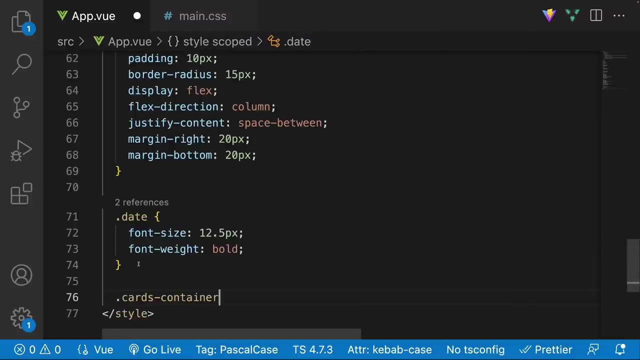 and there we go beautiful looking card so now the only issue is once we start having multiple cards uh so let's say i add another card they kind of stack up horizontally which obviously is not what i want so what we're going to need to do is just very simply uh style this right over here the cards container so we're going to just need to add some flex box styling to this so we're going to 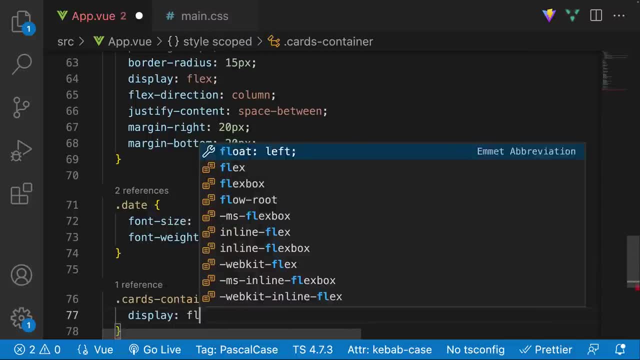 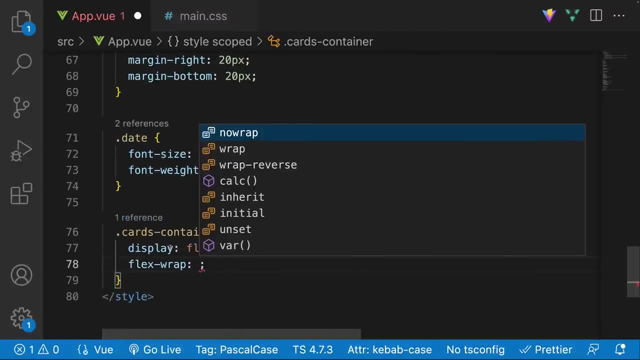 say here display flex and then lastly we're going to say uh flex wrap and if you're unfamiliar with flex i just go ahead and read about it it's kind of a simple thing i i do also have a tutorial on youtube if you are interested 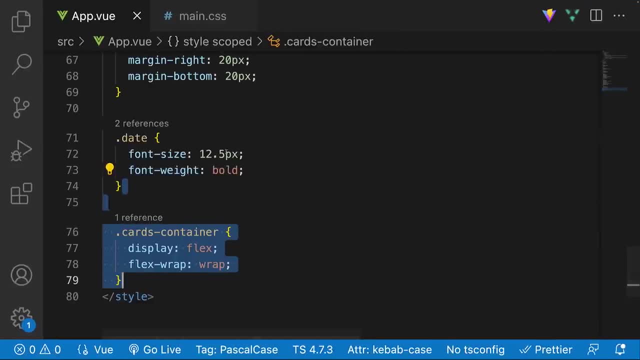 in it i just do not want to spend way too much time on you know css when your expectation is 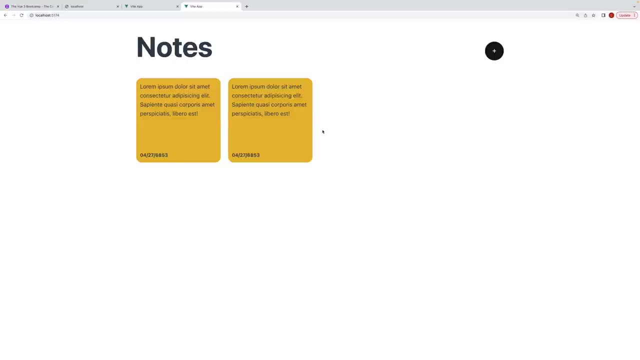 to learn view okay there we go so now you can see it is horizontally um displaced so the last 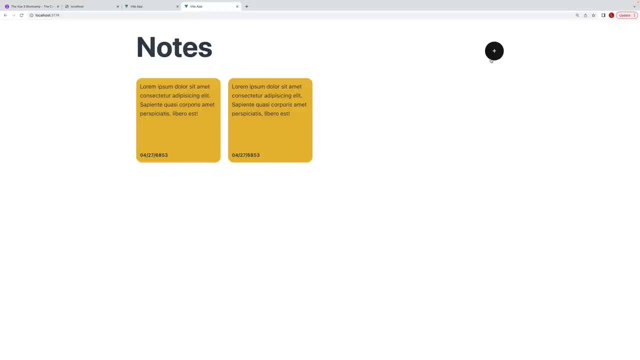 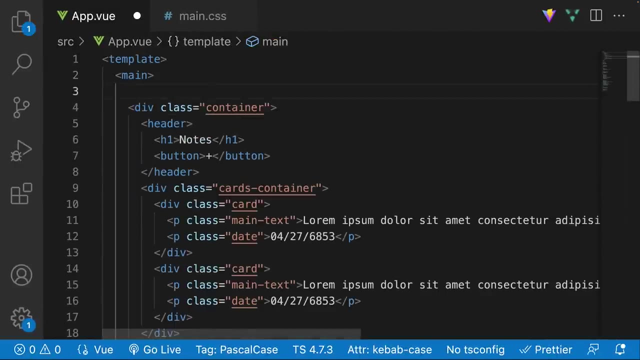 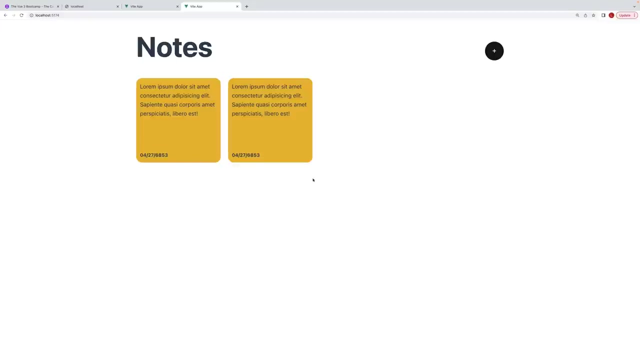 thing that we need is the the modal so this is actually something we're going to build from scratch so right over here so right above this container let's actually create a another div and this div we're going to call overlay so we're going to call this div overlay and the reason why we're going to call it overlay is because it's going to overlay pretty much everything that we have uh over here so we're going to go ahead and style this first and then 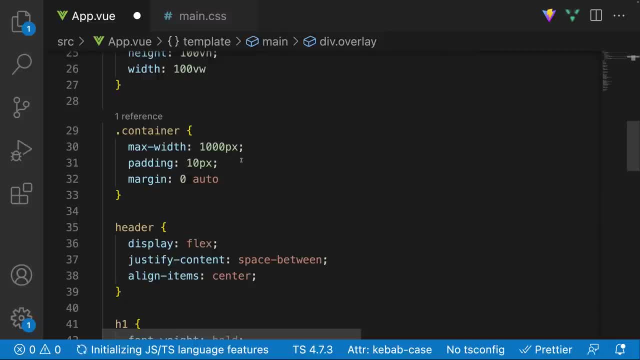 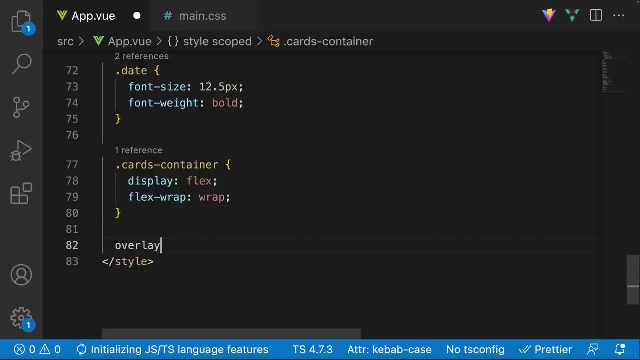 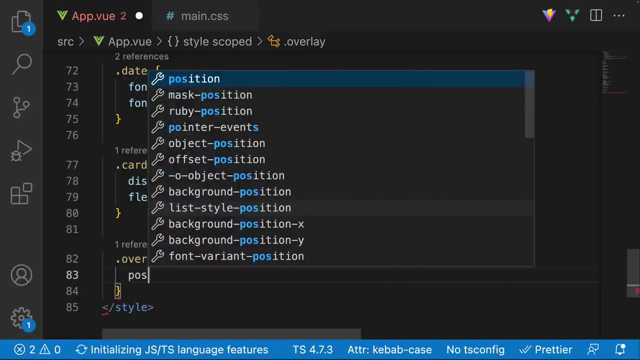 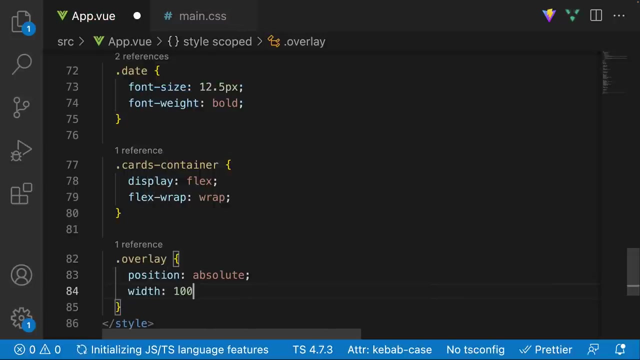 we'll add our modal so let's go all the way down and we're going to go ahead and uh style right here and let's say overlay and we're going to give it just some basic styles so the first thing i want to do is i want to give it a position of absolute so it could just be absolutely positioned above everything we'll also give it a width of 100 percent and this is going to be relative to the main which has a 100 vw and then we're going to say height of 100 percent as well 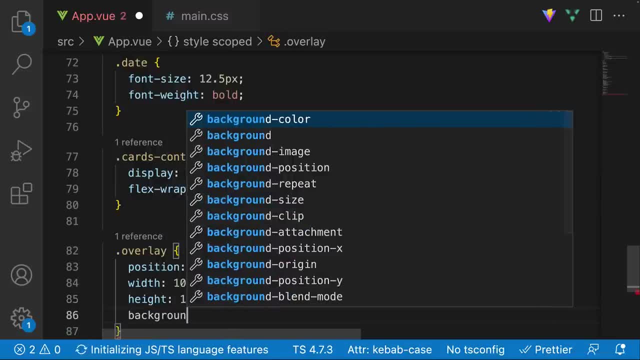 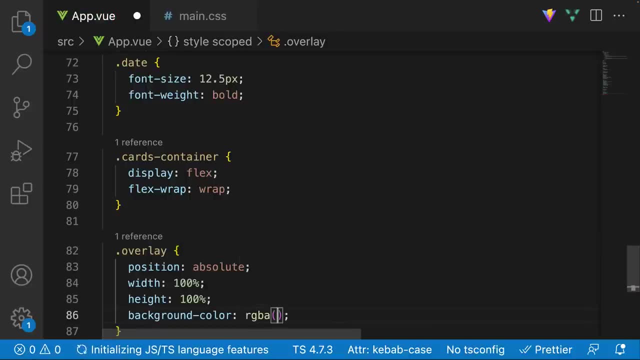 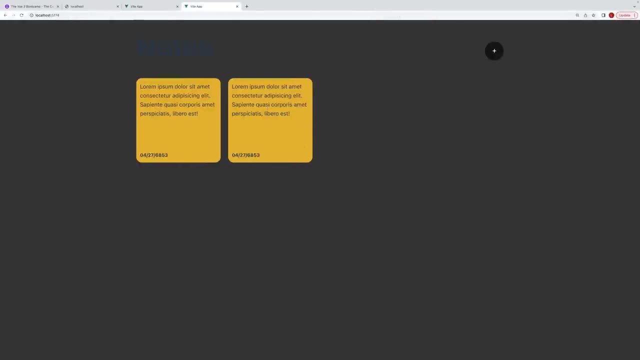 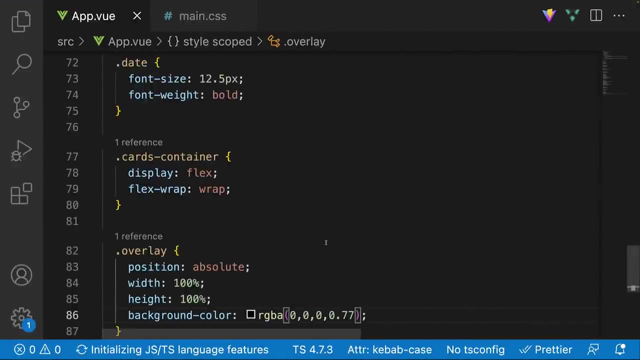 okay now we need a background color so we can say background color here and this time we're going to use an rgba value and then we're going to say 0 0 0 and then 0.77 just so we can have a little bit of opacity now you can see here the cards are kind of like above they're they're kind of more towards you and that's not really what we want so what we can actually very simply do to fix this is just 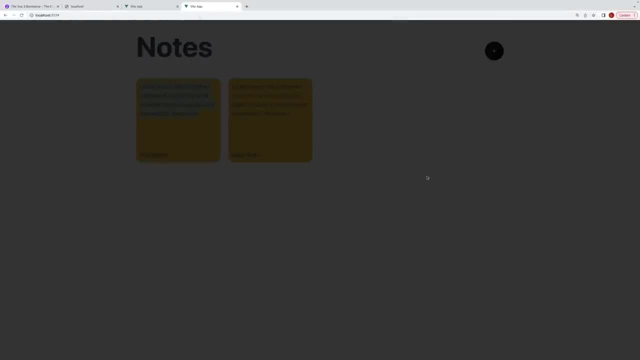 a z index of let's say 10. now you can see now this is above the cards which is what we want 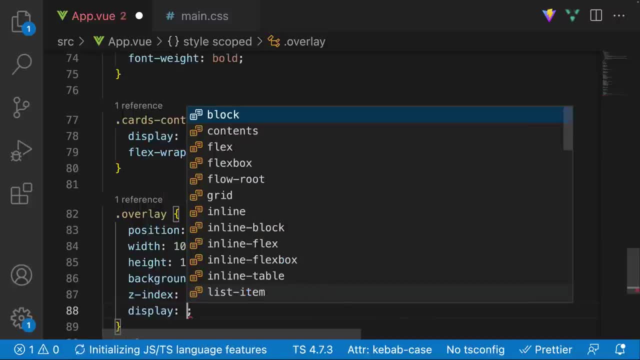 okay so that's pretty good the last thing i want to do is i want to give it a display flex 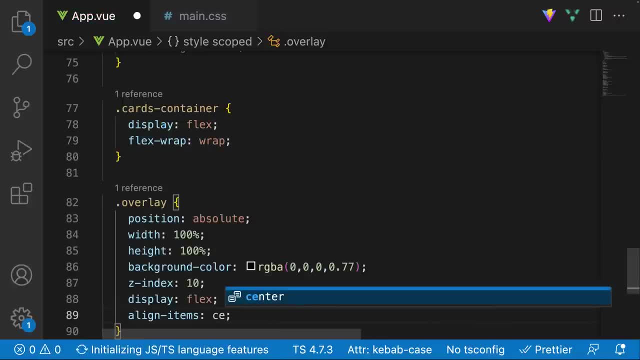 and then align items center and then justify content center as well all right that's pretty 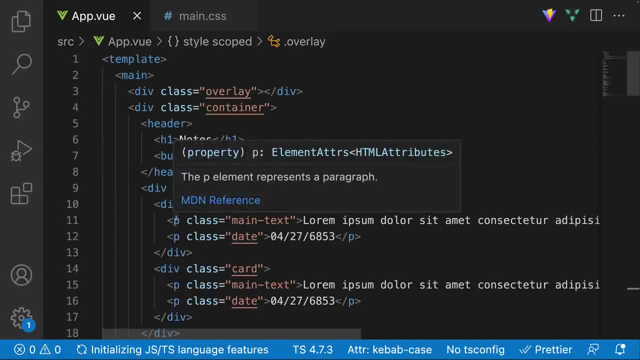 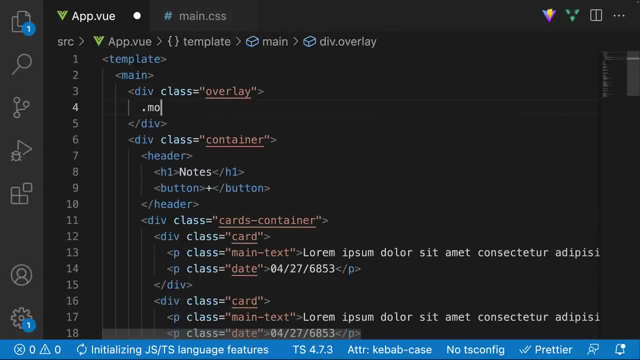 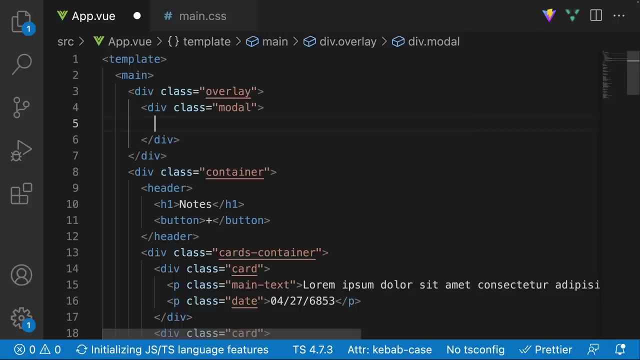 much it for the overlay but now what we need to do is start creating our modal so let's go over here and let's create a div with a class of modal and then within this we're going to have a p tag and 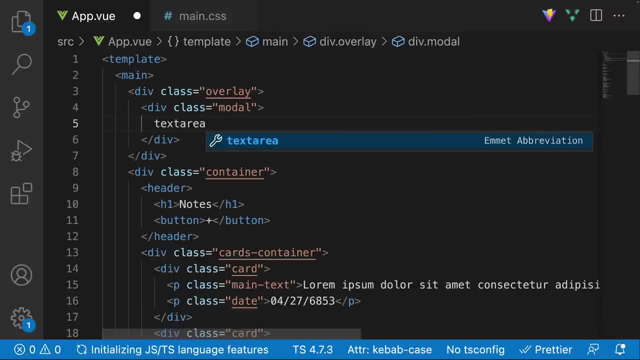 actually know within this we're going to have a text area and we'll just leave it like that we can give this a name of just note an id of note that's fine we'll have this text area and then 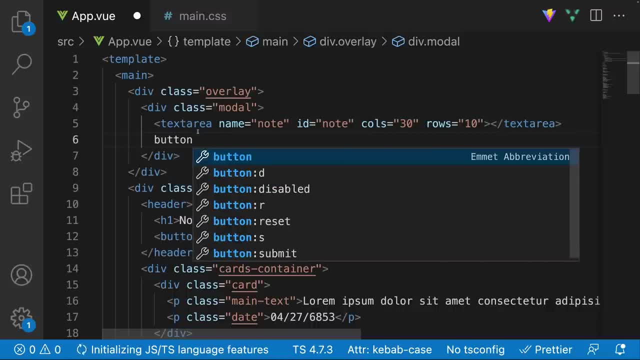 we'll also have a button and uh well that's actually going to start conflicting the styles 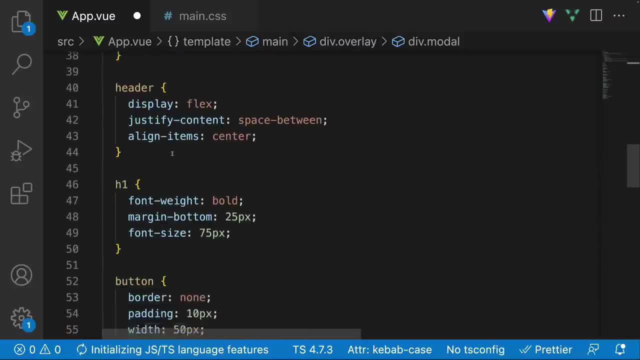 are going to conflict with this button so what i'm going to do is i'm going to go ahead and just go I'm going to do here is I'm going to say header button like this and then over here let's just 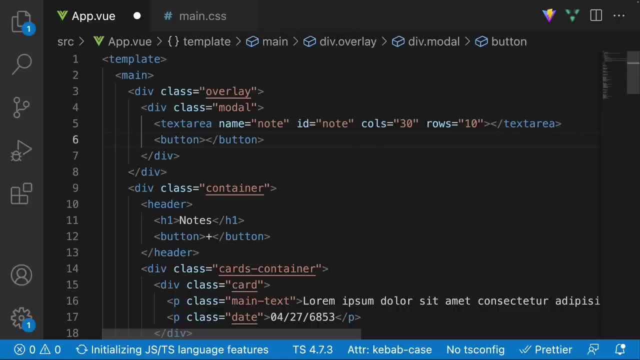 create a button and we'll call this add notes like so all right so that's pretty much all it 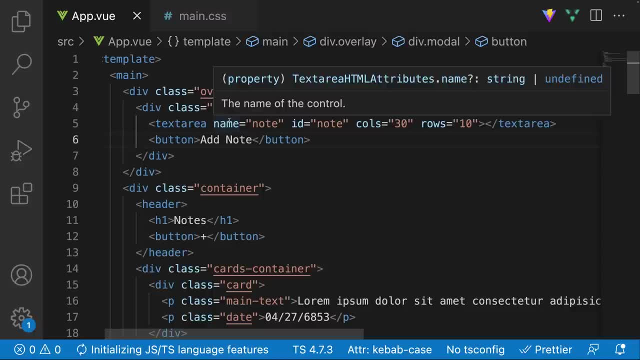 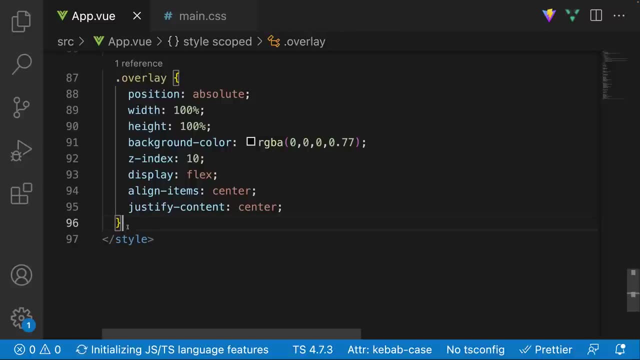 is that we need to do now of course we need to style it so let us move all the way down to style this modal this is kind of why I gave you guys the reason to if you guys don't not interested 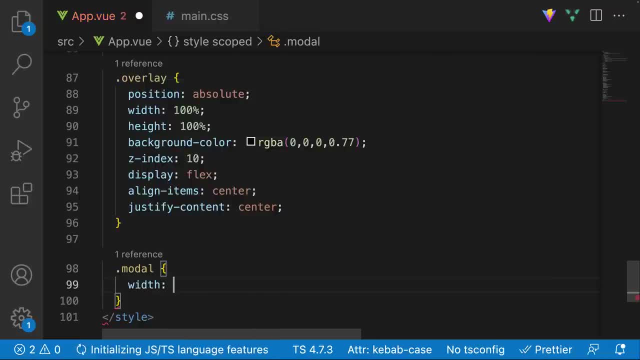 in this you can just go ahead and skip it it's kind of just a bit of styling so we're going to 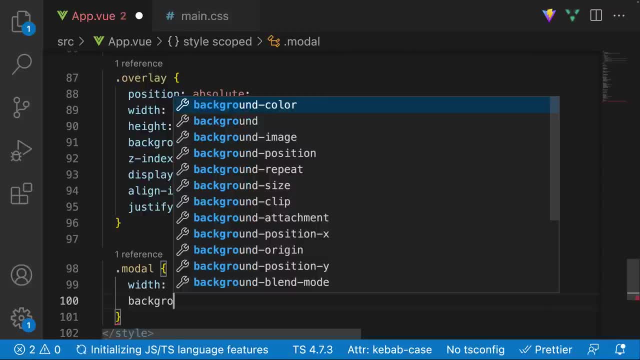 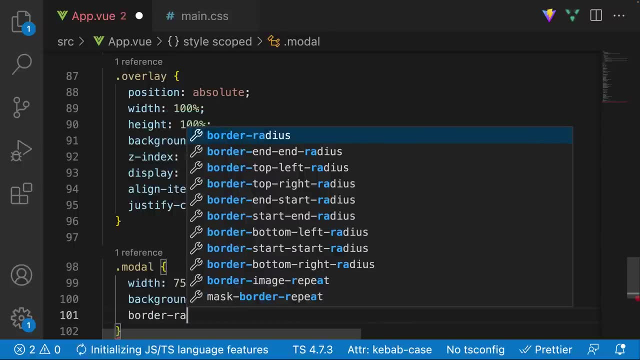 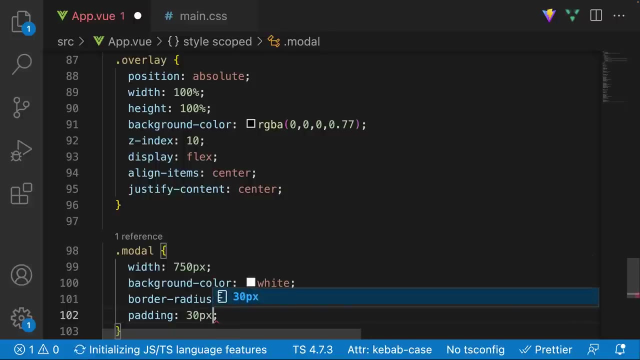 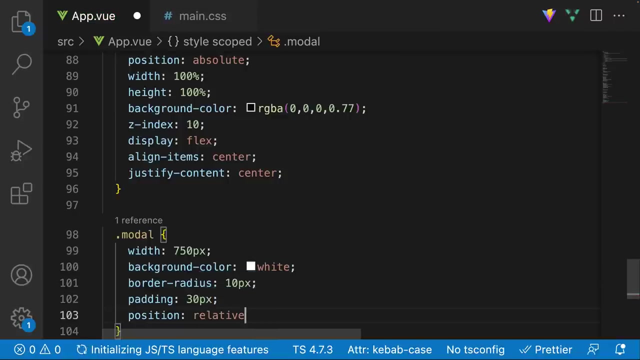 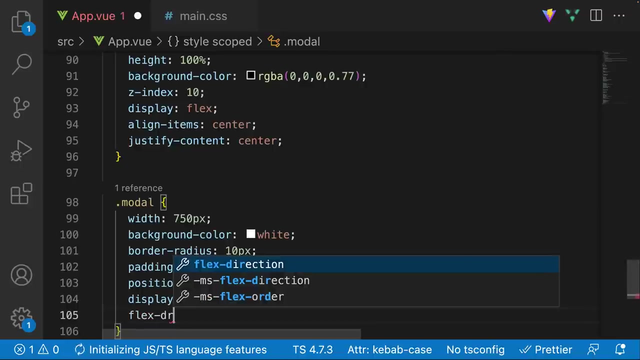 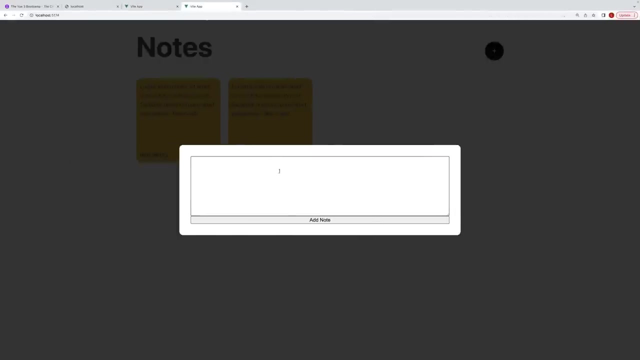 give this a width of 150 pixels we're going to give this a background color of just pure white we'll also give it a border radius of let's say 10 pixels we'll say pass padding of 30 pixels and let's give it a position of relative a display of flex and lastly a flex direction of column beautiful all right so that should create this which is 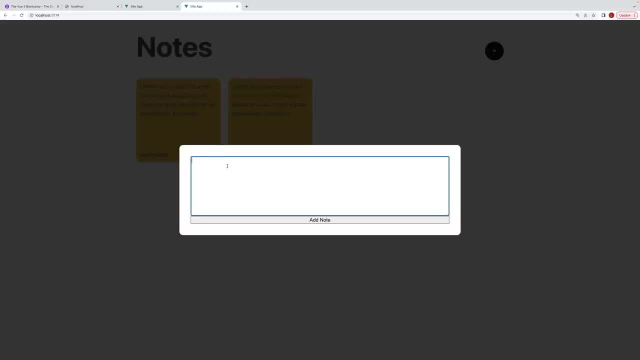 looking pretty good let us now style the uh let's style ohl 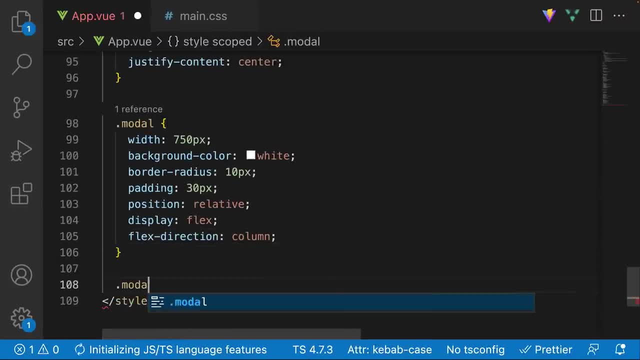 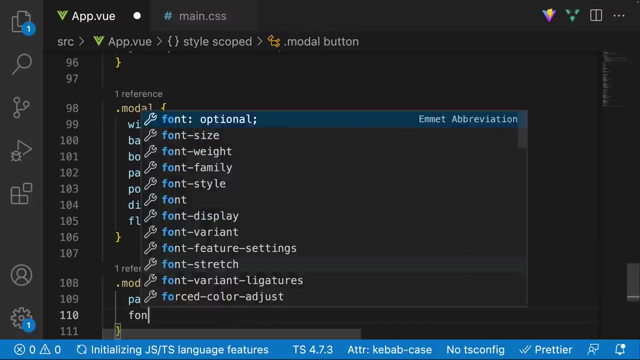 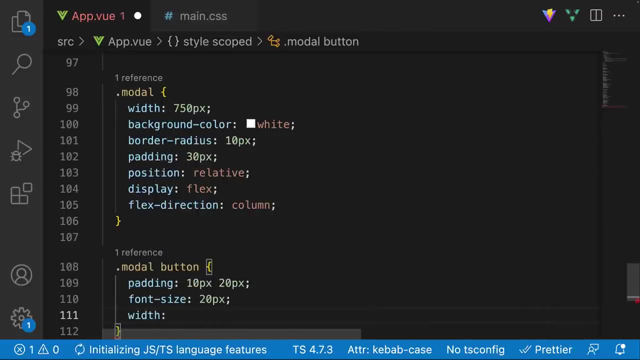 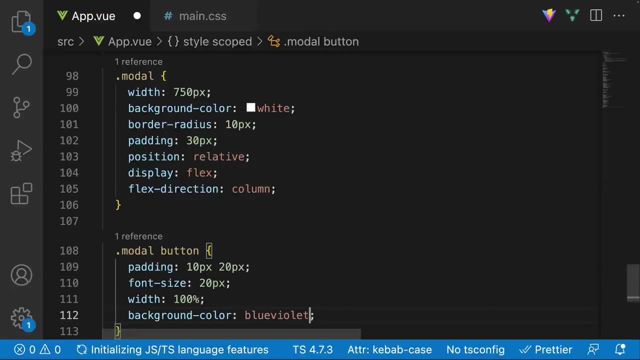 the let's go over here let's style the button first actually so we'll say modal button and we're going to give the button some padding so padding top and bottom so 10 pixels and then left and right 20 pixels and then we'll say font size and then 20 pixels and then width we'll say a hundred percent and we'll say the background color for this will be we'll say blue violet we'll say border of none we'll say color of white 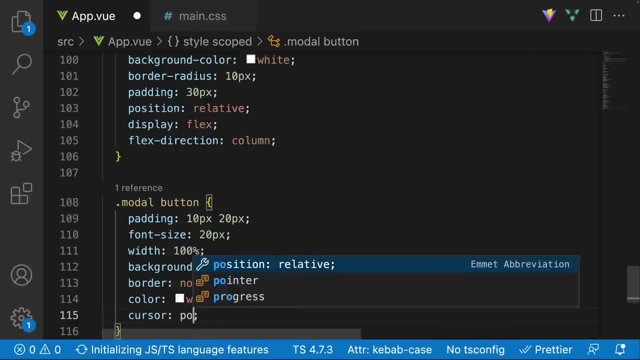 a cursor of pointer and lastly a margin top of 15 and we'll say border of none and we'll say border of none 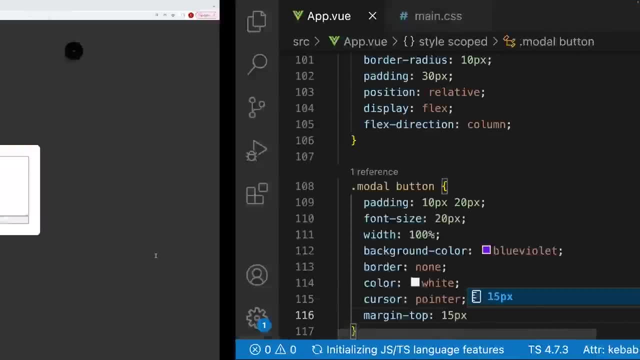 pixels save that there we go we have our button and that's honestly pretty much it the text area 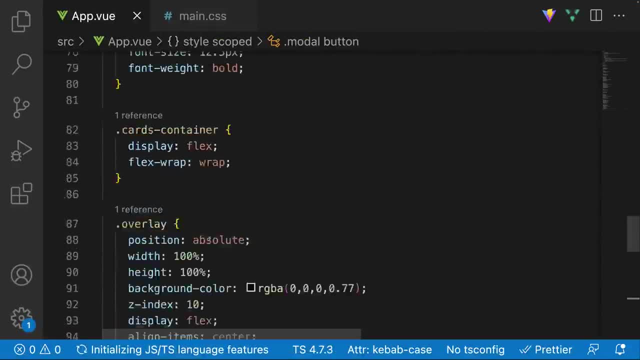 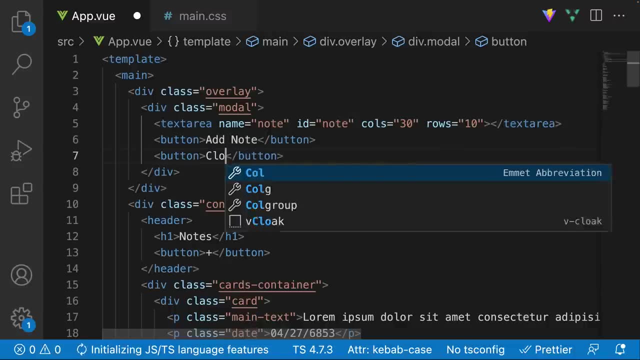 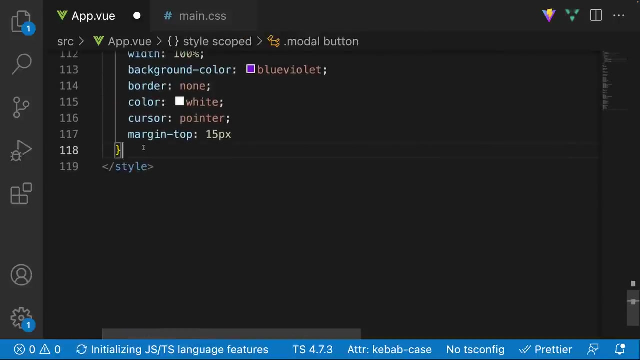 looks pretty good we just need a way to close this so what we're going to actually do here is we're just going to add another button so let's go over here let's add another button and we're just going to say close let's just give this a class of close so over here we can just say dot close and maybe just give it a background color so maybe we can change it to like a darker shade of red and uh it's purple so why is that uh let's say oh let's say node modal 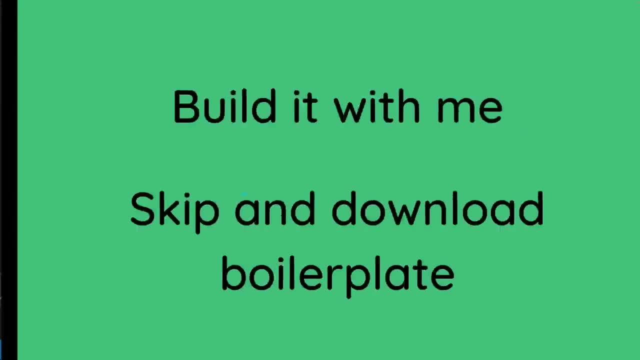 tuted motel dot read look maybe say dot retrospect 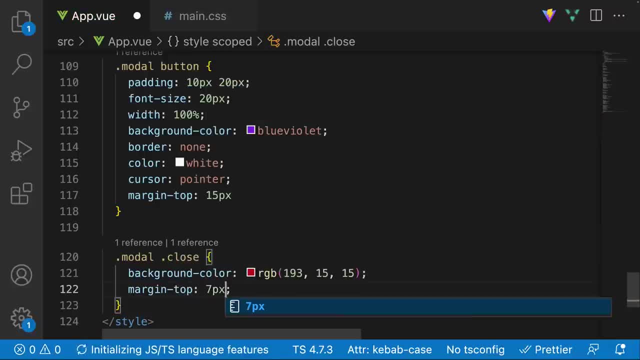 there we go and maybe we can give it a margin top of like seven pixels and there we go looking really good so that's pretty much it that. link 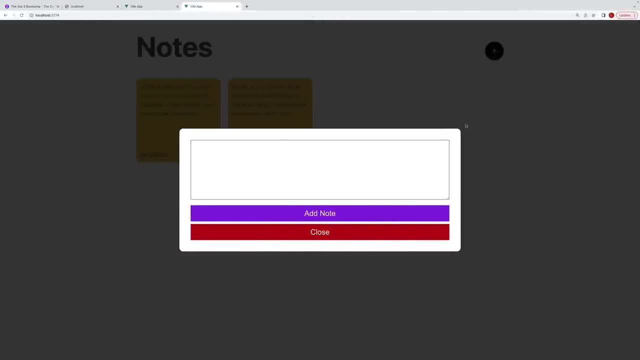 really good so that's pretty much it that is the html structure now for now what we're going to do 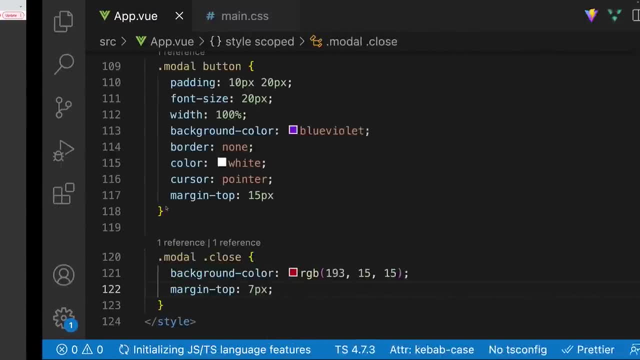 just so we can actually just get out of this modal because i do not want this modal to appear for now 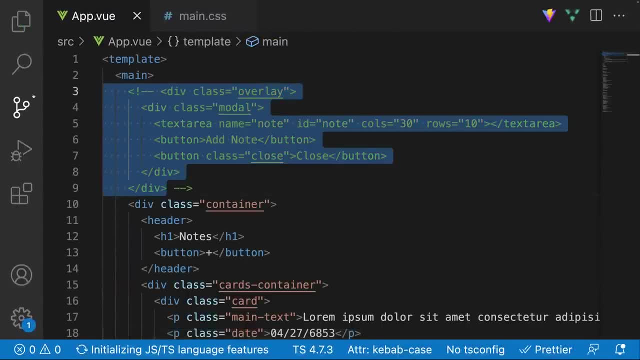 is we're going to go ahead and just comment this out but at least now we have the html and the css 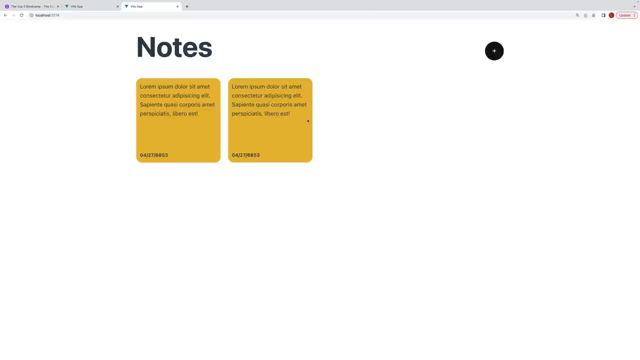 so whether you took the route of just very simply getting the boilerplate or you wrote out the html 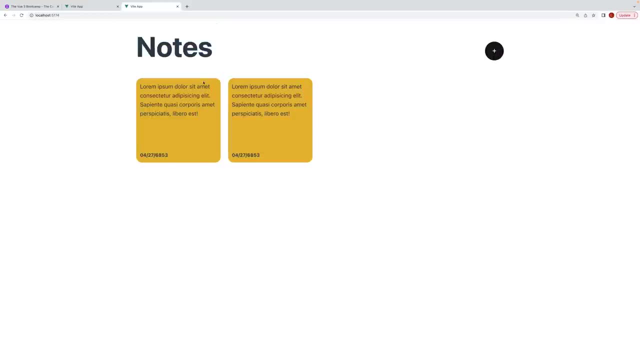 and css at this point in the video you should have an application that looks like this so the 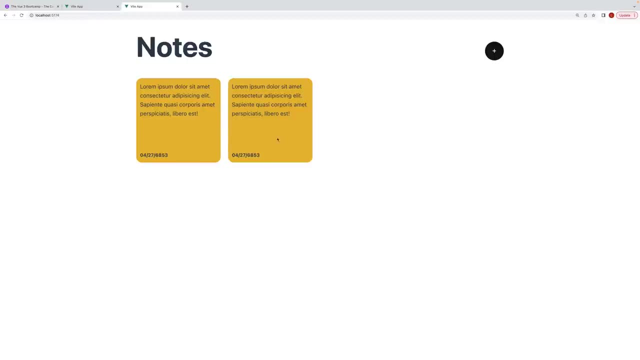 very first thing that i want to do to make our application functional is to very simply make 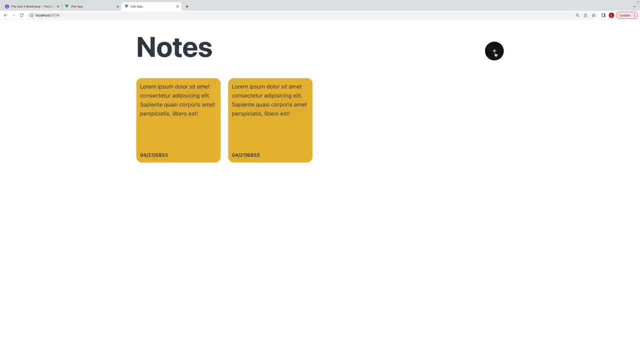 this button right over here work so right now of course when i click it nothing happens however if 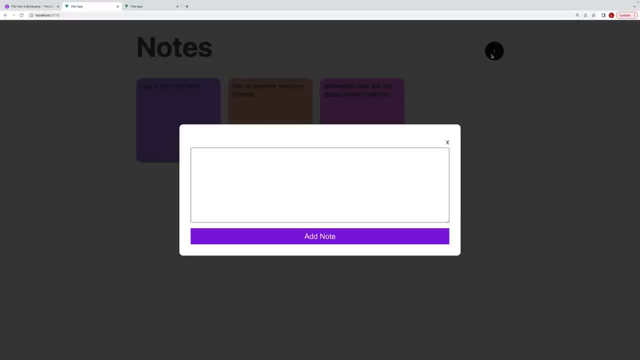 i go to the complete application when i click it it triggers this modal to appear and then when i click close as you can see here 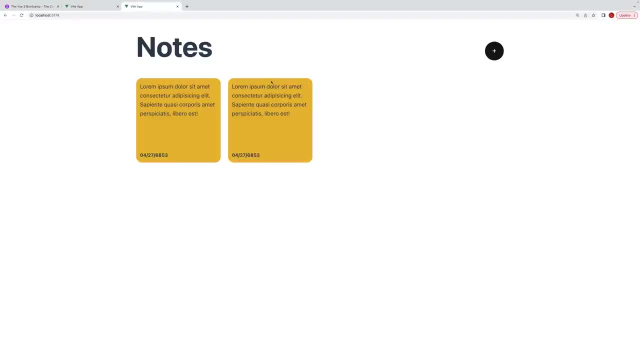 the modal closes so this is what we are very simply going to do in this application so how 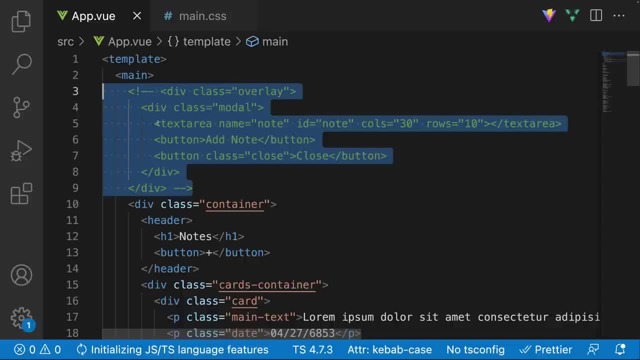 are we going to do that well right over here we commented out the modal html element so if i were 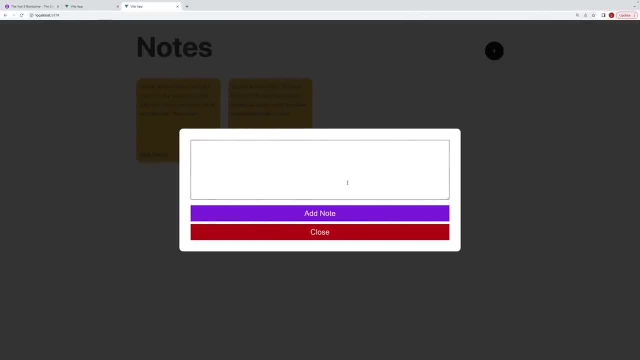 to uncomment them you can see here that we get our modal and instead of having a close sign right 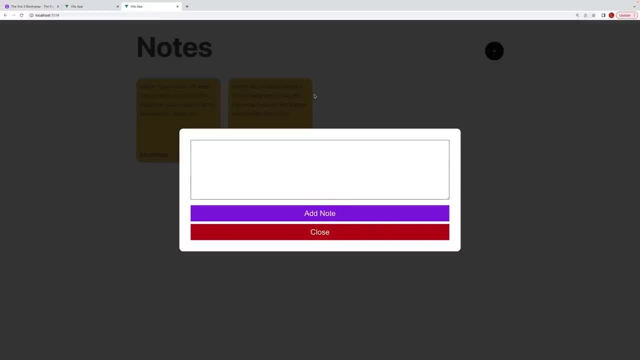 over here i just added a button that's why it looks a little bit different so what we want to 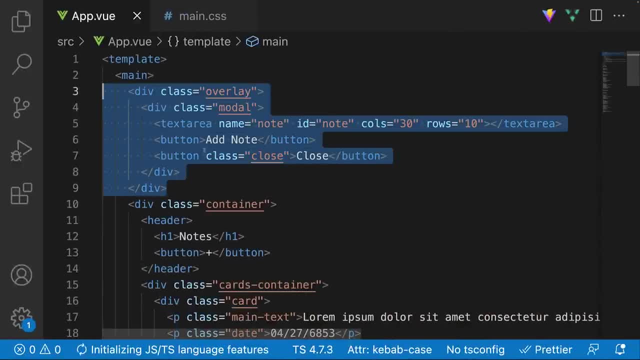 do is to either render these html elements or we can either render these html elements or we can render these html elements or not depending on whether the user clicked this button or not now what 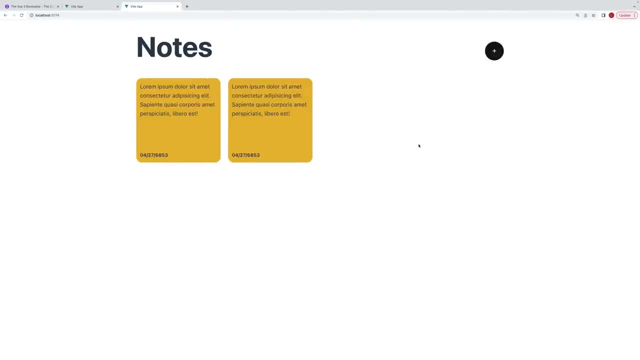 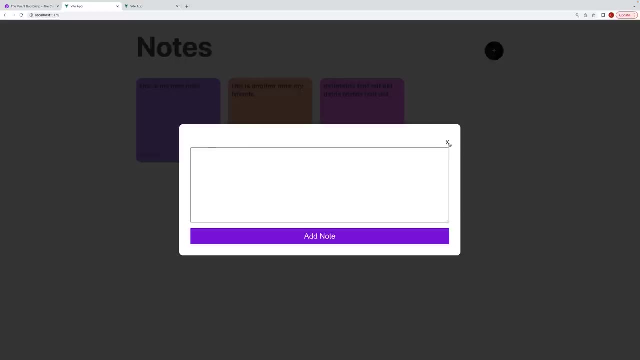 does this sound like to you well this sounds like state to me our application is either in a state where the modal is nice and rendered or it is not rendered so what we're going to need to do is well 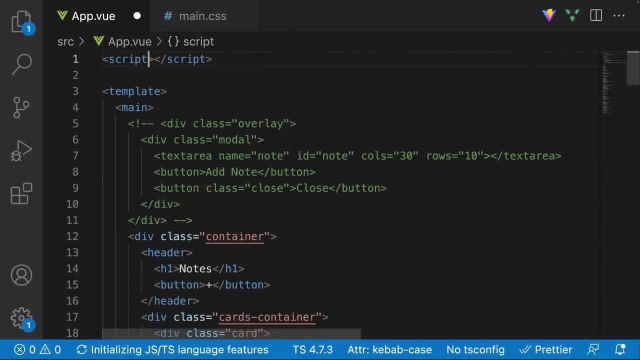 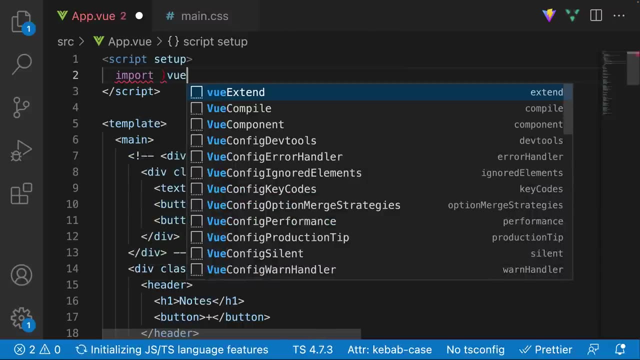 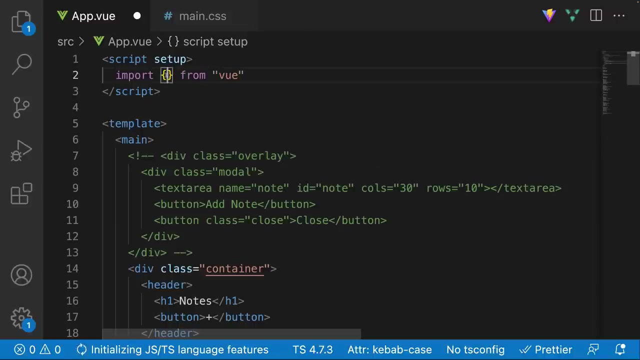 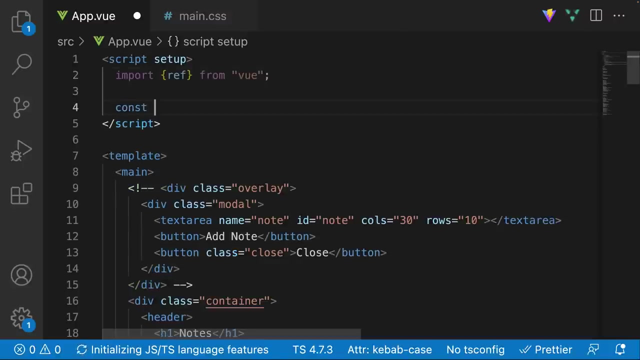 let's go over here we're going to create script tags let's provide the setup and we're going to need to define our state so of course we're going to need to define the state and we're going to define state we have to tell view that this is explicitly state so what we're gonna say here is from view we are going to import something called ref alright so let's go over here now let's go ahead and import that and I'm gonna call my state show show modal like so and then over here I'm gonna say that that is gonna be equal to and initially I'm gonna set this to false so this is gonna be a boolean value and initially it is going to be false so let's actually just go ahead and save this and now actually what I want to do is whenever I click this button right over here this plus button I want to change this to true now 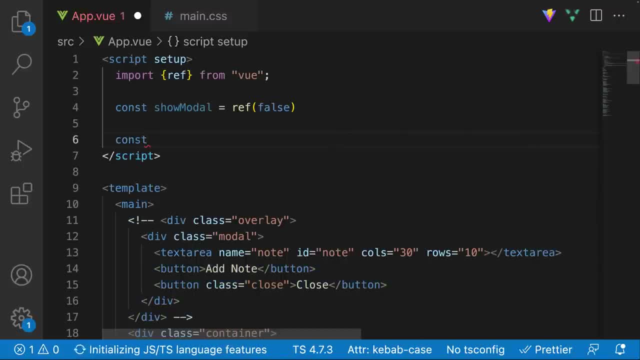 I could create a method handler for this for example I can create something like 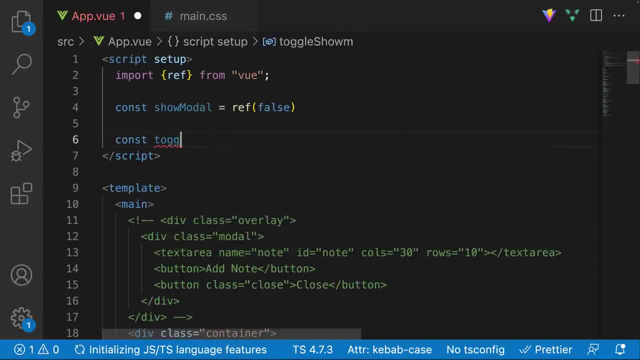 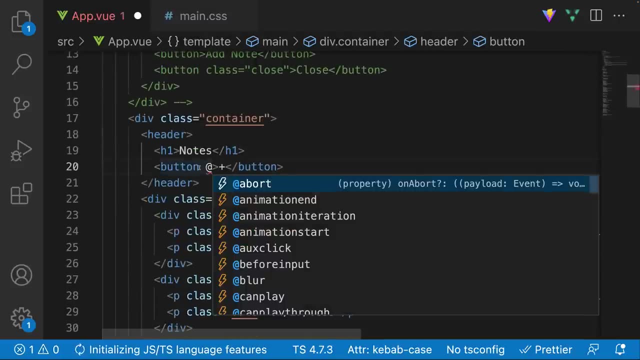 toggle show modal or whatever and then I can invoke that call within here within the the , click handler that I'm going to add here or what I can very simply do 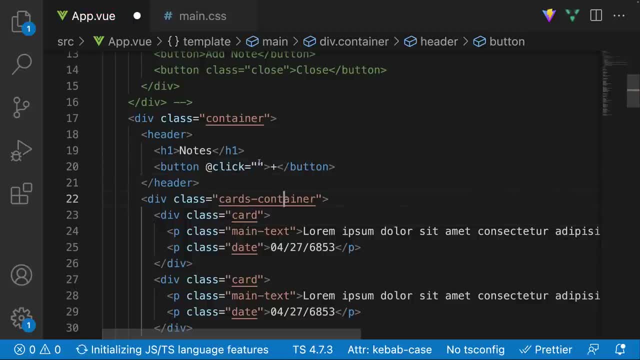 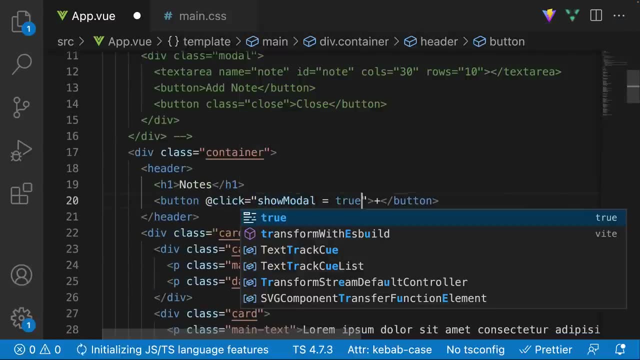 because this is just plain old JavaScript within these strings I can just very simply just say show modal is equal to true so show modal is equal to 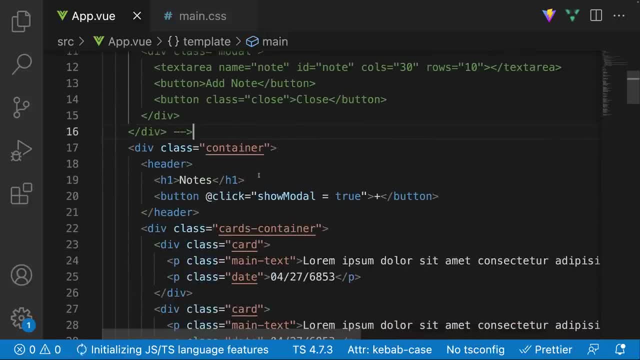 true and that's really all it is that we need to do so just to prove to you that 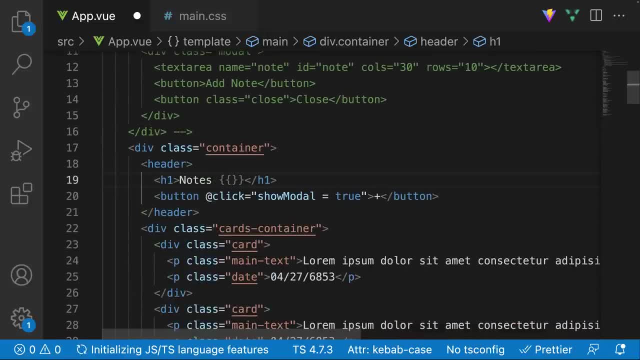 this works right over here so right within the h1 I'm going to use the curly brace curly brace and I'm just going to go ahead and render the show 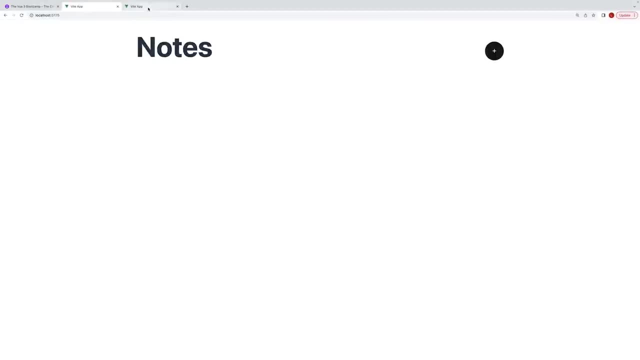 modal value so let me go ahead and refresh this you can see initially it's 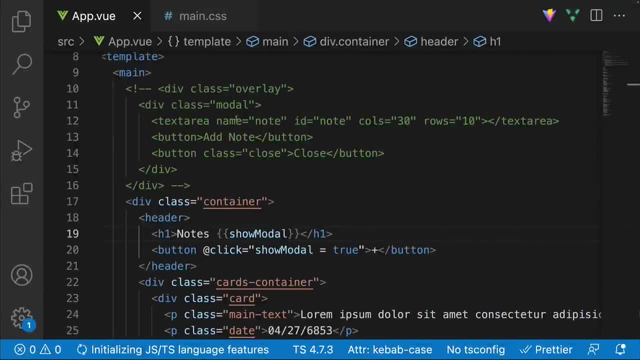 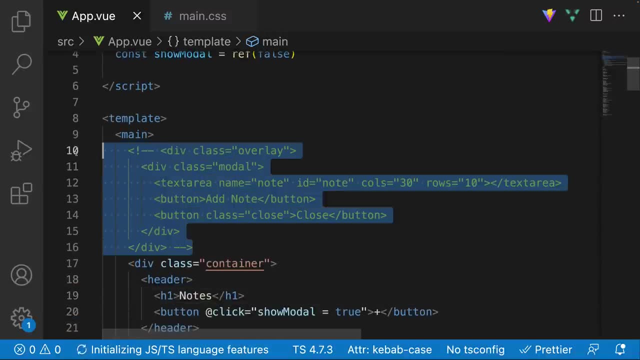 false if I were to click on this now it is true okay so now that we got that out of the way what we need to do now is to well render these HTML elements if this 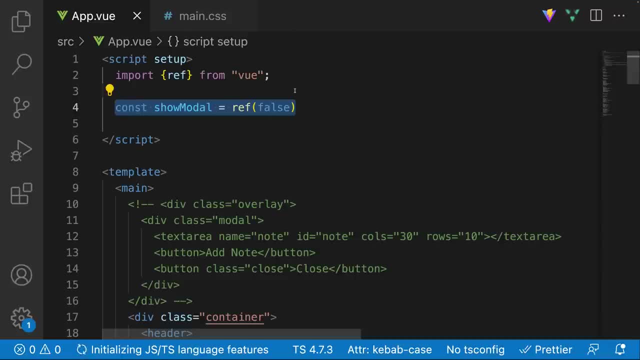 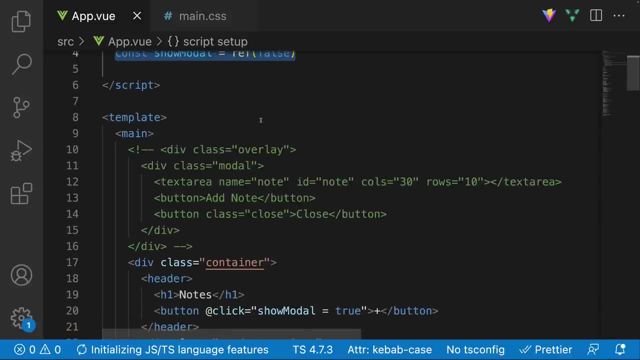 is true however if it's false then we do not want to render them and this actually seems like a daunting task but it is really easy and it's really 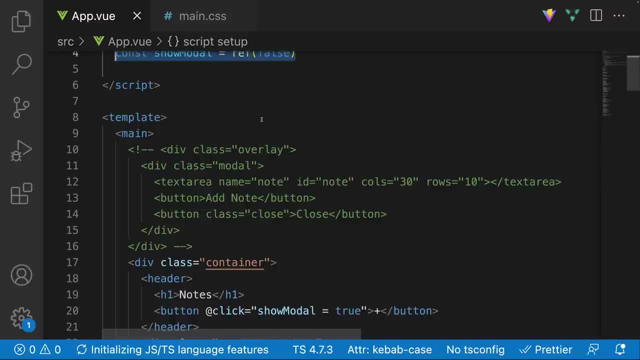 easy because view gives us a bunch of directives that we can utilize to 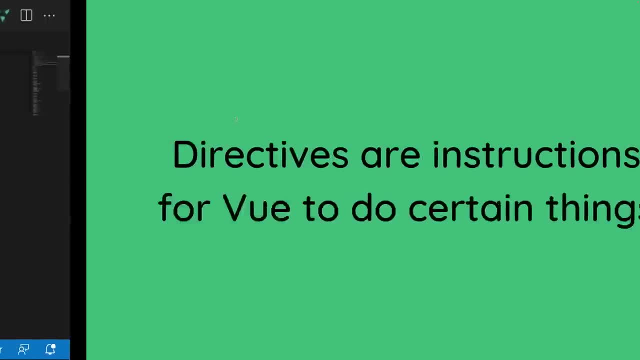 manipulate DOM elements now you might be wondering what in the world is a directive well very simply put this is just a very simple definition a 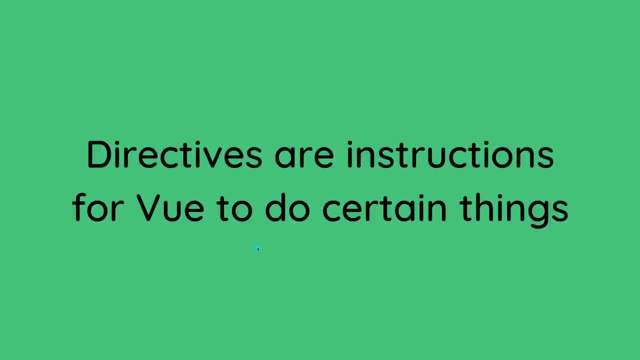 directives or directives are instructions for view to do certain things and they are placed on the HTML elements themselves so what we want to 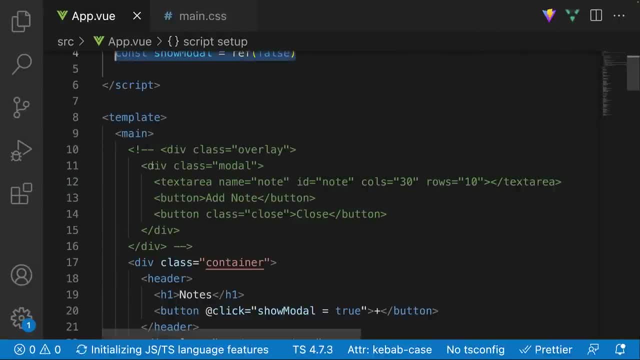 do is we want to have a directive that is going to instruct view hey I want you to just render these HTML 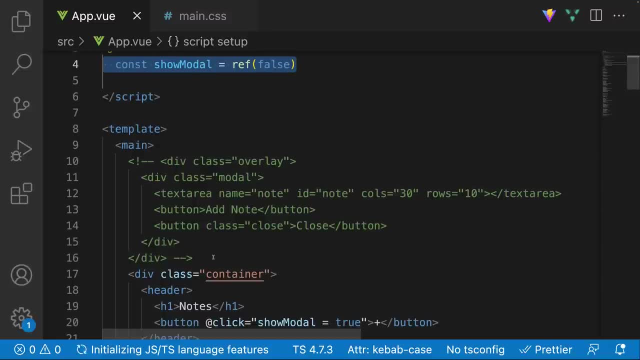 elements if this is true and well if it's not true then I do not want you to render these HTML elements that is the directive that I want so let me go ahead 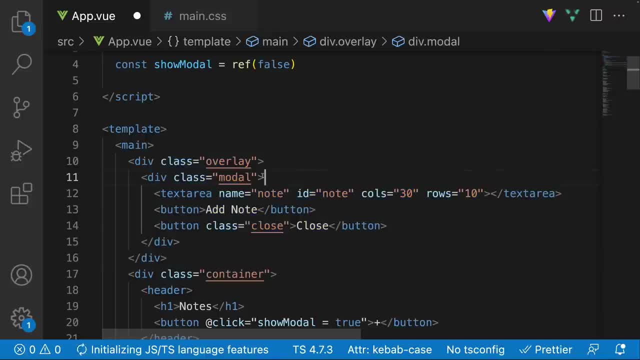 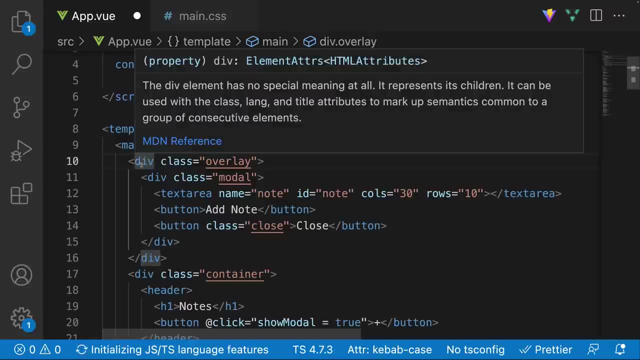 and uncomment this with command and then question mark and then right here on the parent HTML element that we either want to render or don't render we're going to 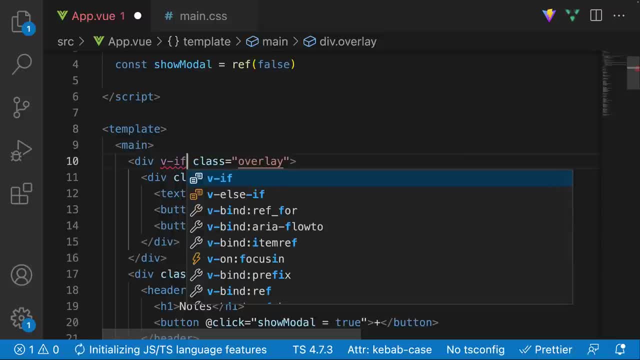 add the V if directive and what this is going to do is going to be equal to some JavaScript and this right over here 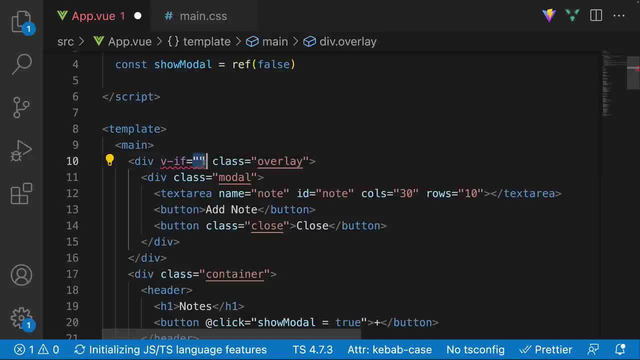 so within this JavaScript this should either be a boolean value should it be a truthy value or a falsi value so very simply here I'm going to say V if show 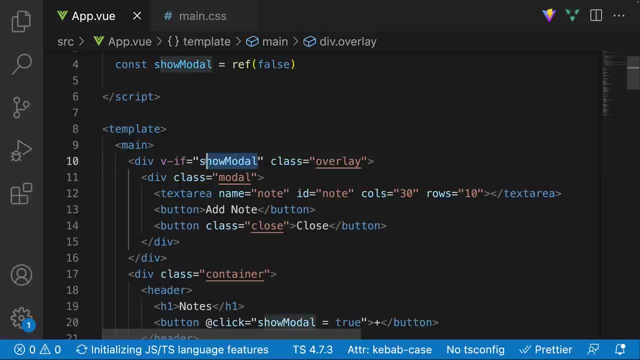 modal so if show modal is true what this directive is going to do is it's going 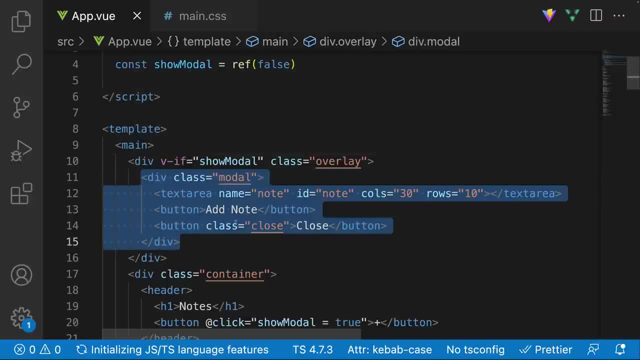 to render this parent element as well as all of its children however if show modal is 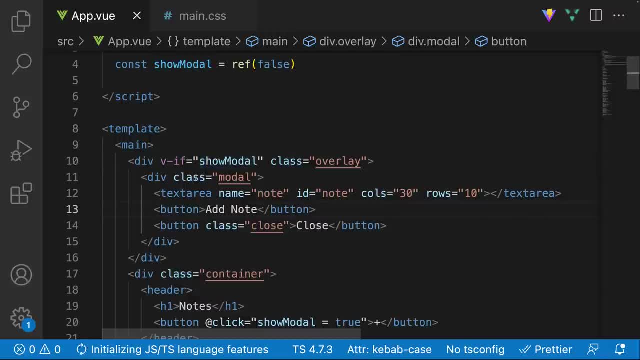 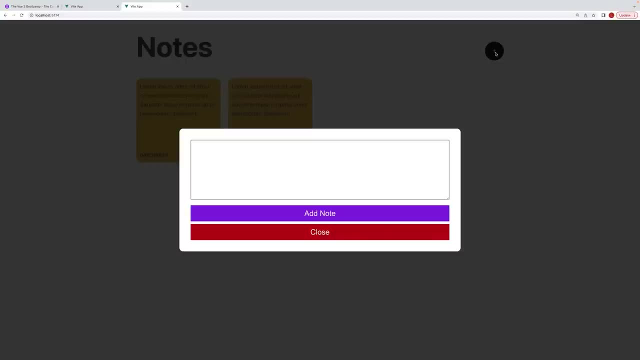 then it is not going to render it at all so I'm gonna go ahead and actually save this and let's go over here and now if I were to click on this there we go you 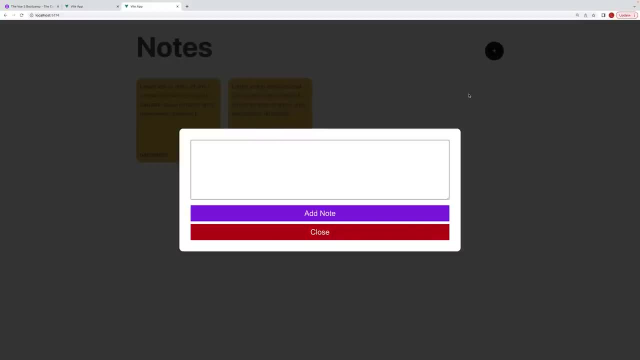 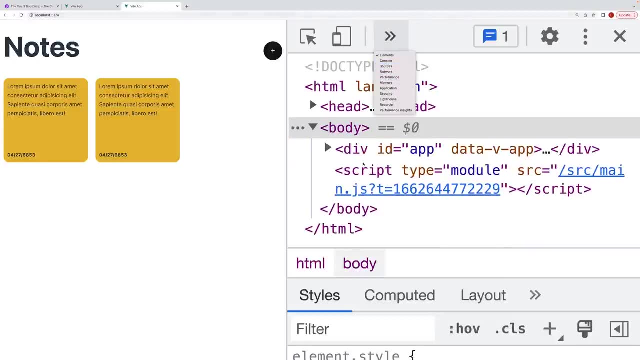 can see now it is rendering it and we can actually inspect that the HTML elements are actually being removed and created so let's go over here to our 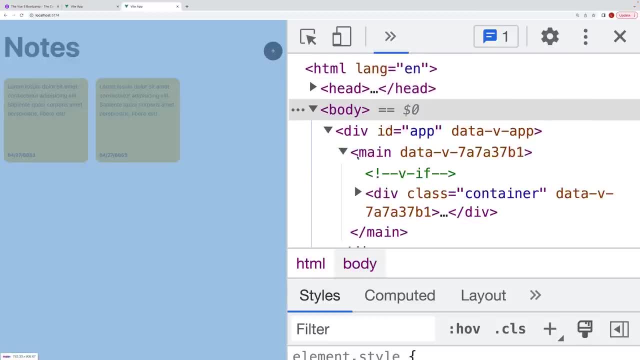 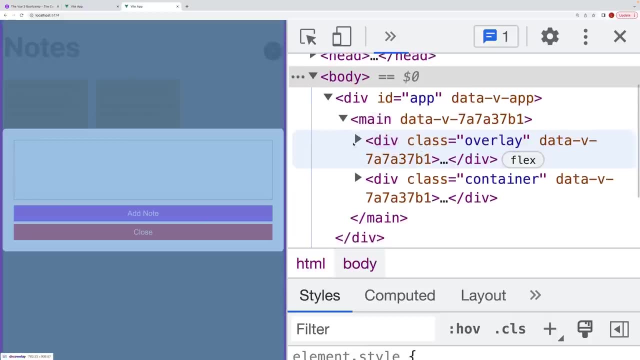 network let's go here let's go to main so you can see here we have this VF comment right over here and when I click on this the VF comment gets replaced 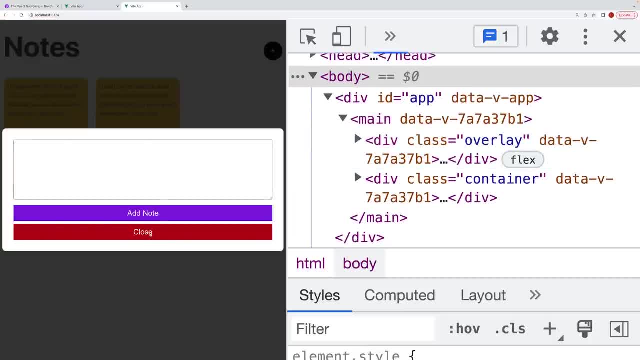 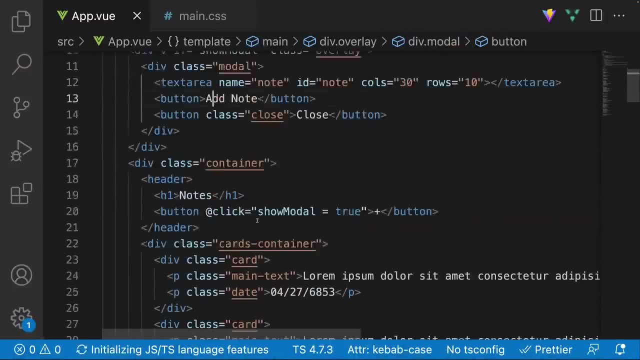 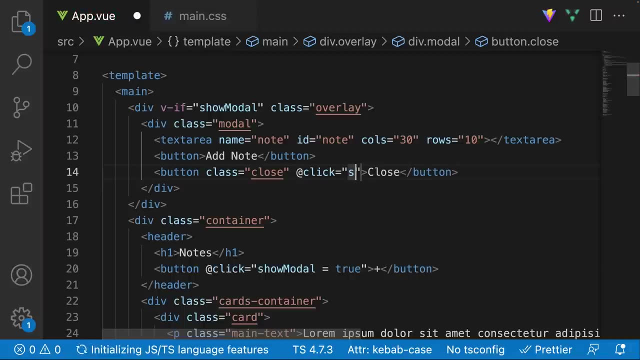 with the actual div elements so now let's actually do the same thing but this time we want to actually remove this when we click this close button so let's go to over here to the close we're gonna say at click and what I'm gonna say is show modal and I'm gonna set that to false like so so there we go you can 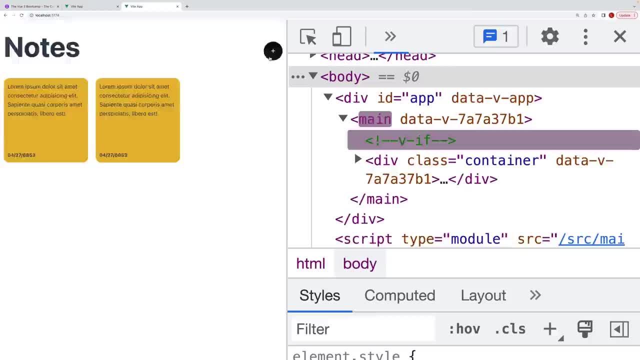 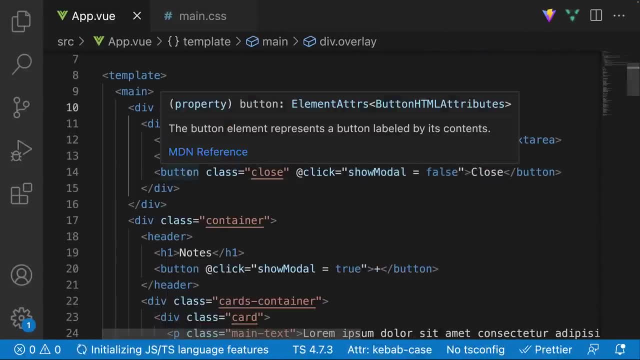 see now we are rendering it back and forth now there's actually multiple different directives that can kind of accomplish the same thing we're gonna go through a list of all of the 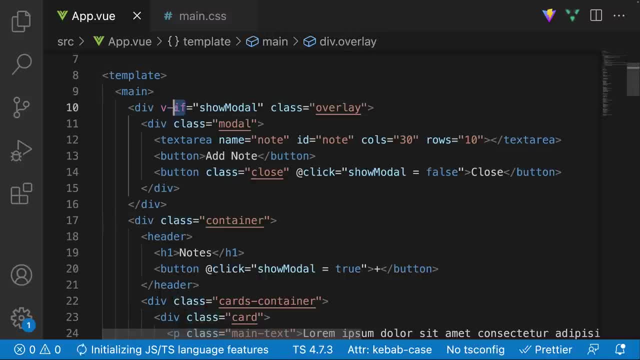 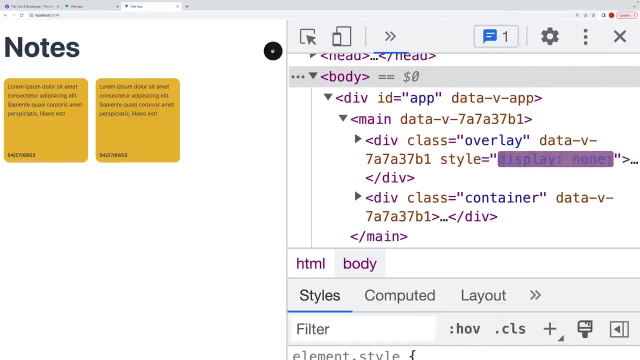 different directives out there we can actually accomplish the same thing with something like the show so if I were to save this and I were to you can see here 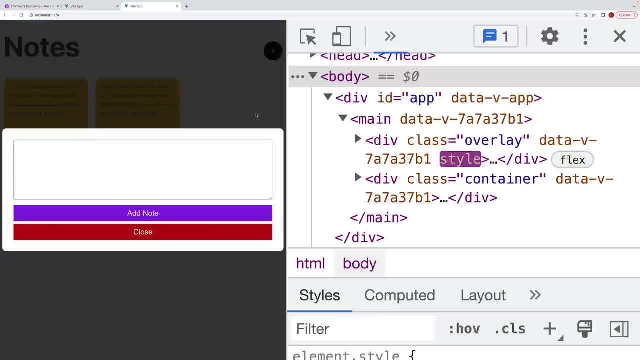 that it is working indeed the exact same way so you might be wondering what is the difference between VF versus the show well let's actually take a look at the HTML 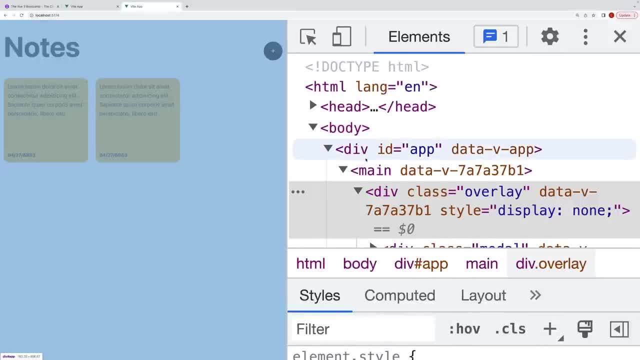 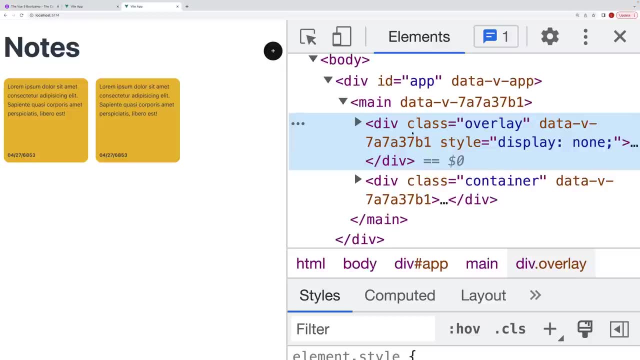 elements so I'm gonna go ahead and quickly refresh and you can actually see with the show the actual overlay div is still there even though we are not 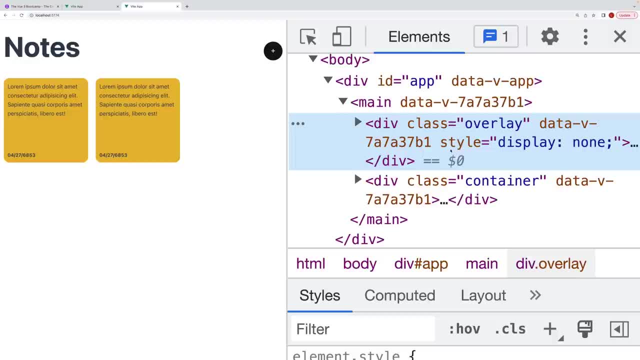 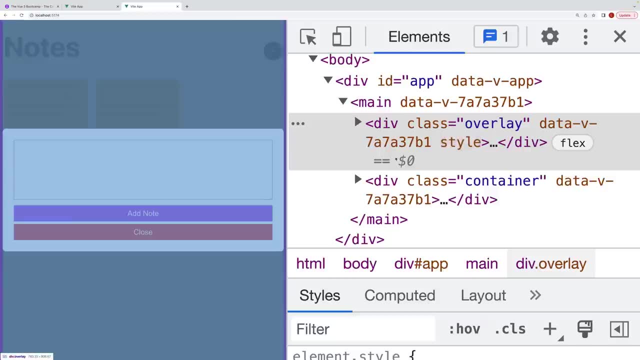 presenting it however stylistically you can see it adds the styles of display none now over here if I were to click on it now that's this the style of display none is gone but the div element is still there and was always there so we 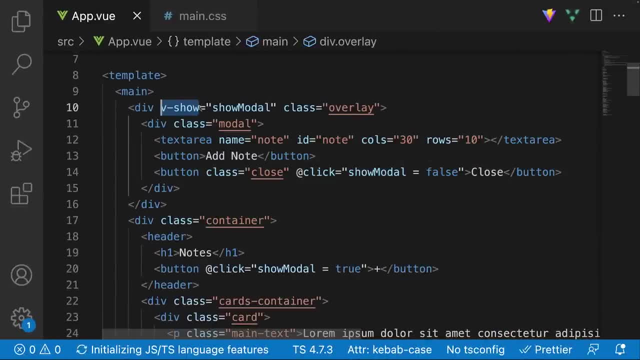 can again accomplish this so VF is not rendering it's showing something different to the overall 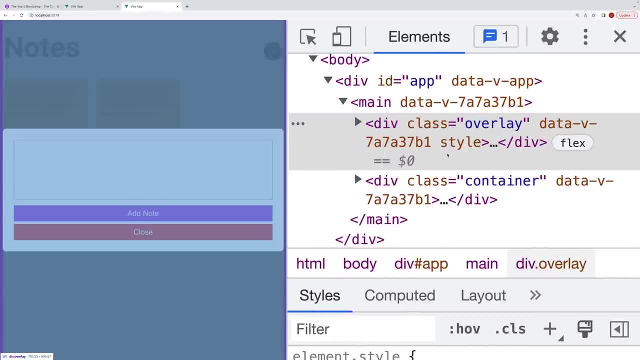 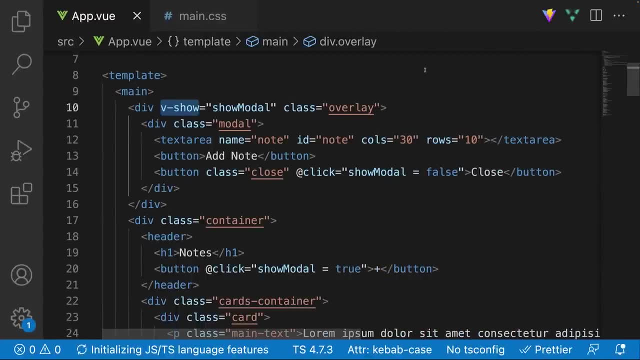 sight and uniformity of the style it has a display of none which means it's just the HTML elements are there but we can't really see them because of these styles and it just toggles that back and forth now when do you want to use one 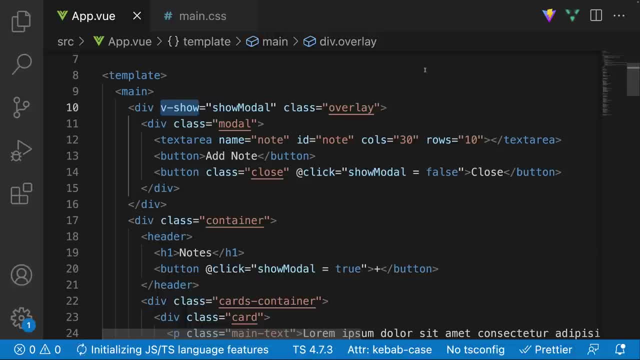 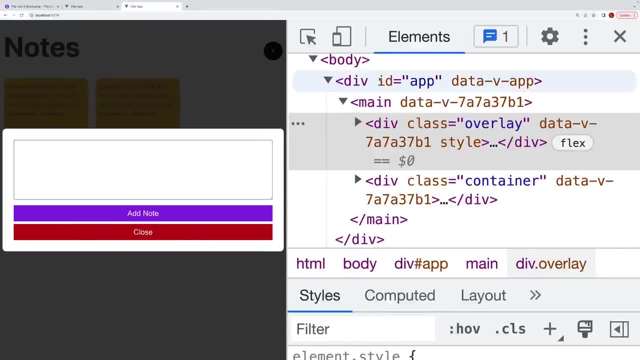 or the other it really depends on your situation maybe you have a lot of information on let's say the disability of any of these elements so it's perhaps interesting to exploit a little bit more of this information around the let's say, your modal or whatever card you want to render, and it's really, really good for SEO, for readers, and it might really promote your website. 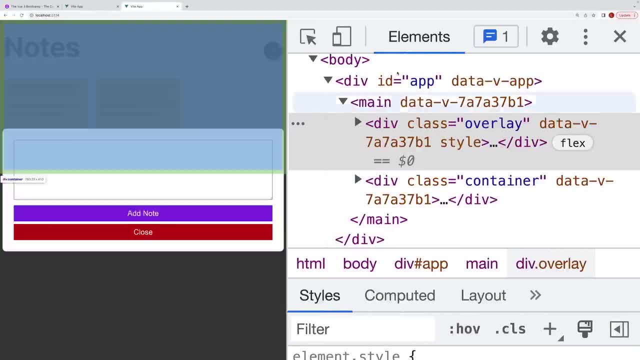 So if you did something like a VIF, that HTML isn't going to be within there. So it's just not going to be caught by the readers, and it won't promote your website. 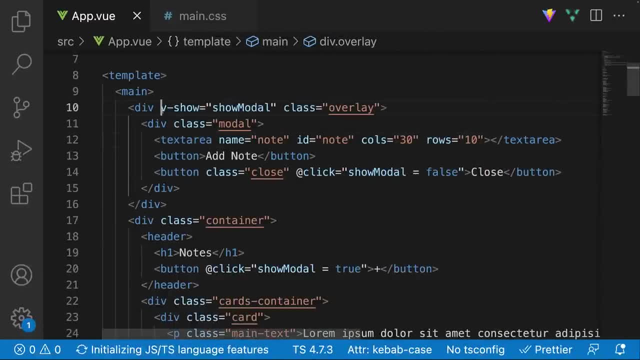 So maybe in that case, it's actually better to do a VSHOW rather than a VIF. However, if it's something like this, 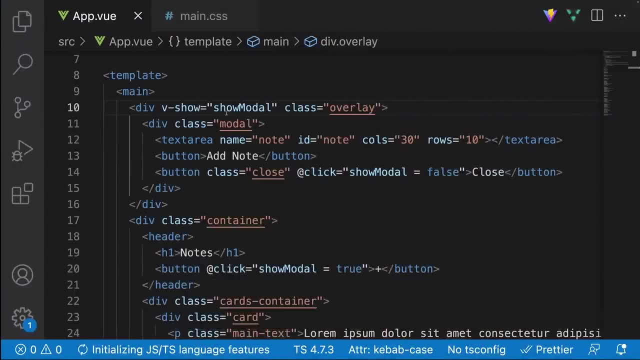 where we don't really care if this HTML element is present or not, we are going to stick with a VIF. 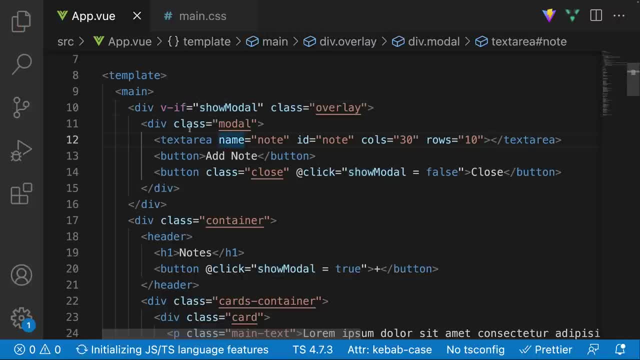 And that is probably the more common convention of doing things. But again, it depends. 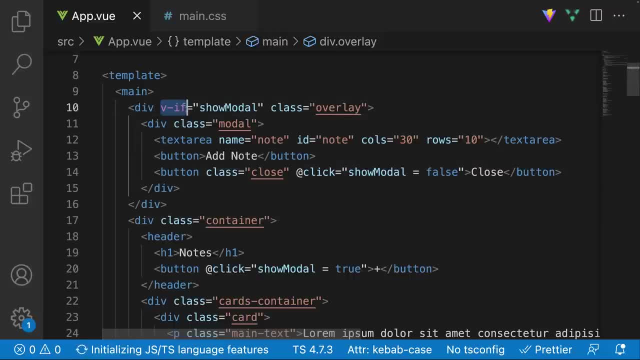 But I want to introduce that to you because, well, these are different types of directives, and we're going to see plenty of directives throughout this project and all of the other projects to come. 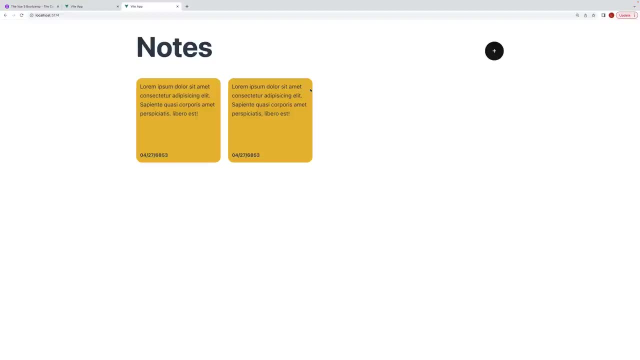 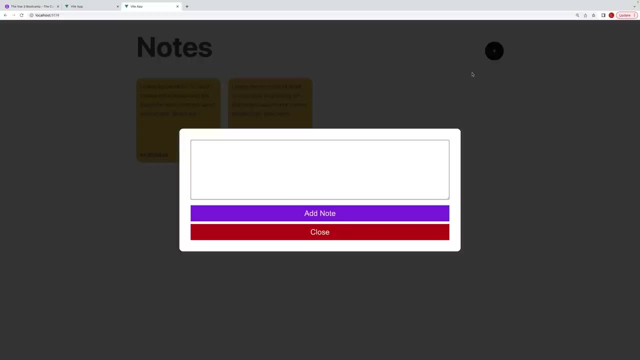 In the last video, we were able to get our wonderful modal to work. So a user can now go ahead and click on this button, and now this... this wonderful modal appears. 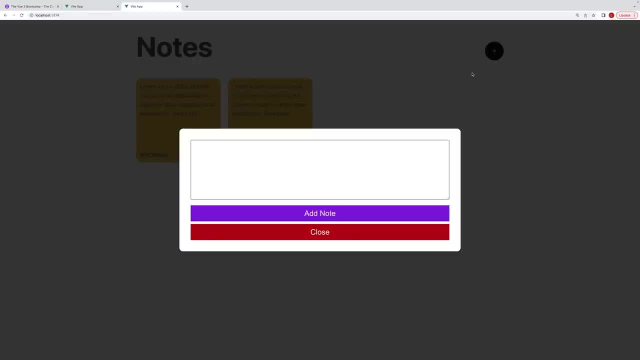 Now, what is the next thing that the user is probably going to do as soon as they click on the button? 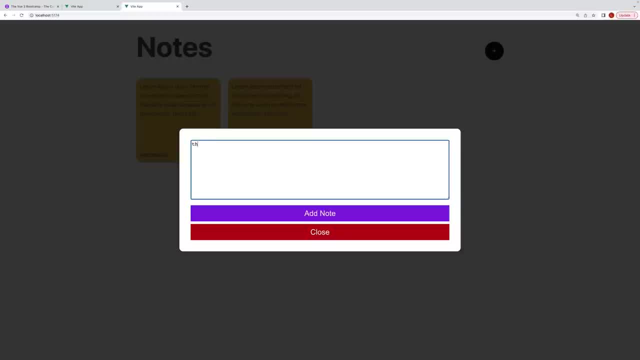 Well, probably they're going to go to this text area and start typing. Type something like, this is a really cool or good course. Please take it. It's good. So they'll probably go ahead and start typing things. 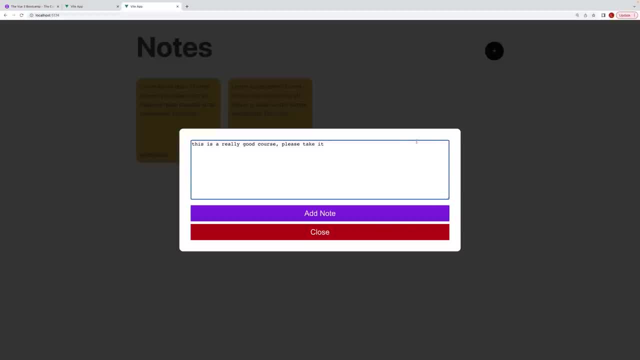 Now, let's quickly talk about exactly what needs to be done when we have some sort of text, text area or input where a user needs to type things inside of a Vue application. You might be thinking, well, there's probably nothing that needs to be done. It's working. Why do I have to change anything? 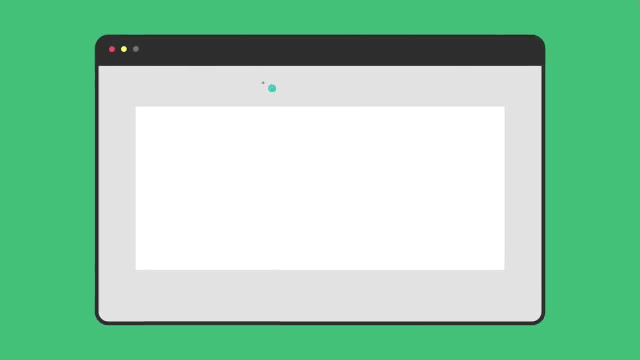 Well, let me explain. So let's go over here to this diagram where we have our browser, and we have this white box that is representative of a input or a text area. 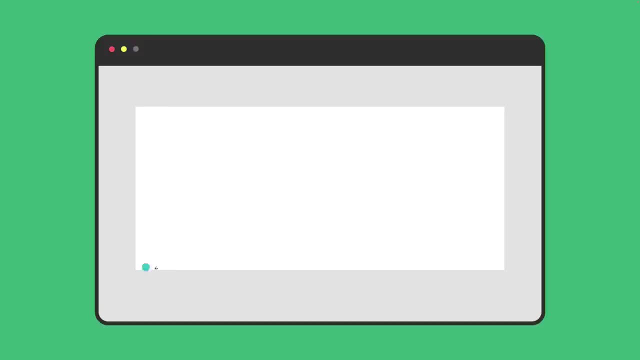 So as soon as a user sees this, it is going to be in a completely empty state. 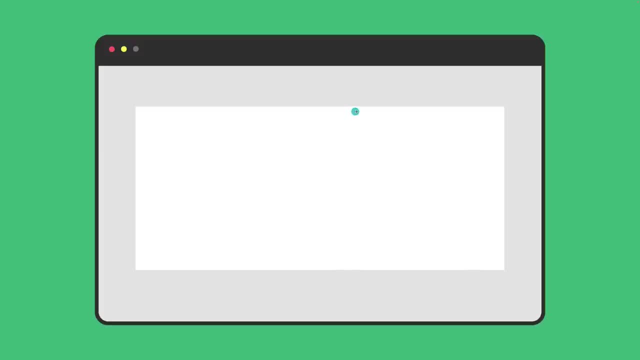 So again, notice the keyword here, is state. 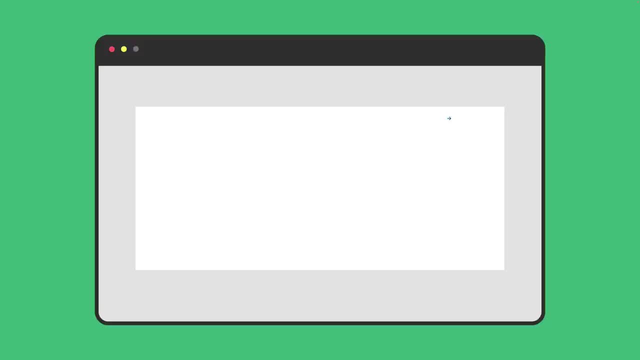 It is completely empty. Our application is in a state where our text area has, well, no value. And then the user is going to start typing into it, which is going to change the state of the text area. So now the text area can say maybe have an H in it, and they can continuously type. 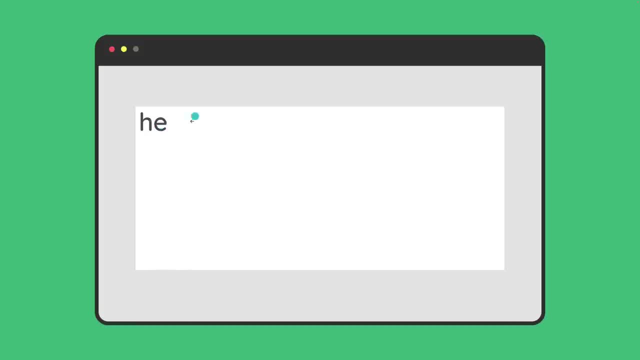 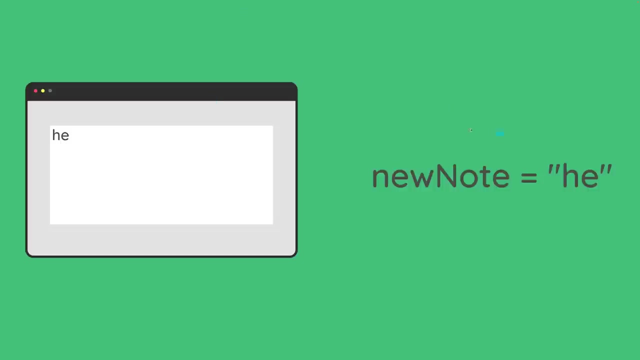 Let's say they type another word in there, H E. Well, now our text area is in a state where it has the value of H. And E now, because we are dealing with state, we actually need to define and store that state within our script tags, similarly to what we have done right over here. So we can call this state, for example, new note, and it should be reflective of the value within our text area. 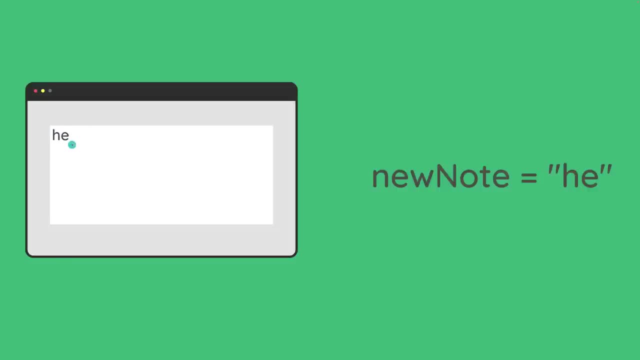 So for example, if we went ahead and added maybe another L that should change our state, so that it becomes H E L. 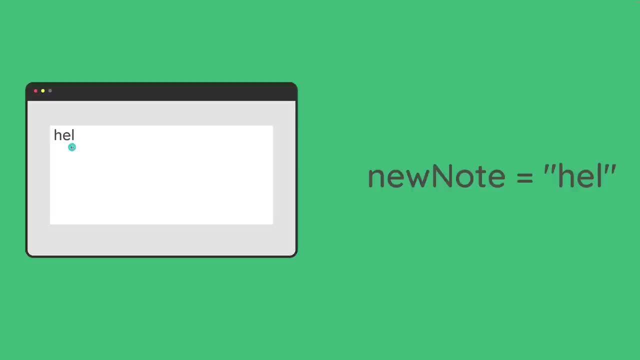 And by the way, I'm trying to spell hello, but I guess in the process it's going to spell hell. So apologies for that. So this is what we need to do. 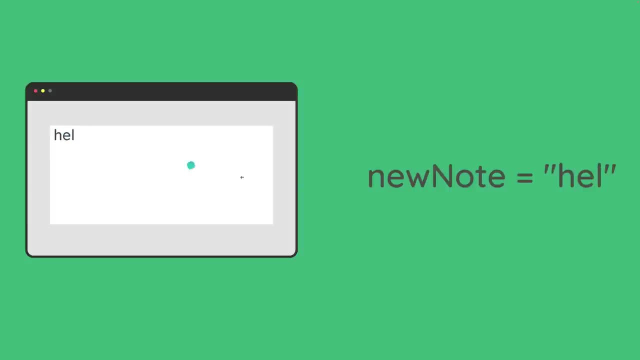 So anytime we update our text area over here, it should update our state. 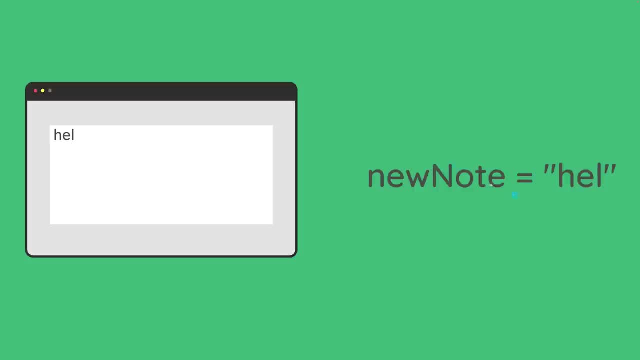 But in a good Vue application, if we update our state, it should also update the text area. 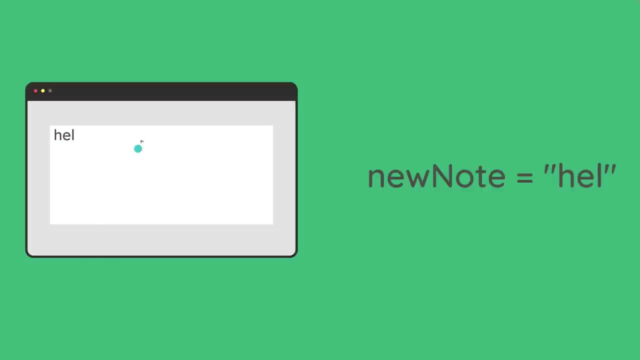 So before we were talking about if I update a text area, or to update the input, 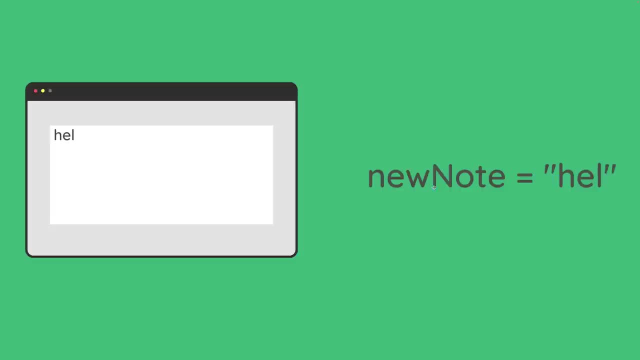 it should update the state, but in a good Vue application, and you'll see why in a second, in a good Vue application, if I update the state, so let's say I add a L here. 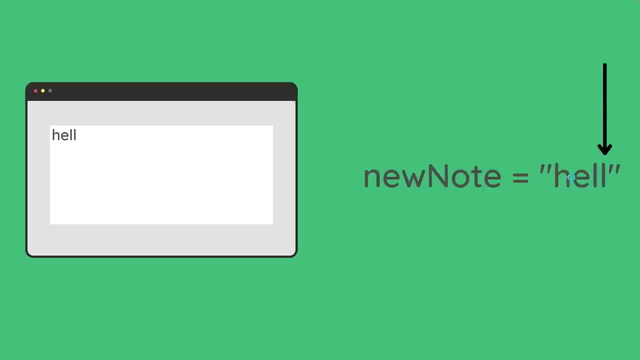 So I update my state. As you can see, the arrow is updating the state and it's adding an extra L in here. 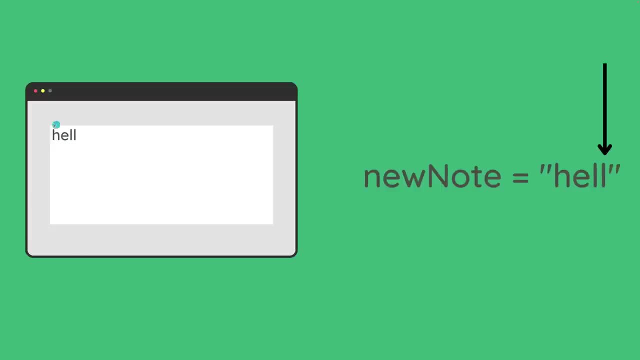 This should also update the text area. So these two should be kind of, well, exactly the same, no matter what. 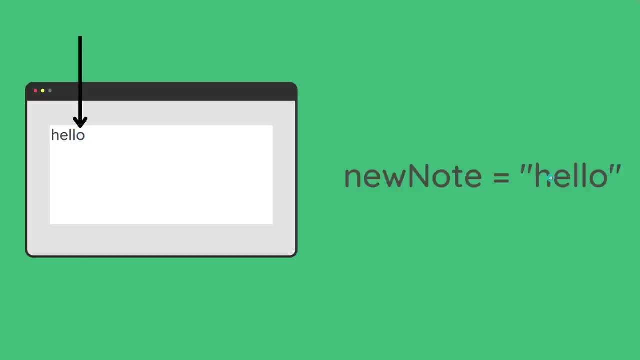 Now if I go back here and let's say I add an O, of course this should update the state so that there's an O. 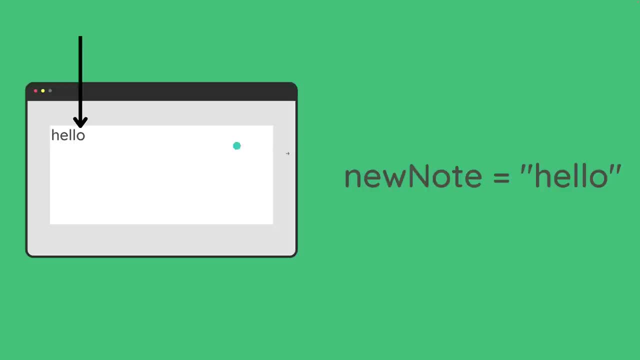 So no matter where the change is, these two things need to be synced up. 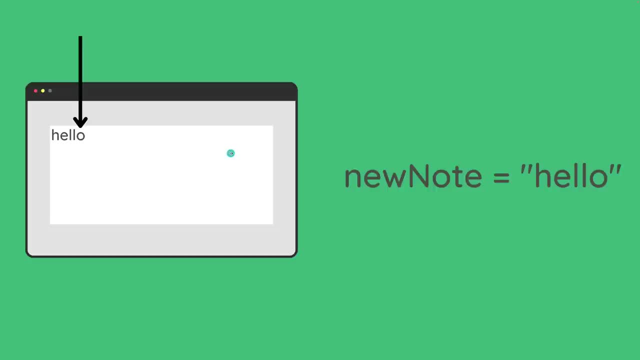 And this is actually a really good thing because let's say what we want to do eventually is maybe clear this text area. 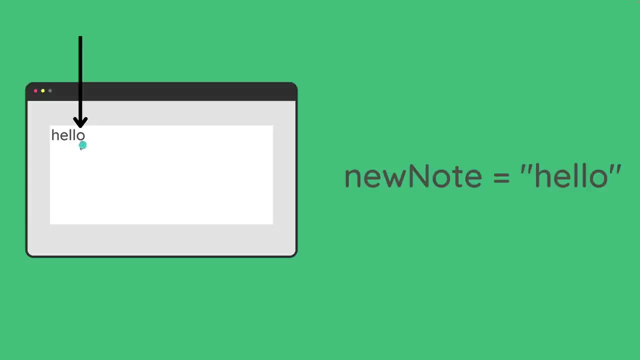 There's a bunch of input in there and we want to clear it. Well, we can't really go into the text area and then do a .innerHTML is equal to an empty string or value equal to an empty string. 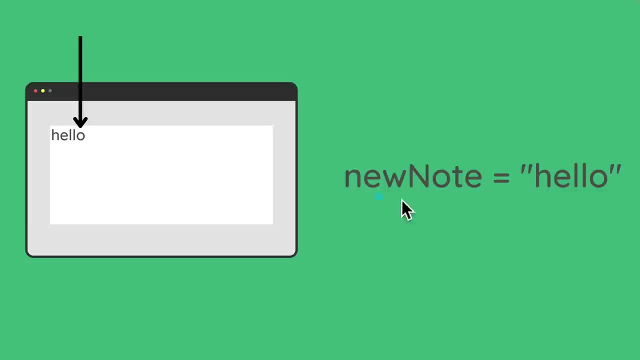 We can't really do that with Vue. So instead what we actually do is we just take this piece of state and we just set it to an empty string. And as soon as we set it to an empty string, 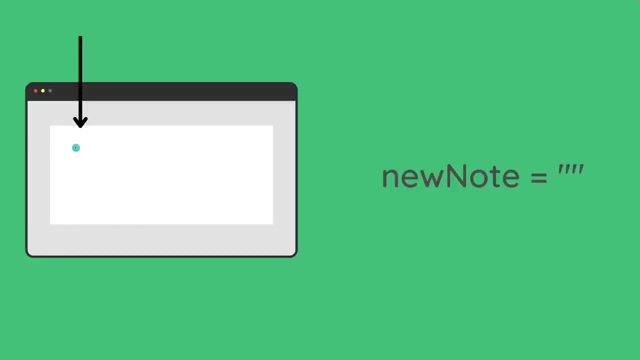 you can see here that our text area is now empty. So I hope that kind of makes sense. 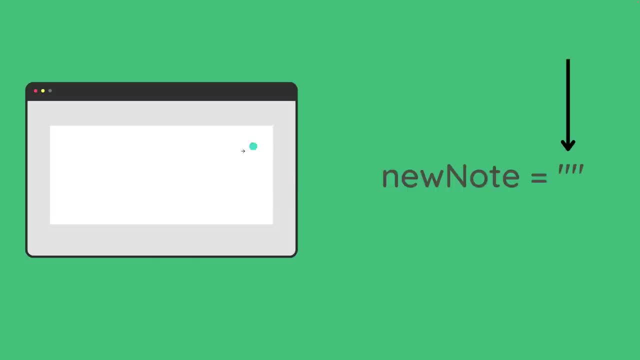 So no matter where we are, we want to have this kind of binding. And this right over here where the value is always going to be equal to the state and the state is always going to be equal to the value and if any one of these changes is going to change the other, this is actually known as two-way binding. 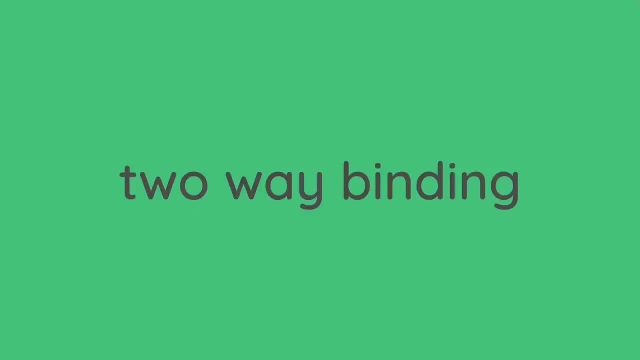 And it is really, really important to implement inside of a Vue application. 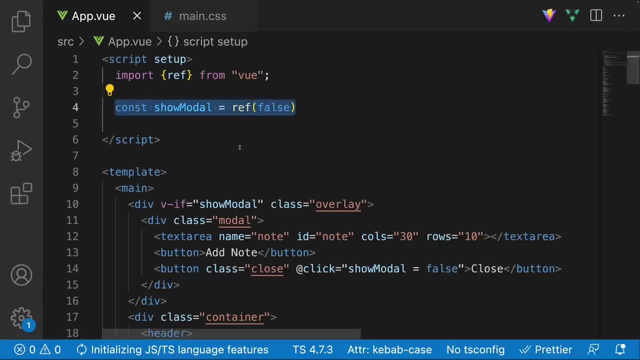 So let's actually just go ahead and implement it. So let's go over here. 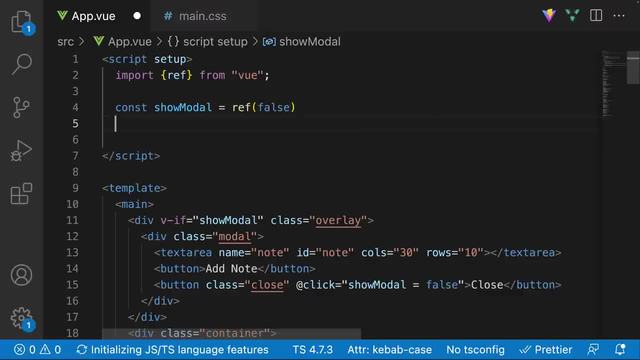 So the first thing I'm going to do is I'm going to define my state. So I'm going to say const. I'm going to call this. I'm going to say new note. And initially, I'm going to give this a value of an empty string. 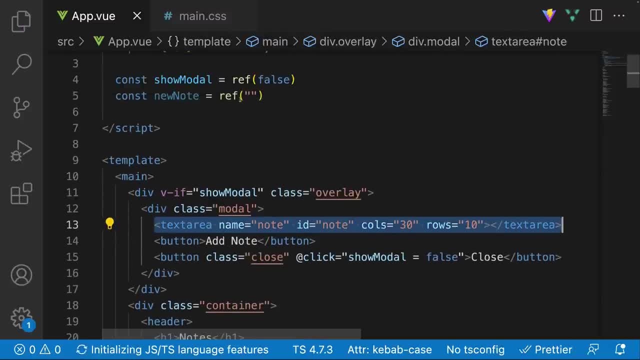 Now, this is the text area where I want to perform this two-way binding with. 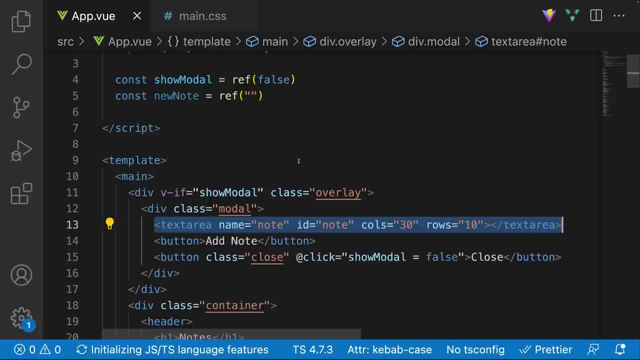 And luckily, this is actually very, very easy because, well, we have directives for this. So there is a V model directive. And this is going to be equal to just some sort of state where we want to perform this two-way binding. And well, in this case, the state is new note. And that's really all it is that we have to do. 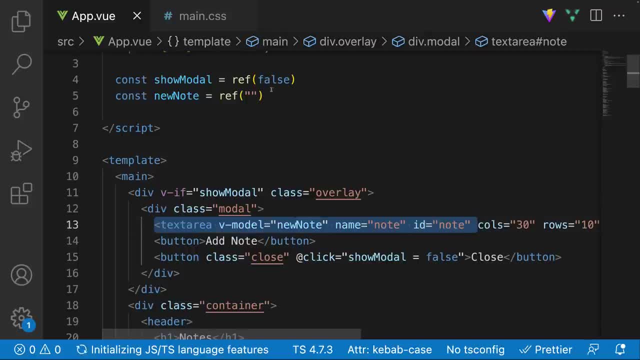 So now, any time we make a change here, it is going to change the new note state. 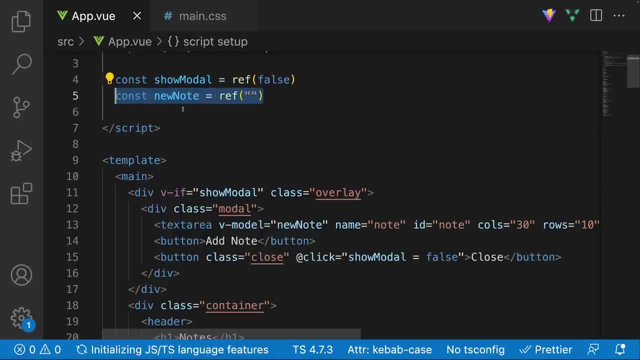 And any time we make a change to our new note, well, it is going to change the text area. 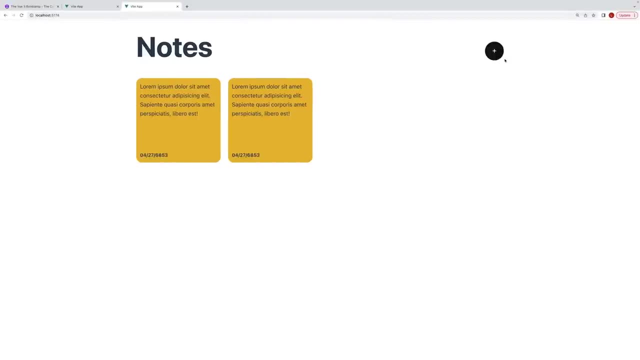 So let me go ahead and just prove this to you. So let's go over here. So we have our text area. 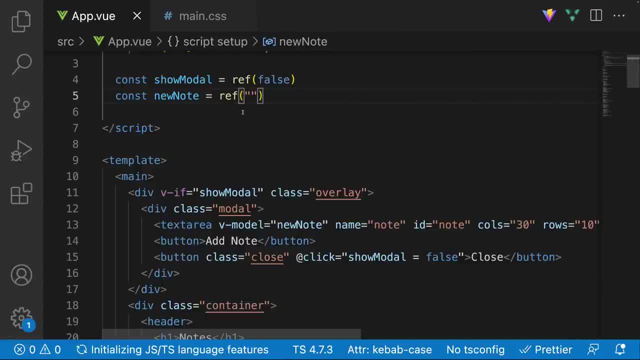 And I'm going to go ahead and just change my state to say something like hello world. 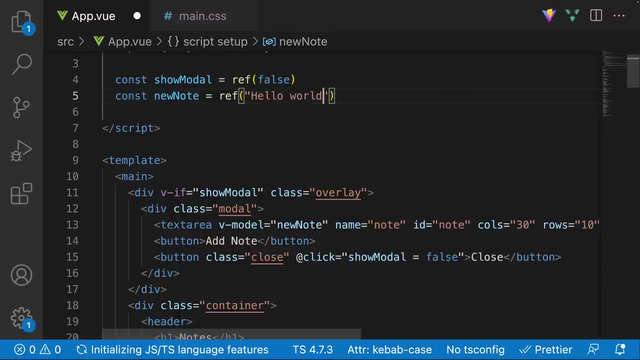 Hello world, that's it. I'm going to go ahead and save this. 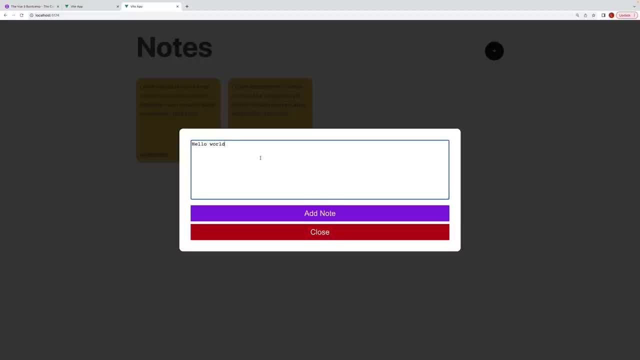 And right away, if I were to click on my modal again, I'm going to zoom in here, you can see it right away starts off with a text of hello world. That's the value that it has. 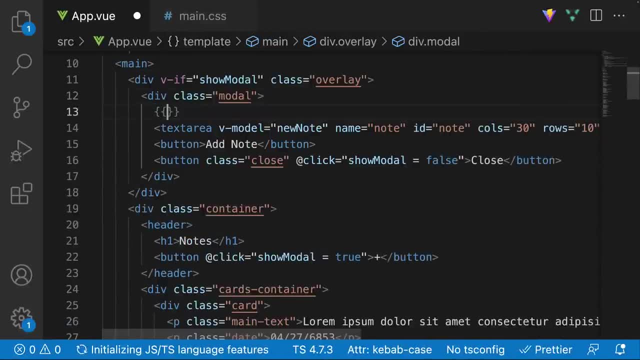 Now, let me actually go all the way to this modal. And I'm going to render the new note input. So the new note input. 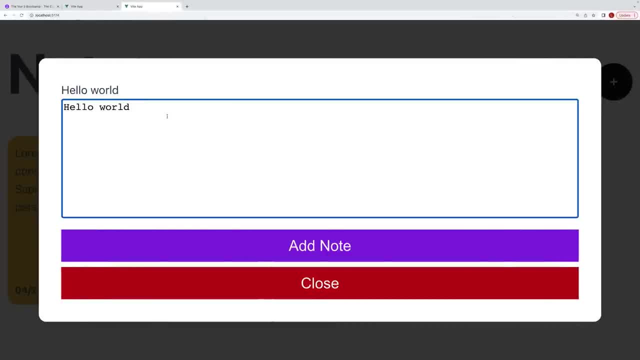 And as you can imagine, this is also hello world. Now, I'm going to start making updates. 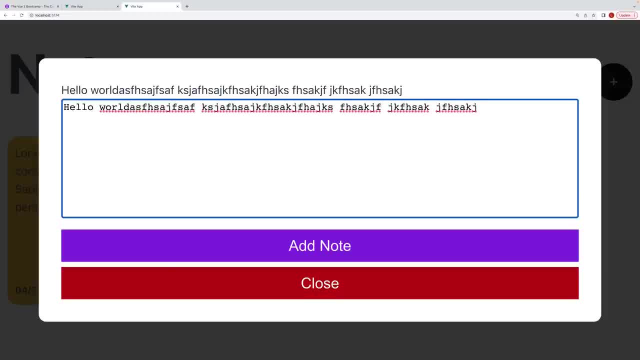 And you can see that this is going to update my new world state. All right. 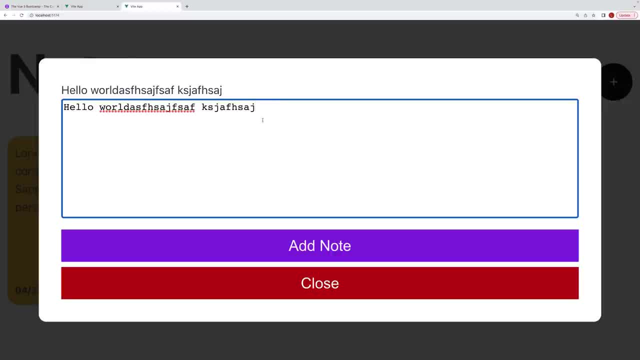 So this is looking really, really good. So that is pretty much all it is that we need to do. 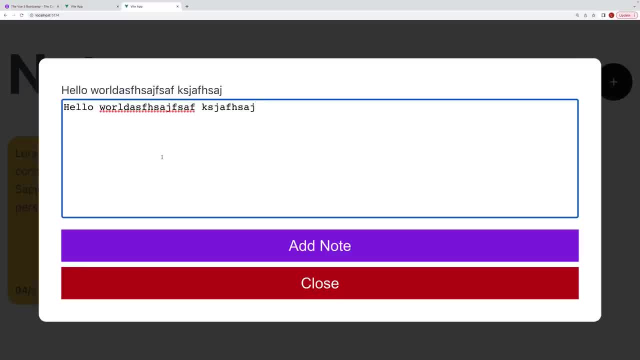 And trust me, later on, we're going to see the powers of this two-way binding in future lectures. 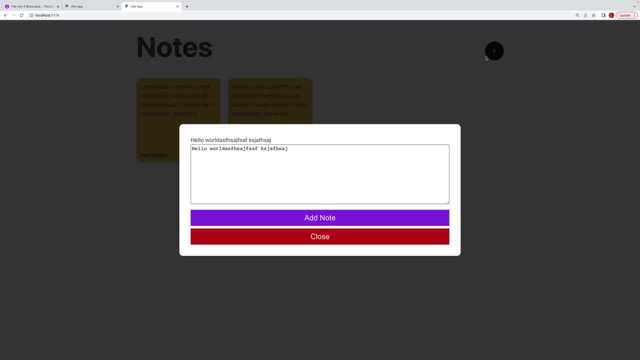 So we set up everything that we need with the click right over here that shows our modal, as well as the two-way binding within the text area. 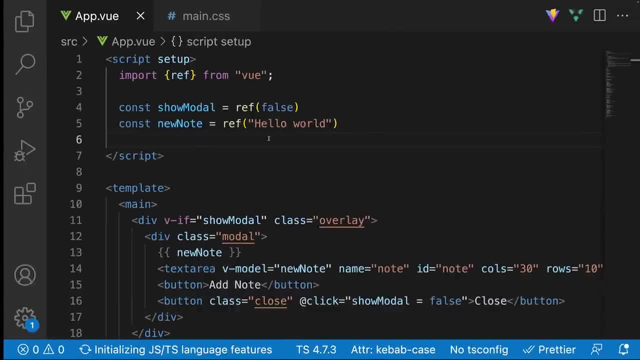 And speaking of the text area, let's just quickly clean up what we have here. 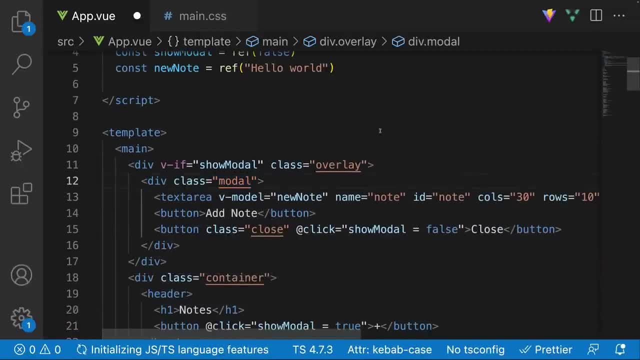 Let's go over here. Let's just remove the new note. 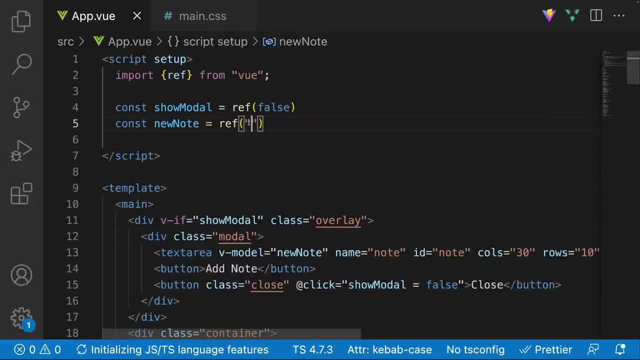 And similarly for the state, what I'm going to do is I'm going to remove the state right here. Looking great. Okay. 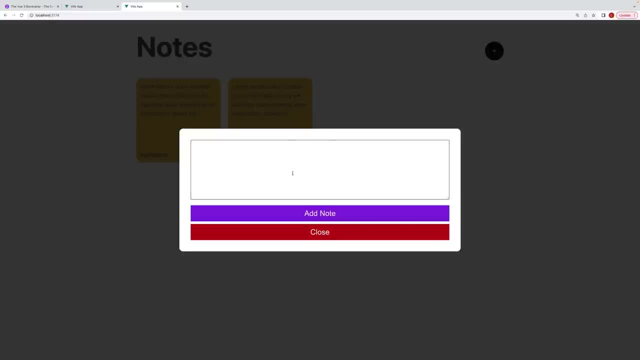 So now if I were to do a little refresh, everything is working fine. 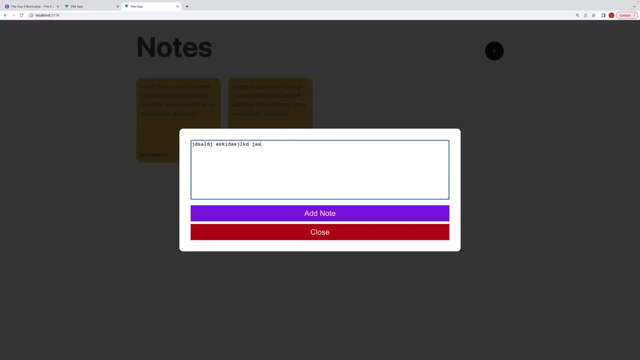 But the next step is for the user to, well, type something. And then, they're going to want to add the note, which is going to add the note to this card right over here. 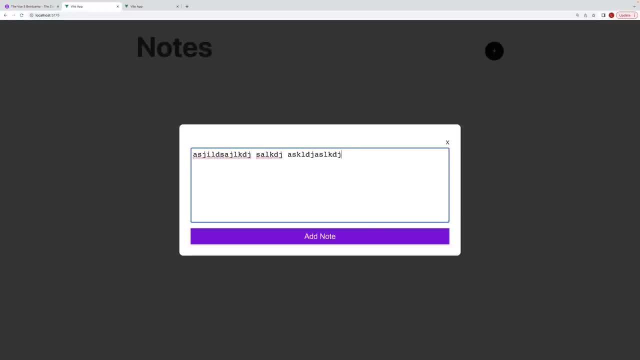 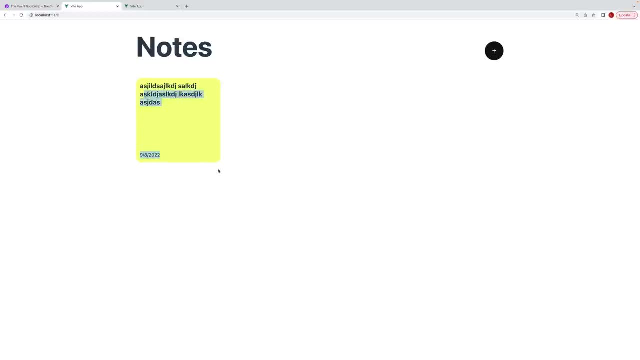 So let's just go to the complete version. They're going to create some sort of note. And that is going to close the modal. And it is going to add a new card. 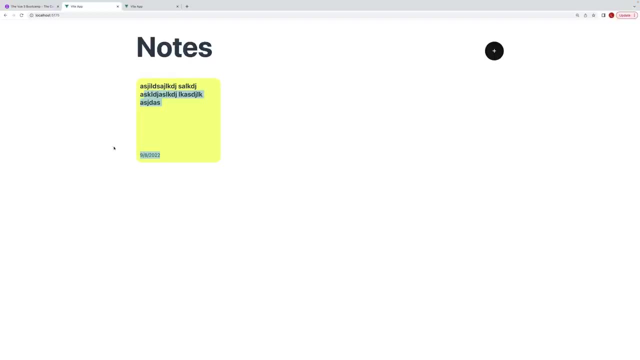 Now I think at this point, you probably understand that this right here, the rendering of cards, is going to be stored in some sort of state. 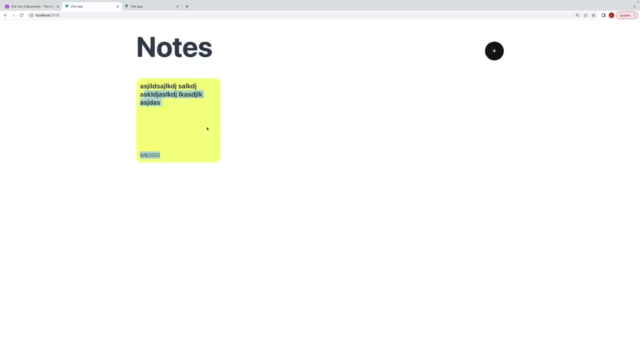 Because of course this is a state that our application is currently in. Currently it is in a state where we have one card. 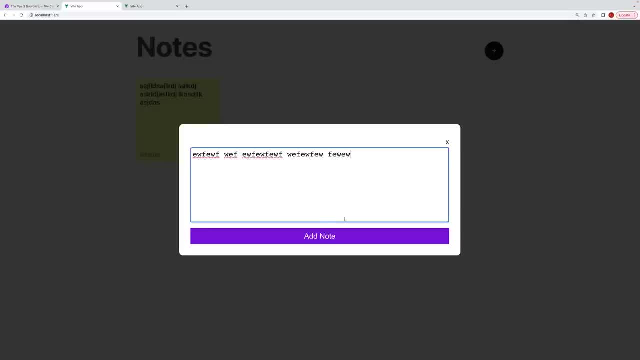 If I were to add another thing, our application is in a state where it has two cards. 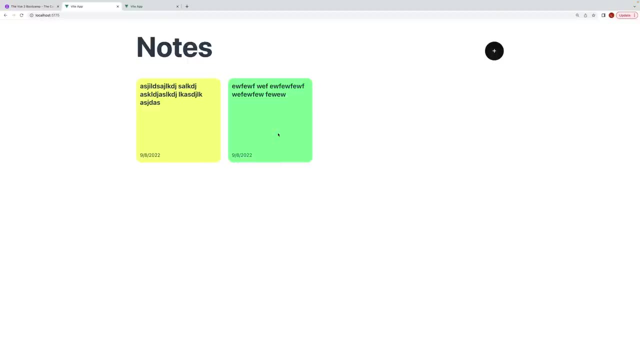 So the cards are going to be stored in some state. Now because we have multiple different cards that we can have, well, we're actually going to store the state inside, or we're going to store the state as an array. Specifically an array of objects. 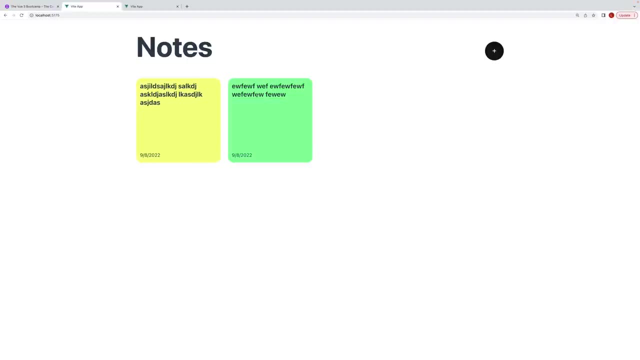 Because each note can have multiple different properties. For example, it has the text itself. It also has the date. And it also has a background color. 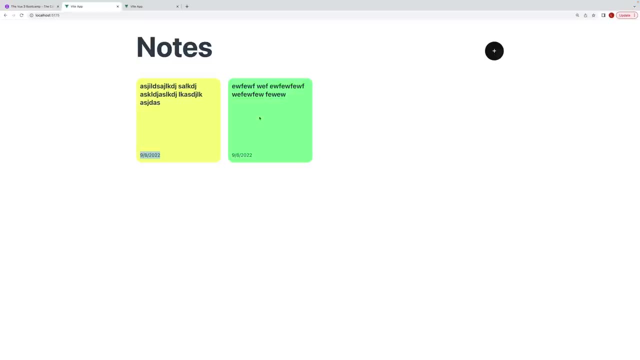 And it probably should have some sort of unique auto-generated ID. Okay, so now that we got that out of the way, let's actually go ahead and create that state variable. 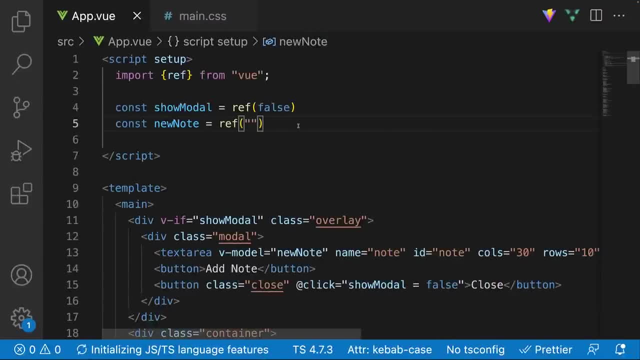 So I'm going to go over here. And I am going to create const. 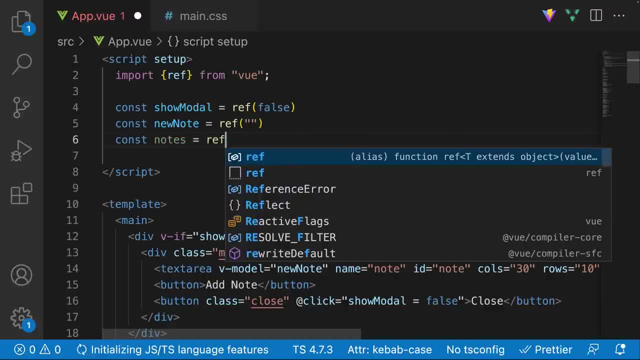 And I'm very simply just going to call this notes. And it's going to be equal to ref. 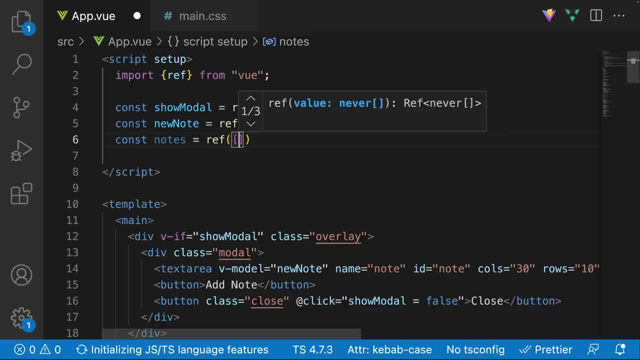 And it is going to be equal to, for now, an empty array. So this is what we are going to have. 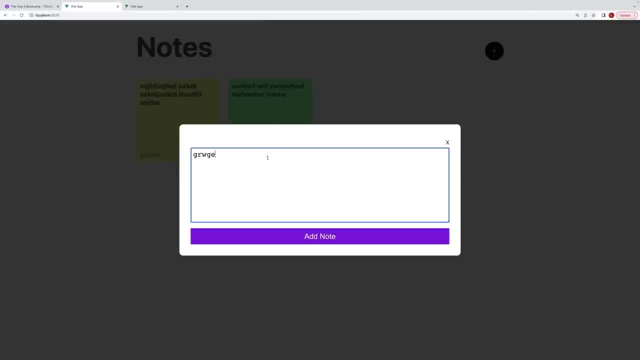 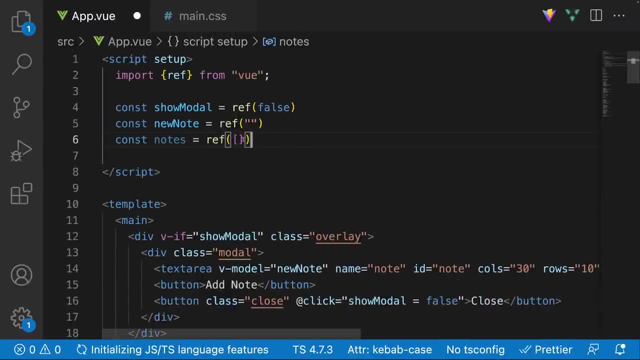 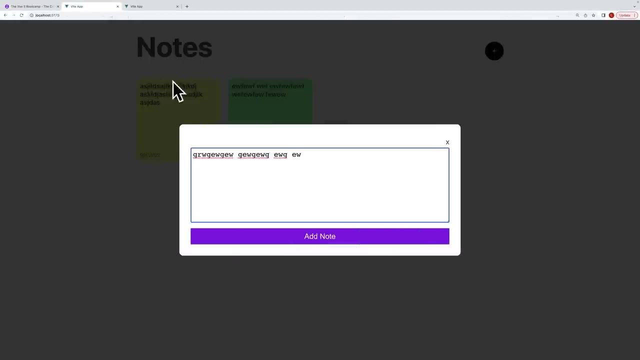 Now what we're going to want to do, as soon as we will type something, is push a new object onto this state array right over here. And that way we're going to have a new note, that eventually we're going to render onto our screen. 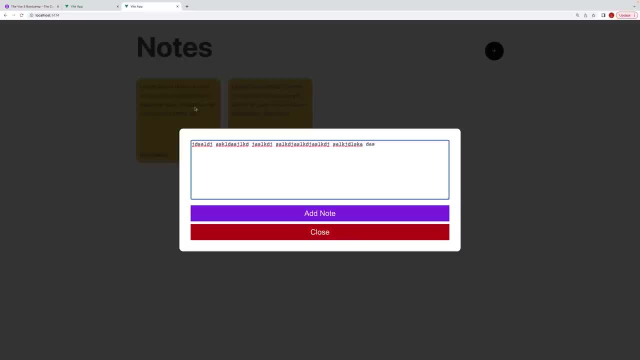 So let's actually go ahead and, well, accomplish that. So let's go over here. 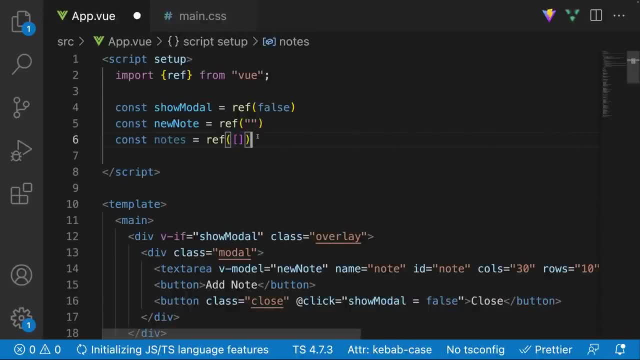 And let's add a handler for our click event. 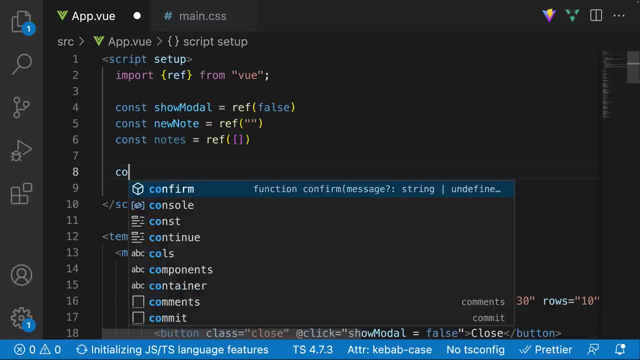 So what I'm going to do is, and if you hear my cat, apologies, or not apologies, the sound of cats are really beautiful. 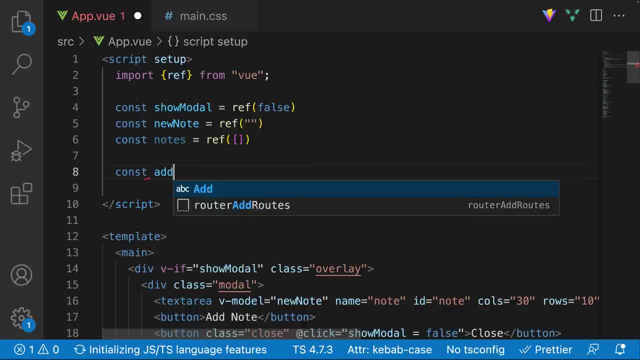 So let's go over here and let's create a handler called add note. That's what we're going to create. It's going to be a callback function. 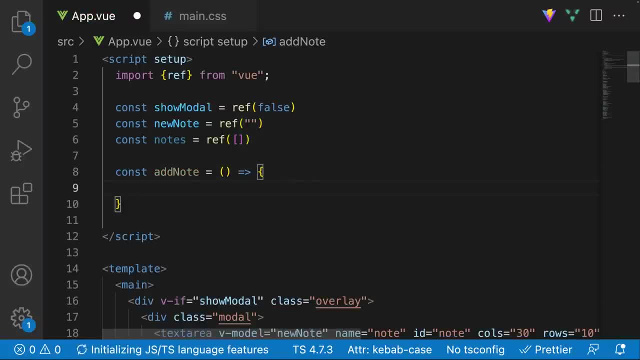 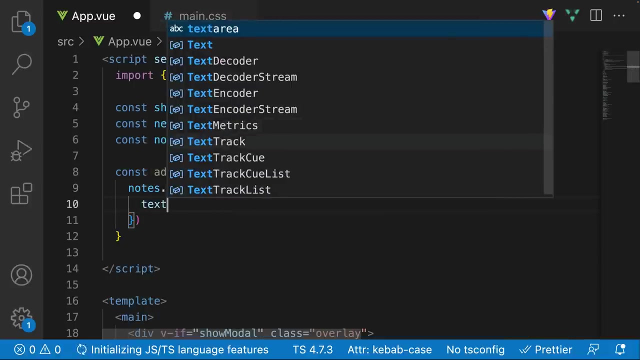 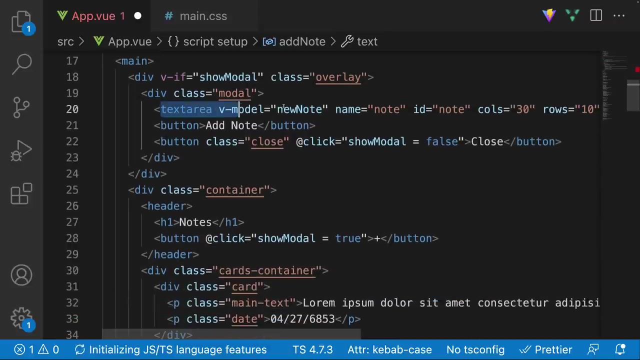 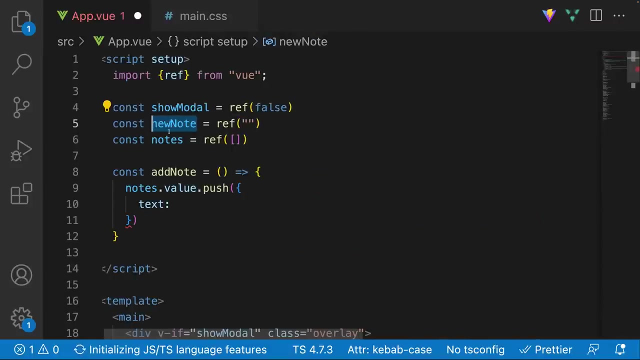 And very simply we're going to have kind of a naive implementation at first. We're just going to very simply just say notes.value.push. And we're going to push in a new object. Now let's remember the properties that it's going to have is the text. Now where is this text going to come from? Well, it's going to be the value of the text area. So it's going to be the value of this text area. Now luckily we have two-way blocks. And we're binding so we can actually access that value with this piece of state right over here. 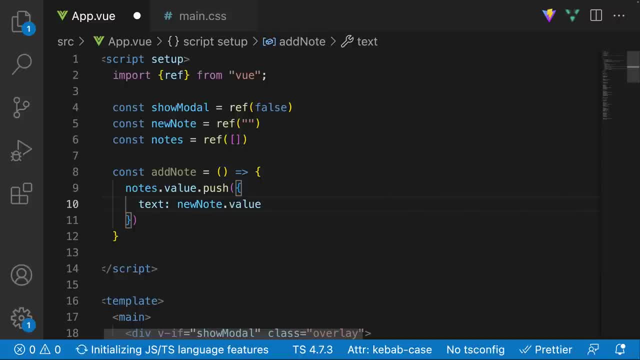 So I can say something like new note.value. Very, very simple. 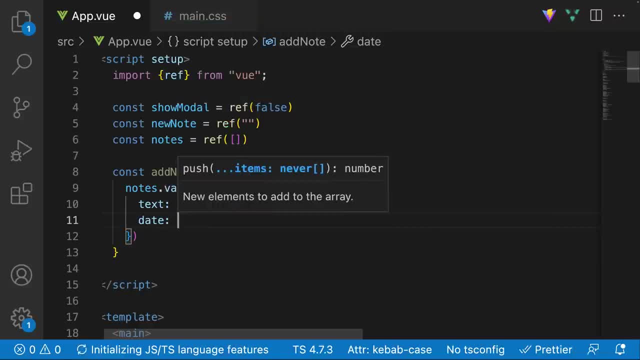 Now it's also going to have a date. Now this date is just going to be the current date at the creation of this note. So let's just say new date like so. 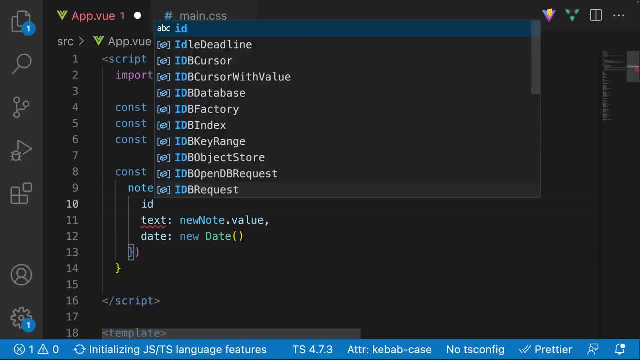 And it's also going to have some other properties. So for example, it's also going to have an id, which it should be just a random unique integer. 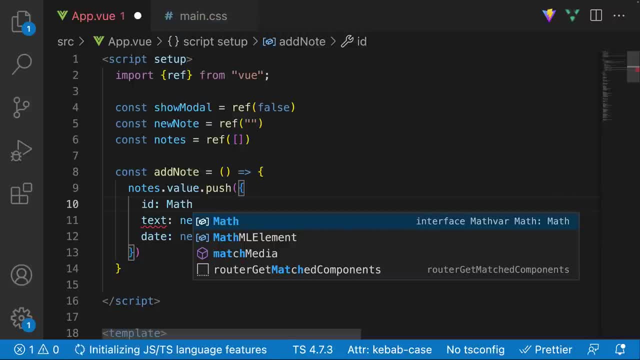 And to actually generate a random unique integer, we can just use some JavaScript for this. We can say math.floor. 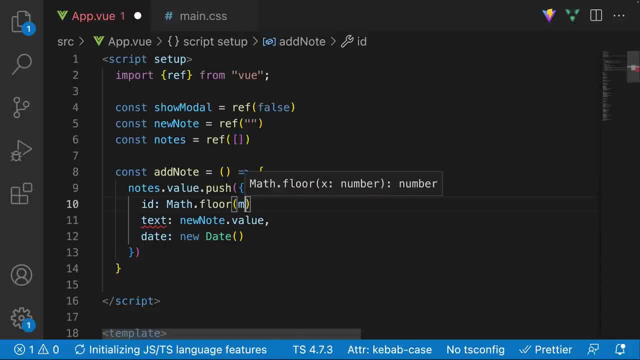 And then we're going to say math.random. So math.floor, math.random. 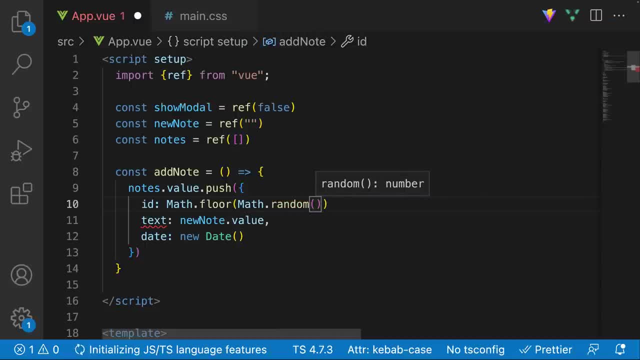 And we're going to invoke math.random. And we're going to multiply it by let's say a million or something like this. 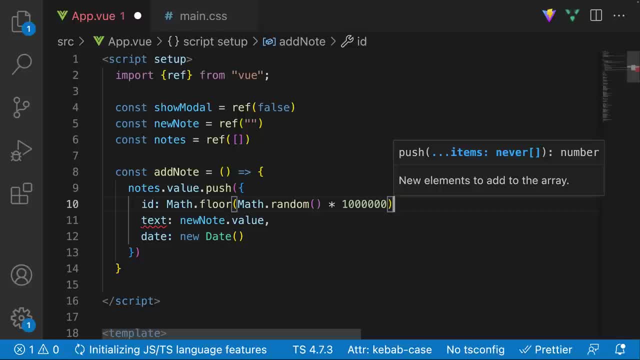 Yeah, this is a million. And so what this is going to do is it is going to just generate a random number between zero and a million, something like that. 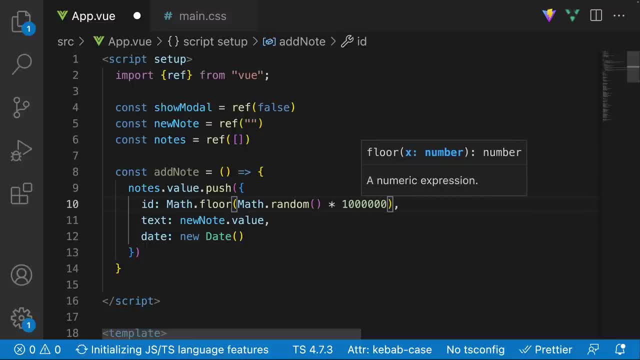 So technically, we could have potentially an id that is the same, but the odds are like one in, I don't know, half a million or something like that. All right. 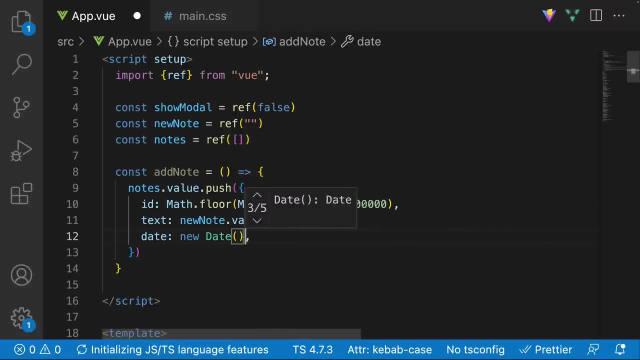 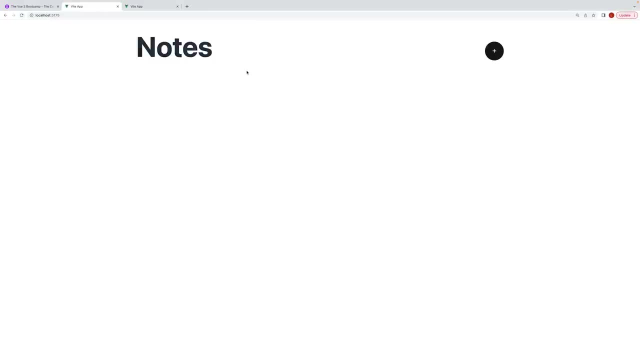 So let's go ahead here and let's add one more thing, which is going to be the color. So this is going to be the background color of the card because remember, it is indeed, random. So you can see here, it's just kind of a random color. 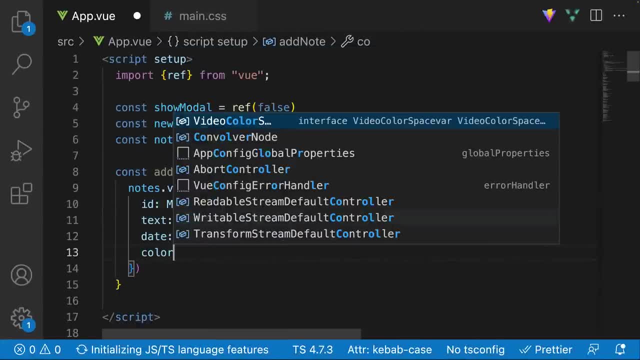 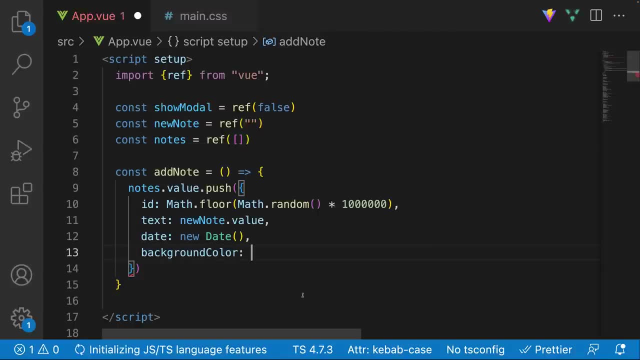 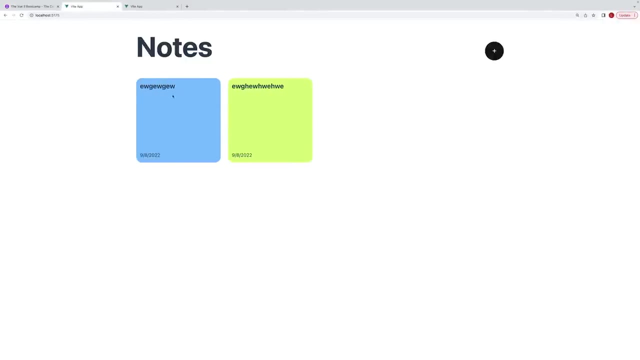 So let's go ahead over here and let's just say color. And we're going to even call this background color. Background color. And over here, we're going to have to randomly generate a color. Now, this color also should be relatively light. So as you can see here, it's a light color. I don't want to have a dark color because then our text is black and we do not want to have a dark color because then at that point, we're not going to be able to read our text. 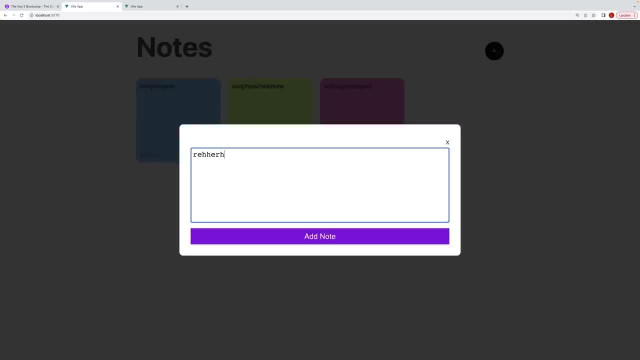 So if you actually notice here, every single time I actually generated a color, it's kind of a relatively light color. 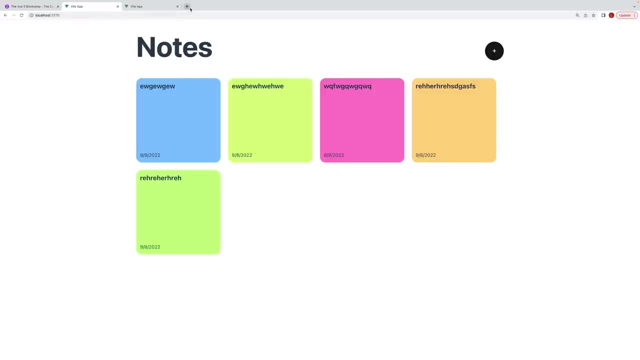 And honestly, I did this by kind of just copying code from Stack Overflow. So I went to Google and I said, JavaScript generate random light color. 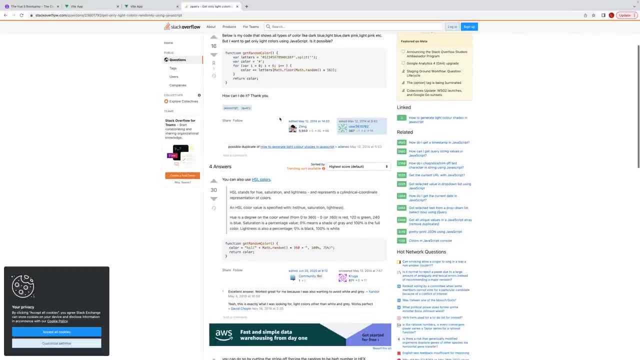 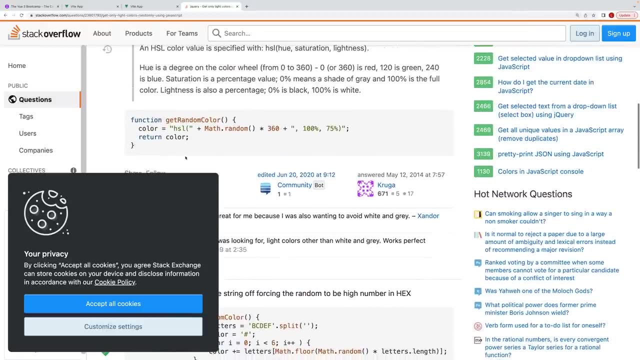 And then I went over here to Stack Overflow. And right here, I utilized this function right over here. Or sorry, this one right over here. 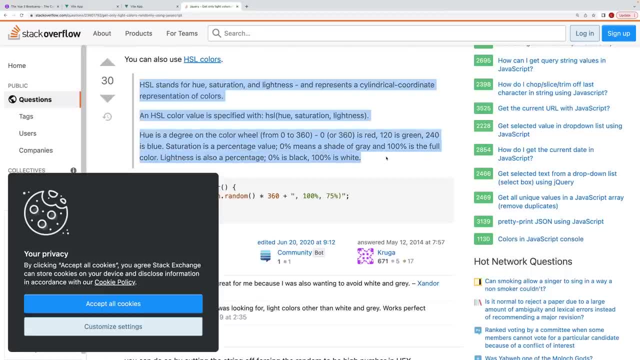 Honestly, there's an explanation for this if you're really interested. But this is just kind of a CSS thing that I don't really understand. 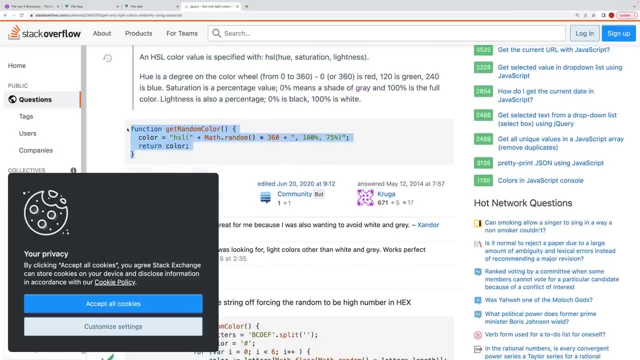 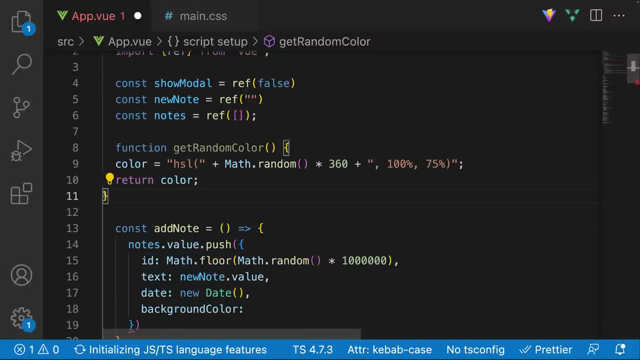 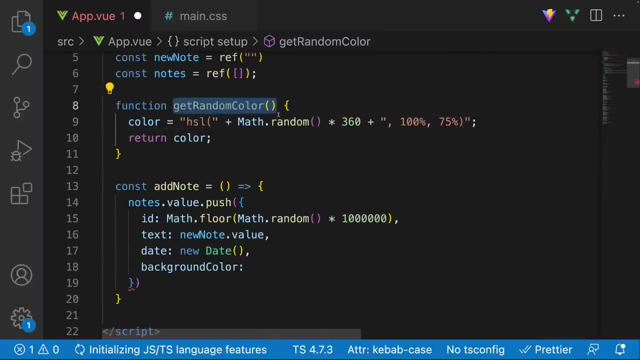 But I just know that the function works. So what I can do is I can just very simply copy this. And let's just go over here. And let's just paste it in there. So we're going to paste in the color. And then we're just going to invoke this get random color every single time we create a new note. 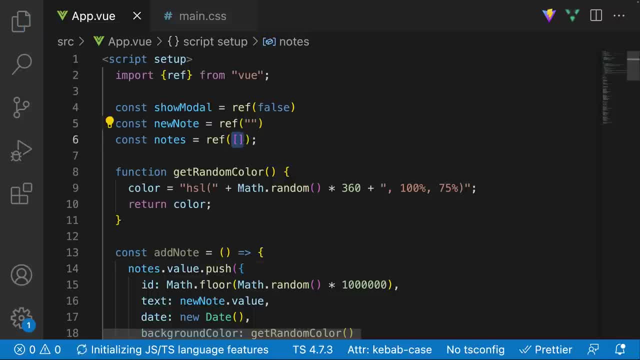 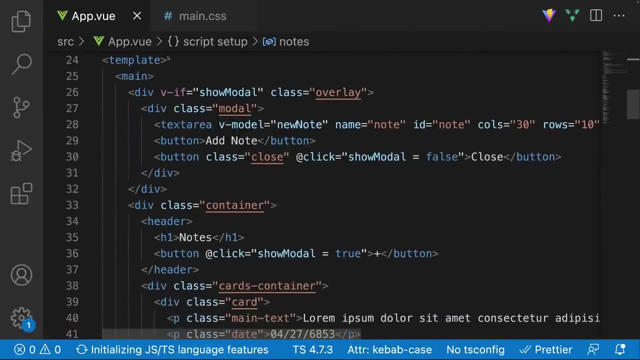 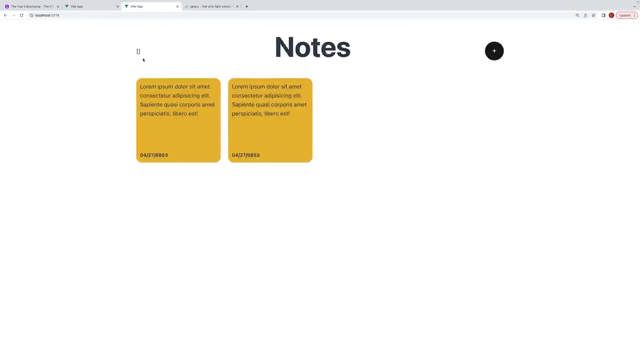 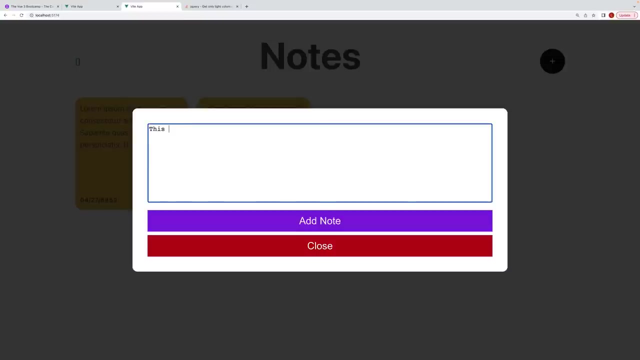 And that's very simply what we're going to do. We're going to push it onto this array. So let's go over here. And just so we can actually see the array being rendered, I'm going to go right here onto this header. And I'm just going to say notes like so. So as you can see, I'm going to zoom in here. As you can see, initially, it is empty. And then I'm going to go ahead and I'm going to add this is my very first note. 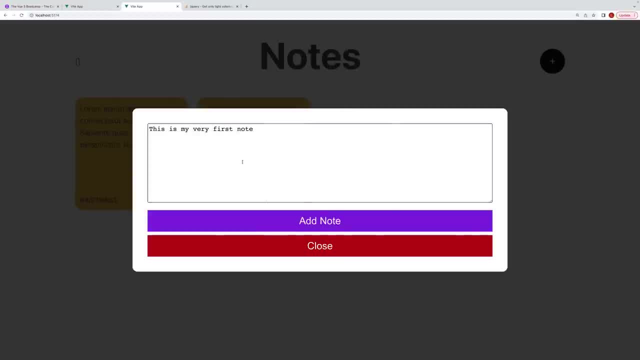 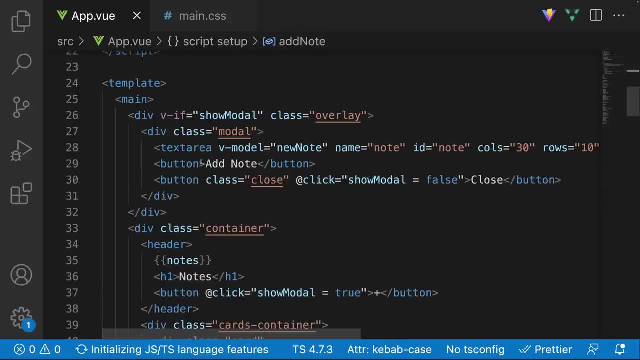 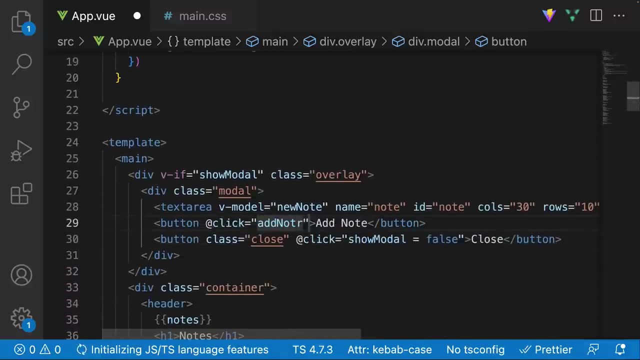 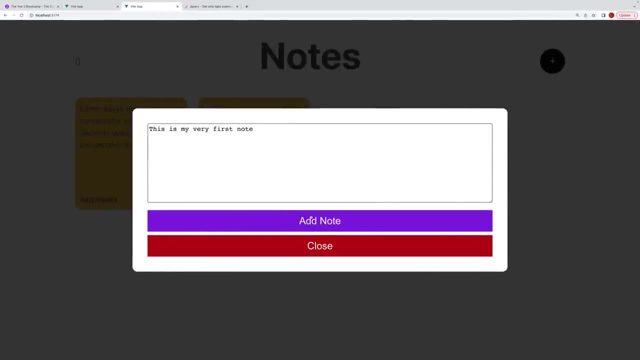 And I'm going to go ahead and add it. And as soon as I add the note, of course, nothing is going to happen. That's because we're not using this handler at all. So let's go over here and let's just say at click. And we are going to say add note. That's the function that we want to call whenever we have a click event. So I'm going to go ahead and click on this again. And nothing is happening again. Let's go ahead and inspect just to see what's going on. 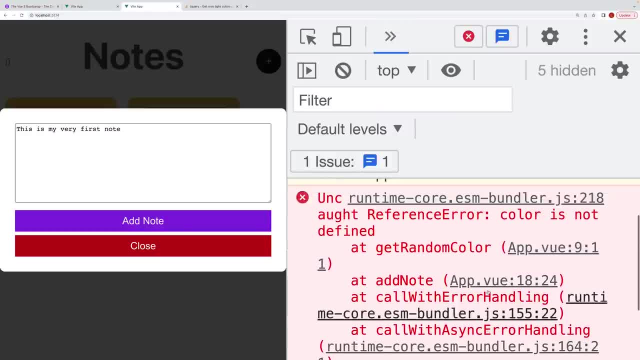 Let's go to our console. So we have some error here saying color is not defined. Okay, no problem. 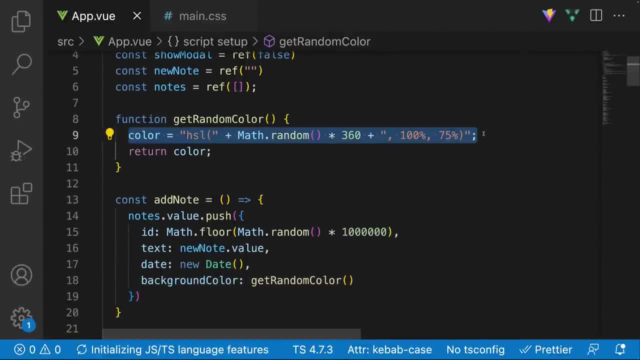 Okay, for some reason, this person treated this like JavaScript or rather than Python. So what we can do here actually is just very simply return like this. Like this. We don't even need to have that variable. 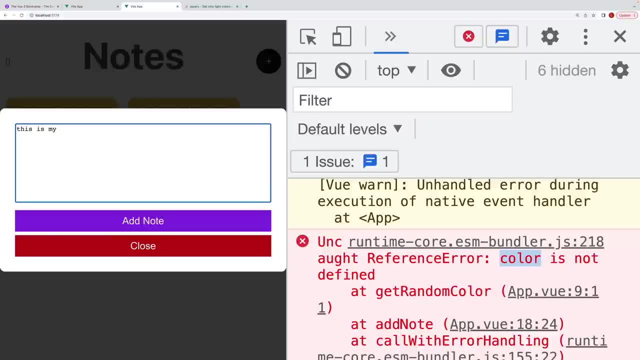 So I'm going to go ahead and say this is my first note. And if I click on this, you can see right away it actually is going to populate my array within UObjects. 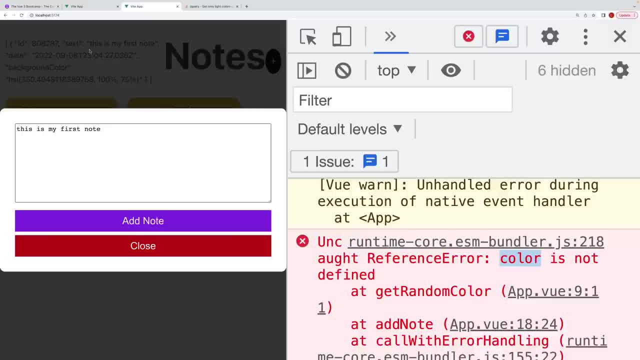 We have this object that has this ID. And then we have this text over here. We got the date. And we also have this random background color. 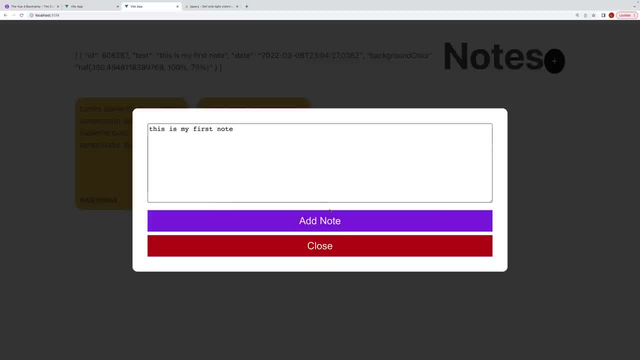 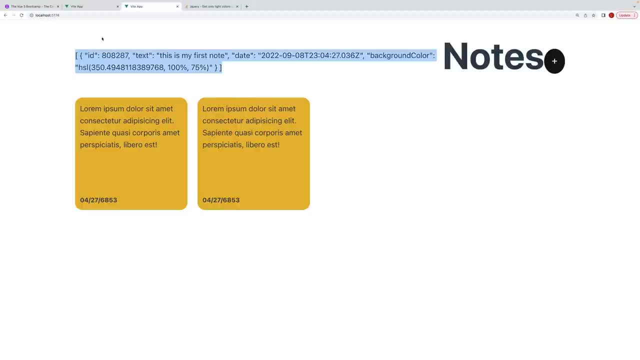 Now one thing that isn't really nice is that as soon as I add a note, I probably want to close this modal. I don't want to have to close it manually. I just want it to automatically close. Kind of like, well, what we did over here. So I add the note. 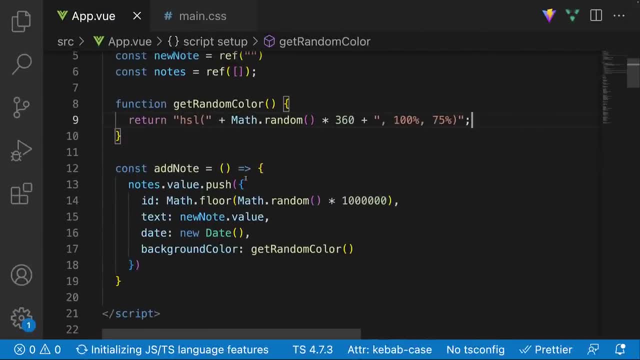 It automatically closes. So we could actually do that relatively easily. 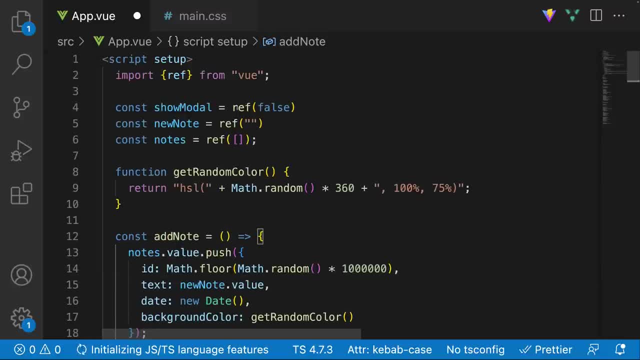 So right after we add the note, we can, well, update the state of the show modal. So let's go over here. 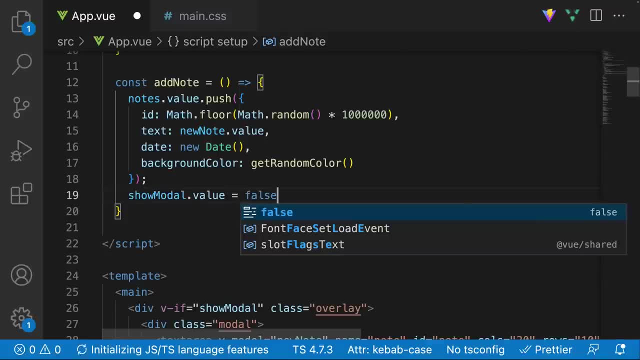 We're going to say show modal.value is going to be equal to. It's going to be equal to false. 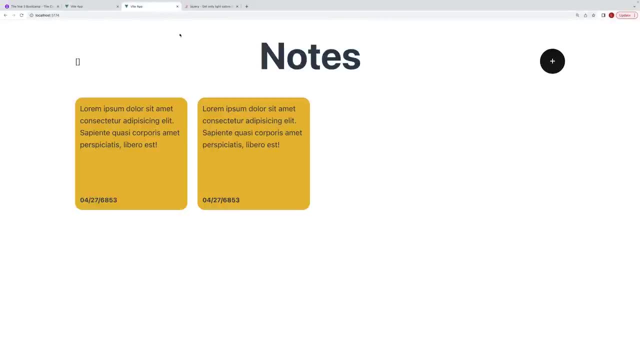 Very simple stuff. So that is going to, as soon as we add a new note, a new note, I'm going to add it. And there we go. 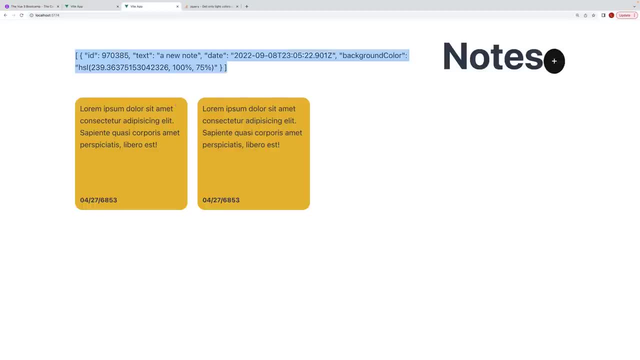 You can see right away it closes it. Now there still is another issue. 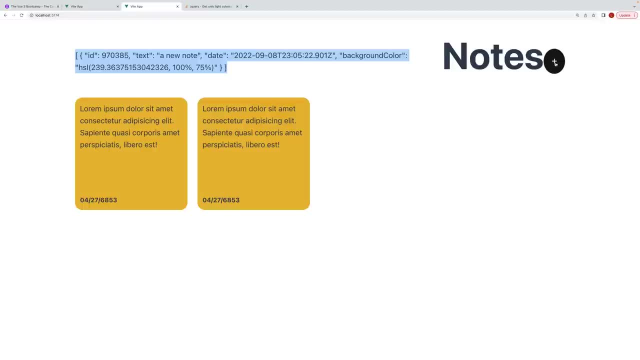 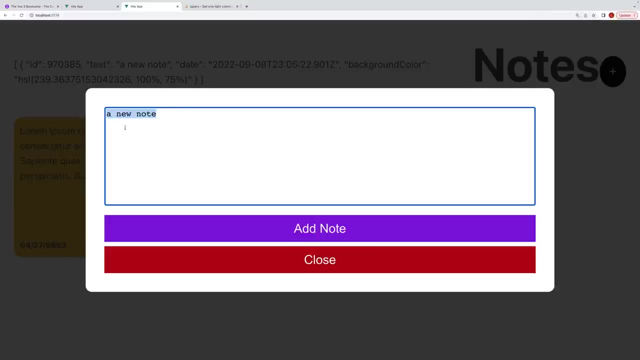 If I want to add another note, I would click on this button. But you can see that my, well, my text area has a value currently. It has a new note value. Now we don't need this anymore. We should probably clear this text area. Well, now we can, because of the two-way binding, we can do that by just very simply setting the state to be an empty string. 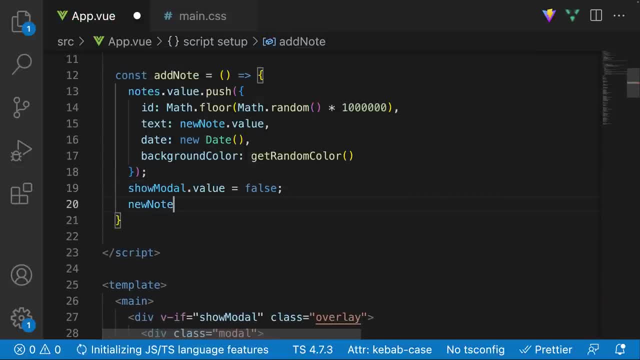 So let's go over here and I'm going to say new notes.value. 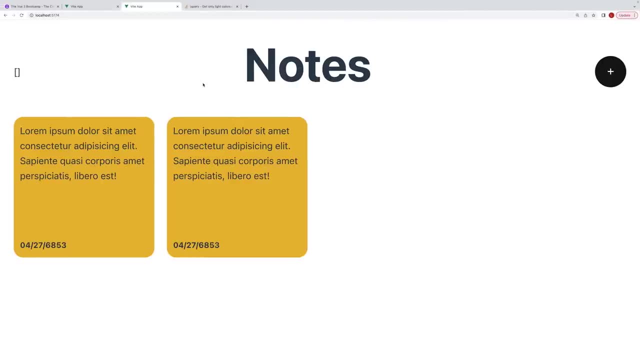 I'm going to set that to be an empty string. So that is pretty much it. 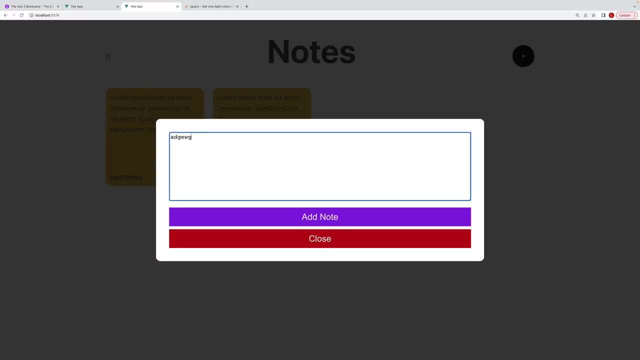 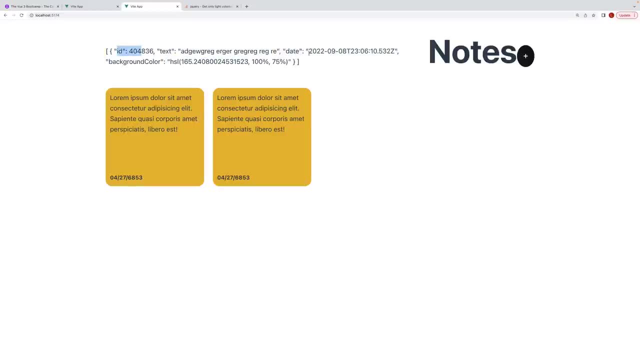 Later on, we're going to do some validation. But now if I add a new note, blah, blah, blah. It adds into the array, gives it a random background color, gives it a random ID, it gives it a date. 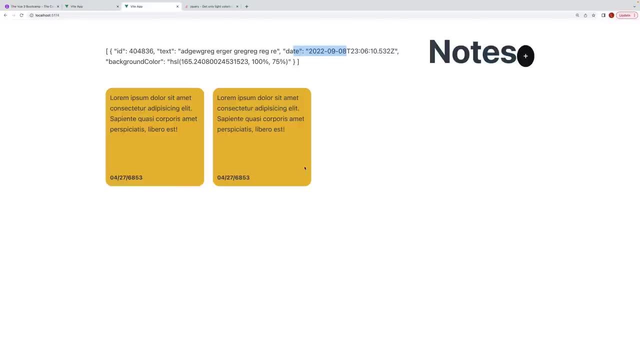 And if I were to click on it again, you can see it is completely empty. Now there are quite a bit of problems to this. For example, a person can just write a note with one letter. That's not good. 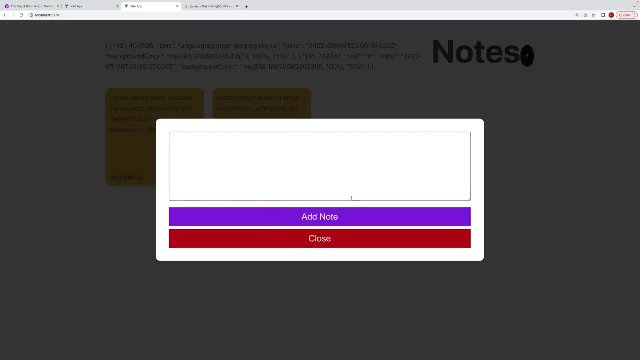 A person can even just go ahead and just add, open this modal, add a note, and that's just going to add an empty note. 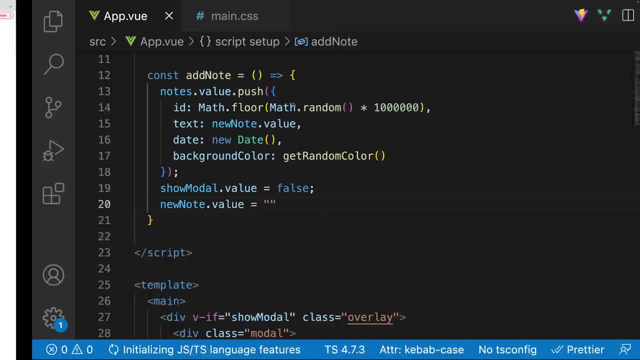 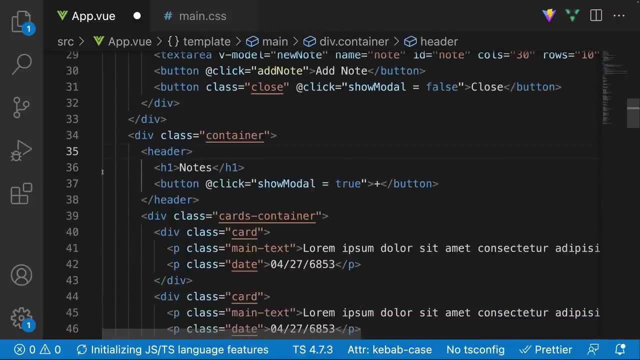 So there are a few problems with this, but we'll fix that a little bit later. But the most important thing is you understand how the handlers work. So let me just remove this over here. Let's go ahead and do a little quick save. And there we go. Everything is a-okay. Now what we want to do is we actually want to get that array. And for each array, we want to render a notes card. So let's actually do that in the next section. 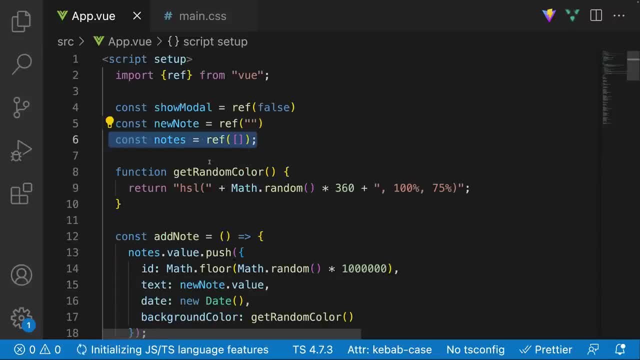 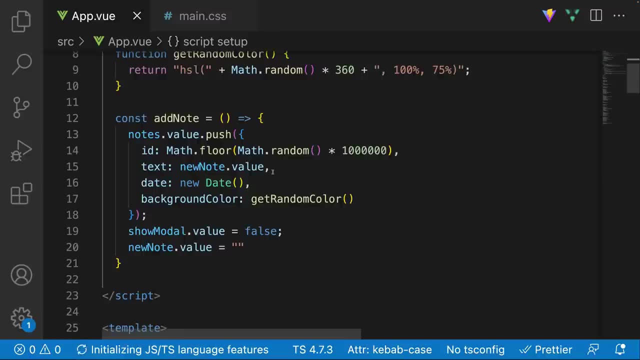 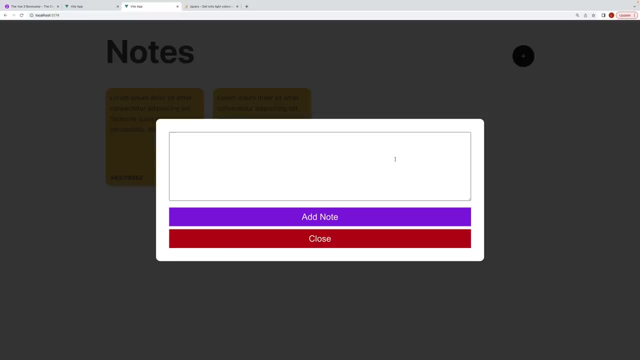 So we created our notes state. And we added the handler that is going to update the state whenever we type something in. And then we click on the add notes button. But of course, no new note cards are being rendered because we haven't added that functionality yet. 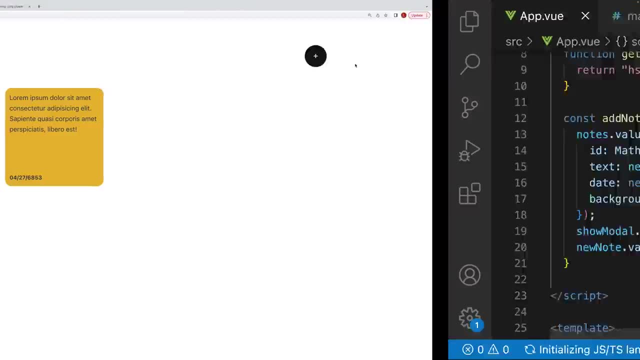 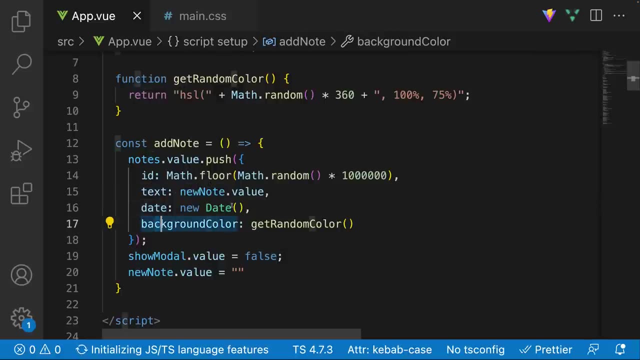 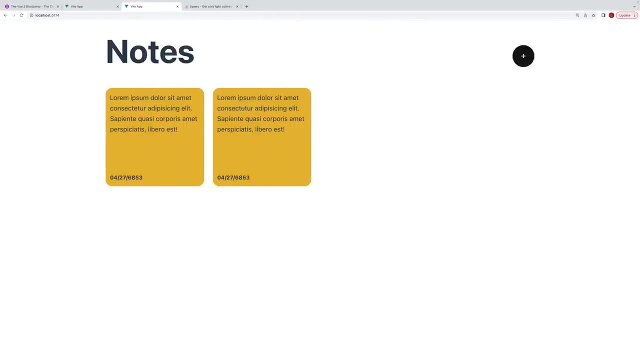 So again, what's going to happen here is it's going to update the array itself by adding a new object within it with an ID, text, date, and a background color. But that array is not being used anywhere. And thus, of course, it is not going to render a brand new card. 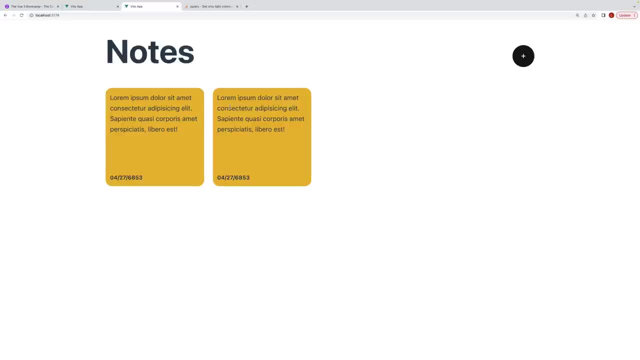 Well, we are going to fix that. We are going to fix that in this video. 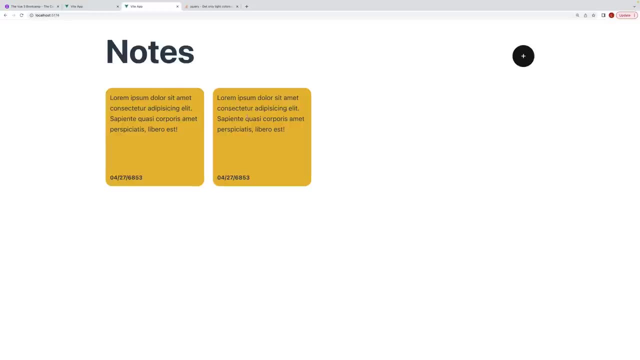 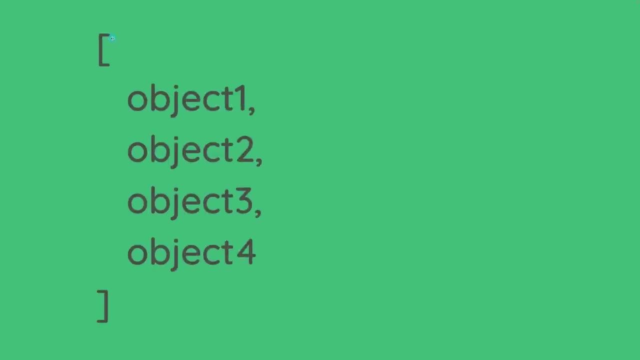 Now for each new object that we add to the array, we want to render a notes card. Let me actually show you a diagram. So let's say that this is our array over here, our notes array. And then within it, we have, let's say, four different objects. And of course, each object is going to be pertaining to a note. So it's going to have an ID, text, background color, as well as a date. So ideally, if we have four objects within our state array, we're going to want to render four different cards, one for each object. 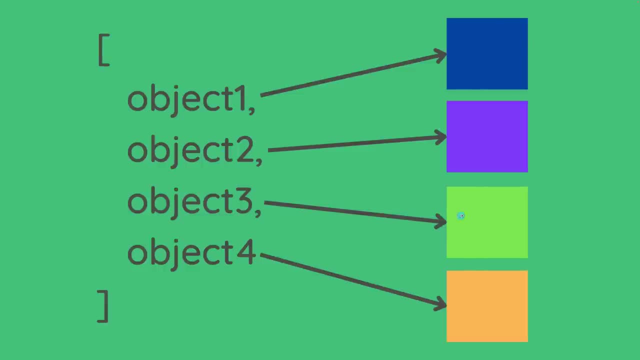 So one note card for this object, one for this one, one for this one, and one for this one. 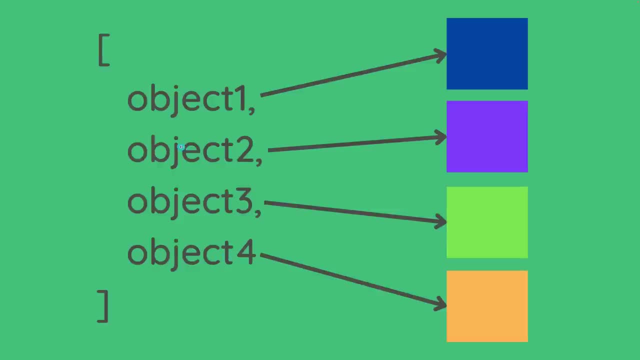 So what are we going to do to accomplish this? Well, this is an array. And thus, what we're going to do to accomplish this is iterate over that array. So we're going to iterate over that array. And thus, what we're going to do is iterate over that array. So we're going to iterate over this array one by one. And thus, what we're going to do is iterate over that array one by one. And thus, what we're going to do is iterate over that array one by one. 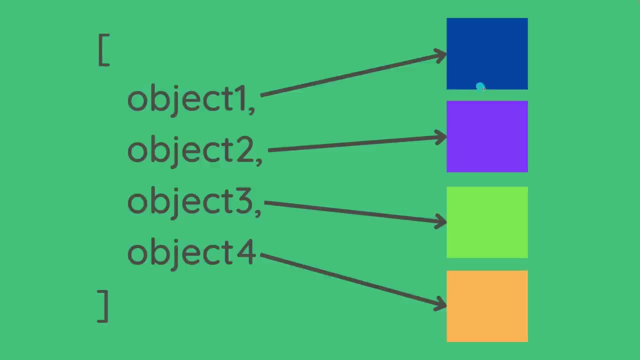 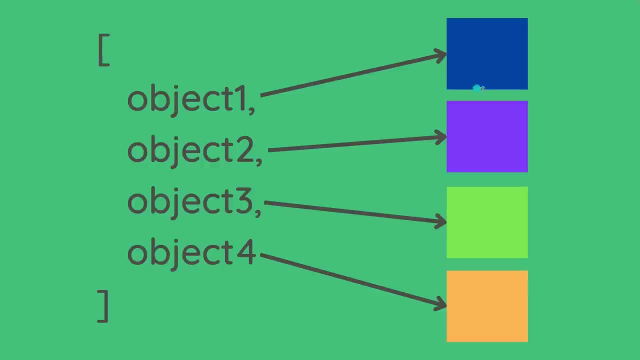 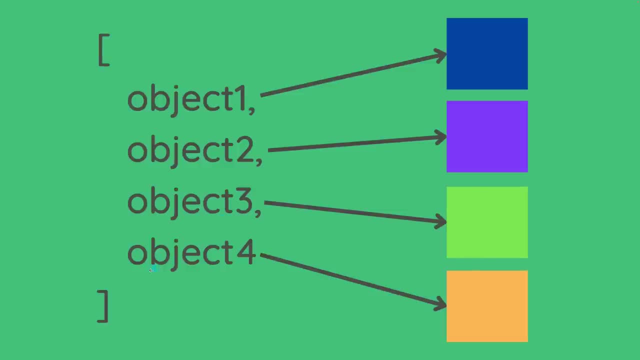 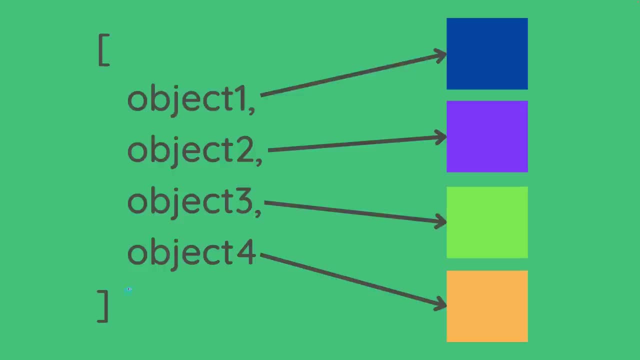 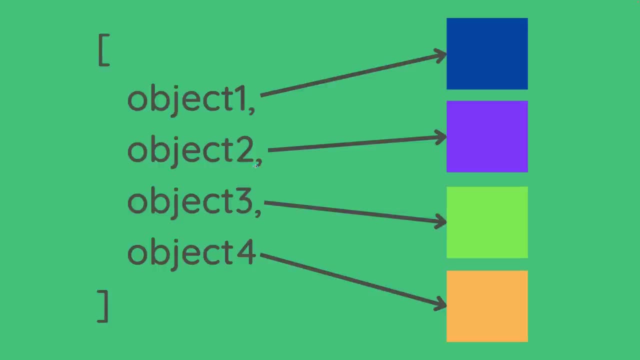 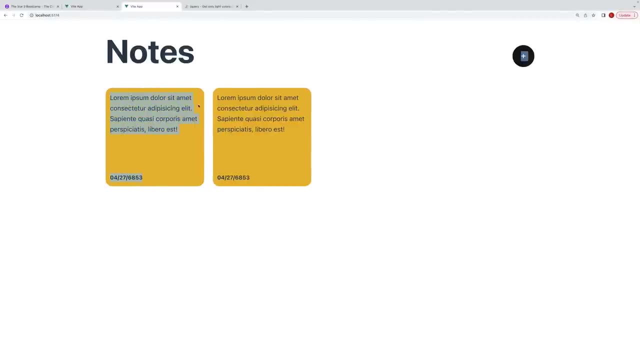 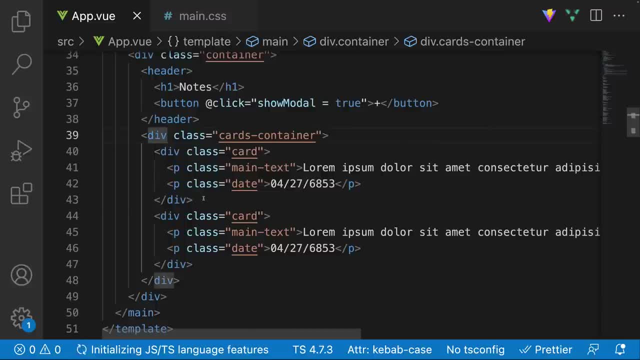 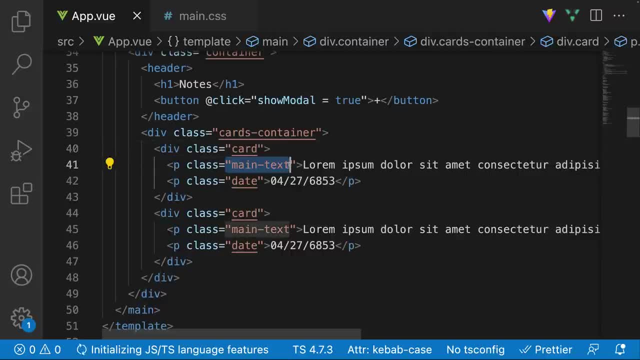 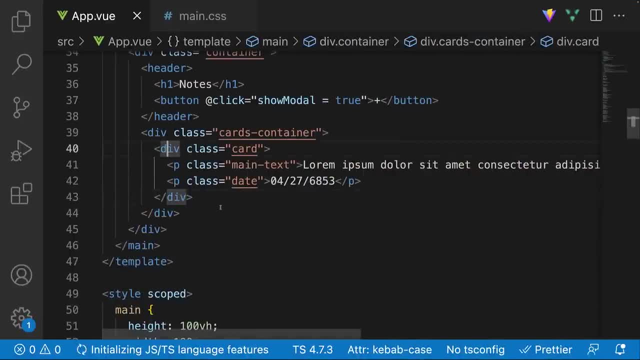 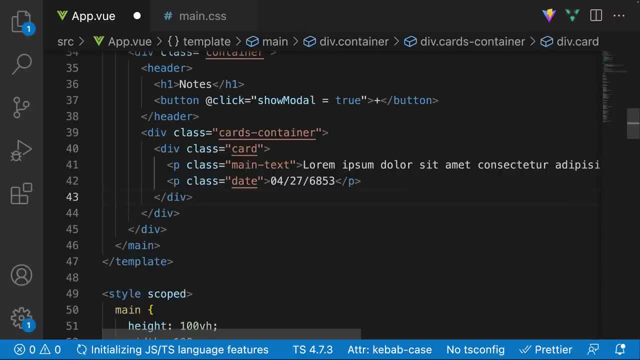 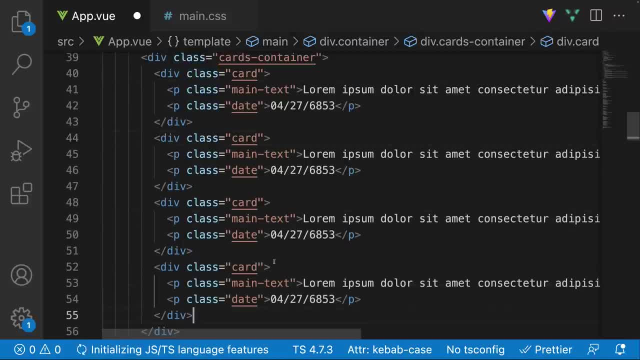 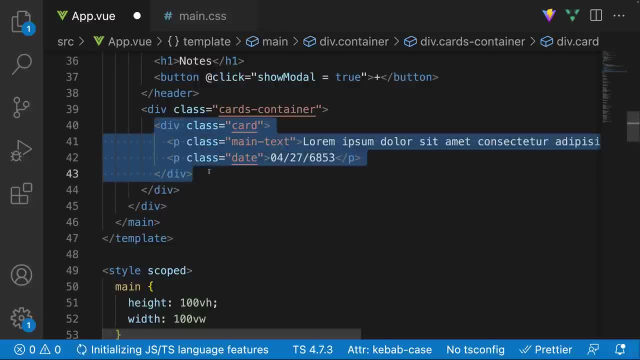 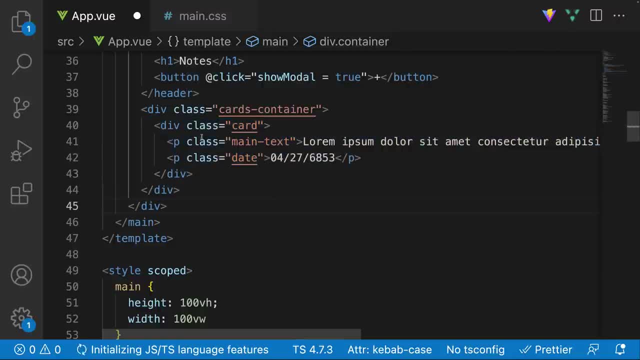 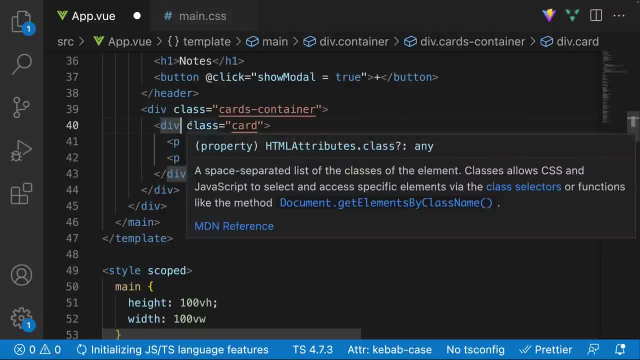 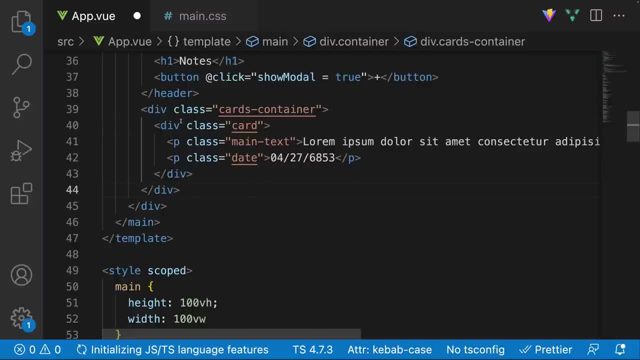 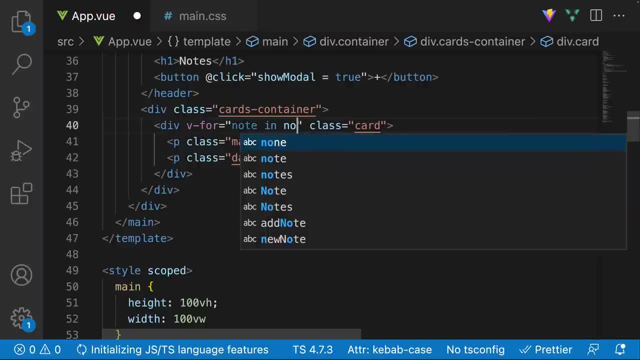 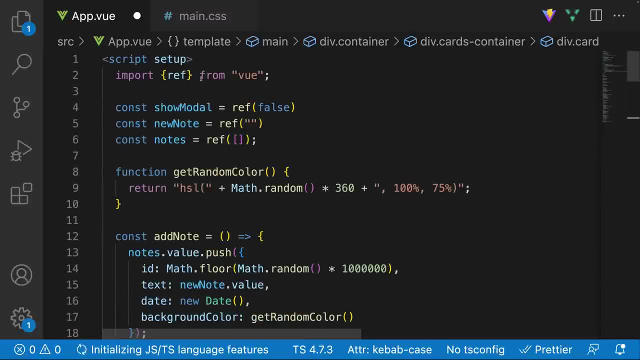 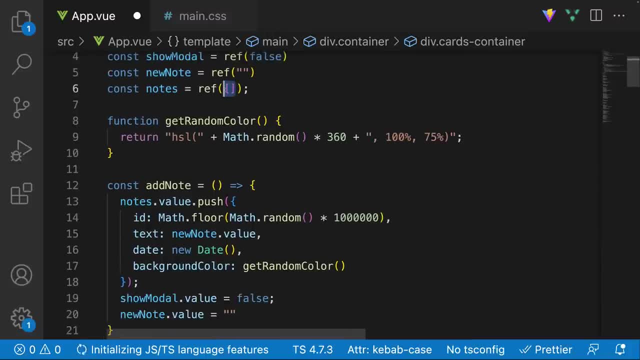 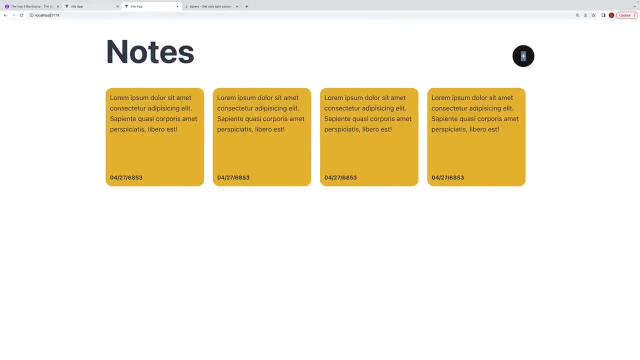 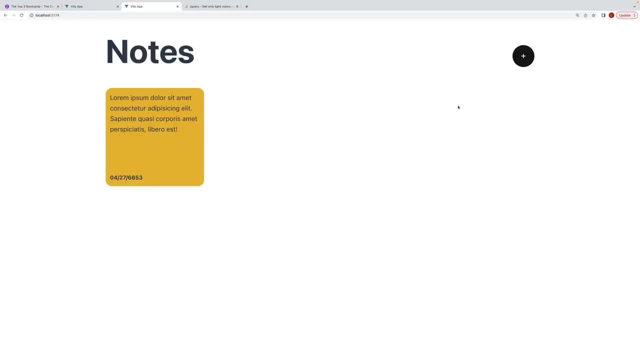 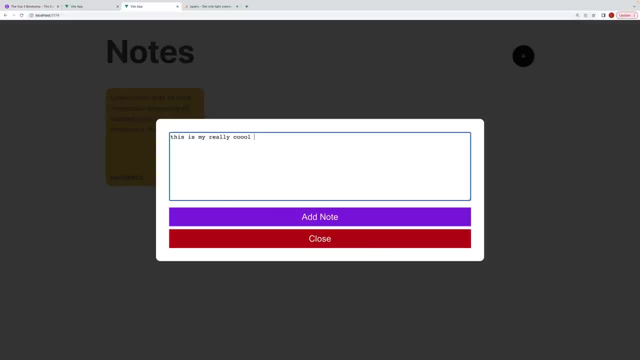 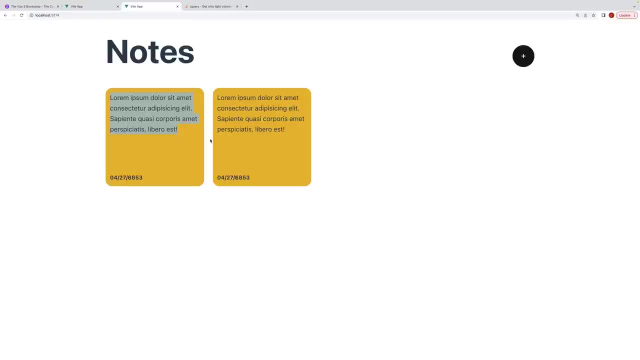 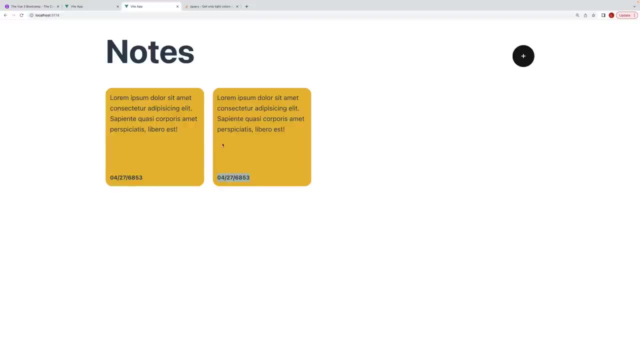 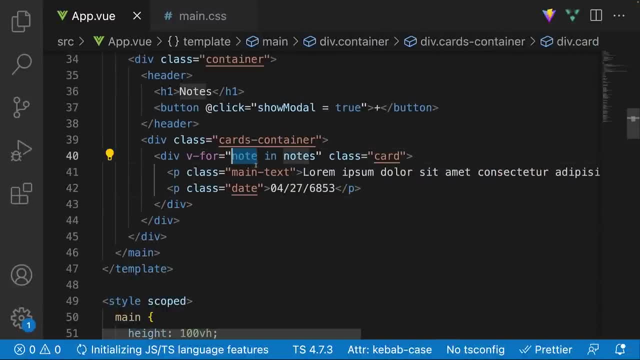 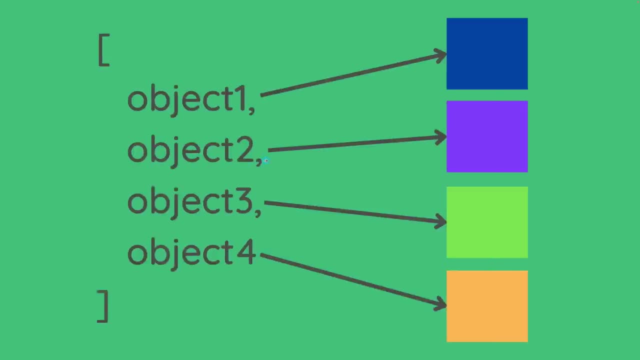 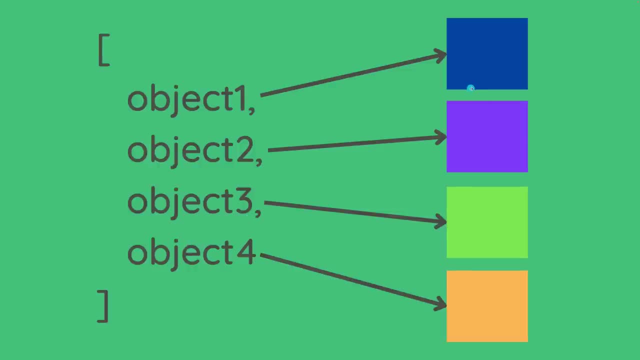 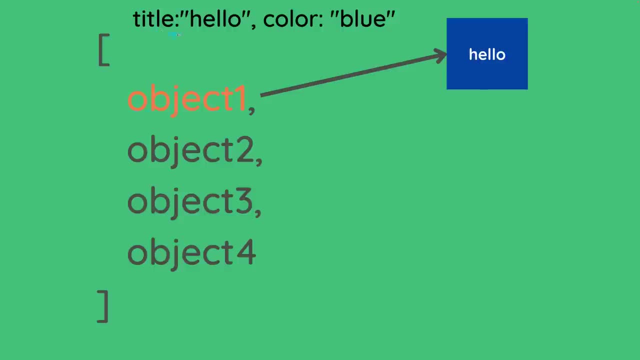 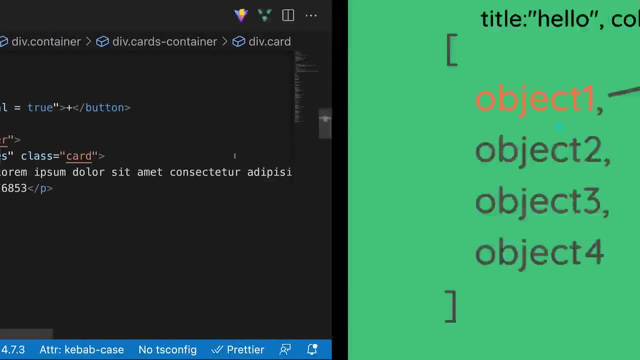 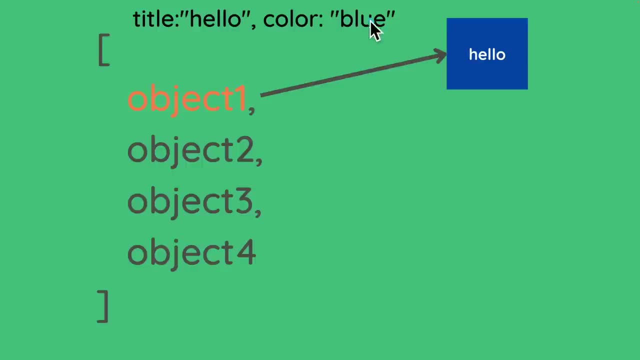 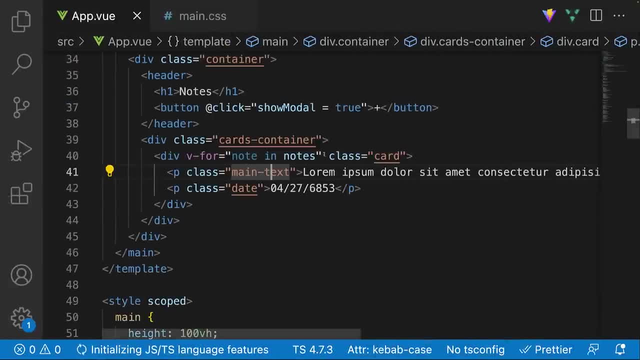 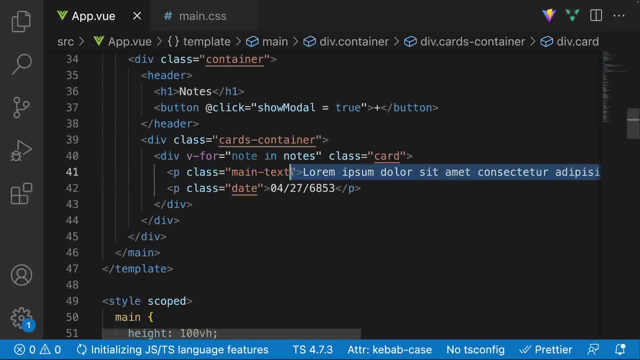 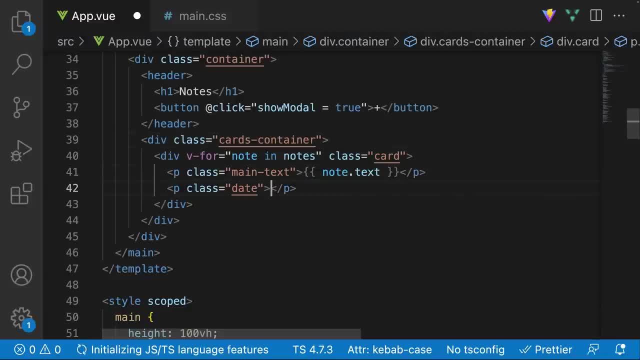 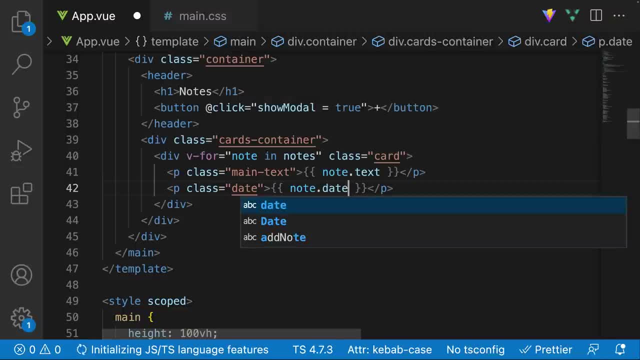 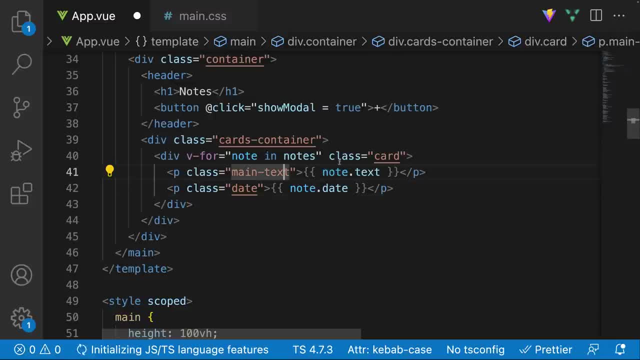 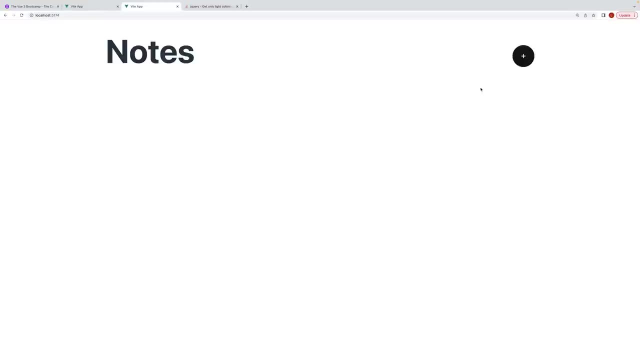 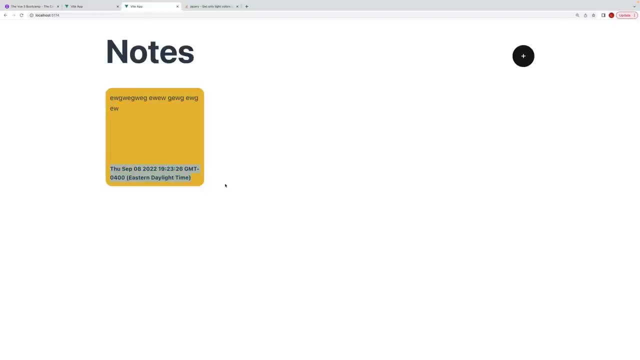 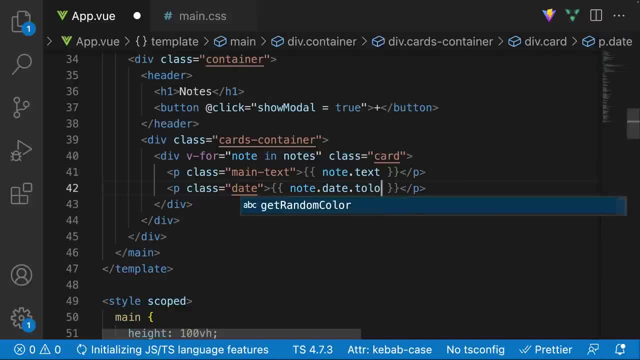 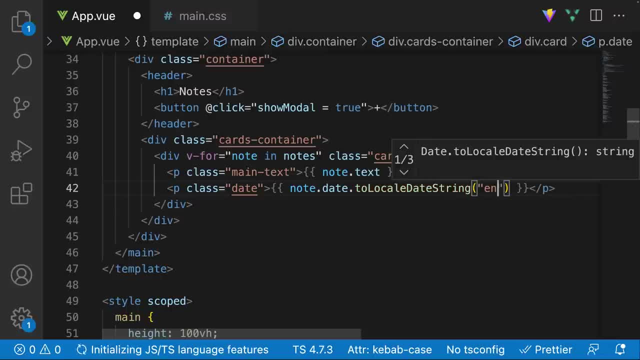 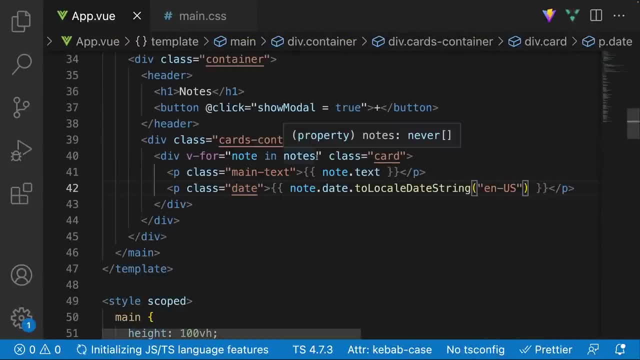 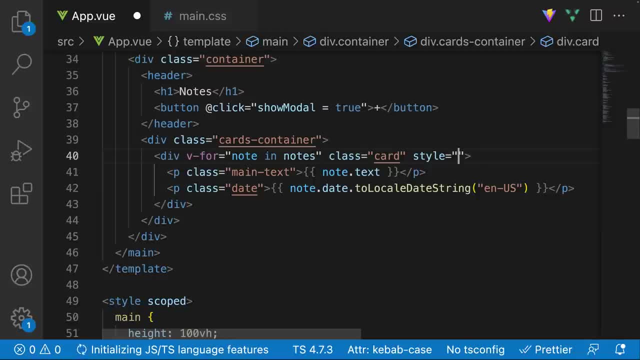 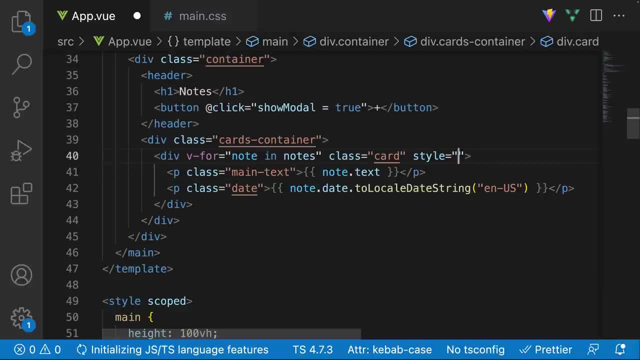 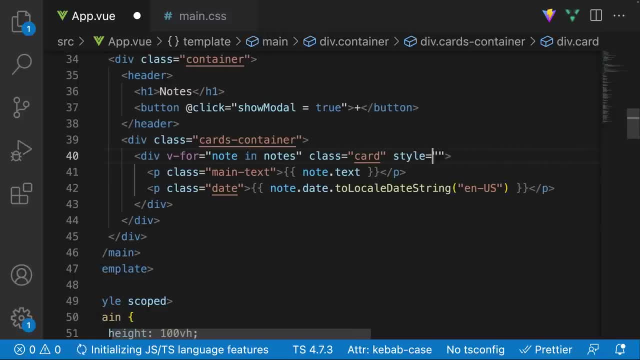 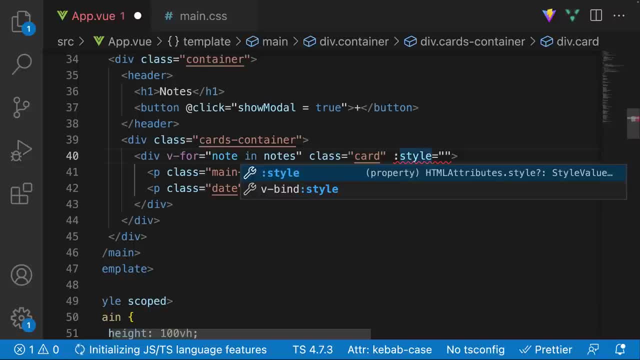 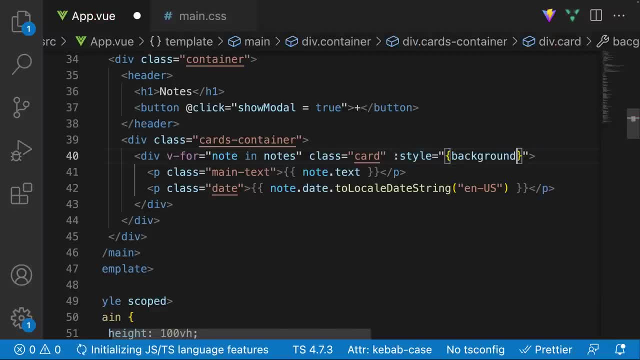 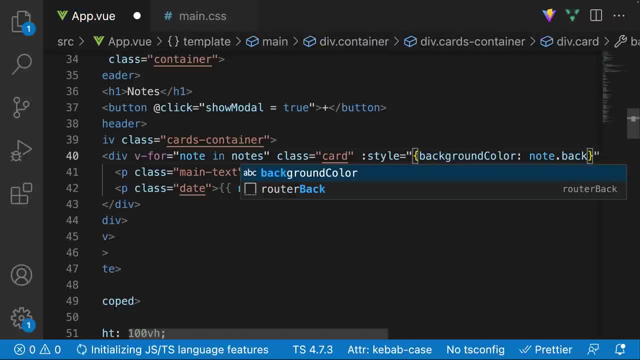 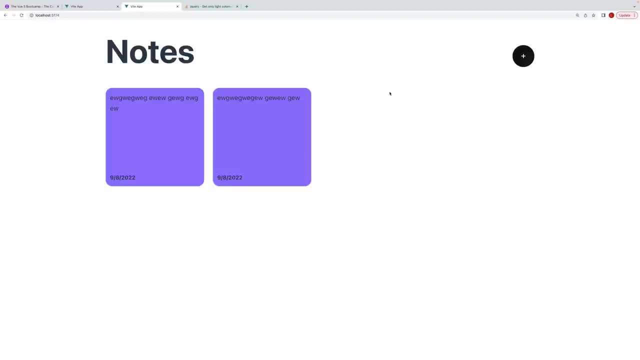 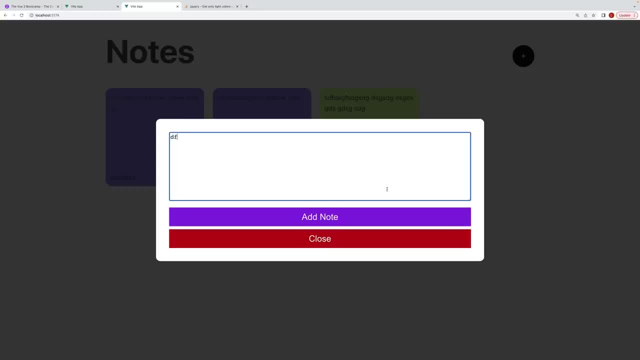 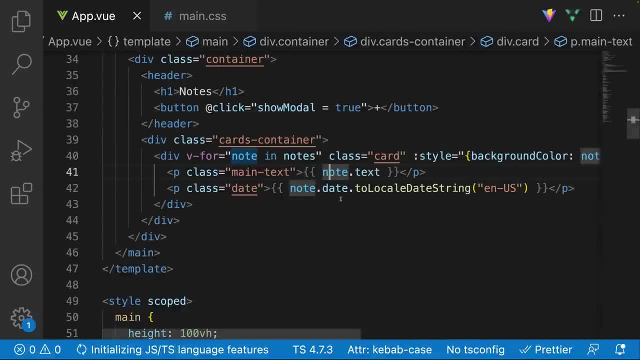 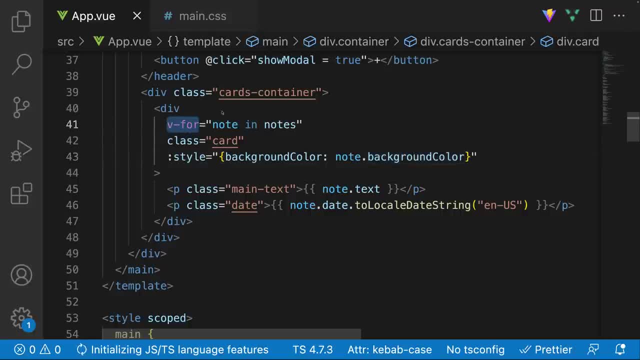 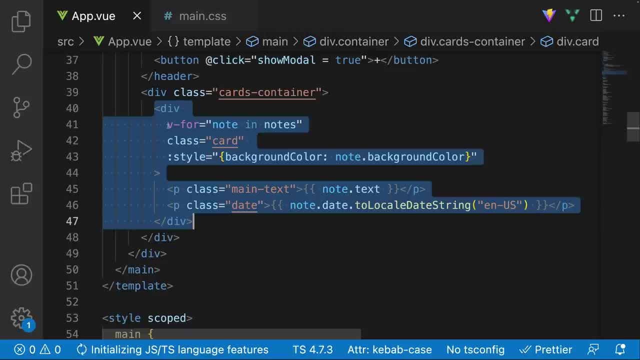 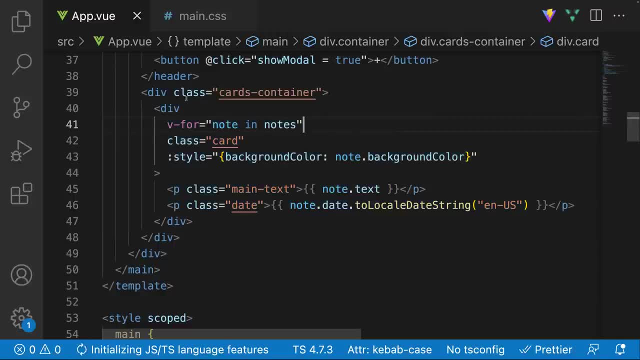 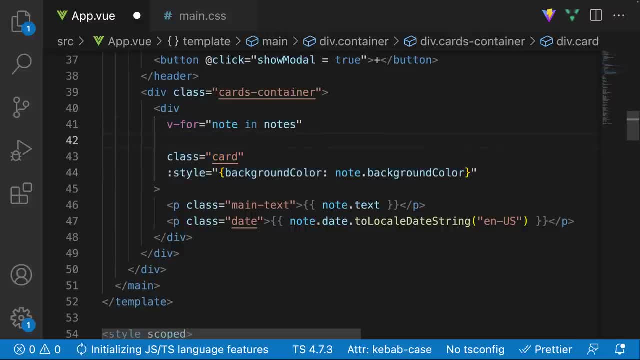 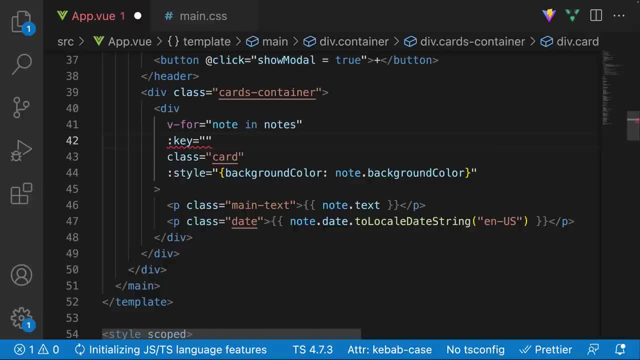 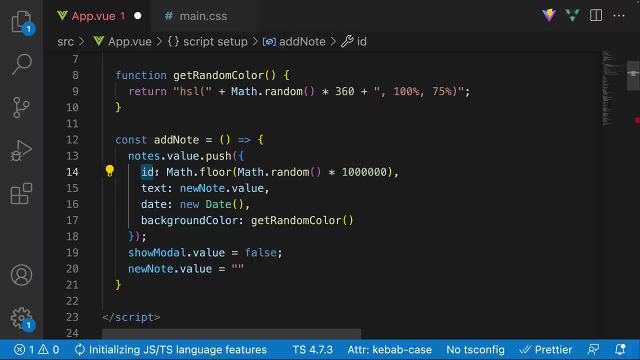 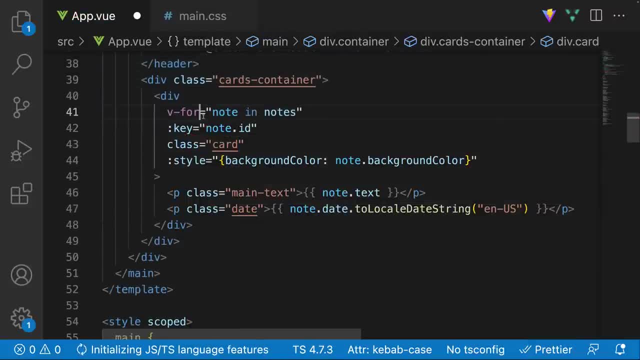 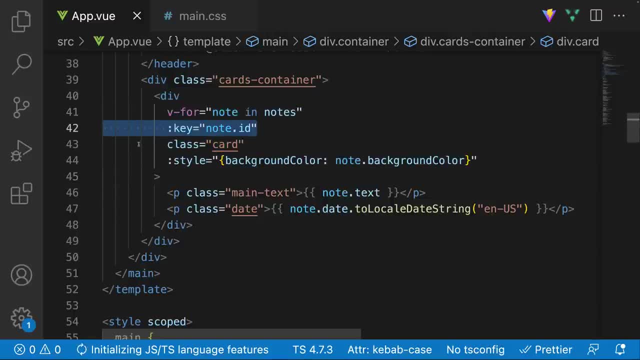 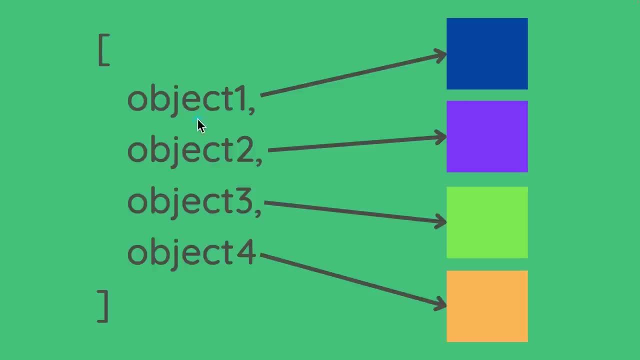 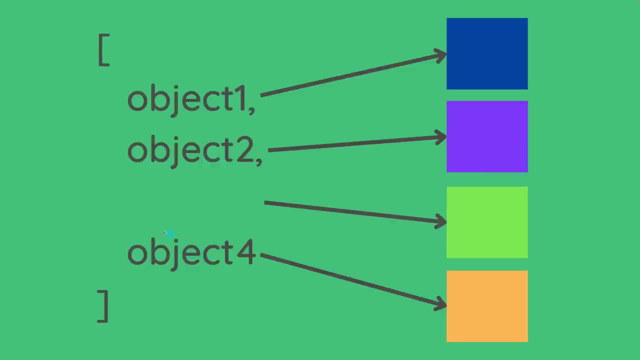 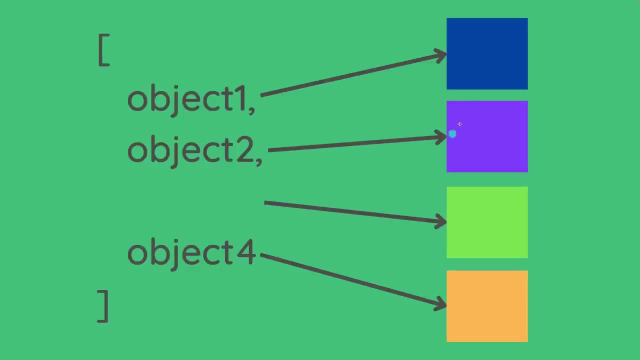 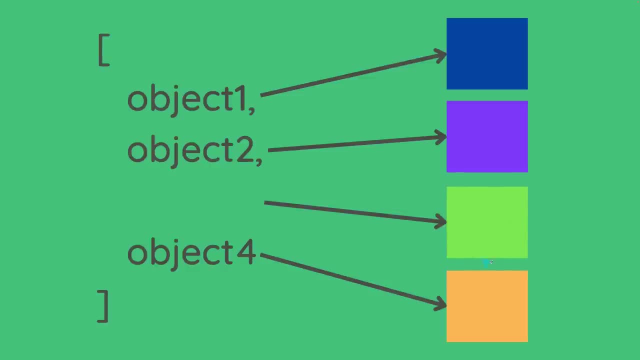 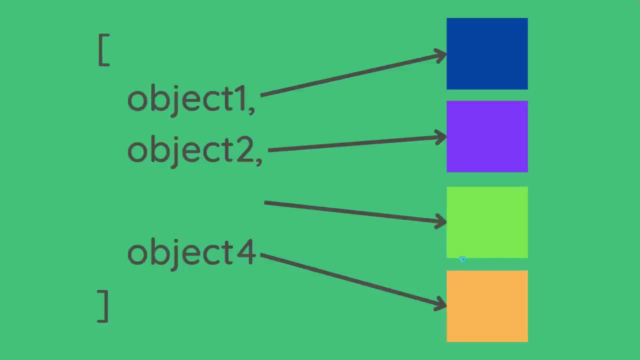 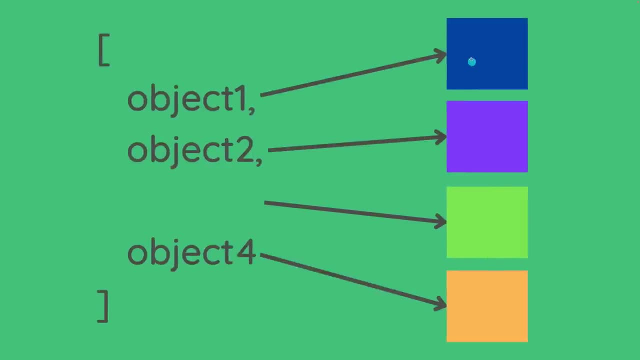 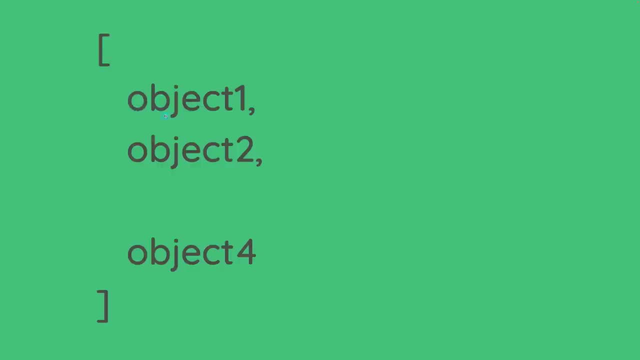 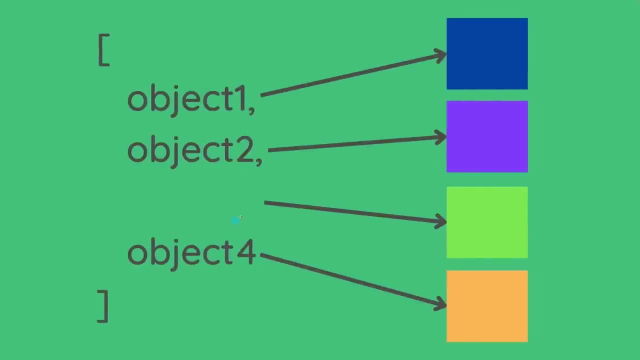 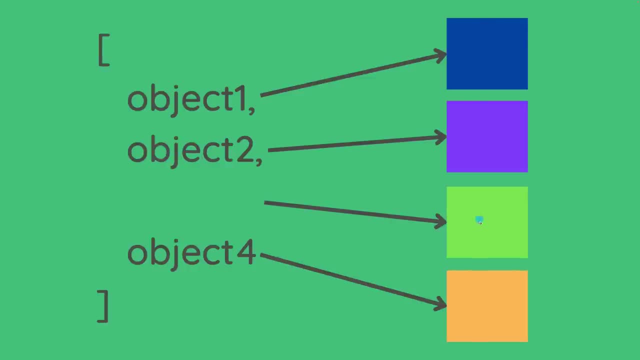 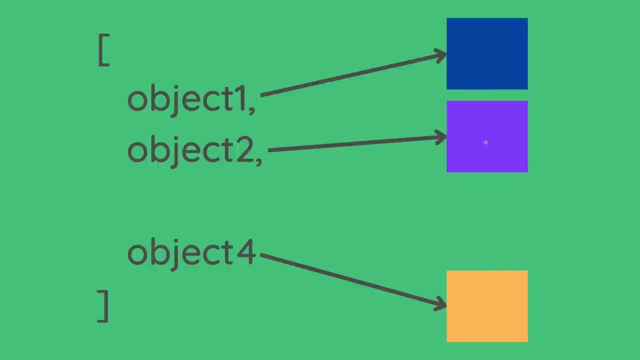 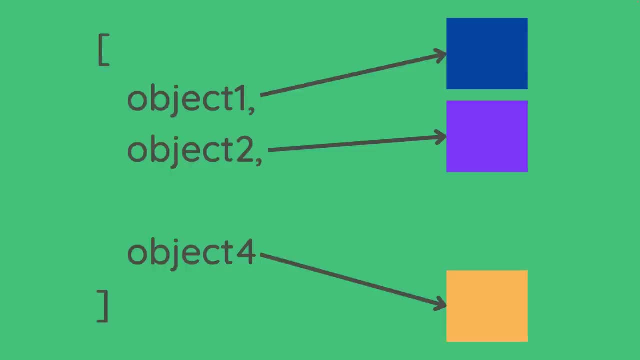 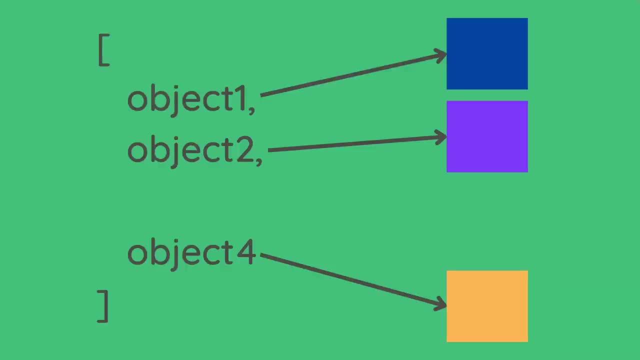 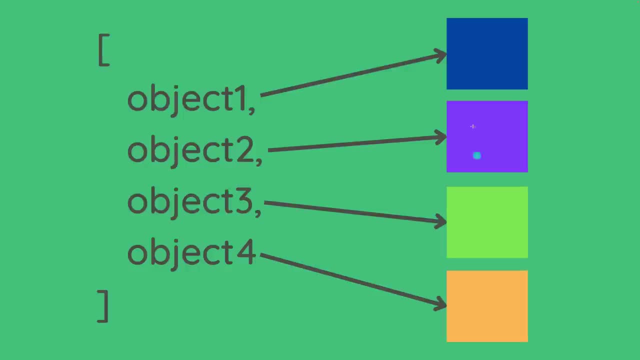 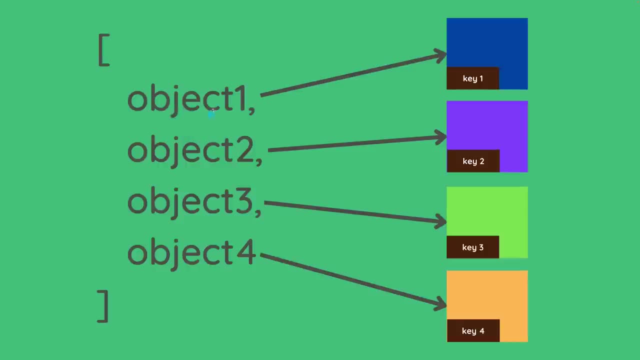 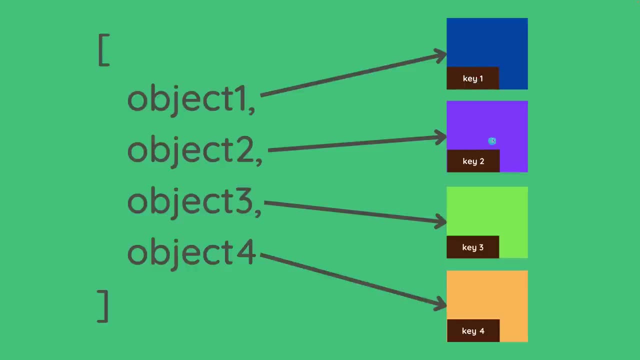 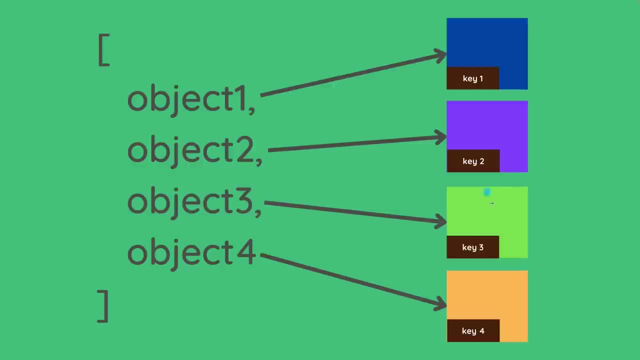 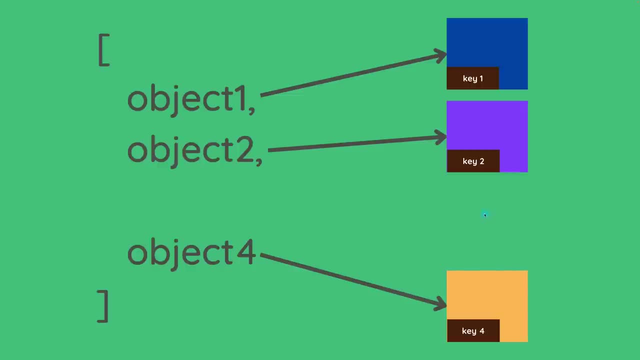 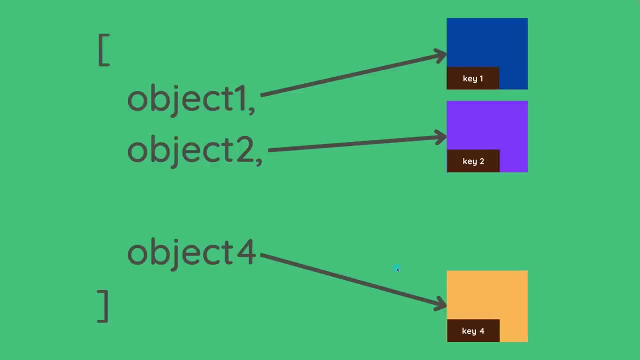 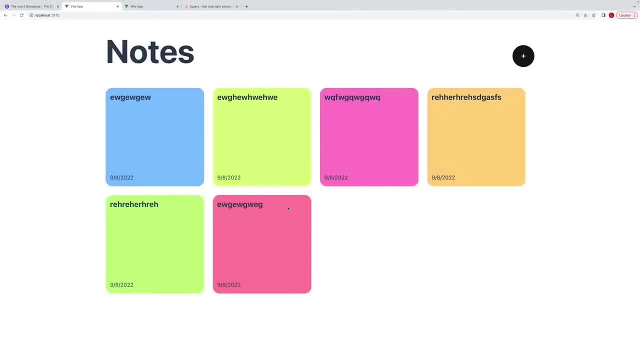 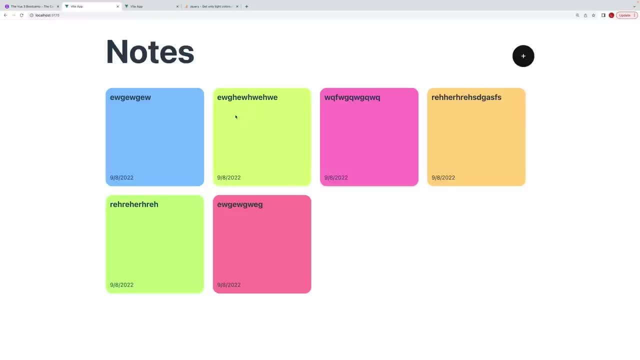 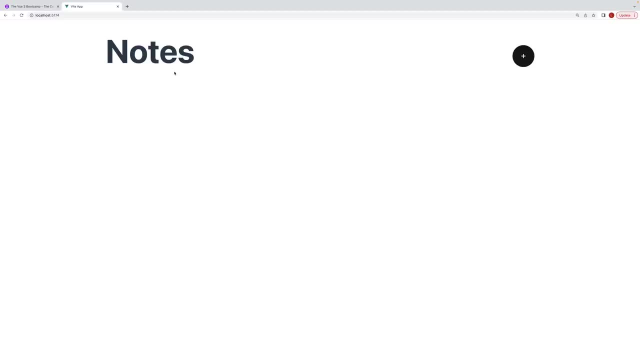 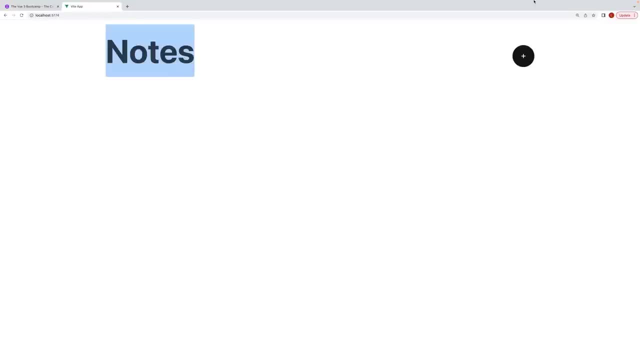 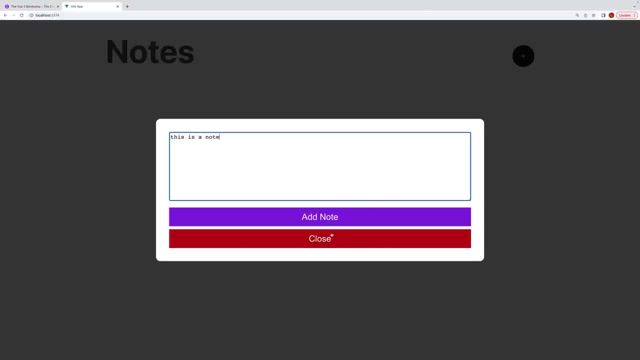 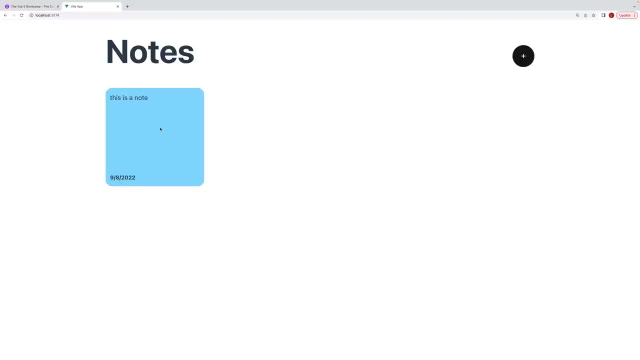 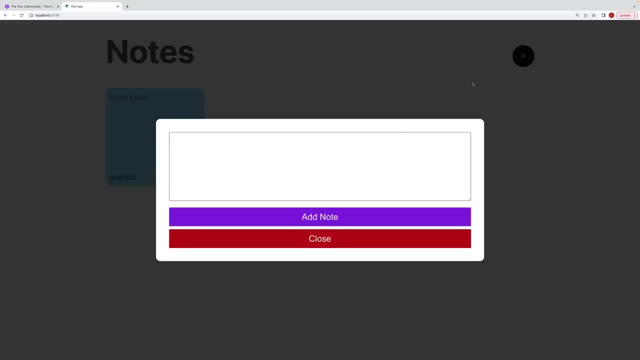 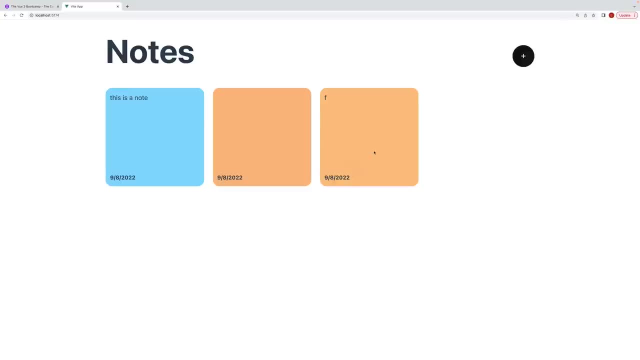 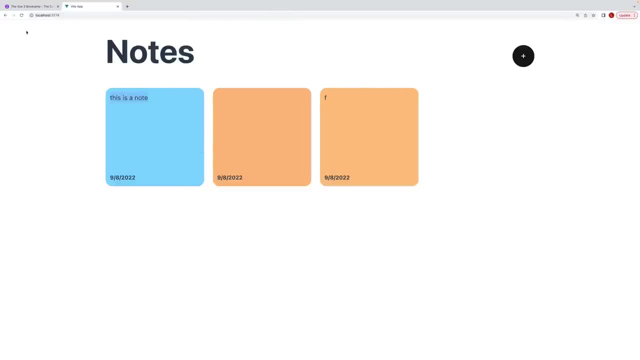 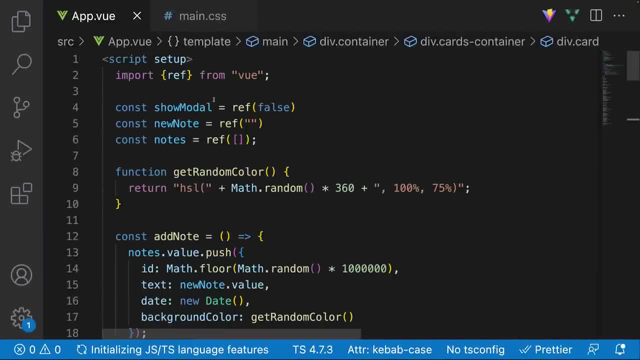 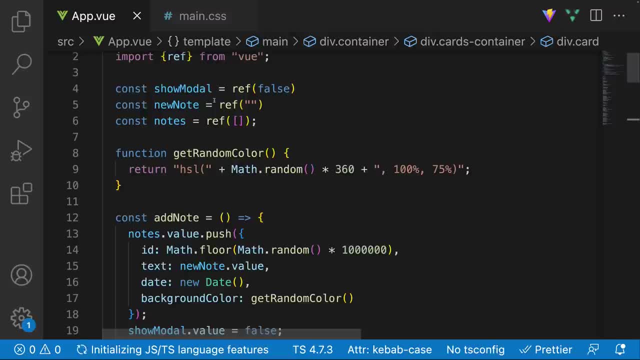 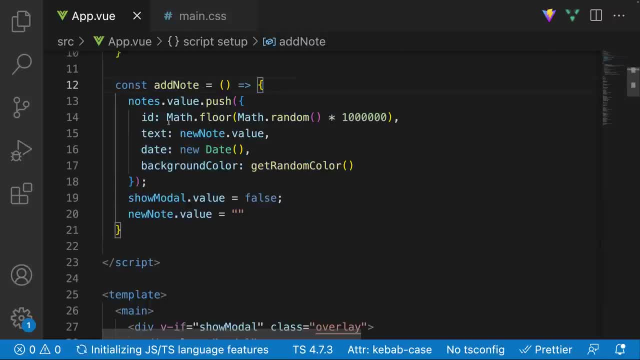 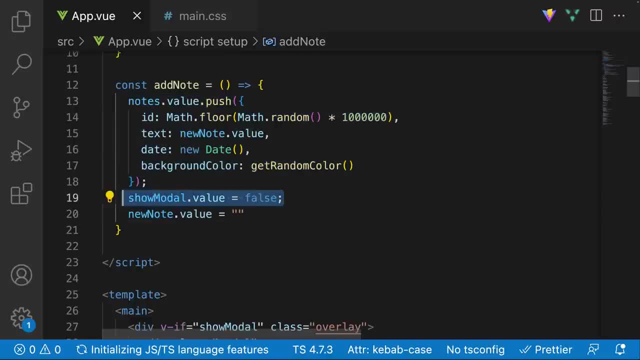 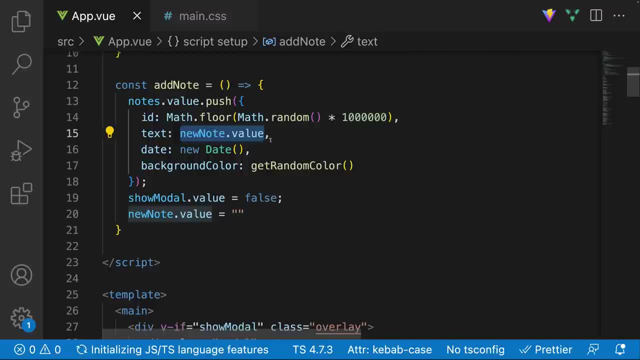 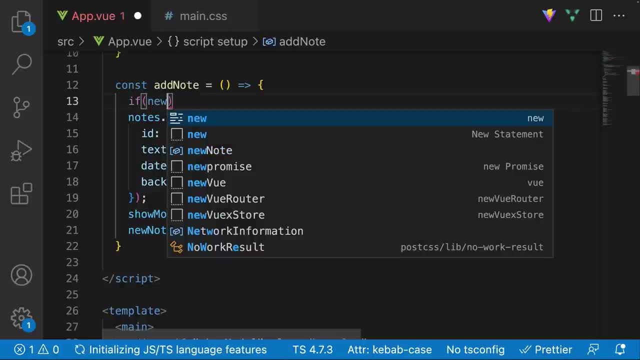 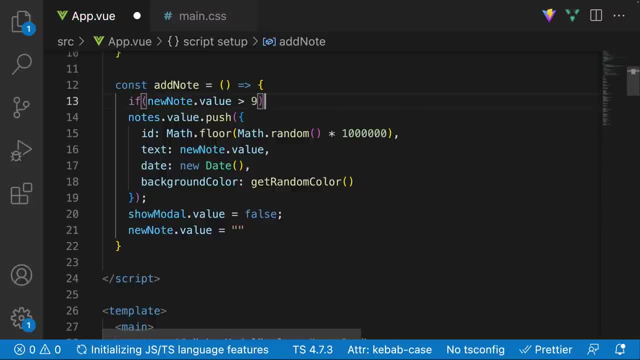 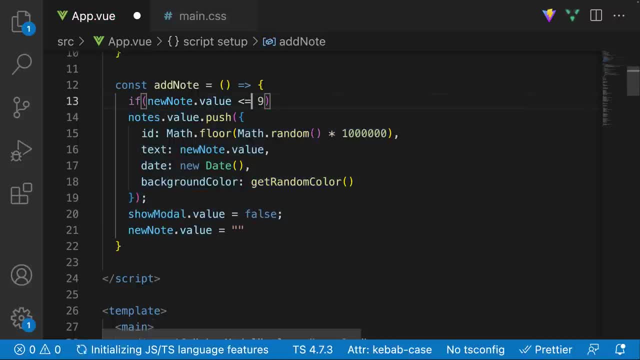 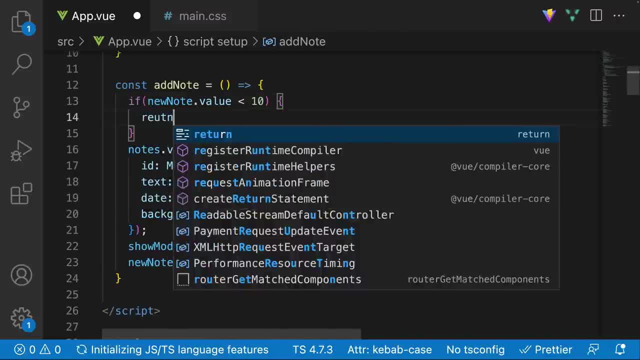 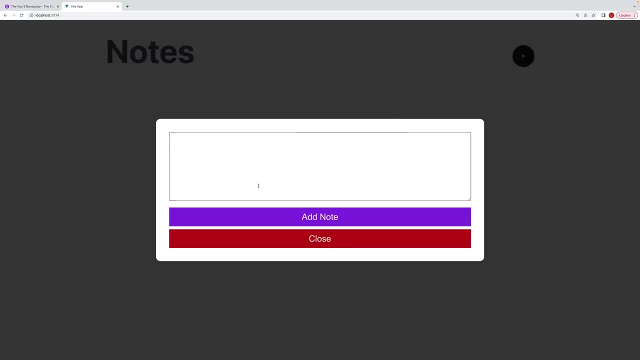 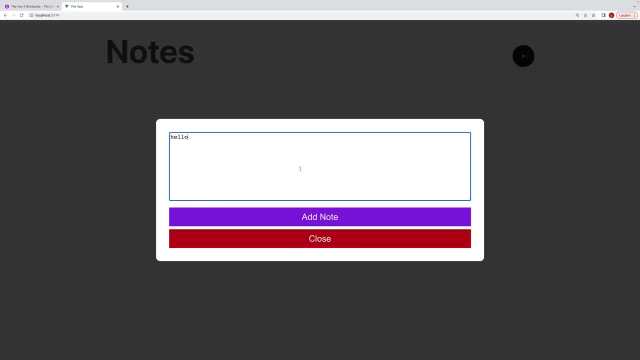 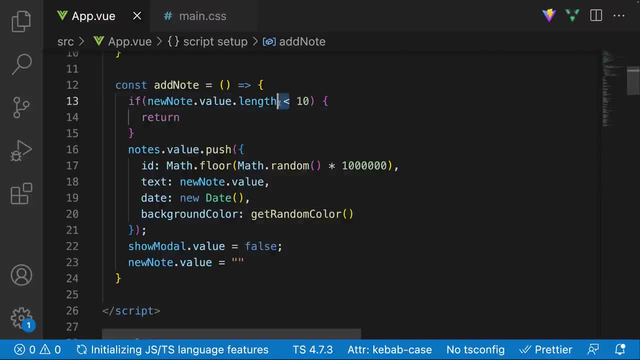 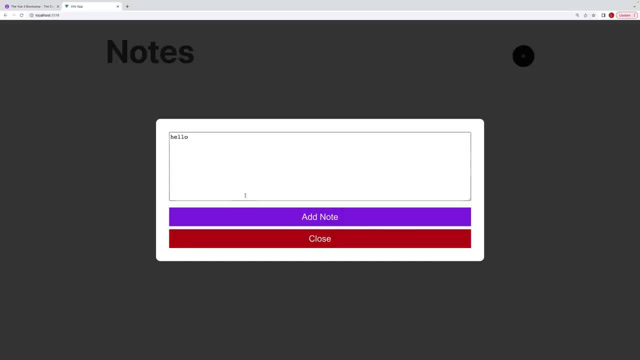 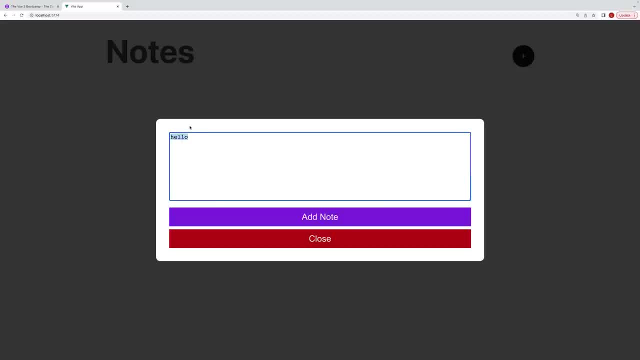 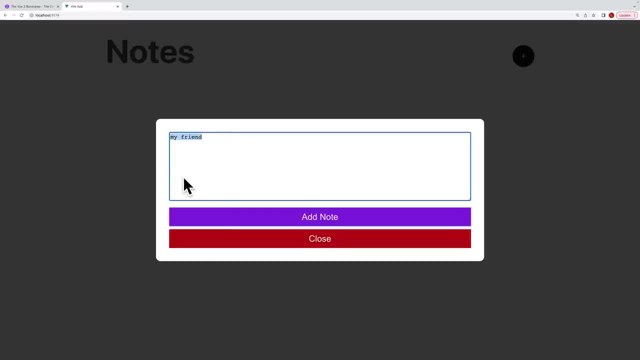 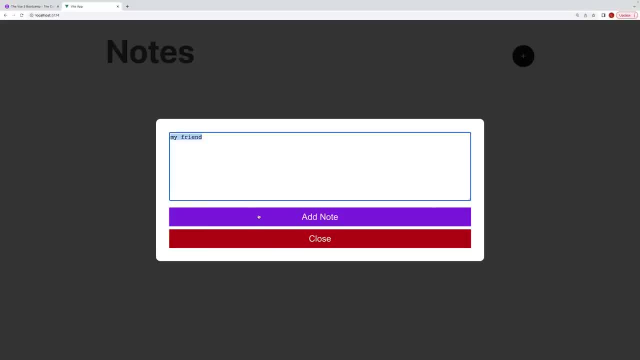 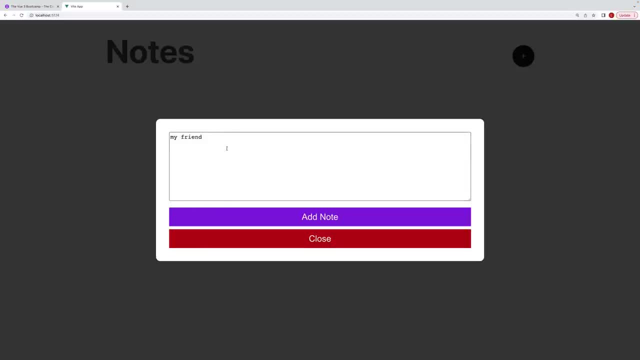 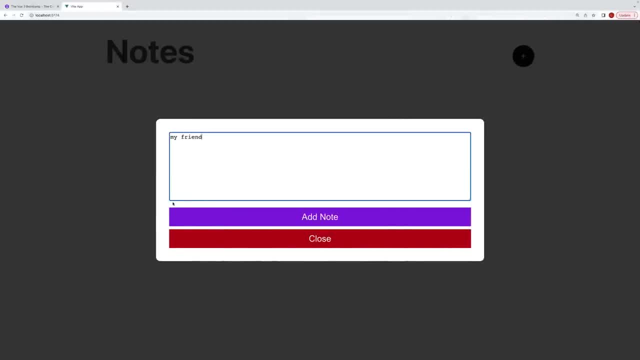 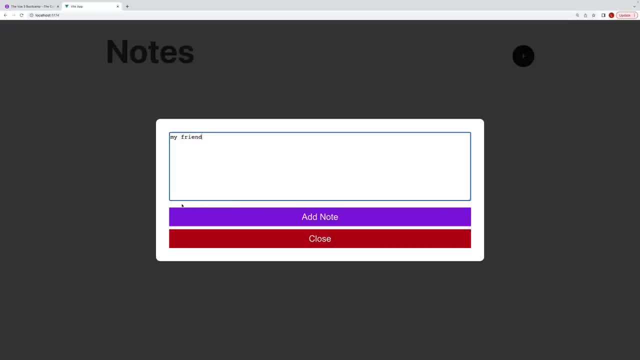 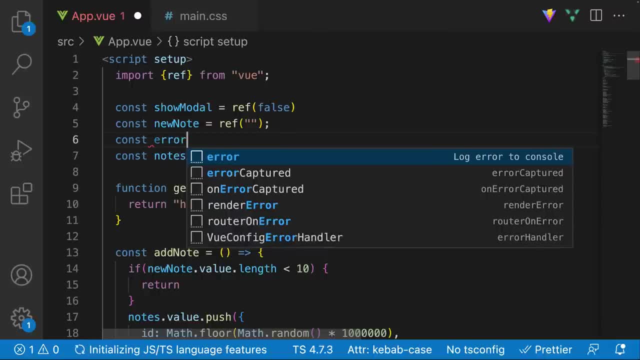 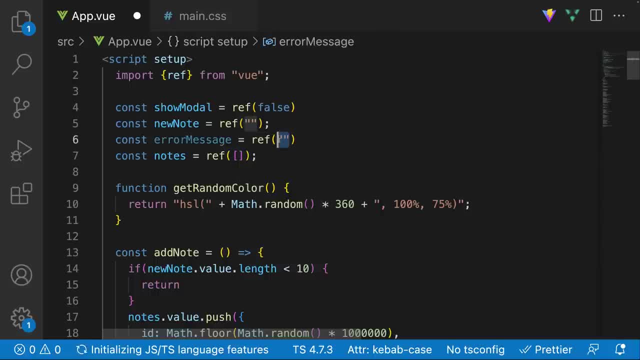 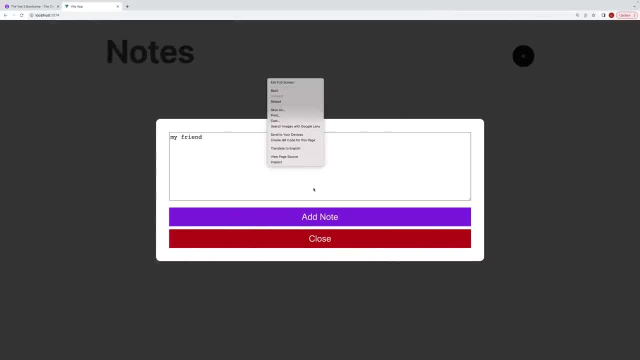 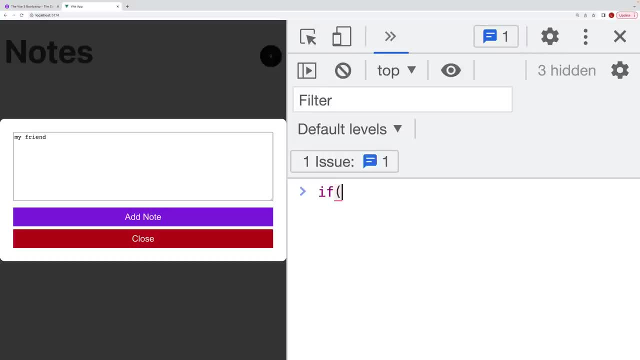 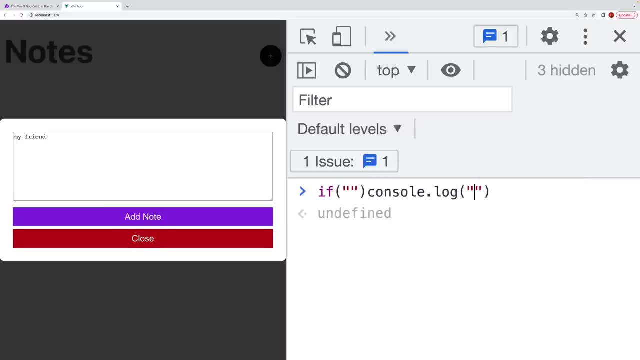 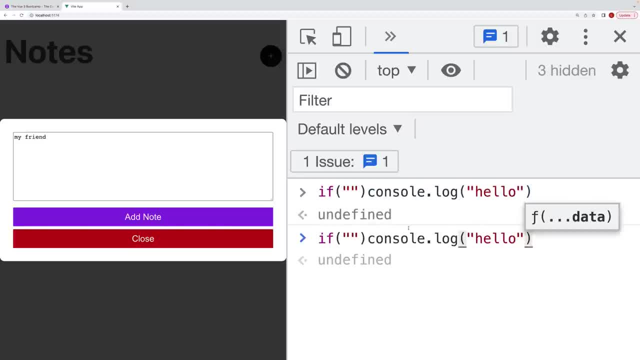 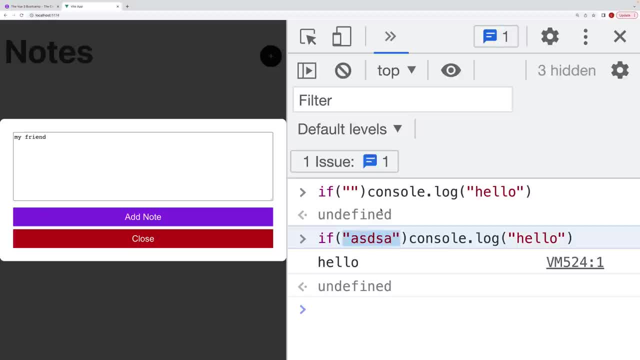 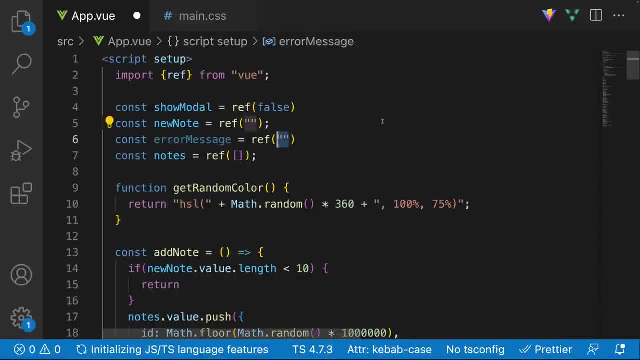 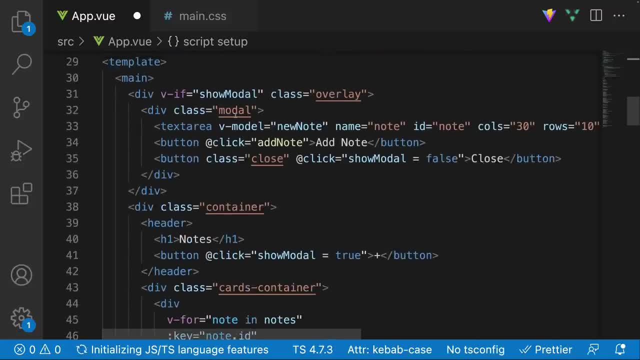 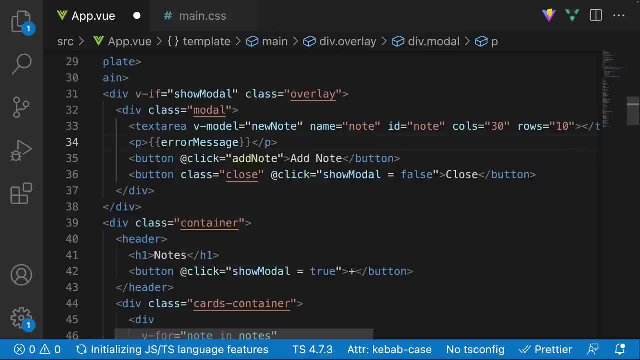 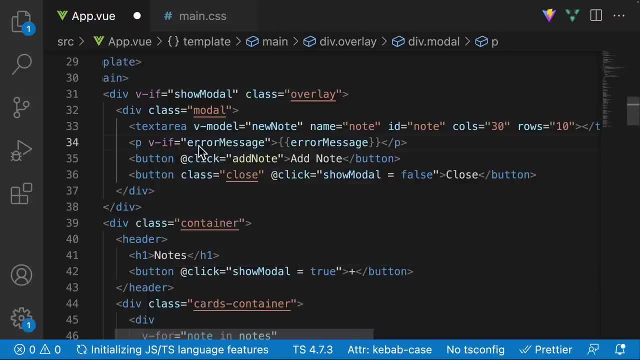 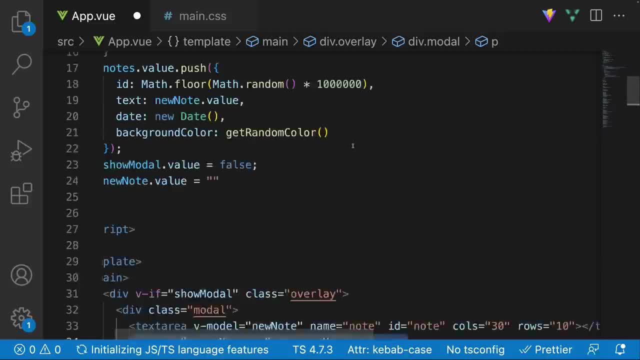 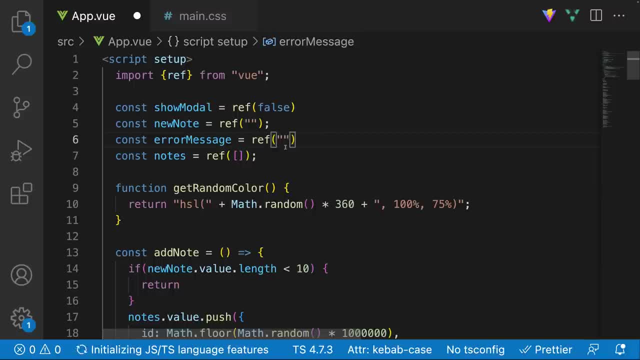 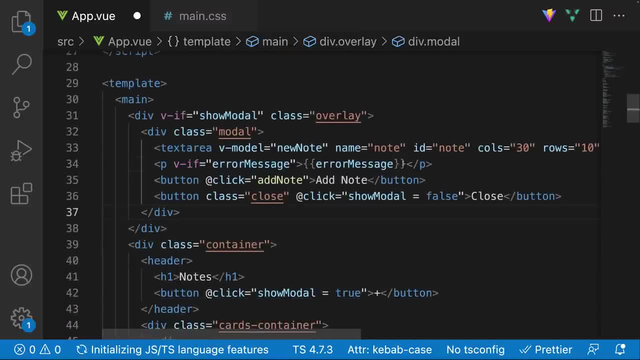 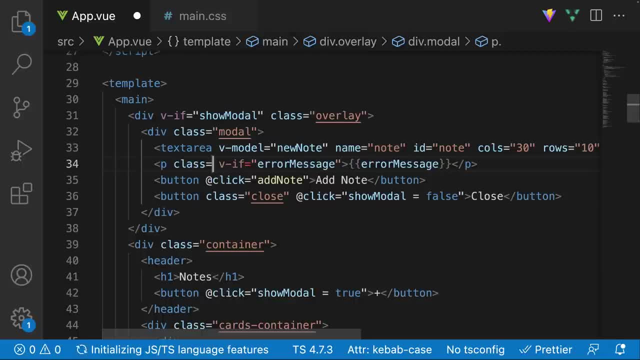 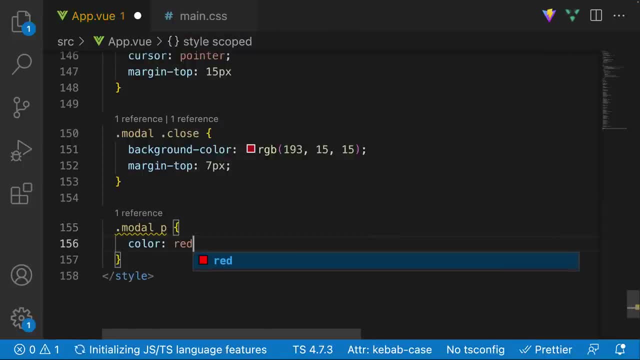 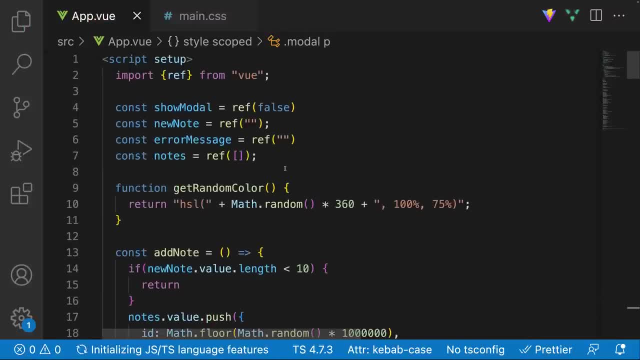 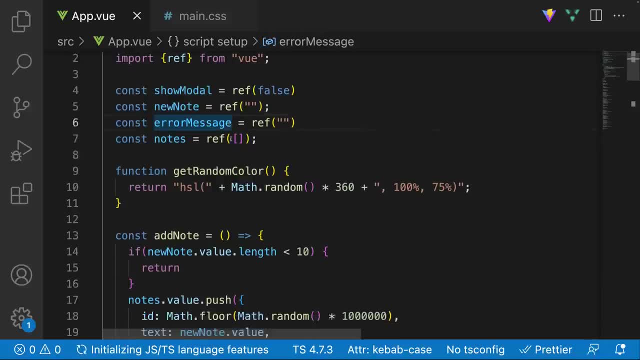 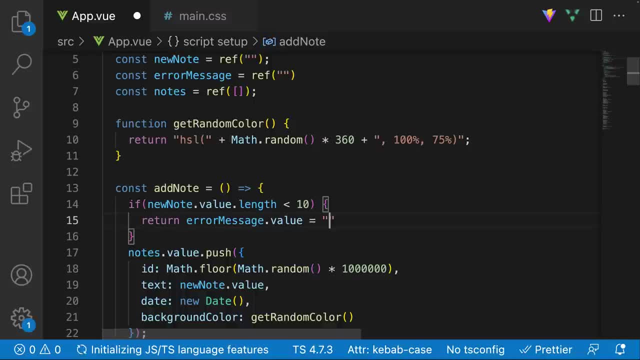 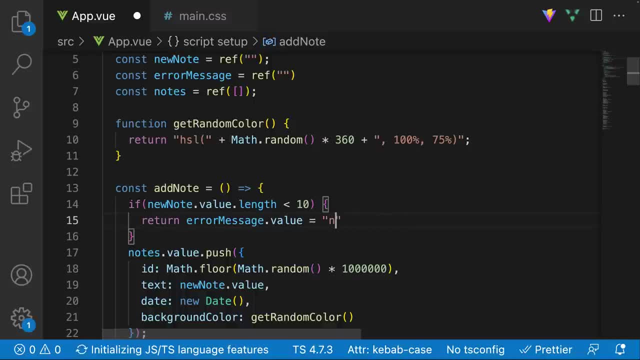 needs note, what am I doing here? Note needs to be 10 characters or more. All right, so let's go ahead and actually give this a little test. And let's go here. And I'm gonna say, hello. I'm gonna say add, and there we go. 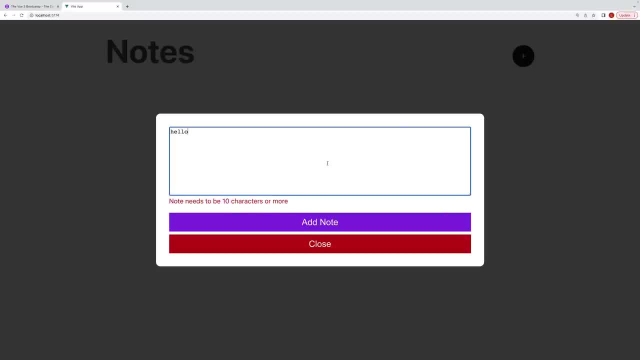 Now we get a nice little error message. All right, cool. 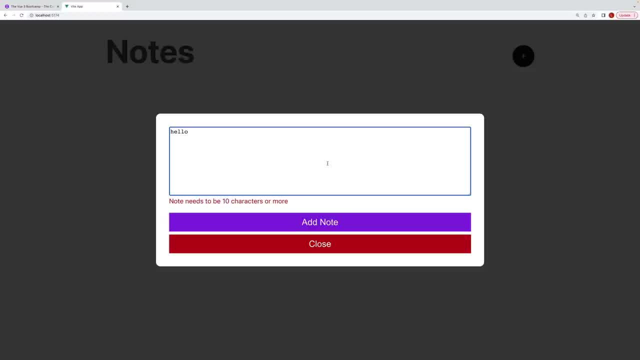 Now there is one little thing that can actually happen that can kind of just break everything. 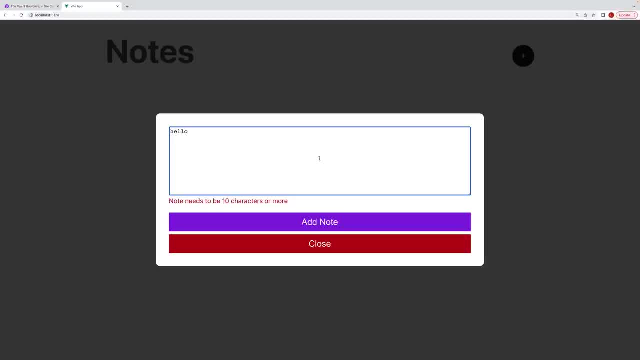 So if a user is smart enough, what they can actually do is very simply just say hello. 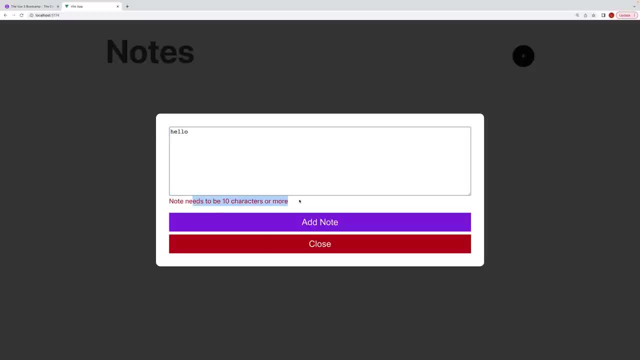 And then they're like, okay, hello. Oh, oh, I need 10 characters. Oh, let me just add a bunch of spacing over here. 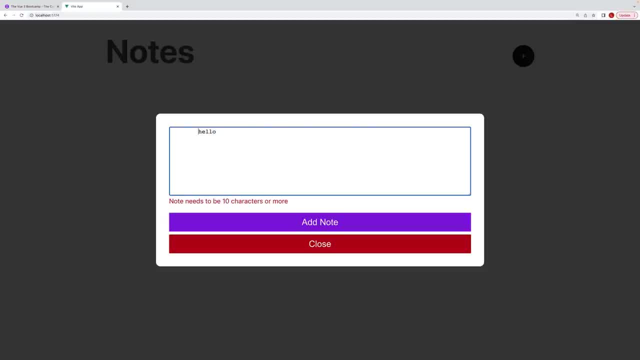 So I'm gonna add a bunch of space here. I can even also add a bunch of space here. 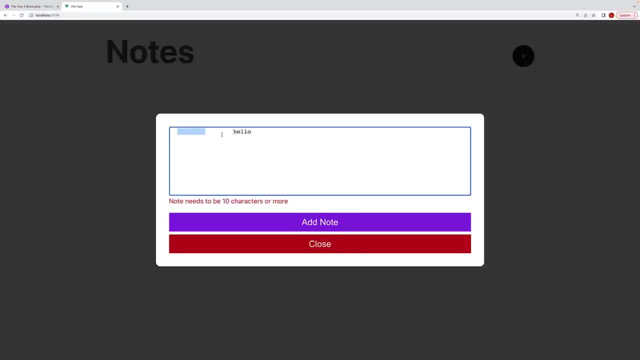 And then our application is gonna treat this as, well, each space is gonna be a character. So definitely it's gonna be more than 10 characters. And the person can go ahead and just add a bunch of space here. And then our application is gonna treat this as, well, each space is gonna be a character. And then our application is gonna treat this as, well, each space is gonna be a character. And then our application is gonna treat this as, well, each space is gonna be a character. And add a note. 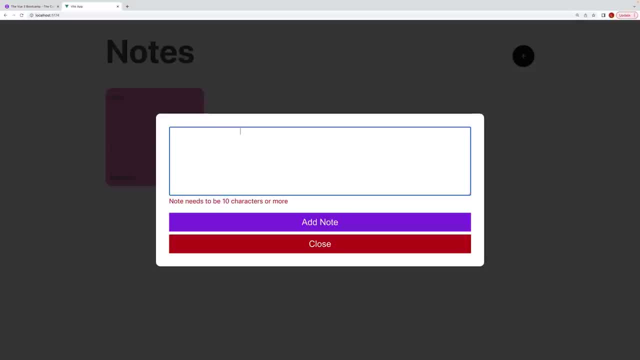 Another thing that they can also do is they can always go over here, just add a bunch of space, and they can just add an empty note. 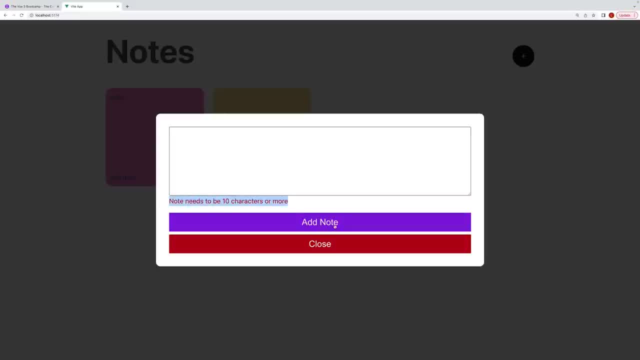 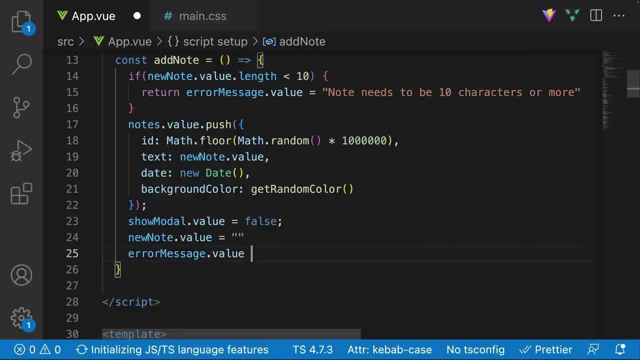 Another thing is this error message is always appearing. So ideally, after we're done, what we can do is also set the error message. So we can say error message.value is equal to a string. 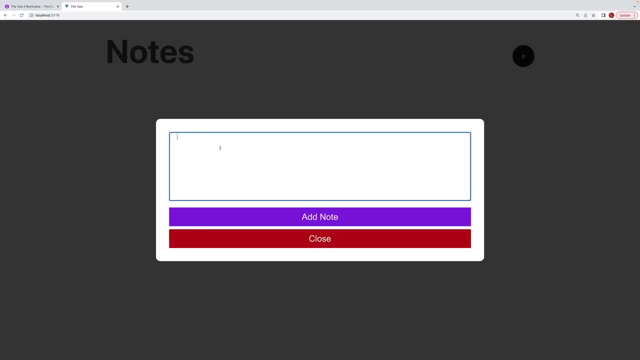 So what are we going to do here in order to fix kind of this spacing issue? Well, very simply, 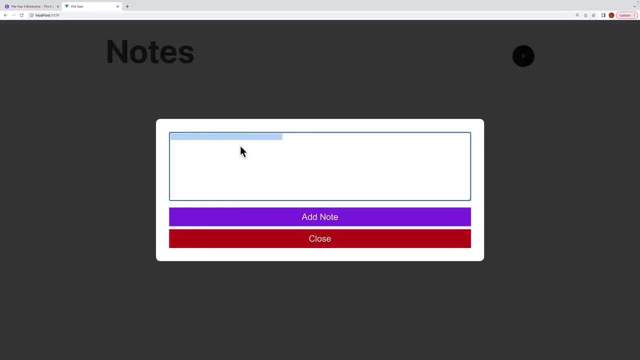 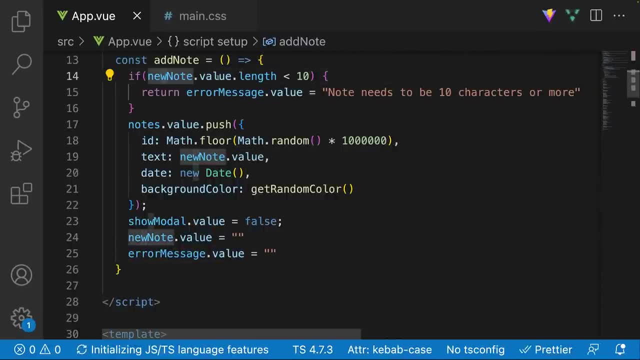 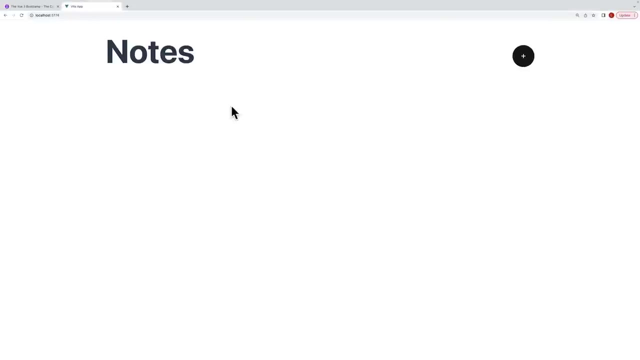 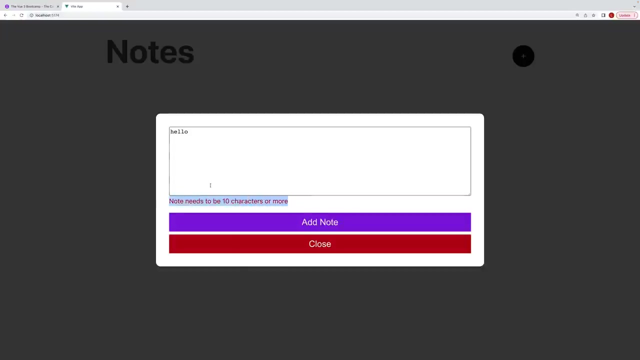 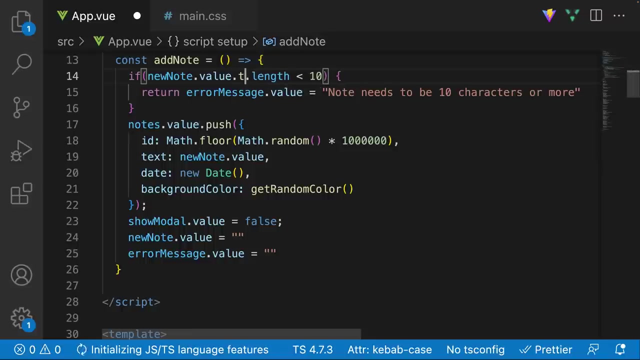 what we can actually do is just trim the white spaces from the front and the back. And we can actually very easily do this in the check itself. So we can say new notes dot value, and then I can say dot trim. And then I can say dot length like so. And now if I were to do this, hello, and add just a bunch of spaces, you can see that we get this error message. The issue with doing it this way is now our state actually has this value over here. So it has hello and a bunch of empty spaces, we just trimmed it in this check. So ideally, we can actually trim it even before it reaches our state. And we can actually do that really, really easily. So let's just remove this for now. 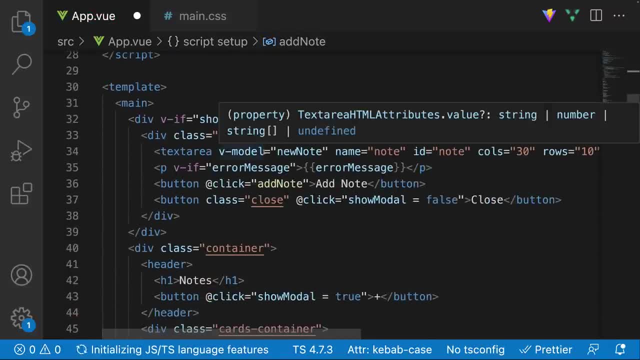 And to do this, what we can do is right on the V model, we can say dot trim. So this is going to perform the two way binding, and it is going to trim anything. So we can say dot trim. And we can say dot trim. So this is going to perform the two way binding, and it is going to trim anything. So this is going to perform the two way binding, 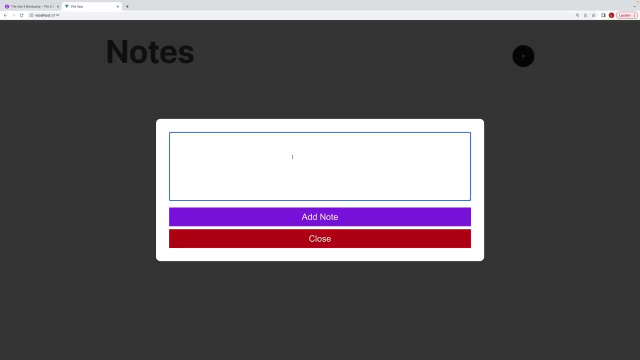 white spaces. So now let's try it again. I'm going to say space, space, space, space, space, hello, space, space, space, space, space, I'm going to try to add the note. And you can see 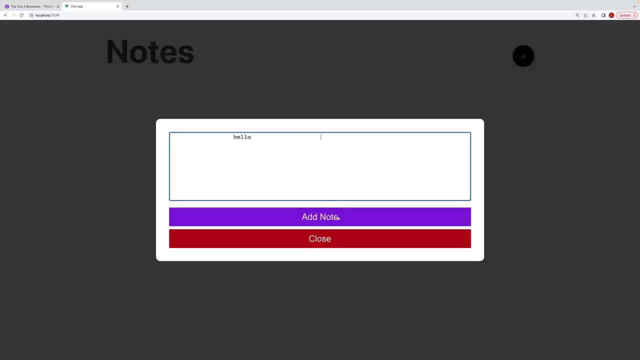 right away, it actually removes all the white spaces because they're just unnecessary, and it 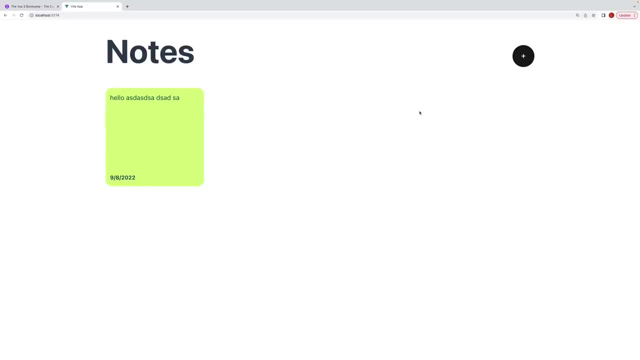 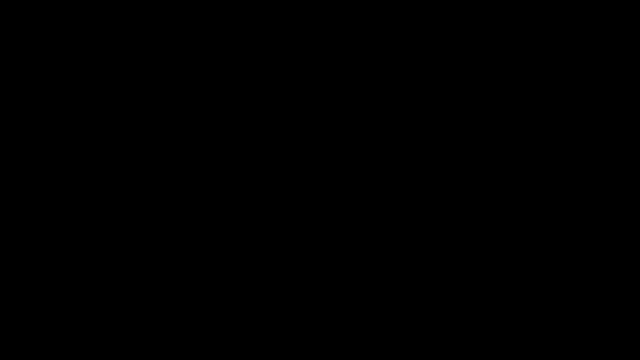 throws the error. Now we can just fix it. And there we go. And if you go right back, everything is working fine. Hallelujah, we just finished our second project. We finished one project. Well, 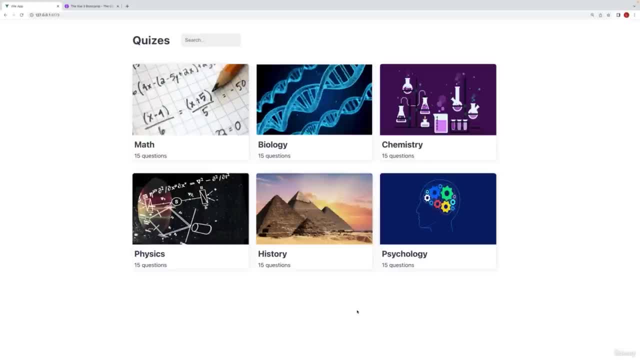 the best thing to do now is to move on to another. This right here is the new project that we are going to be building with view three and the composition API. And it is trust me going to be significantly more difficult and it's going to cover significantly more view topics than the one that we did last time. So I hope you guys are excited. Let me go ahead and do a quick little introduction of the project. So over here, 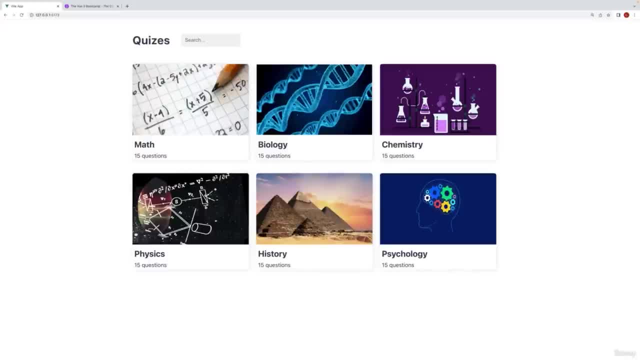 we have a very simple quiz game. And what you can do here is you can just go to on this website and 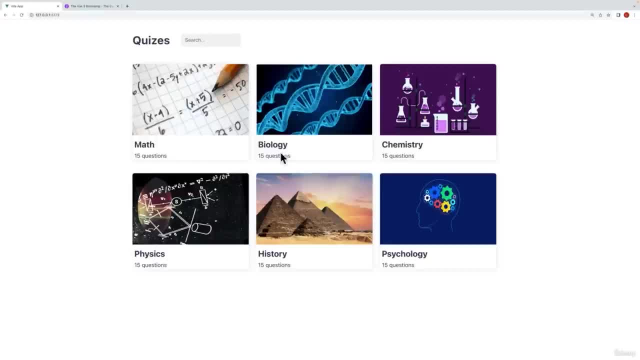 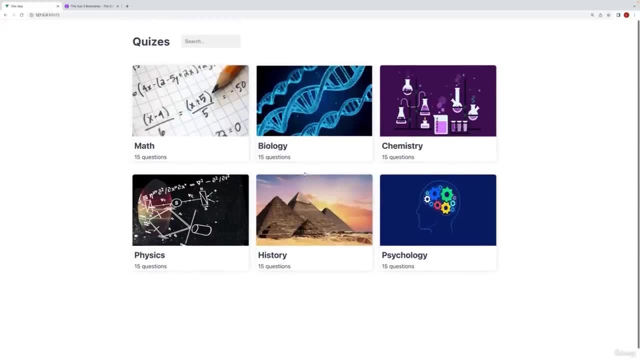 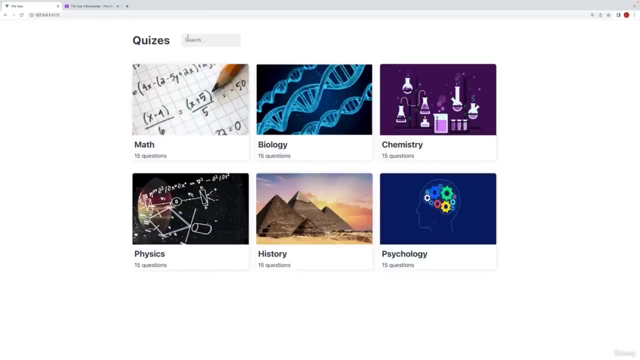 start viewing all of the different quizzes that we have. Math, biology, chemistry, physics, history and psychology is what is appearing right now. Now let's say that this is a very exhaustive list. And maybe what you want to do is you want to search for a particular quiz. So let's say you're looking, you're looking and you're looking for chemistry, but you can't find chemistry, even though it's right here. 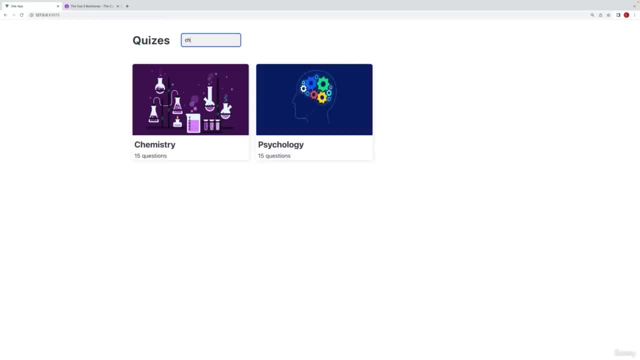 What you can do is you can use this search bar. So over here, you can start typing chemistry. And you can see that it's going to return any cards that has this match right over here. So ch chemistry 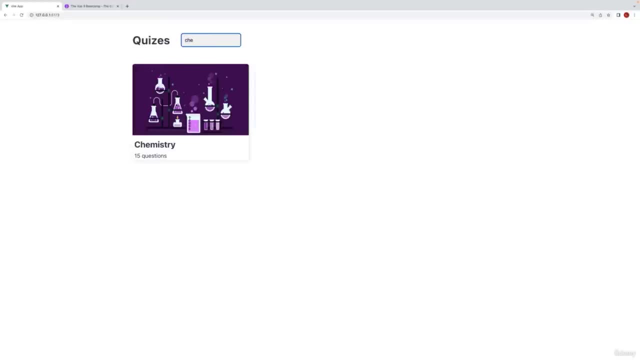 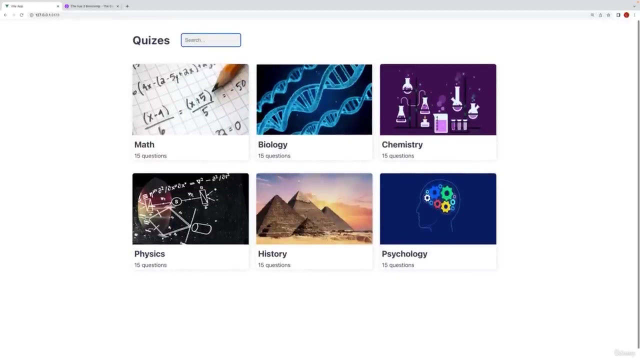 and also psychology has a ch. And of course, you can continuously refine your searches. Now, of course, you can delete your searches and it comes right back. So we're going to have this search ability that is going to remove cards based on your search. Now, of course, what we're going to do is we're going to make these cards clickable. So when you click on a particular card, let's say you 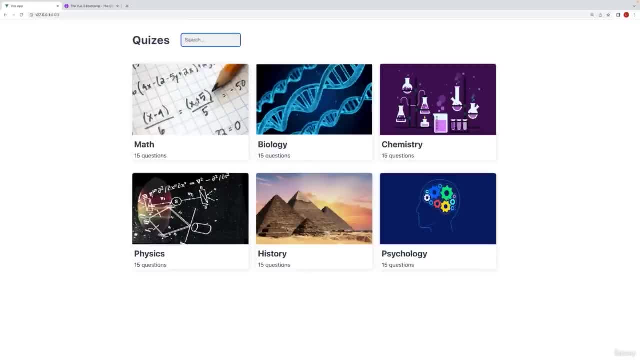 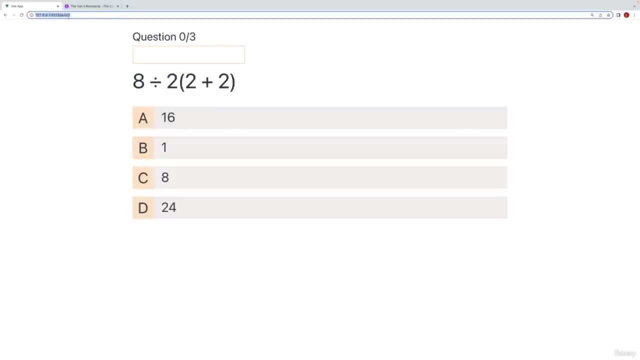 want to learn math, I'm going to go ahead and click on this card. And it is going to actually take you to a brand new page. So over here, you can see that the URL and might be a little tiny for you. But you can take my word on it. It used to be just localhost 5173. But now it's localhost 5173 slash quiz slash the quiz ID. And we're going to talk about all this different things that we're going to see in the next video. So until then, thanks for watching, and we'll talk to you in the next video. Bye bye. 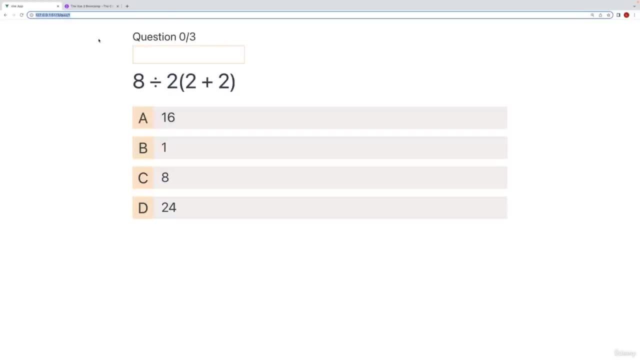 stuff this routing stuff in tremendous detail so you don't have to worry about that right now 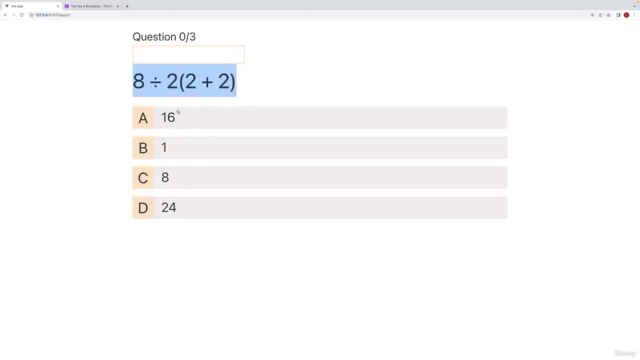 now over here we are greeted with our math quiz of course we can go ahead and we'll start answering the questions so let's say with this i'm gonna say let's say 24 for this i'm just gonna get some right some wrong uh let's just go over here and then this one this one i'll try to get right on purpose so 9 times 9 is or 3 times 3 is 9 divided by uh 3 is going to be 3 uh so 3 plus 3 minus 3 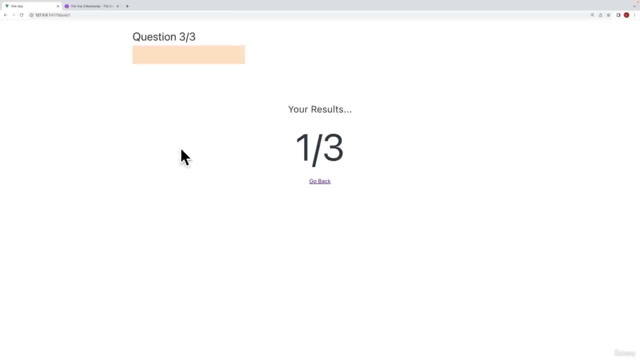 is going to be 3 so right away we get this really cool animation as you can see here we're going to learn how we can do that natively with view and then we get our results which is we got one right out of three and then we can actually go back and we can pick another one now let's try to get a little bit more right this time 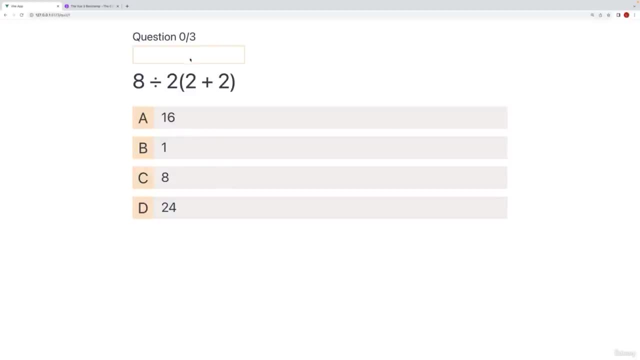 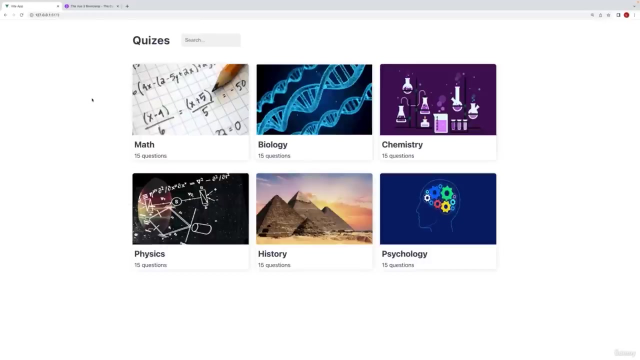 so let's just say this time uh this i believe is 16 this uh let's just say 21 this one's three there we go now we got two out of three right and you guys get the point so this is what we are eventually going to build and there's going to be a ton a ton of different things that we are going to learn when it comes to view so let's get started in order to get this out of the way we're going to need to get this out of the way we're going to need to get this 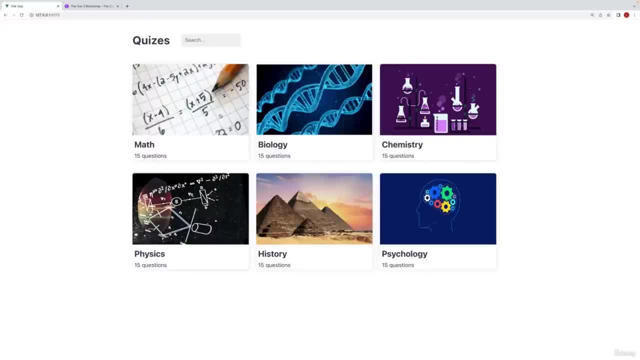 application up and running we're going to need to unfortunately write a lot of html as well as 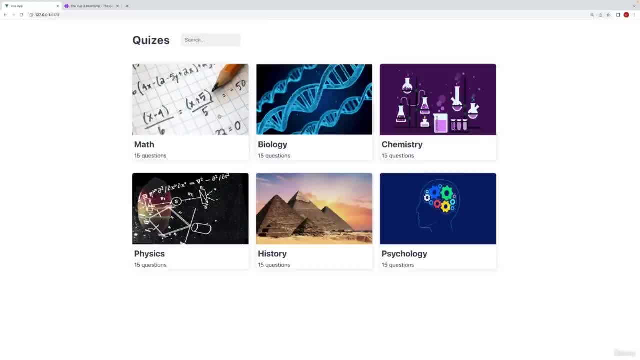 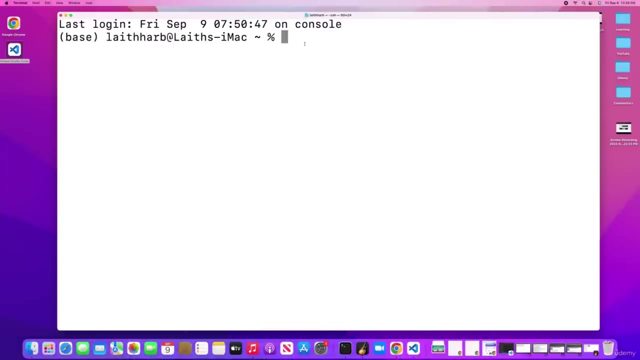 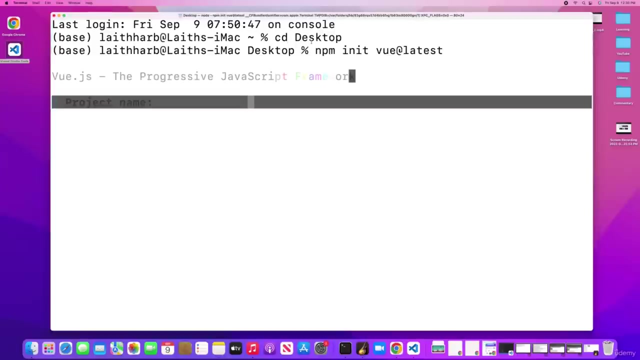 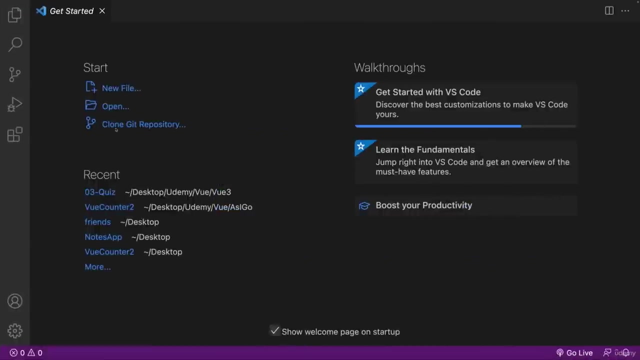 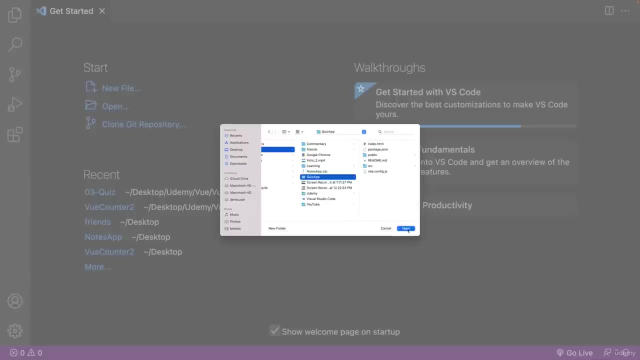 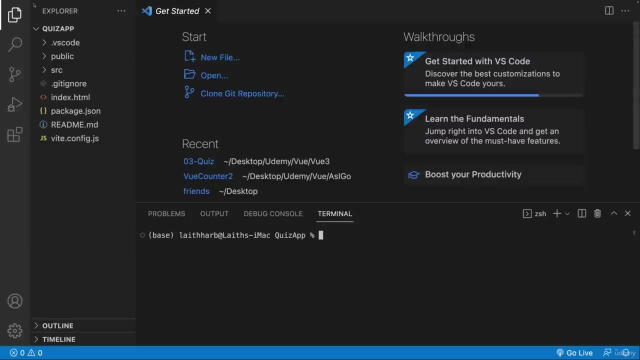 css so what we're going to do is kind of similar to what we did in the last section with the previous project if this is something that you are interested in writing and coding along with me feel free to continue watching this video because in this video we're just going to build the html and css for this web page right over here however if this is something that you're going to want to watch and you want to skip right to the view feel free to download the boilerplate code that is attached to this video skip this video and move on both options are completely fine it just depends on what you prefer so well here's your chance do what you got to do so now what we're going to first do is create our view application so let's open up our terminal and i'm going to move into the desktop and then in the desktop i'm going to go to the desktop and i'm going to run an npm init view at latest so that's just going to create a new project i'm going to call this quiz quiz app package name nothing we'll just say nothing for everything else and now what we're going to do is open this up inside of vs code so let's go here let's open this up go to desktop let's go to quiz app and let's go here and let's go to the desktop and let's go to our terminal and what we're going to do now is just the very simple well first let's zoom in a little bit 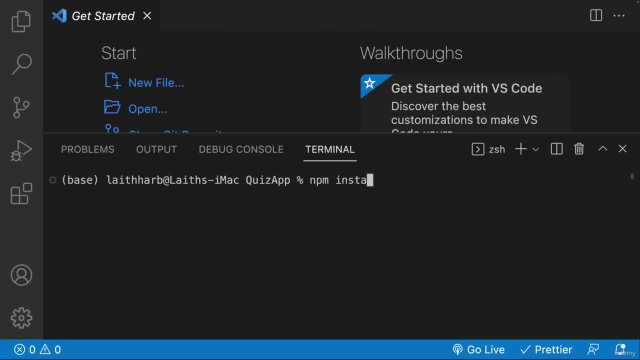 that's too much that's good let's do npm install to install all the dependencies and then we're going to do an npm run dev in order to spin up our development server 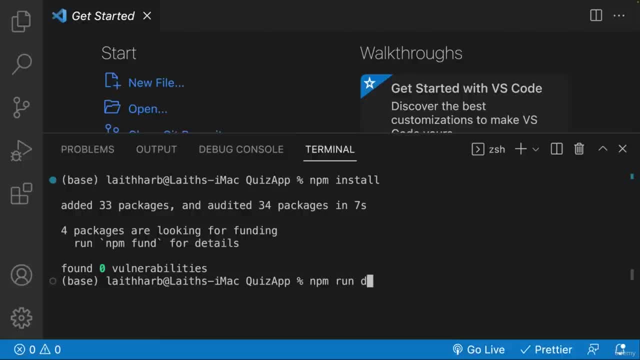 all right so now that we got that up and running for me it's running on localhost 5000 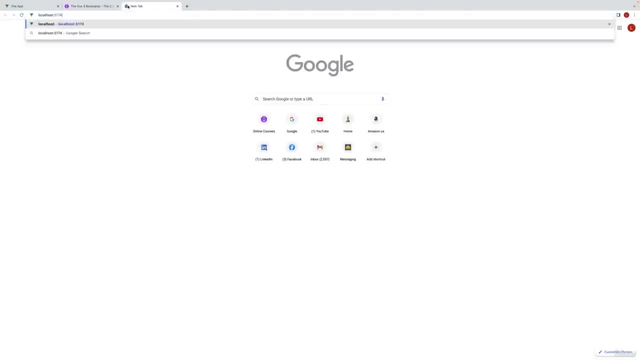 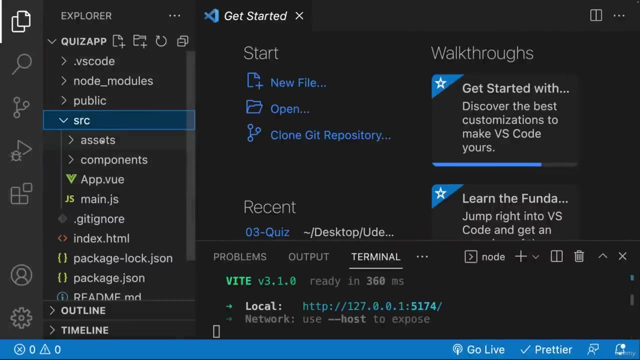 at 154 or 74 rather and there we go we got our view application so what we're going to do first is we are going to go to our main.css just remove all of these styles right here except for the 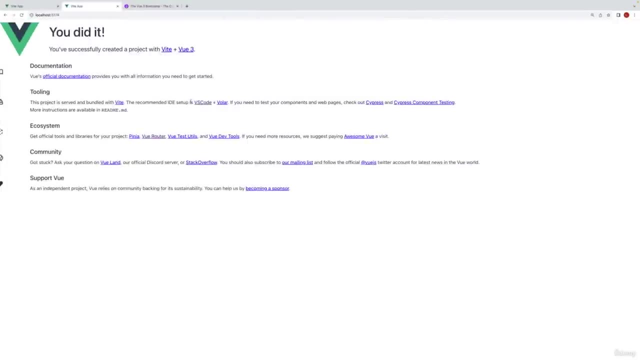 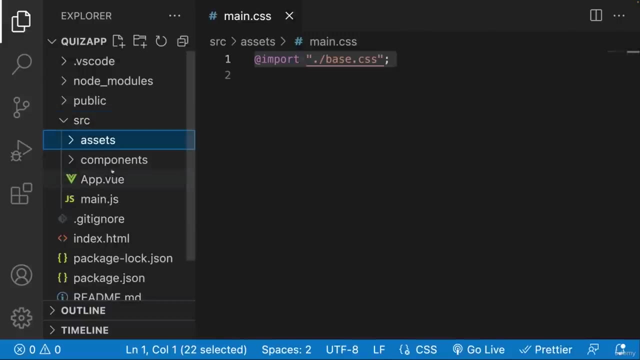 import the import has just some fonts that i i prefer to use over just kind of the regular regular fonts that we used so now that we got that let's actually do a little bit more cleanup 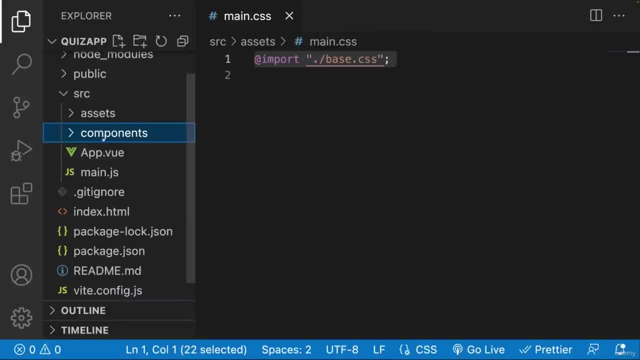 so this components directory and we'll actually talk about components in this project but for now let's delete it 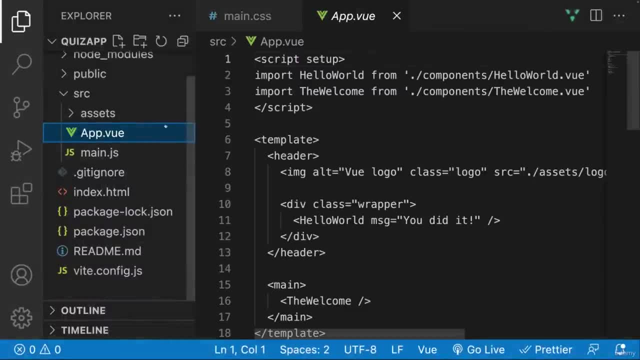 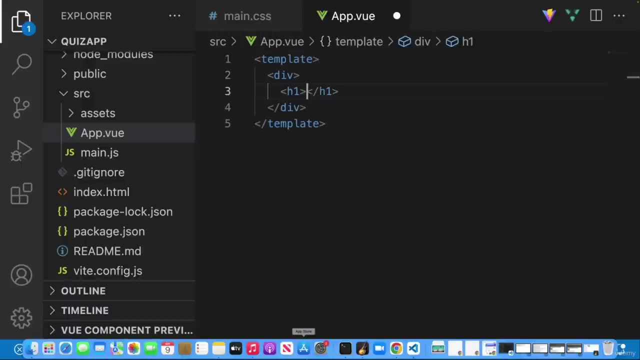 completely get rid of it and inside of the app.view let's completely get rid of it as well let's just add a template with a div and then this has a hello in there all right so there we go so 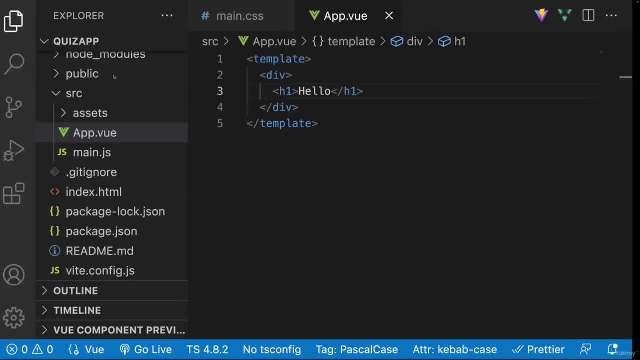 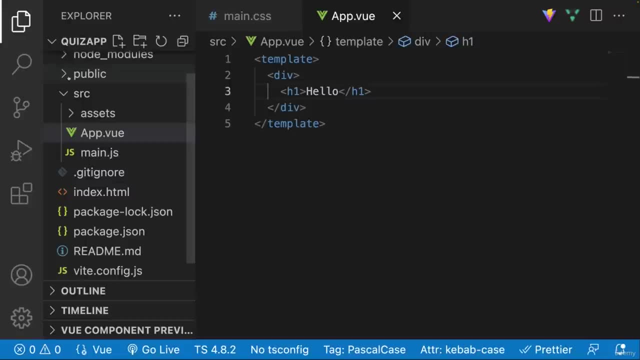 that's really all it is that we need so now all we have to do is very simply just code out the html and the css of our application 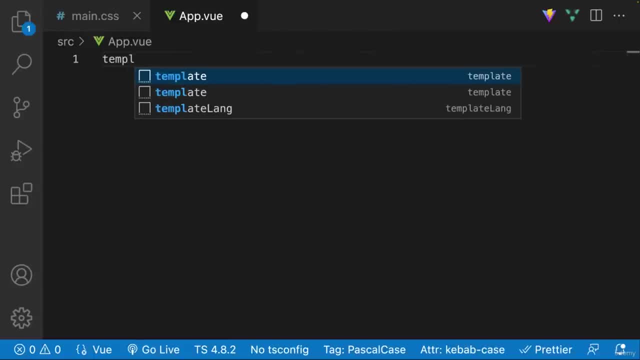 let's go over here and if you want to follow along continue and again if you don't want to follow along 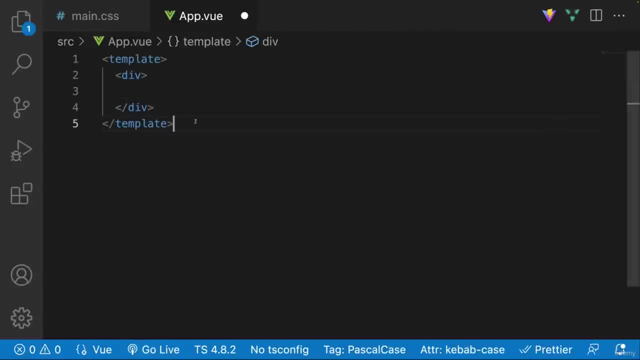 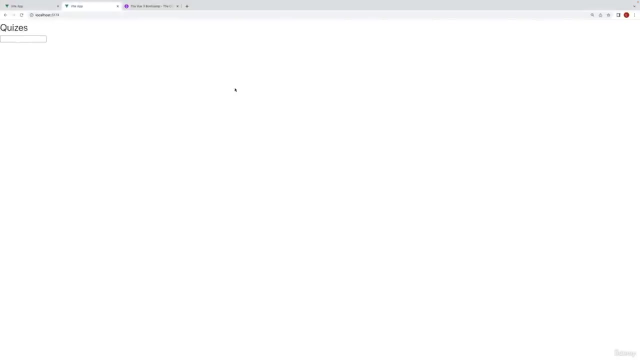 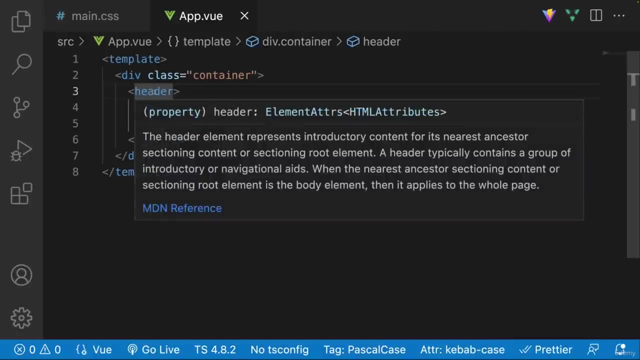 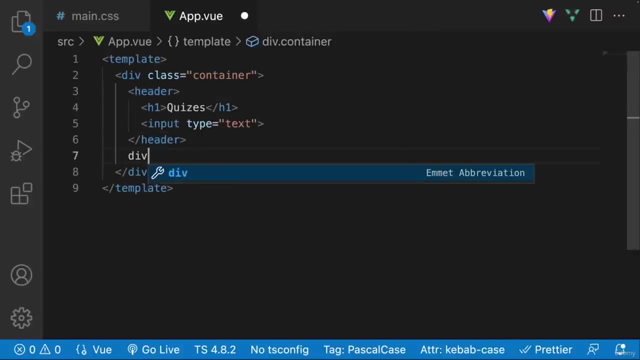 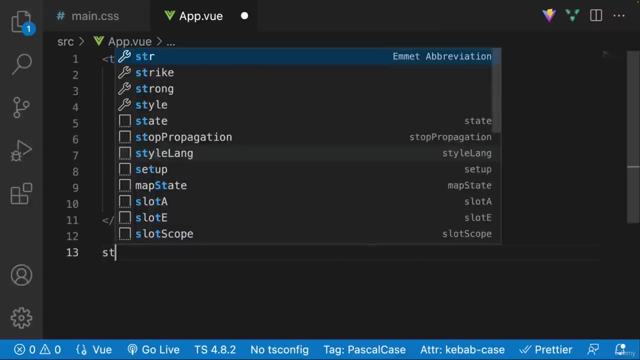 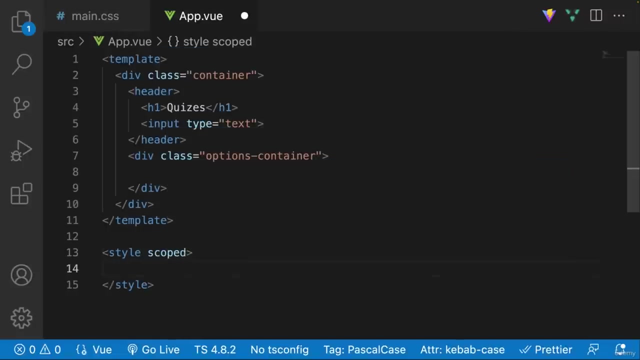 completely fine you can just skip this because i'm not really going to be explaining what i'm doing i'm just going to be writing the html as well as the css all right so the first thing i'm going to do is i am going to create a div give it a class of container and then what i'm going to do is i'm going to add a header and then within this header we're going to have a quizzes always use the w here a quiz is a and we're also going to have an input and this input will just leave as is it's going to be a text so kind of similar to what we had before so now we have the or it's not really refreshing oh let me save there we go we got quizzes we got the input not looking great well but that's because we need some styles and we'll style it a little bit later so now that we got that out of the way now what i'm going to do is i'm going to create a div and i'm going to give this div a class of container class of options container so options container and this is just going to house all of the different cards so it's just going to be our kind of our cards container we can also call it cards container whatever it doesn't matter now let's go ahead and actually style we'll add the cards html a little bit later so let's add some styles now so i'm going to say scoped and let's first style our container we're going to give this a max width of 1000 pixels and we're going to also give it a margin zero auto and there we go so we got it nice 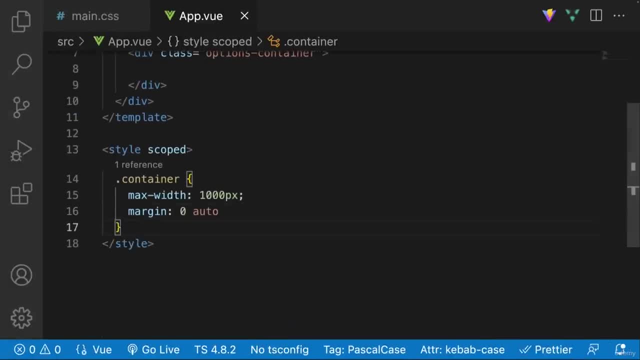 and kind of centered now let's style our header so i'm going to say header and over here we're going to say margin bottom and this is going to be 10 pixels and we're going to say margin top also 10 pixels 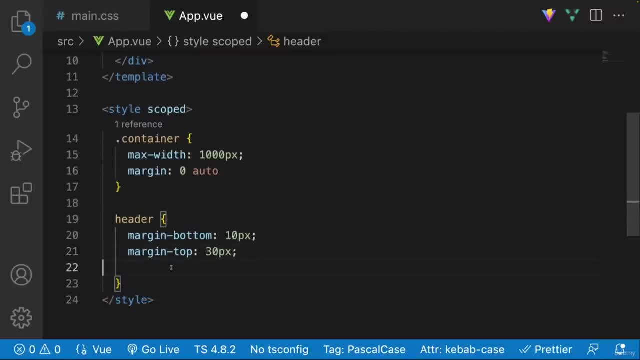 or rather actually we'll do 30 pixels for margin top and then we'll do display flex and then align items of center there we go looking pretty decent now so now let's style the h1 so we're going to 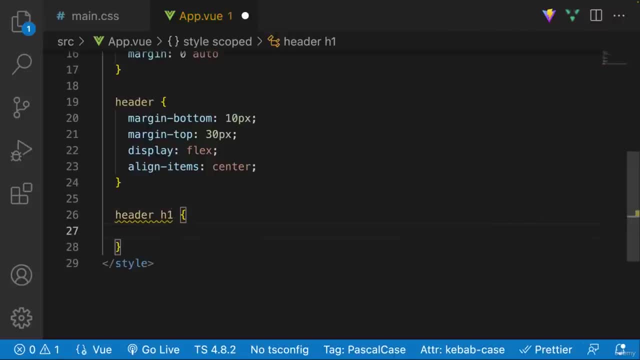 say header h1 and we're going to say font weight of bold and then we're going to say margin right 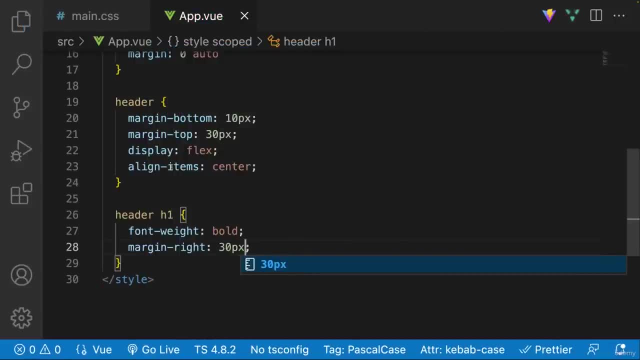 of 30 pixels something like that 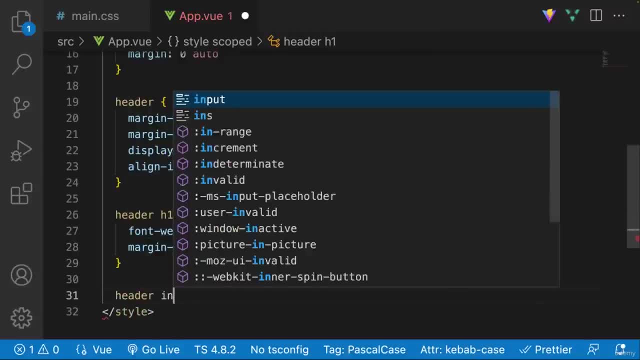 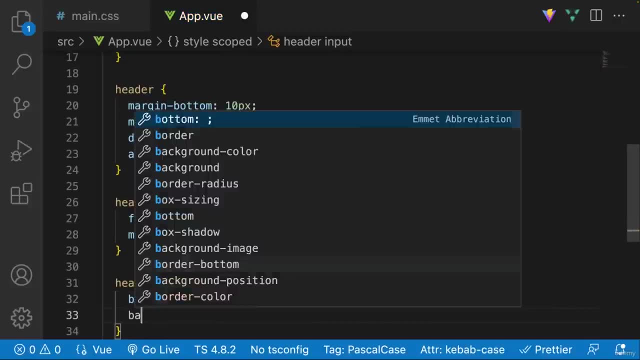 the last thing we need to style within the header is the input so let's go over here let's add some styles for the input we'll say a border of none and we'll say background color 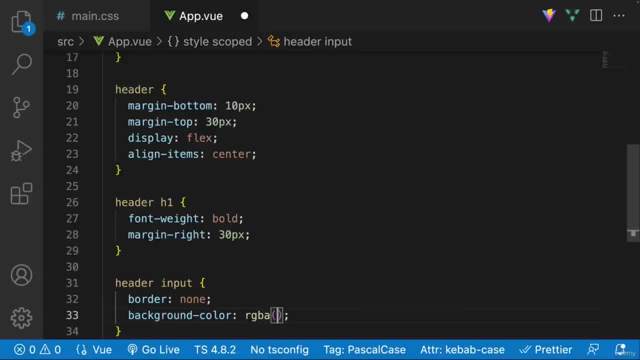 of rgba and we're going to say 128 128 128 and then 0.1 for the opacity and then we're going to have some padding just to make it look like we're going to have a bit of a 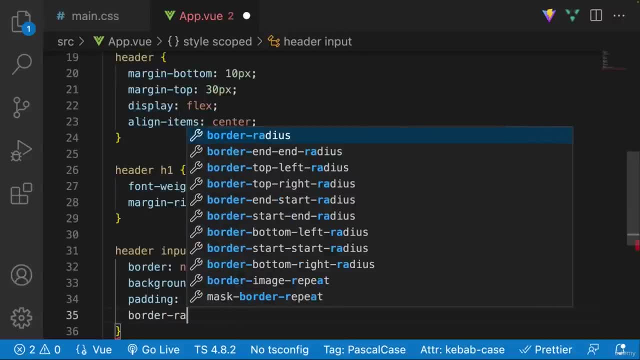 it nice and big 10 pixels and lastly a border radius of five pixels let's go ahead and save 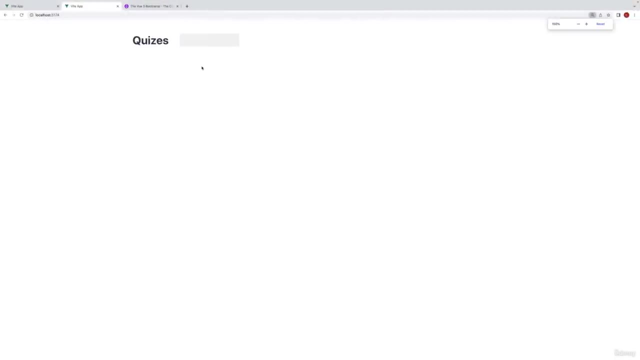 that and there we go this is looking pretty decent to me now again if this is too small or too big 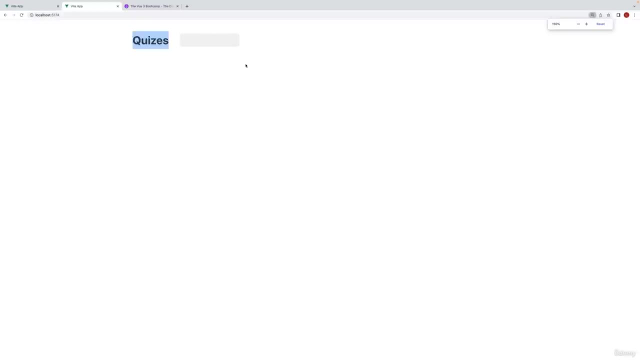 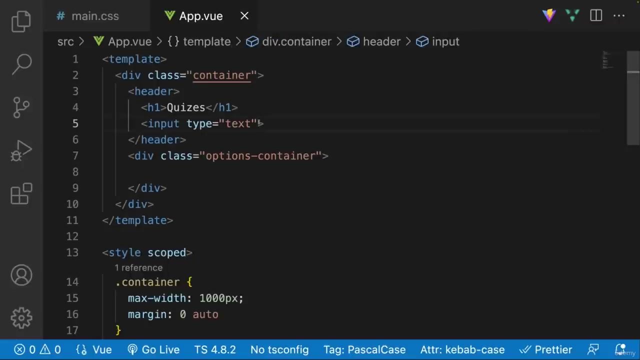 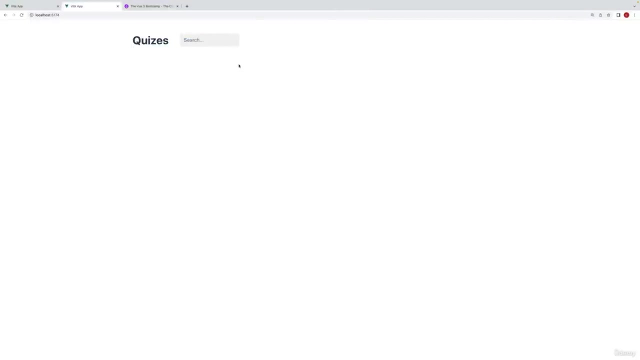 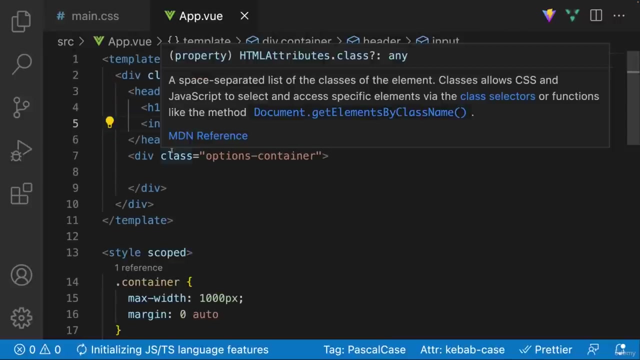 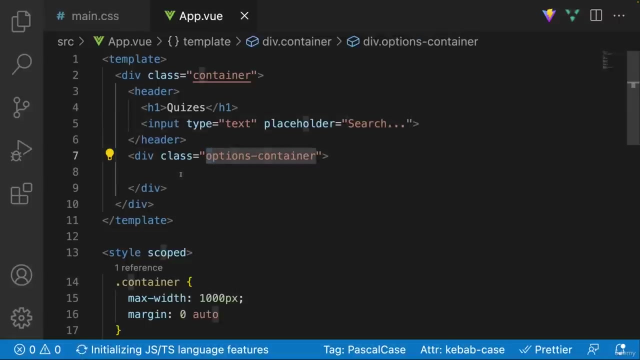 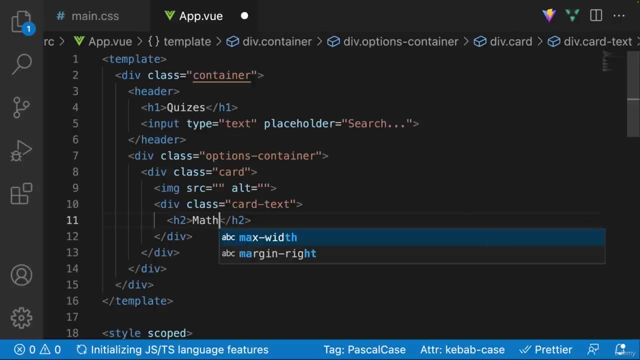 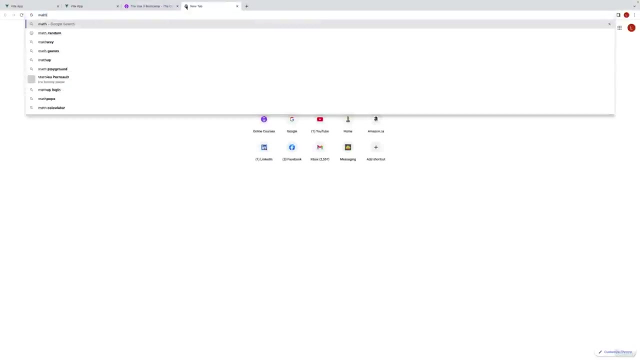 it's not a css course you can adjust it or you can zoom in or zoom out do whatever it is that you feel is best okay so now what i'm going to do is actually go to here and i'm going to add a placeholder because i think the placeholder is really important so we're going to say placeholder we're going to say dot dot dot so search dot dot dot okay so that's looking pretty decent in my opinion now what we actually need to style and actually write the html for are the cards so let's go ahead and actually write the html for the cards themselves and this should be pretty simple i'll just create one card for now so we're going to say div and we're going to give this let's just do it like this so styles of card and then we're also going to have an image within this and we're also going to have another div that's going to have card text and this is going to have an h2 and that's going to be whatever the text is let's just say math for now and we're going to have another paragraph tag and it's going to tell you how much questions are in the quiz for now we'll just hard code 15 questions all right so let's actually just grab something from the internet let's just just search for math and let's just grab some sort of image from the internet I like this one whatever 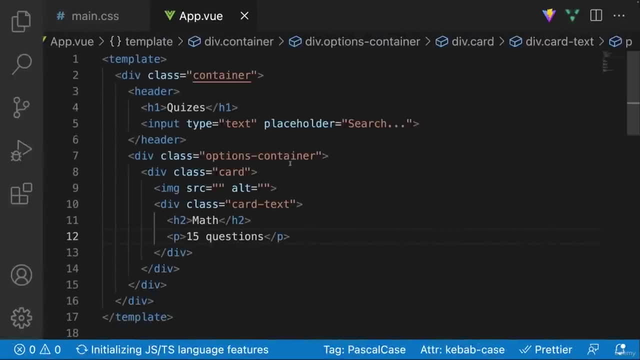 let's just copy the image address and let us go over here and let's just paste that in there so 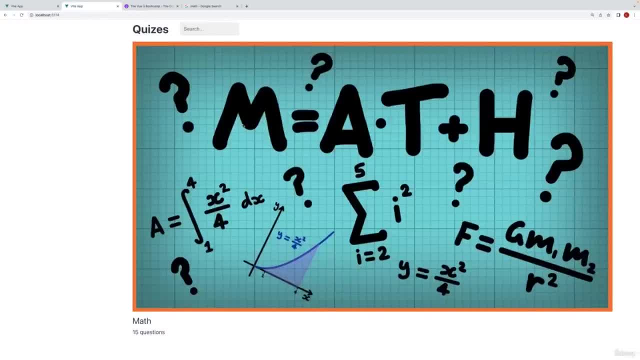 we can have some sort of image so now we have this really uh gross looking card let's 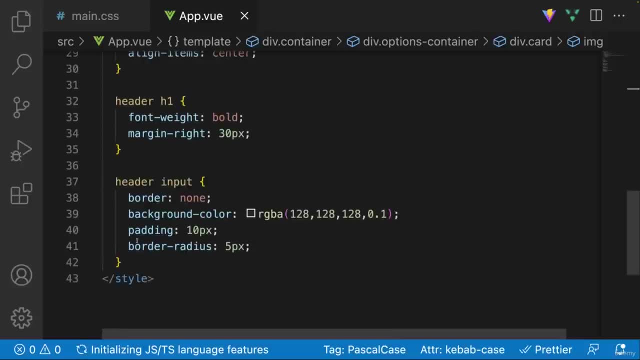 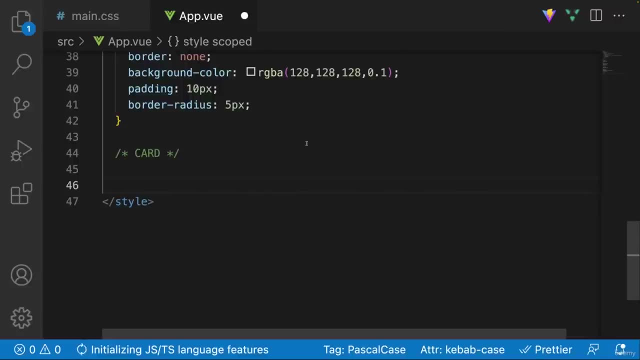 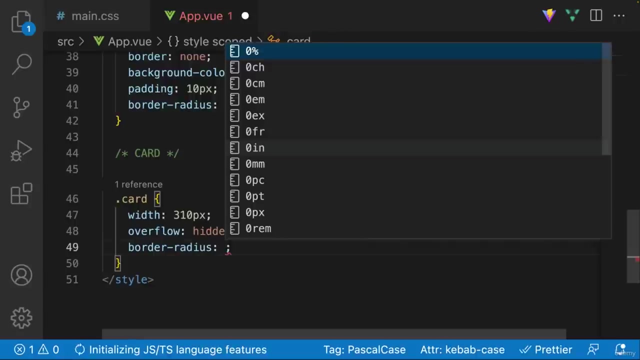 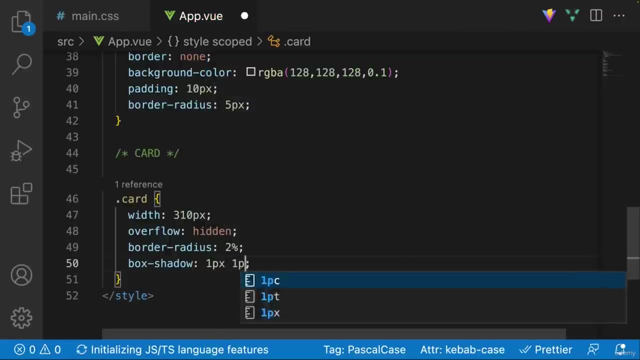 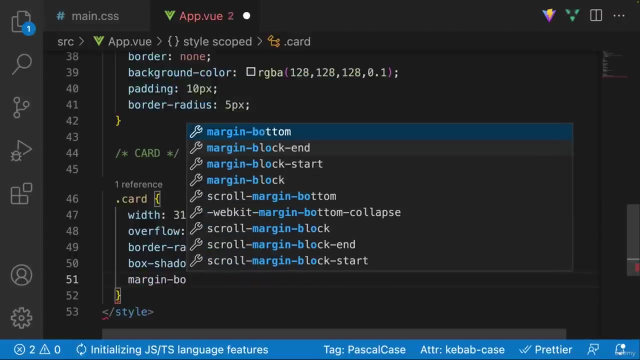 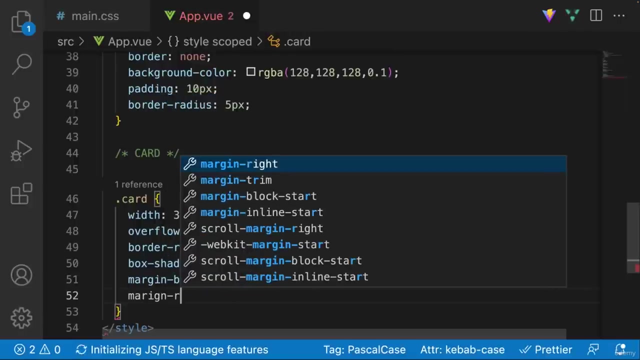 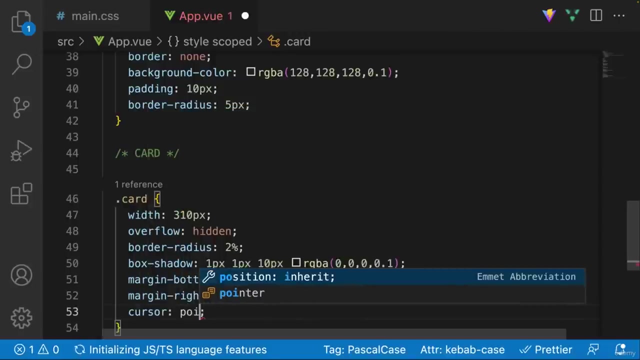 go ahead and style it so let's go over here i'm going to leave just a comment just saying that this is the card that we're styling so anything below is going to be the card and we'll you'll see later on so let's first style the uh card container so i'm going to give this a width of 110 pixels we're going to give it an overflow of hidden we're also going to give it a border radius of let's say two percent and then we're gonna say box shadow we're gonna say one pixel one pixel we're gonna say 10 pixels and then rgba i'm gonna say zero zero zero and then 0.1 so we can make it nice and uh looking like a shadow basically let's say margin bottom i will say 35 pixels uh margin right we will say 20 pixels and lastly cursor pointer because we're going to want to eventually click on it so might as well tell people that hey this is clickable all right so this is looking pretty decent uh obviously there's still quite a bit more let's also style the image because that's obviously making everything really bad right now 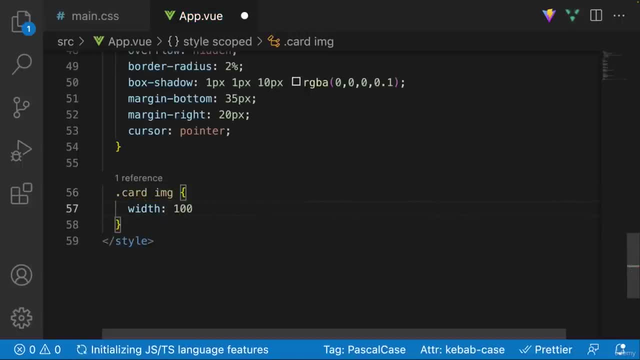 let's give it a width of 100 percent and that should kind of fix that we'll also give it a 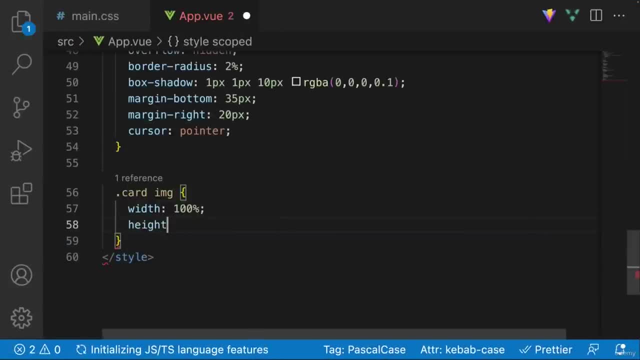 a height so we'll give it a height of 190 pixels and we'll also give it a margin of nothing zero so so it has no margins all right so this is looking pretty great right now 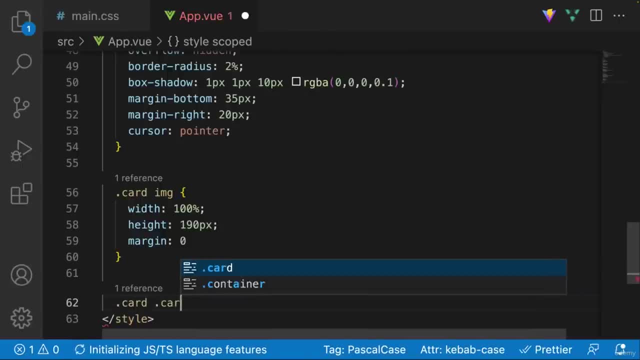 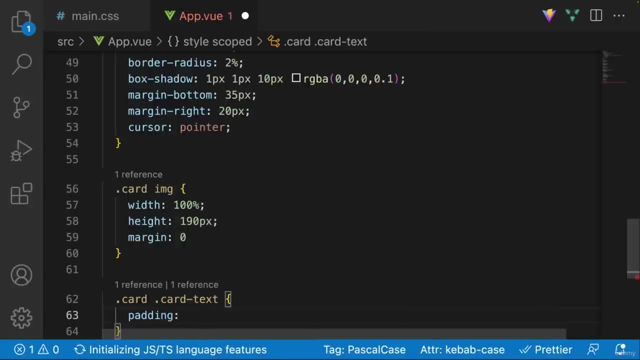 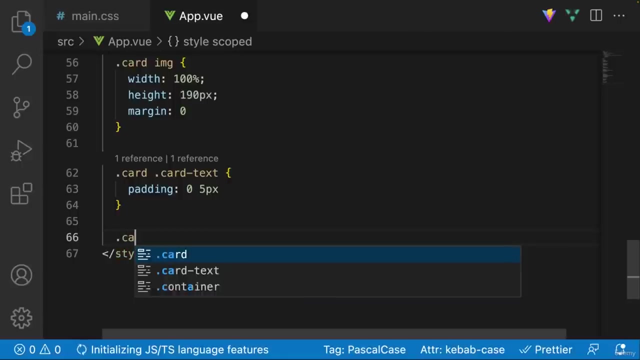 the other things that we need to style of course are the card text so let's say card text we're going to say padding of zero and then five pixels so we can have some padding on the the right and the left and then we also want to style the h2 so 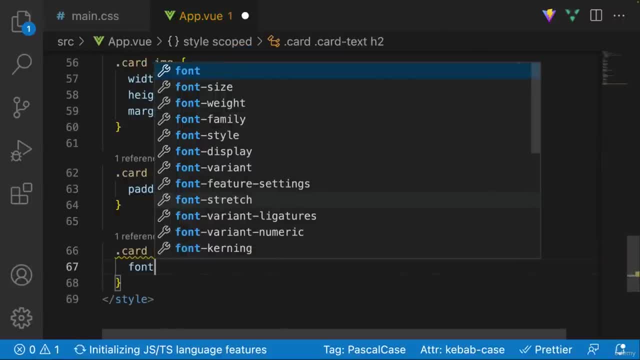 let's style that h2 we're going to say font weight of bold 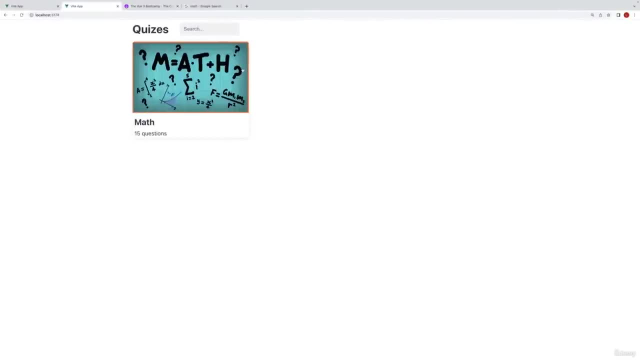 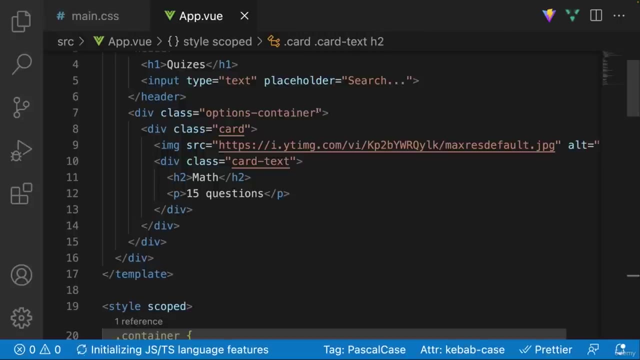 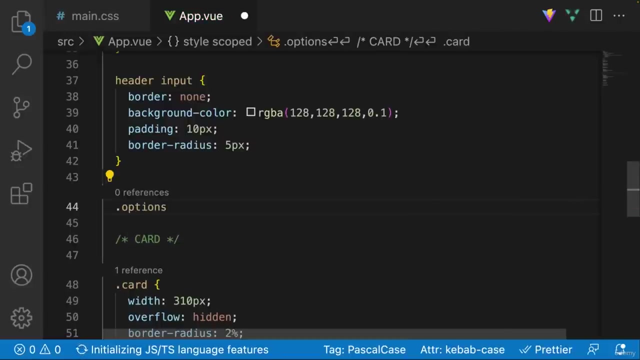 so that's pretty much actually it for it all we now need to do is just add a little bit of styling for the options container so the options container let us we'll keep it here for now above the card because it's not really card stuff or i guess it is card related but it's fine we can just keep it on top 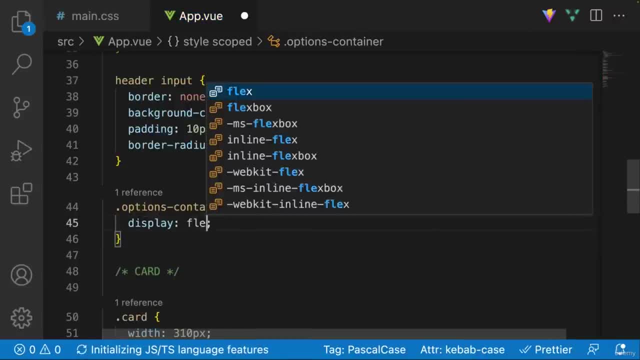 so we're going to say display flex for this and we're also going to say flex wrap and we're going to say wrap and lastly we're going to give this a margin top 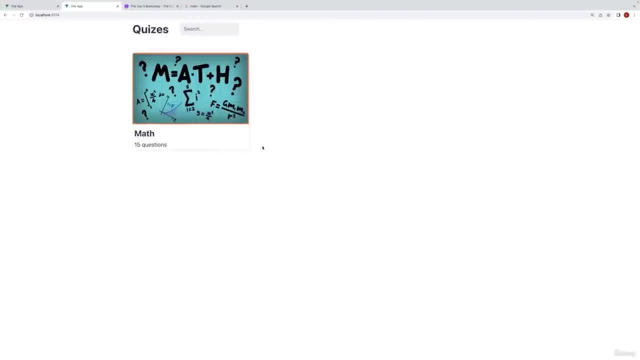 of 40 pixels and that's it so we have completely styled at least the front application so now we can actually start working on this functionality and then we can move on to the other functionalities later 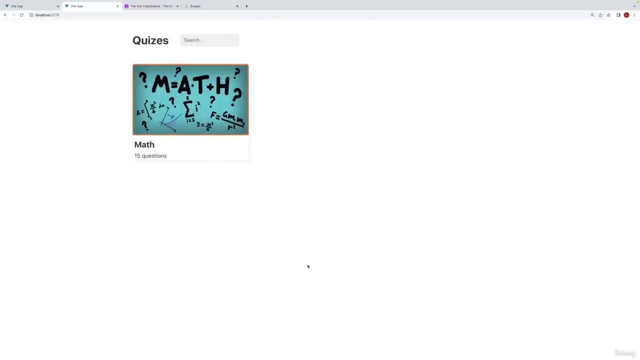 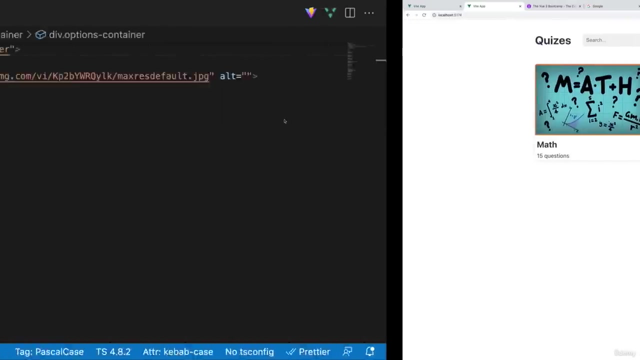 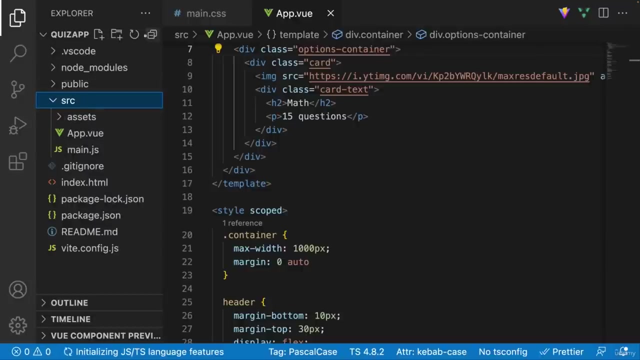 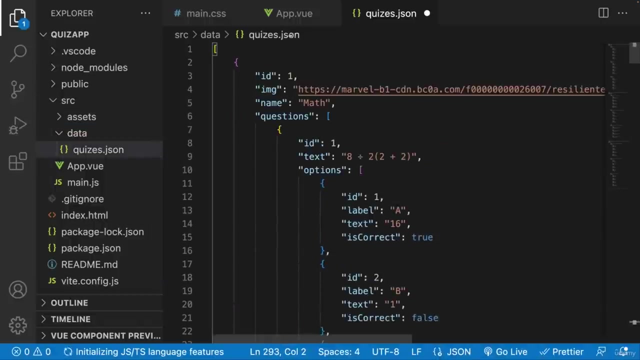 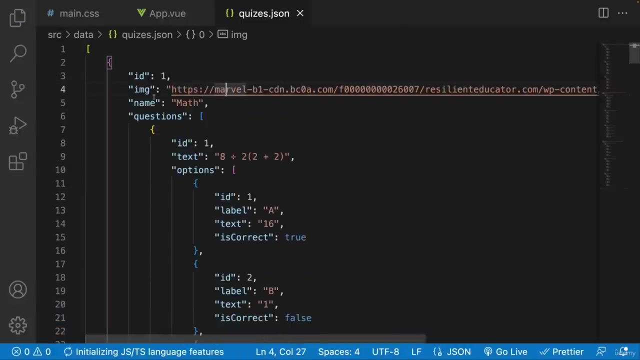 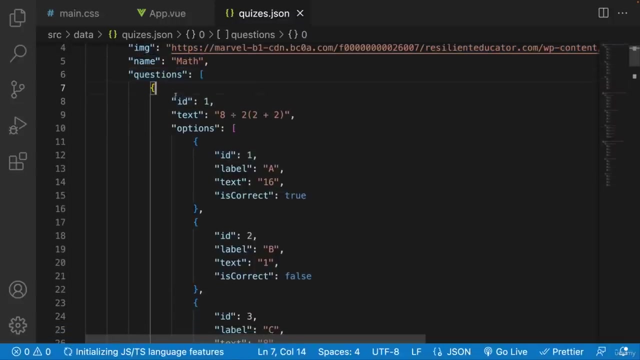 all right my good friends the first thing that i actually want to do is i want to start rendering our cards now of course to render our cards we're going to need some card data so attached to this lecture i have a json file that is going to contain all of the data so go ahead and download it and place it inside directory actually what we're going to do is we're going to create inside of the source directory a data directory and then within this data directory we can have our quizzes dot JSON file again for you you're just gonna have to download it and put it inside of this data directory or honestly wherever it is that you want so let's go ahead and well this I'm gonna go ahead and paste it for you again it should be there but this data should look something like this so JSON is well very similar to JavaScript objects so we have an array of objects each object has an ID it has an image it has a name and then it has an array of questions and each array of question is going to be an object that has an ID the question itself with which is text and then an array of other objects but these ones are options each option is going to have an ID label text 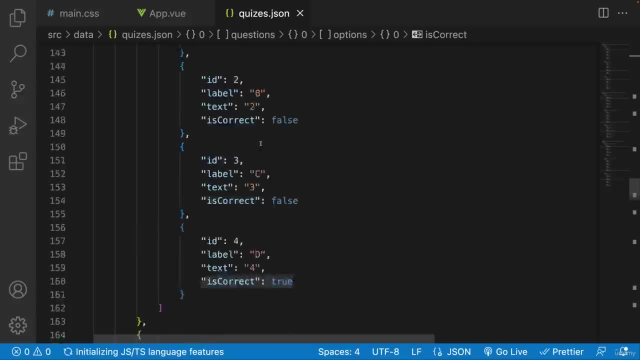 and an is correct value now we should have an array of other objects but these ones are options each option is going to have three different quizzes here but for now let's not worry about this if 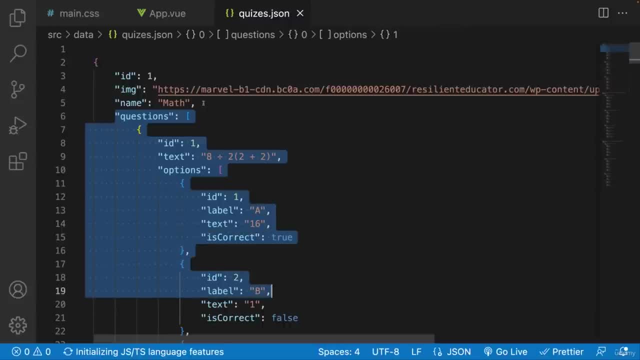 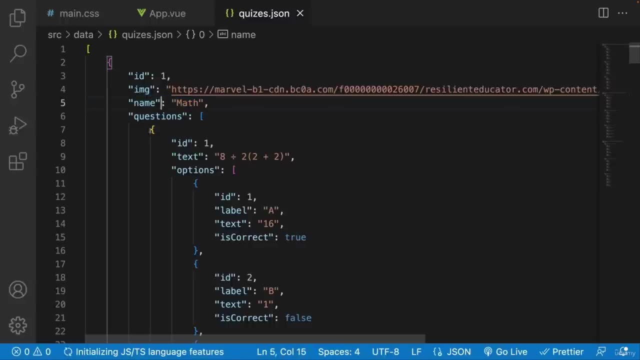 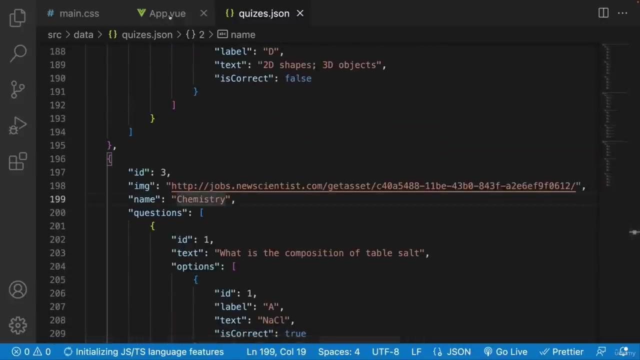 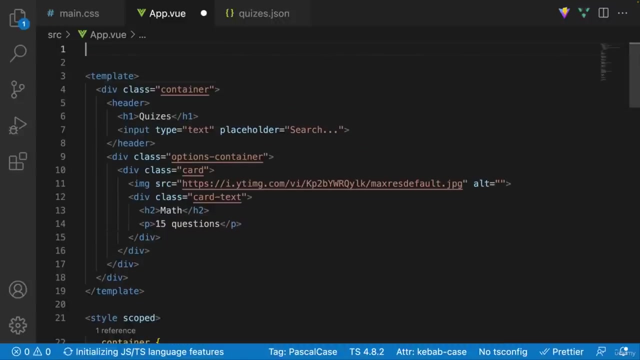 this is a little bit confusing to you this data is a little confusing to you let's not worry about that all we really have to worry about right now is the image and the name in order to render our cards so we have the math quiz and if I go all the way down we also have a biology quiz and if I go all the way down we also have a chemistry quiz so the first thing that I am going to do is we're gonna need to import that data so let's go over here and we're going to 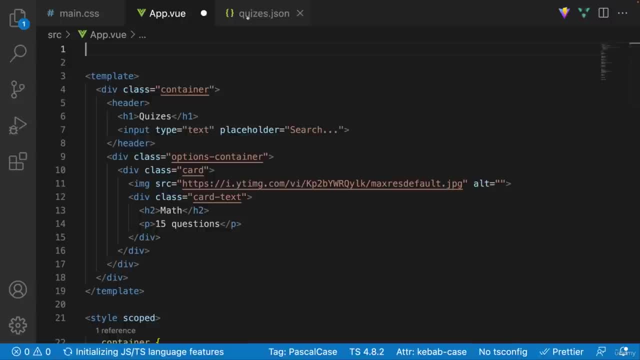 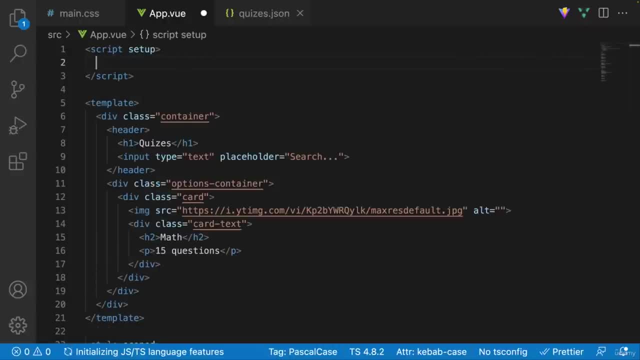 our script tags within it we're gonna our script tags within it we're gonna have our setup function and what I'm have our setup function and what I'm have our setup function and what I'm going to do is I am going to import and going to do is I am going to import and going to do is I am going to import and I'm gonna say import Q for like quizzes I'm gonna import Q for like quizzes I'm gonna import Q for like quizzes and then I'm gonna import that from and and then I'm gonna import that from and and then I'm gonna import that from and I'm gonna go the data directory so I'm I'm gonna go the data directory so I'm I'm gonna go the data directory so I'm gonna move to the data directory which gonna move to the data directory which gonna move to the data directory which is right here and then I'm gonna say is right here and then I'm gonna say 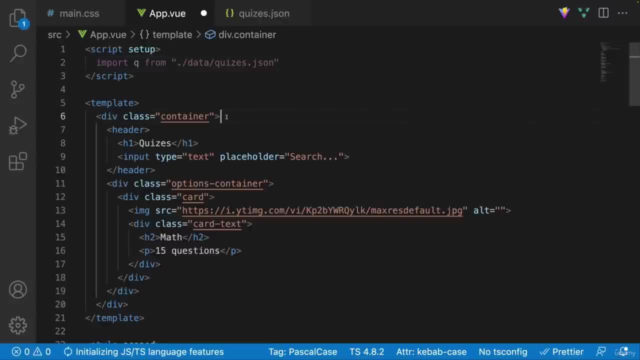 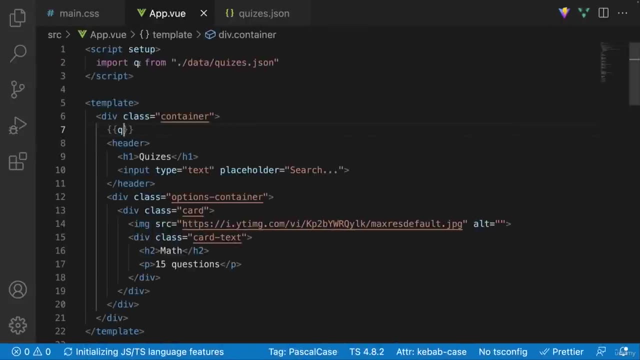 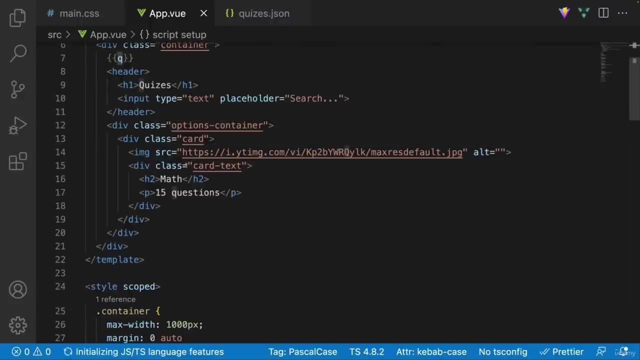 is right here and then I'm gonna say quizzes dot JSON and what this should do quizzes dot JSON and what this should do quizzes dot JSON and what this should do if I render for example Q here we should if I render for example Q here we should if I render for example Q here we should have our data now you might be thinking have our data now you might be thinking have our data now you might be thinking what we can do now is you can just use what we can do now is you can just use what we can do now is you can just use this Q right over here and do a v4 on it this Q right over here and do a v4 on it this Q right over here and do a v4 on it to render our cards and that would to render our cards and that would to render our cards and that would actually work a-okay but let's actually actually work a-okay but let's actually actually work a-okay but let's actually look at the final product remember in 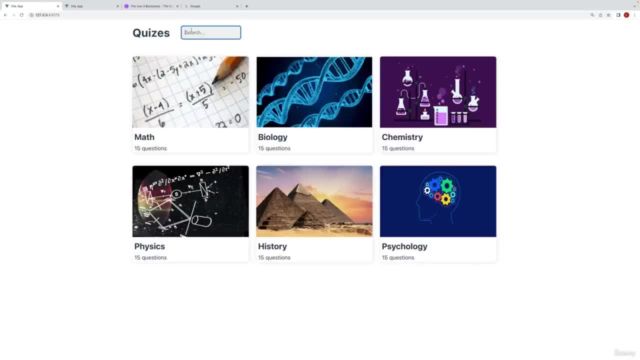 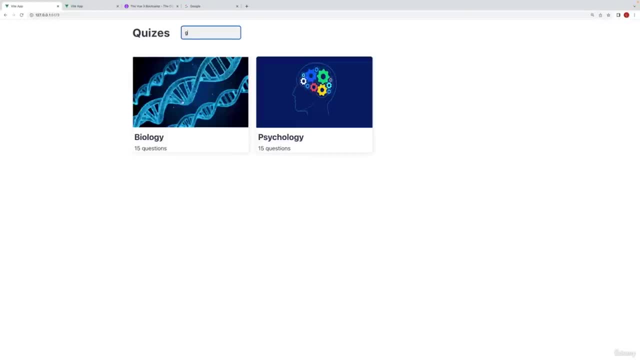 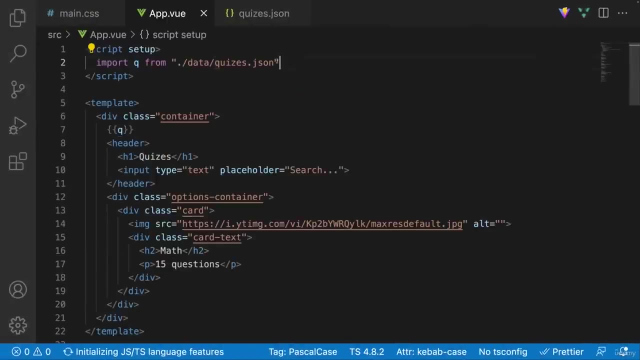 look at the final product remember in look at the final product remember in the final product we're going to have the final product we're going to have the final product we're going to have this search ability where we can search this search ability where we can search this search ability where we can search for specific cards and that is going to for specific cards and that is going to for specific cards and that is going to of course well change the state of our of course well change the state of our of course well change the state of our application and show the cards that application and show the cards that application and show the cards that match this search so we cannot really match this search so we cannot really match this search so we cannot really reasonably have our variable like this reasonably have our variable like this 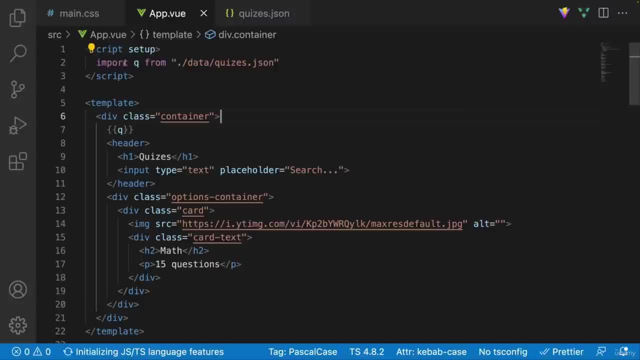 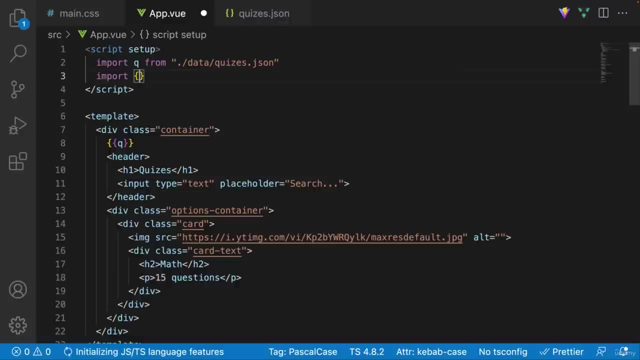 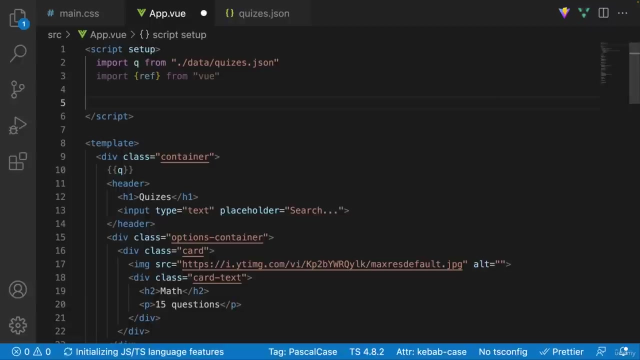 reasonably have our variable like this we actually have to store it inside of we actually have to store it inside of we actually have to store it inside of some sort of state and that's why I some sort of state and that's why I some sort of state and that's why I called it Q because later on we are called it Q because later on we are called it Q because later on we are going to create some state that is gonna going to create some state that is gonna going to create some state that is gonna be called quizzes so let's go ahead and be called quizzes so let's go ahead and be called quizzes so let's go ahead and actually import ref now from view and actually import ref now from view and actually import ref now from view and what we're gonna do here is we're gonna what we're gonna do here is we're gonna what we're gonna do here is we're gonna create a piece of state called quizzes 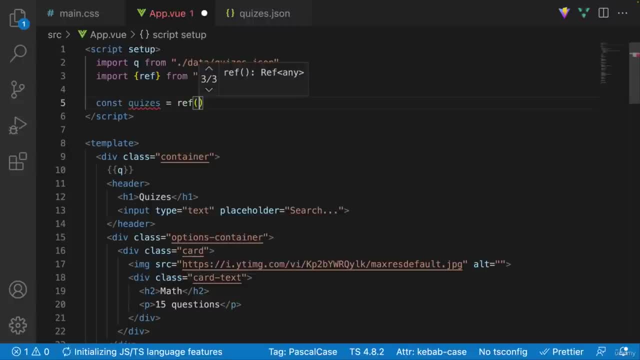 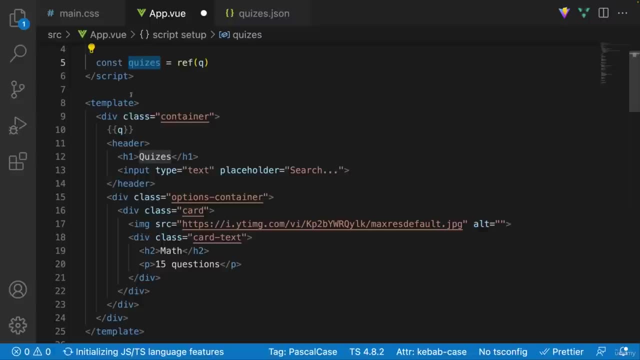 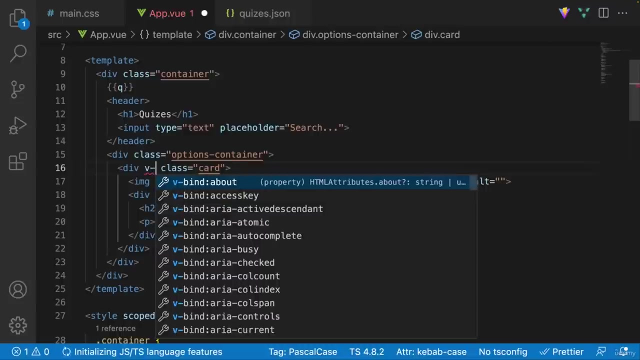 create a piece of state called quizzes create a piece of state called quizzes and that's gonna be equal to ref and I'm and that's gonna be equal to ref and I'm and that's gonna be equal to ref and I'm gonna say Q like so alright so now what gonna say Q like so alright so now what gonna say Q like so alright so now what we can do is we can utilize this and we can do is we can utilize this and we can do is we can utilize this and iterate over it and render some HTML iterate over it and render some HTML iterate over it and render some HTML specifically these cards right over here specifically these cards right over here specifically these cards right over here so let's go ahead and do that so we're so let's go ahead and do that so we're so let's go ahead and do that so we're gonna add a v4 we're gonna say for quiz gonna add a v4 we're gonna say for quiz 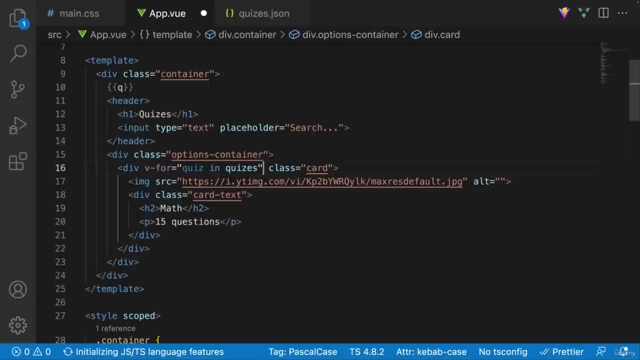 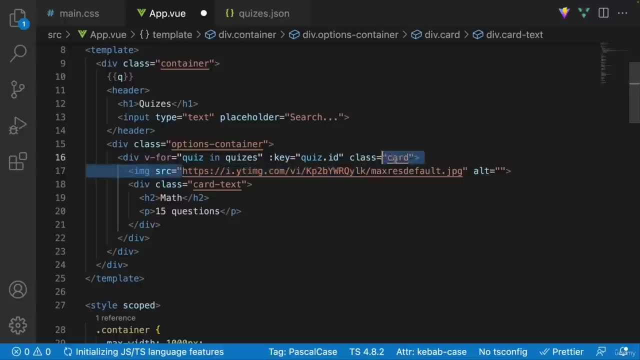 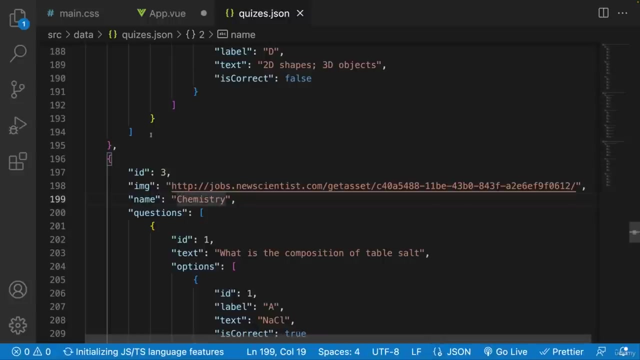 gonna add a v4 we're gonna say for quiz in quizzes and let's also supply it with in quizzes and let's also supply it with in quizzes and let's also supply it with a key right away that's gonna be quiz a key right away that's gonna be quiz a key right away that's gonna be quiz ID so over here you can see that the ID so over here you can see that the ID so over here you can see that the source is a string what we want to do is source is a string what we want to do is source is a string what we want to do is we want to change this to a we want to we want to change this to a we want to we want to change this to a we want to change this to JavaScript so that we can change this to JavaScript so that we can change this to JavaScript so that we can do something like quiz dots and if you do something like quiz dots and if you do something like quiz dots and if you go to the JSON file it's quiz dot image 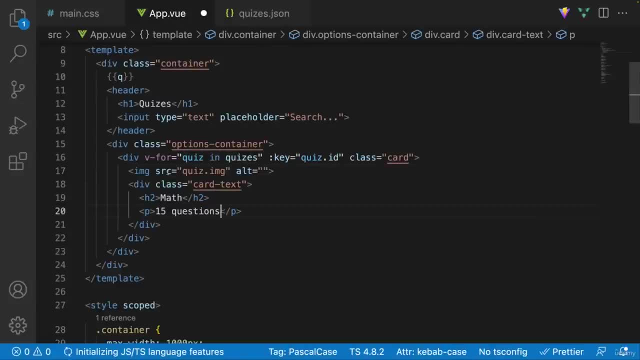 go to the JSON file it's quiz dot image go to the JSON file it's quiz dot image like so so quiz dot image like that so of like so so quiz dot image like that so of 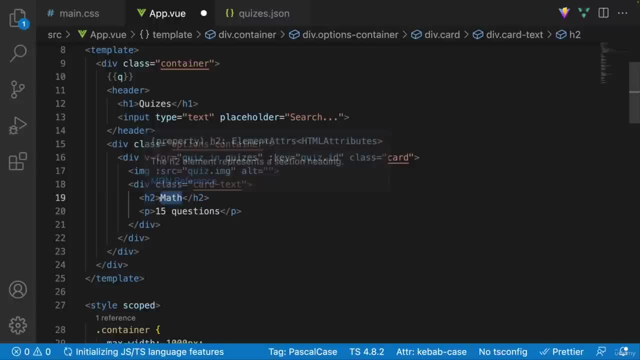 like so so quiz dot image like that so of course we're gonna make this JavaScript course we're gonna make this JavaScript course we're gonna make this JavaScript okay so over here we're also going to okay so over here we're also going to okay so over here we're also going to add those curly braces and we're gonna add those curly braces and we're gonna add those curly braces and we're gonna say quiz dot name and lastly here we can say quiz dot name and lastly here we can 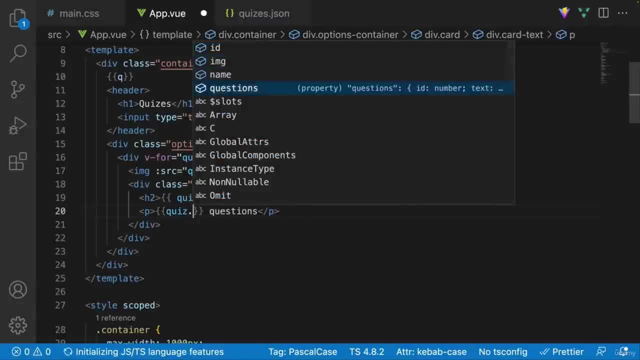 say quiz dot name and lastly here we can change this to quiz dot and then change this to quiz dot and then change this to quiz dot and then questions dot length so that should be questions dot length so that should be 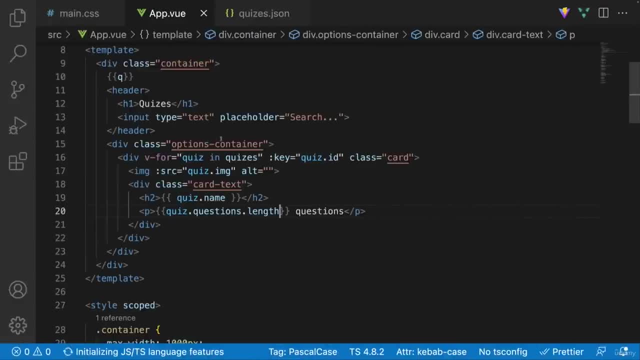 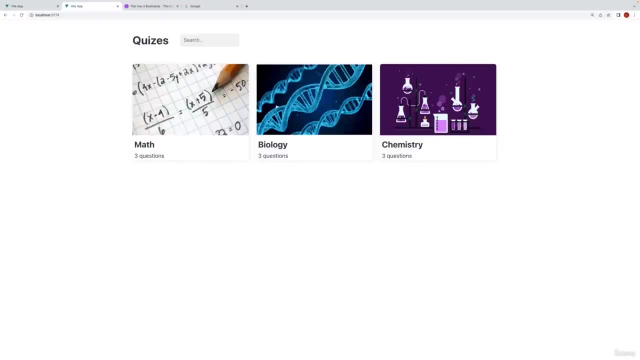 questions dot length so that should be it and if I were to refresh and let's it and if I were to refresh and let's it and if I were to refresh and let's get rid of this queue over here you can get rid of this queue over here you can get rid of this queue over here you can see we get our wonderful quizzes and see we get our wonderful quizzes and see we get our wonderful quizzes and each quiz has only three questions you each quiz has only three questions you each quiz has only three questions you can add more if you want but I actually can add more if you want but I actually can add more if you want but I actually have to write these questions from have to write these questions from have to write these questions from scratch and my well my chemistry and scratch and my well my chemistry and scratch and my well my chemistry and biology and math memory is very low so I 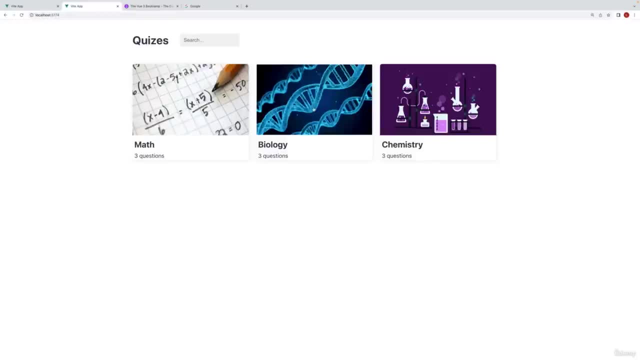 biology and math memory is very low so I biology and math memory is very low so I couldn't really come up with any more couldn't really come up with any more couldn't really come up with any more questions so there we go so now we are questions so there we go so now we are questions so there we go so now we are rendering our cards so we got our cards rendering our cards so we got our cards rendering our cards so we got our cards to render the next thing that we need to to render the next thing that we need to to render the next thing that we need to do is make our input functional so of do is make our input functional so of do is make our input functional so of course when I search for something it course when I search for something it course when I search for something it should filter the cards based on what I should filter the cards based on what I 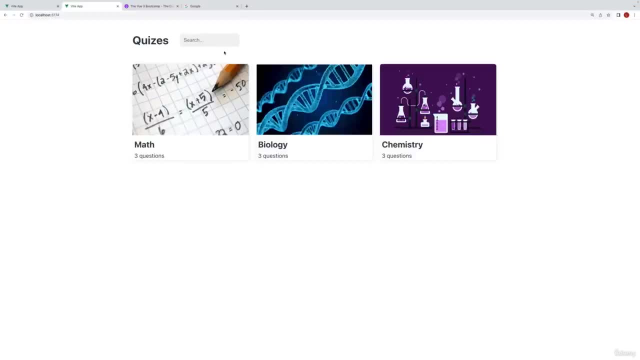 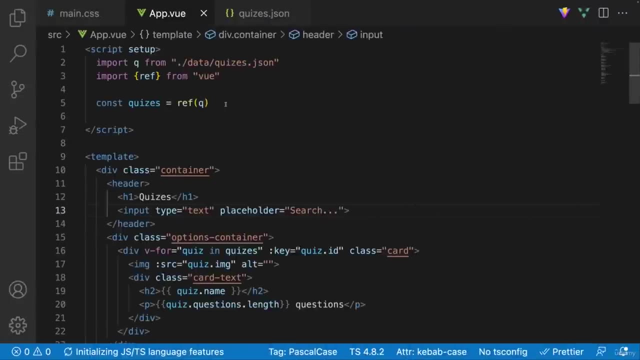 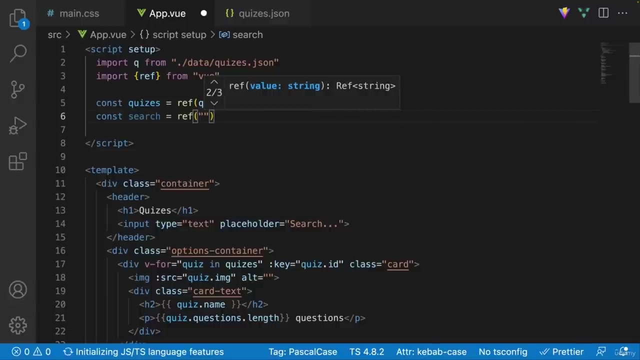 should filter the cards based on what I searched for now anytime that we're searched for now anytime that we're searched for now anytime that we're dealing with inputs or text areas we need dealing with inputs or text areas we need dealing with inputs or text areas we need to add two-way binding so let's just to add two-way binding so let's just to add two-way binding so let's just get that out of the way so we're gonna go get that out of the way so we're gonna go get that out of the way so we're gonna go over here and I'm gonna create a new over here and I'm gonna create a new over here and I'm gonna create a new piece of state with ref and I'm gonna piece of state with ref and I'm gonna piece of state with ref and I'm gonna call this just an empty string like so call this just an empty string like so call this just an empty string like so and then what I'm going to do is I'm 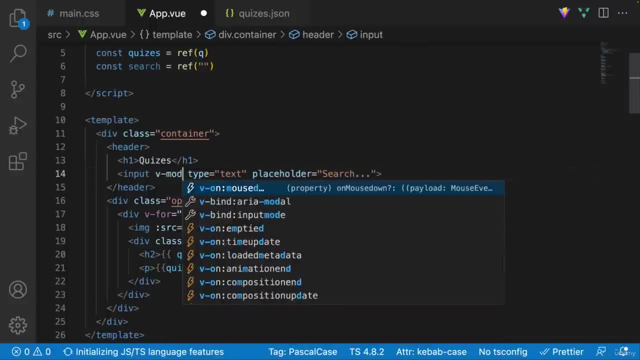 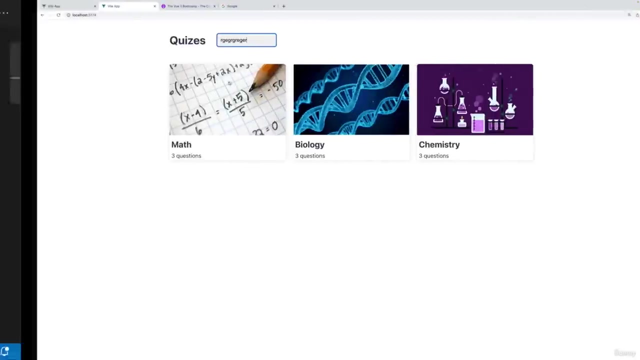 and then what I'm going to do is I'm and then what I'm going to do is I'm gonna go to this input and I'm gonna add gonna go to this input and I'm gonna add gonna go to this input and I'm gonna add the V model so we can have the two-way the V model so we can have the two-way the V model so we can have the two-way binding so I'm gonna say search and I'm binding so I'm gonna say search and I'm binding so I'm gonna say search and I'm actually also gonna add trim so we can actually also gonna add trim so we can actually also gonna add trim so we can trim any white spaces so there we go now trim any white spaces so there we go now trim any white spaces so there we go now we have our two-way binding anytime we we have our two-way binding anytime we we have our two-way binding anytime we make a change over here it is going to make a change over here it is going to make a change over here it is going to be reflective in our state okay so this be reflective in our state okay so this 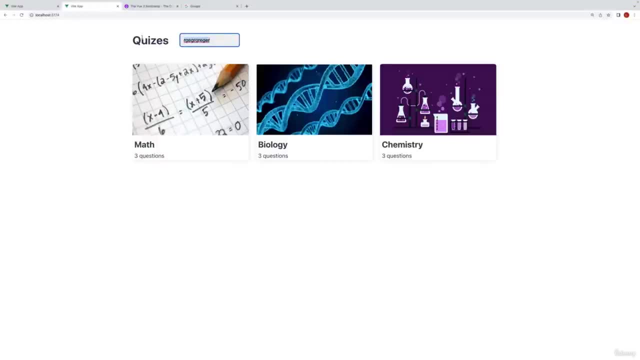 be reflective in our state okay so this is good so now let's actually make this is good so now let's actually make this is good so now let's actually make this completely functional so whenever I completely functional so whenever I 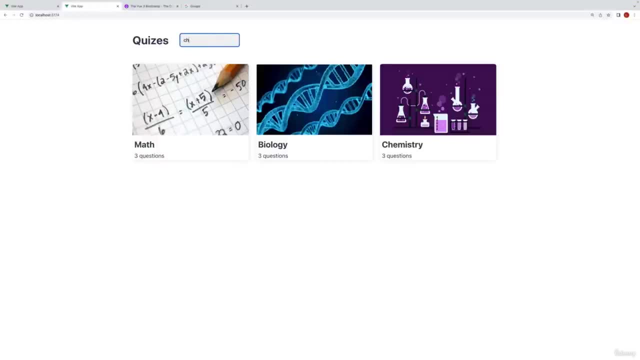 completely functional so whenever I search something so let's say I search I search something so let's say I search I search something so let's say I search I type in CH what should happen is it's type in CH what should happen is it's type in CH what should happen is it's going to look at all of the different going to look at all of the different going to look at all of the different quizzes their names specifically and sees quizzes their names specifically and sees quizzes their names specifically and sees that hey do they have a CH within 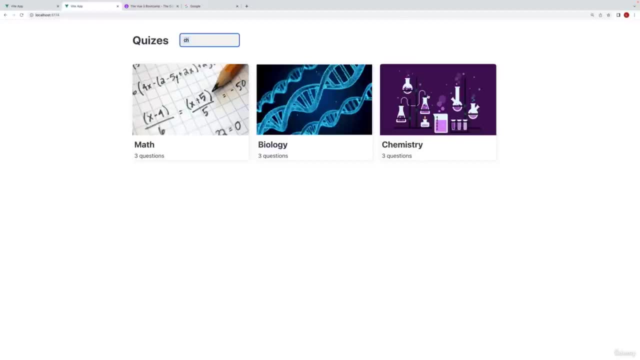 that hey do they have a CH within that hey do they have a CH within their name if they do have a CH it is their name if they do have a CH it is their name if they do have a CH it is going to include them but if they don't going to include them but if they don't going to include them but if they don't it's gonna completely remove them so it's gonna completely remove them so it's gonna completely remove them so over here if I had a CH it's only gonna over here if I had a CH it's only gonna over here if I had a CH it's only gonna show this card while it's not gonna show show this card while it's not gonna show show this card while it's not gonna show these other cards if for example I these other cards if for example I these other cards if for example I started off with an eye well it's not started off with an eye well it's not 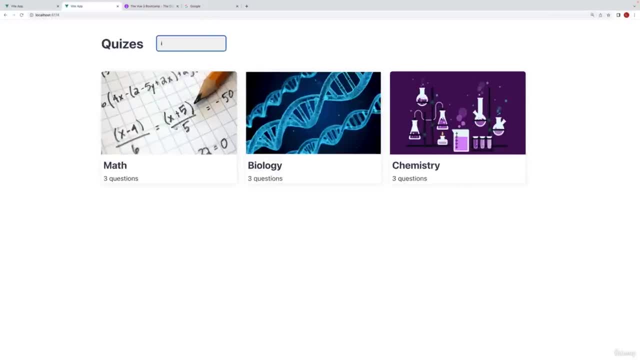 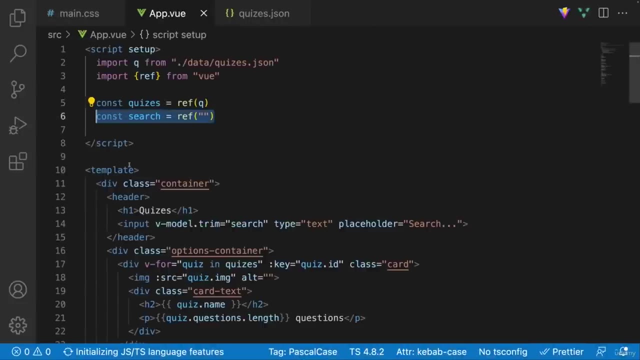 started off with an eye well it's not gonna include the math card and let me gonna include the math card and let me gonna include the math card and let me zoom in here it's not gonna include the zoom in here it's not gonna include the zoom in here it's not gonna include the math card but it's gonna include the math card but it's gonna include the math card but it's gonna include the biology card because because it has an biology card because because it has an biology card because because it has an eye and similarly chemistry has an eye eye and similarly chemistry has an eye eye and similarly chemistry has an eye as well so we should also include this as well so we should also include this as well so we should also include this card you guys get the point so in effect card you guys get the point so in effect card you guys get the point so in effect what is happening here in effect what's 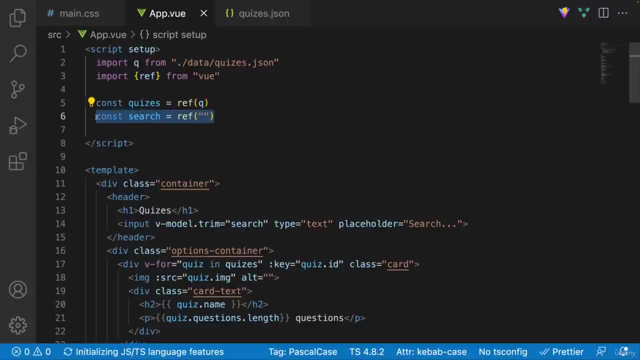 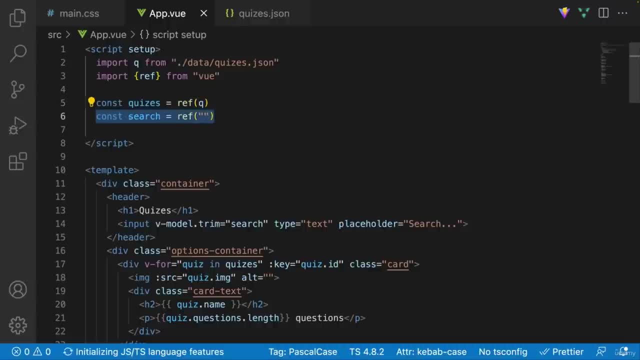 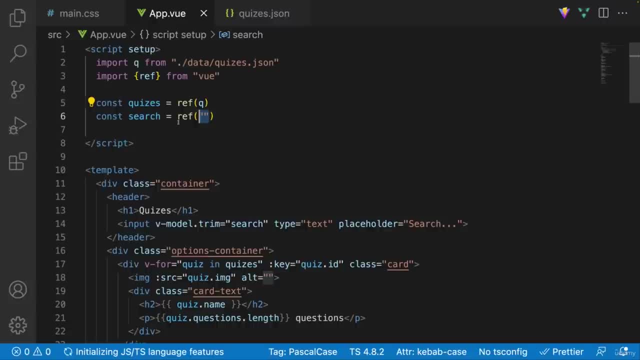 will run the logic again and again and will run the logic again and again and again I hope I got that point across now 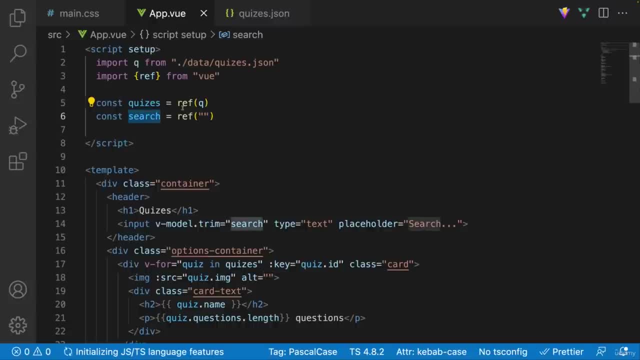 again I hope I got that point across now again I hope I got that point across now we can actually do that very easily with we can actually do that very easily with we can actually do that very easily with something called watch and we're going something called watch and we're going something called watch and we're going to import this from view so so far we to import this from view so so far we 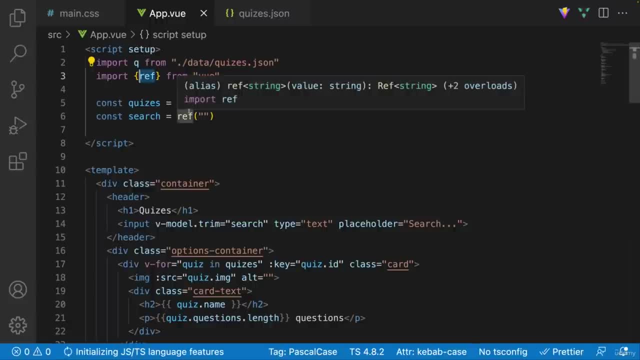 to import this from view so so far we have been only importing ref in order to have been only importing ref in order to have been only importing ref in order to define our state but there are a bunch define our state but there are a bunch define our state but there are a bunch of different things that we can import of different things that we can import 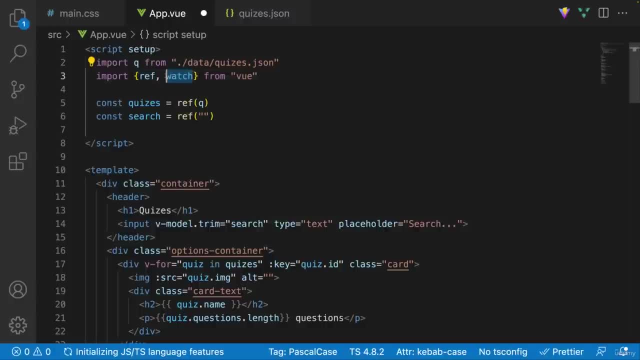 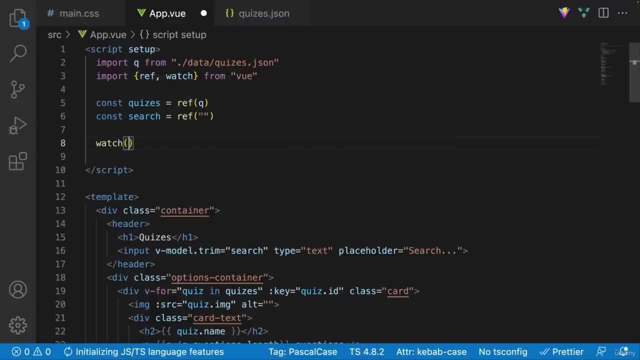 of different things that we can import including watch now watch is going to be including watch now watch is going to be including watch now watch is going to be a function that we are going to invoke a function that we are going to invoke a function that we are going to invoke and it's going to take two different and it's going to take two different and it's going to take two different parameters the first parameter is the parameters the first parameter is the parameters the first parameter is the thing that we want to listen to so in thing that we want to listen to so in thing that we want to listen to so in this case it is search and then the this case it is search and then the this case it is search and then the second thing is going to be a callback second thing is going to be a callback second thing is going to be a callback function and this is where well we're 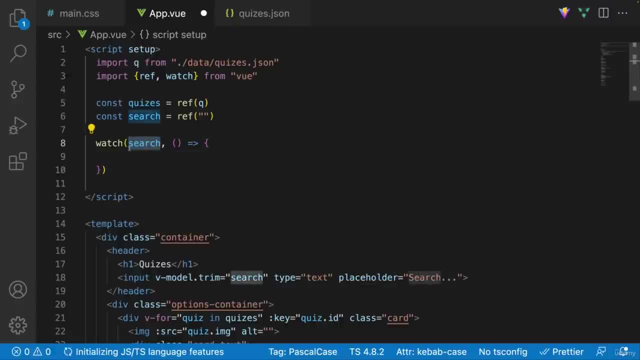 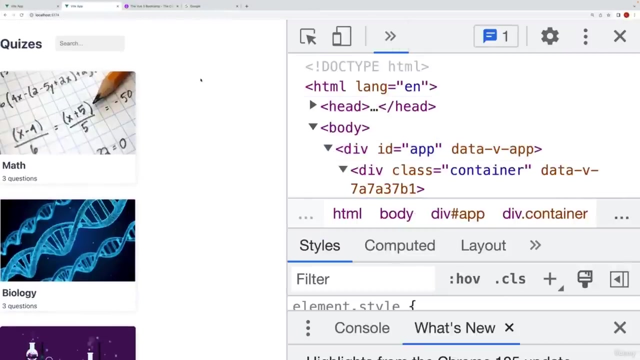 function and this is where well we're function and this is where well we're gonna execute the logic anytime that gonna execute the logic anytime that gonna execute the logic anytime that search changes so let me go ahead and search changes so let me go ahead and search changes so let me go ahead and console.log hello from watch and let's console.log hello from watch and let's console.log hello from watch and let's actually just observe the behavior here actually just observe the behavior here actually just observe the behavior here so I'm gonna go ahead and do a control so I'm gonna go ahead and do a control so I'm gonna go ahead and do a control inspect obviously this looks really inspect obviously this looks really inspect obviously this looks really ugly on on a smaller device whatever it ugly on on a smaller device whatever it 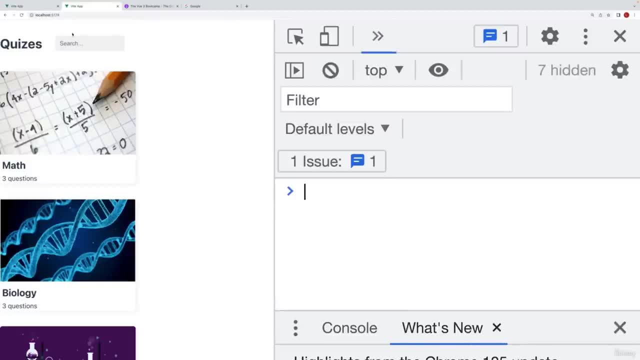 ugly on on a smaller device whatever it doesn't really matter we don't care doesn't really matter we don't care doesn't really matter we don't care about styling we care about view so I'm about styling we care about view so I'm about styling we care about view so I'm gonna do a quick little refresh and now gonna do a quick little refresh and now gonna do a quick little refresh and now what I'm gonna do is I'm gonna start what I'm gonna do is I'm gonna start what I'm gonna do is I'm gonna start updating the search so I'm gonna say H updating the search so I'm gonna say H updating the search so I'm gonna say H you can see now this was called and if I you can see now this was called and if I you can see now this was called and if I update it again oh it was called again update it again oh it was called again update it again oh it was called again it's called again it's called again so 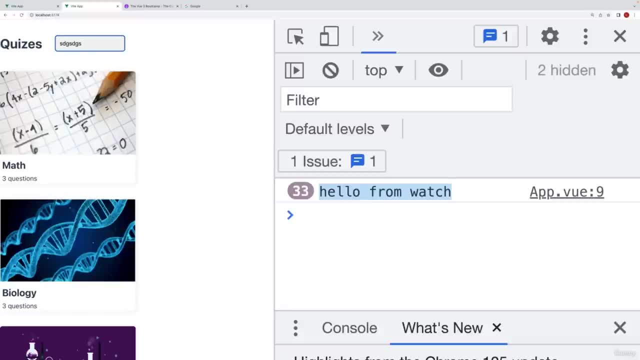 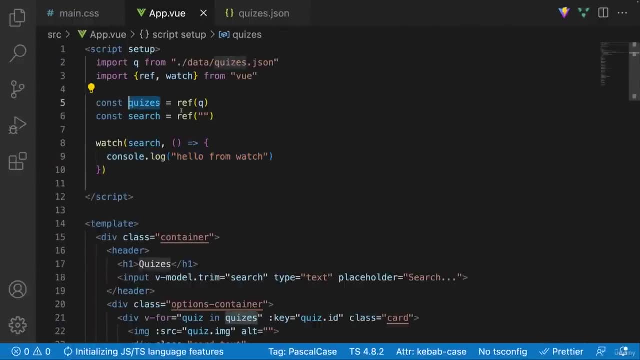 it's called again it's called again so it's called again it's called again so anytime that this changes it is going anytime that this changes it is going anytime that this changes it is going to be called and thus this is going to to be called and thus this is going to to be called and thus this is going to be an excellent place where we can add be an excellent place where we can add be an excellent place where we can add our logic to update our quizzes so let's our logic to update our quizzes so let's our logic to update our quizzes so let's go ahead and do that so let's go over go ahead and do that so let's go over go ahead and do that so let's go over here and what we're gonna do very simply here and what we're gonna do very simply here and what we're gonna do very simply is say quizzes dot value and we're gonna is say quizzes dot value and we're gonna 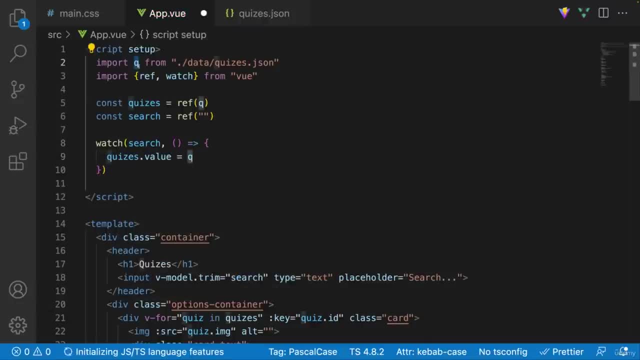 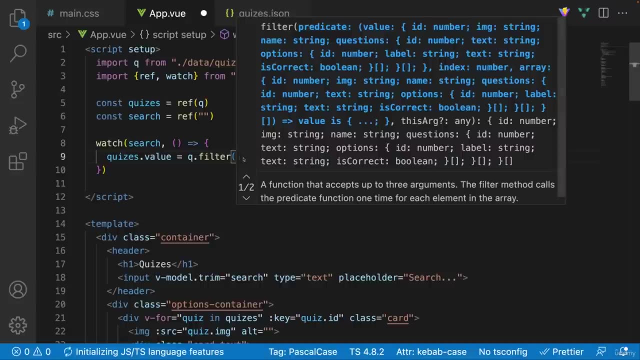 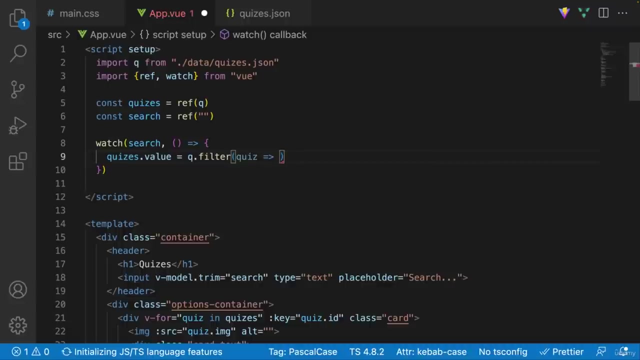 is say quizzes dot value and we're gonna say that this is going to be equal to Q say that this is going to be equal to Q say that this is going to be equal to Q so this is Q that we get from over here so this is Q that we get from over here so this is Q that we get from over here our JSON and we're gonna say dot filter our JSON and we're gonna say dot filter our JSON and we're gonna say dot filter so this is just a an array method a so this is just a an array method a so this is just a an array method a very common array method and then we're very common array method and then we're very common array method and then we're gonna say quiz and what we want to do is gonna say quiz and what we want to do is gonna say quiz and what we want to do is we only want the quizzes that have a we only want the quizzes that have a we only want the quizzes that have a name and let's go ahead and actually 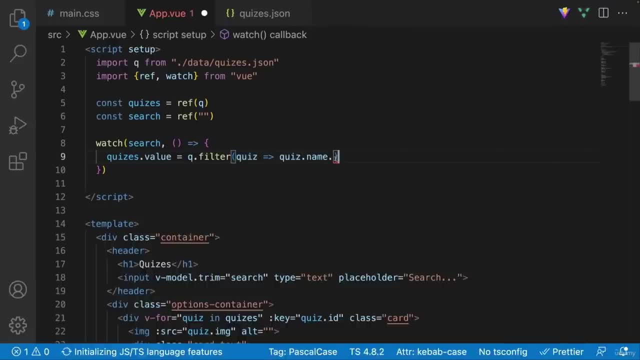 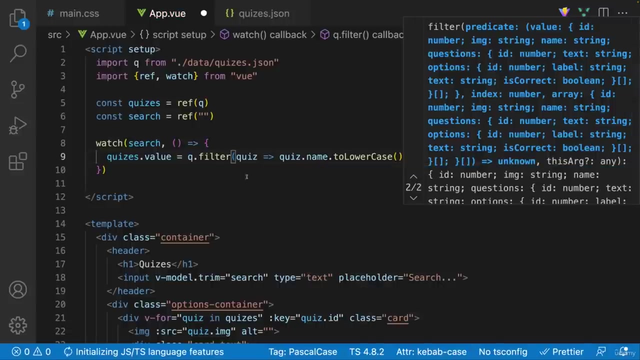 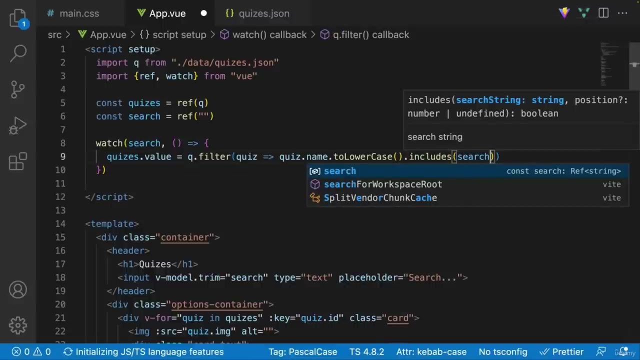 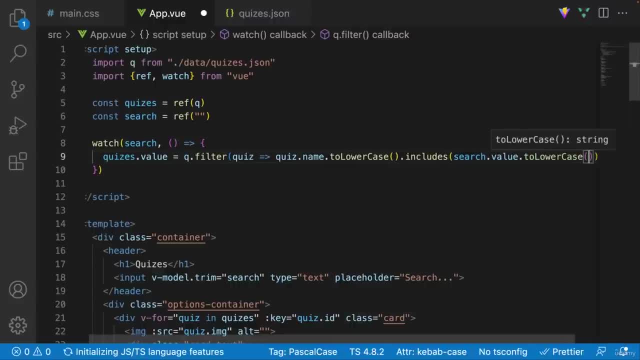 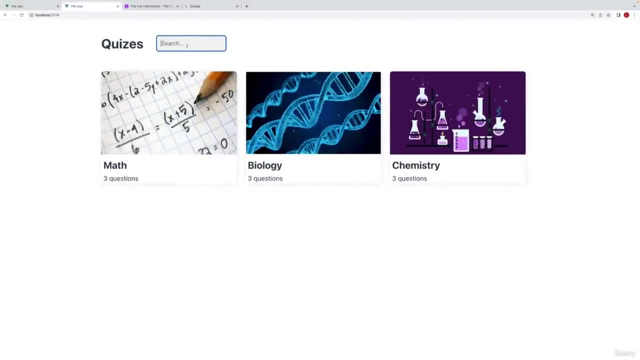 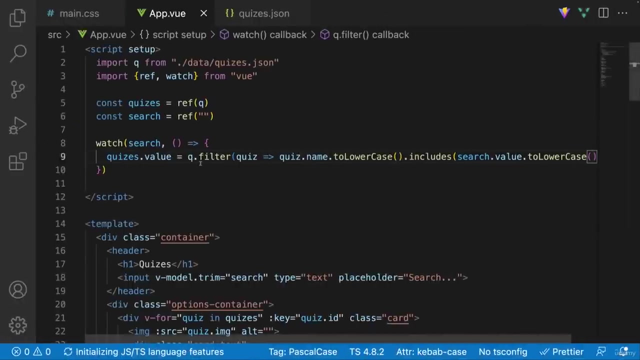 we're gonna say search dot value and also we're gonna lowercase this to also we're gonna lowercase this to also we're gonna lowercase this to lowercase so that's just gonna ensure lowercase so that's just gonna ensure lowercase so that's just gonna ensure that whenever we make let's say the user that whenever we make let's say the user that whenever we make let's say the user types in a lowercase C it's gonna ensure types in a lowercase C it's gonna ensure types in a lowercase C it's gonna ensure that it's gonna show chemistry even that it's gonna show chemistry even that it's gonna show chemistry even though the character over here is a though the character over here is a though the character over here is a capital C that's why we added the capital C that's why we added the capital C that's why we added the lower cases so that's pretty much actually 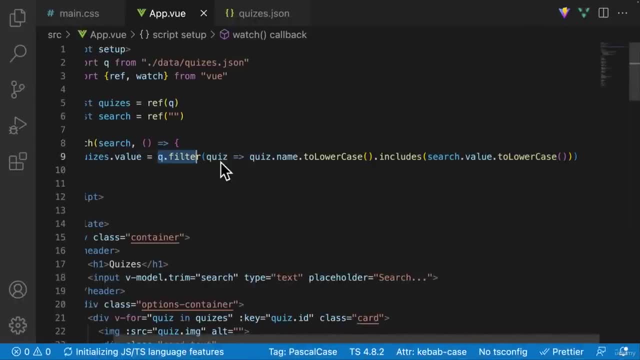 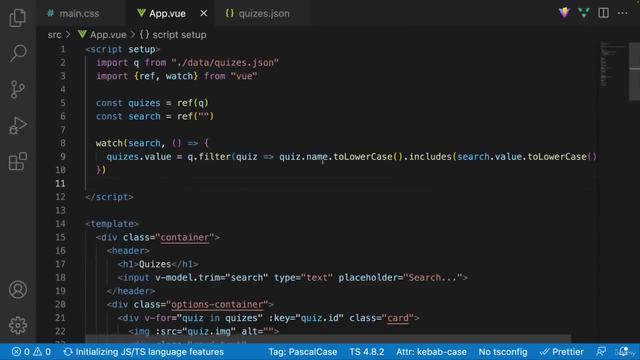 lower cases so that's pretty much actually lower cases so that's pretty much actually all it is that we have to do so all it is that we have to do so all it is that we have to do so again let's just quickly go through this again let's just quickly go through this again let's just quickly go through this because it's kind of a long expression because it's kind of a long expression because it's kind of a long expression we're doing a Q dot filter we're we're doing a Q dot filter we're we're doing a Q dot filter we're iterating over every quiz and we're only iterating over every quiz and we're only iterating over every quiz and we're only keeping the quizzes that have names keeping the quizzes that have names keeping the quizzes that have names that include what is well within this that include what is well within this 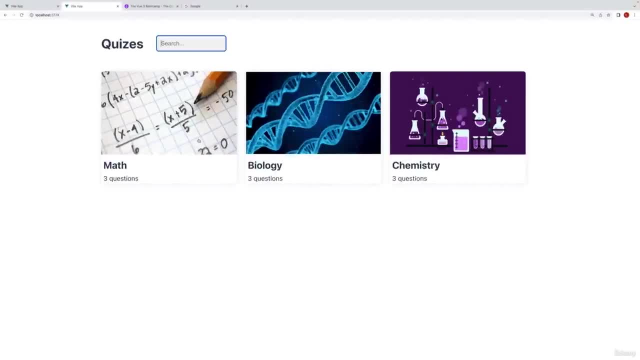 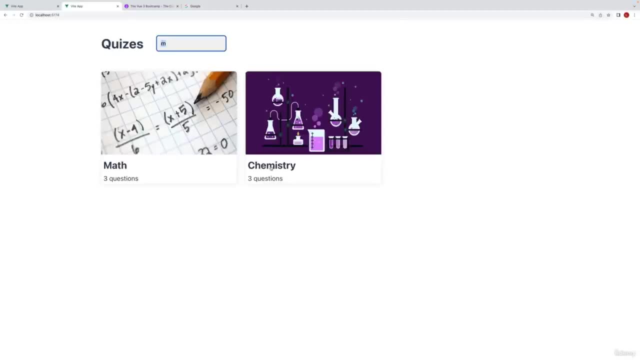 that include what is well within this search right over here so I'm gonna go search right over here so I'm gonna go search right over here so I'm gonna go ahead and save this and let's just do a ahead and save this and let's just do a ahead and save this and let's just do a quick little refresh now if I start quick little refresh now if I start quick little refresh now if I start searching for math or like M for example searching for math or like M for example searching for math or like M for example you can see chemistry and math are there you can see chemistry and math are there you can see chemistry and math are there and if I keep searching for that you can and if I keep searching for that you can and if I keep searching for that you can see now ma if I go back I get chemistry see now ma if I go back I get chemistry see now ma if I go back I get chemistry however here's the issue now if I go all however here's the issue now if I go all however here's the issue now if I go all the way back to an empty string there we 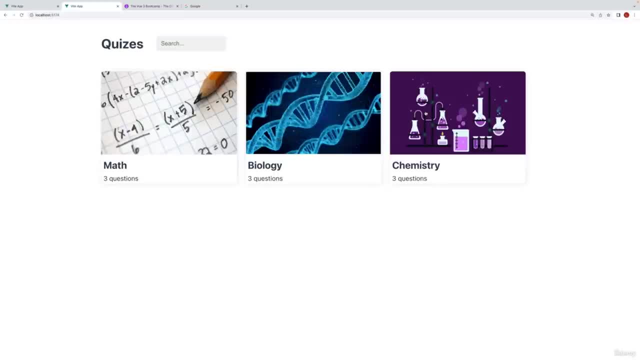 the way back to an empty string there we the way back to an empty string there we go actually that's not an issue it's go actually that's not an issue it's go actually that's not an issue it's working the way that we expect it to 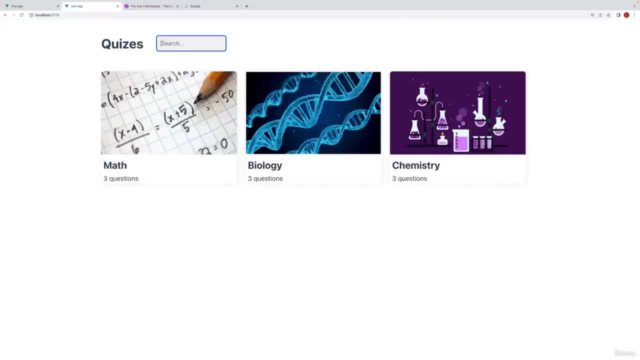 working the way that we expect it to working the way that we expect it to okay so this is great this is awesome so okay so this is great this is awesome so okay so this is great this is awesome so it's working a okay and we learned a new 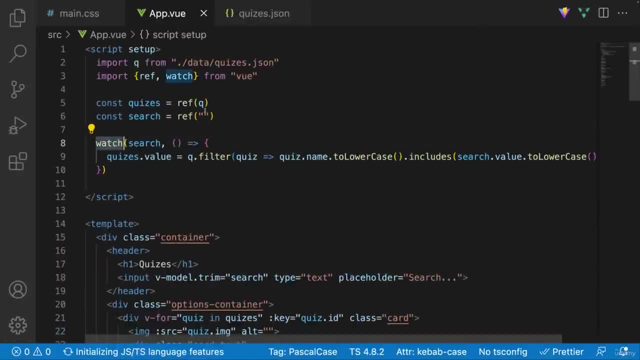 it's working a okay and we learned a new it's working a okay and we learned a new thing which is watch before we move on I thing which is watch before we move on I thing which is watch before we move on I want to quickly discuss the structure 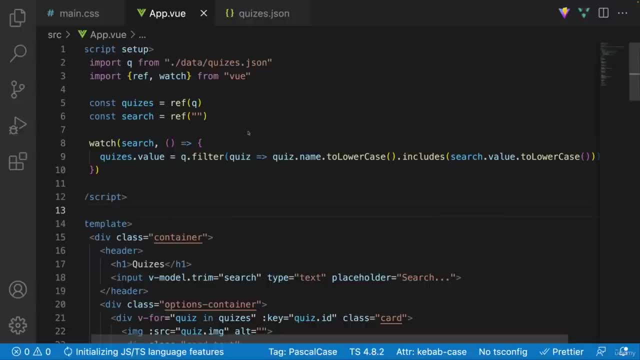 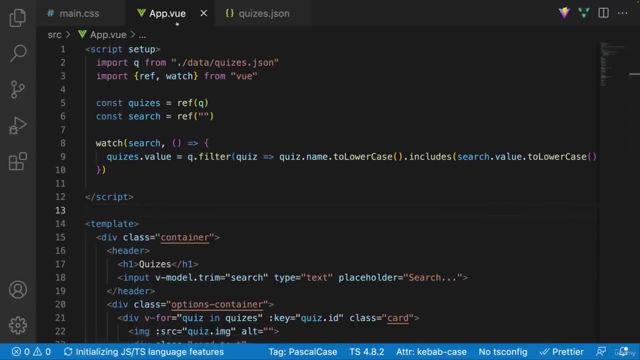 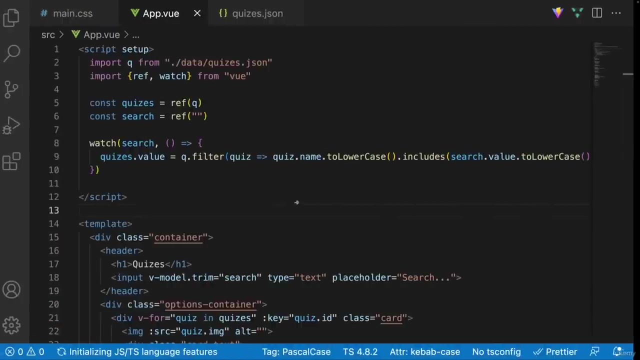 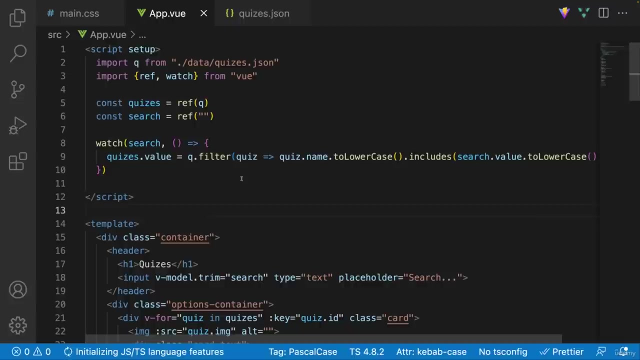 want to quickly discuss the structure of our application currently in this of our application currently in this of our application currently in this project and well old of the other project and well old of the other project and well old of the other projects all of our code existed inside projects all of our code existed inside projects all of our code existed inside of the app dot view file so right over of the app dot view file so right over of the app dot view file so right over here we had all of our code however here we had all of our code however here we had all of our code however later on once this application gets later on once this application gets later on once this application gets bigger and bigger and bigger it's gonna bigger and bigger and bigger it's gonna bigger and bigger and bigger it's gonna be ideal to start separating our code be ideal to start separating our code be ideal to start separating our code into different components and two into different components and two 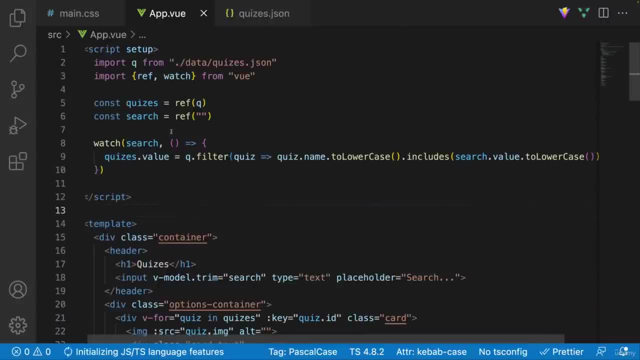 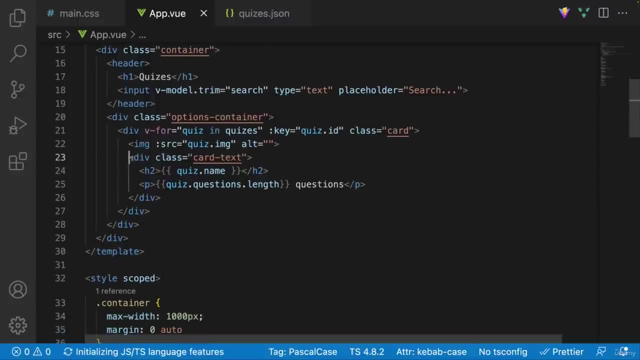 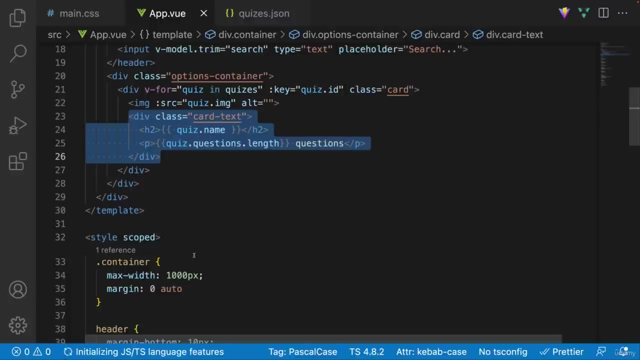 into different components and two different files so for example if you different files so for example if you different files so for example if you look at our app dot view right now I look at our app dot view right now I look at our app dot view right now I actually think that separating our card actually think that separating our card actually think that separating our card HTML as well as the CSS associated with HTML as well as the CSS associated with HTML as well as the CSS associated with it might be a good idea to split it into it might be a good idea to split it into it might be a good idea to split it into its own file so instead of having its own file so instead of having 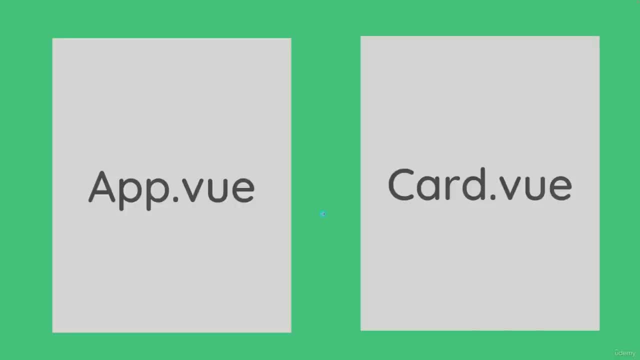 its own file so instead of having something like this app dot view you can something like this app dot view you can something like this app dot view you can have two files one app dot view and have two files one app dot view and have two files one app dot view and then another which is card dot view and then another which is card dot view and then another which is card dot view and right over here is going to contain all right over here is going to contain all right over here is going to contain all of the HTML JS and the CSS that of the HTML JS and the CSS that of the HTML JS and the CSS that pertains to the card now doing it this pertains to the card now doing it this pertains to the card now doing it this way actually adds two benefits benefit way actually adds two benefits benefit way actually adds two benefits benefit number one is it isolates the code so 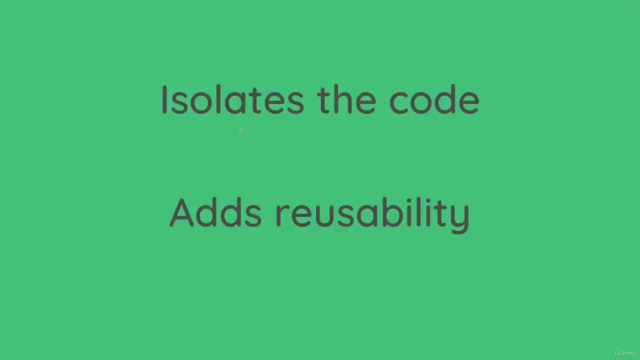 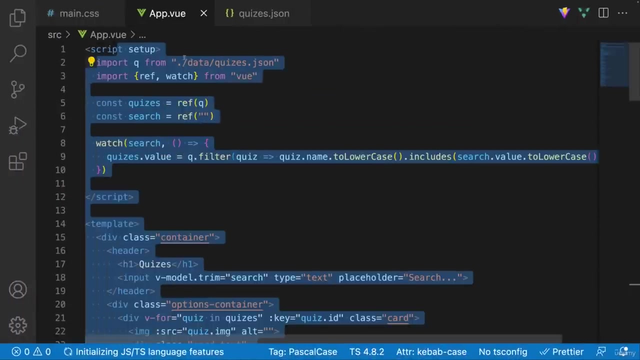 number one is it isolates the code so number one is it isolates the code so let's say later on our application is let's say later on our application is let's say later on our application is really really big and what we want to do really really big and what we want to do really really big and what we want to do is we want to modify our card in some is we want to modify our card in some is we want to modify our card in some way well what do we do if our way well what do we do if our way well what do we do if our application code exists in one file application code exists in one file application code exists in one file right over here the app dot view you can right over here the app dot view you can right over here the app dot view you can imagine that it's gonna be really really imagine that it's gonna be really really imagine that it's gonna be really really hard to point point where the card is hard to point point where the card is 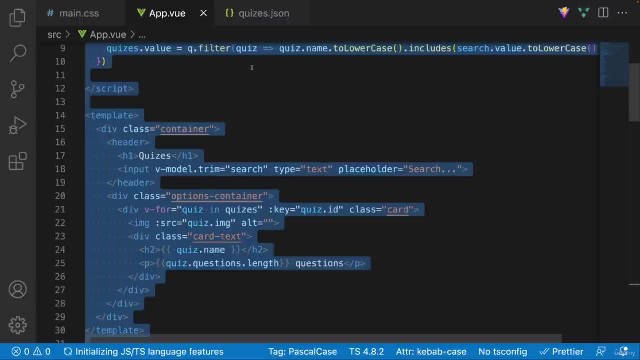 hard to point point where the card is and then modify it without probably and then modify it without probably and then modify it without probably altering something else so that is one altering something else so that is one altering something else so that is one thing it isolates our code so that it thing it isolates our code so that it thing it isolates our code so that it becomes really really easy to modify becomes really really easy to modify 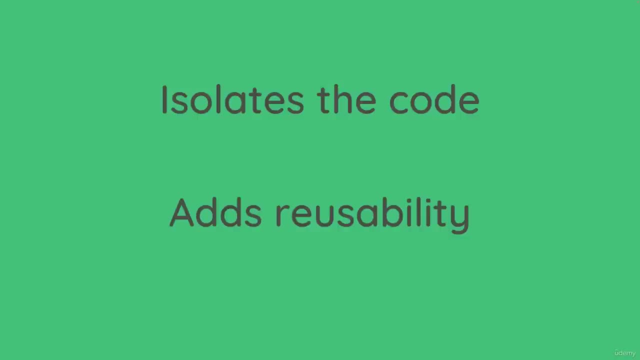 becomes really really easy to modify things the other thing is that it adds things the other thing is that it adds things the other thing is that it adds reuse ability let me show you what I reuse ability let me show you what I reuse ability let me show you what I mean by this and we'll see the powers of 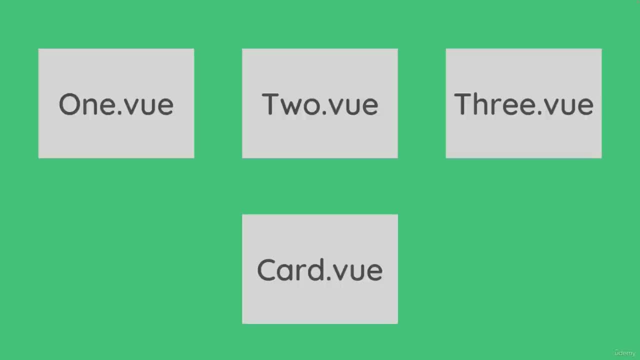 mean by this and we'll see the powers of mean by this and we'll see the powers of this later on so if you don't get it this later on so if you don't get it this later on so if you don't get it right away that's fine but let me just right away that's fine but let me just right away that's fine but let me just quickly do an explanation here so let's quickly do an explanation here so let's quickly do an explanation here so let's say we have three different view files say we have three different view files say we have three different view files one dot view to W and then three dot one dot view to W and then three dot one dot view to W and then three dot view and let's say one dot view and view and let's say one dot view and view and let's say one dot view and three dot view required to have the three dot view required to have the 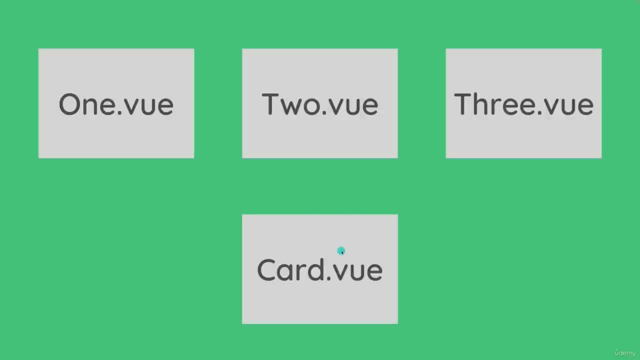 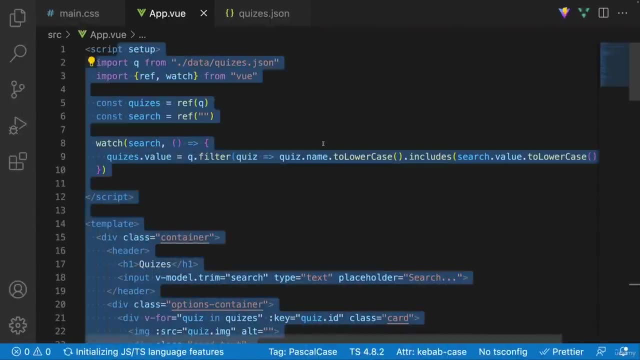 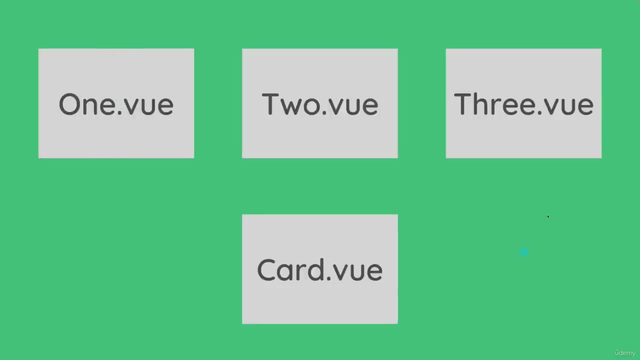 three dot view required to have the exact same card with the exact same HTML exact same card with the exact same HTML exact same card with the exact same HTML elements as well as this CSS well if we elements as well as this CSS well if we elements as well as this CSS well if we didn't separate this into its own file didn't separate this into its own file didn't separate this into its own file what we would have to do is just write what we would have to do is just write what we would have to do is just write the HTML for the card and the CSS in the HTML for the card and the CSS in the HTML for the card and the CSS in this file and then we would have to do this file and then we would have to do this file and then we would have to do the exact same thing in this file right the exact same thing in this file right the exact same thing in this file right over here so you can see that there is a 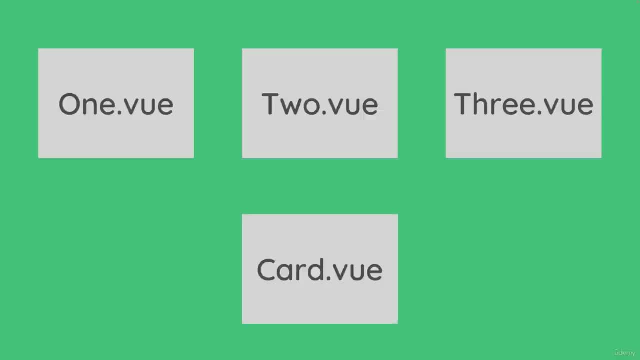 over here so you can see that there is a over here so you can see that there is a lot of duplicate code and let's say lot of duplicate code and let's say lot of duplicate code and let's say sometime in the future we have to do a sometime in the future we have to do a sometime in the future we have to do a modification to our card then what we modification to our card then what we modification to our card then what we would have to do is make that would have to do is make that would have to do is make that modification here and then also make modification here and then also make modification here and then also make that modification here so obviously this that modification here so obviously this that modification here so obviously this is not great instead what we can do is is not great instead what we can do is 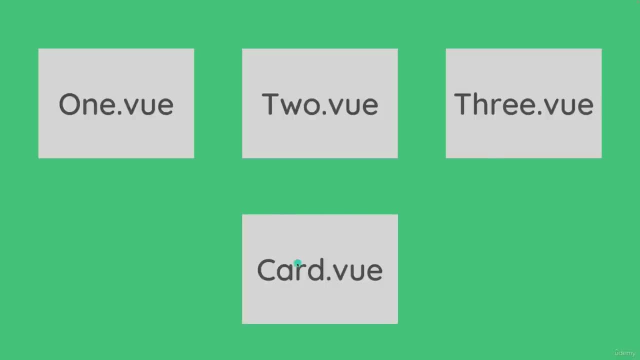 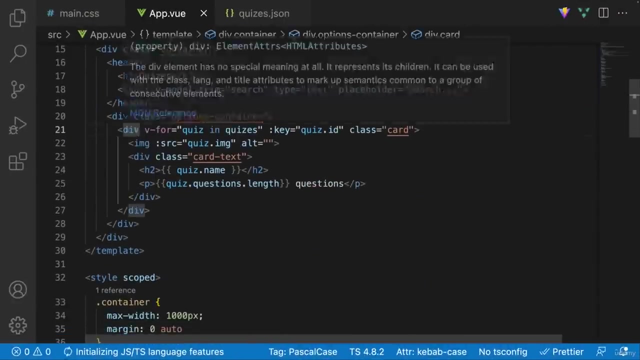 is not great instead what we can do is completely isolate the code for our card completely isolate the code for our card completely isolate the code for our card inside of this own file and what we can inside of this own file and what we can inside of this own file and what we can do is just import that card into the do is just import that card into the do is just import that card into the files that we need alright so this is files that we need alright so this is files that we need alright so this is exactly what we are going to do and exactly what we are going to do and exactly what we are going to do and let's actually just go ahead and do it let's actually just go ahead and do it let's actually just go ahead and do it right now okay so what I'm gonna do here right now okay so what I'm gonna do here right now okay so what I'm gonna do here is just for now we are going to this is 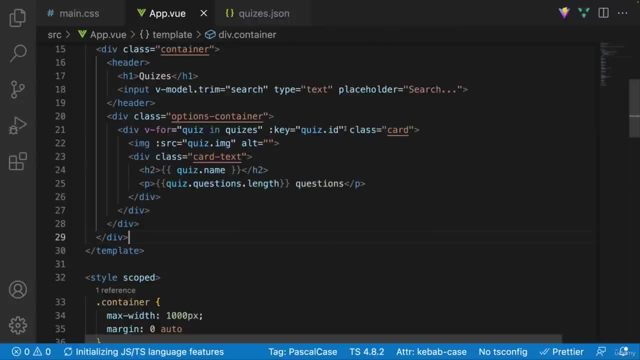 is just for now we are going to this is is just for now we are going to this is this is the HTML for our card just for this is the HTML for our card just for this is the HTML for our card just for now we're just gonna remove the v4 maybe now we're just gonna remove the v4 maybe now we're just gonna remove the v4 maybe we can just cut it out and then put it we can just cut it out and then put it we can just cut it out and then put it over here and comment it out just so we over here and comment it out just so we over here and comment it out just so we can have the code so I'm gonna go ahead can have the code so I'm gonna go ahead can have the code so I'm gonna go ahead and just remove it and let's just remove and just remove it and let's just remove and just remove it and let's just remove anything associated with the v4 itself anything associated with the v4 itself actually you know what let us let us just 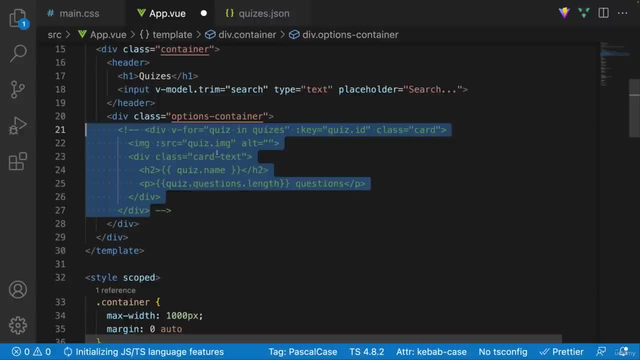 actually you know what let us let us just actually you know what let us let us just write the HTML again so I'm gonna write the HTML again so I'm gonna write the HTML again so I'm gonna comment this out or we're just gonna comment this out or we're just gonna comment this out or we're just gonna write the HTML again in a separate file 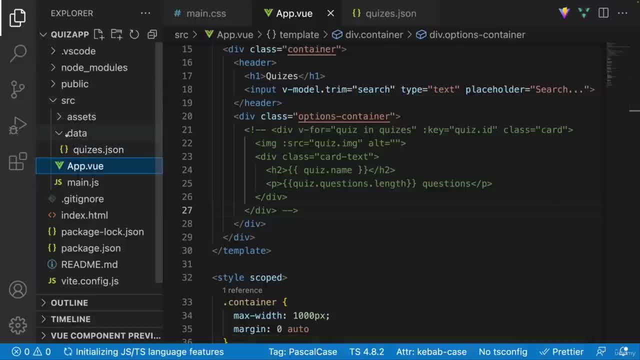 write the HTML again in a separate file write the HTML again in a separate file so what we're gonna do here is we are so what we're gonna do here is we are so what we're gonna do here is we are going to create a new directory and let going to create a new directory and let going to create a new directory and let me zoom in here for a bit we're gonna me zoom in here for a bit we're gonna me zoom in here for a bit we're gonna create a new directory and this is gonna create a new directory and this is gonna 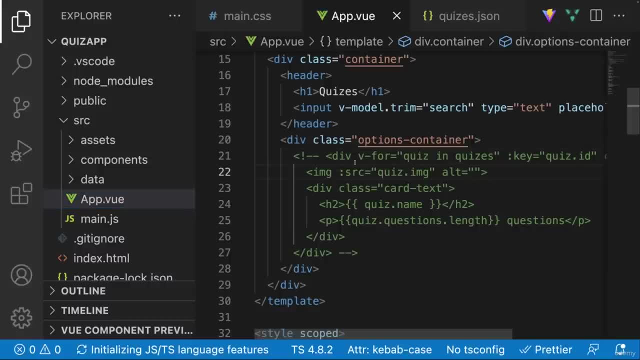 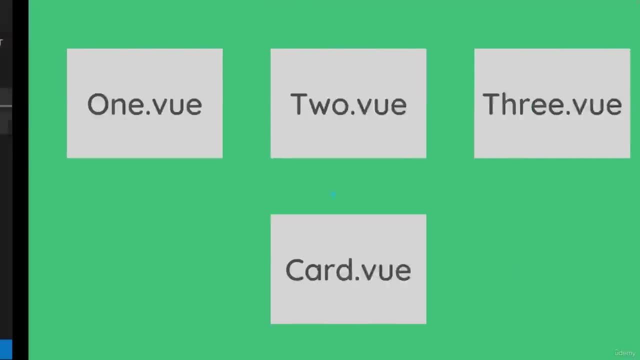 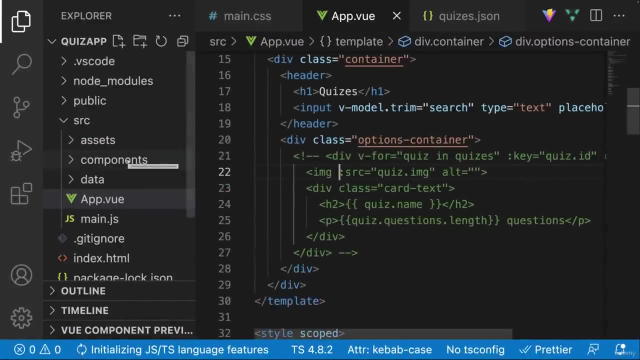 create a new directory and this is gonna be called components because in effect be called components because in effect be called components because in effect what we're doing are creating different what we're doing are creating different what we're doing are creating different components that different file can components that different file can components that different file can utilize so we are creating a card utilize so we are creating a card utilize so we are creating a card component that may be the one dot view component that may be the one dot view component that may be the one dot view file can utilize and the three w file file can utilize and the three w file file can utilize and the three w file can utilize we can create multiple can utilize we can create multiple can utilize we can create multiple different components for example we can 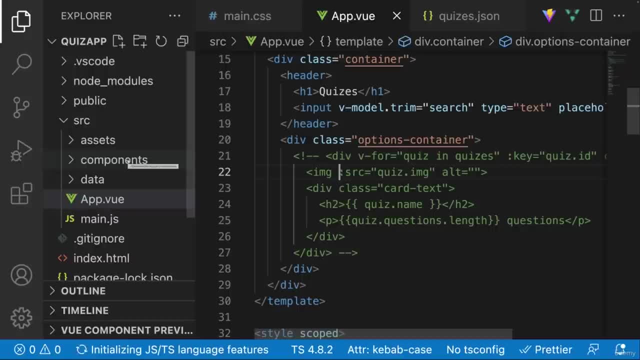 different components for example we can different components for example we can have a not bar component a hero component have a not bar component a hero component have a not bar component a hero component in this case we're gonna have a card in this case we're gonna have a card in this case we're gonna have a card component so let's go ahead and create component so let's go ahead and create 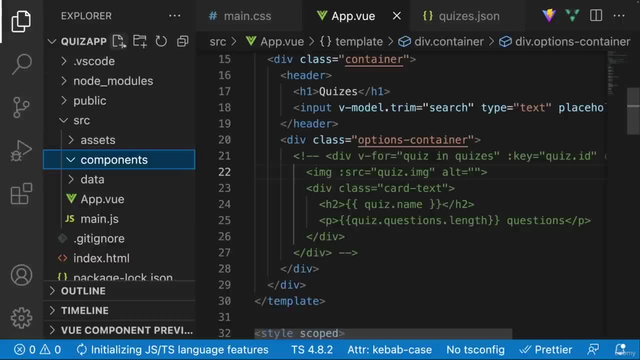 component so let's go ahead and create this card component so let's go over this card component so let's go over this card component so let's go over here and what we're gonna say is card here and what we're gonna say is card 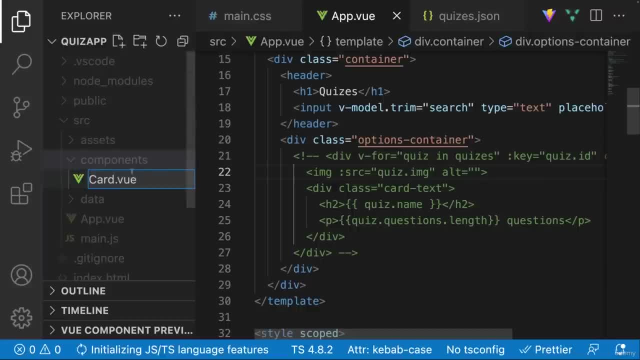 here and what we're gonna say is card dot view so very similar to what we've dot view so very similar to what we've dot view so very similar to what we've had before had before 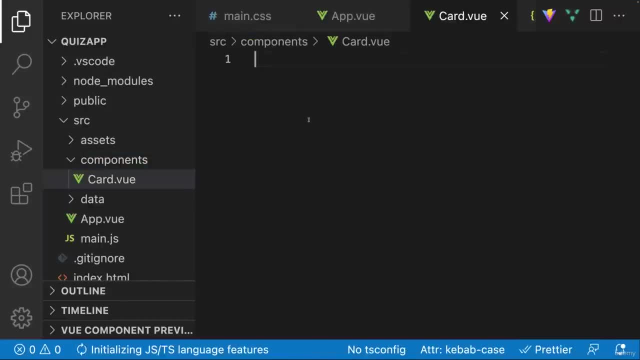 had before card dot view and then in here we're card dot view and then in here we're card dot view and then in here we're going to build out the html structure going to build out the html structure going to build out the html structure for our card so let's go ahead and for our card so let's go ahead and for our card so let's go ahead and we'll start with the templates we'll start with the templates we'll start with the templates and we're gonna have our div and then and we're gonna have our div and then and we're gonna have our div and then we're going to create well what we had we're going to create well what we had we're going to create well what we had right here let me just close this we're right here let me just close this we're right here let me just close this we're gonna recreate what we had right here so 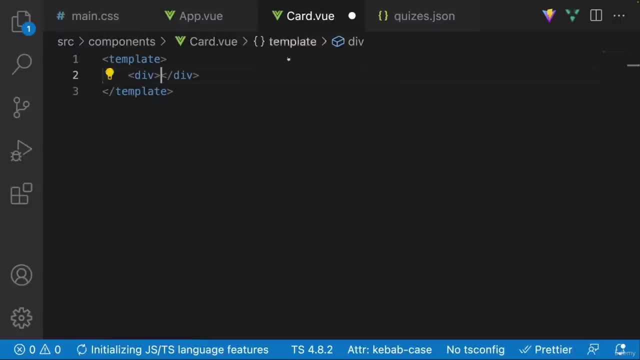 gonna recreate what we had right here so gonna recreate what we had right here so i'm just gonna go ahead and well just i'm just gonna go ahead and well just i'm just gonna go ahead and well just take a quick look so we had a div take a quick look so we had a div take a quick look so we had a div and that had a class of card and that had a class of card and that had a class of card and then what we had was an image and then what we had was an image and then what we had was an image and let me fix that we had an image tag and let me fix that we had an image tag and let me fix that we had an image tag and we'll add just a random source let's and we'll add just a random source let's and we'll add just a random source let's just add a random image right over here just add a random image right over here 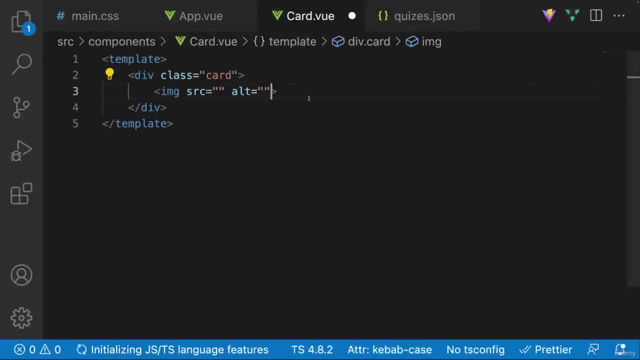 just add a random image right over here let's add math for now let's add math for now let's add math for now just so we can see the card just so we can see the card 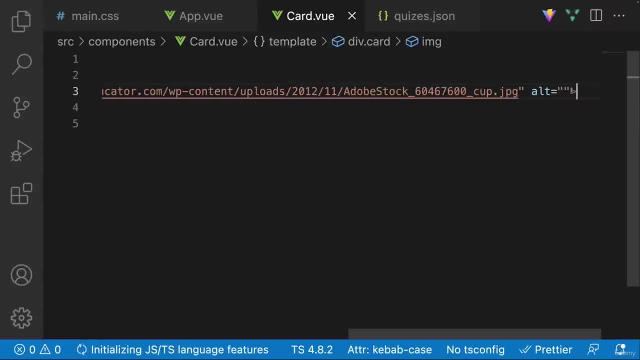 just so we can see the card and there we go so we're going to go and there we go so we're going to go and there we go so we're going to go ahead and just add that image alt who ahead and just add that image alt who ahead and just add that image alt who cares about it 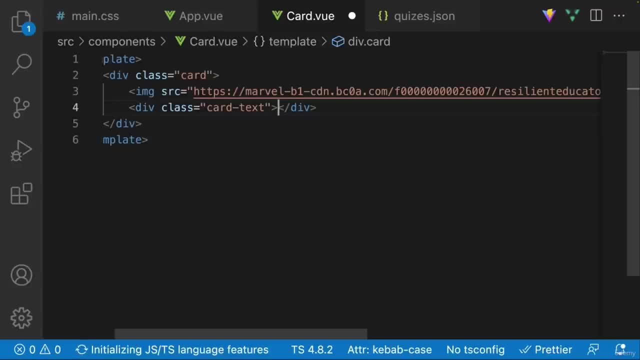 cares about it cares about it and then we're going to have div with and then we're going to have div with and then we're going to have div with card text card text card text and then what we're going to do is have and then what we're going to do is have and then what we're going to do is have an h2 an h2 an h2 for now we'll just hard code math 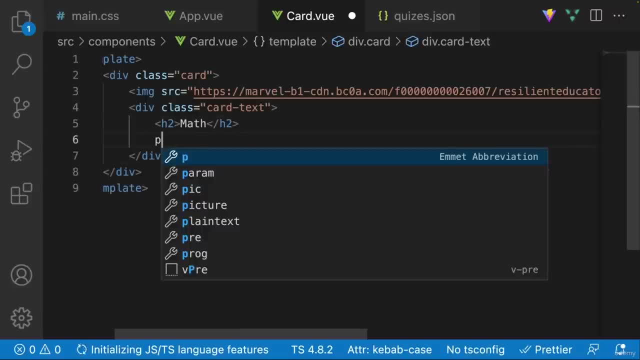 for now we'll just hard code math for now we'll just hard code math and now what we can do is just say p and now what we can do is just say p and now what we can do is just say p tag and we'll say tag and we'll say tag and we'll say three questions we'll just hard code it three questions we'll just hard code it three questions we'll just hard code it for now later on we'll learn exactly for now later on we'll learn exactly for now later on we'll learn exactly how we can pass data how we can pass data 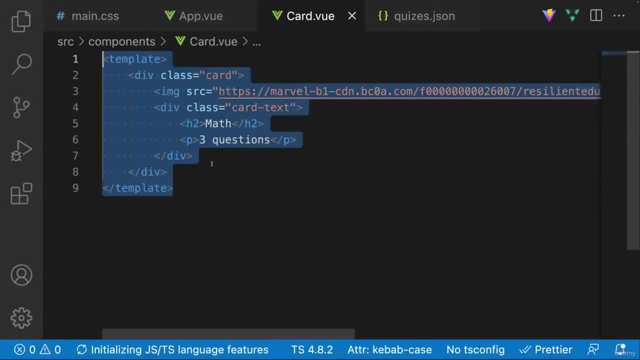 how we can pass data into these components so this is into these components so this is into these components so this is actually all it is that we need to do actually all it is that we need to do actually all it is that we need to do now let's actually go ahead and style 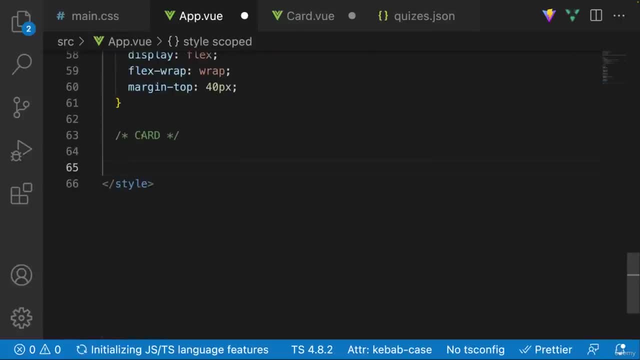 now let's actually go ahead and style now let's actually go ahead and style all of these styles we're just going to all of these styles we're just going to all of these styles we're just going to cut them from this file so you can see cut them from this file so you can see cut them from this file so you can see now we're completely removing stuff from now we're completely removing stuff from now we're completely removing stuff from this file and actually isolating it so this file and actually isolating it so this file and actually isolating it so again it's going to make it a lot easier again it's going to make it a lot easier again it's going to make it a lot easier to maintain 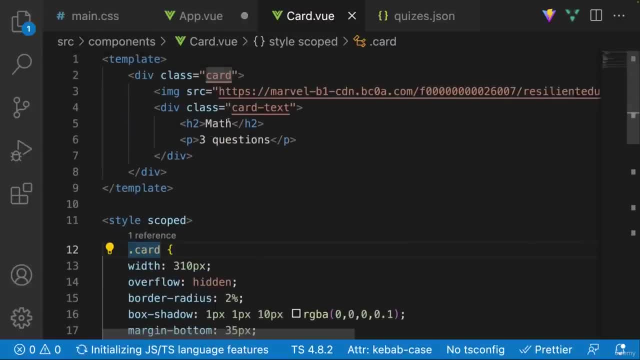 to maintain so we're going to go ahead and save so we're going to go ahead and save so we're going to go ahead and save this this this and now we're done so now what we need 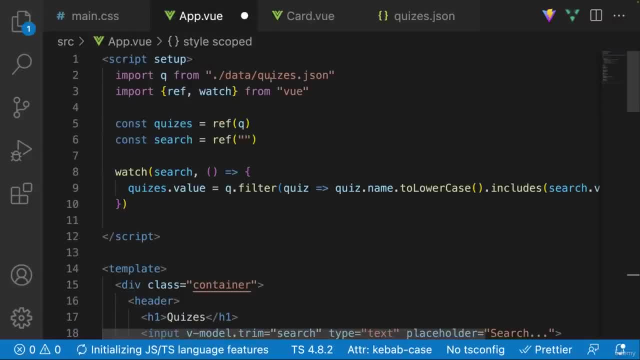 and now we're done so now what we need and now we're done so now what we need to do is actually to do is actually to do is actually render these cards or this this html render these cards or this this html render these cards or this this html element somehow inside of the app.view element somehow inside of the app.view 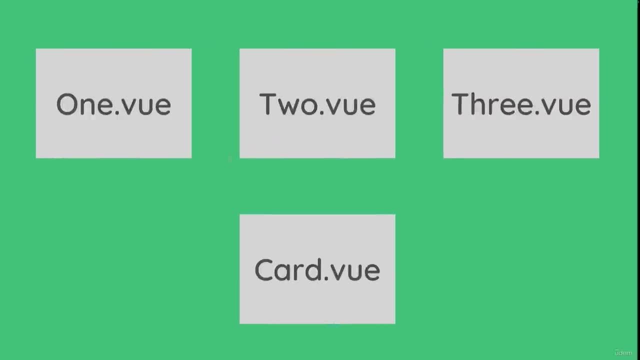 element somehow inside of the app.view so let me go ahead and quickly just save so let me go ahead and quickly just save so let me go ahead and quickly just save this and let's just see what we have this and let's just see what we have this and let's just see what we have thus far thus far 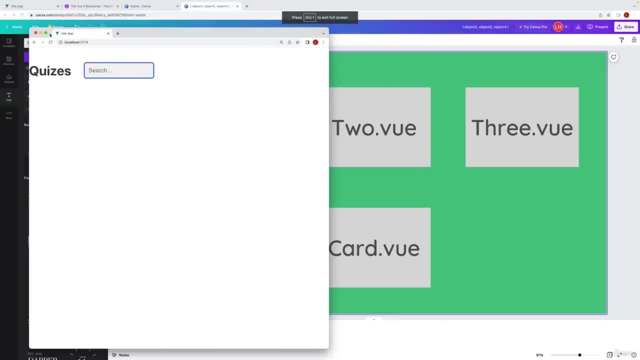 thus far and uh i gotta open this up and uh i gotta open this up and uh i gotta open this up there we go let's open this up 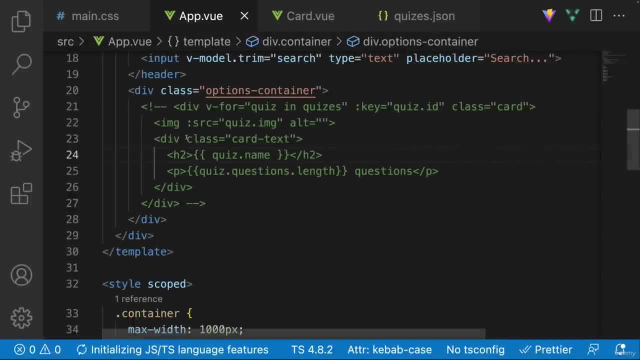 there we go let's open this up over here so right now we have of course over here so right now we have of course over here so right now we have of course nothing nothing nothing so what i want to do is i want to render so what i want to do is i want to render so what i want to do is i want to render this component so how are we going to do this component so how are we going to do 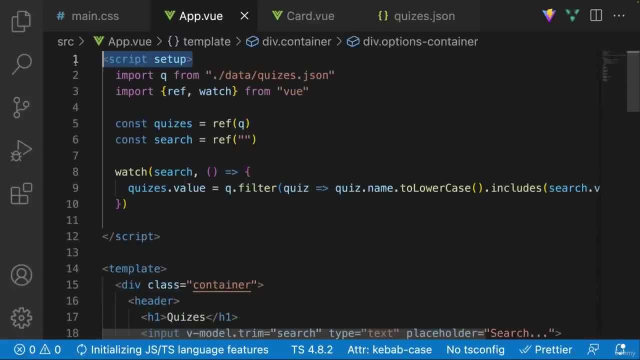 this component so how are we going to do that that that well it's actually going to be really well it's actually going to be really well it's actually going to be really easy we're going to go over here to the easy we're going to go over here to the easy we're going to go over here to the script tag and we're going to script tag and we're going to 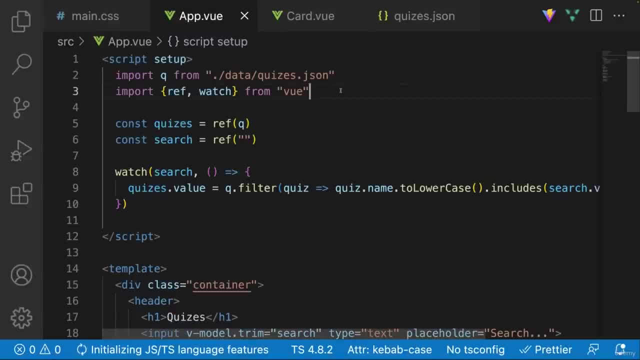 script tag and we're going to import this component in so we're going import this component in so we're going import this component in so we're going to say to say to say import and we can call this whatever it 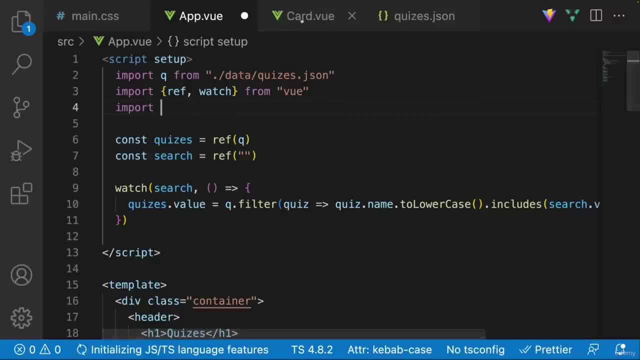 import and we can call this whatever it import and we can call this whatever it is that we want is that we want is that we want typically what we're going to call it is typically what we're going to call it is typically what we're going to call it is the name of the file the name of the file the name of the file and typically it starts with a capital and typically it starts with a capital and typically it starts with a capital letter any component typically starts letter any component typically starts letter any component typically starts with a capital letter with a capital letter with a capital letter it doesn't have to but it is kind of a it doesn't have to but it is kind of a 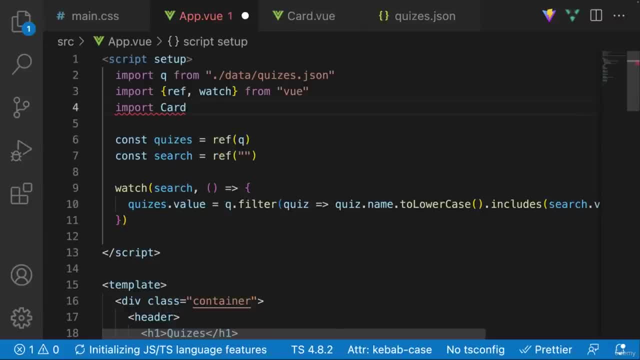 it doesn't have to but it is kind of a more common convention to do it that way more common convention to do it that way more common convention to do it that way so i'm going to say import card and i'm so i'm going to say import card and i'm so i'm going to say import card and i'm going to say from going to say from going to say from and then what we're going to do is dot and then what we're going to do is dot and then what we're going to do is dot slash we're going to move to the slash we're going to move to the slash we're going to move to the components directory components directory components directory and then we're going to say card.view and then we're going to say card.view and then we're going to say card.view so let's go ahead and now render 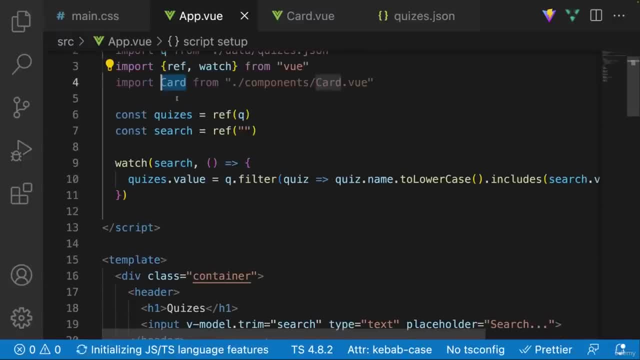 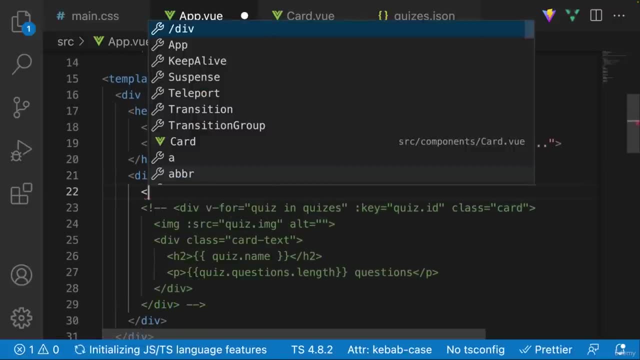 so let's go ahead and now render so let's go ahead and now render this right over here so we can actually this right over here so we can actually this right over here so we can actually treat this treat this treat this kind of like an html tag so very simply kind of like an html tag so very simply kind of like an html tag so very simply we can actually go we can actually go we can actually go right here and we can say right here and we can say right here and we can say card and we can just have this be a card and we can just have this be a card and we can just have this be a self-closing html tag like so self-closing html tag like so 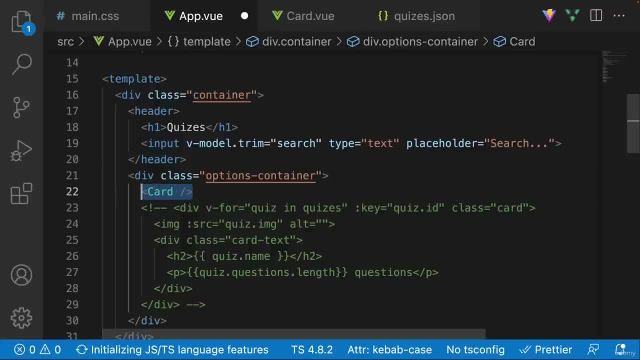 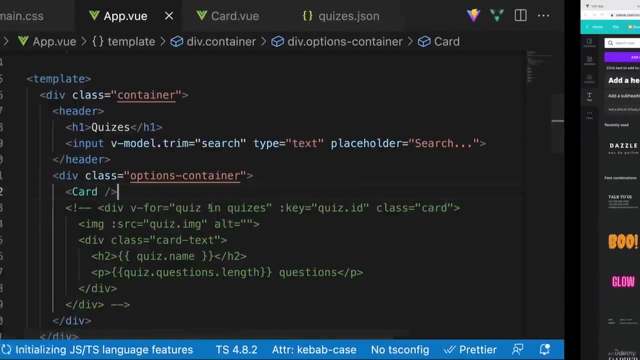 self-closing html tag like so and you can see that the uh the syntax and you can see that the uh the syntax and you can see that the uh the syntax highlighter actually notices that this highlighter actually notices that this highlighter actually notices that this is a component is a component is a component and it goes ahead and gives us a nice and it goes ahead and gives us a nice and it goes ahead and gives us a nice green color green color green color so if i were to save this now and i were so if i were to save this now and i were so if i were to save this now and i were to go back over here to go back over here to go back over here right away you can see that we have our 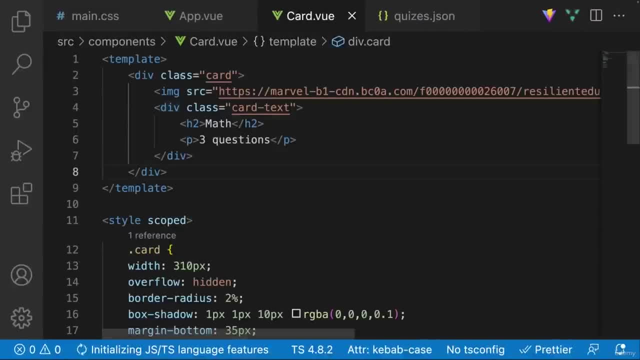 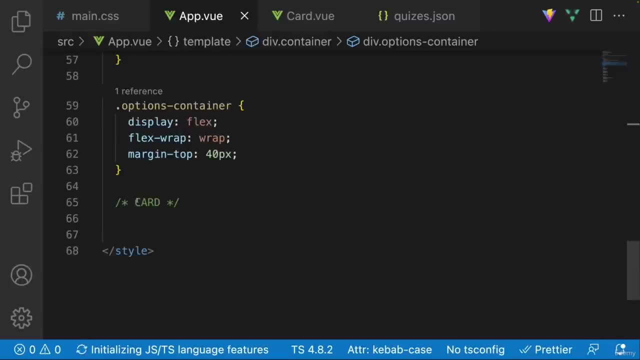 right away you can see that we have our right away you can see that we have our component how cool is that component how cool is that component how cool is that we completely isolated everything we completely isolated everything we completely isolated everything and we're still getting kind of the same and we're still getting kind of the same and we're still getting kind of the same results so instead of having all of this results so instead of having all of this results so instead of having all of this code as well as all that other css code code as well as all that other css code code as well as all that other css code in this file we completely isolated in this file we completely isolated in this file we completely isolated here and of course we can actually here and of course we can actually 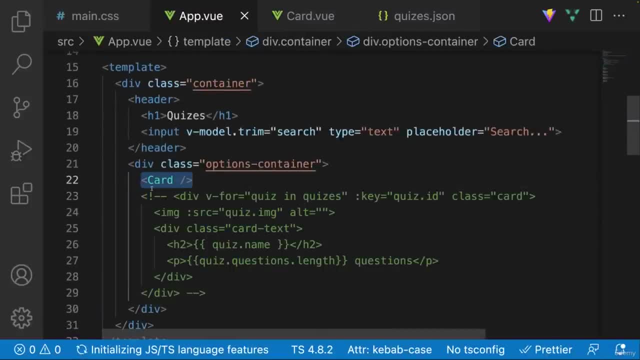 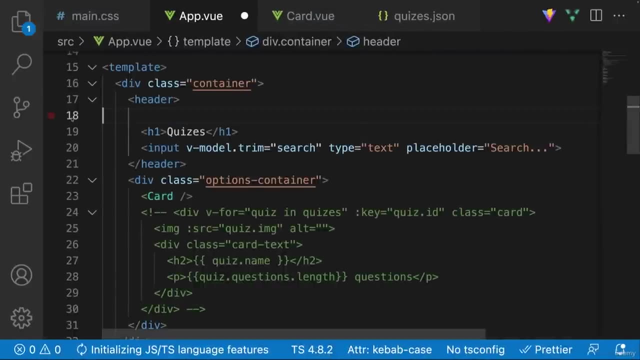 here and of course we can actually duplicate this and utilize this wherever duplicate this and utilize this wherever duplicate this and utilize this wherever we want let's say we need to use it here we want let's say we need to use it here we want let's say we need to use it here as well as here well of course we can do as well as here well of course we can do as well as here well of course we can do the exact same thing so you can see now the exact same thing so you can see now the exact same thing so you can see now we have two cards and we can use this of we have two cards and we can use this of we have two cards and we can use this of course in different files and we'll see course in different files and we'll see course in different files and we'll see that when we have more files in our that when we have more files in our that when we have more files in our application 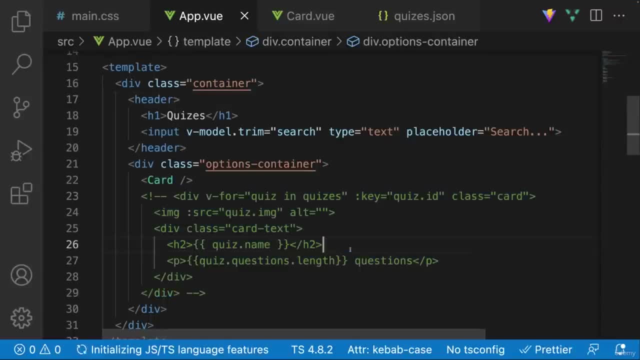 application application now of course what i want to do is i want now of course what i want to do is i want now of course what i want to do is i want to iterate over this quiz right over to iterate over this quiz right over to iterate over this quiz right over here this quizzes array and i want to here this quizzes array and i want to here this quizzes array and i want to render these co these uh these card render these co these uh these card render these co these uh these card components components components now i can very much do the exact same now i can very much do the exact same now i can very much do the exact same thing i can over here just add a v4 thing i can over here just add a v4 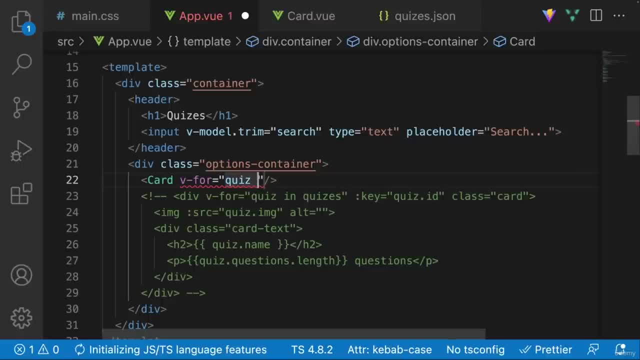 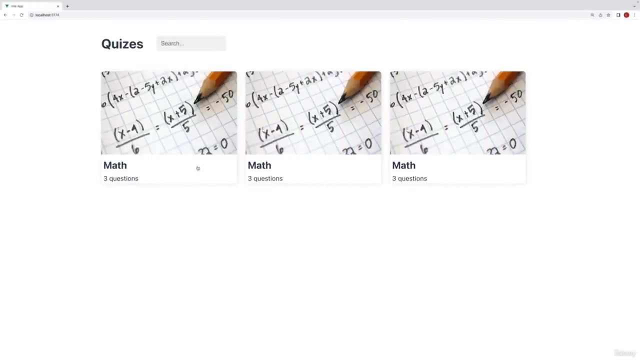 thing i can over here just add a v4 directive and i can say quiz directive and i can say quiz directive and i can say quiz and i can say in quizzes and i can say in quizzes and i can say in quizzes and of course i can also give it a key and of course i can also give it a key and of course i can also give it a key and i can say quiz dot id and very and i can say quiz dot id and very and i can say quiz dot id and very simply now i can go ahead and save this simply now i can go ahead and save this simply now i can go ahead and save this and again it's going to behave and again it's going to behave and again it's going to behave the exact same way however at this point the exact same way however at this point the exact same way however at this point the data is hard coded 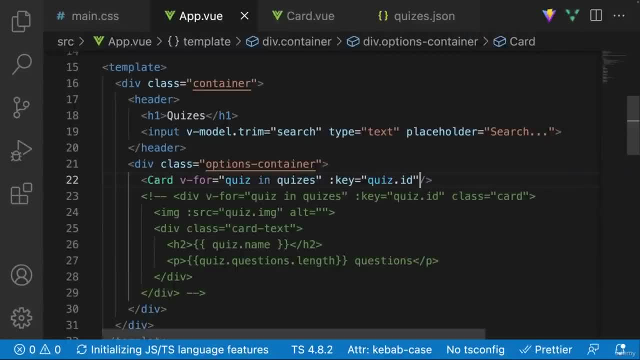 the data is hard coded the data is hard coded so now it's going to get a little bit so now it's going to get a little bit so now it's going to get a little bit tricky how are we going to tricky how are we going to tricky how are we going to kind of pass the information that we need kind of pass the information that we need kind of pass the information that we need to to to to this card component because before what to this card component because before what to this card component because before what we did was well we had the html we did was well we had the html we did was well we had the html right there we were able to modify it right there we were able to modify it 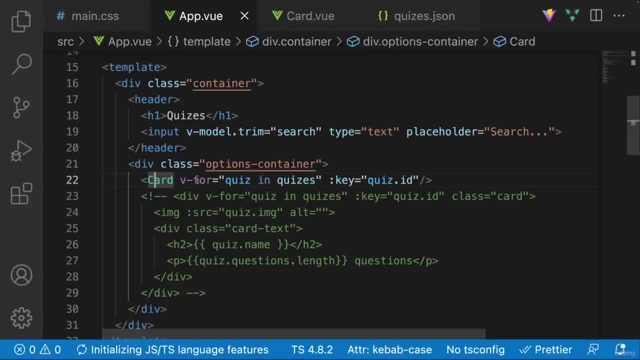 right there we were able to modify it whatever way we want but now well we whatever way we want but now well we whatever way we want but now well we have this card component and have this card component and have this card component and how are we going to kind of pass the how are we going to kind of pass the how are we going to kind of pass the data and tell it hey data and tell it hey data and tell it hey i want you to put it i want you to put i want you to put it i want you to put i want you to put it i want you to put the quiz.image inside of the source of the quiz.image inside of the source of the quiz.image inside of the image tag i want you to put the name the image tag i want you to put the name the image tag i want you to put the name over here and i want you to put the 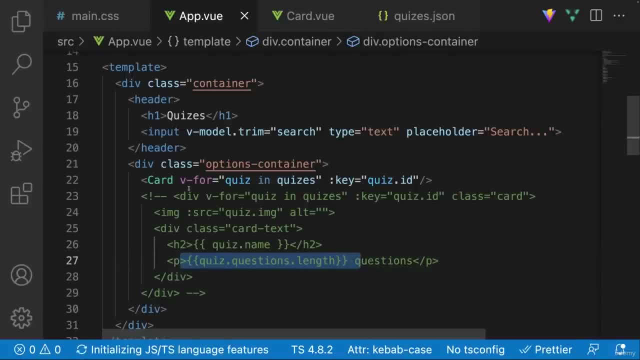 over here and i want you to put the over here and i want you to put the length over here length over here length over here how are we going to do that well let's 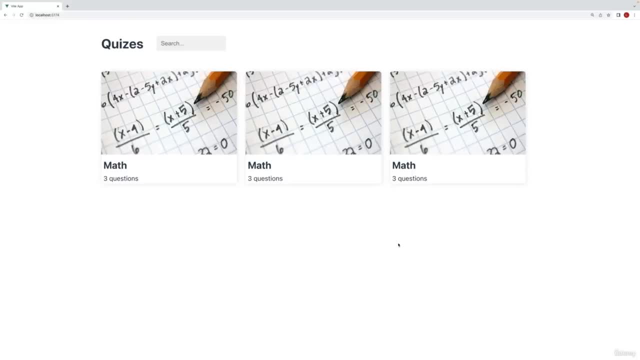 how are we going to do that well let's how are we going to do that well let's actually address that actually address that actually address that in the next video so we managed in the next video so we managed 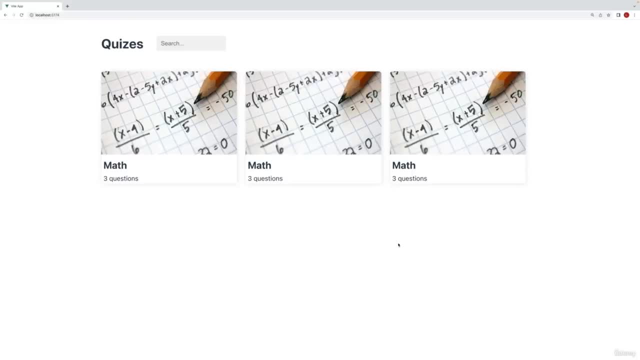 in the next video so we managed to well separate our code into a to well separate our code into a to well separate our code into a component and actually utilize that component and actually utilize that component and actually utilize that component inside of our app.view file component inside of our app.view file 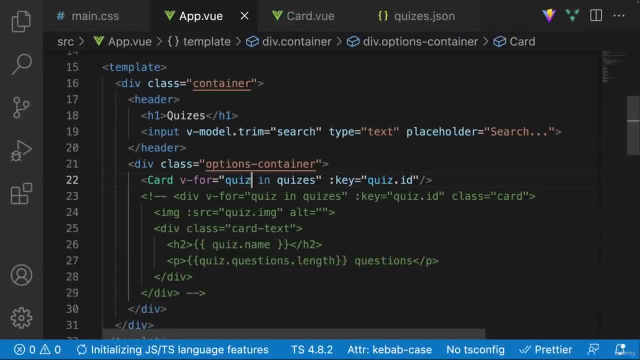 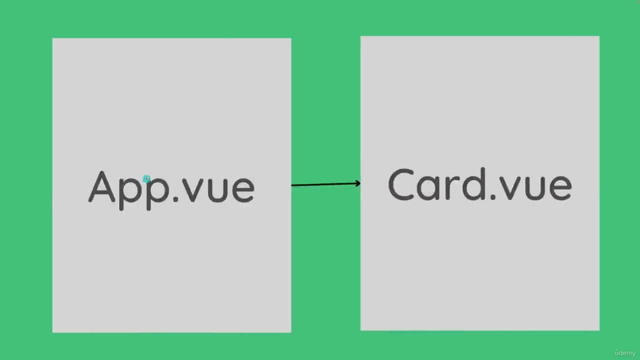 component inside of our app.view file however the thing that we're missing is however the thing that we're missing is however the thing that we're missing is we need to pass this we need to pass this we need to pass this quiz data to this card component quiz data to this card component quiz data to this card component so we need to do something like this so we need to do something like this so we need to do something like this the app.view has a bunch of information the app.view has a bunch of information the app.view has a bunch of information about the quiz the cart doesn't so what about the quiz the cart doesn't so what about the quiz the cart doesn't so what we need to do we need to do we need to do is to very simply pass this data to 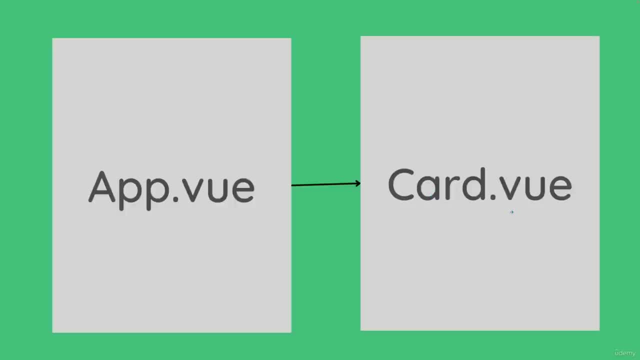 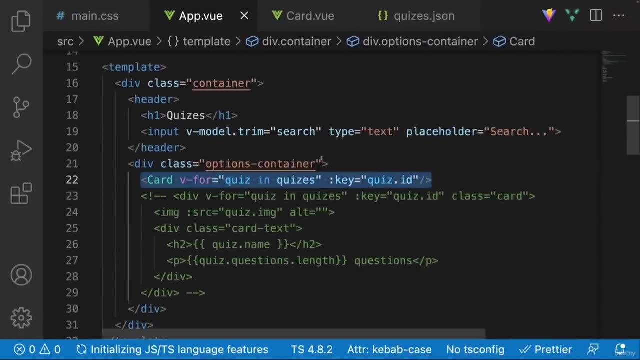 is to very simply pass this data to is to very simply pass this data to the cards.view so it can actually the cards.view so it can actually the cards.view so it can actually utilize it when rendering utilize it when rendering utilize it when rendering the card because of course right now what the card because of course right now what the card because of course right now what we're doing is simply hard coding we're doing is simply hard coding we're doing is simply hard coding everything well we can actually very everything well we can actually very everything well we can actually very easily do that easily do that easily do that with something called props so you know 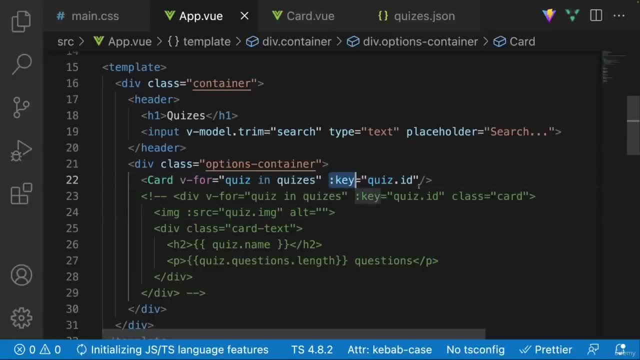 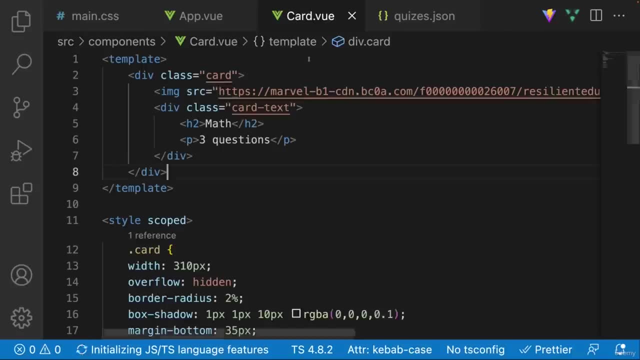 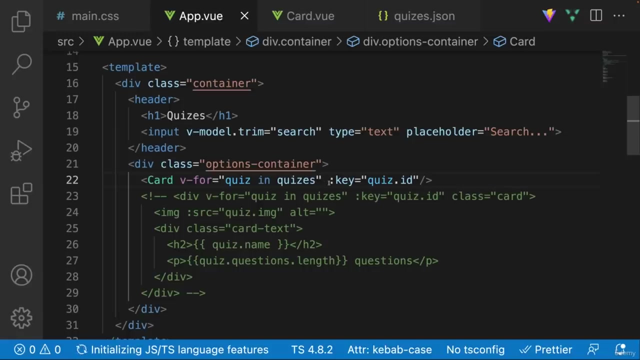 with something called props so you know how over here we have defined this key how over here we have defined this key how over here we have defined this key attribute with this colon attribute with this colon attribute with this colon well we can actually define any well we can actually define any well we can actually define any attribute with a colon and pass attribute with a colon and pass attribute with a colon and pass any data into it and then we can actually any data into it and then we can actually any data into it and then we can actually access that data within access that data within access that data within the card.view file if that doesn't make the card.view file if that doesn't make the card.view file if that doesn't make any sense let's just go ahead and do it any sense let's just go ahead and do it any sense let's just go ahead and do it and i think it will make sense and i think it will make sense 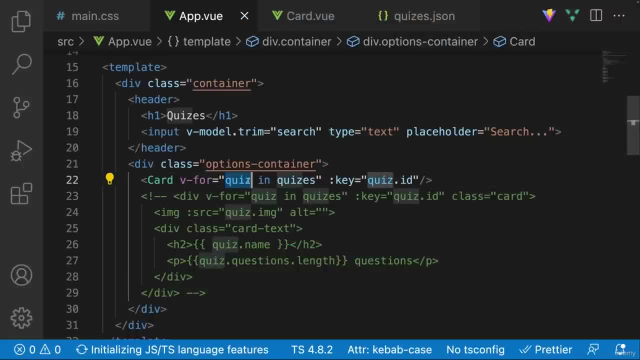 and i think it will make sense so over here what we want to do is very so over here what we want to do is very so over here what we want to do is very simply just pass this quiz 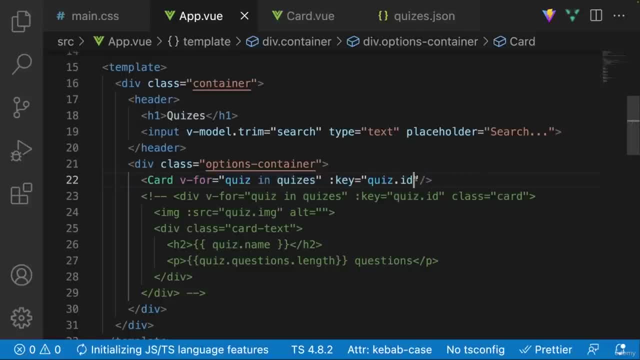 data into this card component so what i'm going to do is i'm going to create another attribute and i'm going to call this quiz and i'm going to go over here i'm going to say that this is going to be equal to and of course this is going to be javascript because i'm adding the colon and i'm going to say quiz so i can call this whatever it is i want this indeed is known as the prop and 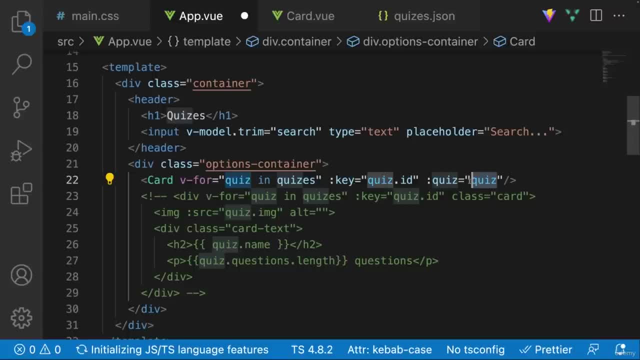 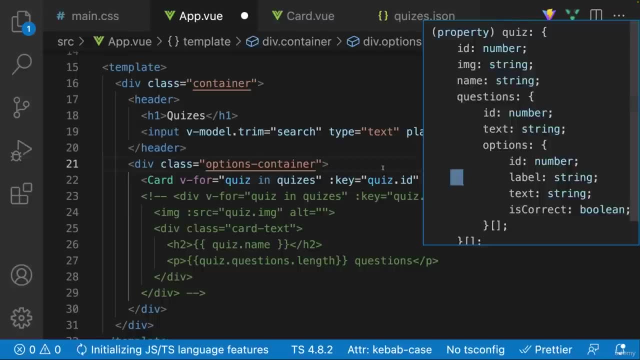 this is what we're going to utilize to access this data which is coming from here which is the object from the card component so again we can call this whatever it is that we want we can call this 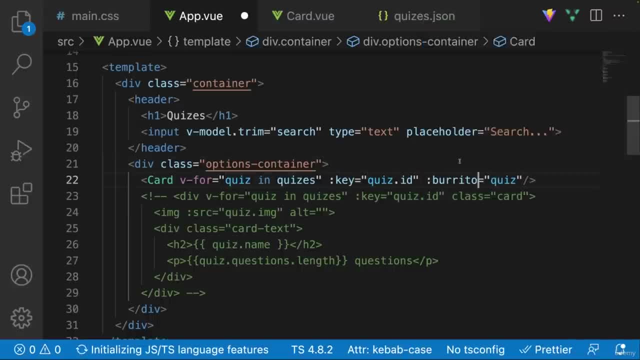 um burrito burrito if we wanted to but it's well good convention to call it something meaningful like exactly what it is because it's a quiz so i'm gonna go ahead and actually save this 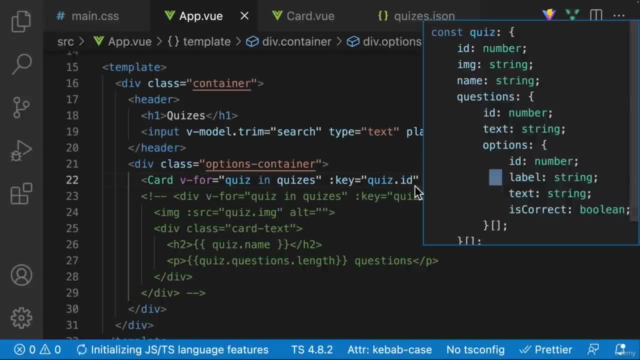 and now we can actually access this data 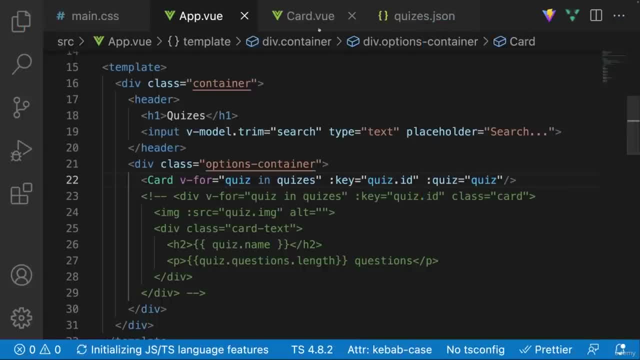 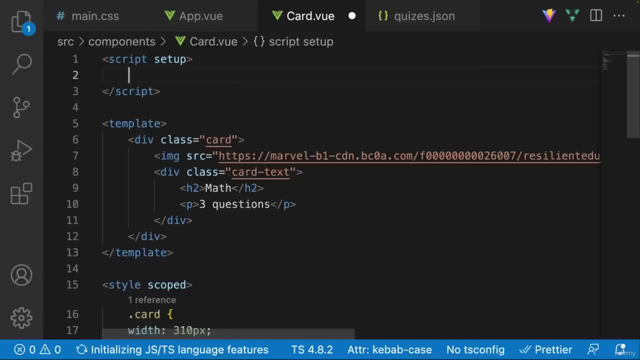 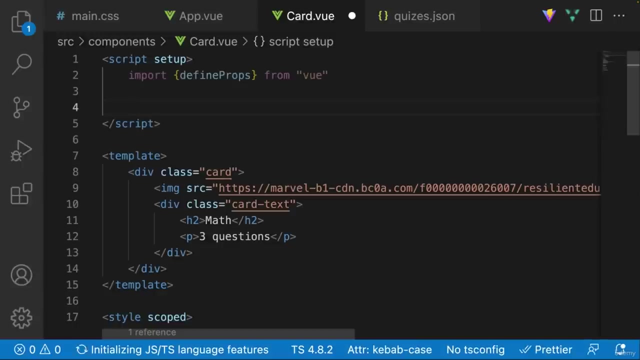 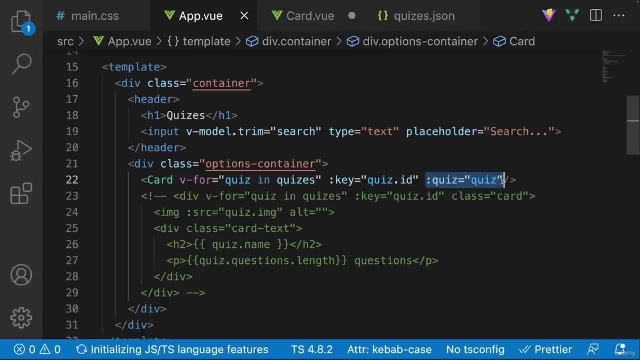 right here like i said but this is going to be able to actually what this would call an object but i'm going to go ahead and actually save this and now we can actually access this data right here over here because we passed it as a prop so let's go over here to our script tags I'm going to say script we're going to say setup and then to access a particular prop we're going to first import something from view so we're going to import something called define props so we're going to say define props like so alright so we're going to import that and then over here what we're going to do is what we're going to create a brand new variable and this variable is going to be called props and it's going to be equal to define props and we're gonna invoke this and this is going to take in a parameter of all of the different props that we want to have access to now in this case we only defined one piece of prop but we could have just as easily passed in many pieces of prop for example maybe instead of passing the object itself we have passed everything separately like for example the image and we could have done here uh maybe we could have called it something like quiz image like so and over here we could have done something 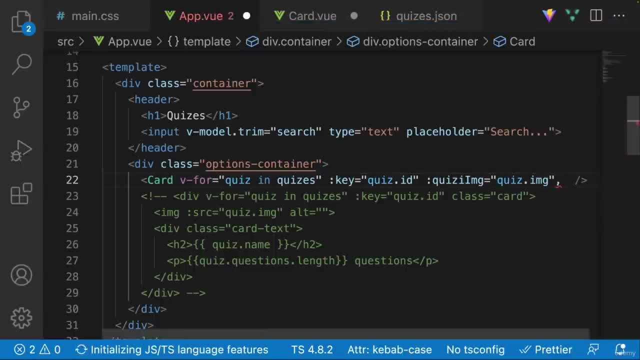 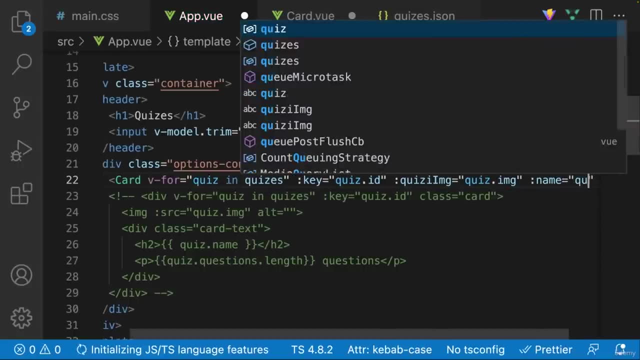 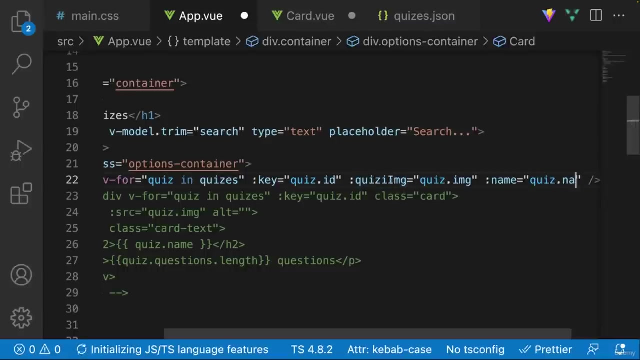 like quiz dot image and then over here we could have also done uh name and then we could have done here quiz dot name so we could have done this just as easily and this would have been just as valid now of course this isn't that elegant i'd rather just pass the whole object itself so let's just go ahead and do that so just because we only passed one that doesn't mean we cannot pass many 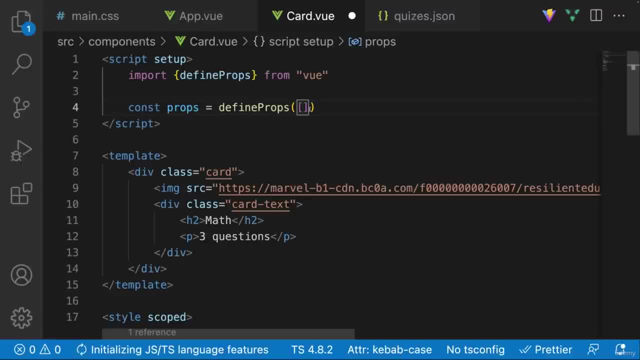 and over here inside of this array we need to define exactly which props we want to have access to within this cart well in this case we just want to have access to the quiz prop and that's really all it is that we need so what i'm going to do here is i'm actually going to go ahead and log the prop just so we can see 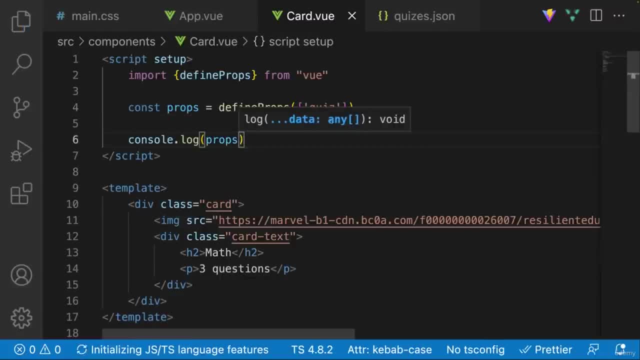 exactly what it looks like so let's do console.log props and if we were to inspect this 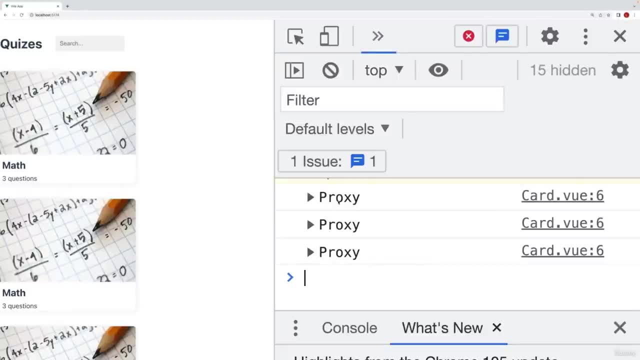 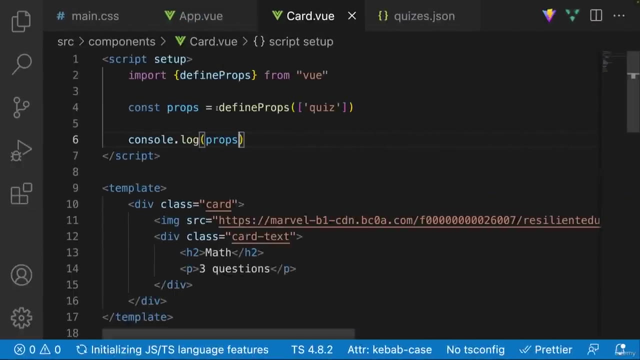 and to console you can see that we actually get this three different times and it seems a little bit funky but really what's actually happening here is it's returning our data back but inside of this proxy so what we can actually very simply do in order to access our data without having to deal with this proxy stuff 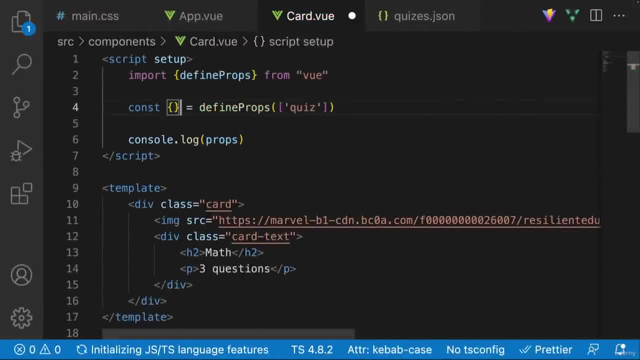 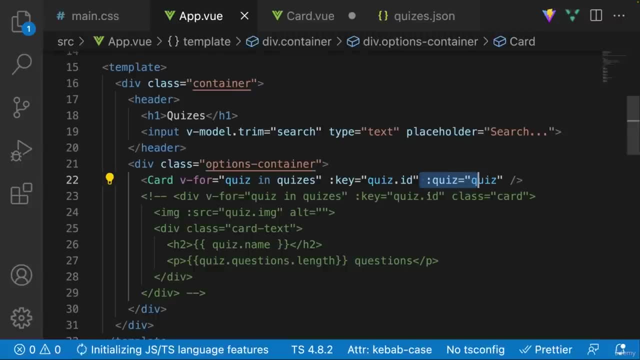 is to just destructure what we want so we're going to say we want the quiz and this is going to be of course the exact same name as we have defined right over here and defined right over here 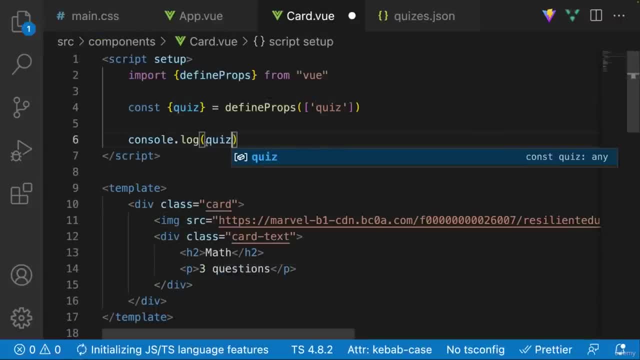 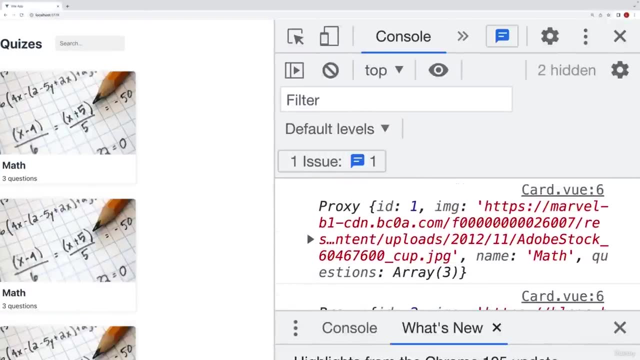 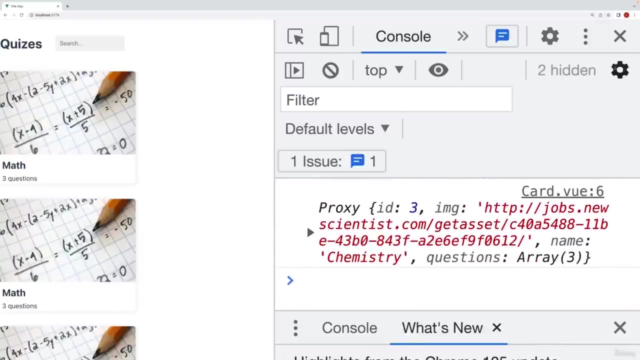 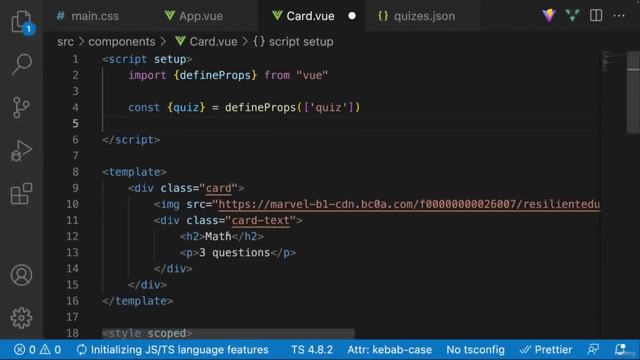 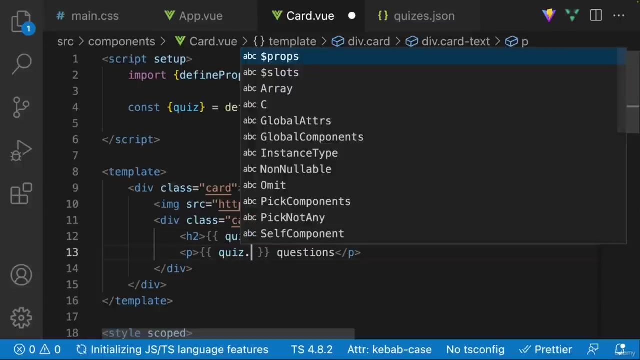 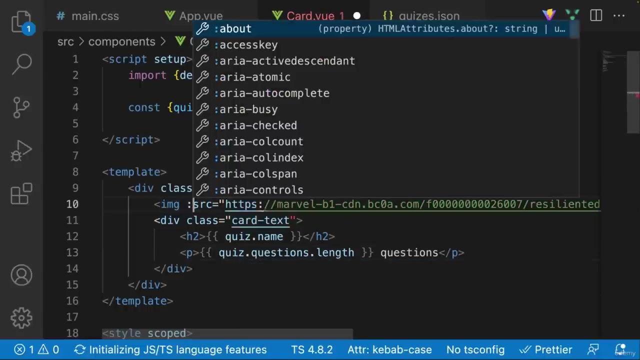 so we're going to say quiz and this time i'm going to go ahead and console.log the quiz prop and if i were to do a quick little refresh you can see here now we get our data so you can see id of one this one has a name of math this one has a name of biology this one has a name of chemistry pertaining to each particular property so that's exactly what we're going to do here so we're going to call it our card so now now that we have access to that data we can use it right over here so now instead of hard coding math we can say quiz.name so you can say quiz.name instead of hard coding the length we can say quiz dot i forget what it was it was uh what was it in the json file it was called question so we can say question dot length and lastly over here we can turn this into javascript remove this over here and we can 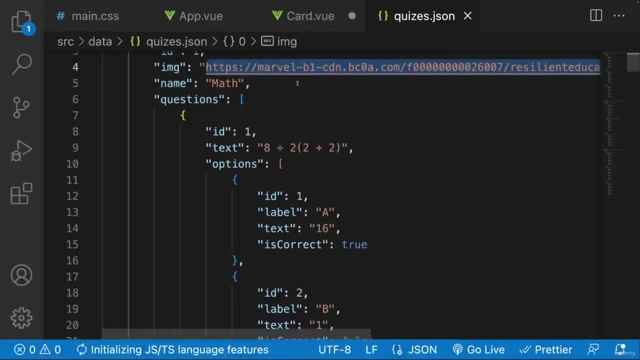 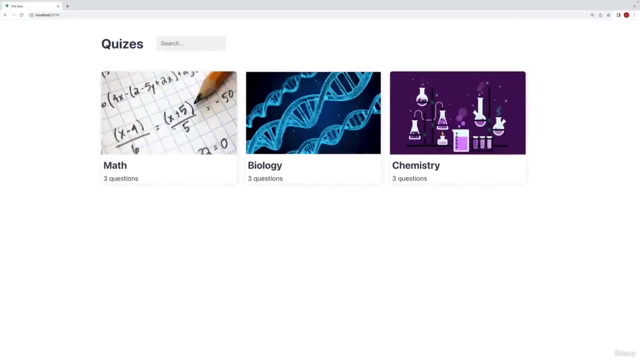 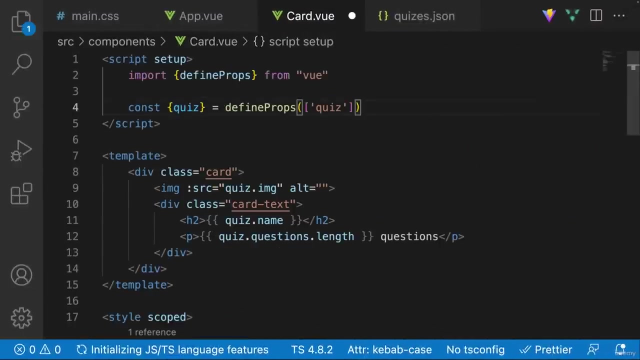 say quiz dot and quiz dot image there we go and there we go so now if i went ahead and saved this you can see we have the exact same behavior but our code is nice and formatted and isolated 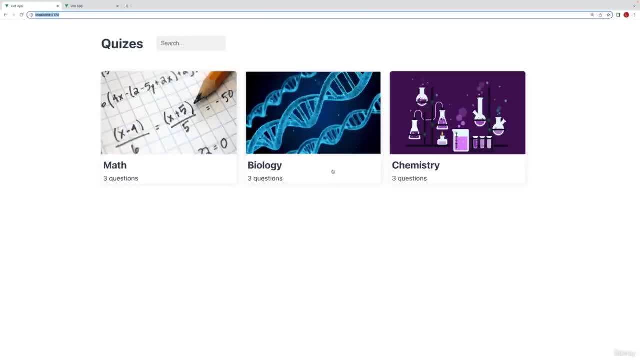 okay everybody welcome to a brand new section so we were able to complete this page right over here we're able to render our cards we were able to of course start filtering for specific cards with watch so this is looking pretty great but now what we want to do is we want to make these cards clickable specifically what we want to do and let's go to the final application here 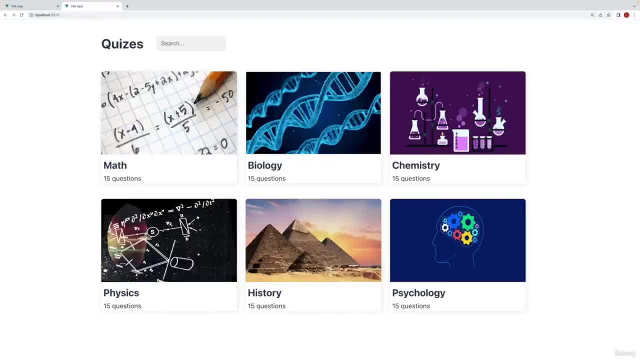 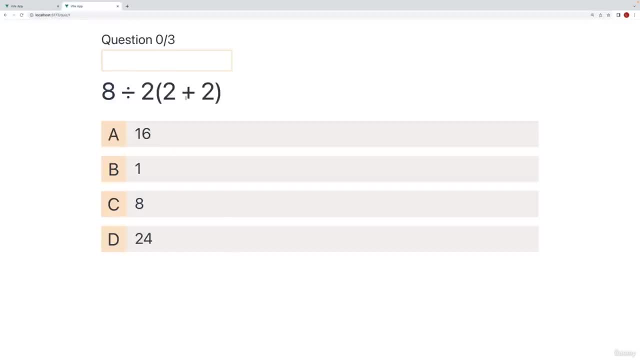 is we want to make these cards clickable so we're going to go to this section here and we're going to go to the final application here and we're going to go to the final application here If I click on a particular card, it's going to redirect me to a different page that is going to be the quiz for that particular card category that I clicked. 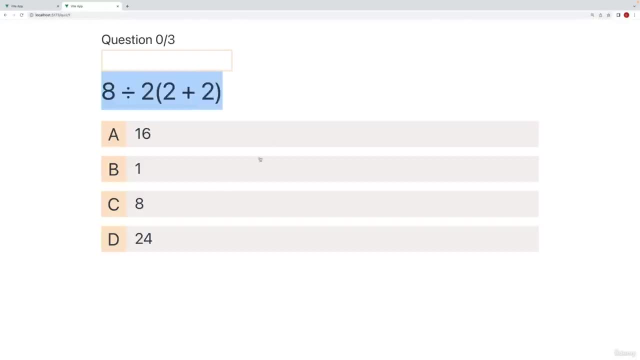 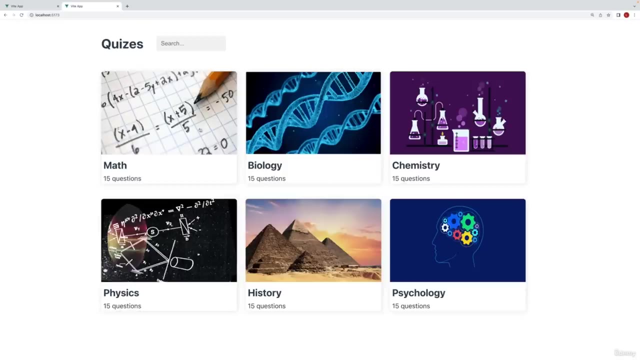 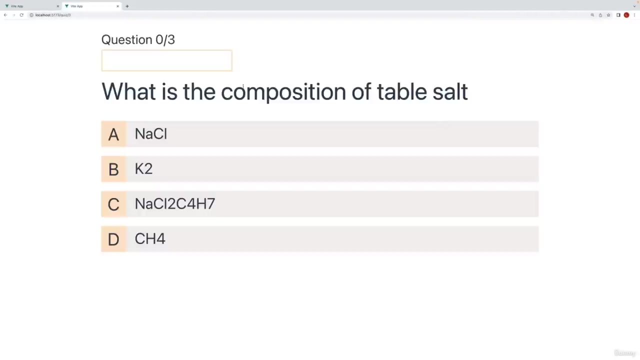 So in this case, it redirected me to this page over here with the quiz of, well, math. And I can go ahead and answer. And then right over here, I can click go back, and it's going to redirect me back to this page. Now, if I were to click on biology, it's going to redirect me now to the quiz for biology. And I can go over here, and I can say whatever it is that I want, and I can go back. So you guys get the point. 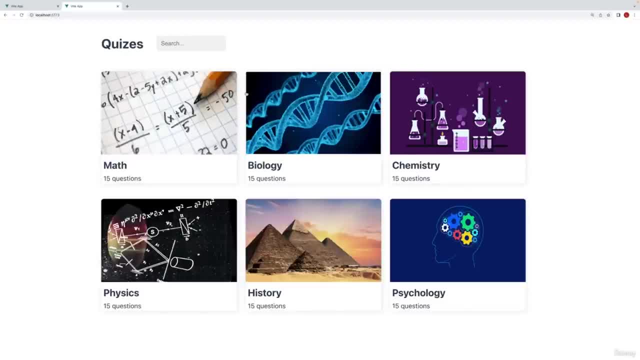 What we want to do now is start introducing multiple pages inside of our view application. And this over here is known as routing. Let me just go ahead and explain with a diagram. 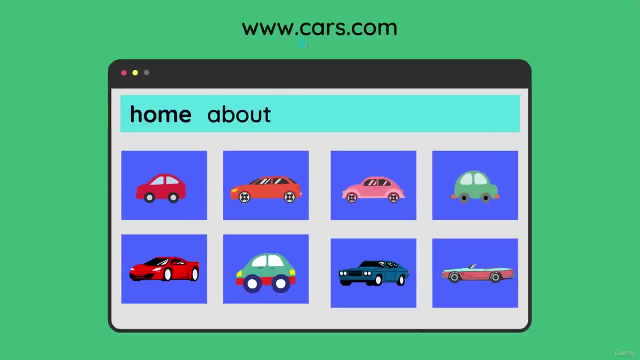 So let's say that we are operating a car website, and our website is on www.cars.com. Very, very simple domain. And as soon as you go on here, you see this nav bar, and you also see a bunch of different cards that you can select. Let's say before you, well, want to purchase any particular car, you want to learn more about the business. So what you do is you click on this about on there. 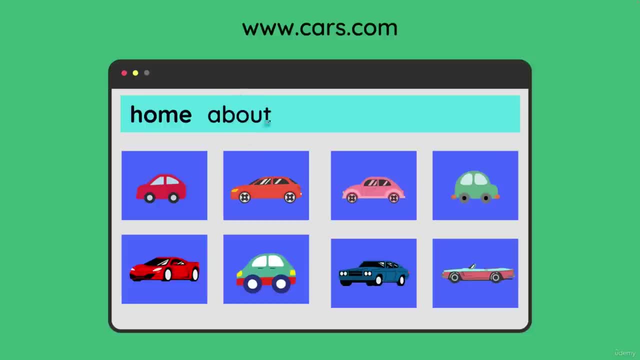 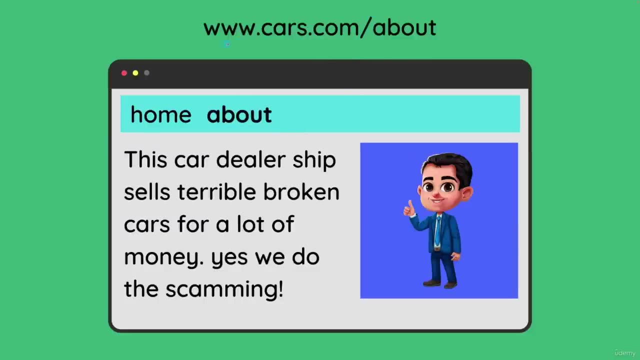 Click on the nav bar, and what this is going to do is redirect you to this page, and it's going to change the route of our application to www.cars.com slash about. 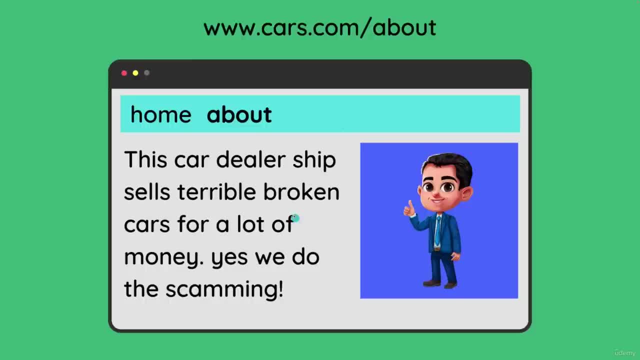 And you can see here that now it's a completely different page with completely different DOM elements. Now we have the dealership and a little text that tells you about the car dealership. Of course, now you can go back and forth, flip back and forth. Different routes that are going to render different types of DOM elements. So this is what we need to know. 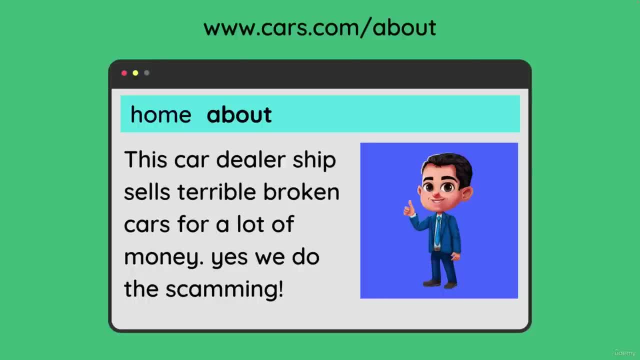 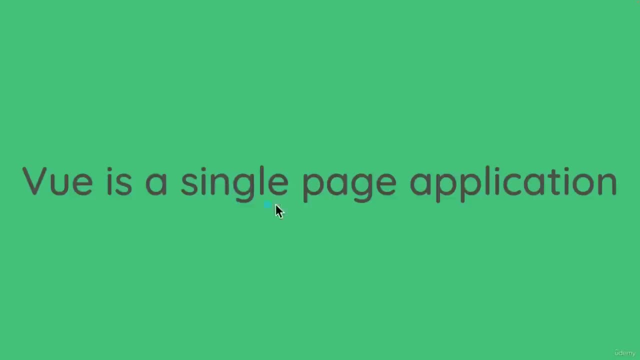 We need to know that routing is just a way that we can render different DOM elements to the user so that we have the illusion of having pages. Now you might be wondering, why in the world am I saying the illusion of having pages? Well, let's quickly remember that Vue is a single page application. Meaning that once we route. 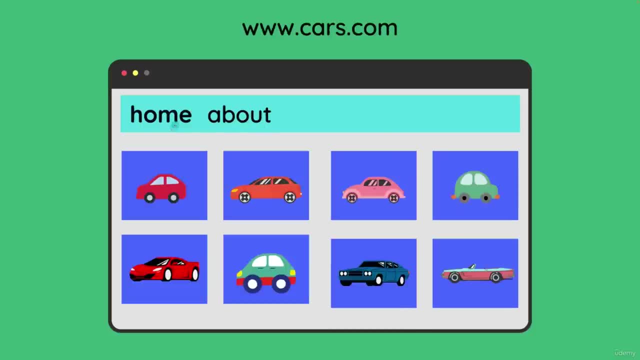 From let's say, home to about, it's still using the exact same HTML file, that index.html file. 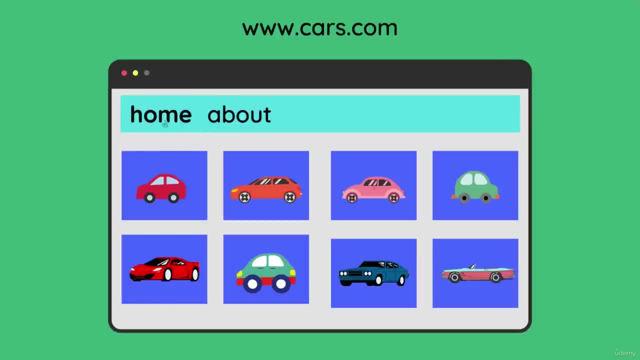 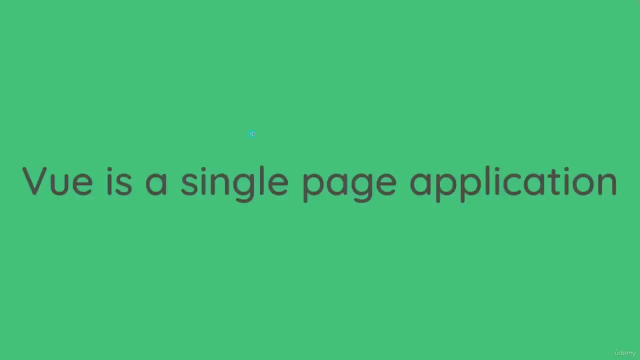 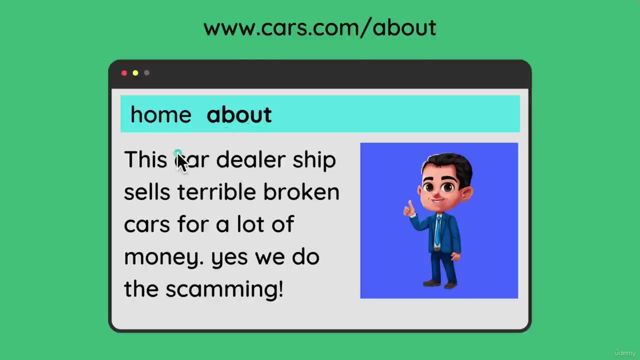 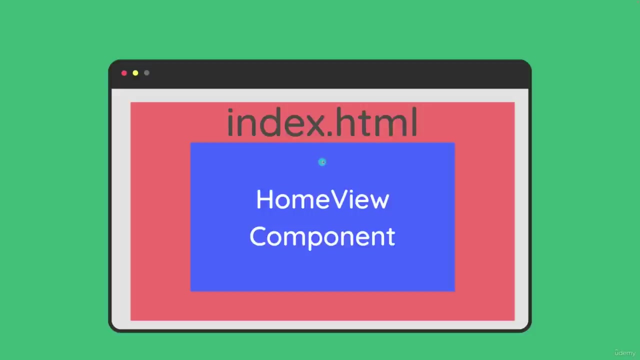 We don't have an index.html file specifically for the home, and then we have another index.html file or another HTML file specifically for the about. We only have one index.html file. So how in the world are we going to be able to render different pages if you only have one HTML file? Well, we're going to do it with components. And that's why it's really important to understand the components. So we're going to have multiple different components. For example, we're going to have the home view component. And if we are at the path of www.cars.com without any particular route, our JavaScript is going to render this component right over here. 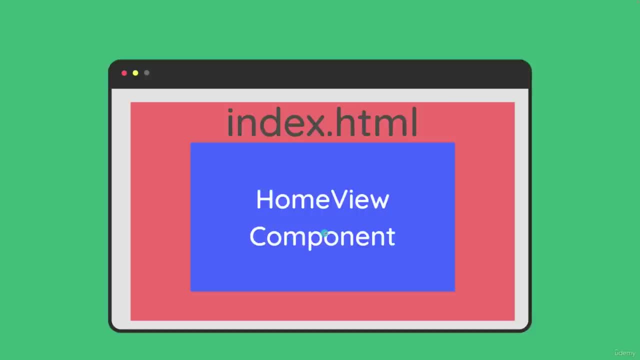 The home view component. However, let's say we go to slash about that route. Then we're still going to use the index.html file. So we're going to have the exact same index.html file, but our JavaScript is just going to remove this component and render maybe the about view component. 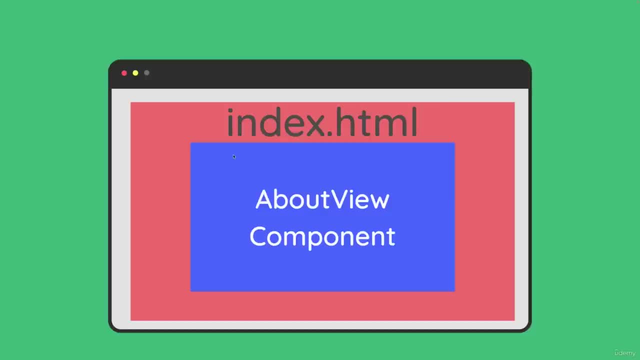 And that way, even though, again, it's one page, we are switching DOM elements unless we have the illusion of having multiple different pages. So this is what we are going to do, and this is what we are going to learn. So let's go about it in the next video. 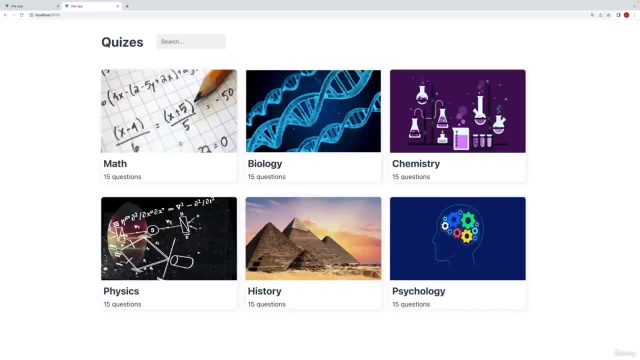 Just because this stuff can be relatively complicated, routing can be a really difficult thing to understand at first. What we're going to do is create a completely blank view application and just work with routing. 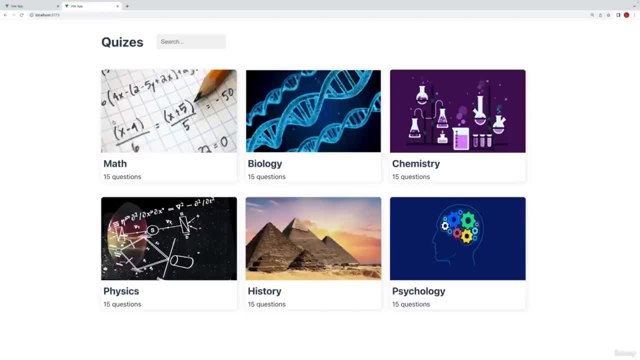 Understand everything that we need to know about routing within that completely blank application. 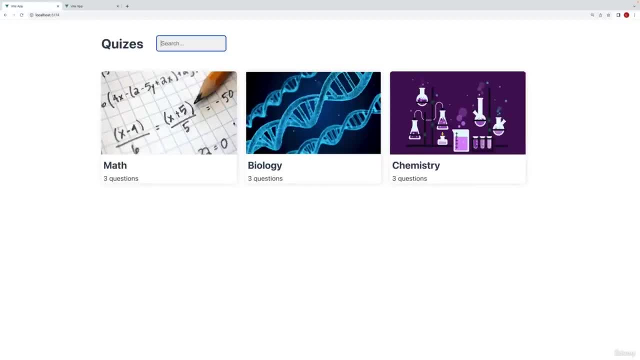 And then we're going to go ahead and translate it to what we have over here inside of our quiz app. So let's go ahead and do that. 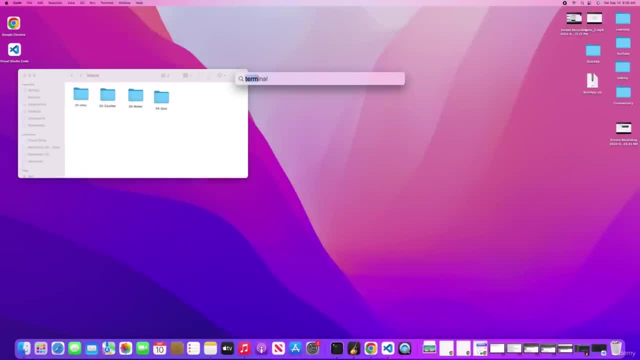 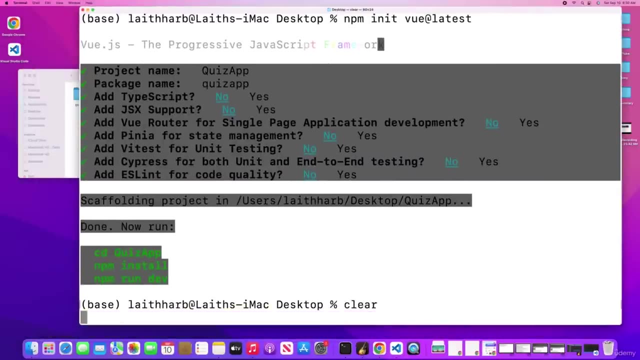 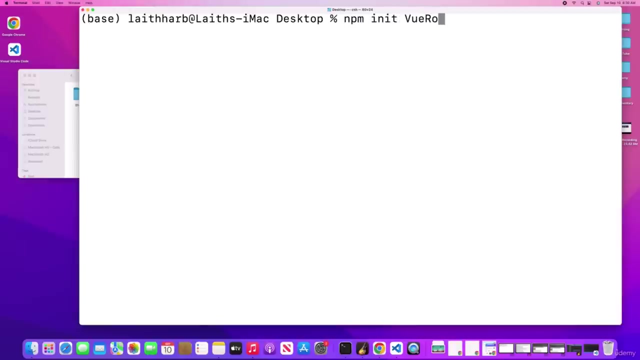 So, of course, what we're going to need to do. Is let's open up our terminal and over here, let's go into my I'm going to do it in my desktop directory and I'm going to create a brand new application with MPM in it. I'm going to say view router and then and then actually we're not going to call a view router that might cause some issues. We're going to call it maybe router view learning. Learning. So that's what we're going to call this. Wonderful app. 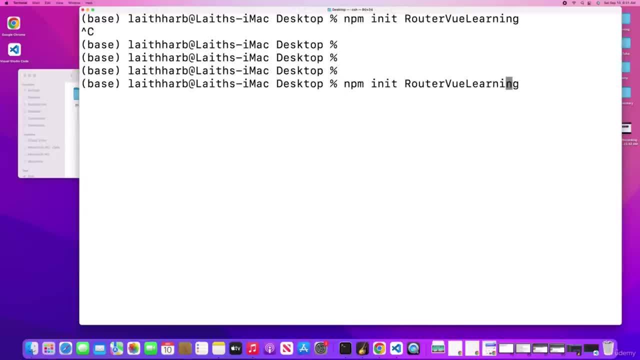 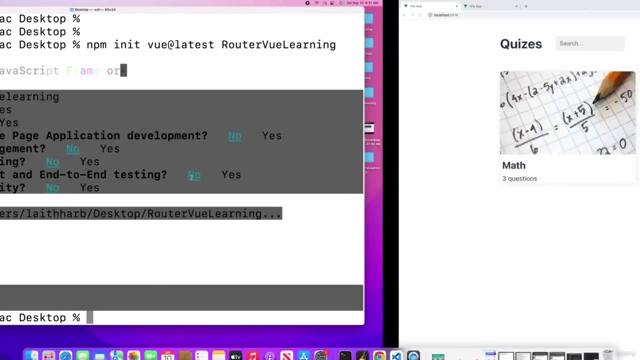 We're going to go ahead and initialize it. And, of course, some have to completely forgot to view at latest. And what we can do is you can actually add space and then give the project a name right away. So you can see it's probably not even going to ask us for the project names could ask us for the package name. So I'm going to say enter, enter, enter, enter, enter, and then enter. And then what we're going to do is we're going to open this application inside of this code. So I'm going to go over here. I'm going to open a new. 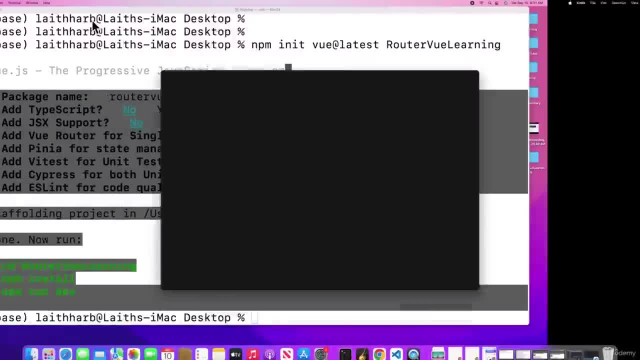 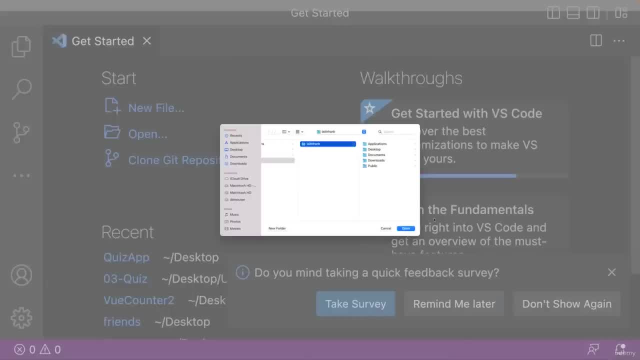 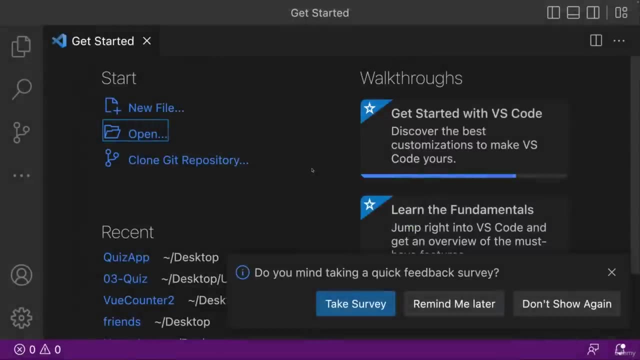 Hex editor and let's just open it up over here. So we're going to say open and we are going to open view router view learning. So we're going to go ahead and open that. And there we go. 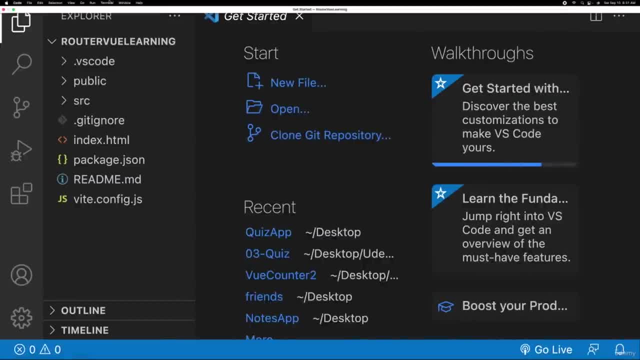 So now it is nice and opened. And now, of course, let's just go ahead and do the MPM install and MPM rundown. So MPM. Sway for the terminal to render taking a while. There we go. MPM install. To install all of the different dependencies. 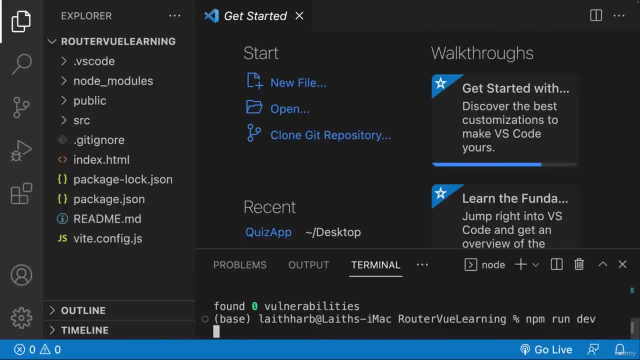 And lastly, let's do an MPM run dev just to run the application. There we go. 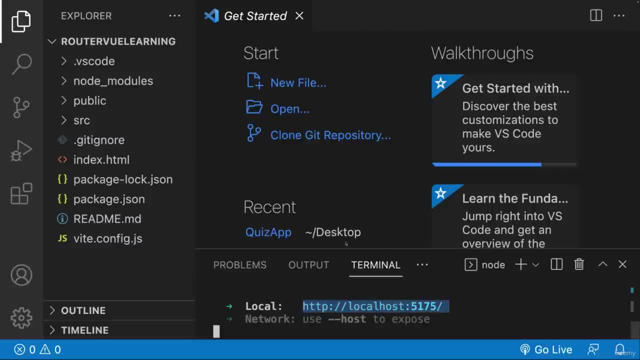 Now it's running on local host five thousand one hundred and seventy five. So for the foreseeable future, we're going to be working on this application until we have a great understanding of React. Router. And then we're going to, of course, translate it back to our app. 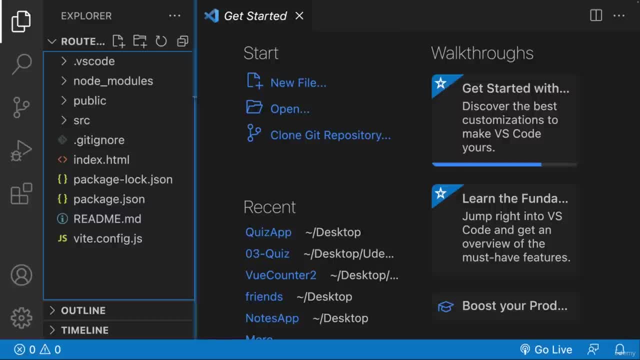 So we just created and ran this boilerplate application. 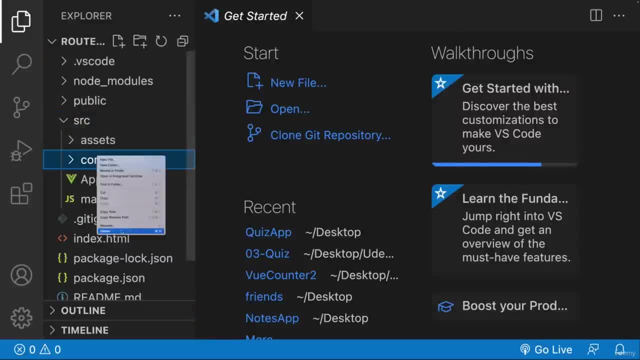 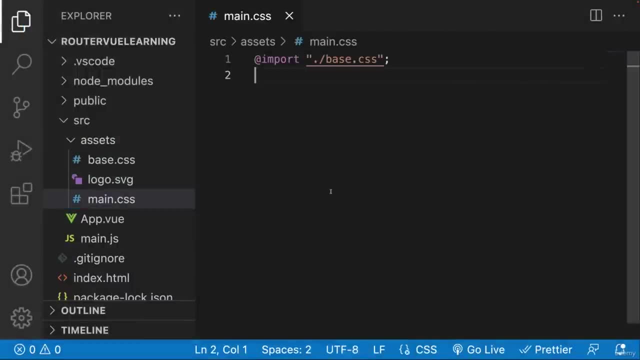 What I'm going to do is we're going to go to the source and just like usual, let's delete the components. Let's go to assets. Let's remove everything under the import. Save that. 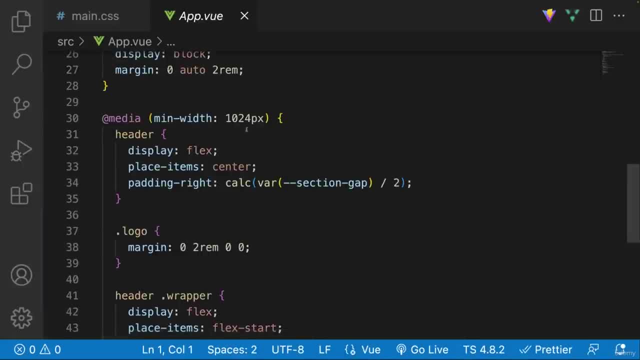 And lastly, let's go to our app dot view file and in our app dot view file. Let's remove everything. So right now we have a completely. Blank slate. 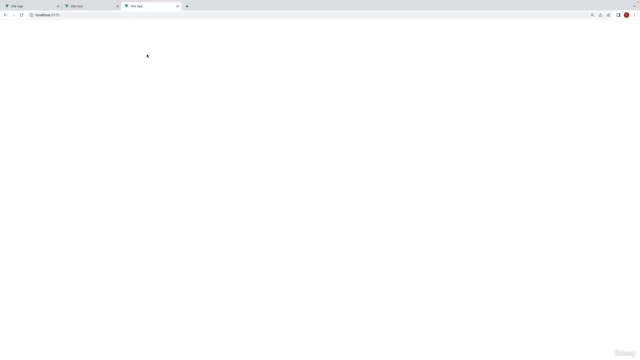 So what we want to have is two different pages, kind of similar to what we had with that cards, cars analogy. 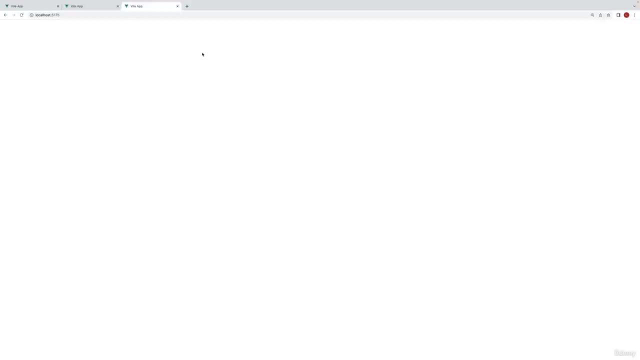 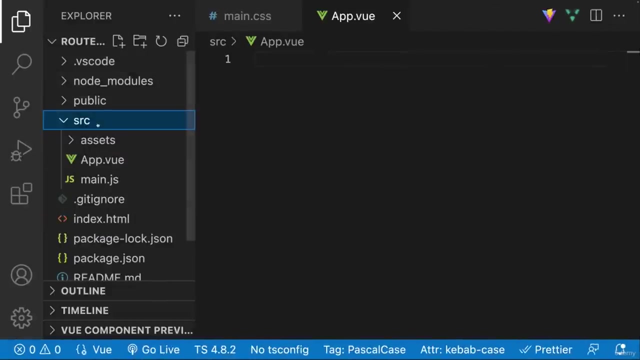 So we want to have a home page and then we also want to have an about page. Now, again, each page is going to be a component within itself. But what we're going to do is actually not store it in the components directory. Instead, what we're going to store it in is a views directory. Now, this doesn't really matter where you store it, but is typically page components. 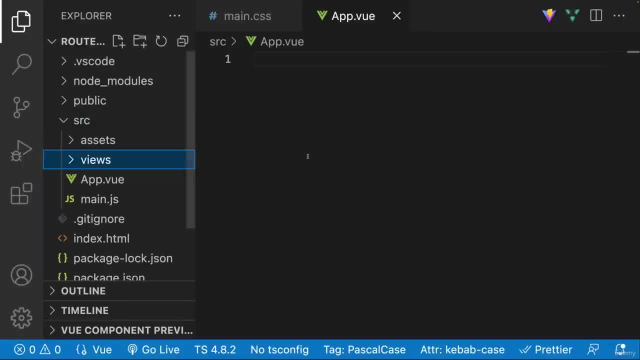 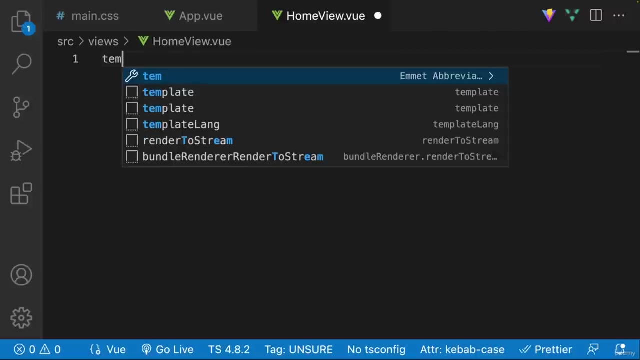 Components are in a views directory, whereas card components or other pieces of components that are reusable across pages are in a components directory. So let's go into this views directory and I'm going to create a home view dot view file. I know that's pretty confusing home view dot view, but notice the spelling is a little bit different. So over here, we're going to have a template and over here, let's have a div. 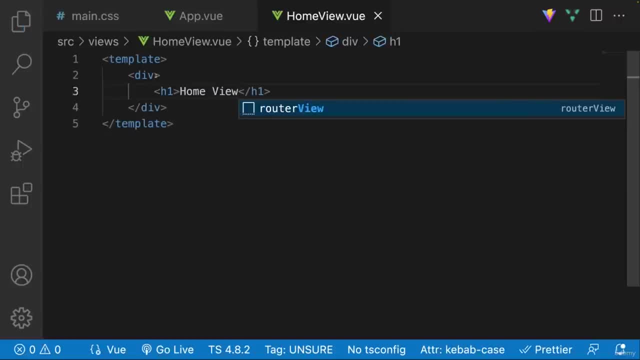 We're going to make this. Very, very simple. We're just going to say home view. That's it. 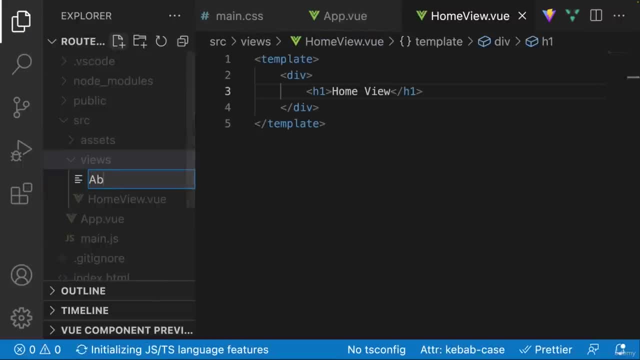 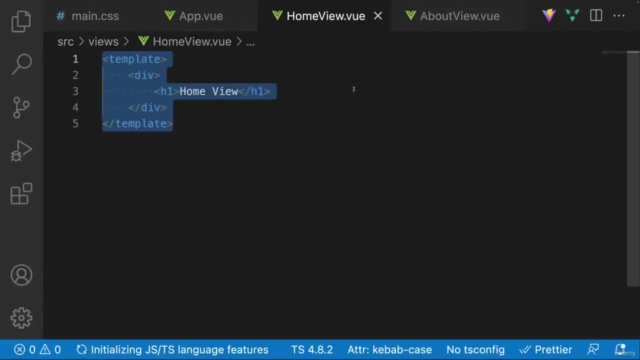 And then we're going to have another page. This one's going to be the about view dot view. And very simply, we're also going to have a div and an H1. But this time, this is going to say about view. 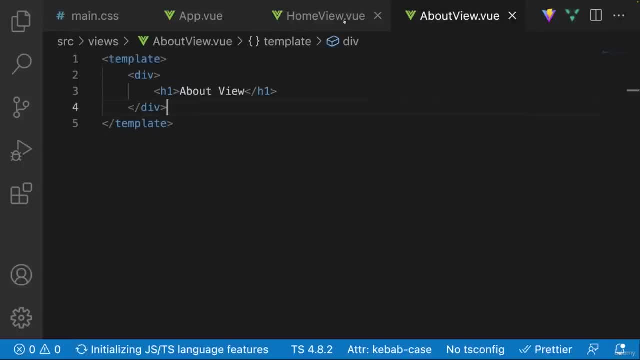 So what we're going to want to do is, of course, conditionally render each component depending on the path. 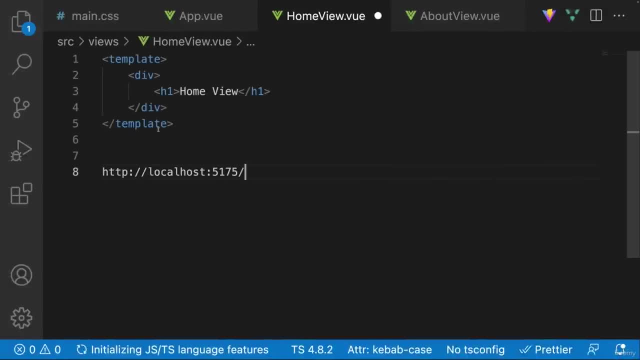 So if we are on, let's say we're on this over here. This path, what we want to do is we want to render the home view. 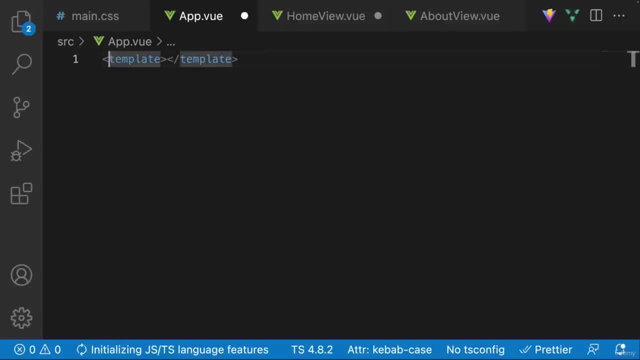 So we would want eventually something that looks like this. Let me just go ahead and import it from the script. 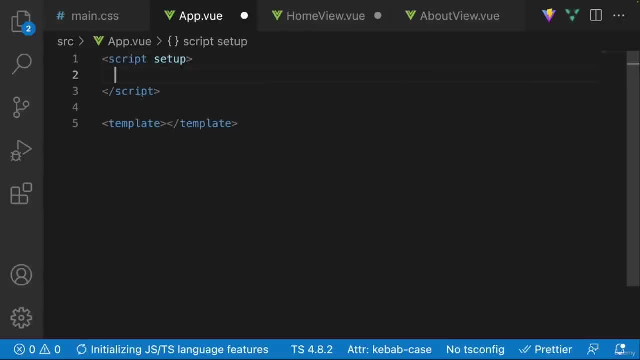 I will say script set up and we're going to import home view from and we're going to import it from the view slash home view. So and let's also import the about view. So about view like so. 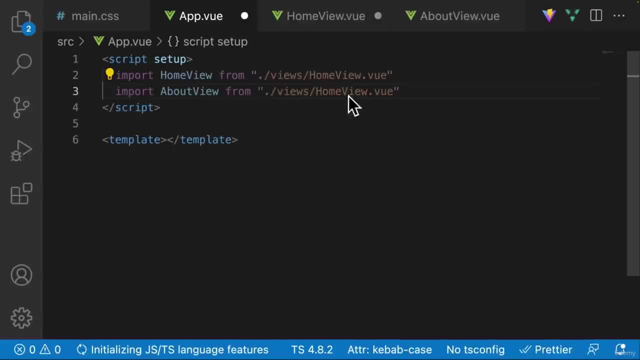 And over here, we're going to get this from about view. So again, if we're on this path right over here, eventually what we're going to want to render is the home view like so. 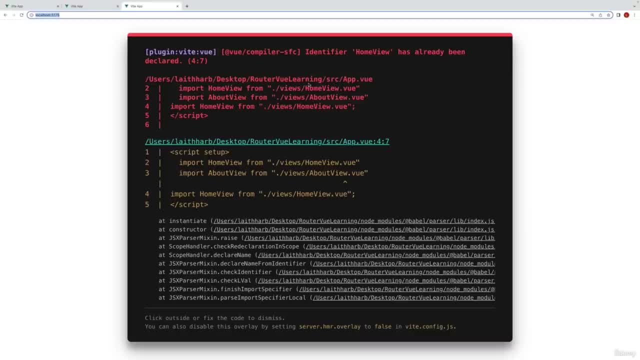 So I'm going to go ahead and save this. And well, of course, nothing is happening here. Home view has already been declared. Yada, yada, yada. 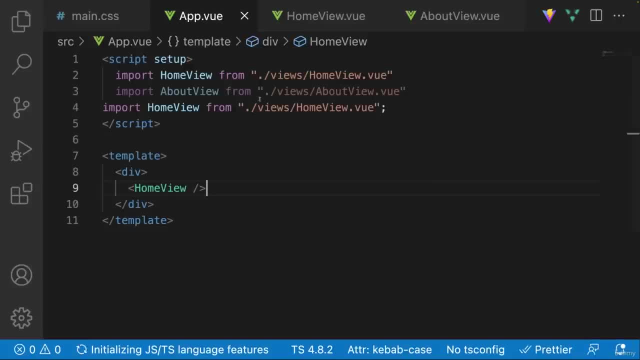 I wonder why that's happening. What's going on here? So home view. Oh, yes. Absolutely. I don't know where that came from. So, yeah. So we're on this path. We want to render this home view component. 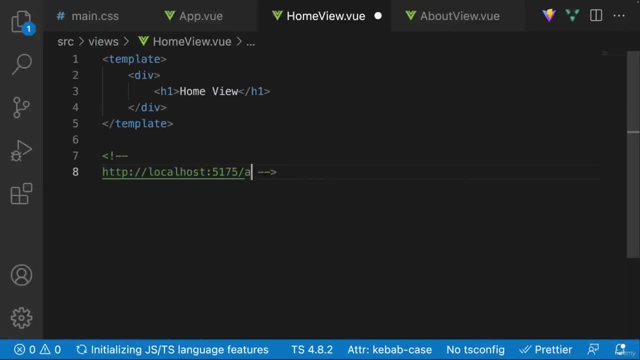 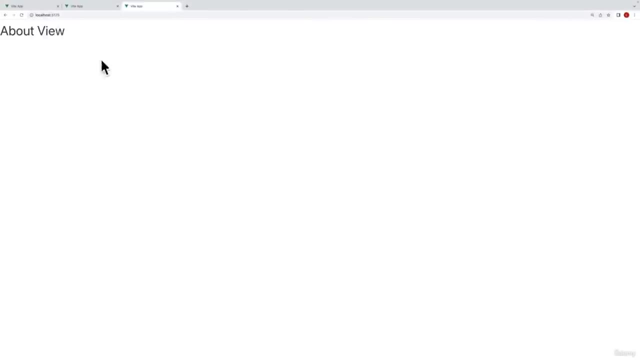 However, if we switch it up to slash, let's say about, then what we want to do is we want to render this component. So, again, the HTML is HTML file is just one one HTML file. 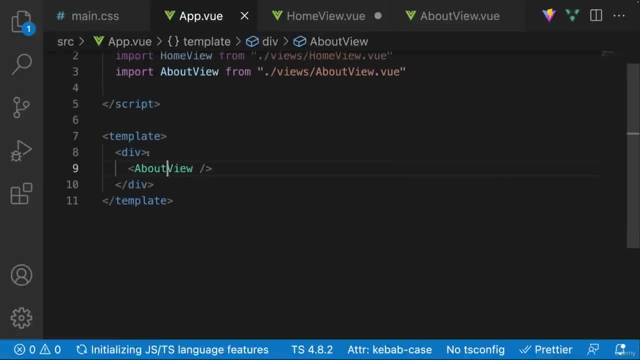 But we're going to be rendering different components. So we're going to actually need to install a library to do this. And we'll talk about that in the next video. 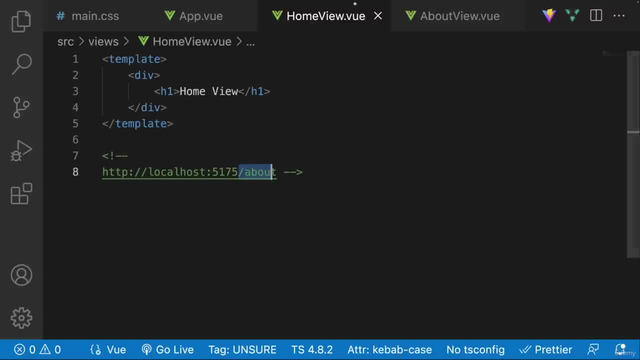 In the last video, we created two different view components. And what we want to do now is conditionally render these components inside of the app dot view file, depending on the path that we're in. 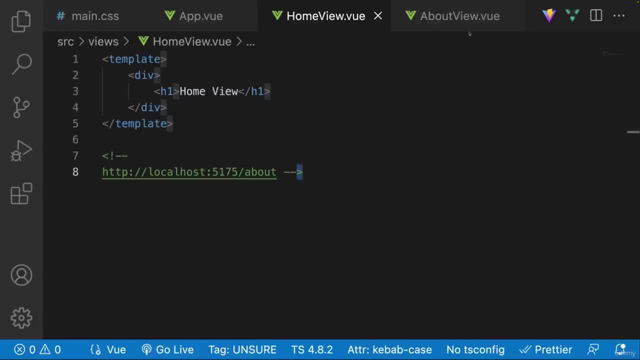 So if we're in the slash path, we want to render the home view. And if we want to go to the slash about, then we want to render the about view component. 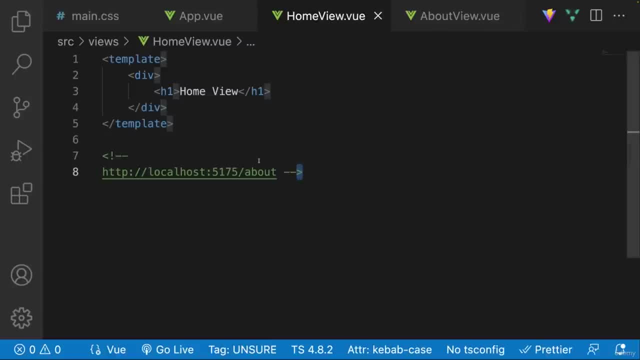 So how are we going to do this? Well, unfortunately, we cannot easily accomplish this with the code that we have ready. So ideally, what we're going to do is need to download some sort of external code that is going to help us out with this. 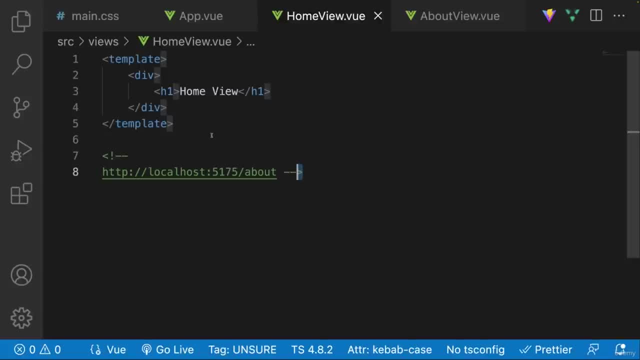 Now, where does this external third party code live? Well, they live as packages inside of MPM. 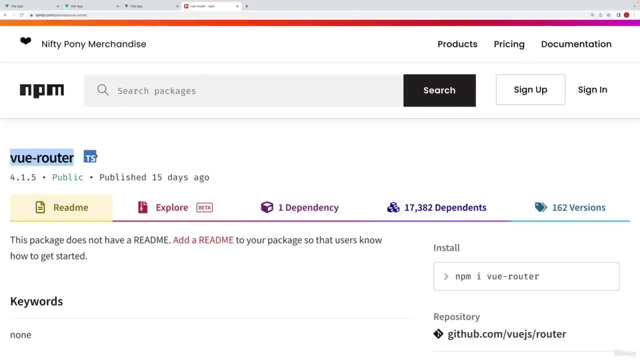 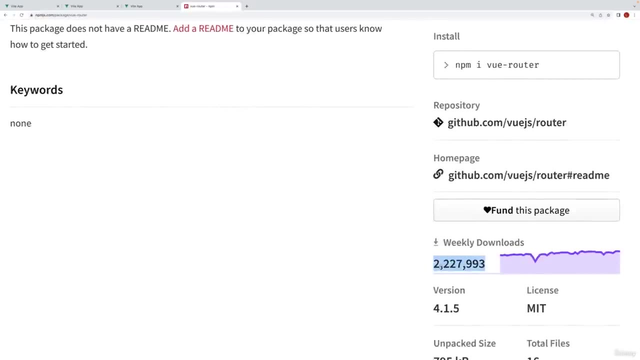 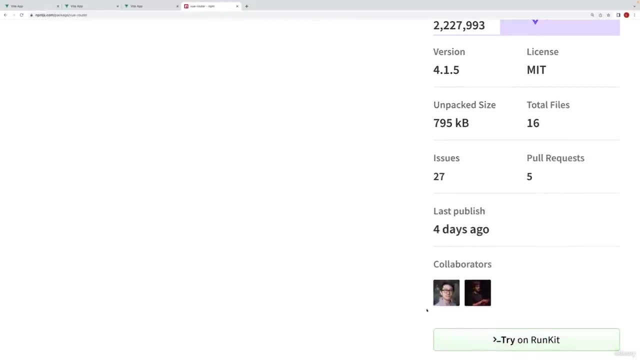 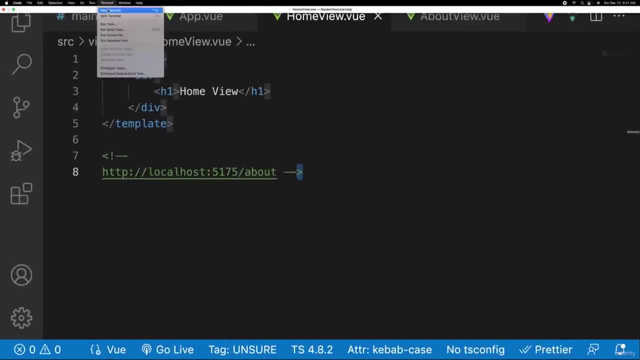 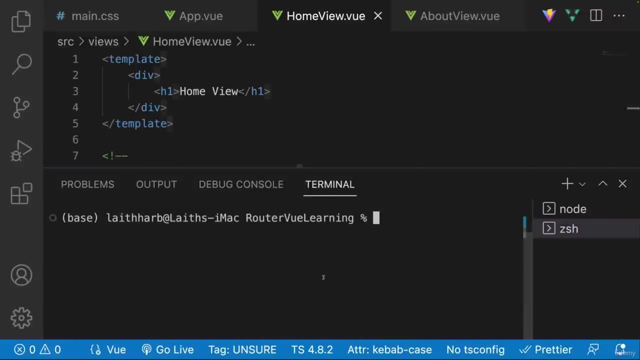 Now, specifically, we're going to download this package right over here, the view router package. And what this is going to allow us to do is, as you can imagine, we'll add routing to our view application. Now, this is an extremely popular package. As you can see, it gets around 2.2 million downloads every week. Extremely, extremely popular. And it is also supported by the creator of view. So it is supported by view itself. So what we're going to do now is we are going to open up our terminal. And we're very simply just going to install this package into our application. 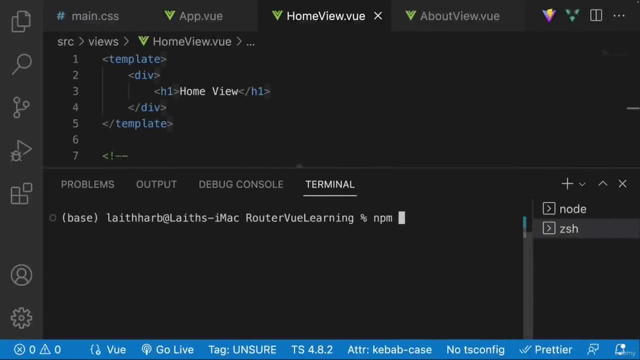 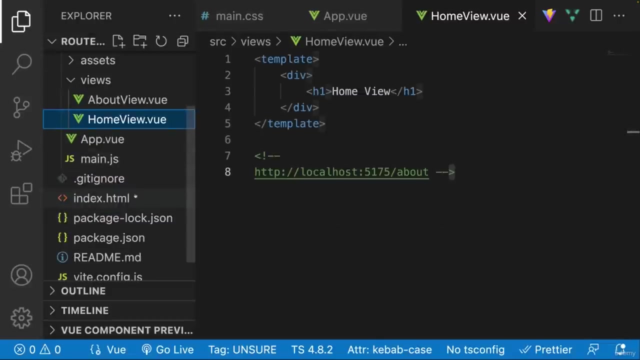 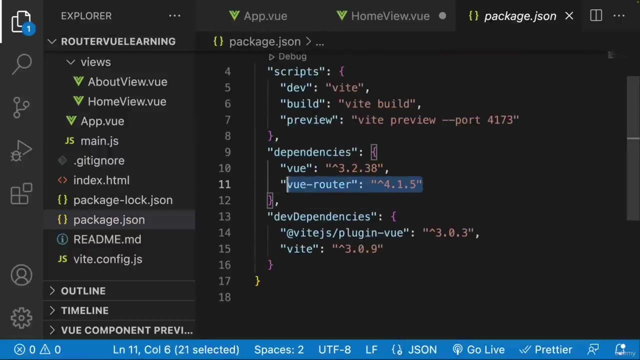 Now, to install a package. What we have to do is MPM, node package manager, install. And we're going to install view router. So this is going to be the package name. So let's go ahead and install this. And what this is going to do is add the source code inside of our node modules. And also, it's going to add it as a dependency inside of our package.json. So you can see over here, we have view router. Let me go ahead and just remove this for now. It's just getting a little crowded. 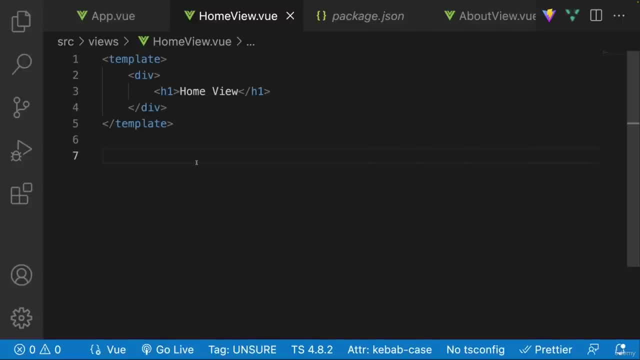 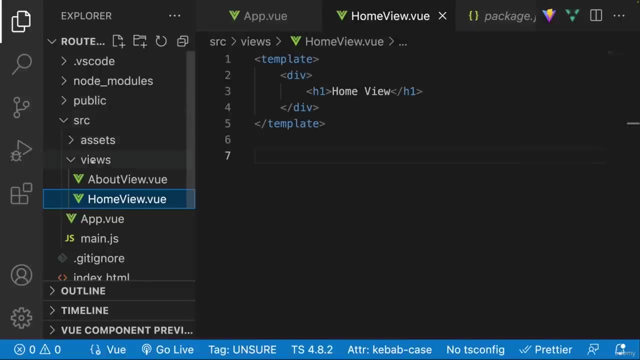 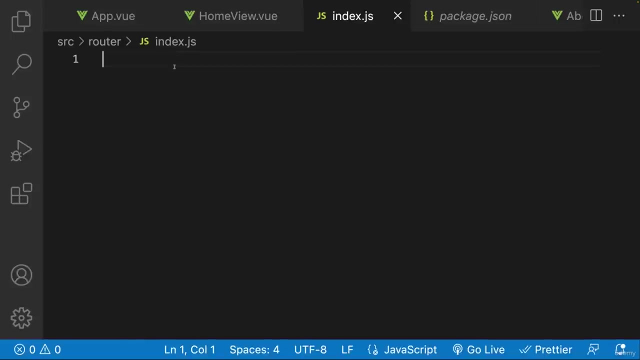 So now that we have that installed, what we can actually do with this is, well, routing. We can actually define our routing rules. So let's go over here. And what we're going to do is we're going to create inside of the source directory a router directory. And inside of the router directory, we're going to create an index.js file. So this is what we're going to do. And in here, we are going to define. I'm going to say define our routing rules. 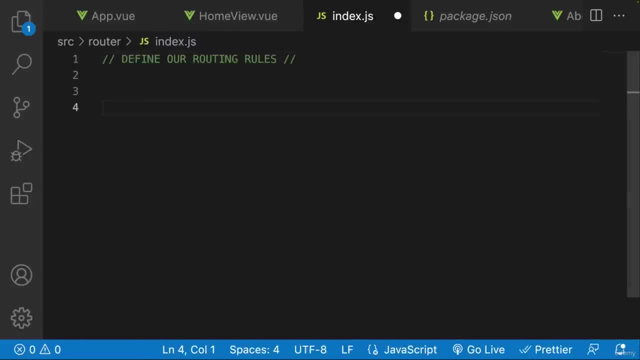 So what are our routing rules? Well, basically, our rules are if you're on the slash route, then we want to render the home view component. 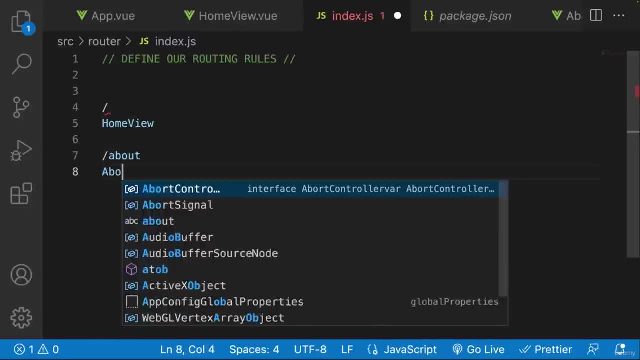 If you're on the about route, then what we want to do is render the about view component. That is what we want to define. 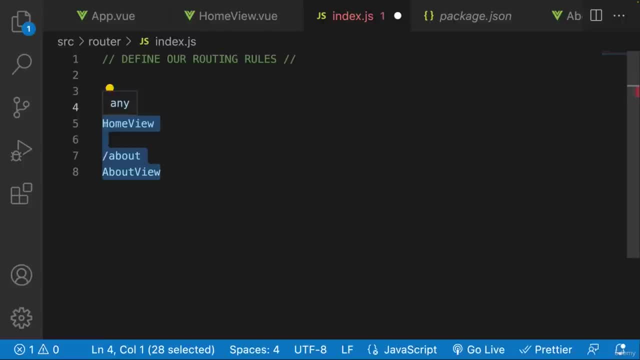 Of course, view doesn't know this right off the bat, so we need to define it. So let's go over here and define it. So in order to define it, what we're going to need to do is import something from the view router. Specifically, we're going to need to import this. We're going to import something called create router like so. 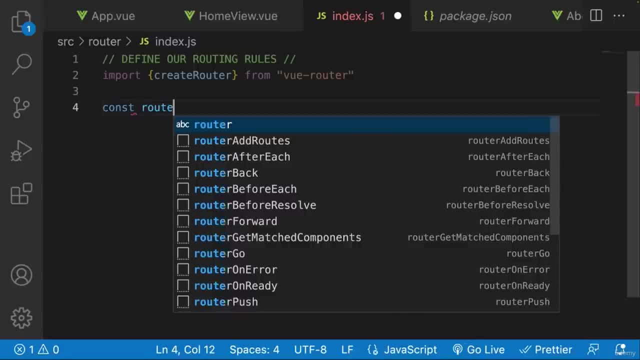 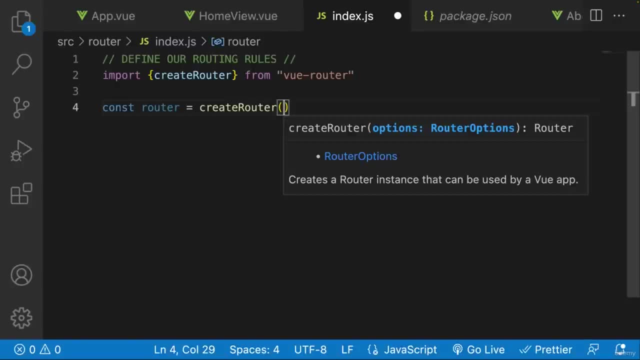 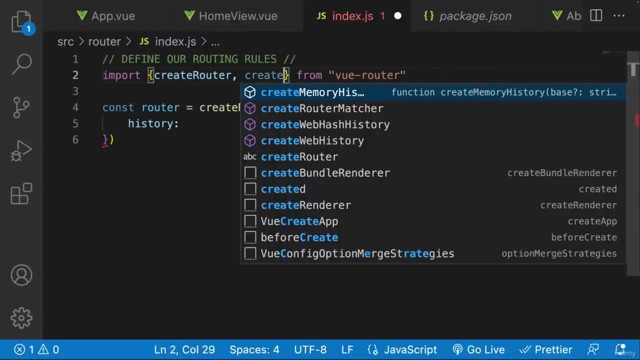 So over here, we're going to say const router. And we're going to say create router. We're going to invoke it. And then we're going to pass in a bunch of options. So this is going to be an object. And then within here, we're going to supply the router with a bunch of different options. So the first option that we are going to supply is going to be the history. And we'll talk about this a little bit later. But for now, what we're going to say is we're going to import something else called create and then web history. 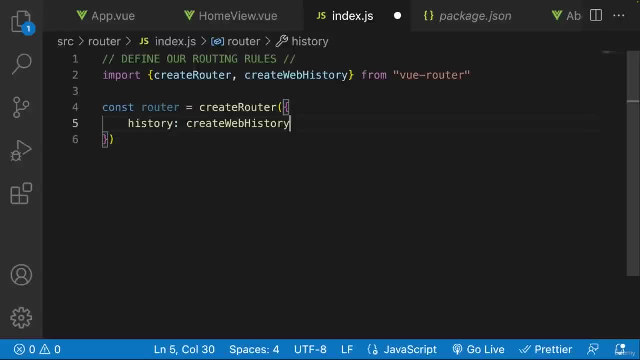 And we're going to say here create web history. 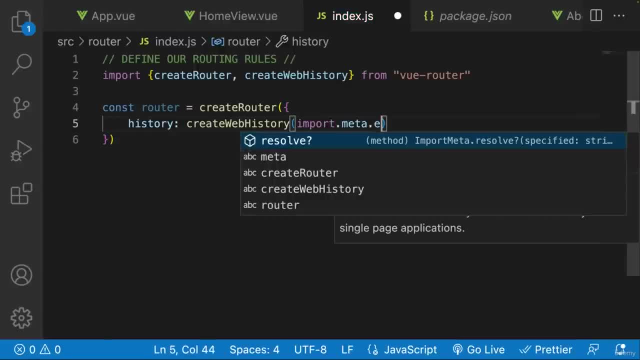 And we're going to do import.meta.env.base underscore URL. So notice the capitalization. So we'll talk about this a little bit later. Do not worry. 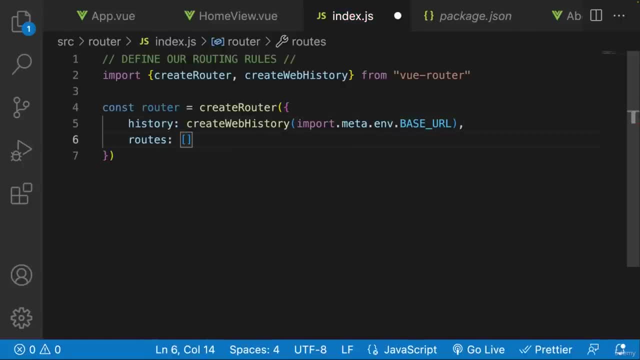 But the other important option that I want to talk about are the routes. And this is actually going to be an array of objects. And we can have as many objects in there as we want so long as we want to actually define them as routing rules. So the first thing is let's go ahead and actually define the rule where if you are on the slash route, then we want to render the home view component. 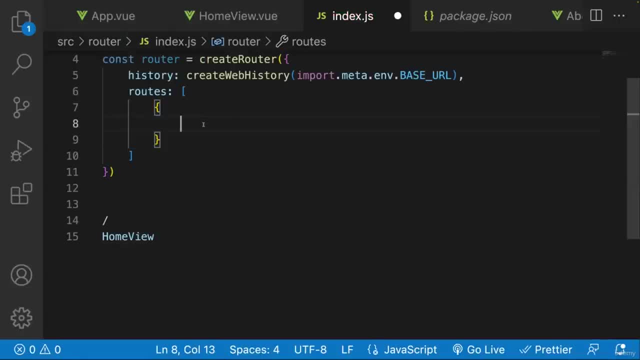 So over here, that's where we're going to define that rule. 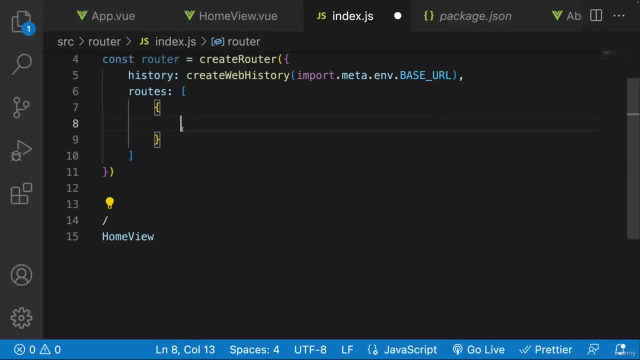 So the first thing to define is this right over here, the path. So we're going to say path. And we're going to say, well, slash. And then if we're on this path, what component do we want to render? Well, you want to render the home view component. 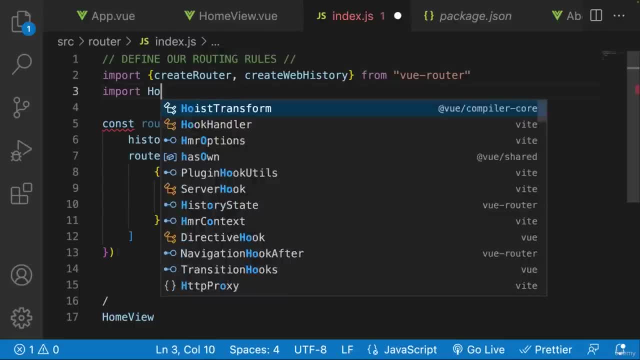 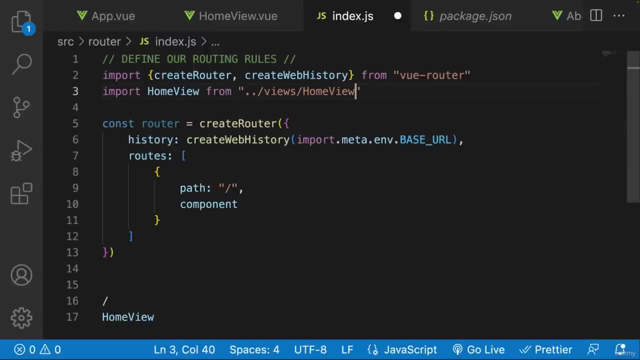 So, of course, what we're going to need to do is actually import that home view component from our views file. So let's go to views. Let's go to homeview.view. 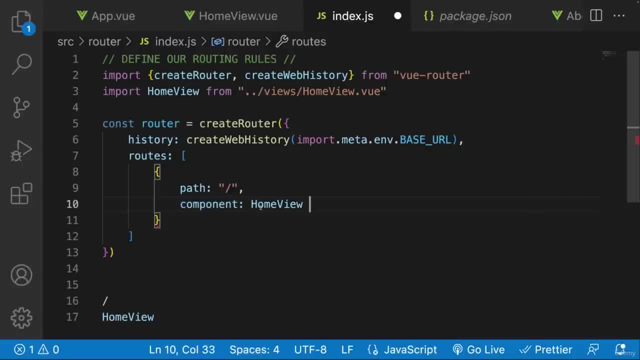 And now what we can do is actually render that component like so. All right. 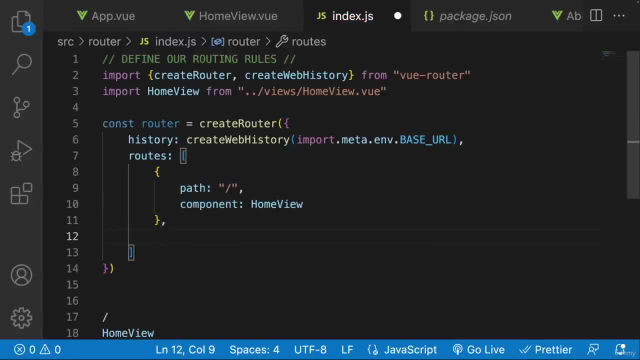 So this is great. Now what we can do is this. 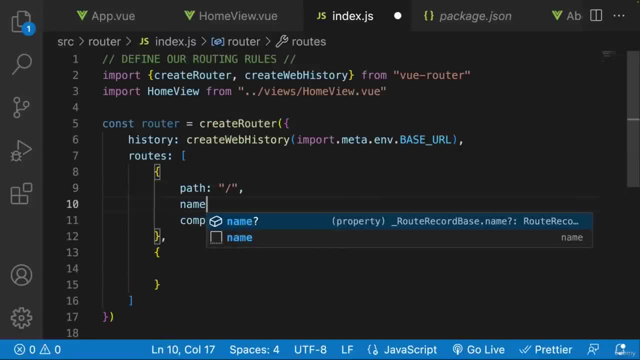 We can define another rule. And actually, it's also a good convention to add a name to your path. So what we're going to say here is this is going to be the home. 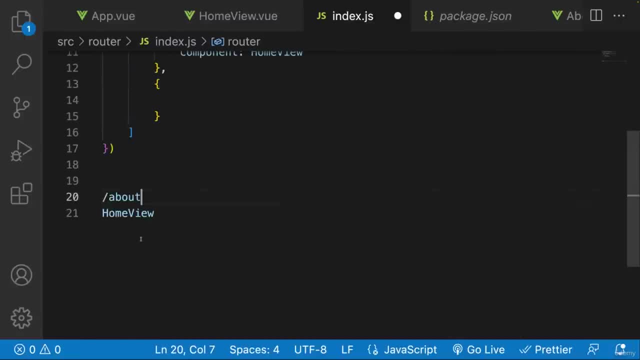 So now let's go ahead and define our other rule where if it's about, then we want to render the about view component. So over here, we're going to say path like so. 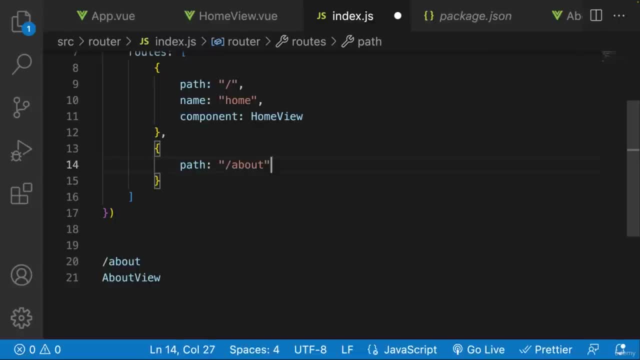 And we're going to say about. So slash about. We're going to give this the name of about. 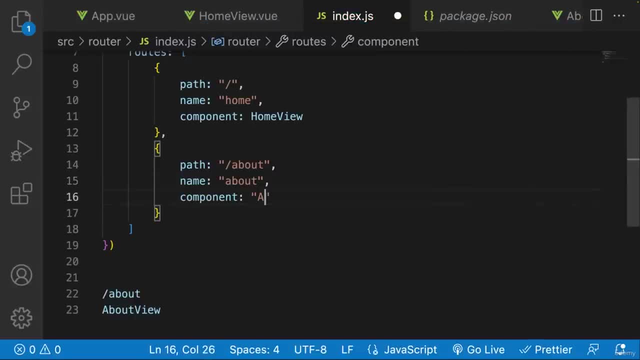 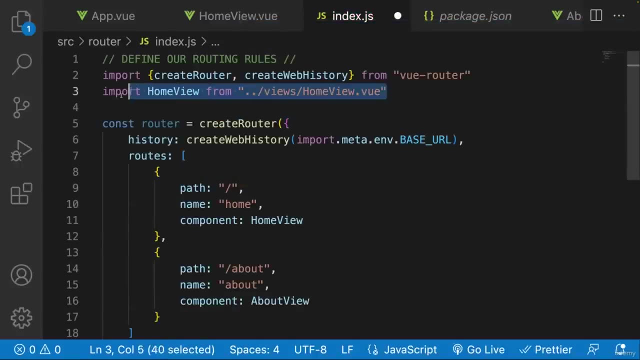 And lastly, we're going to give it a component of about view. So about view like so. Now, of course, what we're going to need to do is import this. 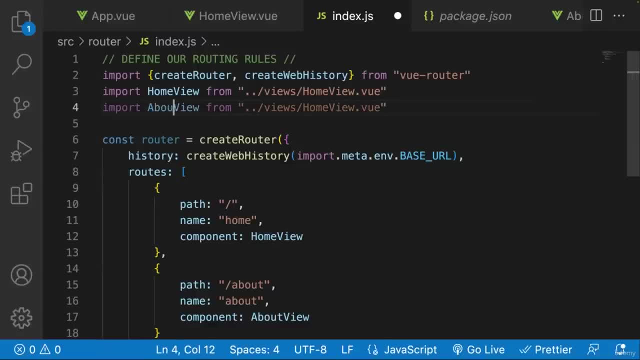 So let's go ahead and import that. So we're going to say about. 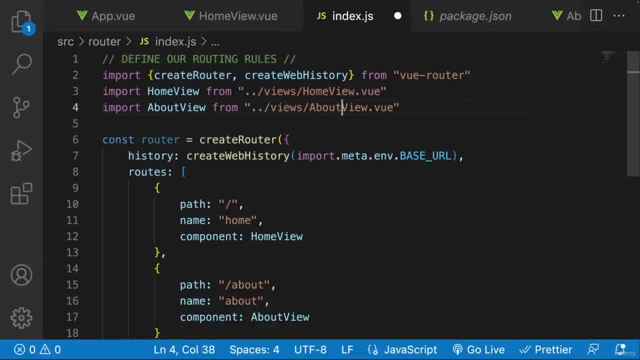 And similarly over here, about like so. All right. Looking great. 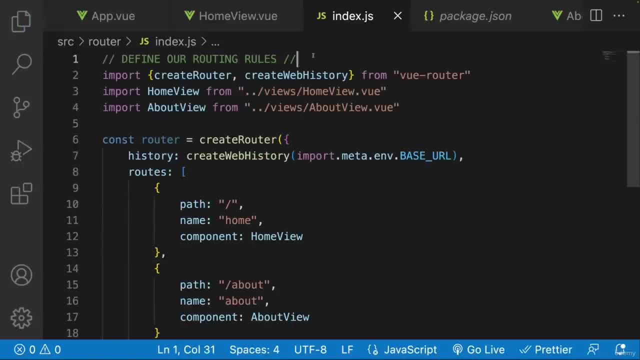 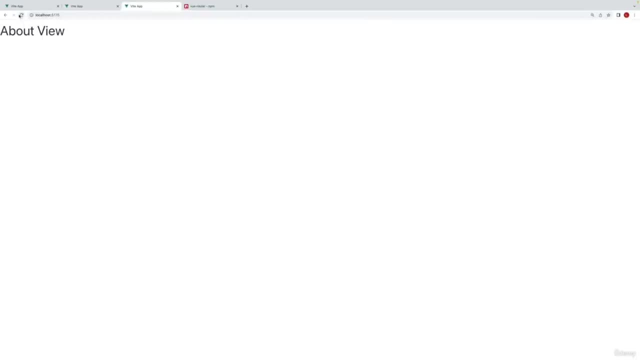 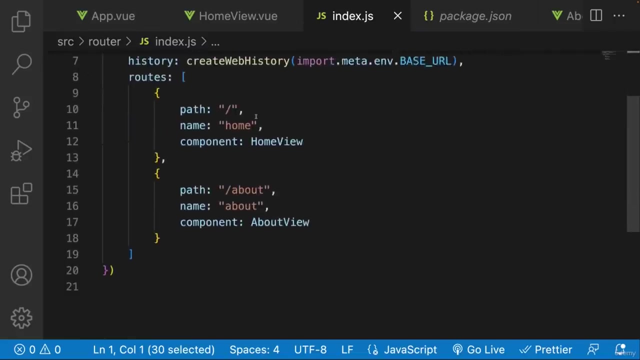 And that's pretty much all it is that we need to do in order to define our routing rules. Now, of course, if we went back to our application here. It's still kind of stuck with our hard-coded about view. So it's not really working. And that's because we just defined the routing rules. We didn't tell view to use them. So now we need to tell view to use these rules. 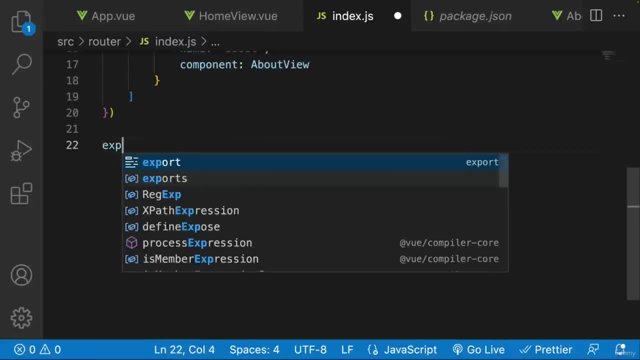 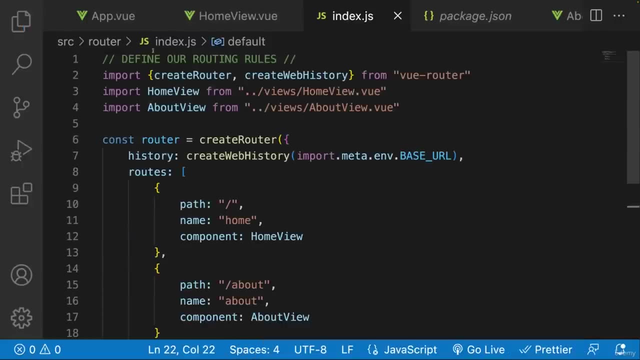 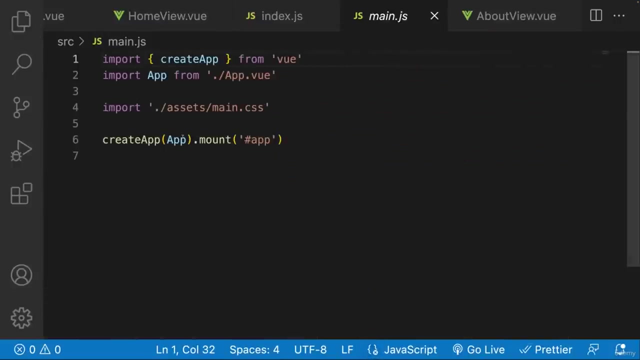 So over here, this router, what we're going to do is we're going to do an export default. And we're going to go ahead and export that router. And now to tell view to use these rules. We're going to go to our router. We're going to go to our main.js file. And then right over here where we actually create our app. Before we create it, what we're going to do is tell our application, our view application, to use the routing rules that we have just defined inside of this file. 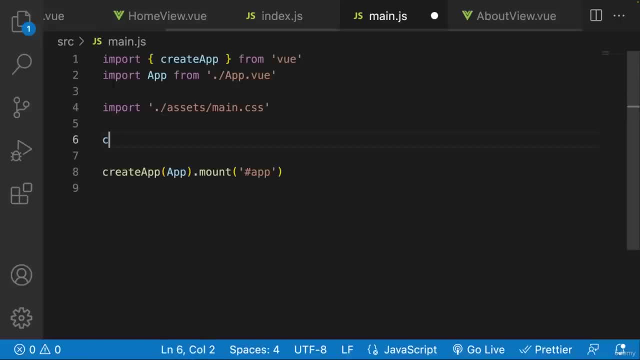 So instead of creating the app and then mounting it right away, what we're going to do is we're going to say const app. 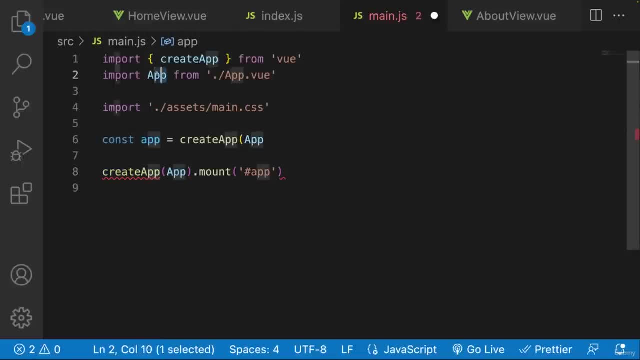 We're going to say that that is going to be equal to create app. And we're going to render the app.view component. So over here, we're just going to very simply say instead of create app.mount, we're just going to say app.mount. And why we did this is now we can actually leverage app before mounting it to utilize different aspects. So what we can say here is app.use. And we can say, hey, we want you to use. And let me go ahead and import the router from the router like so. And we want you to use these routing rules. So now that's pretty much it. 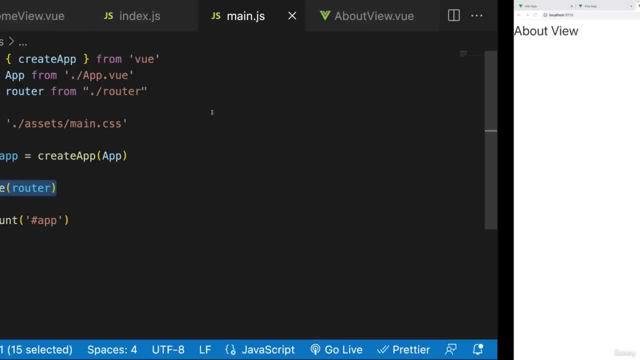 So now we have told view that we want to utilize these routing rules. Now, again, if I refresh, you can see that I'm still seeing the app.view. 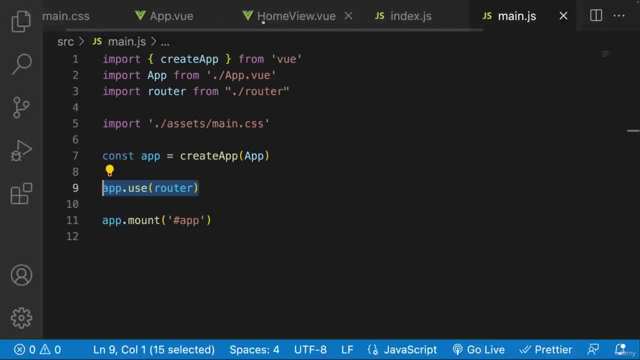 So what did we do thus far? We have defined our routing rules inside of the index.js. 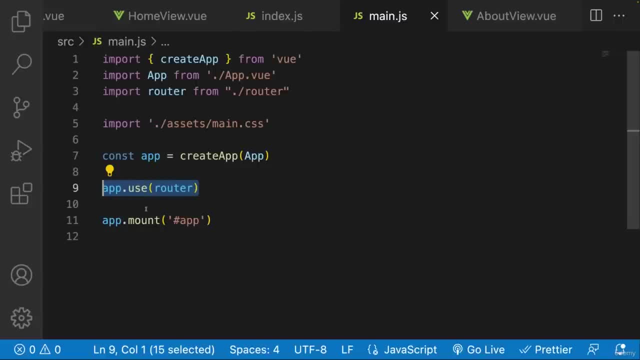 We told view to use these rules by using app.use. But now what we need to do is, 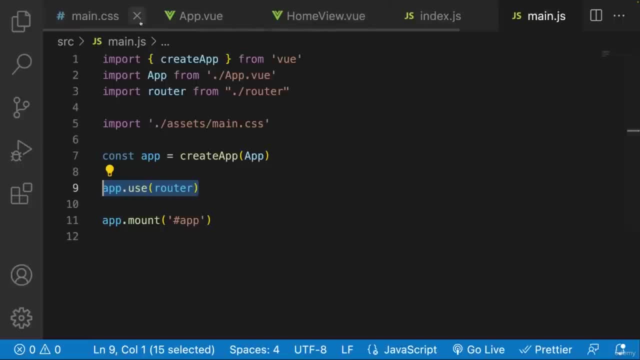 we need to tell view where to use these rules. So specifically, we want to use them inside of the app.view component. And how are we going to do that? 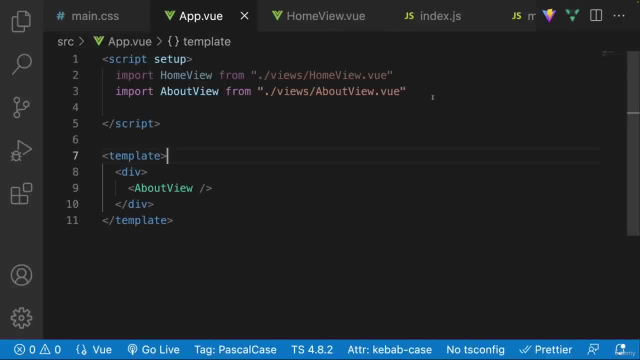 Well, it's actually going to be really, really easy. So instead of actually importing these two, what we're going to do is import another component. And this component is going to be from the view router library. So we're going to say view router. And we're going to import something called router view like so. And we're just very simply going to render this component like so. 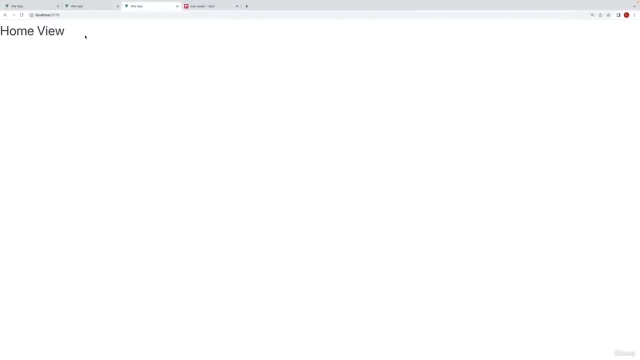 So we're going to go ahead and render this component. And now right away, you can see that we got the home view. 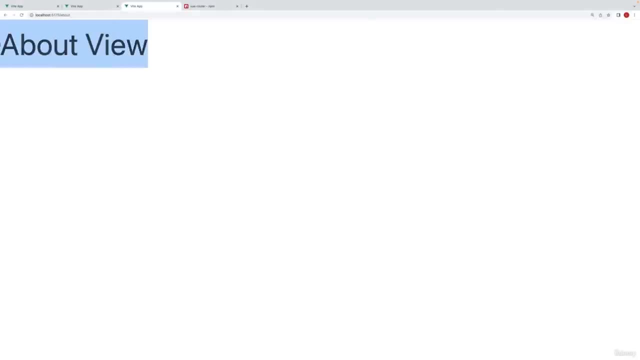 Now I'm going to go to slash about. And you can see that now this changes to the about view. 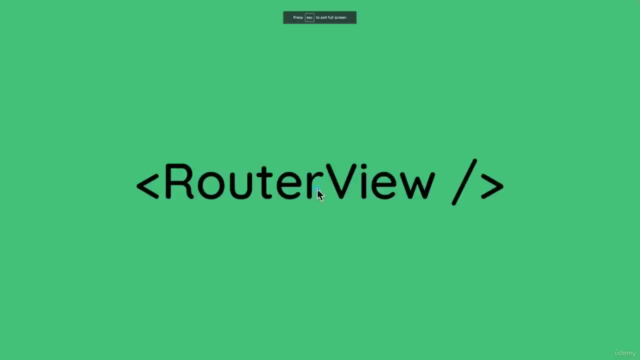 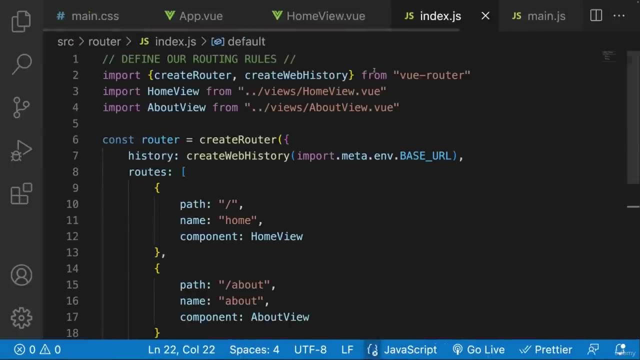 So what is happening here? Well, we have our router view component. And what this is going to do is start reading some of the rules that we have defined over here. So we have defined these rules over here. 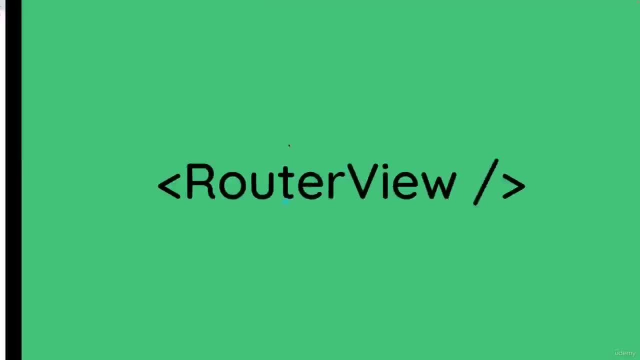 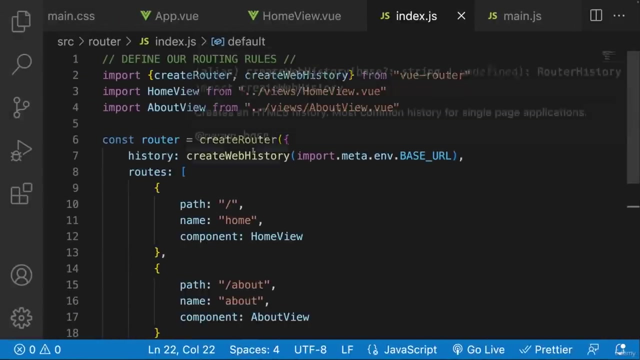 And of course, we connected them to our application. So the router view is going to start looking at the different paths. So it's going to see, oh, we're on the slash path. And because we're on the slash path, it's going to render the home view. And now if we're on the about path, it's going to render the about view. So I know this was quite a bit of setup. But really, this is just something that we have to do once. But it is really, really important to understand. Let's just go through it one quick time. 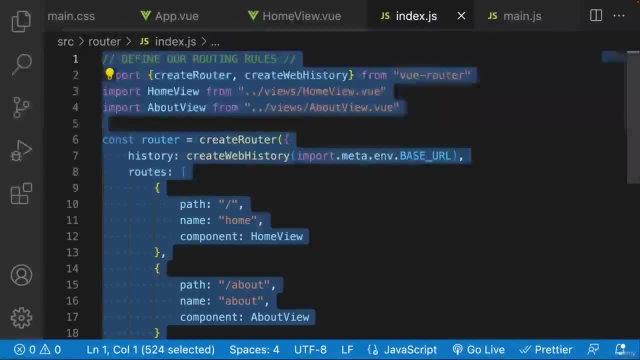 So inside of the index.view, we have defined our rules. That is all we did. 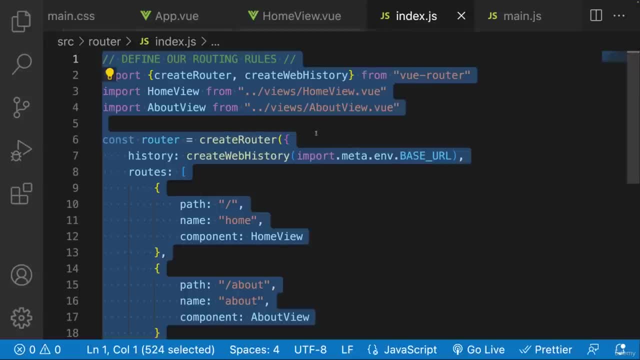 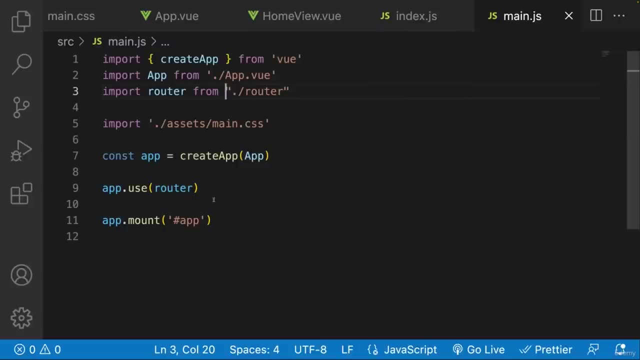 Then what we wanted to do is connect it to our view application. So we went ahead and did that inside of the main.js file. We connected our rules, our routing rules, into our main.js file by basically connecting it to our app itself. 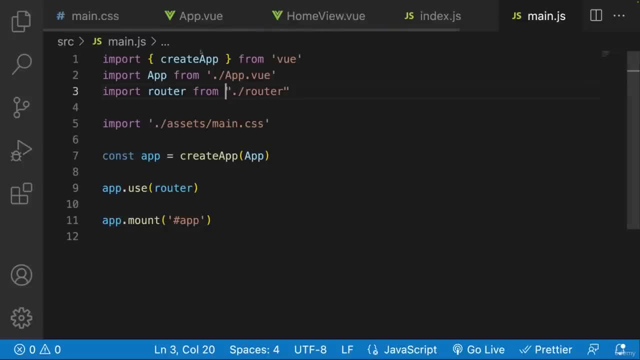 Then what we want to do is, define where we want to start rendering these rules. 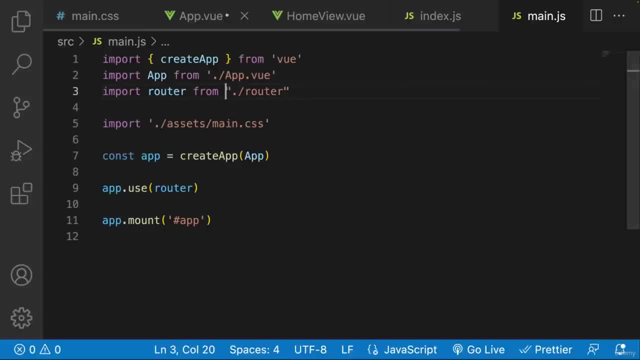 And we can render these rules in any different component that we want to. Well, we want to render these rules inside of the app.view component. 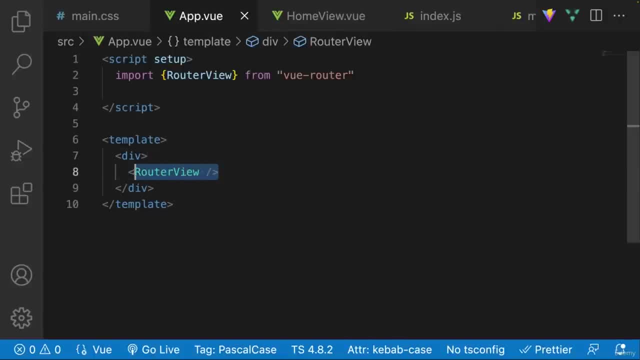 And that's why we created, or that's why we rendered, this router view component that we got from view router. 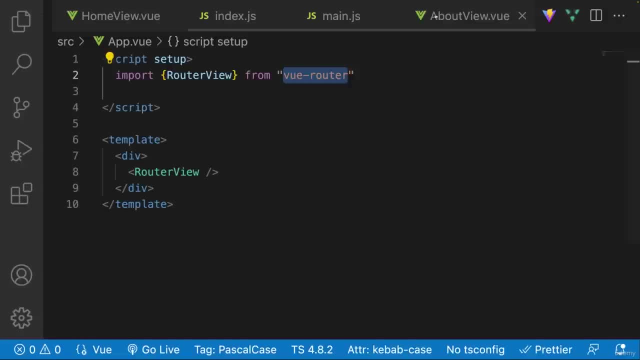 So I hope this is making a lot of sense. And now you have a great understanding of how to do routing. 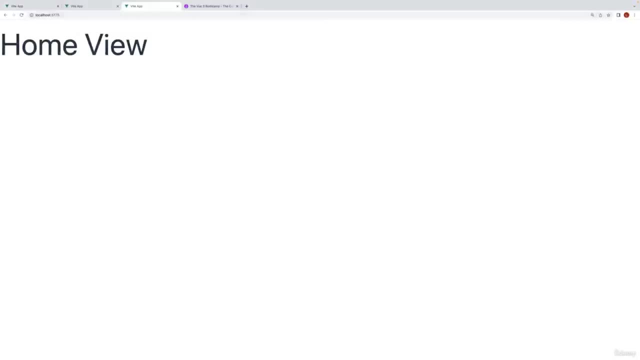 In the last video, we were able to successfully add routing to our application. So if we are on the path slash, this is what we get. If we go on slash about, then we get a brand new component. 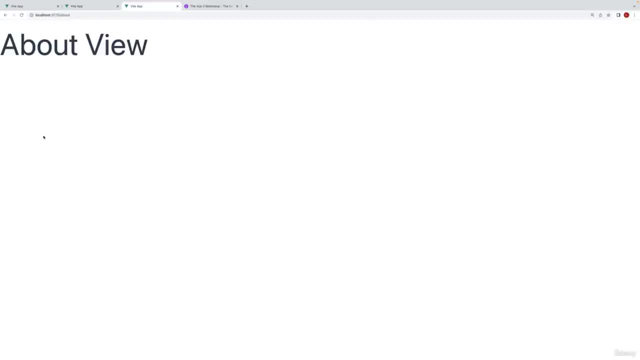 However, obviously this isn't how we want our users to navigate across our application. We don't want them to consciously know that there's a slash about page and then consciously know the path, and then go ahead and write it in the URL, and then have them navigate to it that way. 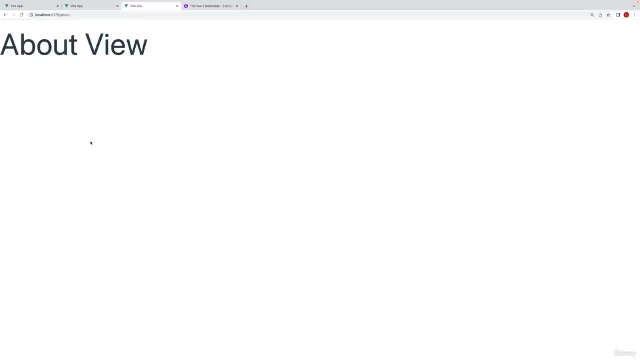 Obviously that is not going to be a good user experience, and most likely our users are never going to know about the existence of our about page. 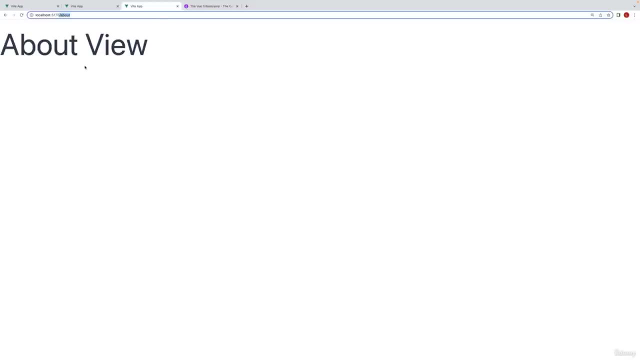 So typically, what do we do in situations like this? Well, very typically we add a nav bar that shows the links to all of the different pages that we have in our app. 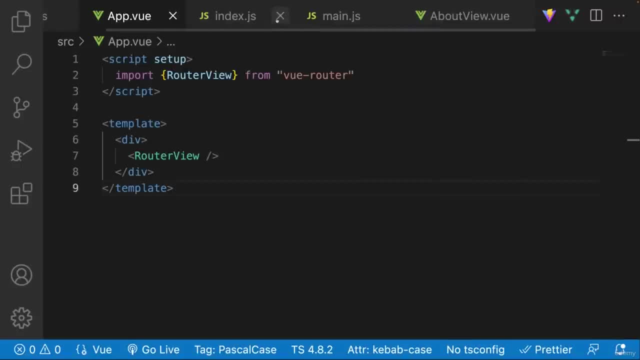 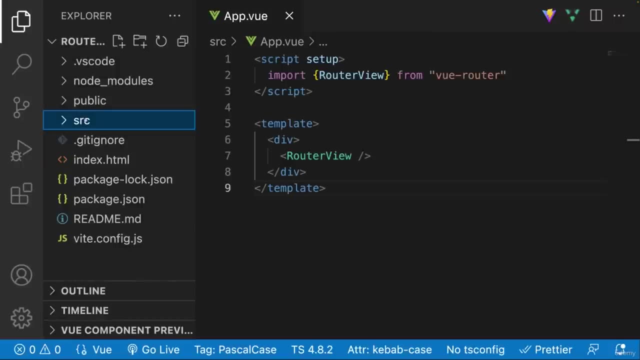 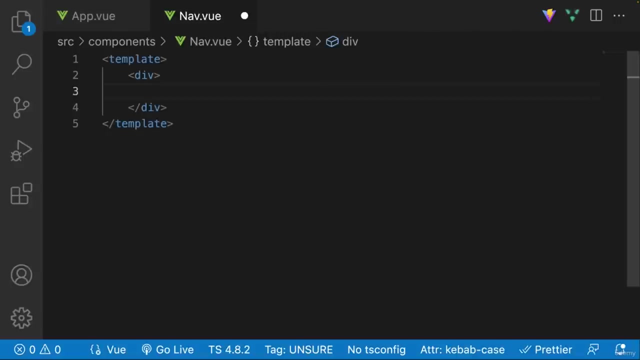 So let's just go ahead and actually add this nav bar. So I'm going to go over here, and I'm actually going to create a new component for this, just so we can get into the habit of creating components. So let's say components, and let's say over here we're going to have a nav.view file. And then over here we're going to have a template, a div, and then for now we'll just add paragraph tags. We'll say home, and then over here we'll also have an about. 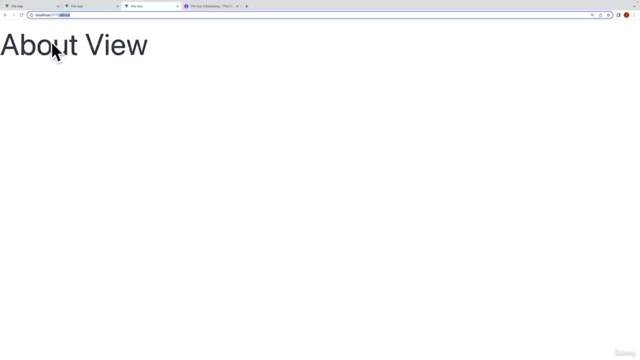 Now what we want to do is, we want to render this probably on every single page that exists. 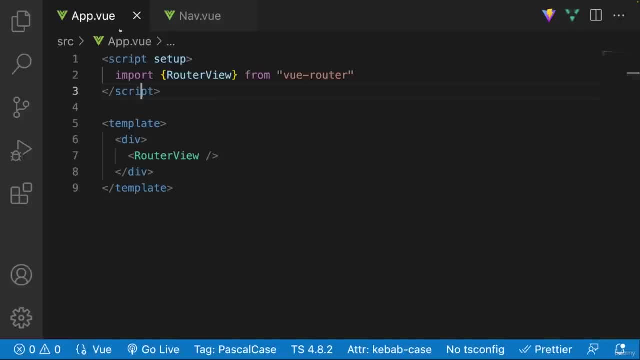 So the best case scenario is to actually go to the app.view and import the nav from our components. So we're going to say from our components, 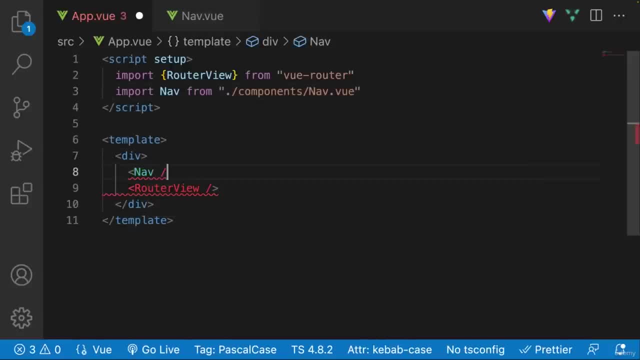 we want to get the nav, and we are going to render it right here. 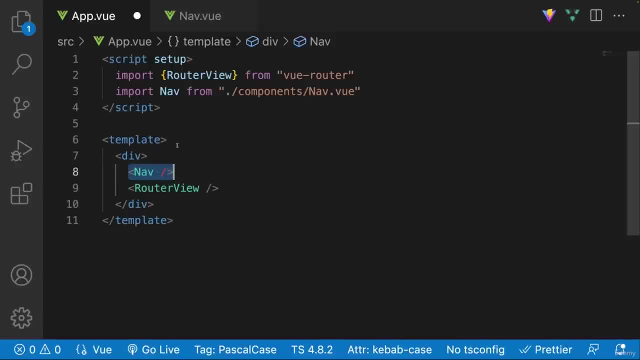 So what's going to happen here is it's always going to render the nav, every single page is going to have the nav, and then our view router then will determine the component that we want to render over here, based on the route. 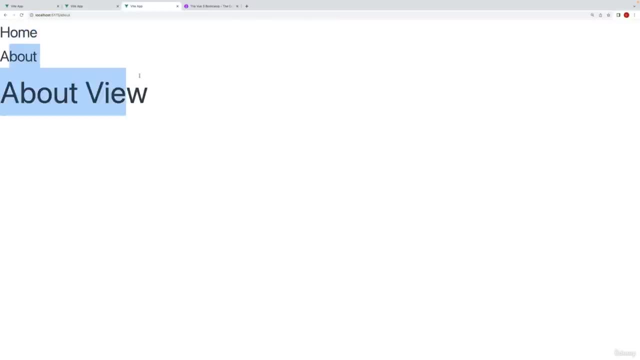 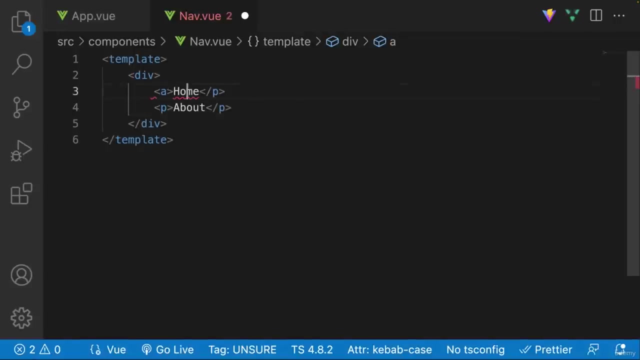 So now as you can see here, we have home as well as about. Now of course we want to make these clickable, and not only do we want to make these clickable, we also want them to update the route of our application. So typically this is actually done with A tags. So over here, anchor tags. So we have A, and then we have an href, and then what we're going to say is, well this one, if you click it, you go to the path of slang. 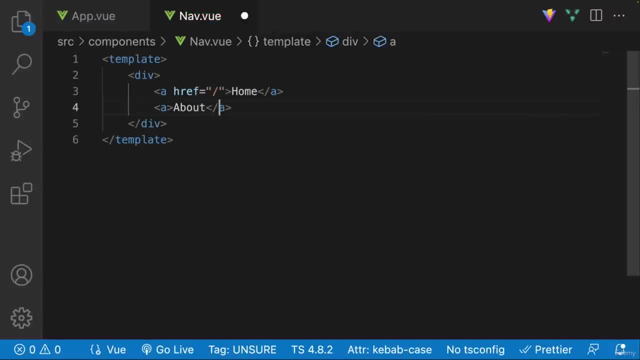 Then over here we'll add another anchor tag, and here we'll say href, and if you click this then you go to about like so. 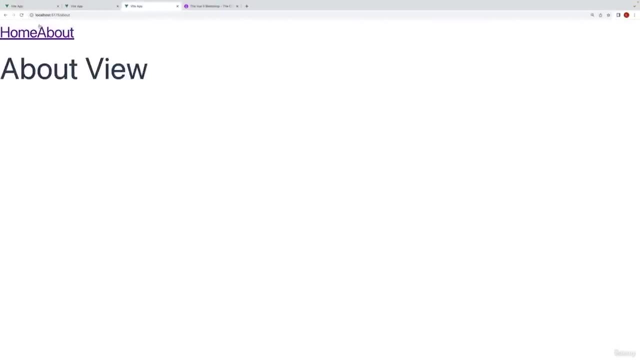 And this is actually going to work completely fine. So now if I go over here to home, you can see we get the home view, if I go over here we get the about view. So this is actually pretty good, but it's also pretty bad. Let me tell you exactly why. 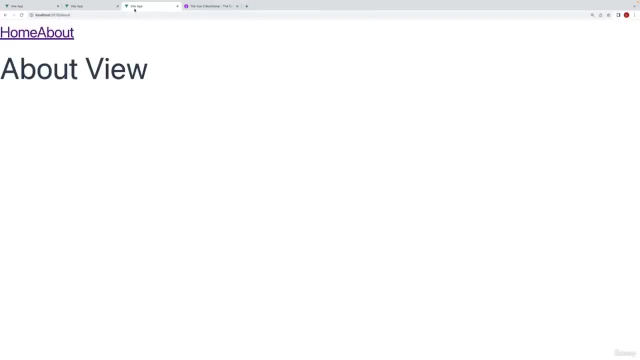 So look over here at home, at this tab right here. What I'm going to do, 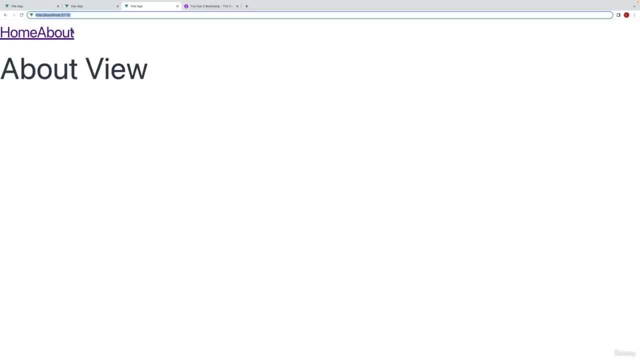 is I'm going to go ahead and click on something, and as you can see, there's like a tiny little refresh. 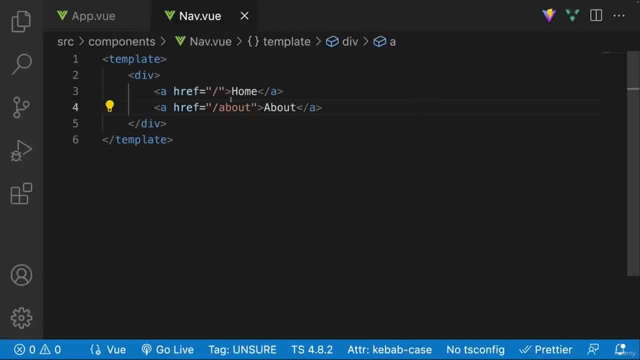 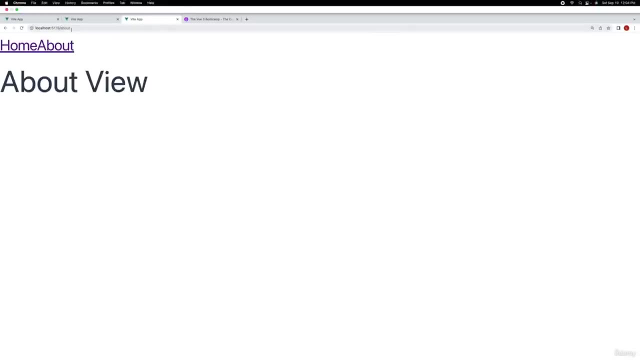 And that's actually what's happening in our application. Anytime that we click on a particular anchor tag, it's actually refreshing our application, and changing our route at the same time. 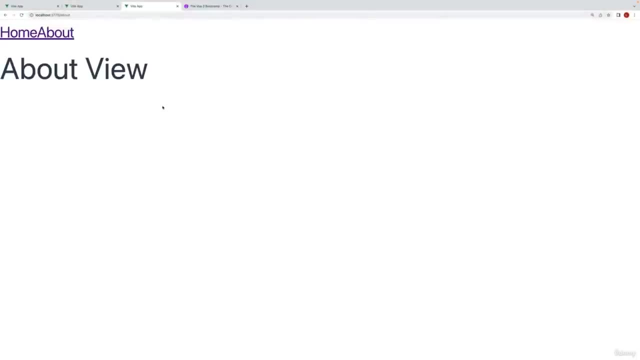 Now because the route is indeed changing, then the view router is going to well catch it, and render the correct component. But it's refreshing our application every time, which isn't really all that great. It's not really good performance wise, and it's also going to refresh our state, and that's going to reset it back to the default value that we gave it, which isn't probably ideal. 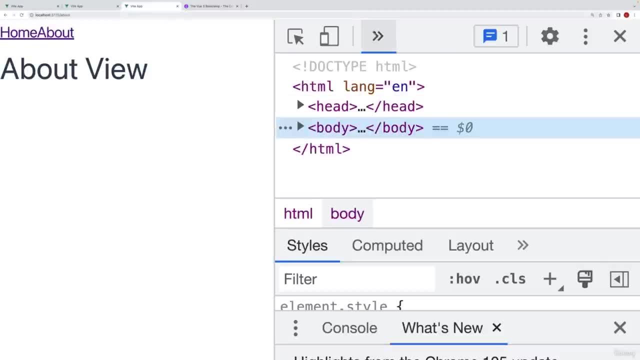 So what we're going to do here, just to prove this to you, is we're going to go over here to the console, and I'm very simply just going to console.log hello. 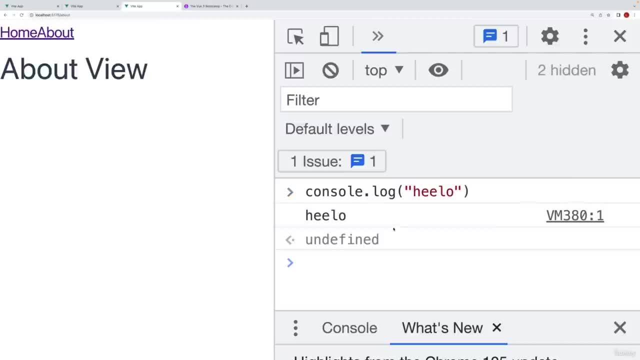 Let's go ahead and console.log hello, and I spelled it incorrectly. 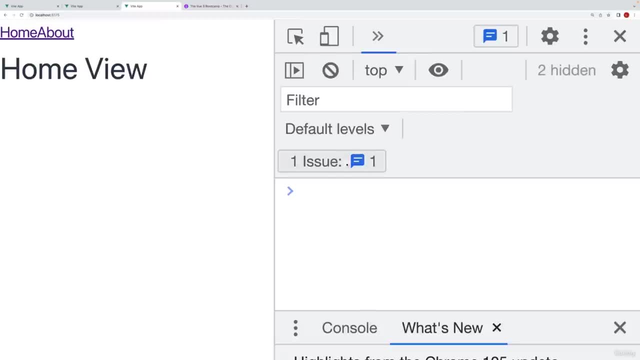 And now what I'm going to do, is I'm going to move to this page, and you can see that console is completely gone, because again, we've refreshed our page. Not what we want. 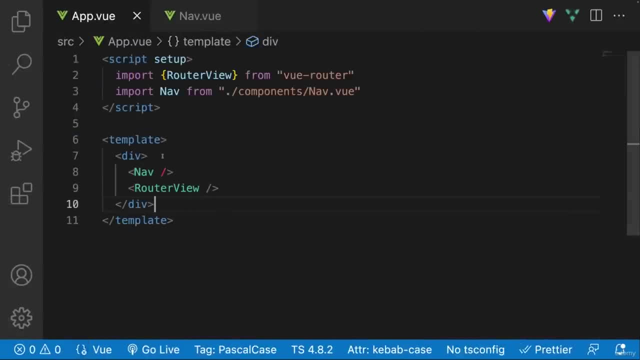 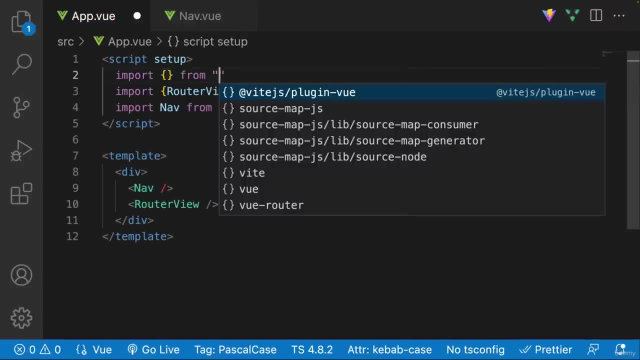 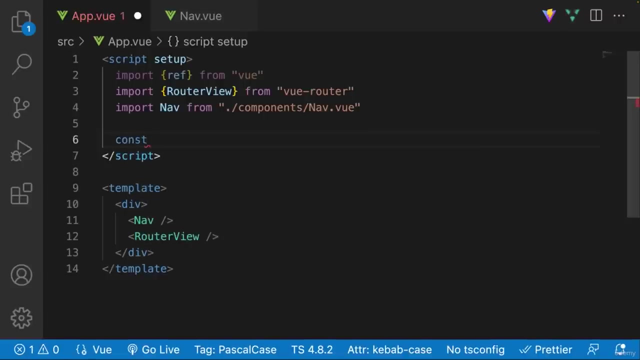 And to show you how bad this is, let me go over here, and I'm going to create a piece of state. So let's go over here, and I want to import from view, I want to import a piece of state, I'm going to say ref here, and let's go here, and I am going to say, let's have a piece of state in here, and we're going to say, what am I doing here? So let's just say just random, 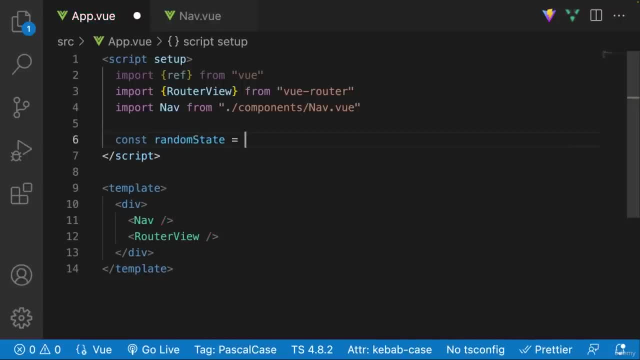 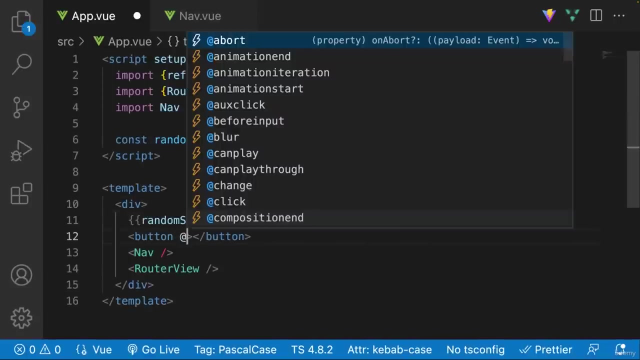 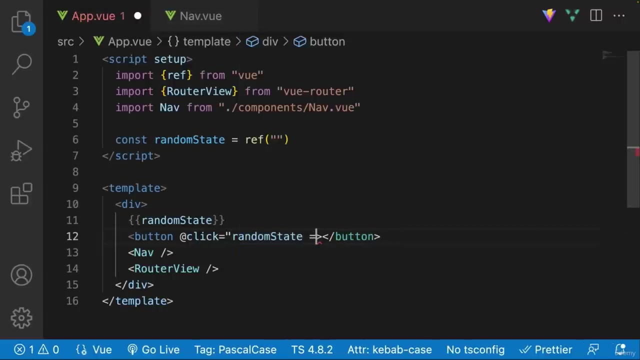 I'm going to say random state, I don't really care what I call it, I'm going to say ref, and initially I'm going to set it to an empty string, and what I'm going to do is, I'm just going to render this random piece of state over here, and I'm going to add a button, that if you click it, it's going to update the state, so it's going to update the random state to, let's just say, hello, we'll say the string, hello there, like so. So very simple stuff. 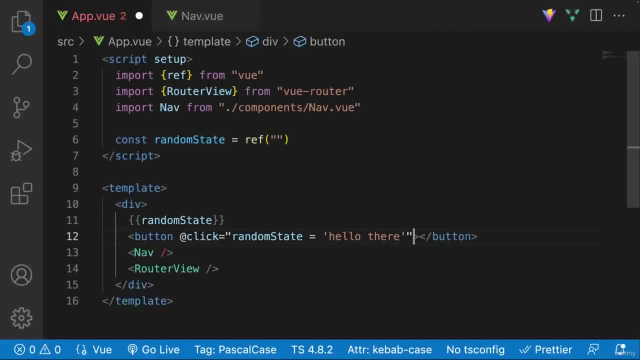 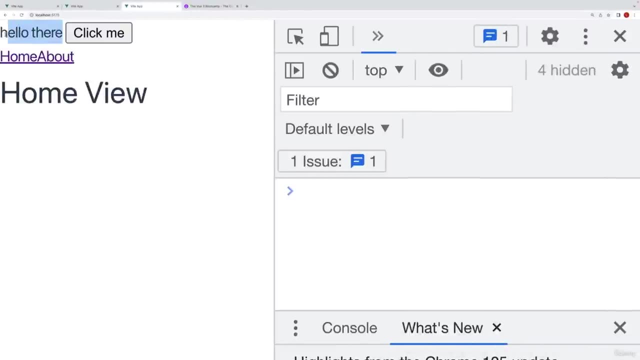 And over here we've got to close this off, like so, looking good, and we'll say click me. So now what I'm going to do is, I'm going to click it, and as you can see, this is going to update my state. 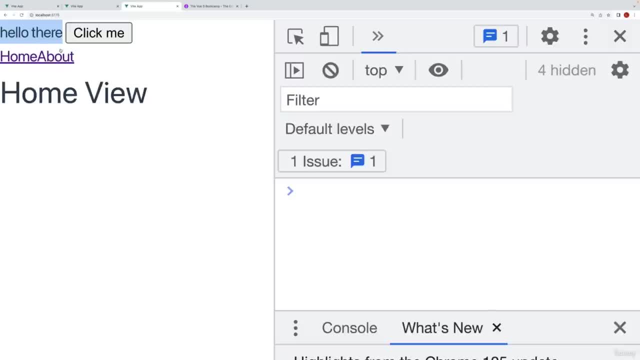 Now of course, I want this state to persist, regardless of the page that I'm on. 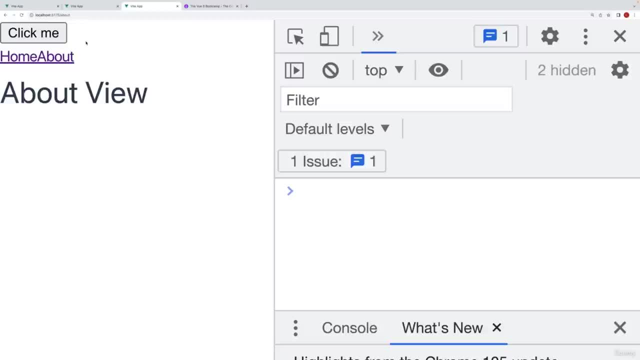 But over here, if I go to the about page, because now we refreshed our application, if I go back to home, you can see that it is completely empty. 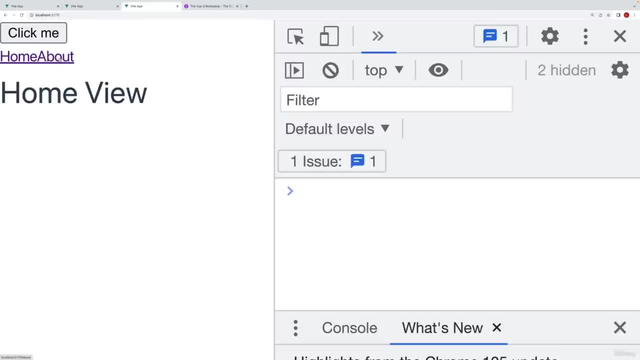 Again, not, not, not what we want. 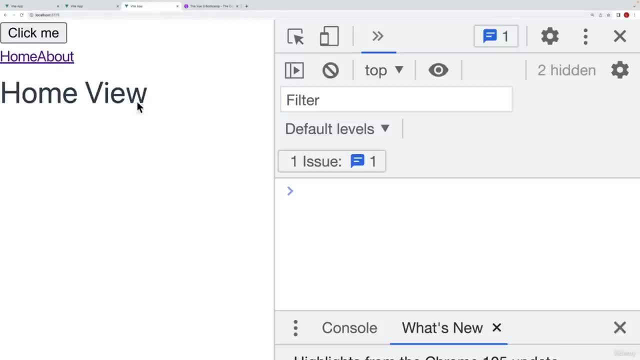 So instead of refreshing our page, we just want to tell our view router, hey, look, we want to change the path, what we want you to do, is to just change the component, associated to this path. 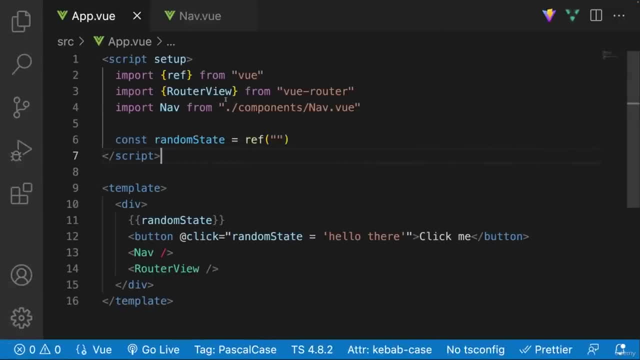 Well, how can we do that? Well, we can do it very easily, with a built-in component, that view router gives us. 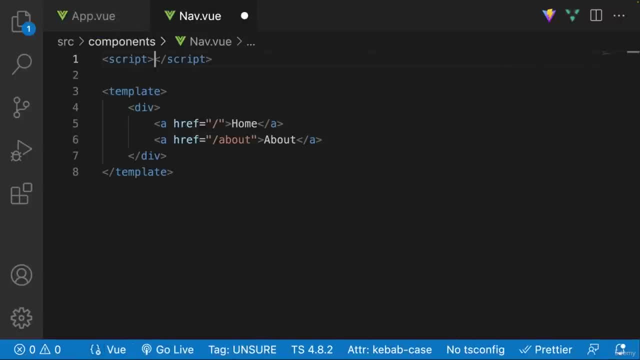 So we're going to go to the nav over here, and let's create a script tag, and we're going to say setup, over here. And what we're going to do, is we're going to import something called view, or from view router, we're going to import something called router link. And instead of using anchor tags, we're going to use router link. 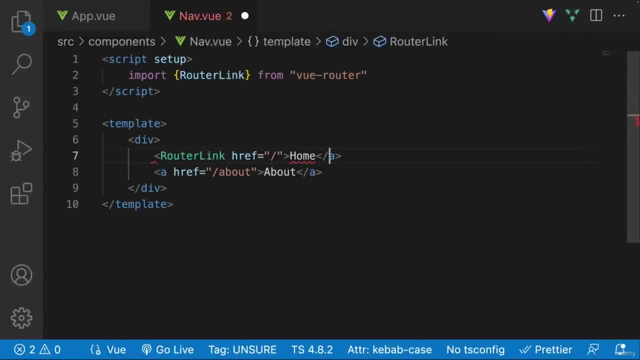 So let's go over here, we're going to say router link, and router link, and then over here, router link, and similarly over here, router link. Now instead of href, we're going to rename this to two, so two, slash, then over here, two, and then about. 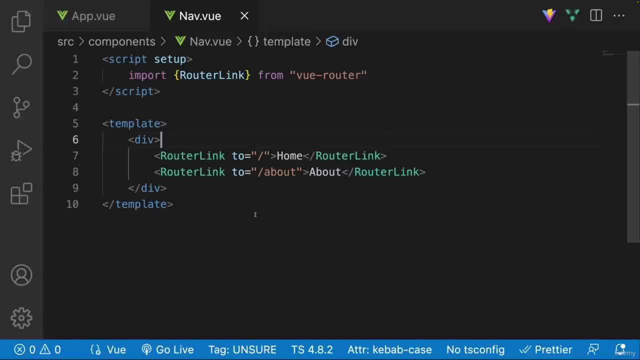 And this is going to do the magic, of not refreshing our page. It's going to change the route, and then change the associated rendered component, but again, it is not going to refresh our application. 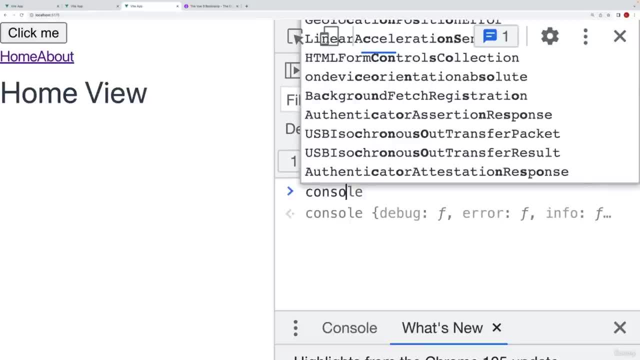 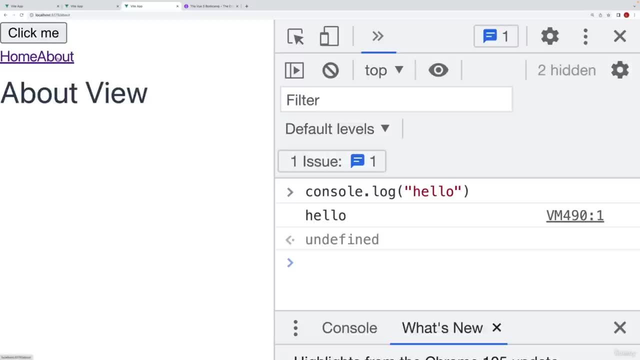 So let's go over here, and this time let me go ahead, and actually console.log something, like hello, like so, and what I'm going to do, is I'm going to click on about, you can see here, that nothing has refreshed, 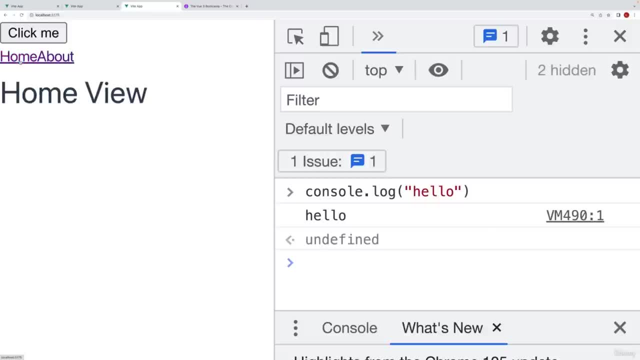 the console is persisting, and if I go over here, you can see everything is a-okay. 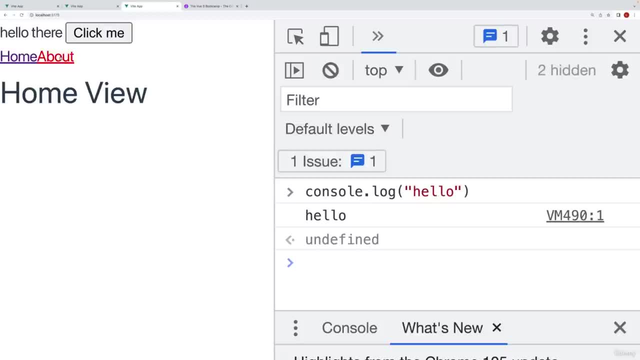 Now let's make sure that the state is persisting, so now we got that state, and now across any component, our state is also persisting, because again, we are not refreshing our app. 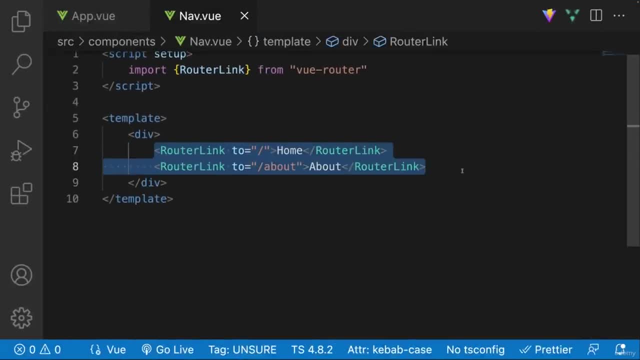 So in almost 95% of the scenarios, you're going to want to use this, to navigate across your application. 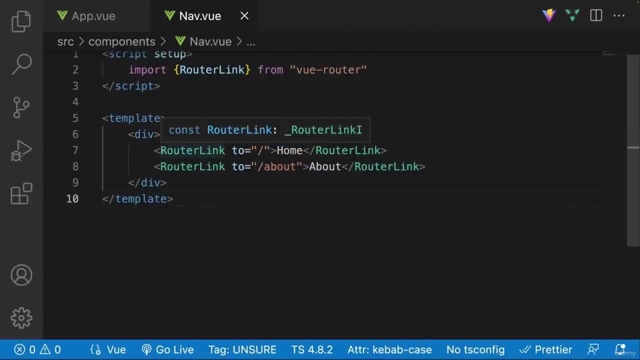 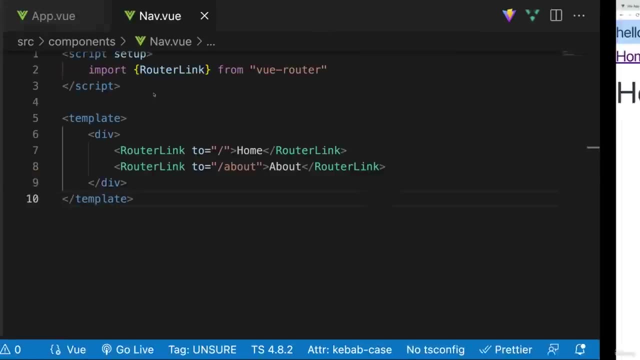 Really the only time, that you're going to want to use an anchor tag, is when you're maybe, linking it to another particular website, that's not associated to your own. 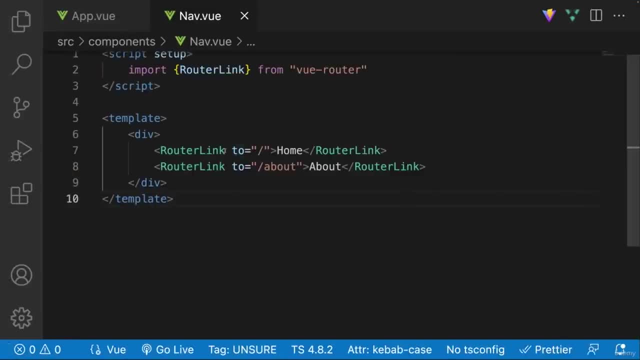 But anytime you want to navigate across your app, you're going to want to use, router link. 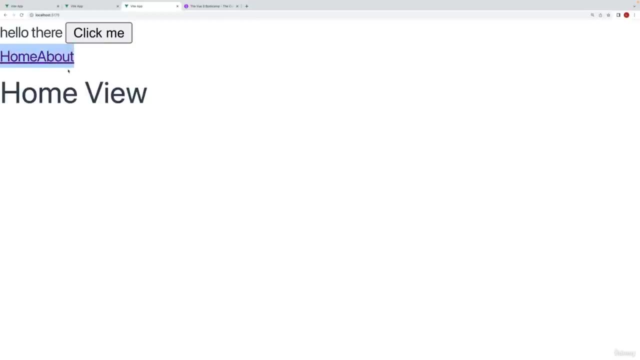 So we were able to create, this hideous nav bar, that is able to navigate across different pages, without refreshing our page. 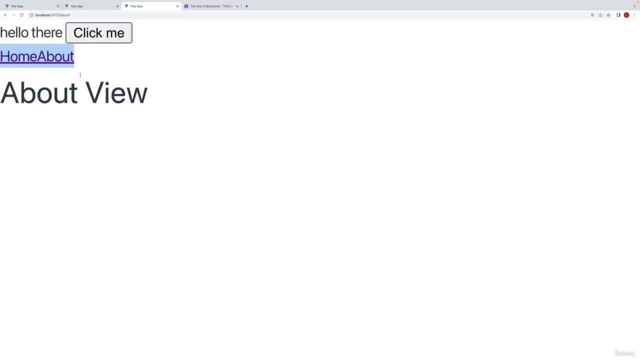 This is terrific. However, we could improve this nav bar, just a tiny bit. And we can, well improve it, by maybe, bolding out the word, where our application is in. 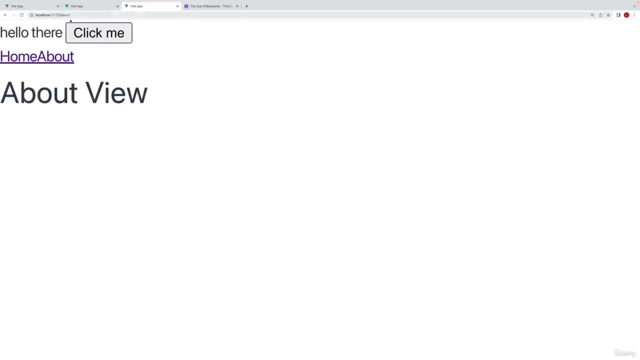 So for example, if we're in the slash about, page, maybe it would be nice, to bold this right over here, the about. And if we're on, well the home page, then we're not going to bold this, but we'll bold this over here. So let's talk about exactly, how we can do that. 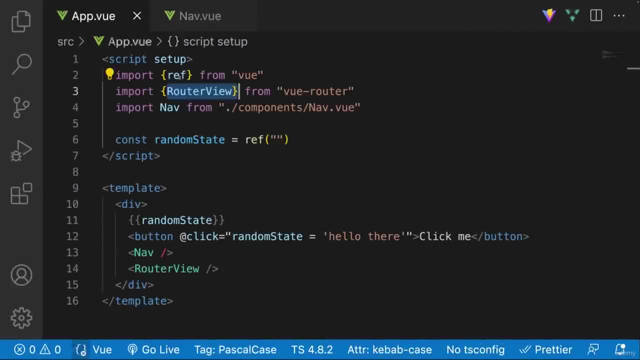 So let's go over here, and actually let's go to our app, and let's just remove this button. I think we get the point at this point. 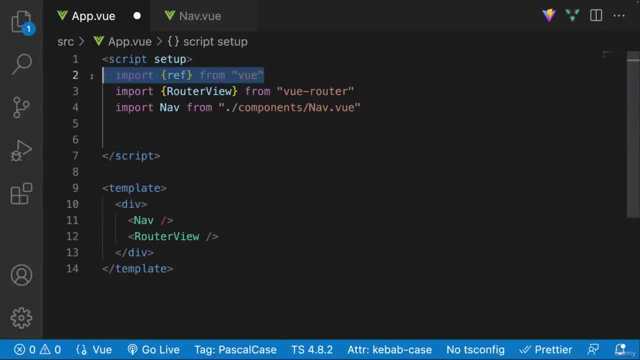 You can remove this, and we can remove that, and also we can remove this. Okay, 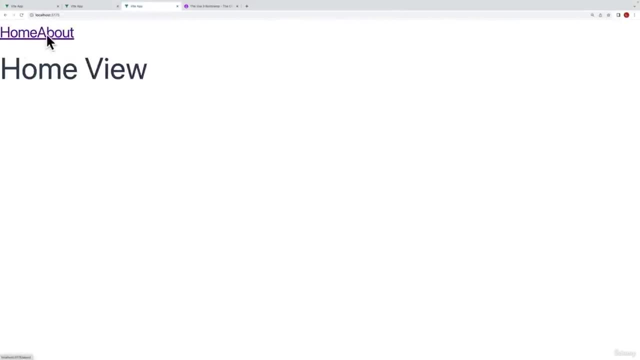 looking terrific. So again, what I, in effect, want to do, is I want to style, the router link, that is associated to the page, that we're in, a little bit differently, than the other router links. 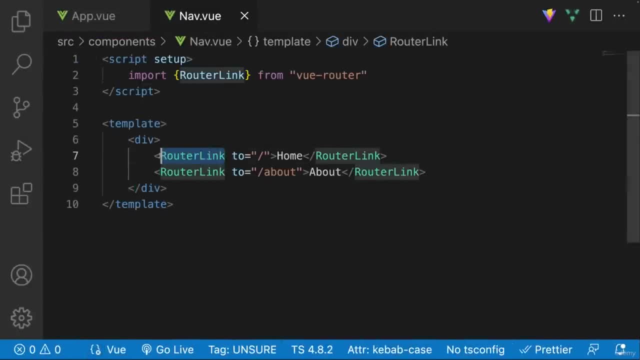 And luckily, this is super, super easy, with the router link component. 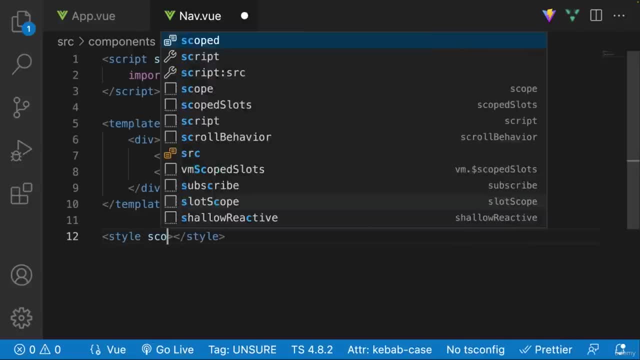 So what I'm going to do first, is I'm going to add some styles, and let's make them scoped. And over here, I'm just going to say active. 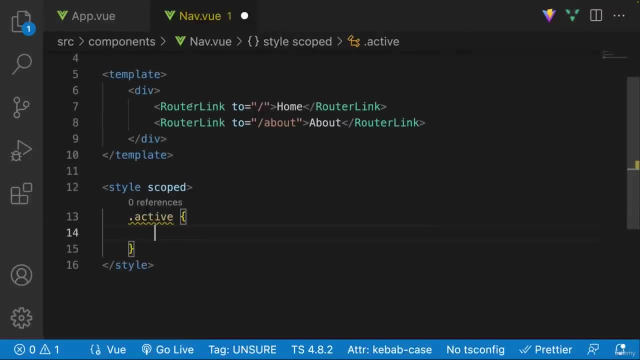 This is going to be the active, class, for our router link. And very simply, maybe I'm going to go ahead, and do a font weight of 900, and let's just really make this apparent. 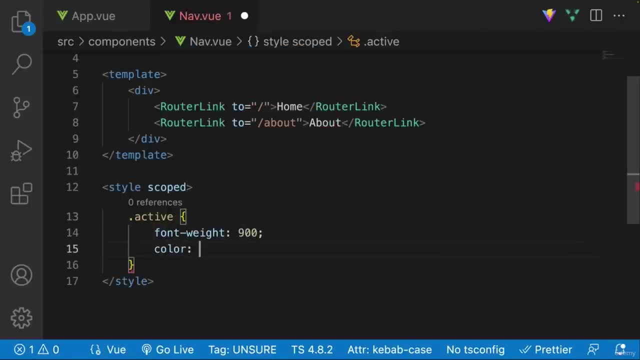 Let's just change the color to, let's just pick a color. I'm going to pick a random color, that's just like very, very apparent. Something like gold, like that. 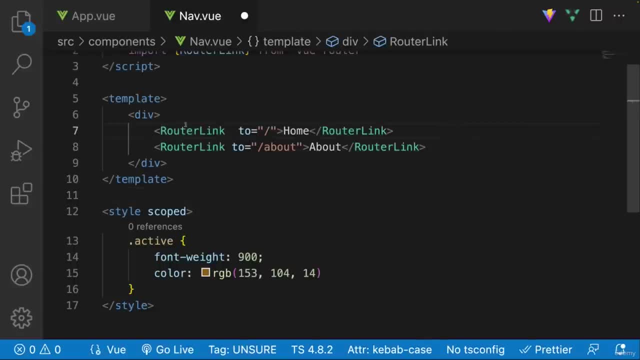 So very simply, to accomplish this, we're going to add a prop, to the router link. 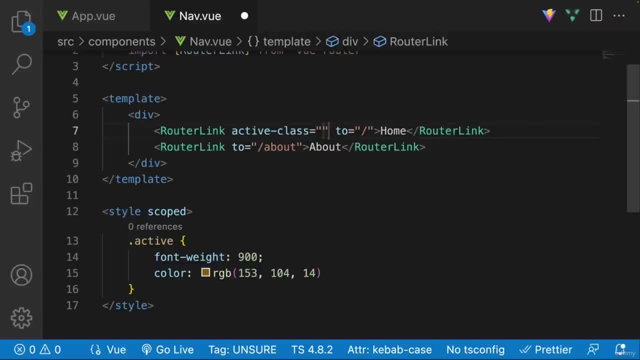 And it's going to be a built-in prop, called active class. And very simply, we're going to pass in, the name of the class, that we want to, for it to utilize, when this is active. And we're going to, of course, pass the exact same thing, over here, to this router link. 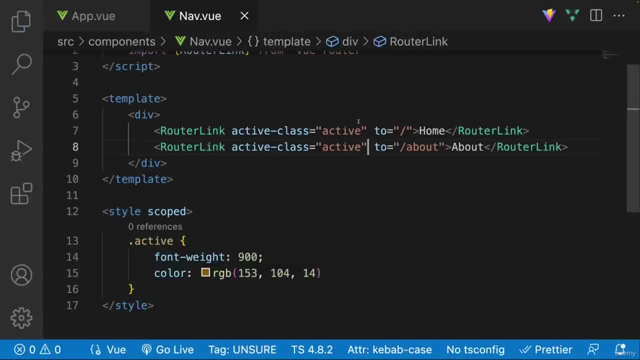 So very simply, what this is going to do, is let's say we're on the homepage, what this router link is going to do, is check, hey, are we on the homepage? If we are on the homepage, then I'm going to give this anchor tag, because in effect, this is an anchor tag, at the end of the day. 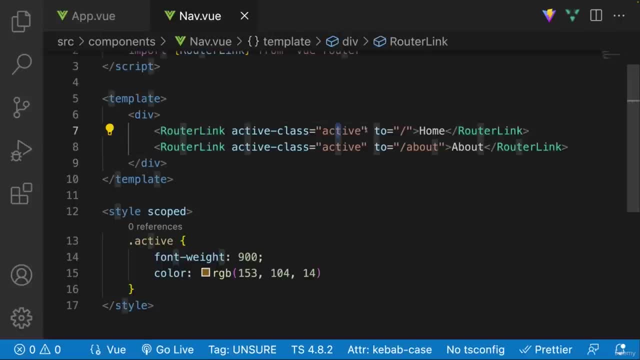 This anchor tag, we're going to give it, a class of active. And that over here, we have defined it. 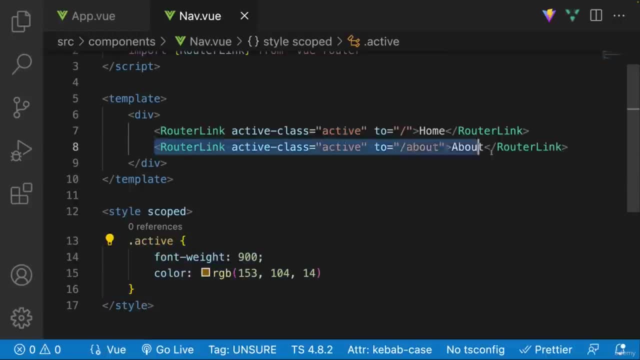 Now in this case, let's say we're on slash, well, this router link is going to do, the exact same thing. It's going to look, hey, are we on slash about? 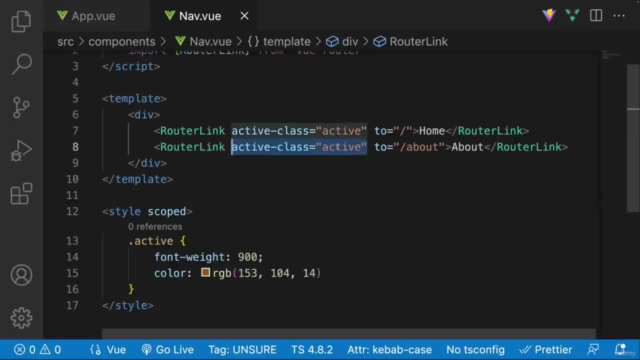 But in this case, we're not on slash about, so it's not going to give this, the active class. 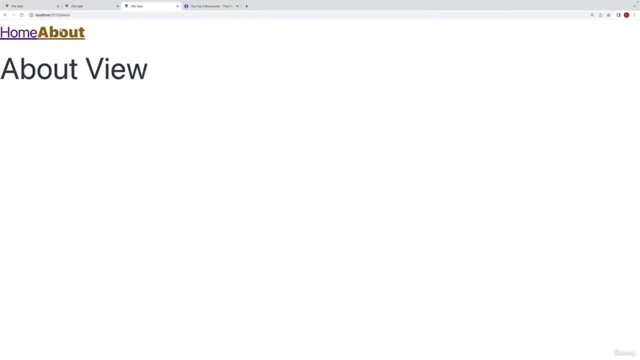 So let's go over here, and as you can see, right away, we can actually see the styles. 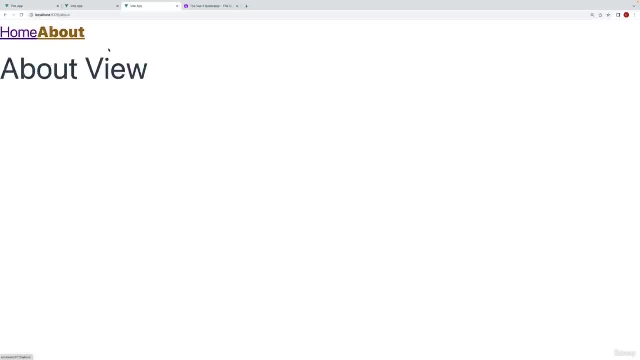 And now we can actually render, these styles, back and forth. 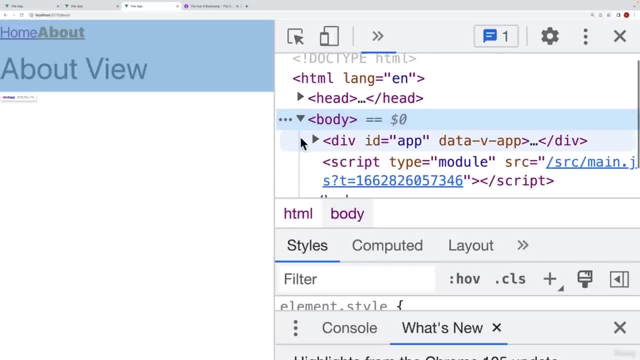 Now, let's just go ahead, and actually inspect, the elements. So let's go over here, elements. 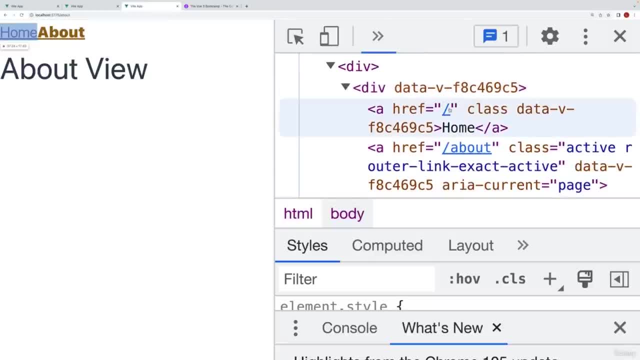 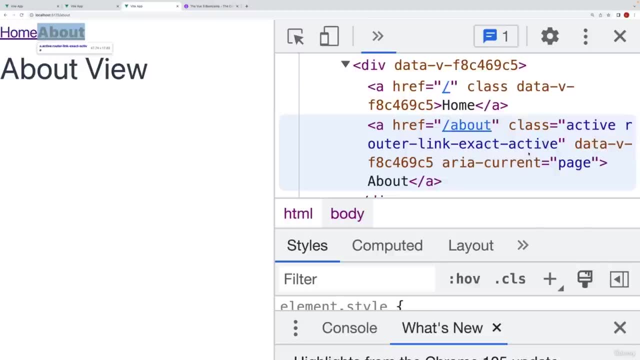 Let's go here. So we have our anchor tags. You can see we have the slash, and then we have the slash about. And you can see now, this has the class of active, because that's currently, what we're on. If I go to home, you can see now, the about doesn't have, that class anymore. But this time, this anchor tag, 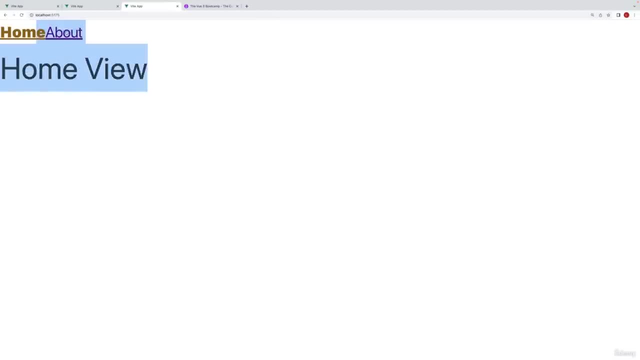 does indeed have it. So this is terrific. Now we can style it, so the user can have, an actual idea of exactly, what page they're on. 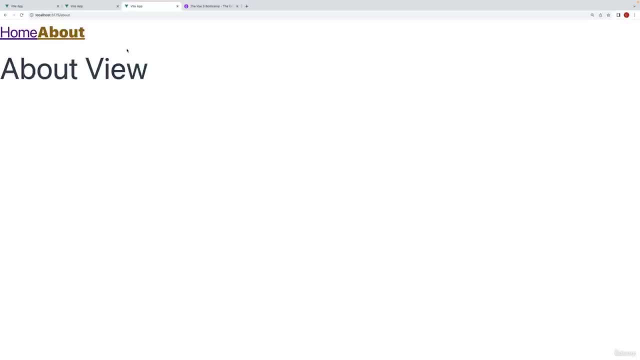 Without having to look, at the URL. All right, my good friends. 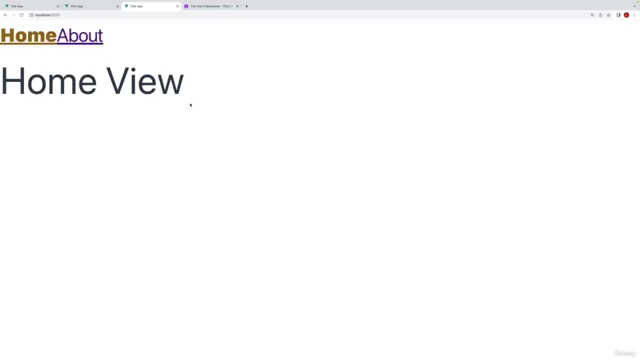 So far, we have created, a two page application. 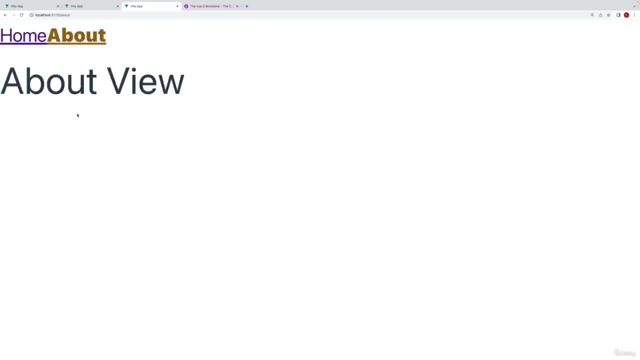 With the home view, as well as, the about view. 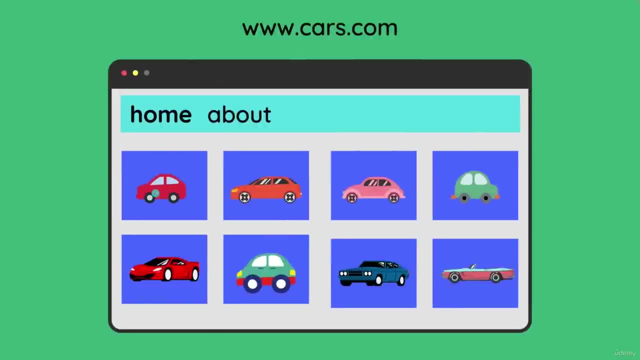 However, if you look at our car application, over here, eventually, what we're going to want to have, is make these car cards, clickable. 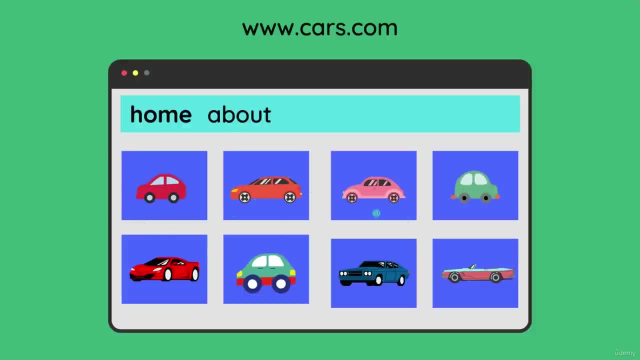 And as soon as they click, on a particular card, we want to redirect the user, so that they have more information, about the card, that they clicked on. 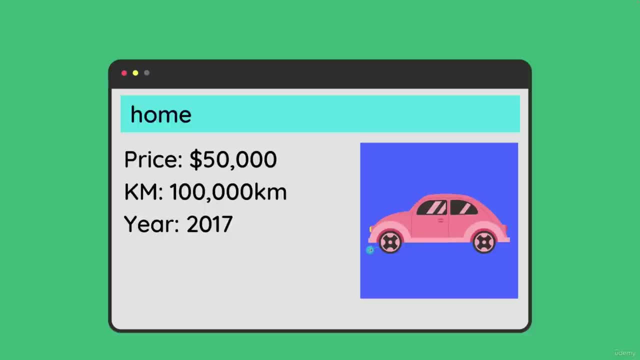 And I keep saying card, but I mean car. So, sorry, apologies for that. So over here, let's say that they click on this car, right over here. And it's going to redirect them, to this page. 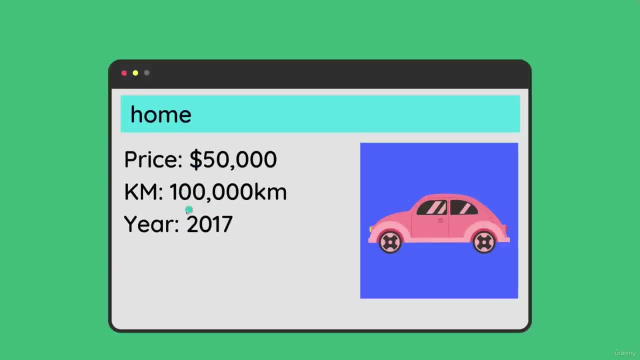 It's going to have an image, it's going to have a price, their kilometers, as well as the year. 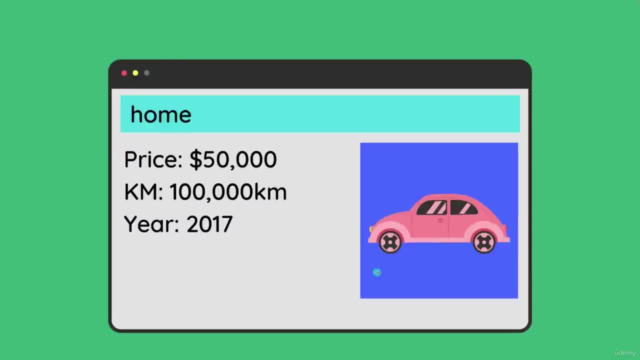 However, if they click on this car, right over here, the page format, is going to be exactly the same. 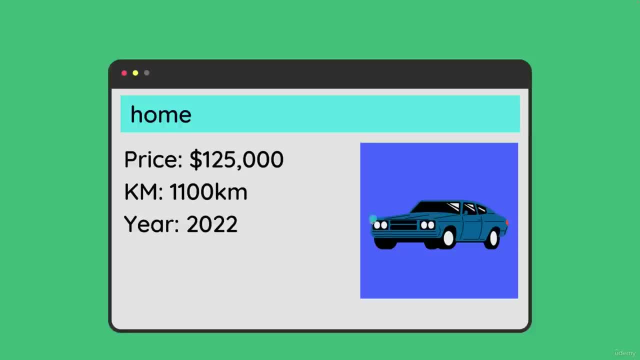 However, the data is going to be different. We're going to have a different, image. 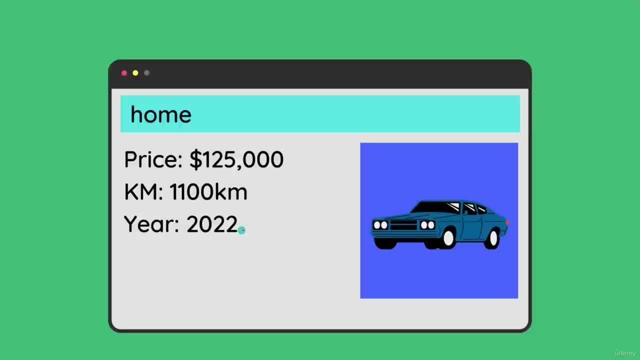 We're going to have a different, price, kilometer, as well as year. So this is actually going to present, quite a big challenge. 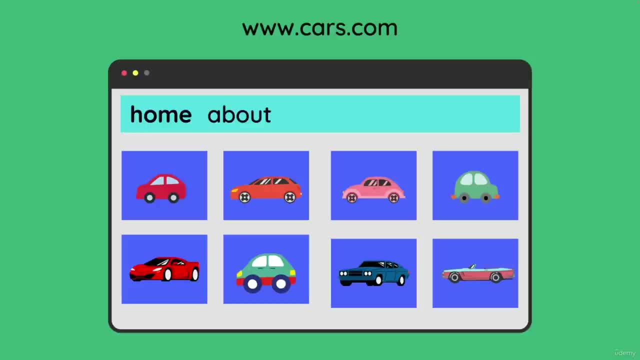 Are we going to have a component, for every single car? Well, no. Obviously, that is way too unrealistic. 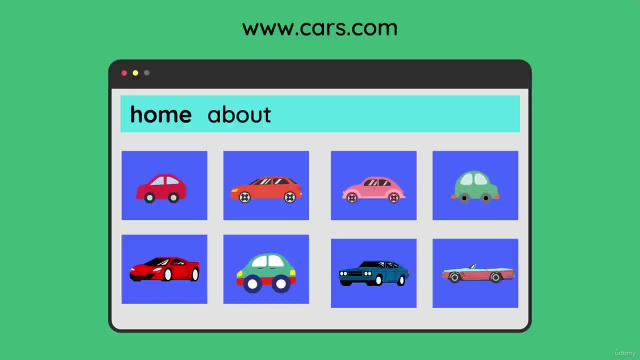 And eventually, we might have our data, coming from a server. And thus, we're going to have no idea, how many cars, that we're going to have. 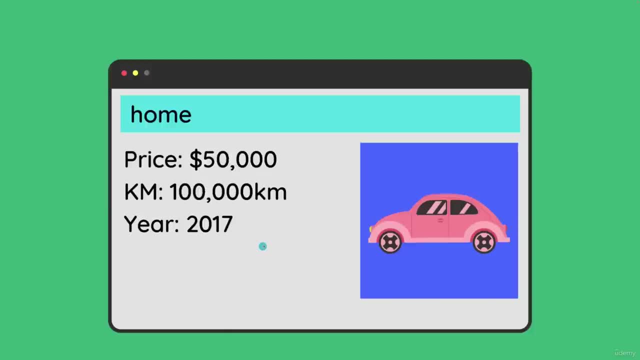 Now luckily, we can actually look at, these two different pages. And again, the format of the page, is exactly the same. The HTML is the same, as well as the CSS is the same. The only thing, that is different about it, is the data. 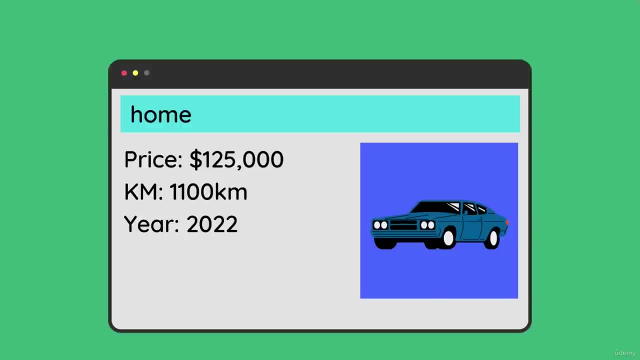 So what we can actually do, is create one component, with the HTML structures, and the CSS. And then we can figure out, how to populate the data, dynamically, depending on, the car, that they clicked on. 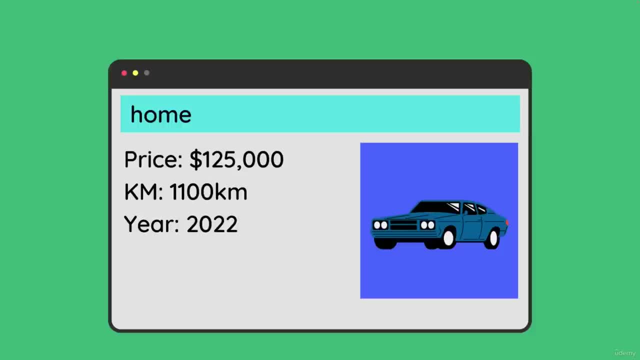 And we're actually going to do that, with the path, and the route. Let me explain, so let's say they clicked on, the pink car. What we're going to do over here, is we're going to redirect them, to slash car, and then slash, that car's unique ID. 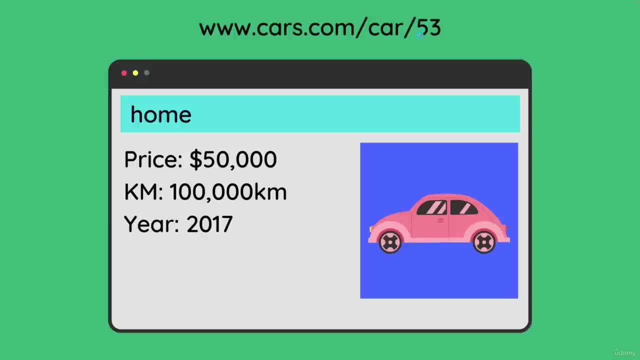 So let's say this car, has a unique ID of 53. 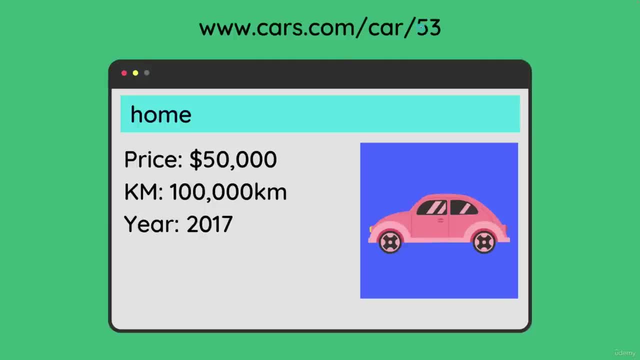 So that's what we're going to do, it's going to be, slash car, slash the unique ID, of the car. 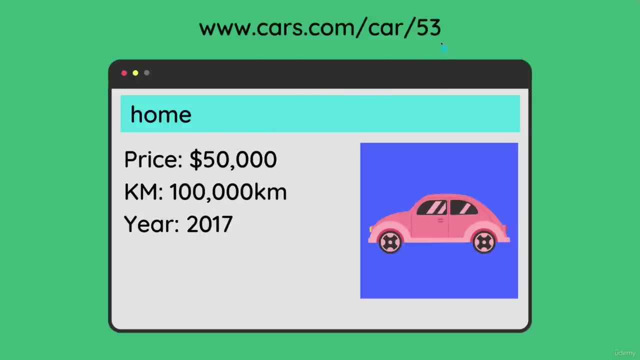 And then what we're going to do, is inside our component, we're going to extract this ID, from our path, and then figure out the data, that we need to render, based on that ID. 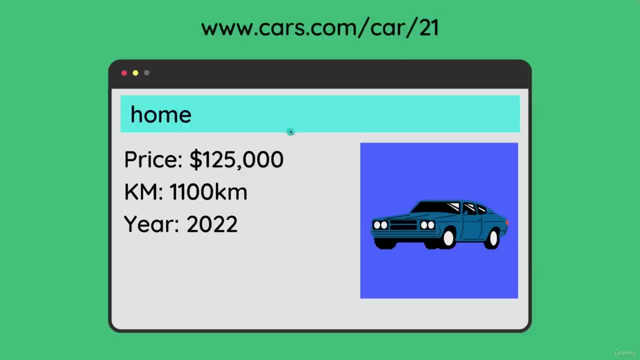 So now, if they click on another car, maybe something like this, the path is going to be, slash car, and then slash 21. Our page is going to extract that 21, and figure out the data, that he needs to render, based on that car's ID. 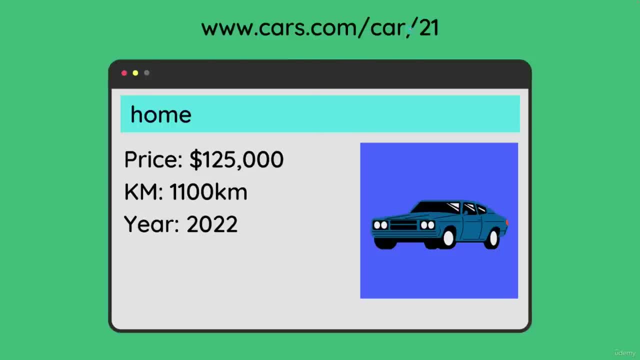 So over here, the path is always going to be, slash car, and it's always going to be, slash car, slash ID. 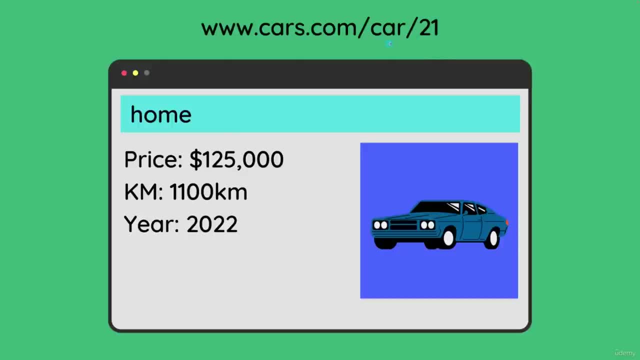 However, the slash car part is static, and is never going to change, but the ID part is dynamic, and will most likely always change, for every single car page, that we go to. 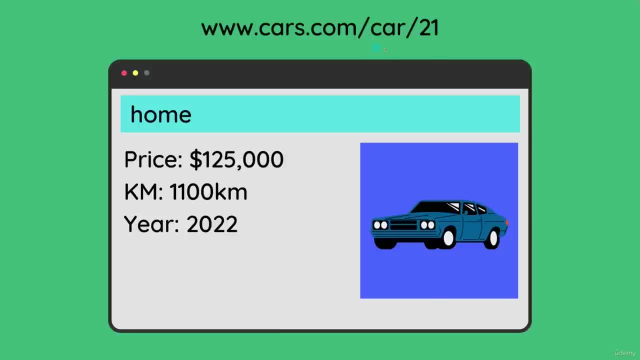 So we're going to need to figure out, how we can accomplish this. 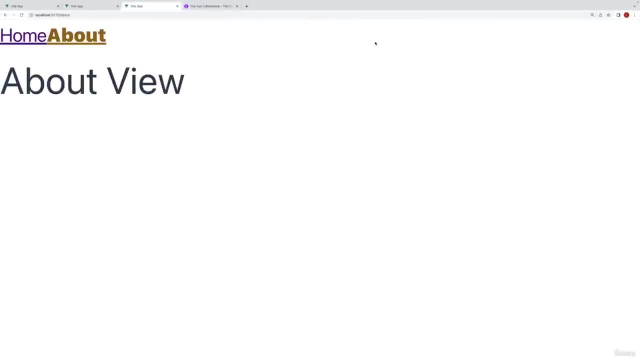 So let's actually go ahead, and code it out. 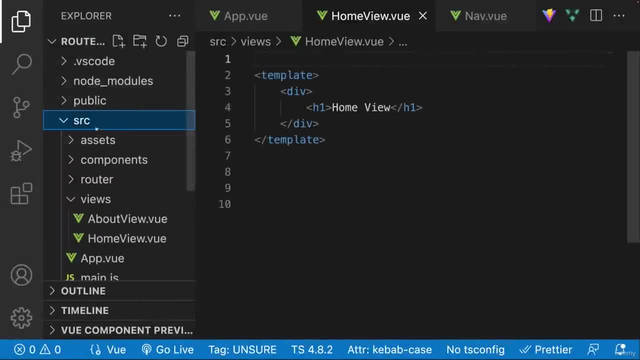 So over here, what we're going to do, is we're going to create, inside of our source directory, we're going to create just some data, for our cards. 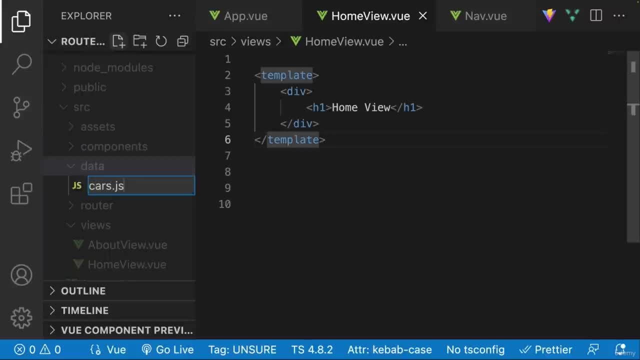 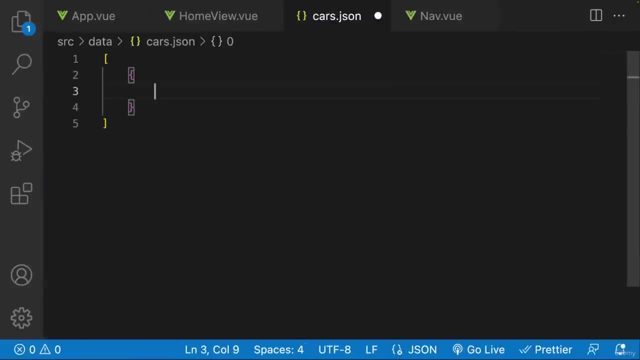 So let's go over here, we're going to say data, we're going to say cars.json, and this is just going to be a JSON file, that's going to be an array of objects. So each object is going to have an ID, which is going to be just a unique identifier, for the car. We're going to have the name, which we'll say is, let's say Chevy, and we'll also have a price, which is going to be, let's say 15,000, and we're also going to have a year, 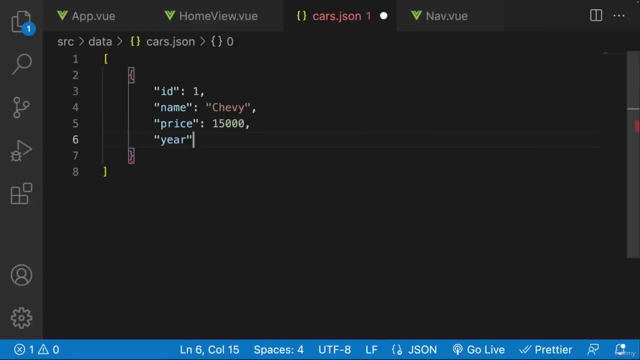 and this is going to be, let's say, 2015. So this is all the data, that we are going to have. 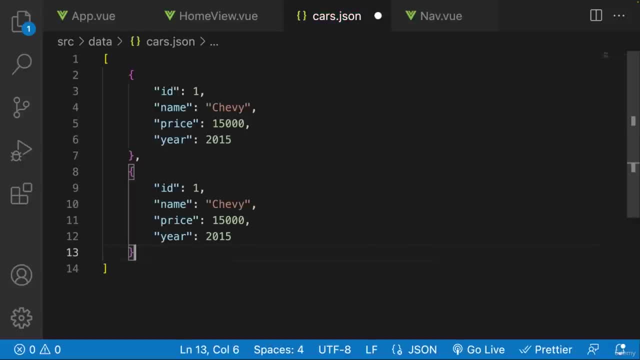 So let me go ahead and copy that, and we're going to do the exact same thing, maybe five more times. 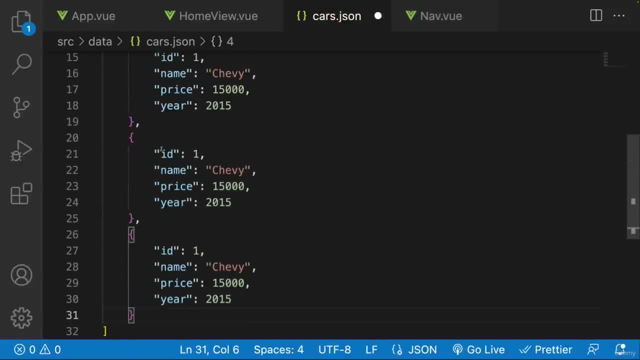 So let's go here, let's just change this up, let's change this to, two, three, four, five, 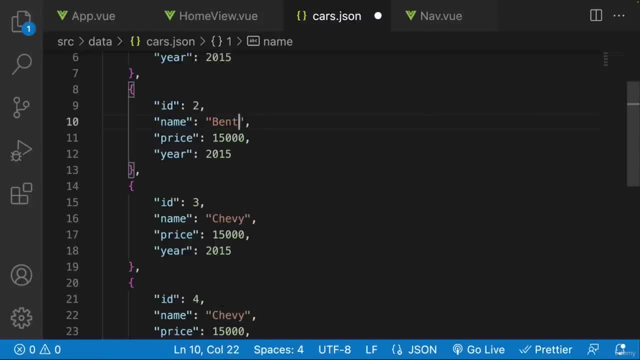 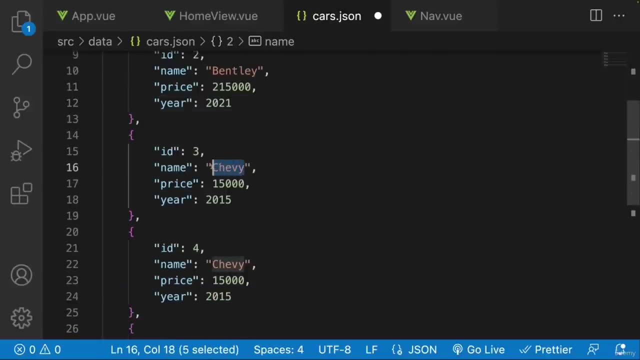 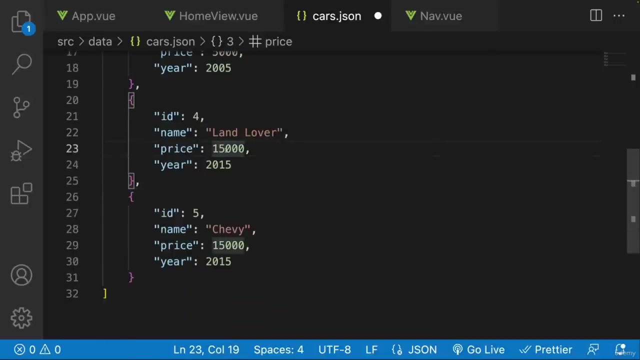 now let's change these things up, Bentley, let's say, this one's going to be 200, and we'll say 21 here, and this one's going to be a Ford, let's say this one's 5,000, the year is 2005, over here we're going to say, let's say Land Rover, and this one's going to be around 85,000, this one's going to be a 2019, and lastly we're going to have a Nissan, Nissan, this one's going to be 25,000, and a 2019. 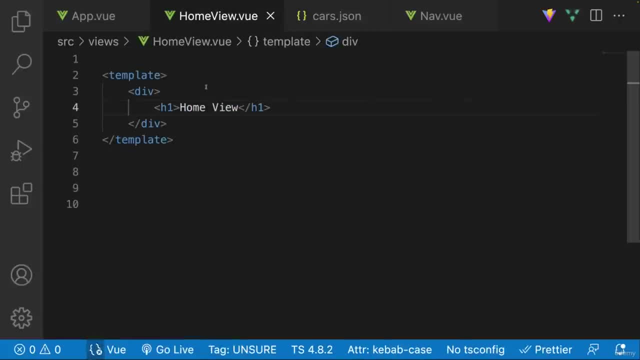 Alright, so this is looking pretty good. So now what we're going to do is, we're going to go to our home view, and what we're going to do is, we're going to iterate over this data, and we're just going to render some cards. So we've done this before, and we know how to do it with the V4. 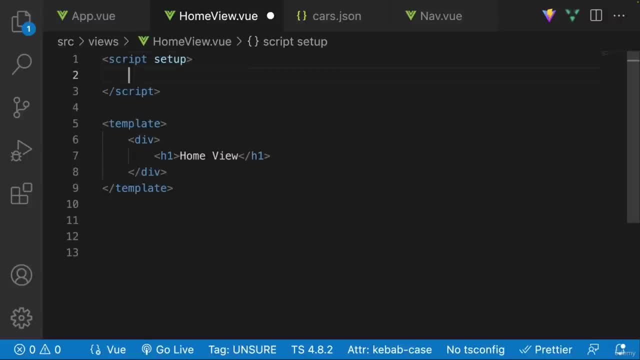 So let's go here, and let's import our, cars, from, the, data, cars, and what we're going to do here is, let's say, over here we have the cars, and then over here we're going to create an anchor tag, that is going to house all of our different cars. 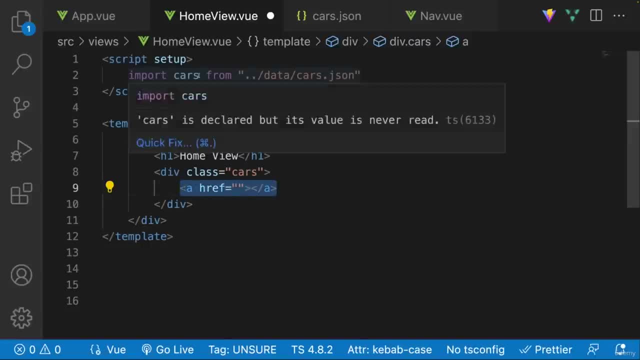 Now of course what we're going to do is want to generate multiple different anchor tags, depending on how many cars that we have. So over here we're just going to say, AV4, and we're going to say car in cars, and we're also going to give this, a unique ID, of car.id, like so. 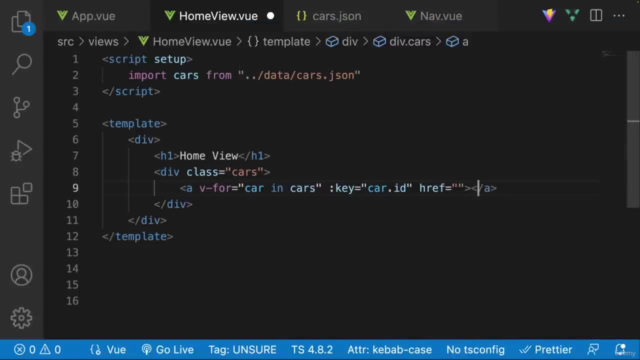 Okay, so this is looking pretty good, and then inside of the anchor tag, what we're going to do is, 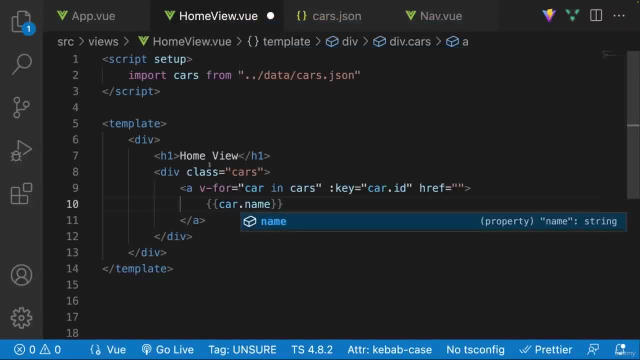 we're going to have the car.name, like so. Alright, so this is looking pretty good. 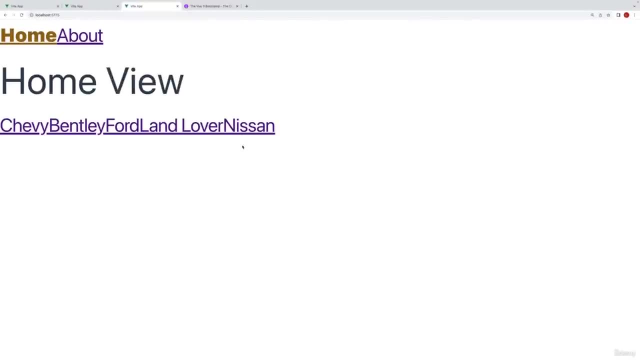 Let's go over to our home view, you can see now we have all of our different cars. Let's just do a little bit of styling, just to make it a little bit nicer. 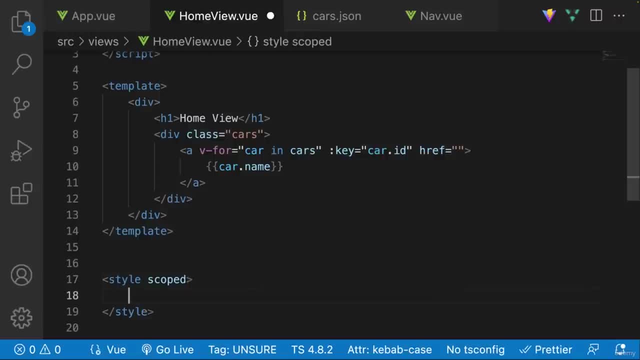 So we're going to say style, and we're going to say scoped, and let's say the cars, we're going to give this a, we'll give it a display of flex, and I think that's it for now. 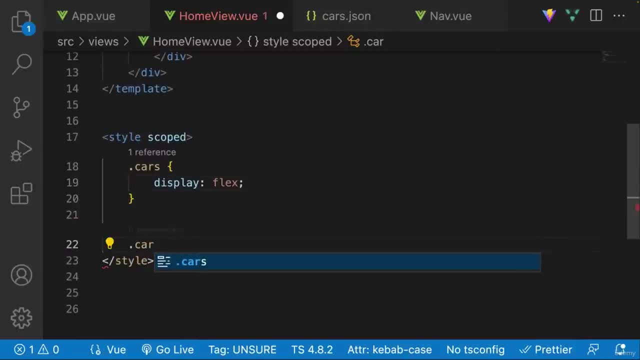 And then for the anchor tags, so cars, anchor tag, let's give this a text decoration of none, 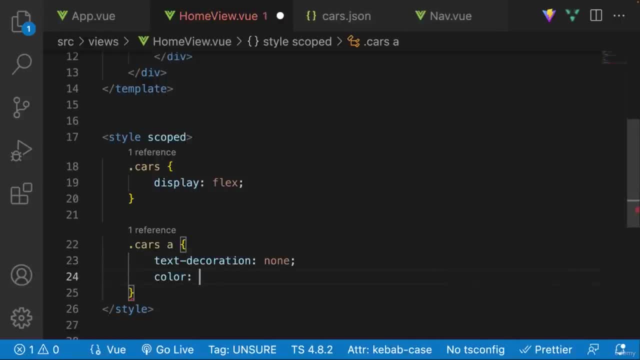 we'll give it a color of just black, or white, we'll do black of course. 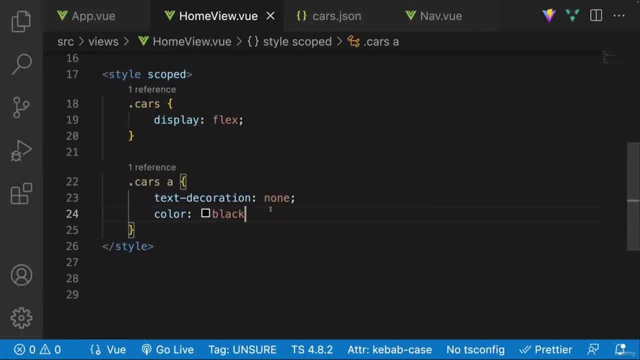 And okay, so this is looking pretty good. Maybe we can give it a width of, let's just do 100%, 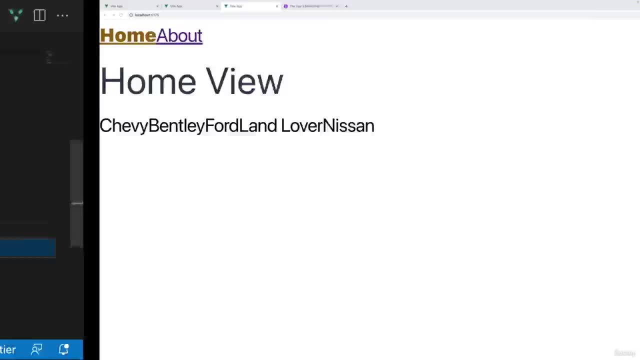 100% width. Alright, let's refresh. 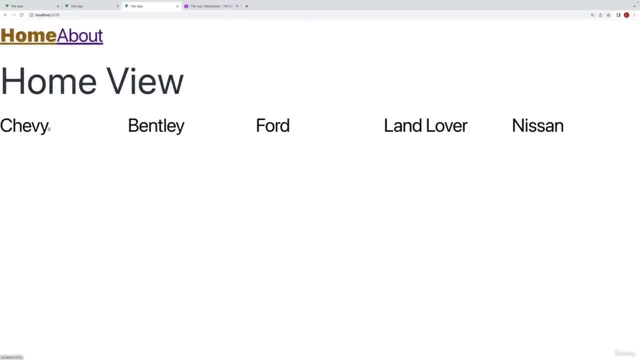 Okay, looking pretty decent now. And let's also give it, 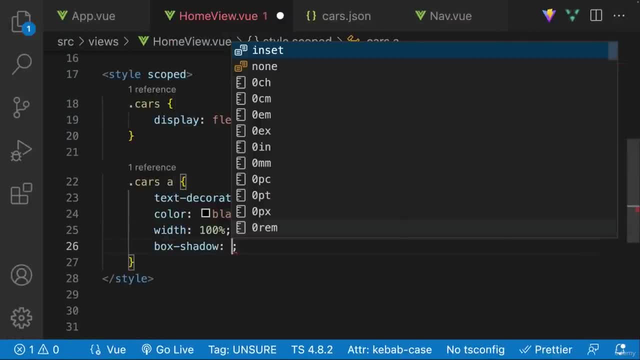 maybe a box shadow, of zero, or let's do one pixel, one pixel, one pixel, and then maybe a blackish color here. 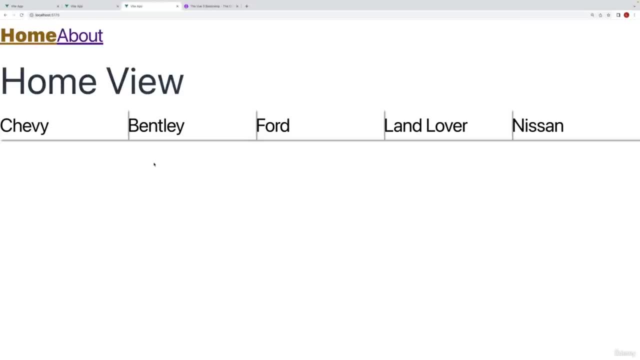 See how that looks. Alright, this is looking pretty okay. Not great, but it's okay. 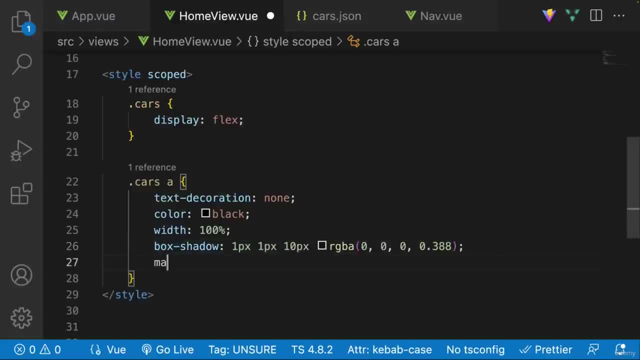 And let's also give it just some margins. We're going to say margin, and we'll say 10 pixels. So let's do a quick refresh. There we go, okay. 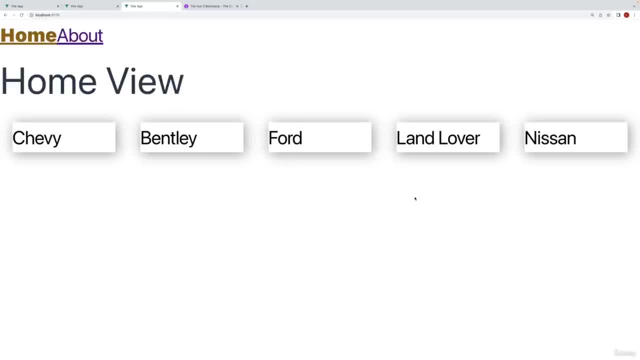 Obviously this doesn't look beautiful, but who cares? We want to learn about routing. 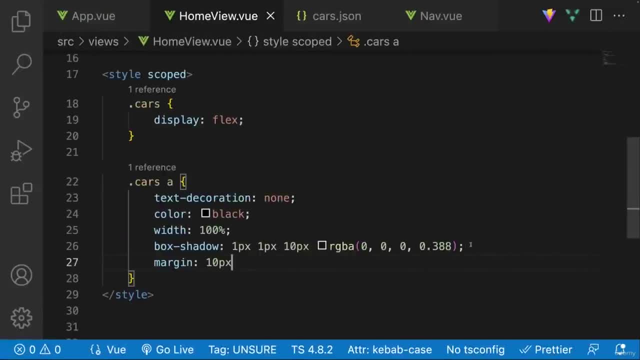 We don't want to care about styling. So now we have our cards, but this is just hideous. 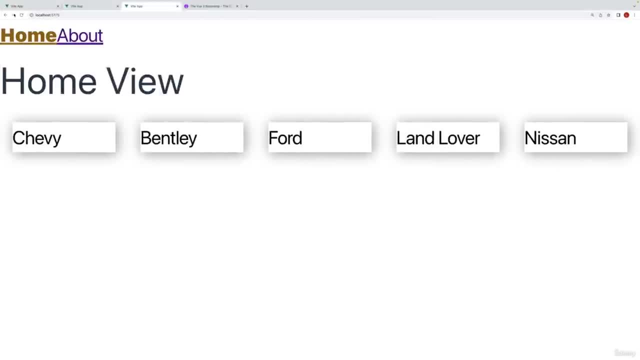 Let me just reduce the opacity a little bit. Okay, there we go. 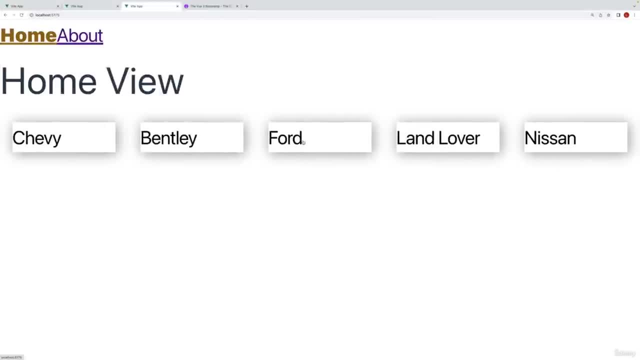 So this is a little bit more variable. Okay, so when I click on a particular card, 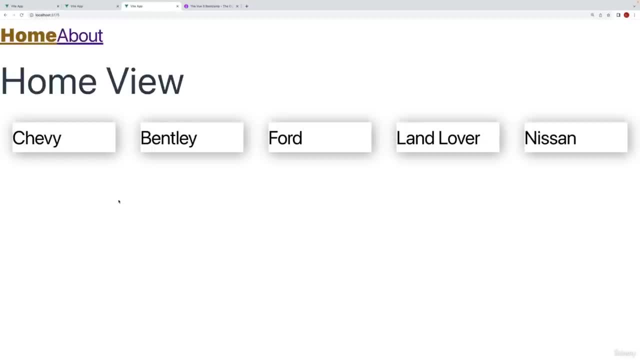 what I want to do is I want to get redirected to slash cars, slash that particular car's ID. 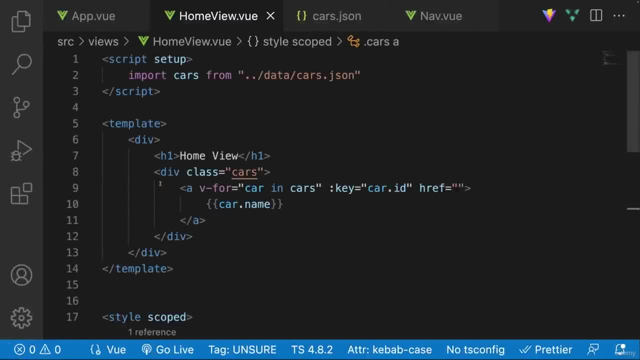 And this is something that we, you and I should already be able to do. 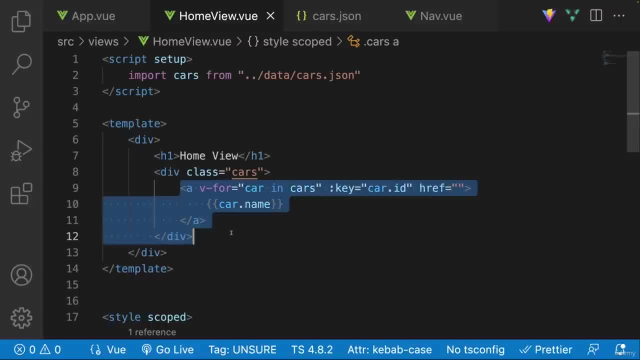 We've already learned how to do this. So we want to redirect. So we could keep it as an anchor tag, but of course this is not great because it's going to refresh our application. 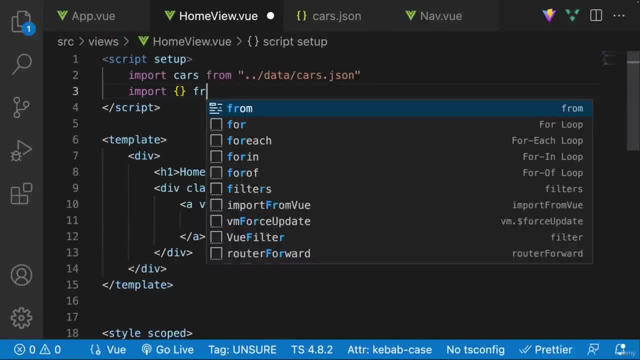 So instead what we're going to do is we are going to import the router link from view router. 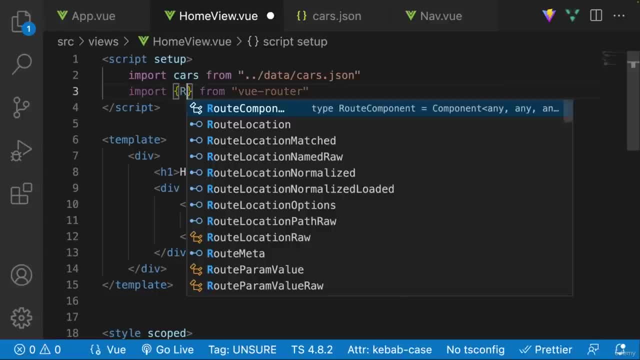 So we're going to say router link. We're going to import that from view router. 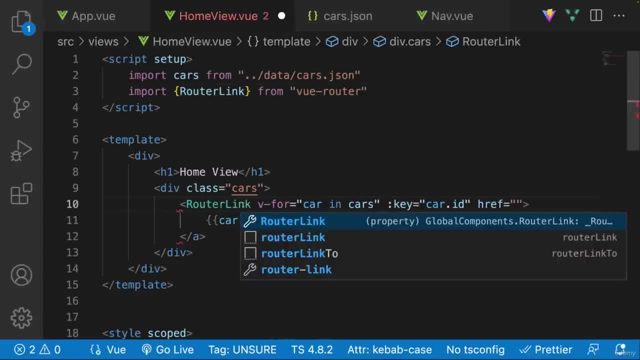 And then over here, router link like so. 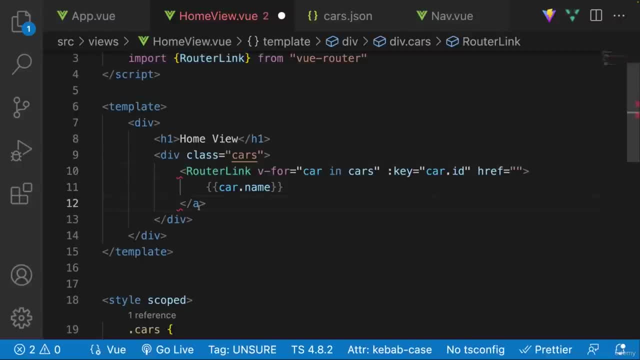 And let's copy this. And let's go ahead and do that. 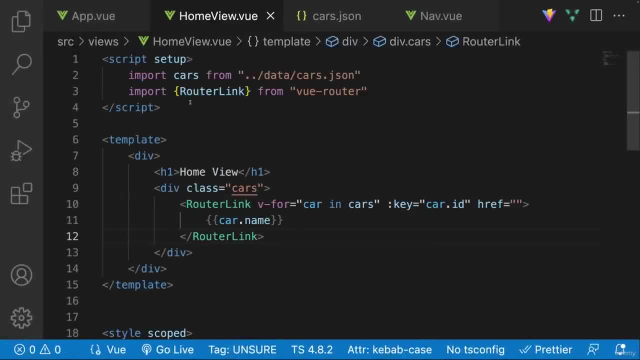 So obviously these styles, well, I mean the application at this point is the cars are not showing up because we need to add a two. 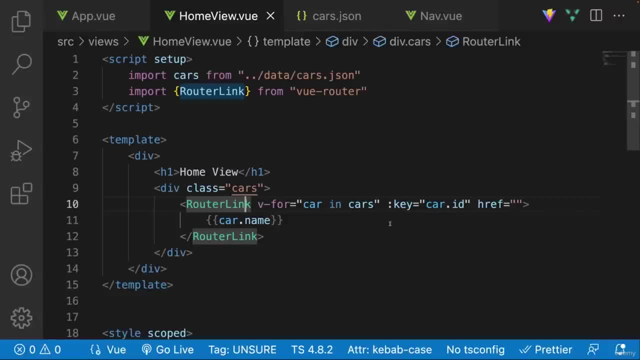 But the style should remain the same because this is still an anchor tag. 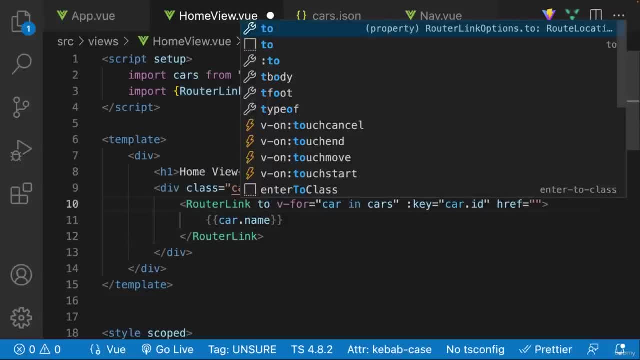 So let's go over here. And we're also going to add a two. So remember we have to define where this is going to. So again, what we wanted to do is we wanted to go to slash cars, 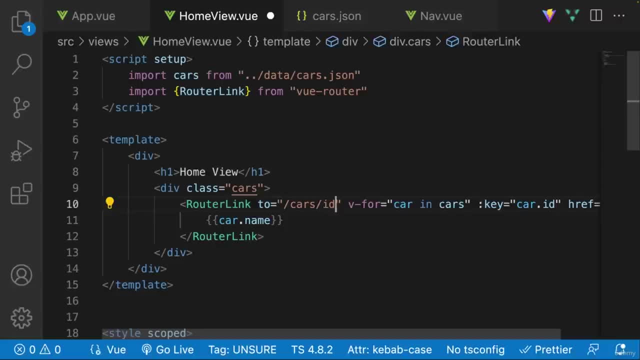 slash whatever that car's ID is. Now that car's ID is going to come from over here, car, and then dot ID. 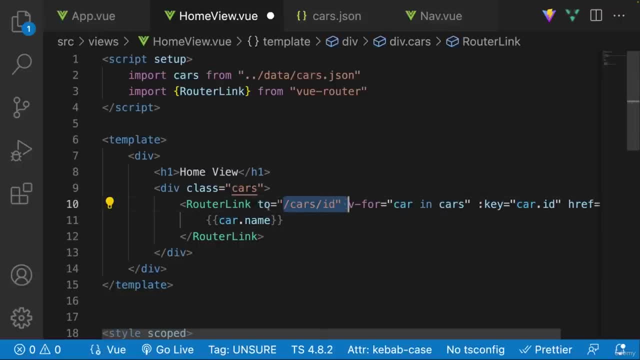 So we need to turn this into JavaScript rather than an ordinary string. 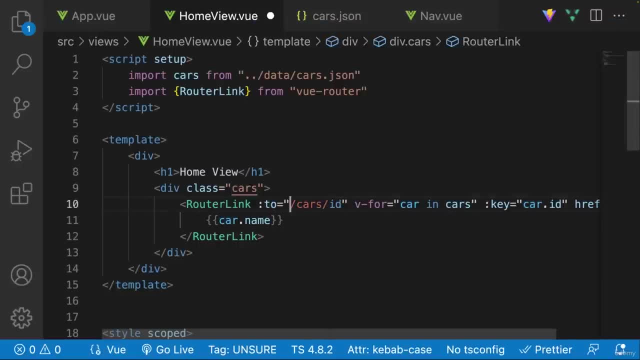 So to do that, of course, we're going to add the colon. And now over here, we're going to add template literals. 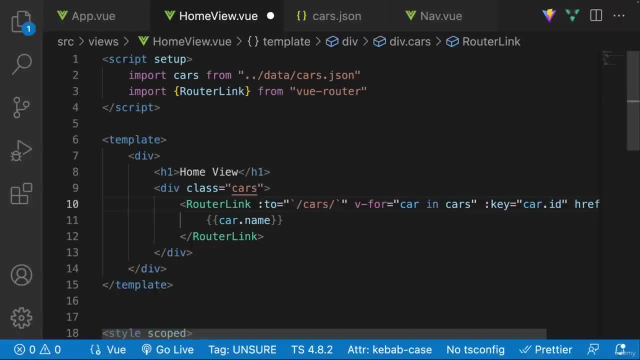 So template literals. And then here we're going to say dollar sign, curly brace. 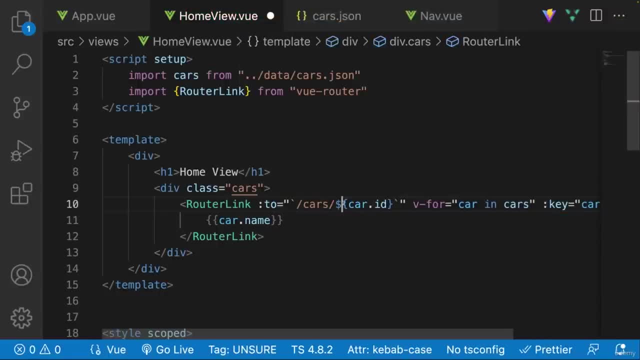 And then we're going to dynamically add the ID. So now we're going to have slash cars, slash whatever the ID is. 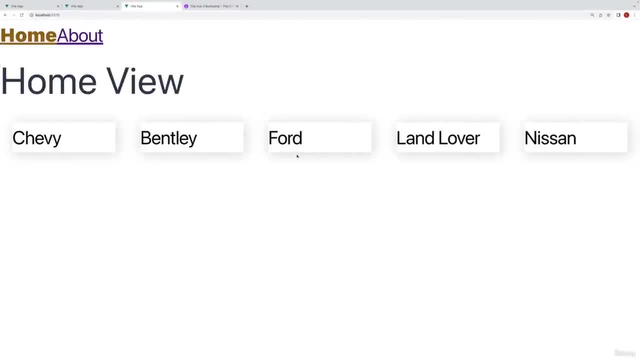 So let's go ahead and save that. And now we get our card. 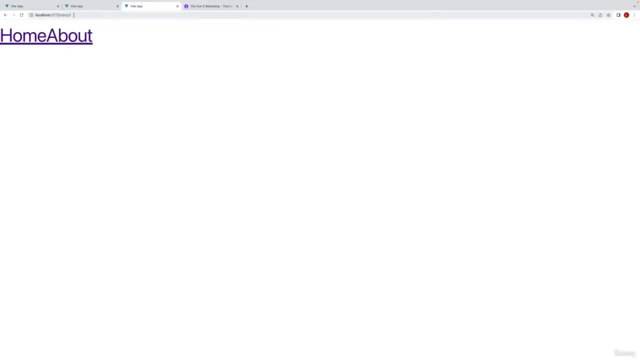 And if we go over here, you can see that we actually get redirected. And unfortunately, I cannot zoom in here, so you might not be able to see it. 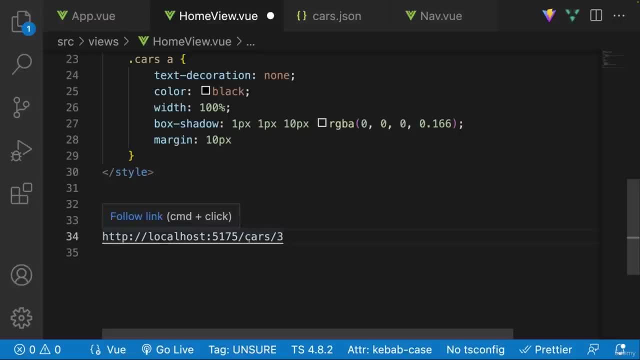 So I'm just going to copy it. So we got redirected to slash car, slash three, which is terrific. 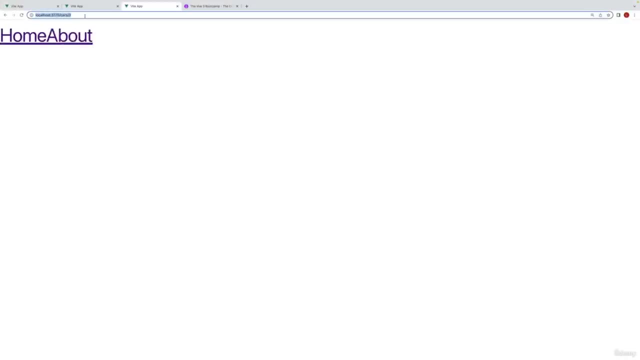 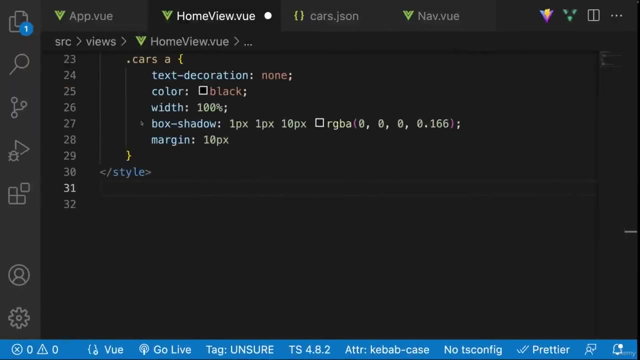 So now what we actually need to do is to, well, actually dynamically render a page. So how are we going to do that? Well, we're going to need to define some new routers. 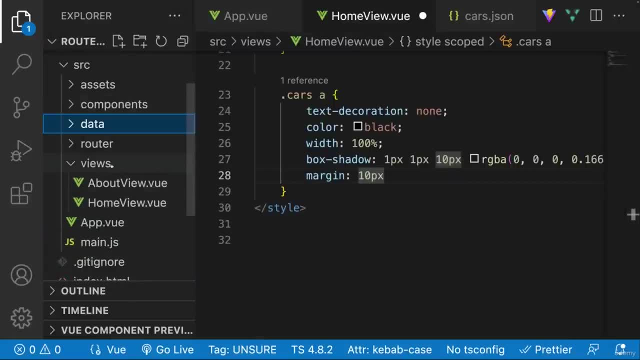 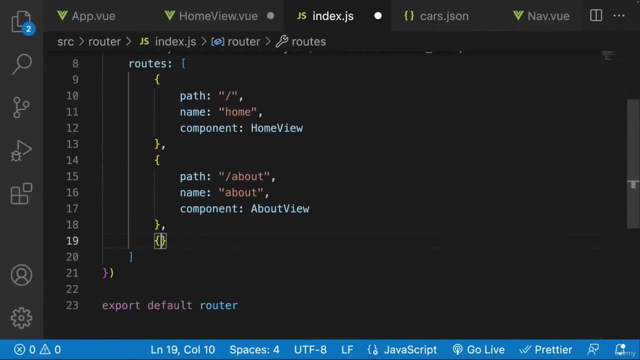 So I'm going to go over here. Let's go to our router. We're going to define some new rules. So over here, what I'm going to say is I want some new rules. We're going to define a path. Of course, we're going to call this name. We're going to call it card because we're really just looking at one particular car. 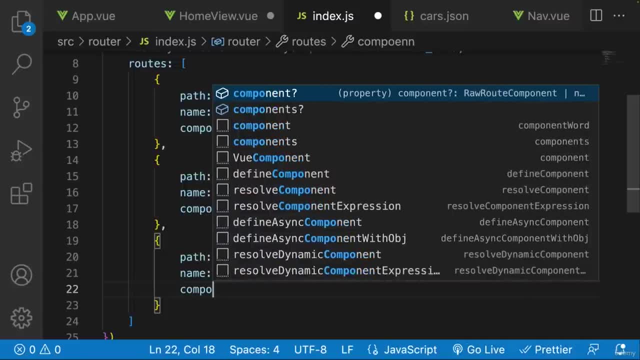 And we're going to say the components. So the component is, and we haven't really created the component yet. So let's go ahead and create this view component. 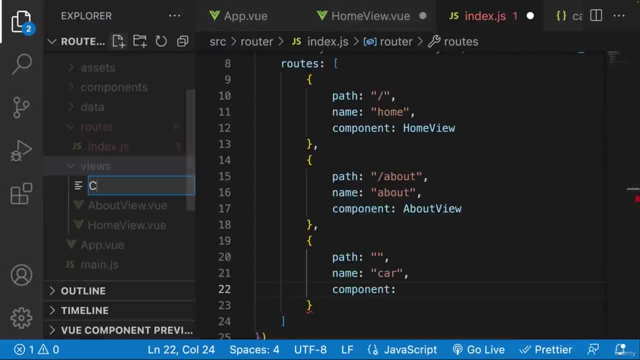 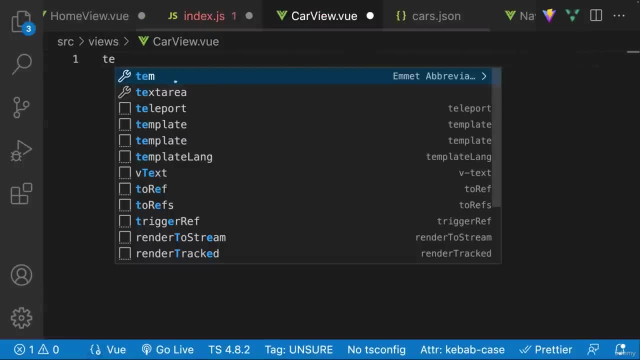 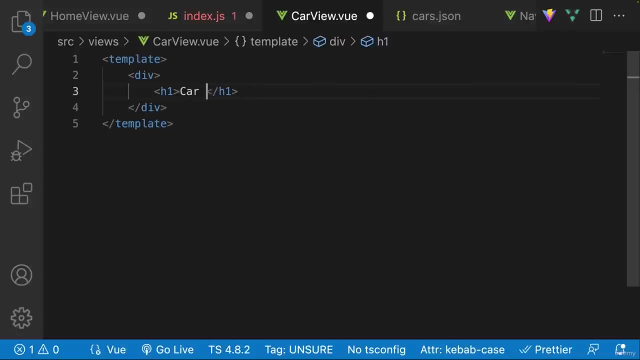 And we're going to call this car view dot view. And over here, we'll just say templates and div. And we're going to say H1. We're going to say car view like so. 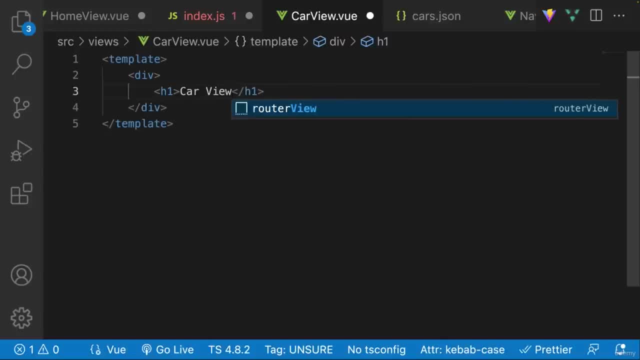 So we want to render this render this component over here. Anytime we have a path of slash car, 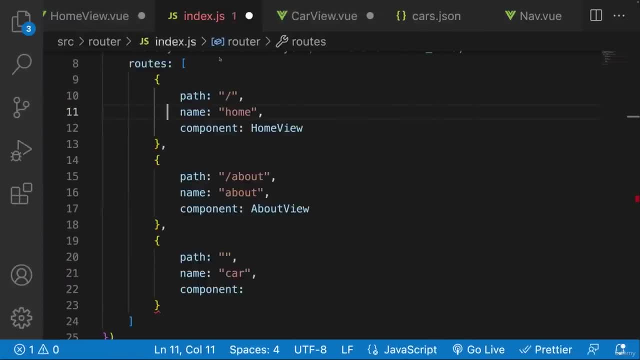 or I think we call this slash cars. Yeah. Slash cars. So anytime you have a path of slash cars, 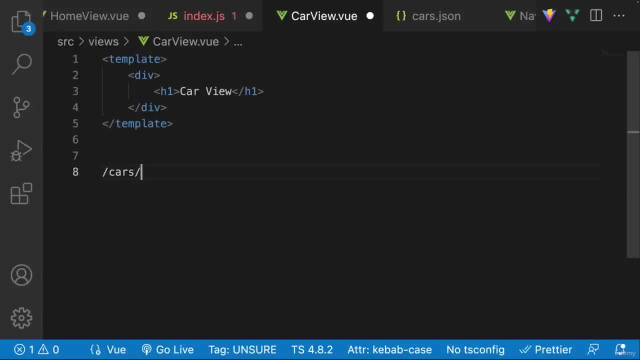 slash any ID over here. So it could be anything. Five, six, seven, eight, nine, 10. 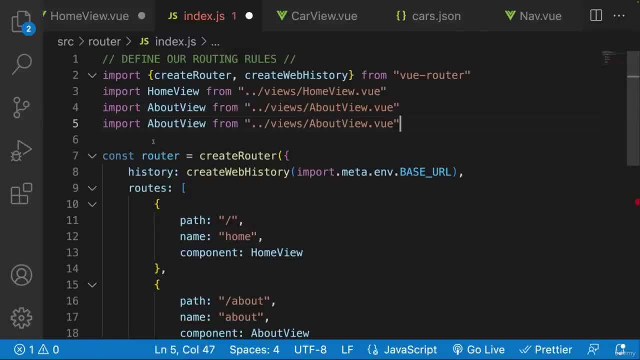 So that's what we want to render. So let's go back over here to our index dot JS. Let's import our car view or yeah, 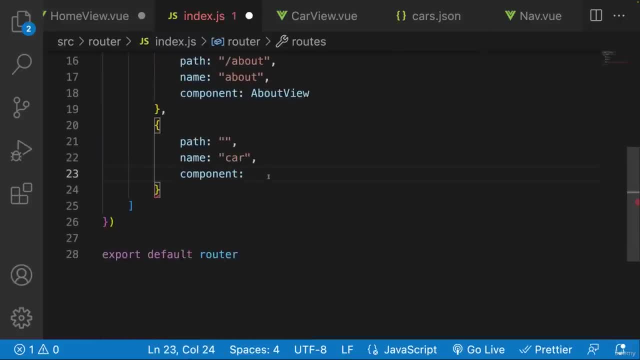 car view, car view like so. And this is the component that we want to render the car view. 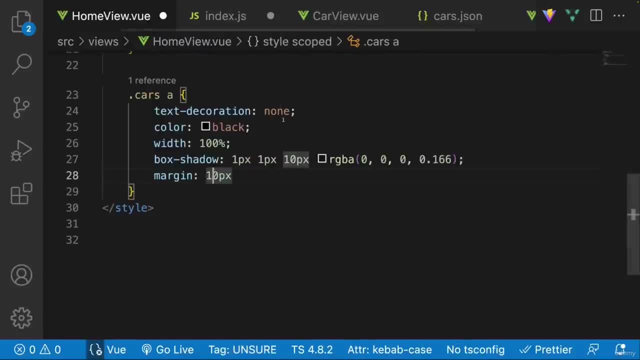 So now let's talk about the path. This is where it's going to get a little bit tricky. So let me just go ahead and save this for now. 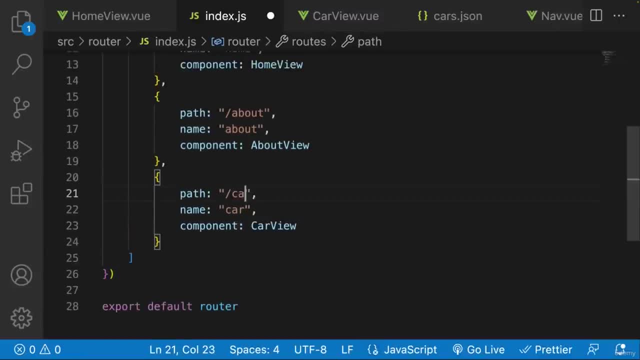 So the path this time is going to be slash cars and then slash a dynamic ID. So it could be anything. It could be whatever it is that we want. 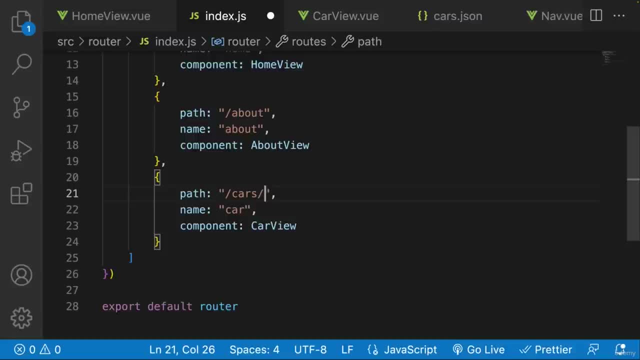 So what are we going to do in order to specify that this is going to be dynamic? Well, very easily what we're going to do is we're going to do slash and then we're going to say colon. And then we're going to give this dynamic. Path a variable name, and we can call this whatever it is that we want. 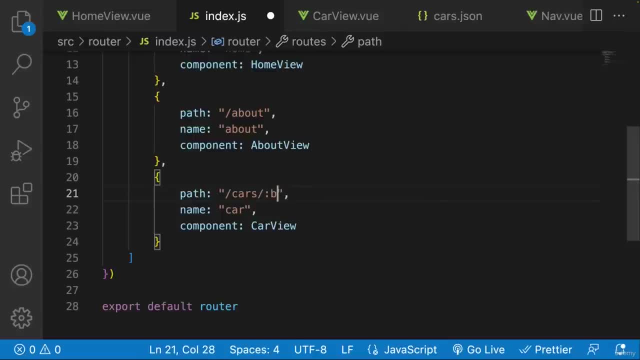 We can call it ID. We can call it banana. We can call it whatever it is that we want. 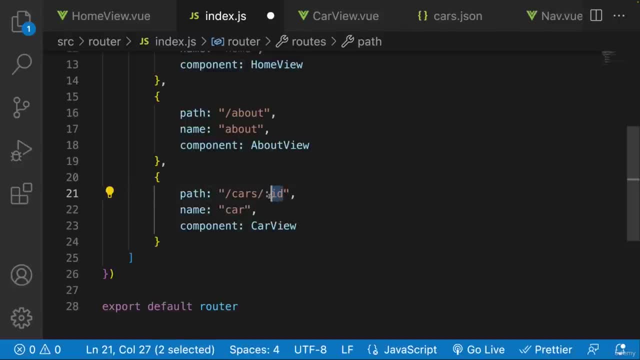 But by adding this colon and then giving it a variable name, we are essentially saying, Hey, we want to render this car car view. 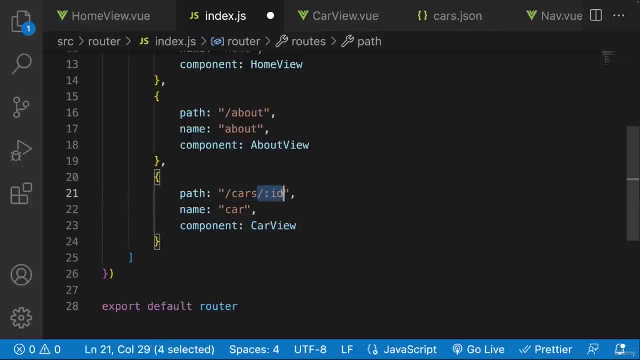 Anytime you go to slash cars slash some dynamic path over here, this could be anything. 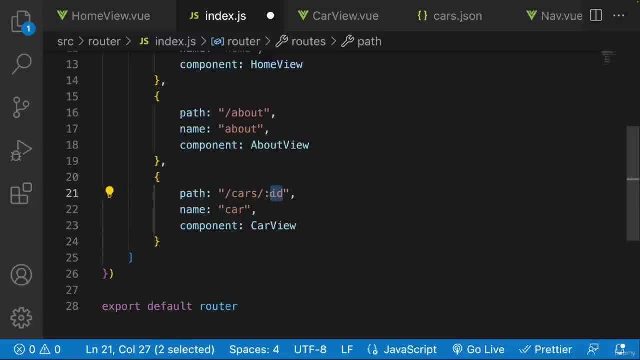 And we're going to assign that dynamic path to the variable of five. ID. So now that's pretty much all it is that we need to do. 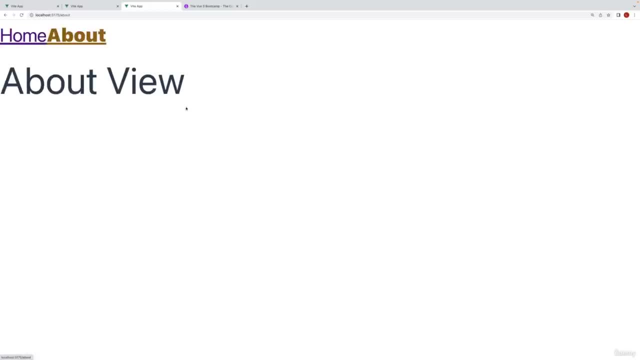 Now, if I go home and about, if I go home and I click on Ford, for example, you can see, I got redirected to this car view, even though my path is slash cars slash three. 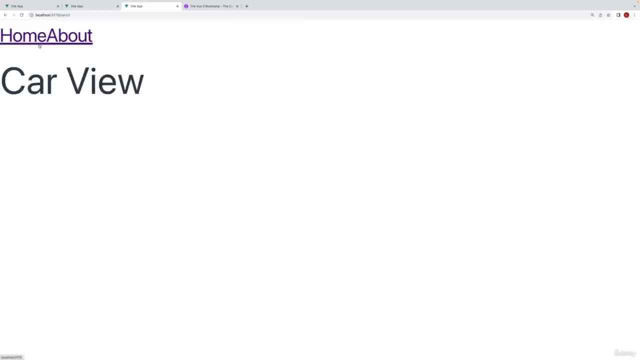 If I go to Nissan, same thing, same thing, same thing. 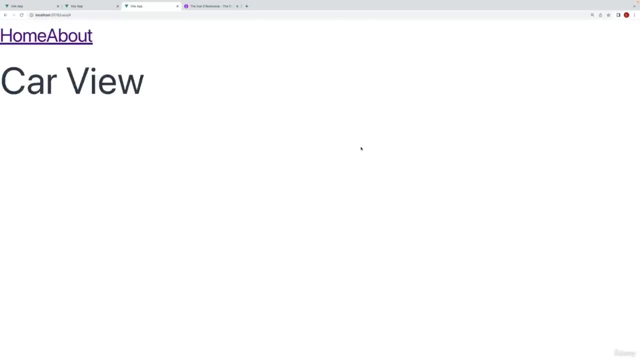 So now we figured out how to dynamically render a component based on some dynamic routes. So we have created these wonderfully dynamic pages. 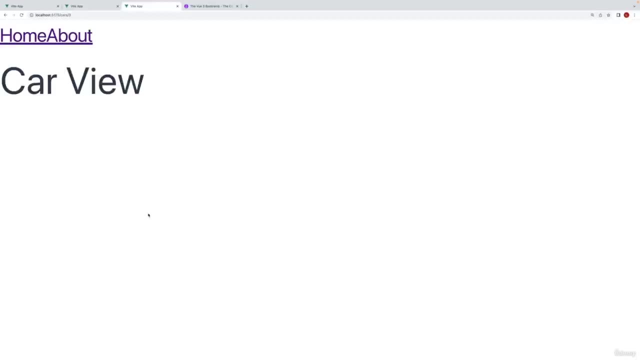 But now what we want to do is within these dynamic pages, we want to render the data of that particular car. So what we're going to need to do is somehow extract the ID from the path that we have defined. 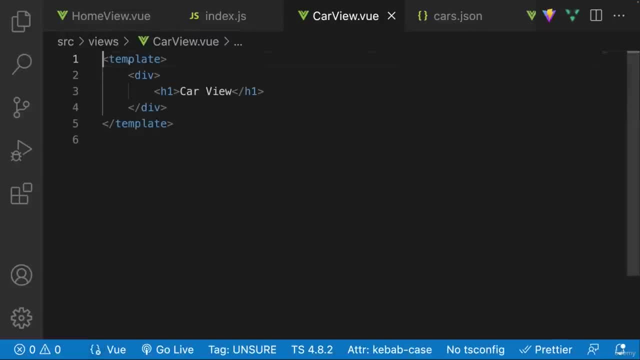 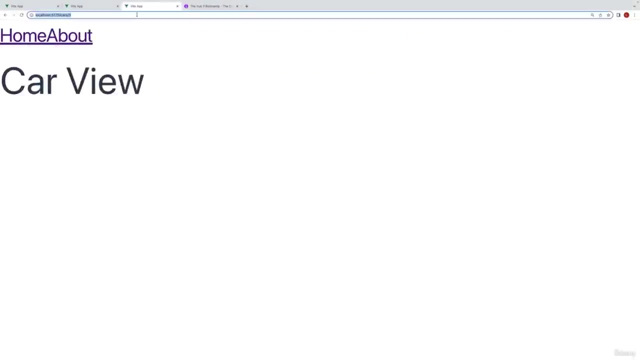 So let's actually go ahead and go to our car view and let's create some script tags. We're going to say script set up like so. And then right over here, what we're going to do is we're going to need to figure out a way to extract the ID from this path. So again, over here it's going to be slash three. 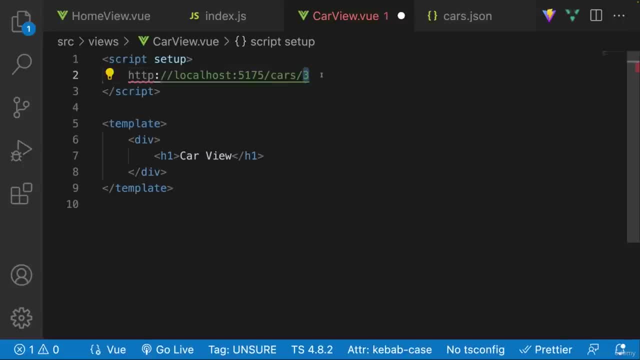 And this right here is given the variable of ID. So we can actually do this by importing something called use routes from view router. So over here we can say view router and we can import something called use routes. 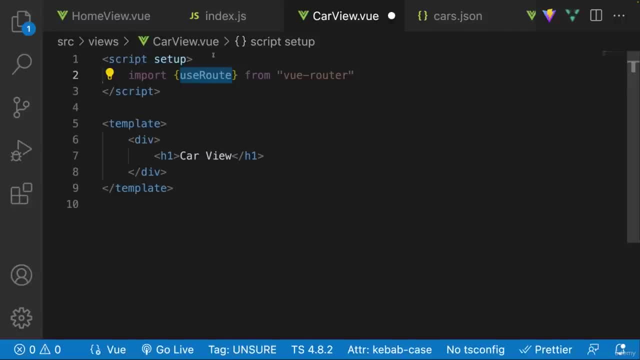 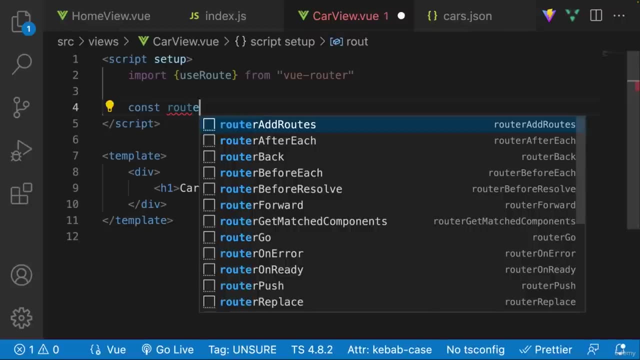 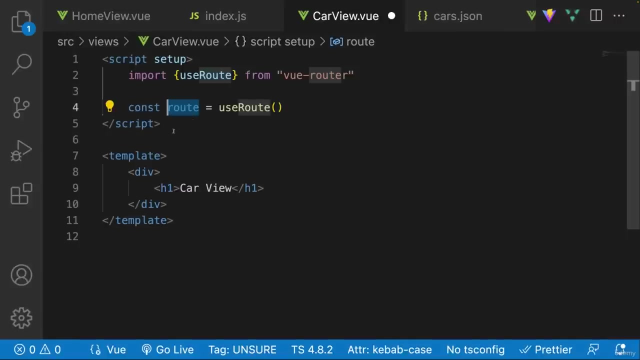 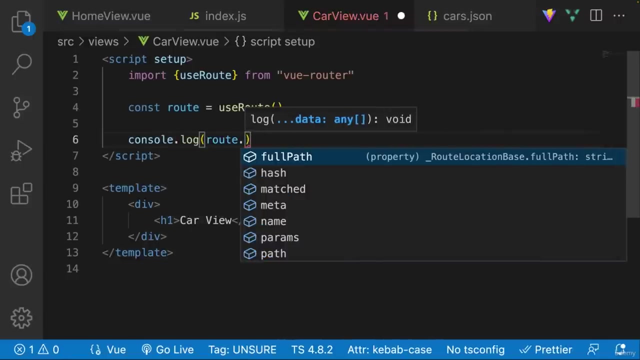 And this is actually something known as a composable that we'll talk about a little bit later in the course. But now in order to actually utilize this, what we can say here is route is going to be equal to use route and we can invoke it. And we can actually get all of the different information about the route that we are currently in by utilizing this route variable. Specifically, we can get the params. So if I were to console dot log, route dot param. So let's say params can go ahead and log this. 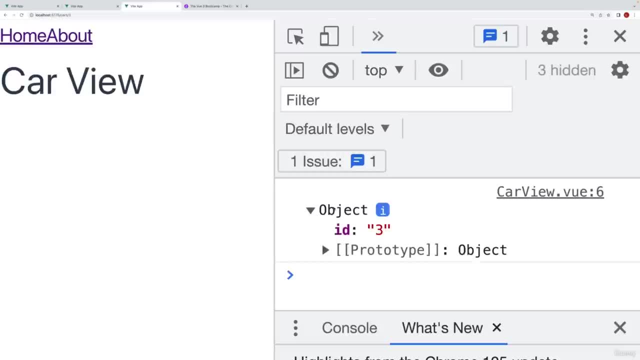 And if I were to go to the log, you can see this is an object and you can see we have the ID variable. 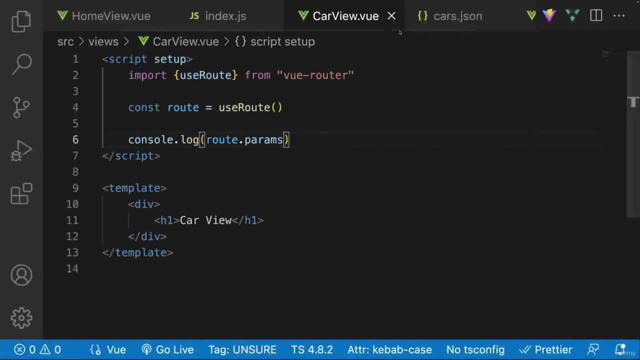 Remember, this is a variable. And right over here, 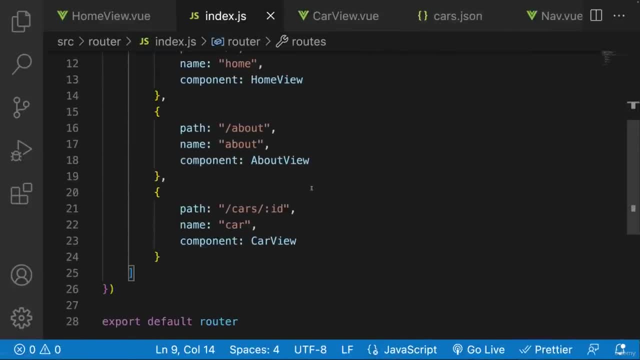 it's a variable because we assigned it right over here as ID variable. 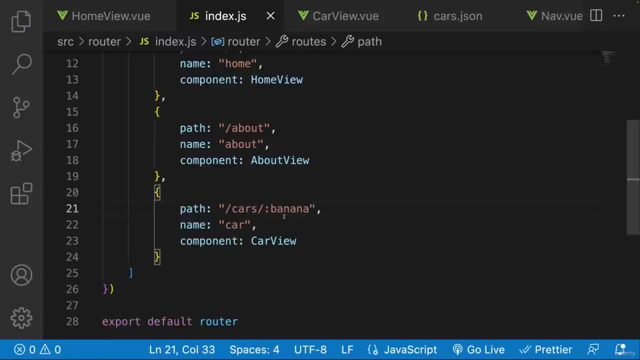 Now again, if I change this to like banana, then the object is going to be banana like so. So I hope this helps. I hope this makes sense. 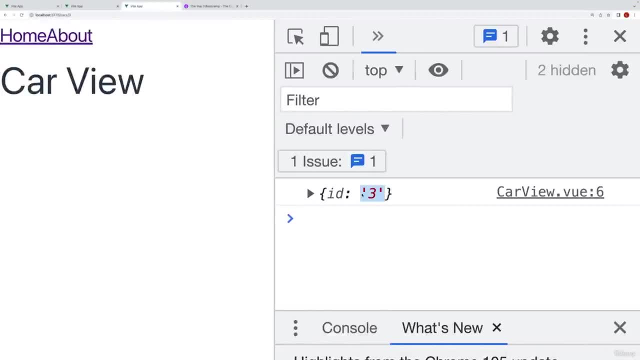 This is the variable that we assigned it to. And its value is the string of three. 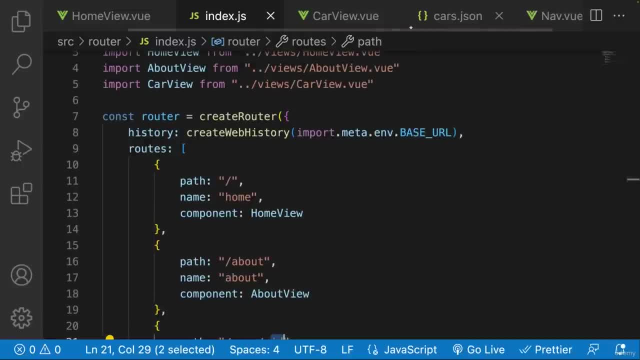 So even though over here, it's actually an ID. 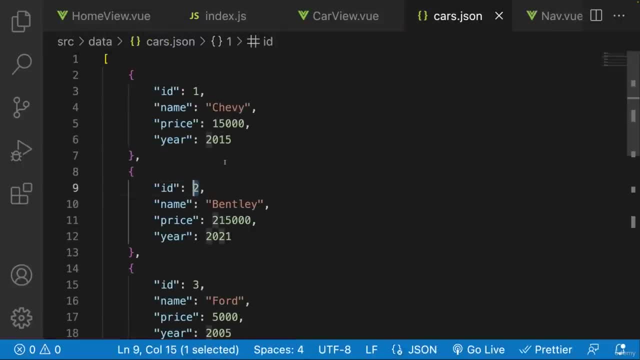 So in our JSON file, it's actually a number inside of the path param. 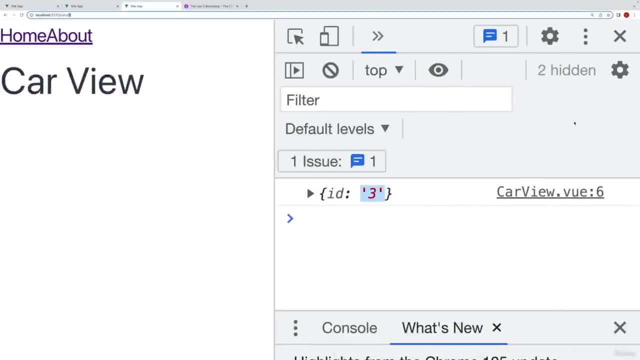 Even if it is a number is always going to be returned back to us as a string. 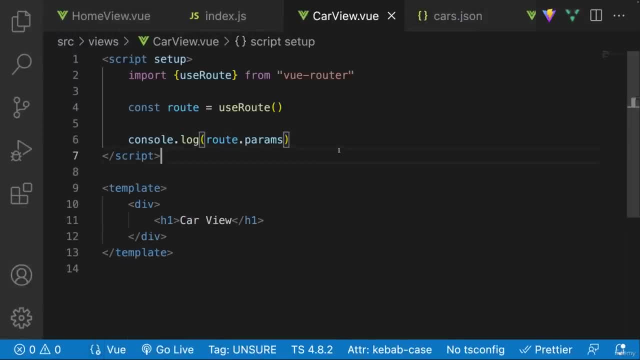 So nonetheless, now we got the information that we need. 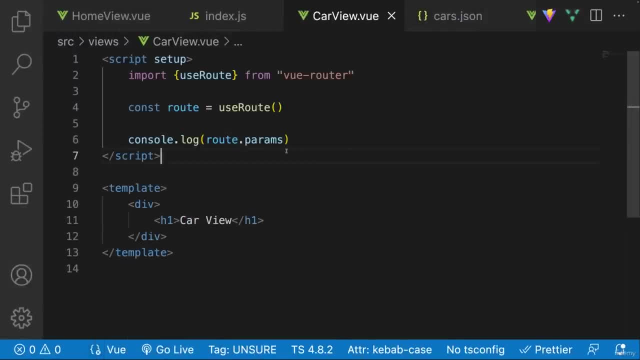 And of course, now we can utilize it to figure out which car data do we need to show. 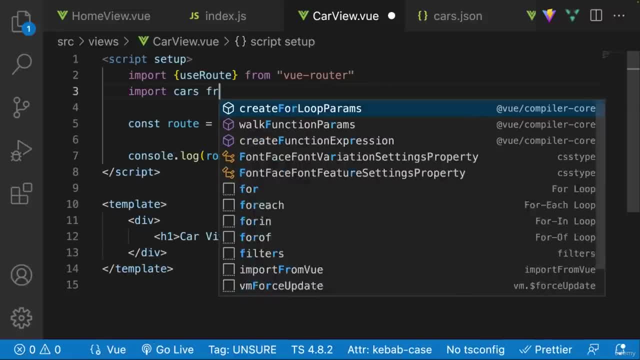 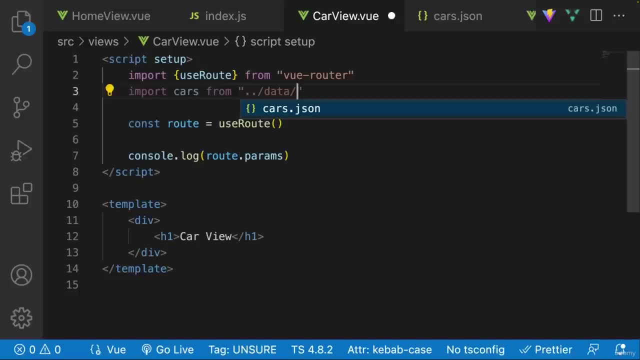 So let's go over here. And we're going to import cars from, and we're going to import cars from, let's say data slash cars. 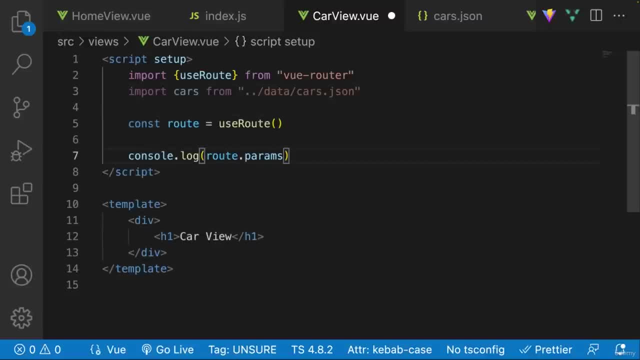 And we need to find the particular car that we want. 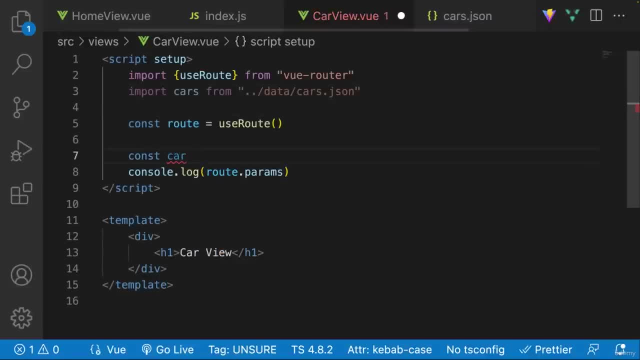 So what we can say here is const car. And we can say over here. Well, 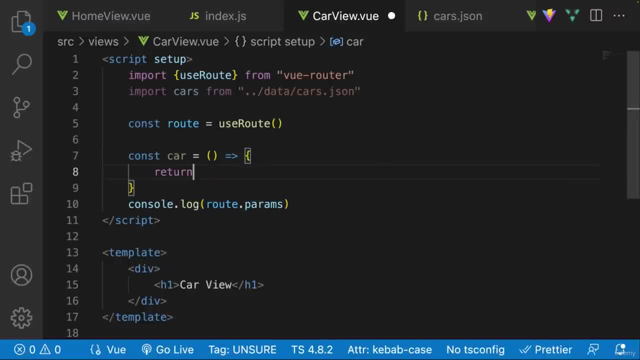 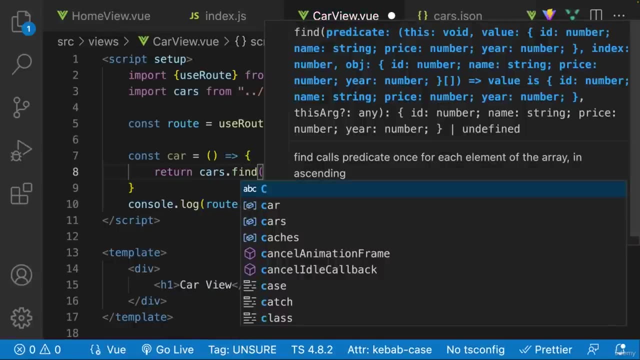 what we want to do is we want to return. Well, we are going to, yeah, we're going to return cars dot find, and we're going to find the car that has the ID that is equal to. 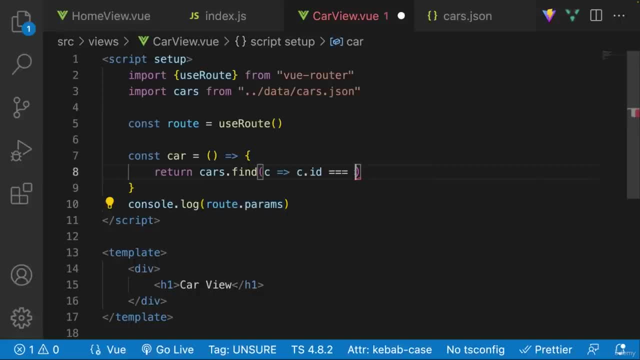 And over here, what we can do is utilize this and we can say parse int, 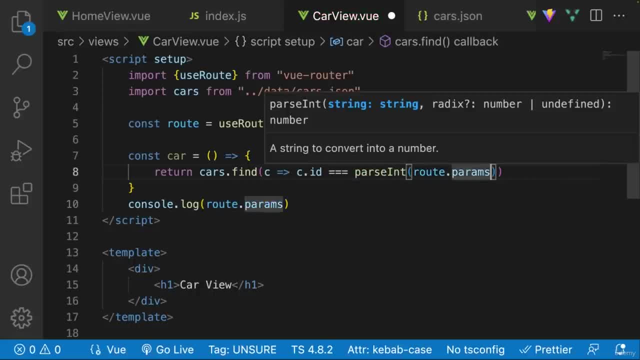 because remember this is going to be a string. So we can say parse int route dot params dot ID like so. And now what we can do, if I were to. 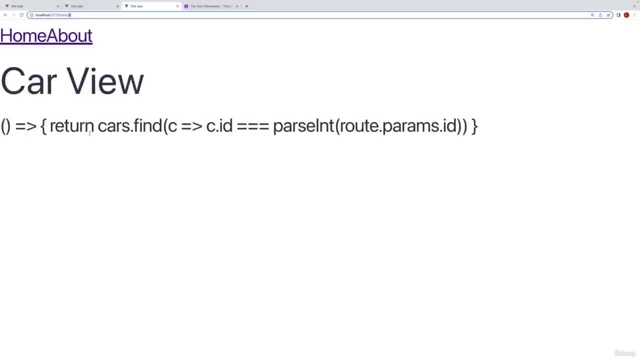 Right here, render the car data. Okay. 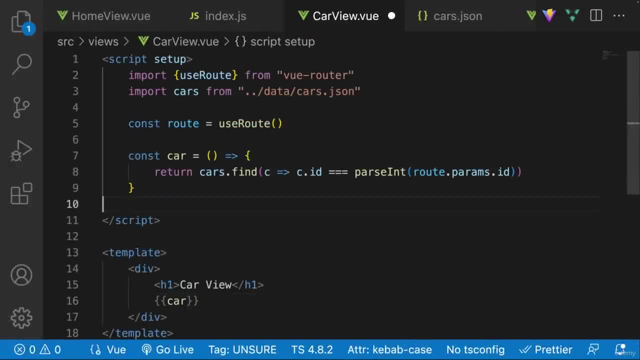 So this is looking pretty good. So over here, 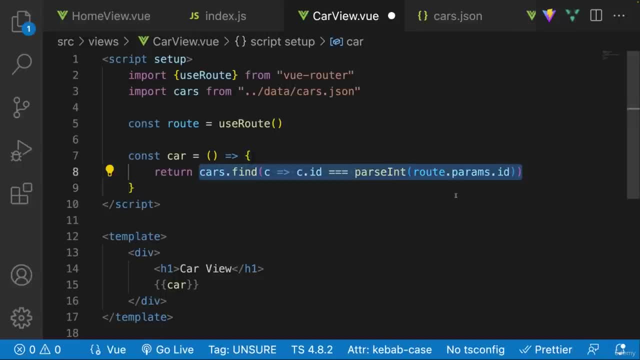 actually what we can do is this shouldn't be a function. It should be kind of like this. There we go. So now there you go. You see, 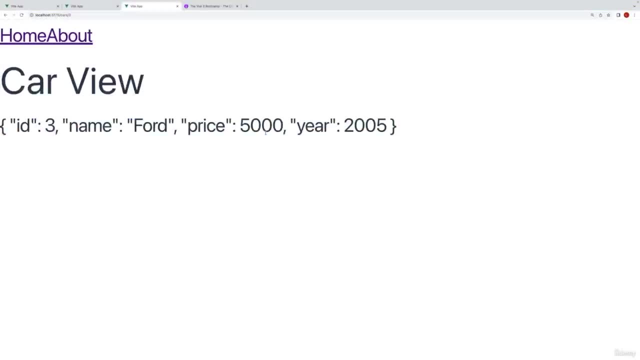 we have this object that has an ID of three and name of Ford, the price and 2005. 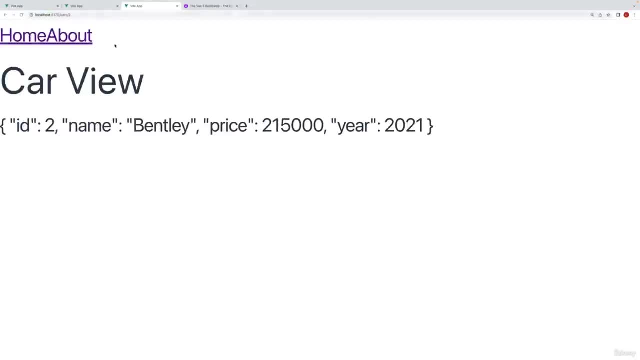 Now, if I were to change this to, let's say two, for example, you can see now we get different data. 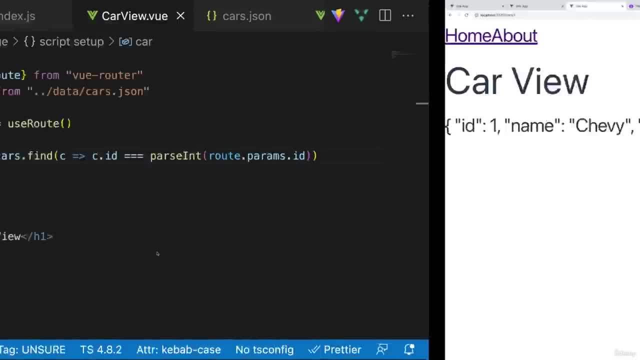 So now we can actually render all of this data that we need. So let's go over here. 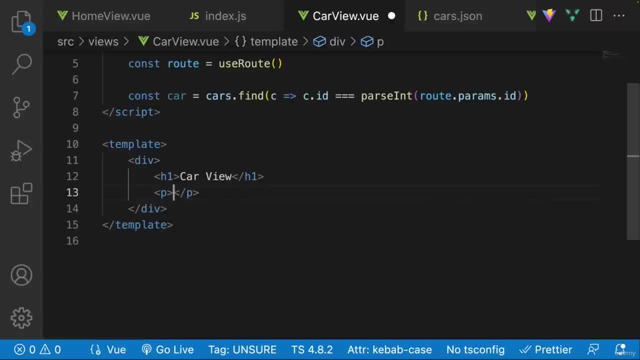 Now we can start showing more information. So we can say something like car dot name and let's add some more stuff. 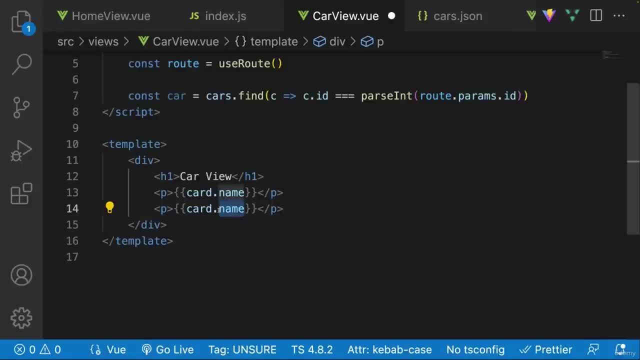 So let's add the car dot year. And lastly, I believe it was car dot price. So there we go. 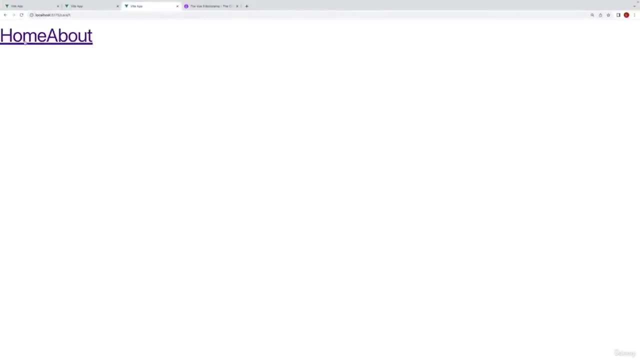 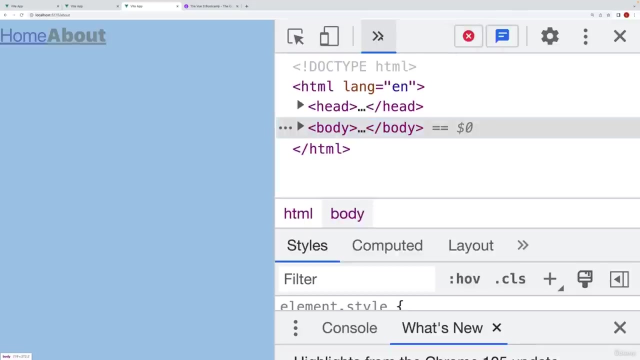 So now if I were to read, refresh and I were to go to my home view and well, something's going wrong. Let's see what that is. Let's inspect console. And we have some air handling here. So it's saying here cannot read property. No. Okay. That is completely fine. 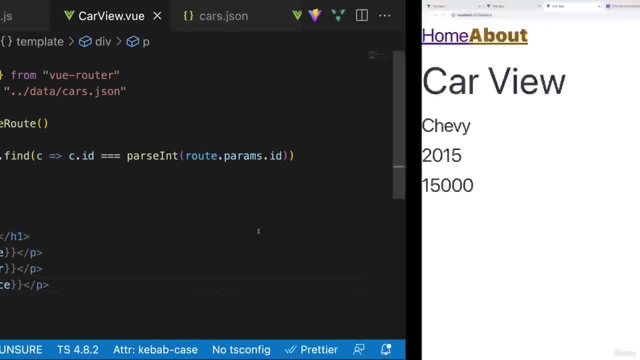 Oh, oops. It's not car. It was car, not card. 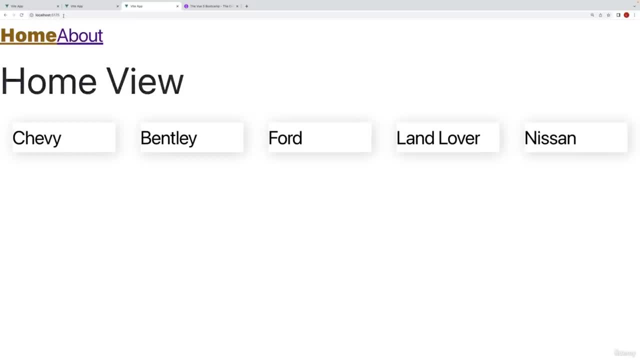 There we go. All right. So let's go now to our home view. 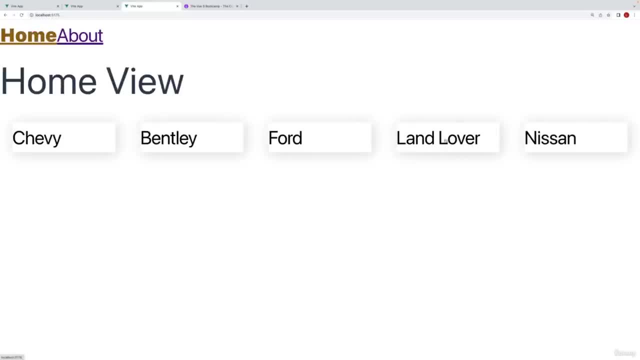 So this is our home view. If I click on Land Rover, for example, I get to Land Rover. If I go to Chevy, I get the Chevy information. If I, let's go back home. If I go to Nissan, I got the Nissan information. 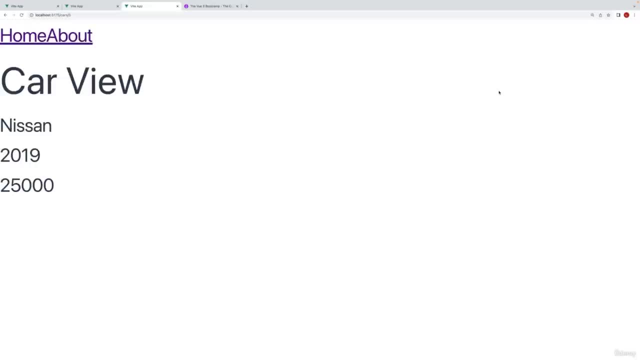 So this is how we can actually dynamically have different data, but really still have the same exact path. Okay. So this is what we have thus far. When we click on a particular car, 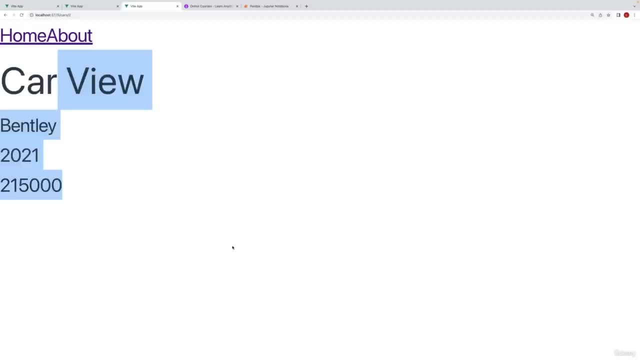 it shows us the information about that car. This is great. And actually some pretty advanced use cases. Oh, the view router, 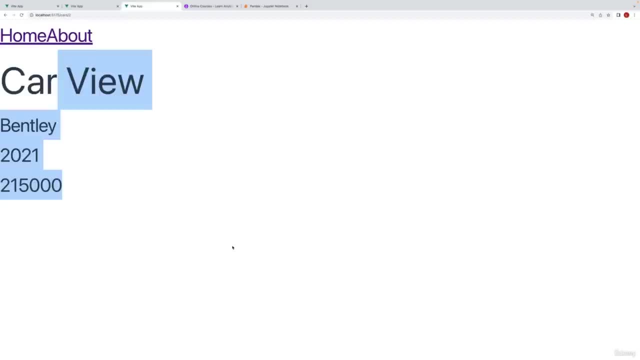 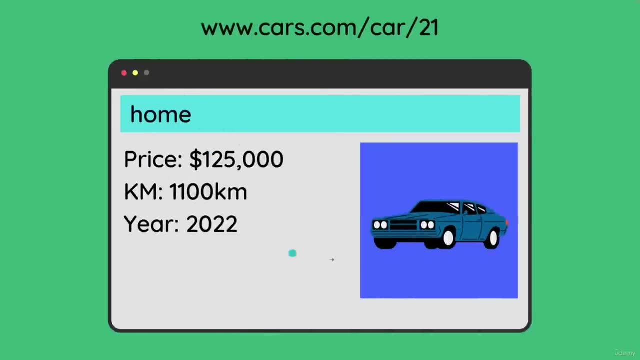 but let's actually take this one step further. So let's look at this page and let's of course, imagine that it's kind of similar to this page. We have just information about the car itself. Obviously stylistically, it's not there. 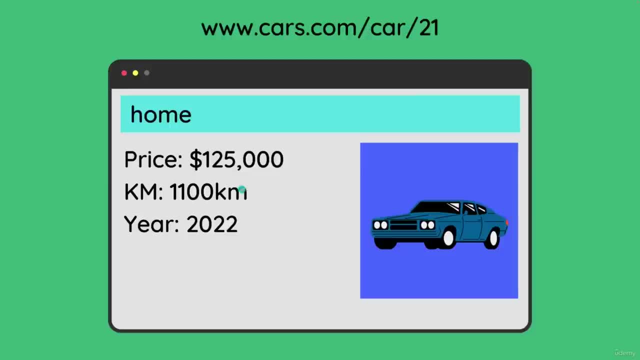 We don't have an image, but this page is representative of this page as this page has information about a particular car. And so does this one over here. 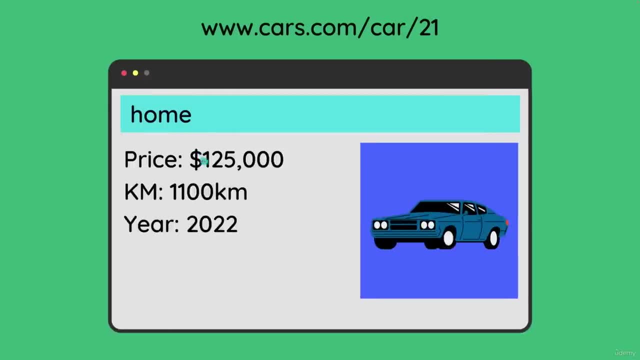 So let's go over here and let's say we want to add a new car. So let's say we want to add a new component where a user can actually contact the dealer that is responsible for selling this car. 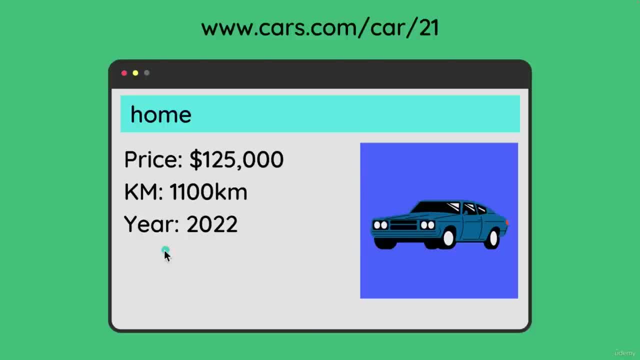 Now they can only access the component within this page. If they go to the path of slash car, slash 21, and then slash contact. 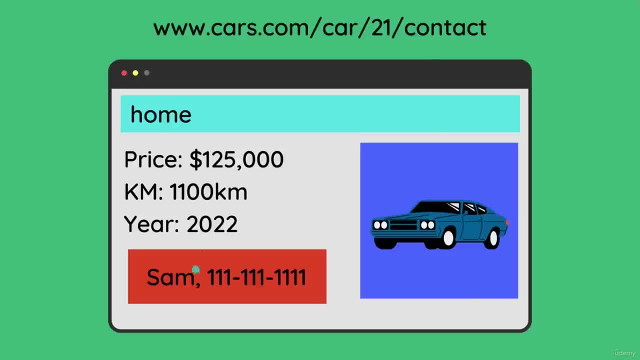 And only when it's slash car slash 21 slash contact. Do we display this component? 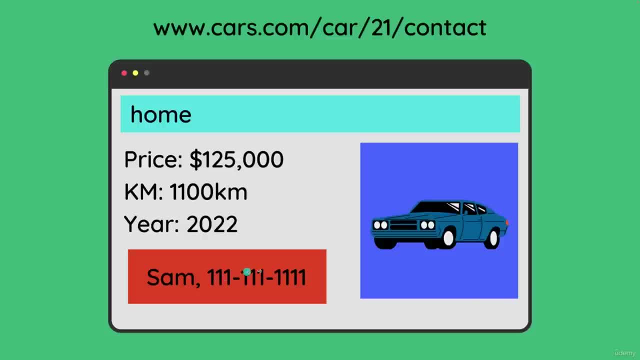 Now, this is actually a little bit different than what we've been doing before 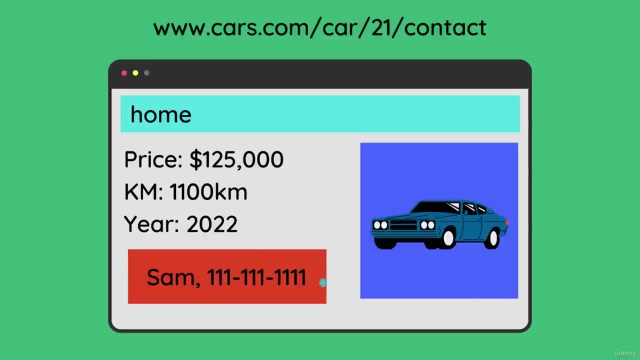 because this right over here is actually a nested route. So we have a nested route within an existing route. And only once we get that particular nested route or this child route, do we show this component? 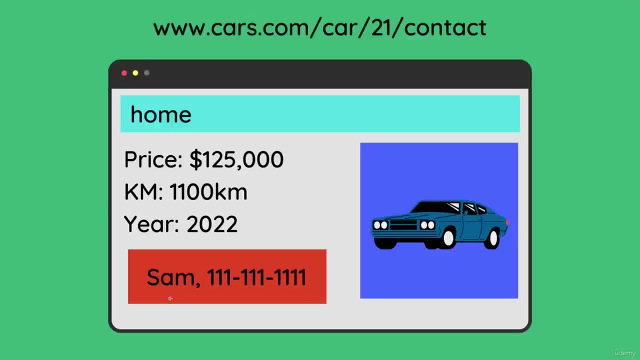 Now, the way that we do it is actually kind of overall the same. 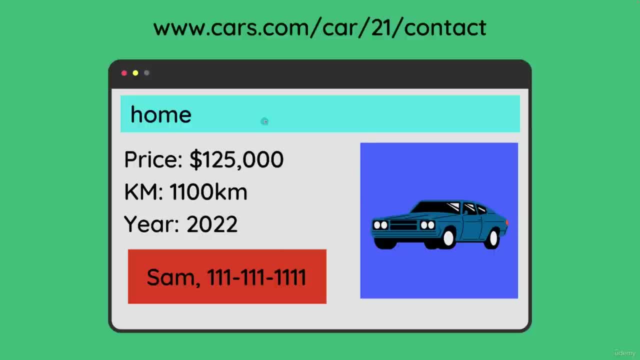 However, we're going to be dealing with this page right over here. 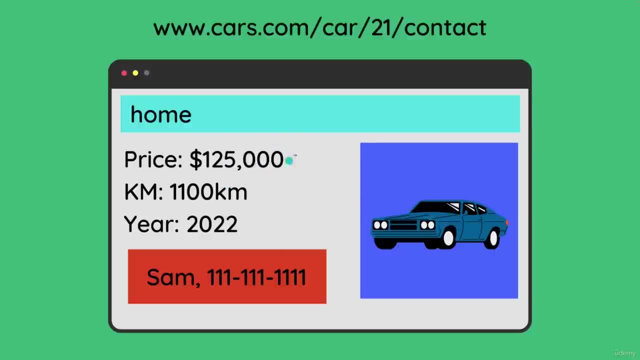 Now, if this makes sense, let's just actually go ahead and code this out. And hopefully by then it will. All right. 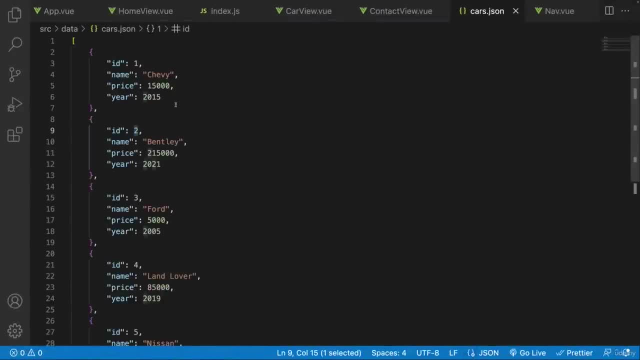 So what I'm going to do now is I'm going to go to my cars dot JSON. And I'm just going to add a little bit more data. 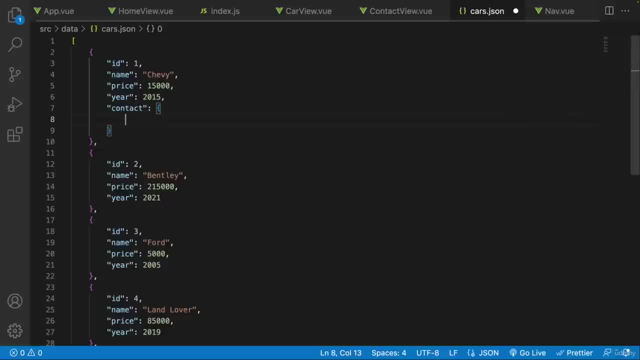 So I'm going to go over here. I'm going to add contact. And this is going to be an object. And we're going to say dealer. 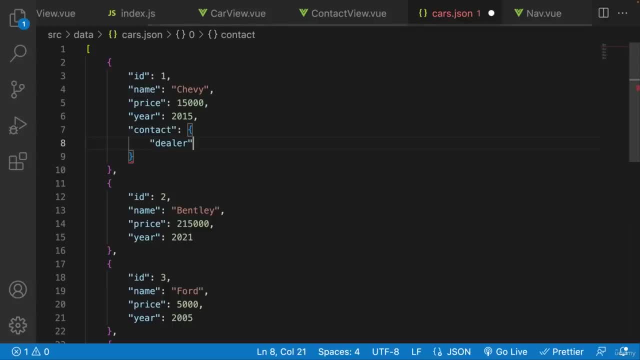 Let me zoom in here for you guys in case that's a little bit too small. There we go. We're going to say dealer. 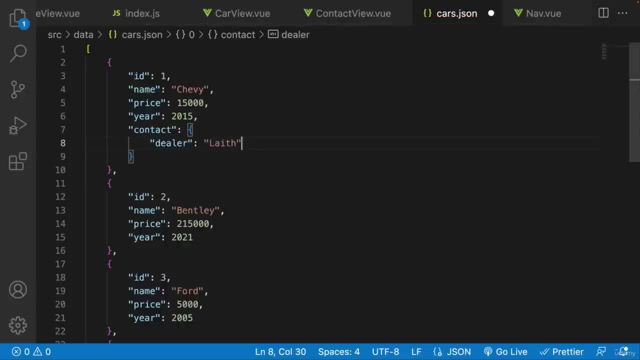 You can give the dealer any name you want. I'll just call it late. 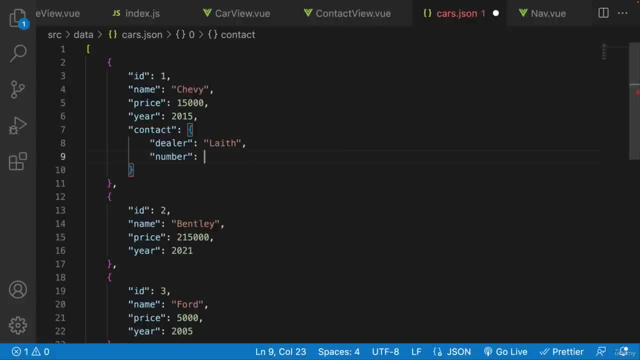 And then over here, we'll give them the number. 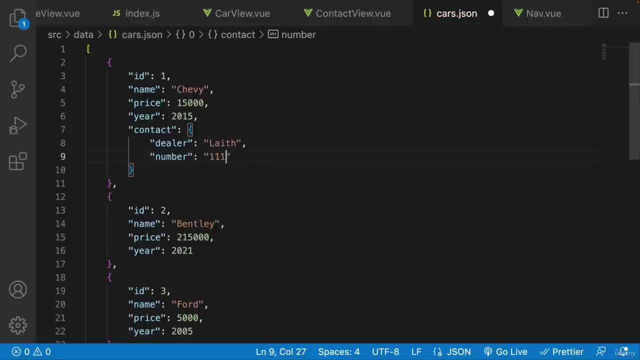 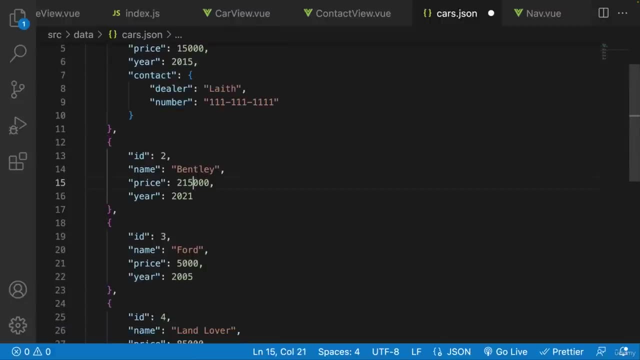 And we'll say the number is going to be one one one dash one one one dash one one one. So let's go ahead and actually do this for every single individual, every single car we have. So let's go here. I'm going to go ahead and paste that in. 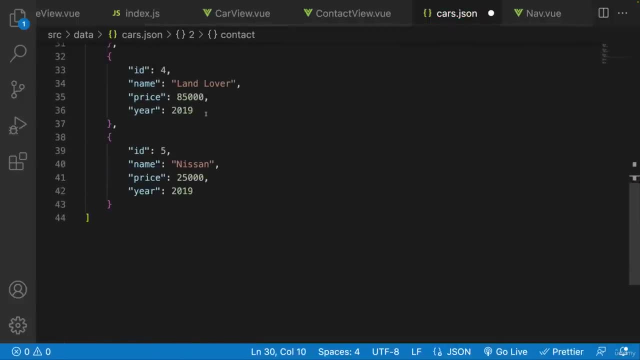 And let's paste that in and paste that in and paste that in as well. Okay. Looking great. So now let's just change the names up. 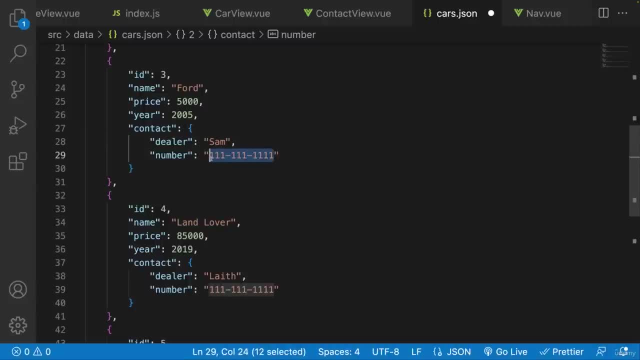 So let's call this person Sam. And we'll change the number to 222-222-222-222. 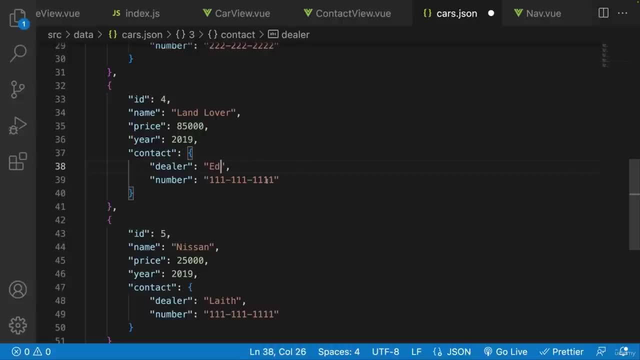 Similarly over here, we'll call this person Ed. 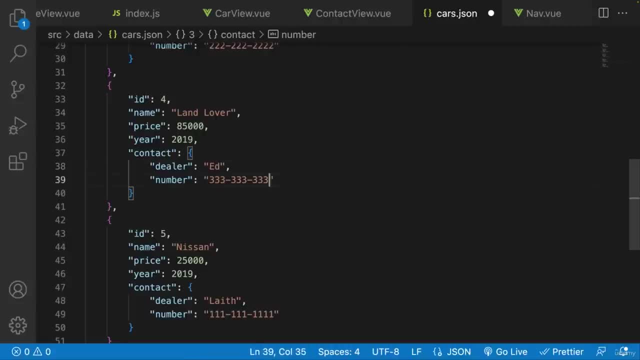 And we'll say 333-333-3333. Okay. I missed the person here. 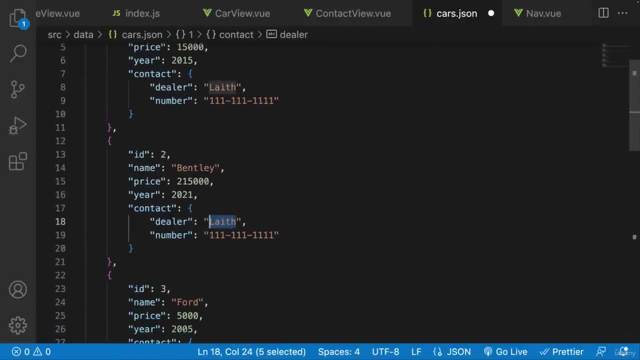 We'll call this person, let's call this person Turner. 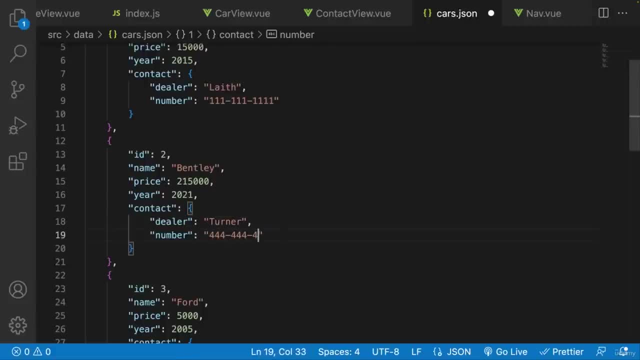 And we'll say this person is 444-444-4444. And lastly, 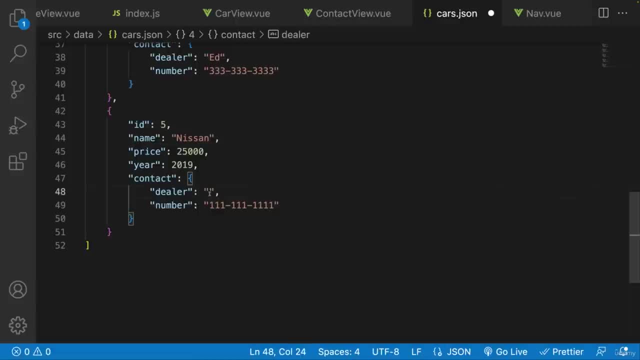 let's go over here and let's say Jess. 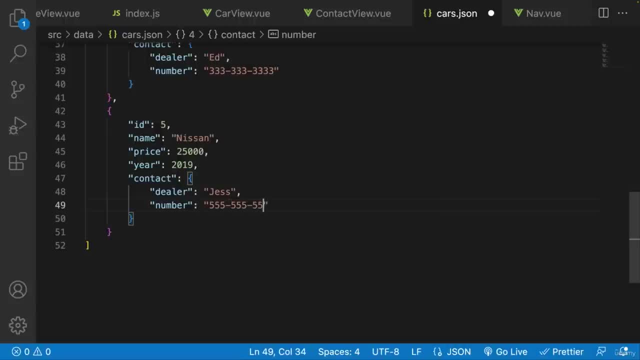 And this is going to be 555-555-555. Okay. Looking great. 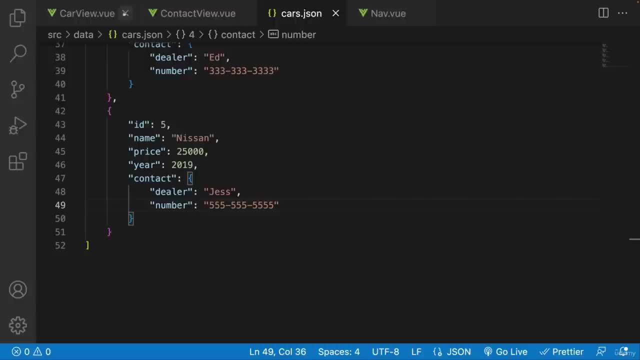 So now what we're going to want to do is let's just close everything up just to make this a little bit cleaner. 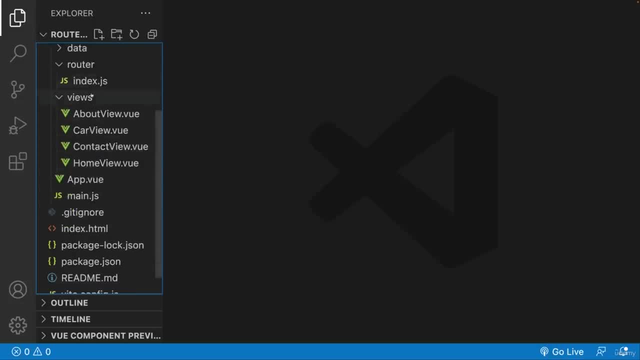 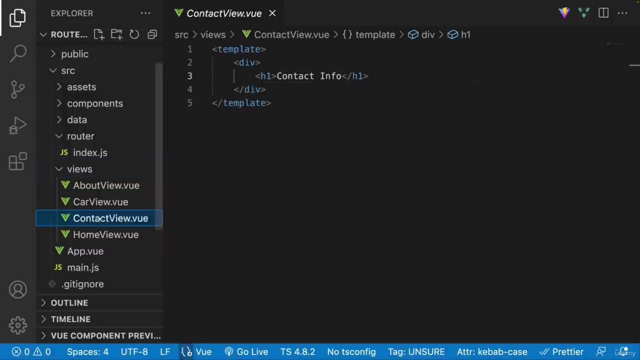 So we're going to go over here to the views. And then within here, we're going to create a, and we're going to call this a contact view. Dot view file. So contact view dot view. And actually I already have a contact view. Guess I was working on this before. I'm just going to go ahead and delete it and then we'll just do it again. 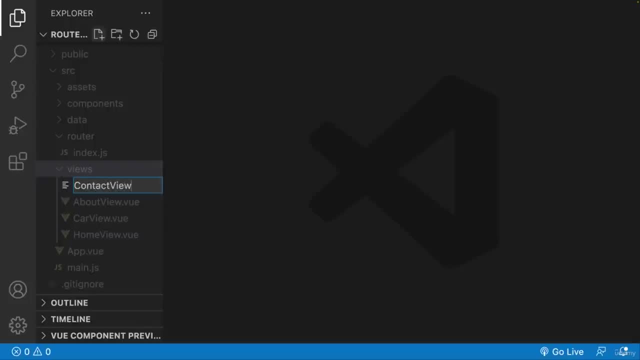 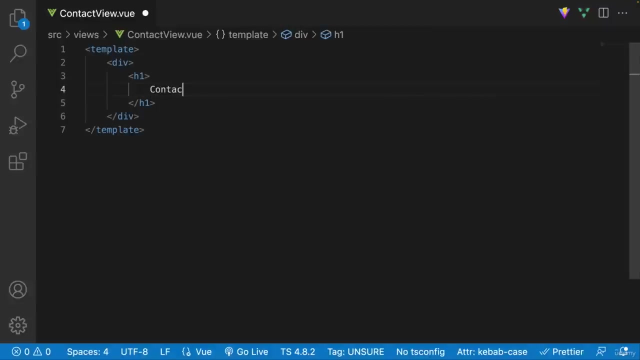 So let's go here and we're going to say contact view dot view. And over here, let's just very simply add a template, an H1 and, or sorry, let's make it a div. Then we're going to have an H1. And then in here, we'll just say contact info. We'll hard code this for now. Okay. 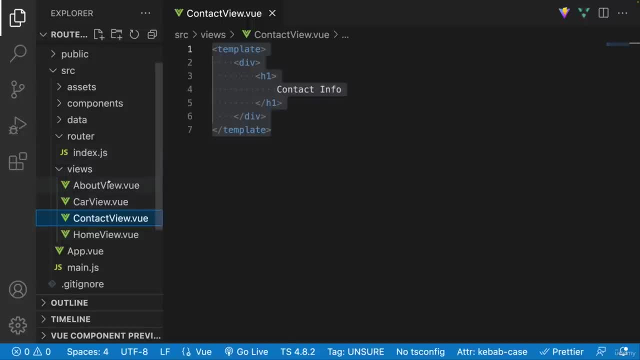 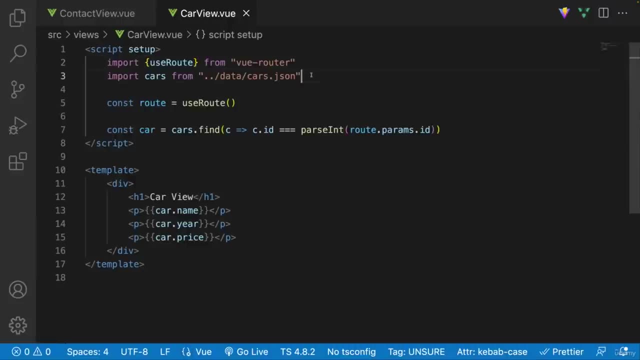 So again, what do I want to do? Well, inside of this right over here. So this car view, eventually what I'm going to want to do, and I'm just going to do this for now, I'm going to import the contact view from contact view. 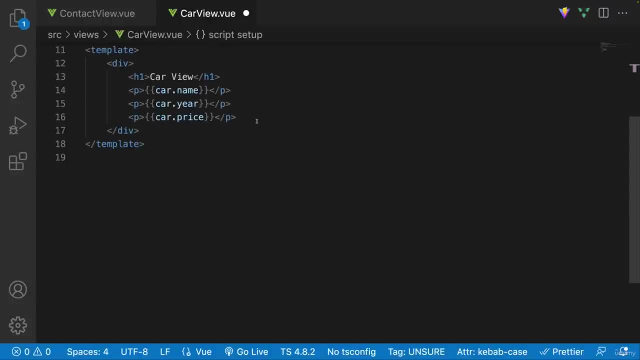 Just, just for now, later on, we're going to have to remove this. 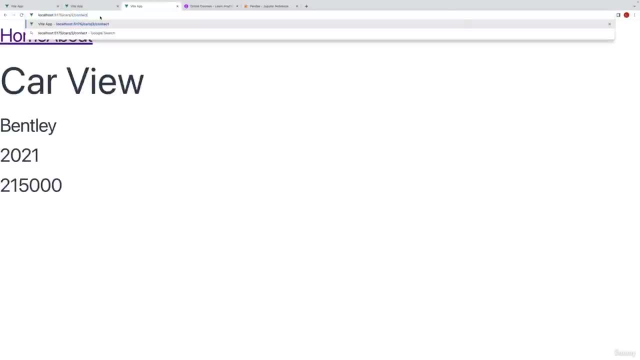 But what I'm going to want is if I go to slash contact, I want to, well, of course, I want to render everything that I have here. 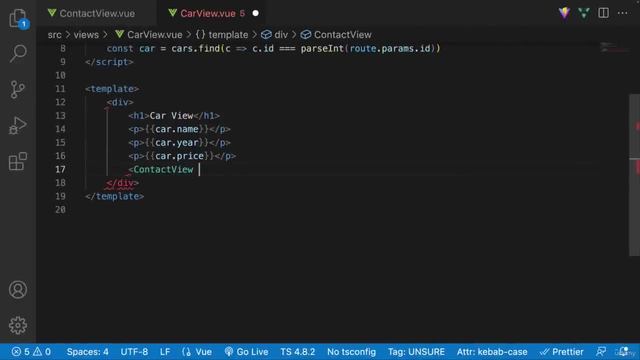 And then I also want to render the contact view component. And I'm probably going to want to pass in some information through props, but we already know how to do that. Okay. So that's looking good. 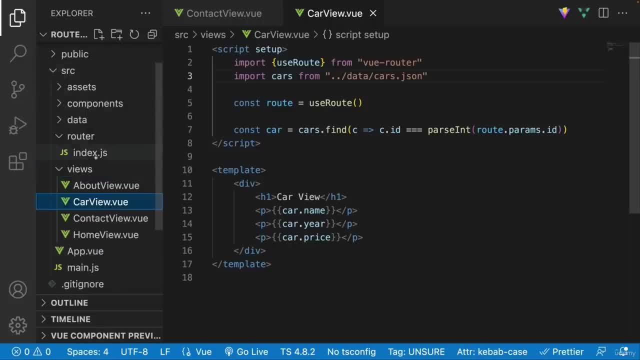 Now, how are we going to do that? Well, we're going to have to define this rule inside of our index dot JS. 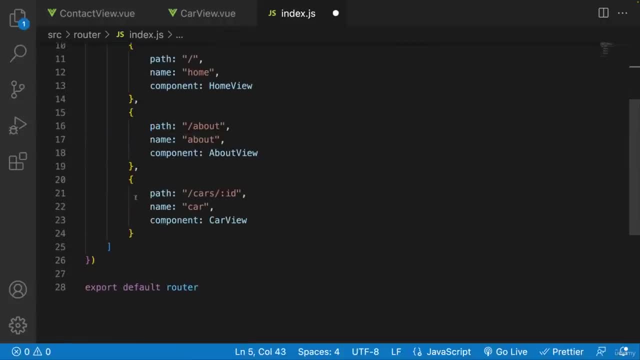 So what we are going to define is right over here inside of this path. We should have a child path, a nested path that is going to go to slash contacts. And we can actually do that by saying comma and then children, because overall, these are going to be children paths to this overall path over here. So this is going to be a, an array and we're going to have, well, different paths inside of this array. And we're going to have the same overall structure. So we're going to say path, and then I'm going to say contact. 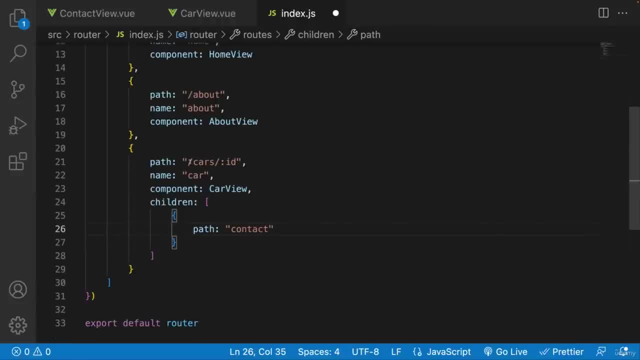 So what's going to happen here is when we go to slash contacts, when we go to slash cars and then slash ID slash contact, then what we're going to do is render the particular component. So we're going to say render, and we want to render the contact view component. 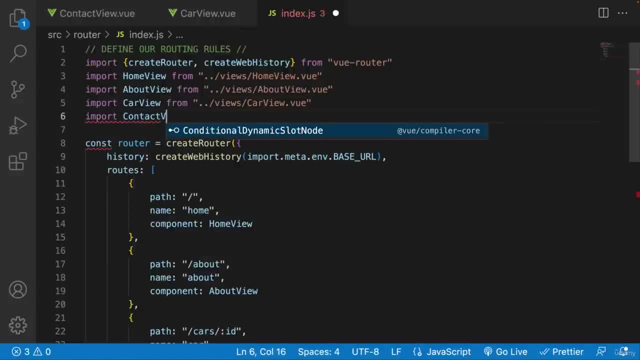 So import contact view, and we're going to go ahead and import that from views slash contact, view dot view. 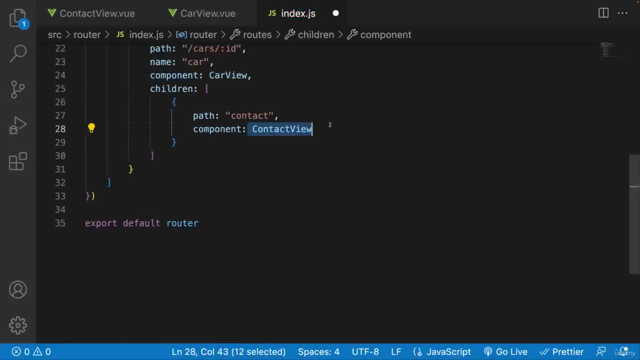 And we're going to go over here and we're going to render this component. So let's just take a look at what's happening right now. 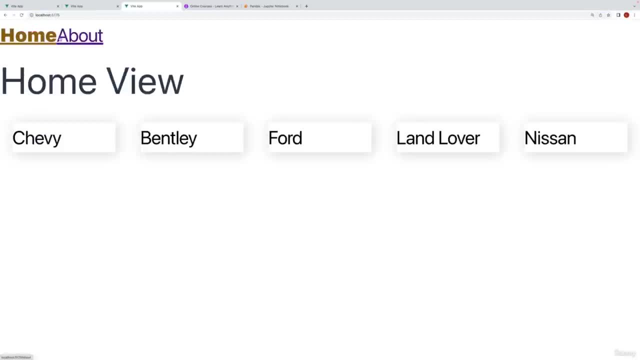 So we're going to go over here and let's go home. Let's pick the Bentley. 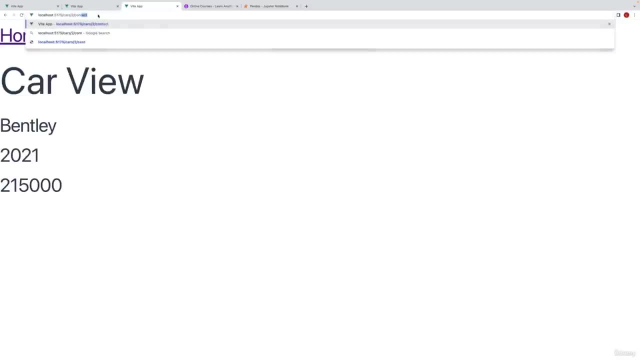 And now what I'm going to do is I'm going to go to slash contact manually. And right now, as you can see, we are only rendering the car view. 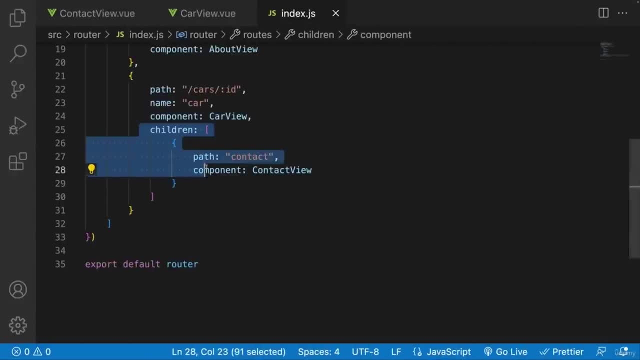 So what eventually ends up happening is because this is nested, this component is going to be rendered within this page right over here. 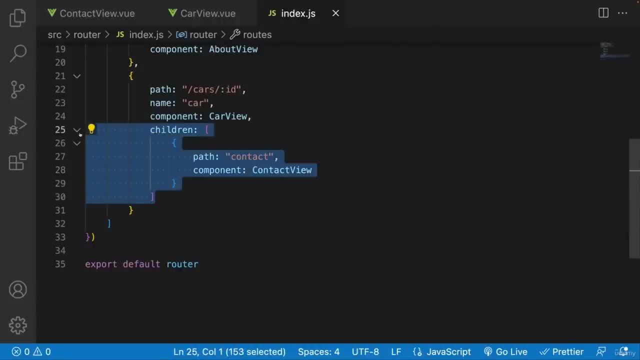 So remember when we actually didn't define this, so let's say, let's comment this out, and we didn't define this, and we went to slash contact, you can see that we actually don't have anything. 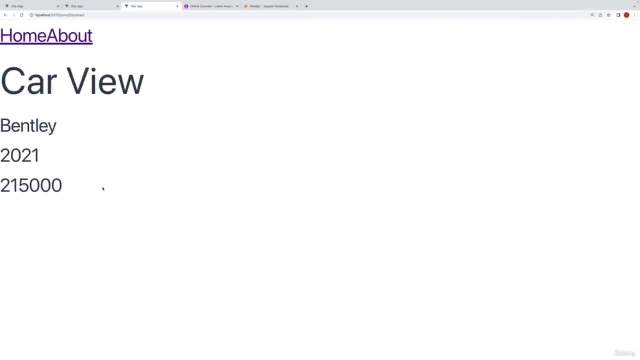 But now because we have defined it, we're going to render the car view, and then we are going to render the contact view. 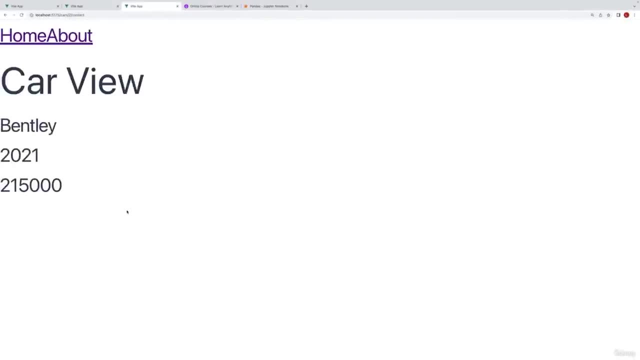 Now, as you can see here, there is no contact view. So you might be wondering where it is. 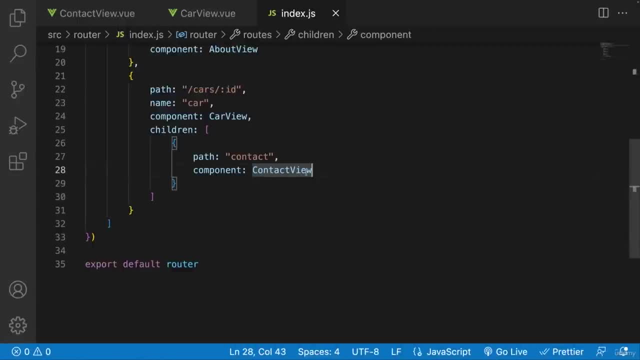 Well, now we have to exactly define where do we want to render this view when we hit this particular route. 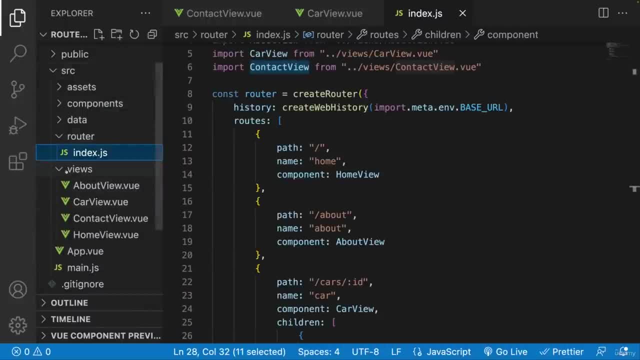 And very similarly, we're going to do this very similarly to the way that we did it with the app.view. So with the router view right over here. 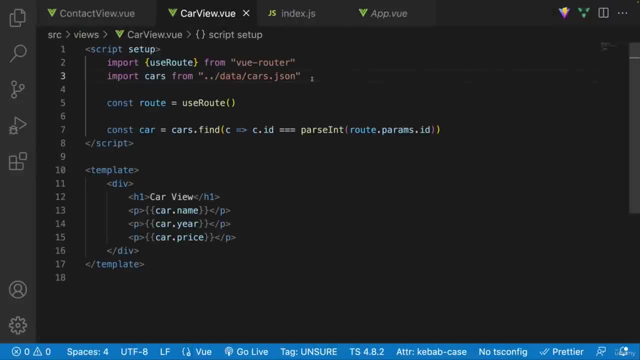 So we're going to have to go to the car view. And then over here, we're going to get the router view. 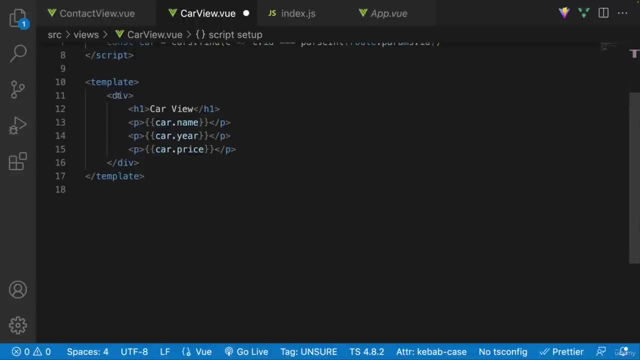 And over here, we are going to go and render the router view. 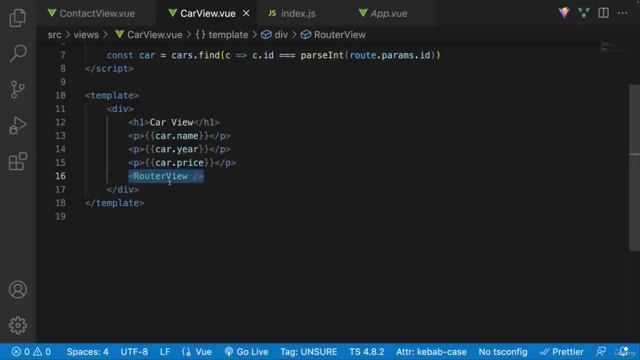 And so what this is going to do, the router view is going to be really smart. It's going to basically tell, oh, this is the view itself. 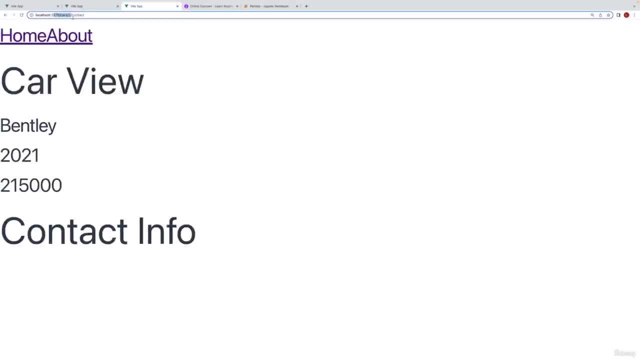 And this view has this path right over here. So I'm going to see if there's any children associated with it. And yes, it does have children associated with it. 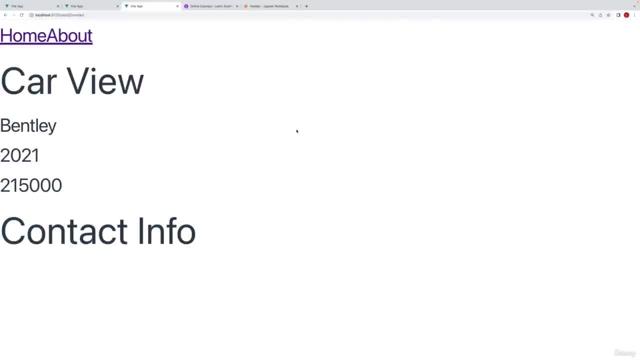 And we are at the path where we do want to render the children. And there we go. 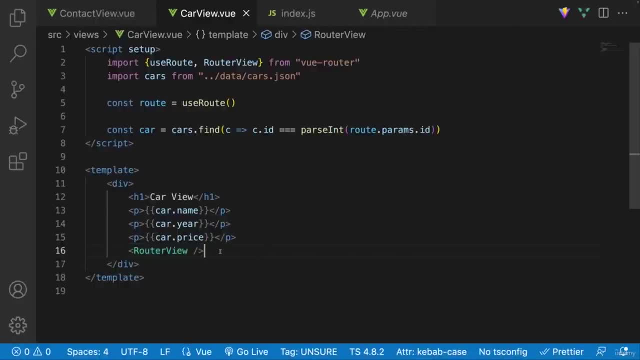 Now you can see that we actually have the contact being rendered over here. So how terrific is that? That's really just some really cool, powerful stuff. 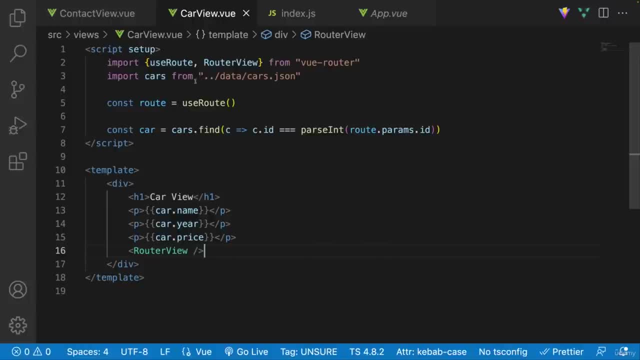 So now let's actually just go ahead and very simply, what we're going to need to do is pass the data to the contact view. 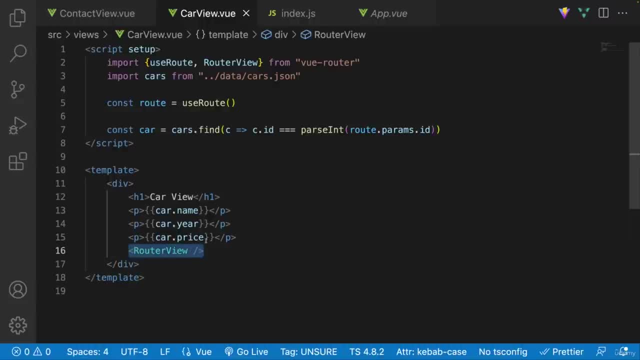 Now, unfortunately, this is not a component, so we can't really pass data that way. 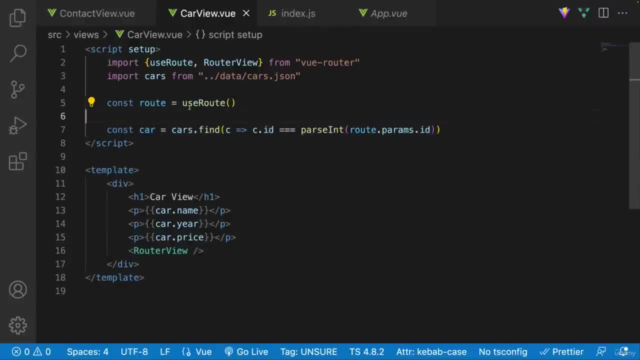 So we're going to have to do kind of something similar to what we've done over here. So we're going to have to do the use route in order to get the ID. 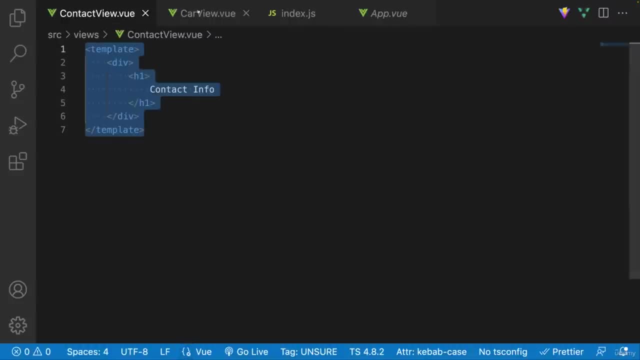 And then what we're going to need to do is find the car and then render the car information. 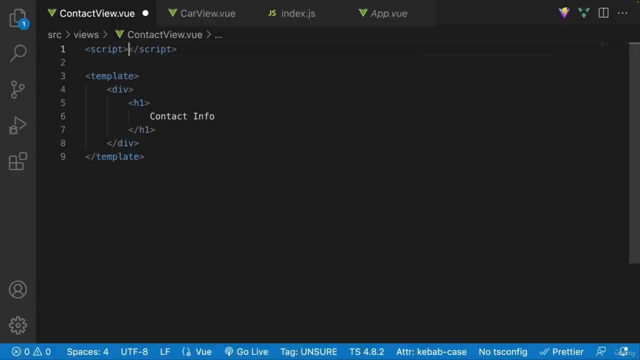 So over here, what we can do is we can say script setup. And over here, let's just do an import. 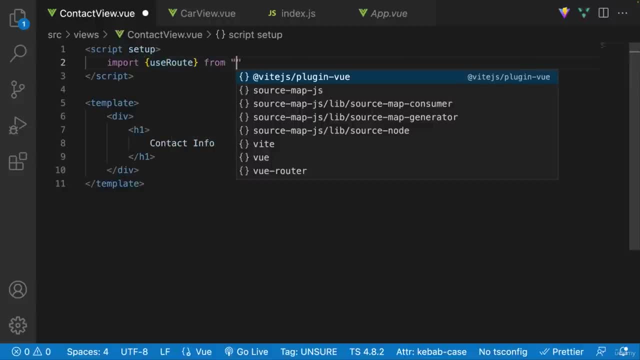 And we're going to use route so we can get information about the route that we're currently on from ViewRouter. 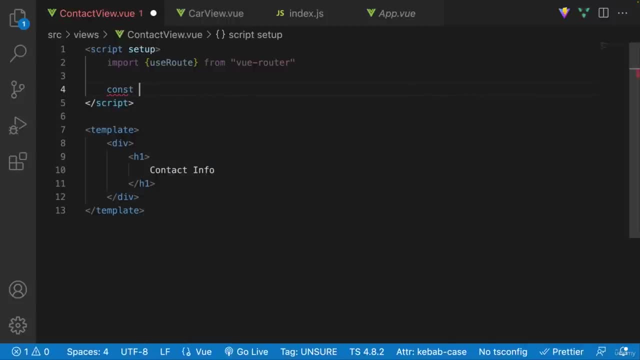 And we're going to say const route is equal to, and we're going to say use route like so. 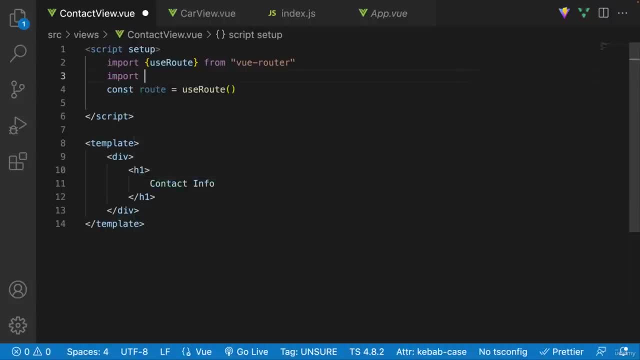 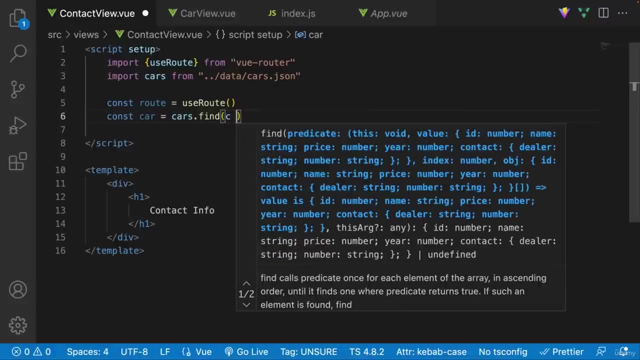 And let us go ahead and import something. So we're going to import the actual cars from the JSON file. So we're going to say from data slash cars.json. And then what we're going to do is, very simply, we're going to do const. And we're going to say car is equal to cars.find. And we're going to go ahead and try to find that car. So we're going to say c, or just maybe, yeah, we'll just say c for now. 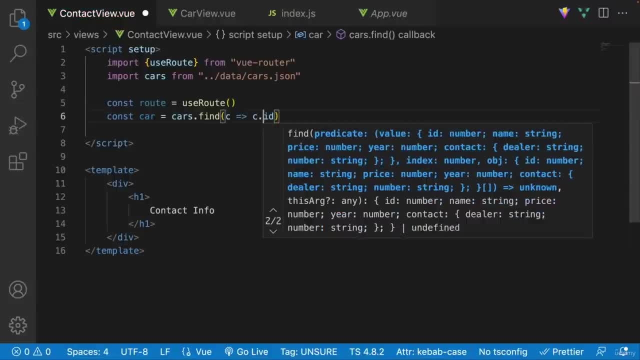 And we'll say c.id is equal to route.param.id. So over here now, we can just start rendering some of the contact information Let's say, p tag over here. We can say car. 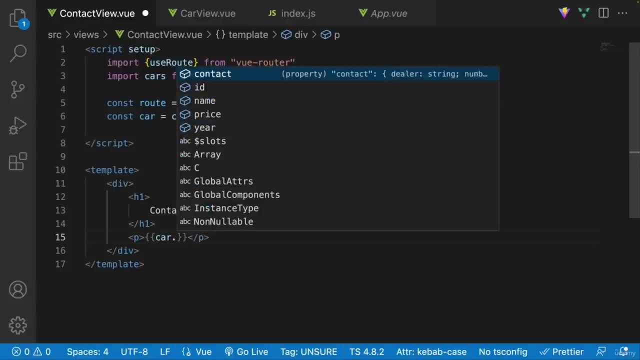 And we can say, let's go, we want contact.dealer. 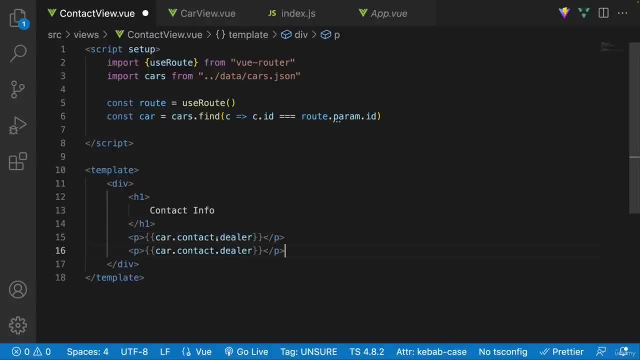 And then over here, we can say car. 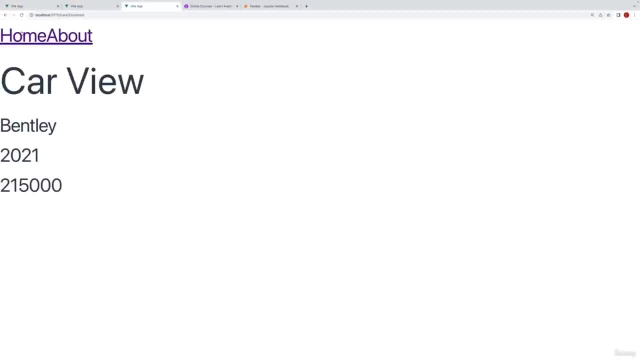 And we can say number. So now, 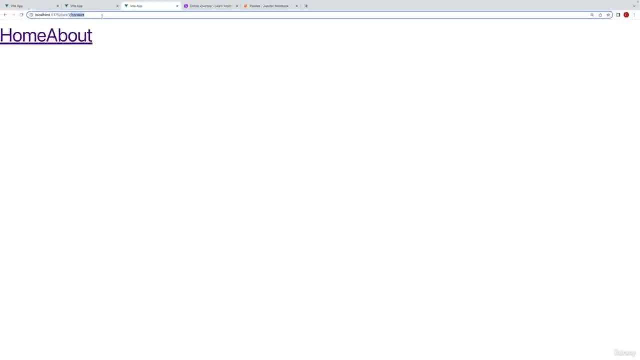 let me just do a quick little refresh. Let's go here. And I'm going to go to, slash, contact. And everything fails. Let's see why that is. 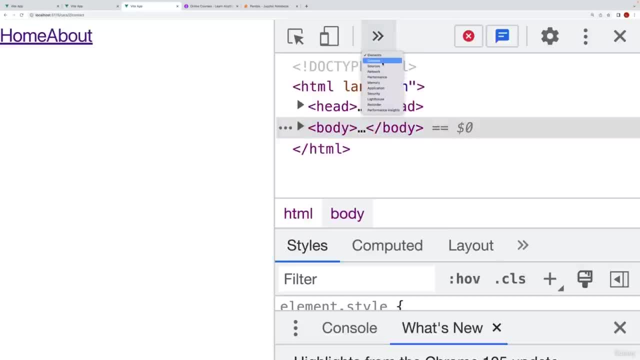 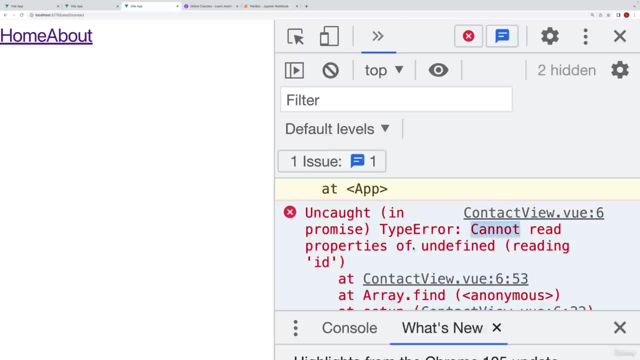 Let's go ahead and inspect our console. Let's see what is erroring out here. So cannot read property of undefined. Not a big deal. Let's see why that is. 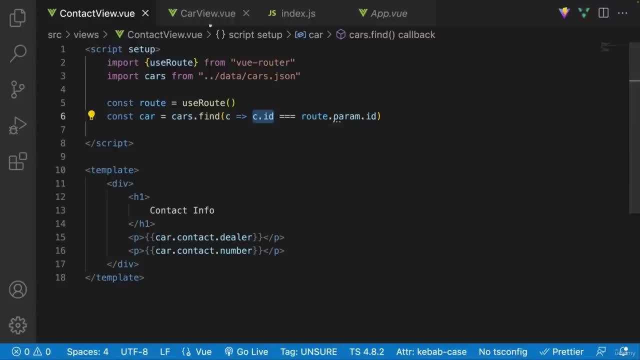 So it's probably saying that c.id is undefined. So let's go to our car view. 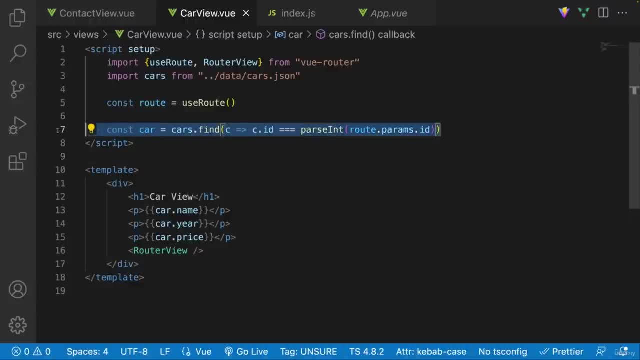 Let's just see how we did it here. Oh, parse int, of course. 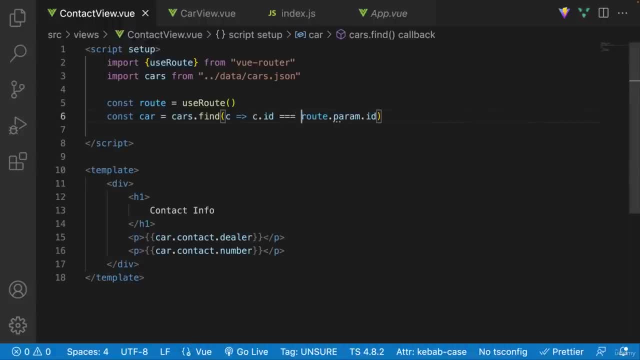 Let's just go ahead and copy this. Because remember, this is actually a perfect example. This right here is a number. But this over here is actually a string. So that's why we're getting that error. 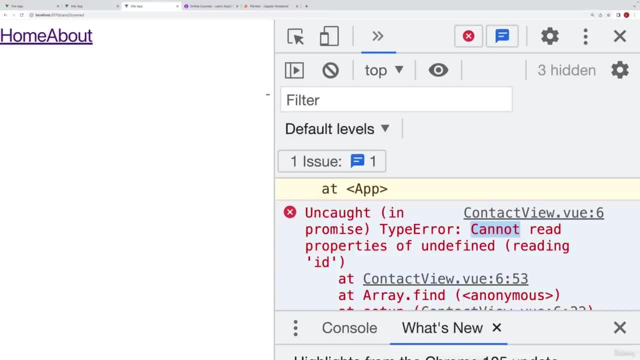 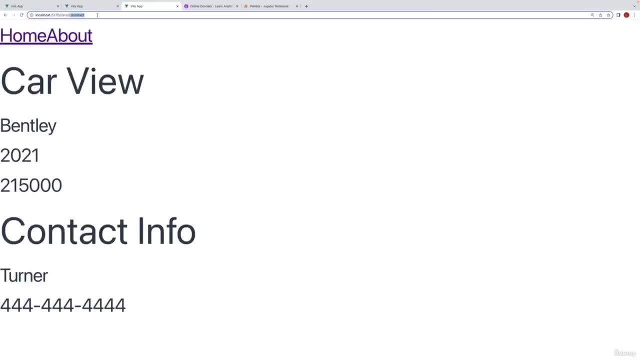 So I'm going to go ahead and now do that that way. And let's just refresh now. And there we go. Now we get our information. How cool is that? So that's pretty much it. 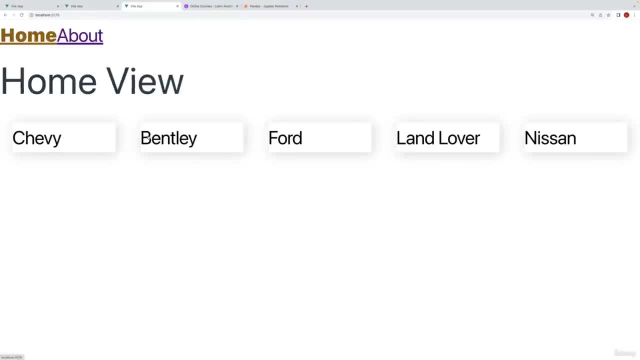 So now we know how to actually implement nested routes. Now, another nice thing that we might want to do is not have them have the ability to go to slash contact by writing it out. 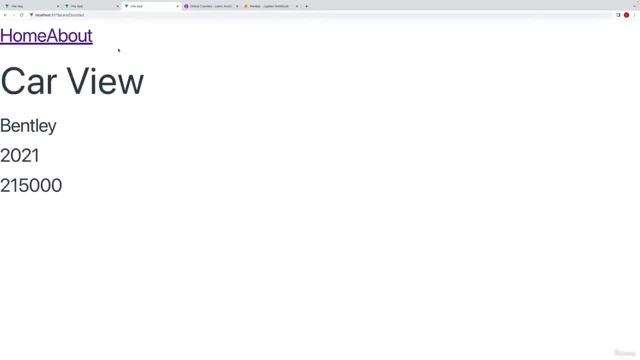 You might want to add maybe some sort of button in here. Now, 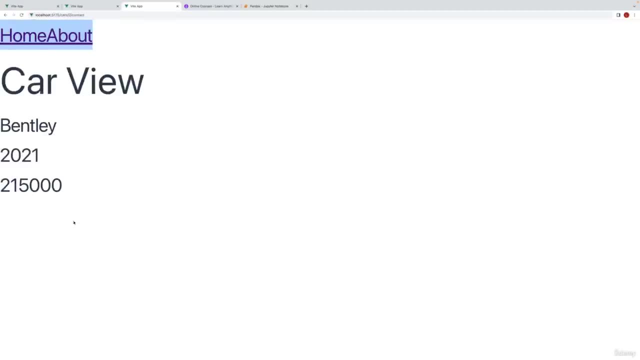 before we have been using router link, but let's say we don't want to use a anchor tag for this particularly. Maybe we want to use a button. 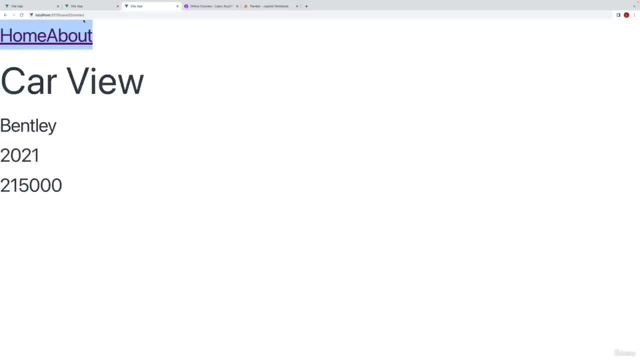 So how are we going to programmatically add this navigation in order for them to go to the specific route that they want? Let's talk about that in the next video. Okay, my good friends. 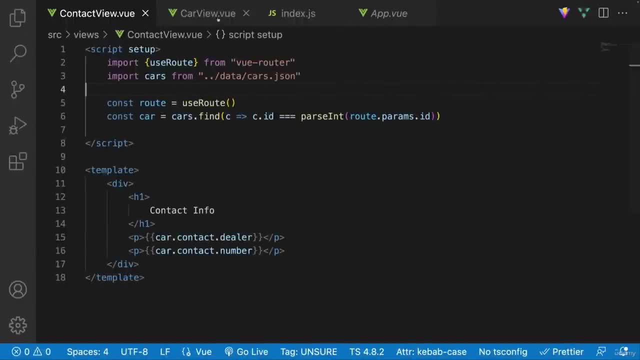 So now we need a way to actually get to the slash contact page from the car view. 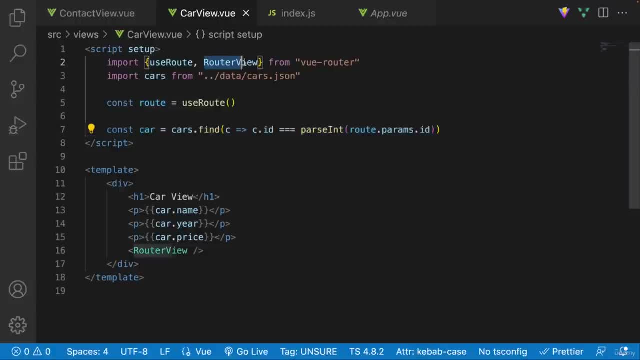 Now, we can do this relatively easily by utilizing a router link, but that will force us to use an anchor tag, which we might not want to use. 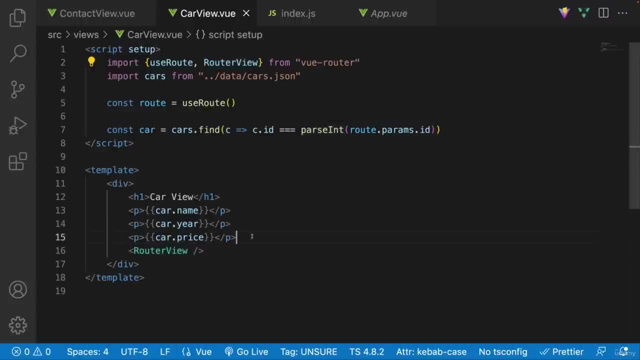 Maybe we want to explicitly utilize a button. So over here, I can say button and I want, you know, click, click me for contact. And once I click this button, 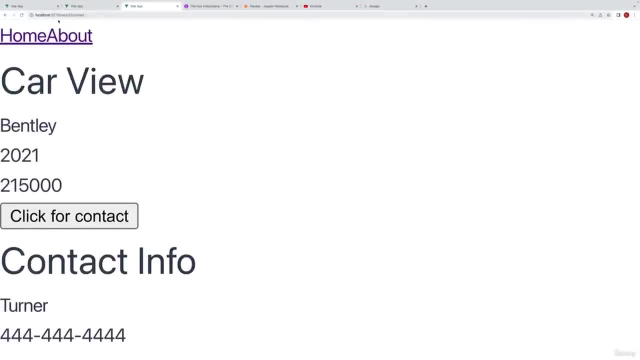 it is going to programmatically going to adjust my route to slash contact. 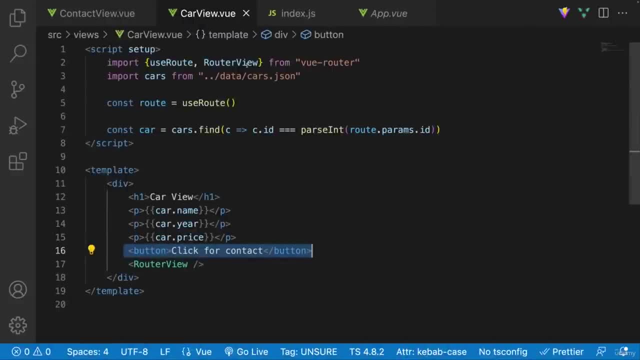 So obviously this isn't going to be possible with the router link components because again, 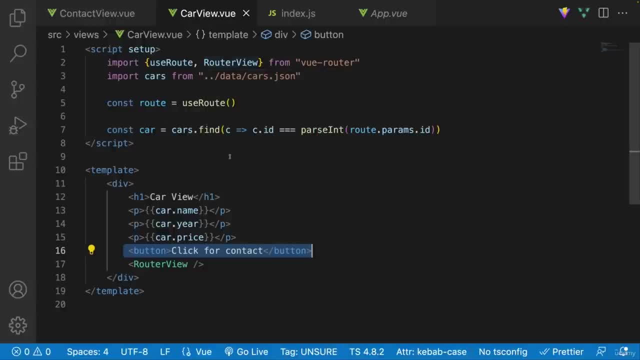 the router link is an anchor tag, but it is very much programmatically possible to adjust the route. 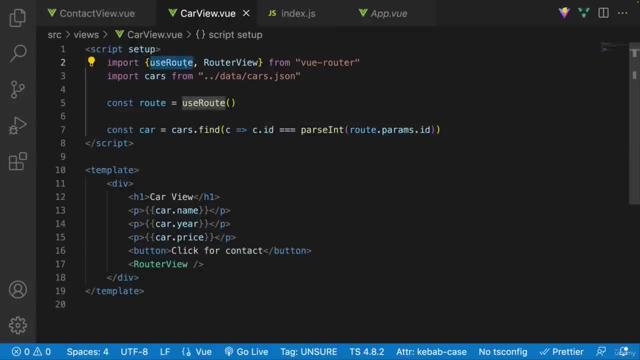 And we can actually do this by using another composable. And this composable is going to be called use router, like so. 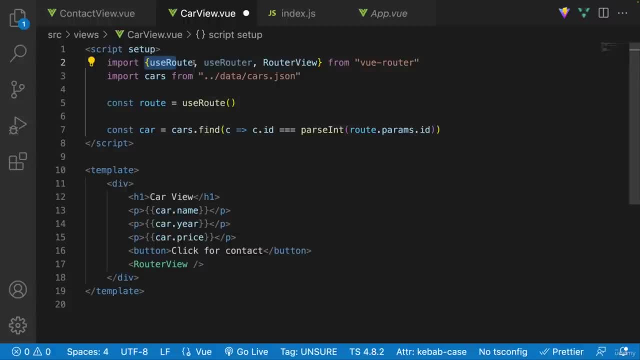 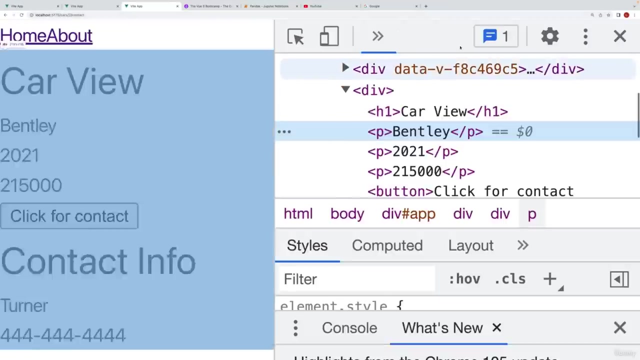 So this might be a little bit confusing. What's the difference between use route and use router? Well, use route is a composable that is going to allow us to extract information about the current path that we're in. So for example, we're able to extract the params. So these query params, and if I were to go ahead and console dot log the route, you can see all the different things that we can utilize to extract information about this path. So let's go over here to the console. And if I were to, I guess we can't really see much here. 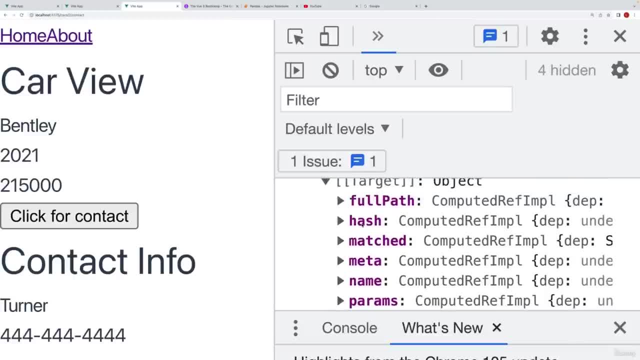 Oh, there we go. We can see the full path. That's something that we can get. We can get the hash. We can get the match. We can get the name of it. 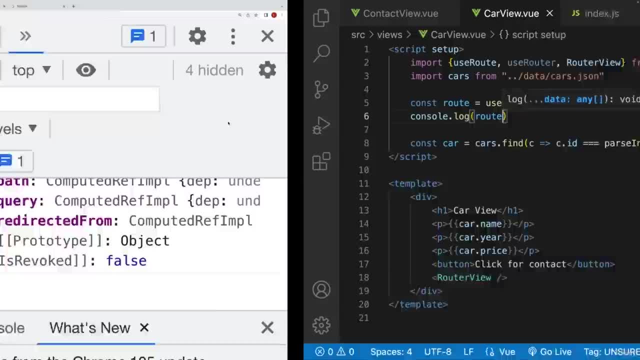 You can get the queries. We can get information about the path. However, 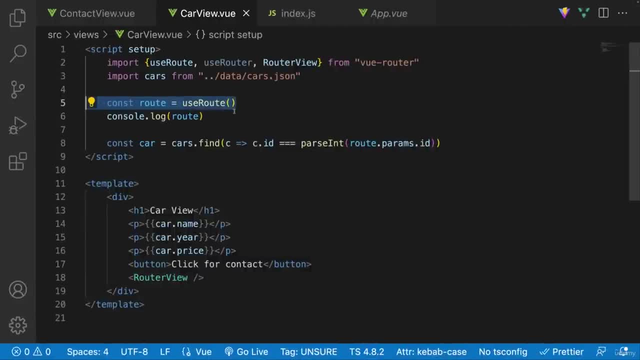 something that we cannot do with the use route composable is to adjust our path. So do some modifications on our path. And this is where we're going to need to utilize the use router. 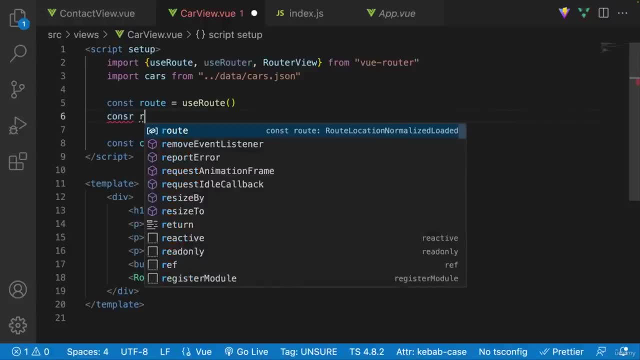 So over here, if I were to go and say const router, router, I'm going to say use router like so. 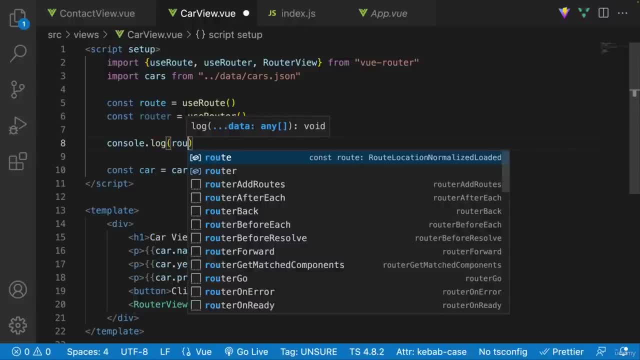 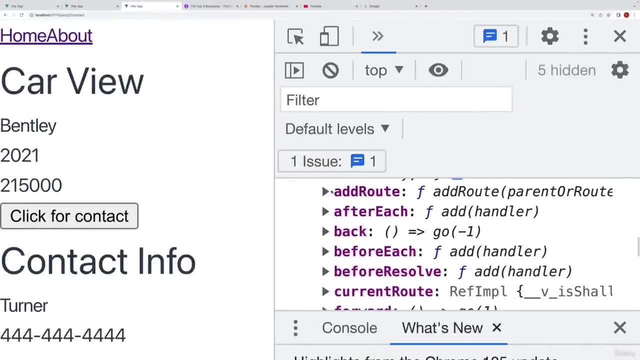 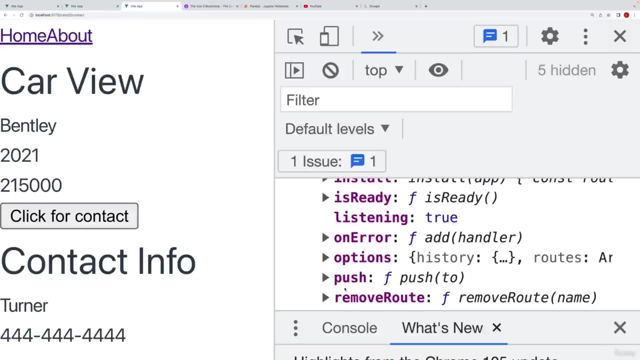 I'm going to go ahead and invoke it. And I'm going to go ahead and console dot log the router. And now let's take a look at all of the other methods that we can utilize within the router. So you can see here, these are going to be methods that we can utilize to actually manipulate and change the path, like add routes. We can go back if we want. We can go forward if we want. We can push if we want. 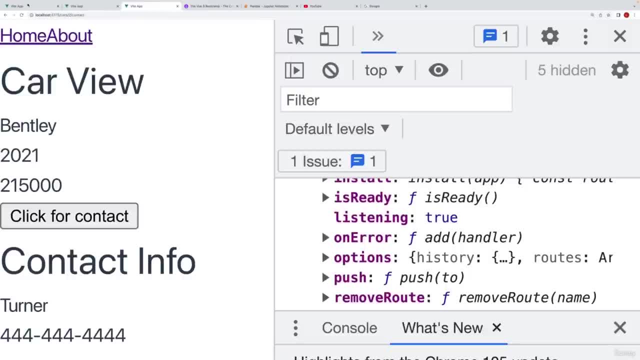 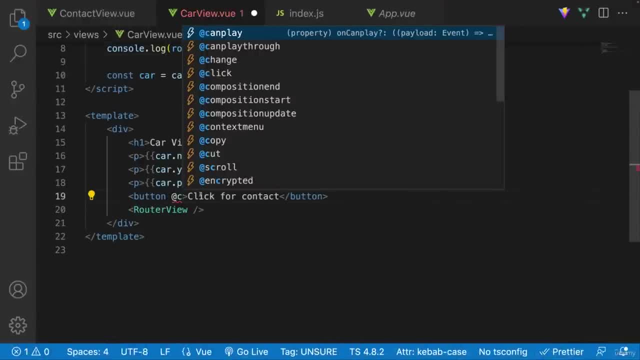 And that's exactly what we're going to do in order to push a certain path to this URL. Let's actually just go ahead and do that. So over here, when I do an at click, what I want to do is I want to do a router. So router dot push. And I'm going to push the path here. That's the path that I want to go to. So it's going to be slash cars and then slash that particular car's ID. 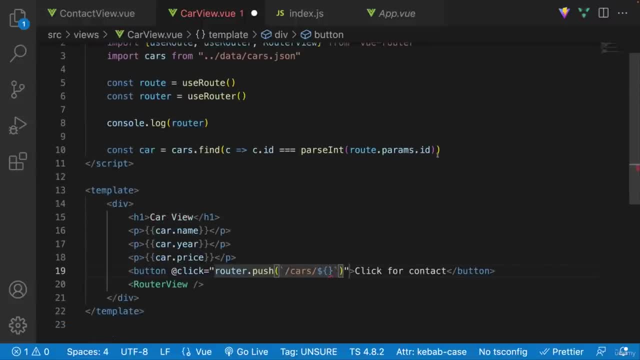 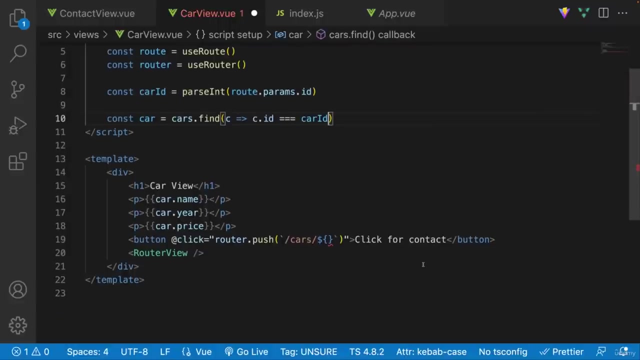 So let's go over here and we're going to get that from right over here. Let's actually store this as a variable. So I'm going to say const. And I'm going to say, let's say this is going to be ID or car ID. We're going to store that as a variable like so. So we can utilize it over here, as well as over here. And then we're going to say slash contact. 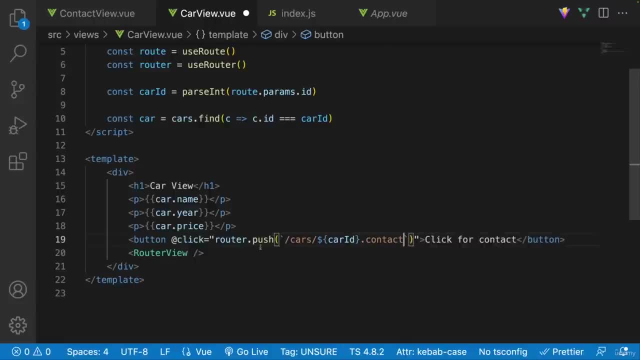 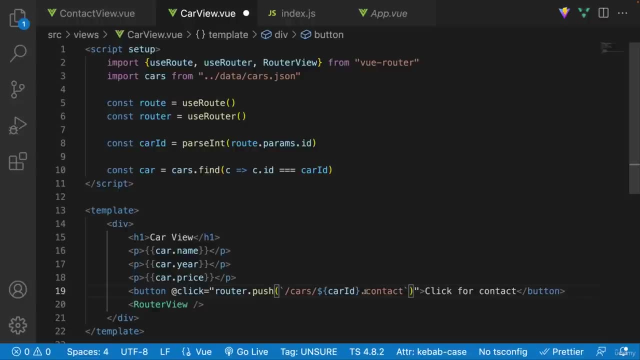 And this is how we're going to programmatically do this. Now we can actually, of course, add this as a function within over here. And maybe with certain conditions, we can adjust it or not. But this is, in essence, how we're going to programmatically change the thing. 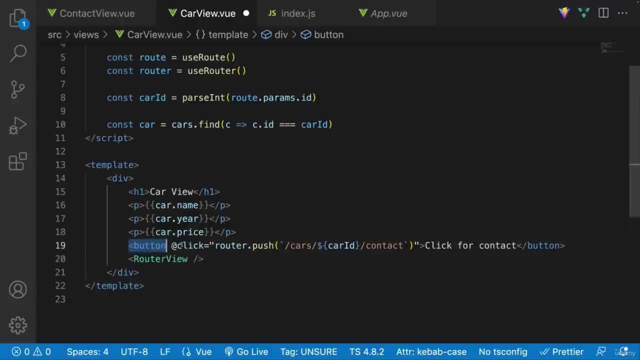 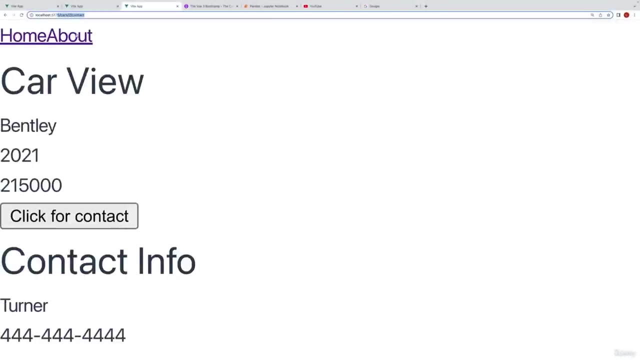 And of course, we can always do this with any sort of DOM element. It could be a div. It could be a header. It could be whatever it is that we want. It doesn't have to be an anchor tag. So I'm going to go ahead and save this. And that's pretty much it. So let's go over here. Let's go to about. Let's go to home. Let's go to Bentley. 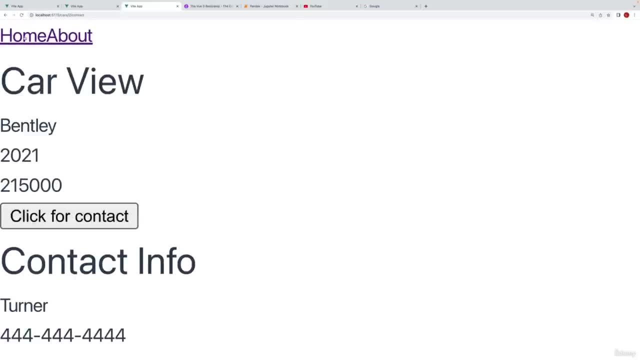 Click for contact. There we go. Now we got the contact information. 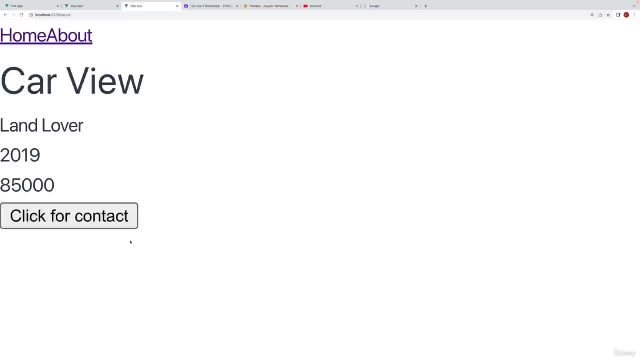 So now you can see how we can actually programmatically adjust things. How terrific is that? 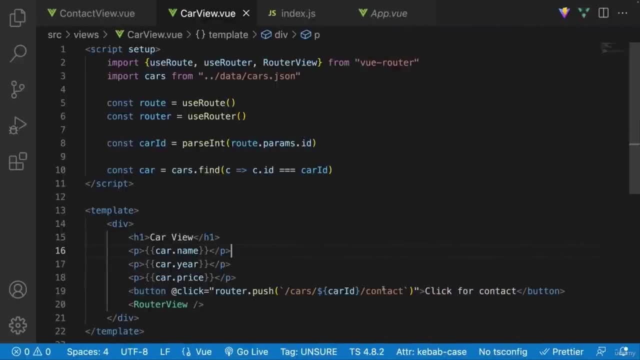 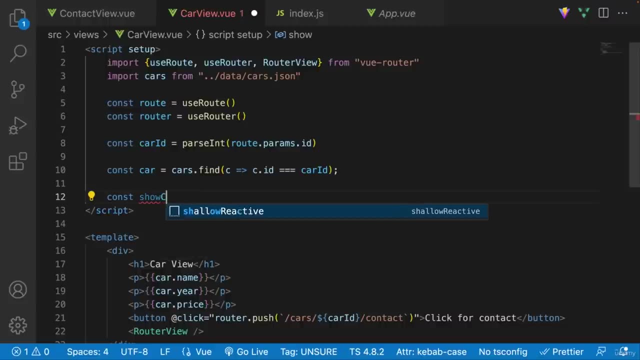 Now one thing that we can do if we want, and just to show you the powers of programmatically doing this, is we can create a function so I can say function and I'm going to say show contact. 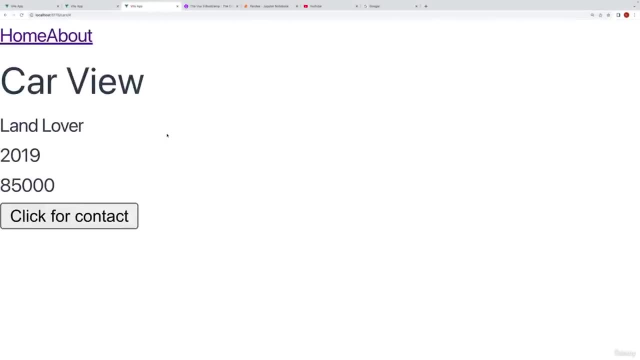 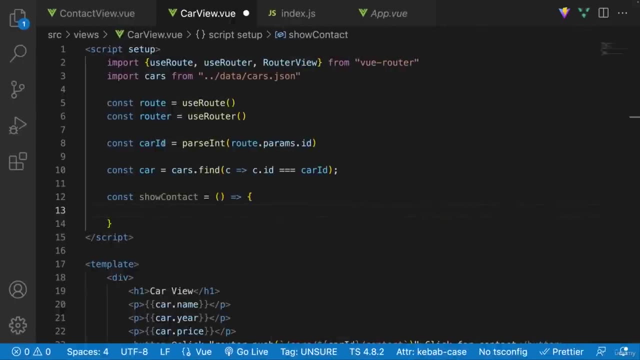 And maybe we do not want to show the contact for certain cars for some reason. Maybe if it's this Land Rover, we do not want to show the contacts for this particular car. 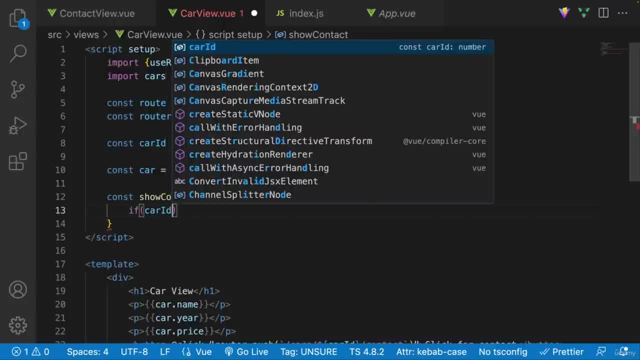 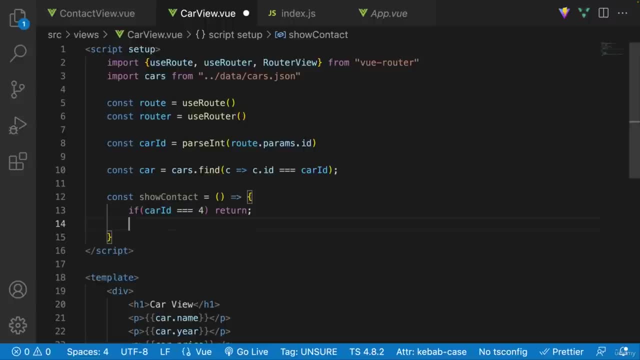 So maybe I can say here if car ID is equal to four. So if the car ID is equal to four, we're just going to return early. And then if it's not equal to four, then we want to execute this logic. 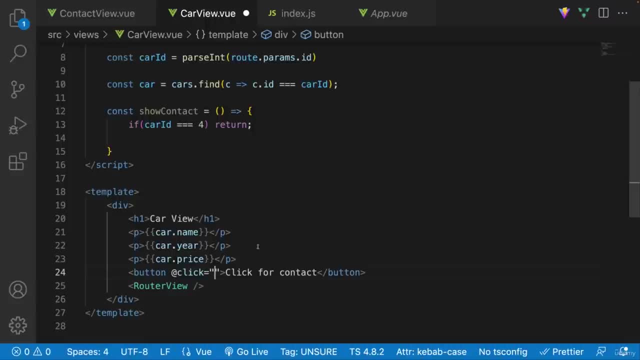 So now we can actually conditionally route users using this programmatic stuff. 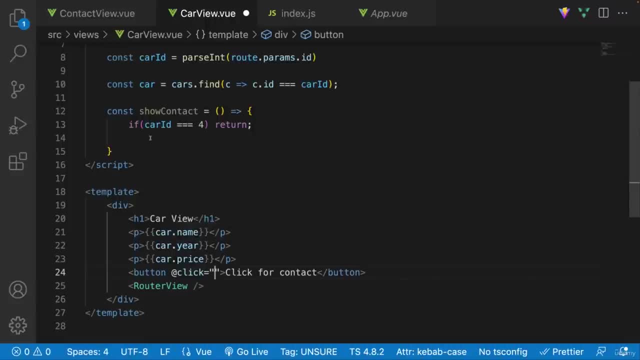 Whereas with the router link, we couldn't do that programmatic kind of stuff. 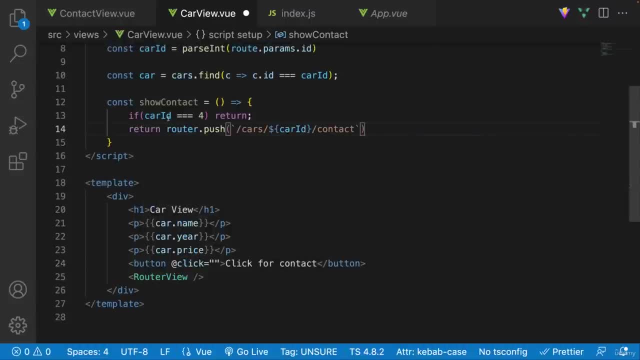 So over here, we're going to say instead return. And then we can say router.push. And then that particular path. 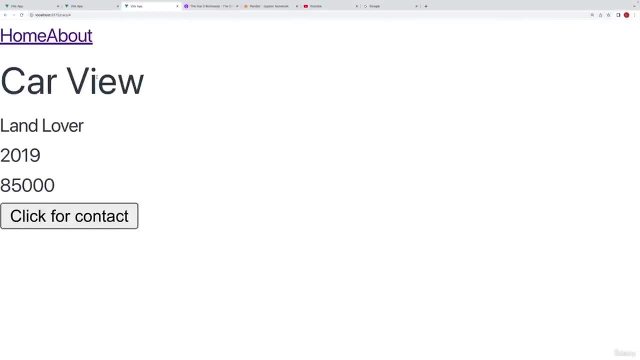 And I'm going to go ahead and just show contact. So now let's just go home. Let's go to Chevy. Click on this. 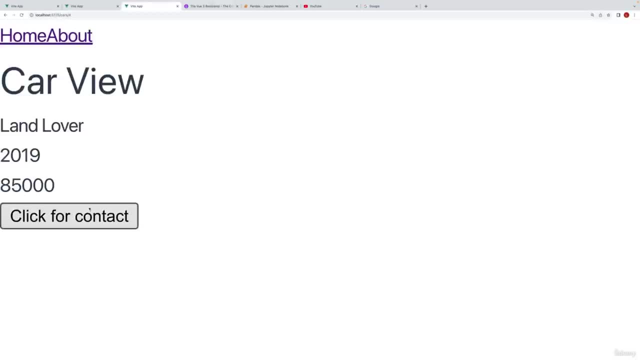 Okay, this is great. And let's say for some reason we do not want to show the contact. 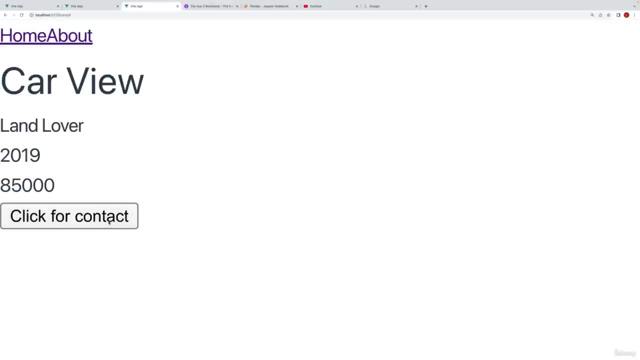 We probably shouldn't even show the button. But now when we click this button, you can see it doesn't work. 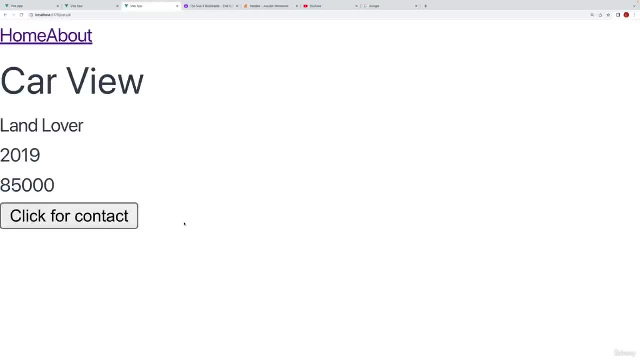 So you can see that there are definitely going to be some use cases where we might want to run some logic. And if some sort of condition occurs, we want to navigate them to a different page. 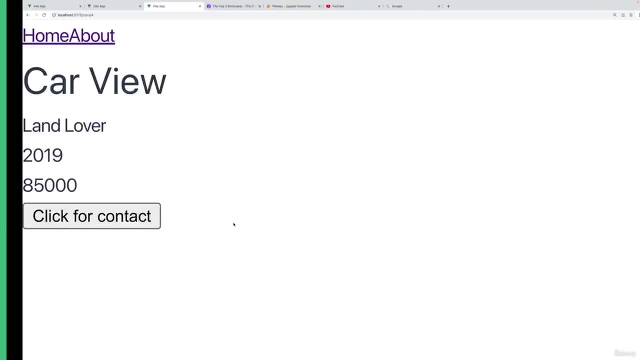 And again, we cannot do that with the router link. We're going to have to do that with the use router composable. 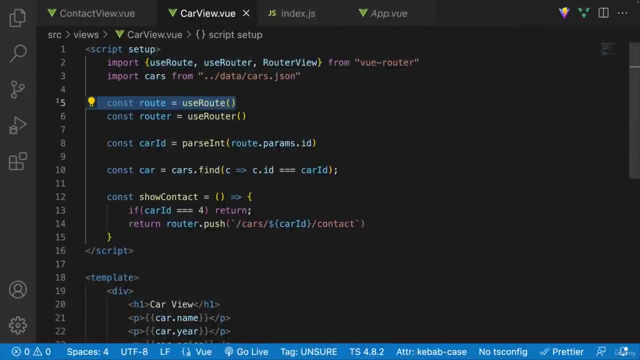 So as a quick summary, use route is going to get information about our path. Use router is going to kind of mutate and adjust our path the way that we want it to. 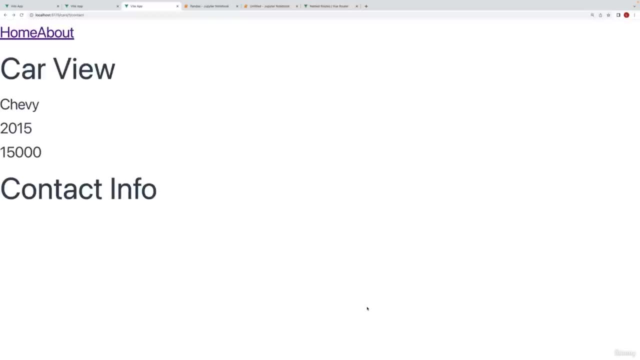 All right, my good friends, the next thing that I want to discuss 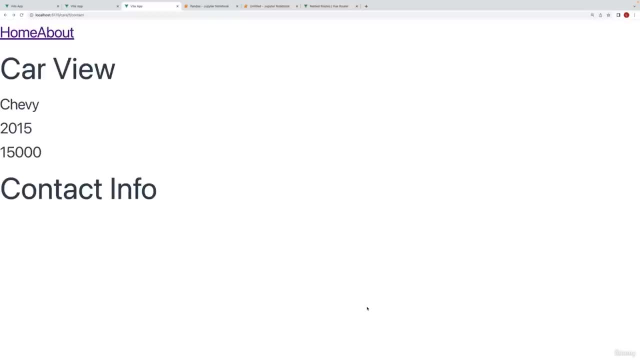 are times where a user searches for a particular page that doesn't really exist. 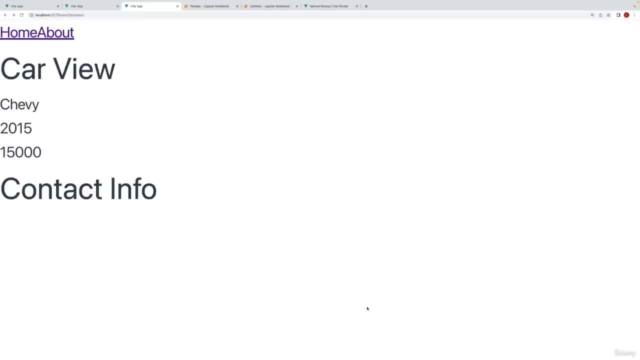 And at least in our application, we have two different scenarios that could exist. 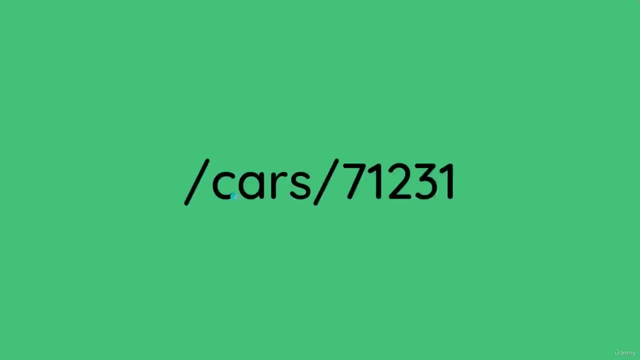 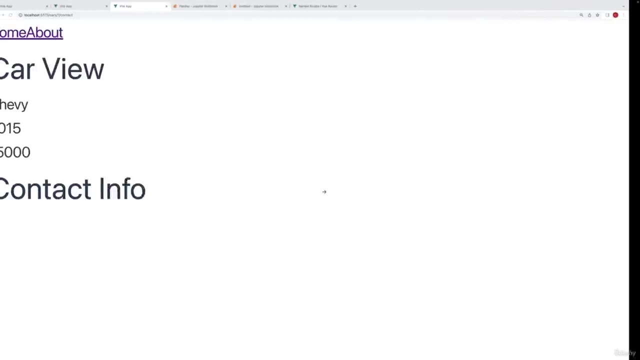 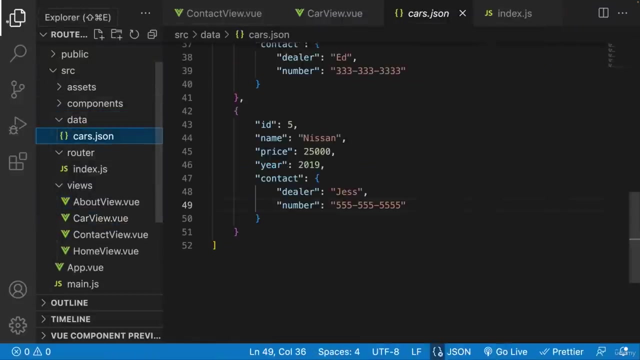 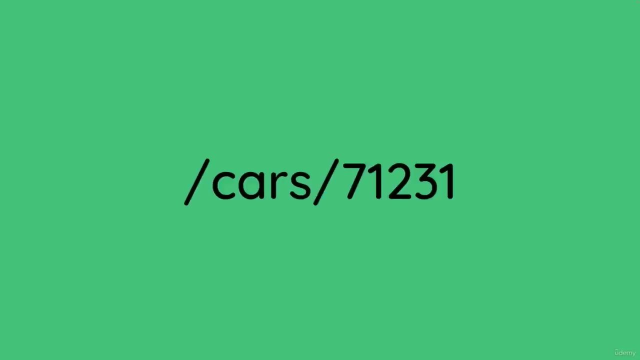 So the first scenario is that a user tries to search for a car using a car ID that doesn't exist inside of our data. Now, typically, of course, this data would probably come from a database. But right now, our data is coming from this JSON file. And we only have, well, cars from ID of 1 to ID of 5. We most definitely do not have a car with an ID of 71,231. 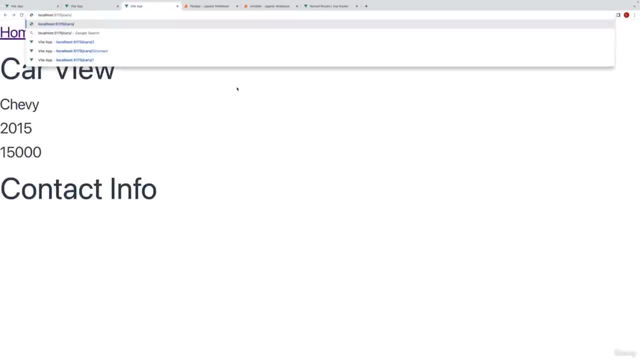 Now, if I actually went ahead and tried to fetch this, an error is going to occur. 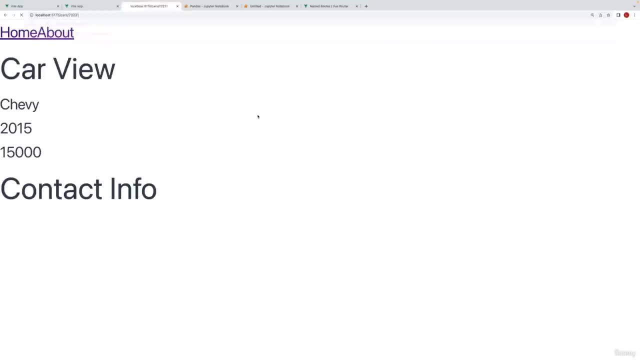 So I'm going to go ahead and say 7,000. I'll just say whatever, anything. 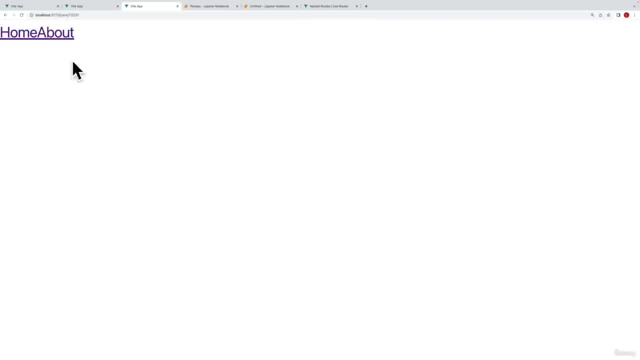 And as soon as I do this, you can see that nothing is being presented, which kind of makes sense. 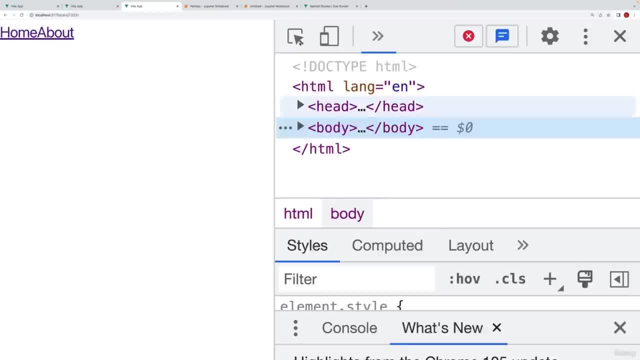 But really what's happening is we're getting an error inside of our browser, which isn't a good thing. 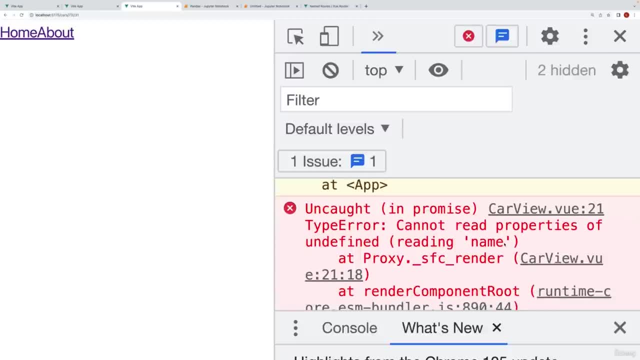 So you can see that the error is, hey, we're trying to read the name of something that is undefined. 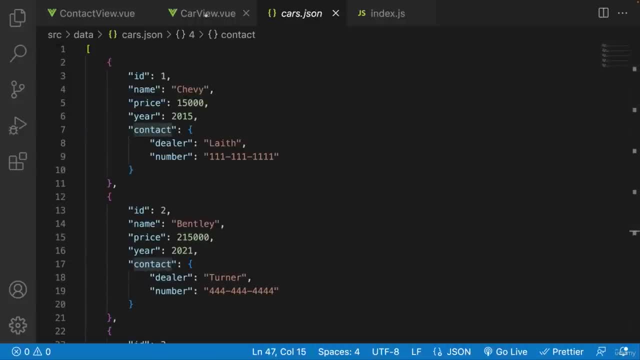 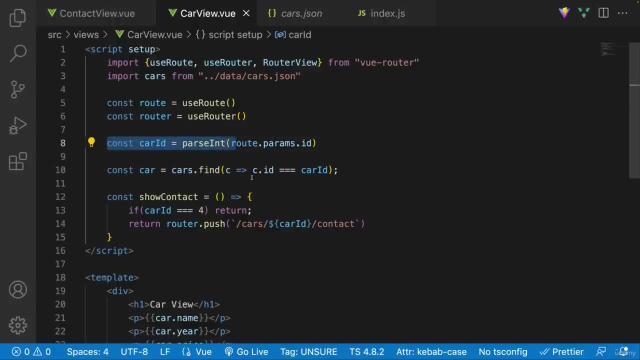 Let me show you exactly why that's happening. Let's go over here to our car view. And right here in our car, what we're doing is, well, we are fetching the car that has the particular ID that is in the route.params.id. Now, if it can't find that car, this isn't going to be an object. 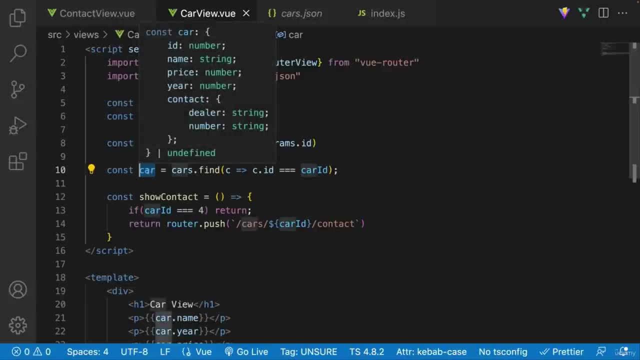 Instead, this is going to be undefined. And actually, if I hover over it, you can see the type of it. So it's either going to be an object with an ID, name, price, blah, blah, blah, or it's going to be completely undefined. 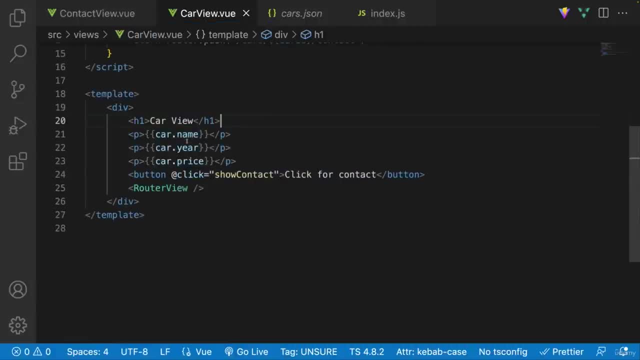 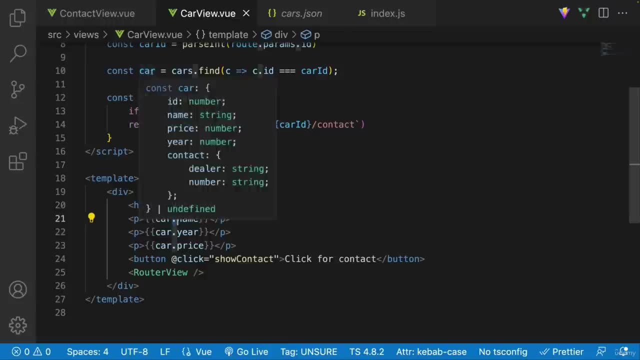 And then right over here, what we're trying to do is, well, we're trying to access different properties of this car. Now, if this was an actual object with this data, that is terrific. 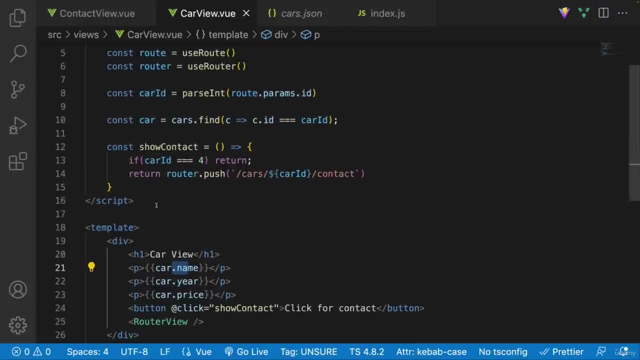 We can access this data. We can access the name. We can access the year. We can access the price. A-OK. 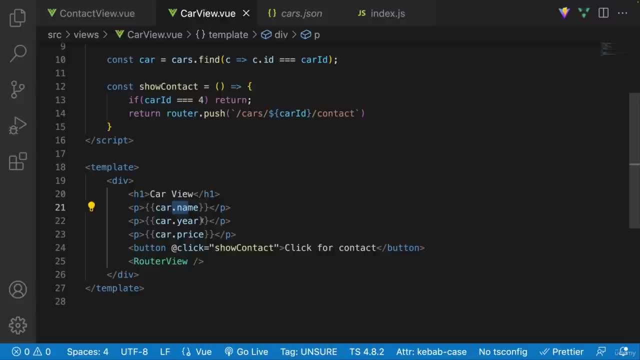 However, of course, if this is undefined, we can't do this. We can't get properties off of undefined. And that's exactly the error that we're getting. 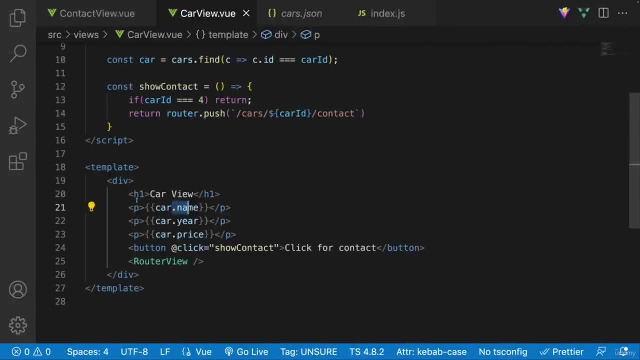 So to kind of fix this, we can actually very simply use a vif velse directive. 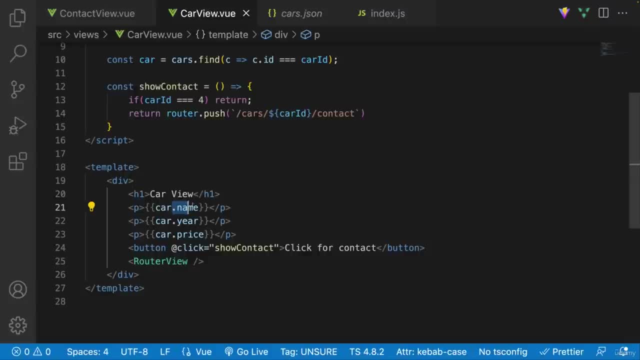 Now, we've seen the vif directive. But now let me go ahead and actually introduce the velse directive as well. 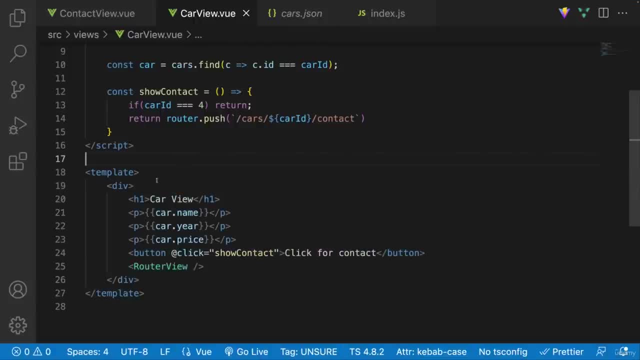 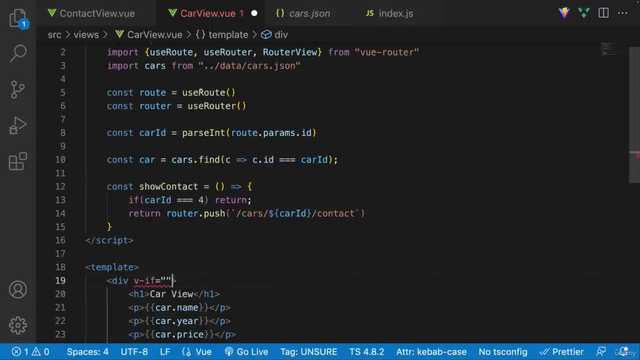 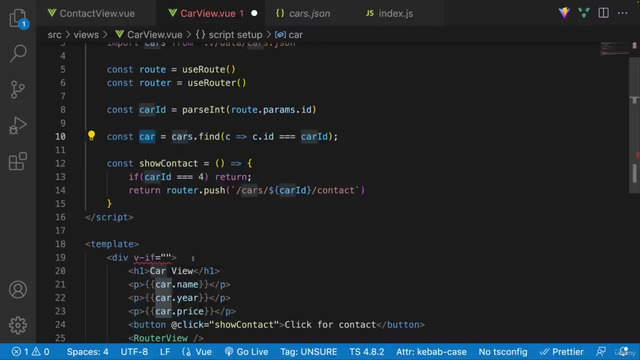 So what we can do here is we can go ahead and actually render. So we can say vif. And we can render this div as well as the content below it only if, only if, well, we actually have a car, the object. So we can say here vif car. 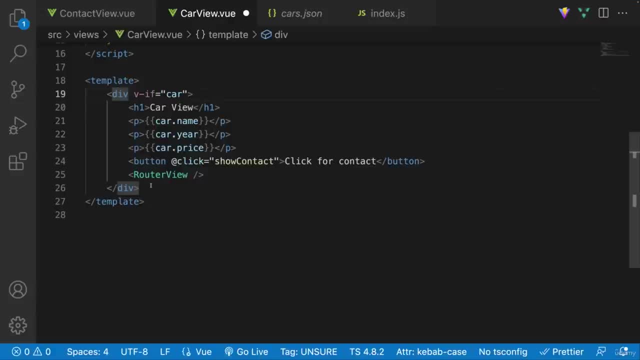 Then we want to render this. Now, in case that this actually, this condition doesn't pass, 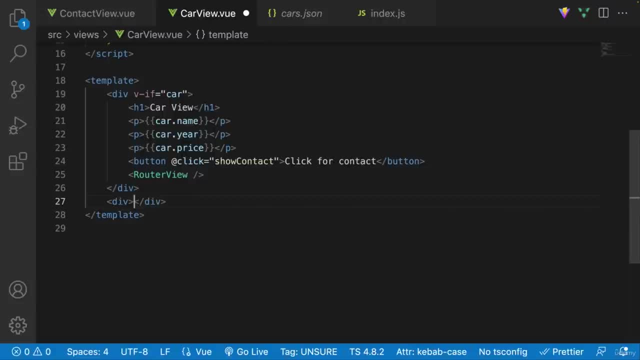 then we also do want to render some HTML. Let's say we want to render this div right over here. 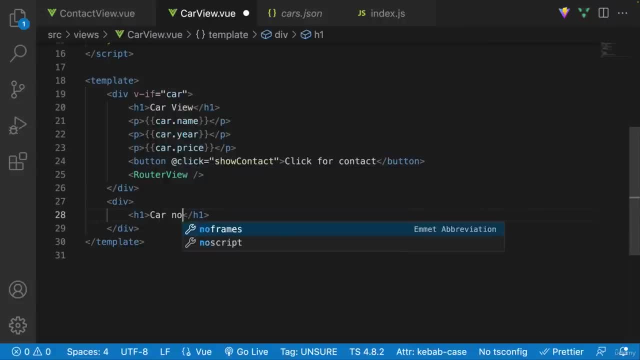 But then we want to say something like car not found so that the user can actually know what the error is. 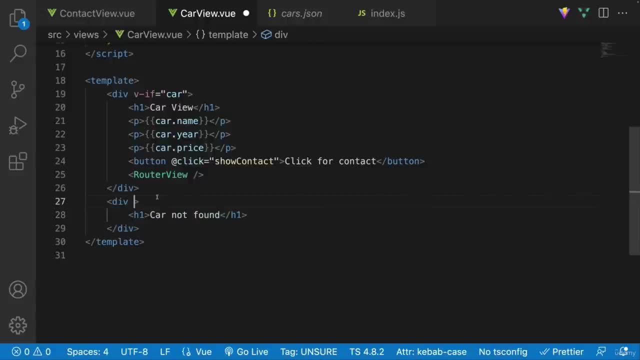 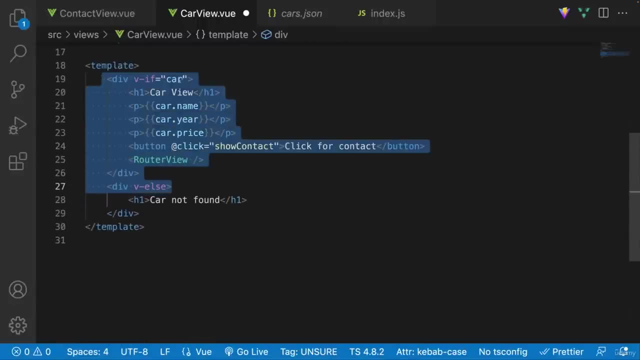 So what we can actually do here is actually use another directive known as velse. So very similar to an if-else statement. So we can say here, if we have a car, we want to render this HTML block. 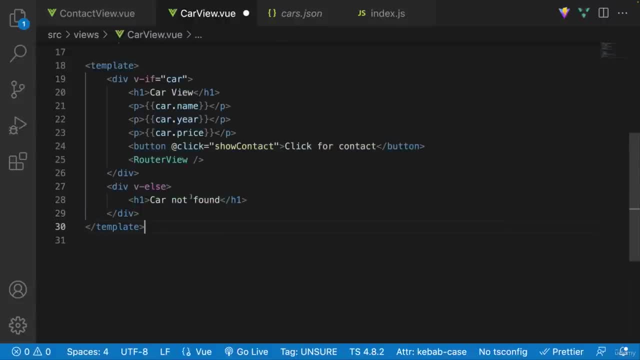 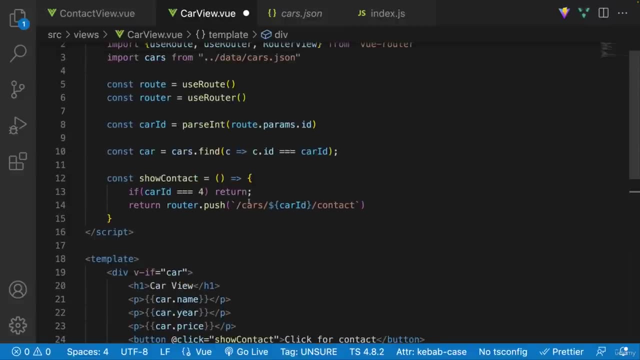 Else, what we want to do is we want to render this HTML block. And that way we can actually kind of safeguard against these individuals that will want to search for particular data that doesn't really exist. 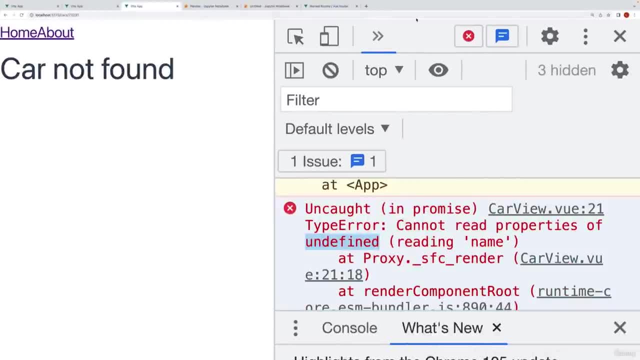 So let me go ahead and save this. 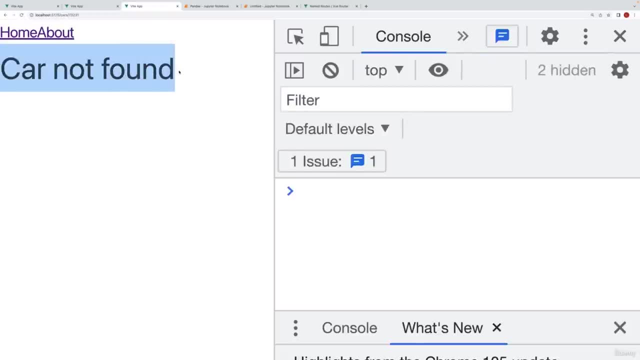 And let's go over here. You can see right away we're getting the car not found. 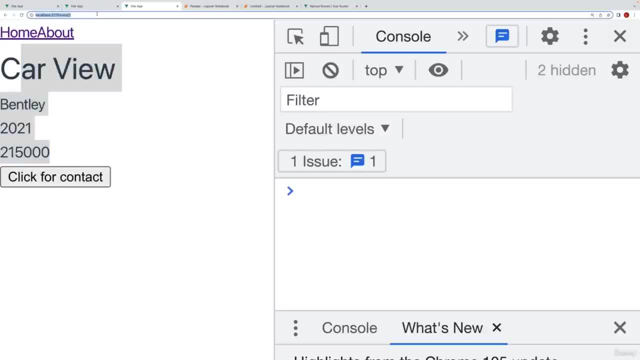 So now if I go home, I go to Bentley, and you can see I get my data. If I were to change the ID manually for some reason, you can see here car not found. 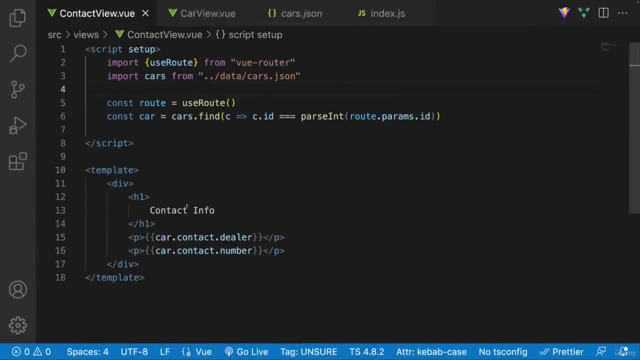 Now, of course, ideally we can also do the same exact thing for the contact view because this is going to prompt us with the exact same error. 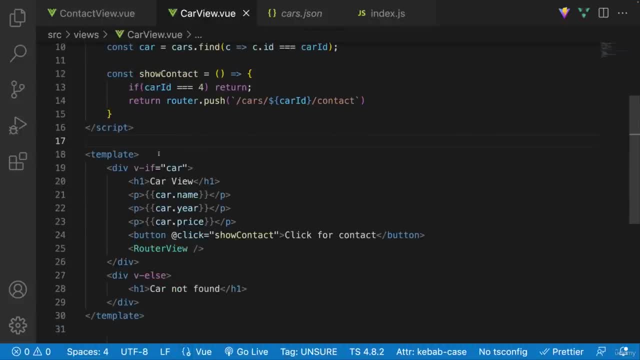 I'll actually leave this up to you just because, well, this is just the exact same step. You know what? Actually, let's just quickly do it. 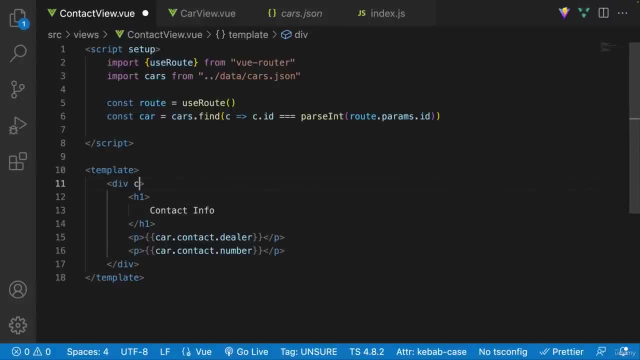 Might as well. So over here, we're going to do a quick vif. We're going to say vif car. 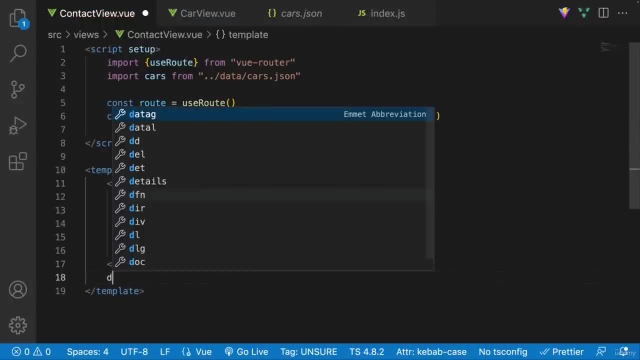 And then we are going to have maybe a v else. And actually, you know what? 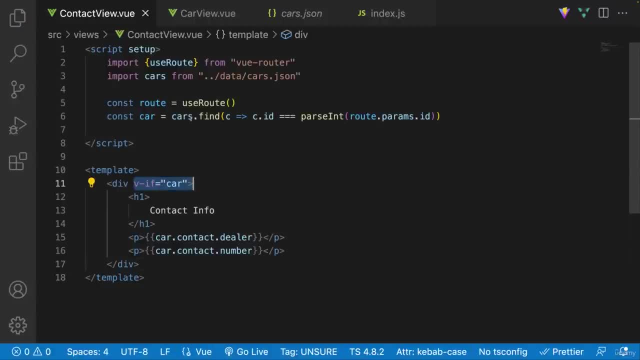 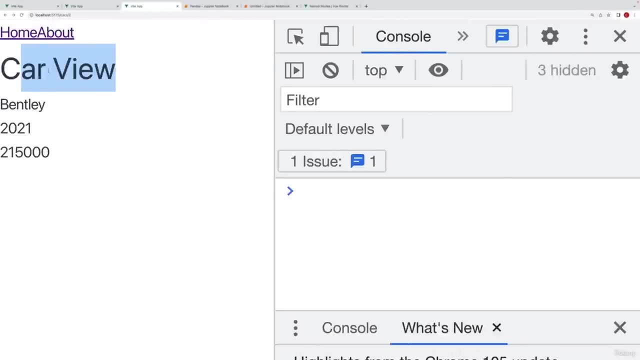 We can just leave it like this without a v else because if, let's say, we do not have a particular car, let's just not render anything because we already have this information right over here saying the contact or the car is not found. So let me just say here let's just put in some random ID. I'm going to add slash contact. 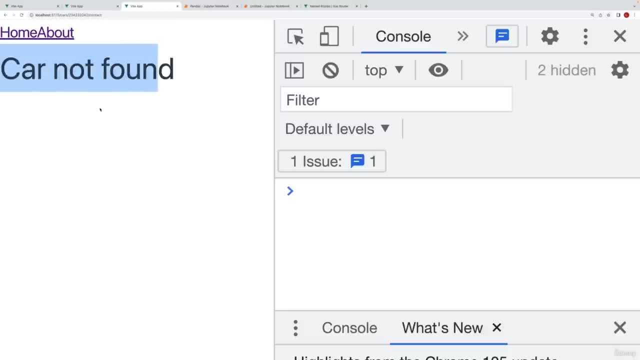 And you can see here all that is being rendered is the car not found. The contact is not even being rendered as well. And we also have no errors. Okay. 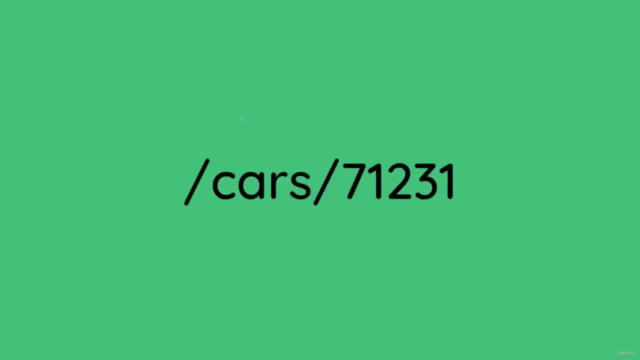 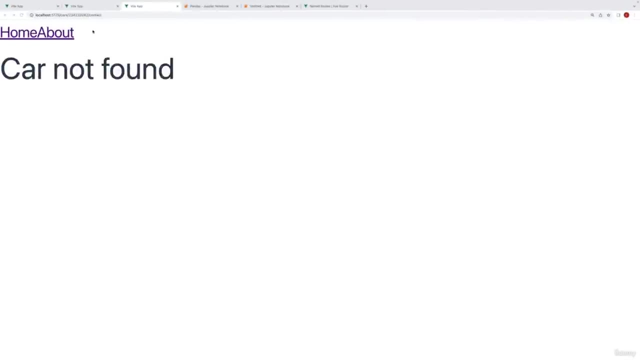 But there's also some other cases where a user can just put in some kind of random route that really doesn't exist inside of our application like slash bananas. So if they actually went ahead and did that, our application is actually going to behave the way that we configured it. 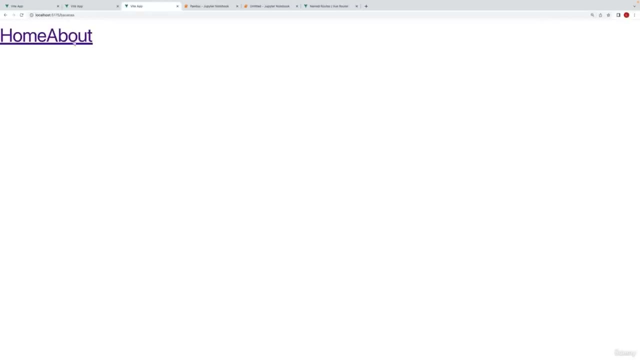 So if we did slash bananas, you can see that all we see is our nav bar because that's what we defined inside of our app.view. 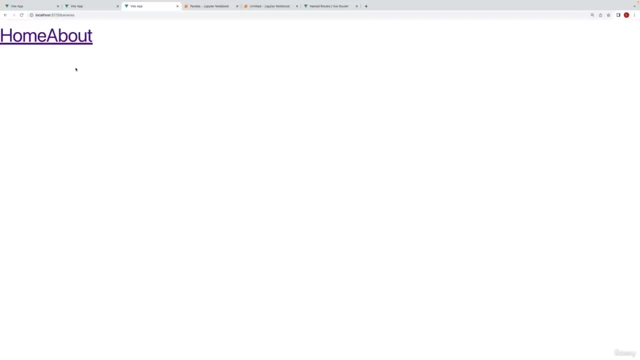 And because there's no path that we have specified in our rules about slash bananas, it's not rendering any component. 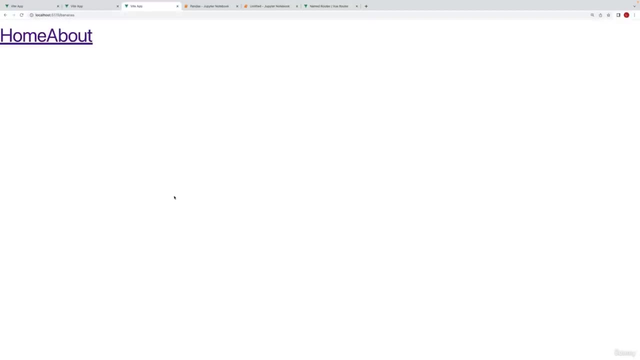 I think it would be a nice idea if for every other path that we haven't defined in our application, we render some sort of not found page, a 404 not found page. 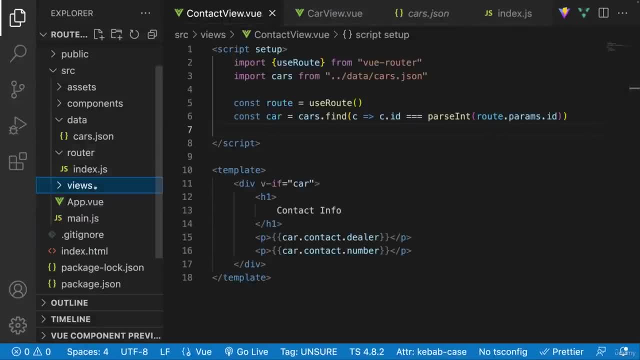 So I'm going to go over here and I'm going to create a brand new view. 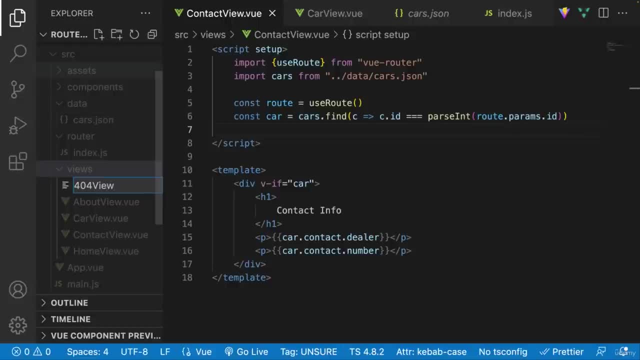 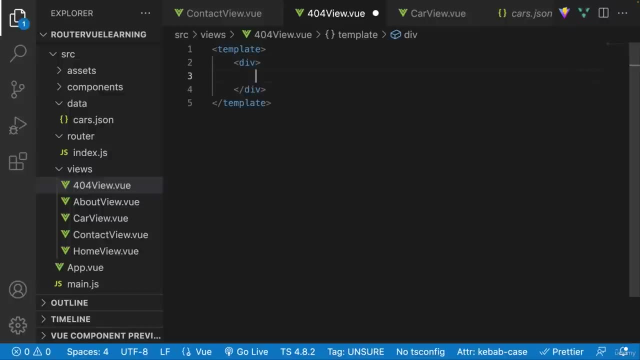 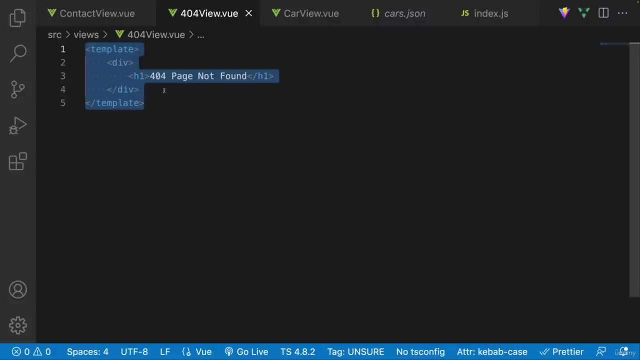 I'm going to call this 404 view. And I'm going to say dot view like so. Let's create a template. Let's create a div for this. We're going to have an h1. We're going to say 404 page not found like so. So we're going to say page not found. So we want to render this anytime we go to a particular page that we haven't defined a rule for. 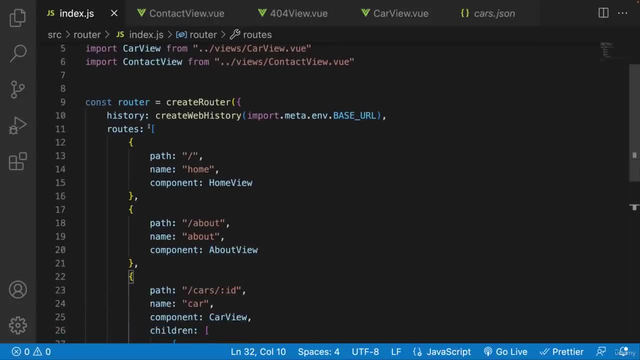 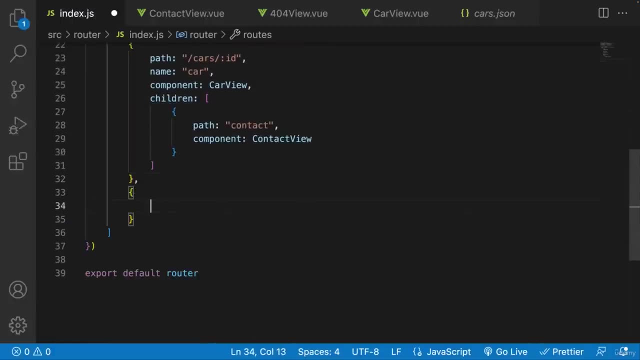 So what we're going to do is we're going to go to our index.js file and we're going to specify a new rule. So let's go over here. And this time this is going to have kind of a very special path. So we're going to say path. And then right away we're going to say something like colon and then we're going to say something like catch all. And this is actually going to be a regular expression that is going to catch all of the different paths that we haven't defined. 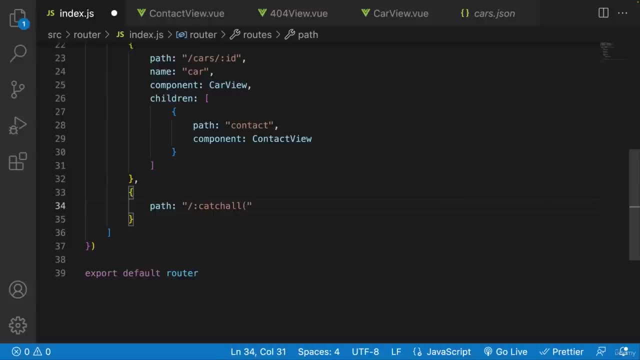 In order to do that, what we're going to do is we're going to do brackets, brackets. Then we're going to do dot star, dot stars on 8. And then right after the brackets we're also going to say star as well. What this is going to do is very simply anything that is not defined over here, well, we're going to have a component that we're going to render for it. And we've already created this component. So let's say not found. And over here we're going to say component. Let's go ahead and actually import that component. 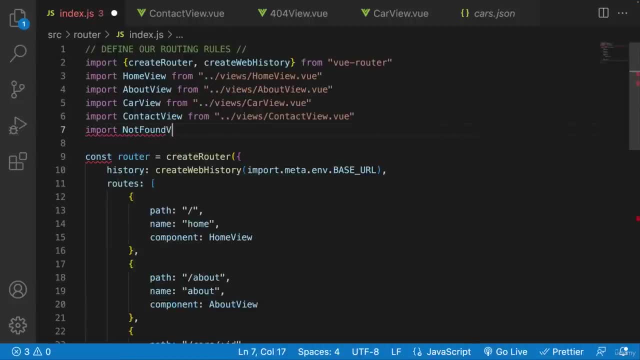 So we're going to say import. Let's say not found view. 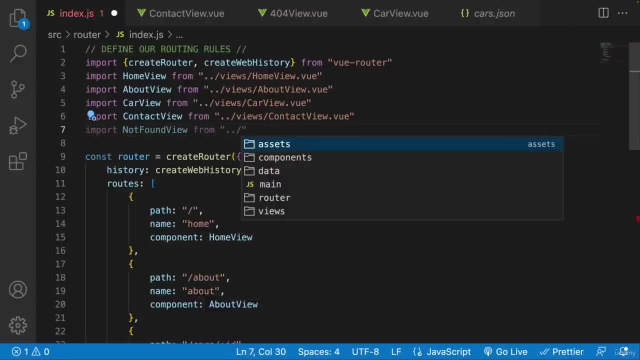 And we're going to get that from, we'll get it from views. And then over here we'll say 404 view. I believe that's what we called it, 404 view dot view. 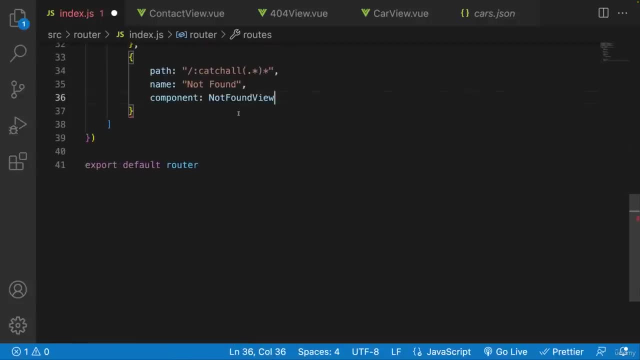 All right, so over here now what we can do is we'll render this component. Now if you're unfamiliar with regex expressions, 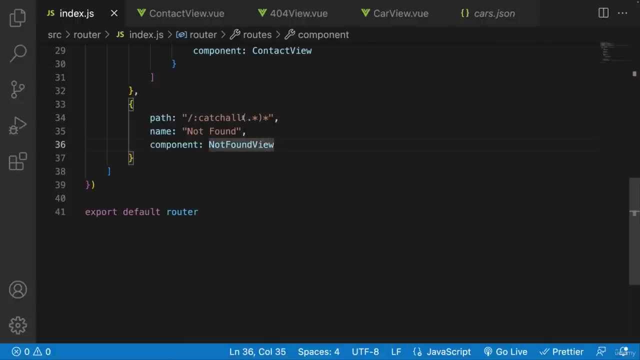 highly go ahead and I suggest kind of learning them. But this is how we can actually utilize regex expressions inside of our path. 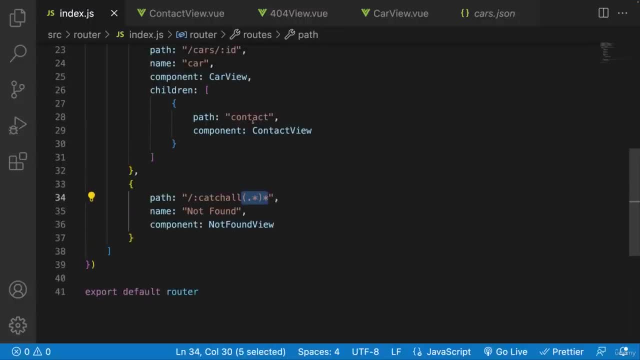 And this right here is the catch all. This is the catch all regex expression that's going to catch anything that we haven't defined. 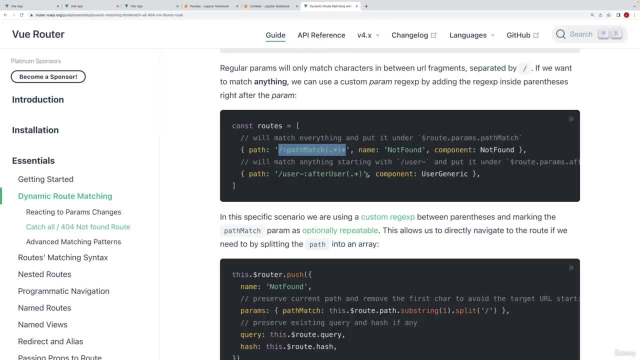 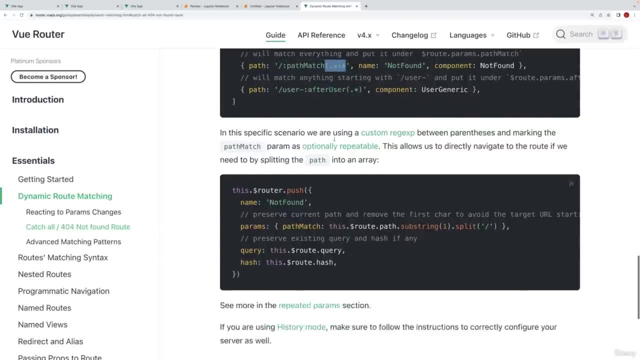 You can actually go to the documentation to see some of the other regex expressions. You can see I pretty much basically just copied it from here. And you can see that this is the catch all regex expression. Now there's a bunch of others. 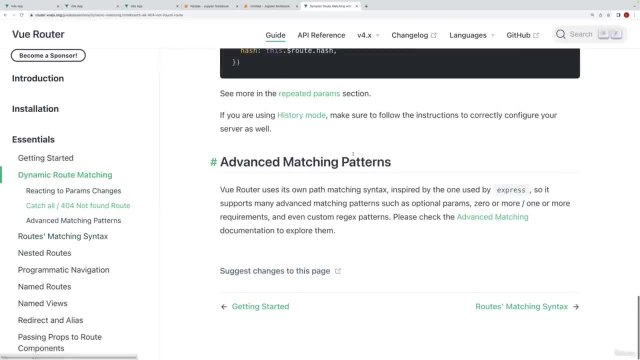 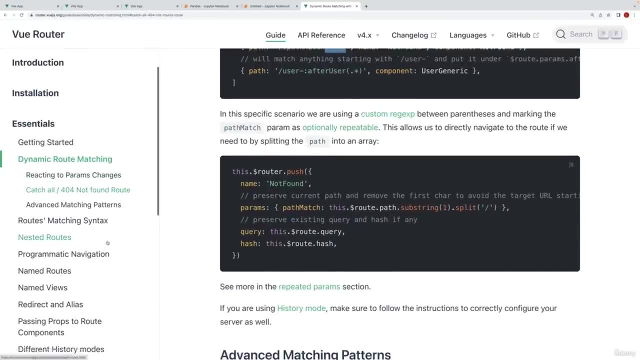 So if you go over here, maybe to the advanced matching or over here, that's somewhere in the documentation. I honestly do not even know where it is. 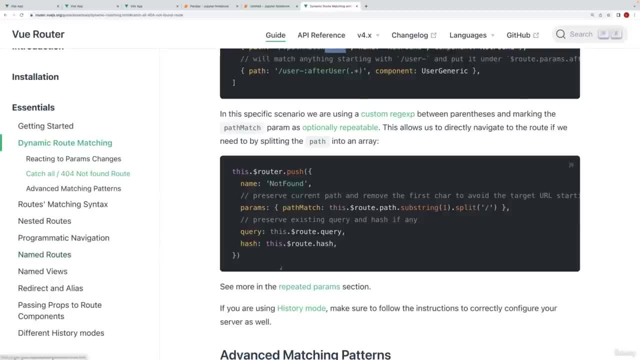 But there's somewhere here where it has more kind of regex expressions. 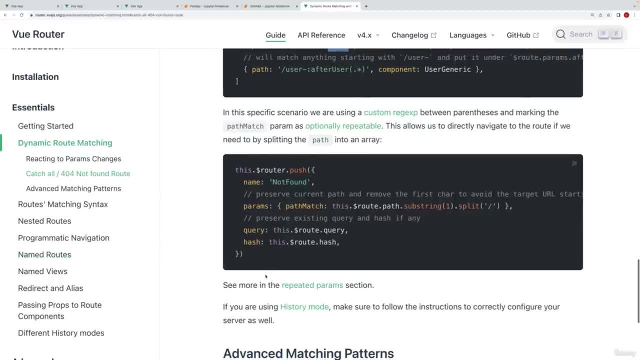 Or maybe you can force it to be a number or a string or whatever, etc. Okay, nonetheless, this is what we have. 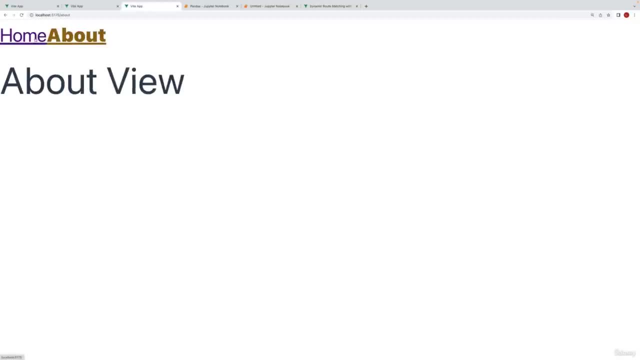 Let's take a look at our app. So currently our app is working a-okay. If I go to Bentley, I can just click around. Everything is perfect. But now if I go to slash bananas, 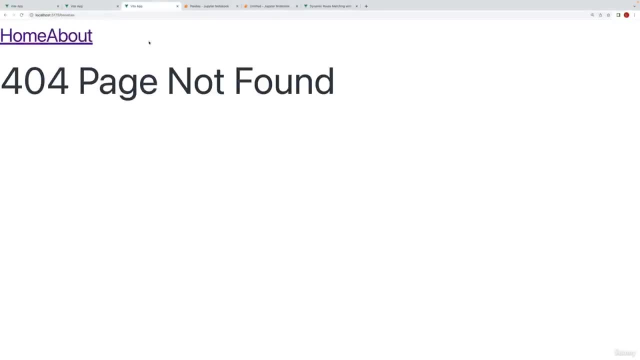 which is a route that doesn't exist in our application, you can see here we get a 404 page not found. And this is terrific. This is awesome. 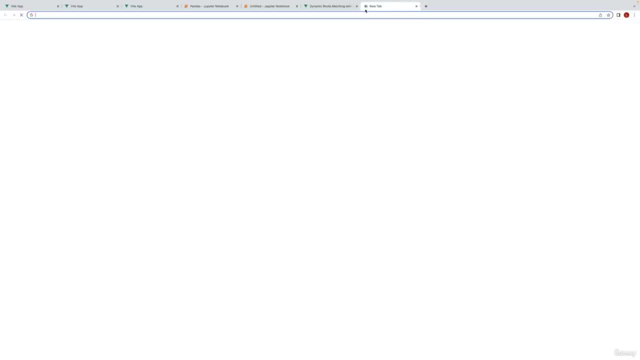 Now, of course, the styling could be better. A nice example of some really good styling for a 404 page is GitHub. 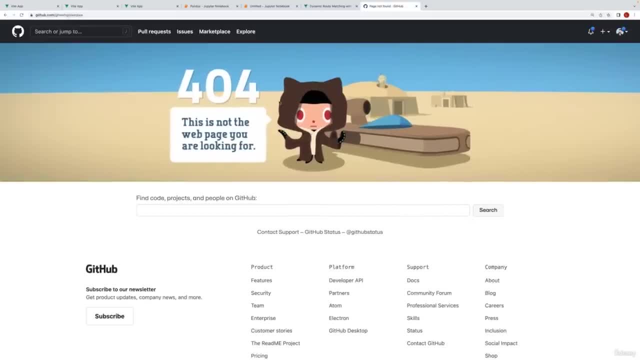 So if I put in like just some random path, you can see here we get this 404 page. 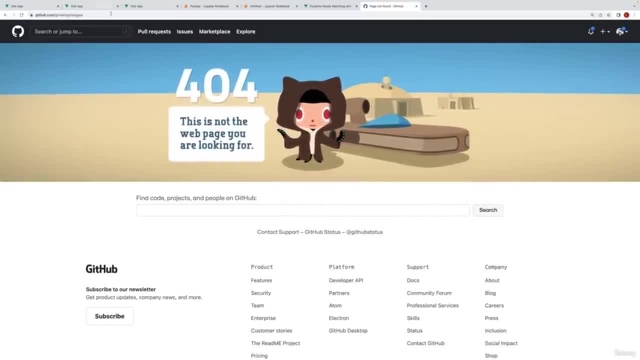 And this is, in effect, working in the exact same way. But obviously, it is styled way better. All right, my good friends. 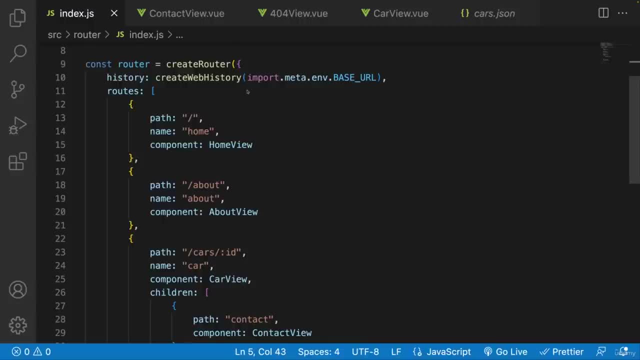 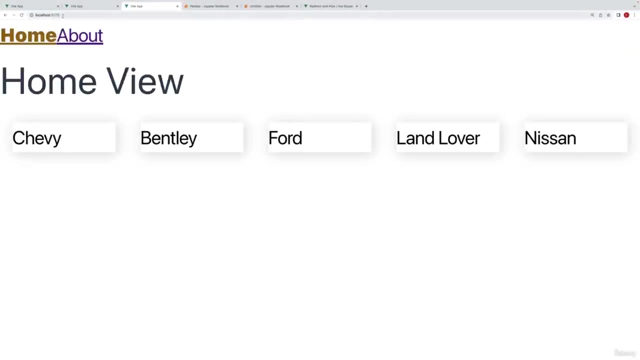 Now what we're going to talk about are redirects. So let's say that we have a scenario where a lot of our users are going to the slash home page expecting to see the home view component. So what they do is instead of just going over here to the actual website, what they do is they go to the slash home and they enter this and they get this 404 not found. 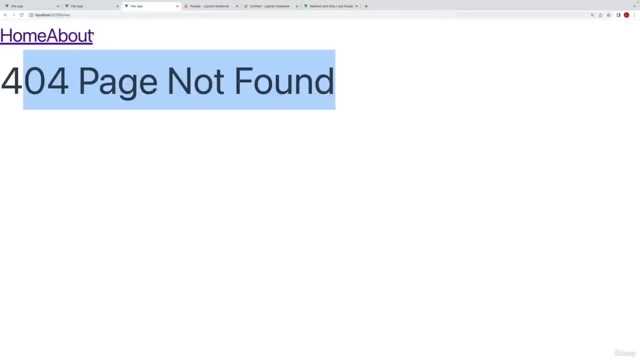 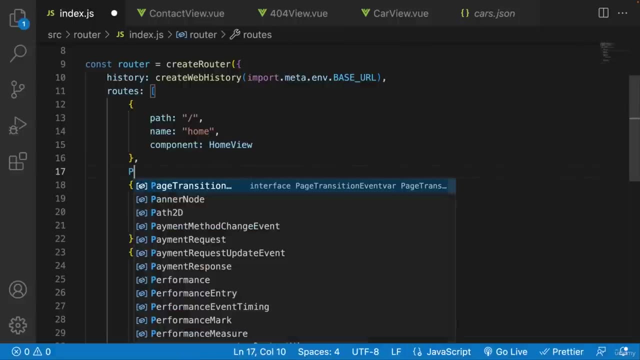 Well, a lot of our users are doing this. So it would be nice if we go to the slash home page. We also render the home view component. So one thing that we could do is very simply just add a new rule here. And we can say something like, and I'm just going to go ahead and copy this. And I'm going to go ahead and paste it as well. And we're going to say slash home. 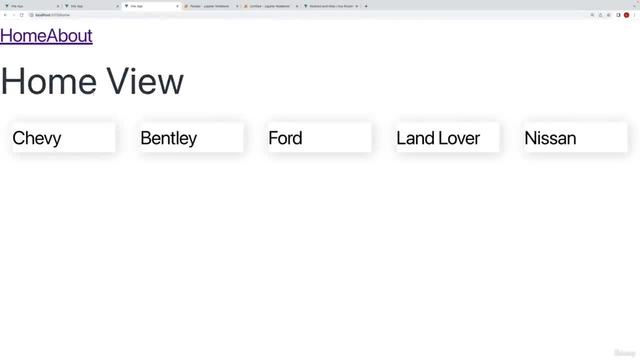 Go ahead and save this. And now if you go to the slash home page, you also see this as well. 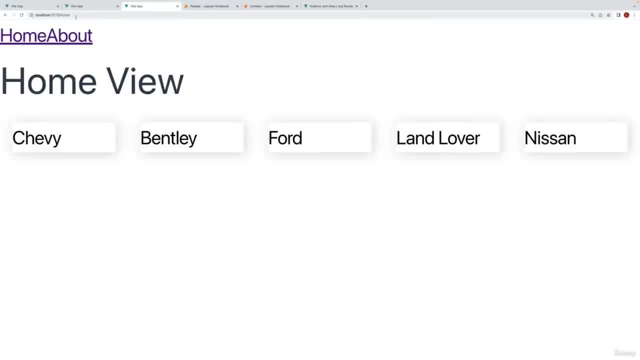 However, I actually kind of don't want this. I do not want to maintain all of these different paths. 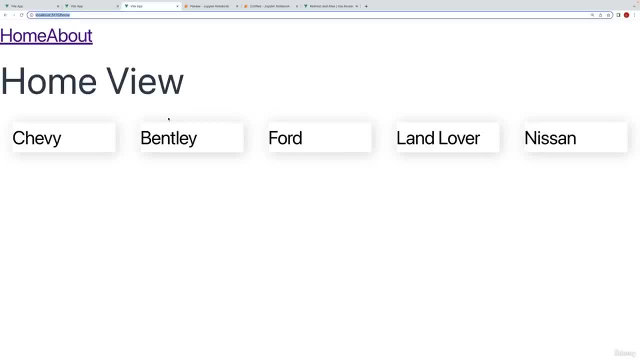 But again, if a user goes to the slash home view, I want to redirect them to this component right here. 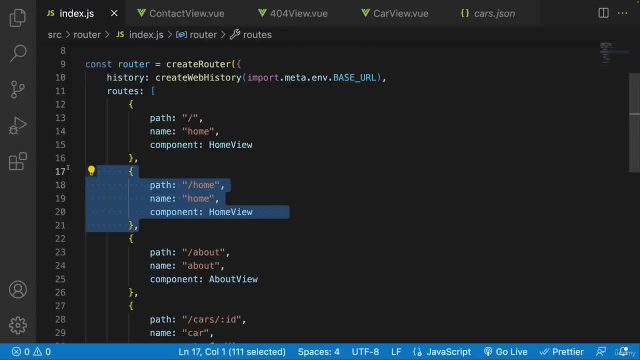 So how can I do that without adding another route that I have to maintain? 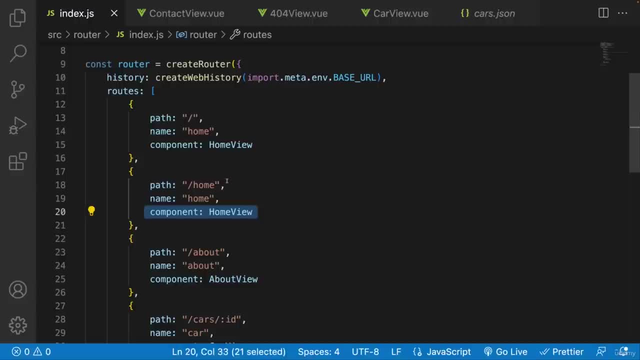 Well, very simply, instead of actually rendering a component for a certain route, what I can do is if a user goes to the slash home, what I can do is very simply redirect them 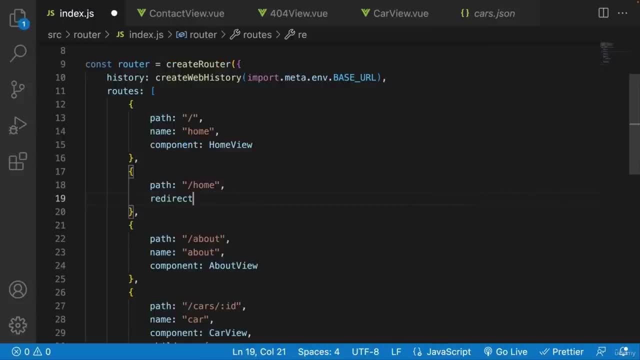 to the slash path. So I can actually say redirect and then slash like so. 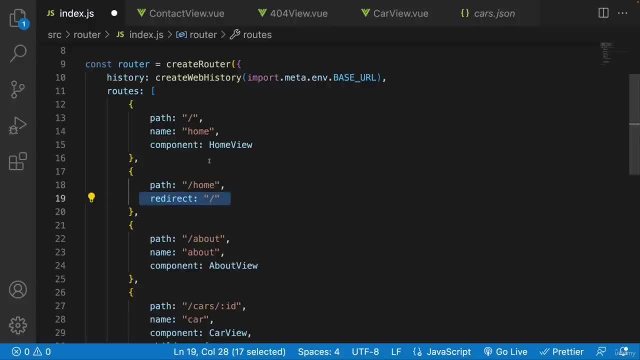 So again, if you go to home, I'm going to redirect you to slash, which means that I'm going to change the path to slash, which means that we're going to follow this rule over here, rendering the home view. 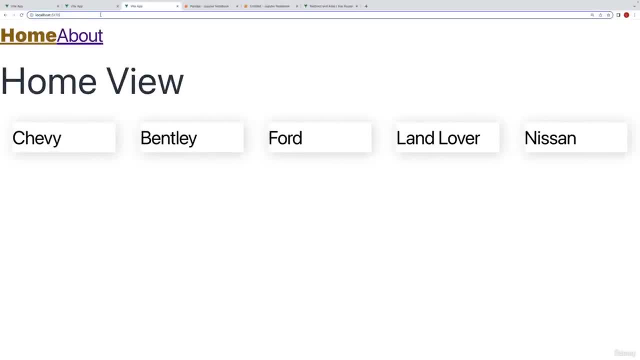 So let's go over here and go ahead and type slash home. And as soon as I type this, you're going to see that it redirects us to the slash. 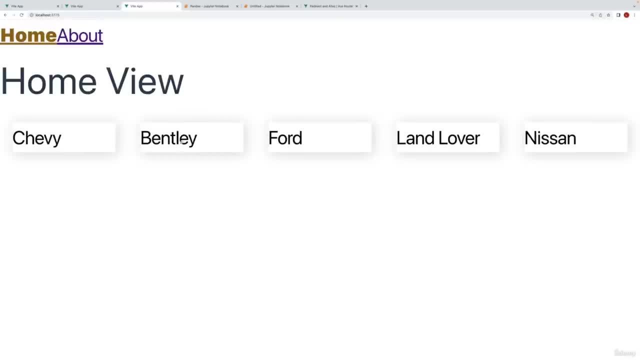 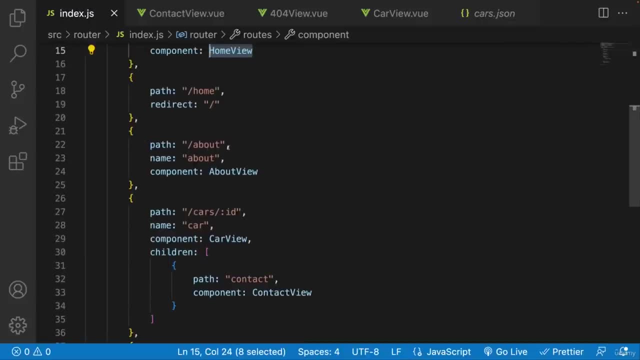 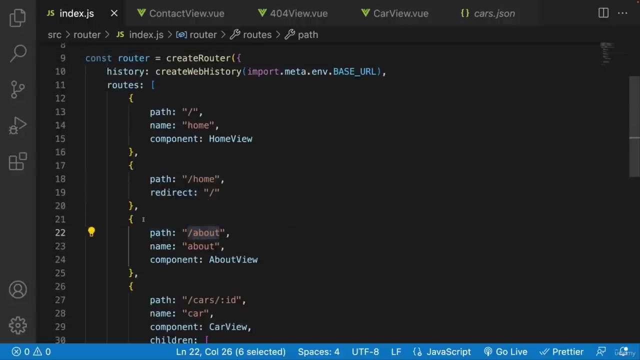 So it completely removes that slash home. Now, of course, this can be done anywhere. If we have slash info and a lot of our users are going there, we can, of course, redirect them to slash about. So this is just another neat trick that I wanted to discuss. 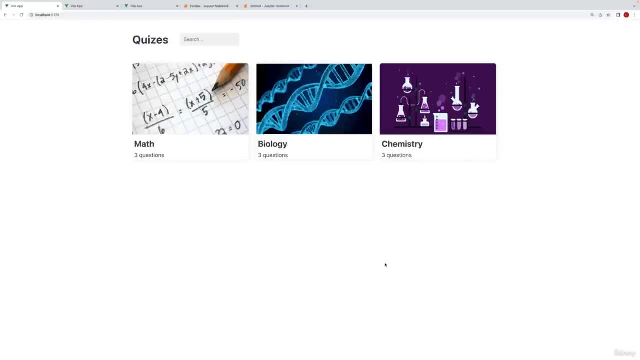 Now that we have learned pretty much everything it is that we need to learn about Vue Router, I highly suggest that you go back to the quiz application and you implement the routing for this app. 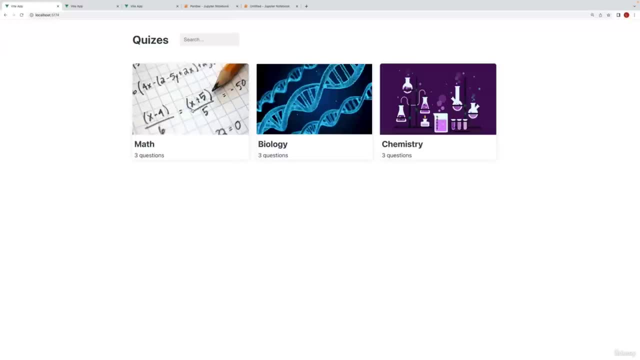 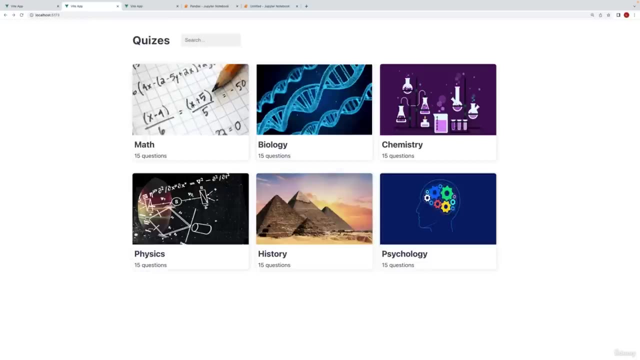 So just as a quick reminder, this is how the routing works. When you click on a particular card, let's go to the final version here, let's say you click on the math card, it's going to route you to slash quiz 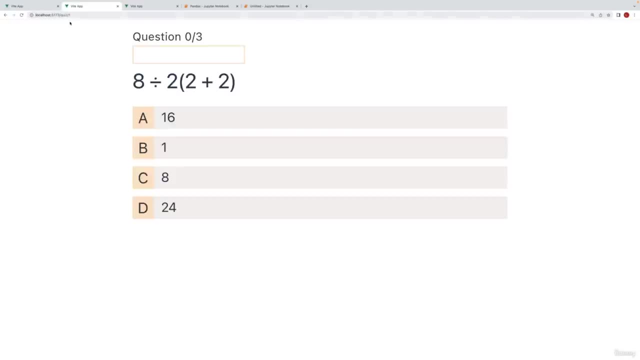 slash that specific quiz's ID. So it's going to again be slash quiz slash ID. 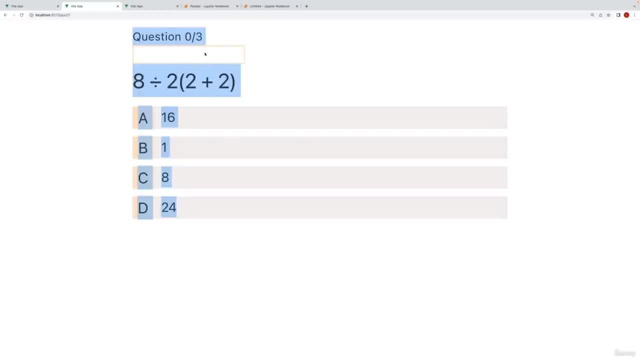 Now, of course, you don't have to work on this part over here or work on this one together, but I just want you to work on the path. 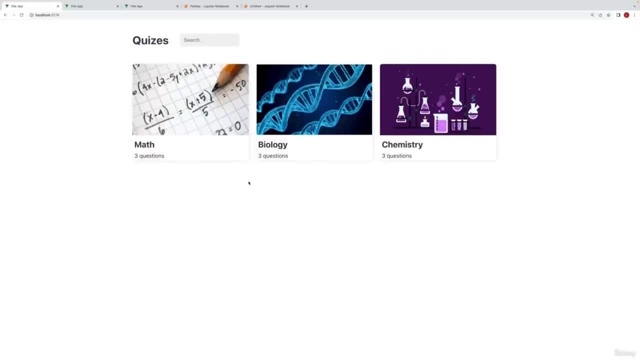 So go ahead and try it on your own. So pause this video and try it on your own as kind of a challenge and an exercise to reinforce your Vue Router skills. 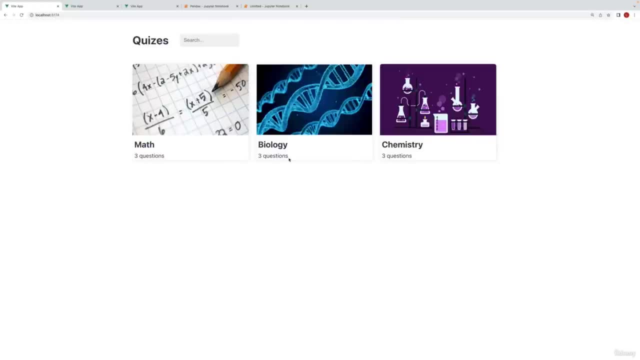 Now, I'm going to assume you paused it and I'm going to go ahead and actually, well, go through with it right now. 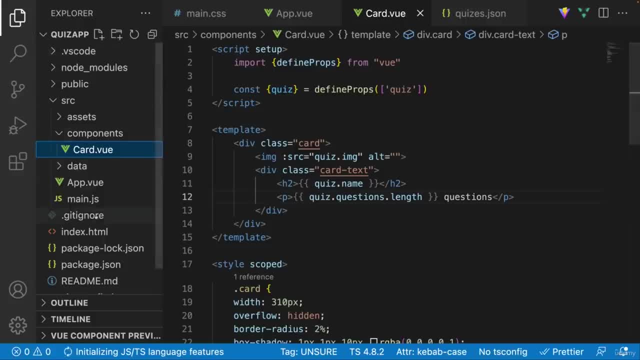 So over here, what we're going to do is we're going to go to our package.json and we're going to observe that we haven't yet installed Vue Router. 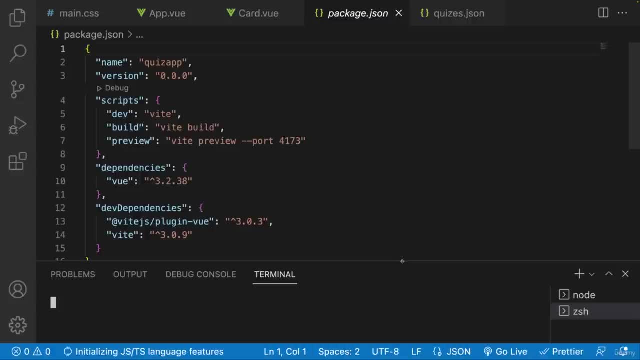 So that's exactly what we need to install. We're going to go ahead and install the Vue Router library. 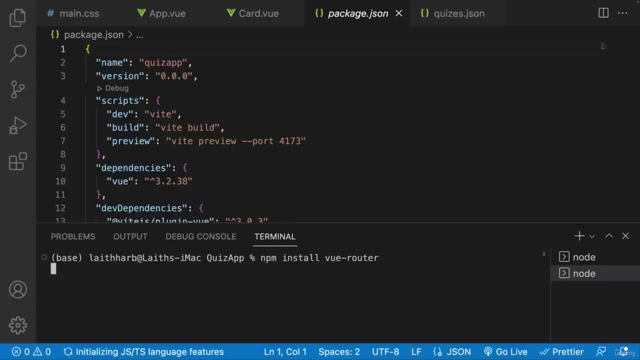 So Vue Router, like so. So now that we installed that, remember, the first thing that we have to do 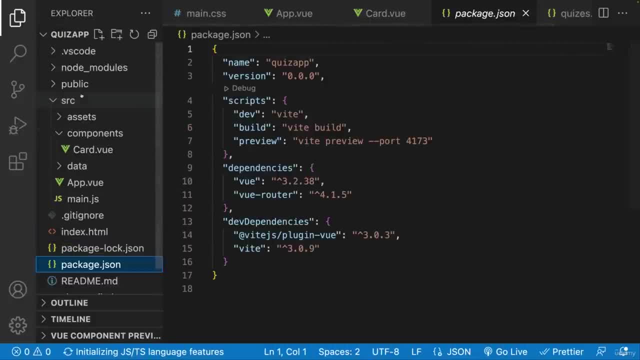 is to define our routing rules. So let's go over here and let's go to our source and let's create a router. 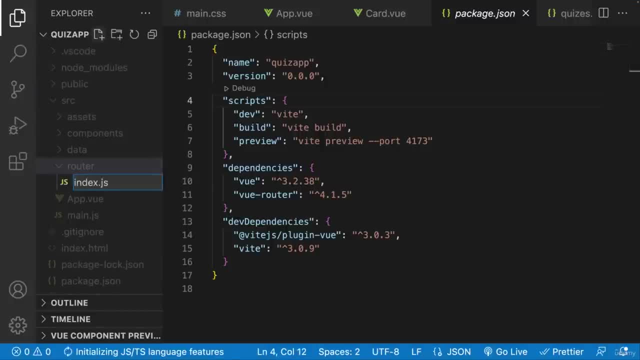 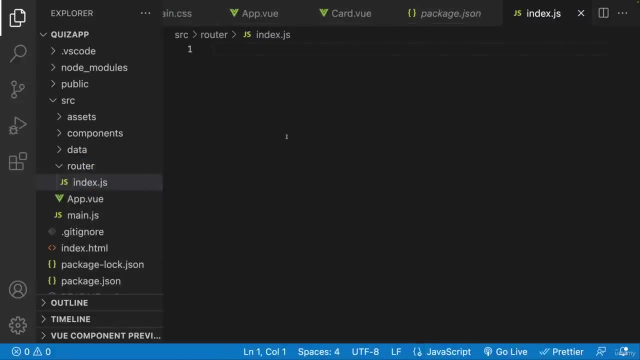 And within our router, we're going to create an index.js file. And this, of course, is where we're going to define all of our different routing rules. So let's go ahead and import createRouter and createWebHistory from Vue Router. So from Vue Router, like so. And what we're going to do here, and let me just zoom in once more. 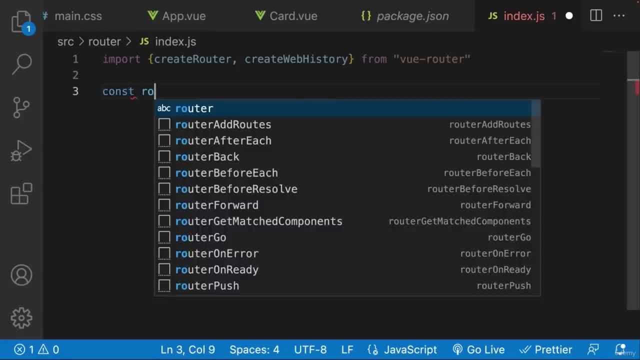 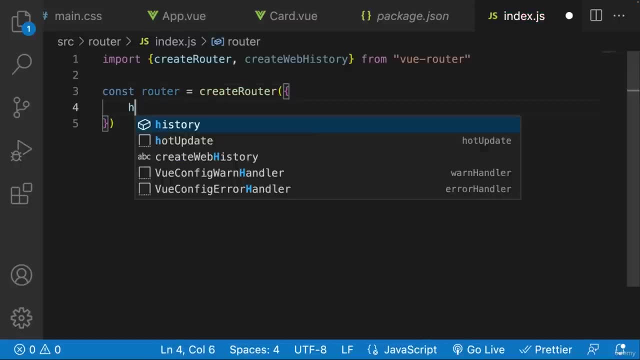 There we go, looking good. What we're going to do is we're going to create our router. And this, of course, is going to be equal to createRouter, invoke it, and we're going to pass in some options. The first option is going to be history. We're going to say createWebHistory. 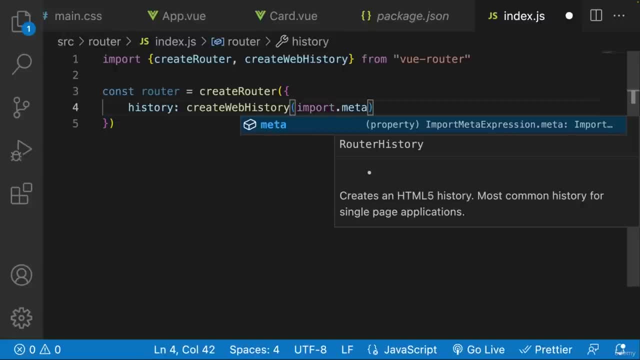 import.meta.env.baseurl All right. So that's the very first thing. 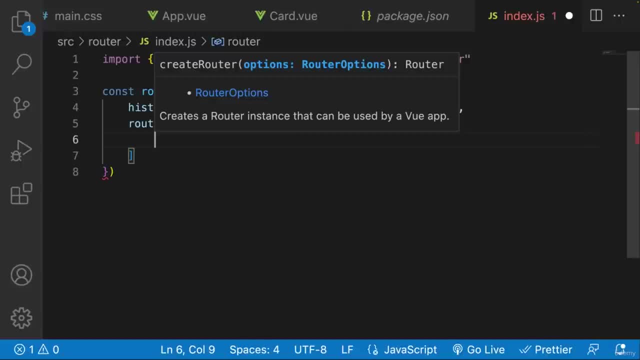 The second thing are the routes. And we're really only going to have two routes in our application. 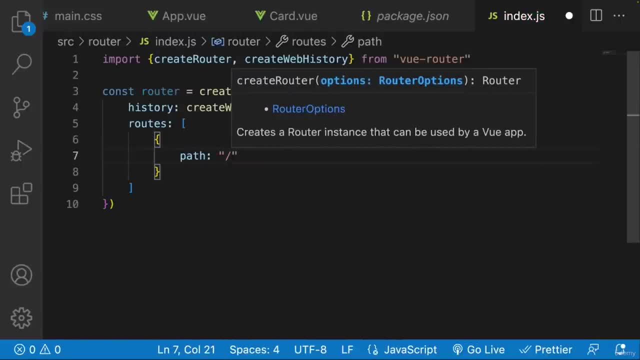 So we're going to have to have two different objects. So the first one is going to be the slash path. 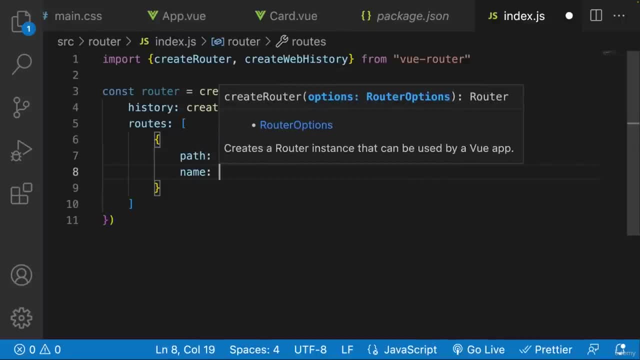 And this one is just going to show all of the different quizzes. 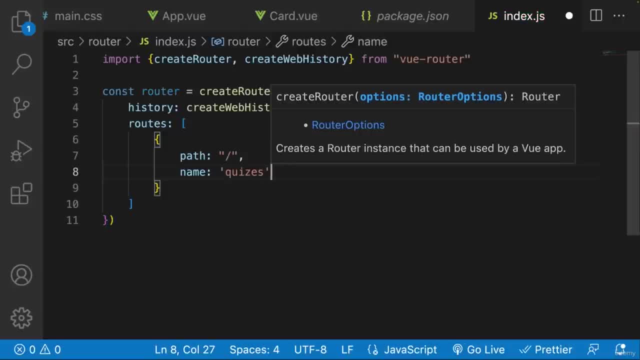 So we're going to say name, and we're going to say quizzes, like so. 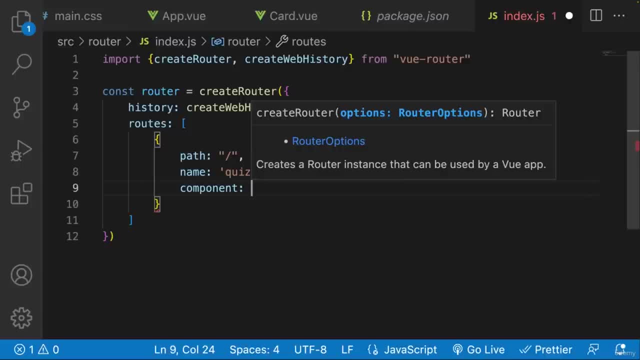 And then what we're going to do is we're going to, well, render a specific component. 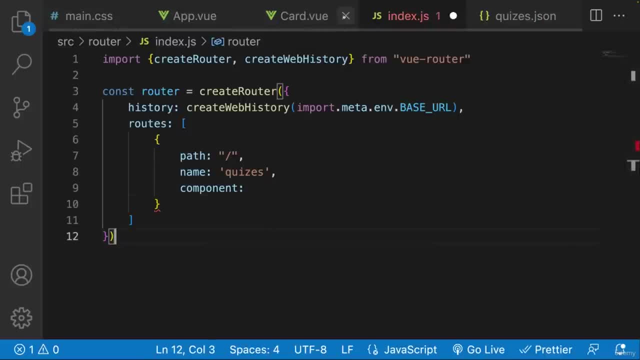 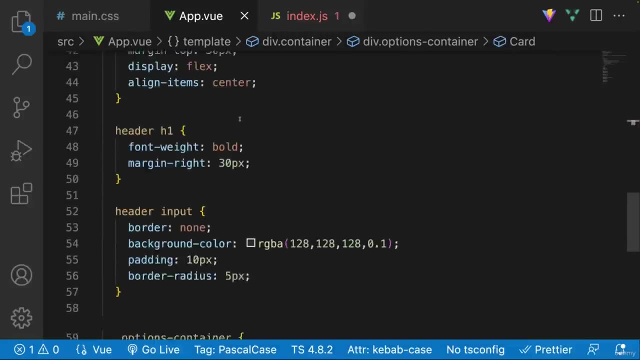 Now at this point, we're kind of running into an issue because what we did was we added all of our code right over here inside of the app.vue, which obviously at this point is not sustainable. So let's go over here. 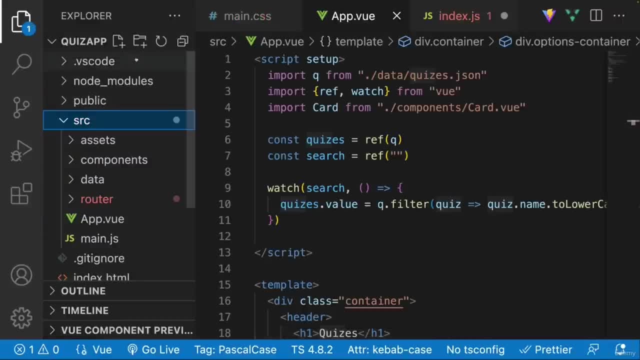 And what we're going to need to do is to create a Vue directory. So we're going to go here. 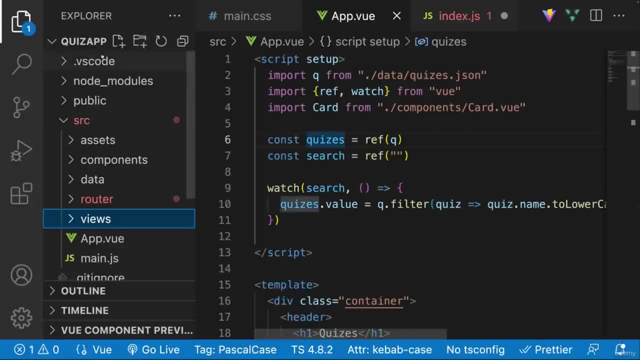 We're going to say views. And within this, we're going to create a quizisvue.vue, like so. 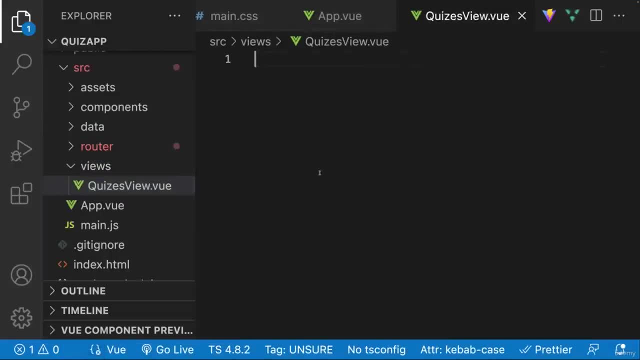 And we're going to really pretty much just copy and paste all of the different code that, well, we have created in here. 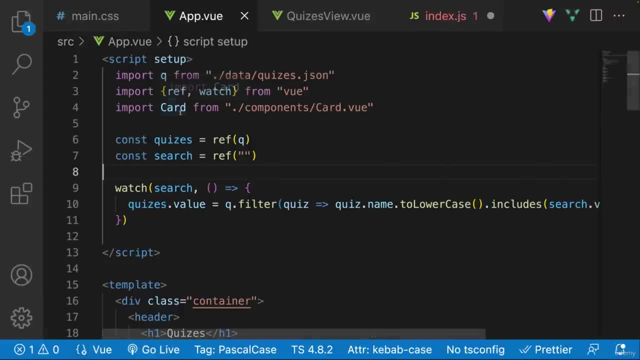 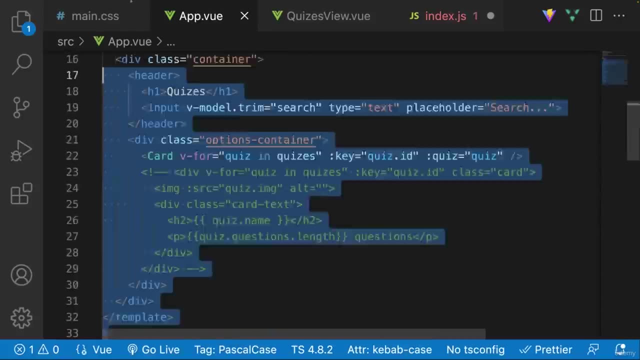 So let's go to our app. And, well, we have our setup. Okay, that's good. Let's go to our template. I think what we can do is just very simply 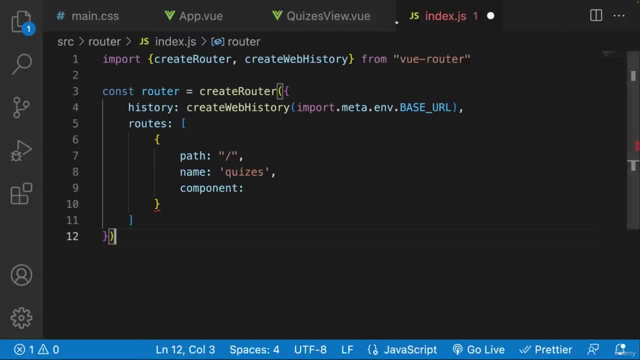 copy everything we have here and just paste it inside of here. 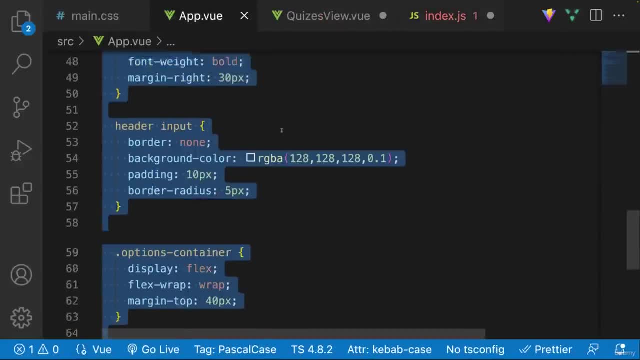 And instead of having any of this logic directly in my app.vue, we're just going to very simply have a script tag. 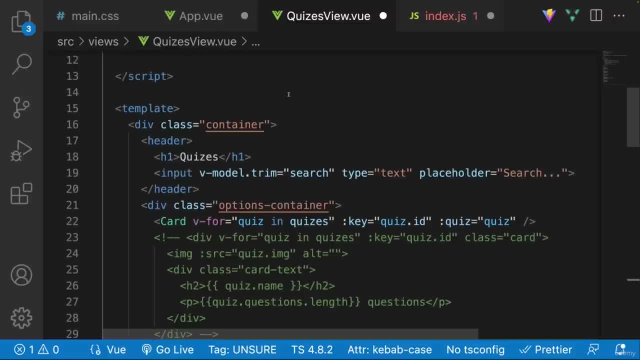 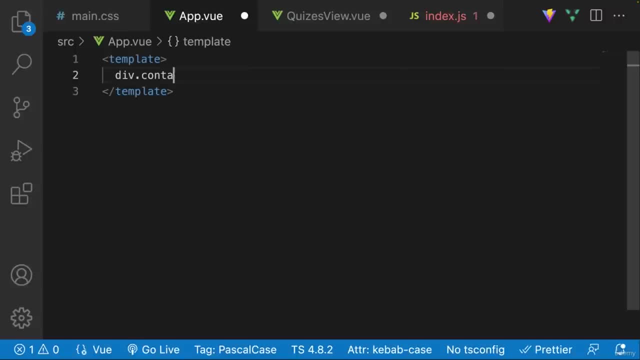 And what we're going to do is actually, let's actually have a div with a container. Container. And over here, we'll have some style. Scoped. And we will have our container styles. Where is that? Right here. 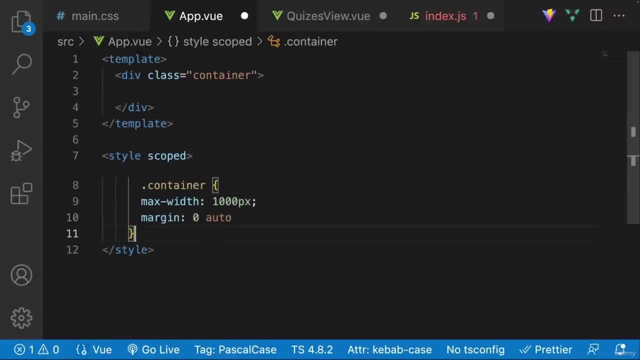 We'll cut that out from here and we'll put it right in here. Just so we can have this container style for every single page within our application. 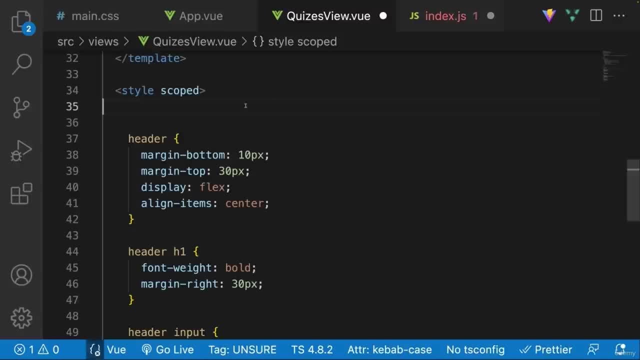 All right, so that's looking good. We'll save that. 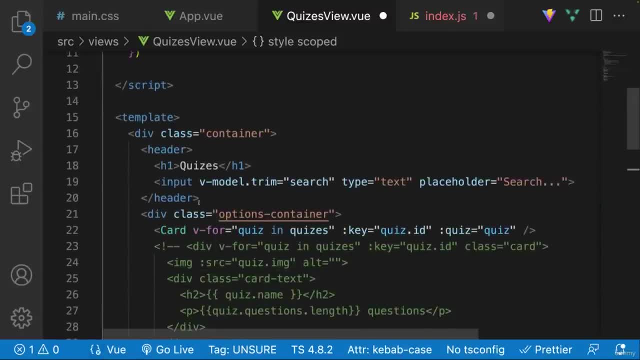 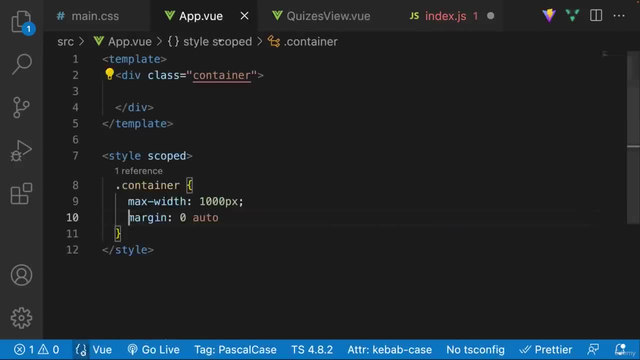 And because we did that, we can just remove the class container from here. All right, so now if I actually went ahead and I decided to render the quiz view component here, 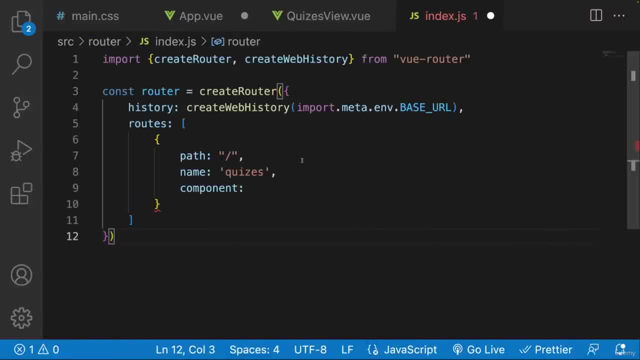 it should look a-okay. But that's obviously not what we're going to want to do for now. 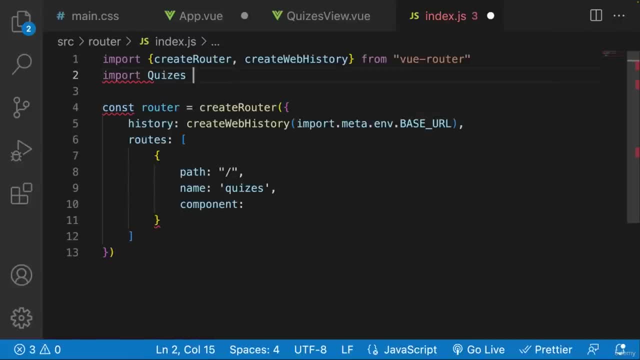 So let's go over here and let's import the quizzes view from. 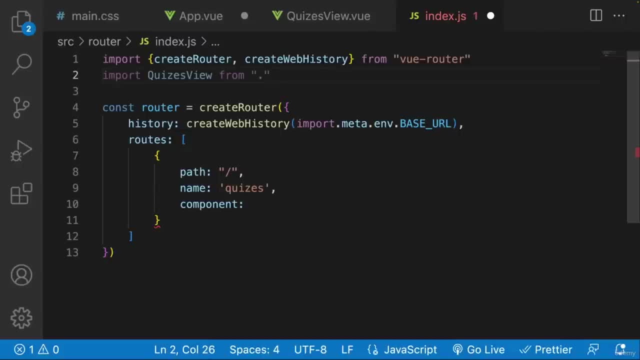 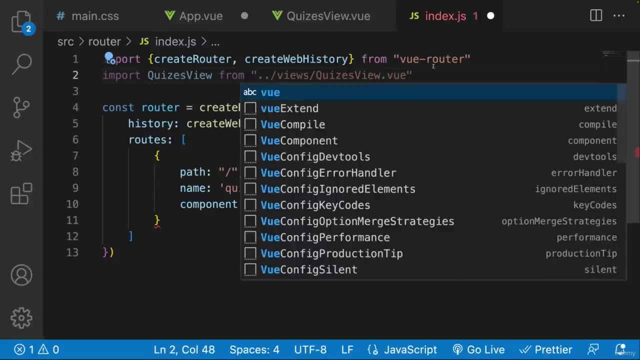 And we're going to. Let's find that directory. That's going to be views slash. And then we're going to say quizzesview.com. And that's the component that we want to render. 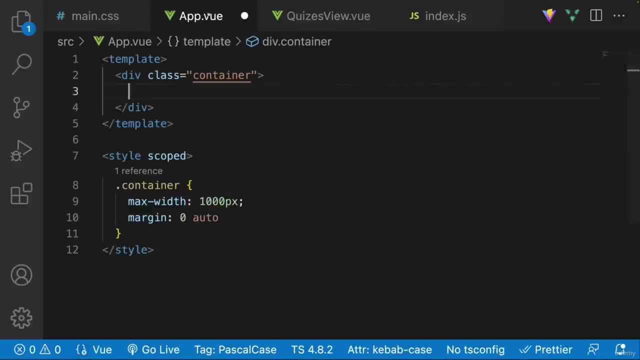 Now, of course, how are we going to render this in the app.view? Well, we're going to use that router view from view router. So let's go over here. Script setup. 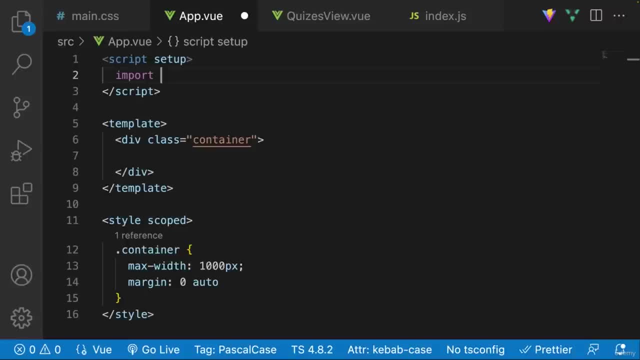 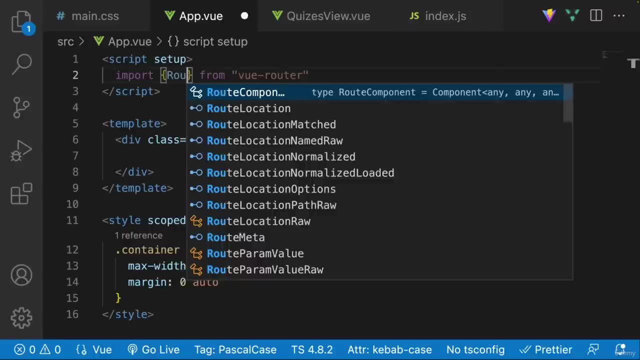 And then what we're going to do is we're going to import. We're going to import from view router the router view. Right so. 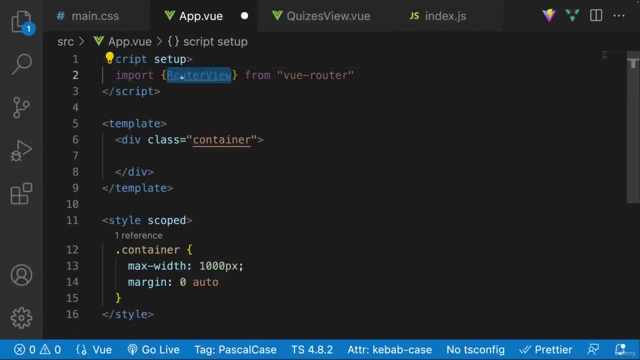 So let's remember what this is going to do is look at the path and figure out exactly what component it needs to render. So now if we save this, theoretically, our application should look exactly the same. So let's go over here. 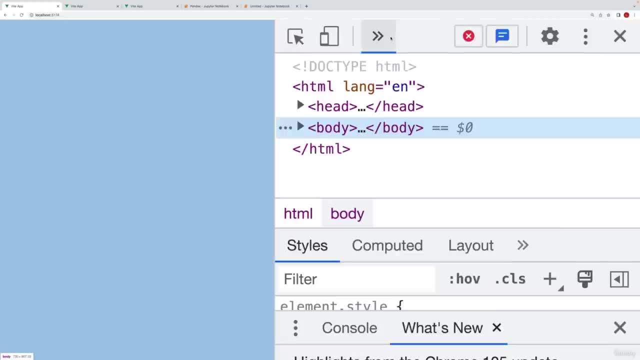 And of course, that was theoretical. Something will always go wrong. 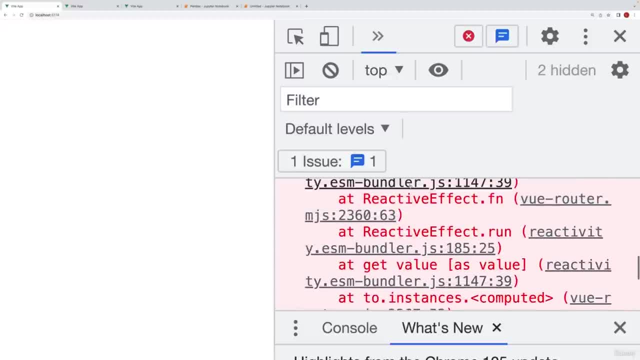 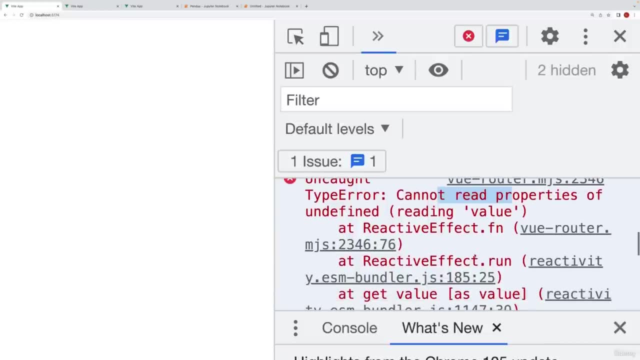 Let's look at our console and it's yelling at us for something. And it is yelling at us for saying cannot read property value of undefined. Nice. All right. 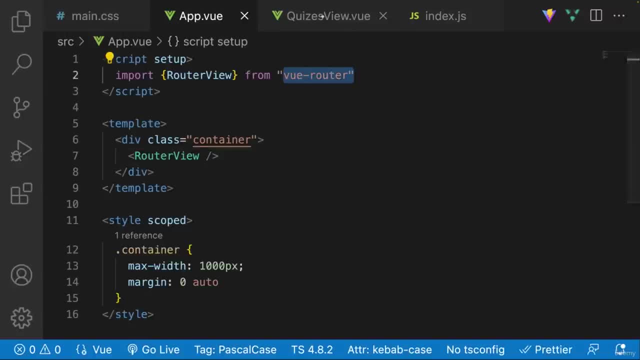 Why is that? So we got the router here. We got the quizzes. Do we have anything here? Oh, quizzes dot value. 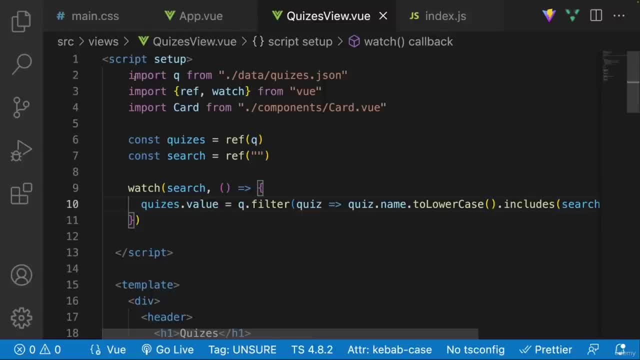 Oh, yes, yes, yes. So so because we have moved our thing around, what we're going to start needing to do is is update our paths. 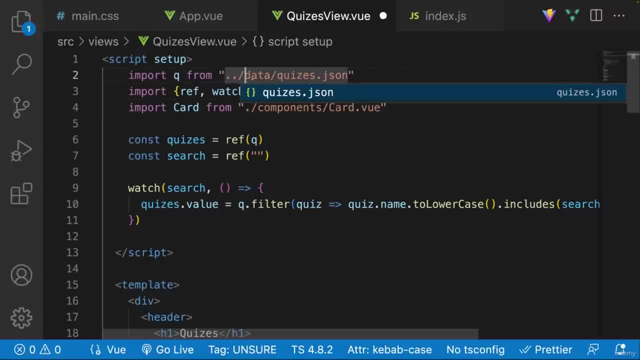 So now it's going to be slash slash data because we're going to need to move out of that directory. 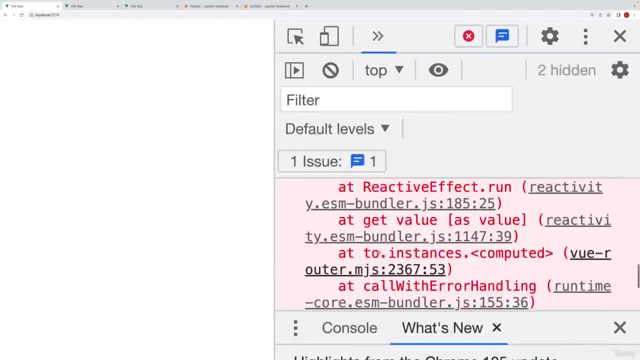 And now if I refresh. Do we still get that error? Yes, we do. Okay. So let's see. All right. Let me go over here. Comment this out. And let's refresh. 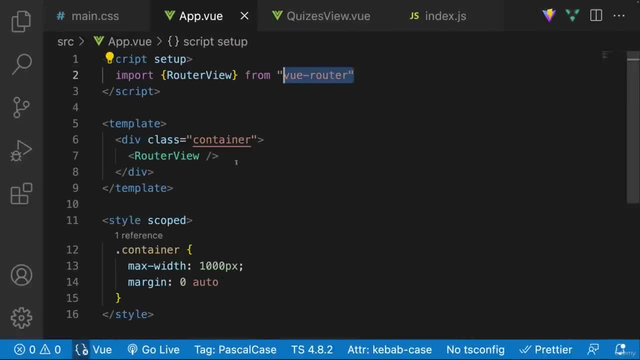 Okay. So it seems as though when I render the quizzes view. So let's just go ahead and just try to render the quizzes view itself. So I'll say quizzes view. I will say from. We need to go to. 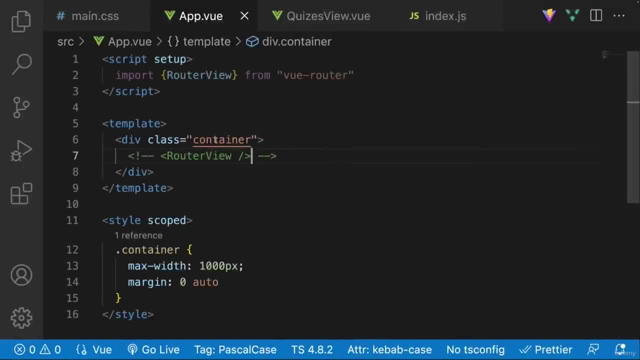 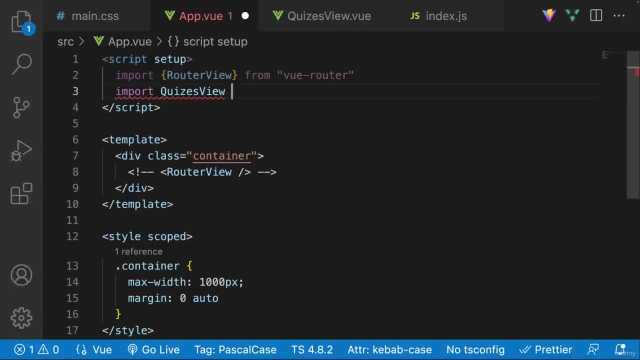 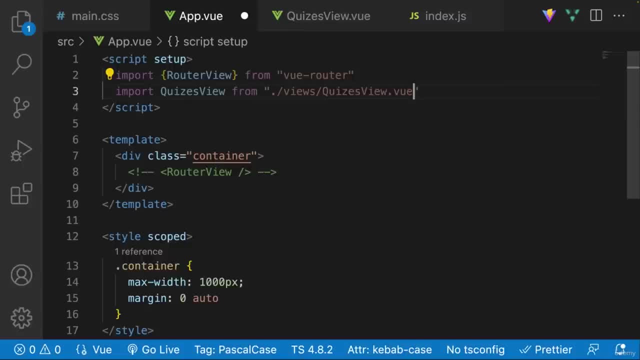 We need to go to the source. Or sorry. Not the source. We need to go to the views slash quizzes view. And let's go ahead and just render the quizzes view itself. And it seems as though. There we go. We're getting some sort of error. Seems as though. 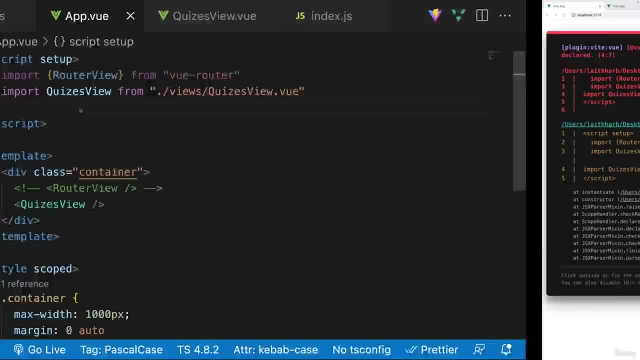 We got an auto-import here. Let's get rid of that. Okay. So that's looking good. 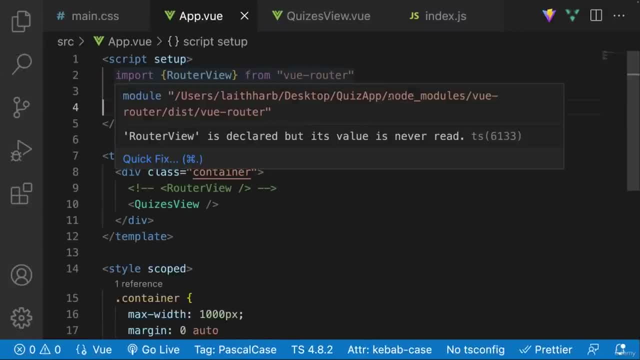 Let's do a little refresh. So that's working. So now. 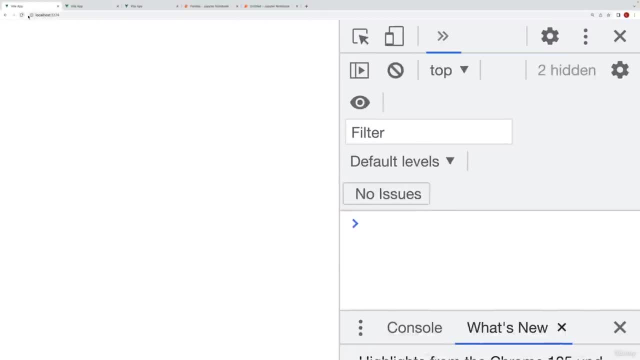 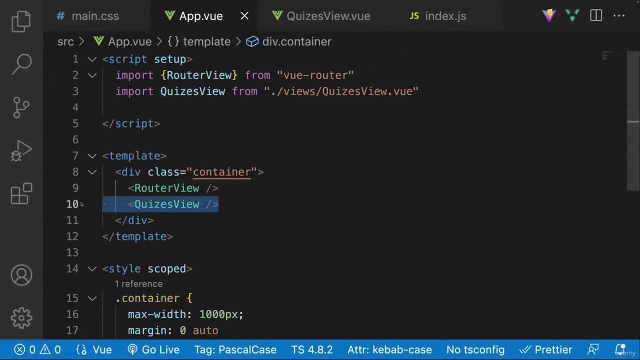 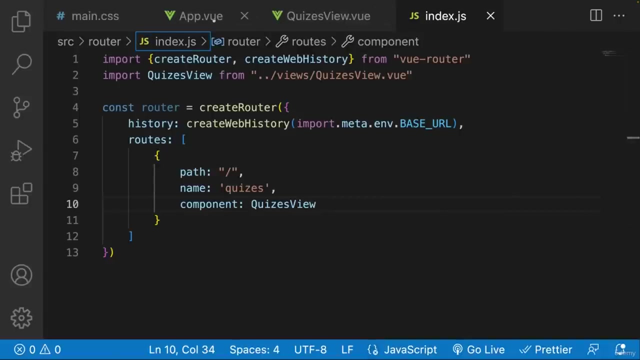 try to render the router view and it is completely failing hmm interesting type error cannot read property of undefined that is oh oh my goodness all right so so yes we have defined the rules but i can't believe i forgot this we have defined the rules and then over here inside of the app.view 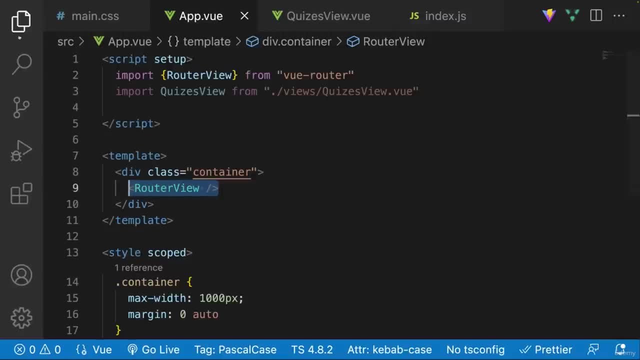 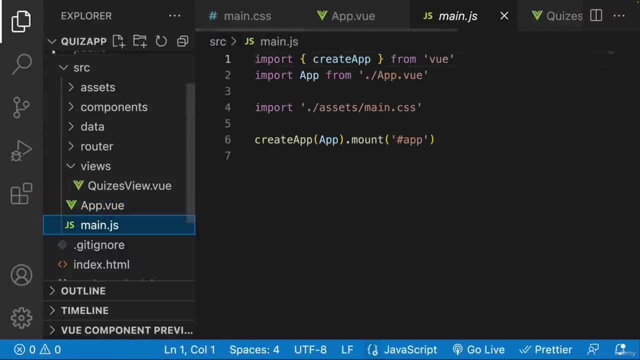 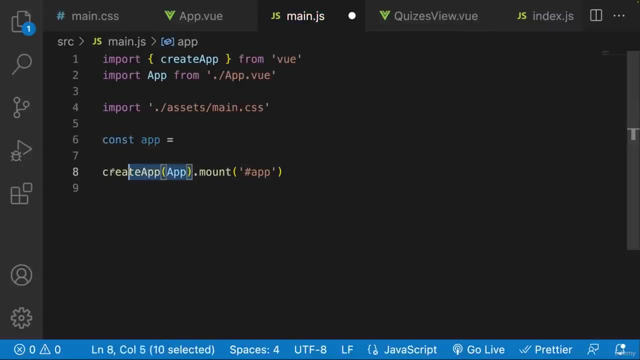 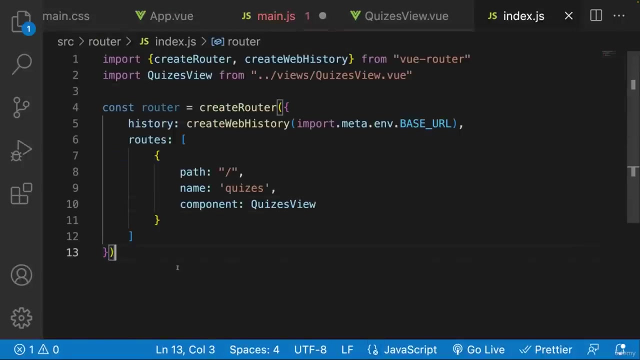 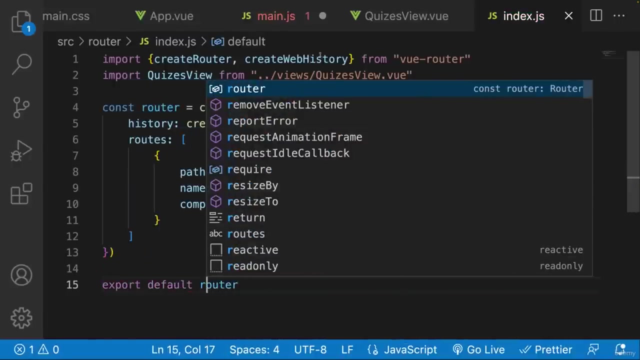 we have defined where we want to utilize it but now what we need to do of course is to connect it to our view application so over here we're going to need to go to the main.js file and what we're going to need to do is do a const app is equal to create app like so and then we're going to say app.use and then we're going to say over here we're going to utilize our application so let's go over here and we're going to say app.mount and we're going to utilize the router that we have just created so we're going to say router from we need to make sure that we're export defaulting the router so export default router so let's export default that and then we're going to say from we're going to say router 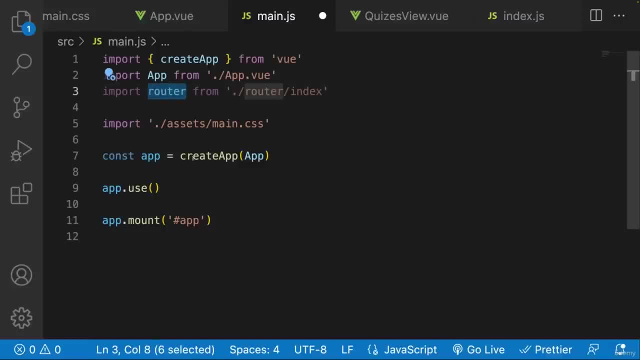 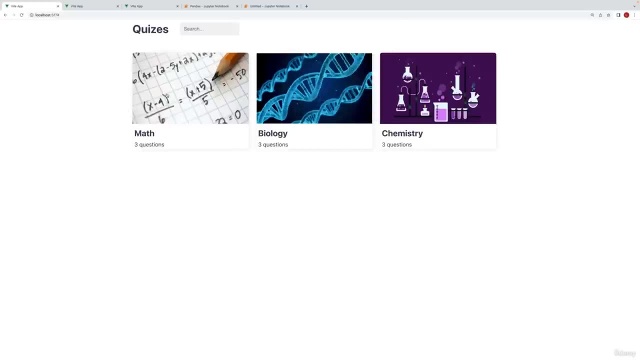 index like so and then we're going to utilize that router all right and there we go so theoretically again everything should be fine so we're going to say app.mount and we're going to be working a-okay but this time we're utilizing routing all right so the last thing that we need to do is actually make these cards clickable so when we actually click on these cards we can 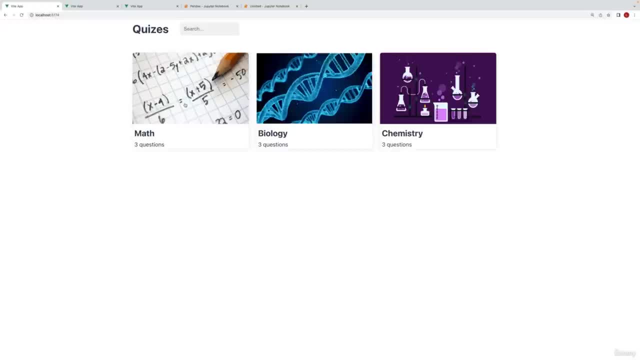 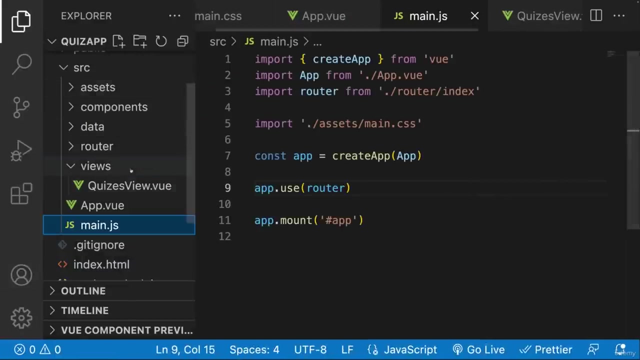 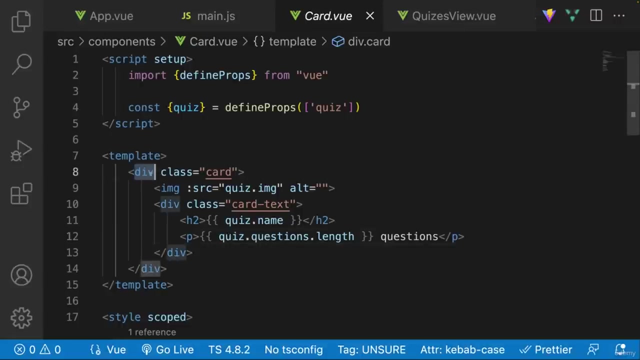 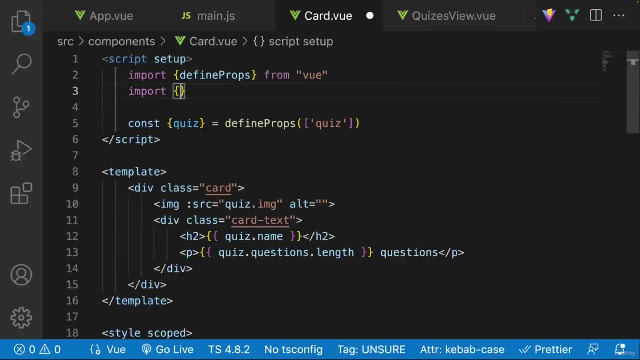 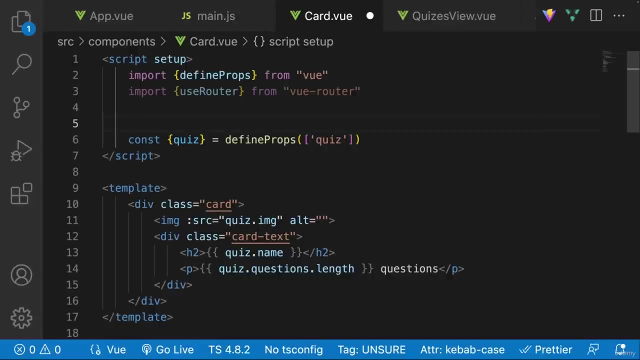 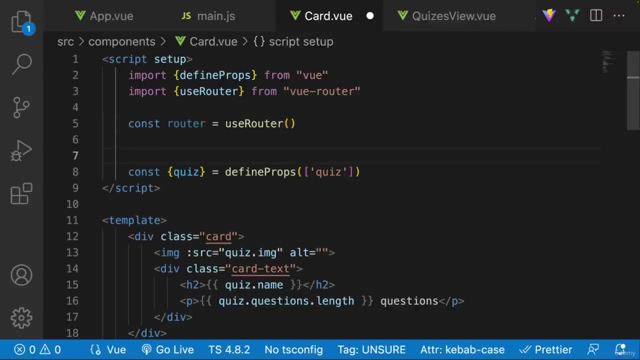 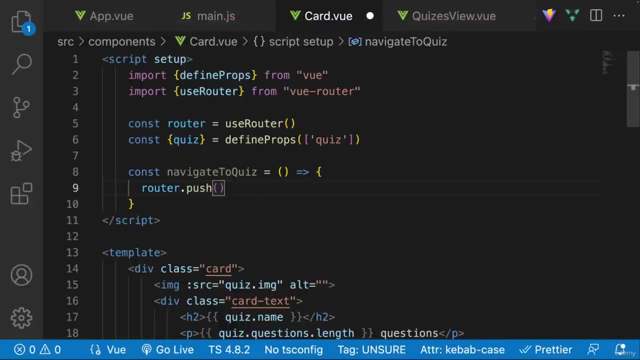 navigate to the page that we want now we have two choices here we can either use a router link or we can use a more programmatic approach now because these cards are actually indeed divs and i probably do not want to change it to an anchor tag i'm going to use the programmatic approach so let's go ahead and do that so let's go here let's go to our components our card so over here we're going to use the programmatic approach instead of using the router link approach and changing this div to an anchor tag so in order to use the programmatic approach we're going to need to import something so let's let's remember that we need to import use router so we're going to say use router not use route use route to get information from our application or from our paths whereas use router is to actually mutate and modify it so we're going to say const router and we're going to say that this is going to be equal to use router we're also going to create a function so let's create a function right over here i'm going to say navigate to quiz and then this is going to be an arrow function and we're going to say very simply router.push and we're going to use template literals here we're going to say slash quiz and then dollar sign curly braces to use some javascript and we're 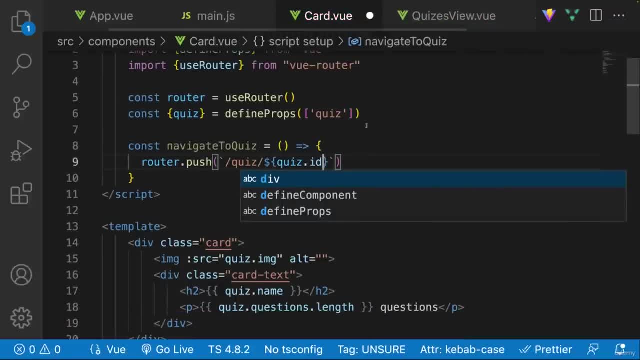 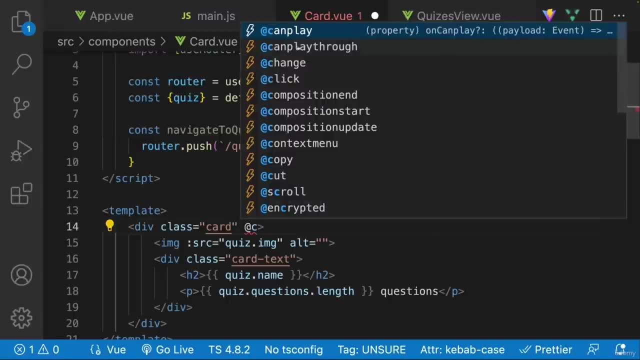 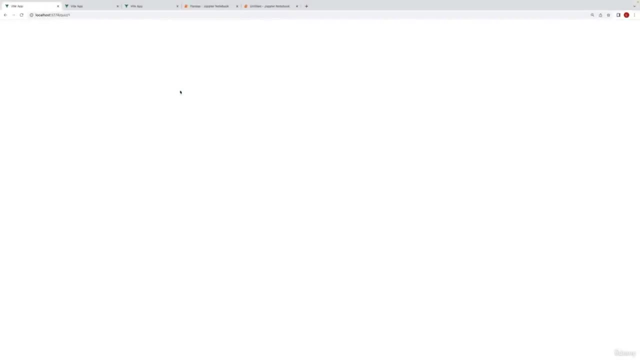 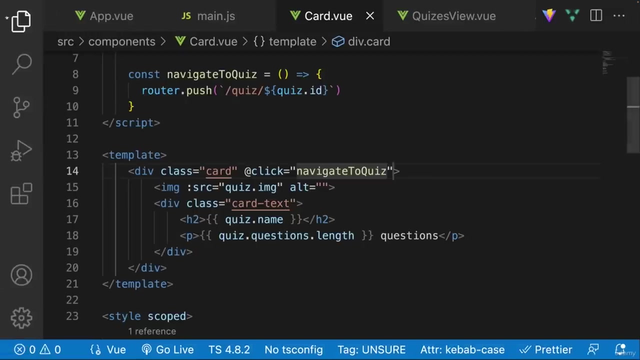 going to say quiz.id very simply the quiz that we get from the props and if we click on this so if you add a click listener here we're just going to say navigate to quiz so now if i were to click on this you can see it actually does indeed navigate us to that path which is really good but of course there's nothing really 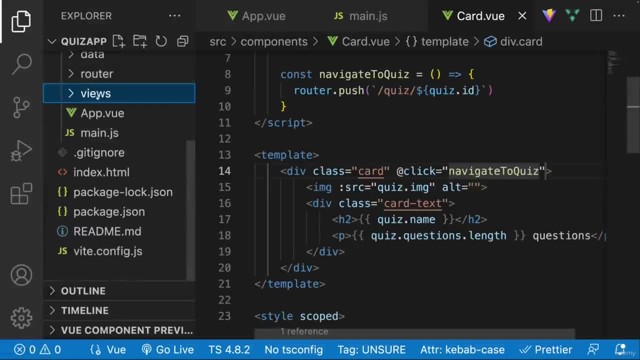 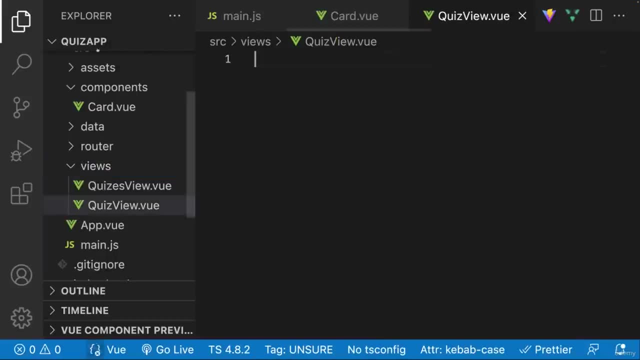 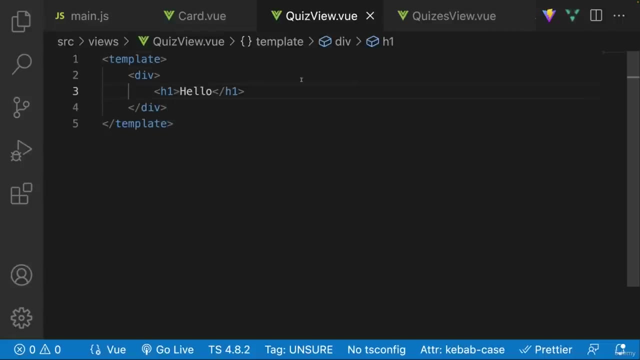 being presented there so what we can do to fix this is to go over here let's just create a quiz view dot view and for now we'll just have a template a div an h1 that says hello very simple stuff here 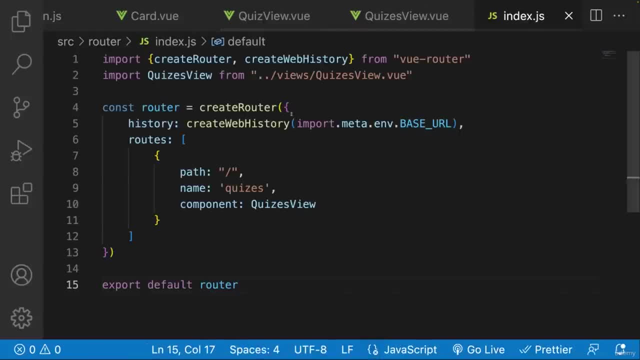 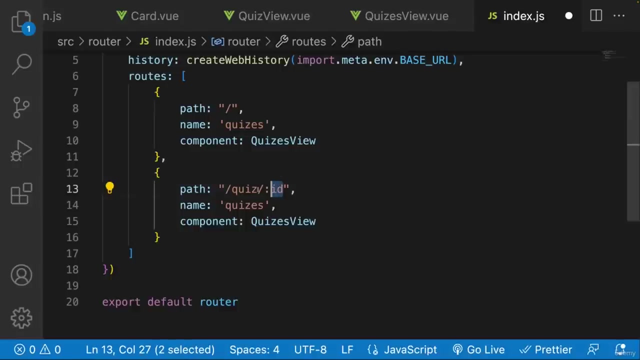 and then what we're going to do is we're going to go to our route file right over here we're going to add a new rule so we're going to say whenever you go to slash quiz and then slash that particular quiz's id and that's what we're going to call it the id is going to be the variable name for that path and this over here we're going to say the name is quiz and what we want to render let's just import this so we want to render the quiz view 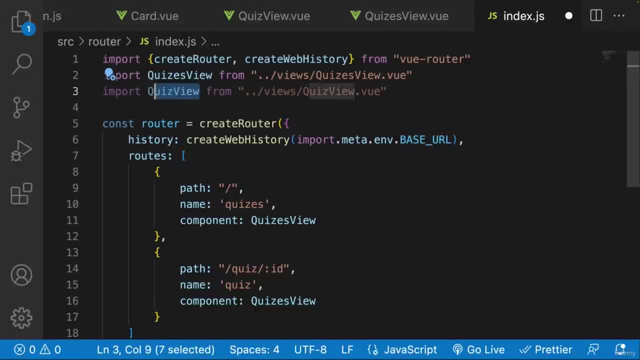 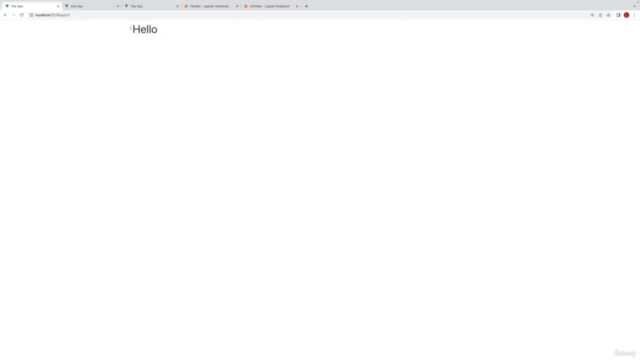 we're going to get that from the quiz view dot view and that's what we want to render so if you go here we'll render this so if you click you see we get hello of course eventually we're going to modify this page to look like this all right everybody welcome to a brand new section now in 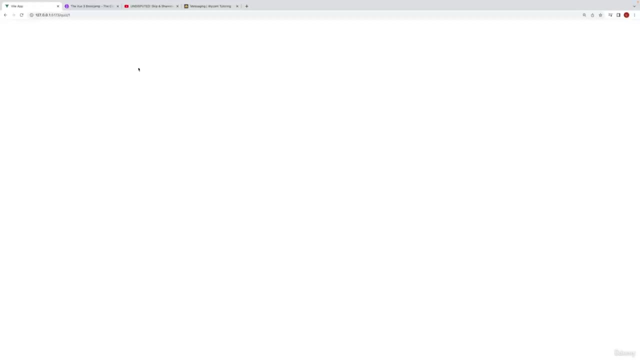 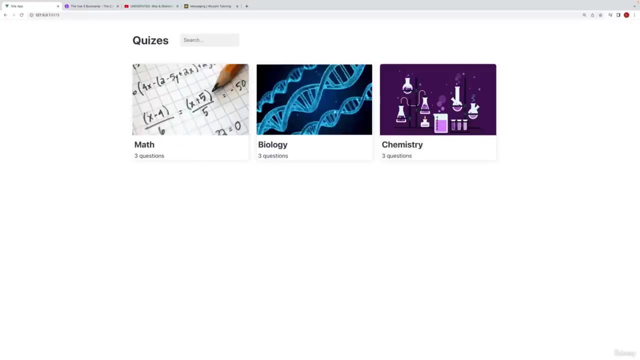 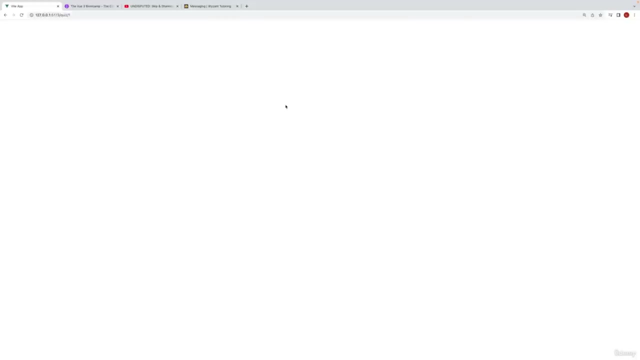 this section we're going to kind of complete our application by building out the quiz page so again we just worked on this in the last section but if we went over here we go to our quizzes and if we were to click on a particular card it's going to redirect us to the slash quiz slash quiz id page now of course right now there is no html as well as css so that is what we are going to tackle in this video we're just going to write the html as well as css for our application now as per usual if you are not interested in writing the html as well as css and you kind of just want to dive straight into the view 100 completely fine we're not going to be tackling any view in this lecture so what you can do is you can actually skip this lecture and just download the source code attached to this lecture and you can just utilize that however if you do want to write the html as well as well as the css then continue on but again you're not going to be missing it out on anything if you skip this lecture and just download the source code 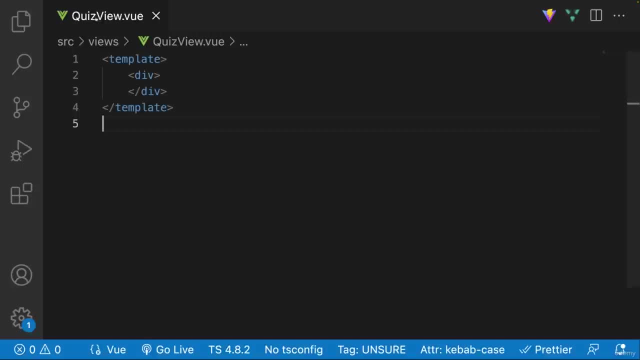 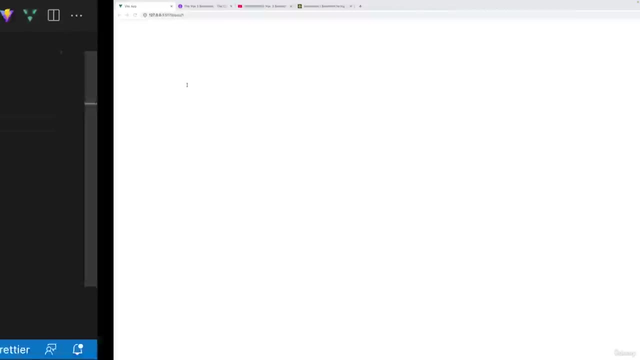 all right so let's go ahead and let's move into our quiz view because this is where well we're going to have our html as well as our css for that particular page so what i'm going to do first and 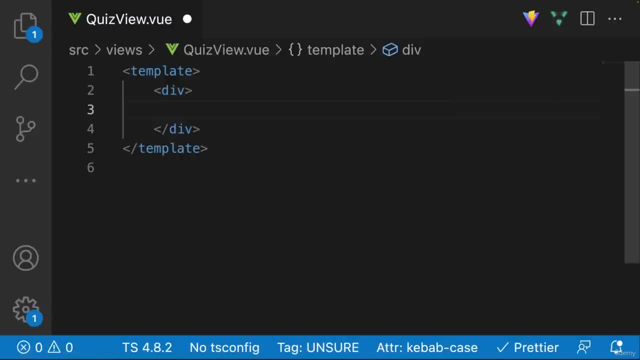 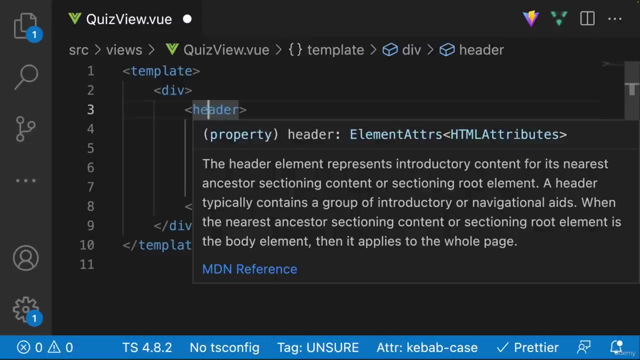 foremost is i am going to add a header let me just zoom in just a tad bit so we're going to add a header and inside of this header we're going to have an h4 and we're going to have a question and this is where we're going to have the question status so it's going to be something like question three of one you're on the first question and then you're going to have the question status out of three questions and then we're also going to have our bar so we're going to have div we're going to give it a class of bar and then we're also going to give it a class of completion and this is just kind of going to be the completion uh status of our bar and then we'll talk about that we'll see the styling a little bit later don't worry all right so now that we have our div let's just go ahead and actually style this first so that's the very first thing that we're going to style 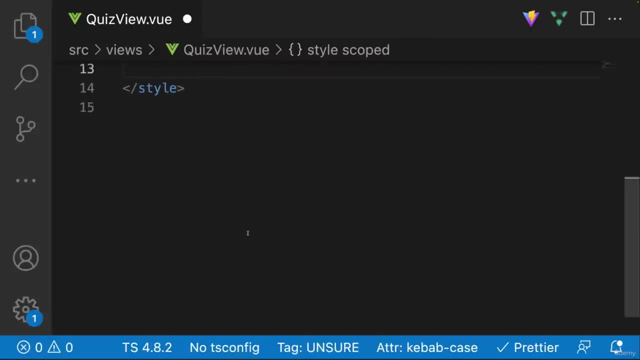 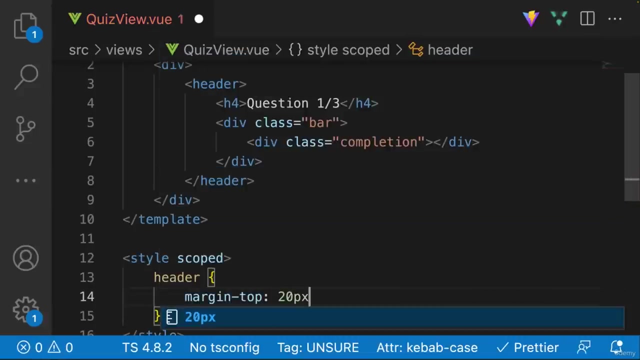 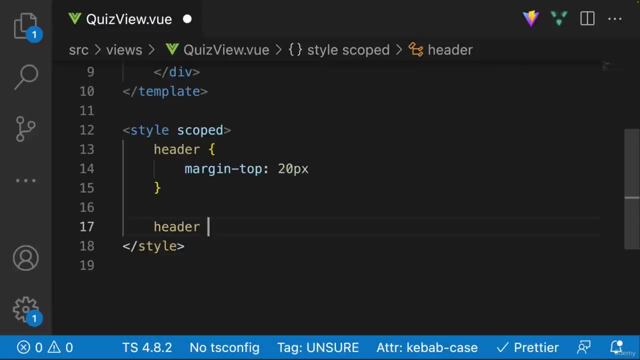 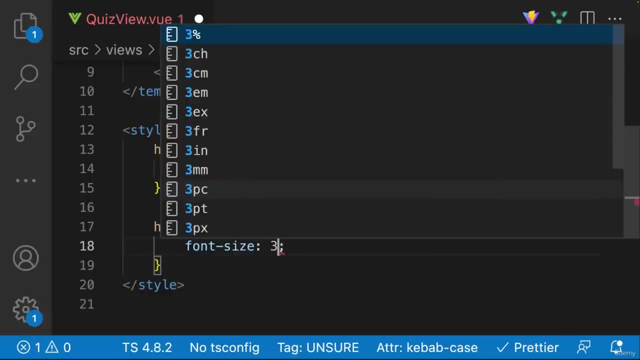 so let's add scoped here and let's go all the way to the bottom and let's just begin by styling the header so the header itself is just going to have these styles of margin top of 20 pixels and of course you can always take a look at it looking pretty good i think the h4 is a little bit too small so let's just do header h4 and then we're going to say font size and we're going to say that the font size of this is 30 pixels looking great looking great all right so that's pretty 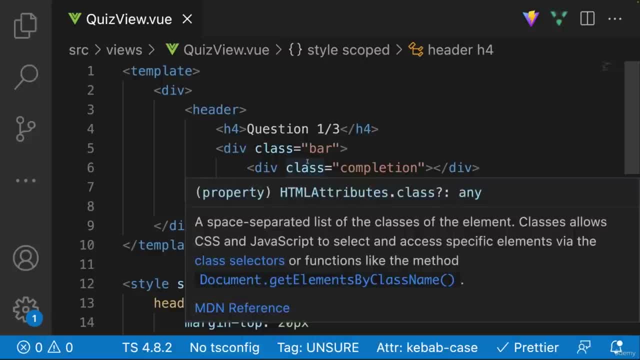 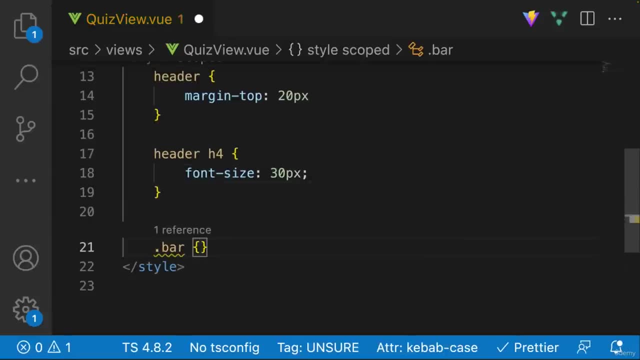 much it for that let us now move on to styling our bar so let's go over here i'm going to say dot bar we're going to give this a width of 300 pixels we'll give it a height of height of 50 pixels 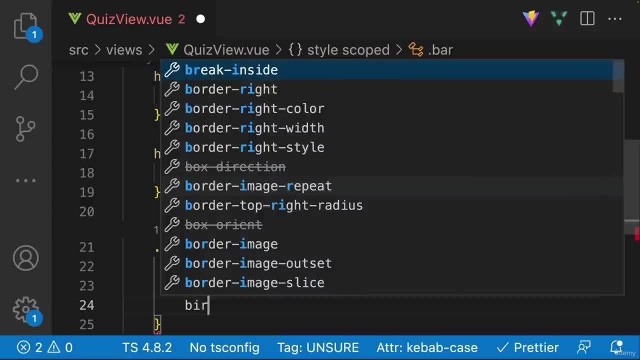 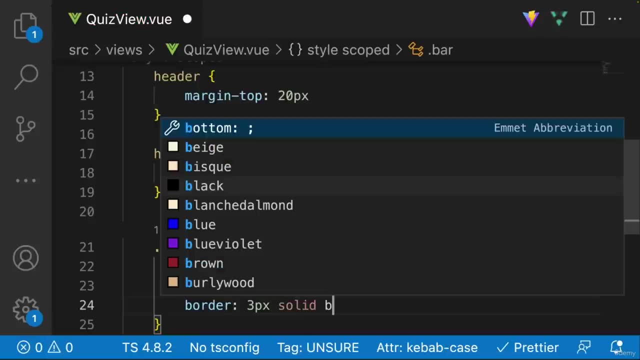 and lastly let's give it a border so we're going to give it a nice little border of three pixels solid and then we'll give it this color whatever this color is i don't really know but we'll give 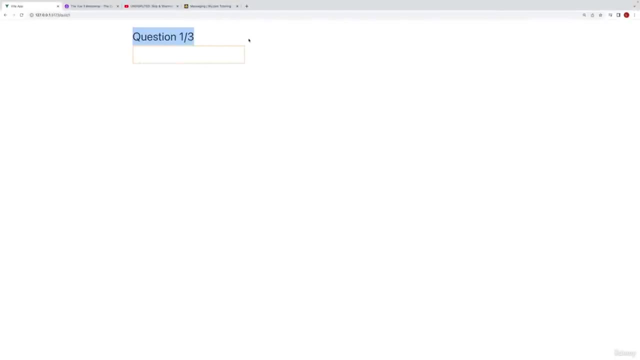 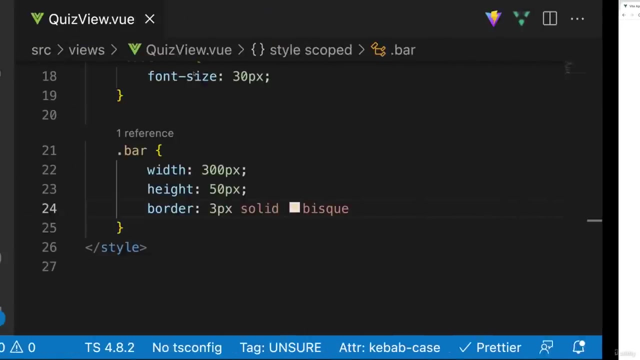 it that color so now you can see we have our uh our uh status right over here as well as the bar so this is actually looking good now let's actually style the completion div so the completion div so 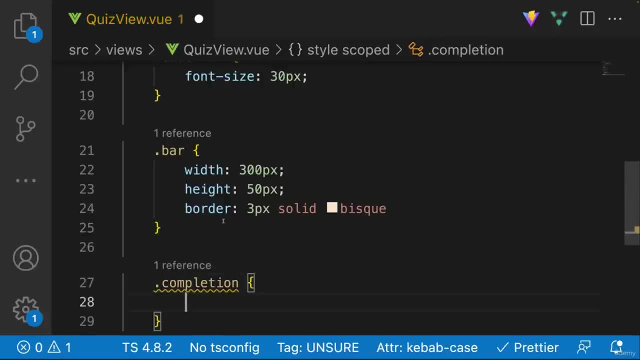 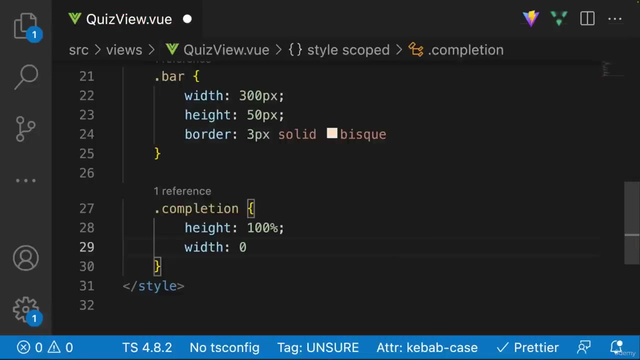 we saw that's going to have a we'll we'll give it a height of 100 so height of 100 and we're going to give it a width initially of zero percent and lastly we're going to give it a background color of we'll give it a background color of the same color 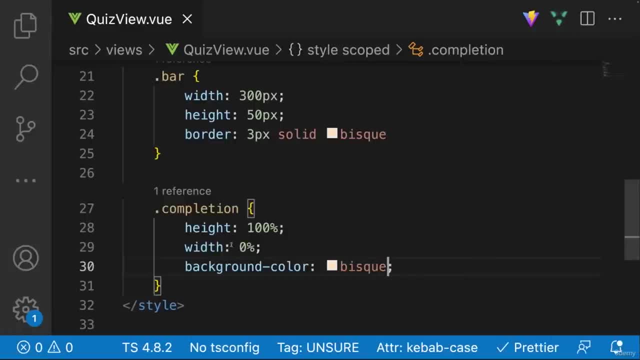 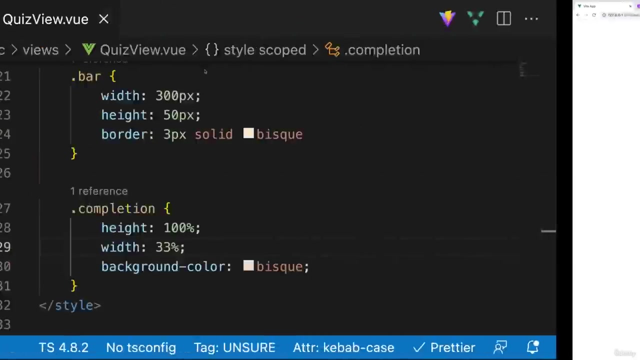 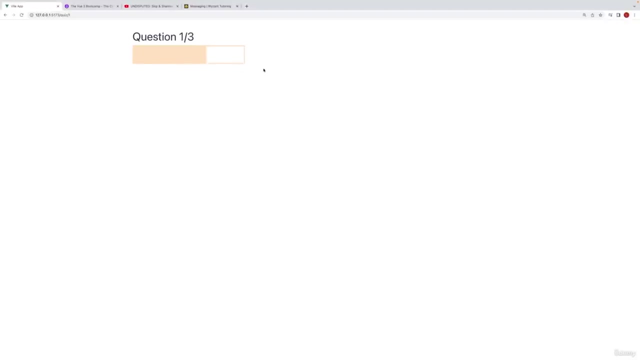 so now of course if you go there you can see that there's nothing changing however this one we're going to actually manipulate with our javascript depending on the status so if we finally answered the very first question then this is going to be something like 33 and it's just going to be dynamically changing like so so if i answer the next question then it's going to be 66 like so and then it's just going to keep going until it's completely full and i finished the quiz but for now we're just going to leave it at zero but then programmatically 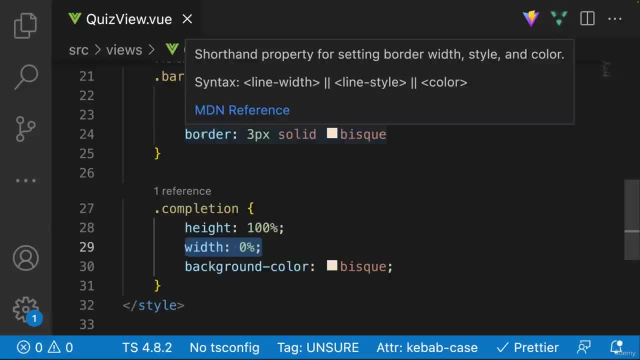 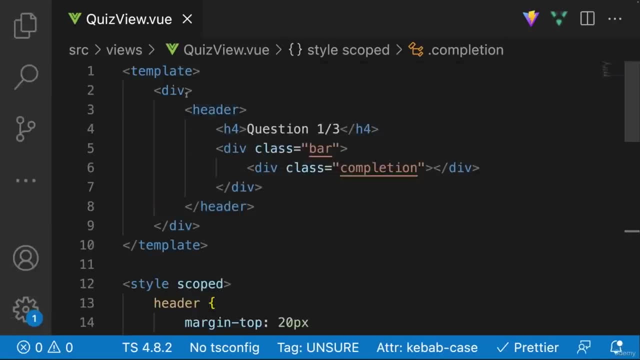 we're going to change these styles all right so i think this is actually looking pretty good i think this is a okay let us now move on to the question portion of this uh of this of these 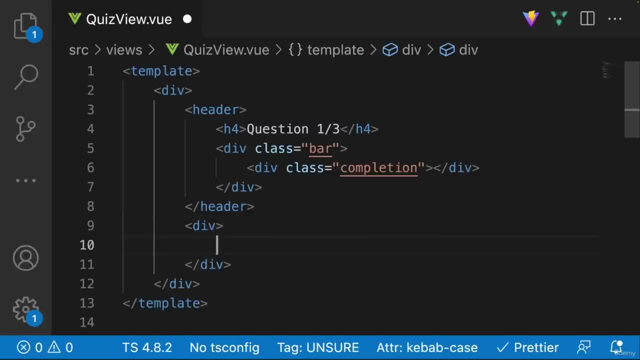 styles so let's add a div here and right in here this is where we're going to have all of our different questions now later on we're actually going to kind of just separate our stuff out in components but for now let's just write the h tml for the questions themselves so i'm going to go here i'm going to create a class and i'm going to call this question container so question container and this is going to have an h1 with a class of question and of course this uh is something the value of this we're not going to hard code but for now we'll hard code it so we'll just say what is the what is the chemical value 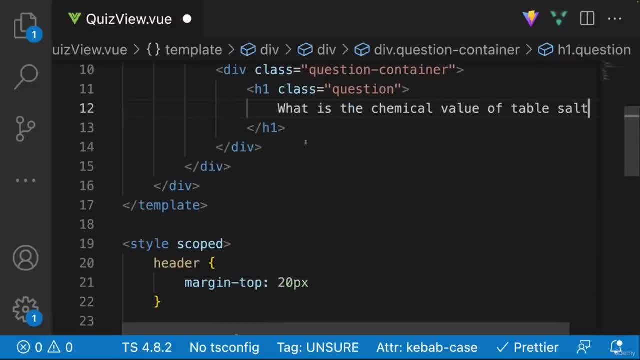 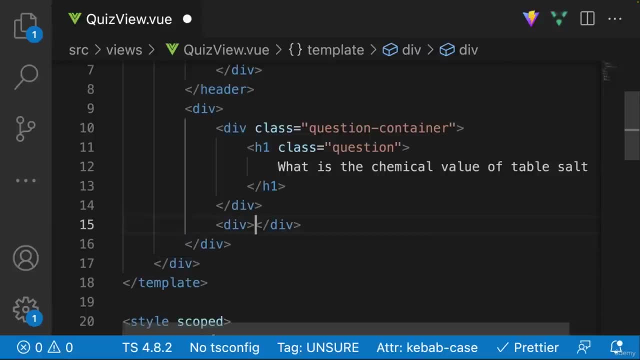 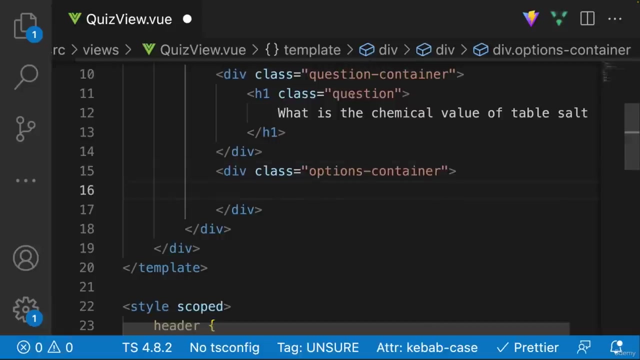 of table salt so this is like a chemistry question again later on we're gonna kind of remove that all right so that's what we have here then let's have a div and what we're going to have is so this div is going to contain all of the different answers and just for documentation purposes we can also say answers container answers container like so okay so over here what we can have is all of the different options or maybe we can even call this options container that probably makes more sense so these are all the different options that we can possibly pick for this question 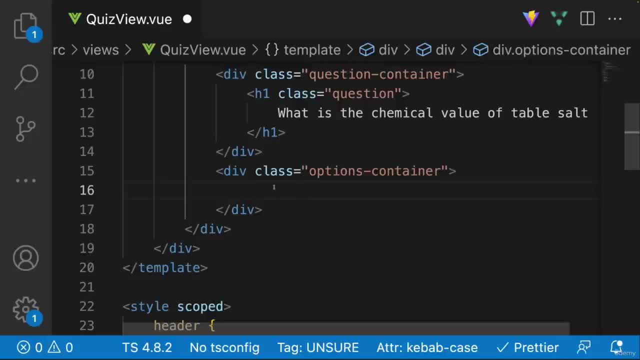 because this is going to be a multiple choice uh quiz all right so let us uh add a div in here so this is going to be the option and eventually we're going to want to v4 over this depending on 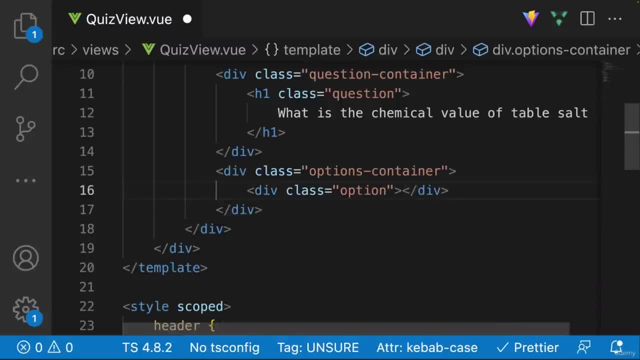 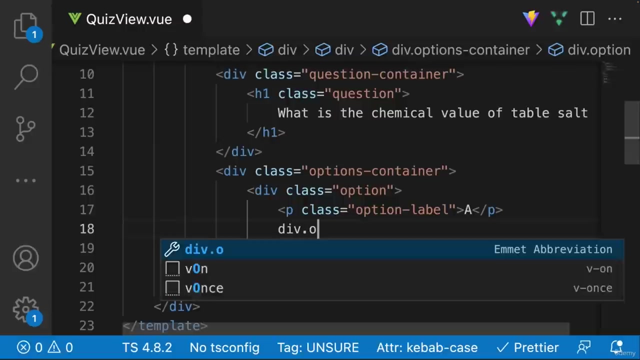 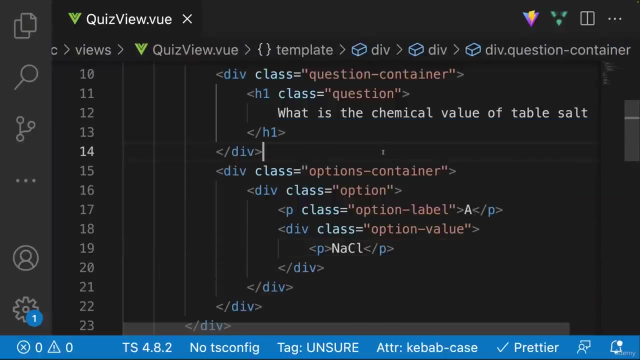 how many options we have which in our case will always be always be four so we're going to have our option and then within it let's have a paragraph tag that is going to have the option label and the option label over here and this one is going to be a b c or d and then let's have another div we're going to give this the option value like so and then within this div let's have a paragraph tag that has the value itself so n a c like so all right so this is looking pretty good if i were to go here you can see obviously 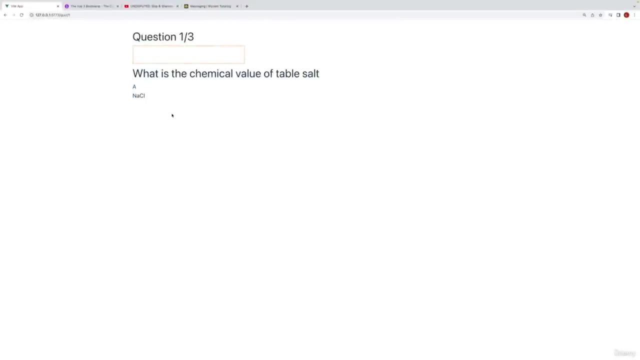 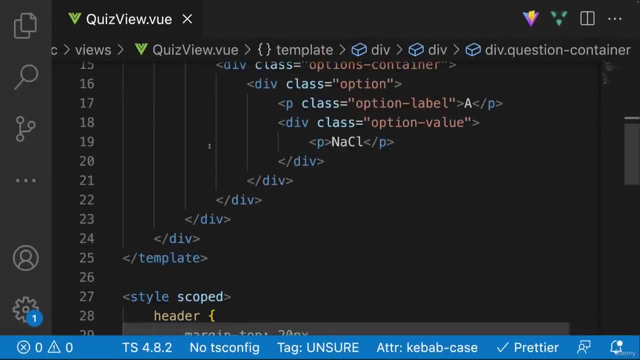 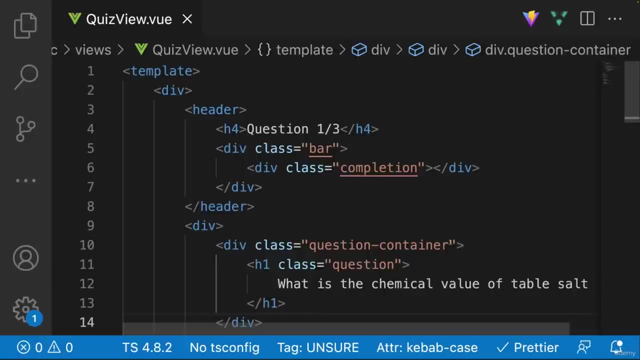 stylistically not the greatest so let's work on uh styling our application first and then we can move on so let's go over here and the first thing that i want to style is probably the question so let's go here to the question container actually let's grab the question container and i am going to give the question 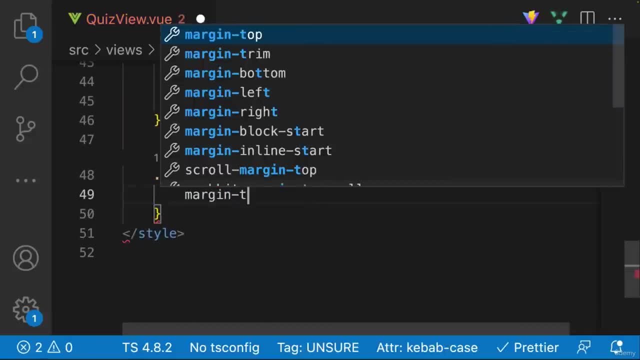 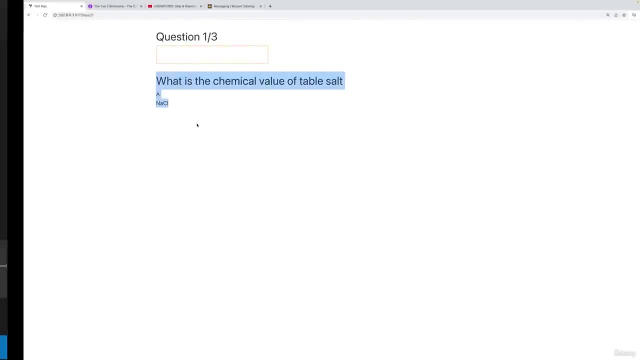 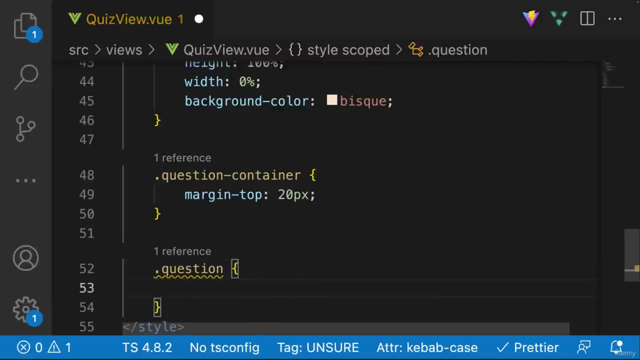 container a margin top of let's say 20 pixels just so we can have some spacing between the status as well as the question itself now over here let's now style the question so the question itself which is going to be the header we'll give that a font size of 40 pixels and we'll give it a margin of 20 pixels and we'll give it a margin of 20 pixels and we'll give it a margin of 20 pixels 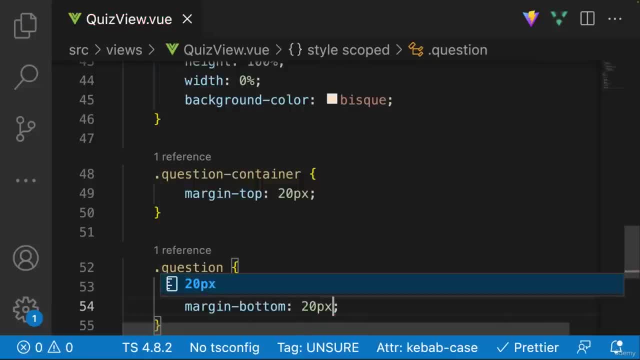 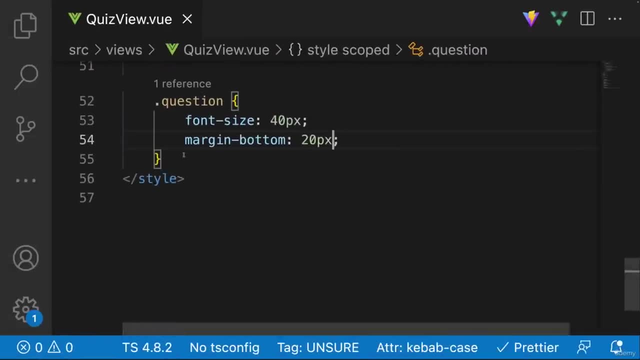 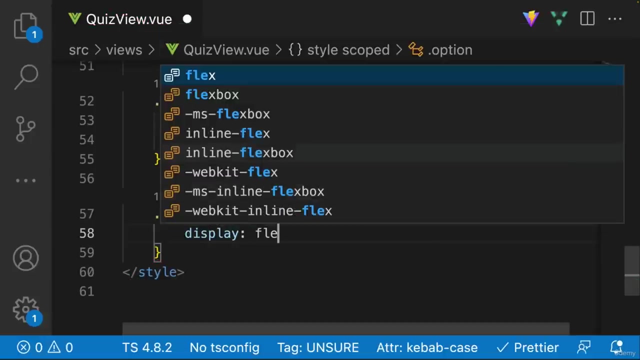 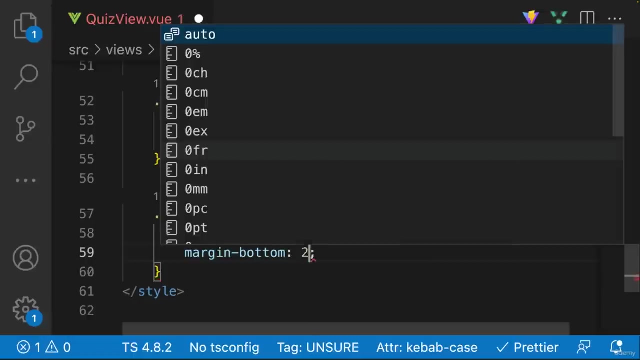 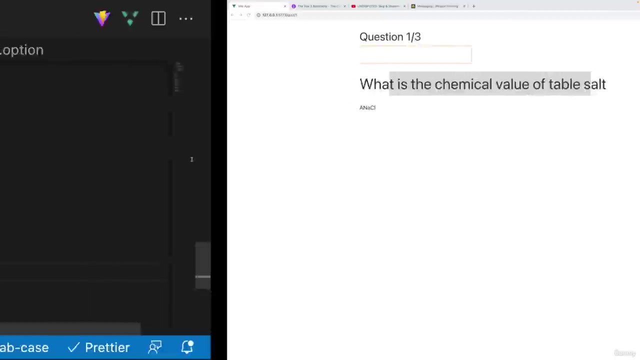 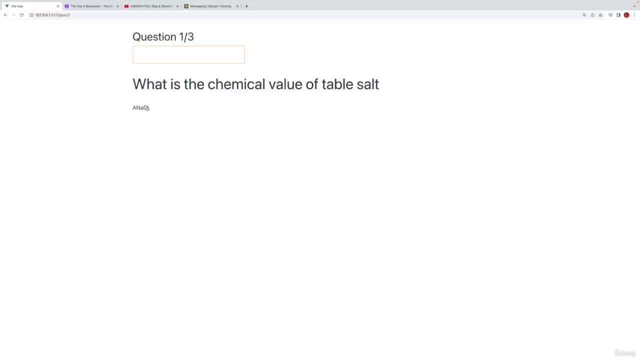 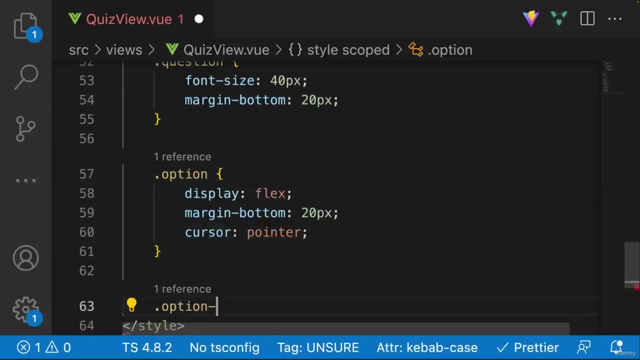 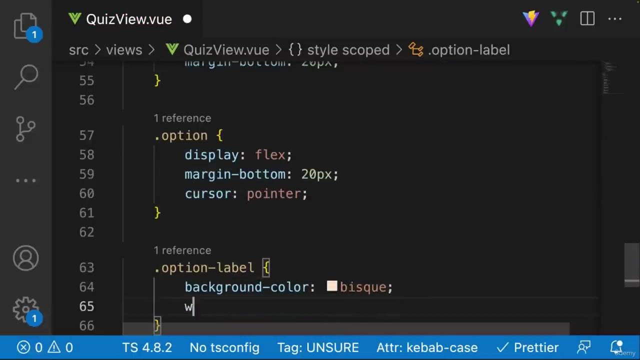 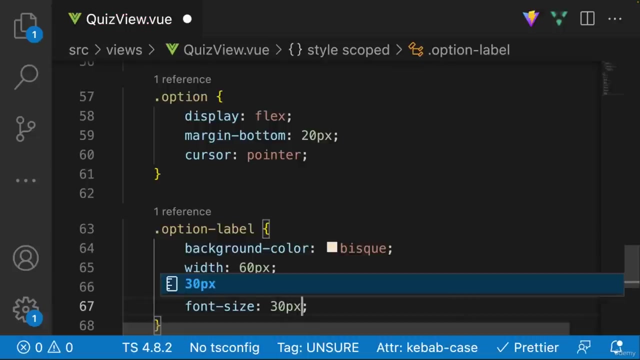 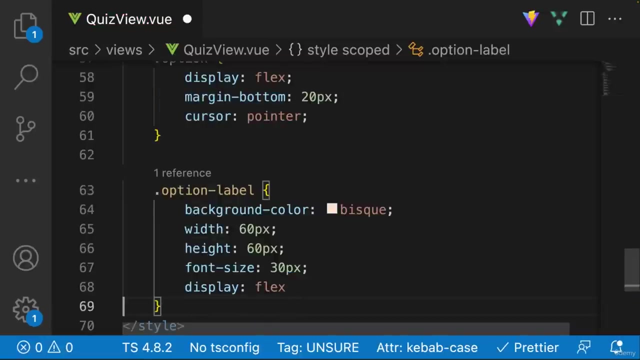 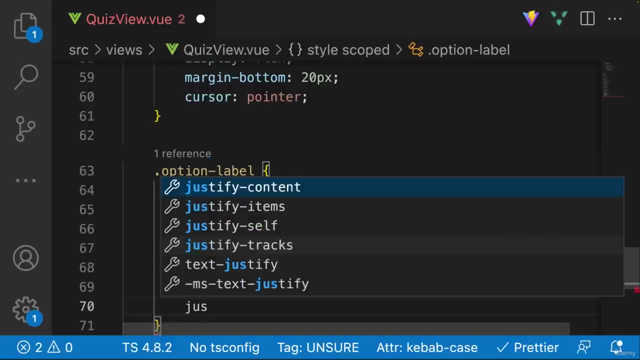 margin bottom of 20 pixels there we go looking pretty good and now let's style the option so it's not really much styling we have to do for the option so we can say option like so and we can say display flex for the option and we're going to say margin bottom and this one's going to be 20 pixels and then we're going to say cursor pointer like so and then we're going to say margin bottom like so cursor pointer all right so looking good oops sorry about that guys my uh my machine is beeping for some reason all right so there we go and now let us style the option label so the option label is going to have a background color of the same background color that we have been using we'll give it a width of 60 pixels a height of 60 pixels and then we're going to style the option label so the option label is going to have 60 pixels we'll also give it a font size of let's say 30 pixels uh we'll also give it a display of flex and we will give it an align item center and lastly justify content center looking good 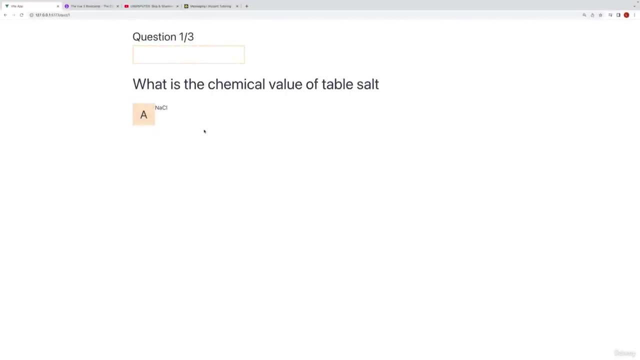 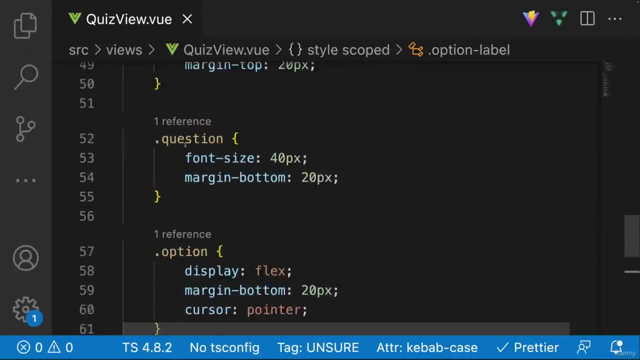 all right so this is going to be one of our options here and you might honestly i think this is a little bit too big maybe we can say 50 pixels so over here that has okay i think it now is completely off all right there we go so now we go we have this option so now all we got to do really 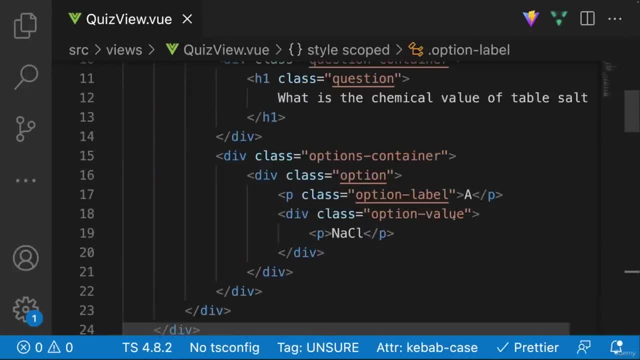 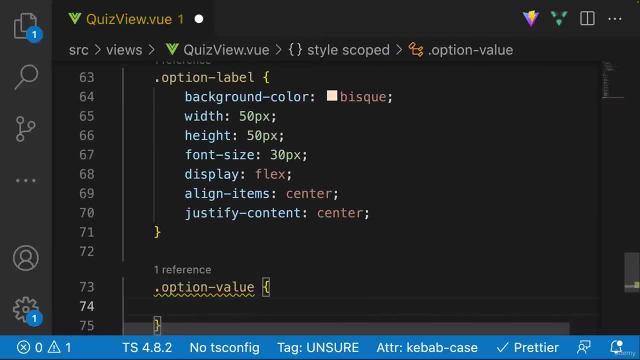 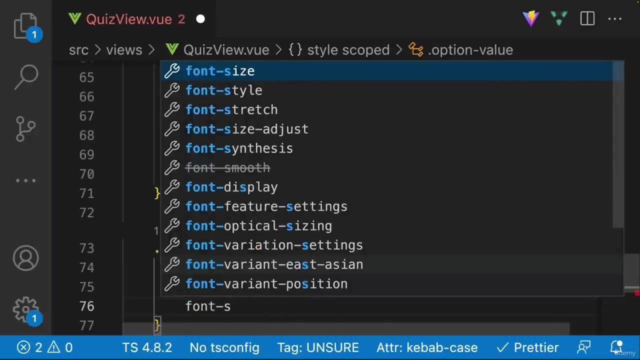 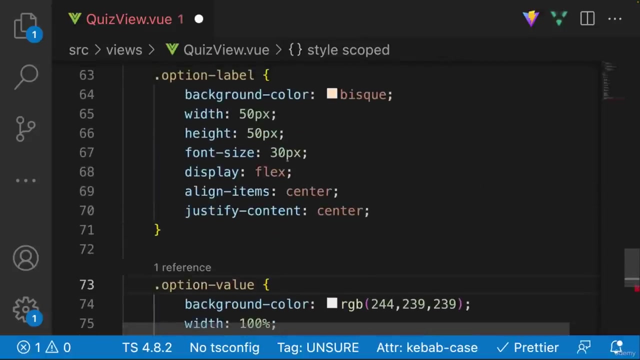 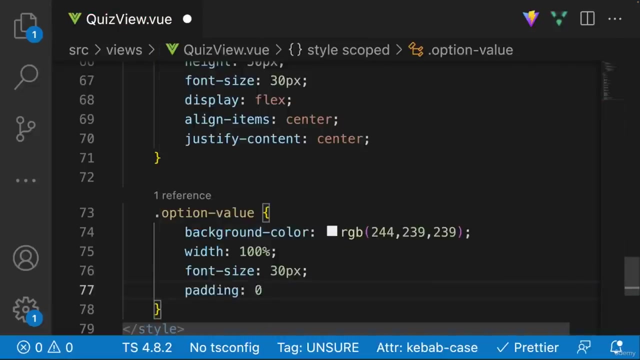 is style this over here which is going to be the option value so that's the last thing that we really need to style so we're going to give this also a background color this one's going to be an rgb it's going to be kind of like a whitish grayish color so let's do two four four two uh three nine and lastly two three nine as well and then we're going to give it a width of 100 and a font size of let's do exactly the same amount of pixels we did here so we'll just say 30 pixels so let's say 30 pixels maybe we'll make it a little bit smaller and lastly padding of zero and 20 pixels 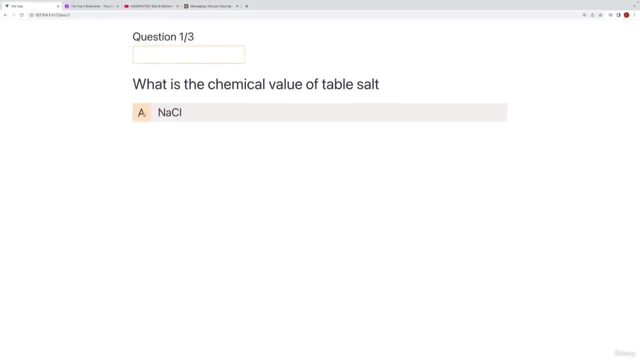 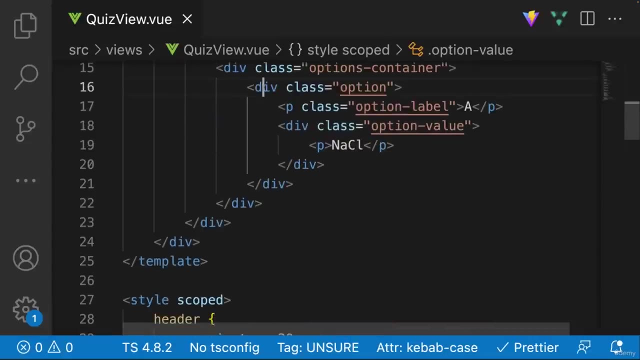 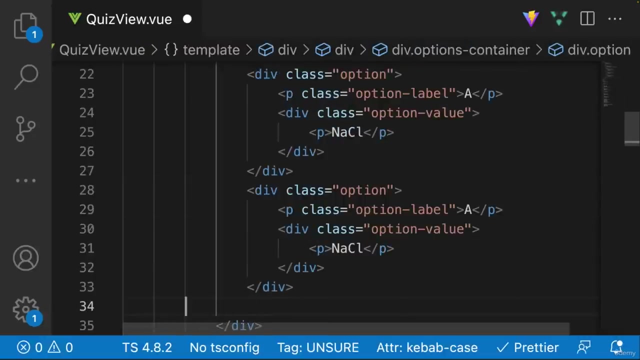 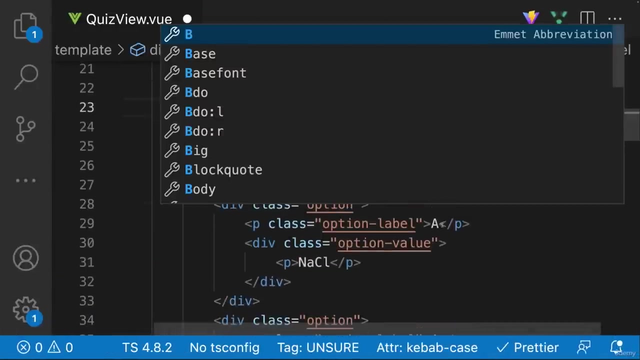 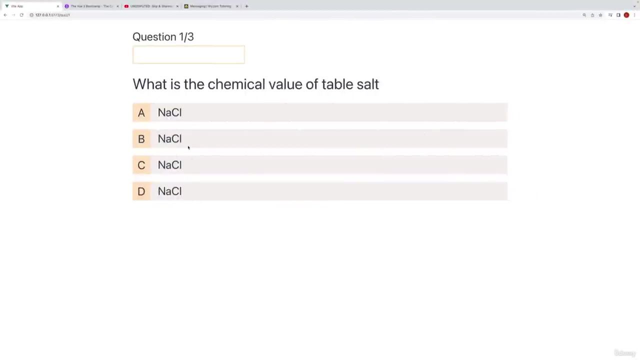 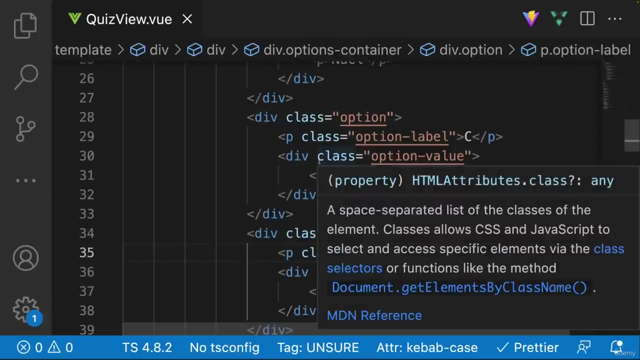 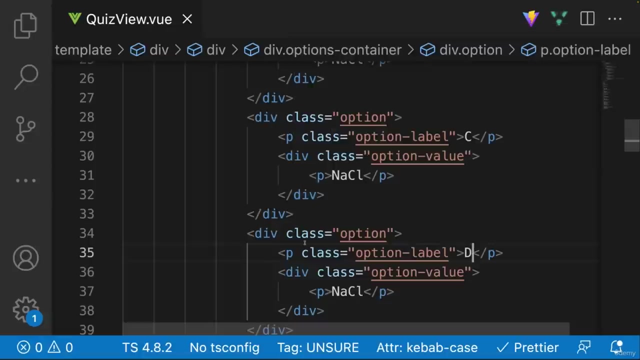 and there we go so that looks good pretty good to me to be quite frank um and that's pretty much it that's really all the styling that we need to do for our app now obviously over here for our options we're going to have multiple different options so it's going to be an option here an option here an option here it's going to kind of look something like this and of course this is going to be b c and then d and then obviously the value values are going to be a little bit different but this is something that we're actually going to v4 over so i think we actually got a good template but now let's let's start doing some of the stuff that we have been doing uh like separating our stuff into components as well as uh you know 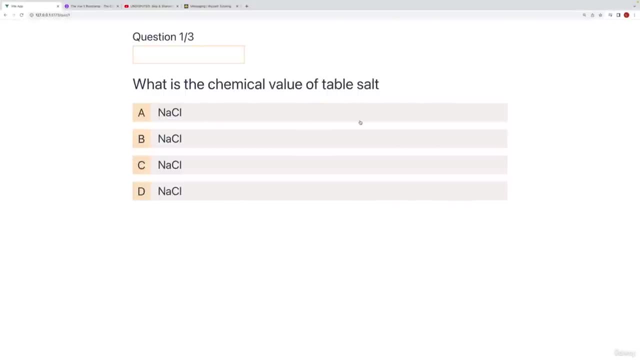 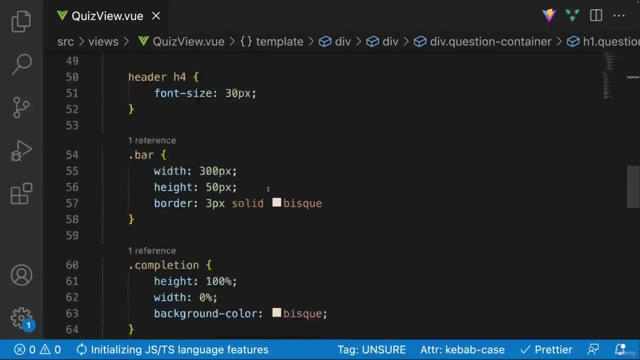 utilizing v4 to iterate over our data whether you wrote out the code with me or you just downloaded the boilerplate your quiz 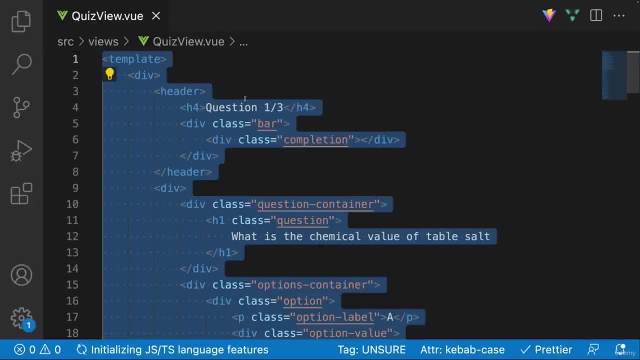 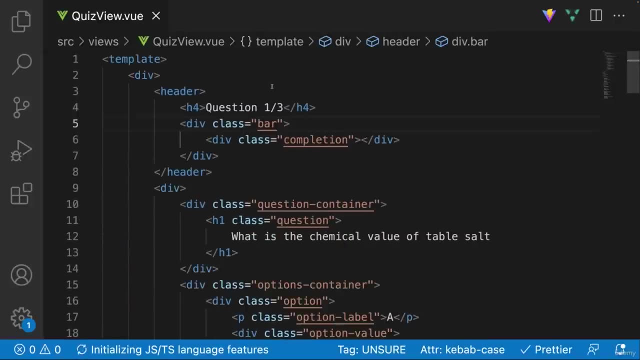 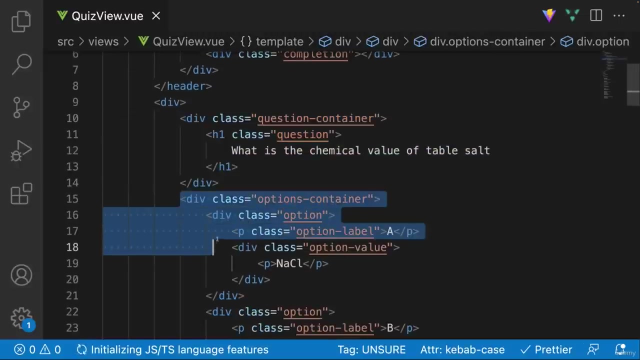 dot view file should look a little something like this now in my opinion this is kind of getting a little bit bloated for my liking and when things get a little bit bloated the best thing that you can do is start separating them into their own components now specifically actually what i want to do is separate this right over here so the question header as well as the question options into their own components so this part over here should just be its own component 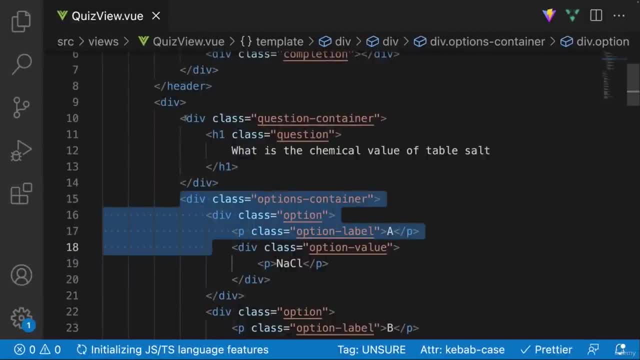 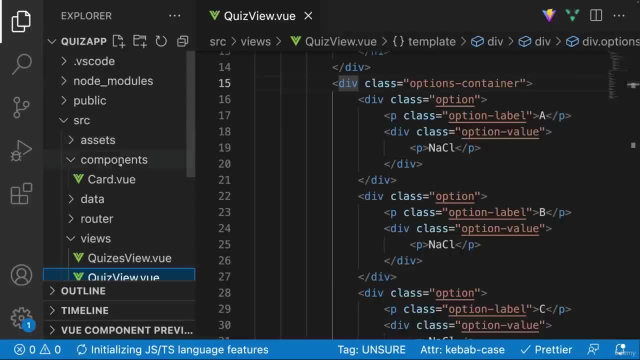 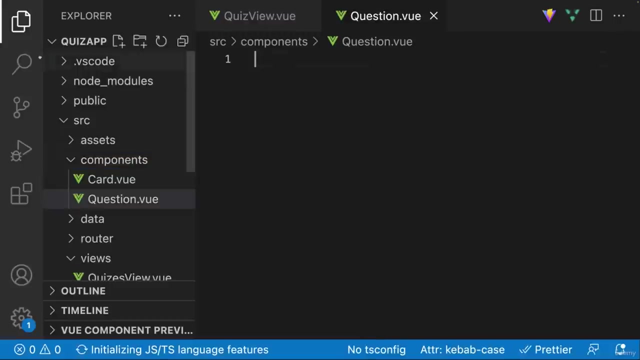 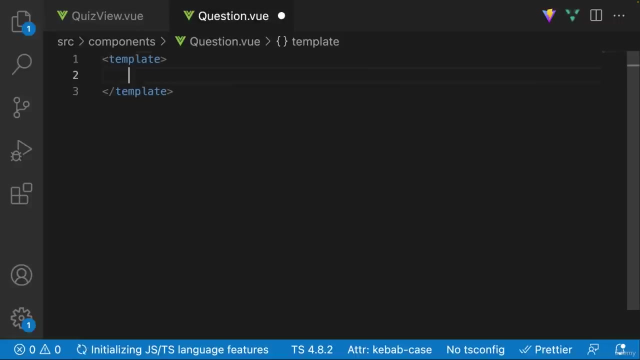 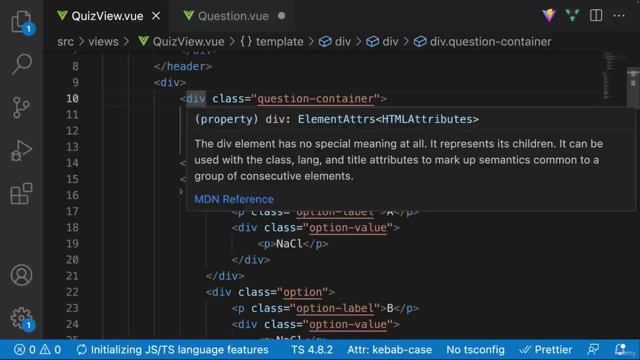 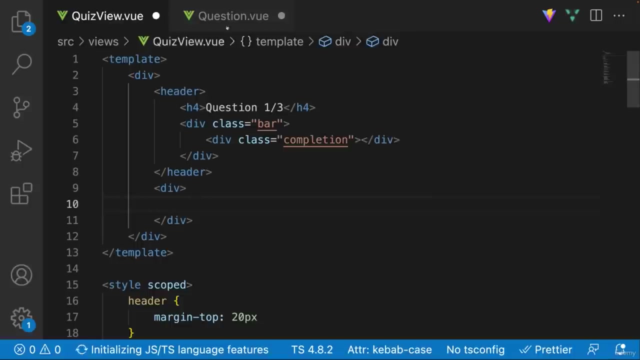 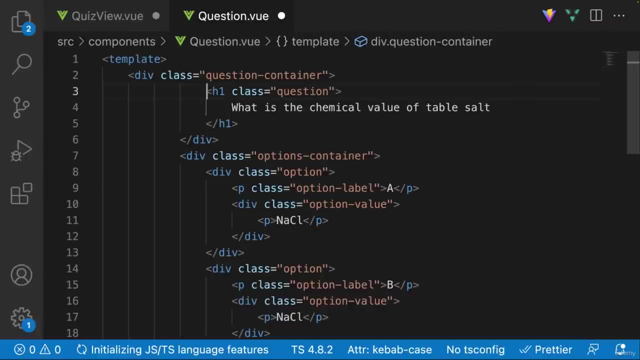 and then from here we just go ahead and pass in the data that we need to so let's actually go ahead and do that so what i'm going to do here is i am going to create another component and i'm going to call this question because this is really just a question uh that we are uh well the html is just basically a question at this point so what i'm going to do here is we're going to say template and then i am going to copy this as well as the so this div right over here as well as this div we're going to copy both of them and we're going to cut them out and we're going to paste it right in here and we can fix some of the indentation of course you can probably use a format on save to do this but i don't have that 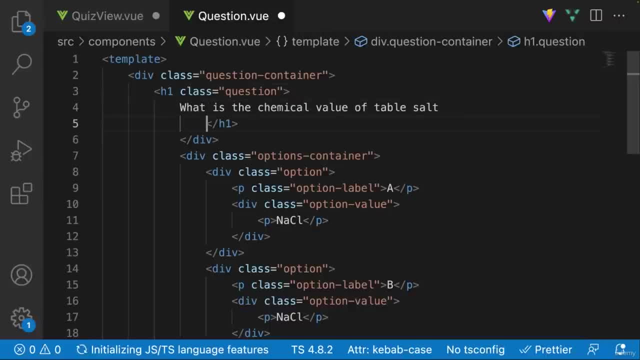 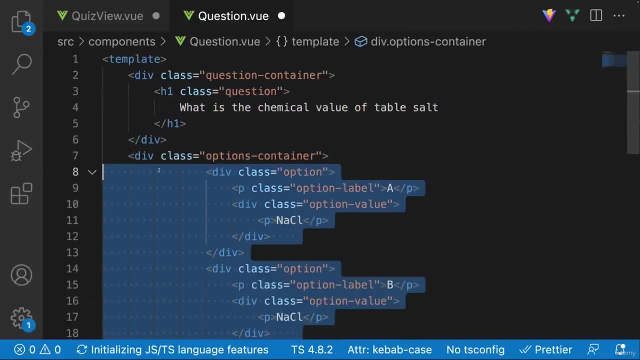 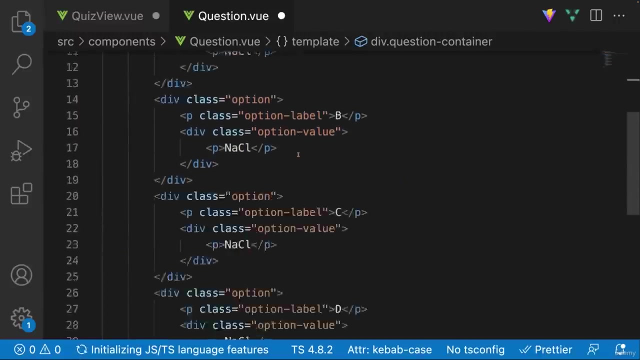 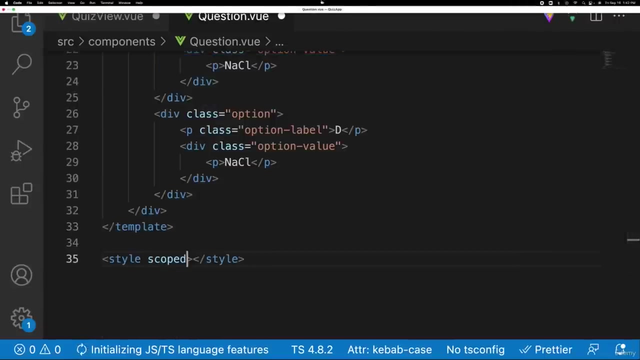 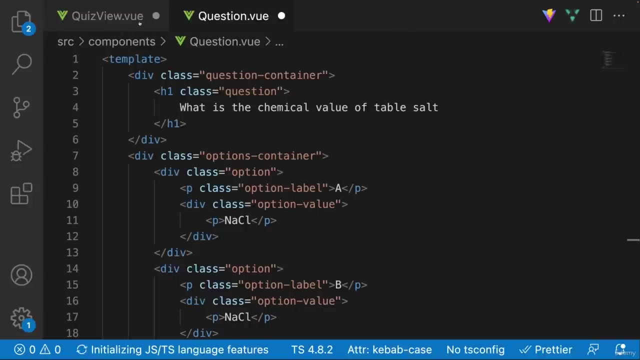 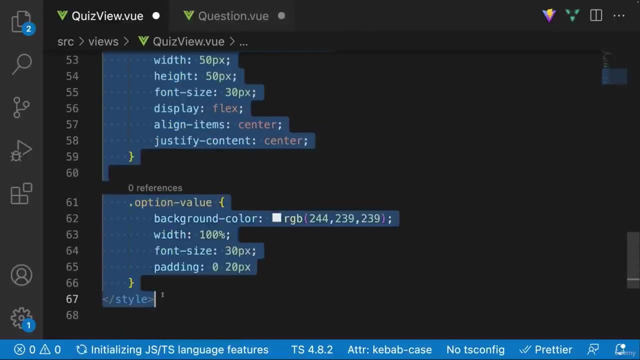 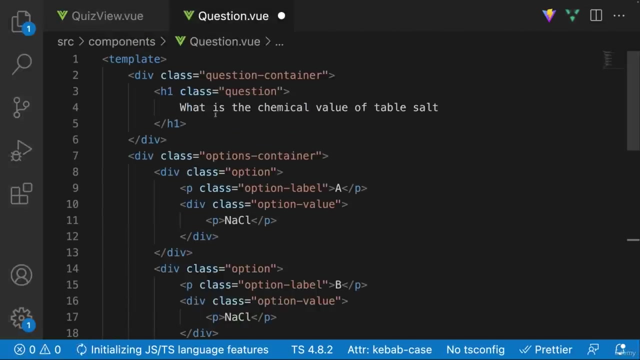 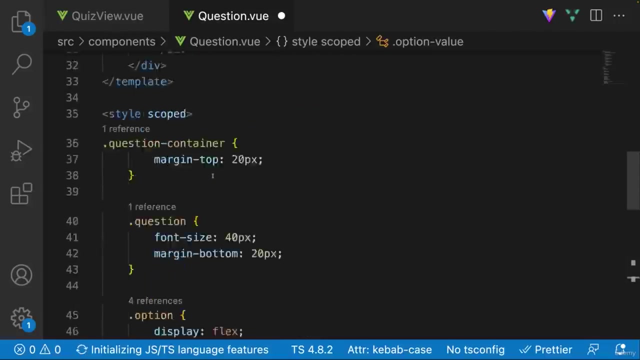 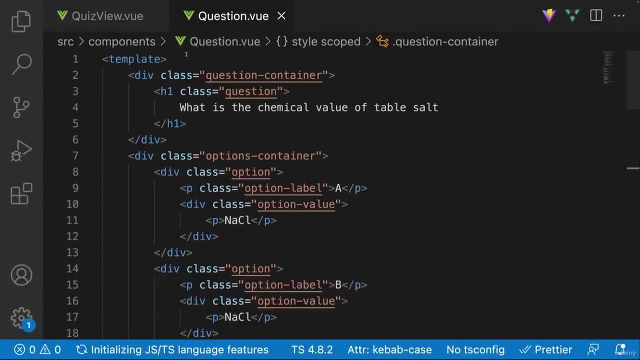 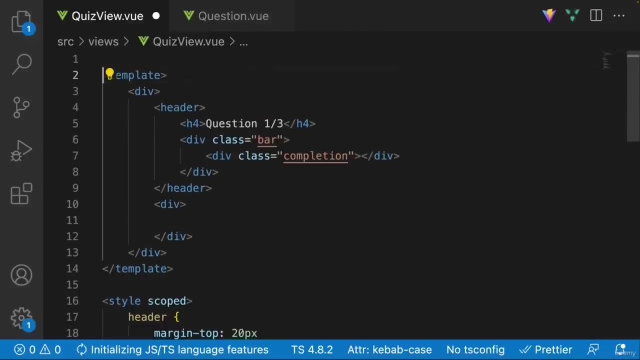 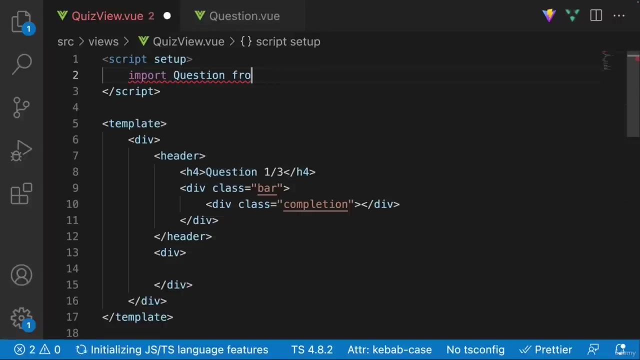 set up for view so i'll just fix it out myself manually not the best process but oh well let's fix out some of that indentation uh and what we can actually do now is we're going to go ahead and now so we fix this this this i'm just going to go ahead and highlight everything and then just do a command and then uh square braces and there we go that's just going to fix a little bit of the indentation all right so we got that but of course now what we need to do is grab these styles so we're going to say scoped and we're going to go right over here and what styles do we need well we need the questions container question and options so literally everything right here so everything right here we're going to go ahead and cut that out and let's just save this for now so it should be kind of empty and we're going to go over here and we are going to paste that in there all right so this is looking pretty good let's tabulate that looking good so now of course we what we want to do is eventually of course use this component inside of the quiz view so this is where we want to render it because that's of course where we moved it so to do that what we're going to need to do is grab a script setup and we're going to need to do some import so we are going to import question and we're going to import that from the components directory so we're going to move into the components directory we're going to get 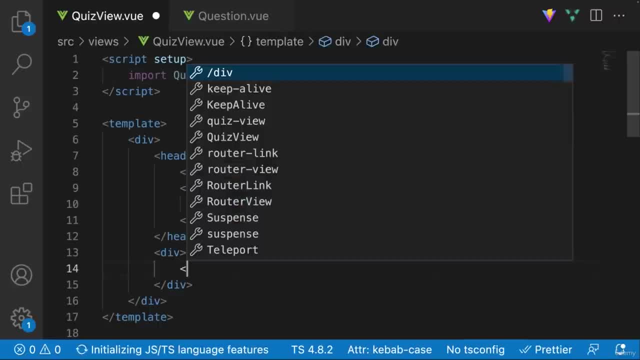 question.view and then i'm going to go ahead and render it let's go ahead and put question right over here as the components 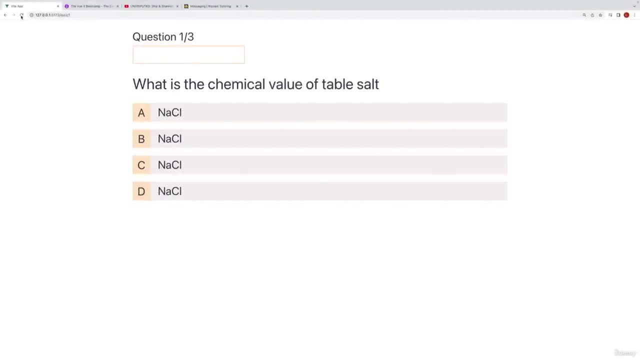 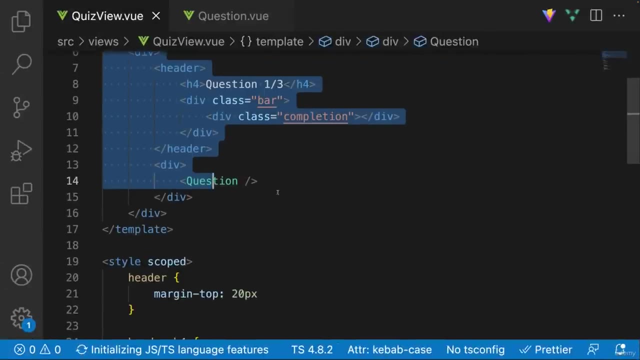 and if we were to save this you can see that everything is fine but now we have completely removed a lot of the bulk from our application over here and honestly we can also do the exact 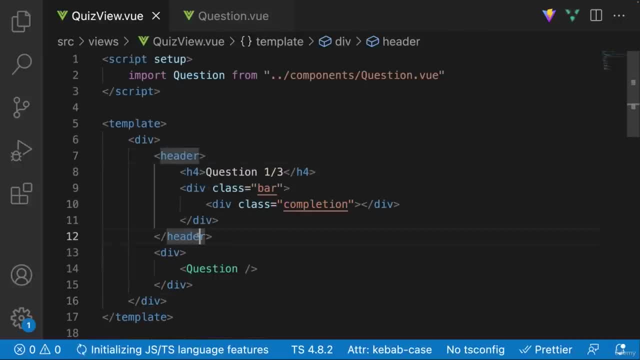 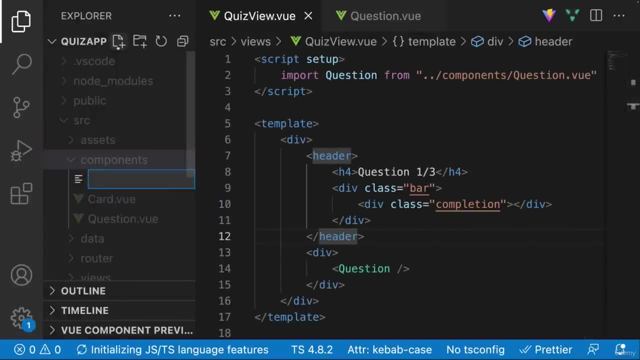 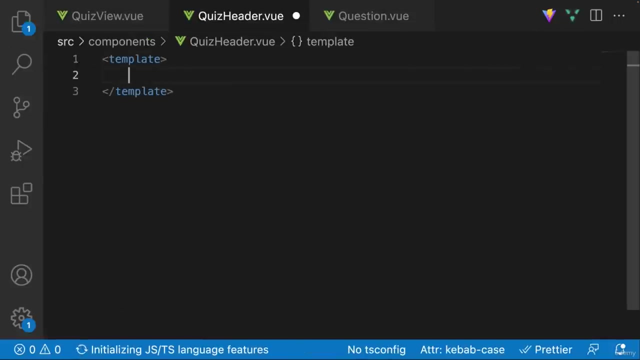 same thing with this right here with the header so let's actually go ahead and let's go and create a new component for this we're going to say quiz header dot view and this one's going to be very simple we're going to say template we're going to say oh we'll just cut what we have over here so header i'm going to go ahead and paste what we have here now so header and let's just let's just do a yeah that looks good to me now of course what we're going to need are some of these stylings so 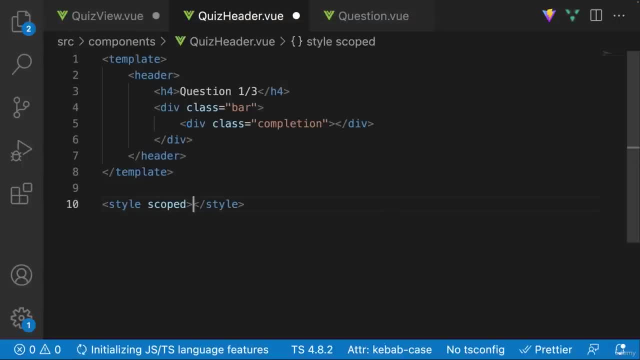 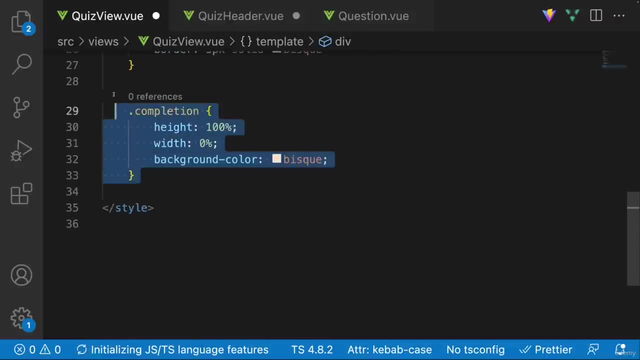 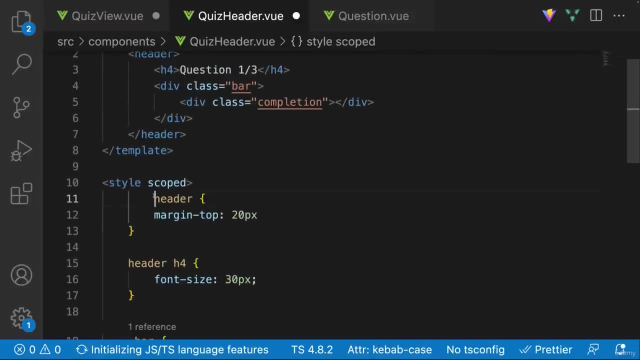 we're going to say style and scoped and we what we want to do is grab the header and then we're going to go ahead and paste that over here what we want to do is grab the header header h4 so literally there's going to be no styling inside of this file so let's grab that paste that in there let's go do that 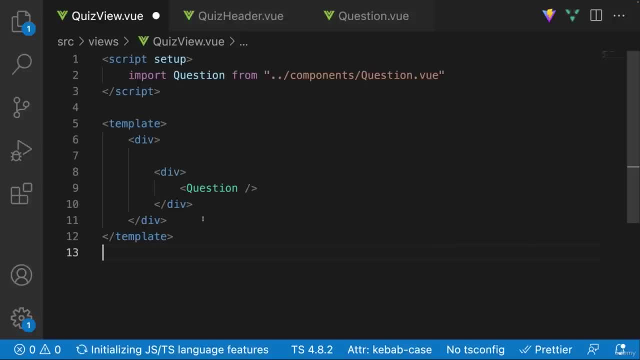 all right so this is looking good we can actually remove this style entirely and from here we can import the quiz header from quiz header dot view so quiz header dot view 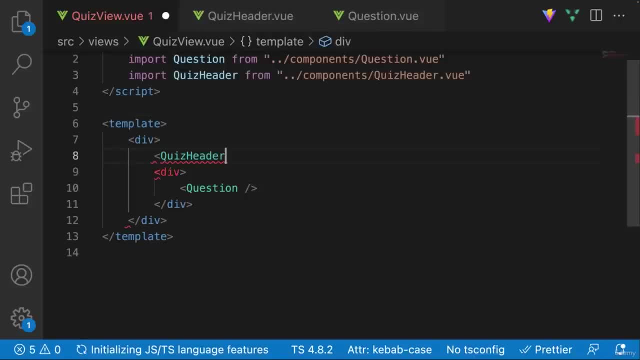 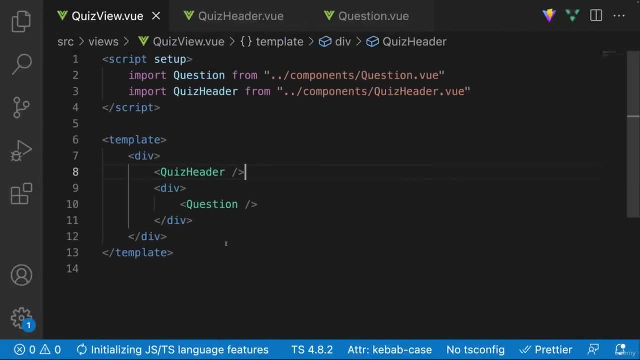 go ahead and render that right here and there we go so now we got this uh wonderful looking uh a file that is completely empty and anytime that we want to work on anything it's going to be specifically in the component itself so this is really good you might be thinking maybe we can just actually just grab these divs and just put that in there but later on we're going to actually utilize these divs to conditionally render either a question or the completion status 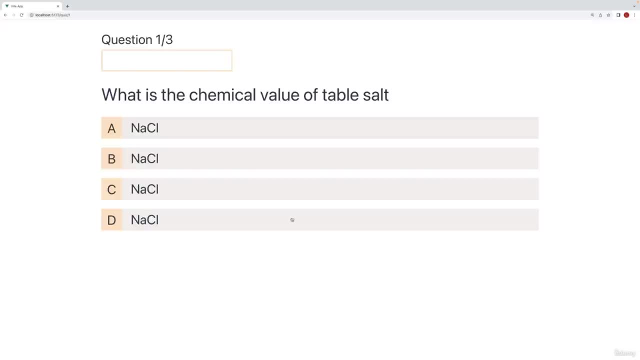 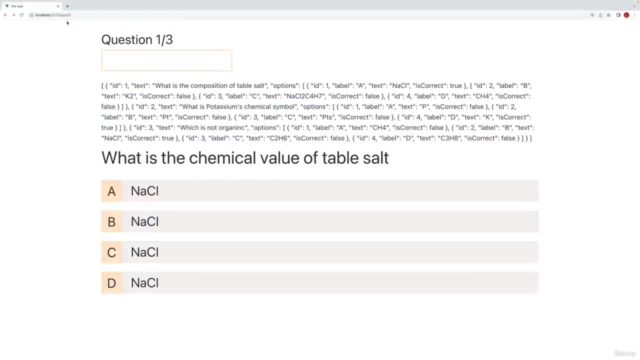 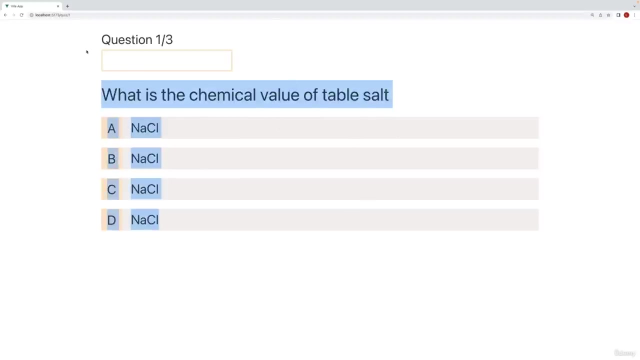 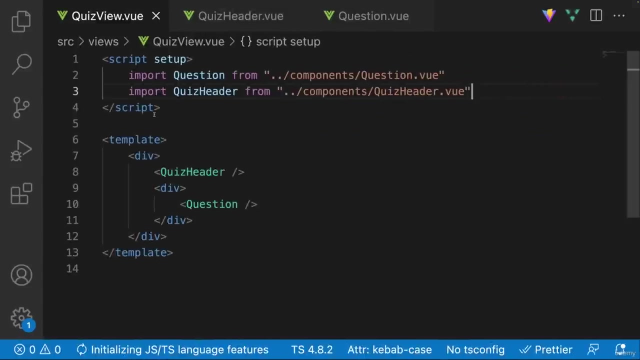 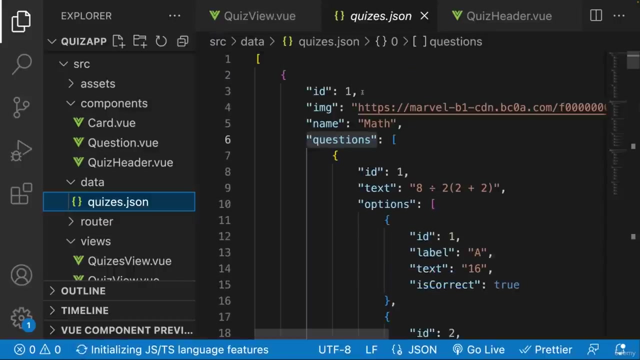 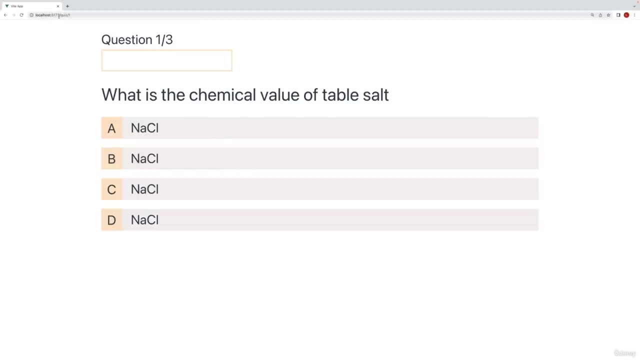 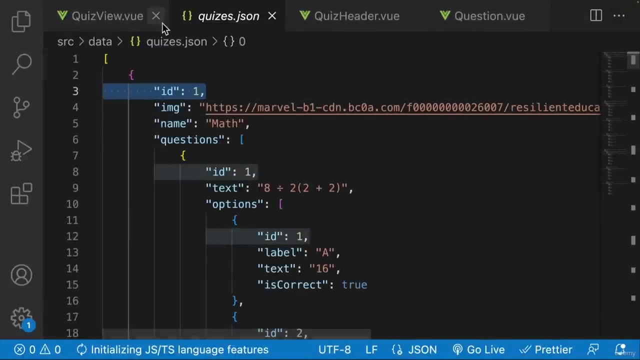 so we'll keep that div in there for now now that we got this right over here the next step of course is to show the correct questions based on the quiz that you went on so of course if you went to let's say the math quiz you're not going to want to see the chemistry quiz which of course at this point we have just hard coded so let's go ahead and actually kind of make this dynamic now as a quick reminder our data lives inside of the data and then JSON file. And it has an ID that is always going to be the same as the path right over here. So if I click on math, my path is going to be quiz slash one, and that one is going to be the ID of that particular quiz. So of course, what we're first going to need to do is extract that query parameter 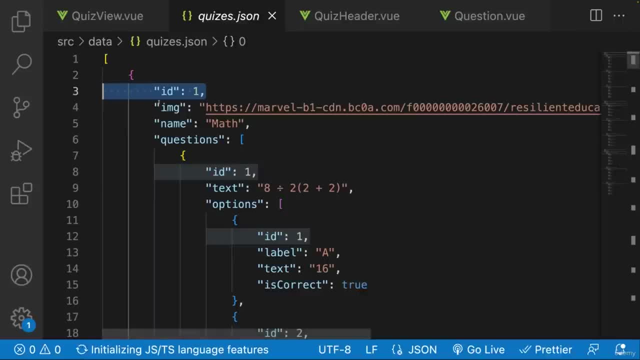 from our path, and then utilize that to find the appropriate quiz within our quizzes.json file. 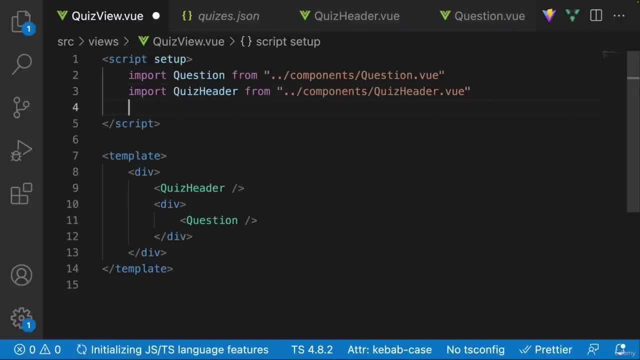 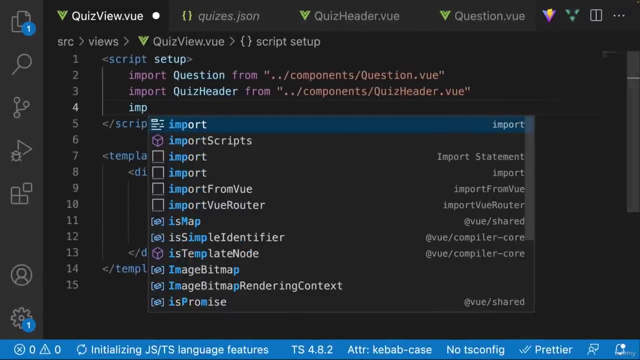 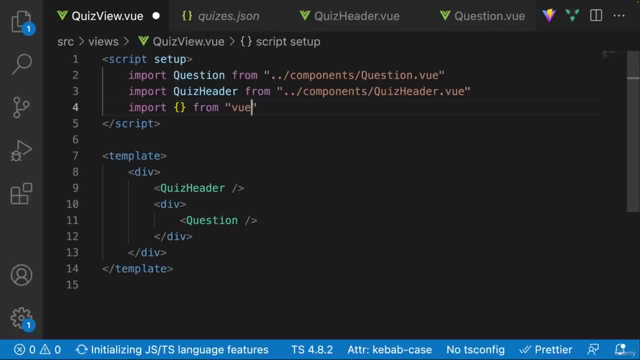 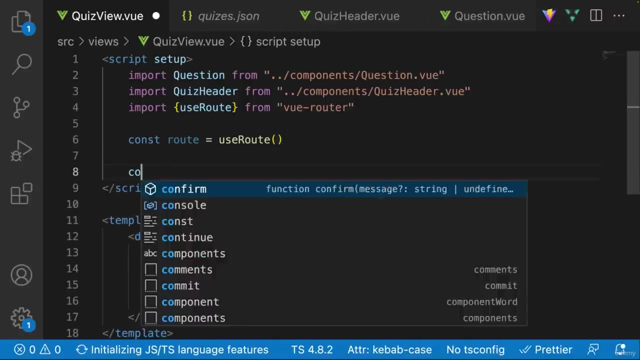 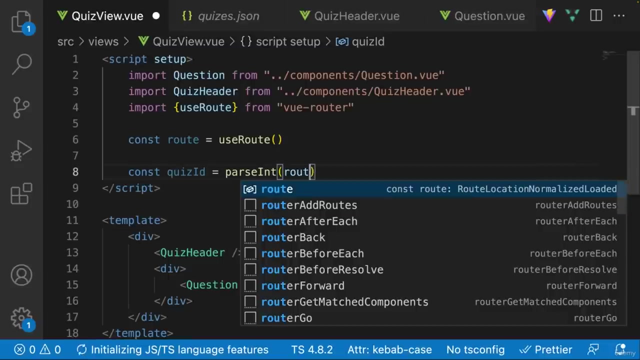 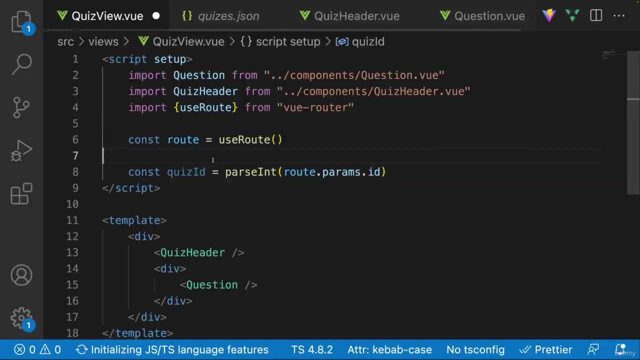 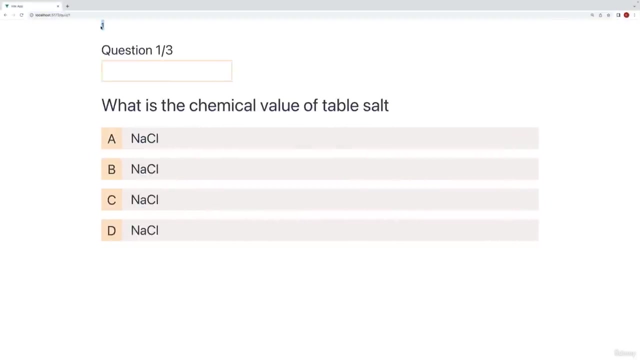 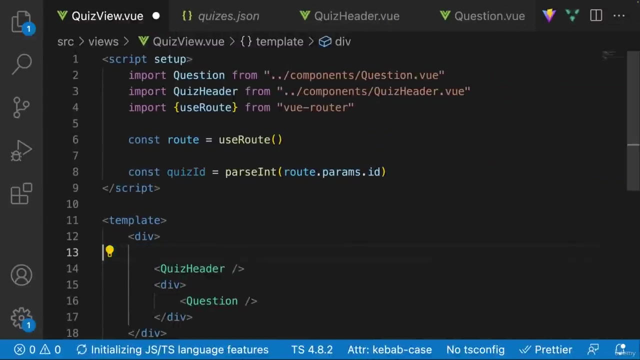 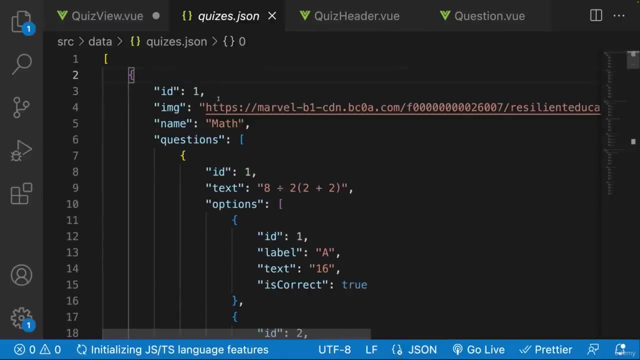 So let's first do that. So again, step one is to extract the query param from over here. So of course, we're going to need to utilize the use route composable to do this. So we're going to go over here, we're going to say from view router, so view router, we're going to get the use route composable. So use route composable. And over here, we're going to utilize that composable by saying const route is equal to and then use routes, and we're going to go ahead and invoke it. Now in order to extract the ID, very simply, what we can do now is just say const. And then we can say quiz ID, you can say that that's going to be equal to parse int, because remember, this is going to return back to us a string. So we're going to say parse int route dot, and then we're going to say route dot params dot ID. Very simple stuff right there. And just to prove to you that we indeed got our ID, we can go over here, you can see I have a one. And if I go to slash two, you can see we have slash two, etc, etc. Alright, so that's pretty good. But now what we need to do is we need to actually pass the current question that we're on to this question component. And what I mean by the current question that we're on is remember, the quiz itself is an object that has an ID image and the name. 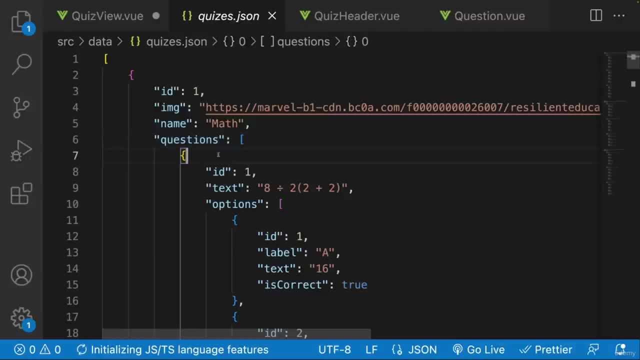 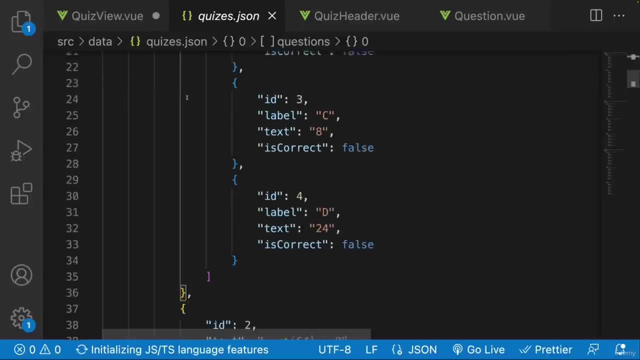 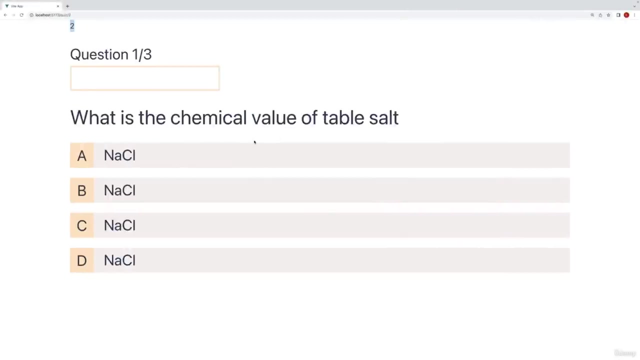 But it also has a questions array, which also contains multiple different objects. So as soon as we click on a particular quiz, this right here is the the first object is going to be the data for that very first question. So we're going to have the text here. And here are all of our options. Then of course, we're going to move on to the next question, which is this one and then this one. So what we need to do is first keep track with what question we are on. Now initially, as soon as we render, 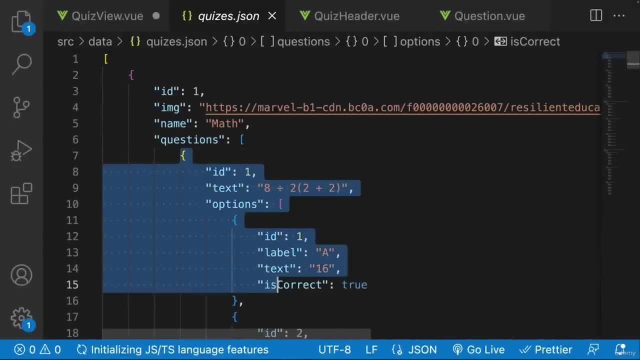 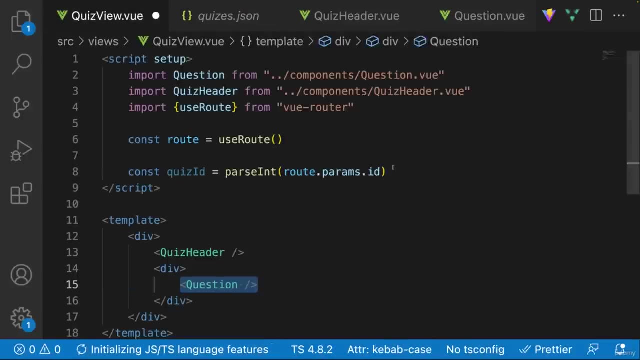 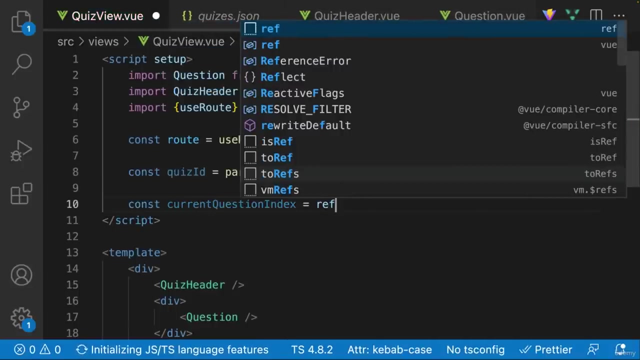 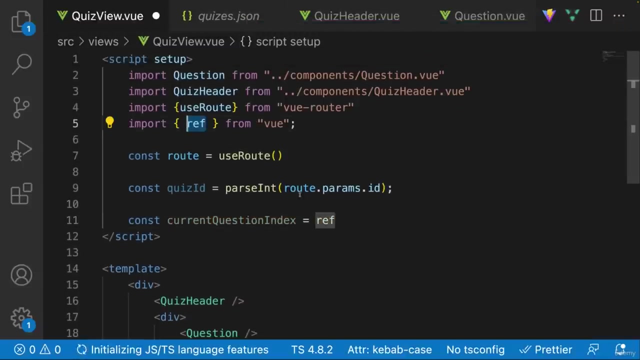 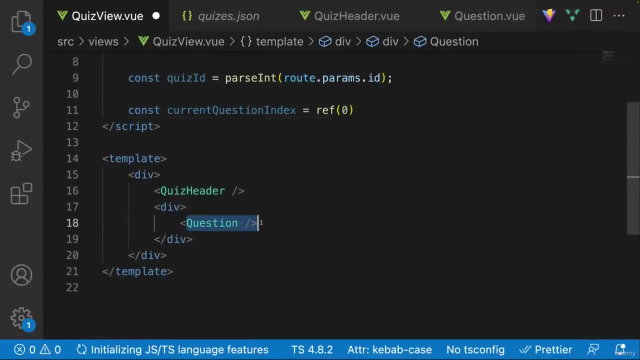 this quiz, we want to be on this question, the very first question with an index of zero. So that's actually what we're going to do here. So we're going to go over here. And we're going to create a piece of state saying const current question index. And this we're going to store as ref, of course, because this is going to be state. And right over here, we're going to of course, have to import this from view it auto imported it for me. And initially, we're just going to set this to zero like so. And later on, we're going to modify it once we want to click. And once we finish a particular question, we're going to modify it to one, then two, and then three, if we have it. Alright, so that's pretty much actually all it is that we need to do in order to pass the data that we need in here. Now, of course, the most important thing that we need to do is actually find the quiz that 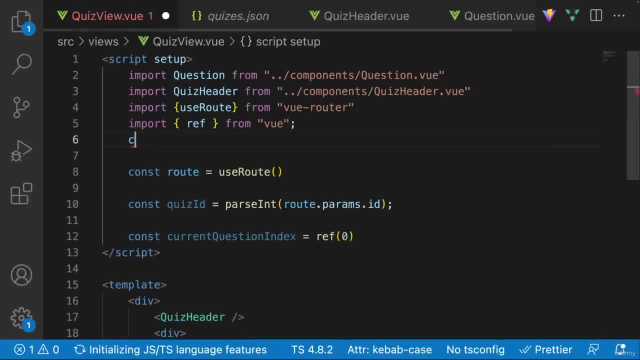 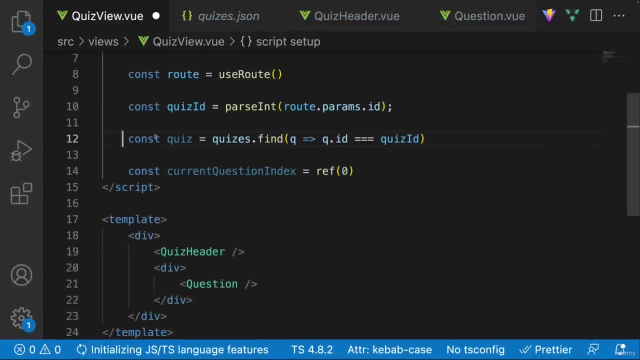 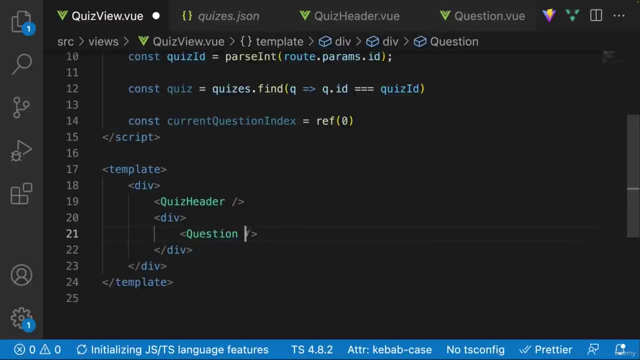 has this quiz ID. So let's go over here. And I'm going to say import quizzes from and I'm going to say from slash slash data slash quizzes dot JSON. And we're going to go over here. And we are going to create the actual quiz that we're on. So we're going to say const quiz. And we're going to say quizzes dot find. And we are going to find and we're going to call this queue. We'll call it queue like so. q dot ID is equal to the quiz ID. Now notice right now, we actually utilize this within the script setup. But later on, I'm going to actually show you a more elegant and a more view efficient way of doing this. So for now, we'll just leave it as is. But later on, we'll we'll move it around. Okay, so now we have our quizzes, we have the current question index. So what we can do actually is pass this data to our question. So let's go over here. And I'm going to say a prop called question. And that's going to be equal to quiz and then I'm going to say quiz dot questions. And then we have to specify what question Well, for that we're going to utilize the current question index. So I hope that is making sense. 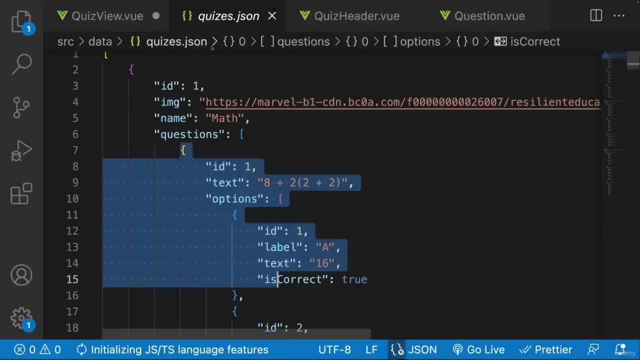 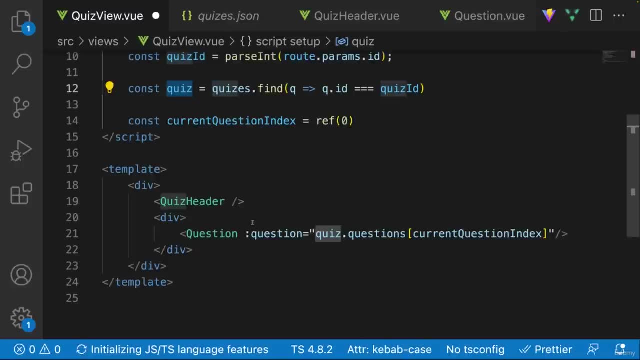 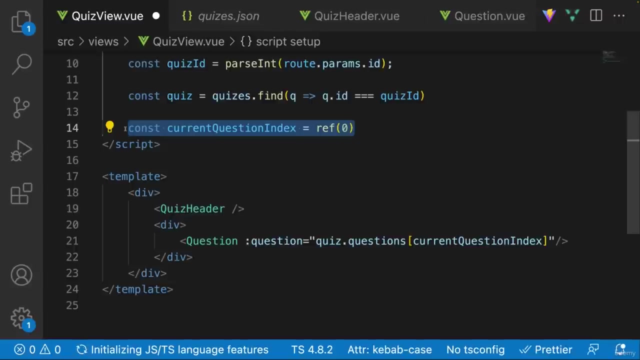 I know it's quite a lot because right here we have this quiz object, it has a questions property, which is an array, but we want a specific question to pass in here, we don't want to pass all the questions. So that's why we're going to utilize the current question index, which initially, we're going to use the current question index, which initially, we're going to use the current question index, which initially is set as the very first object. So I hope that is nice and clear. 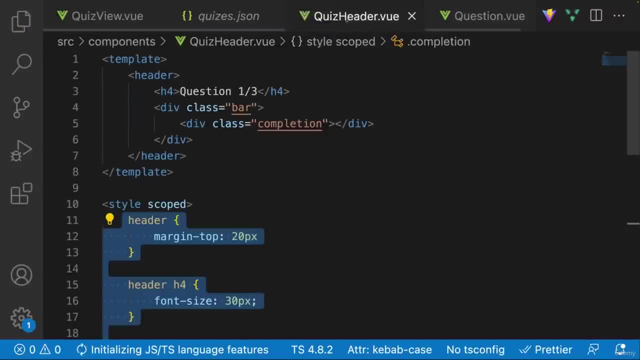 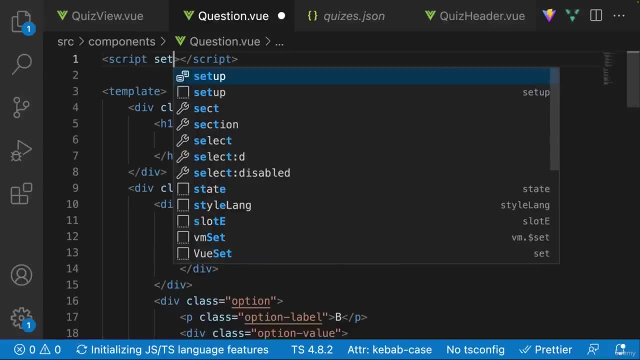 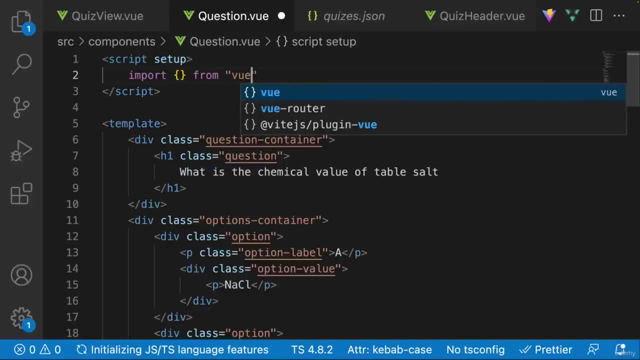 Alright, so now that we got that we can actually utilize the current question index within our question component. So of course, let's do some script setup over here. And let's import define props, because remember, we pass this as a prop. So we're going to say define props. 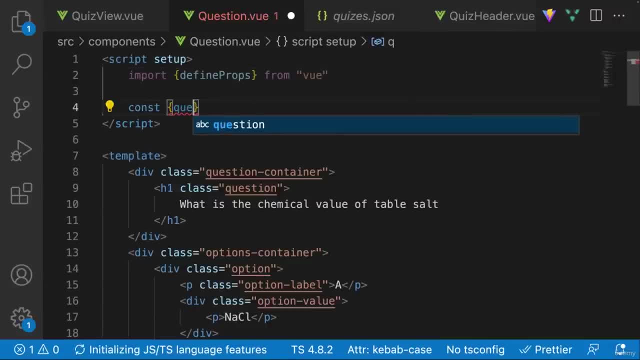 And we're going to say, Hey, I want to get the question. And I'm going to say I want this from defined props. And question like so question like so. So that is, of course, going to give us the question. So now we can actually utilize that instead of hard coding our information. 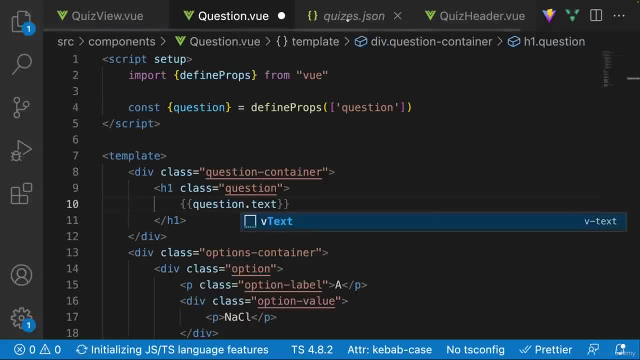 So I can say question dot text, which I believe is what I called it question dot text. And there we go. So now let's actually just test this out to see if everything's okay. 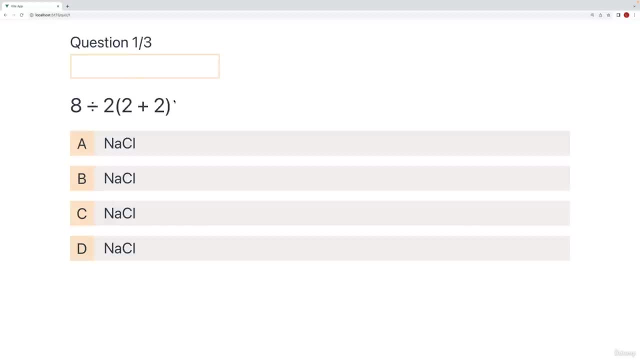 So let's go back here, if I click on math, you can see now we get the actual first question for each particular quiz. So the Krebs cycle occurs in, but of course, the options are hard coded for now. 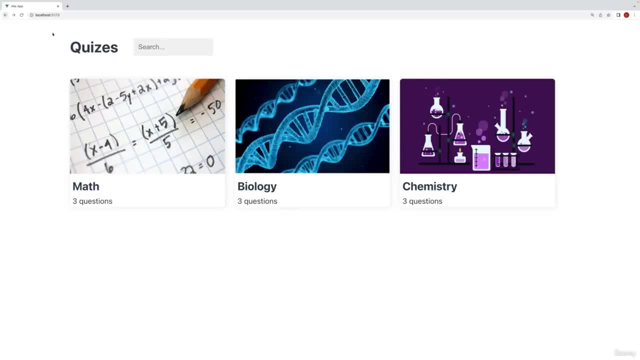 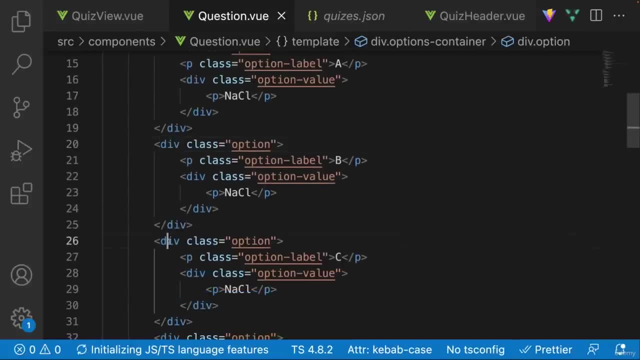 But the questions are obviously different. What is the composition of table salt? Alright, so now that we have that, what we can actually do is instead of hard coding all of these, we can just iterate over the options. 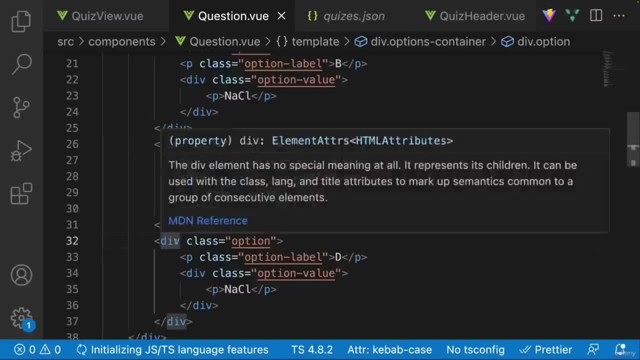 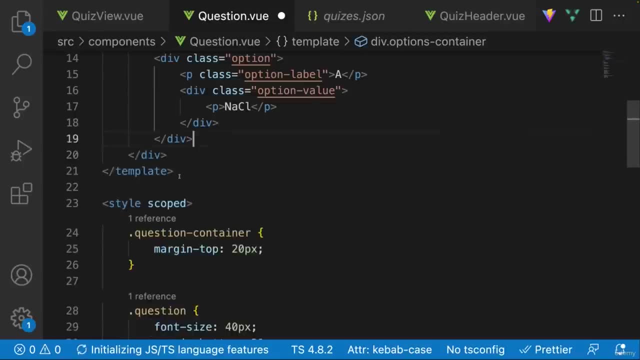 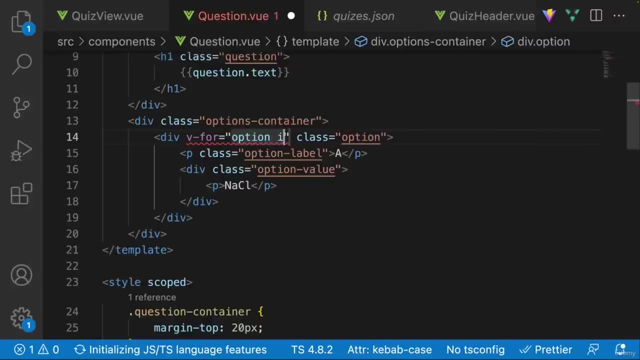 Through a v4. So I'm going to get rid of this, let's get rid of that, let's get rid of this, let's get rid of this, we only really need one. And within that one, we're going to say v4, I'm going to say for option in question dot options. So of course, we're going to also need to supply it with a key, let's supply it right over here, right after the the actual v4. 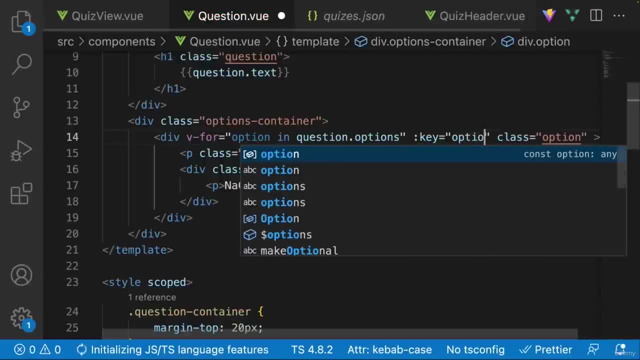 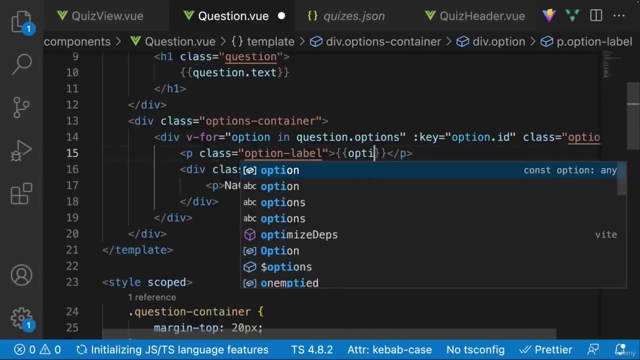 And we're going to say option dot id, because of course, each option also has its own unique ID. Alright, so that's pretty much all it is that we need to do now we only only have to change the label as well as the option itself. So I'm going to say here option dot, and then I'm going to say label label. And then over here, we're going to say option dot. And this 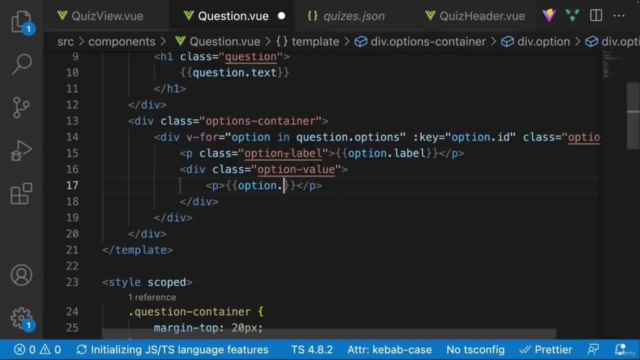 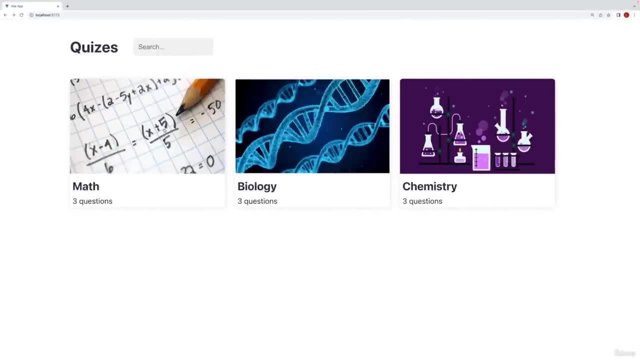 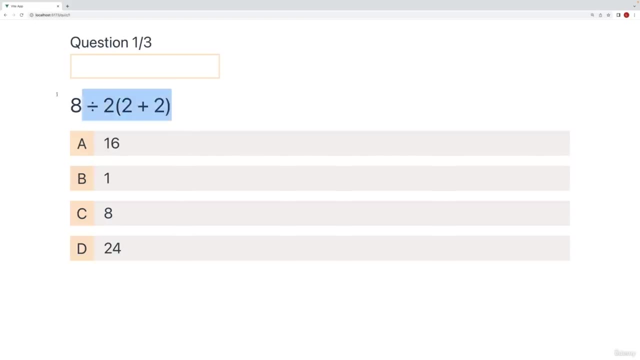 time I am going to say text so text like so let's go ahead and save this and refresh and now if I were to click on math you can see now I have the question 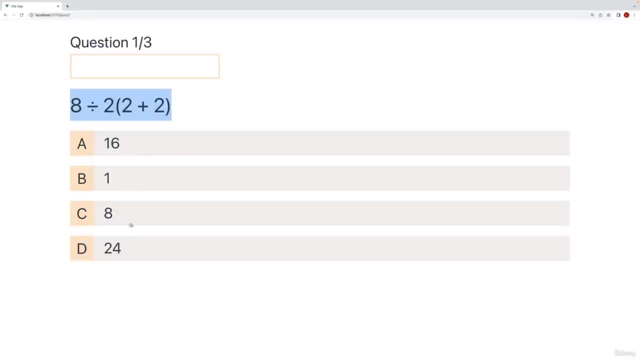 as well as all of the different options so we have 16 1 8 and 24 and this is 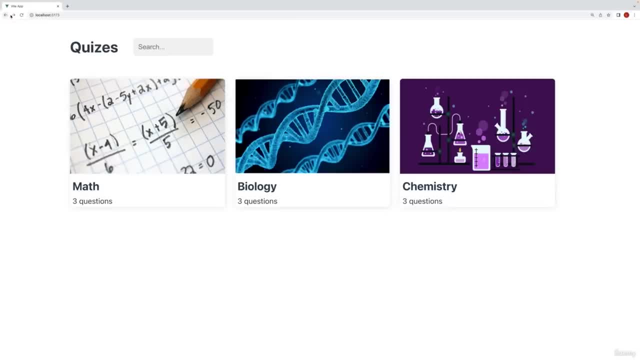 actually a tricky question so I highly suggest maybe try to figure this one out on your own biology the Krebs cycle occurs in the mitochondria the nucleus 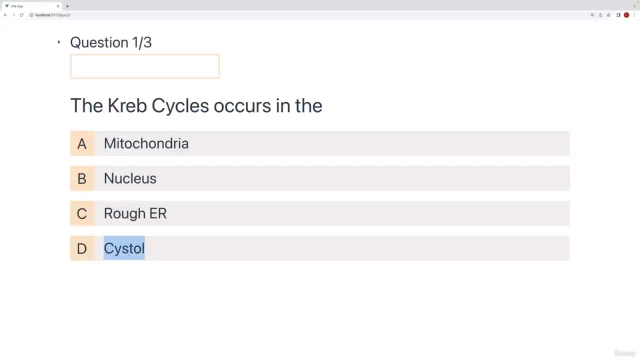 the rough ER the systole I don't know if I spelled that correctly doesn't matter I think it's a mitochondria but I'm not sure I actually kind of forget and 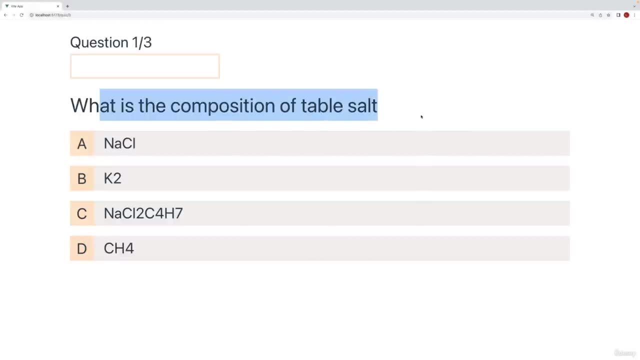 lastly what is the composition of table salt this one is pretty easy obviously it's k2 all right so now we got that done but of course if we want to make 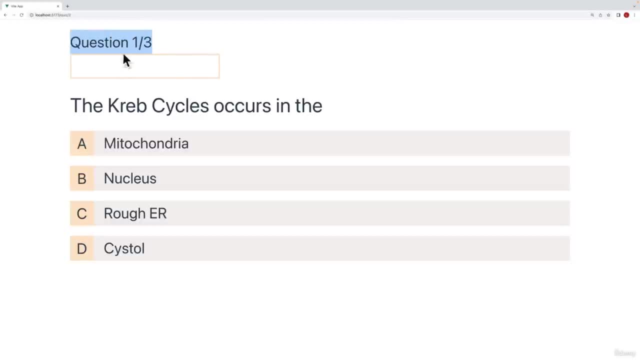 this dynamic over here so let's actually go ahead and do that in the next slide so let's actually go ahead and do that in the next slide so 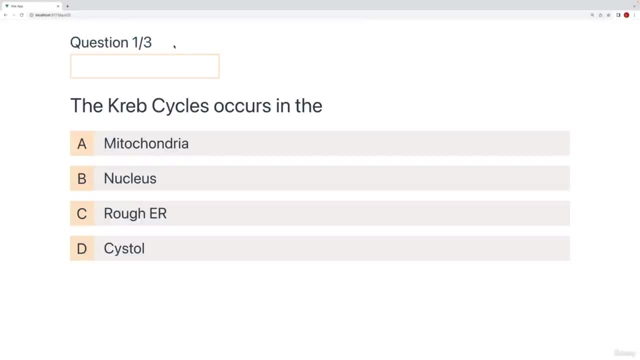 let's actually go ahead and do that in the next slide so let's actually go ahead and do that in the next video the process should be the next slide so let's actually go ahead and do that in the next video the process should be the next slide so let's actually go ahead and do that in the next video the process should be relatively the same 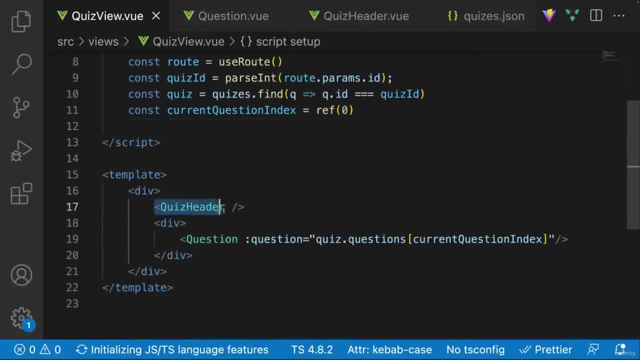 all right my good friends the next thing all right my good friends the next thing all right my good friends the next thing that we need to do is pass the necessary that we need to do is pass the necessary that we need to do is pass the necessary data through props to the quiz header 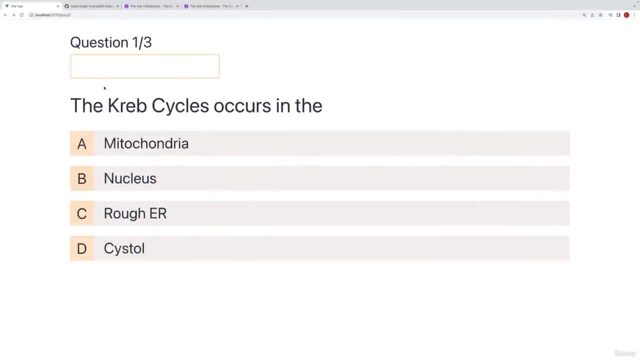 data through props to the quiz header data through props to the quiz header component because of course at this component because of course at this component because of course at this point it is hard-coded now let's quickly point it is hard-coded now let's quickly point it is hard-coded now let's quickly think about exactly what we need to pass think about exactly what we need to pass 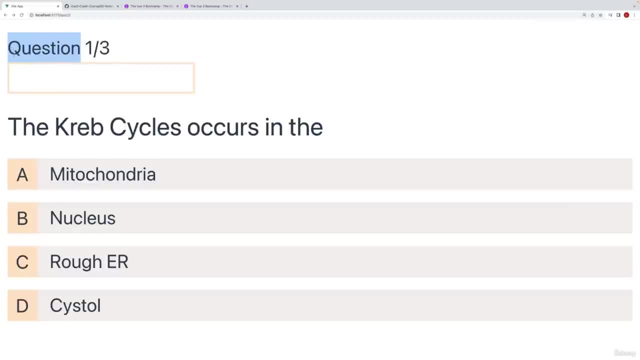 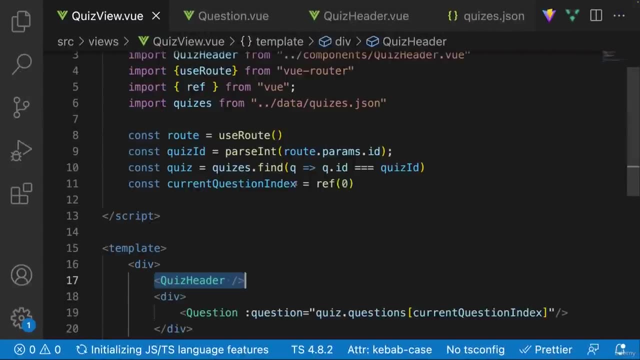 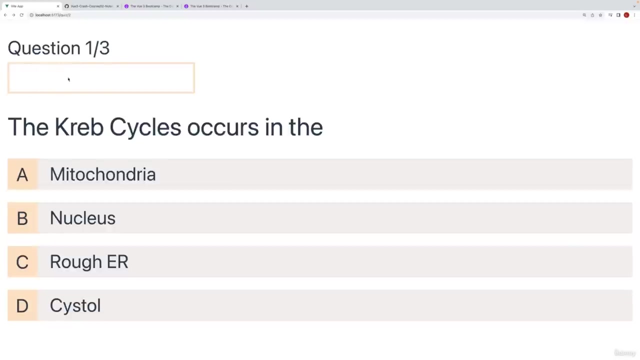 think about exactly what we need to pass in so we're always going to have this in so we're always going to have this in so we're always going to have this right over here so we're always going to right over here so we're always going to right over here so we're always going to have this label question but this over have this label question but this over have this label question but this over here is going to be dynamic and it's here is going to be dynamic and it's here is going to be dynamic and it's going to be dependent on the current going to be dependent on the current going to be dependent on the current index and then also the length of our index and then also the length of our index and then also the length of our quiz array and then this over here is quiz array and then this over here is quiz array and then this over here is also going to be kind of the division of 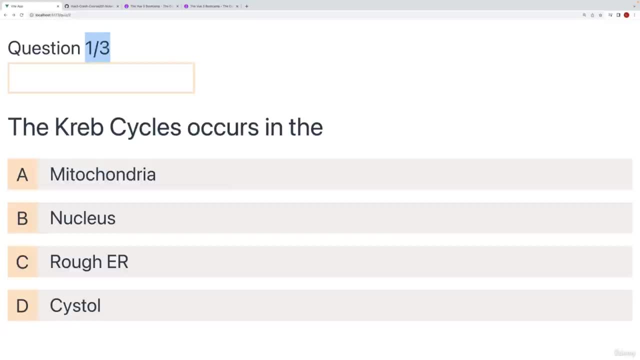 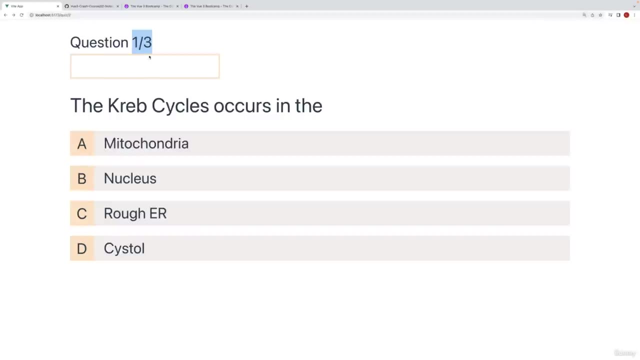 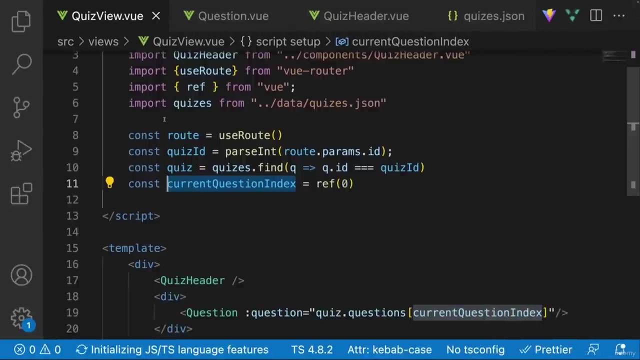 also going to be kind of the division of also going to be kind of the division of what we have over here so if is one out what we have over here so if is one out what we have over here so if is one out of three then this should be 33% so this of three then this should be 33% so this of three then this should be 33% so this is the information that we need to pass is the information that we need to pass is the information that we need to pass into this component so let's actually go into this component so let's actually go into this component so let's actually go ahead and let's just begin with this ahead and let's just begin with this ahead and let's just begin with this portion right over here because of portion right over here because of portion right over here because of course this is the simplest so what we course this is the simplest so what we 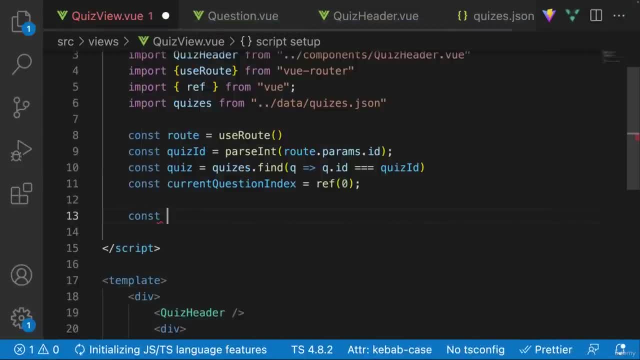 course this is the simplest so what we can actually do to achieve this is very can actually do to achieve this is very can actually do to achieve this is very simply just say well question status we simply just say well question status we simply just say well question status we can say that this is going to be equal can say that this is going to be equal can say that this is going to be equal to a template literal and very simply we to a template literal and very simply we to a template literal and very simply we can just grab the current question index can just grab the current question index can just grab the current question index do a dollar sign curly braces and say do a dollar sign curly braces and say do a dollar sign curly braces and say dot value over and then dollar sign dot value over and then dollar sign dot value over and then dollar sign curly brace to use the JavaScript again 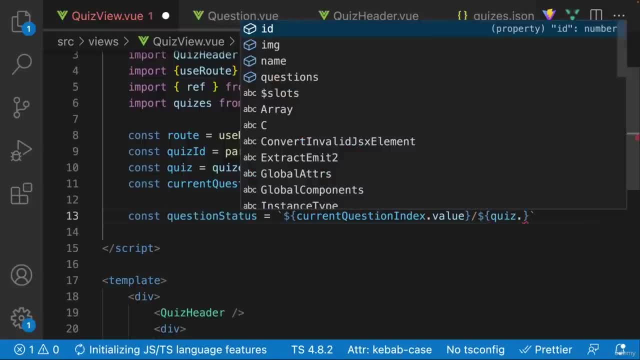 curly brace to use the JavaScript again curly brace to use the JavaScript again and we can say here quiz dot question 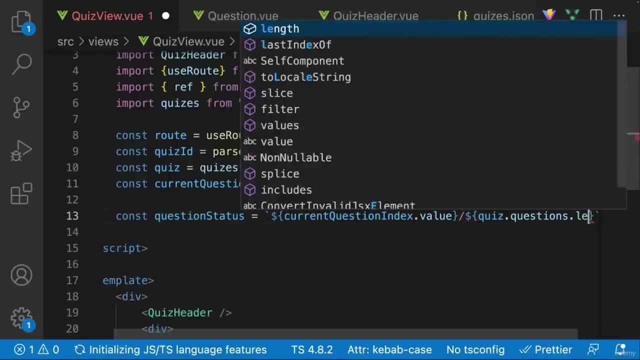 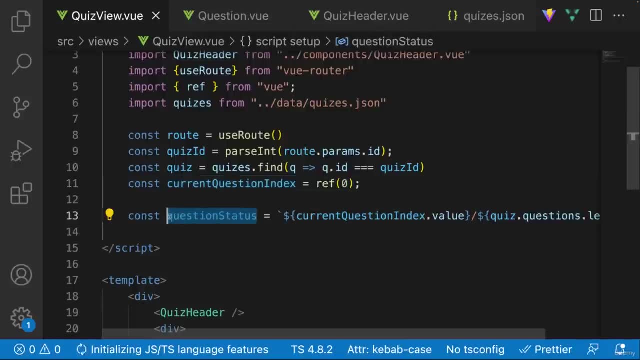 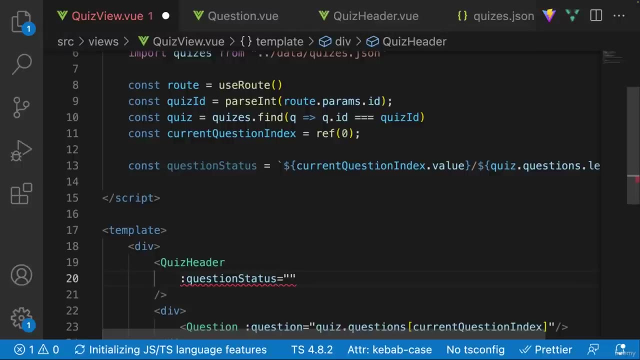 and we can say here quiz dot question and we can say here quiz dot question dot questions dot and then dot length dot questions dot and then dot length dot questions dot and then dot length like so so let's go ahead and just very like so so let's go ahead and just very like so so let's go ahead and just very simply save that and what we can do now simply save that and what we can do now simply save that and what we can do now is actually pass this as a prop so we is actually pass this as a prop so we is actually pass this as a prop so we can go here pass this as a prop say can go here pass this as a prop say can go here pass this as a prop say question status is equal to question question status is equal to question 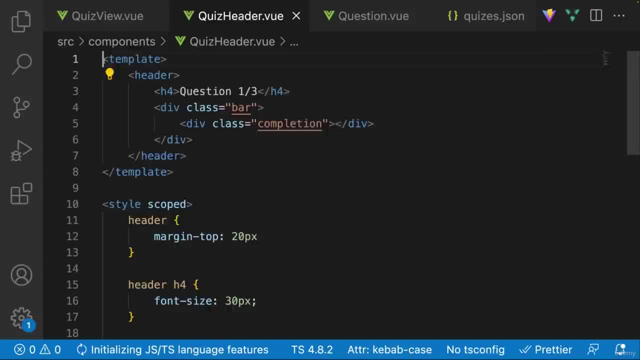 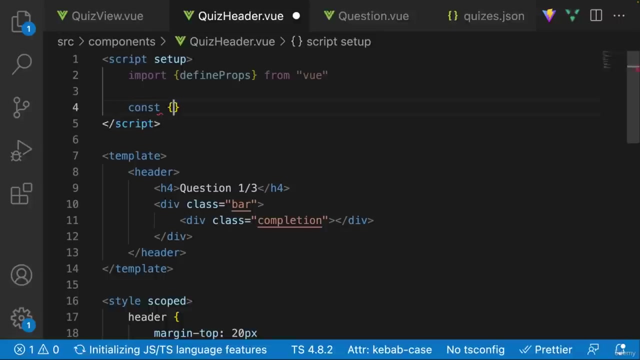 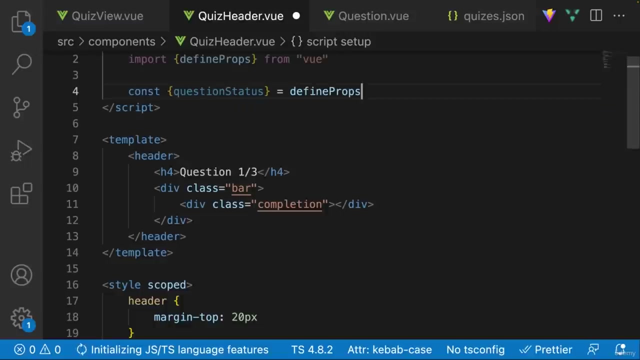 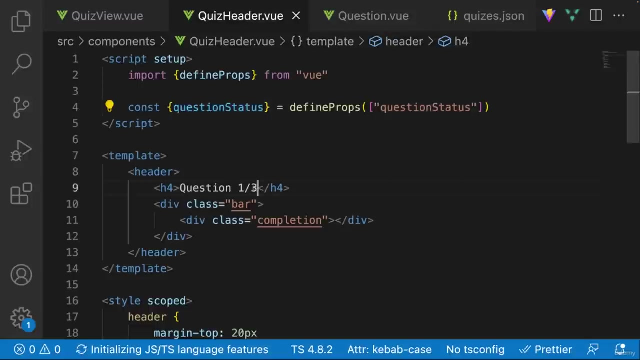 question status is equal to question status we can then go to our question status we can then go to our question status we can then go to our question header and very simply create the script header and very simply create the script header and very simply create the script setup and over here we can import define setup and over here we can import define setup and over here we can import define props from view and then we can say props from view and then we can say props from view and then we can say question status is equal to define oops question status is equal to define oops question status is equal to define oops define props and then an array where we define props and then an array where we define props and then an array where we have the question status so have the question status so have the question status so over here we can just grab this and 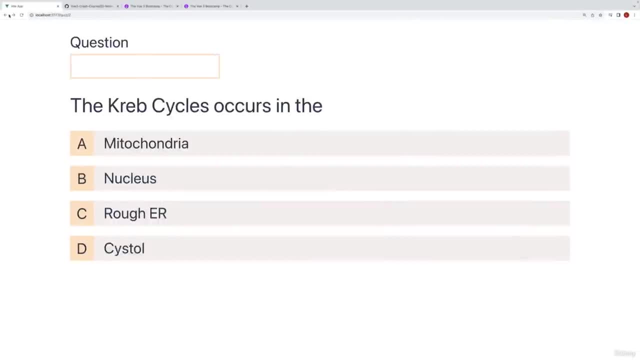 over here we can just grab this and over here we can just grab this and instead of having this we can just say instead of having this we can just say instead of having this we can just say question status and if I were to refresh 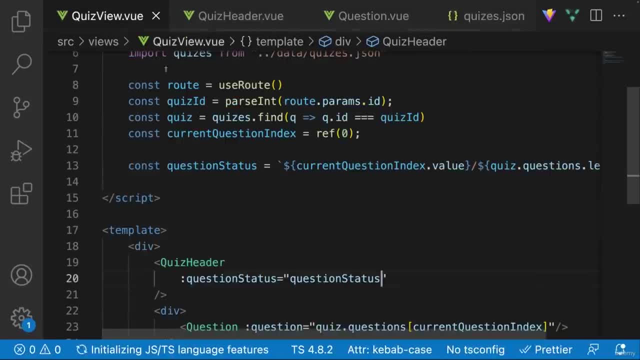 question status and if I were to refresh question status and if I were to refresh you can see we get zero out of three but you can see we get zero out of three but you can see we get zero out of three but now let's actually take a look at what 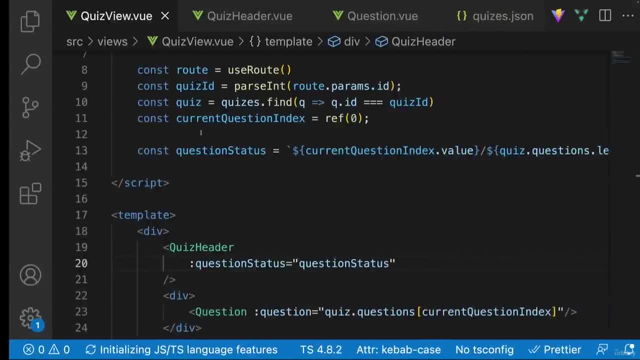 now let's actually take a look at what now let's actually take a look at what happens when we will move on to the next happens when we will move on to the next happens when we will move on to the next question so what I'm going to do just question so what I'm going to do just question so what I'm going to do just for now is I'm going to create a button for now is I'm going to create a button 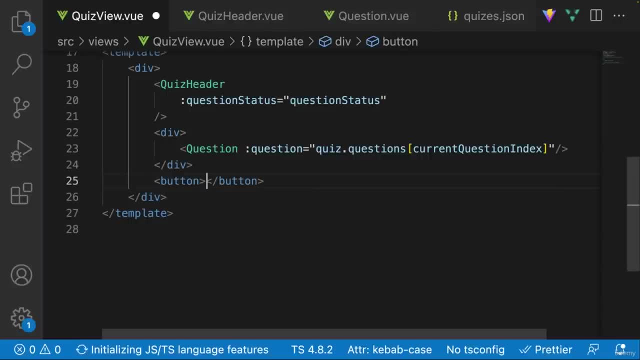 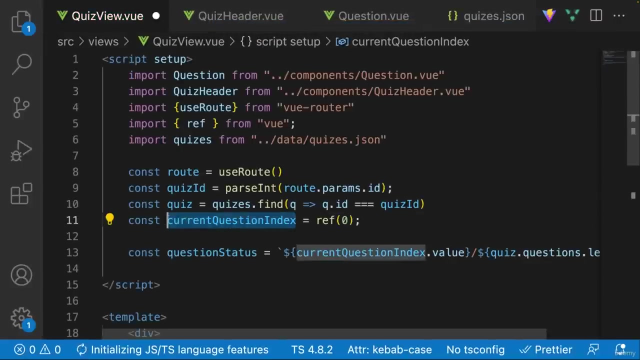 for now is I'm going to create a button and this is just gonna have a text of and this is just gonna have a text of and this is just gonna have a text of next question next question and of next question next question and of next question next question and of course later on we're gonna remove this course later on we're gonna remove this course later on we're gonna remove this but just for now I'm gonna have that but just for now I'm gonna have that but just for now I'm gonna have that button we're gonna have an at click button we're gonna have an at click button we're gonna have an at click handler and remember to move on to the handler and remember to move on to the handler and remember to move on to the next question we're gonna change this next question we're gonna change this next question we're gonna change this state to the next index so we're gonna 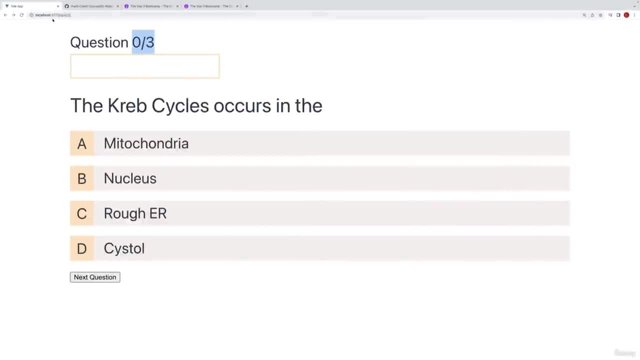 state to the next index so we're gonna state to the next index so we're gonna say here current index plus plus and say here current index plus plus and say here current index plus plus and let's just refresh and if I were to let's just refresh and if I were to let's just refresh and if I were to click on this you can see here nothing click on this you can see here nothing click on this you can see here nothing is changing and hopefully at this point is changing and hopefully at this point is changing and hopefully at this point this is expected the reason for this is this is expected the reason for this is this is expected the reason for this is because this is not state and it is not because this is not state and it is not because this is not state and it is not causing a rerender of this particular causing a rerender of this particular 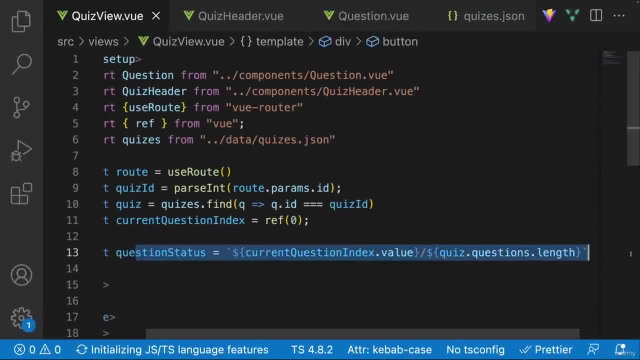 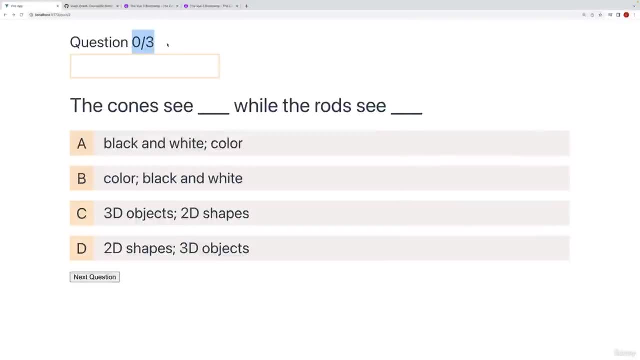 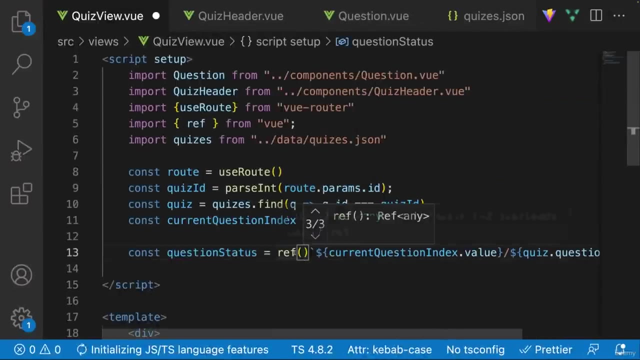 causing a rerender of this particular component because again we're not component because again we're not component because again we're not storing it as a piece of state where we storing it as a piece of state where we storing it as a piece of state where we would need to store it as a piece of would need to store it as a piece of would need to store it as a piece of state if we want to well rerender our state if we want to well rerender our state if we want to well rerender our component and actually see that output component and actually see that output component and actually see that output within our application so you might be within our application so you might be within our application so you might be thinking okay easy peasy late let's go thinking okay easy peasy late let's go thinking okay easy peasy late let's go ahead and change this I'm gonna say I'm 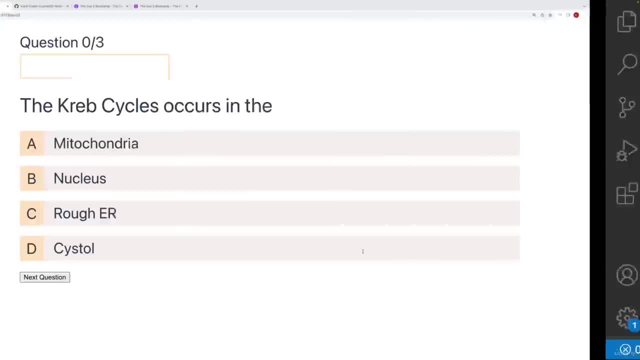 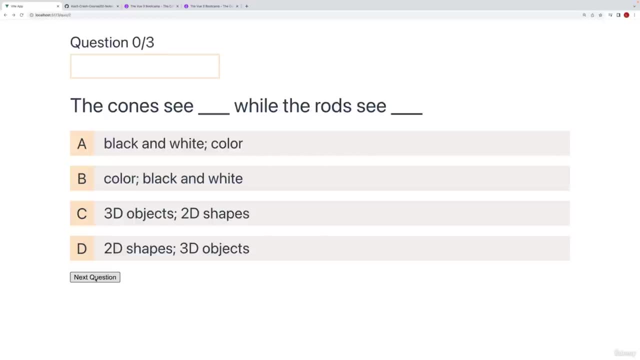 ahead and change this I'm gonna say I'm ahead and change this I'm gonna say I'm gonna change this to a piece of state gonna change this to a piece of state gonna change this to a piece of state because that's exactly what you told me because that's exactly what you told me because that's exactly what you told me to do so I'm gonna go ahead and do a to do so I'm gonna go ahead and do a to do so I'm gonna go ahead and do a quick refresh and now you can see we get quick refresh and now you can see we get quick refresh and now you can see we get kind of the same exact problem so yes kind of the same exact problem so yes 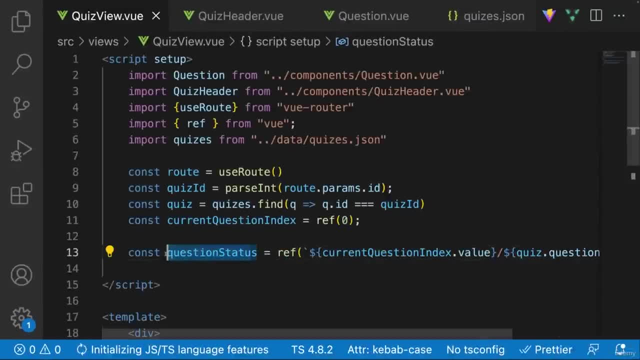 kind of the same exact problem so yes this time we have changed our question this time we have changed our question this time we have changed our question status to state an actual piece of state status to state an actual piece of state 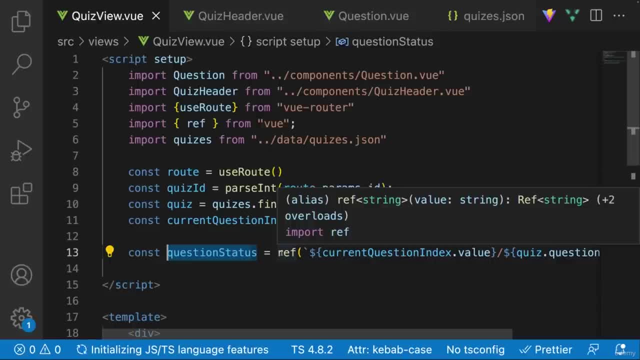 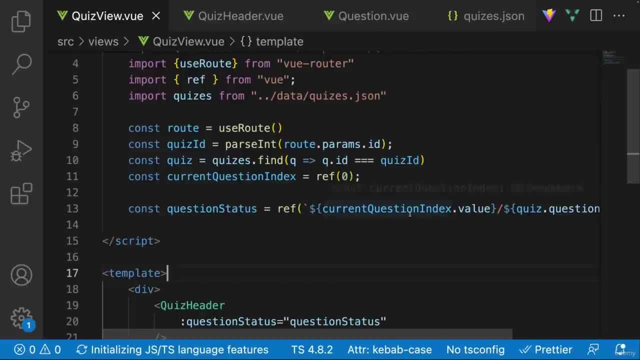 status to state an actual piece of state however we're not actually updating our however we're not actually updating our however we're not actually updating our question status we need to actually question status we need to actually question status we need to actually update it even though this is changing update it even though this is changing update it even though this is changing this over here the question status this over here the question status this over here the question status itself isn't and it's always going to be itself isn't and it's always going to be itself isn't and it's always going to be the default value that we have well gave the default value that we have well gave the default value that we have well gave it so how are we going to do this well it so how are we going to do this well it so how are we going to do this well the question status we want to change it 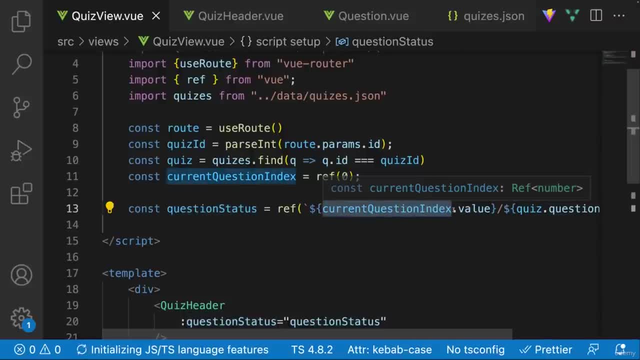 the question status we want to change it the question status we want to change it anytime our current question index anytime our current question index anytime our current question index changes as well so whenever our current changes as well so whenever our current changes as well so whenever our current question index changes we want to change question index changes we want to change question index changes we want to change our question status so what we can our question status so what we can our question status so what we can actually do is watch for any changes that actually do is watch for any changes that actually do is watch for any changes that occur to the current question index dot occur to the current question index dot occur to the current question index dot value anytime there's any particular value anytime there's any particular 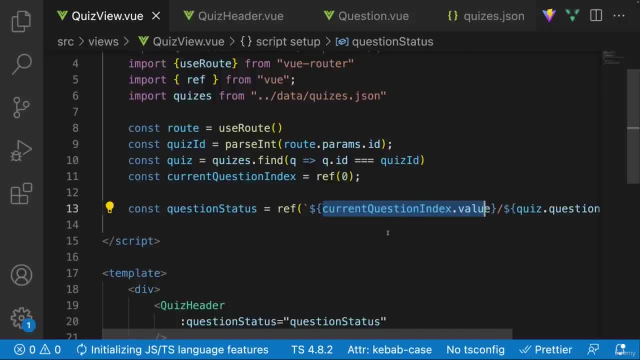 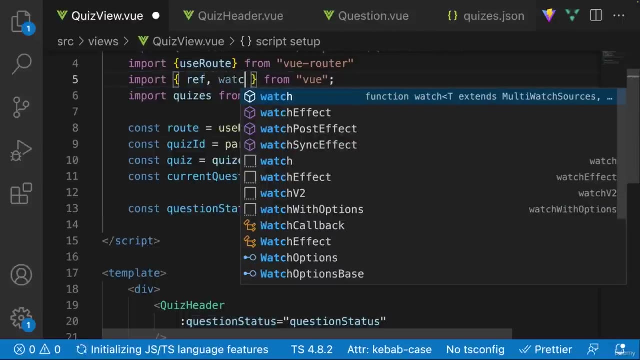 value anytime there's any particular change to this we can actually run some change to this we can actually run some change to this we can actually run some logic and in this case the logic is logic and in this case the logic is logic and in this case the logic is going to be to update this piece of state going to be to update this piece of state going to be to update this piece of state over here now this might be a little over here now this might be a little over here now this might be a little bit confusing so let me actually go ahead bit confusing so let me actually go ahead bit confusing so let me actually go ahead and show you what I mean so within the and show you what I mean so within the and show you what I mean so within the view we can actually import something view we can actually import something view we can actually import something else called watch and again what this is 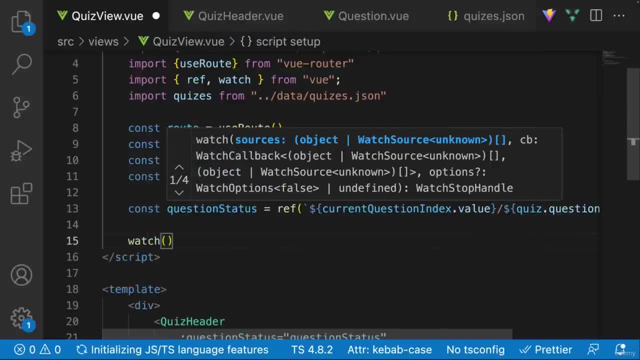 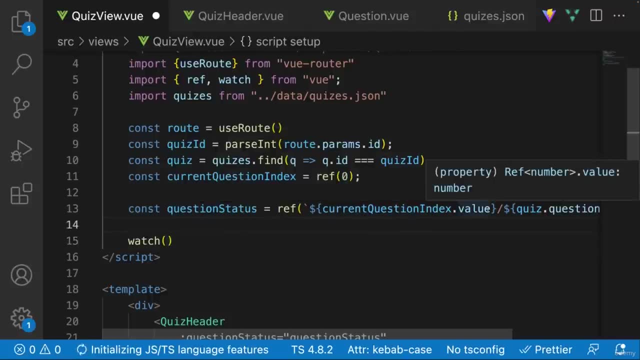 else called watch and again what this is else called watch and again what this is going to do is well we're gonna go ahead going to do is well we're gonna go ahead going to do is well we're gonna go ahead and invoke it and it is going to watch and invoke it and it is going to watch and invoke it and it is going to watch for a particular entity a particular for a particular entity a particular for a particular entity a particular thing that might potentially change in thing that might potentially change in thing that might potentially change in this case it is the current question this case it is the current question this case it is the current question dot value so we're saying here we want dot value so we're saying here we want dot value so we're saying here we want you to watch for the current question you to watch for the current question 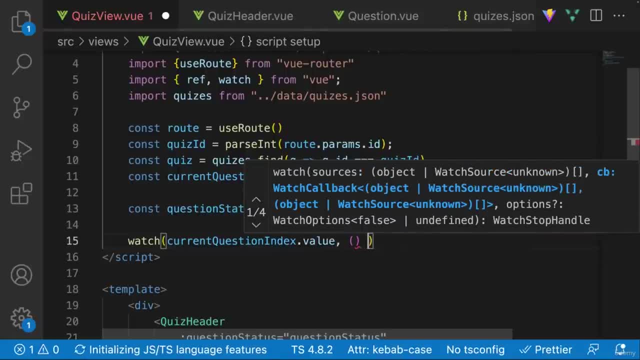 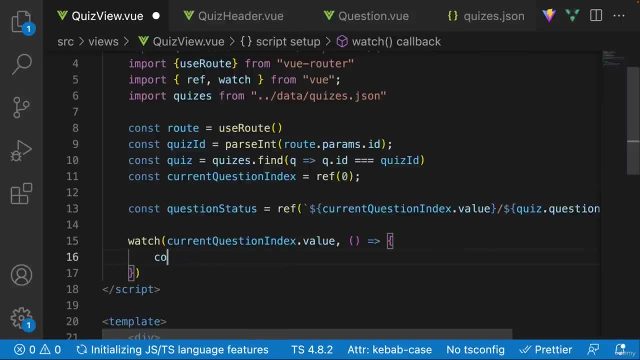 you to watch for the current question dot value and anytime that it changes as dot value and anytime that it changes as dot value and anytime that it changes as the second parameter we're gonna pass the second parameter we're gonna pass the second parameter we're gonna pass in a callback and we want you to run this in a callback and we want you to run this in a callback and we want you to run this callback so let me just go ahead and do callback so let me just go ahead and do callback so let me just go ahead and do a quick little console dot log here a quick little console dot log here a quick little console dot log here console dot log I'm just gonna say hello console dot log I'm just gonna say hello console dot log I'm just gonna say hello or maybe something more descriptive I'm or maybe something more descriptive I'm or maybe something more descriptive I'm gonna say current question index or 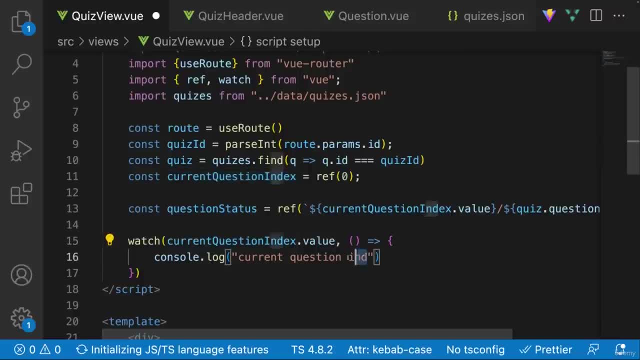 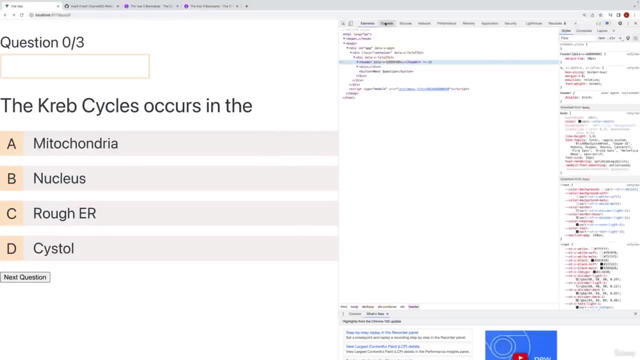 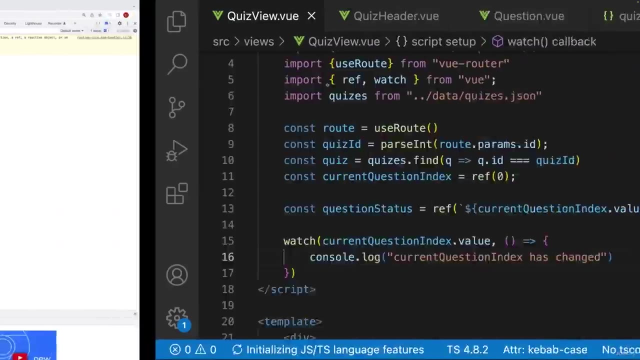 gonna say current question index or gonna say current question index or let's just say this like so current let's just say this like so current let's just say this like so current question index has changed so let's go question index has changed so let's go question index has changed so let's go ahead and save this I'm gonna go inspect ahead and save this I'm gonna go inspect ahead and save this I'm gonna go inspect my console and I'm gonna do a quick my console and I'm gonna do a quick my console and I'm gonna do a quick little refresh so at first there's little refresh so at first there's little refresh so at first there's nothing but then when I change it nothing but then when I change it nothing but then when I change it there's still nothing and actually that's there's still nothing and actually that's 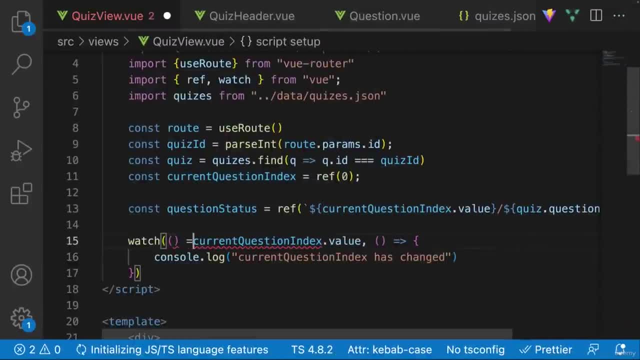 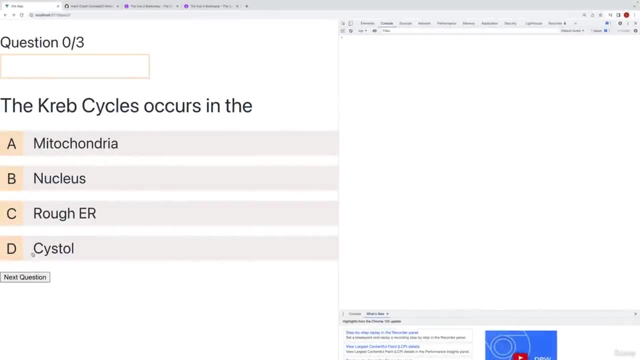 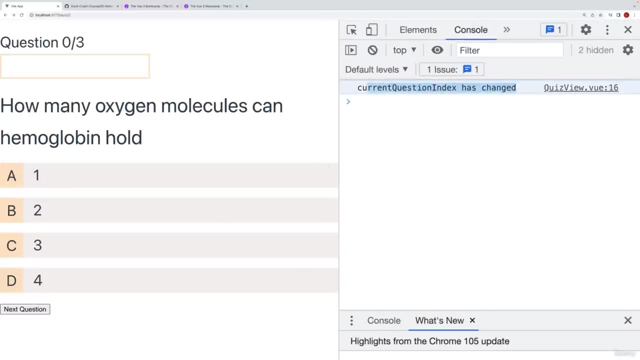 there's still nothing and actually that's because this over here my apologies because this over here my apologies because this over here my apologies should be a function so it's a function should be a function so it's a function should be a function so it's a function that is going to return what it wants to that is going to return what it wants to that is going to return what it wants to listen to so let me go ahead and listen to so let me go ahead and listen to so let me go ahead and actually refresh this and now you can actually refresh this and now you can actually refresh this and now you can see here current question index has see here current question index has see here current question index has changed so it's changed from 0 to 1 if I changed so it's changed from 0 to 1 if I changed so it's changed from 0 to 1 if I click it again it gets console logged 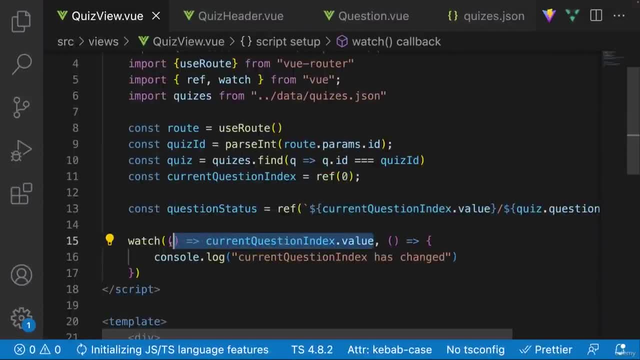 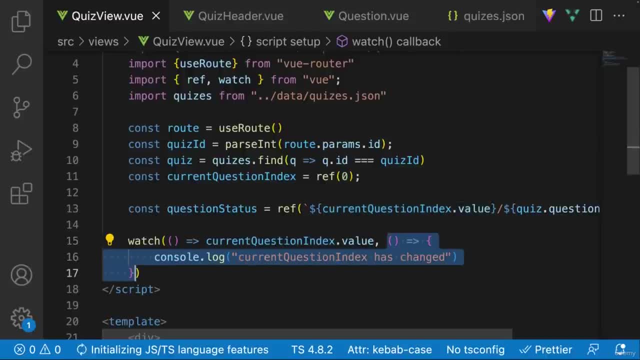 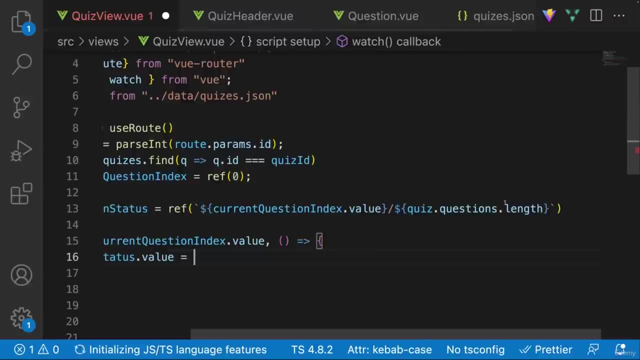 the second parameter is another function and this is going to be kind of the and this is going to be kind of the and this is going to be kind of the callback handler that we are going to callback handler that we are going to callback handler that we are going to call whenever this value changes all call whenever this value changes all call whenever this value changes all right so now what we can very simply do right so now what we can very simply do right so now what we can very simply do is say is say is say well well well question status dot value is equal to question status dot value is equal to question status dot value is equal to and we can say that it is equal to 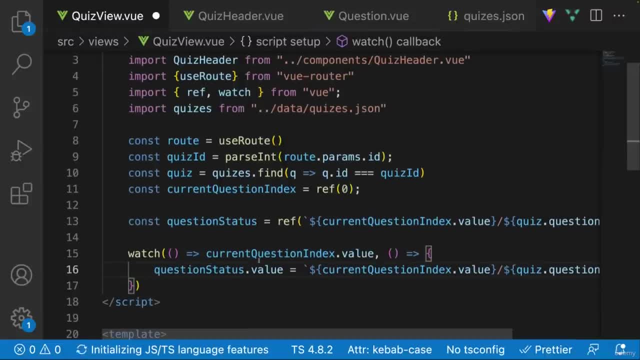 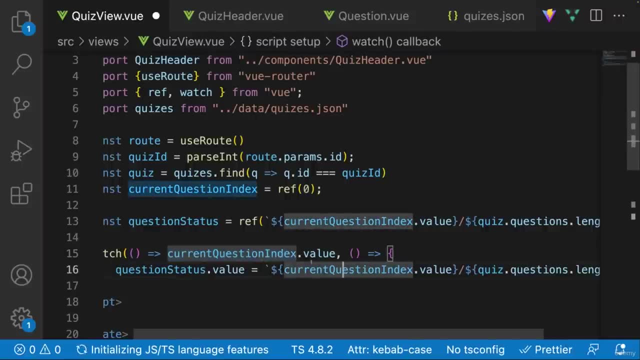 and we can say that it is equal to and we can say that it is equal to basically the exact same thing basically the exact same thing basically the exact same thing so we can just say question status dot so we can just say question status dot so we can just say question status dot value is equal to this but this time value is equal to this but this time value is equal to this but this time this value is going to be different this value is going to be different this value is going to be different because the current question index dot because the current question index dot because the current question index dot value has changed value has changed value has changed so now let's give this a quick go so so now let's give this a quick go so 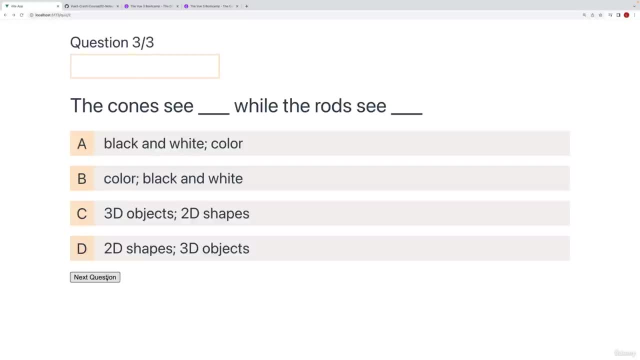 so now let's give this a quick go so refresh and there we go you can see that refresh and there we go you can see that refresh and there we go you can see that it is updating now of course if i it is updating now of course if i it is updating now of course if i continue on continue on continue on we're going to get some sort of error in we're going to get some sort of error in we're going to get some sort of error in the console but you can see that it is the console but you can see that it is the console but you can see that it is indeed working so that right there is indeed working so that right there is indeed working so that right there is the watch and we're going to be the watch and we're going to be the watch and we're going to be utilizing this quite a bit throughout 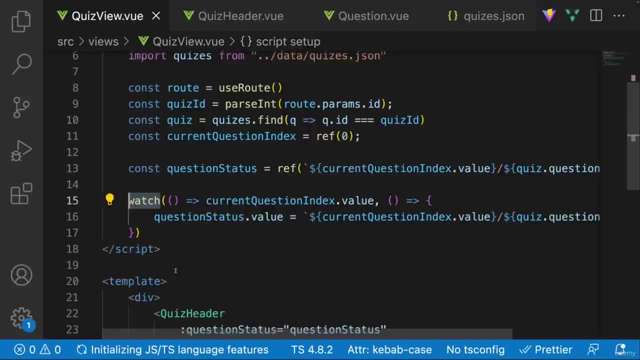 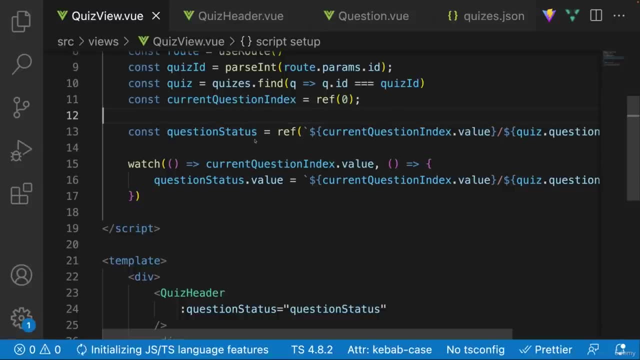 utilizing this quite a bit throughout utilizing this quite a bit throughout this course whenever we want to do this course whenever we want to do this course whenever we want to do something anytime a piece of state something anytime a piece of state something anytime a piece of state changes changes changes so we were able to successfully so we were able to successfully so we were able to successfully calculate our question status and then calculate our question status and then calculate our question status and then pass it into our quiz header however we pass it into our quiz header however we pass it into our quiz header however we had to perform two different steps in had to perform two different steps in 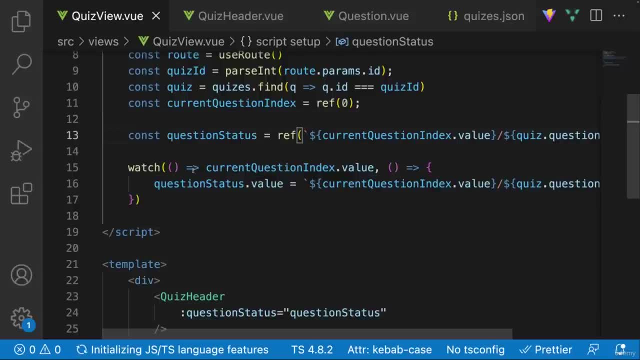 had to perform two different steps in order to do this we had to first define order to do this we had to first define order to do this we had to first define our state and then we had to have this our state and then we had to have this our state and then we had to have this listener and anytime this listener and anytime this listener and anytime this current question index changes we current question index changes we current question index changes we updated our question status to utilize updated our question status to utilize updated our question status to utilize the new current question index the new current question index the new current question index and there's actually a much more elegant and there's actually a much more elegant and there's actually a much more elegant and faster way of doing this now this is 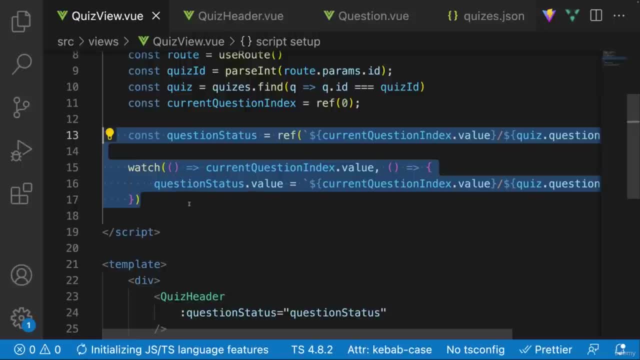 and faster way of doing this now this is and faster way of doing this now this is working this is completely fine but working this is completely fine but working this is completely fine but there's a better way in terms of code to there's a better way in terms of code to there's a better way in terms of code to do this do this do this so right here this value very simply is so right here this value very simply is so right here this value very simply is heavily dependent heavily dependent heavily dependent on this value so whenever this changes on this value so whenever this changes on this value so whenever this changes of course we want to change of course we want to change 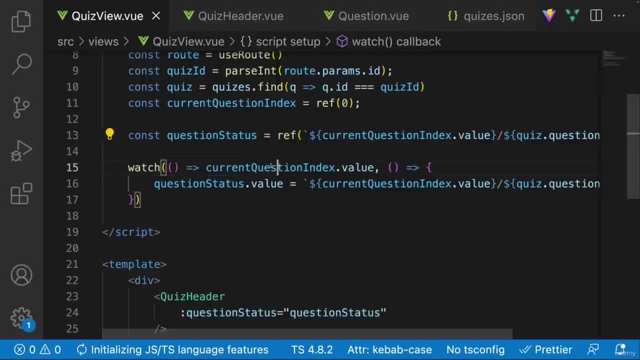 of course we want to change this value but that's pretty much all it this value but that's pretty much all it this value but that's pretty much all it is that we want to do is that we want to do is that we want to do we just want to change this value to we just want to change this value to we just want to change this value to accommodate changes to this value we accommodate changes to this value we accommodate changes to this value we don't really need this watch method don't really need this watch method don't really need this watch method because this watch method what it does because this watch method what it does because this watch method what it does is it gives us the ability to do a bunch is it gives us the ability to do a bunch is it gives us the ability to do a bunch of other things so for example maybe 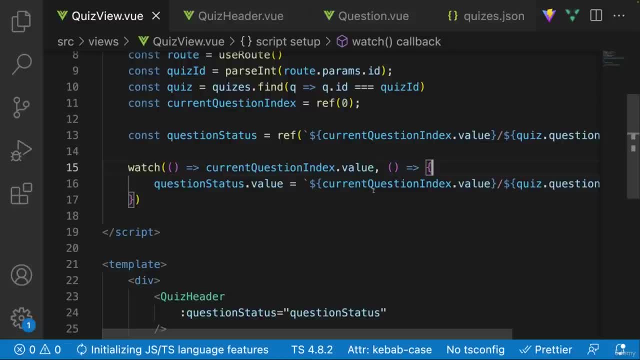 of other things so for example maybe of other things so for example maybe we change the value and we need to fetch we change the value and we need to fetch we change the value and we need to fetch some data from an external api we can go some data from an external api we can go some data from an external api we can go ahead and do that here and then we can ahead and do that here and then we can ahead and do that here and then we can do some checks here and everything etc do some checks here and everything etc do some checks here and everything etc etc but what we're doing right now is etc but what we're doing right now is etc but what we're doing right now is very simply just very simply just very simply just using this watch to update our well using this watch to update our well 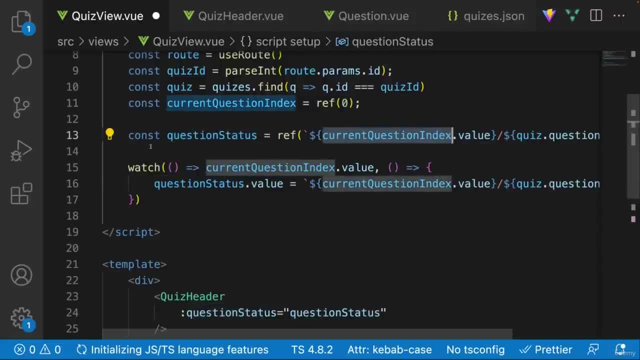 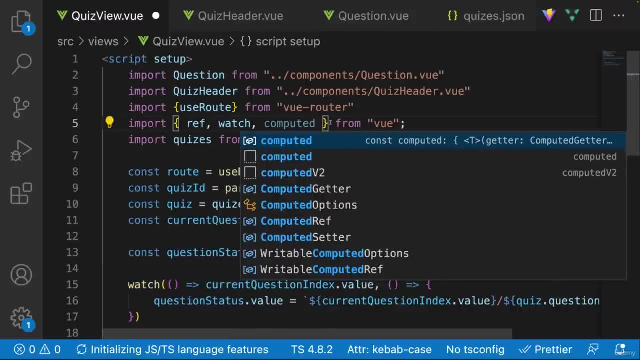 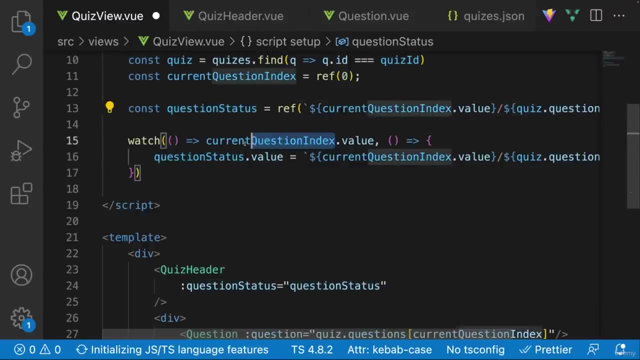 using this watch to update our well question status anytime that this question status anytime that this question status anytime that this changes and for this piece of changes and for this piece of changes and for this piece of functionality there's actually functionality there's actually functionality there's actually another thing that we can use called another thing that we can use called another thing that we can use called computed so we can use this computed computed so we can use this computed computed so we can use this computed anytime we want to compute a certain anytime we want to compute a certain anytime we want to compute a certain value that is based off of another value value that is based off of another value value that is based off of another value and if this value ever changes the 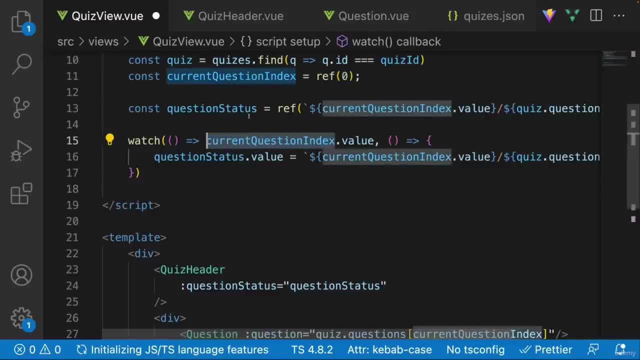 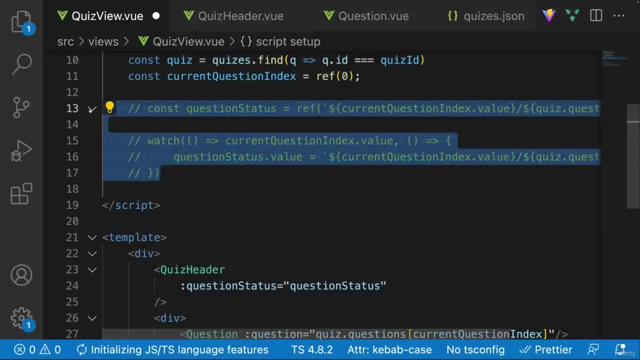 and if this value ever changes the and if this value ever changes the computed status is going to actually computed status is going to actually computed status is going to actually know that and then update this value know that and then update this value know that and then update this value accordingly well enough of the accordingly well enough of the accordingly well enough of the explanation let me just go ahead and explanation let me just go ahead and explanation let me just go ahead and show you what i mean so i'm going to go show you what i mean so i'm going to go show you what i mean so i'm going to go ahead and comment this out and then i'm ahead and comment this out and then i'm ahead and comment this out and then i'm going to say cons and then question going to say cons and then question 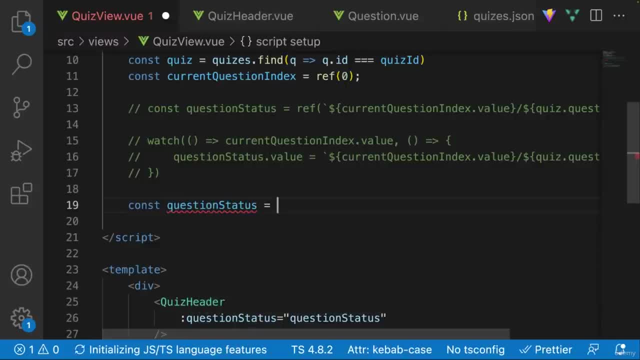 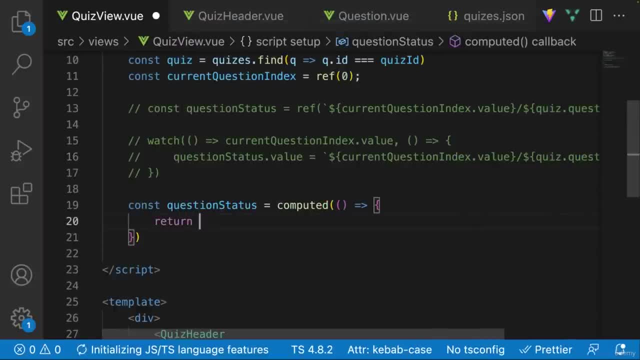 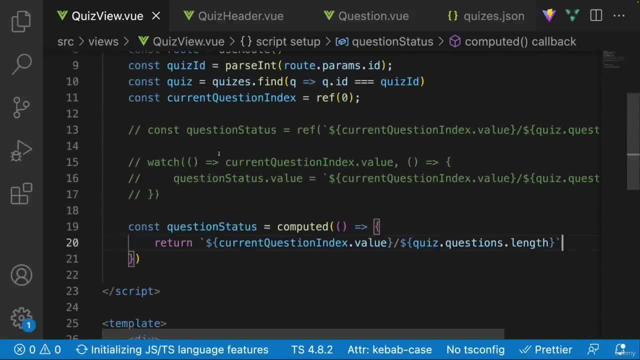 return it's going to return return it's going to return this right over here so i'm going to say this right over here so i'm going to say this right over here so i'm going to say return and i'm going to go ahead and return and i'm going to go ahead and return and i'm going to go ahead and return that return that return that and that right there is actually all it and that right there is actually all it and that right there is actually all it is that we need to do is that we need to do is that we need to do instead of doing these two things right instead of doing these two things right over here and just to prove to you that 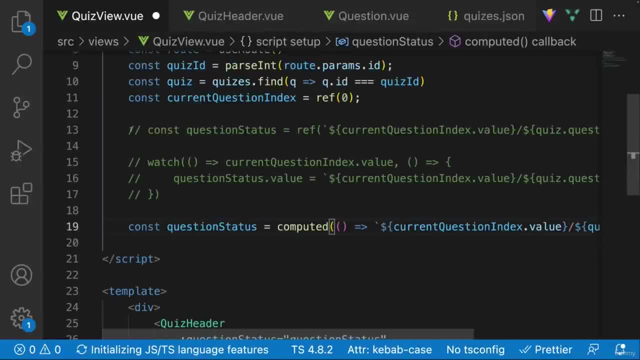 over here and just to prove to you that by just removing the curly braces by just removing the curly braces by just removing the curly braces and you can see we have just removed five and you can see we have just removed five and you can see we have just removed five lines of code lines of code lines of code and we have made one line over here so and we have made one line over here so and we have made one line over here so what this is very simply doing is in what this is very simply doing is in what this is very simply doing is in essence what we did essence what we did essence what we did right here so it listens to any of the right here so it listens to any of the right here so it listens to any of the values that are values that are values that are in this computed function this computed 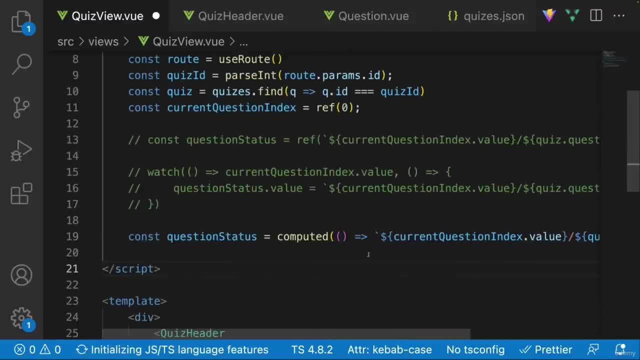 in this computed function this computed in this computed function this computed callback so if any of these change callback so if any of these change callback so if any of these change what it does is it recomputes the what it does is it recomputes the what it does is it recomputes the question question question status which is exactly what we want 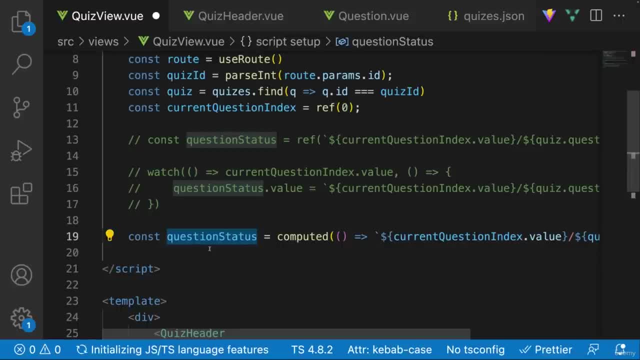 status which is exactly what we want status which is exactly what we want and it treats it like state so if this and it treats it like state so if this and it treats it like state so if this changes is going to changes is going to 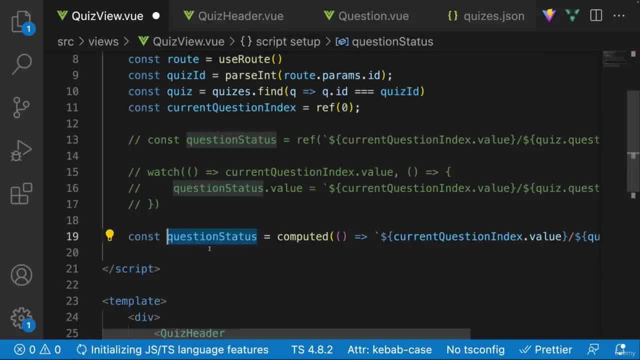 changes is going to re-render any particular component re-render any particular component re-render any particular component that utilizes it so again that utilizes it so again that utilizes it so again we get kind of the best of both worlds we get kind of the best of both worlds we get kind of the best of both worlds by having this very very simple line but by having this very very simple line but by having this very very simple line but we have the same we have the same we have the same exact functionality i'm going to leave exact functionality i'm going to leave exact functionality i'm going to leave this functionality here just as a comment this functionality here just as a comment this functionality here just as a comment just so you can see that this right here 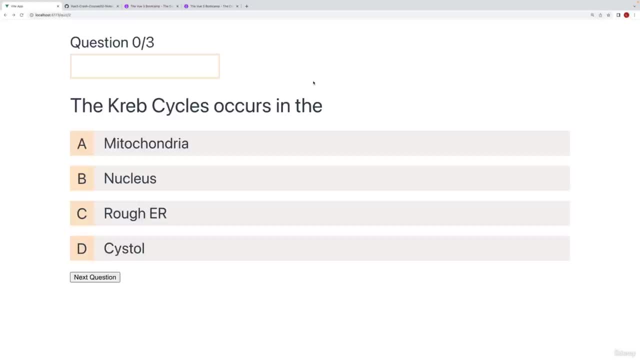 just so you can see that this right here just so you can see that this right here is the equivalent of this is the equivalent of this is the equivalent of this the next thing that we need to pass into the next thing that we need to pass into the next thing that we need to pass into our header right over here our quiz our header right over here our quiz 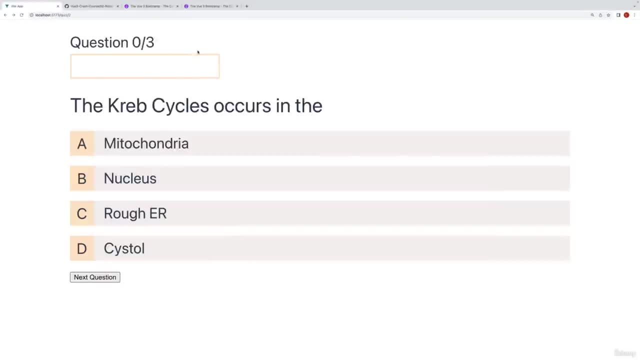 our header right over here our quiz header is the status of our bar now this header is the status of our bar now this header is the status of our bar now this is similarly going to be something that is similarly going to be something that is similarly going to be something that we are going to compute and actually we we are going to compute and actually we we are going to compute and actually we can probably even compute it with the can probably even compute it with the 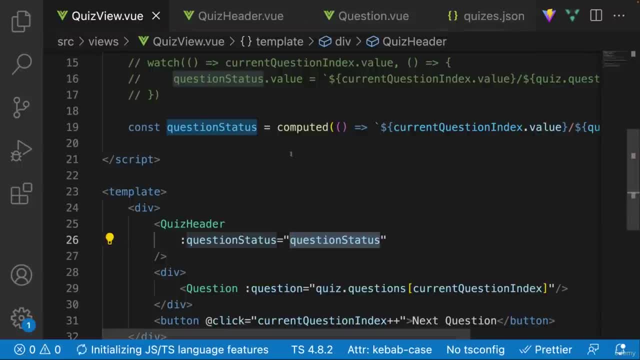 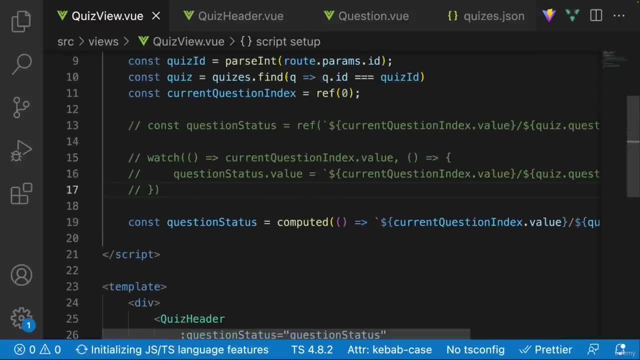 can probably even compute it with the question status within our quiz header question status within our quiz header question status within our quiz header but also we can do it over here and pass but also we can do it over here and pass but also we can do it over here and pass it to our quiz header as well it to our quiz header as well it to our quiz header as well so this is very simply just going to be so this is very simply just going to be so this is very simply just going to be the division of the current question the division of the current question the division of the current question index divided by the length of the index divided by the length of the index divided by the length of the questions in this particular quiz and questions in this particular quiz and questions in this particular quiz and then what we're going to do is just add 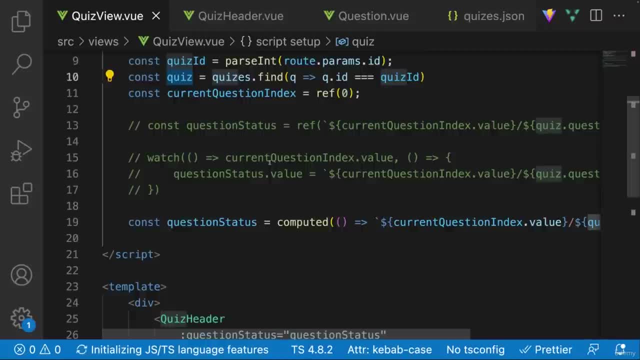 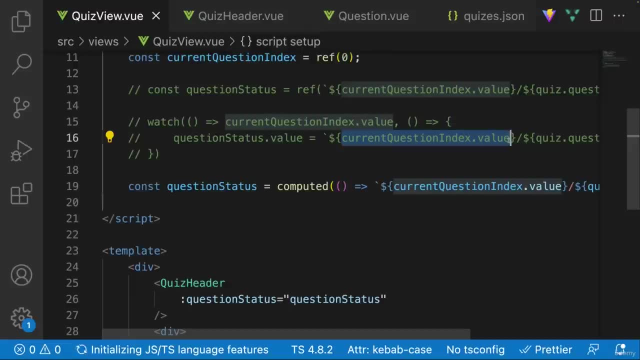 then what we're going to do is just add then what we're going to do is just add a percent sign to it because this is a percent sign to it because this is a percent sign to it because this is what we're going to utilize to style our what we're going to utilize to style our what we're going to utilize to style our app so this of course is going to be a app so this of course is going to be a app so this of course is going to be a computed value because this value is computed value because this value is computed value because this value is going to be dependent on the value of going to be dependent on the value of going to be dependent on the value of this so let's just go ahead and actually this so let's just go ahead and actually this so let's just go ahead and actually create that so let's just say here const create that so let's just say here const 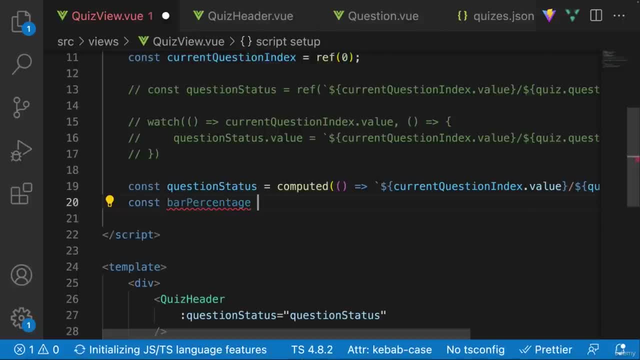 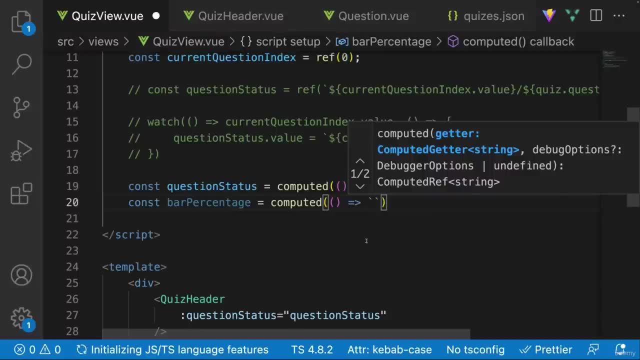 create that so let's just say here const i'm going to say bar percentage i'm going i'm going to say bar percentage i'm going i'm going to say bar percentage i'm going to say computed to say computed to say computed and this is going to be a function and and this is going to be a function and and this is going to be a function and very simply this function is going to very simply this function is going to very simply this function is going to return a string and we'll use template return a string and we'll use template return a string and we'll use template literals for this and we're going to do literals for this and we're going to do literals for this and we're going to do a dollar sign and then curly brace and a dollar sign and then curly brace and a dollar sign and then curly brace and we're just very simply going to do 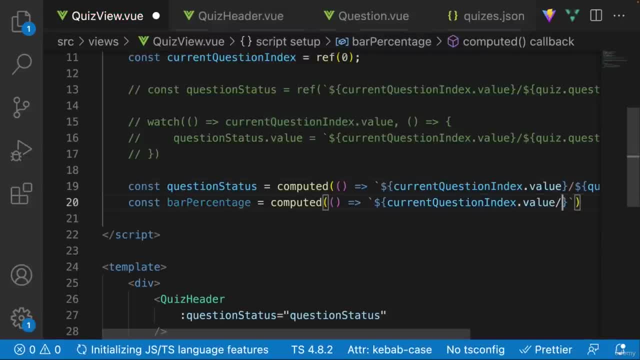 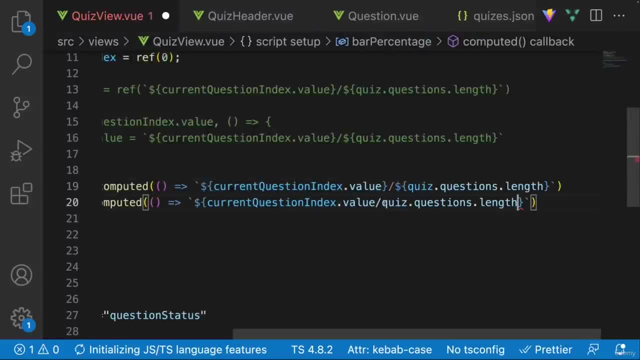 we're just very simply going to do we're just very simply going to do the current question dot value and then the current question dot value and then the current question dot value and then divided by we're going to divide that by divided by we're going to divide that by divided by we're going to divide that by the length the length the length and then we're going to multiply it by and then we're going to multiply it by and then we're going to multiply it by 100 to get the actual percentage so 100 to get the actual percentage so 100 to get the actual percentage so we're going to we're going to divide we're going to we're going to divide we're going to we're going to divide them so if it's 0 divided by 3 it's them so if it's 0 divided by 3 it's 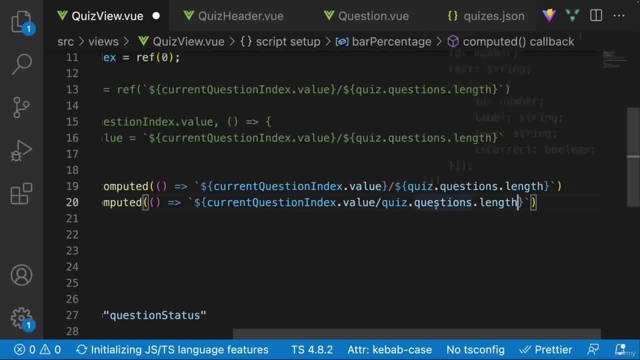 them so if it's 0 divided by 3 it's going to be 0 times 100 so 0 if it's 1 going to be 0 times 100 so 0 if it's 1 going to be 0 times 100 so 0 if it's 1 divided by 3 it's going to be 0.333 divided by 3 it's going to be 0.333 divided by 3 it's going to be 0.333 times 100 so it's going to be around 33 times 100 so it's going to be around 33 times 100 so it's going to be around 33 so let's go here and let's do times 100 so let's go here and let's do times 100 and then over here we're going to add the percentage shine so we can have 33.33 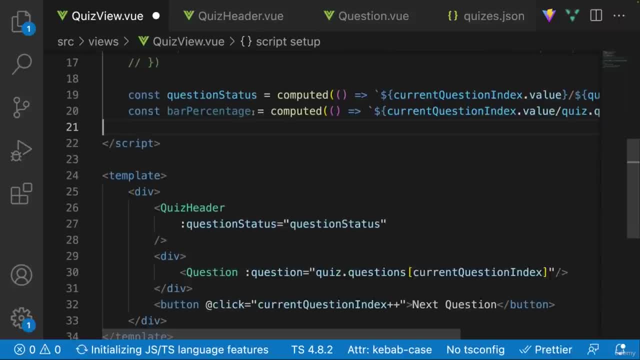 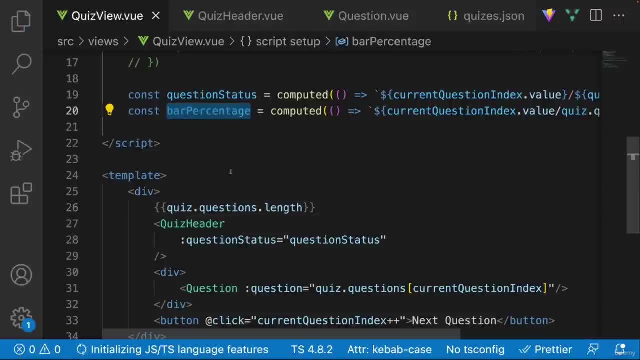 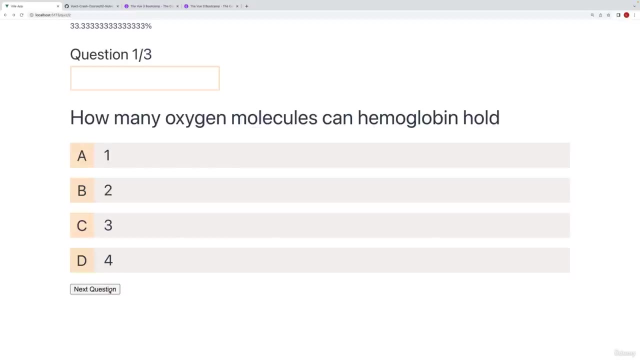 percent so we can actually pass that into the quiz header so that's pretty much all it is that we need to do let's just quickly verify that this is indeed working the way that we expect it to so let's just go ahead and actually log this in here save that and as you can see here it starts off at zero percent moves on to 33 then 66 all right really cool stuff all right so let's go 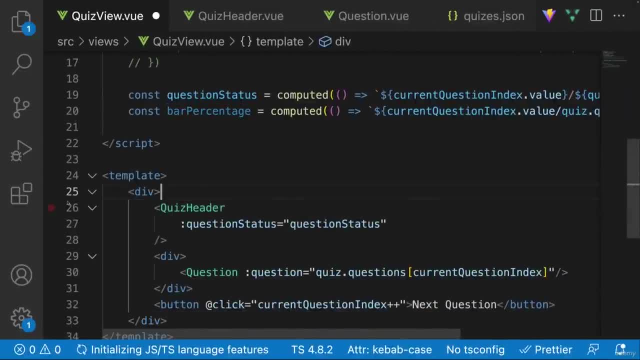 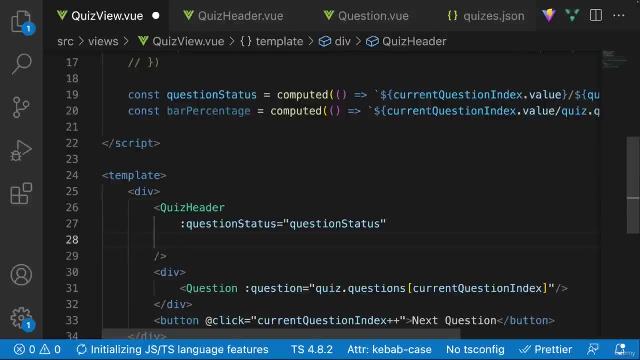 ahead and actually pass this as a prop now so far we've only really been passing one prop at a time but we can actually pass multiple props to a component so over here we can actually say 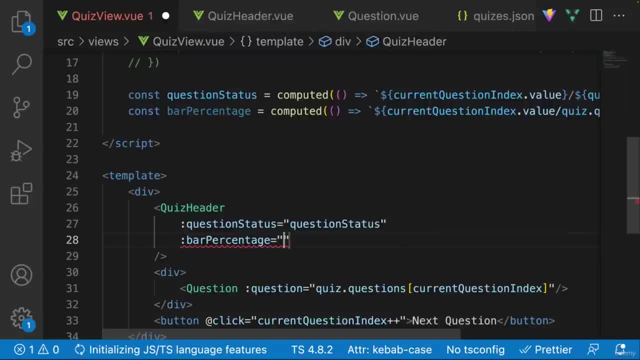 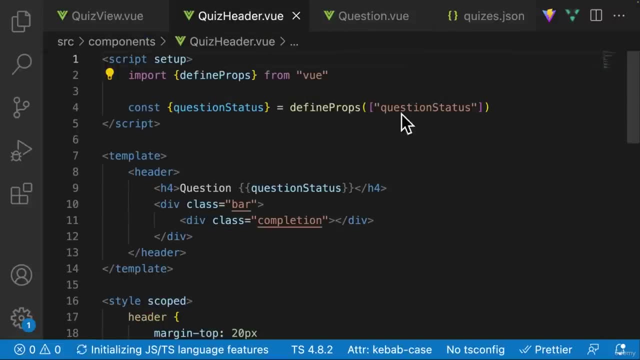 another prop and we can call this well bar percentage and over here i can go ahead and say bar percentage so now we have passed in two different props and now we can actually utilize that prop within our quiz header so let's go ahead and extract that prop from here and we can also define that as another string within our array 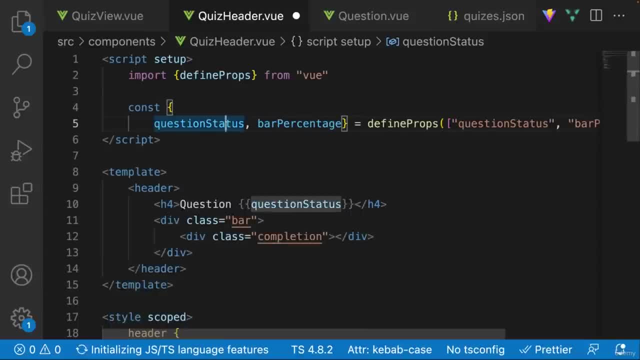 and just so i can make things clear we can actually have multiple different lines so this is just a kind of a syntax thing you can either get a formatter that's just going to 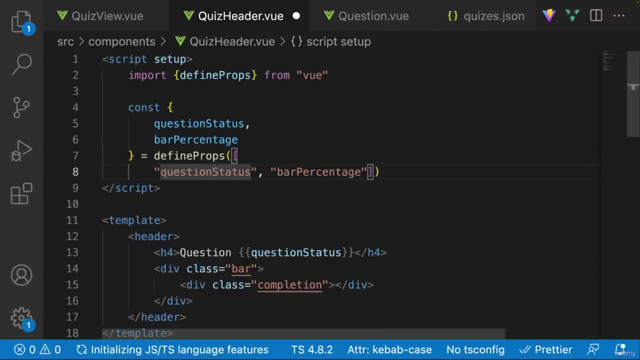 automatically do this for you or you can just do it yourself let's go yeah this looks good 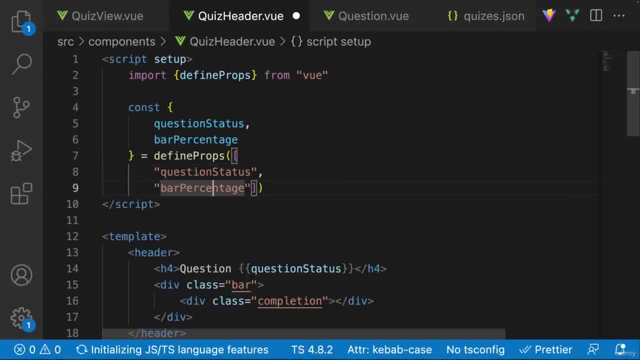 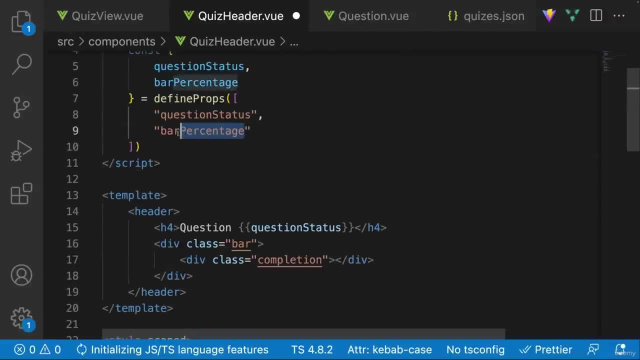 and this looks great as well and let's get rid of that and that there we go what nice and beautiful all right so now we can actually utilize the bar percentage as a style for the 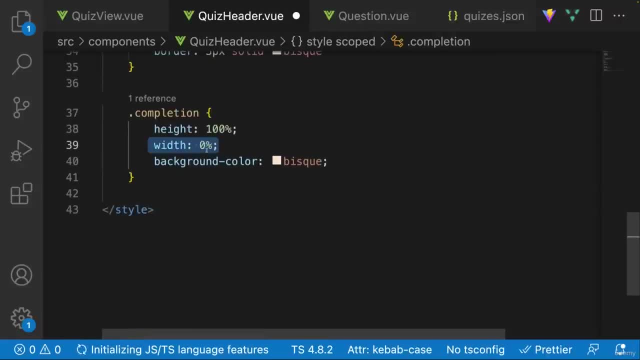 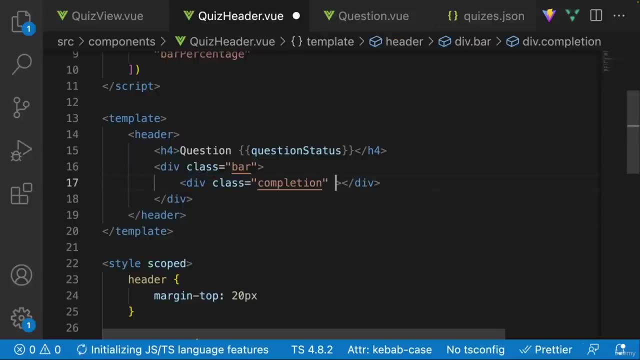 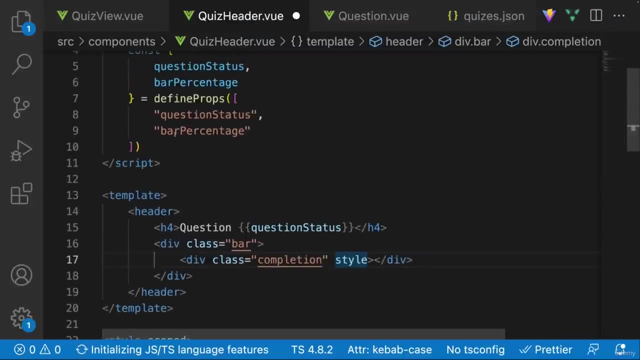 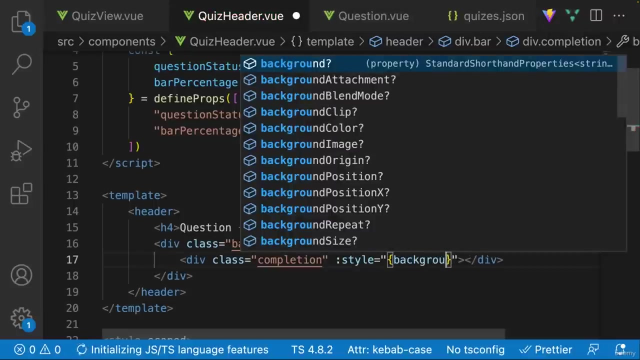 width so remember we actually hard coded the width to be zero percent but now we want to dynamically do it with javascript so over here what we can do is we can define the style so we can say style but this time this is going to be dynamic and from javascript so we're going to add the colon to make this a directive a vbind directive we're going to say that this is going to be equal to some strings and then over here we're going to define the style so we're going to say background or sorry not background color we're going to say width and 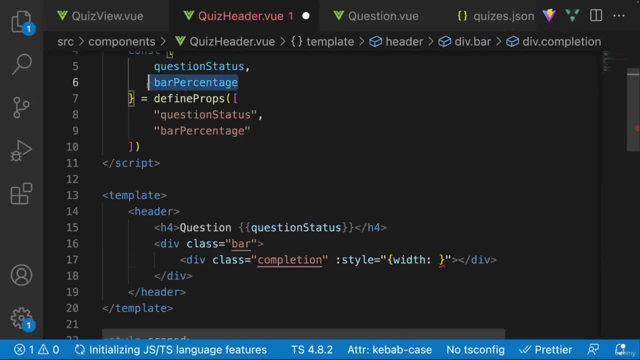 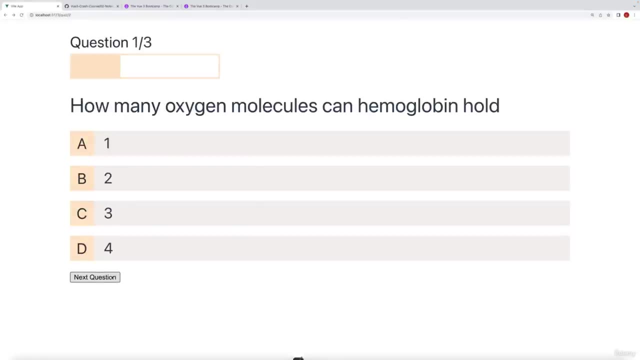 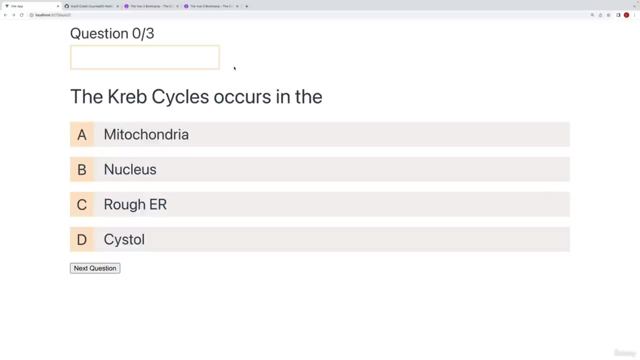 this width is going to be well the bar percentage that we have just defined so you can say bar percentage like so and that's pretty much all we have to do so if we do a quick little refresh you can see here that the bar percentage is working so now we get this working as well as this working and everything is working a okay all right my good friends i think we are in a wonderful position at this point we have our header we have our question and when i click on 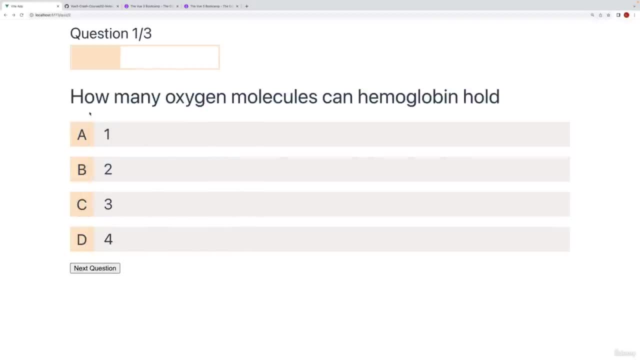 this particular button you can see that everything is updated accordingly the question has changed as well as the options and over here our header is updated correctly now this seems all fine and dandy but of course we do not want to have this button over here that is going to move us on to 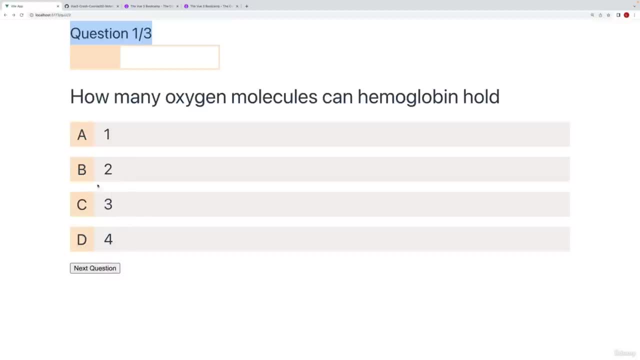 the next question we only really want to move on to the next question when we select a particular option so once i select a particular option do i want to move on to the next question and then if i select another option then i'm going to move on to the next question and so on and so on so of course we do not want to have this button we really only added it for testing purposes all right so you might be thinking well that's going to be really easy all i can do is pretty much just do 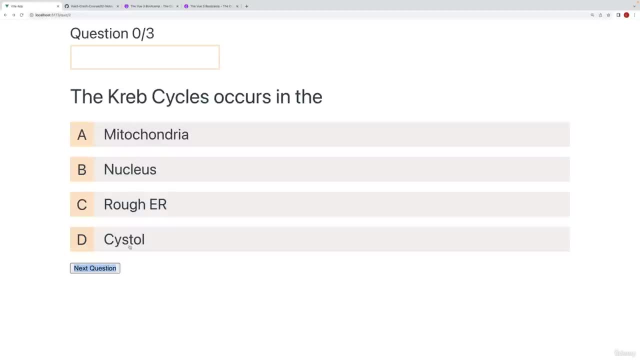 what i did over here for this button and i can do the same thing within these options and if you thought that well you're kind of 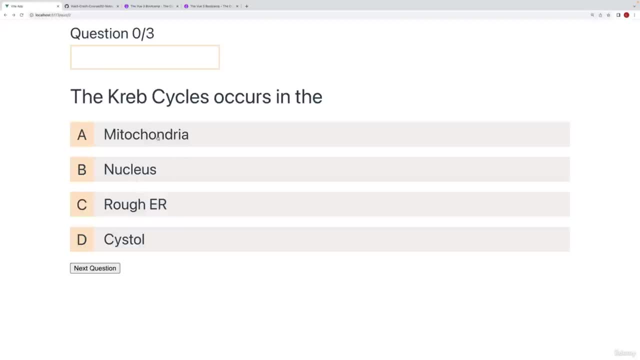 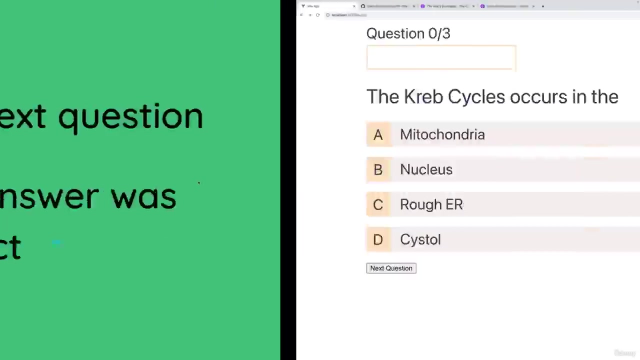 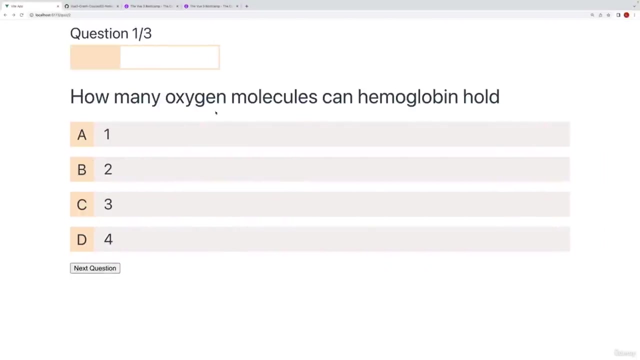 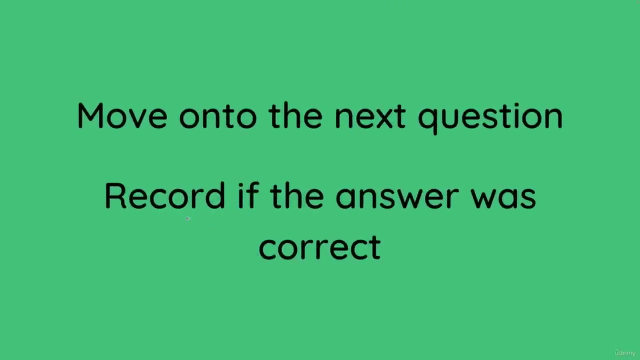 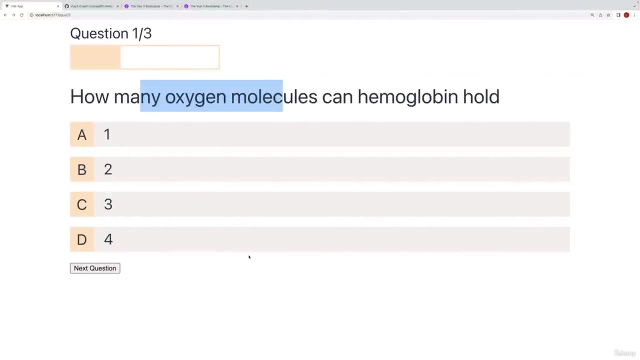 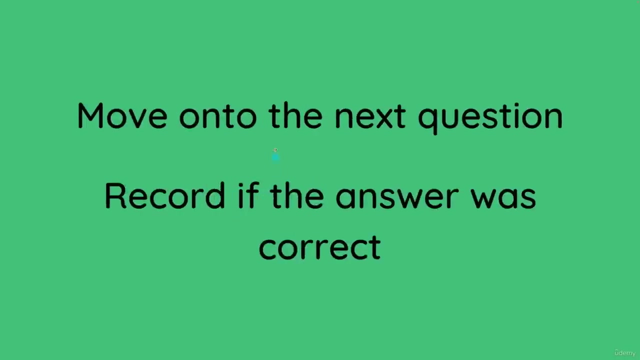 wrong because actually having this functionality within the options is going to be a tad more complicated than having the functionality within the question and let me tell you exactly why so when i select a particular option i actually want to do two different things so the first thing is of course i want to move on to the next question and we've seen that with the button so we want this functionality the other thing that we want to do is eventually we want to record the button we want to record the button we want to record the button we want to record if the answer that the person has answered is correct or not because at the very end of the quiz you want to display the results so you got four out of five right or three out of five right so for example how many oxygen molecules are in hemoglobin i think it's four so if the person selects three you want to say oh they got it wrong that means so far they have zero right but if they selected four then oh they got one right so i'm gonna well say now they have one right move on to the next question and let's say that they select this one which is let's say this one is right then it is going to increment the right value by one now they got two right and at the very end of the quiz once we reach it what we want to do is display a you got two out of three correct so we want to store that information now in order to understand exactly where to store the 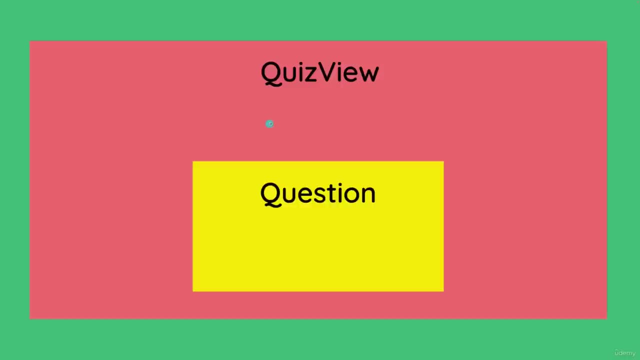 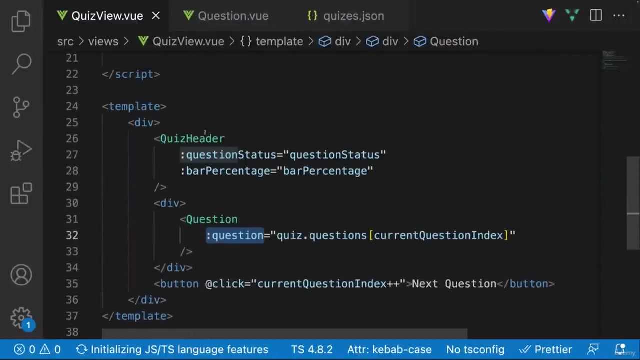 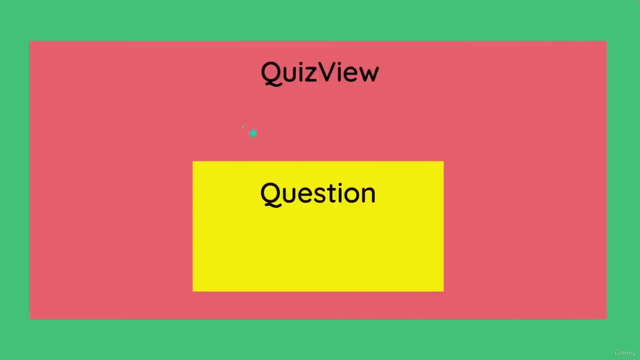 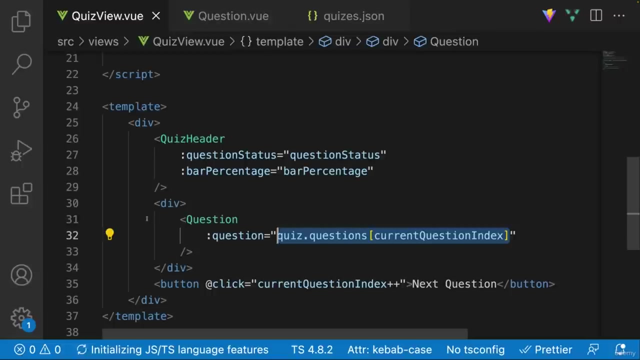 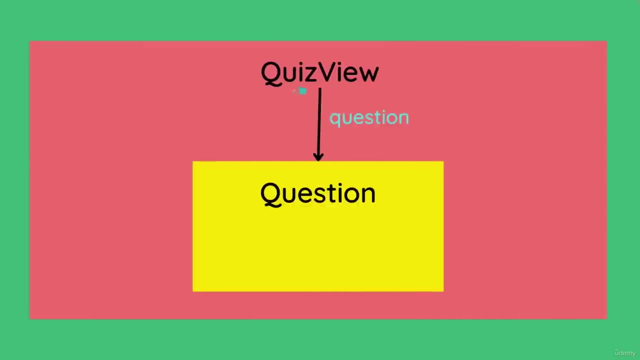 information let's just look at our component structure so right now we have our quiz view component and within our quiz view component we are rendering the question component so this over here is the parent component and this is the child component because this component is rendered within the parent and of course we can always see this so we can go to the quiz view component and right over here we are rendering the question component now let's talk about exactly how communication happens across these components so for example if the question component says that I want to store this information I can go to the quiz view component and I can see that this needs information from the quiz view component about let's say which question you need surrender so which question and which options it should have well we will provided that information through props so we pass that data down through a question prop and again of course we can see that right over here so this information lived inside of the quiz view component but we passed it down to the question component through this question prop all right so this makes quite a bit of sense so we have a question component we have a quiz view component we're passing data in through props in this case it is the question prop now eventually once we reach the end of the quiz what we're gonna want to do is not display a question component but maybe 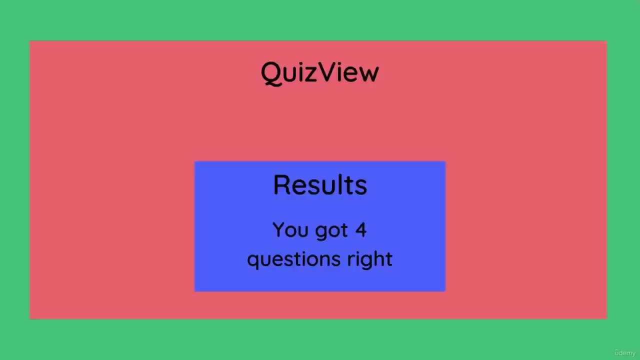 completely remove that component and then instead display the results component and then over here within the results component you can say hey you got four questions and you got five questions and you got four questions right so something like that and this actually kind of presents a tricky problem so the problem is well where is this data going to live how is the results going to know exactly how many questions it got right and well in this case what we're gonna need to do is actually pass that down from the quiz view component down to the results component so what we're gonna need to do is basically have a quiz view component and then pass that down through the results component so this number of correct answers needs to live inside of the quiz view component now this kind of presents a little bit of a tricky problem so let's actually just go through that quiz again from the very first question so we're rendering a question component and then we're going to have a question component and let's say that this person answers the question incorrectly so as soon as they answer a question incorrectly what we want to do is actually modify the state values within the quiz view component so even though the action itself has taken place inside of this component we want to modify the state in the quiz view component so this is actually a little bit tricky because well before what we were doing was we were doing a quiz view component and we wanted to modify the 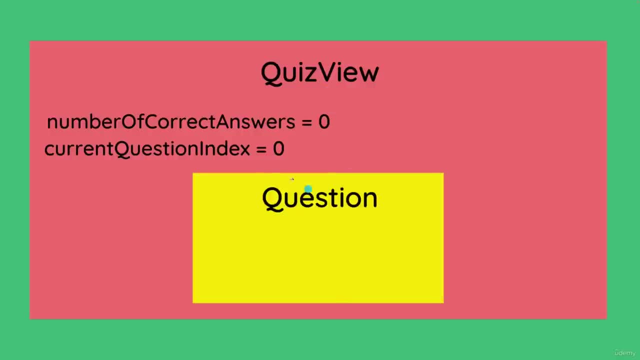 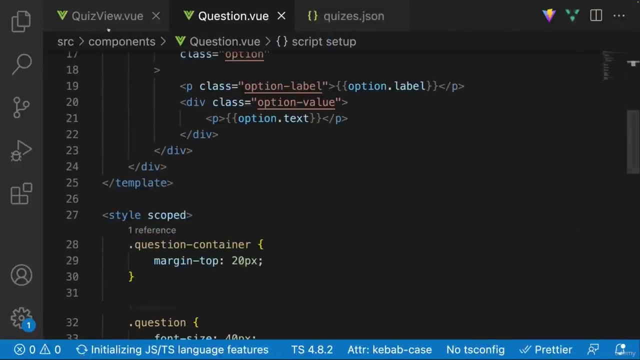 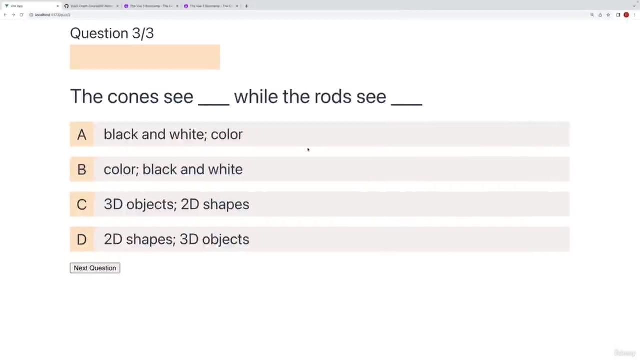 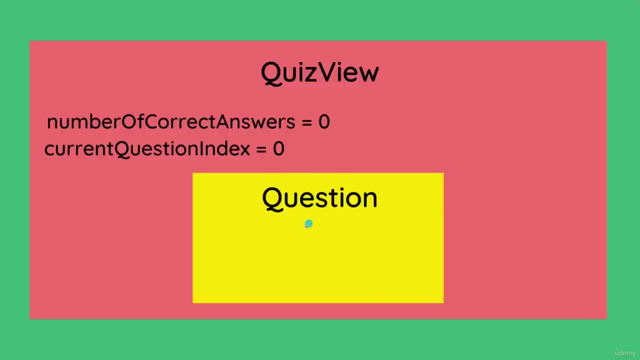 state of the specific question so in this case what we're doing is we're passing information down from the parent to the to the child but now in essence what we want to do is pass information from the child to the parent and we can't do that through props because if I were to go to the question component well I'm not rendering the quiz view component in here at all so how am I supposed to pass that information down as a prop so that's not something that we actually cannot do so let's say this person P33 2 is going to be a pointer at this point and what we're going to do is we're going to do that so instead hey goes ahead and answers it incorrectly somehow some way what i want to do is i want to leave the number of questions number of correct answers to zero but i also want to update the current question index to one just so we can move on to the next uh index so that's what we want to do and now we move on to the next question let's say that this person now or the same person obviously answers this question correctly well now what we want to do is we want to update the number of correct answers to one and the cur current question index to two and then eventually we're gonna reach the end of the quiz and we have all of the information that we need within our quiz view component to well display the correct results so that begs a question how are we going to communicate information from the question component to the quiz view component because again 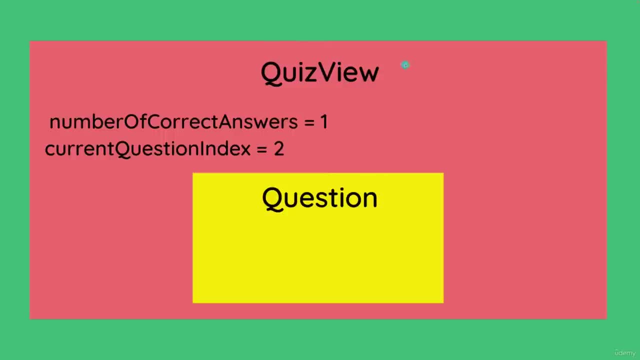 so far what we have been doing is communicating information from the parent to the child, not from the child to the parent. 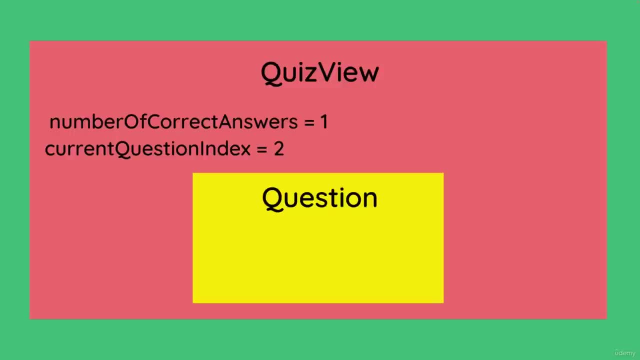 Well, we can actually easily do that by something known as emitting events. Let me show you exactly what I mean. So what we're gonna do here, 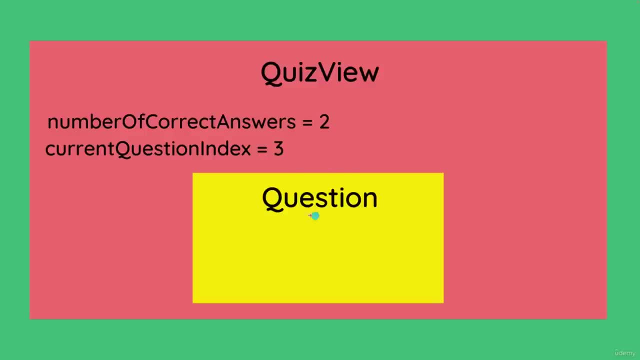 and oh, I just forgot about this example. So let's say that this person goes ahead and answers this question correctly, and then it goes ahead and moves on to the next question. Whatever, nonetheless, let's move on. 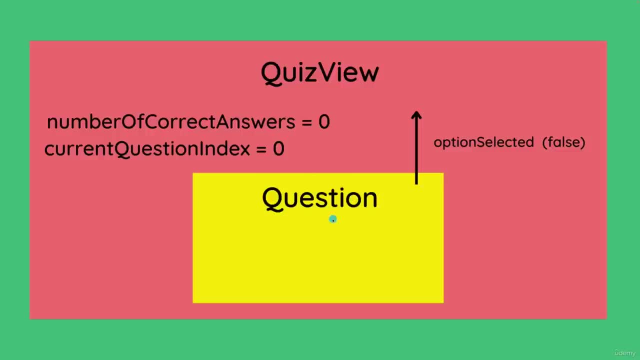 So this is what we're gonna do. So anytime that a option is selected, what we're going to do is we're going to emit an event. And let's say we could call this event whatever we want. Let's say we call this event option selected. And once we emit this event, we can also pass any data that we want. So we can pass in false, true, whatever it is, an object, an array, whatever it is that we want. 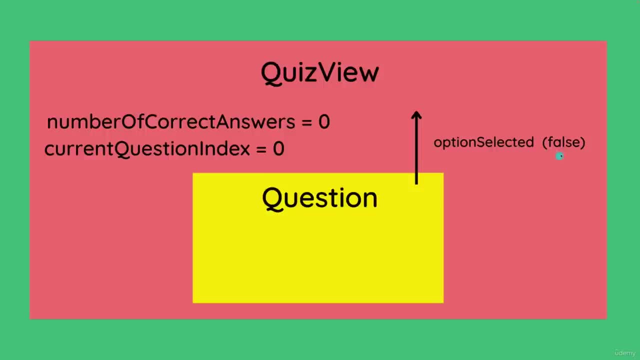 In this case, we're probably gonna just want to pass in a Boolean value, whether the person got the question right or wrong. 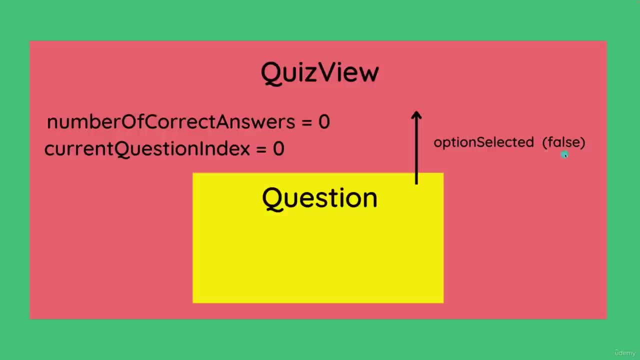 So false or true. So we're gonna go ahead and emit this event. And then the quiz view component is going to continuously listen to this event. Kind of like an event handler, like an at-click handler. 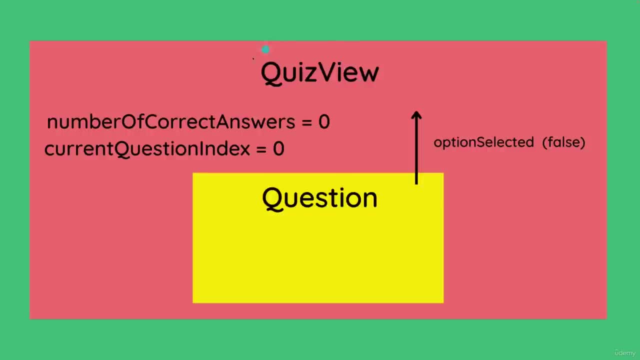 It's going to continuously listen to this event. And well, once this event occurs, it's going to run some sort of logic that we are going to have inside of a function. 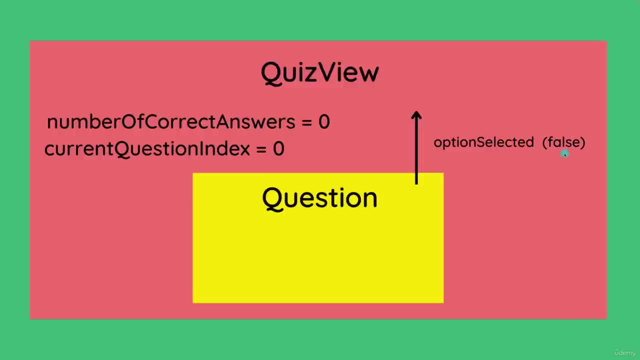 So it's going to listen to this event. It's gonna check, oh, is this false or true? Is this false or true? If it's false, then it's going to keep the number of correct answers to zero, but then it's going to increment this by one, the current question index by one. 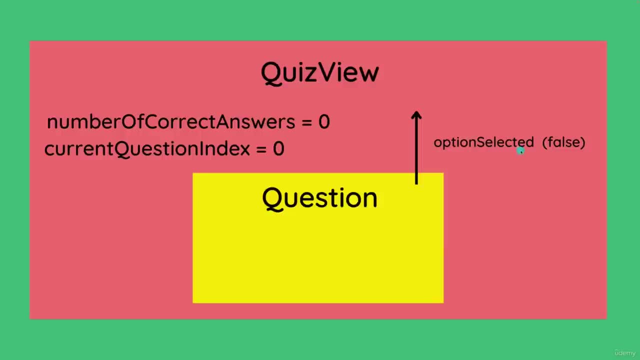 And then let's say we select another option. It's going to go ahead and emit another event. Let's say this time it is true. The quiz view component is going to listen to that event. And then it's gonna say, 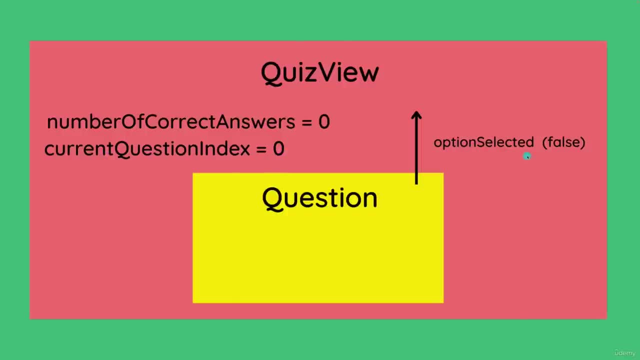 okay, I'm gonna increment the current question index by one. And this time it's true. So I'm also going to increment the number of correct answers by one. 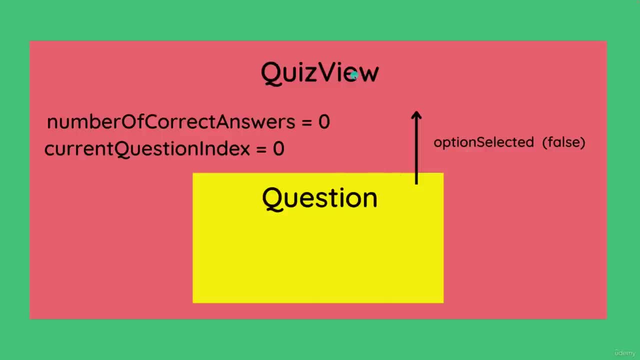 So that is exactly what we're gonna do. In order to get child-parent communication, what we need to do is emit events. So now that we got that, well, got that kind of understanding, that conceptual overview, let's actually go ahead and code it out in the next video. 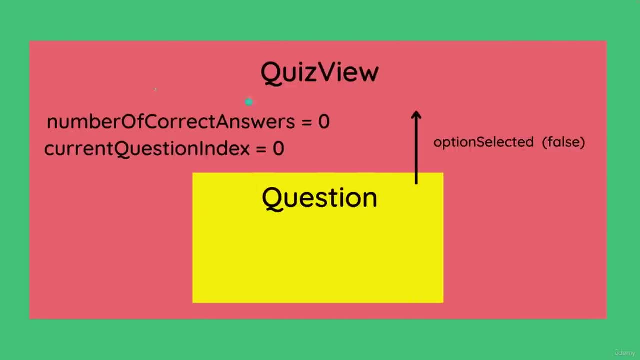 All right, my good friends, in this video, what we're gonna do is actually implement what we talked about. 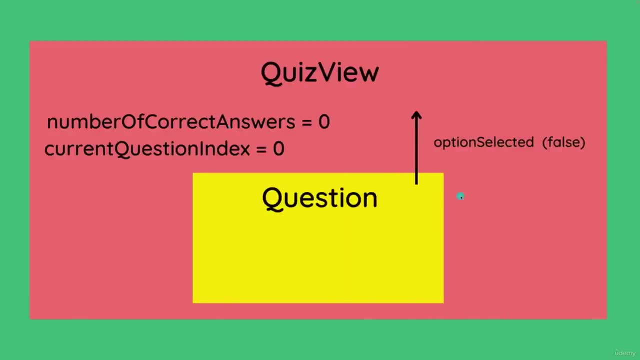 Anytime that we click a particular option, what we're gonna do is emit an event called option selected with a particular value, in this case is going to be a Boolean value. 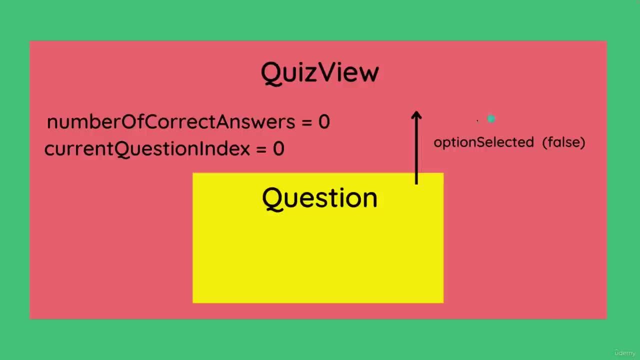 Then the quiz view component is going to listen to that event and run some logic. 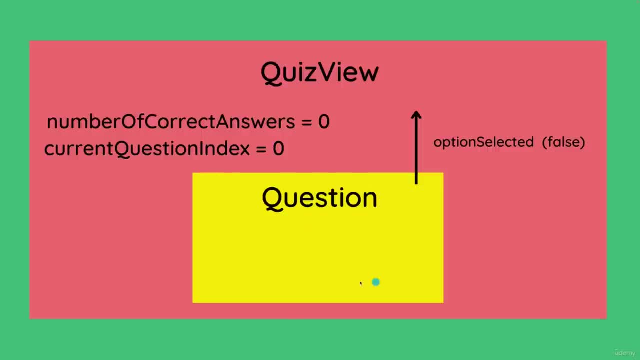 So the first thing that we're gonna do is, okay, when I click this over here, when I click a particular option, let's just go ahead and emit an event. 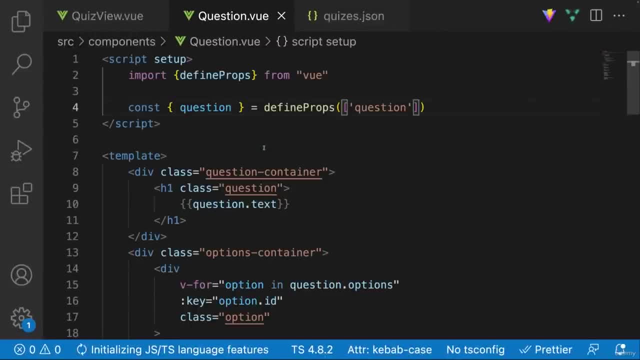 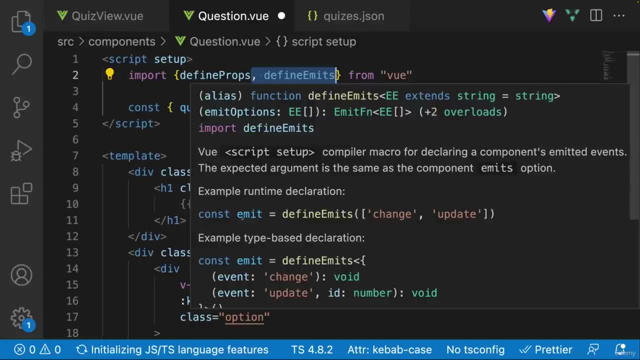 So let's go to our question component. And the first thing that we want to do is we want to grab something called define emit. And that's exactly what we're, that's exactly what it means. We first have to define the emit events that we want. And we use it exactly like this. So we say const emit is equal to define emit. And then over here, we have all of the different events that we can emit because a component can emit multiple different events. 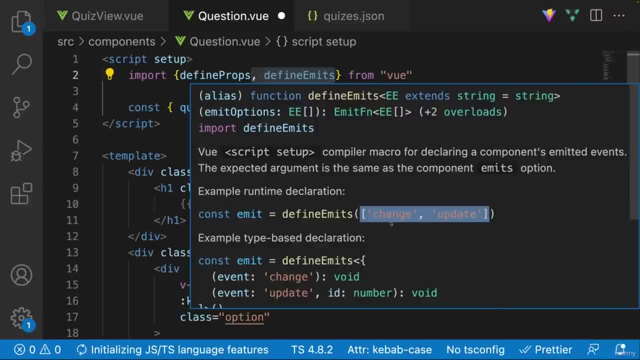 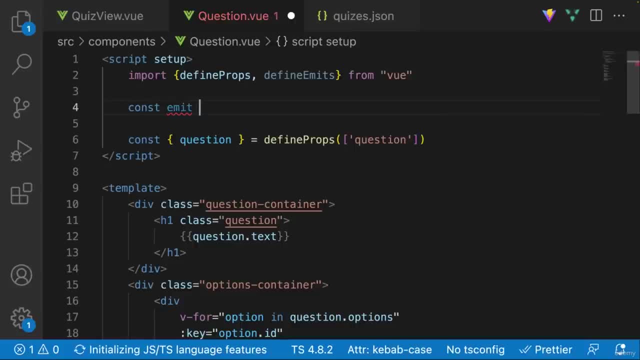 In this case, it's only gonna be one, but again, it can emit multiple. So over here, let's go. And what we're gonna do is we're gonna say, const emit is equal to, and we're gonna say, define emits. And we're gonna say, in this case, we have a select option emit. 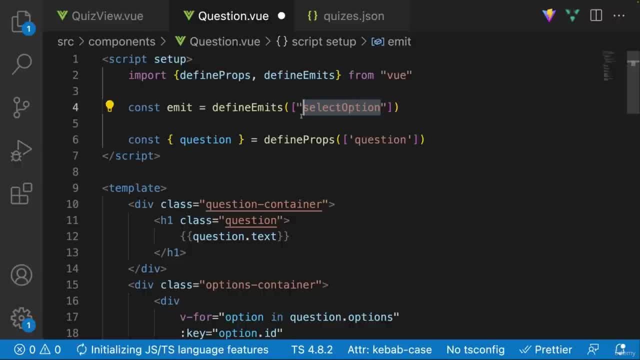 So that's what we did, a select option. All right, so this is looking pretty good. 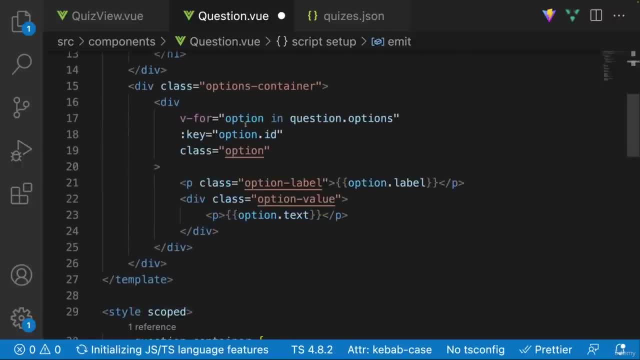 So what we want to do is we want to emit this event anytime that we click on, well, this div, any one of these options. So let's go over here to our div. 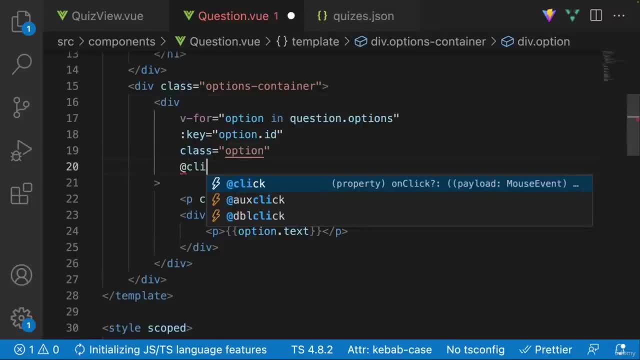 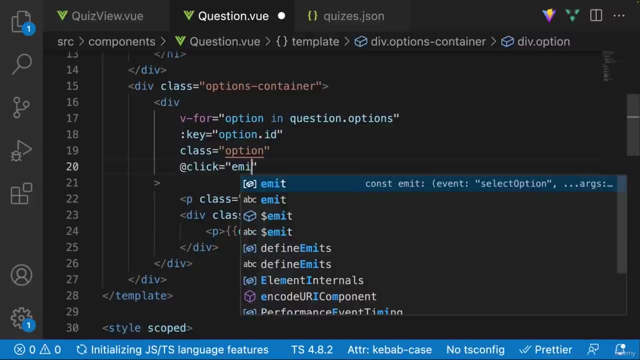 And what we're going to do is we are going to say at click, and let's just run a function called, let's call this function, let's call this function selected option, or maybe we can call this emit selected option. 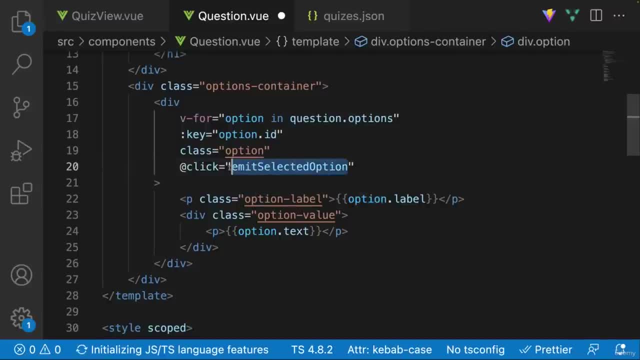 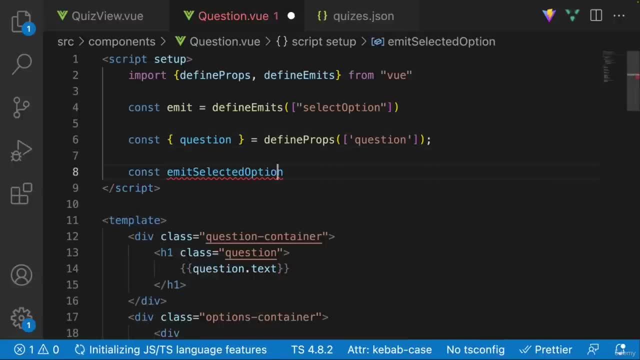 We can call this function, whatever it is that we want. We haven't really created it at this point. So let's go above here and let's just create this function. So I'm gonna say const, and then I'm gonna say emit selected option, and we'll just make this function. Let's make this an arrow function. And once we call this function, what we want to do is we want to pass in whether the person got the question right or wrong. 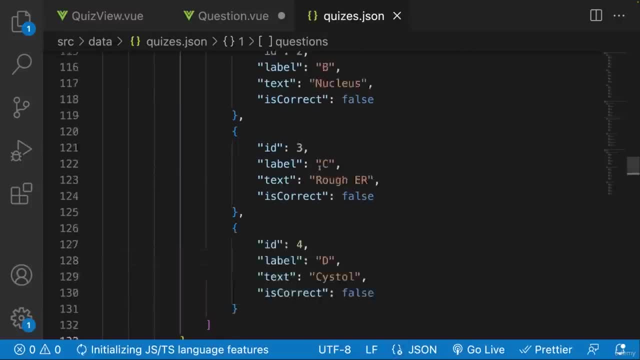 So they could have selected any one of the options. And if you go to the quiz, you can see that each option has a value of is correct, 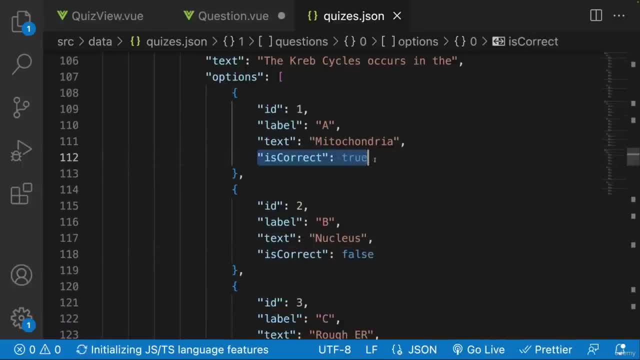 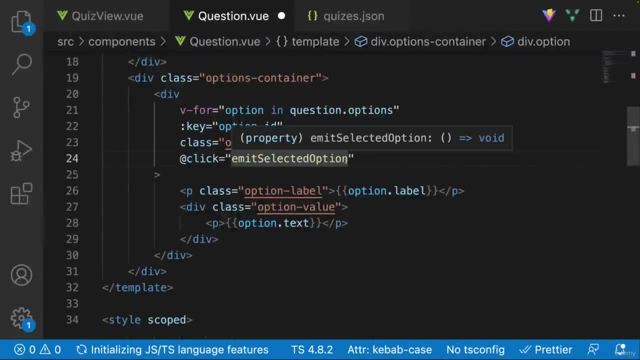 and it can either be true or false. So in essence, what we want to do is we want to pass in the is correct value. So let's go over here to emit selected option. We're gonna go ahead, and pass in some parameters. 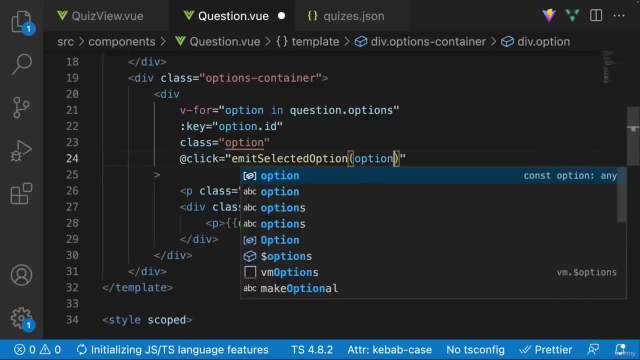 So we're gonna say option, and then dot is correct. So option dot is correct like so. 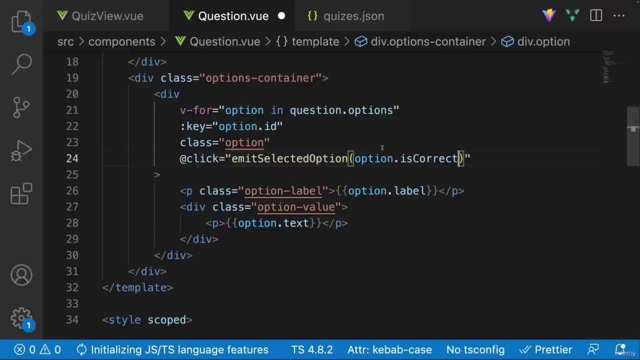 And this is either gonna be a Boolean or, well, a true value. It's gonna be a Boolean value or, well, it's gonna be a Boolean value. It's either gonna be true or false. Hope that makes sense. 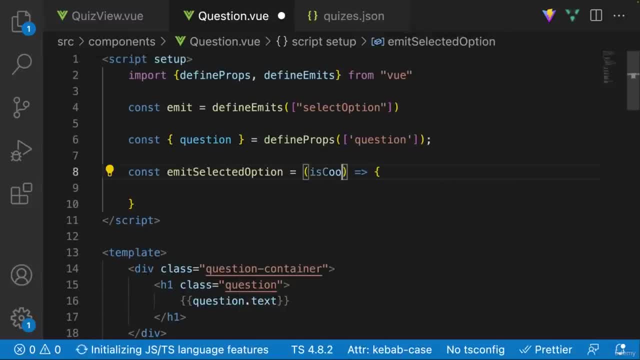 So let's go over here, and we're gonna say is correct. We're gonna get that from the parameters. And what we want to do is, 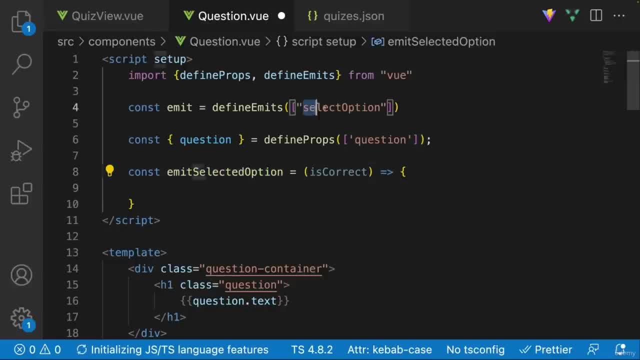 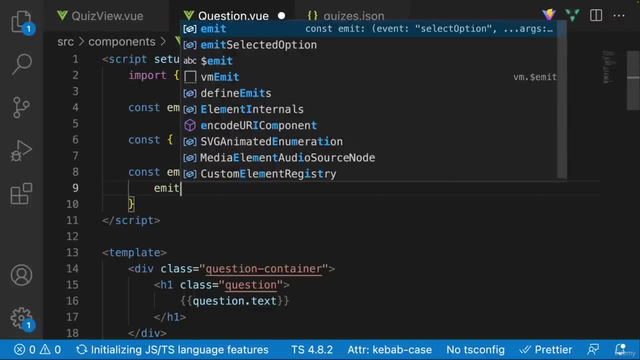 very simply, just emit a select option event, and we want to pass this information within it. So how do we do that? Well, what we do is we call emit, and then we, well, in a string, we select the event that we want to emit. 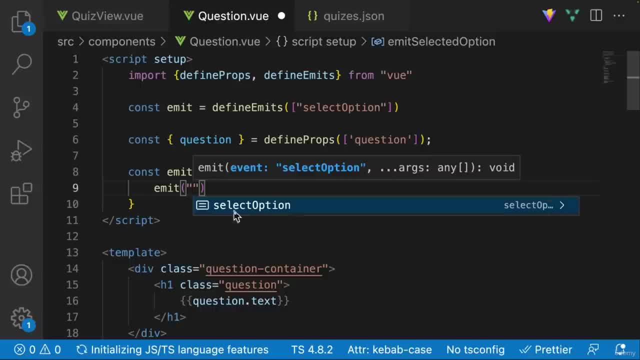 And actually, you can see here, we get kind of this type helping, telling us, well, the only real option that we can emit is this select option. If I went ahead and added another event, and I tried to add a string, it gives me both of these. Now, of course, I want this one. So let's go ahead and remove this. 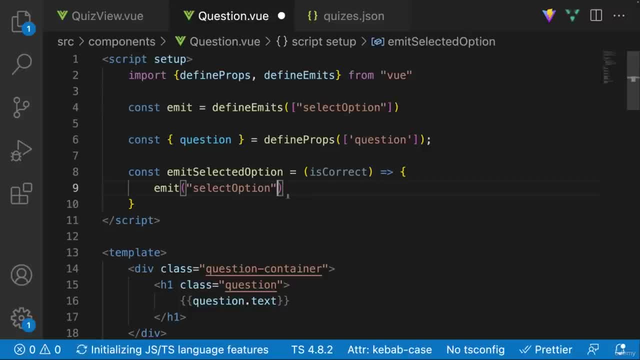 And as the second parameter, we can pass in any data that we want. In this case, what we want to do is we want to pass in the is correct. All right, so that's pretty much it. 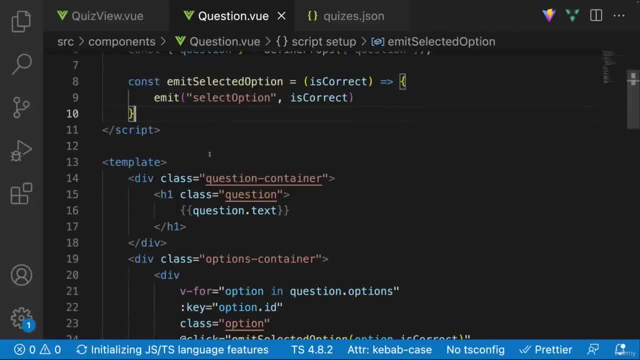 So at this point, we are successfully emitting an event called select option 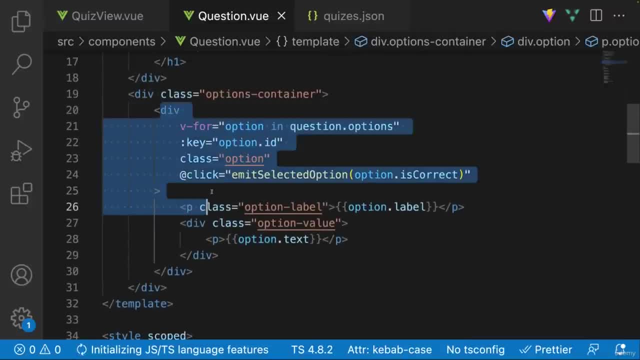 any time that we click on this particular option. So we are completely done with this portion right over here. And let me just do a quick little refresh. There we go. 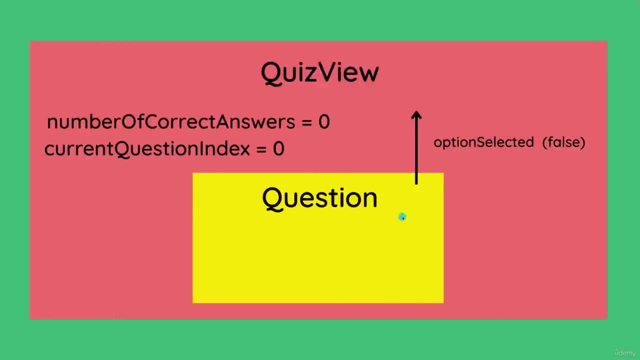 So we're completely done with the question component over here. 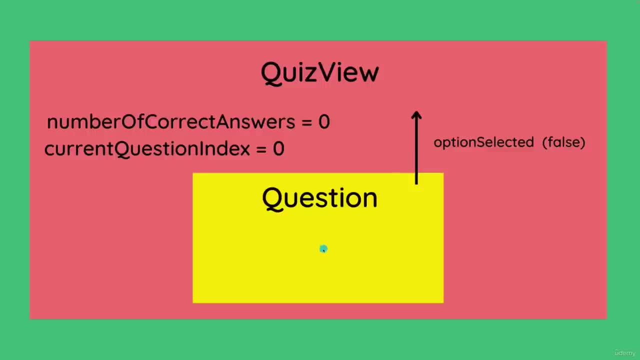 So the question component is indeed emitting event any time that we select an option, and it is passing in the correct information. 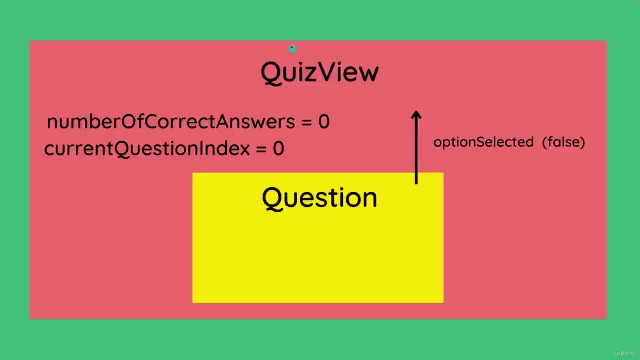 So is it correct or is it not? This Boolean value. 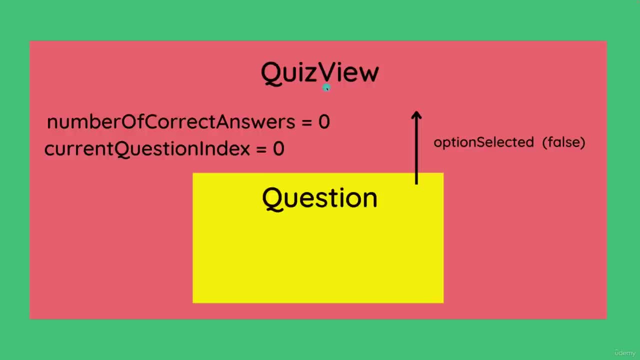 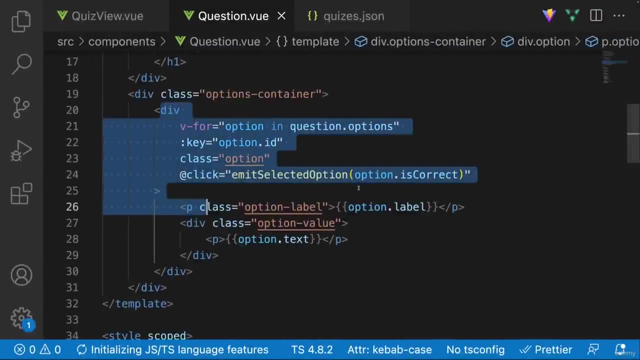 So now what we need to do is actually start working on the quiz view component. So within this component, we need to start listening to this event that we have just created, and then modifying our values appropriately. All right, so how are we going to listen to a particular event? Well, let's remember that our question component is emitting this select option event. 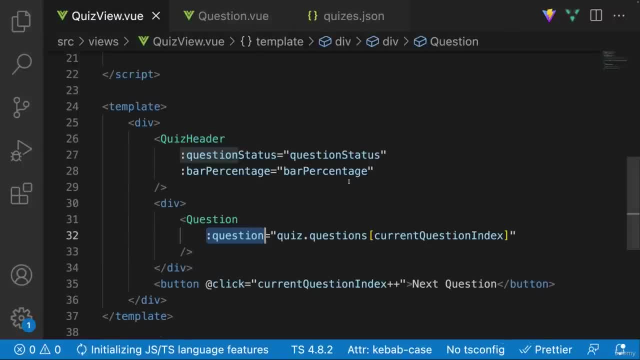 So let's just go ahead and copy that. So in order to listen to a particular event, we actually do the exact same thing that we do when we listen to an event 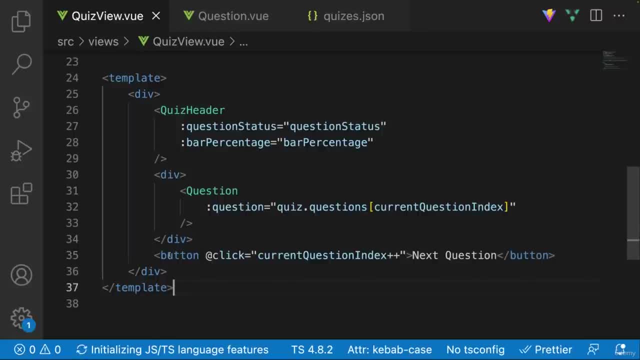 on a regular handler, like on a regular HTML element. So like on this button, in order to listen to it, to listen to a click event, we did at click, and then we ran some logic. 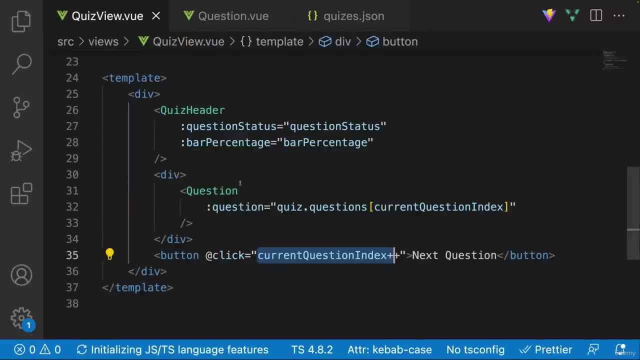 Now, in order to listen to a select option event on this question component, 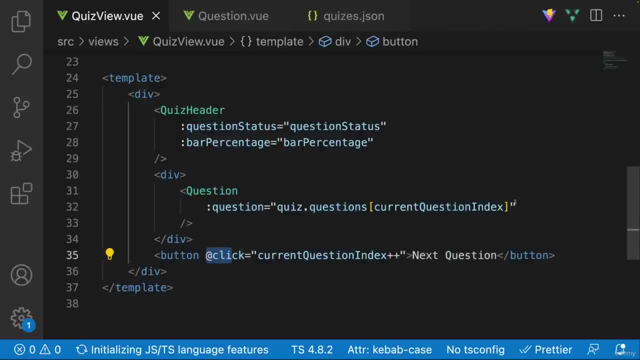 we actually do the exact same thing. So over here, what we can do is we can say at, and then select option. And then once this event is happening, and that's only once it is emitted when we click a particular div on the question component, then we want to run some logic. 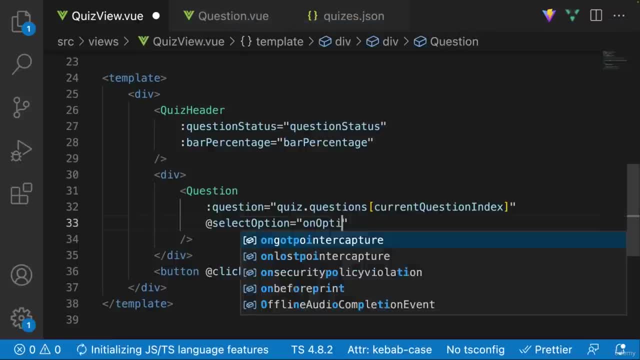 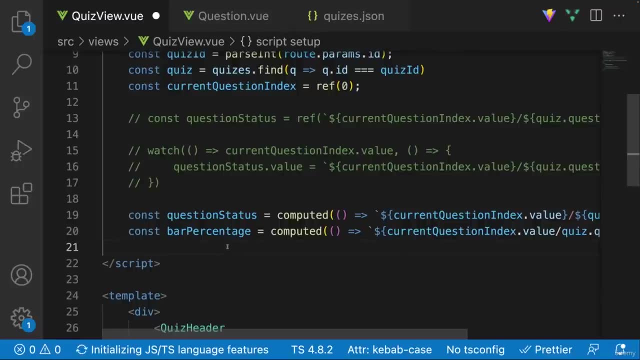 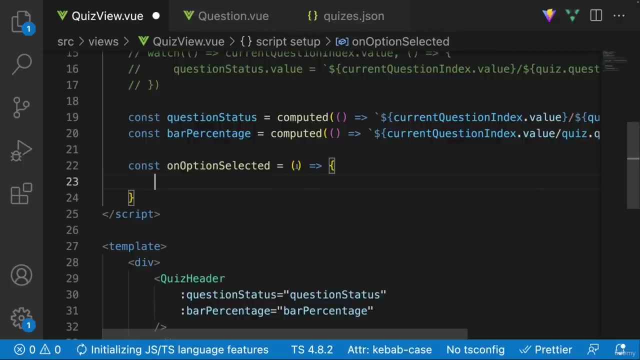 So let's actually go ahead, and create a function called onOptionSelected. Because this is the function that is called once an option is selected. Now we haven't created this function, so let's say const onOptionSelected, and let's go over here, we'll make this a arrow function like so. So over here, this is actually going to take in the boolean value, so whether it's true or false. 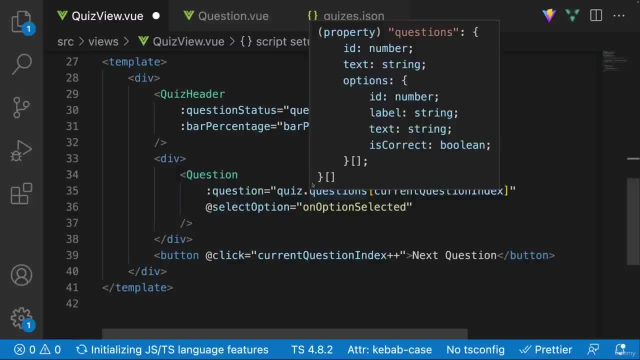 Because remember when we emit this event, we are also supplying it with the boolean value. 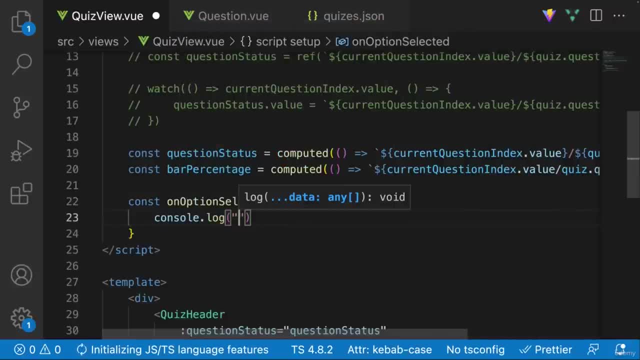 And what we can do just for now, just to see that if this works, let's just go ahead and log emitted event. I'm gonna say is correct, like so. So I'm gonna go ahead and inspect this for now. 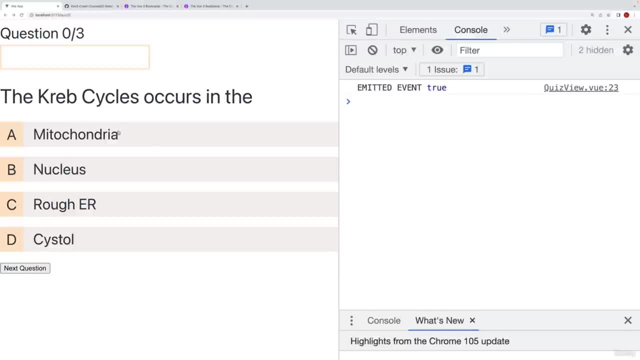 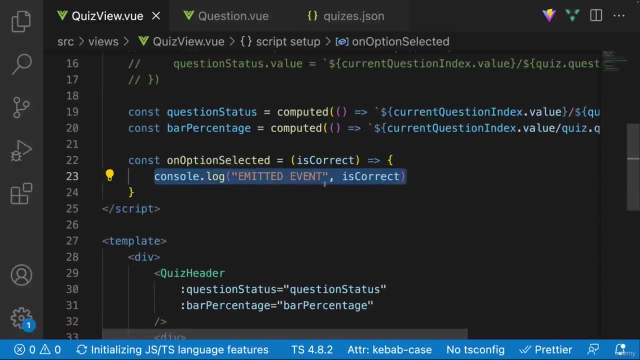 Let's go to the console, refresh. I'm gonna click and as you can see here, emitted event true. If I select this option, emitted event false. Select this option, emitted event false, emitted event false, emitted event true. So you can see that it is indeed actually reaching the quiz view component and it is running the function that we want it to. So in here, well, very simply now, we can just update our logic the way that we want. 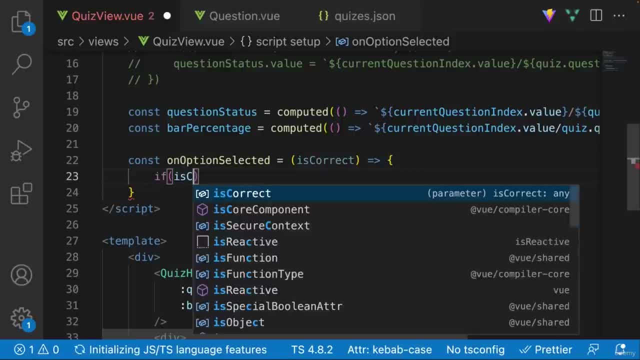 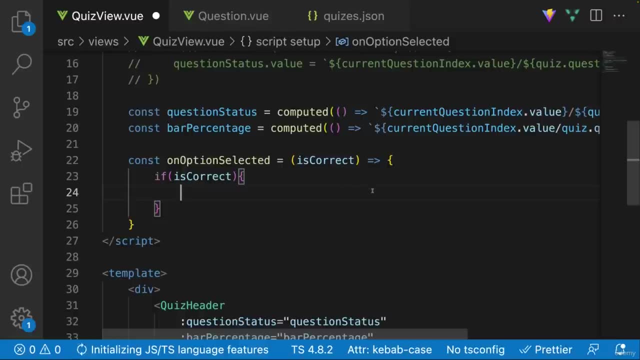 So for example, we can say, hey, if this is correct, so if is correct, then what we can do is we can increment the number of correct answers by one. 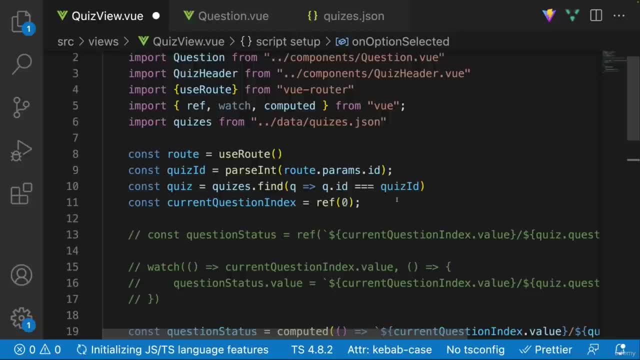 Now, of course, we actually didn't create this piece of state now. So what we're gonna do here is we're gonna create that state right now. 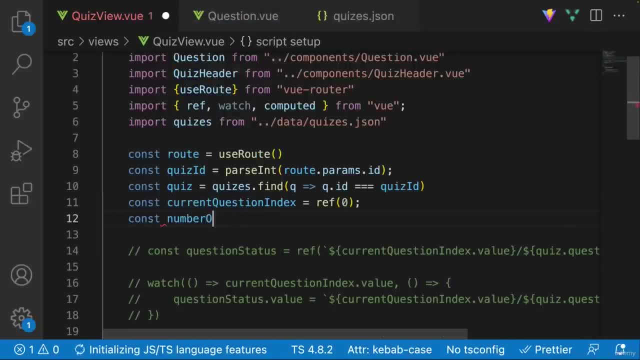 So we're gonna say const, and we're gonna say number of correct answers. 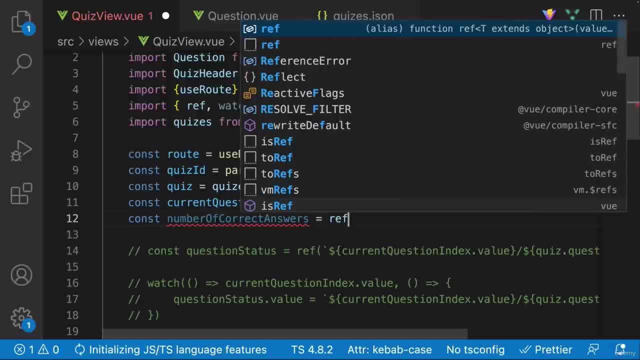 And we're gonna say that that is gonna be equal to ref. Initially, we're gonna say, obviously, this is gonna be zero. 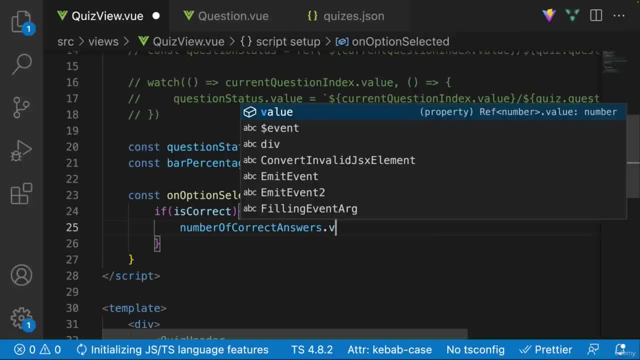 So let's go ahead and actually increment this. So if it is correct, we're gonna say dot value. And then we're gonna say plus plus to increment it by one. 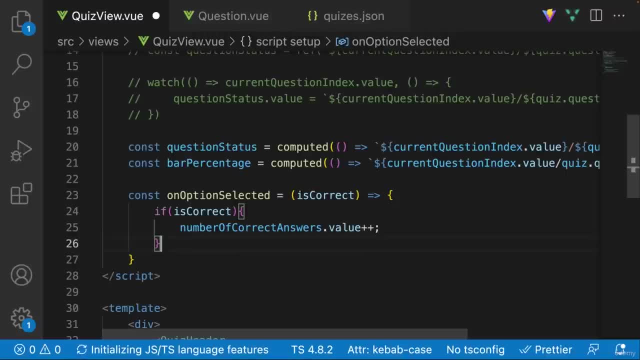 All right, so this is really, really good. So now what we wanna do is, of course, well, we want to go ahead and regardless if the question is right or wrong, we also want to increment the current question index. 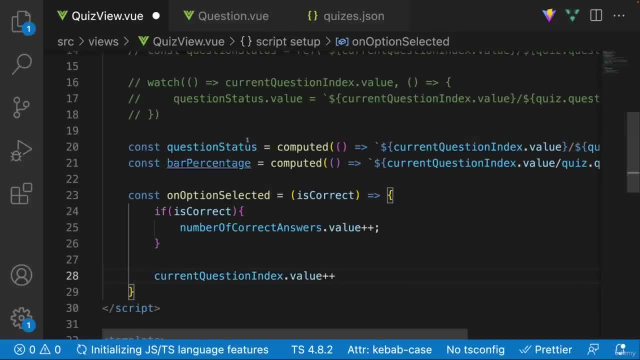 So I'm gonna say current question index dot value plus plus. All right, so that's pretty much all it is. 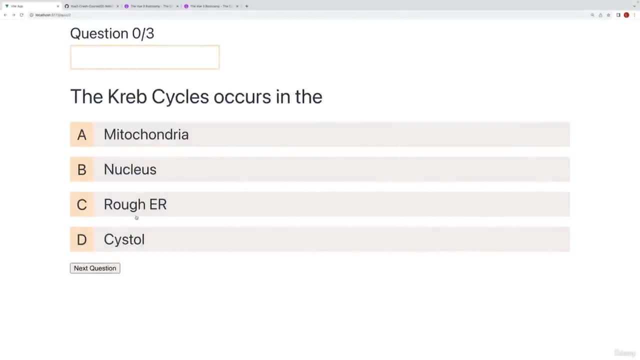 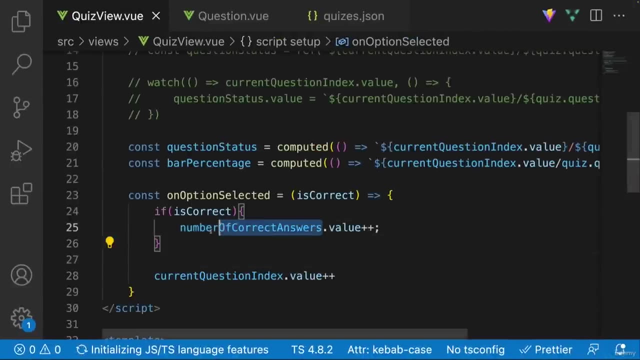 And now, theoretically, if I click on a particular question, it should obviously move us on to the next question. And also, it should also update the number of correct answers. But of course, we're not using that anywhere in our HTML, so we can't really see that. 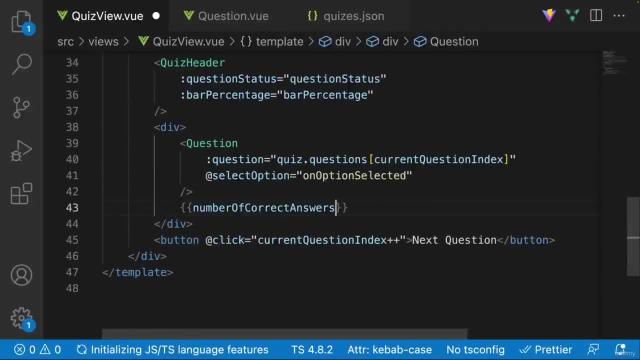 But just to see that it is indeed working, let's just render it anywhere, like render it right here. So now you can see it's zero. 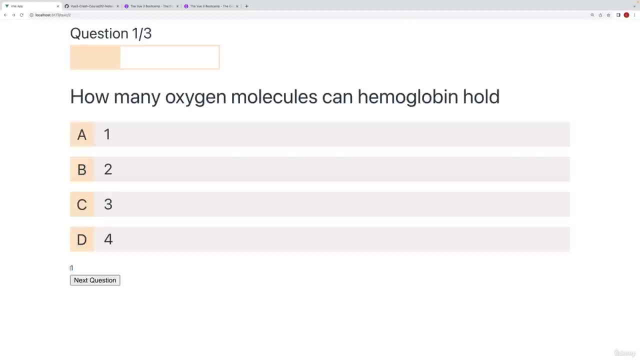 So I'm gonna go ahead and get this answer right, mitochondria. You can see now this is updated to a one. 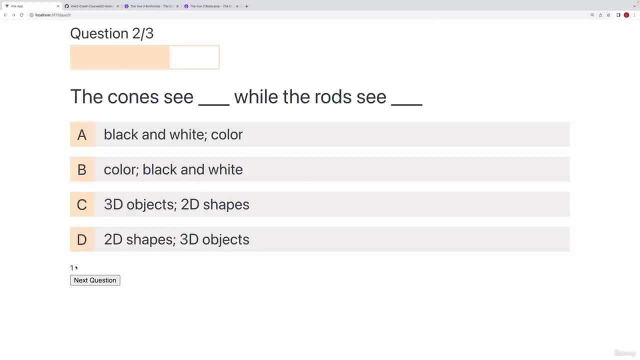 I'm gonna get this question wrong. It's gonna move on to the next question, but it's gonna leave this one at one. 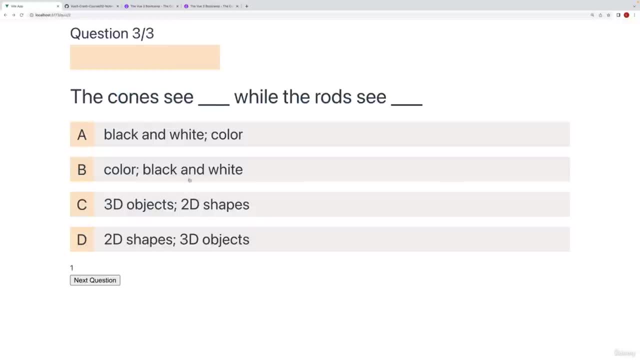 Cones are for color. And then rods are for black and white. I think that was the case. Was that not the case? Let me see. 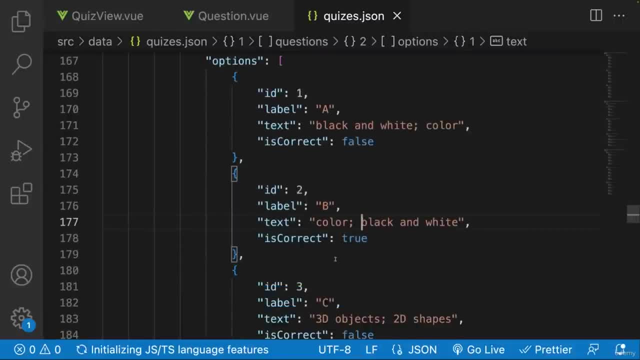 I may have just gotten the question wrong. Let's see here. No, it was correct. Hmm, very suspicious. Let's try that again one more time. 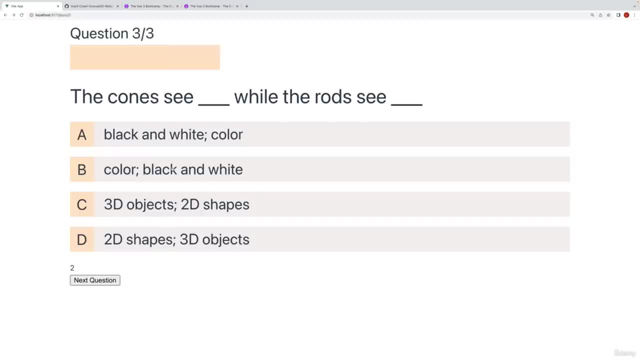 So mitochondria, four, and then here. 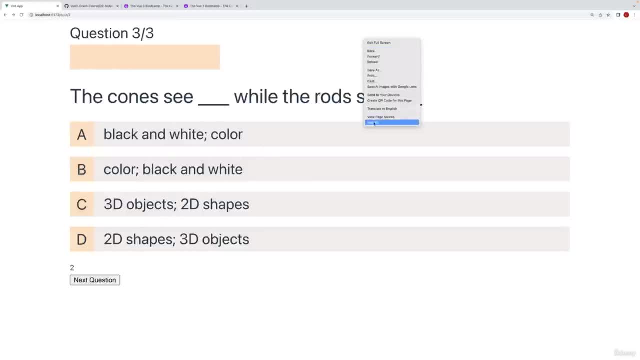 And I think some kind of goofy things are going on. I think what's happening here, and we'll probably fix this later, is we're getting some sort of error. 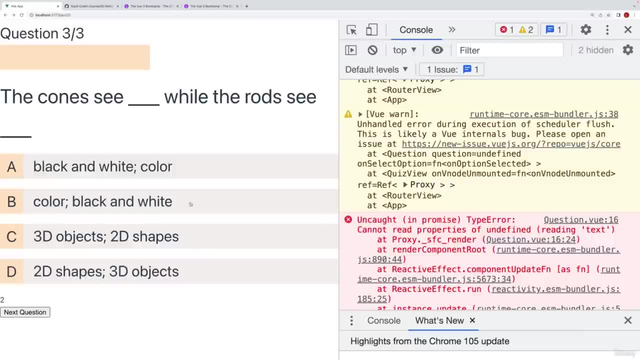 And that's because we're reaching the end of the index. So we'll actually end up fixing that a little bit later. And that's why this isn't working. So let's actually do that in the next video. 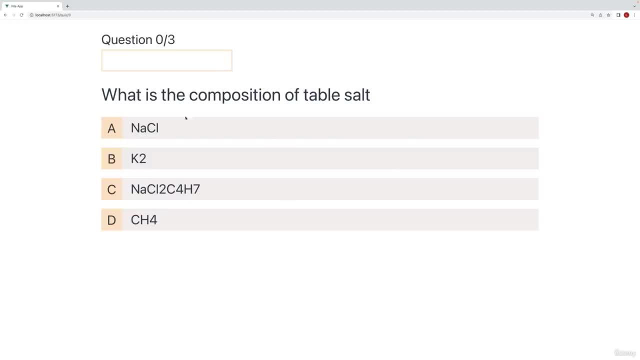 The next thing that I want to work on is what happens when we complete the quiz. Right now what happens is if we complete the quiz, well, we can just continue going answering this final question, and it just continues and continues and continues. 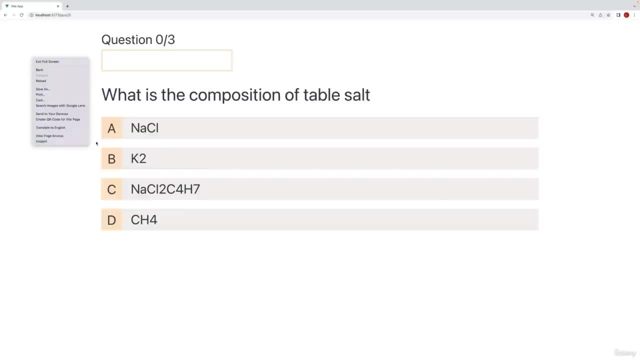 So of course, this is not what we want. And actually, it's going to trigger a bunch of different errors 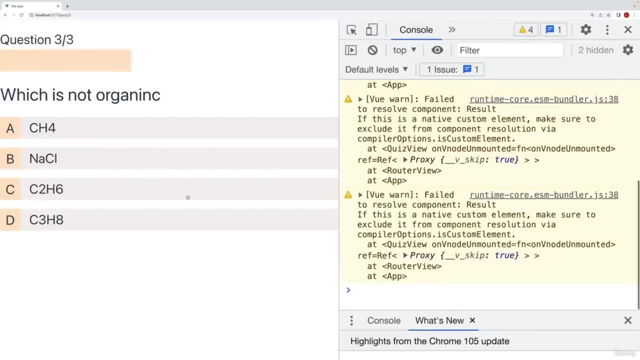 in the console that we don't actually see. So if I were to go to the final answer, 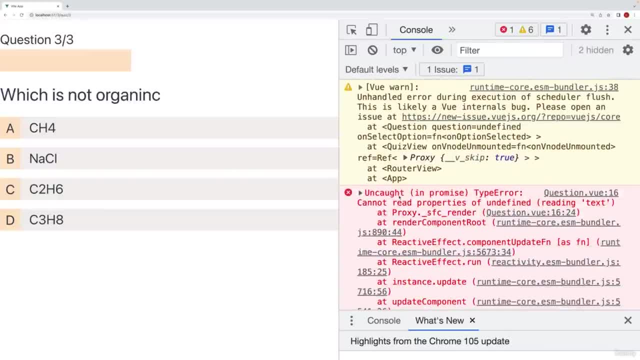 you can see here, right away we're getting some sort of, some sort of, hey, I cannot find a particular property, which makes complete sense because we are now in a current index that is not inside of our array. 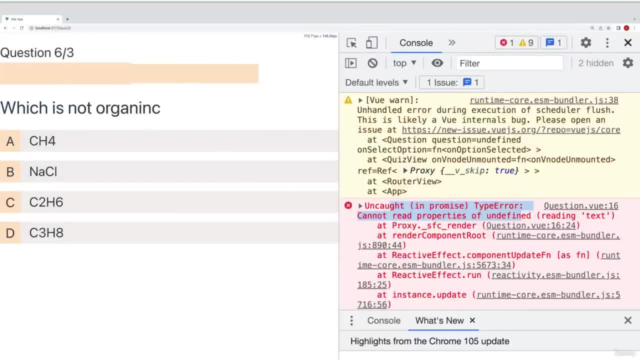 So you can see that we're getting a bunch of errors, and obviously this isn't a great experience. 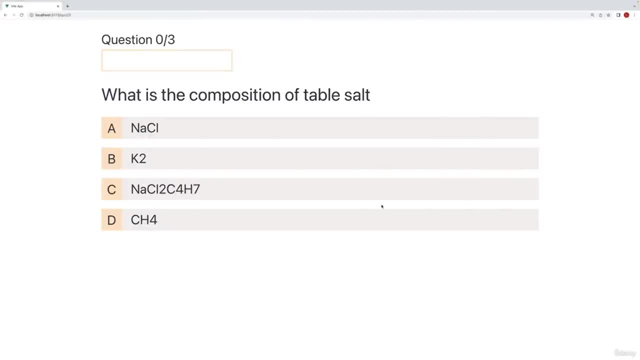 So instead of what we want to do is instead of, rendering this component, this question component, what we want to do is render a result component 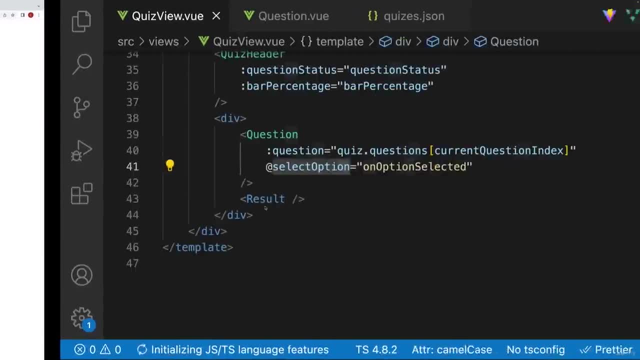 whenever we are completely done this quiz. So what we want to do is again, instead of rendering this component, we want to render this other result component that we haven't created yet. 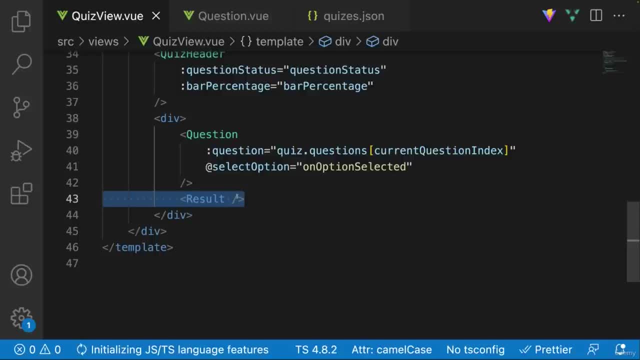 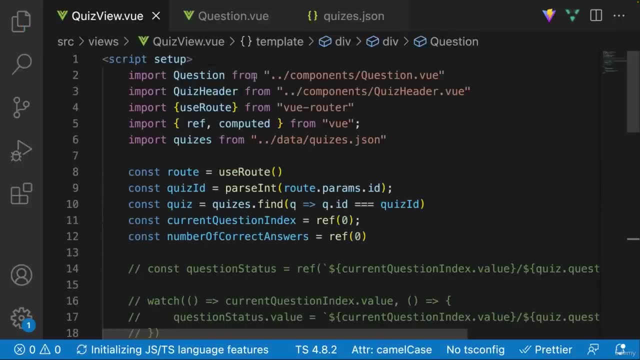 I just added it there so we can have a nice little visual. So let's actually go ahead and create this result component, and then we're going to go ahead and work on the logic to render it a little bit later. 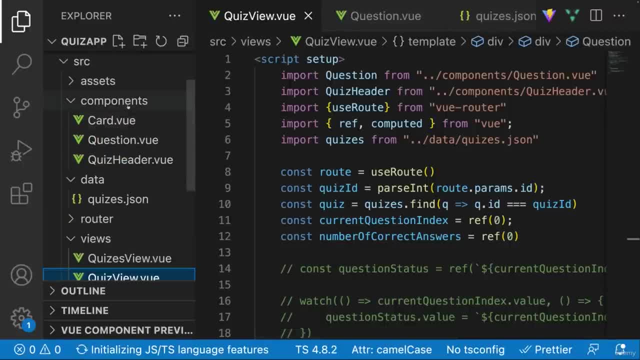 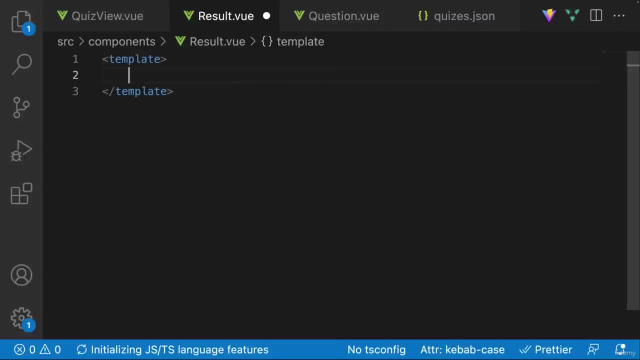 So let's go over here. We're going to go to our components directory, and inside of our components directory, we will create a result dot view file. And within here, well, of course, we're going to write the HTML, as well as the CSS for this results dot view. 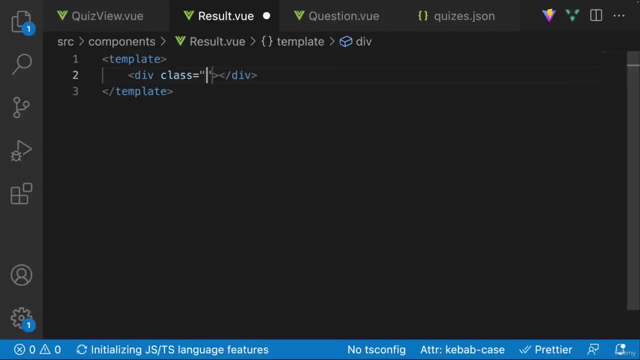 Now this is going to be relatively simple. So let's just go ahead and quickly bang it out together. So I'm going to say, I'm going to create a div with a class of results, and I'm going to have a P tag, and I'm going to say, your results, and then dot, dot, dot. And then I'm going to have an H1, and then within this H1, we're going to have some results. 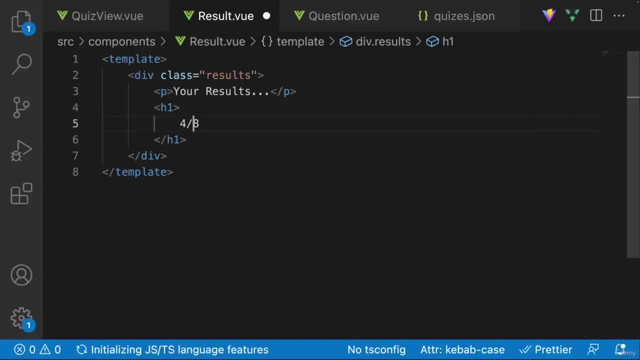 So for now, let's just hard code some results, like you got four out of eight correct. All right, looking great. 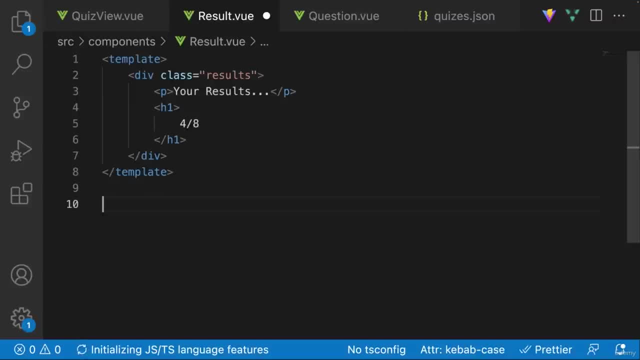 Let's go ahead and just very, very quickly do some styling here, just so we can have a more elegant and beautiful application. 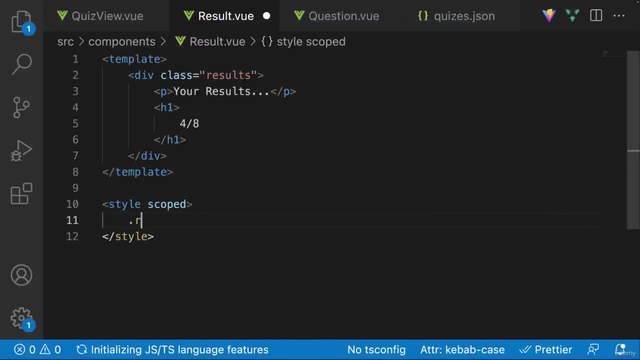 So we're going to say style scoped, and over here, we're going to say results, and this is going to be the actual div that's going to contain everything. 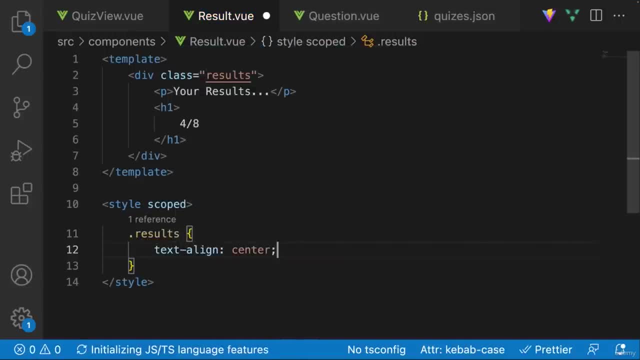 Let's just do an align or text align of center, as well as a padding of 100 pixels and then zero pixels. 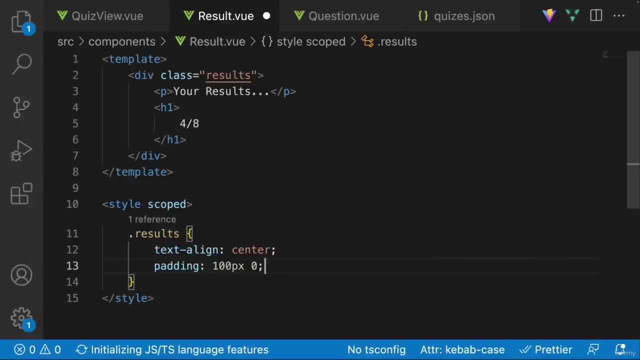 So 100 pixels to the top and the bottom, zero pixels left and right. 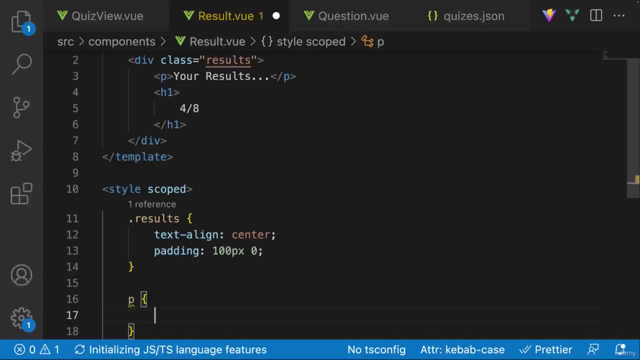 Let's quickly style our P tag. So we're going to say for the paragraph tag, 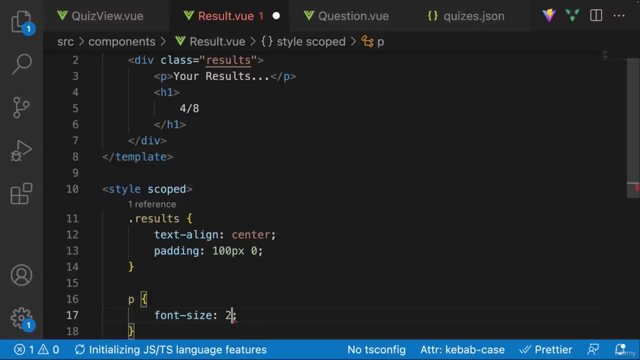 let's give it a font size of 25 pixels. And for the H1, let's give it a font size, of 80 pixels. 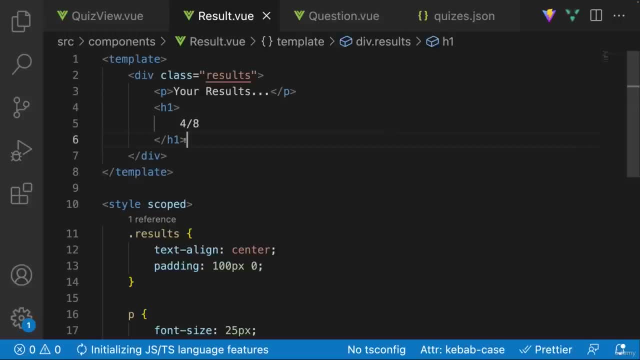 And I think that's pretty much all it is that we need. Later on, we're going to add a button that's going to allow us to navigate back to the quiz page, but that's going to involve view routing. 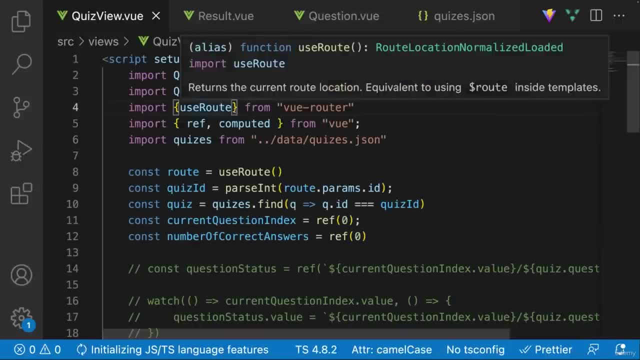 So we'll talk about that when we are done with this. All right, so let's go over here 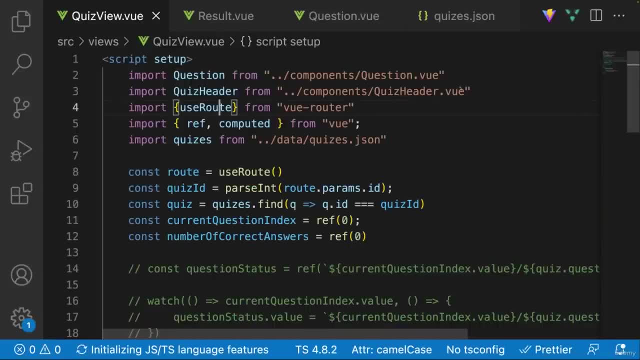 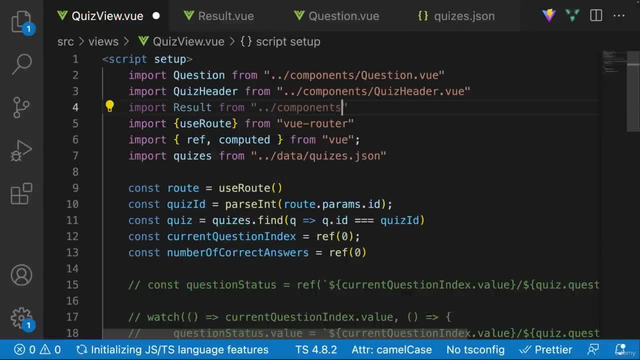 and let's render that result component just to see how it looks like. So over here, we're going to import results and we're going to say from components slash result, and what we're going to do now is go ahead and just render it. 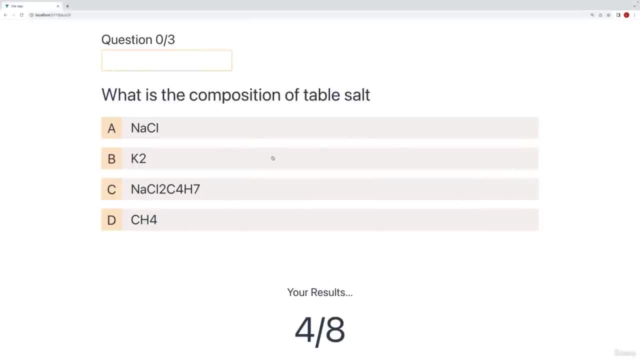 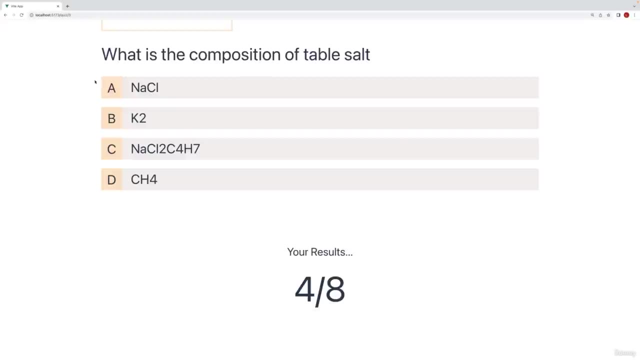 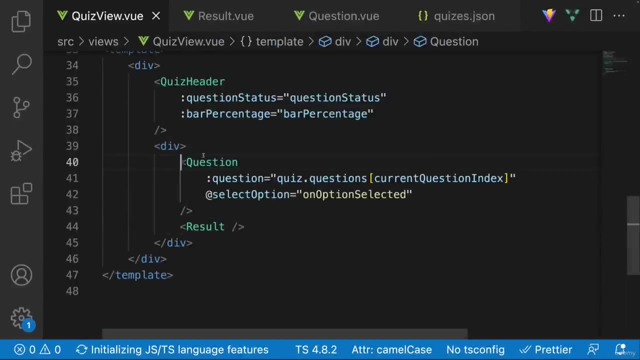 So we're going to go ahead and render it like so. And you can see here we get this quiz component and we also get this really nice looking result component. So of course what we want to do is we want to either render this component or this component based on a condition. And that condition is we completed the quiz. So if you completed the quiz, then we want to render this component. If we haven't completed the quiz, then we want to render this component. Any time we want to render, we want to render components on a particular condition, we're going to use the vif velse directive. 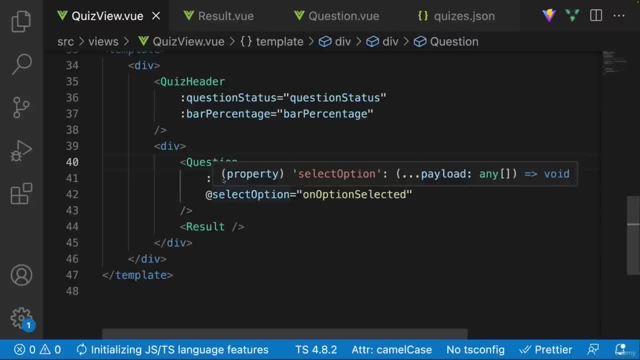 So that is exactly what we are going to utilize. So it's going to look something like this. So we're going to have something like vif. So we're going to say vif and let's just say some condition. Let's say that condition is true. Then we're going to render the question component. And then over here, we're going to say velse. So we're going to go and render it like so. But of course, right now, it's always going to render the question component because we literally hard-coded true. 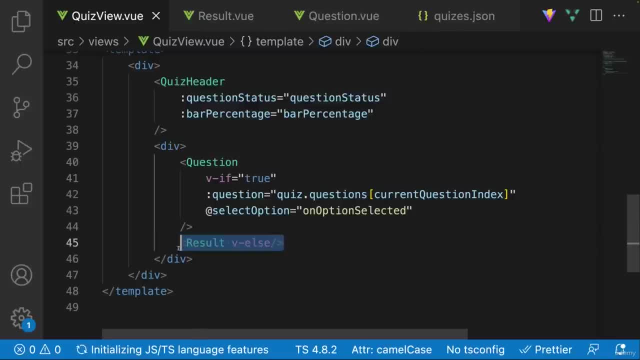 And actually, you can kind of see that, that the result component is pretty much dimmed out. So now let's go ahead and actually work on our condition. So our condition is actually something that is going to be a piece of state because we wanted to re-render our HTML whenever it is changed, because of course we want to either render this component or this component. 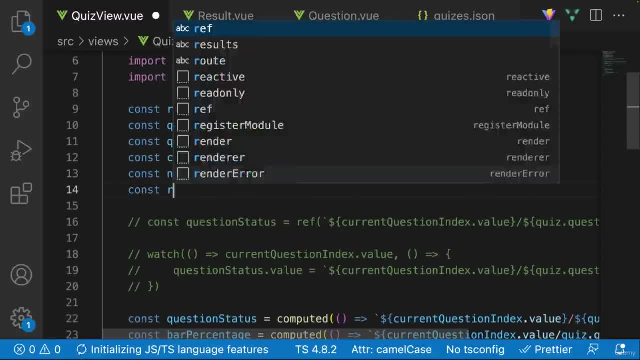 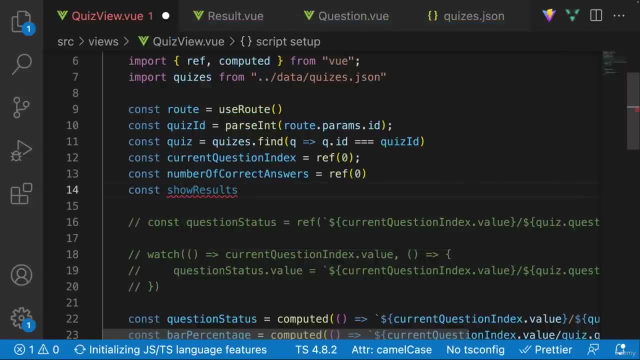 So what I'm going to do here is as a piece of state, I'm going to create a new variable, a new piece of state called showResults. So I'm going to say showResults. I'm going to say that this initially is equal to false. So I'm going to say showResults. Initially, I'm going to say that's equal to false. And let's actually just go ahead and use that. 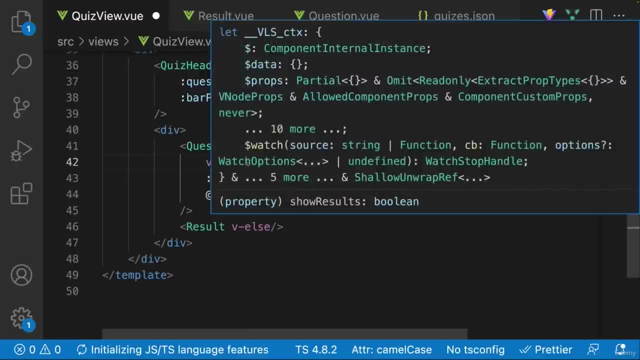 So I'm going to say vif and I'm going to say showResults or actually if not showResults, then what I want to do is I want to go ahead and render this. 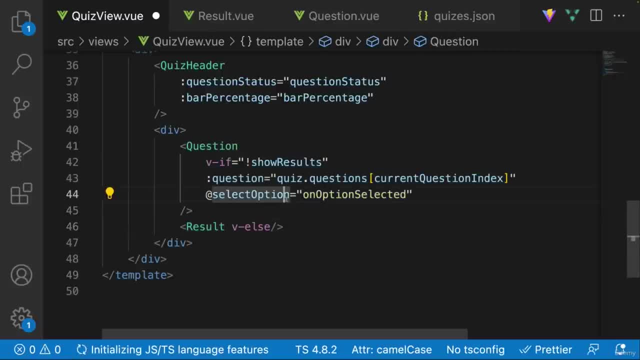 However, if this is now true, then I want to render this. the result. So I'm going to go ahead and save that. And again, as you can see, it works exactly 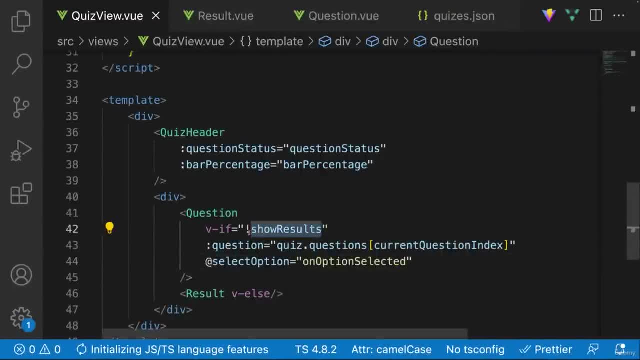 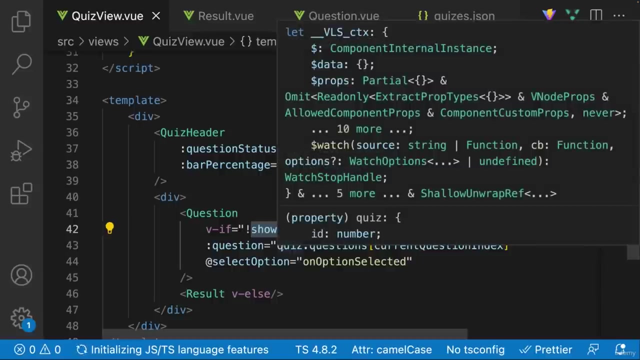 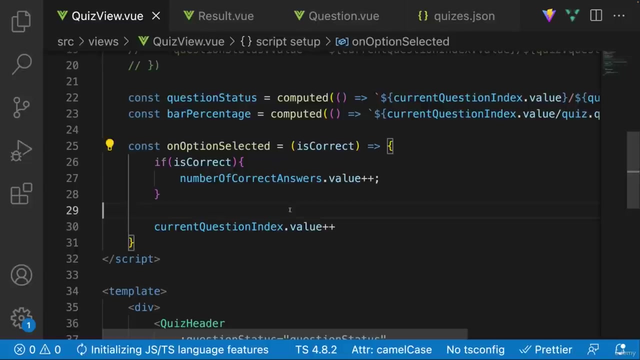 the same way. So now what we actually need to do is to well figure out where we actually update the show result piece of state. And personally, I think the best place to update the show result state is right here inside of the on option selected function or method that we have just created. So remember, this is going to be called anytime that we select a particular option. So 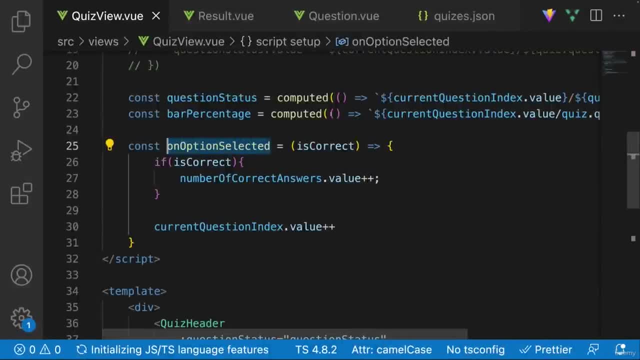 when we select a particular option, our question component is going to emit in an event, and it is going to result in us calling this function over here. So it'll be actually nice to well figure out, oh, did we just answer the last question? If we did, let's just go ahead and we'll show the results. So let's just go over here. And right now, we have a question that we have to answer. So let's just go ahead and we'll show the results. So let's just go over here. And right now, we have a question that we have to answer. So 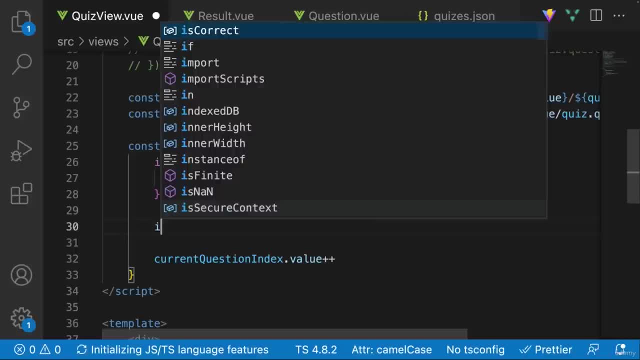 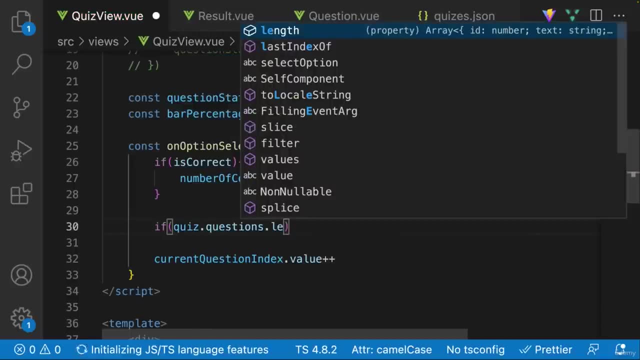 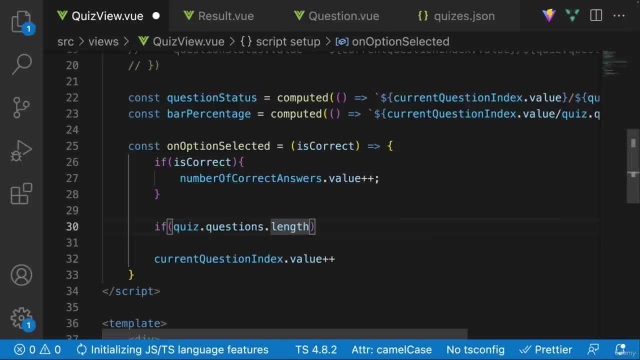 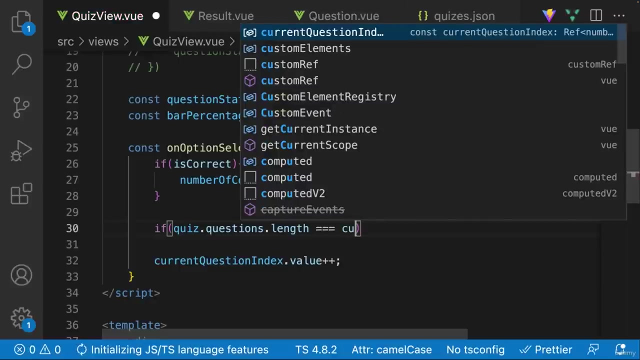 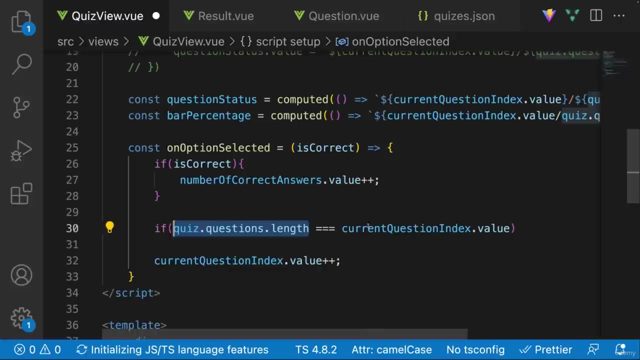 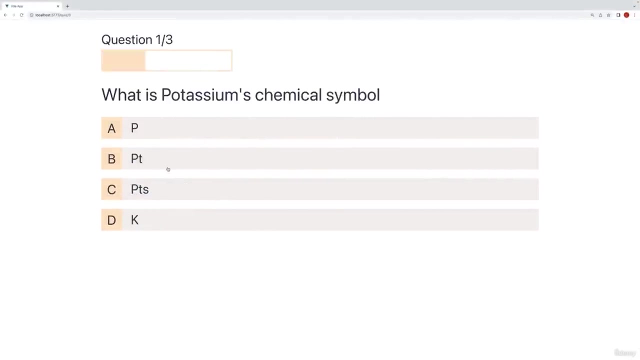 let's just go ahead and we'll show the results. So let's just go ahead and we'll show the results. So right after the if is correct, what I'm going to do is I'm going to say if, and then I'm going to say if the quiz dot questions dot length, so this is going to be the length of all of the questions that we have. Now, at this point, we only have three questions for each quiz that we have. So we can say that this is going to be three. And then I'm going to say that this is going to be equal to the current question index dot value. However, the problem is, is that this is going to be three once we reach the end of the array. And then this is actually going to be two once we reach the end of the array. So let's actually just go ahead and do a minus one just to keep them in sync. And that's because of course, this starts at the index of zero, while as getting the length starts at one. And very simply, now all we need to do is just say show results dot value, we can say that that is going to be true. I'm going to go ahead and save that. And let's just do a quick little refresh. And let's test it out. 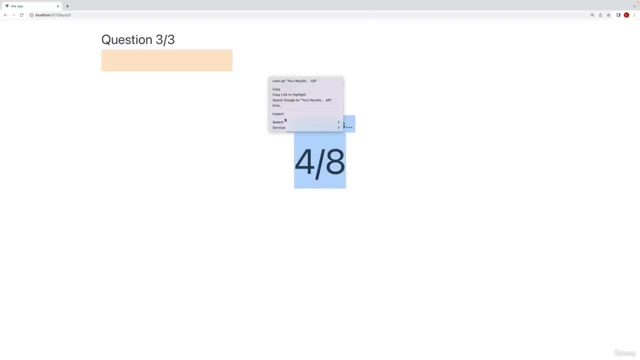 And there you go. How terrific and cool is that. And if I were to inspect the console, you can see that there is no errors occurring. There we go. How cool is that? Now, of course, this isn't the final product that we want, we want to not hard code this value. So let's go over 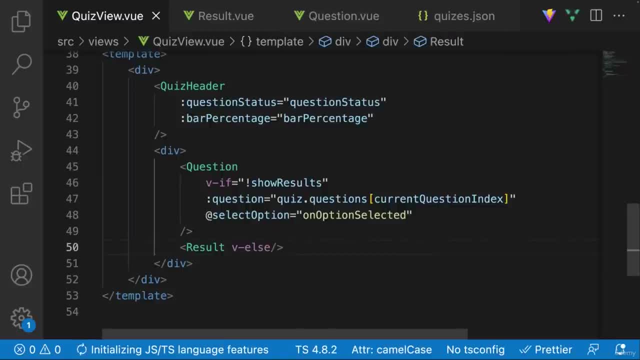 here. And let's just pass in some props. So we need to pass in some data. So let's go over here. And I am going to pass in, we can pass in either two props or one prop that is just going to say 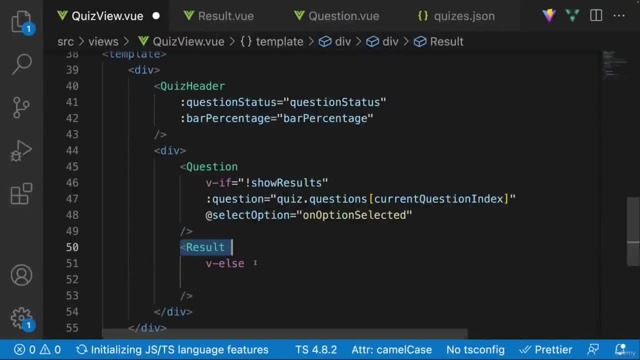 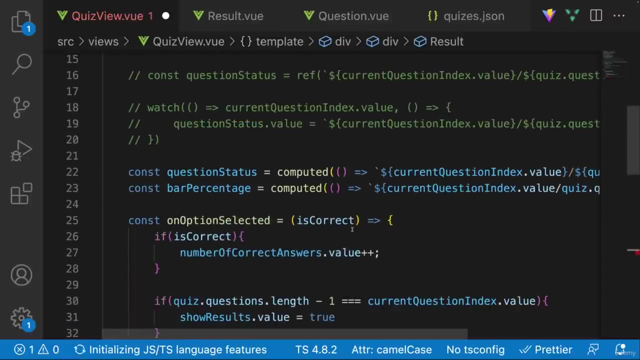 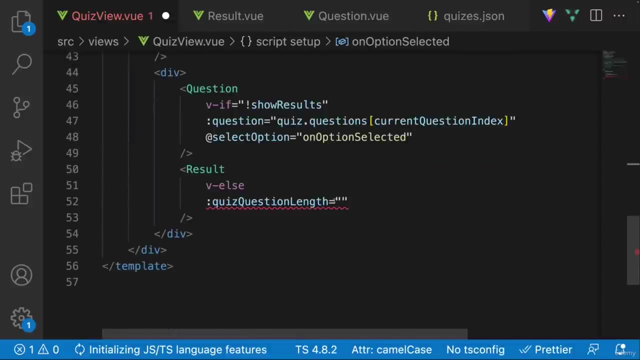 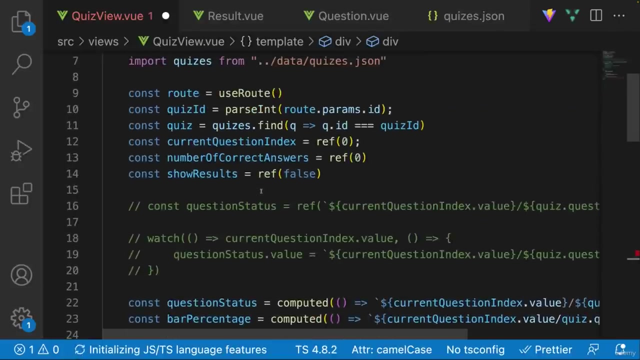 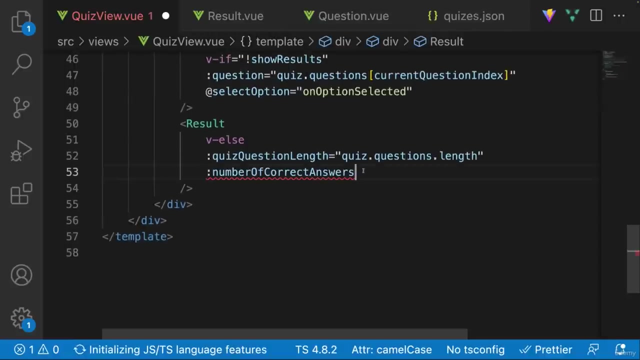 the results, I'm going to go ahead and pass in two props, I'm going to let the results component render exactly how it is that we want it wants to use it because maybe later on, it's going to actually need those values to do something else. So the first thing I'm going to say is the question length. So I'm going to say quiz, question length, I'm going to say that that is going to be equal to, well, it's going to be equal to this over here. So let's just go ahead and grab that. We're going to go ahead and pass that in as a prop. The second prop that we need is how many answers that we got correct. And remember, we stored that value right over here. So we're going to say number of Correct answers. So I'm going to go ahead, and paste that in there. And we're going to say number of correct answers, looking great, looking great so let's go over here and let's just get our props from our script tag so I'm going to say 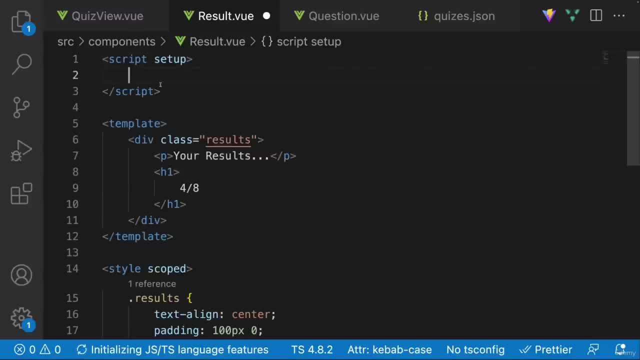 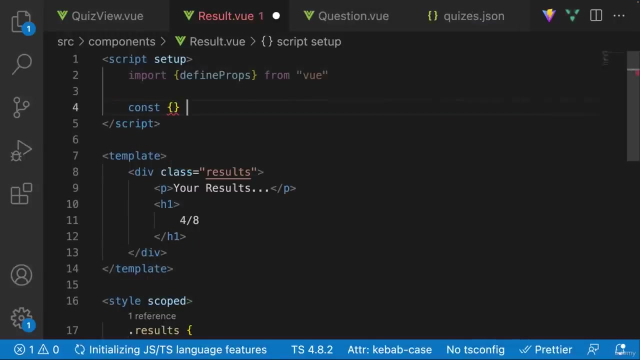 script setup and over here let us import and we are going to import define or from view we're going to import define props so I'm going to say define props like so and I'm going to say const and I'm going to say define props I'm going to invoke it define all of the different props that 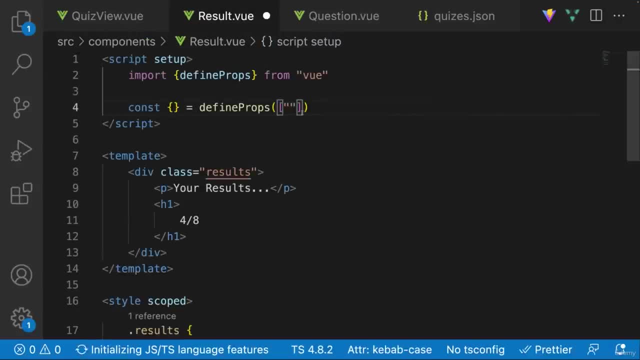 we have so we have the quiz question length and we also have the number of correct answers so let's grab that as well let's go over here and let's copy that and paste that in looking good looking 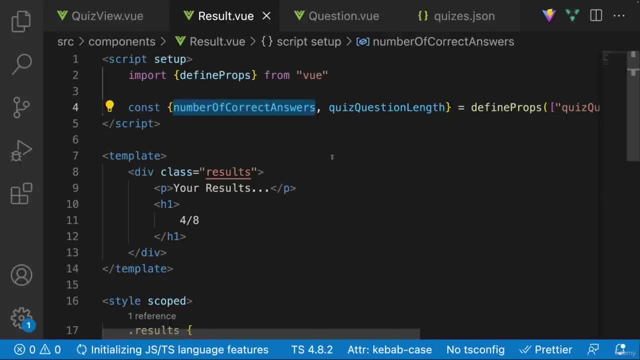 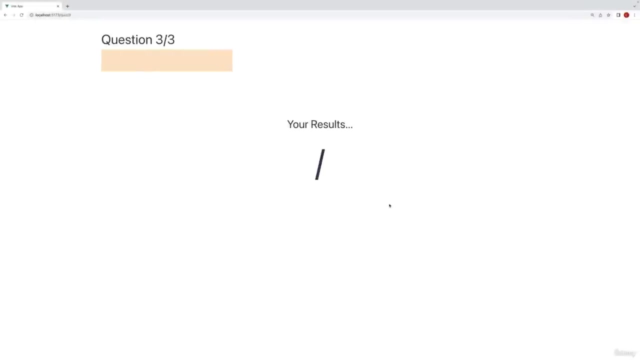 good so now what we can actually do is just derive this ourselves we can create a computed component or we can just derive it ourselves it's very simple so instead here what we can say is instead of four we can just hard code you can dynamically code number of correct answers and then over here I can say question or quiz question length go ahead and save that and for now it seems kind of goofy what's going on so let me just go ahead and refresh and there we go you can see that we actually get our results so the last